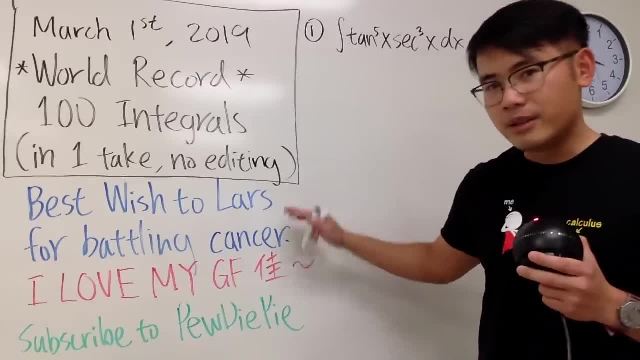 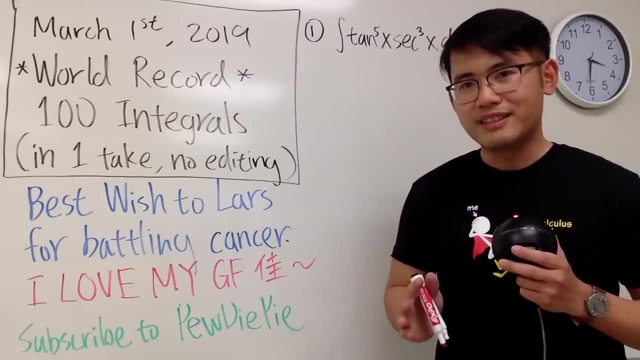 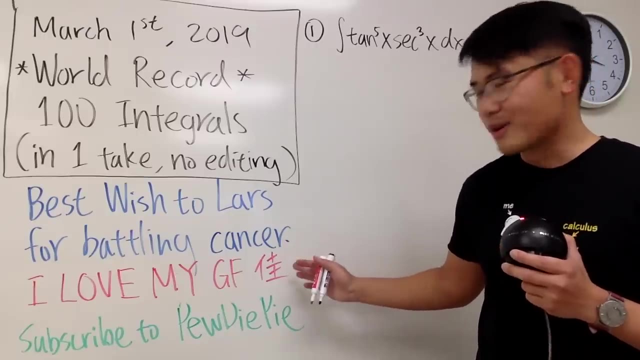 to give my best wish to Lars because he's battling with his cancer and you know. I want to thank you for your nice message and I really wish you the best. you can do it and this video is greatly supported by my girlfriend. I love her so much, my girlfriend Jia, and you know what the hell. 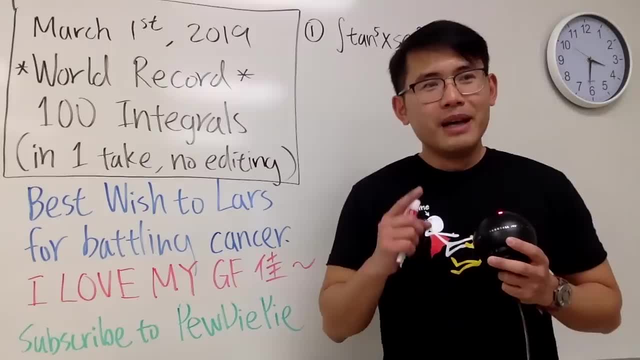 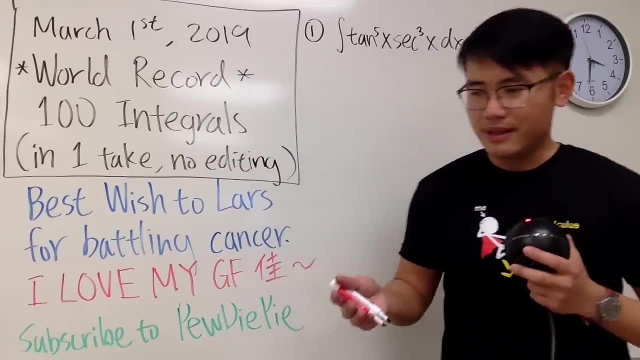 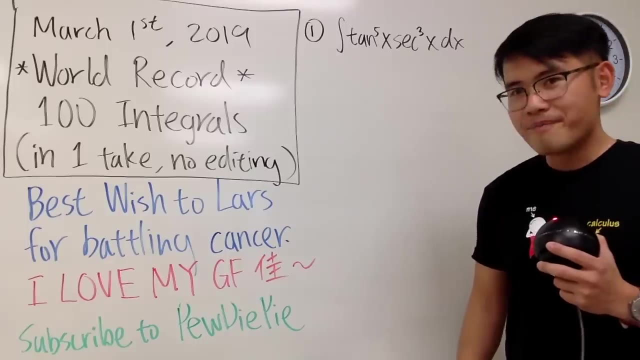 subscribe to PewDiePie, but, on a more serious note, subscribe to, you know, my friends Dr Payen, Wu Han, Monica Max and all my guest speakers in the past. thank you, and, of course, subscribe to my channel. okay, so here we go. I really don't know how long this will take. 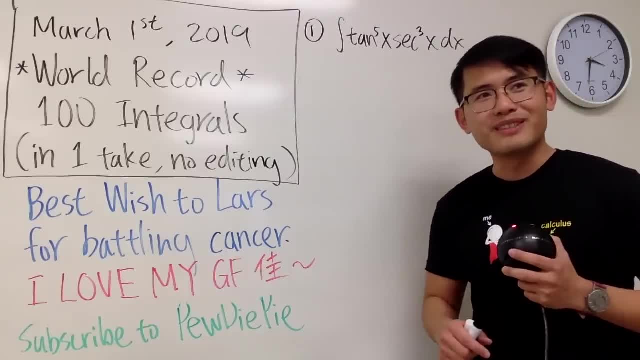 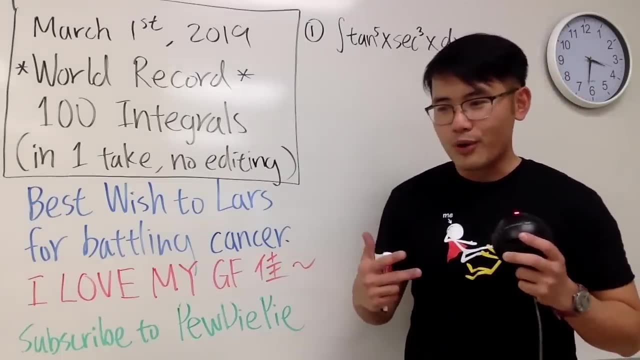 I don't even know if I can do it, but like I don't even know if my laptop can record that long, so we'll see. anyway, here's the deal for all these questions. they will be good for Cal 1 and Cal 2 and I will try to show most of the work, but sometimes, if I'm not, I'll just you know just. 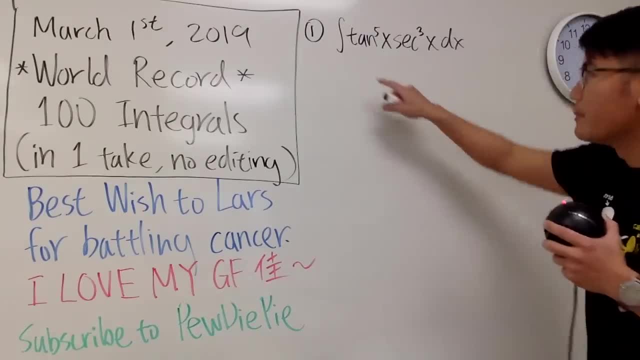 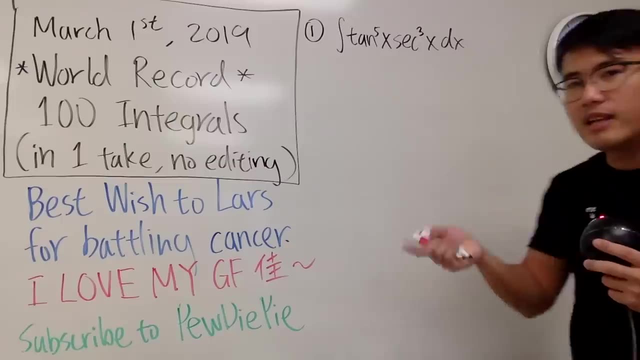 say we'll do it, but in our heads all that. okay, enough talking. let's talk about how to integrate tangent to the fifth power times, secant to the third power, x. all right, so we have a tangent secant situation and both of them are with odd power. so I think it's a good choice, if you can. 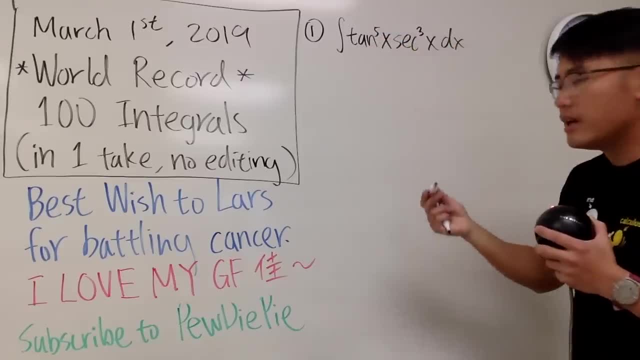 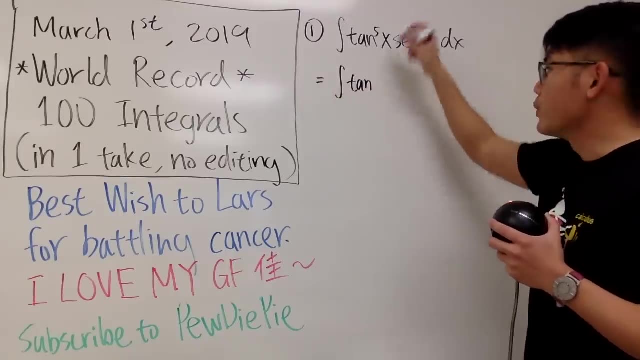 take one of the tangent out and also take out one of the secant. so, with that being said, let's do the following: let's look at this integral as the integral and, as I said, I will take one of the tangents out. so we'll get attention to the fourth power. 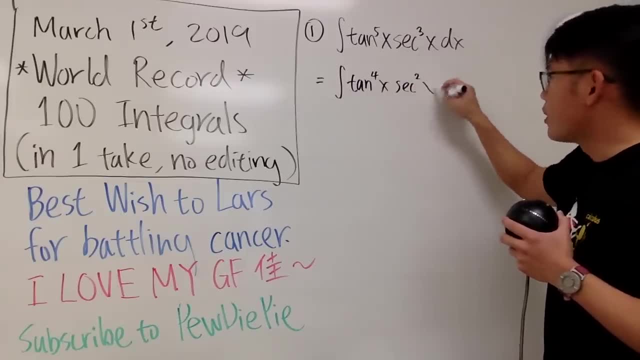 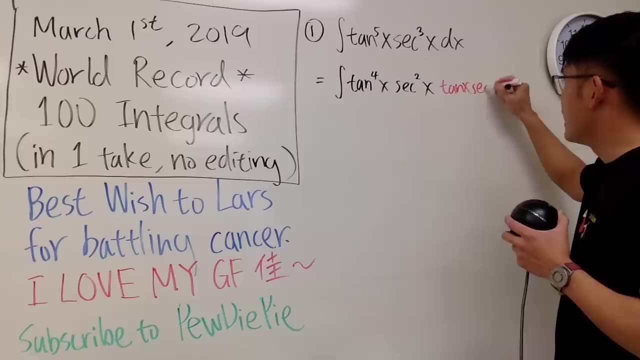 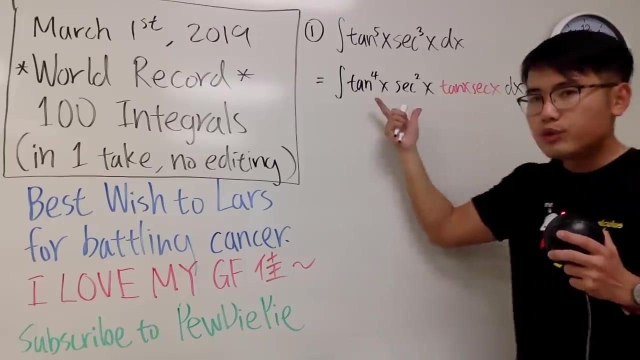 of x and then times secant over the second power of x, and then, right here, I will write the tangent x, secant x and then the dx right here. well, if I have this on the outside, I hope to write this right here as the expression in terms of secant, and to do so. we know this is fine, but this is not good yet. 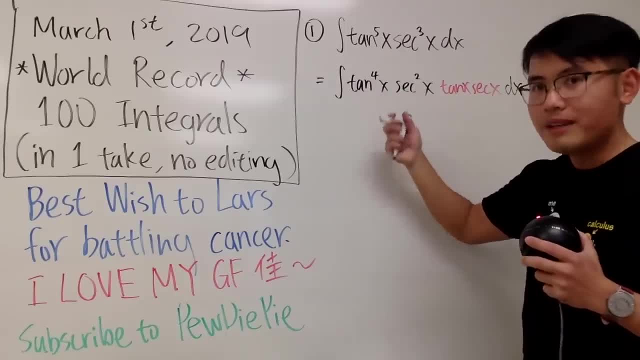 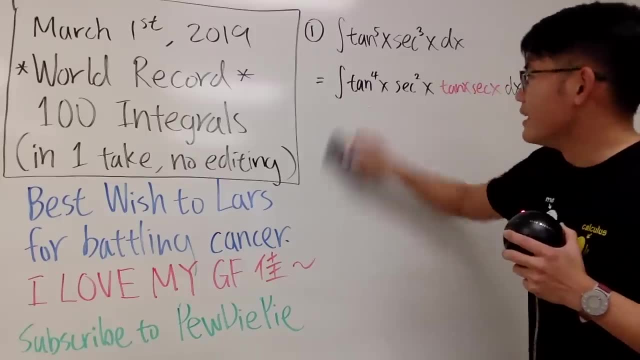 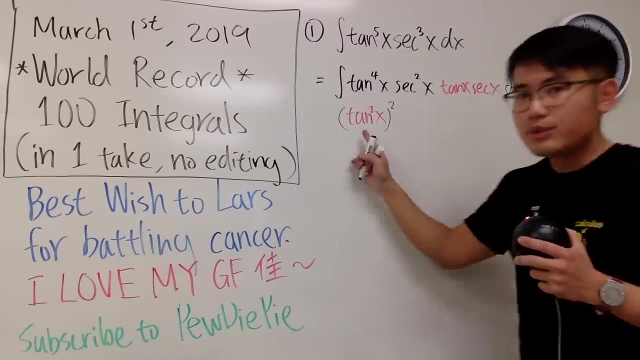 problem though, because we know tangent to the fourth power is the same as we can look at this as secant square. we can look at this as tangent square and then square, right tension square and then square, and, as we all know, tangent square is the same as secant square x minus 1. 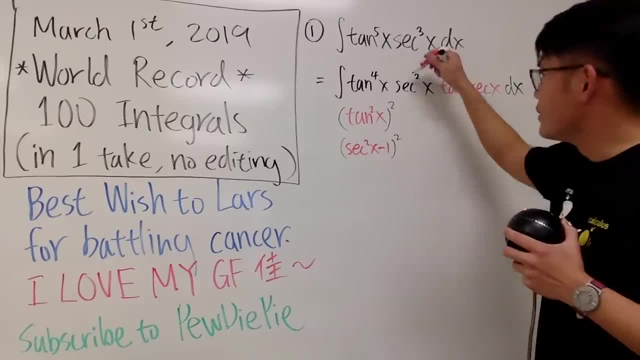 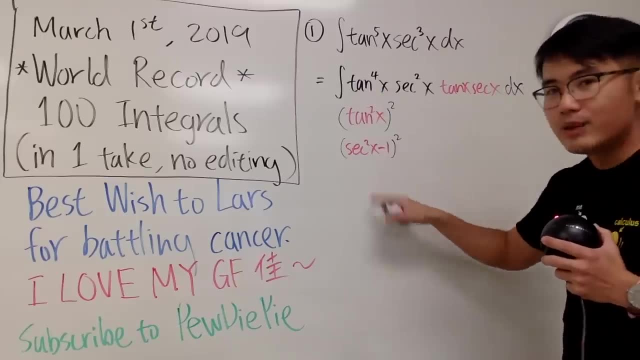 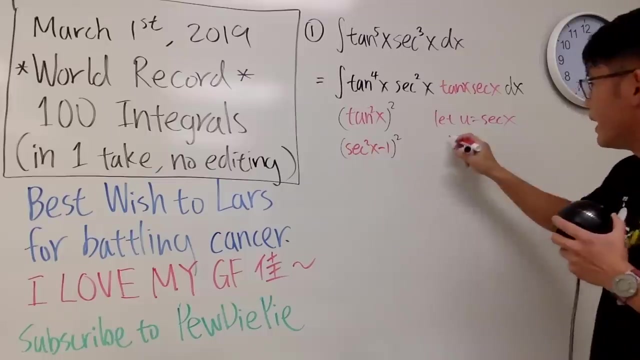 and then you have that square. so, as you can see, we can just take this and distribute, but you have to do some work here on algebra first. well, the deal is that if you look at this as that, we can do a little. u sub real quick. so, with that said, I would just say: let u equal secant x, and then we have the du being secant x. 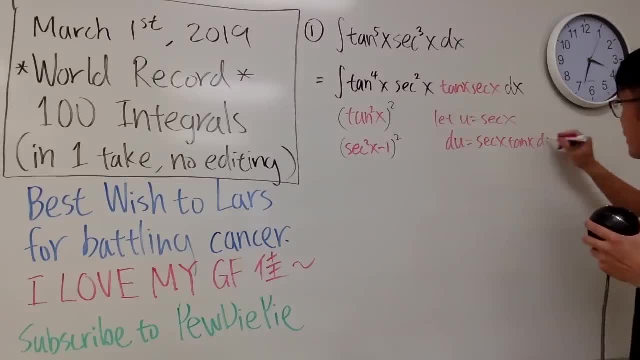 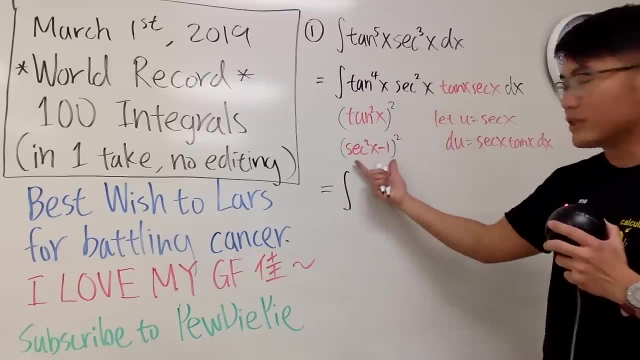 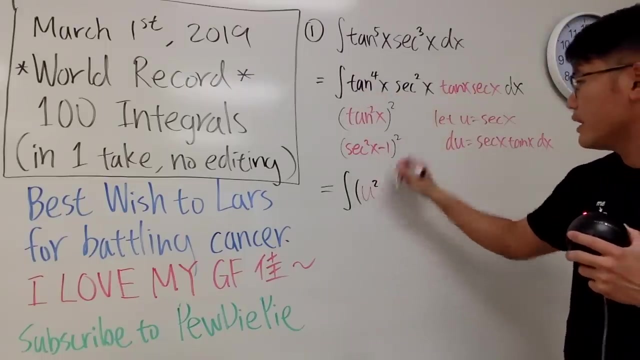 tangent x, dx, and of course we can take this integral to the? u world now, and that's very, very nice. so we'll see, this is the integral and I'll just put this down for the tangent to the fourth power, and namely we will have u and we'll have the square, and then minus 1, and then that's square. 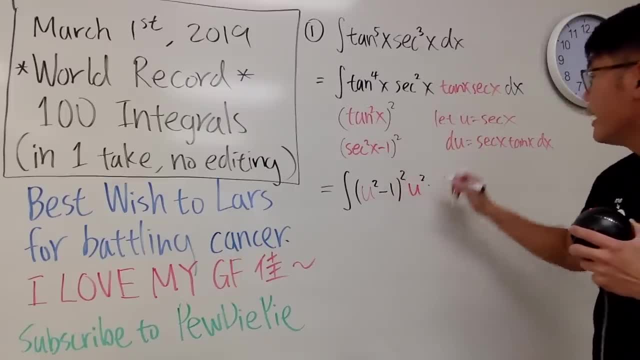 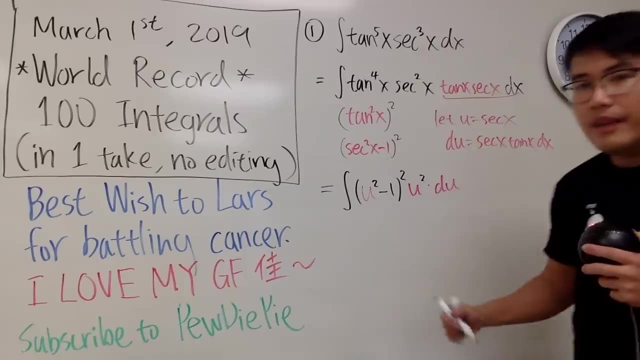 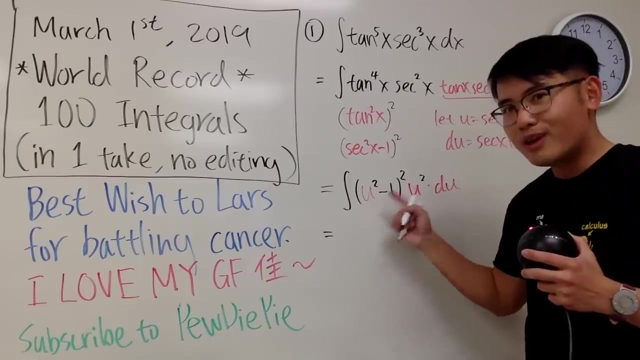 and then this: right here it's another u square. and all this, this right here, is just my you. so this is very nice, and now we can just do some algebra to simplify this a little bit. as we all know, this right here is going to be u to the fourth power minus 2u square and then plus. 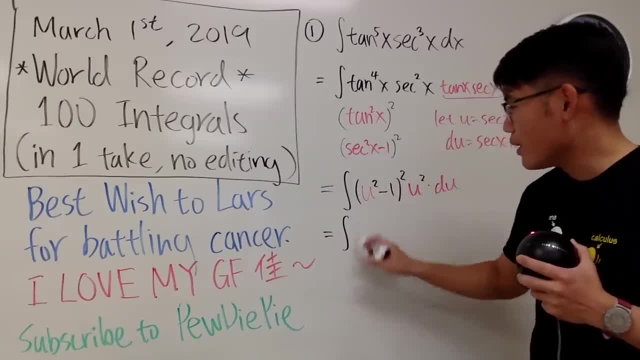 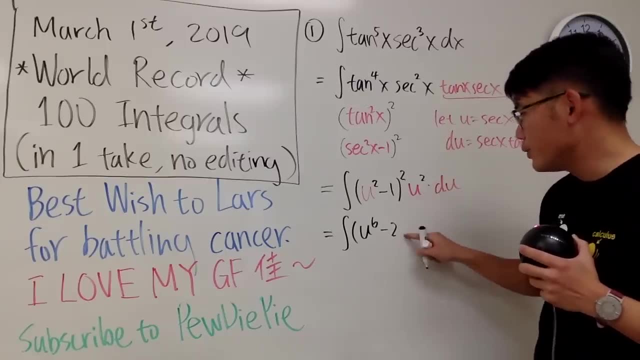 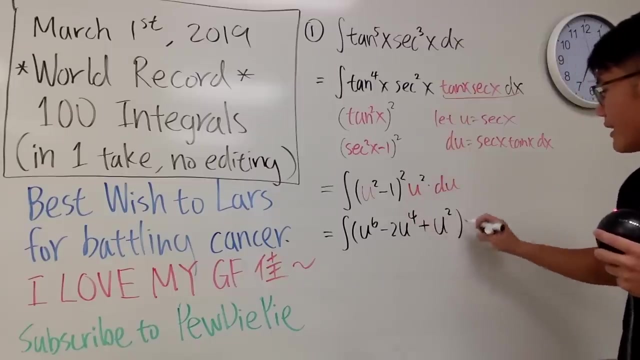 1 and then distribute the u square so you end up with the integral parentheses: u to the fourth power, times u squared. we get u to the sixth power and then minus two: u squared times this, which is u to the fourth power, and then plus one times that, which is u squared like that, du okay. so of course. 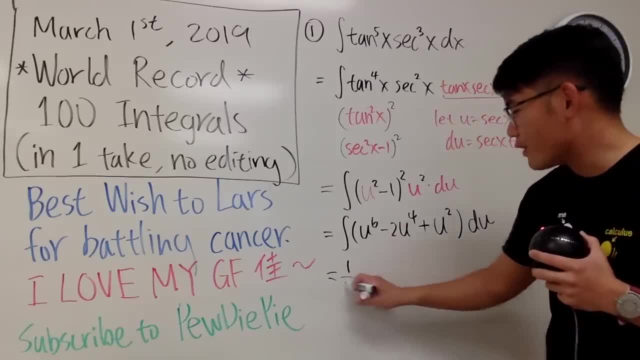 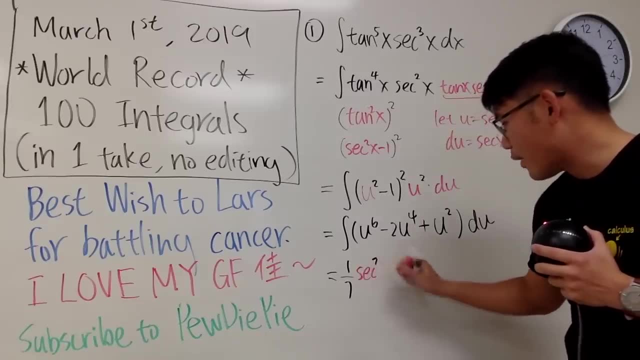 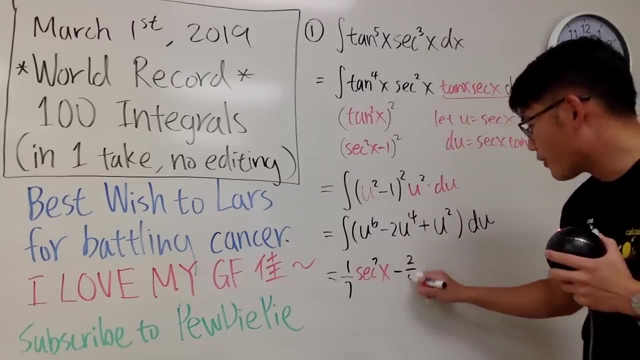 now we can just integrate all these guys. so right here we get one over seven, u to the seventh power, and we know u is secant, so let's just write it down. we have secant to the seventh power and the x and then minus. well, add one to the power divided by that which is two over five, and then we have. 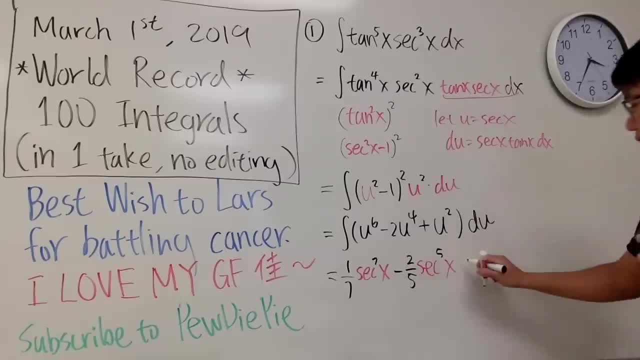 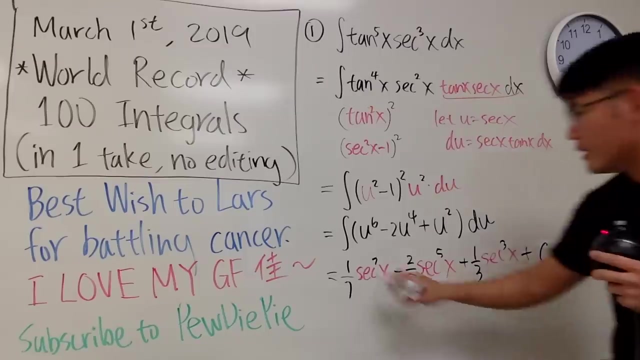 secant to the fifth power, x, and then this right here will give us one third- one third should be black- and we have the secant to the third power of x, like that, and then we're all done, so we can put a plus c, and i'll only put on a plus c for the final, final answer, which is this one right here: 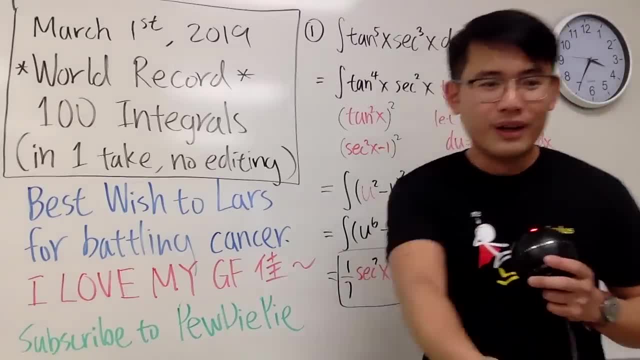 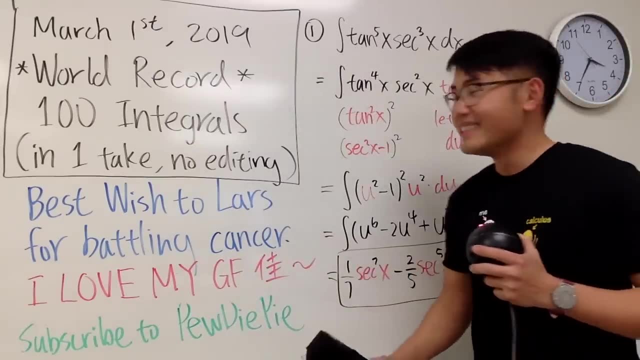 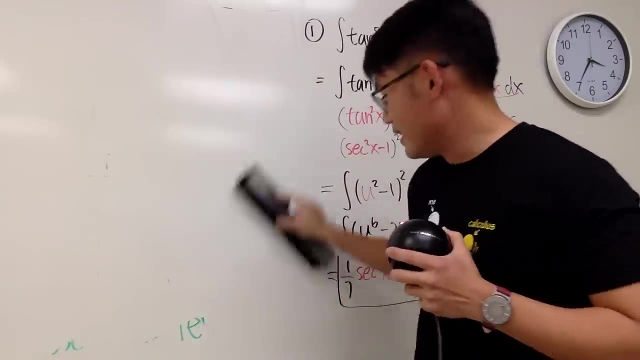 so this is the first one, and we have 99 more to go, and let's see what the next one is. okay, so we'll see. i'm going to erase this now, and there's no way for me to fit in 100 integrals on one board. there's just no way. so i will be erasing this along the way, right? so the second. 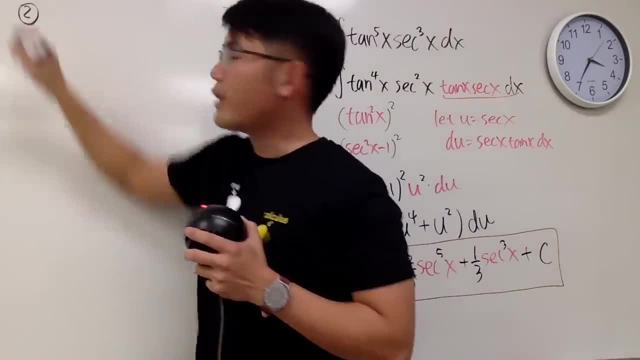 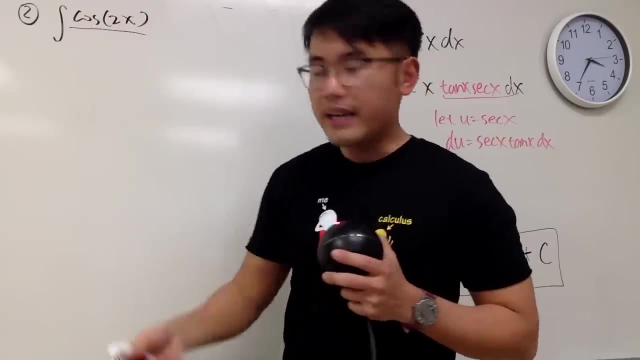 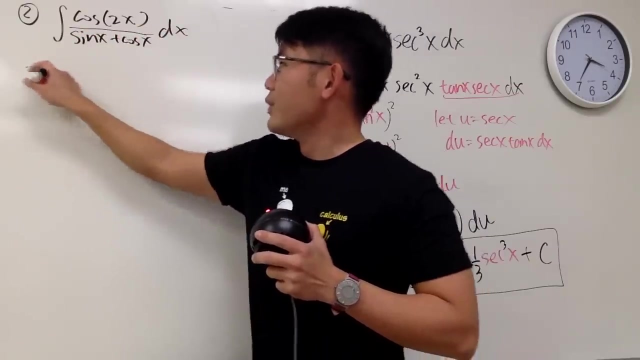 integral i have for you guys is this: let me just put this down right here for you guys: we have to integrate cosine of 2x over sine x plus cosine x and, of course, don't forget the dx, even though you know we will be doing 99 more. 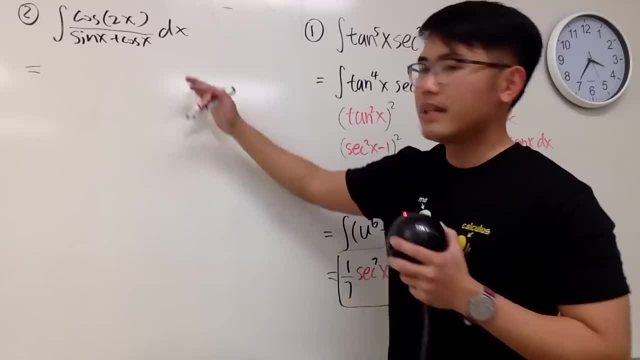 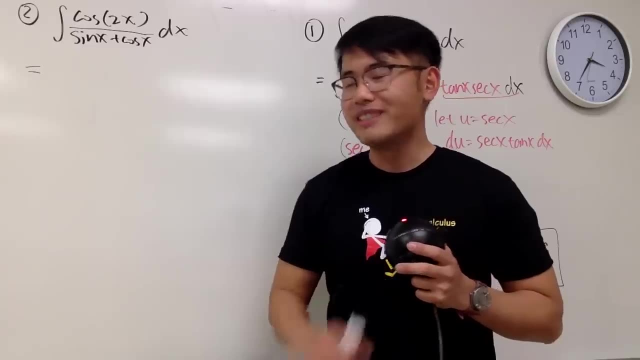 integrals, but don't forget the dx. anyway, let's think about it. how can we do this? well, cosine of 2x. we have the double angle formula for that, and the best version that we can use is: we can write this down as, and let me just indicate, we'll write this down. 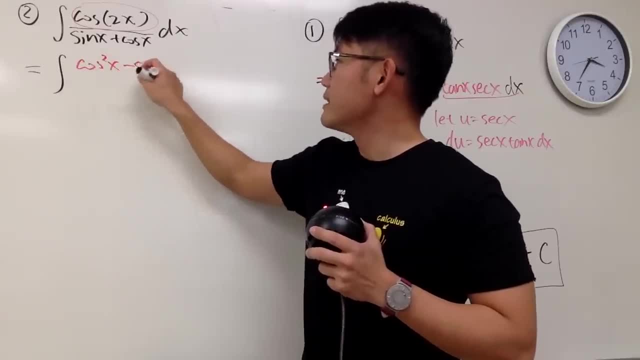 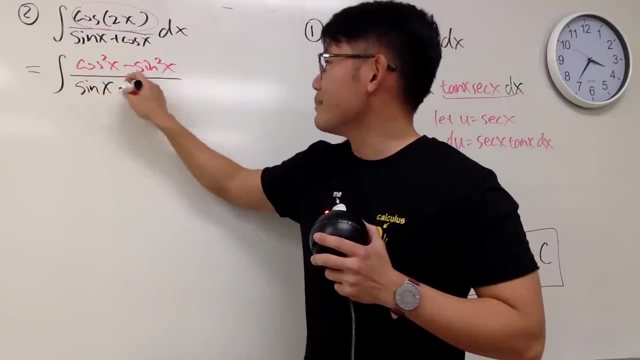 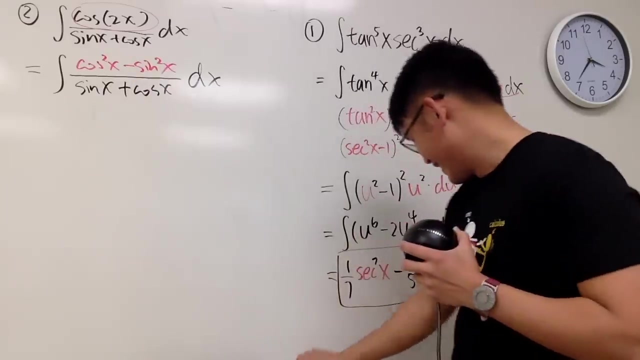 as cosine square x minus square x in our situation, because the denominator is sine x plus cosine x. Well, what good does this do? Yes, we can factor this out, isn't it? So I will, of course, do this in blue. 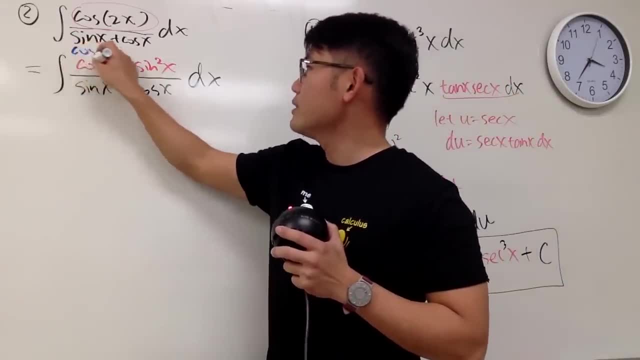 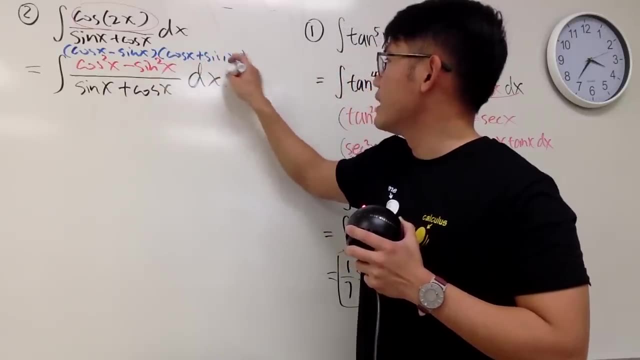 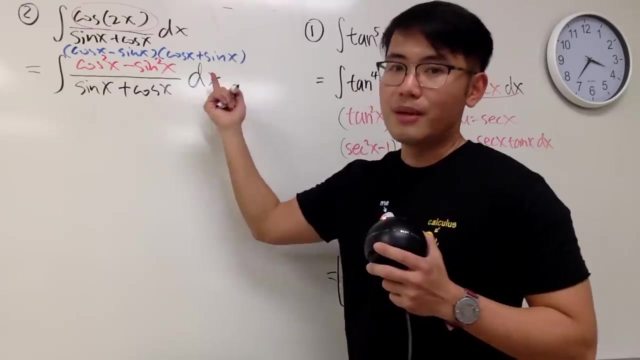 If you factor this out, you will get the difference of two squares, which is going to be cosine x minus sine x times cosine x plus sine x, like that, and with that being done, all we can do next is see this and that they are exactly the same. The order doesn't matter. 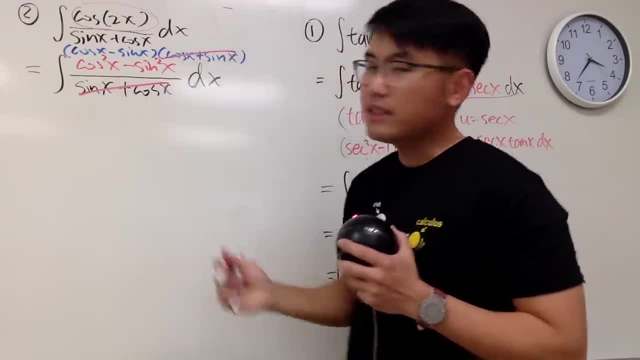 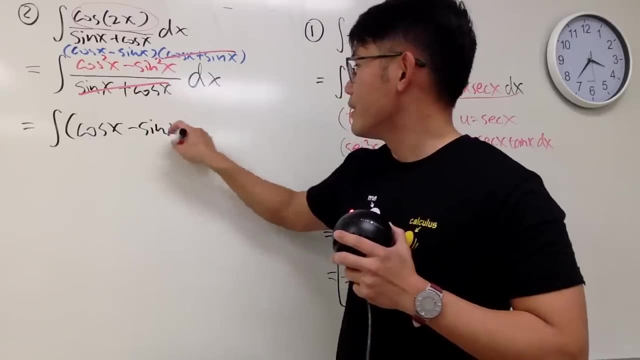 so of course you tweak it, but anyway this and that can be canceled and we get the integral of this only, which is the baby integral, and of course we can integrate this real quick. The integral of cosine is positive sine. 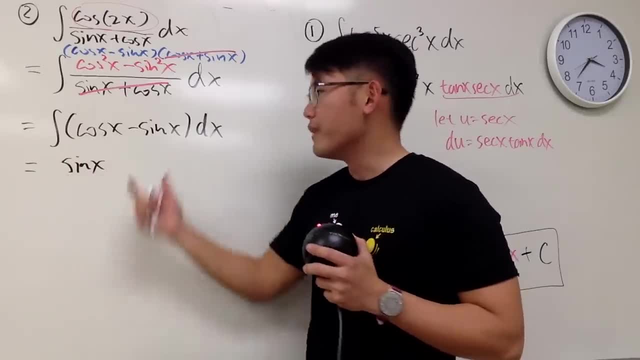 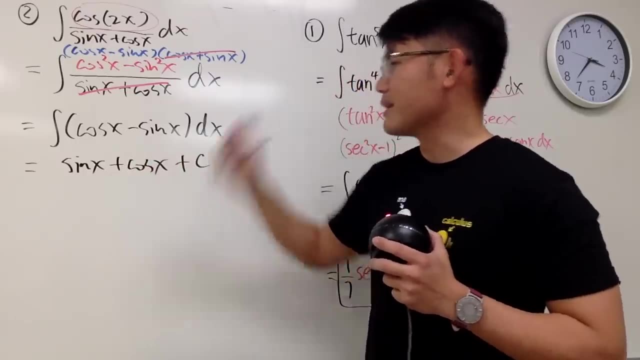 so you get positive sine x, and the integral of negative sine x is positive cosine. so you just put on plus cosine x and you are done. put on plus c, And of course you can do a quick check if you differentiate. 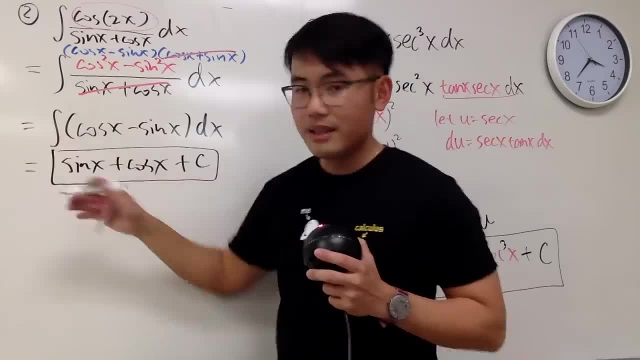 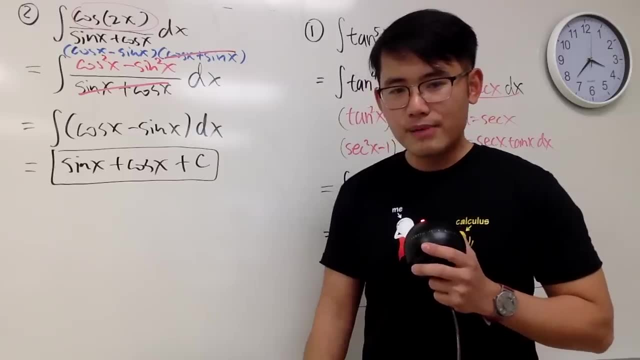 this. you will end up with that. so you know this is correct. so we got that very good. And, yeah, let's see for the next one perhaps. hmm, we have this right here. okay, we have this right here. 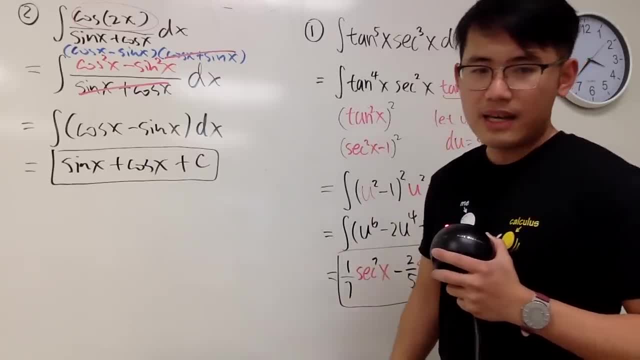 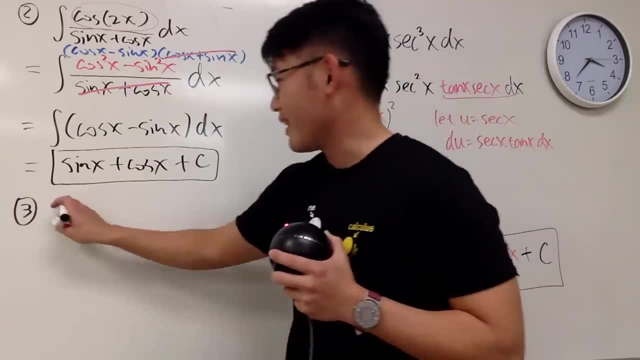 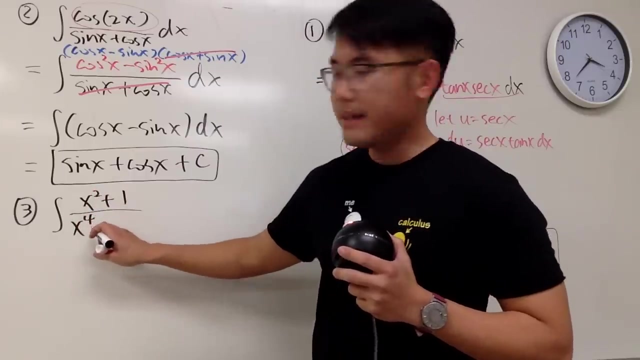 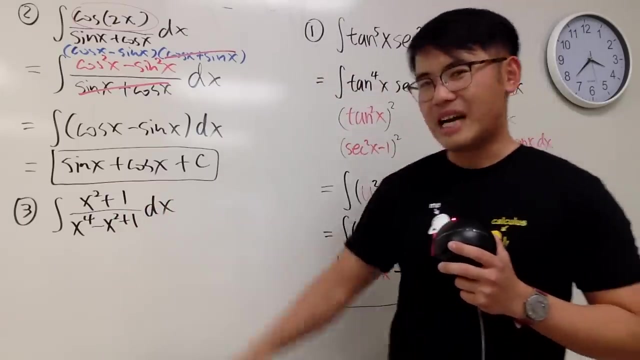 and I think I will try to fit in here. okay, there's a way, I think. Let's take a look at the integral of x squared plus 1 over x to the fourth power, minus x squared plus 1. dx The denominator, we cannot factor it. 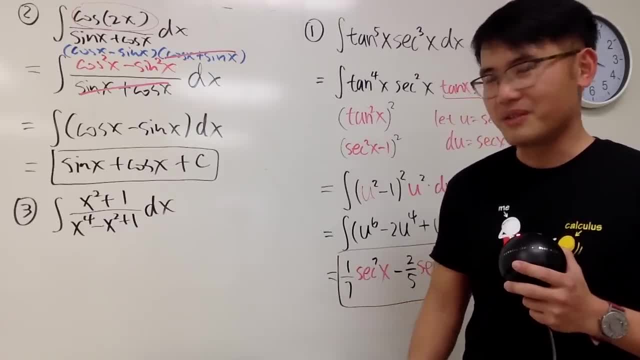 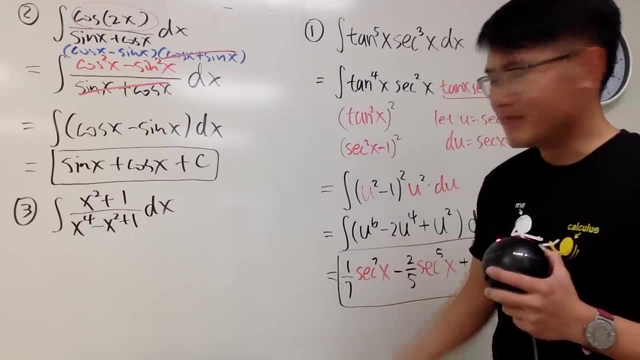 This is not easy, but it can be easy. if you are watching this video to learn the technique right. Well, of course, you can pause the video and try this first, but you can just watch us do it. So this is how we are going to do it. 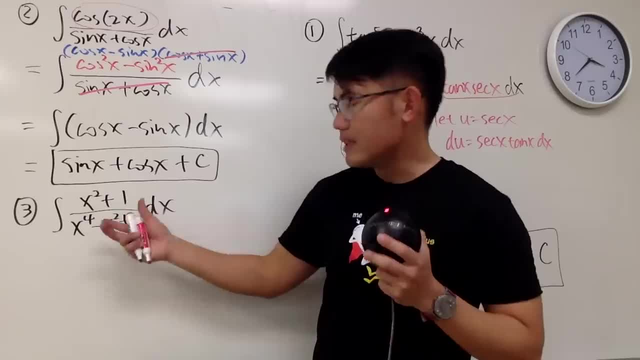 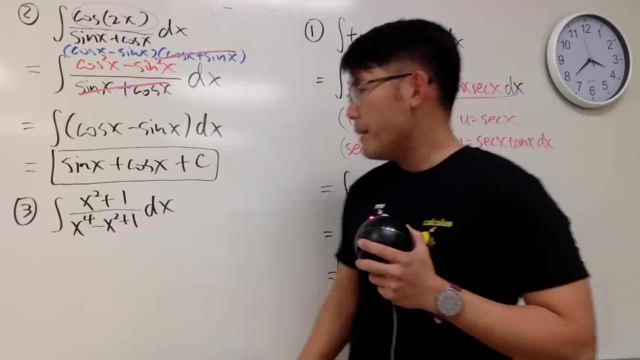 On the bottom. this right here is not a. it's not factorable, but it's almost like a perfect square, though, if you have a minus 2 x squared instead, And better yet, we are going to actually divide everybody by x squared. 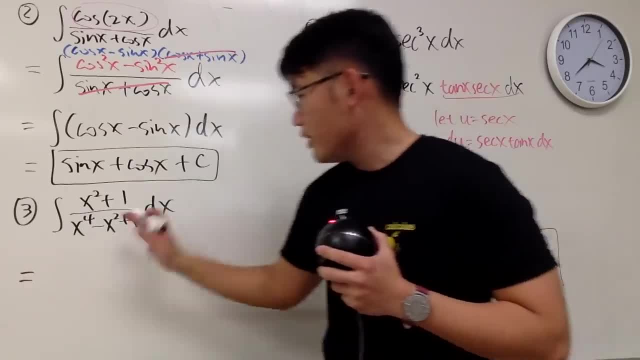 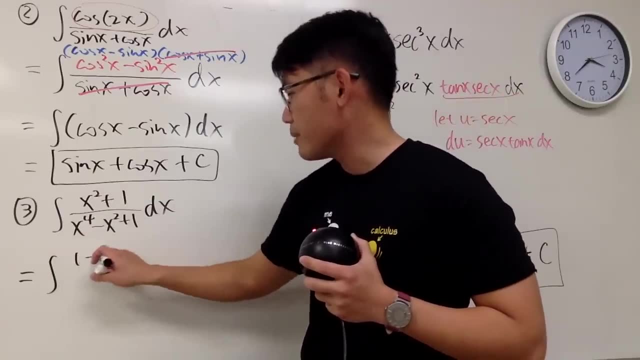 and you will see why. Well, if you don't divide by x squared, you can also, you know, do it later on. but like I'll just divide everybody by x squared, and if you do that, you get 1 plus 1 over. 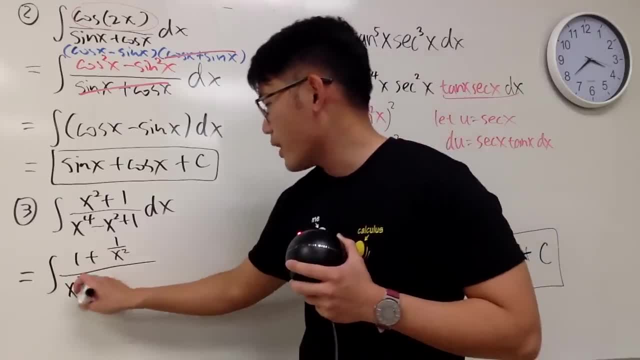 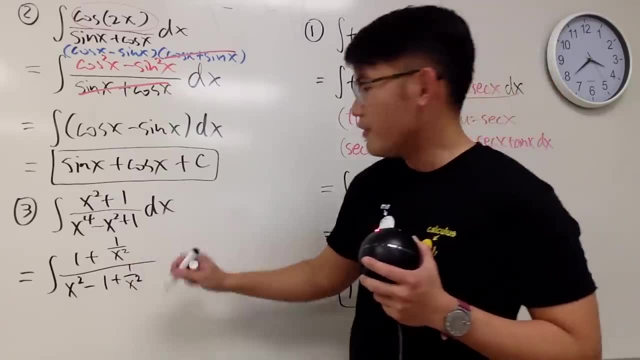 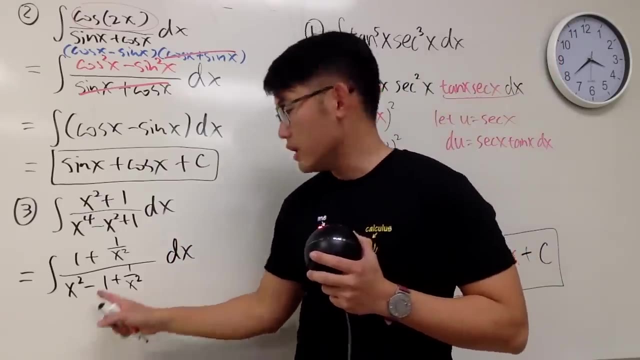 x squared over. here we get x squared and you get minus 1, and then you have plus 1 over x squared. like that, We're just dividing everybody by x squared and again, as I said, this is almost a perfect square if the 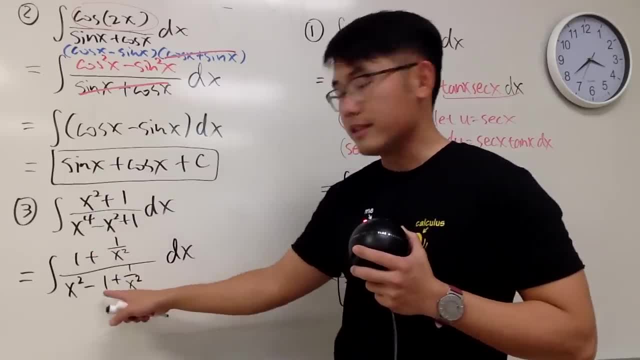 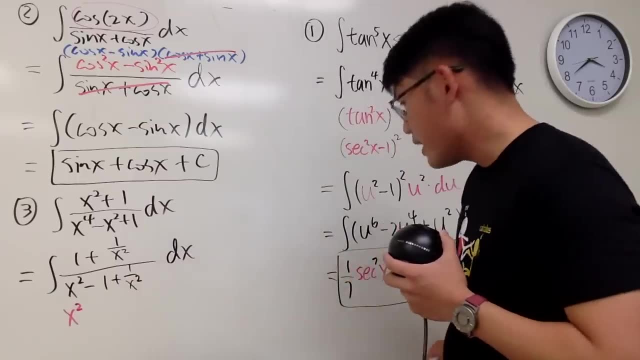 middle right here was a minus 2 x squared right, So that means I should have a minus 2 right here, And what I will do is I will look at this as x squared and then, for the minus 1, I will look at that as minus. 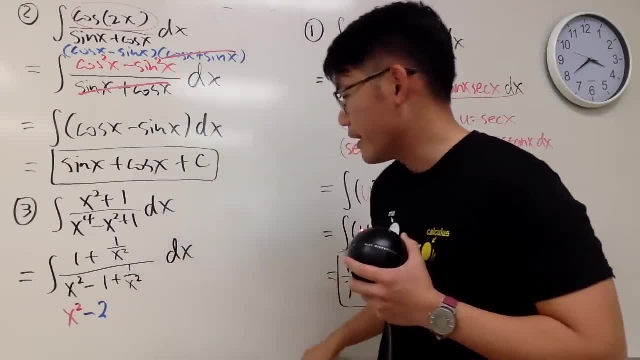 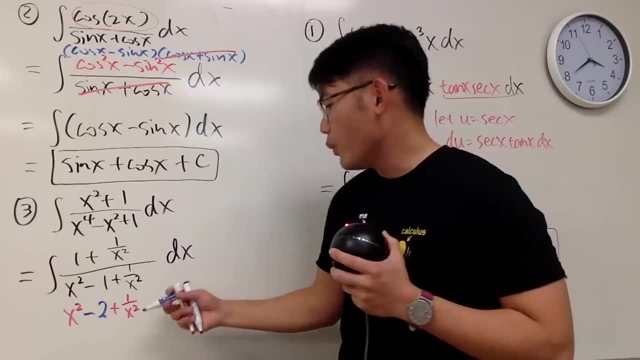 2. Minus 2.. And then we will add 1 over x squared, but of course this is not the same as that anymore. We are going to be adding the 1.. So it's like minus 1 and then plus 1.. So that's the idea. 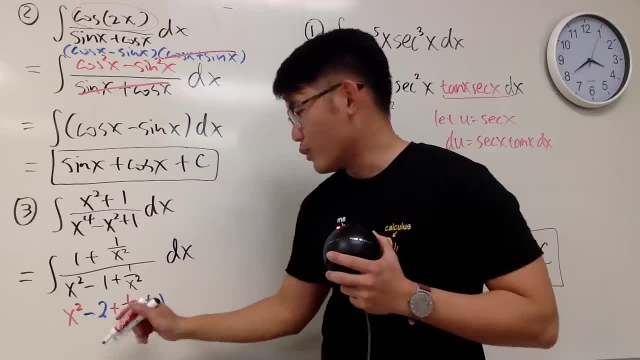 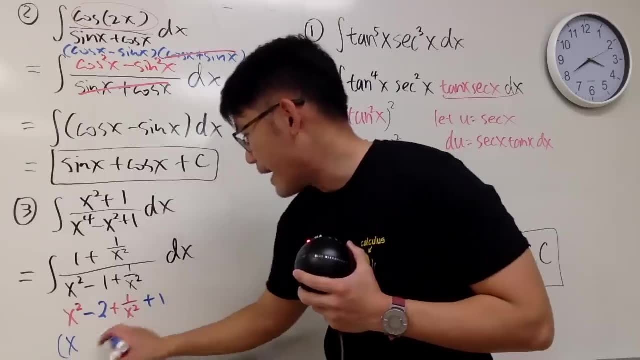 And the beauty now is this right here is factorable, and when you factor that- I'll just put this down in blue for you guys- This right here will give us x minus that, which is 1 over x, And that's a perfect square. 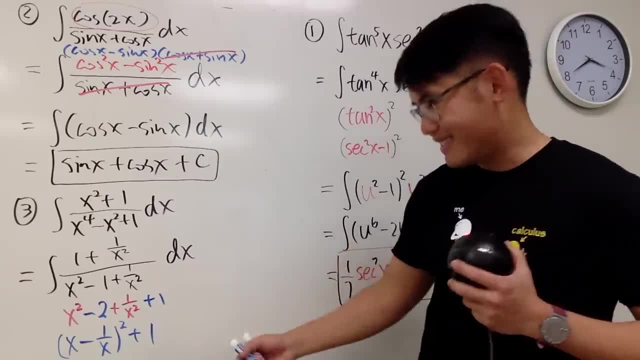 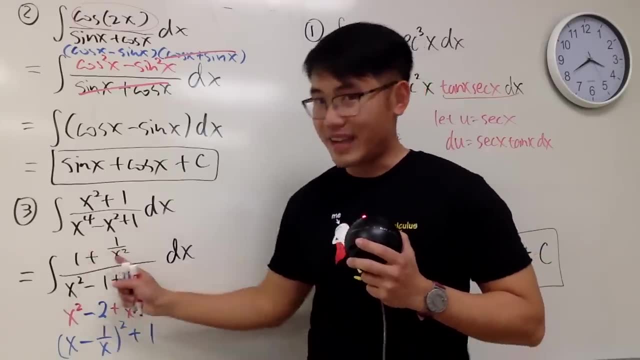 and then you have plus 1.. And what's this? Yes, You can just take a u sub. let u equal to this right here, and the derivative of this is precisely the top right here. So you can just finish this by u sub. 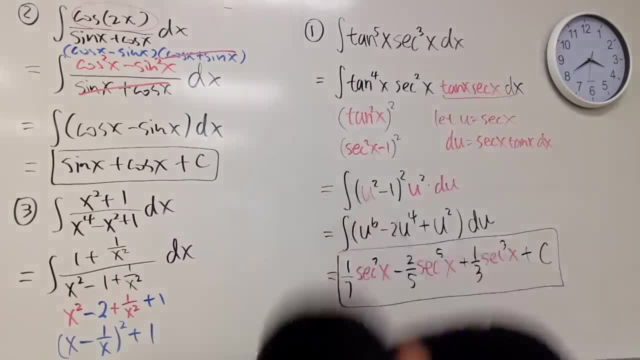 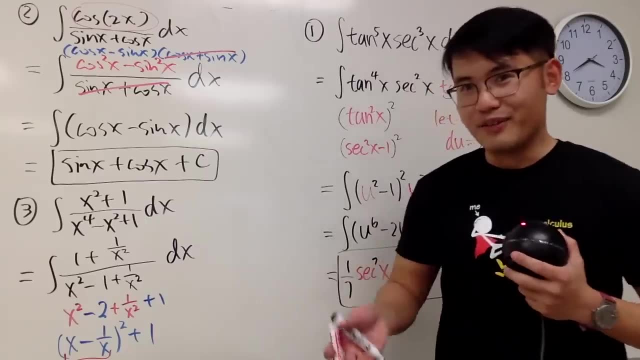 So let's do it real quick. I will take u to be the inside right here. These are the things that you don't see, because usually I just cut this off, you know, but like today, you will see everything. So anyway, we'll. 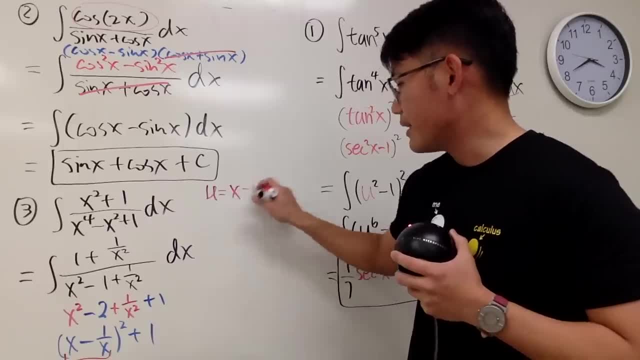 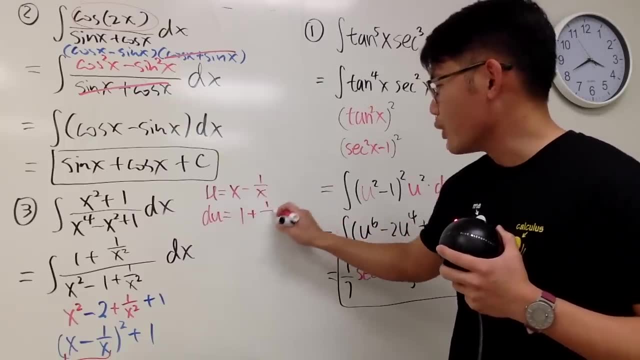 take u equal to x, minus 1 over x and notice when you differentiate this you get 1, and the derivative of negative 1 over x. we do get plus 1 over x squared dx. So this integral, you know. 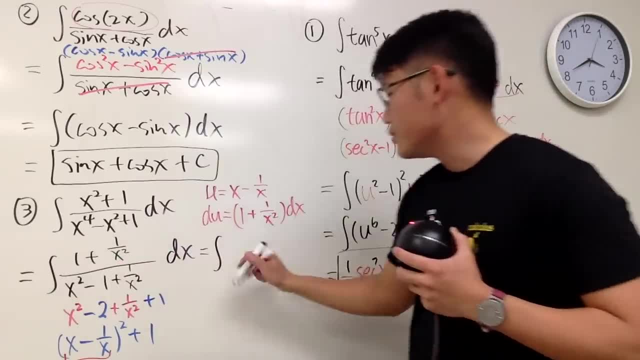 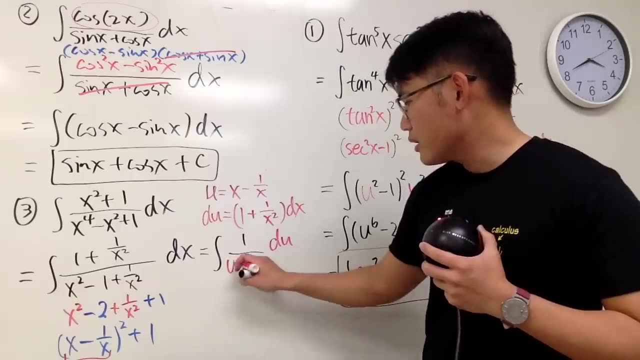 we can take that to the? u world right away. This is going to be the top, which is du, Let me just put down on the side- And then on the bottom we have that which is u squared plus 1. And what's this? 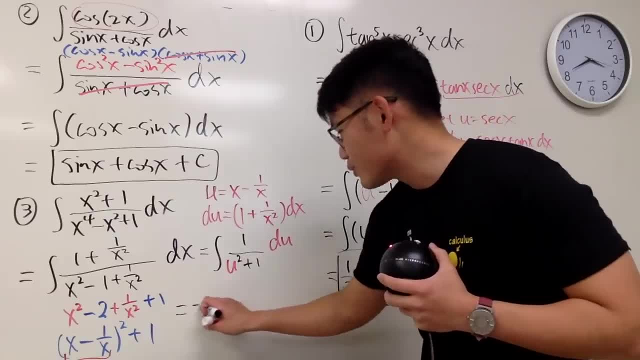 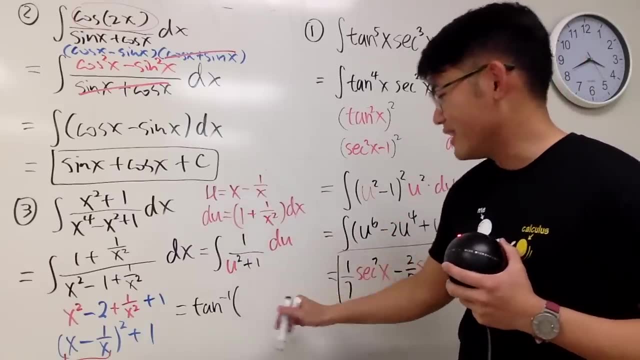 Inverse tangent of u. Very good, So I will just write that down for you guys: Inverse tangent, And we can just put a u right here, and that's it. So I just put down x minus 1 over x. 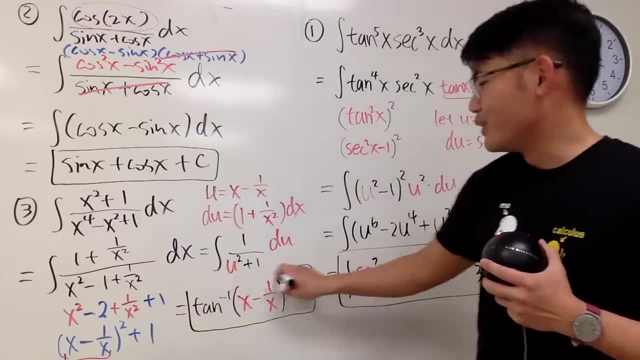 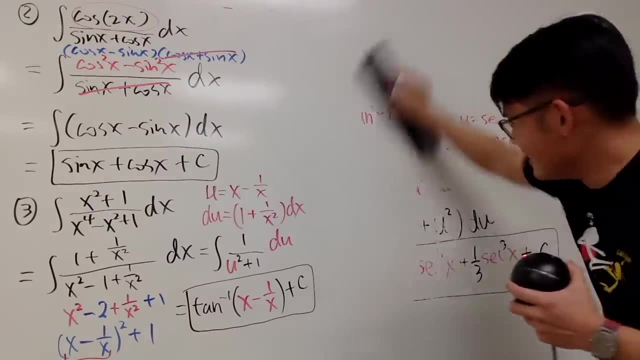 And we are done. So put a plus c. I told you we could do this right here, right, Okay. so 97 more to go, Yeah. And, by the way, this is how I feel when I run marathons too. 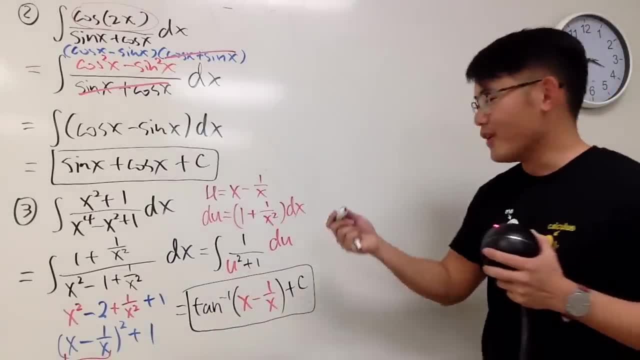 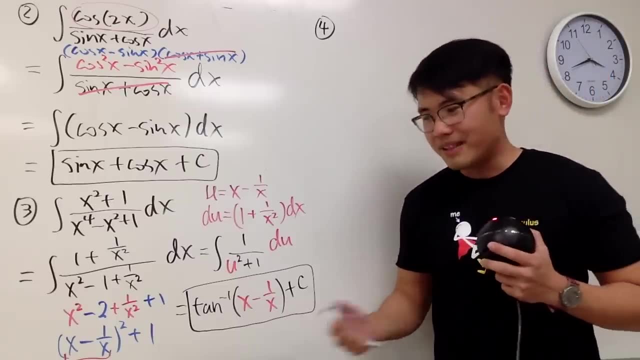 because it's like in the beginning that you will feel excited and then in the middle you'll start to do that- oh man, can you really do it? And you start to regret, and then by the end you are like, oh so. 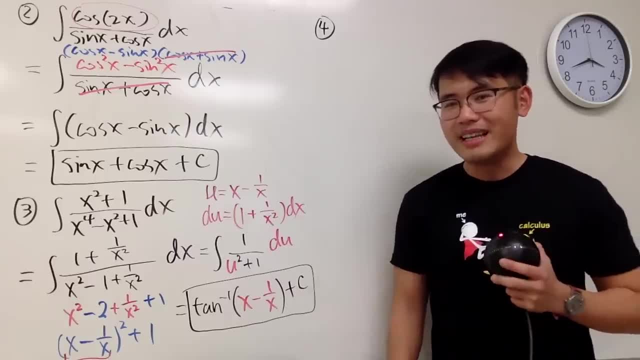 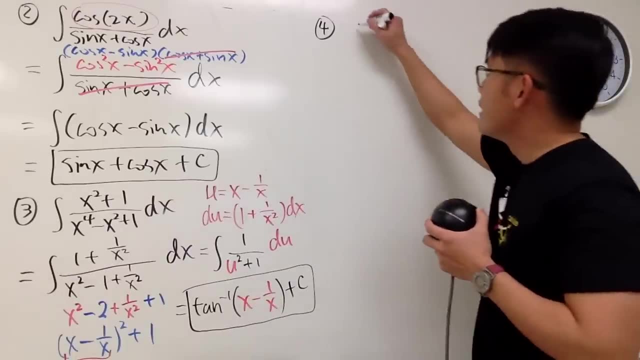 tired, but you can see the hope and you get happy, the joy, and after you finish, you feel so proud of yourself. Anyway, okay, number four, we have to integrate x plus e to the x square dx. right, 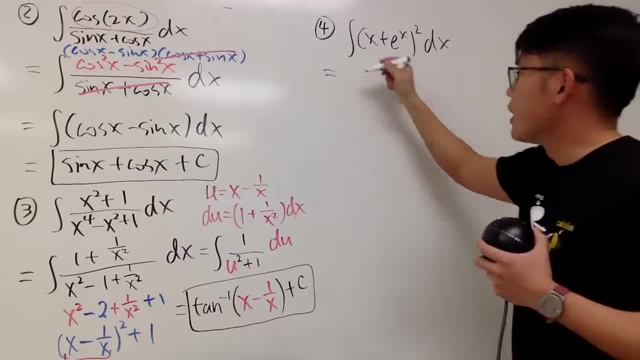 Alright. so to do this, I'm just going to expand it. so I will just say: this is going to be okay, this thing's square which is x squared, and then we add two times this and that which is x. 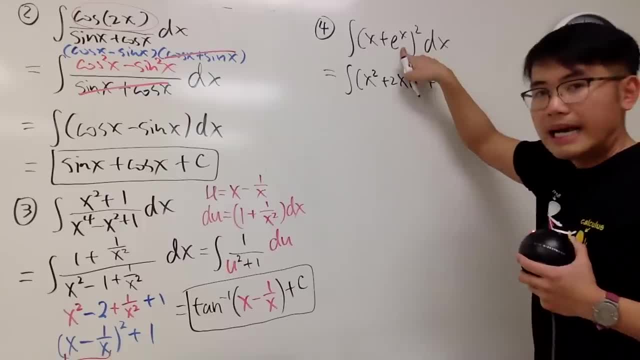 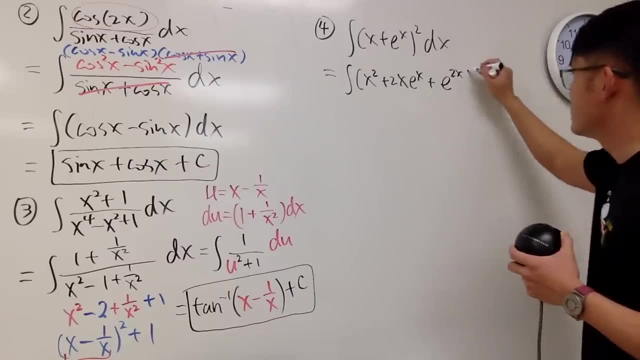 and e to the x. and lastly, we have to add this square: e to the x squared, we get e to the 2x. You just multiply the powers, so it's this and you have dx. Alright. so this and that are. 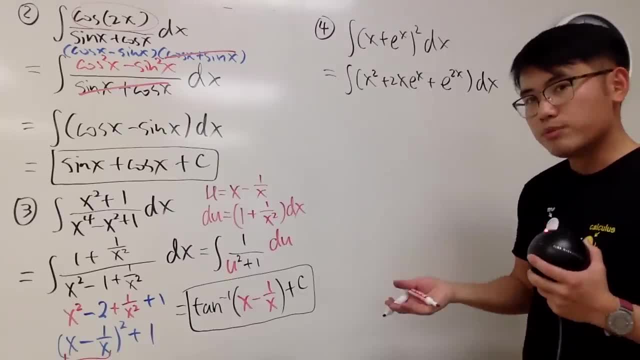 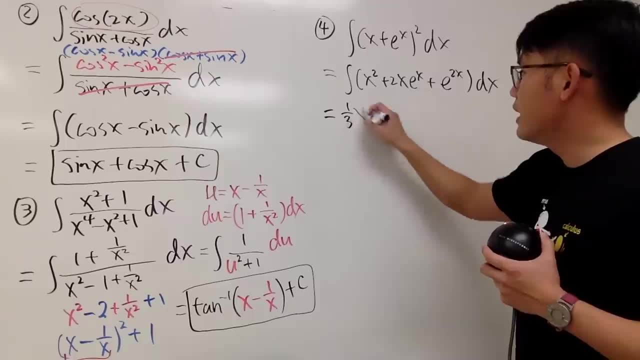 easy. but in the middle we technically have to do the integration by parts, and of course I'll do the di method for you guys. So let's see this right here. let's do it. we get one third x cubed and then 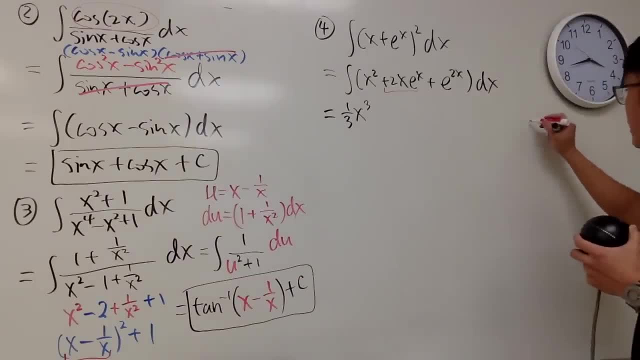 for this. let me just put it down on the side. right here I'm going to do the di method, so I will be differentiating 2x and I'll be integrating e to the x plus minus plus. this is enough, because when you 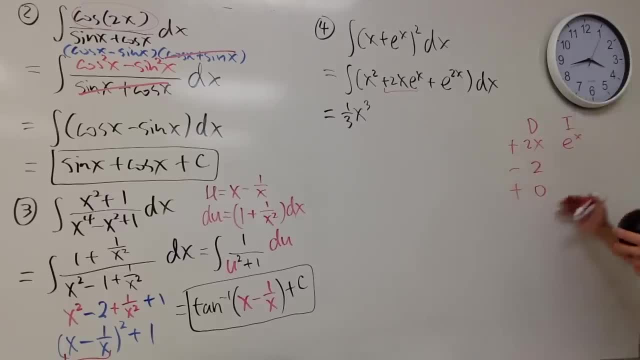 differentiate this one time, two times, you get zero. And then, of course, when you integrate e to the x, it's always e to the x. so that's good. And with that said, don't forget, you do this times, this, this times that you get. 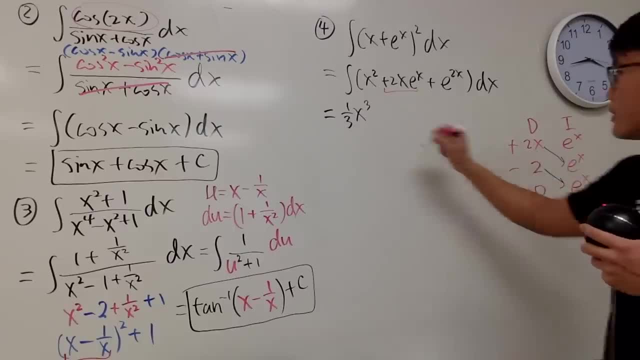 the answer. So the first part of the answer is this times that: so I'll just put down plus 2x e to the x, and then you subtract, don't forget the sign. so subtract 2 e to the x, like. 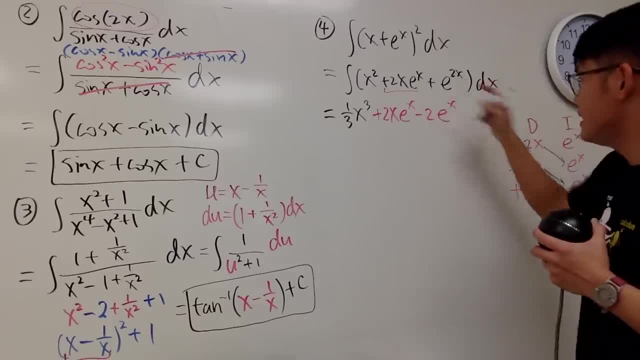 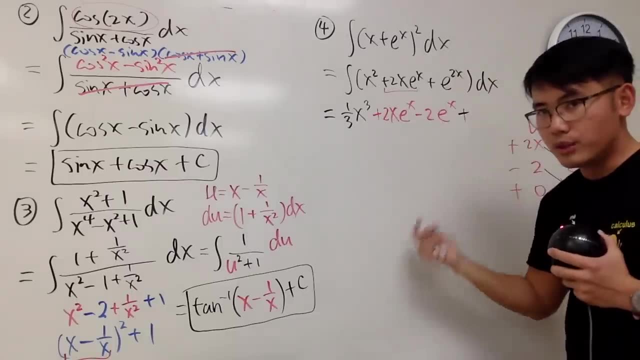 that. So we are done. And lastly, this right here, When we integrate e to the 2x and notice that the derivative of 2x is just a 2, so we can do the following. We can: just keep the e to the 2x as how it is, but don't forget the chain loop. but you have to do it backwards. The derivative of 2x is 2, so you have to actually divide it by 2,, which is the same as multiply by. 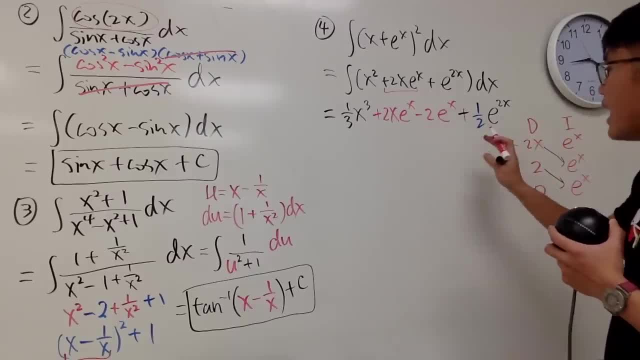 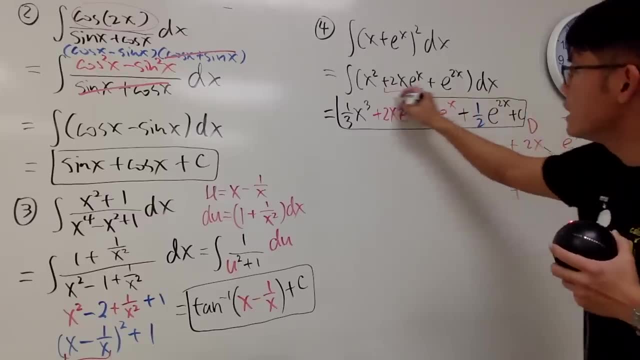 one half right there. And with that we are done. And I don't think there's anything we can simplify. we'll combine. so we just put plus z and this right here. is it right? Okay, doing good, doing good, I guess. 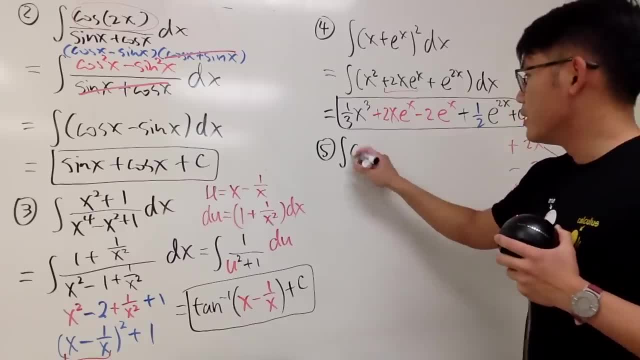 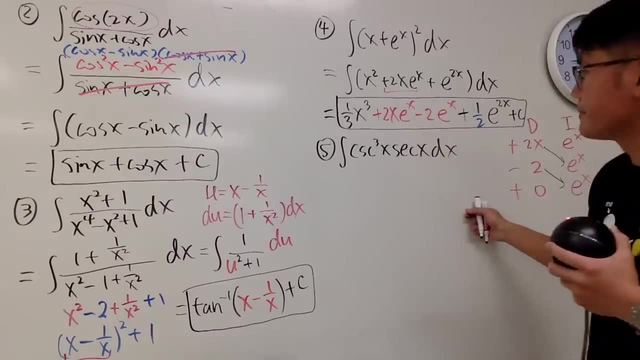 Number 5, integral of cosecant cube x times secant x dx. Hmm, Okay, this is an interesting one actually. Let's see. Well, that's the integral. I don't think I want to work with cosecant and secant, because I don't. 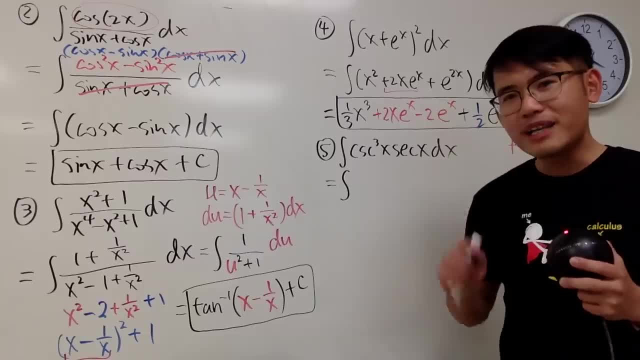 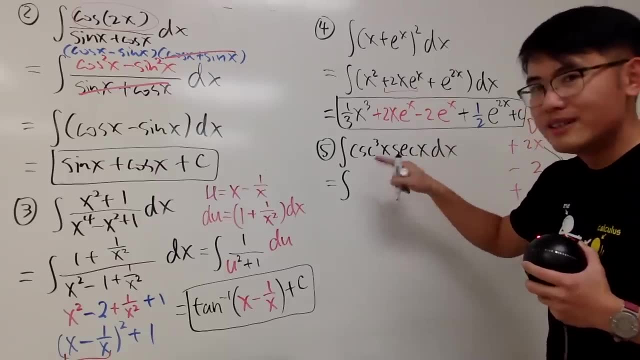 think they get along with each other that well in integrals. I know, sine cosine, they get along with each other much better in integrals, right? So I'll look at this as 1 over sine to the third power, and this is 1 over cosine. 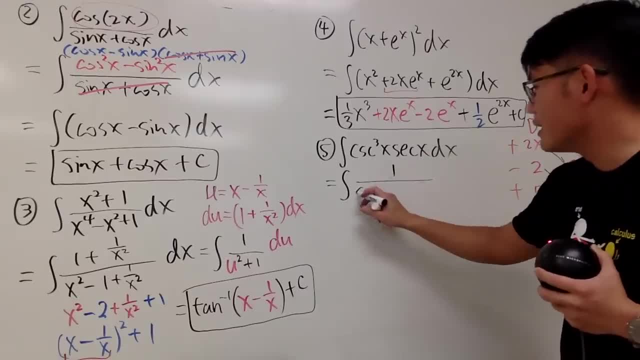 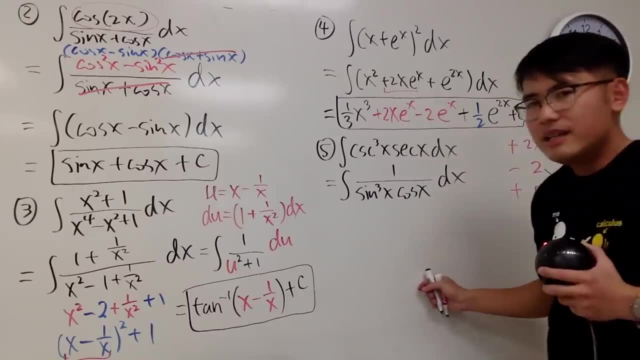 right. So I will just put down 1 over this being sine to the third power, x, and then this being cosine x, dx, like that. So this is good, but I don't think this is enough to work with, because if I want to do u sine, 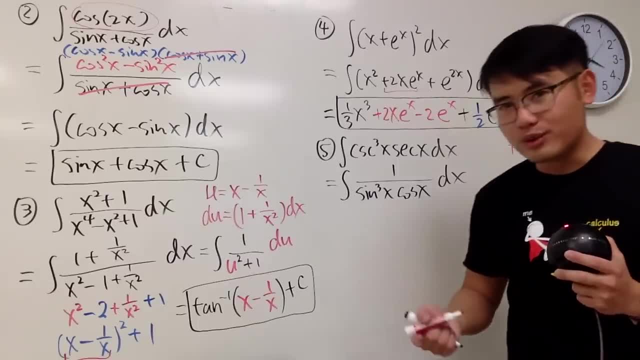 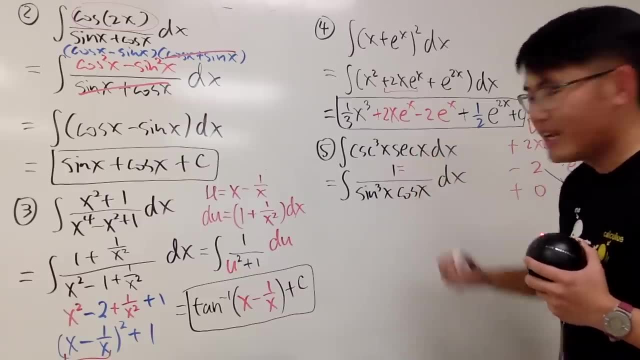 then I'm stuck right. I want to have more things to come with, and the deal is that I will be utilizing this 1.. As we all know, we like to look at sine squared plus cosine squared being equal to 1, but today, 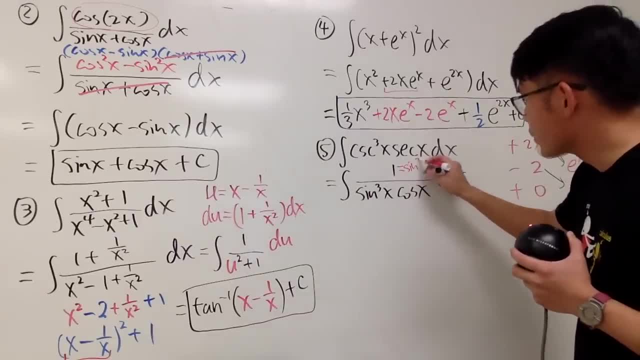 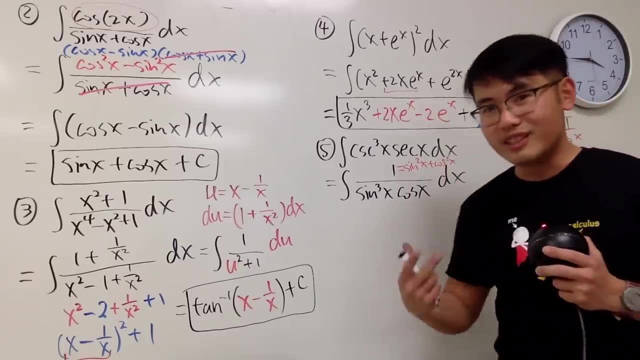 we'll do it backwards. We can look at 1 as sine squared x plus cosine squared x, like that. How's that? And again, the purpose is: I want to have more things to work with and the denominator is just of one term. And the beauty of doing. 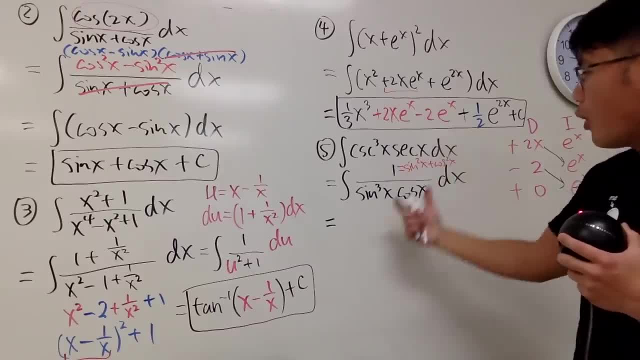 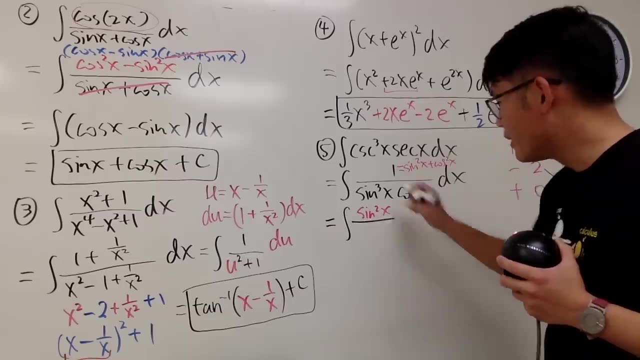 so is. I can do the first term on the top over that on the bottom. So I'll write this down right here for you guys. I will get sine squared x over this denominator, which is sine cubed x, cosine x, And then we add: 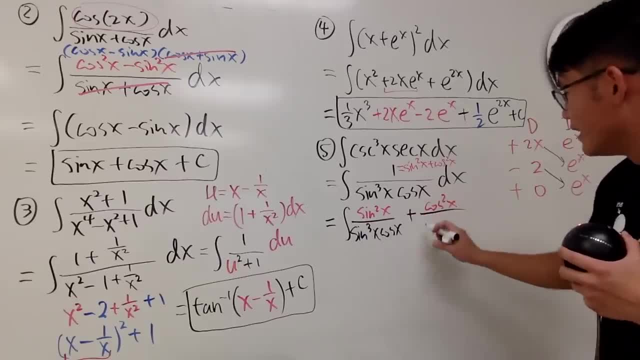 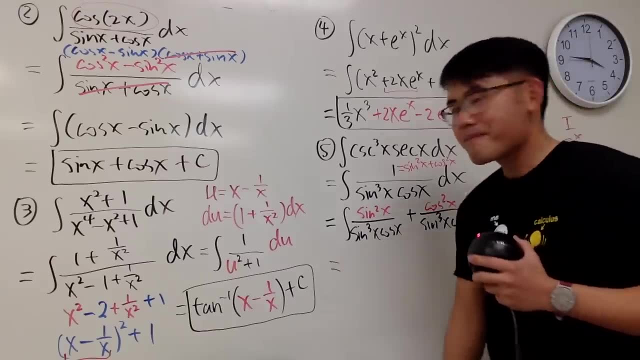 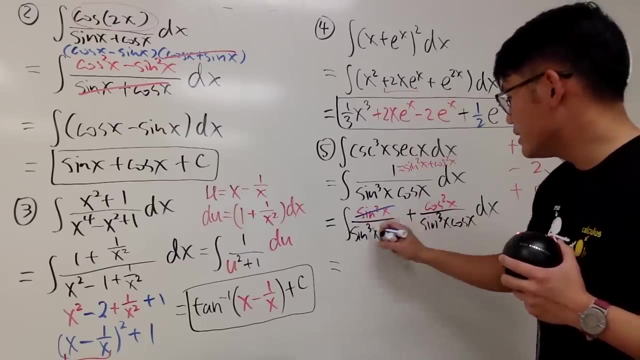 cosine squared x over sine cubed x. cosine x like that dx. Okay, This right here is pretty nice because, as you can see, we can actually just cancel this and that, so you have one power right here. So that's okay. 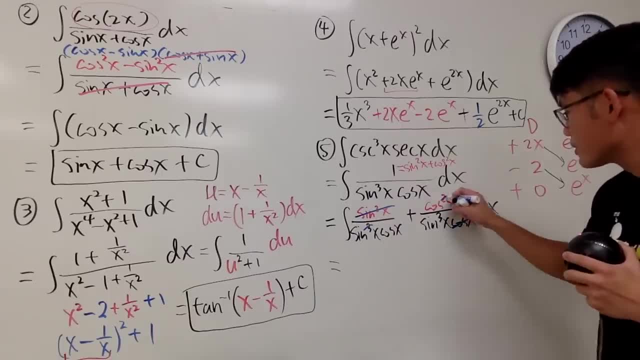 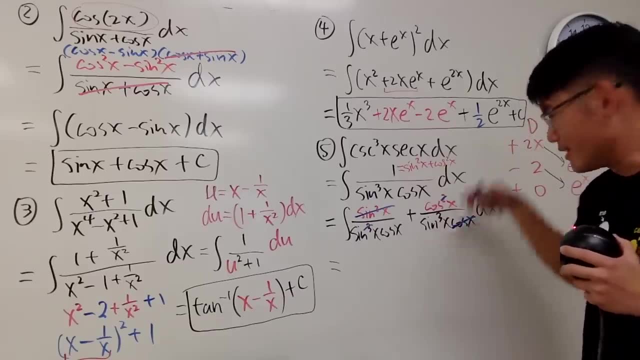 This right here is actually easier, because when you cancel the cosine and cosine you have sine x in the denominator. and then to a third power, right here, right, You can do u-sub because you have the cosine x on the hub to help you out. 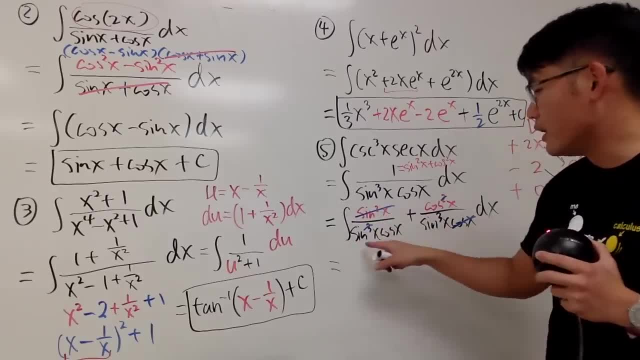 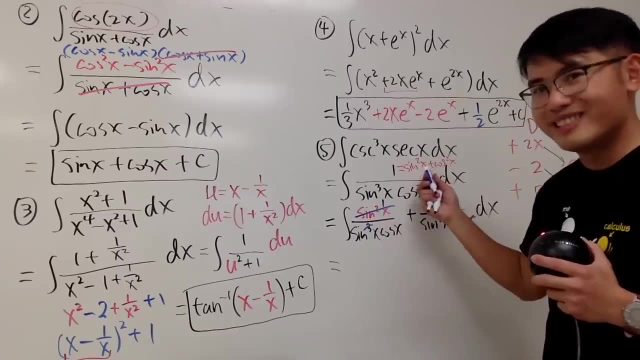 But the problem is that how can we integrate 1 over sine x times cosine x? Well, don't forget this, right here is technically a 1 now, and we can do this again. So I will write this down right here for you guys. This is the. 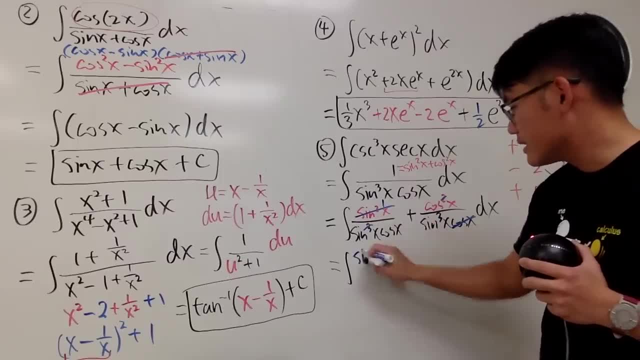 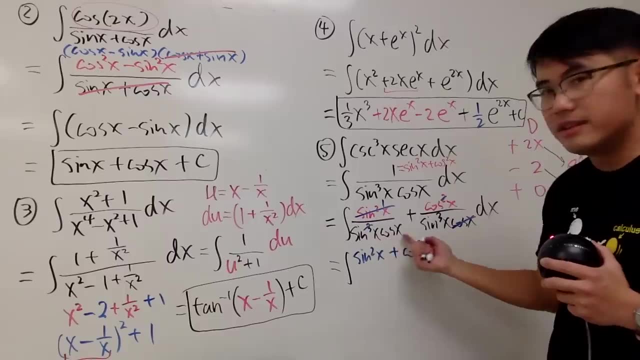 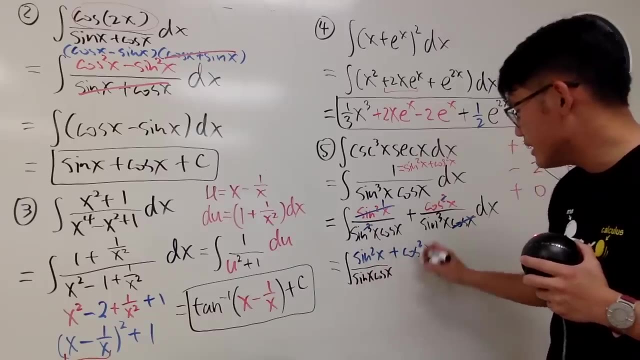 integral. I will write the 1 as again sine squared x plus cosine squared x, and then both of them are over this denominator right. So I will just divide this by sine x, cosine x, and I will divide this by sine. 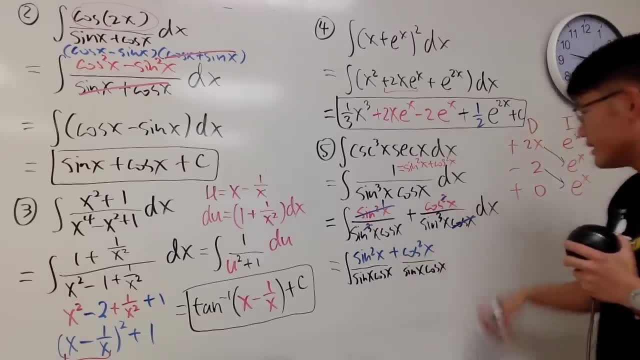 x, cosine x, like that. And let's, let's see- I might as well put this down right here together: why not Cosine x? well, yeah, cosine x over, and this was sine to the third power, x like. 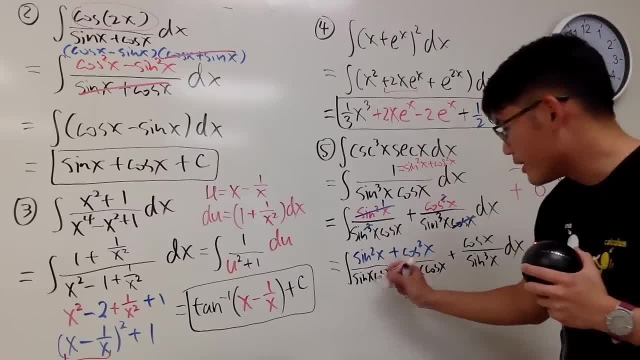 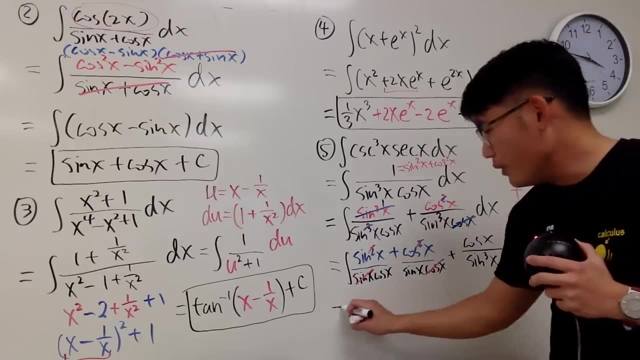 this: More cancellations happening. Look this right here is good, This and that cancel. you have the first power on the top now, and then this and that cancel- very good, So all in all, we are just doing three. 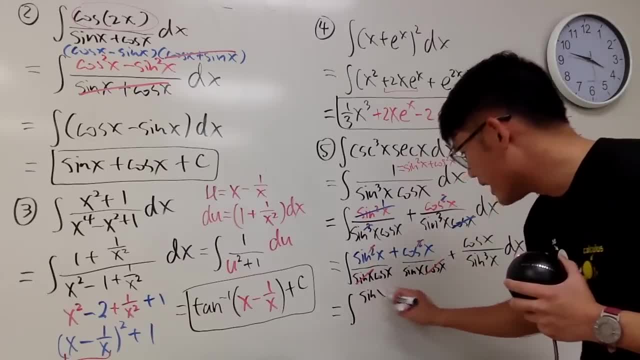 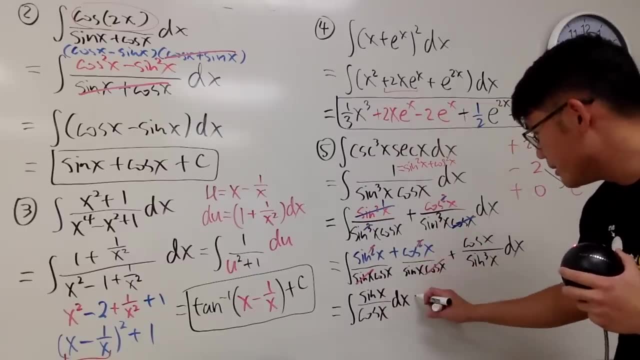 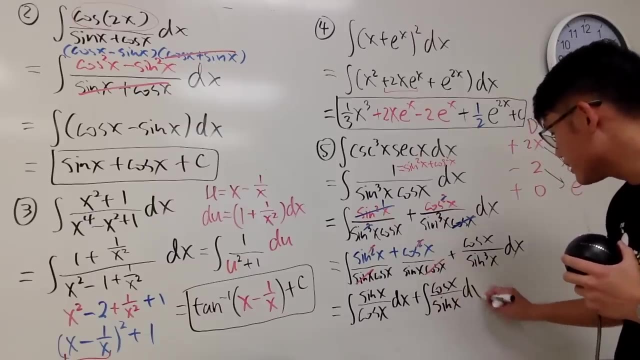 little integrals. The first one is the integral of sine x over cosine x, and let's close that, so put down the dx. and then the next one is this being plus integral: cosine x on the top over sine x on the bottom, and then the dx and 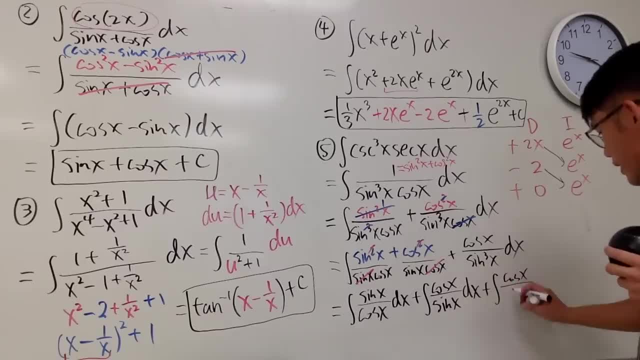 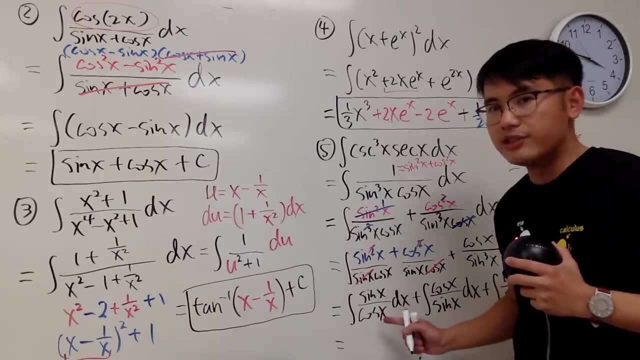 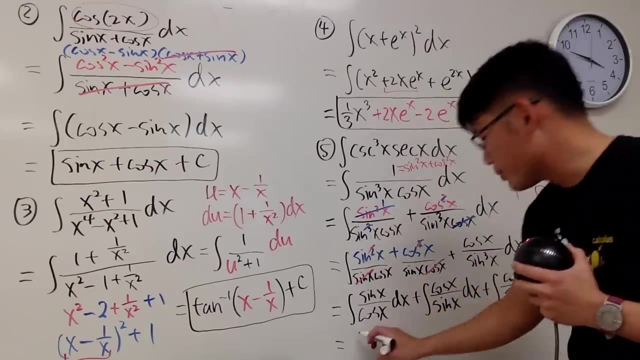 this right here: integral of cosine x over sine to the third power, x, dx. Alright. so, as you guys know, this right here is just tangent and if you integrate tangent you get natural log absolute value of secant. so I will just put that down right here. 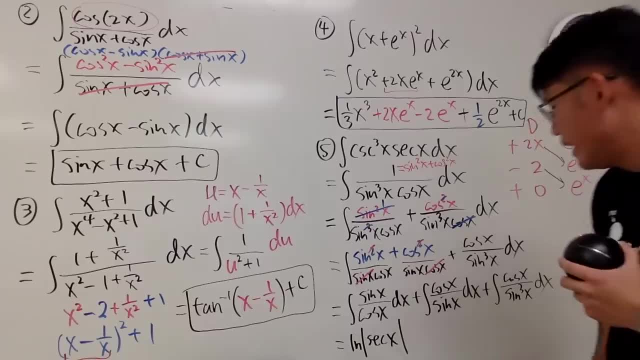 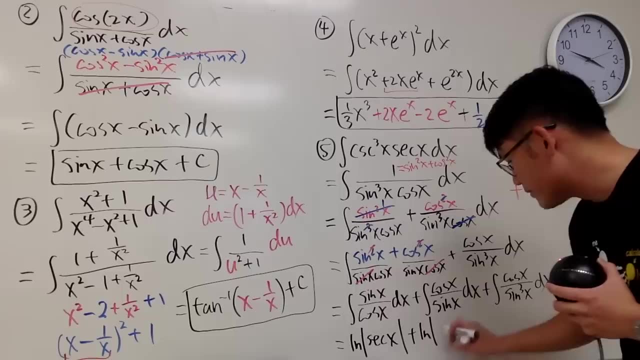 for you guys: natural log- absolute value of secant x. and this right here is technically cotangent and of course you can also do u-sub, but either way that will tell you this is just the natural log absolute value of sine x. 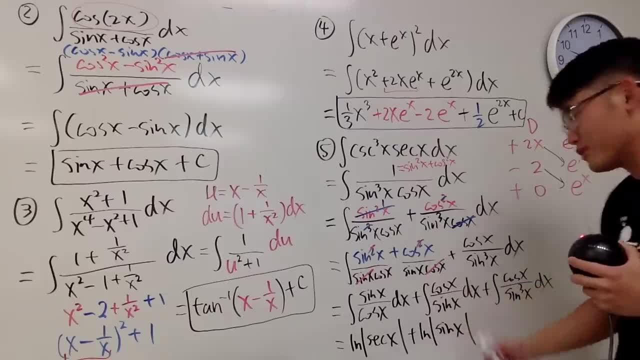 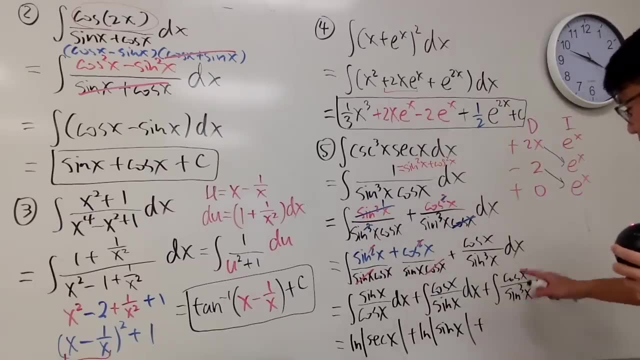 because if you let u equal to sine x, you get that. So everybody right here is pretty much similar. Lastly, do not have the ln addition. This right here is going to give us 1 over u to the third power, because you: 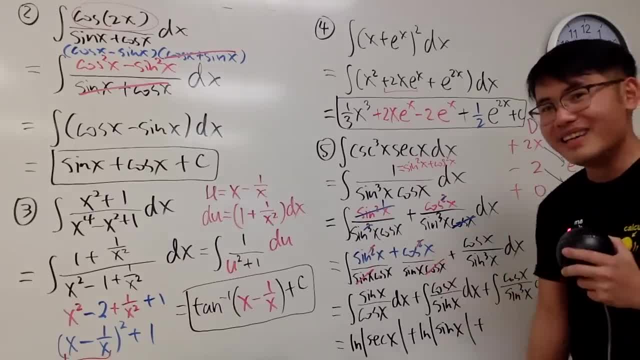 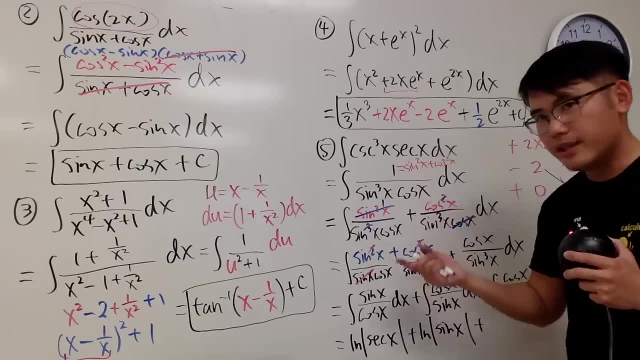 have that sine to the third power and we cannot do the natural log Alright. so 1 over u to the third power, in other words, u to the negative 3, plus 1, which is negative 2, divided by that. 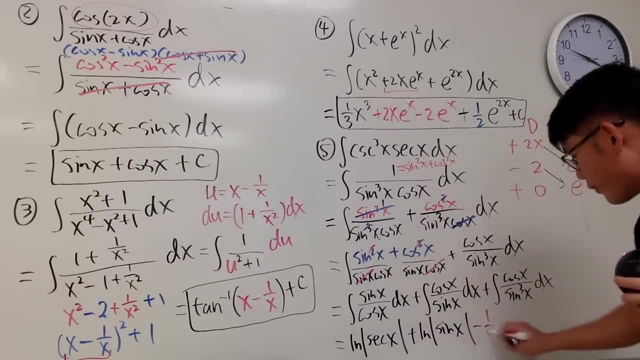 you end up with negative 1 over 2. And you get u to the negative 2 power where u is the sine. so I will just put down the sine in the denominator right here. Okay, Sine to the second power, x like that, And: 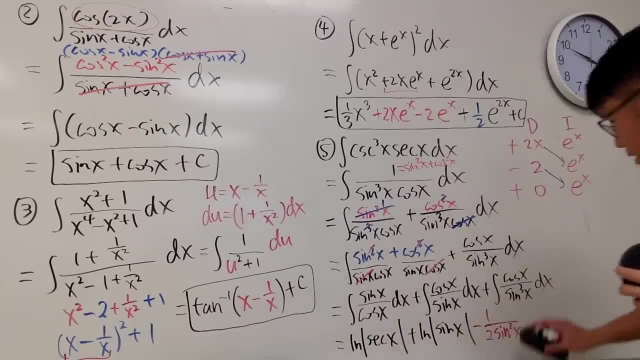 of course, you can also write this down as what? Cosecant. So if you like, you can also write this down as cosecant. Actually, let me just write it like this for now: Sine squared x, Okay, And. 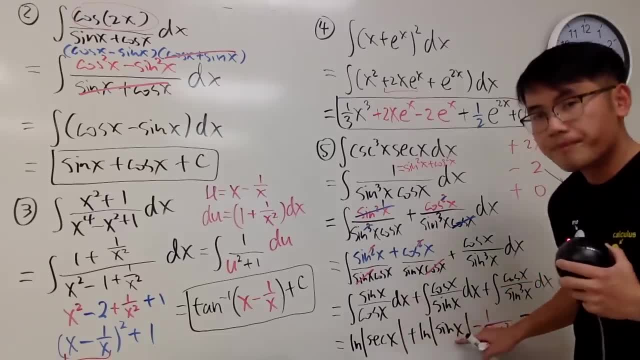 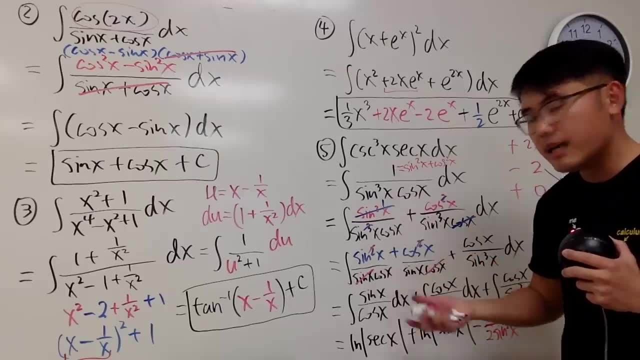 the truth is, you can put this and that together. When you have this and that together, of course you are doing sine times secant, In other words sine divided by cosine. so the black part will give us natural, log, absolute value of. 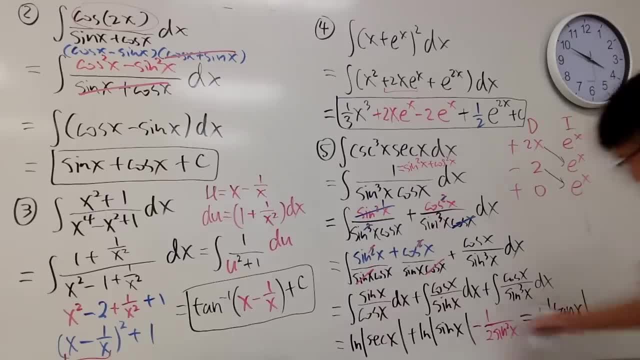 tangent x And of course now I will fix this- This is minus 1 half. I will put this down as the cosecant Secant. Yeah, I guess I can still see Cosecant squared x And we are done, So put. 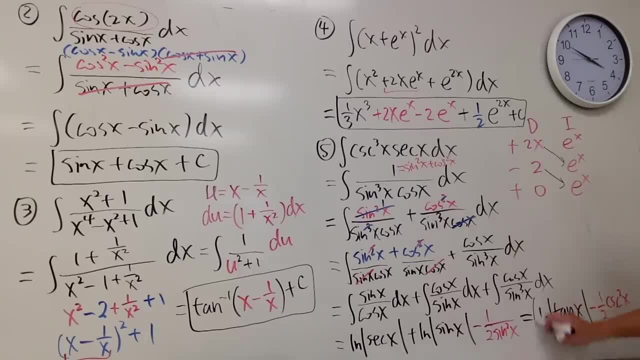 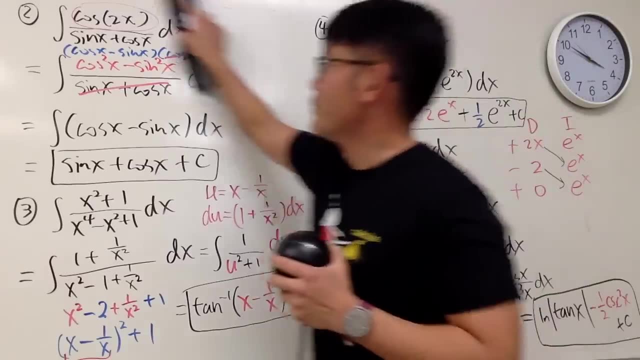 a plus c somewhere that you can see. So put a plus c right here. Very good, Okay. so, wow, I can fit 4 integrals right here. That's pretty cool. So now let's see 5 integrals done. Took me. 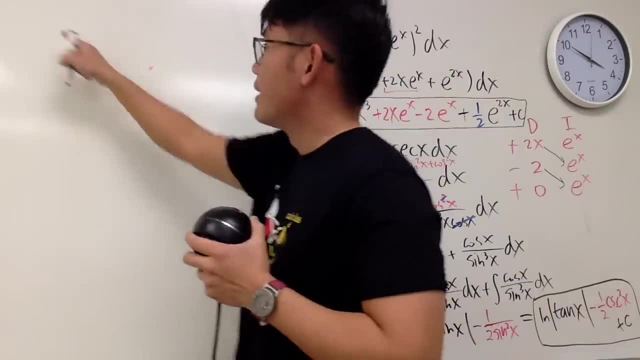 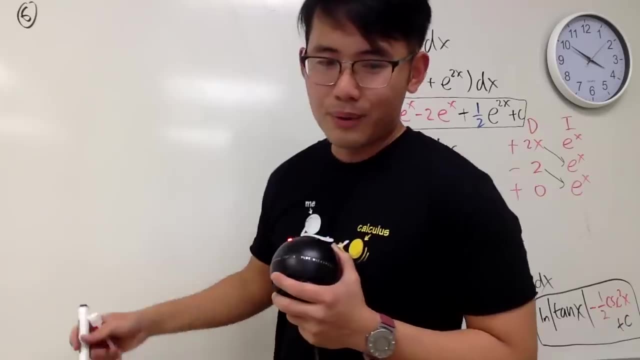 20 minutes. Right, let's see number 6 right here. Whew, I feel it's kind of getting tired, but it's okay. It's like the 6th mile or so. Anyway, integral of cosine x over we have. 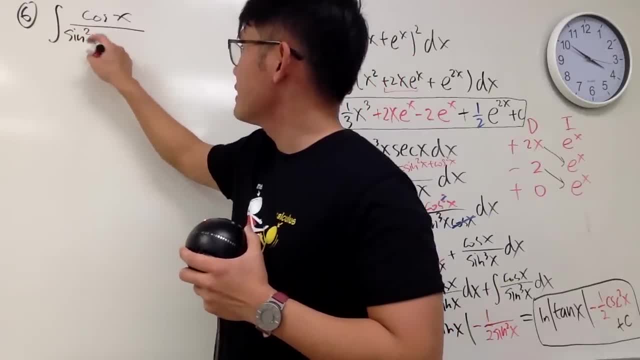 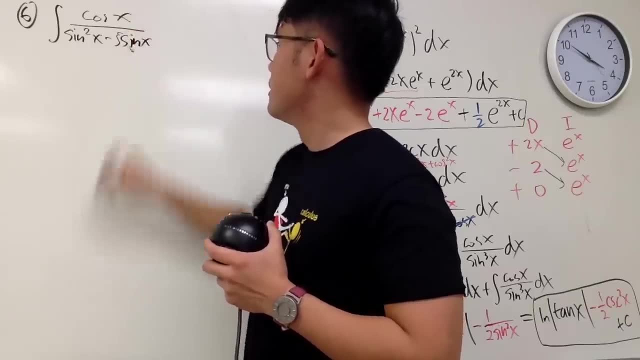 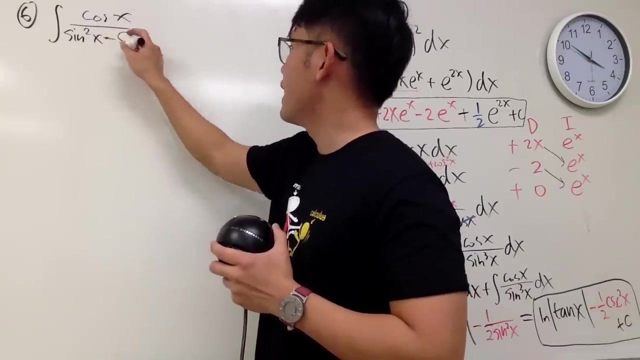 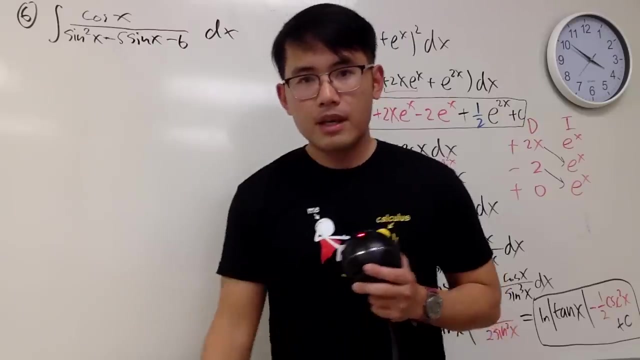 sine squared x minus 5 sine x minus 5 sine x minus 6.. Right, so this is the question, right here. Minus 5 sine x minus 6, dx, like that, What's the cosine x on the top? Well, notice that. 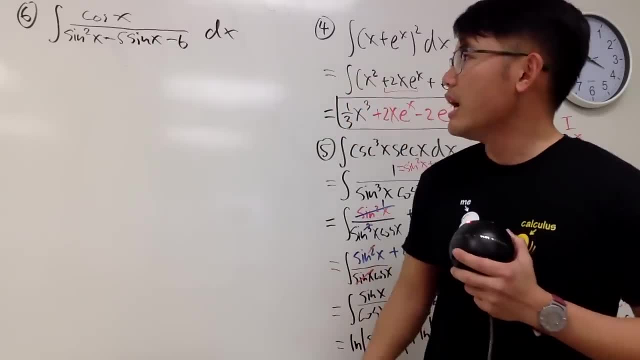 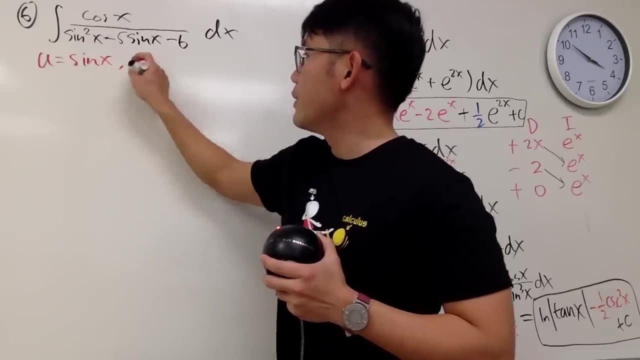 again we have sine cosine in an integral, So that's actually a good news And I can take a u sub real quick. I can just let u equal to sine x And with that said, we know du will be just cosine x, dx. 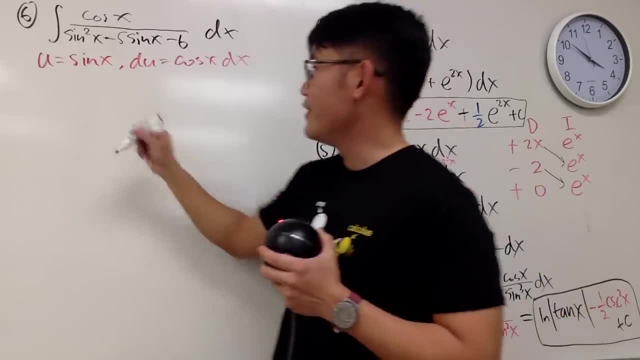 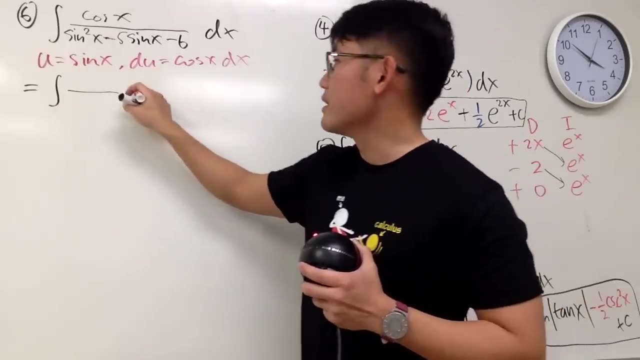 So, thanks to the cosine x on the top, we can do this very nicely, Right? So, as you can see, this is going to be the integral, This and that is the du. so I'll just put that down on the side right here for you guys. On the top it will be just 1.. 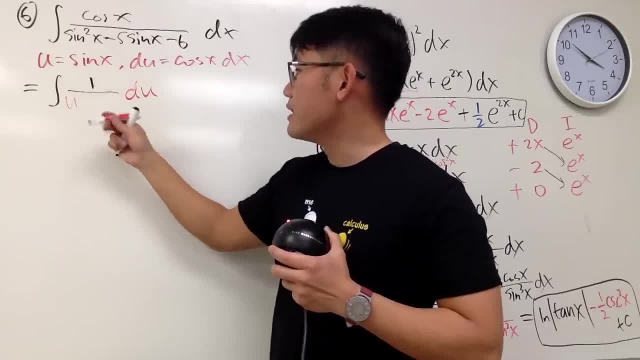 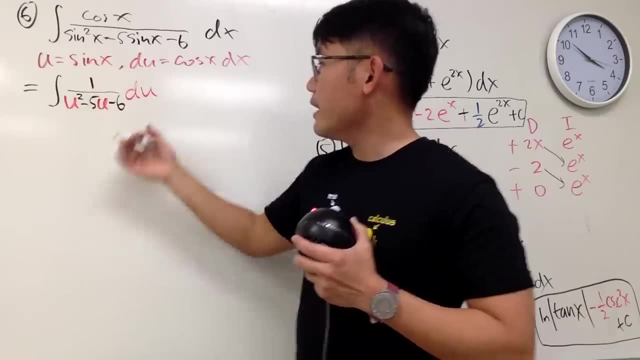 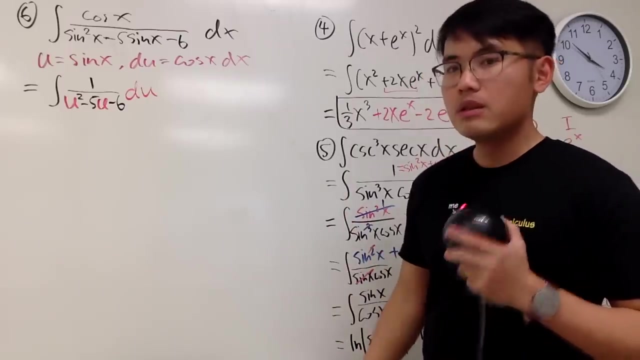 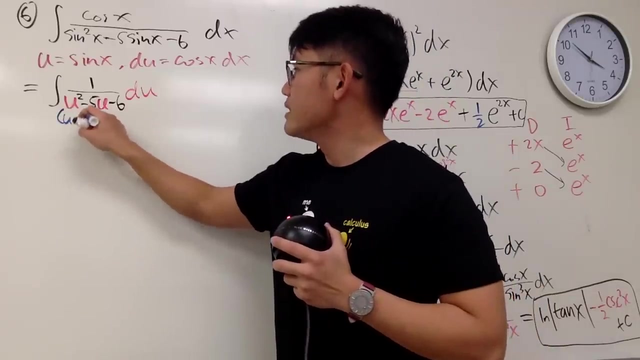 This is going to give me u squared minus 5u minus 6.. Alright, now we have a rational function to deal with. Hmm, of course do partial fraction and, of course, top-down method. So here's the deal: If you factor this, you get u minus 6 times. 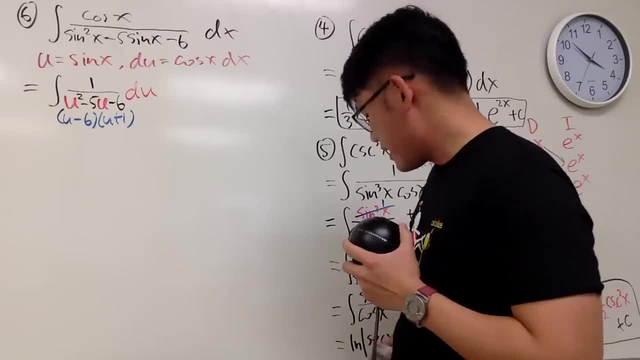 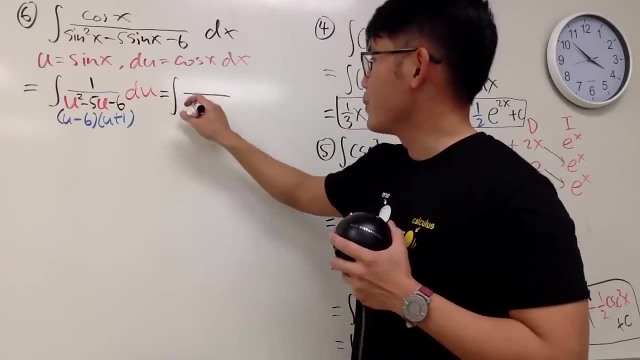 u plus 1.. So that's the factoring for that, and then we are going to do this by the 58: 00 to curry method for the partial fractions. so we know we have the? u minus 6 here, and then you add–the other one. 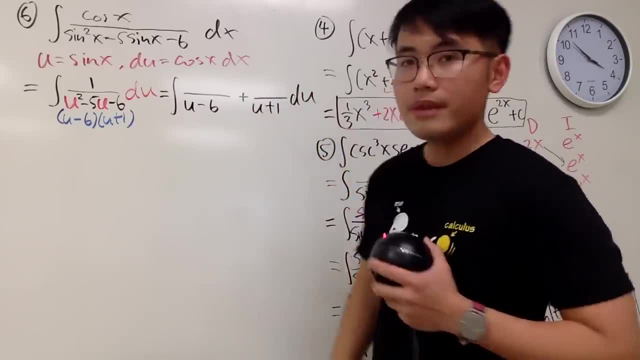 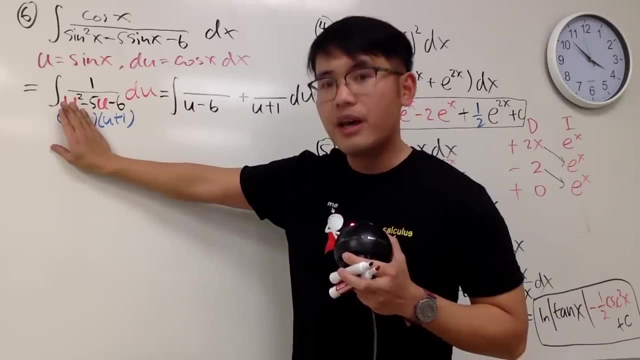 is the u plus 1 du. Okay, here is the deal to figure this out. you are going to come back to the original, you're going to cover up the same denominator and you have to ask yourself: how can you make u minus 6 be zero? Well, x- u has to. 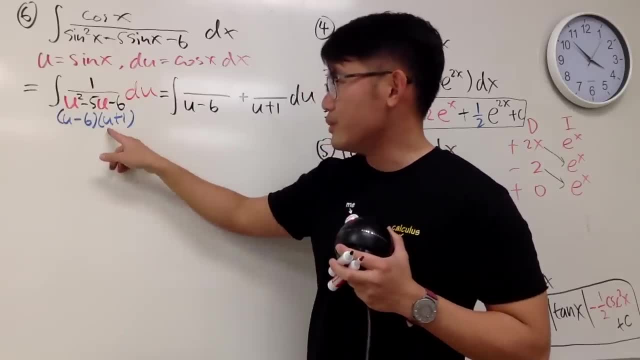 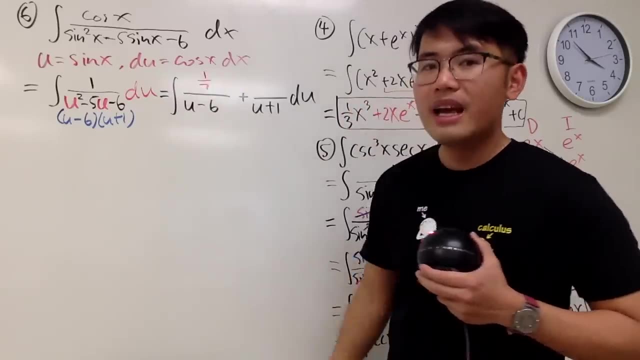 be 6.. And you are going to put 6 into this u and you have 1 over 6 plus 1,, which is 1 over 7.. So you have 1 over 7 here And to figure this out right here, you are going to go back to the. 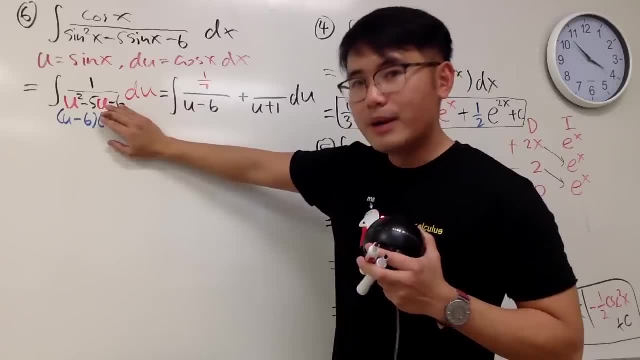 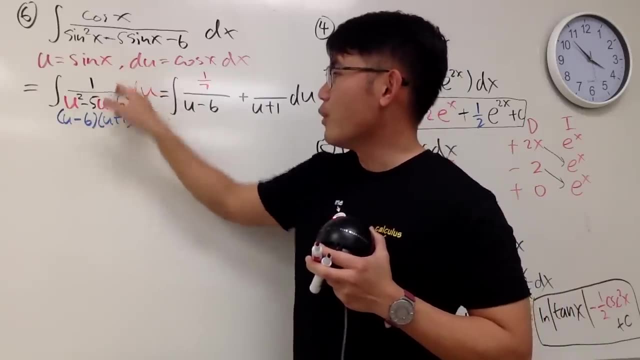 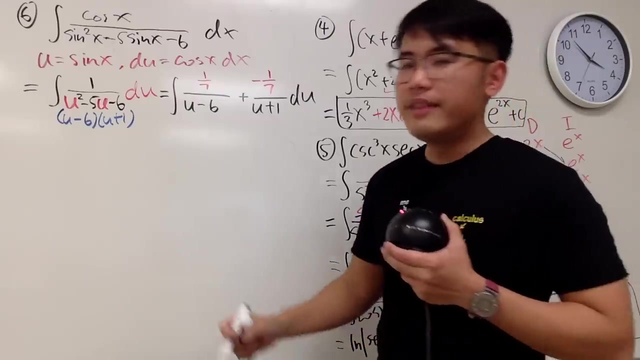 original fraction and you are going to cover up the same denominator. And how can you make u plus 1 to be 0?? u has to be negative 1.. You put this here, which is going to give us 1 over negative, 1 minus 6, in another word, negative 1 over 7, like this. And now we can just integrate: 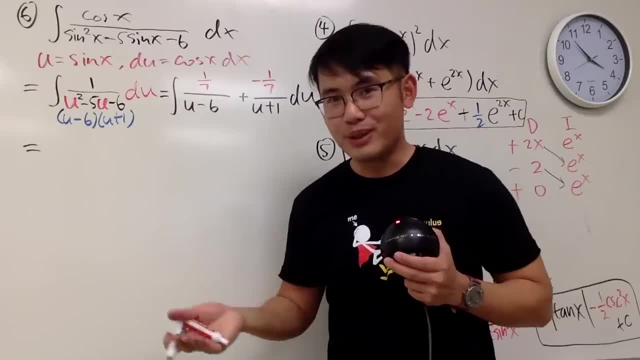 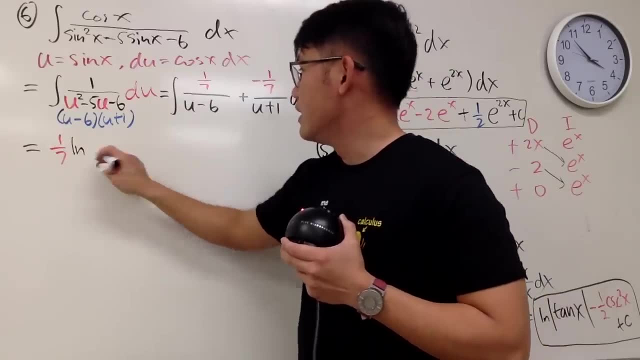 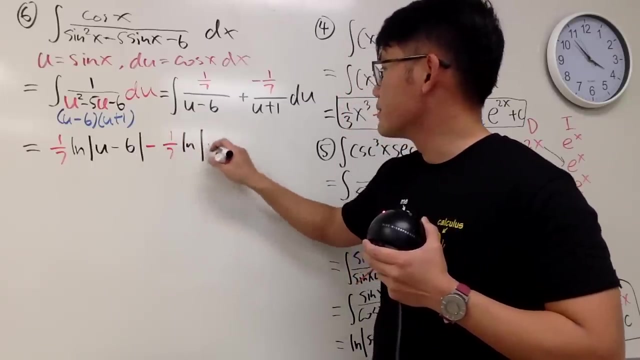 these guys- And yes, these are the natural log situations, because the buttons are just linear. So for the first one, we have 1 over 7, natural log absolute value of u minus 6.. For the second one, minus 1 over 7, natural log absolute value of u plus 1, like this: 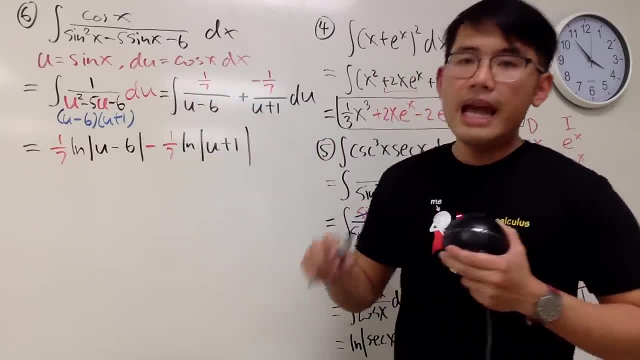 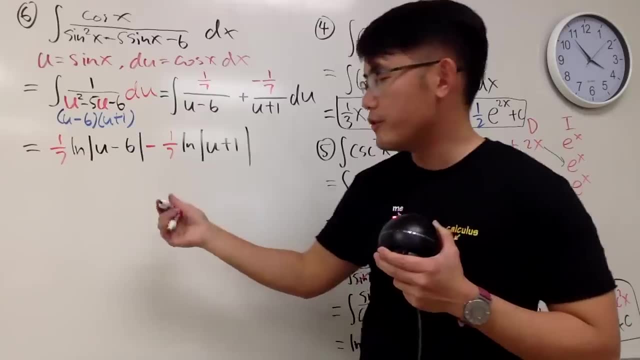 I'm not going to put it on the plus c yet, Because u is sine x And also we can combine the natural logs together. Perhaps I will leave the 1 over 7 on the very front. So I'll write this down. I will factor out the 1 over 7,. 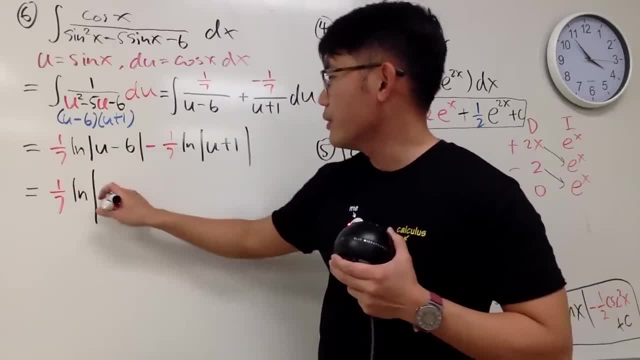 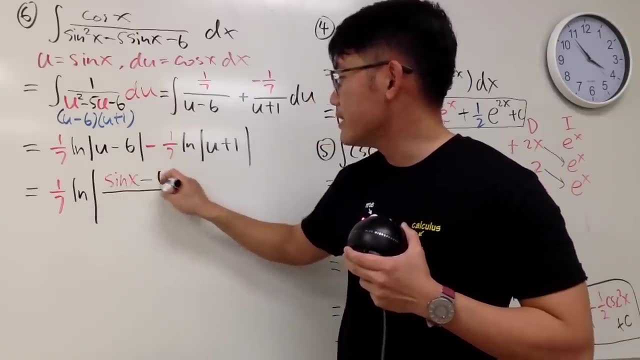 and I will just write down one big natural log with the absolute value. This will be on the top and u is sine x. So I'll put down sine x here and then minus 6. And then for the other one it will give us sine x plus 1.. 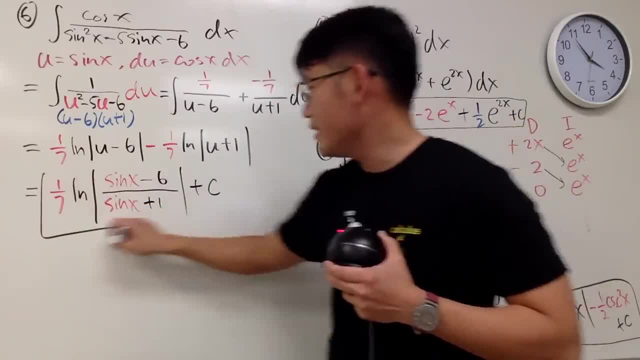 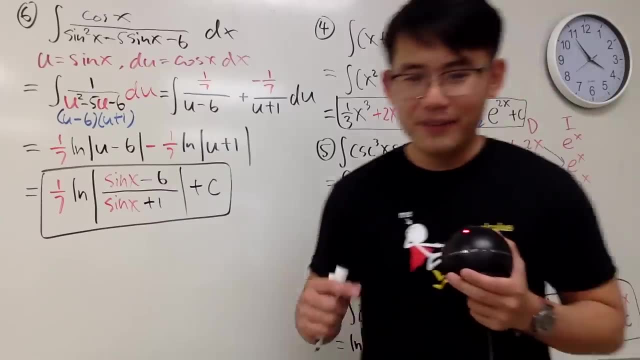 Like that, And we are going to put a plus c And here is the answer. Very nice, huh, I cannot go. We have a lot more to go. We have 94 more to go. So next one: Okay, slightly easier. 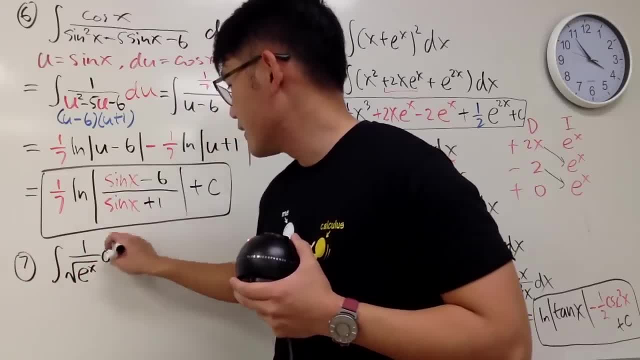 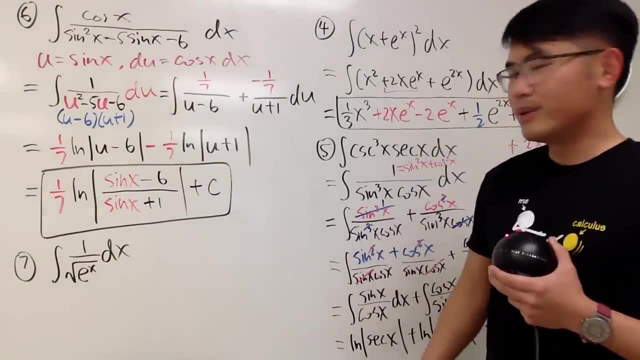 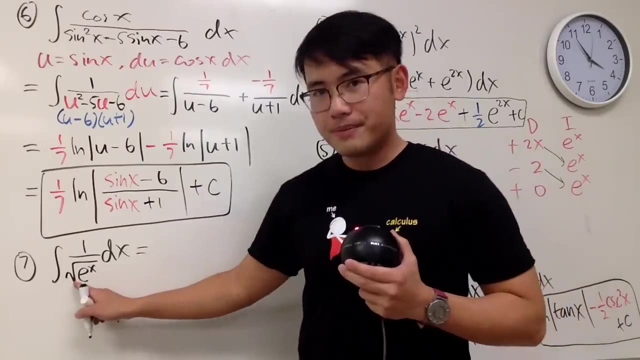 Integral 1 over square root of e to the x, dx. All right, Right there. What can we do? Don't worry too much, This is not that bad. This right here. remember the square root. it's the same as saying the one half power. 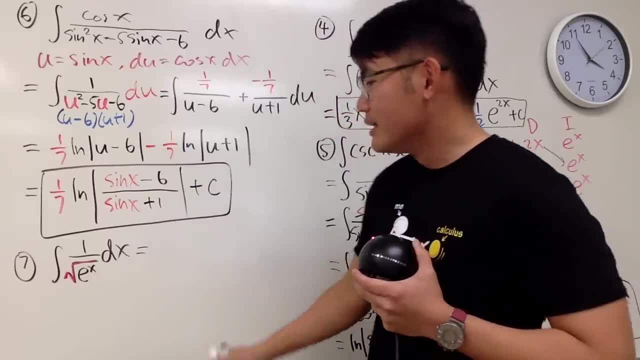 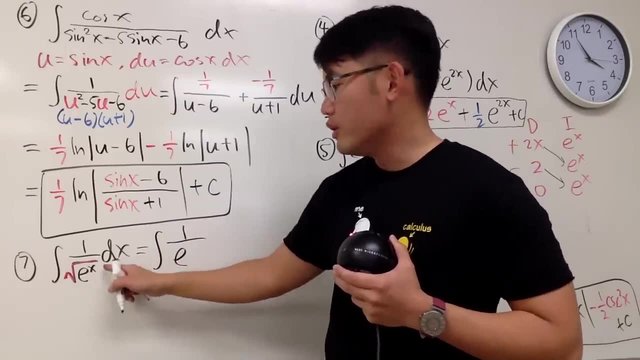 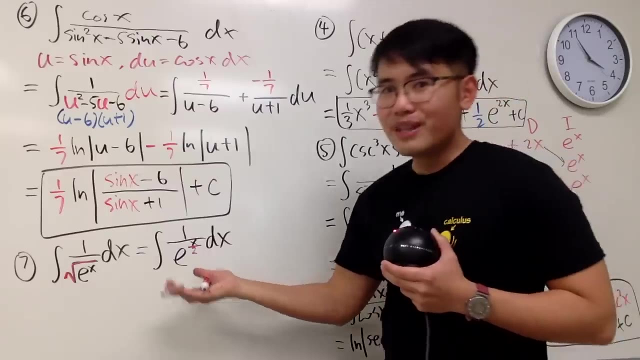 You almost always look at square root as the one half power. So in other words, this right here is just the integral of 1 over e, And when you have the one half power you multiply by the x, So you just get x over 2.. And don't get upset with this, because when you have this in the 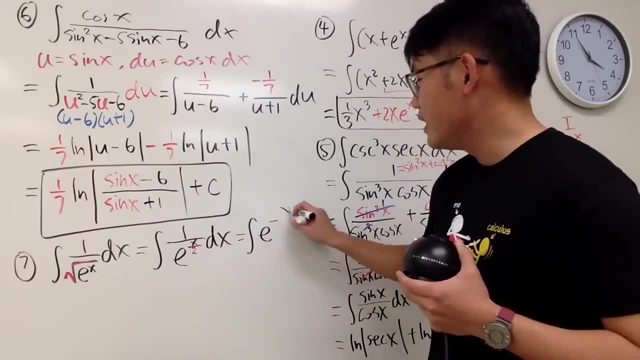 denominator. you can just bring this up- which is the integral of e to the negative x over 2 power, And this is x over 2.. So this is x over 2.. So you can just bring this up, which is the integral of e to the minus x over 2 power. 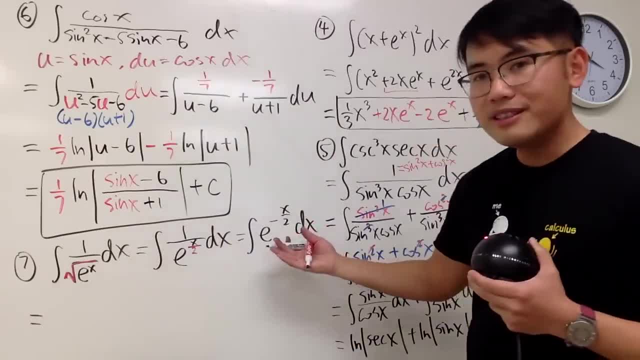 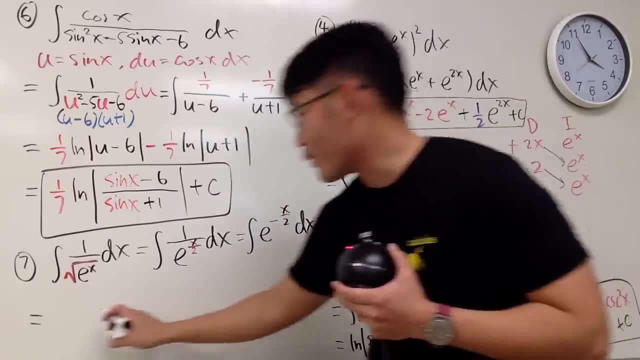 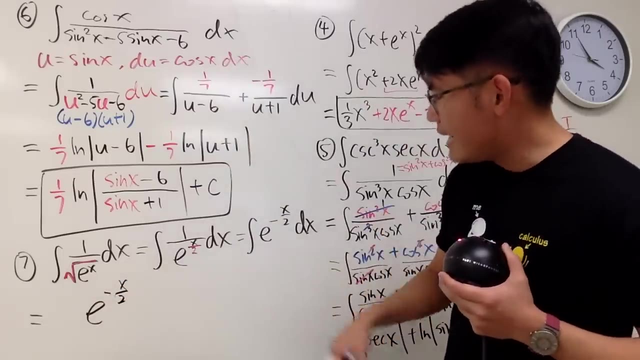 actually very nice because to integrate this, notice that the derivative of this is just negative 1, half, and you know we can just first keep this part right here. e to the negative x over 2, and the reverse. Chengdu says we have to divide it by the derivative right here. so we have. 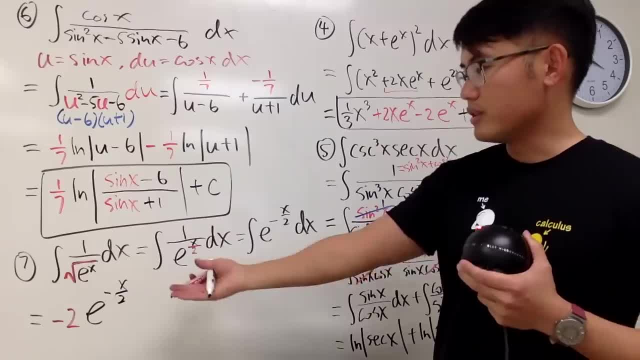 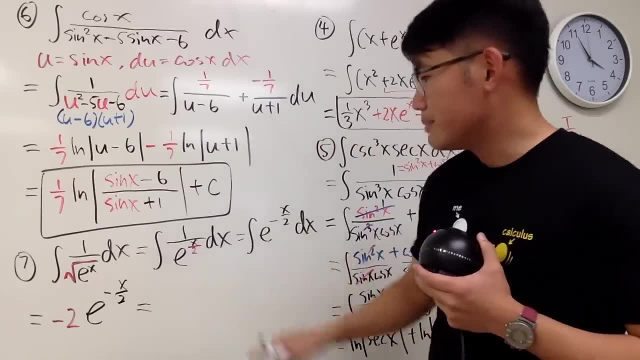 to multiply by negative 2, just like that. And of course you can do a quick check: if you differentiate this, you will end up with that. But anyway, perhaps I'll write this back in the original form, because negative 2, I can put that down in the numerator and we can put this down. 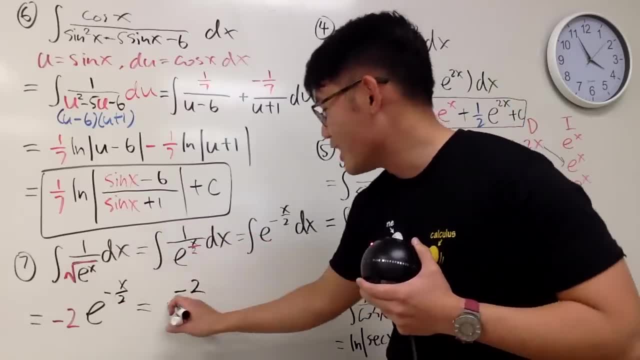 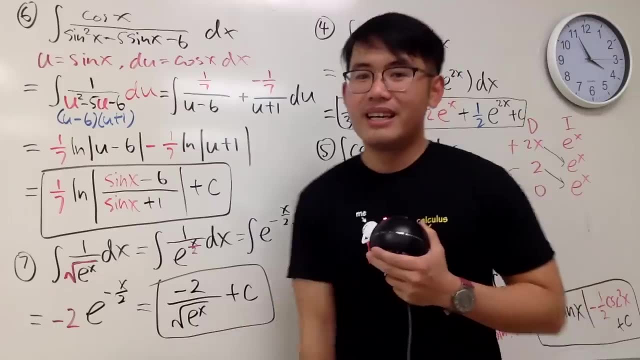 in the denominator and we can write that back as the square root. So it's negative 2 over square root of e to the x, like that, and then put a plus c like this. right, Cool, Now the flavor. 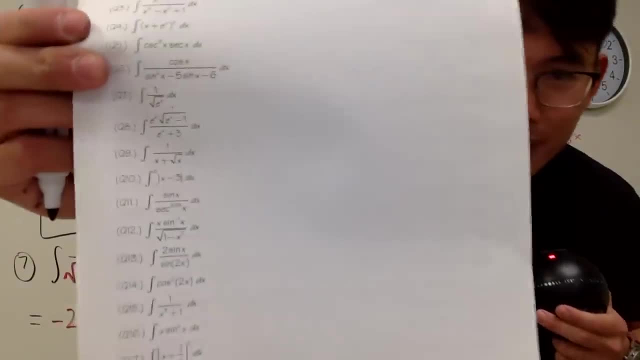 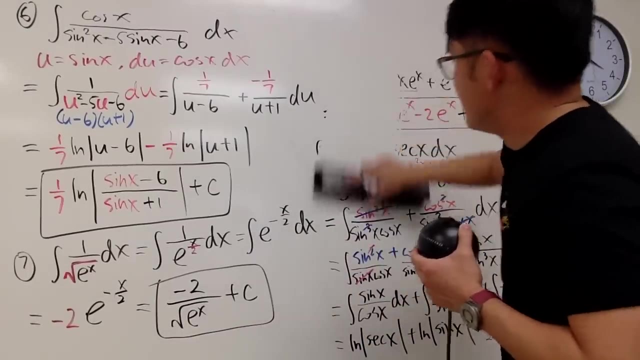 is slightly different, Number 8, we have a much bigger one. So of course we will have to erase the board now And let me know if you guys like this clock and take a guess: how did I put a clock on the white? 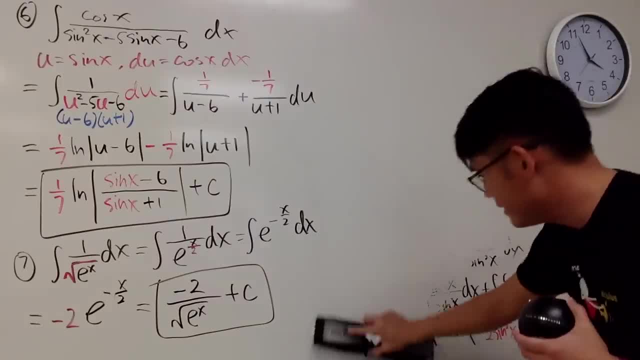 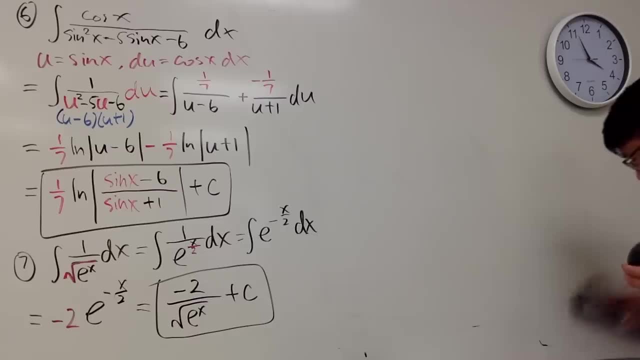 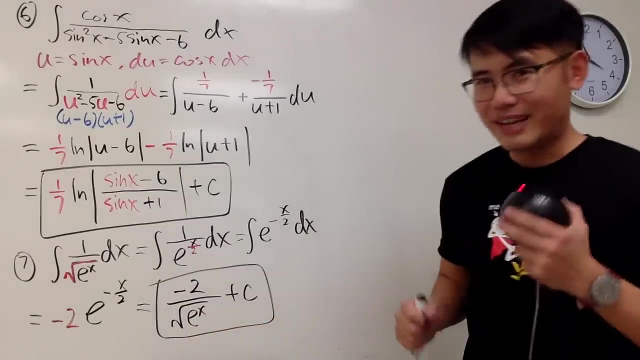 board. right, Let me see. And I feel like I have to conserve energy because, as I said, I have about 93 more to go, so I cannot be too excited for this right here. just that I run my results. I have to make sure I pace myself well, But anyway. 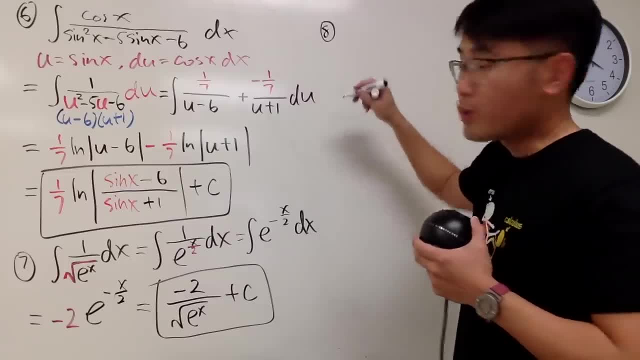 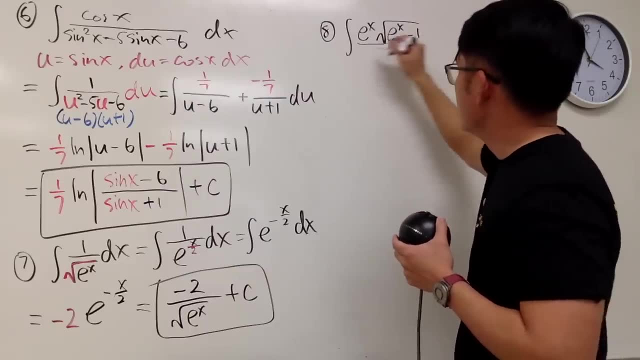 number 8, here we go, number 8,, number 8,, number 8, we have to integrate e to the x times the square root of e to the x minus 1, over e to the x plus 3.. Oh my god, who comes? 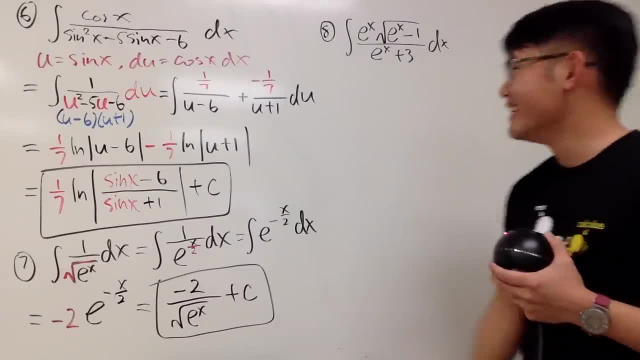 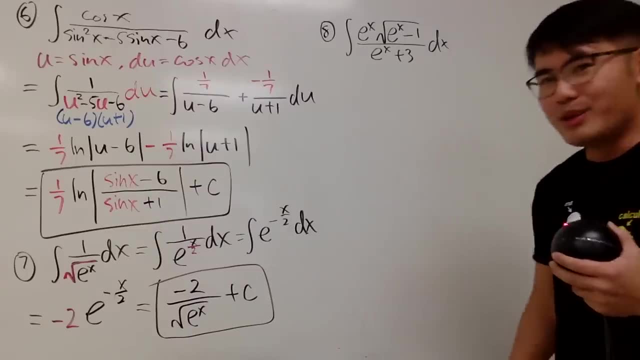 up with these integrals- And yes, that person is me. okay, I handpicked all these integrals right here for you guys, But let's think about how to integrate this. Well, why don't we just do u sub and especially? 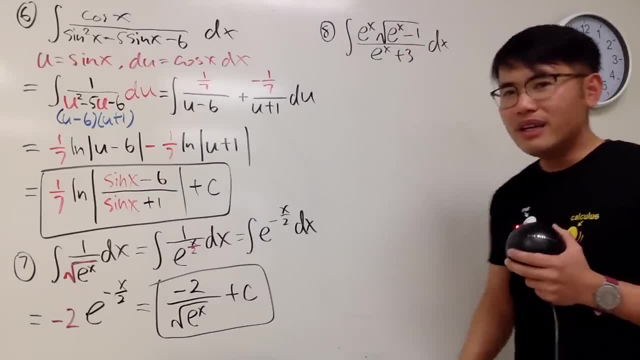 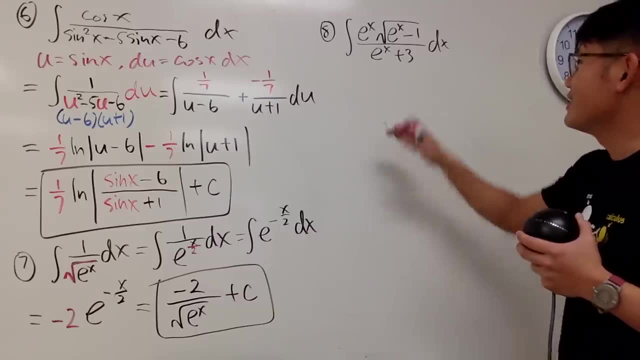 I have the square root with e to the x minus 1, and let's just make u equal to that and let's see what happens, Because at the moment we cannot do partial fractions, you cannot do integration. I don't think you want to do integration by parts for this. 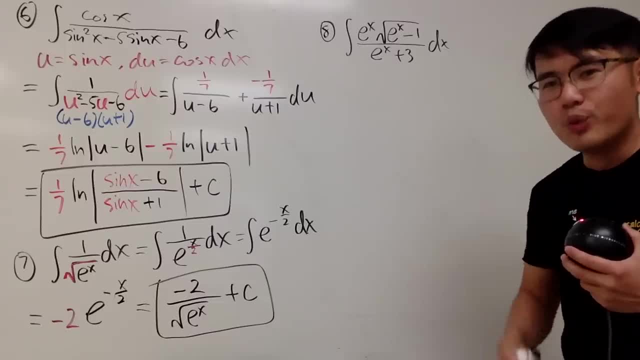 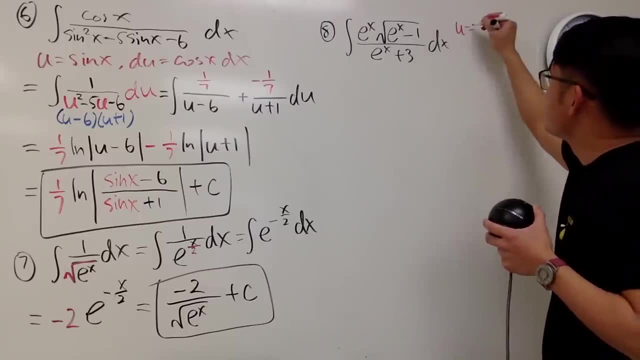 Let's just do u sub. Maybe the life is better in the? u world than the x world, right? So let's take a look at the? u world instead. Let u equal to the square root of e, to the x minus 1,. 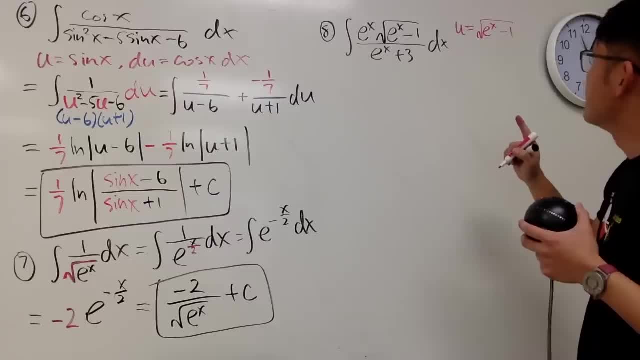 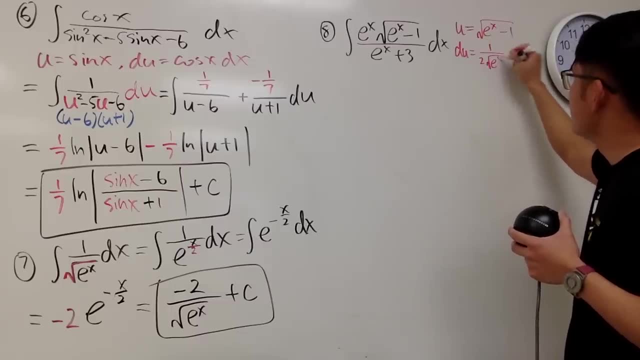 and I want to get the dx, and perhaps let's just go ahead and differentiate. du is going to give us 1 over 2, square root of e to the x minus 1, and of course, don't forget the Chandu. you multiply by the derivative of this. 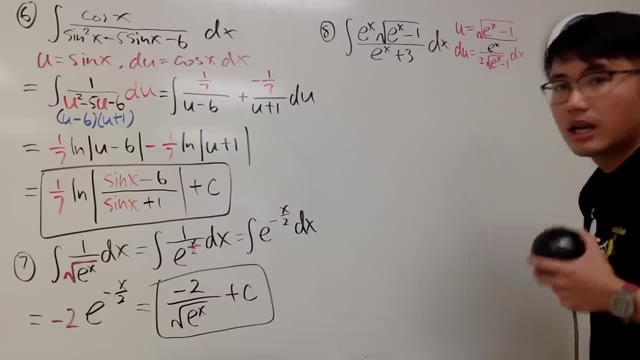 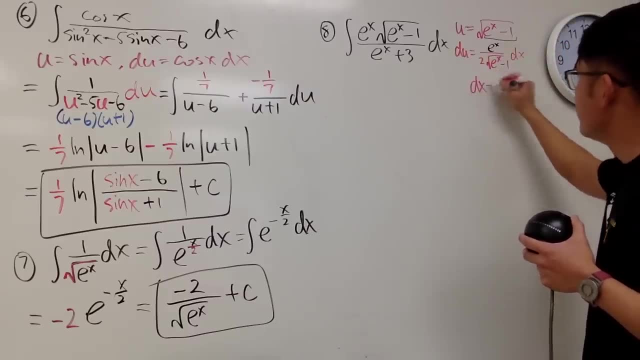 which is e to the x, and then you have the dx right here, And I will of course get the dx by itself by multiplying the reciprocals on both sides. so I get dx being this on the top over e to the x. 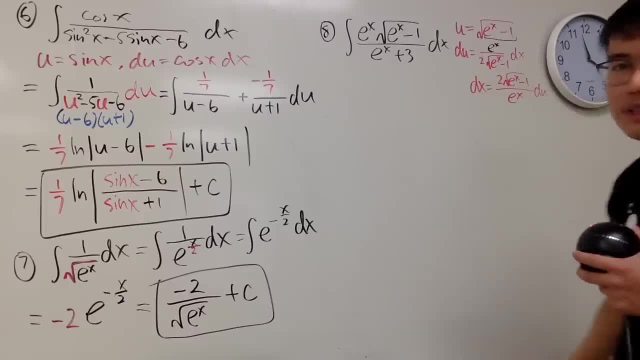 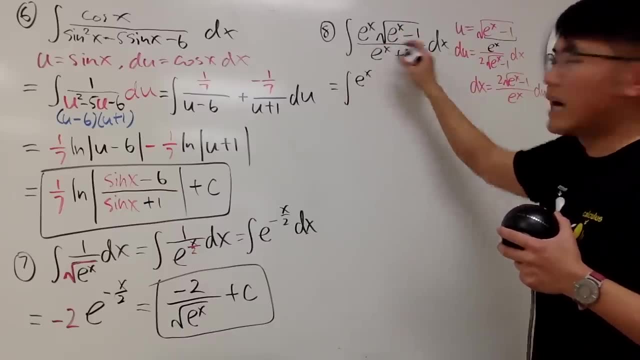 and let me just keep this as how it is and we'll see what happens. So here we go. This right here will give us integral e to the x is still e to the x. this guy is the u, so I'll put that down as the u. 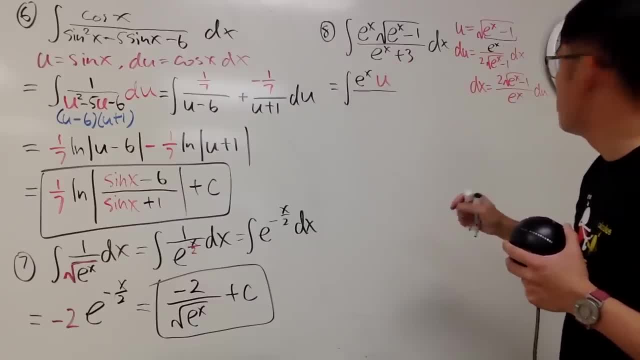 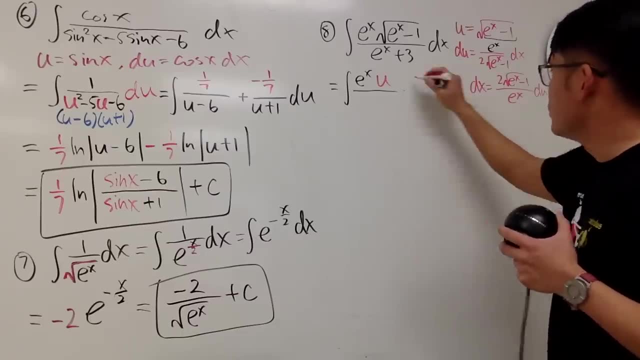 over. I have e to the x plus 3.. Hmm, I don't know that too well, But I know dx is this, so I can write that down right now, which is 2, and notice the square root of e to the x minus 1 right here. 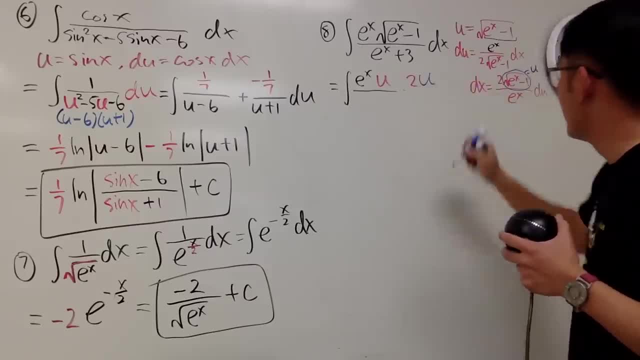 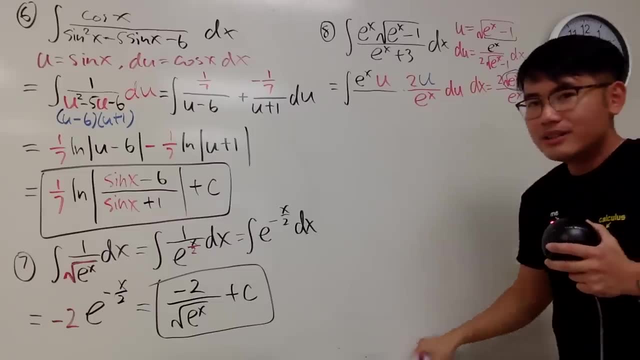 This is just the u, so I can put down the u right here as well, and we have this over e to the x and then we have the du right here. So far, so good, and you see that the e to the x and e to the x will be cancelled. that's good. 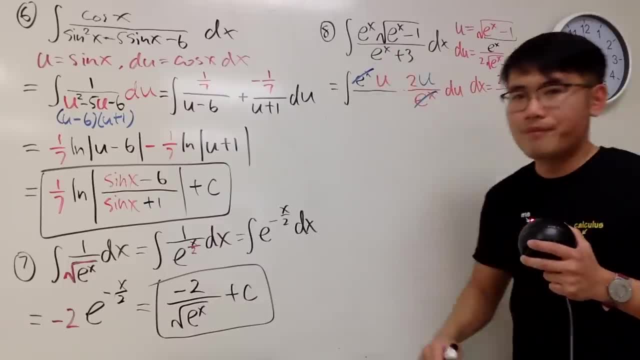 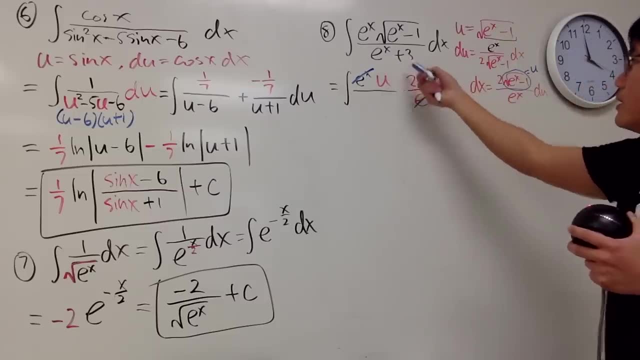 But we also have to figure out what's e to the x plus 3, though. Well, we have to look back to this then, because we need to get this expression in terms of u right. So let's see, Let's see if my hair is okay, okay. 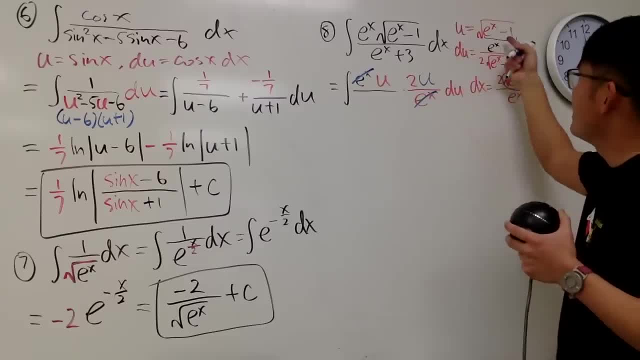 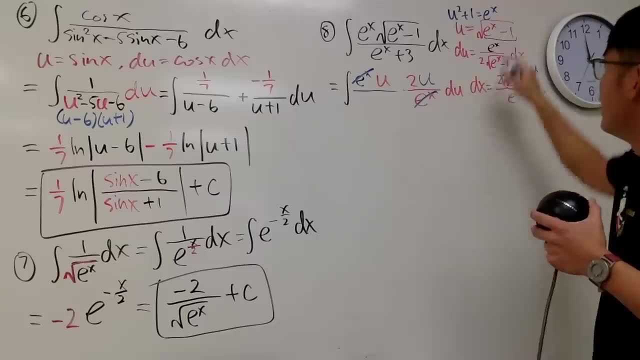 So I will see, I will square both sides right here and then I will add one on both sides. so in another word: u squared plus 1 will give us e to the x. okay, Well, e to the x is just u squared plus 1,. 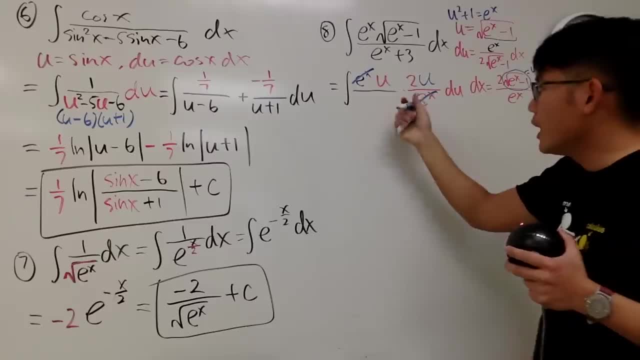 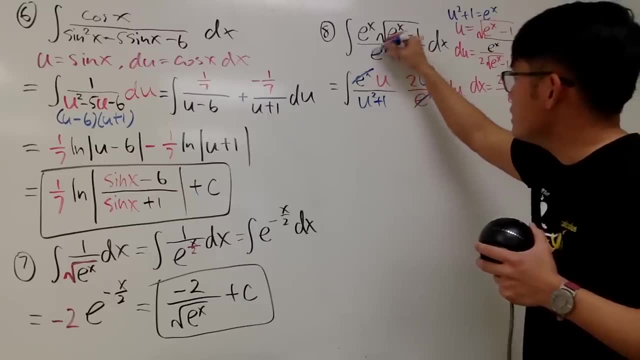 so right here I have this, and then plus 3, so all in all we end up with u squared plus 4.. But let me just write it down right here for you guys: plus 1 for the e to the x. 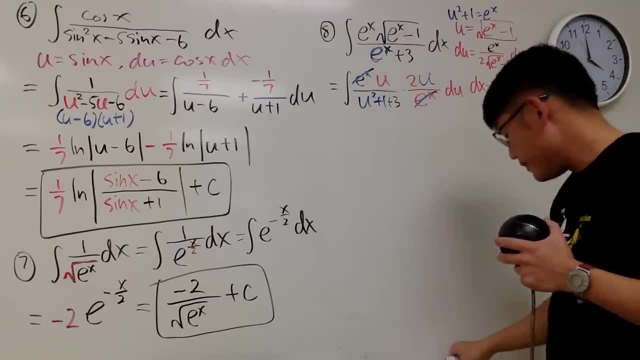 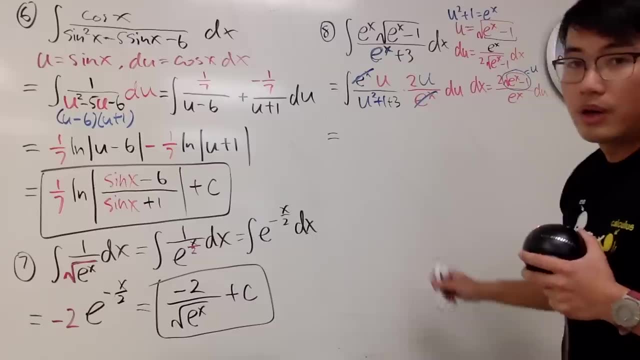 and then plus 3 after that, Right. So let's try to show as much work as possible, but it depends on the situation. All right Now. as you can see on the top, this times that is just u squared. 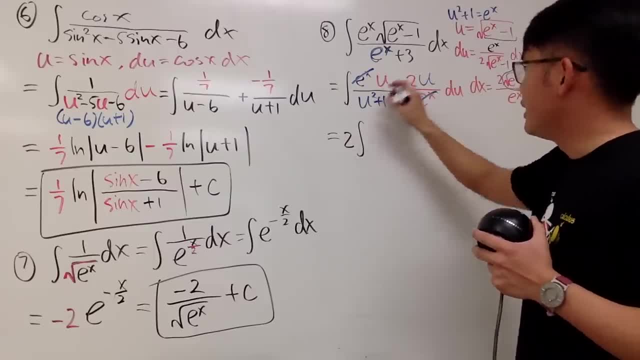 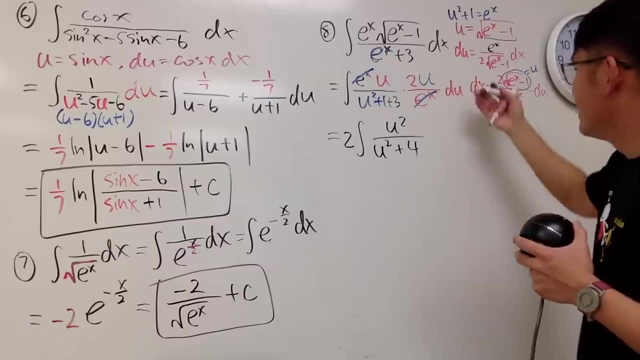 but we have a 2, so we can take that outside. And then u times u is of course u squared, and here we have u squared plus 4 instead, right, So that's so far what we have, but here's the trouble. 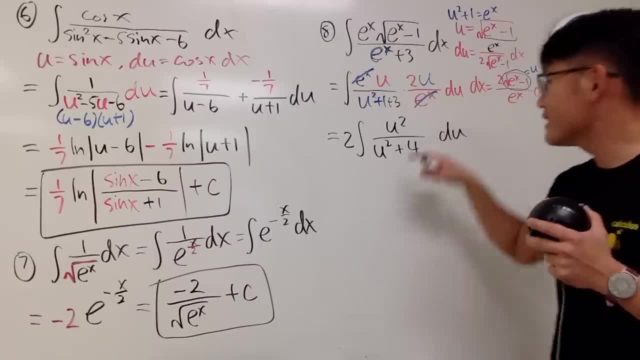 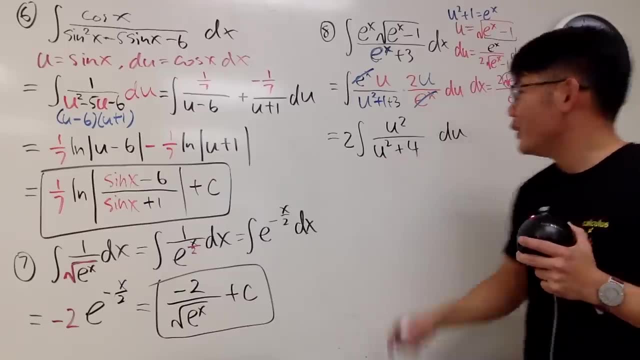 How can we interpret this? And you have two choices. One, notice that the degree on the top is 2, and the degree on the bottom is also 2, so you can do long division. But you can also think about: wouldn't it be nice if the top is also u squared plus 4?? 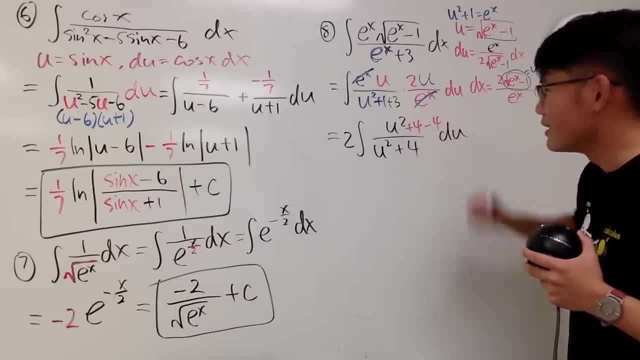 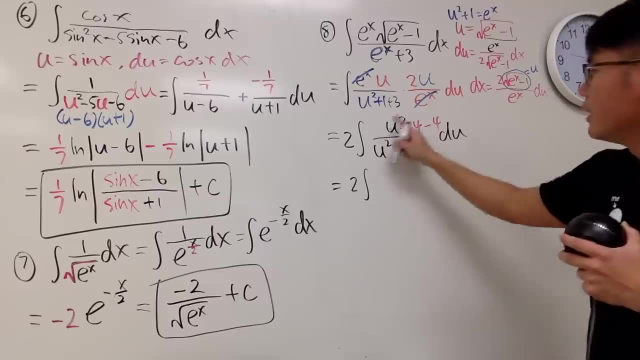 That would be so nice, isn't it? In the meantime, don't forget to minus 4 to make things happen. So, as you can see, this right here is going to be 2 times the integral. this is just going to be 1,. 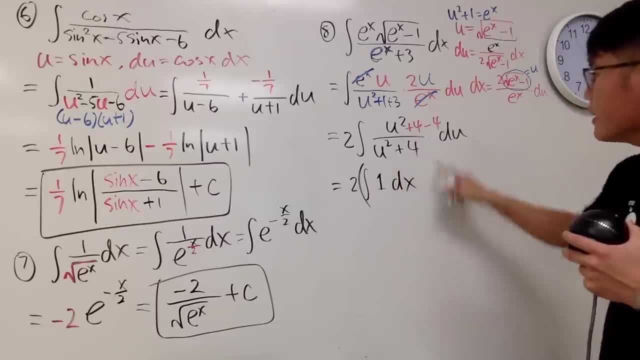 and then this right here. let me just close that, okay. And then we have this part, which is: we subtract the integral with 4, let me just put down the 4 in the front, this 4, okay, And then it would be 1 over u squared plus. 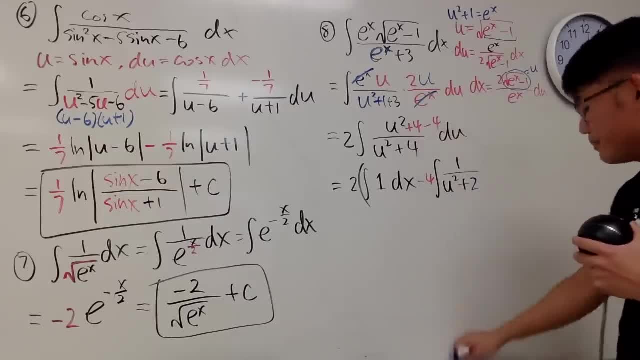 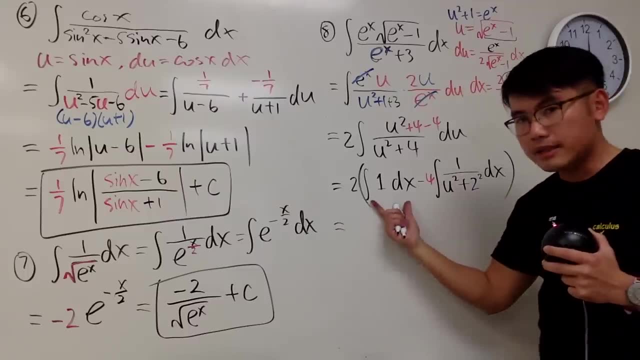 this 4 is the same as 2 squared. We need that because we need to use the r-tension formula, right? So now this is going to give me x. So let's see two parentheses. this is x. 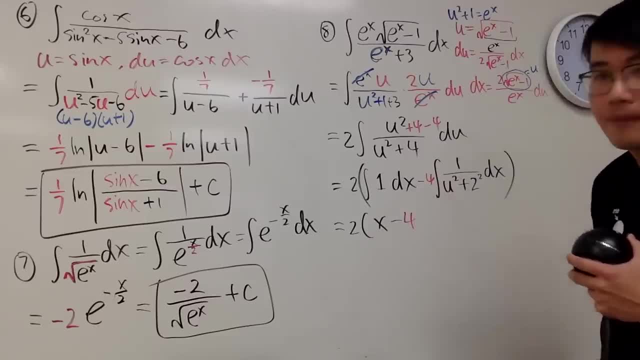 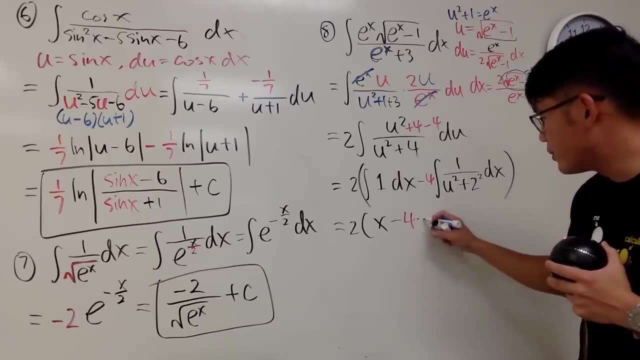 And then minus the 4 from here: Inverse tangent formula for this integral right, And the a-value is 2.. So don't forget: you divide it by 2, so you multiply by 1, half, right here. 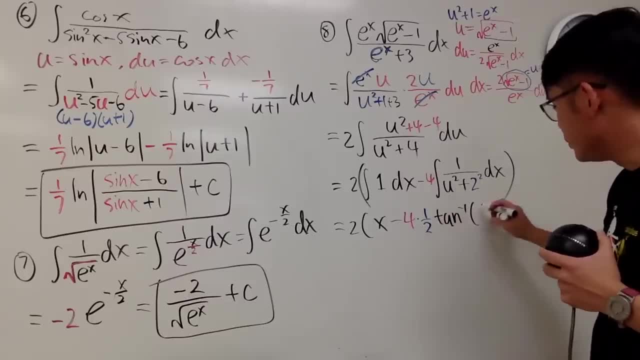 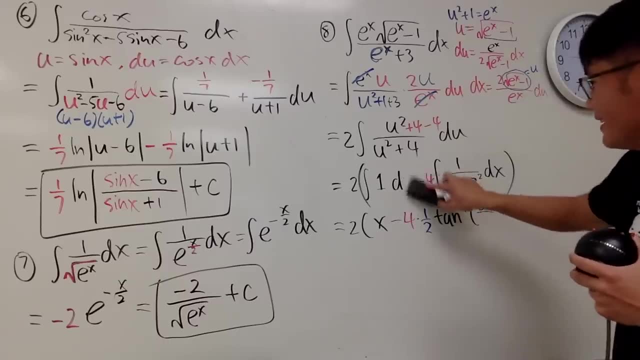 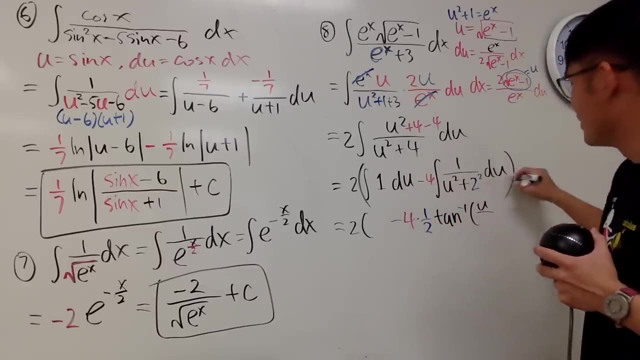 and then you have the inverse tangent and the input is u over 2, like this: No, sorry, this right here should be the u. This is really bad, I'm sorry. This right here should be u. this right here should be the u. 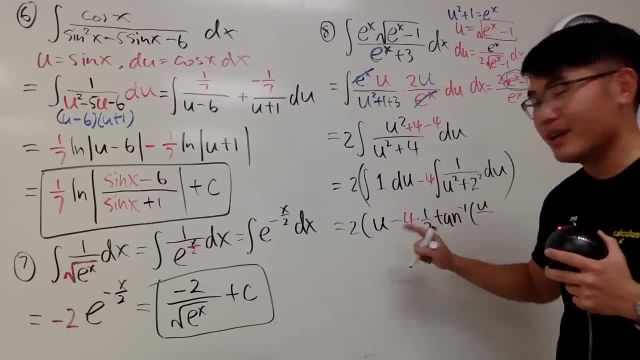 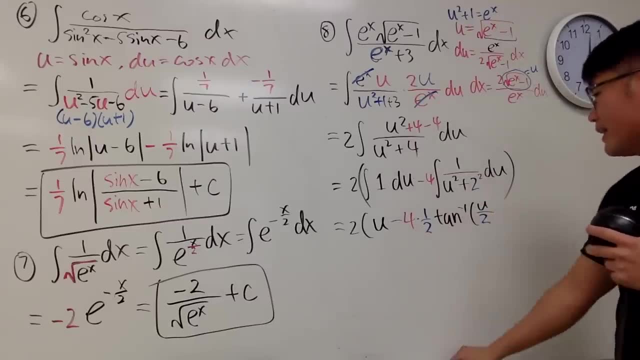 So when you integrate 1 in the u-world, it should have been a u. okay, Anyway, right here we have u over 2, like that. By the way, this is a really common mistake, and sometimes I make it myself too. 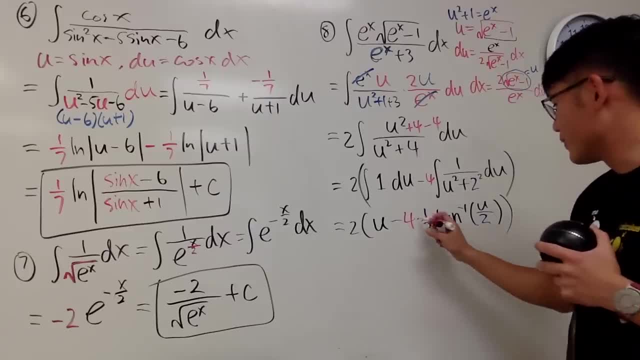 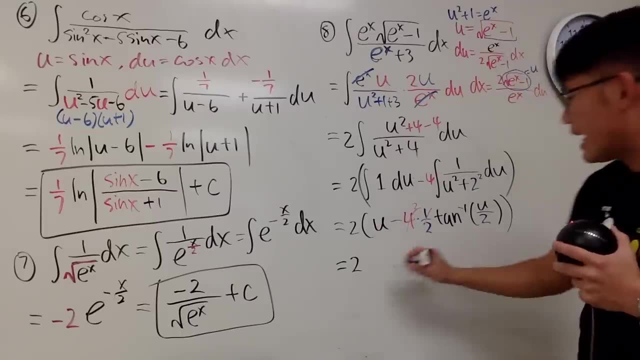 so just be really careful with it. So now I will just do the rest for you guys. This right here is just going to be 2 now And of course you distribute the 2, and the? u. you look back, it's this guy. 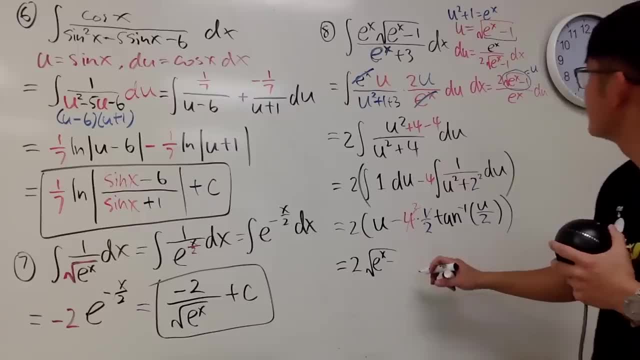 so it's square root of e to the x minus 1.. And then we have the 2 times 2, which is 4, so minus 4.. Inverse tangent of u is the square root of e to the x minus 1 over 2, like this: 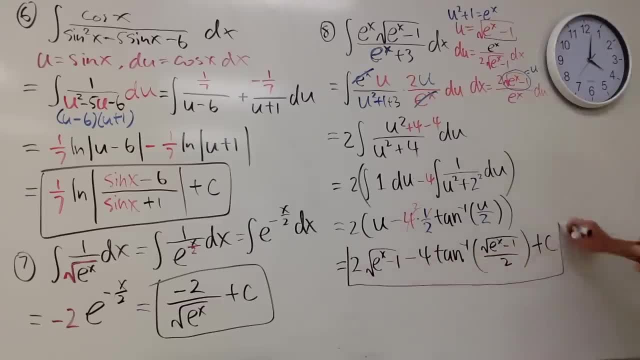 And we are done, So we can put plus z This right here, is it? Let me just triple check. I think this is good. Let me see, let me see, let me see. Yeah, I think this is good. All right, so let's see. 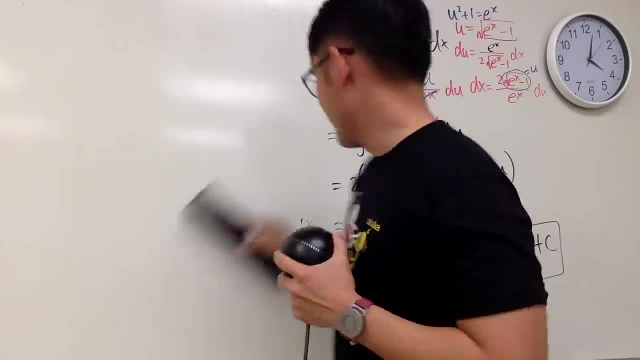 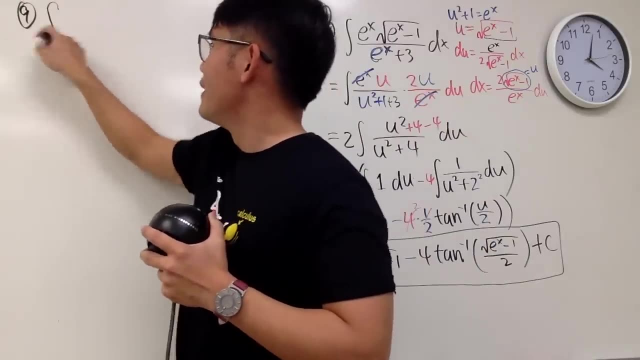 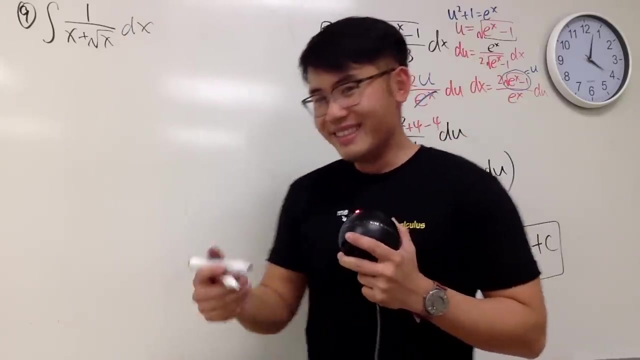 So that was number 8. And we are going to continue. stay strong. Number 9. Here we have the integral of 1 over x plus the square root of x- dx. So do not have the natural addition seriously. Do not just say this is equal to the natural law of absolute value of x plus the square root of x. 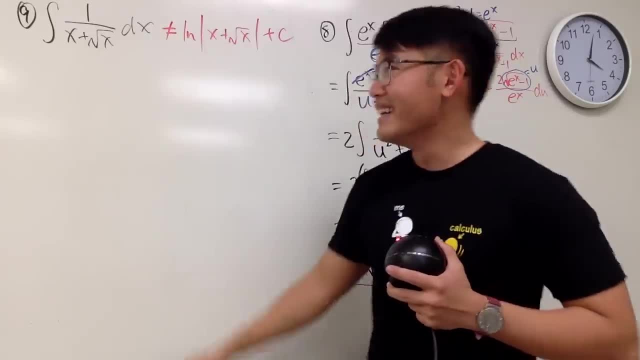 Yes, if you put on plus z, but no, this is still wrong. Don't do that. okay, Don't just say you have 1 over, you have x to the first power. no, Because you have the square root of x right here as well. 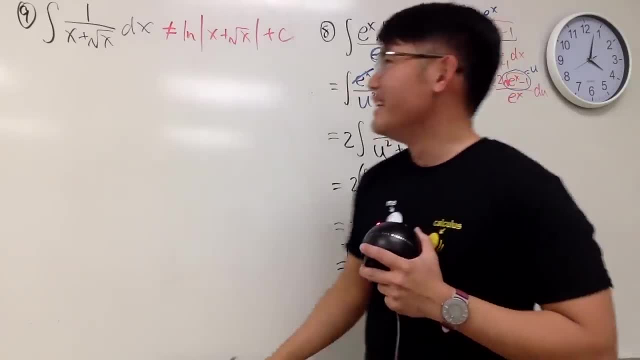 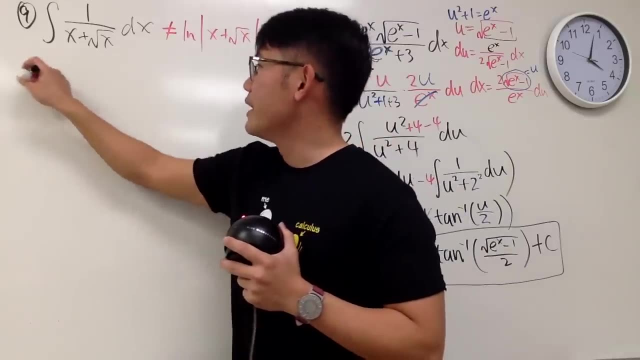 And you might be wondering who put the square root of x, and that person is me. okay, Anyway, this is how you do it Right. here we can technically factor out the square root of x, So when we do that, we get the integral of 1 over. 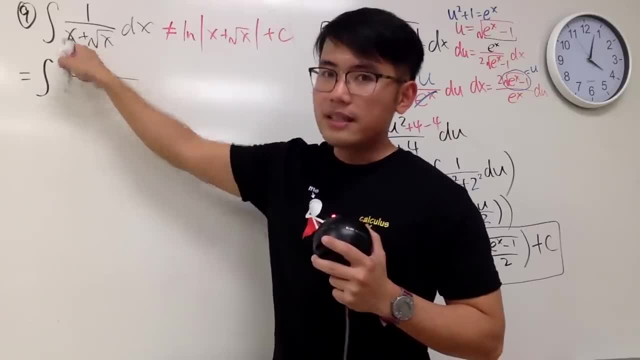 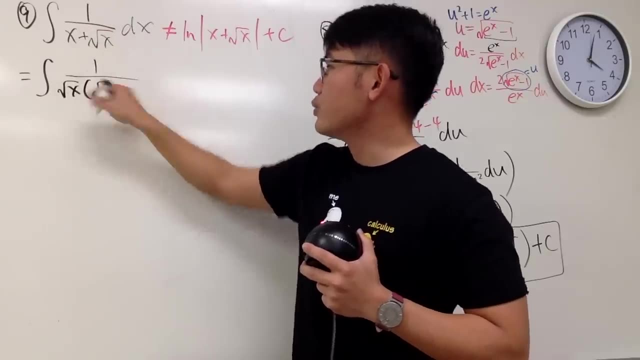 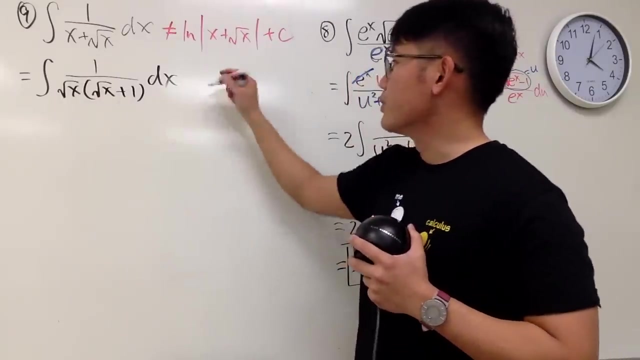 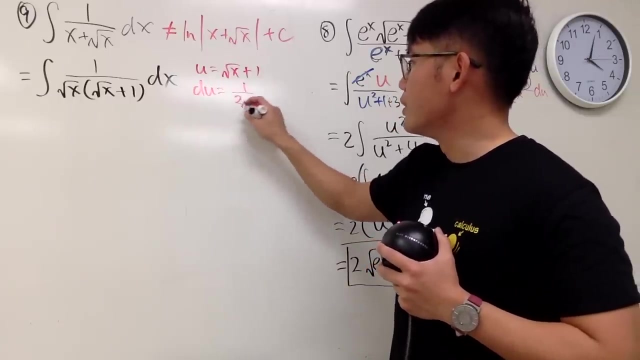 we'll factor out the square root of x, Because x is the same as square root of x times square root of x. so when I factor this out, I will have square root of x and this will be 2 over 5 over 10 to the power of x plus the square root of x. 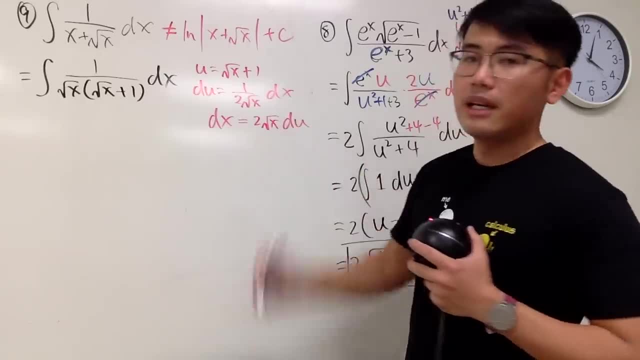 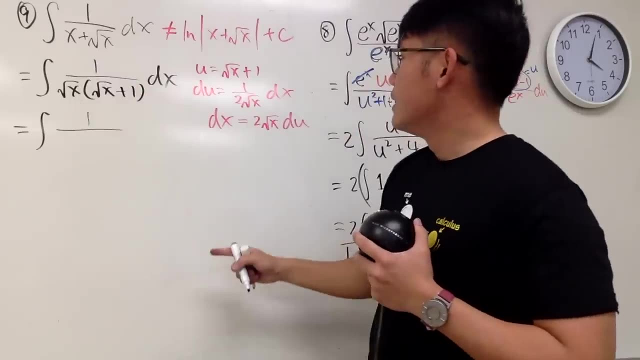 multiply this on both sides. so we have that and you will see. if you take this integral to the u-world, you get the integral 1 over square root of x. well, don't worry, somebody is going to get cancelled out, so we'll just write it down right here: square root of x. 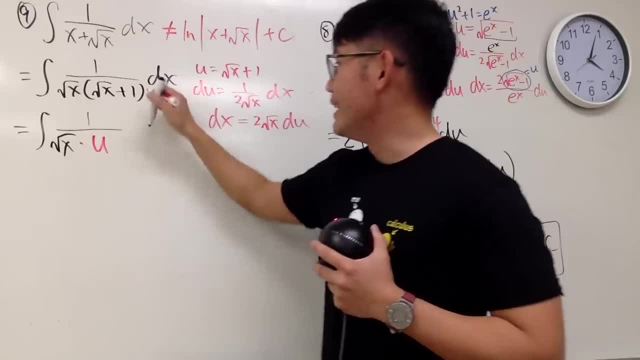 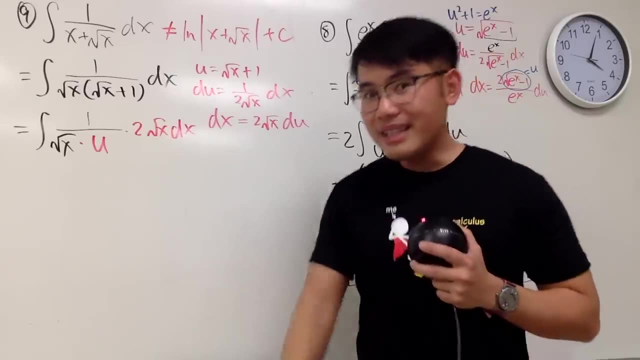 and this guy is the u. so you multiply by u and dx is this guy and you see you have 2 square root of x, like that, and then the du and, as I told you, we have somebody. you. 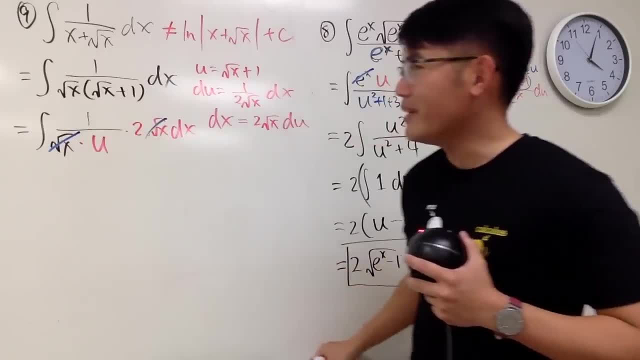 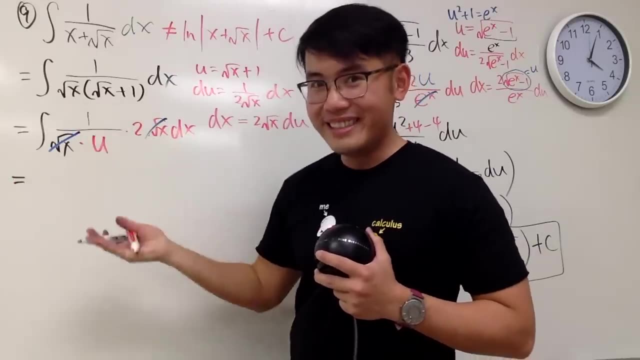 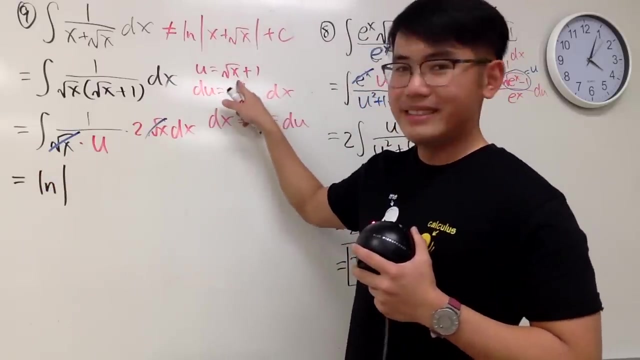 know being cancelled out now, which is the square root of x, right here and right there. and here we have the? u part. this right here is actually right 1 over u. this is the natural part. we get natural log, absolute value. well, what's u? u is this, and I will. 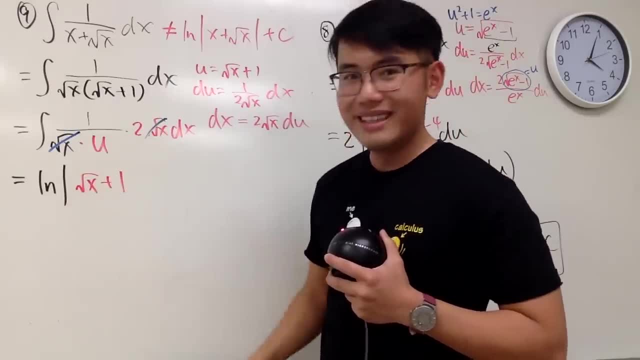 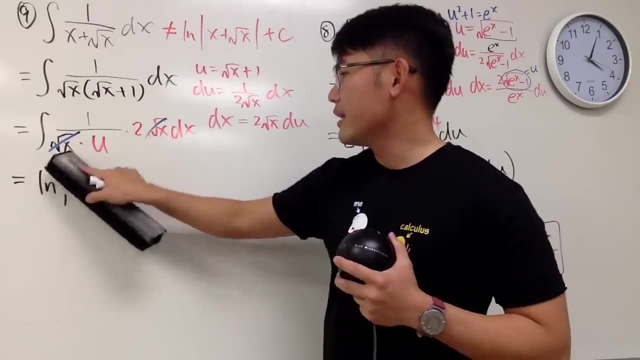 just write that down right here for you guys, which is the square root of x plus 1, this is legit, okay, and notice: 1 is positive and square root of x is always positive. technically, I can just write this: 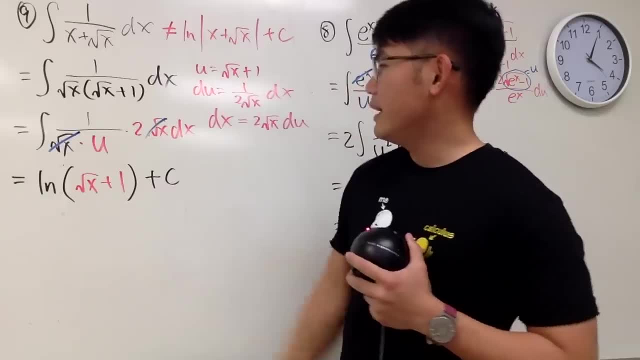 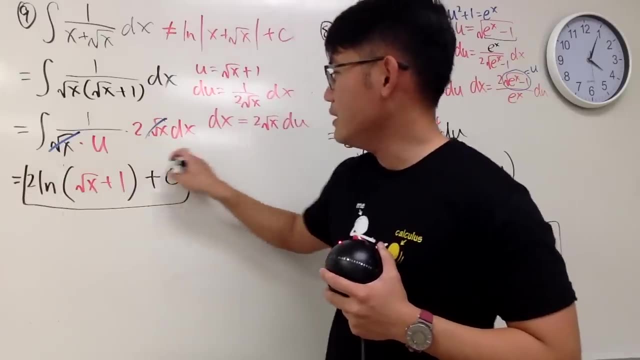 Write it down as parentheses. I don't need the absolute value and that's it, and of course, don't forget the 2 right here as well, so let me just put it down right here. so here is the answer: 2 in the front and all that right. so you have to do this one legitimately. 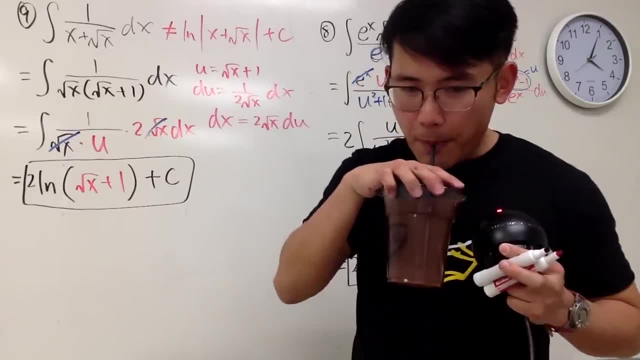 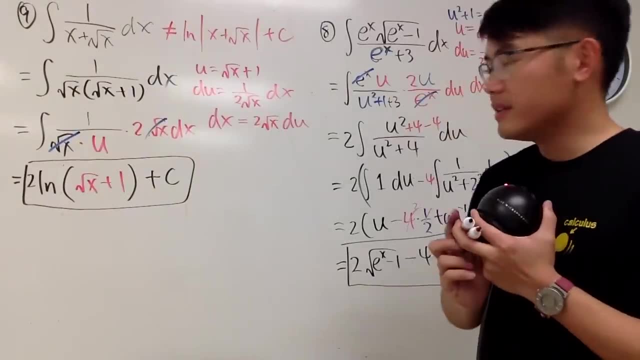 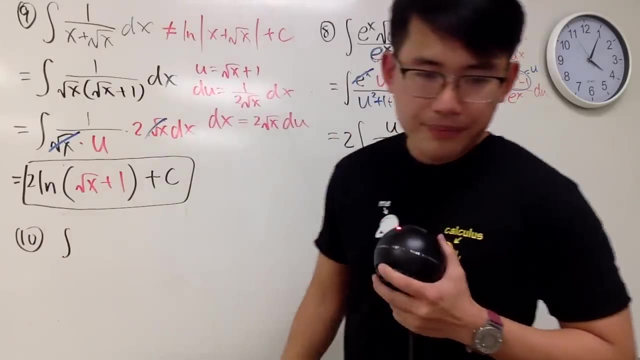 okay, alright, so let's see next one. and, by the way, for every 10 integrals we'll be doing a definite integral. So here is the first definite integral that we are doing: the integral of negative 1 to. 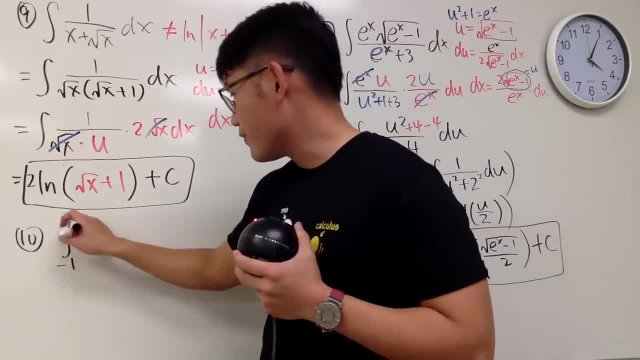 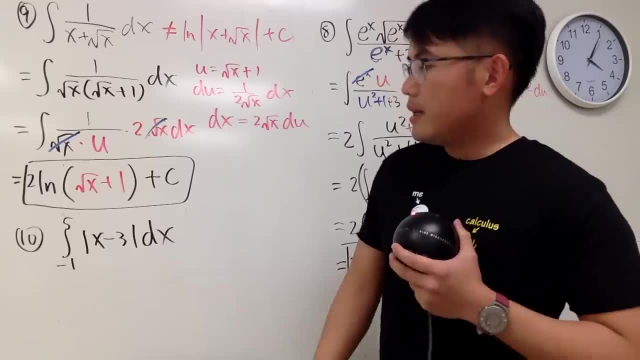 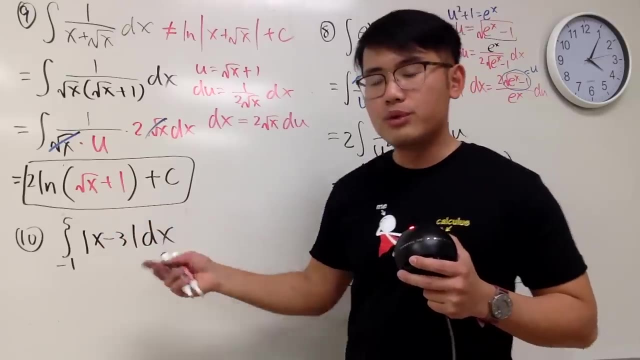 the not negative 1 to the 5th power, from negative 1 to the 5th absolute value of x minus 3, dx. huh, first of all, you can do this by change the absolute value of x minus 3 into a piecewise function and then just deal with that. that's fine. or you can just: 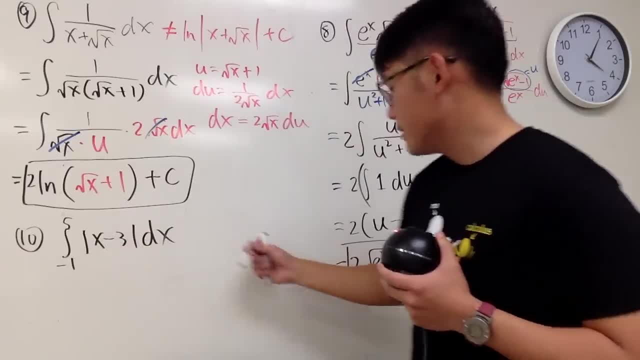 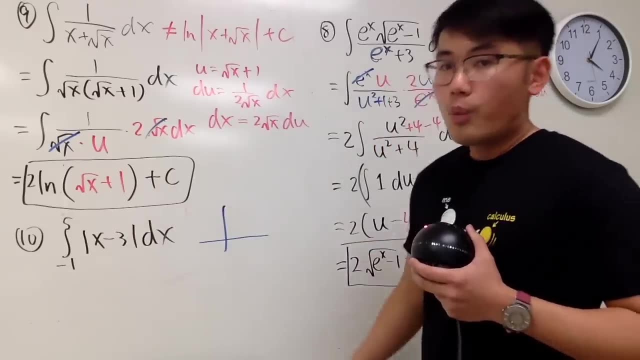 do this geometrically. Let me show you if you graph this and let me put this down in blue. let's take a look at the graph of the absolute value of x minus 3,. well, you pretty much just shift the absolute. 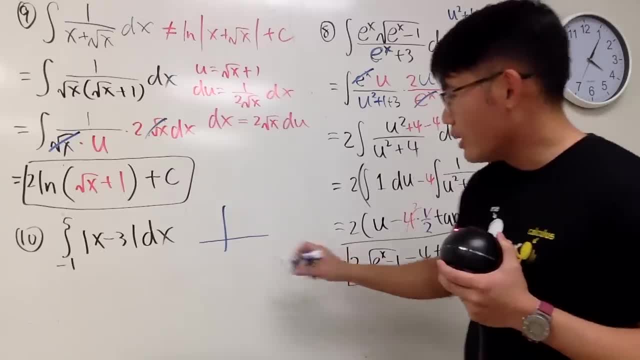 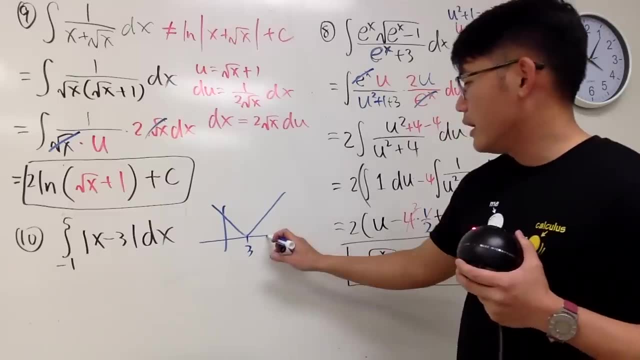 value of x 3 times to the right. so I'll just put down the 3 right here, and then it's going to look like a phi, right? so it's going to look like this, right, and, of course, you. 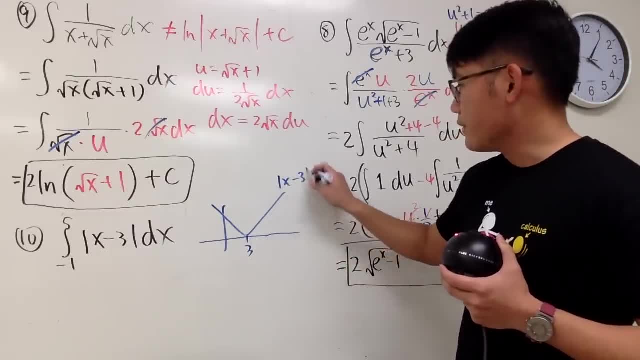 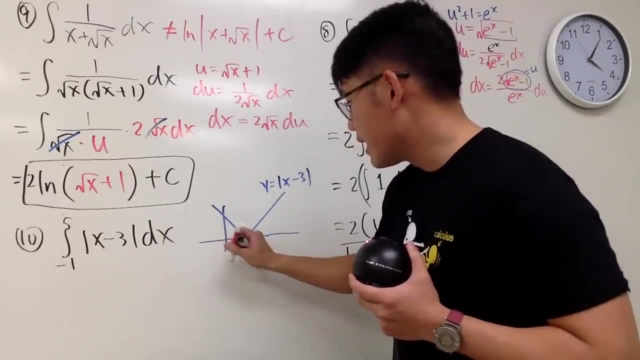 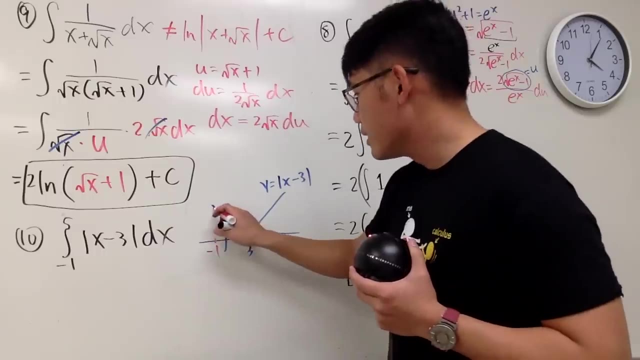 are going to have some triangles being involved, so of course you have to know your area of the triangles. Here's the deal: when x is negative 1, let's put it down here- put negative 1 here. negative 1 minus 3 is negative 4, take the absolute value, you get the y value being 4, so as 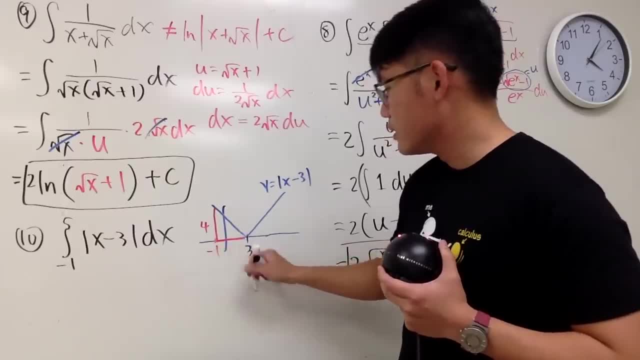 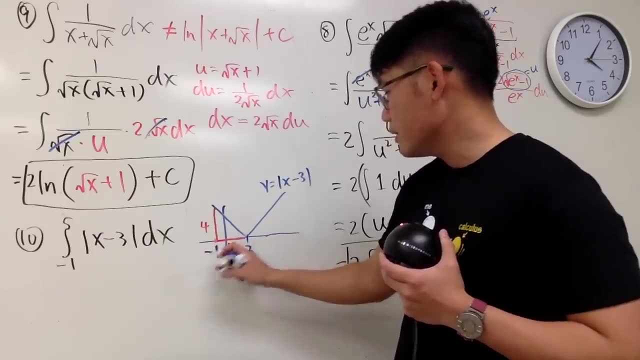 you see, this is 4, and notice what's this? from negative 1 to 3,, this is also 4, right? so negative 1 to 3,, the distance is 4, and then, when you have 5,, let's say it's right. 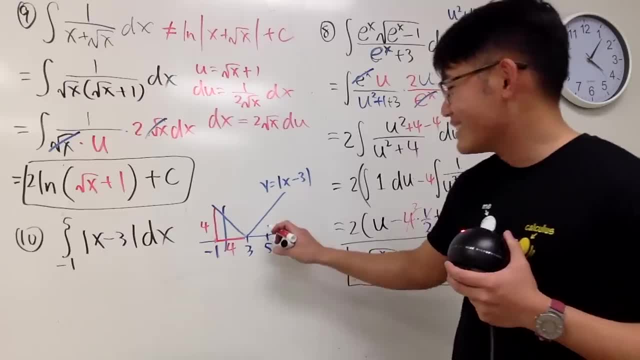 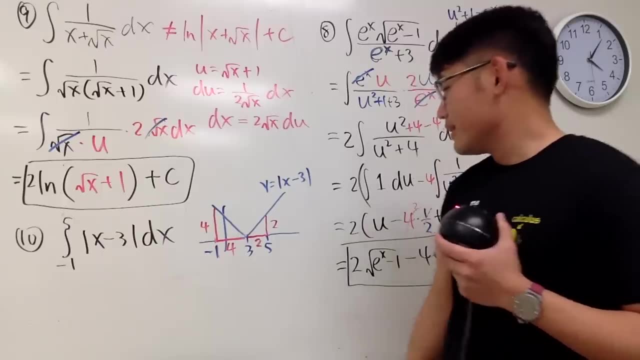 here. putting 5 in here, 5 minus 3 is 2, so this vertical distance is 2, and what's this right? here it's also 2, right. so the deal is that. okay, what's the area of this triangle? 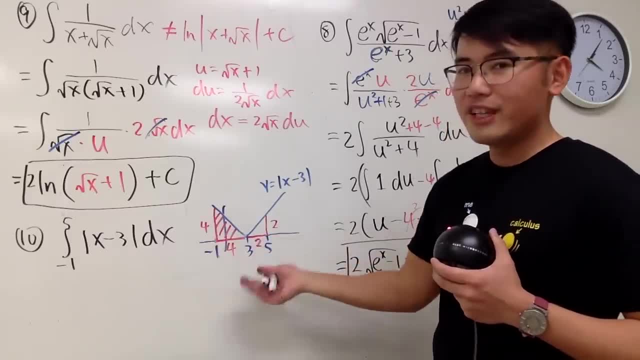 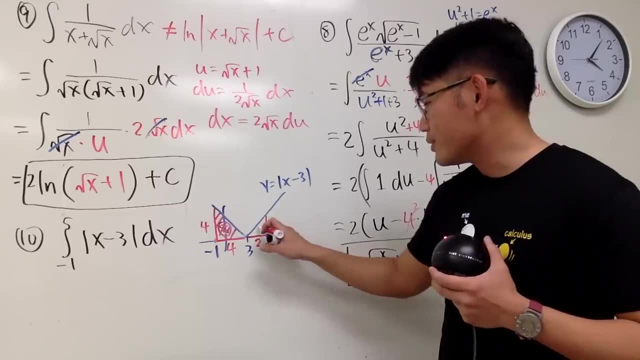 One half base times height, this is 16, divided by 2,, which is 8,. so this right here is 8, right, and then 2 times 2, divided by 2, which is just 2,. so that's the deal. so this right. 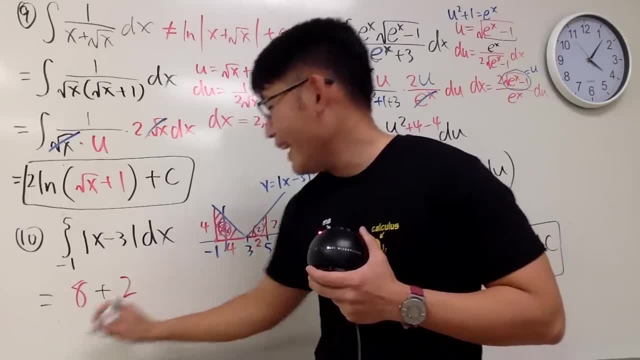 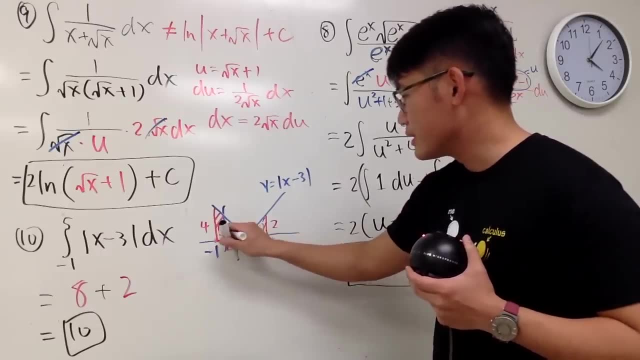 here is just 2.. Just 8 plus 2, and you are done. this is 10, right again. the area of this triangle is just 8, right. so that's it all, right now. continue, continue, continue, we can. 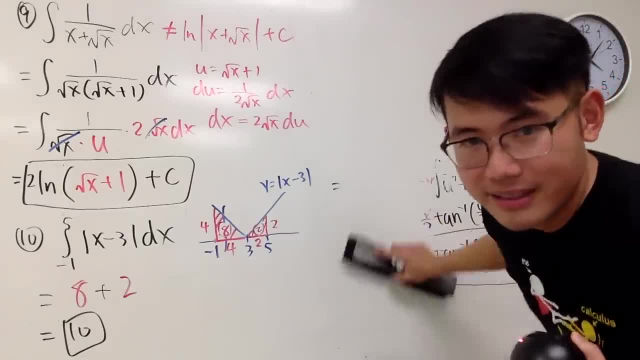 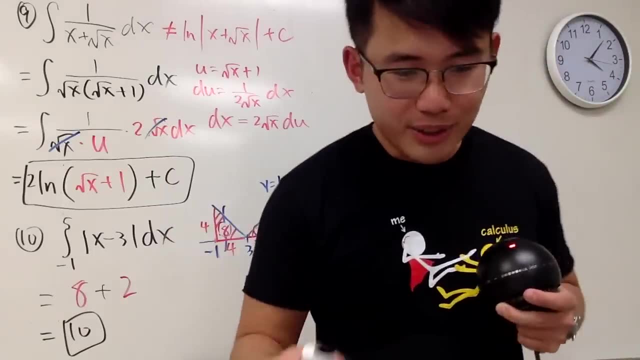 do this. we can do this, we can do this. it's only been 37 minutes, it's okay. I just have to do this 10 more times. 10 times 10 is 100, so we can do this, we can do this, we can. 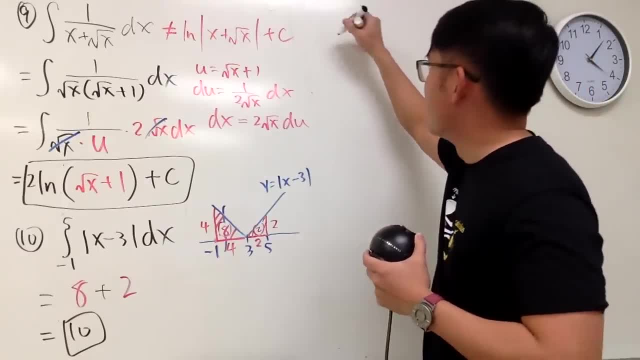 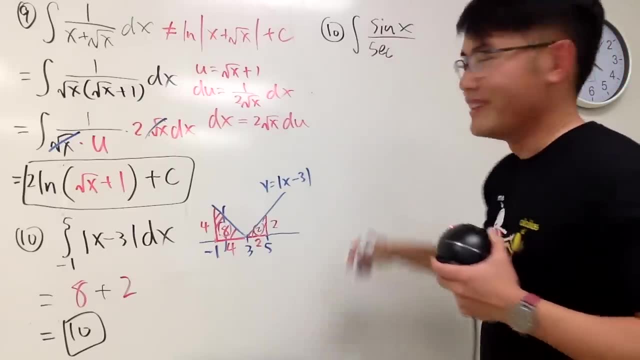 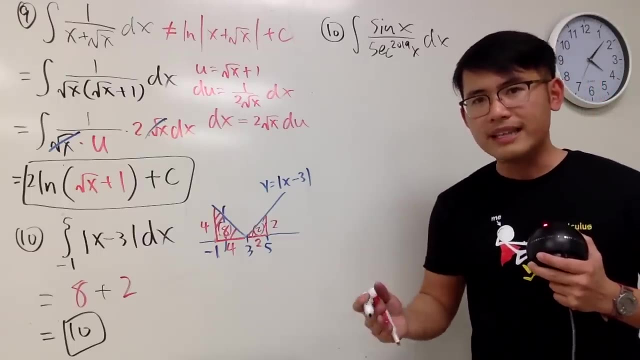 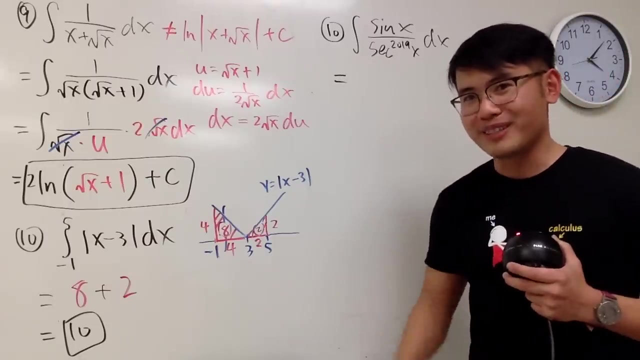 do this Number 10, right here? and have I told you guys talking is actually harder than running right? so, yeah, anyway, integrating sine x over secant to the 2019th power of x. well, well, of course, we don't like secant to be on the bottom, we like secant to be on the. 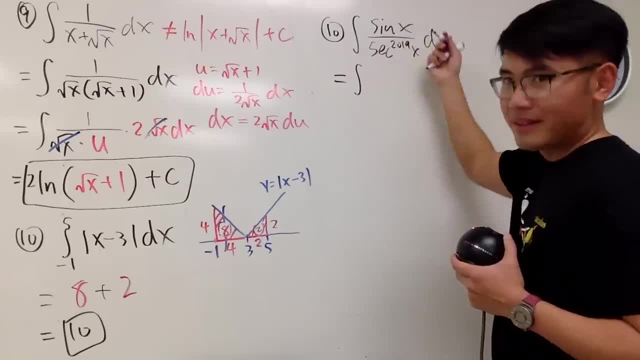 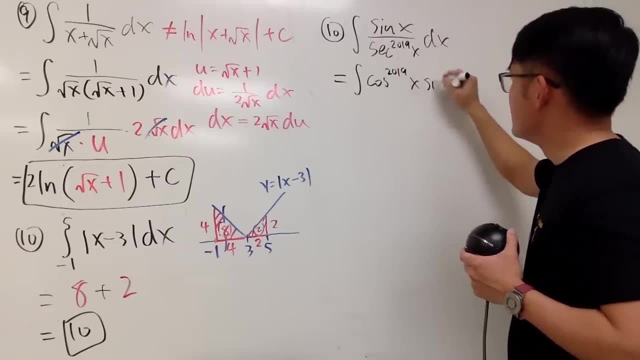 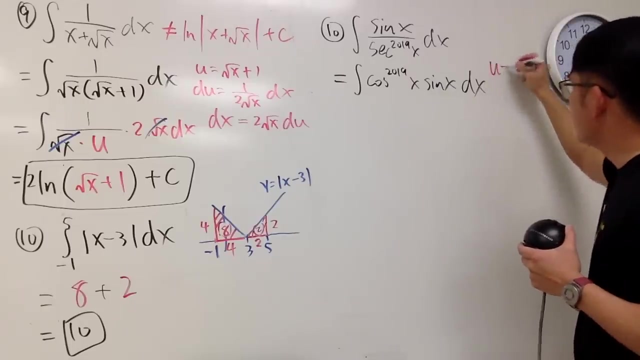 top. so we'll look at this as this: being the top will give us cosine. so look at this as So cosine to the 2019th power of x times sine x, like this dx. and with that being done, this is actually pretty easy. we can take a u sub, let u equal to cosine x and 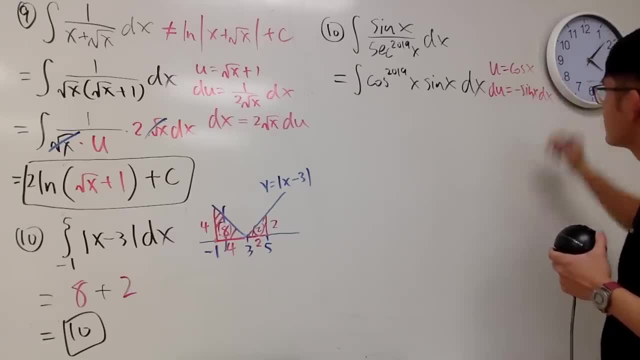 you see, du will be negative sine x, dx, so you are going to have some negative signs along the way. all right, so dx is the du over negative sine x. if you want to see the cancellation, this will be it. So you will see, this is the integral. 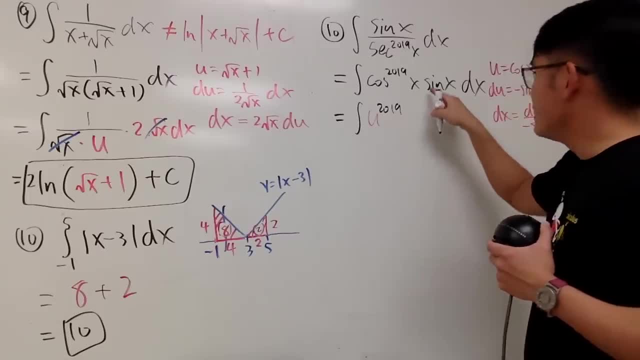 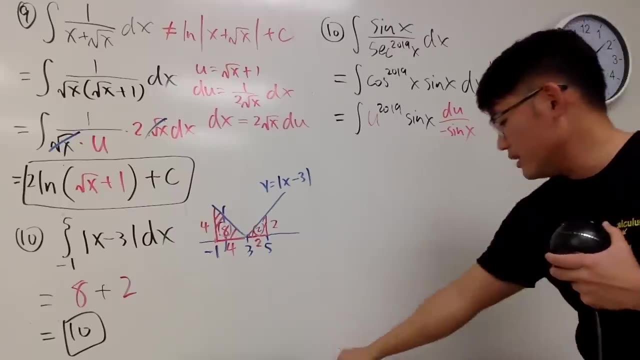 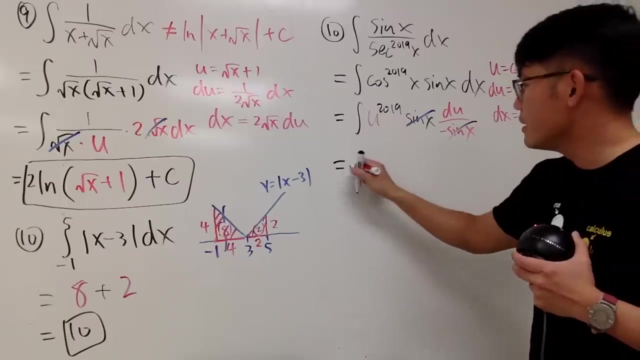 So u to the 2019th power and let's write down the sine x, if you would like, and then dx is du over negative sine x. this is how you can show the cancellation, if you would like. right, so you are going to put a negative on the outside and then let's integrate u. 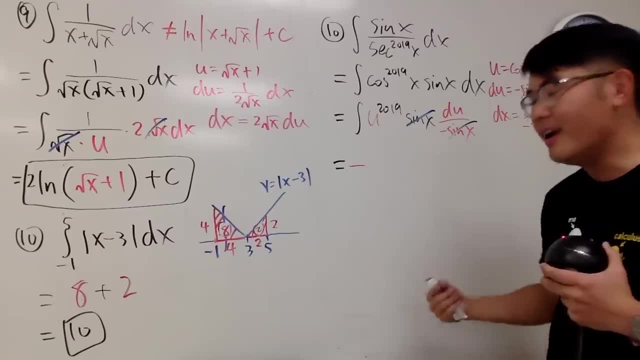 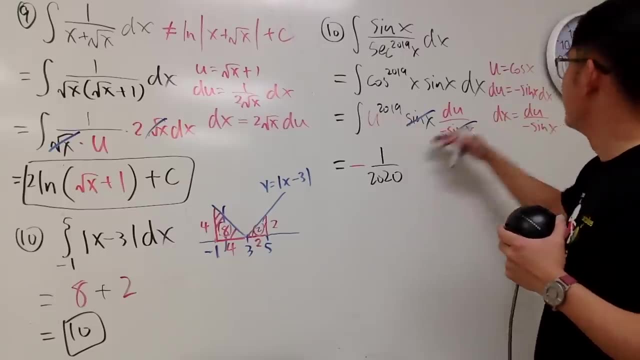 to the 2019,. you add 1 to it, which is next year, and you divide it by next year, which is 1 over 2020.. And then u is cosine, so you put that back, so you have cosine to the 2020th power and 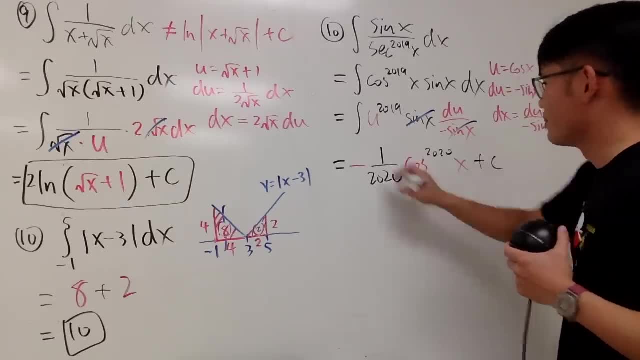 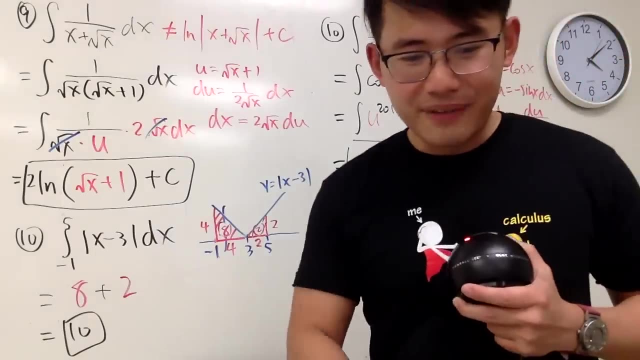 you have the x right here. That's it right. So you are done. put plus c. this is it. Oh, I wish all the integrals are this easy. but if it's that easy, then it's not fun. 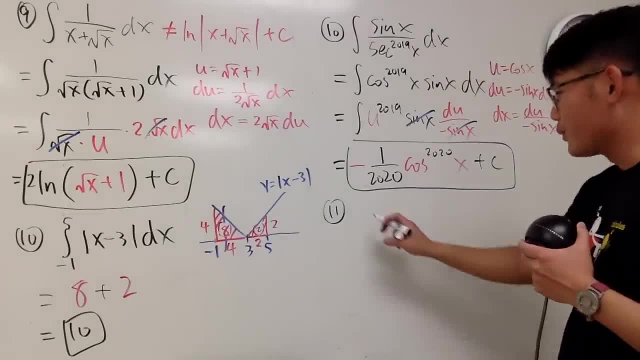 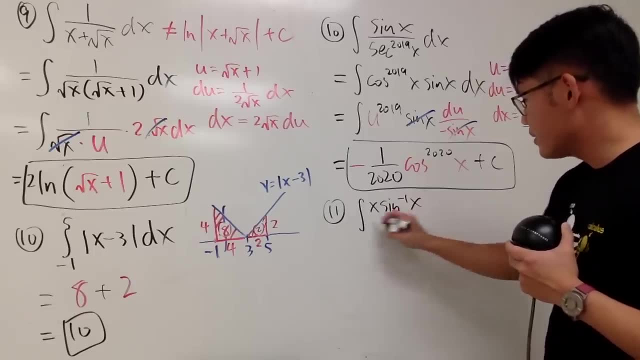 so no, All right. next one: all right. so you have a pretty big one. let's see if I can fit in here The integral of x times inverse of sine x over dx. Oh, that's it right, That's it. 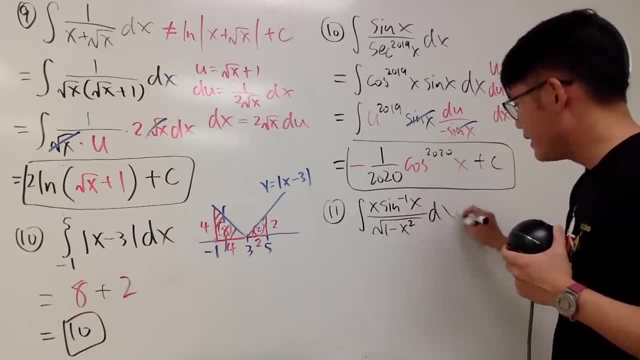 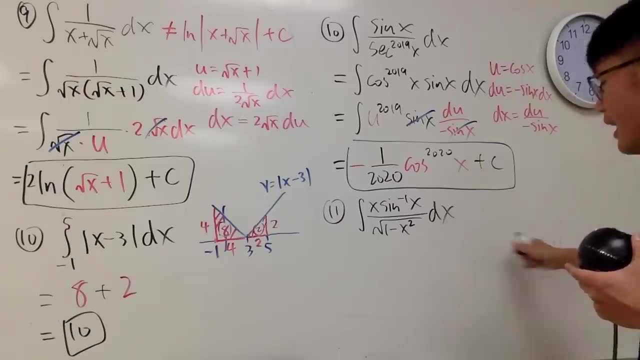 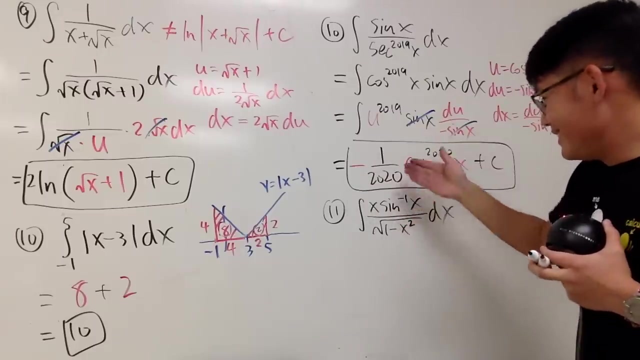 over the square root of 1 minus x squared dx. Oh my god, I don't wish Who put that x there, man? Because if I don't have the x, because the derivative of the inverse sine x is 1 over the square root of 1 minus x squared right. 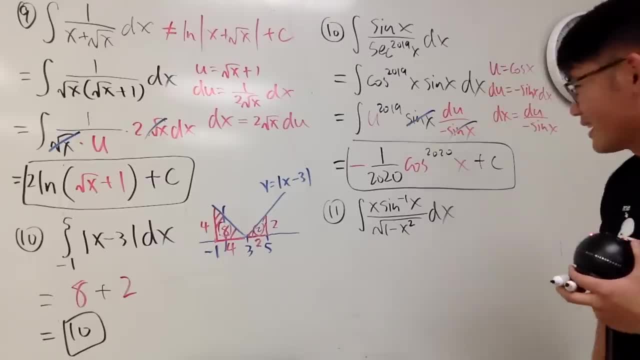 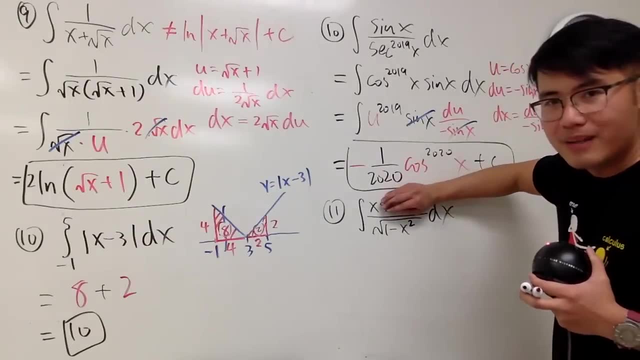 I can just do USAP for that if I don't have the x. Oh my god, Who ever put that x? Horrible person, man. But anyway, check this out. In fact, we can integrate this guy by doing a simple USAP. 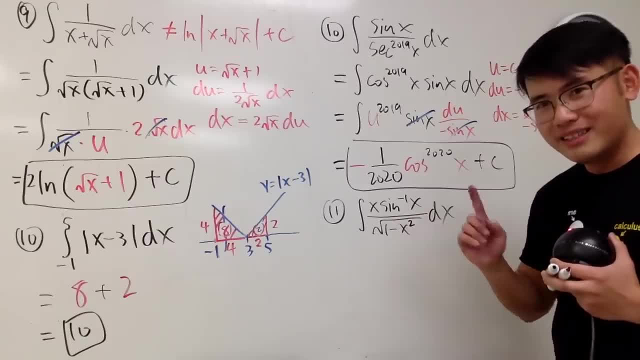 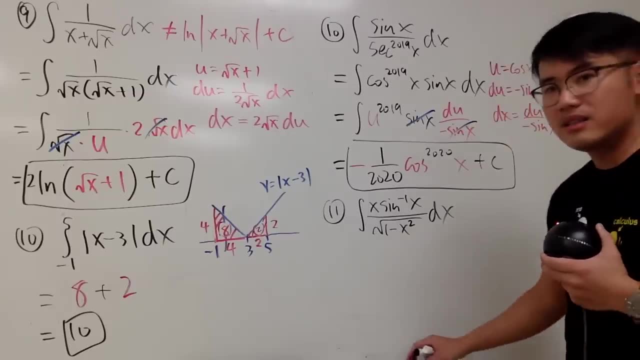 I know how to differentiate this guy. So, with that being said, this suggests us to do the integration by parts, And I will actually do integration by parts, right? Yeah, let's just do it right here, Why not? Let's see. 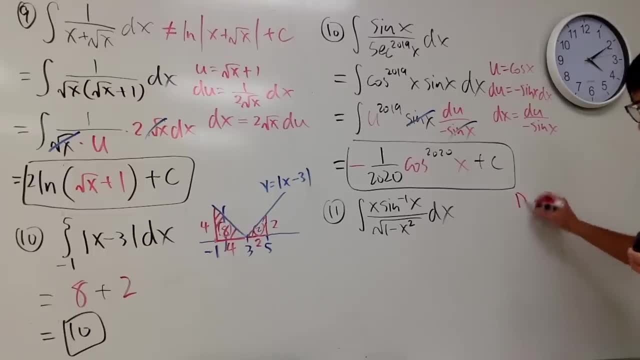 Now I want to keep my usual way to work in my work, so I'll put down d and an, i I want to. I want to integrate x over square root of 1 minus x squared, And then I want to differentiate inverse sine x. 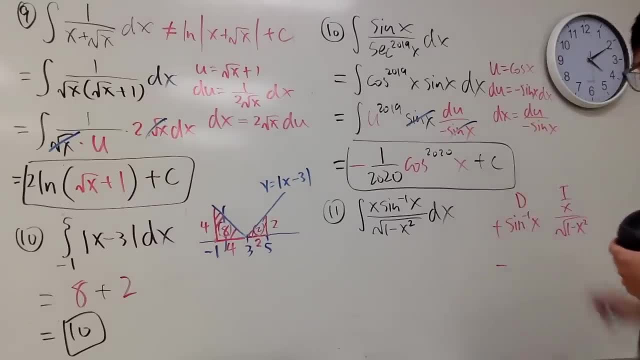 And don't forget the plus minus Two rows will be enough. When you differentiate this, you get 1 over square root of 1 minus x squared. When you integrate this Right, Let's do the USAP in our head okay. 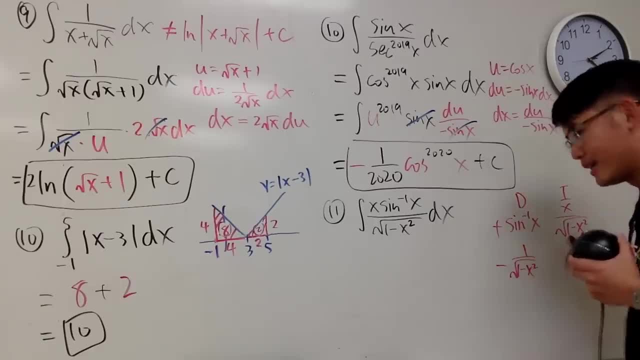 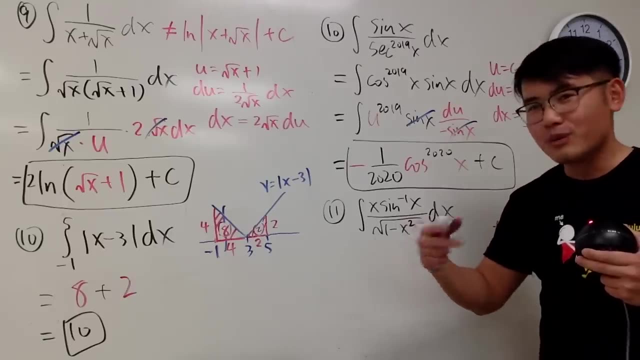 Let u equal to this guy And you end up with You know what. Let me just tell you guys the answer, Because here's the deal. You should be differentiating square root of 1 plus or minus. the x squared a lot already. 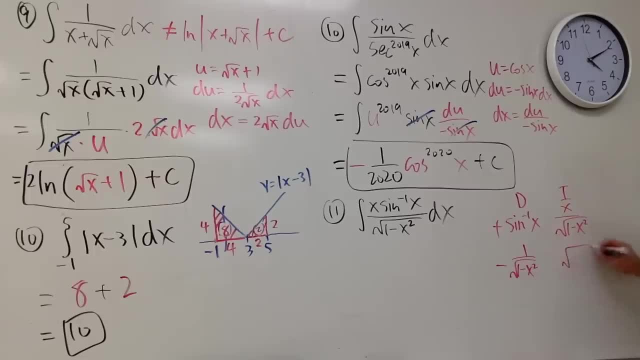 When you integrate this guy, you do the USAP on your own if you would like, But you end up with the square root of 1 minus x squared. Let's see if this works or not. We have to have some sign, maybe. 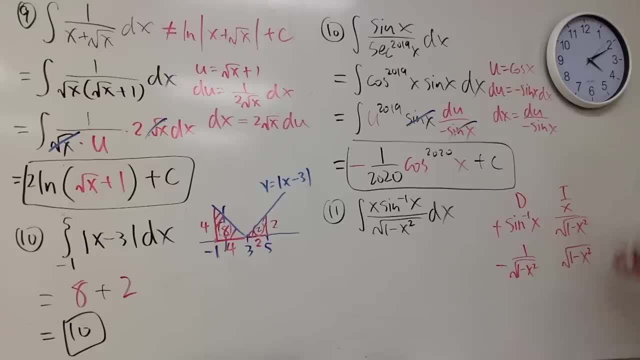 When you differentiate this, you get 1 over. You get 1 over 2, right, You get 1 over 2, square root of 1 minus x squared. But you have to multiply by the chain rule, So you have to multiply by negative 2x. 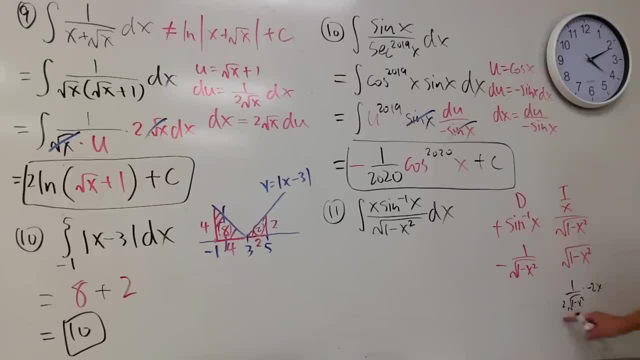 Alright, so I got the x back. They cancel, but I need a negative, So I need a negative right here. So that's how you can do it real quick, right? So if you have a negative, then the derivative would be that. 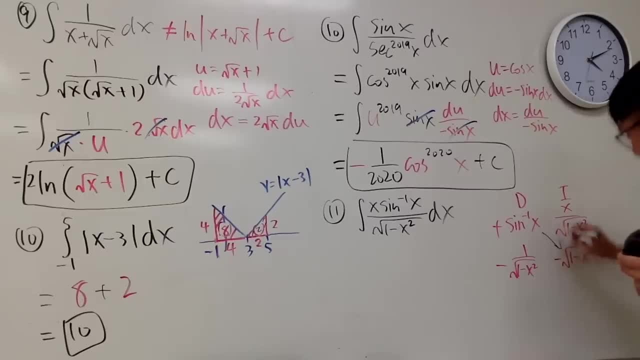 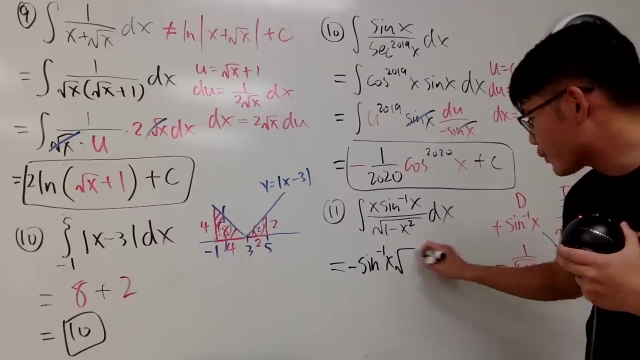 Anyway, just do it whichever way that you want. And then you see, the nice thing is, The first part of the answer is this times that We have a negative, And perhaps I'll put an inverse sign first. Inverse sign of x times the square root of 1 minus x squared. 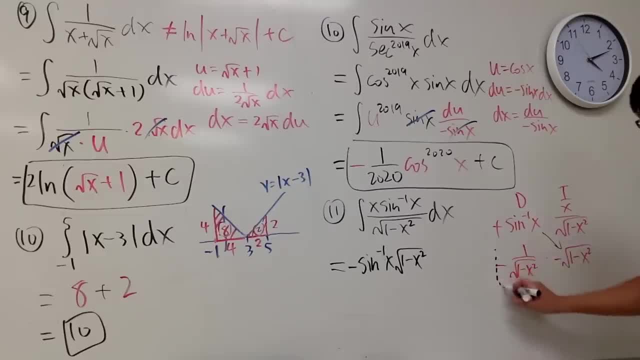 And then you do this times. that- And of course, don't forget, this- is technically still an integral, But the beauty of this is that they cancel each other. That's very nice, isn't it? So again, you have an integral of all this. 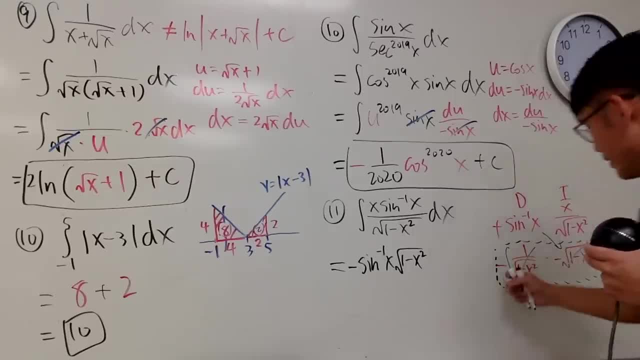 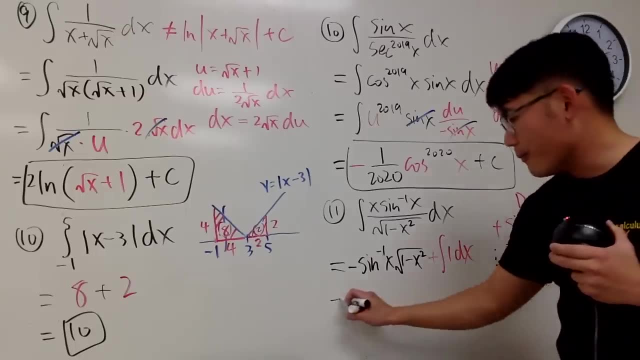 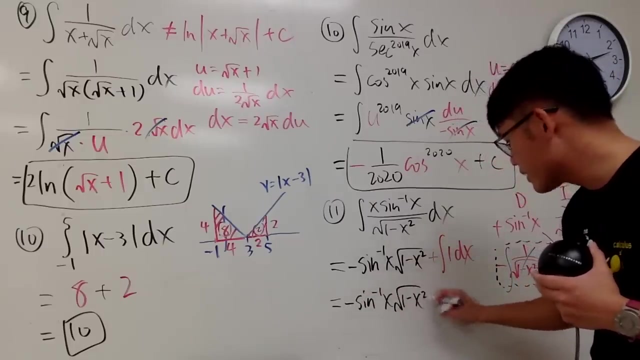 but they cancel out when you multiply And you technically have to add the integral of 1 now, And then of course you have the dx. So all in all, the answer is just this: Negative inverse sign: x times the square root of 1 minus x squared. 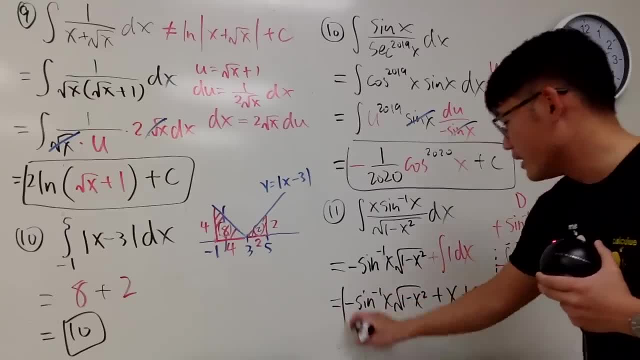 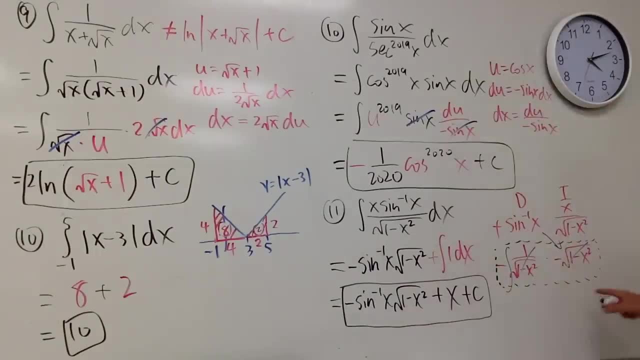 And then the integral of that is just plus x And you're done. Plus plus c. This right here is not bad at all And I dropped the eraser, okay, So let me just triple check. The derivative of this is: 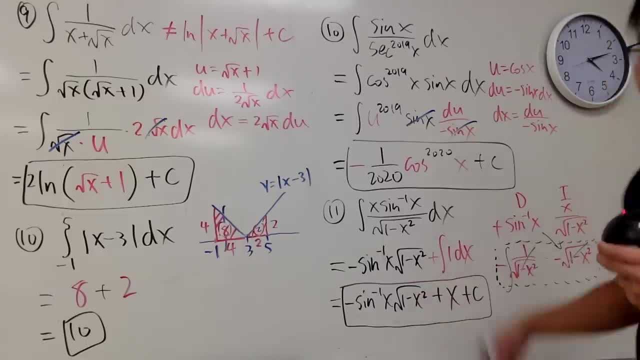 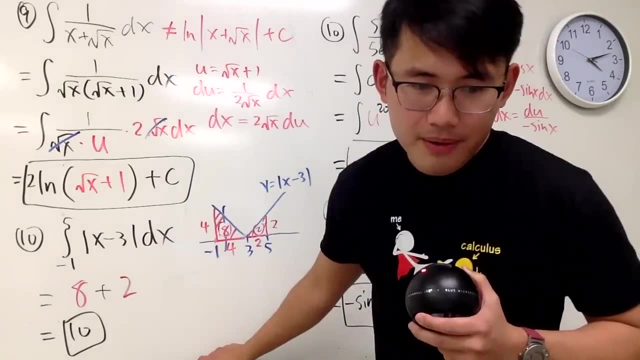 That is correct. and now that thing is correct. Everything is correct. This is good So far, so good, right, Yeah, All right Number. Wait, I have 10 twice. All right, That's number 10.. 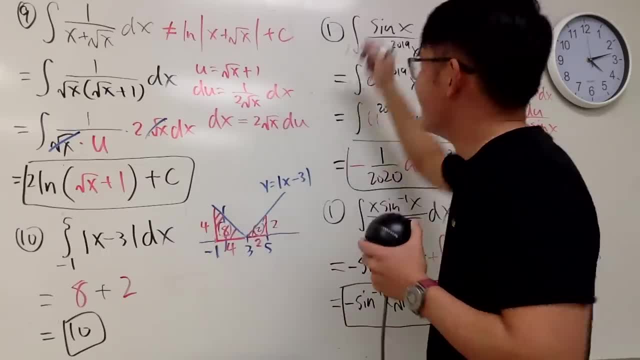 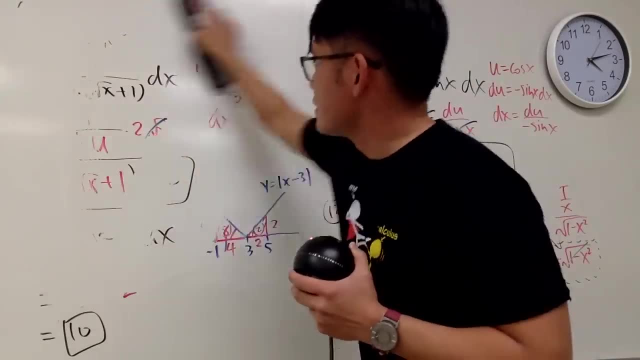 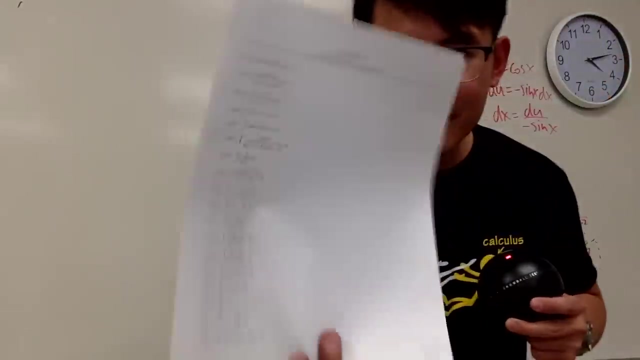 This right here should have been 11 and 12.. Number 11, number 12, right, I'm not tired yet. Hopefully not. All right, let's see Number 13.. We have this guy right here, So I will put this down right here for you, guys. 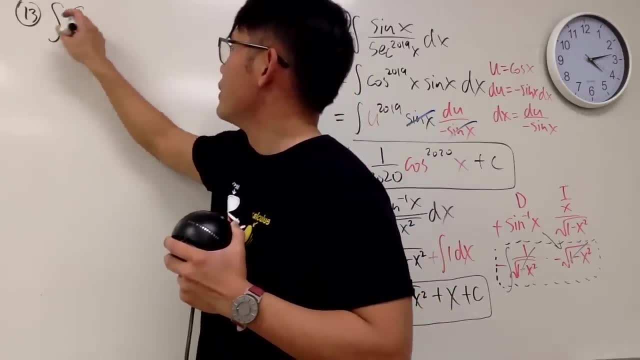 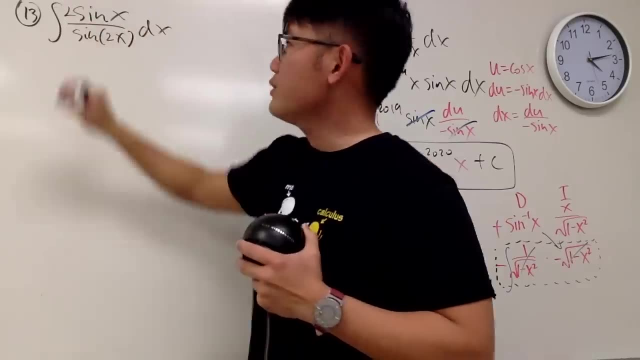 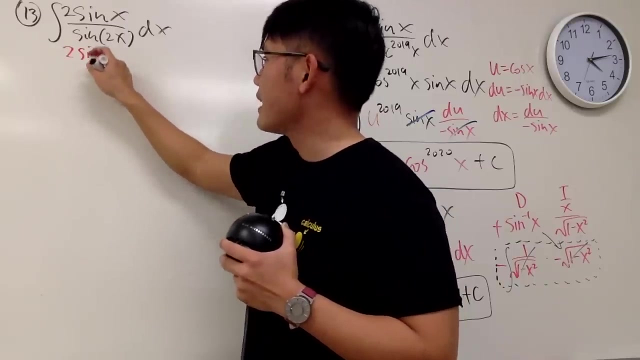 Number 13. We have the integral of 2 sine x over sine of 2x like this. This right here. it's actually very easy. Why? Because if you use the double angle formula for that, you end up with 2 times sine x. 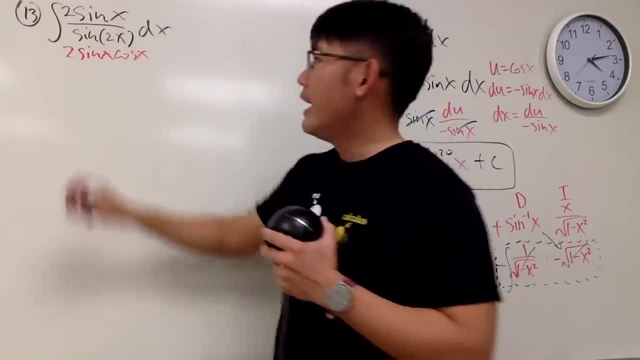 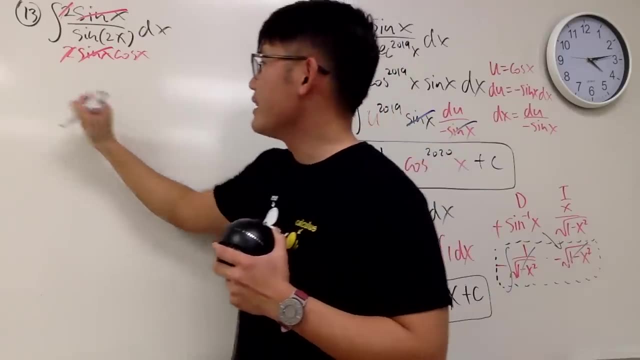 and you also have another cosine x And, as you can see, the 2s cancel and then the sine x cancel, so you just have 1 over cosine. In another word, you have the integral of secant x And you know, perhaps you forgot- 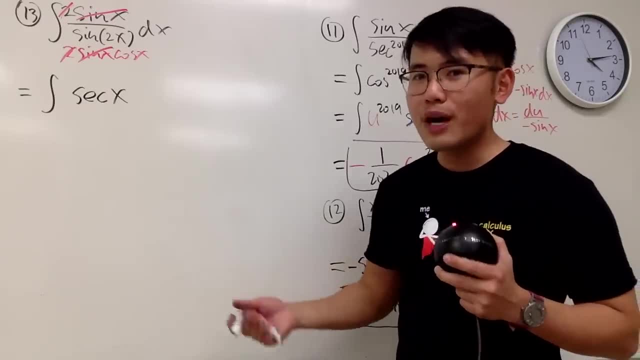 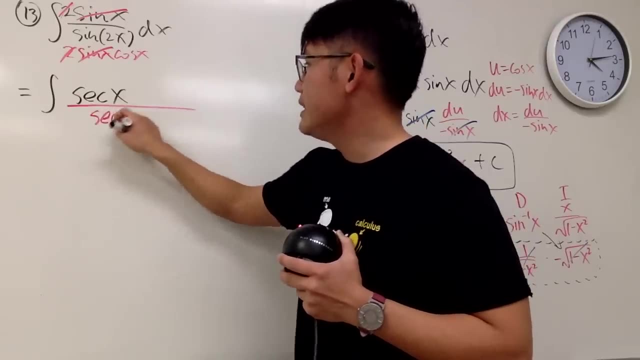 how to get the integral of secant x from scratch. so I'll show you guys this real quick. To integrate secant x from scratch, you are going to multiply the top and bottom by secant x plus tangent x, right? So multiply this by secant x plus tangent x. 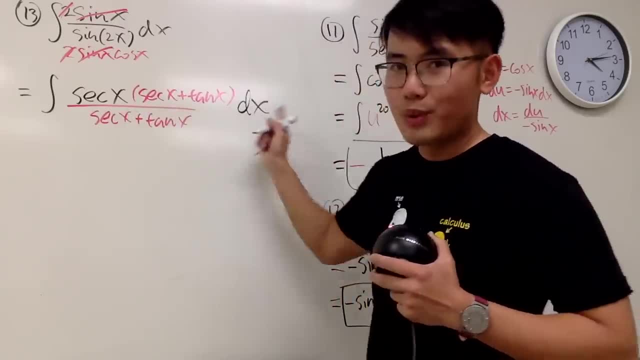 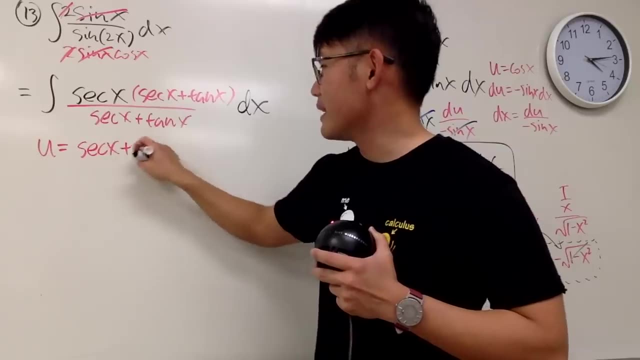 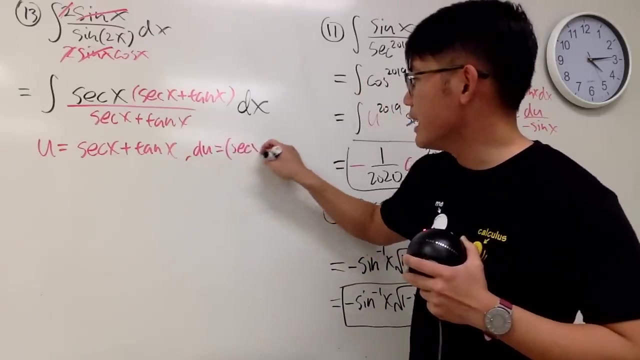 And this is why I haven't put down the dx earlier- And then you take a u sub let u, equal to the denominator secant x plus tangent x. When you do that, you get du being the derivative of this, which is secant x, tangent x. 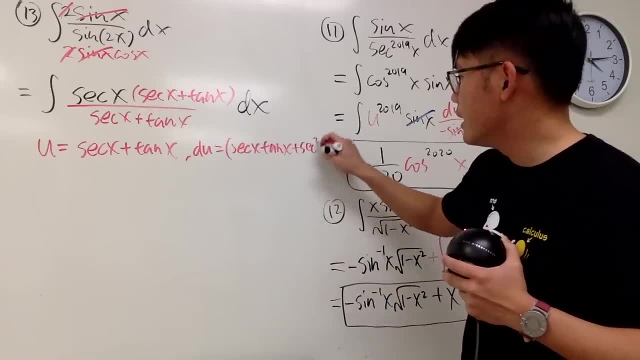 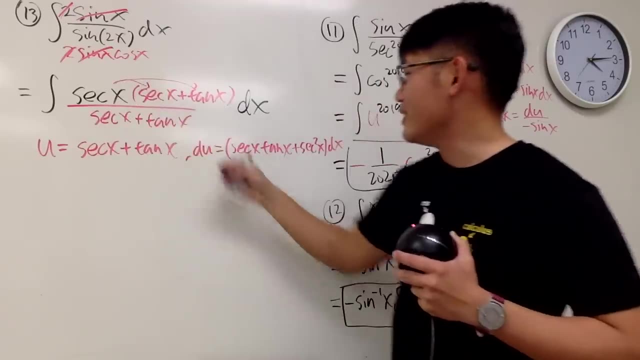 and the derivative of that is secant squared and then x, dx. That's exactly what you have on the top. You see secant squared and then secant tangent, which is exactly our du. So in another word, this right here is just the integral of 1,. 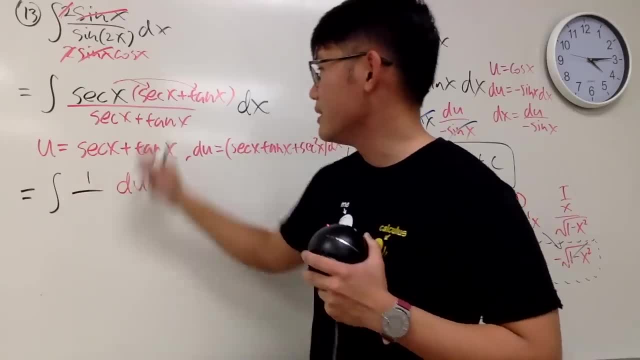 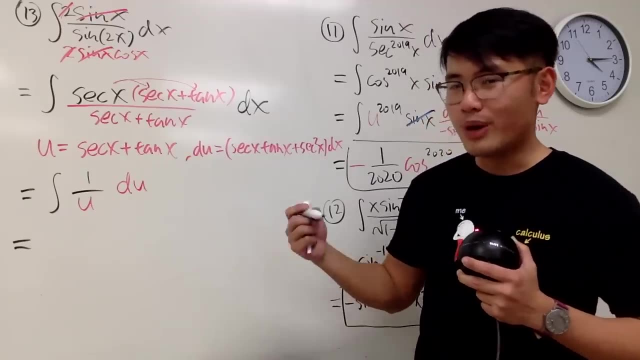 and then let's put the du on the side and then the bottom is our u. So that's how you do it And, by the way, this right here is the standard result when you have the integral of secant x. 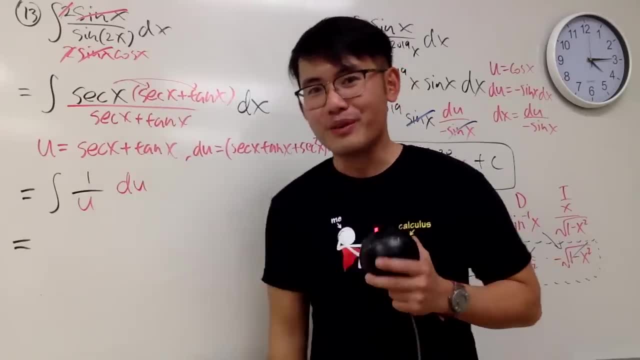 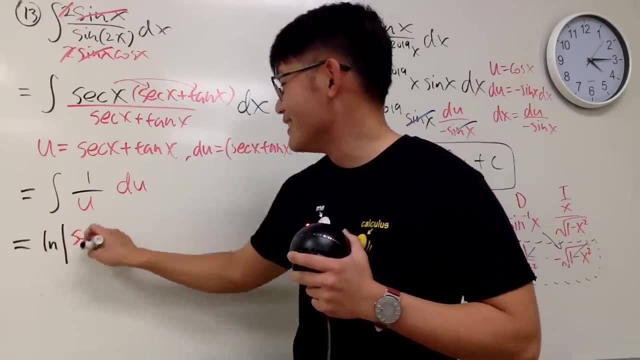 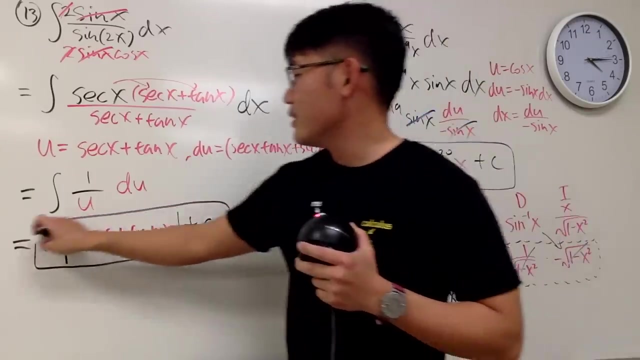 And there are other ways to get the integral of secant x. You guys can check out my other video for it. Yeah, but I will just write down natural log: absolute value of secant x plus tangent x And, of course, if you're just doing the test, 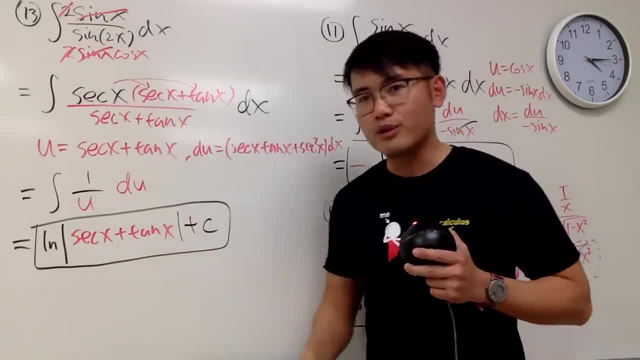 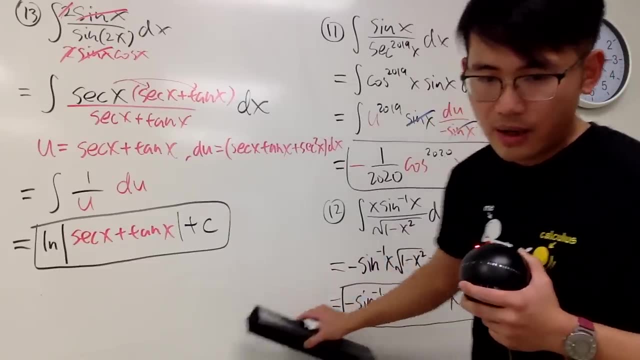 you can actually just go from this to here without showing this every single time, unless the question wants you to do so. All right, so that was number 13,, and now we are going to do number 14,, which is going to be right here. 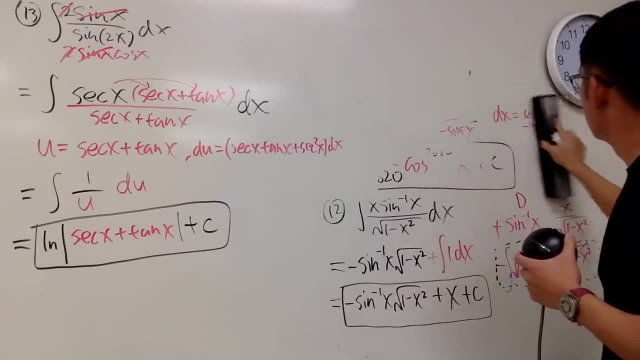 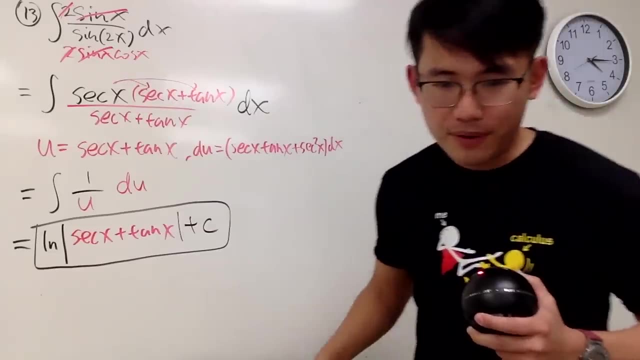 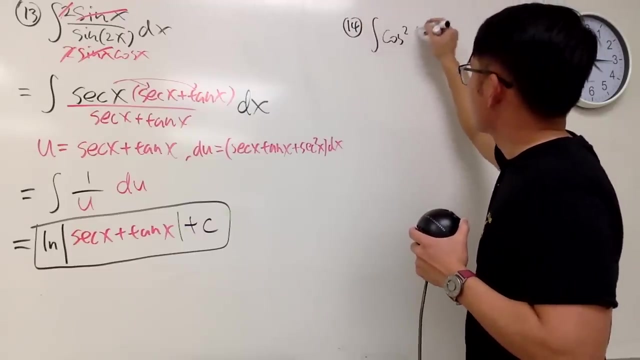 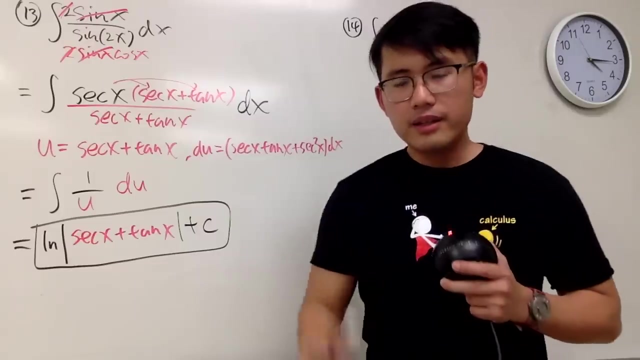 Let's see Number 14, right here, maybe. Sure, why not Number 14, integral of cosine squared of 2x, Like that right? Okay, the power is 2.. We don't like that. We want to have the power to be smaller. 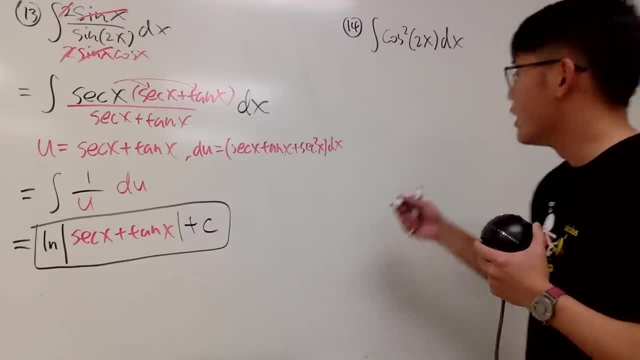 and to do so we are going to use the power reduction formula, which is the following: okay, I'm looking at the cosine version, so I'll make a note right here. So I'll make a note right here for you guys. 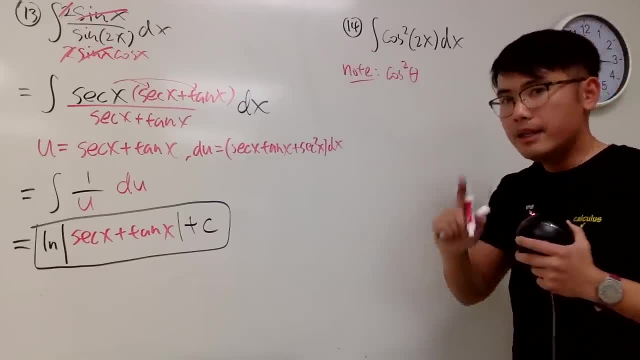 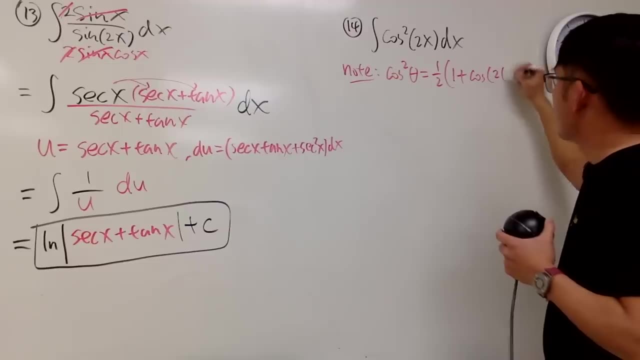 We know that cosine squared theta- this right here- is equal to 1 half times 1 plus cosine of 2 theta like this: Well, in our case, here you see, the theta is actually 2x. So you are going to plug in 2x, right here. 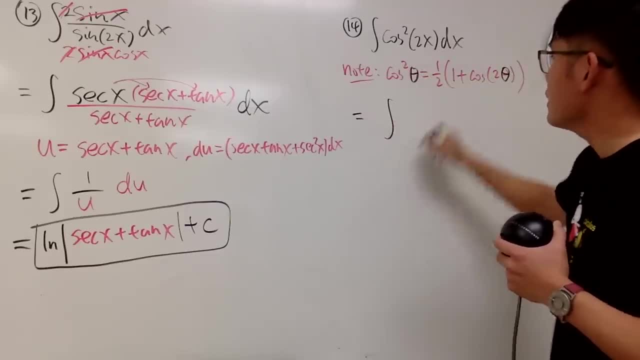 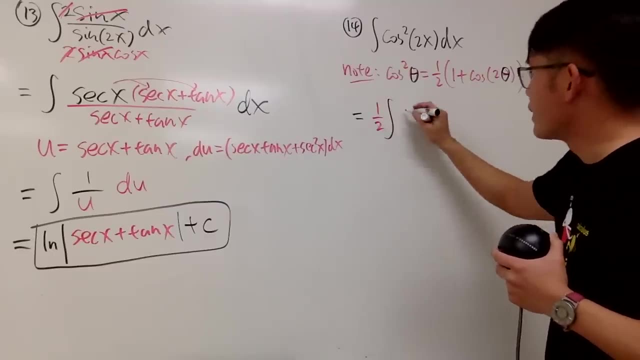 So in another word, we are integrating: 1 half is just a mod, It's just a constant multiple, so we can take that outside And then we have the 1 right here, And then we add cosine of 2 times 2,. 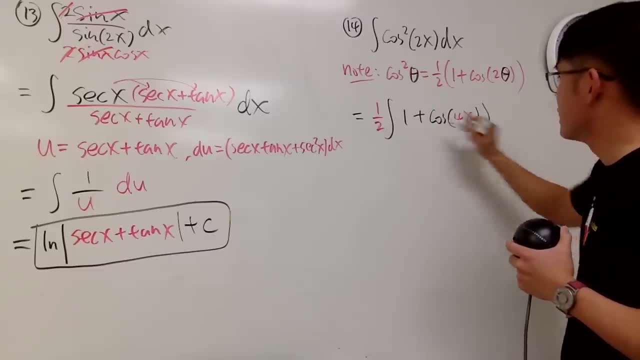 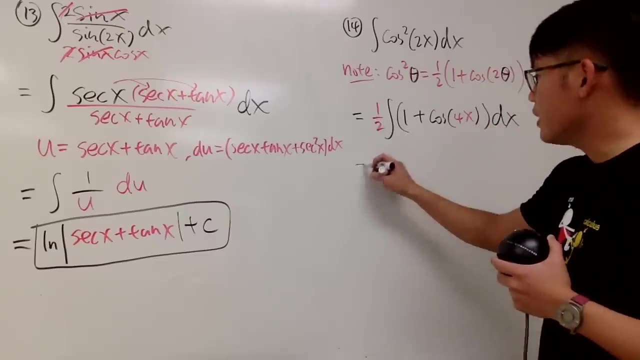 which is, of course, 4, and then x like that. So that's what we do, right, That's what we do. You just use this identity to help us out. So let's see, We have 1 half times integrating x. 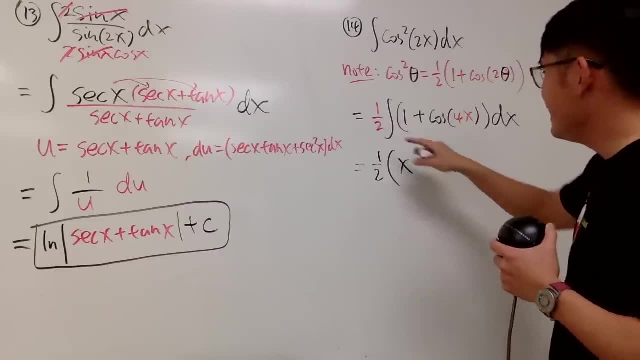 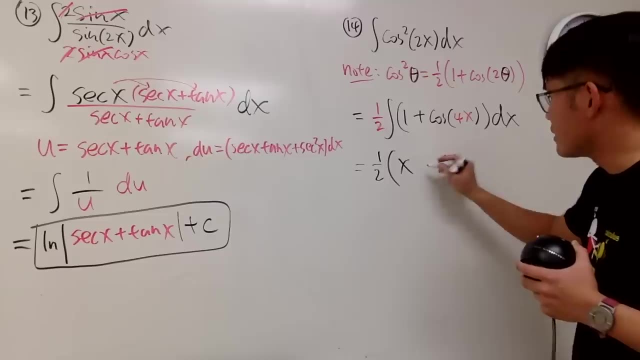 Sorry, that's the answer. Integrating 1 into x, where we get x, And then integrating this. do it slightly carefully. The integral of cosine is positive sine, So the sine right here stays the same, And then the input 4x stays the same. 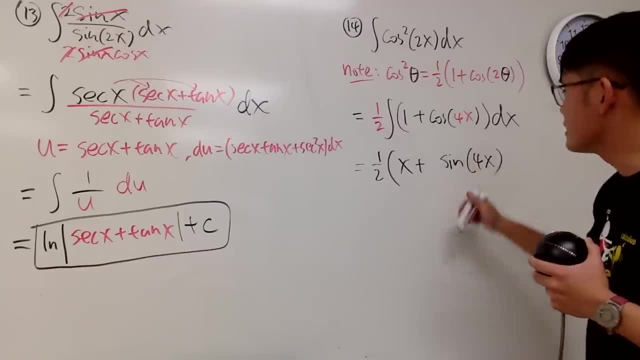 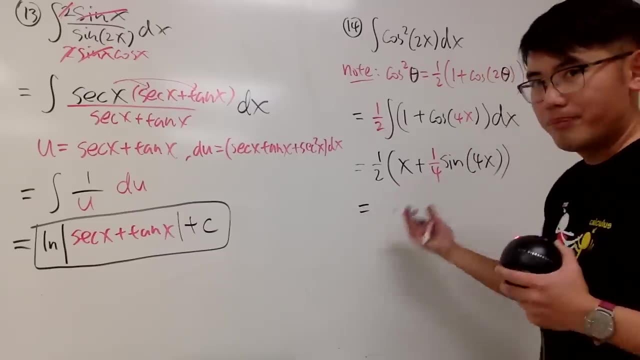 But you are doing this backwards, so you have to divide it by the derivative of 4x, So you are going to multiply by 1 over 4, like this. And we're not done yet because, you know, just be polite. 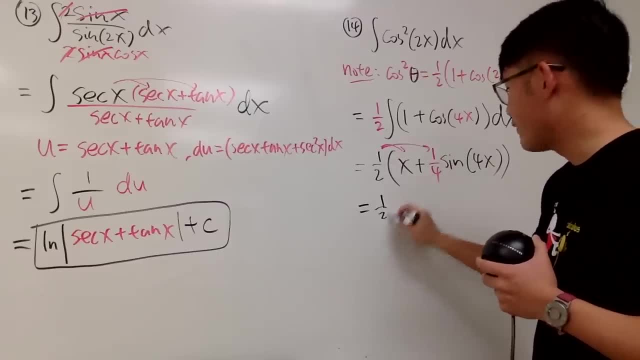 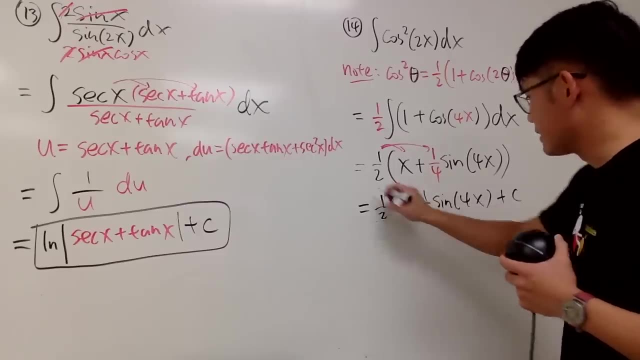 Just distribute the 1 half right here, so you get 1 half x, This times, that is 1 over 8. And then you have the sine, which is the sine of 4x plus c, like that, Right. 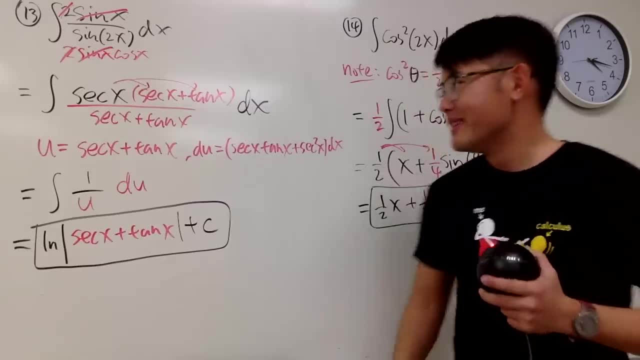 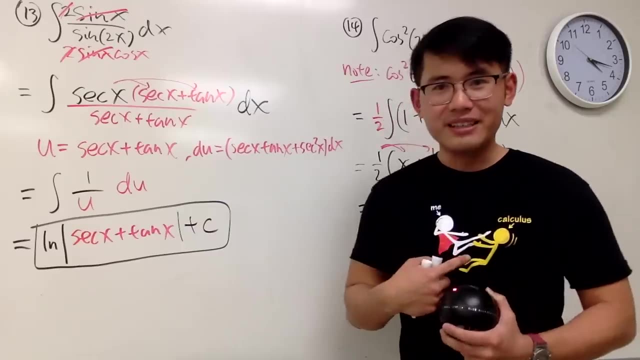 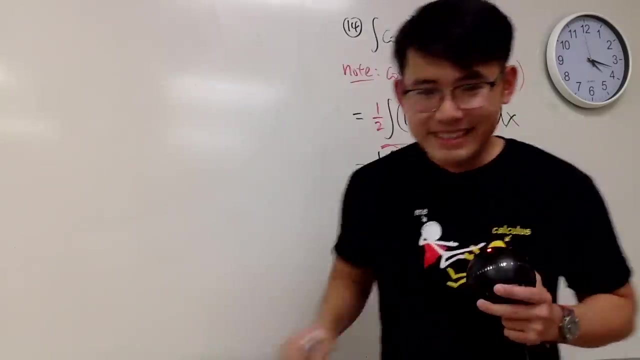 By the way, thank you so much for designing this t-shirt for me. Thank you, Alright. So this right here. you will remind me that you know I'm staying strong. We can kick calculus in its head, Okay. 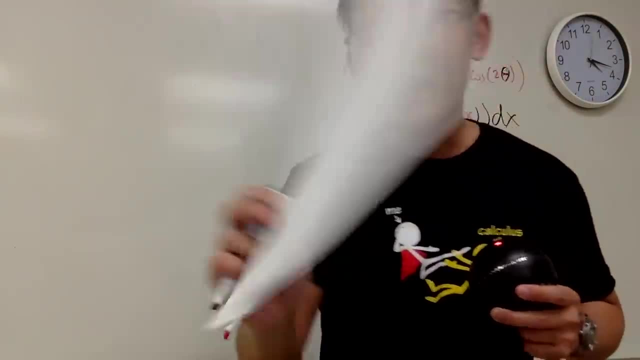 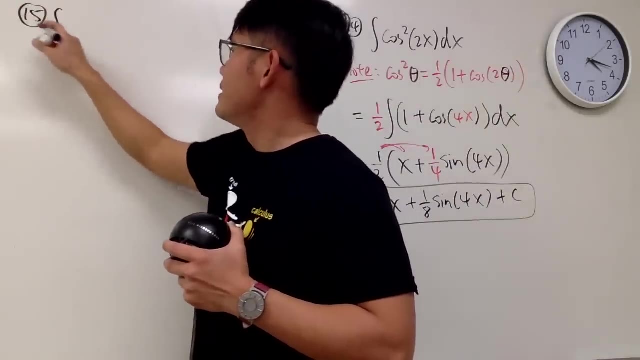 Now number 15.. This is a tough one, But put it here I really don't know why. Maybe I should change it, But it's too late now. 1 over x cubed plus 1.. Yes, you are seeing this right. 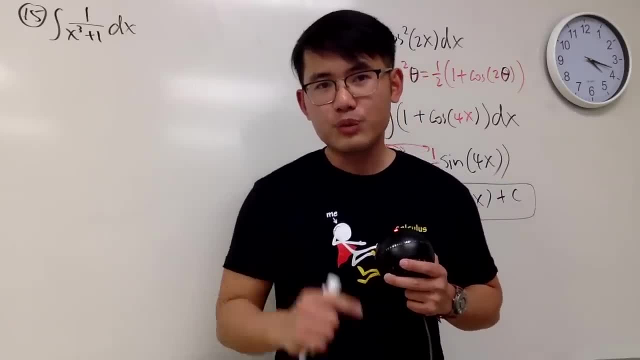 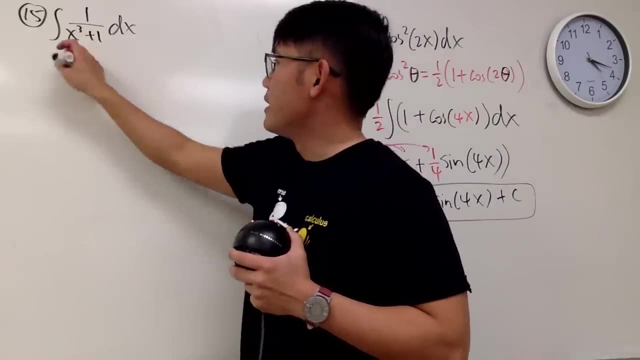 Integrating 1 over x, cubed plus 1.. Yes, we have to factor the denominator and we have to do some partial fraction. The dirty work Alright. When you factor the denominator, you are going to get x plus 1,. 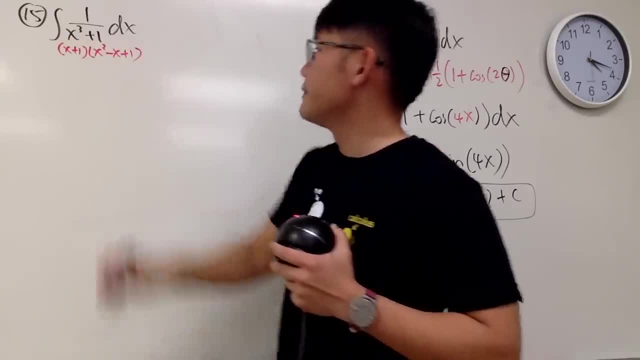 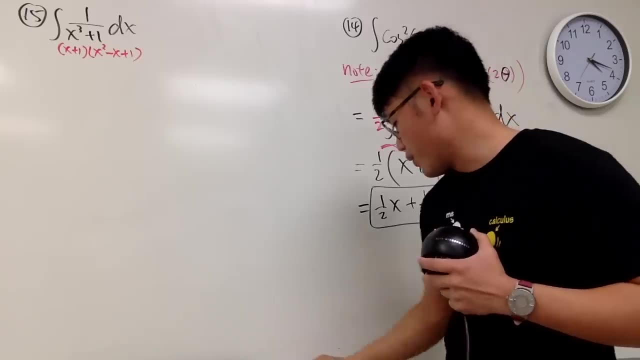 times x squared minus x plus 1.. So let's see, Perhaps I'll put the final answer right here. So I will do the partial fraction right here in blue for you guys. First of all, I will just be writing this down as: 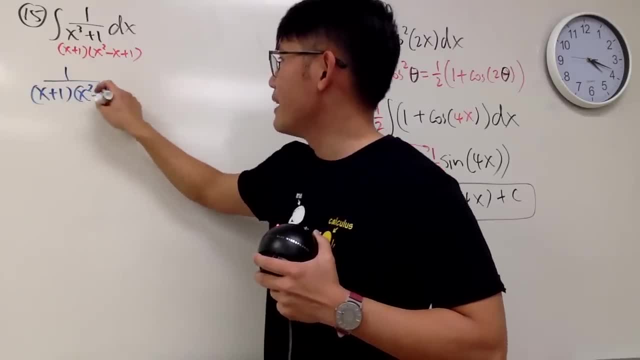 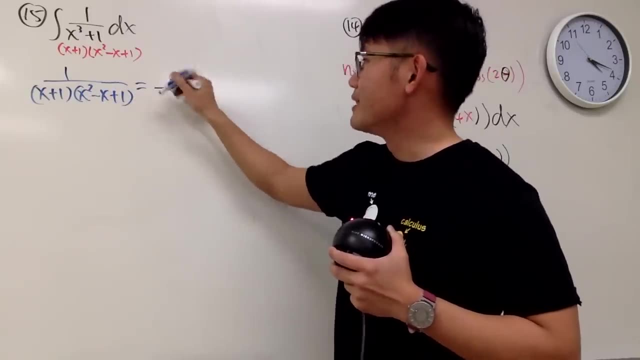 1 over x plus 1, times x squared minus x plus 1.. We have two factors. The first one is linear, so I'm going to say this is equal to some constant a over that denominator, which is x plus 1.. 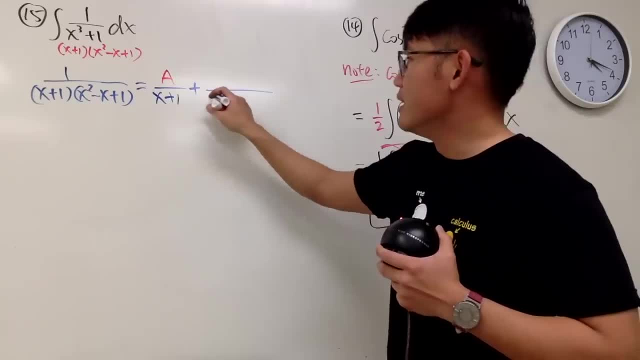 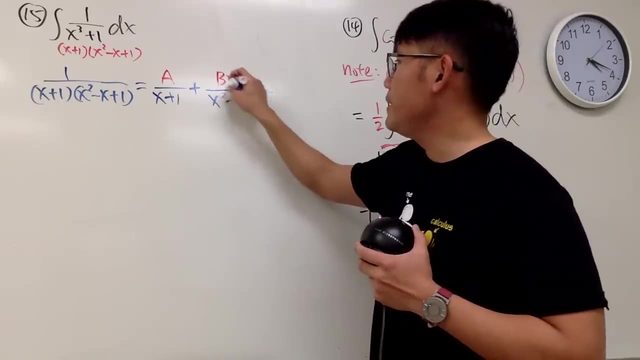 And then the other one. I'll just say plus. This guy is an irreducible quadratic. Therefore, on the top we have to set a linear. In another word, we have to put down bx plus c, Alright, A. it's easy to figure out. 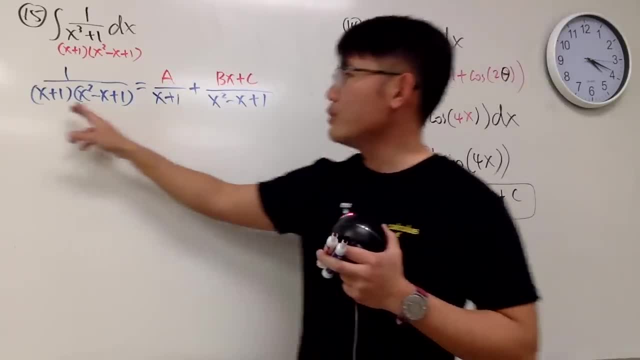 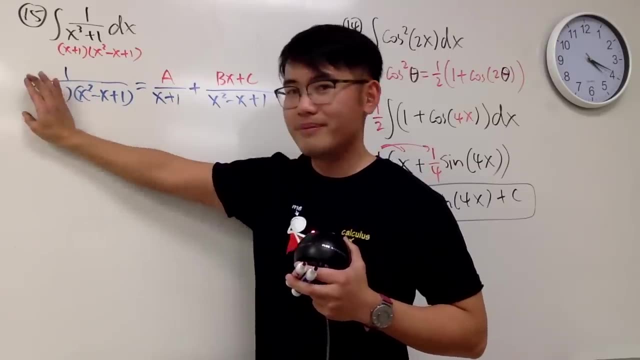 because we can do the cover-up method. I'm going to go to the original denominator, cover this up, and I will ask myself: what do I need to put in to make this 0?? I need to put in: x equals negative 1.. 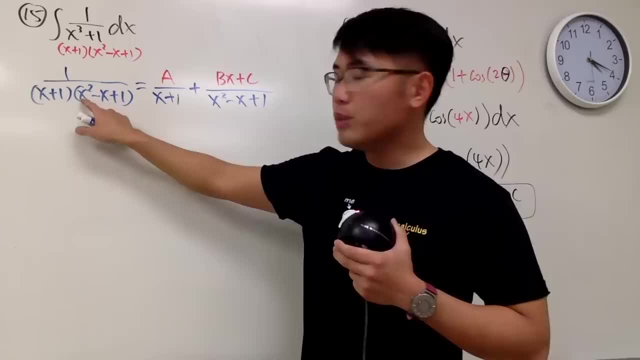 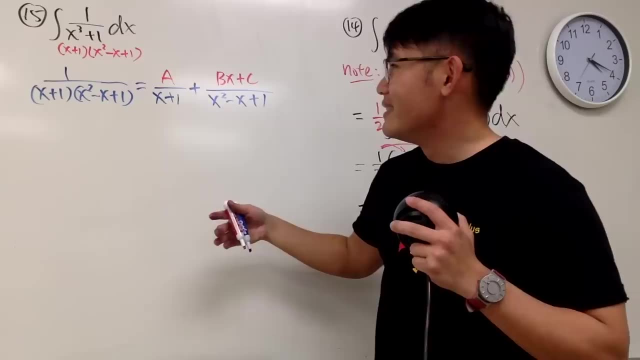 Put in negative 1, negative 1 here. Check this out: Negative 1 squared is 1.. Negative negative 1 is another 1, so I have 2, and the plus 1 is 3.. So yeah, 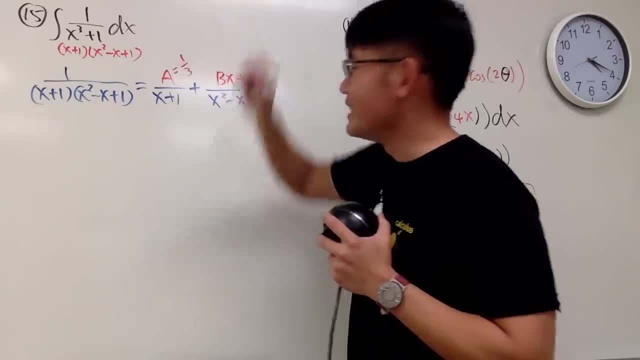 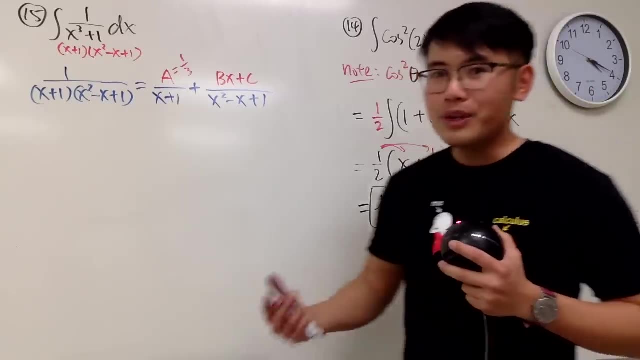 that's it: 1 third a is equal to positive 1 third. That is very nice, And we also have to figure out the b and the c. Well, the deal is that we can just plug in whatever x values that we want. now. 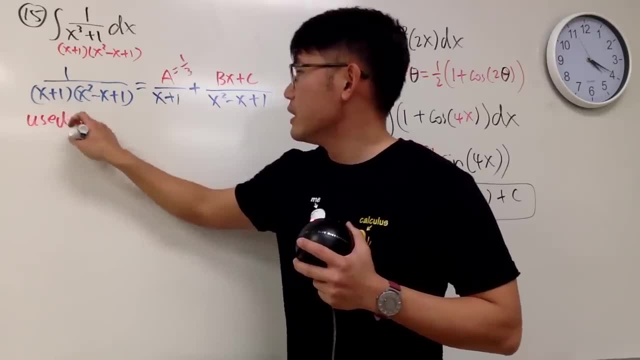 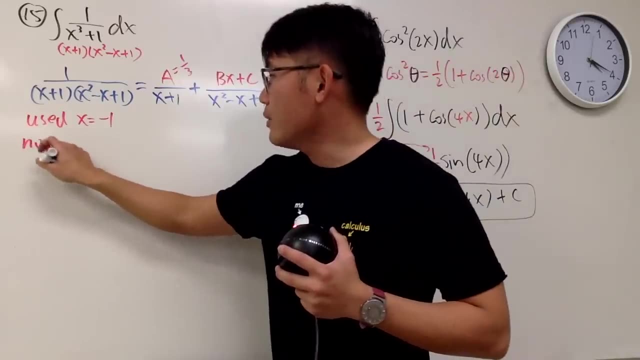 But let me just make a note. We used x being negative 1 to figure out a, so we cannot use negative 1 anymore. But we can now use, let's say, x is equal to 0.. We're going to do this in your head, okay. 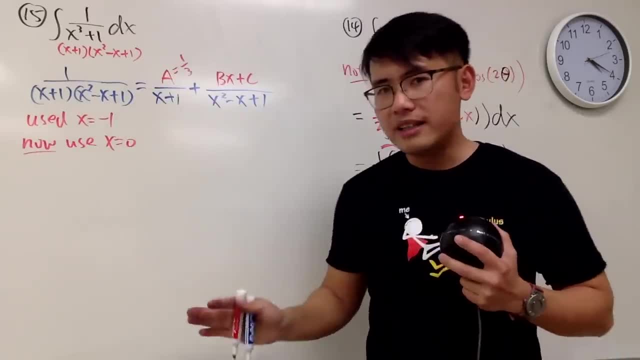 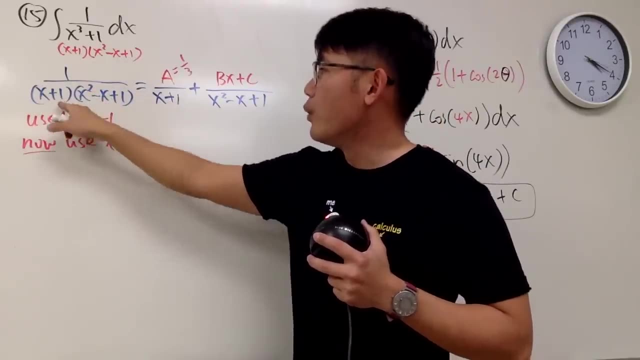 When you're putting x equal to 0, this right here, we cannot cover anything up. so you put x equal to 0 for all the x On the left hand side. this is 0,. this is 0,. this is 0,. 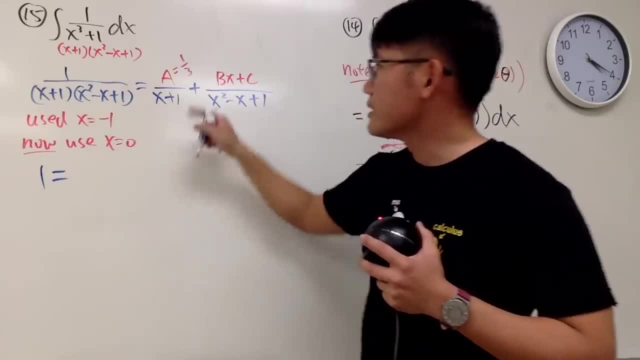 1 over 1 times 1, so you have 1.. And on the right hand side this is 0, so 1 third divided by 0, so you have 1 third. Well, the beauty of putting 0 is that. 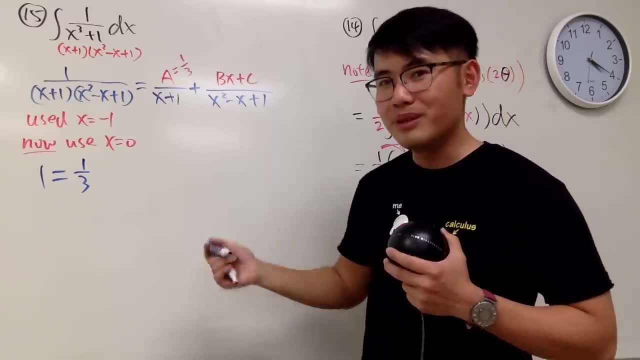 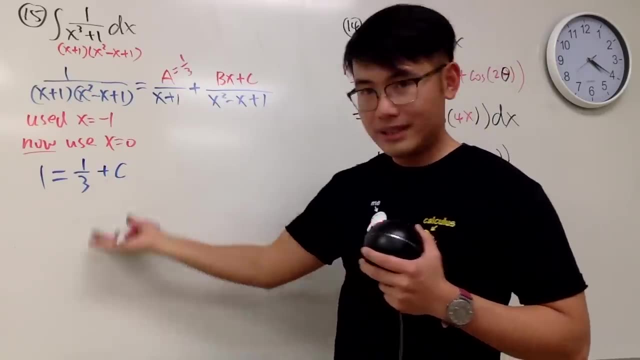 you see b times x, in another word b times 0, this is gone. So this is gone. So 0, 0, so it's 1 on the bottom. so you get plus c. That's what we have. 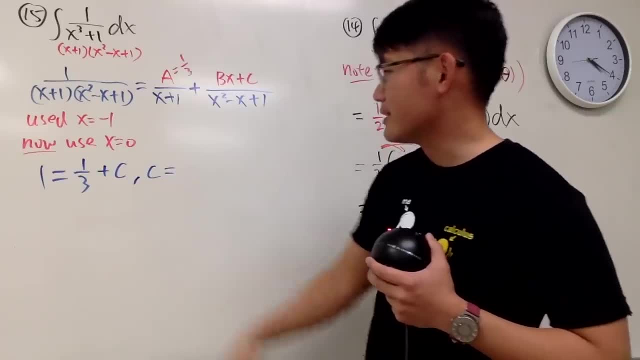 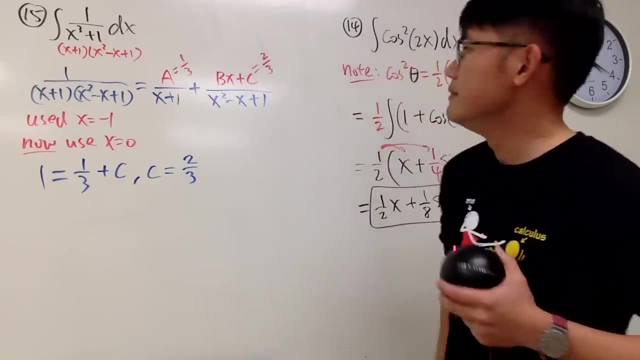 In another word. you see that c is equal to minus the 1 third on both sides. You get positive 2 third for that. so that's very nice, Okay. And to figure out b, well, we used 0 and negative 1 already. 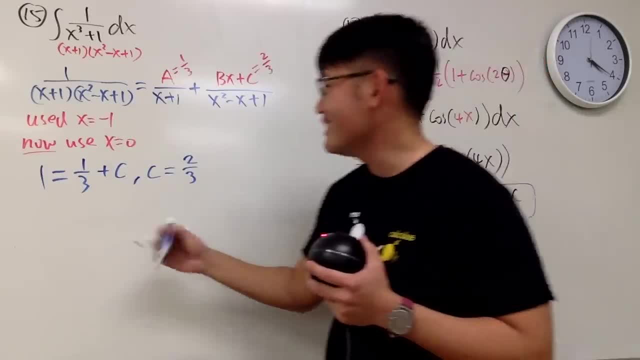 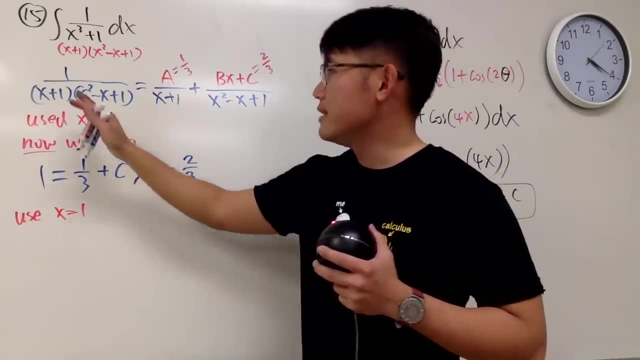 Let's pick another easy number. Let's say positive 1. Why not, right? So now I will just say: use x equal 1. Plugging 1 into all the x, not cover anything up. okay, So you get 1 over. 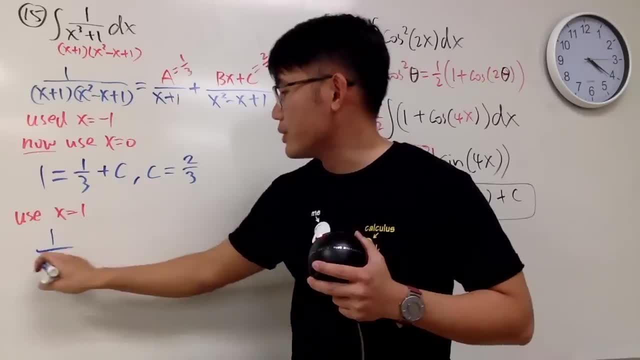 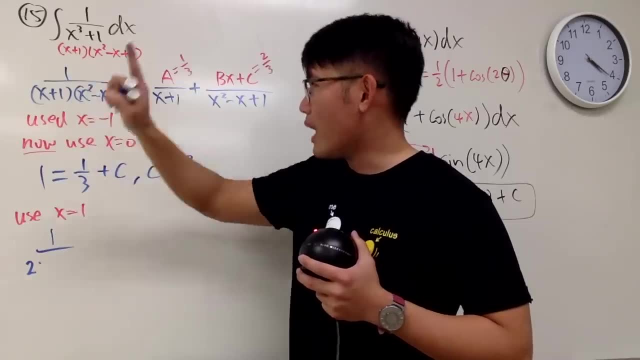 let's see, do this carefully: 1 plus 1 is 2.. Yes, you heard me right: 1 plus 1 is 2.. I said that. Anyway, putting 1 in here, 1 squared is 1,. 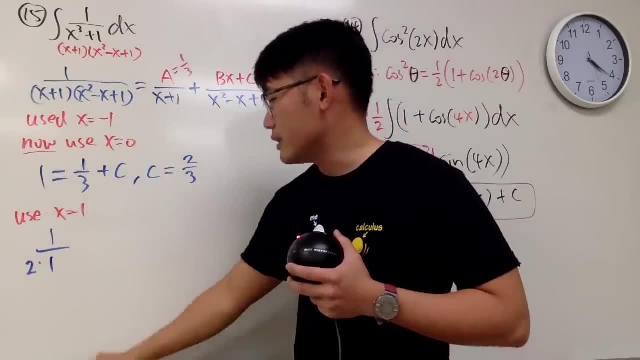 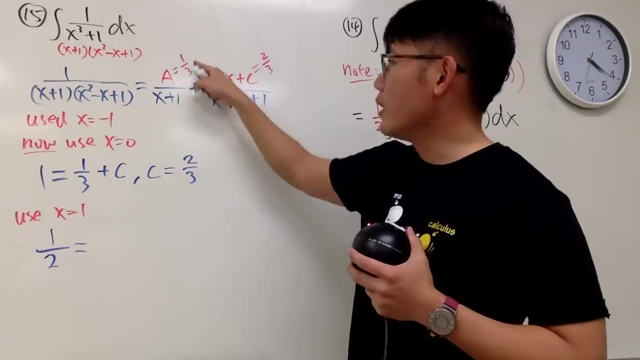 minus 1 is 0, and you have just 1, so you have that. So it's pretty much 1 over 2 on the left-hand side. Still not that bad. Now putting 1 in here, you have 1 over 3. 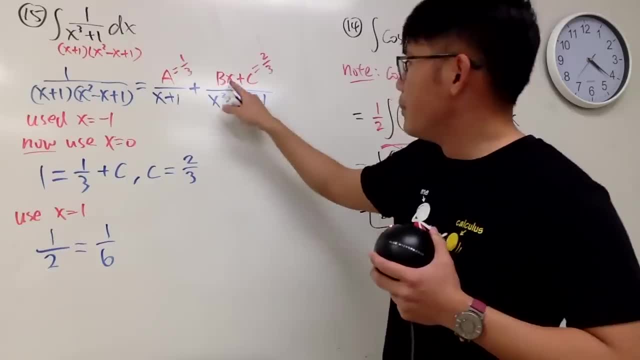 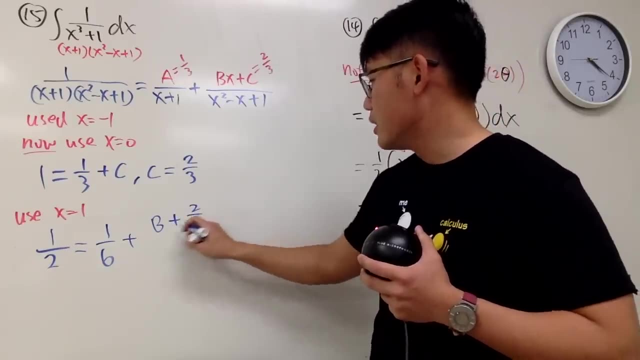 divided by 2. In another word, you have 1 over 6. Putting 1 in here- so you have b on the top and then you have plus c, is 2, third over. and then if you're putting 1 in here, 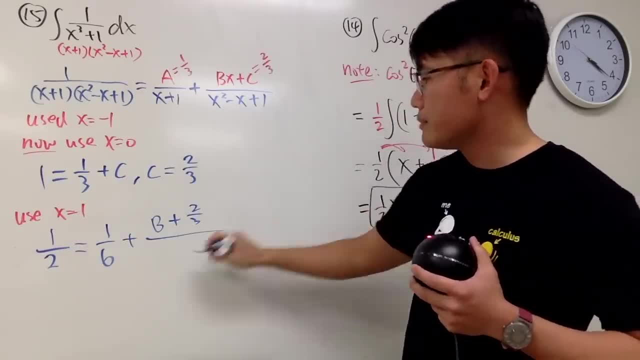 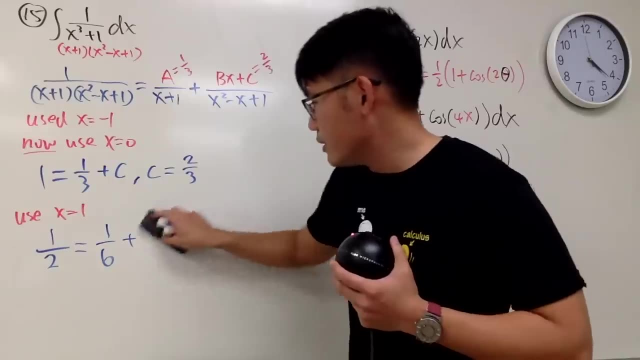 1 minus 1 is 0, so you have over 1.. So in another word, this doesn't matter, so you just have this, And then you can just solve this little equation. now, That should remind you of the good old. 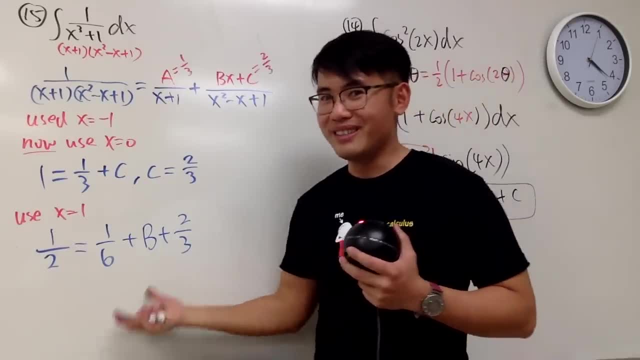 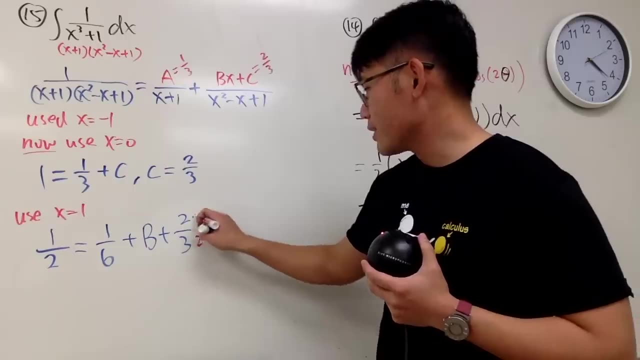 algebra days. You can just solve this and you get everything right. That's the whole question, right? Okay, let's see What can we do. We have to do fractions. Multiply this by 2,. multiply this by 2,. 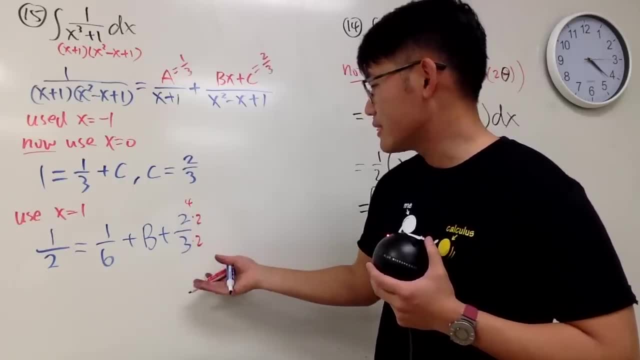 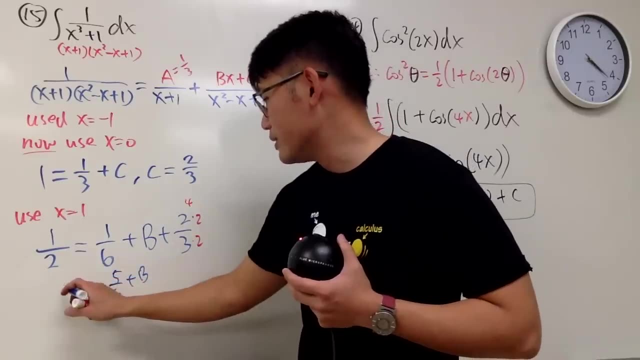 so you get 4 over 6, right. So altogether this is 5 over 6, plus b, and on the left-hand side, of course, this is 3 over 6, minus 5 over 6 on both sides. 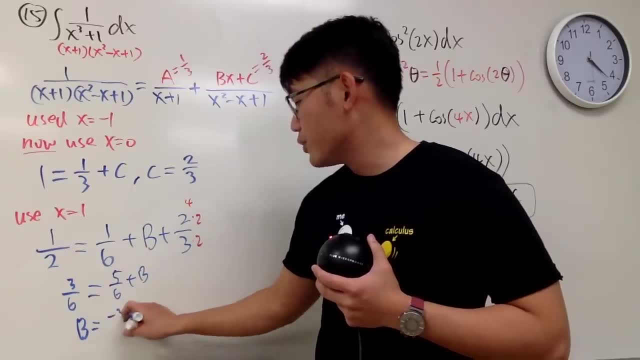 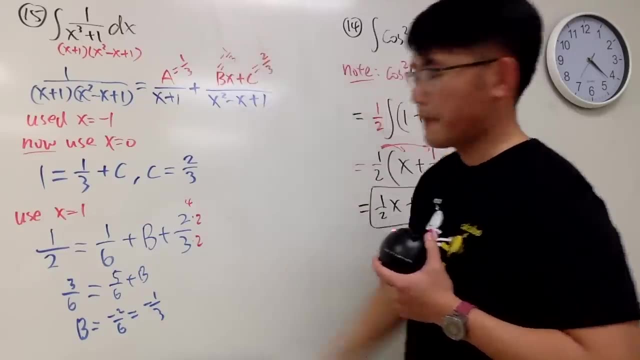 b is equal to negative 2 over 6,, in another word, negative 1 third. So b is negative 1 third, like that, Okay, Anyway, that's the partial fraction part and I'm going to erase this. 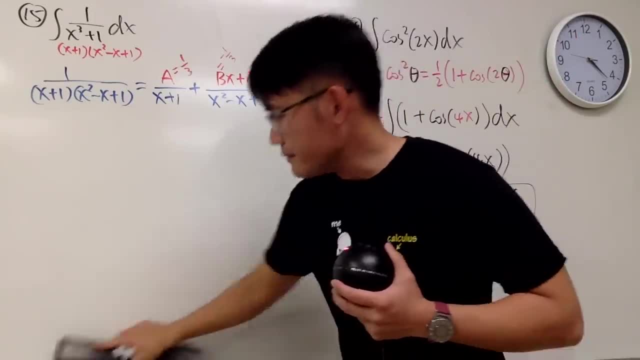 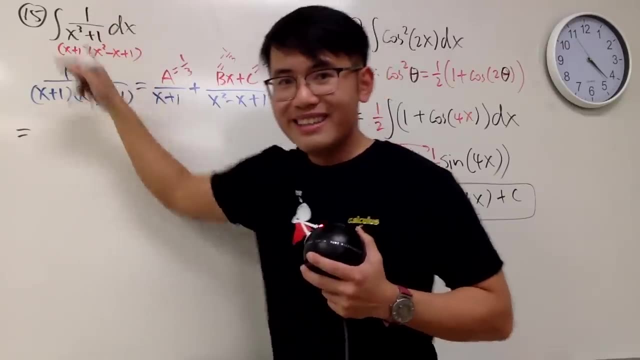 and I will be looking at the integral now. So we'll see we will have to integrate the following: This right here is the same as integrating this and that, so I will just write this down right here for you: Integrating 1- third. 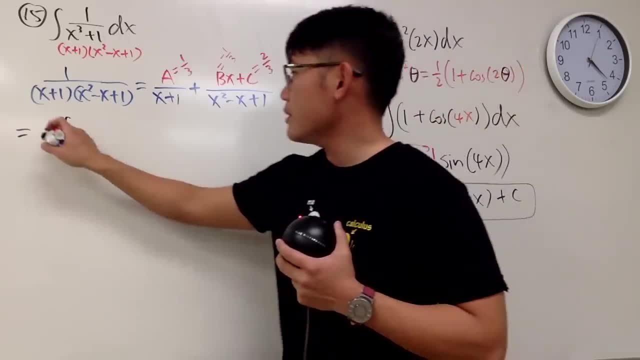 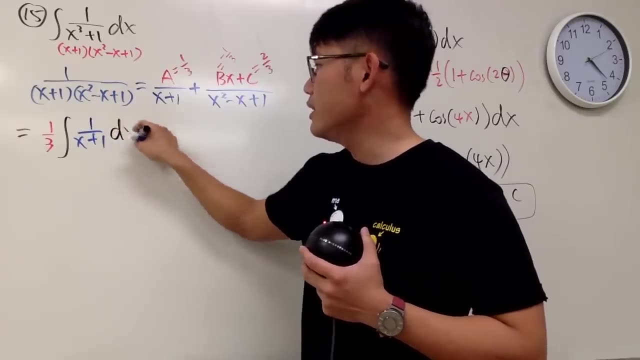 let's just put that down right here in the front, and then we have the 1 over x plus 1, like this. and then let's close this integral, why not? And then for the second one, I will just write it as plus: 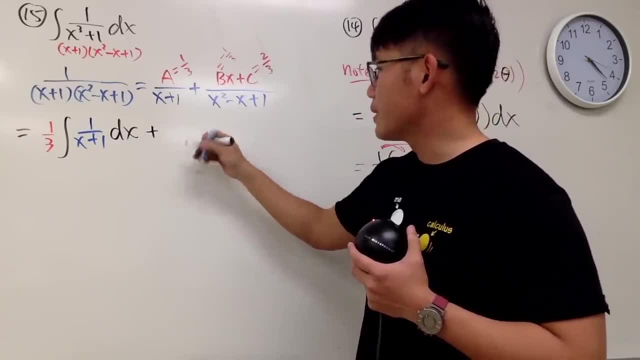 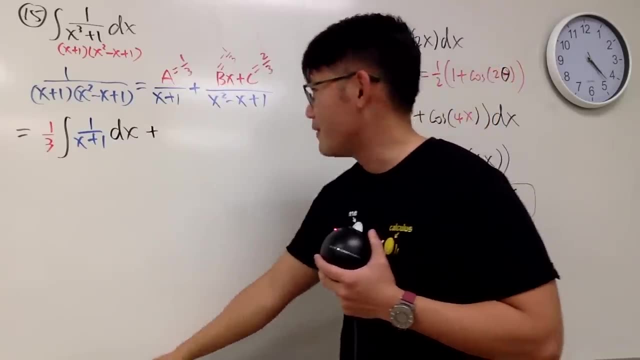 and in fact I will just keep them as how they are. so perhaps I will write down: we have the. well, both of them have the third. I can factor that out right. So perhaps I'll factor that out, and I have to do this carefully. 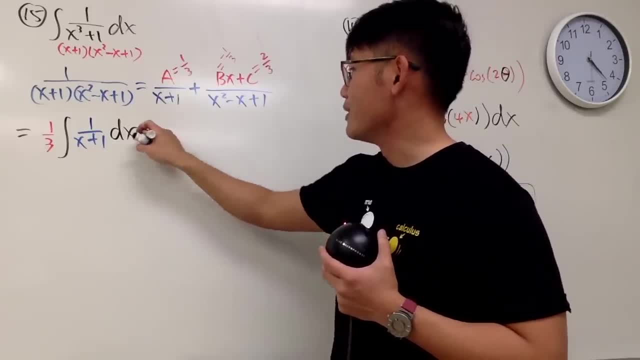 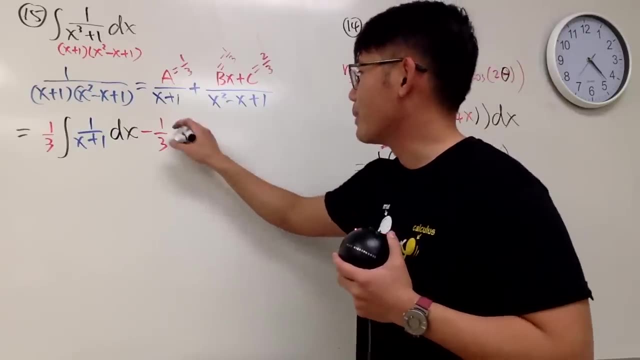 because I've been doing like 15 integrals already. so we'll see it's not that bad. Thank God I didn't put this into like a 95th integral, otherwise I don't know what will happen. 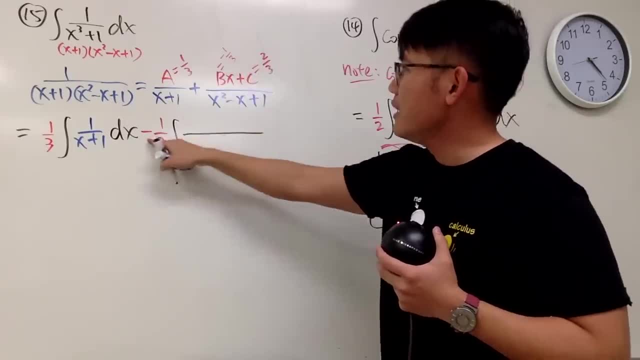 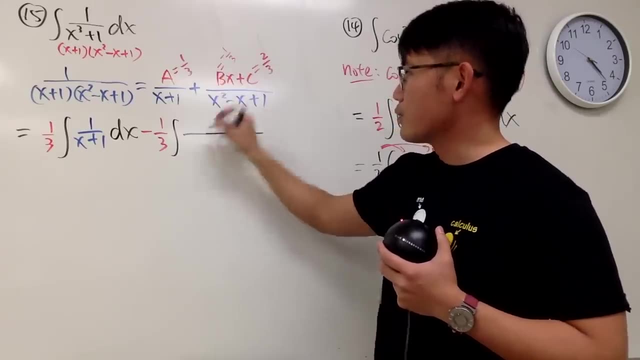 Anyway, integrating, I put the negative 1 third in the front. okay, I factor out the negative. so the b right here is this right here is just going to be x, and then this right here is going to be a minus. 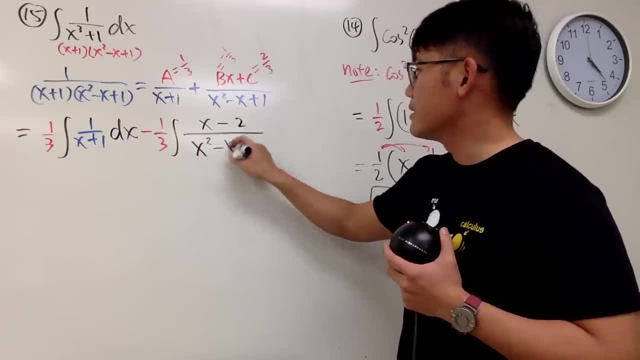 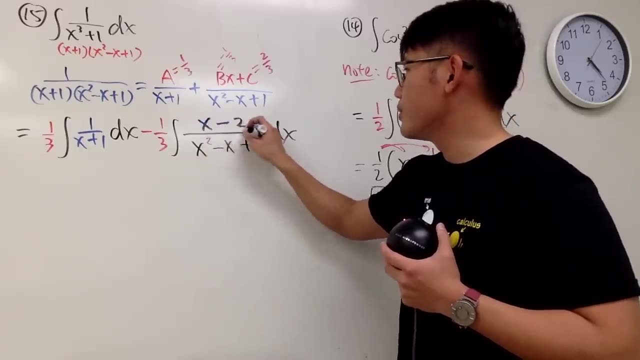 2, so it's going to be a 2, and then the bottom will stay the same: x squared minus x plus 1, like that right? Oh, I should put this down in blue. let me just do it real quick. 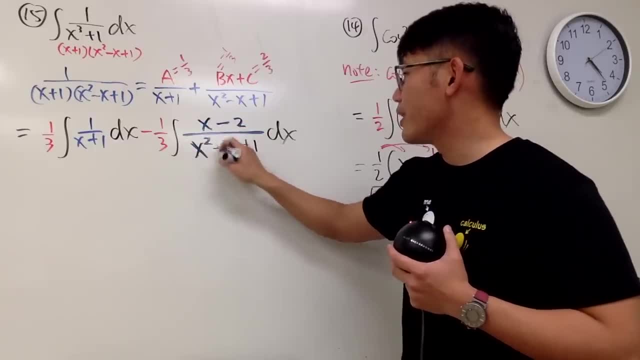 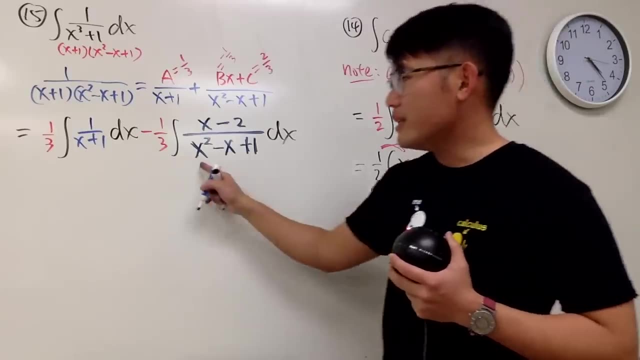 x minus 2 over x squared minus x plus 1.. Okay, we are going to look at this slightly more carefully. Notice, I will just put this down for you guys. That was easy, by the way. So look at this. 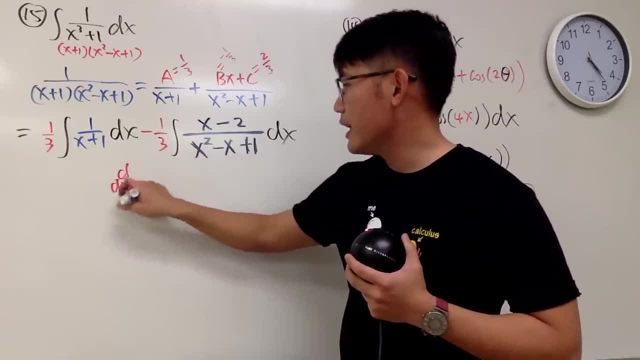 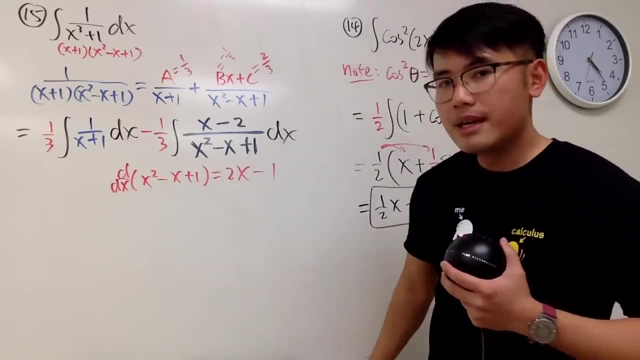 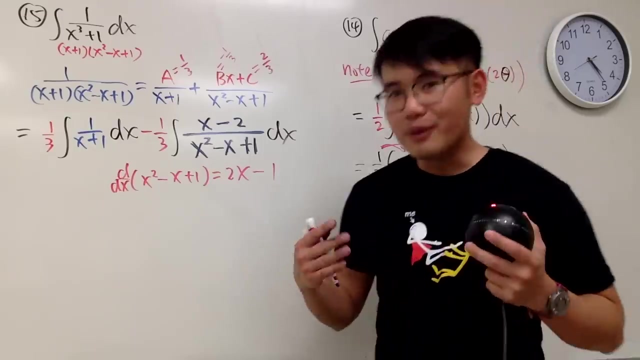 Notice: if you differentiate, if you differentiate x squared minus x plus 1, you get 2x minus 1.. On the top, I don't have 2x minus 1,, unfortunately, I have x minus 2.. I'm going to somehow. 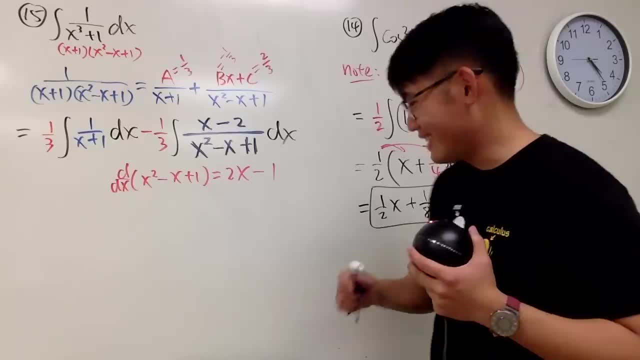 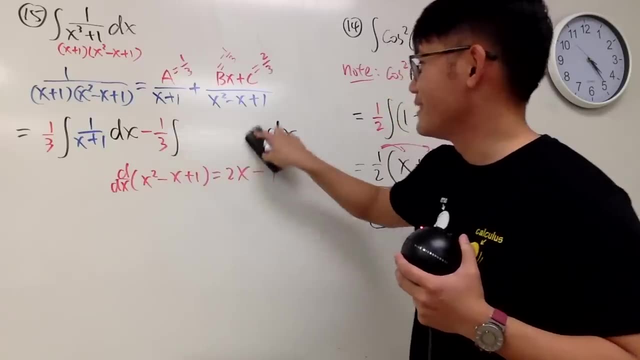 manufacture the 2x minus 1 to help us out. and this is how we can do it. I will do this. I should have put this down in black. Let me just actually put this down in black. Sorry, Yeah, Again. 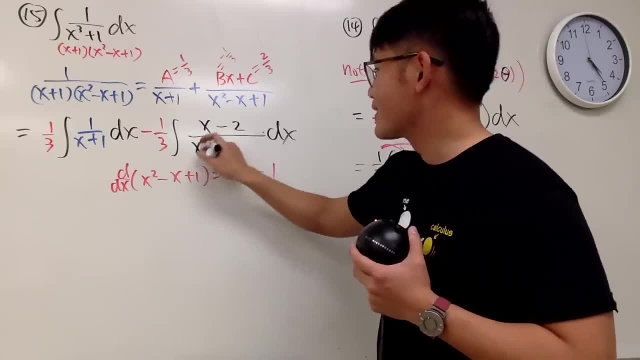 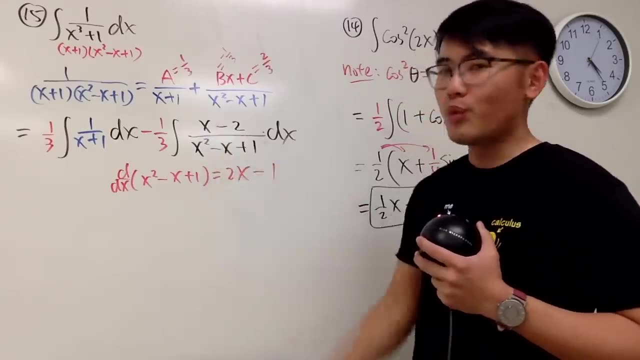 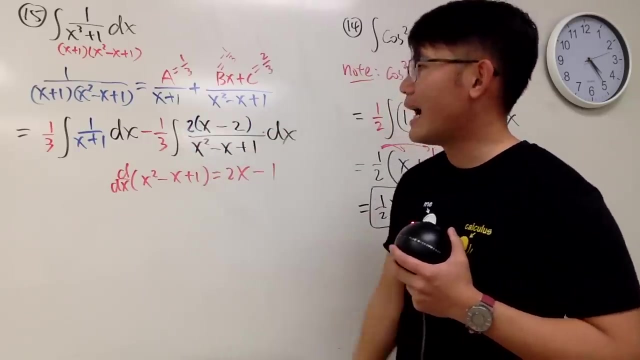 x minus 2 over x squared minus x plus 1.. This is serious. now I want to have a 2x minus 1 on the top to help me out. This is how Well I'm going to multiply the top by. 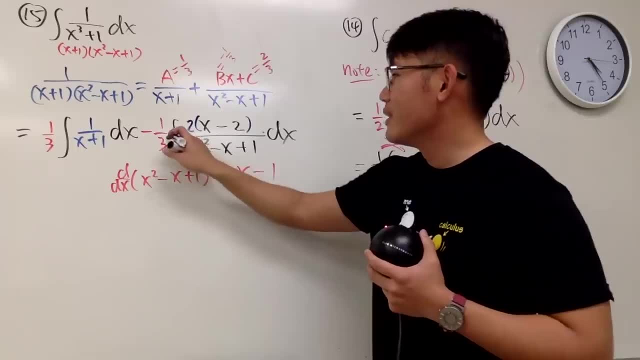 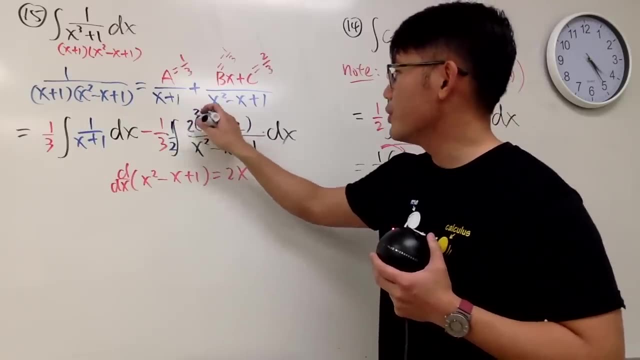 2. Of course, if I do that, change the whole thing, it's okay. I can just divide the 2 in the front like that. So that's still legit And if you look at this right here, it's going to be. 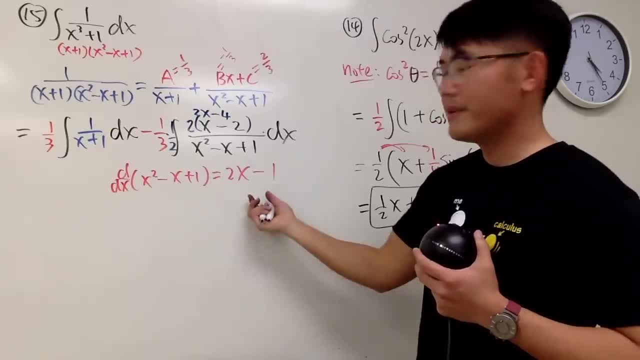 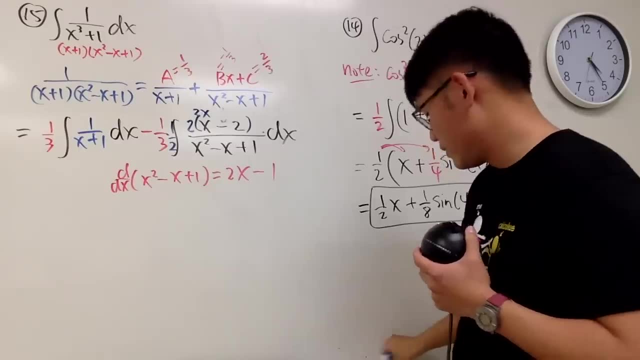 2x minus 4, right, But I want to see a 2x minus 1.. So it's okay, though, We can just look at this as 2x minus 1 and then minus 3, like that. 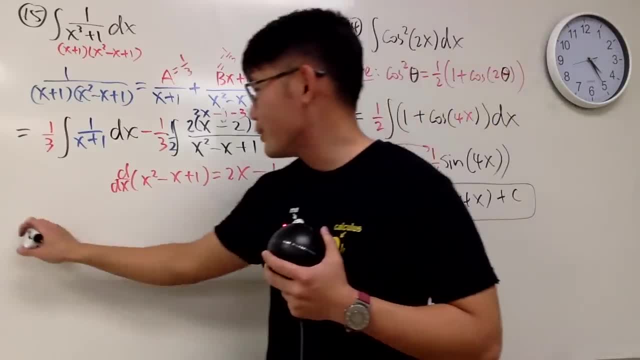 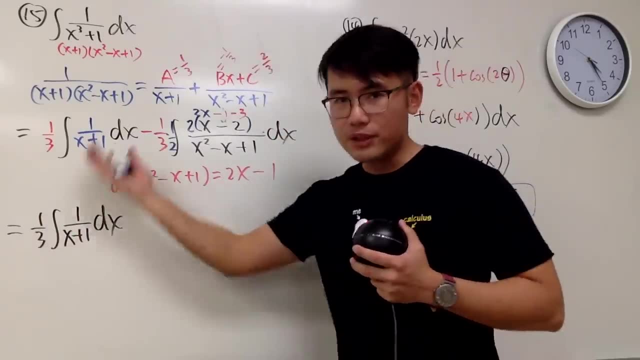 And there's the reason why I want to do this. So let's see, I'm not going to integrate this yet, I'm just going to write this down again and I will do all the integration at the very end. The first one stays the same. 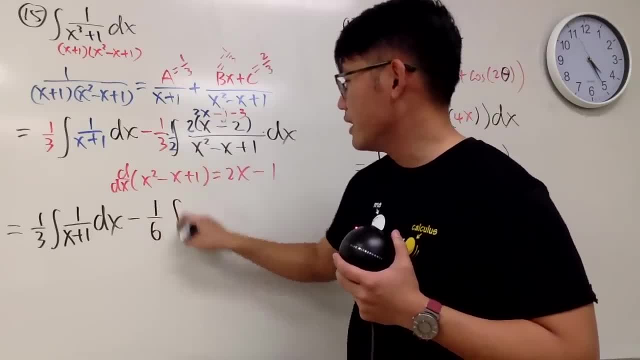 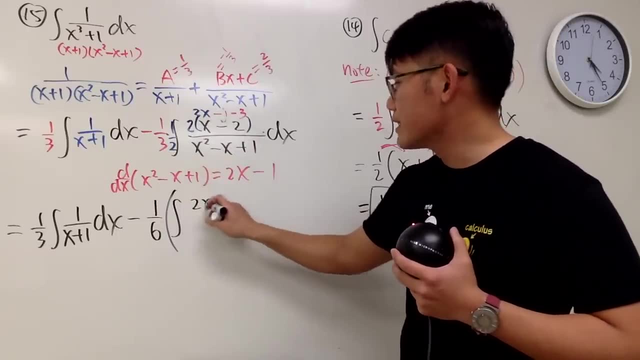 and then the next one will have minus. When you multiply, you get 1 over 6.. Integral- I'll put parentheses. Here's the deal. I will pair this with this denominator, which is 2x minus 1 over x, squared minus x plus 1.. 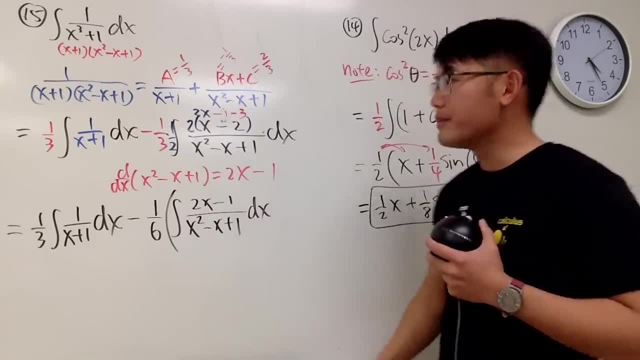 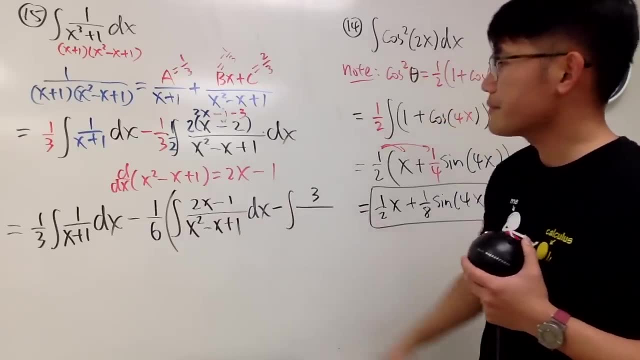 And I will close that. And then I am going to minus. this is still minus inside, okay, So I'm going to minus the integral 3 over. here's the deal. In order for me to do this, I will have to compute the square for that. 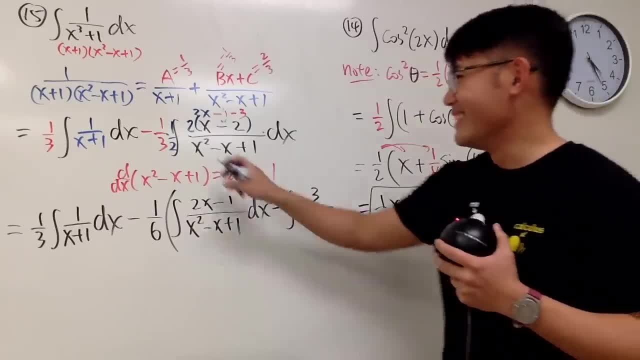 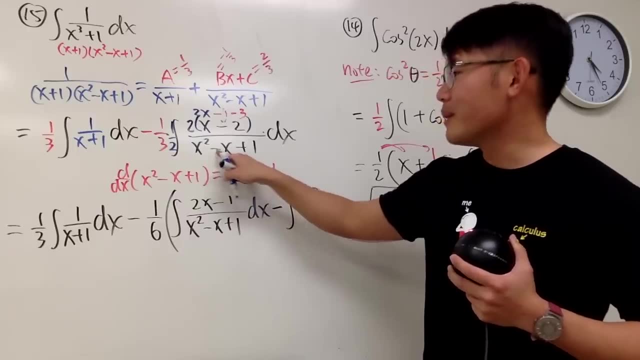 So let's see What's this? Complete the square for this. I wish to have minus 2, right, So I will have to minus 2 here, minus another x here and then plus x. What did I say? 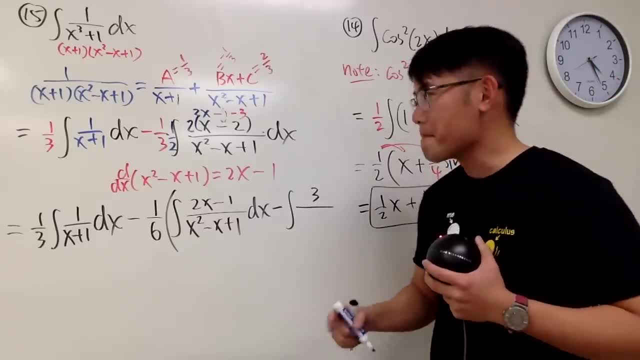 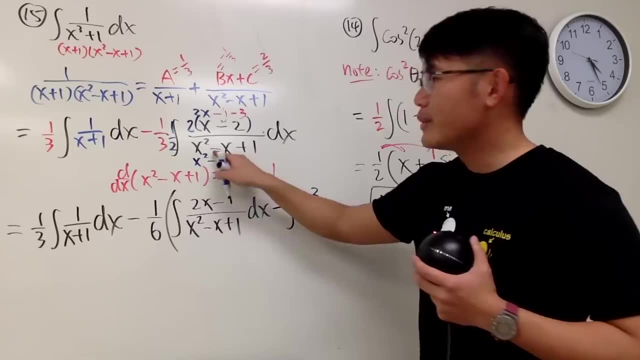 No, no, no, no, no. I cannot do that. That's the force power situation. Okay, here's the deal: x squared minus x To complete the square right here, I look at half of the, yeah, half of the coefficient of x. 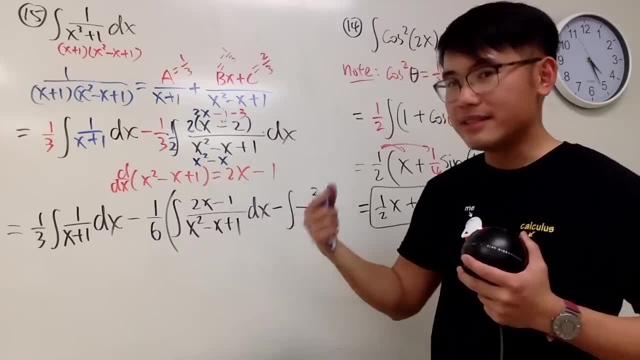 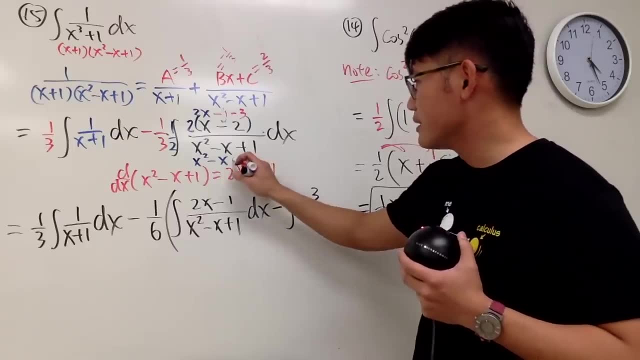 which is negative 1.. And half of that is negative 1, half. You are going to square that and that's the magic number. So I will look at this as plus 1 over 4, right, But originally I have 1,. 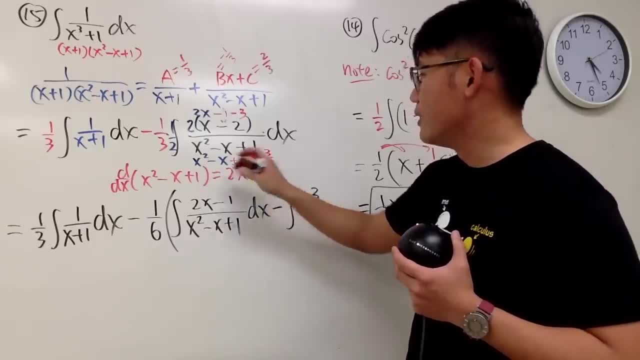 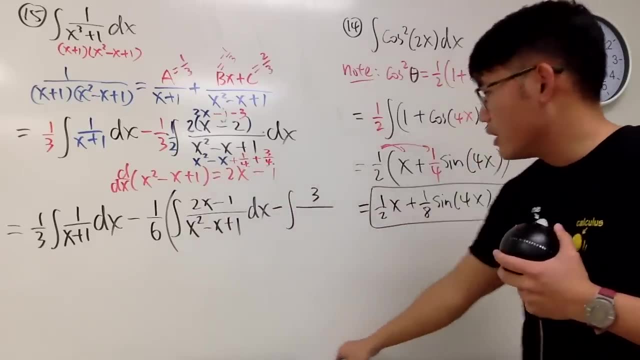 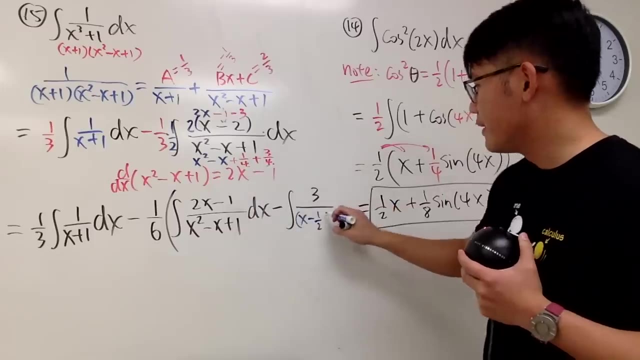 so I need plus 3 over 4.. And, as I said, this, and that is still the same, And this, this, that will give us a perfect square. And the perfect square is going to be x minus 1 half square. 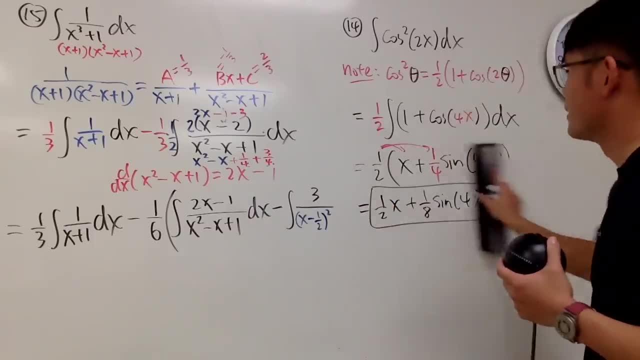 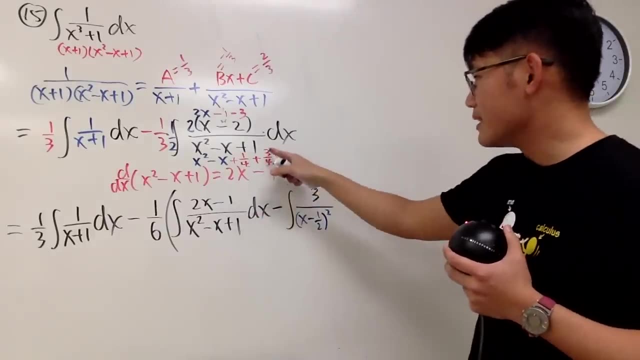 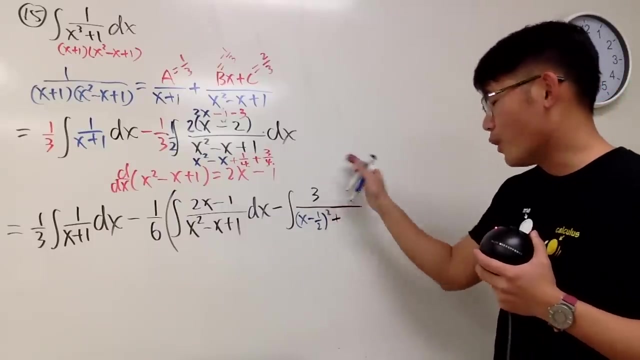 like that. Okay, And perhaps I'll erase this right here now because I don't need it, And right here we have plus 3 over 4, and this is what I will do. I will say plus. I need to look at this in the 1 over. 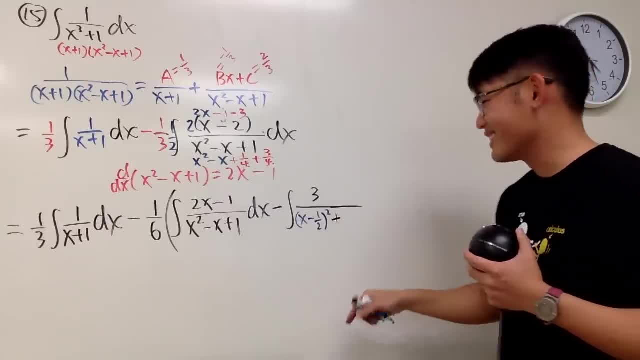 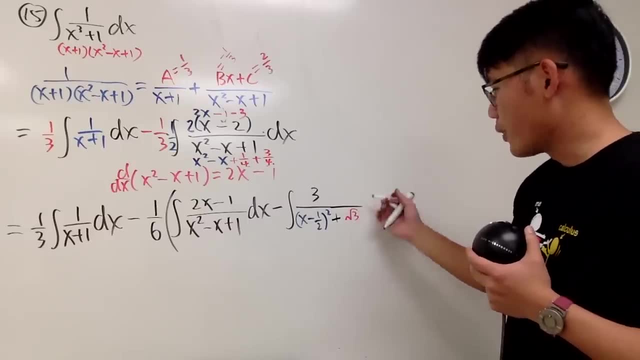 like u squared plus a squared, You can put a 3 in the front, So I'm going to look at this 3 over 4 as square root of 3, squared. but we also have the denominator, so let's put down this: 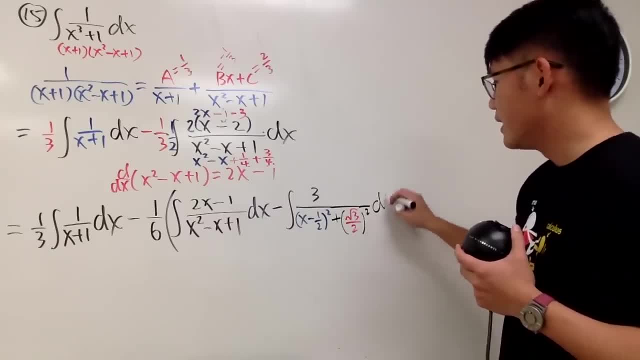 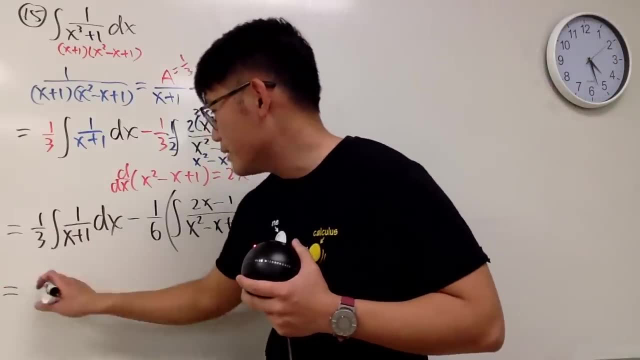 over 2, and then we'll have that being squared like that: dx, Whew, Yeah, Okay, Finally, let's integrate This right here: easy. 1, third natural log: absolute value of x plus 1. Done. 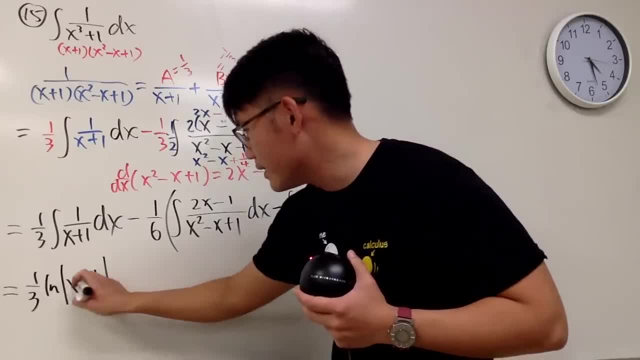 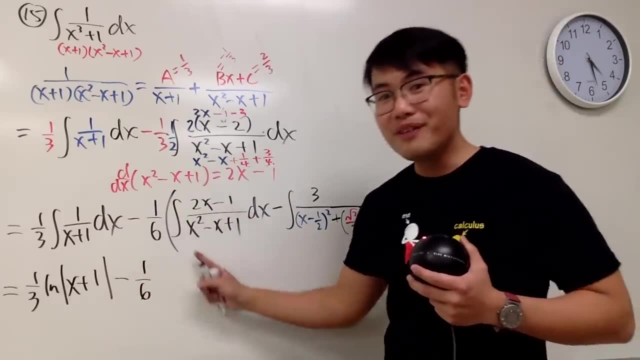 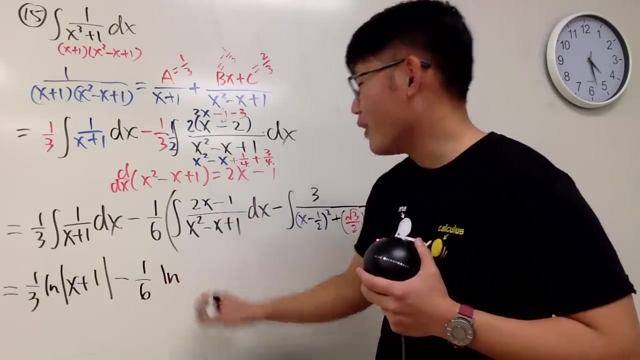 Right Done, But it's done better. Okay, Minus 1 over 6 times this. And the beauty of this is that the derivative of the bottom is exactly on the top. So this right here will give us precisely natural log of the denominator. 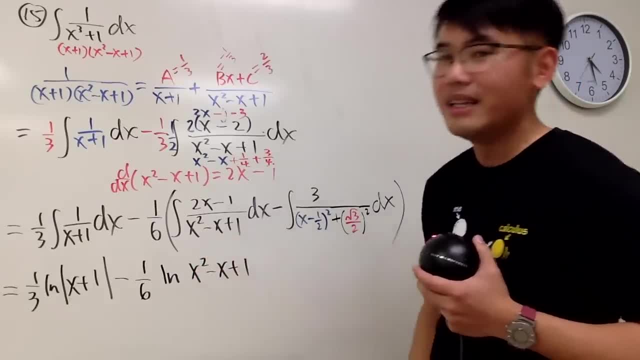 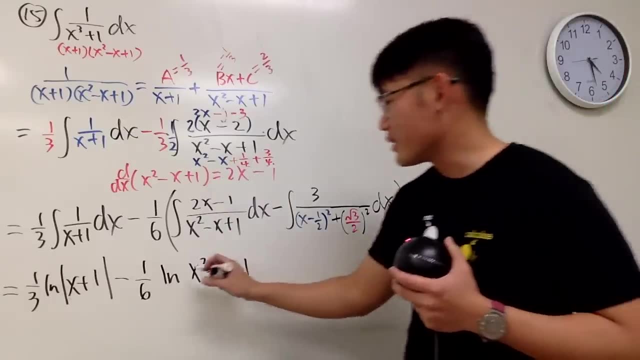 which is x squared minus x plus 1.. And the truth is, if you see the denominator, which you can complete a square right here, you're always going to get positive. So, in other words, you can just put down parentheses for this. 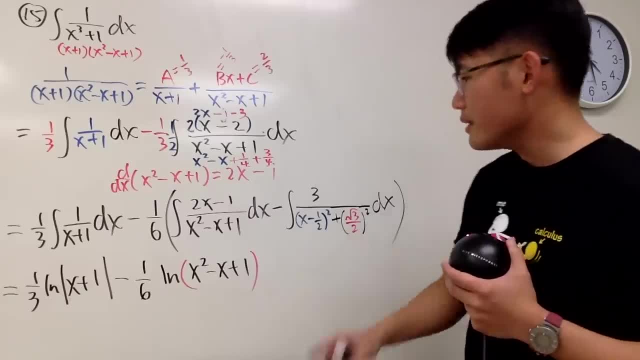 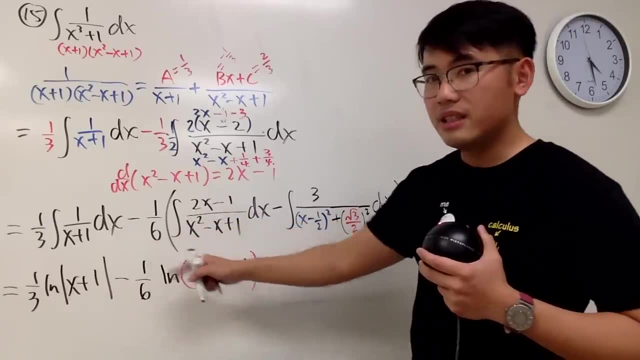 And I put 1 over 6 times this already. so we are good. Now negative times. negative will give us positive. And then 3 over 6 is 1 half Okay, So this is 3 over 6.. 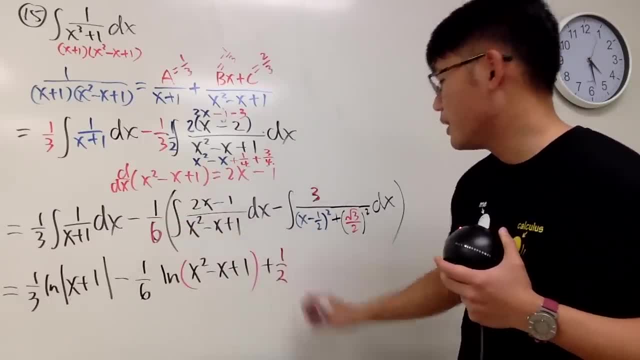 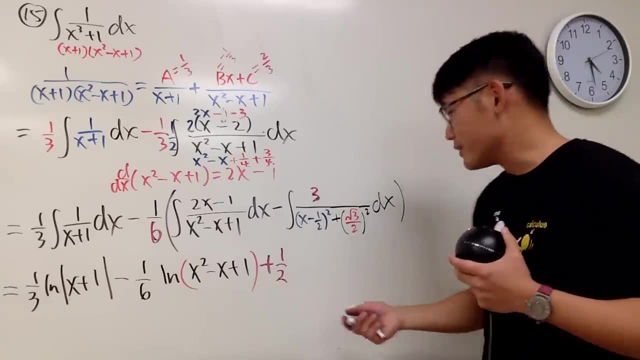 That's how we get 1 half Okay And of course, negative times. negative is positive. Here is a small trouble part. You're going to end up with the inverse tangent part, So you are going to do the reciprocal of this first. 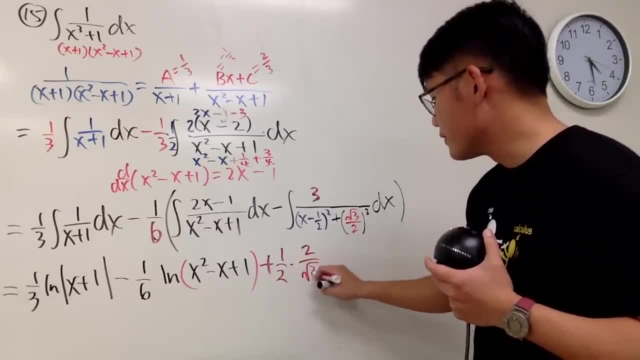 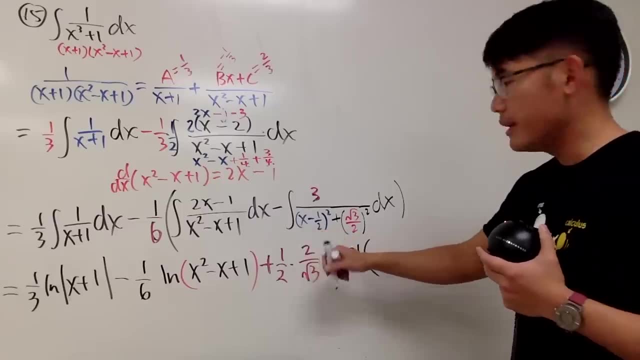 Namely, you multiply it by over square root of 3, and then the inverse tangent And the input is going to be this as your u, And thank god, the derivative of this is just going to be 1,. so that's good. 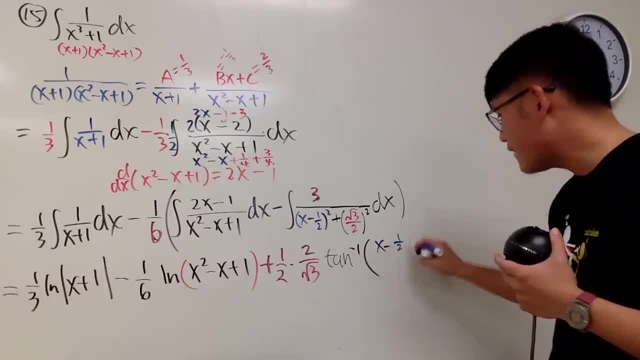 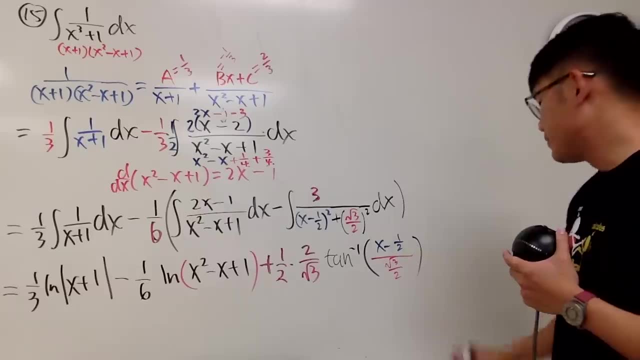 So you put this down, which is x minus 1 half, And then you divide it by this guy, which is the square root of 3 over 2, like this. That's pretty much it, But I will simplify this a little bit for you guys. 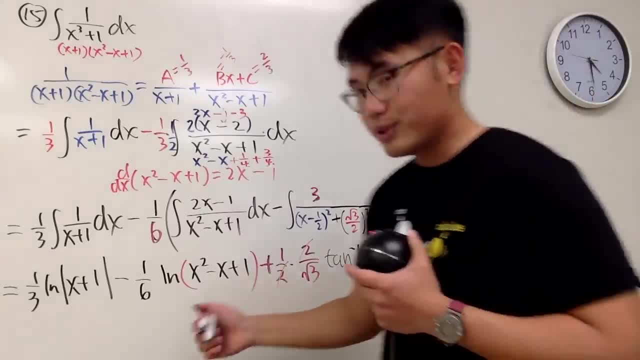 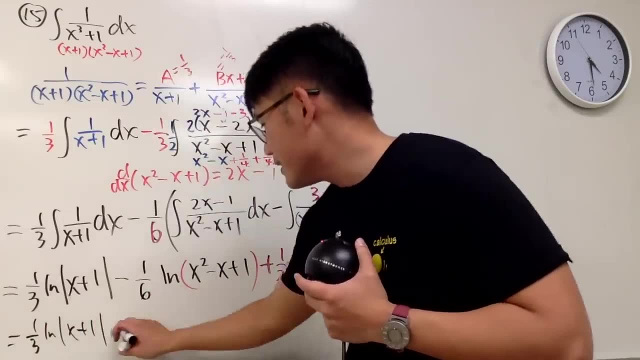 Alright, So we have just 1 over square root of 3 right here, So I will just write this down again. Here we have it: 1 third natural log: absolute value of x plus 1 minus 1 over 6 natural log parentheses: x squared minus x plus 1.. 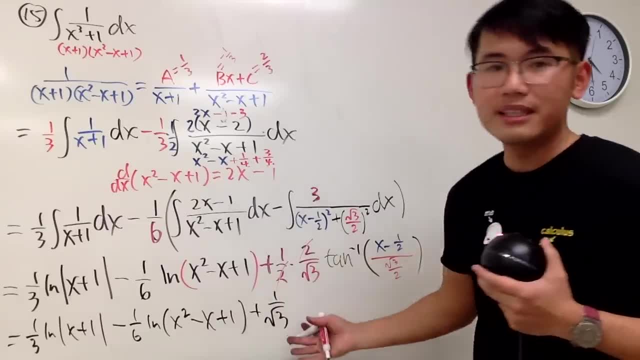 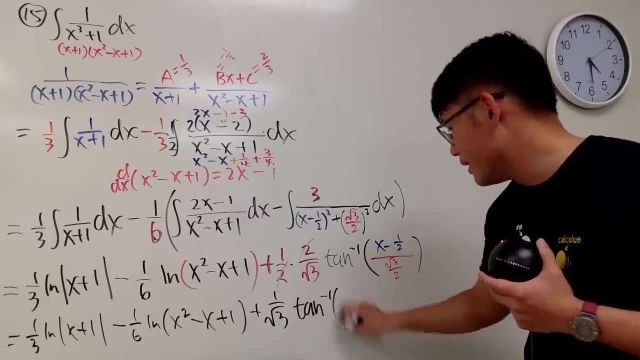 This right here, plus 1 over square root of 3, like this: Okay, so let's just write it down like this: okay, Inverse tangent, and I'll put this as the reciprocal, namely 2 over square root of 3.. 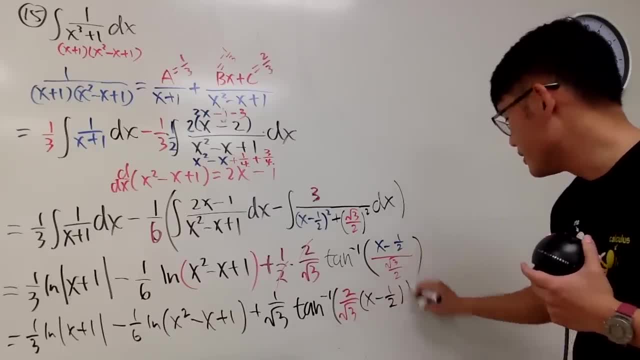 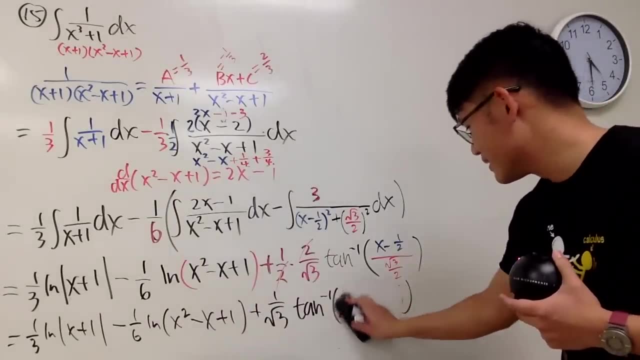 We're okay with this. I'm not going to distribute it. please don't make me distribute this. You can, but let's just do it. So you have this times x, right? So you have this times x. you have the 2 over square root of 3 times x. 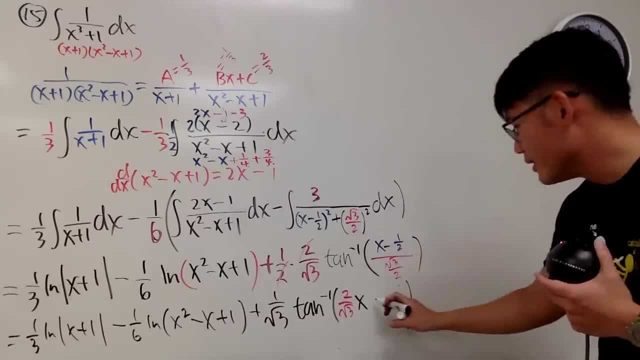 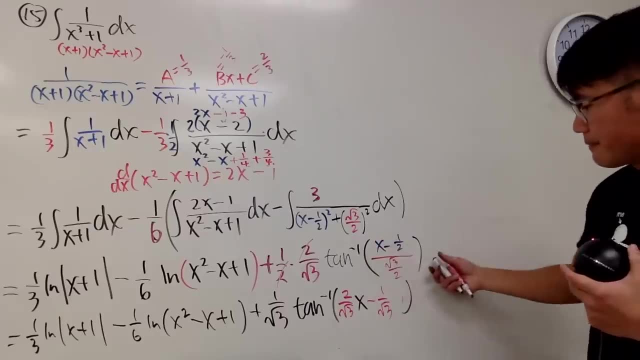 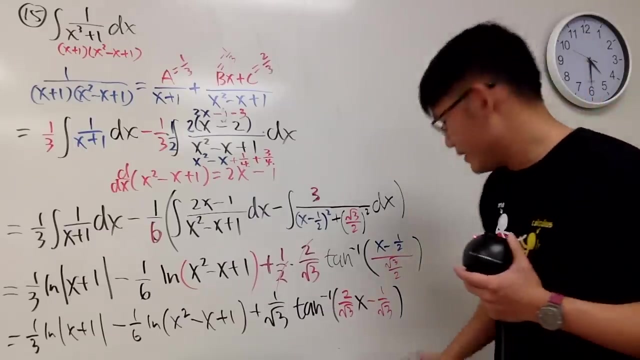 and then the 2, and that 2 will cancel each other out, so you will have minus 1 over square root of 3, like that. Yes, I think this is correct. All right, We're done. Don't forget to put a plus C. 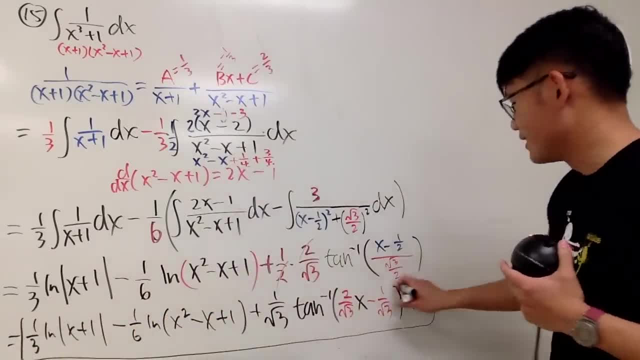 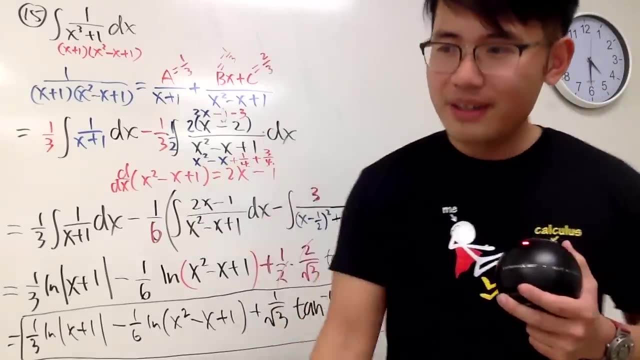 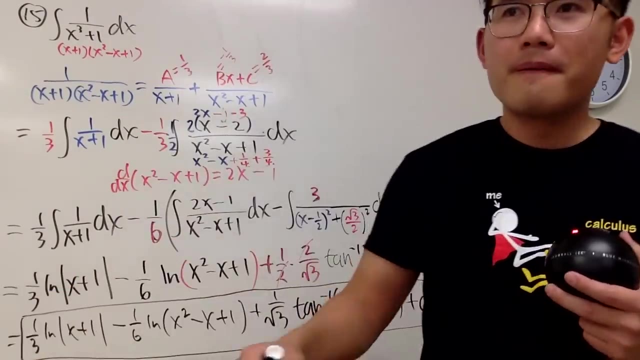 If you don't put a plus C, that will suck. So don't forget to do that. Don't forget to do that. Well, that was a long one. It's been an hour, So I deserve a sip of coffee. This is crazy. 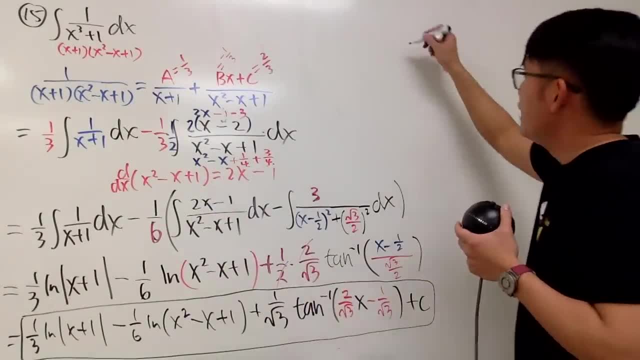 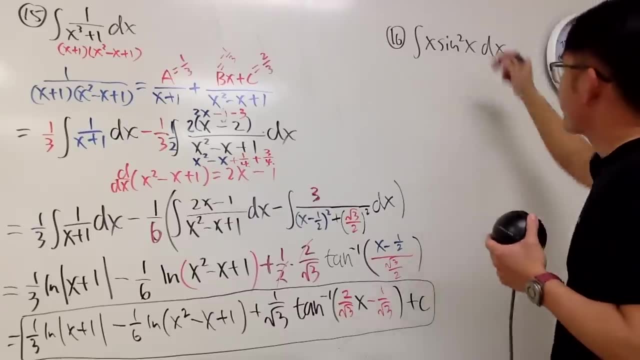 Yeah, I don't think that was just a tough one. Anyway, number 16, I'm going to speed up a little bit: Integral of x times sine squared x, dx. Well, well, when you see this, we can use the pole reduction formula. 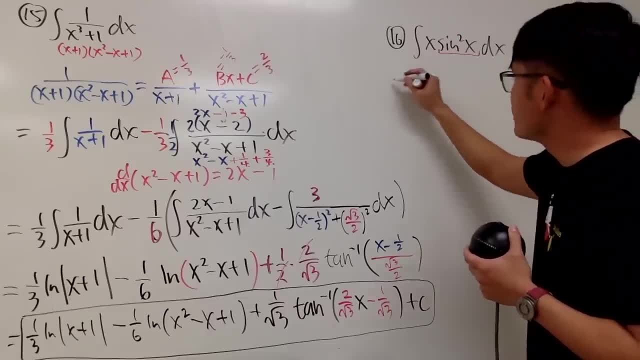 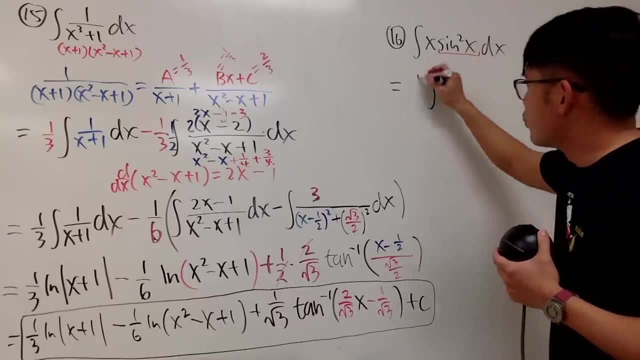 and x times that right. So what I'm going to do is I'm going to look at this as integral of x and x. I mean sine squared. x is the same as 1 half times 1 minus cosine of 2x. 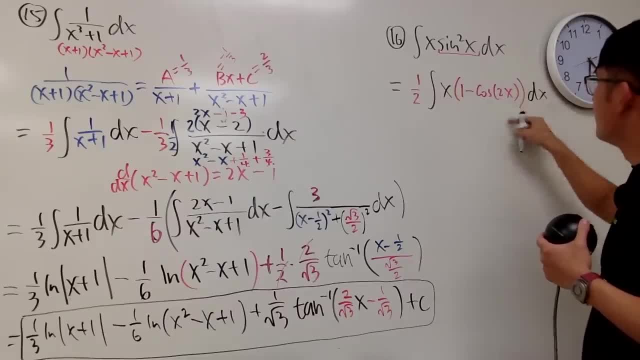 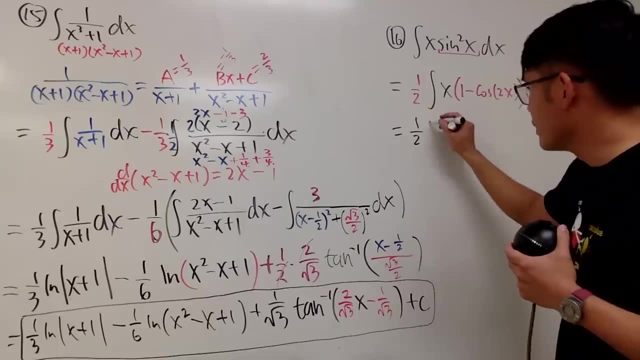 like this. So reduce the power, And then, of course, you can just distribute this a little bit. So this is 1 half all the way in the front and we have the integral. The first one is just x in the x world. 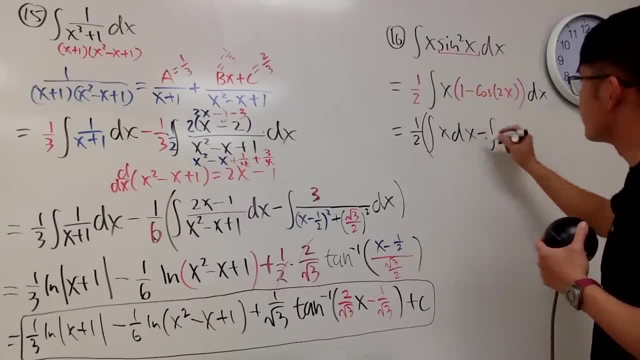 And for the second one, we have to minus the integral. And actually let me put it down like this: We're going to plus, okay, I'll put a negative inside, And then, of course, next times that. so it's x times this guy. 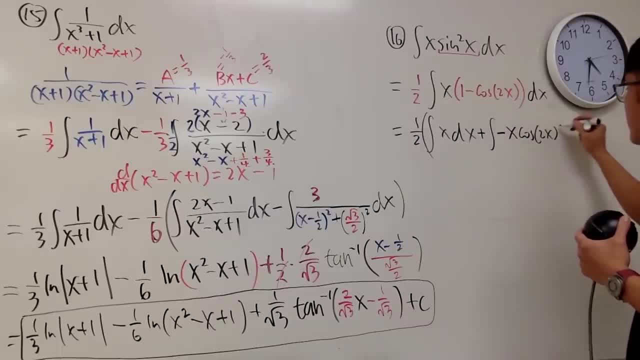 which is cosine of 2x, like this dx. Okay, So here is the deal. I will do this one in blue for you guys. Right, I'll do this one in blue. To do this, we will have to use integration by parts. 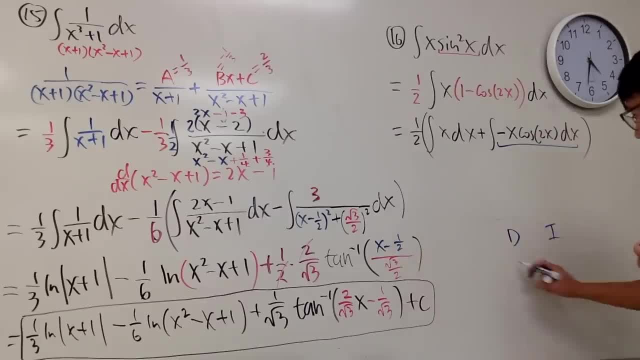 Of course we will do the DI setup right. DI method: Plus minus, plus on the side to get ready. I will be differentiating negative x Right. If you put a negative x, this is easier setup And I'll be integrating. 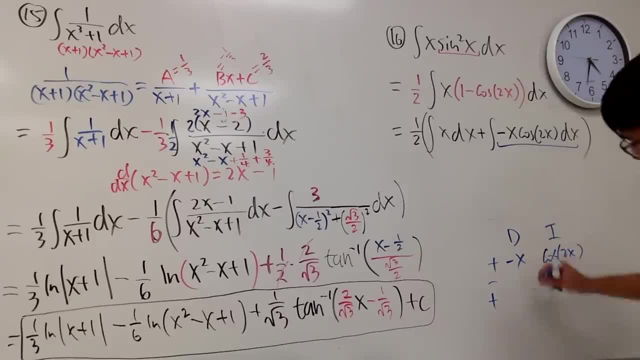 cosine of 2x. like this: Integrating negative x, you get negative 1.. Integrating negative 1, you get 0. So you are done. I mean differentiating, Okay, Differentiating negative x, you get negative 1.. 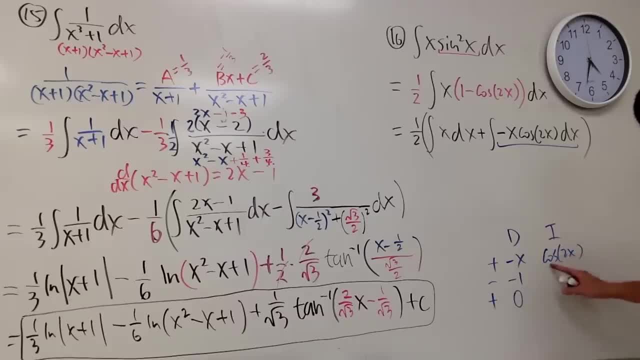 And differentiate this again, you get 0.. So you are done Now integrating cosine of 2x. First, you end up with positive sine of 2x, But don't forget to divide it by 2.. And then: 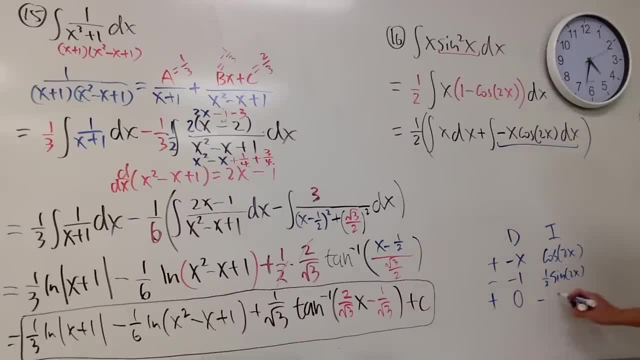 when you do it again, the integral of sine is negative cosine and then the input state is the same. But don't forget to divide it by 2 again, so you have 1 over 4.. So you pretty much have it. 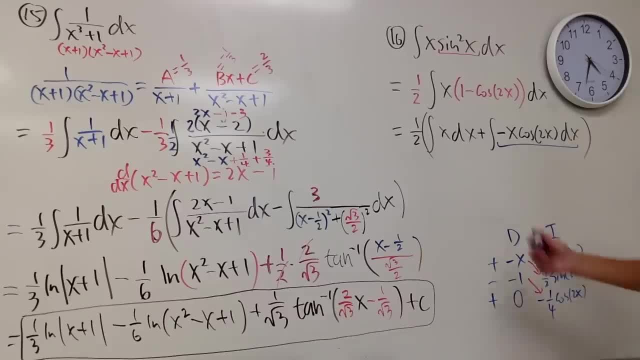 Now let's see. I'm going to just multiply this and that, So we'll see what the answer is. Perhaps we have the 1 half times this, So I will just write down: 1 half Integral of that is: 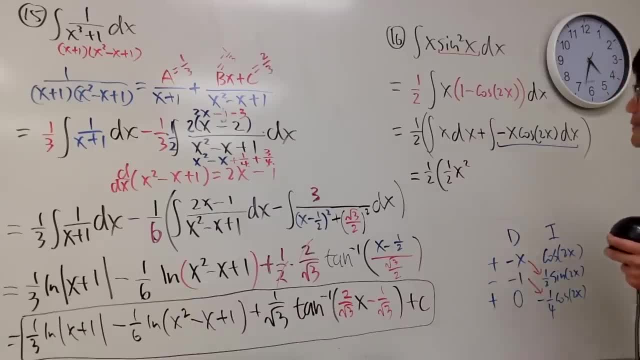 1 half x square Right. Don't forget that. Now, for all this, it's just this this time, So I will put this down in blue for you guys. Okay, So here we have negative 1 half x times sine of 2x. 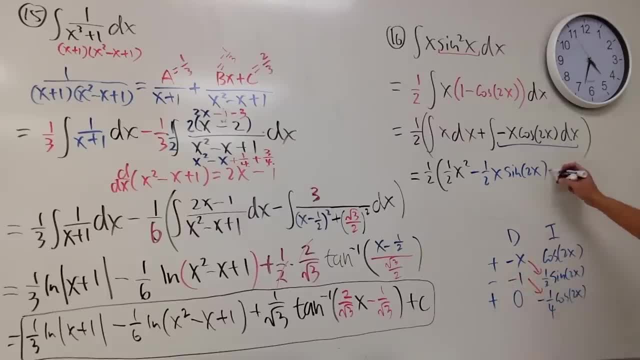 Yes, And then negative, negative, negative. So it's still a negative, I believe. so, Yes, And then 1 over 4, cosine of 2x, Like that. Okay, Let's double check, It's correct. 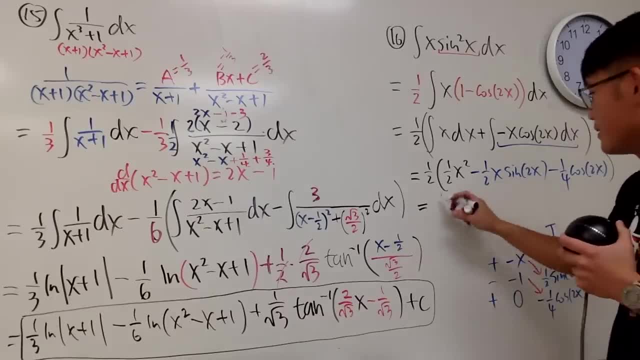 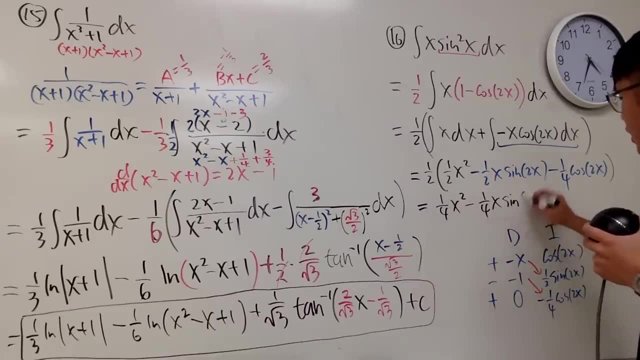 Okay, So we are done. Distribute the 1 half, just to be polite, you know. So you have 1 over 4 x, square This times. that is minus 1 over 4 x, And then sine of 2x. 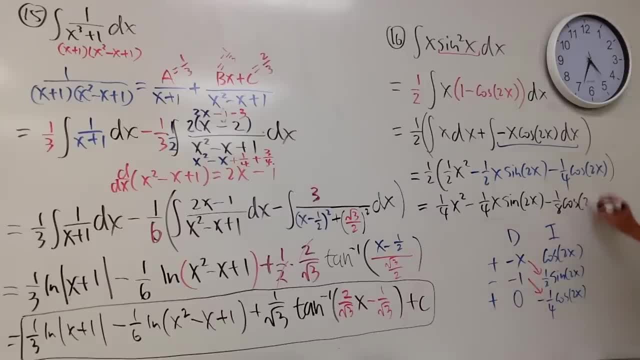 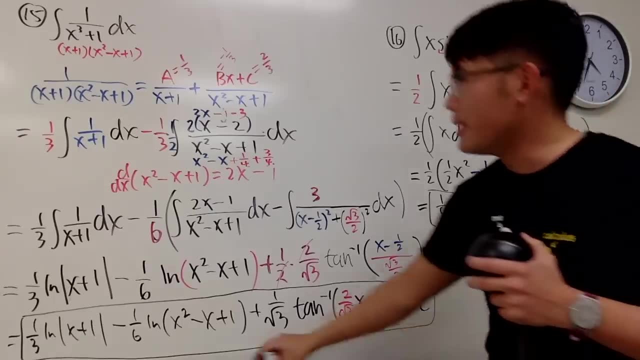 And then this times that is negative, 1 over 8, cosine of 2x, Like that, And then in the end you put plus C And here you have it. This is your answer. It's not that bad. 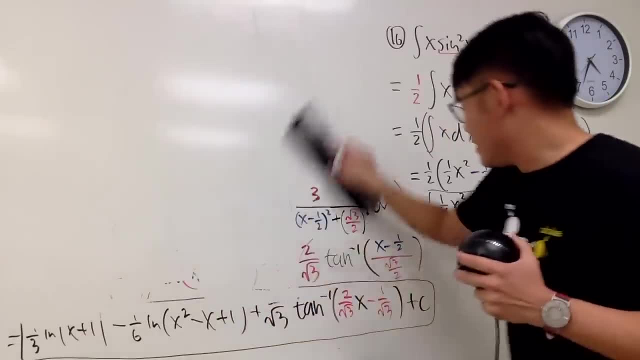 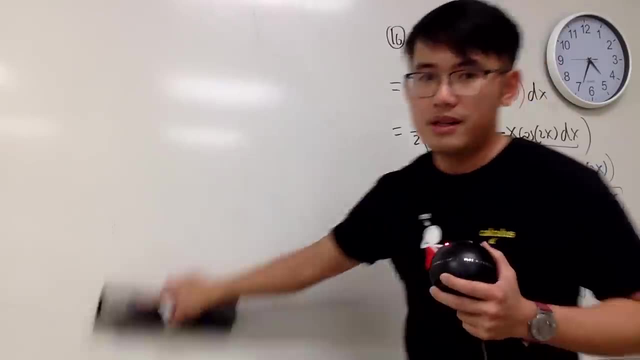 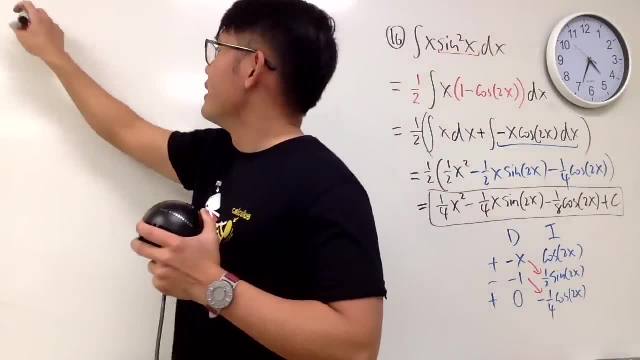 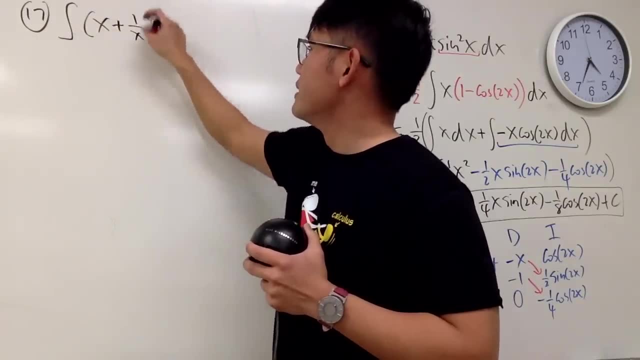 a nice one, Number 17. Integral of parentheses, And we have x plus 1 over x square dx. Don't do use of, You don't need to, Because you can just expand this. It's nice, So you are just integrating. 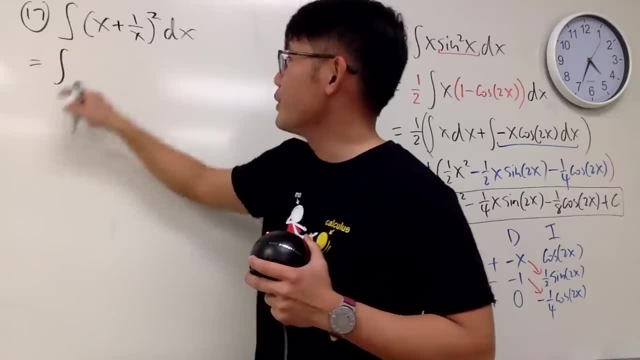 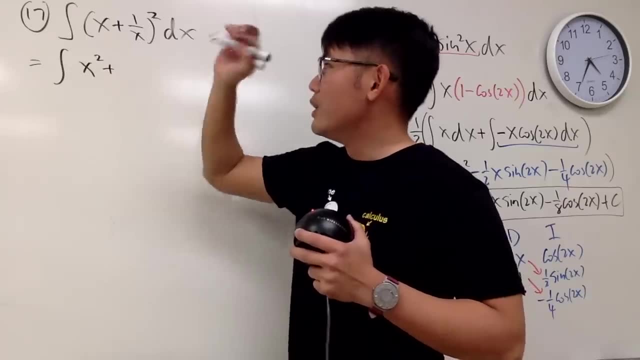 Your binomials was expanded, So you get 1 over 4 cosine and you expand it So you get x square, And then you are going to add 2 times this and that, which is nicely equal to 1.. 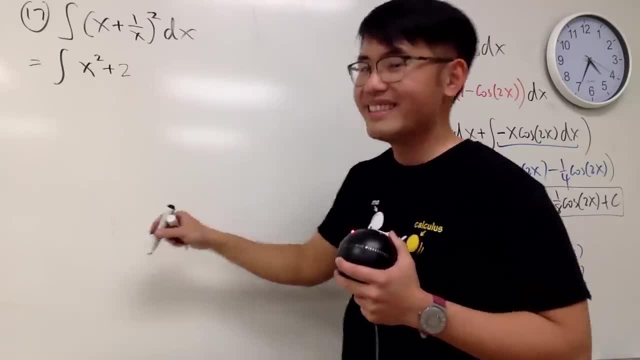 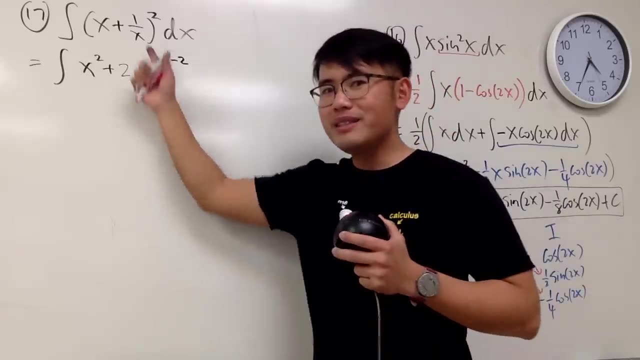 So you just add 1.. I mean 2 times 1, like this, And then this square, which is the same as plus x to negative 2.. And did we see this kind of thing earlier? Yes, we did. 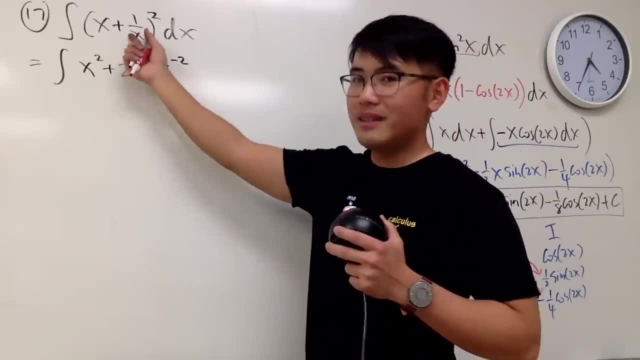 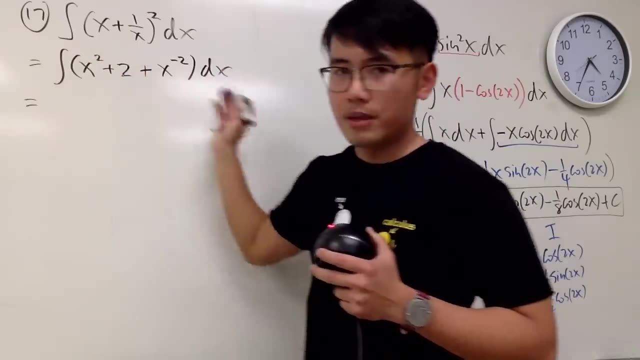 Back in question 3. We used this to factor to get that Right. So you expand it this time, So you get 1 over x and then we can just integrate this term by term. You get 1 third x, cube. 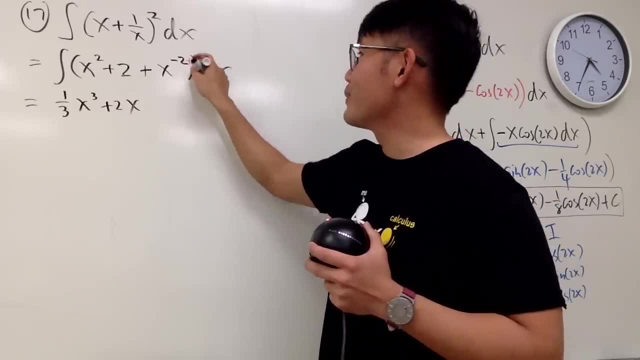 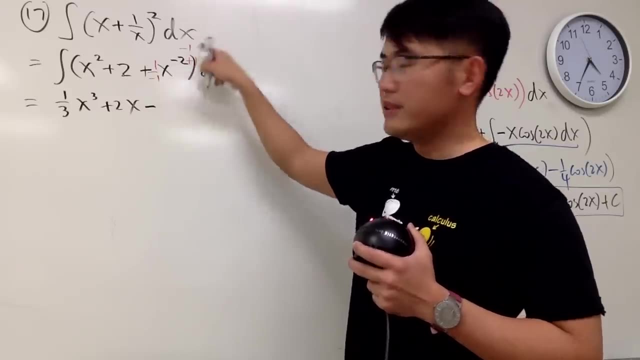 and plus 2x. This right here, it wasn't a natural log situation. You have to add 1 to the power. You get negative 1 and then divide it by the new power. So you have minus x to the 1. 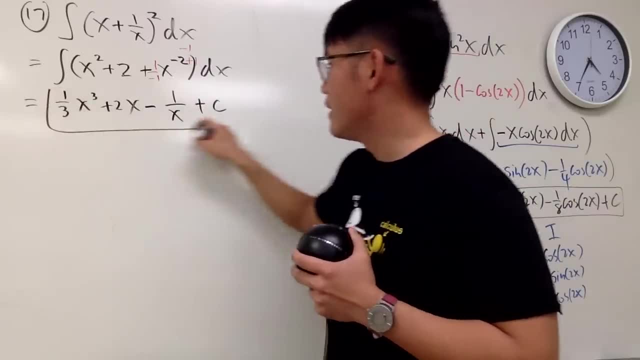 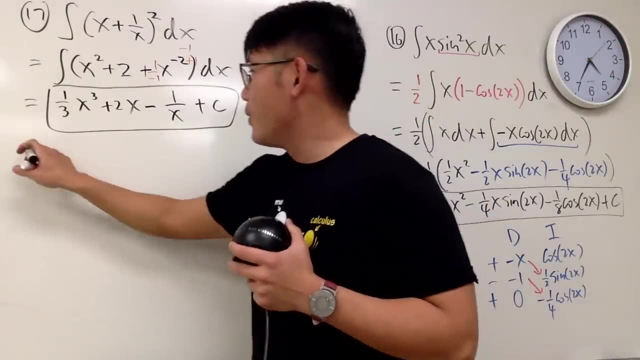 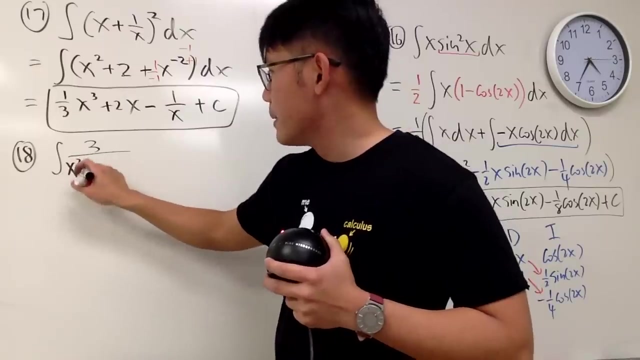 x to the negative 1 power. In other words, 1 over x, and you're done. Plus c. Nice and clean. Okay, Number 18.. We have the integral of 3 over x squared plus 4x plus 29. 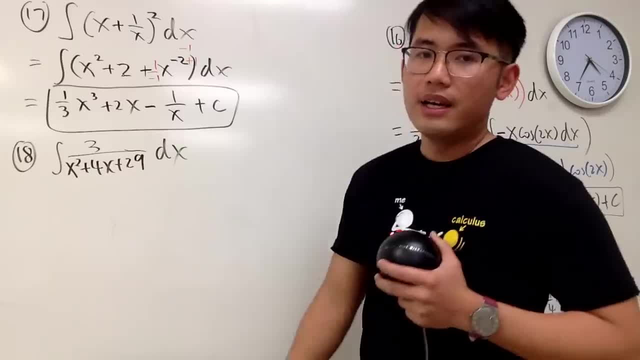 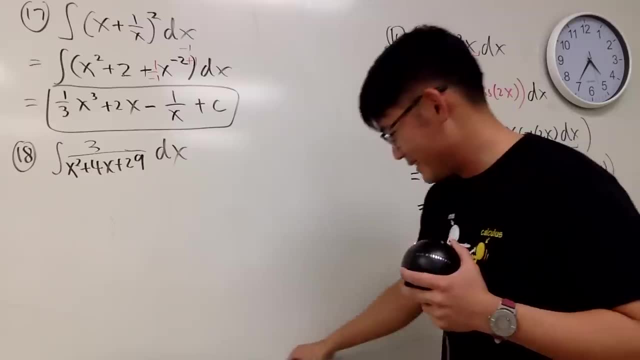 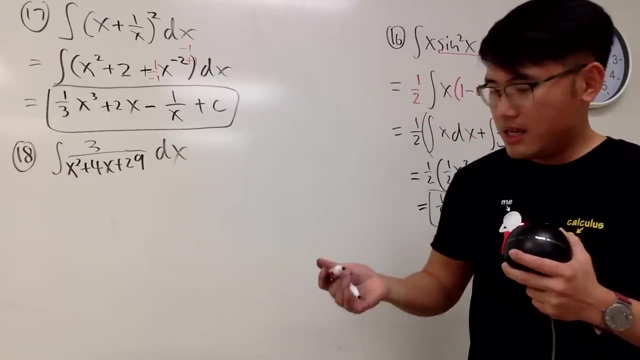 dx. Well, here is the deal. Just want to make sure that I close the markers because they are going to be with me for the next- I don't know- 4 or 5 hours. Can we factor the denominator Yes? 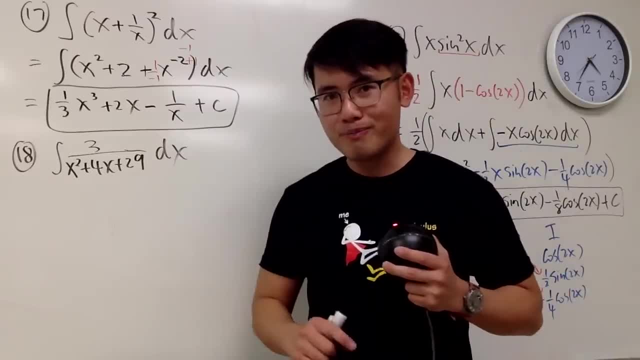 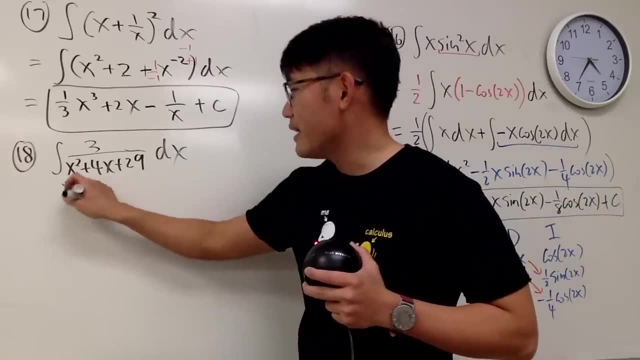 we can. Can we factor the denominator, Say no, Thank you. But can we complete a square, Say yes, Thank you? This, right here, is the same as saying x squared plus 4x plus 4 and then plus 5,. 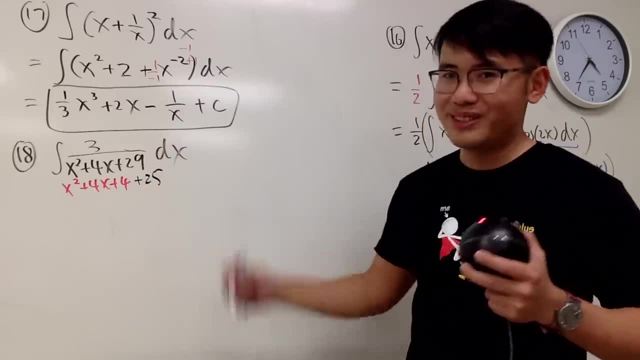 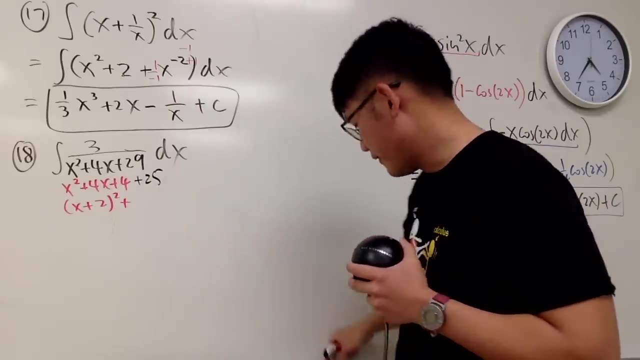 isn't it? Let me not 5, plus 25, which is, you know, 5 squared. So this right here is just x plus 2 squared, plus we can look at this as 5 squared, as I mentioned it earlier. 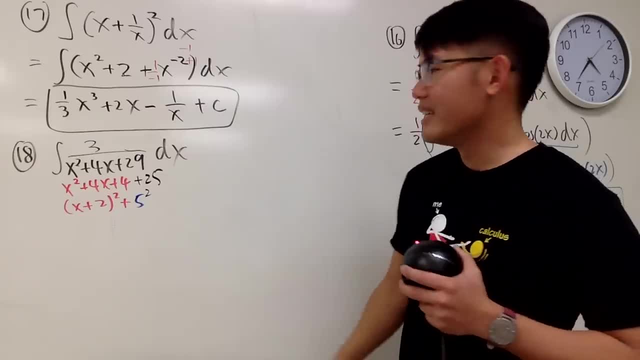 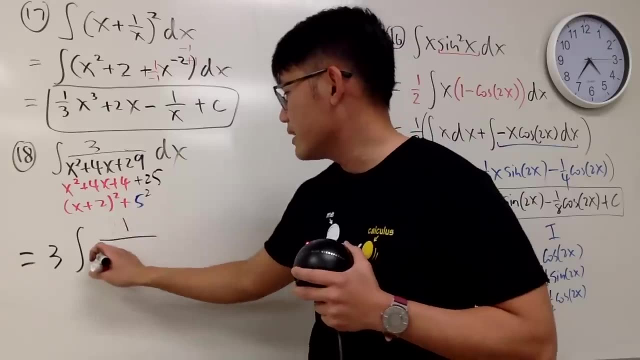 Like that, Like that, Very nice. So, in another word, we can do the following: I will put a 3 in the front and we will look at this as integral: 1 over, as I said, the x plus 2. 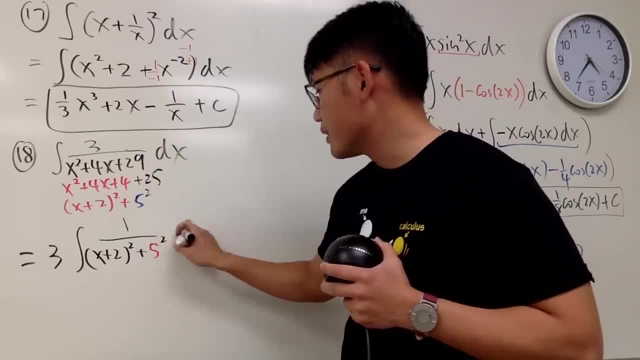 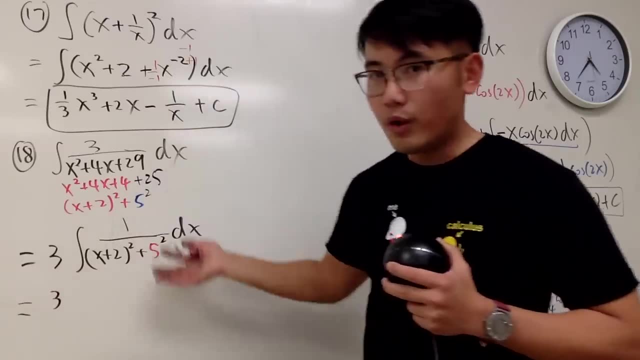 squared, and then we add the 5 squared dx, And this is the inverse tangent situation, and we end up with 3 times the 1 over 5, which I can just put it as 3 over 5 here, and then we do the. 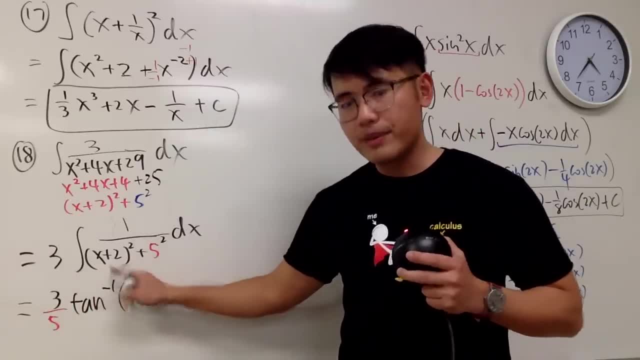 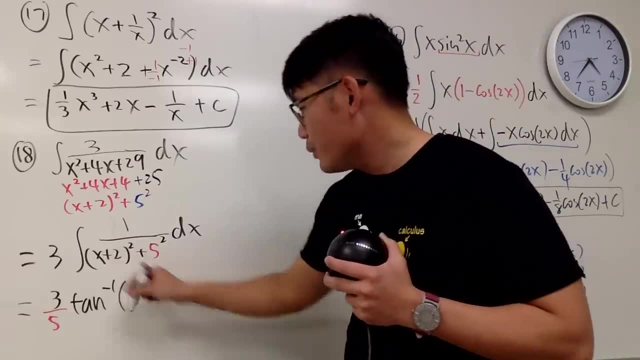 inverse tangent of this being our input. Technically, we should take a u to be x plus 2, but du will be the same as dx, so that's nice. Anyway, we are going to have x plus 2 right here, but don't forget. 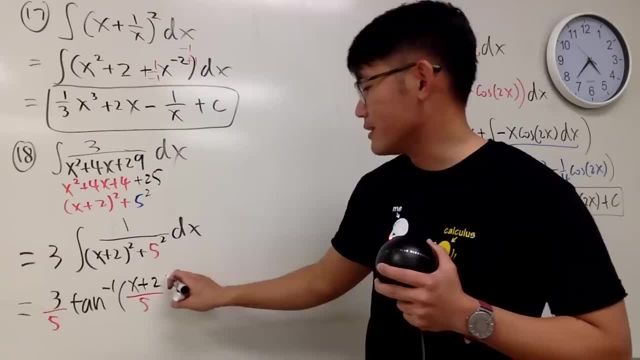 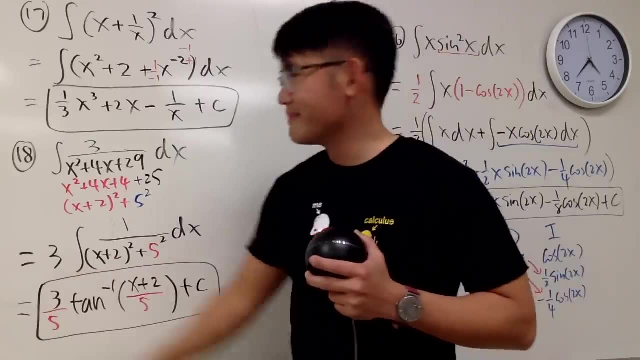 to divide it by 5.. Right, The formula says so. This input divided by that number, and you are done plus c, This is number 18.. Okay, Number 19.. Let me put number 19 in here. Next one: 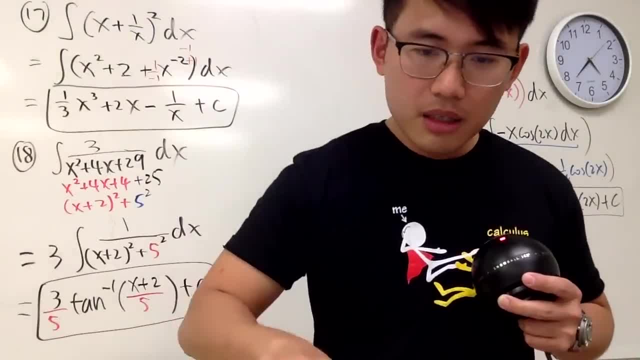 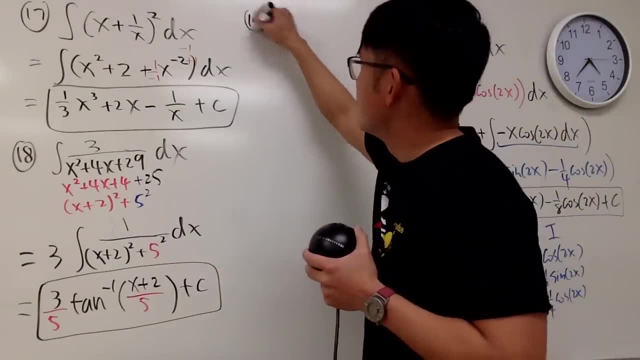 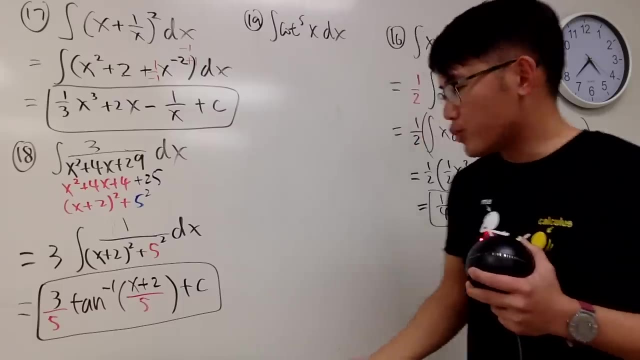 Cotangent to the 5th power. Oh my god. Let's see Number 19.. Let me see if I can fit in here. Integral of cotangent to the 5th power. x, dx. Some of you guys might want to try this. 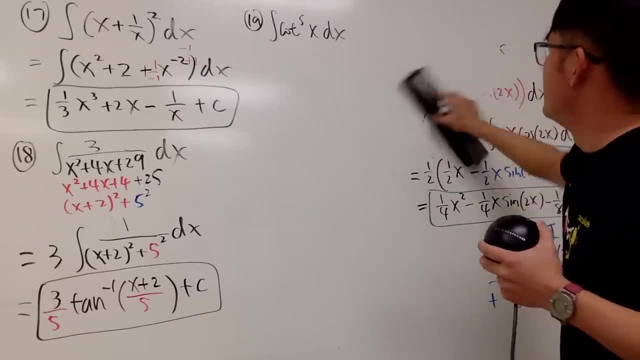 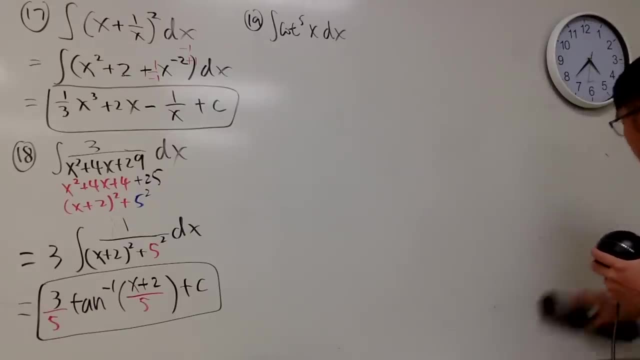 to use the cotangent and cosecant. That's okay, but you will have to know how to deal with the integral of cotangent to the 3rd power. So that's why you have to do more work for that. It's not ideal. 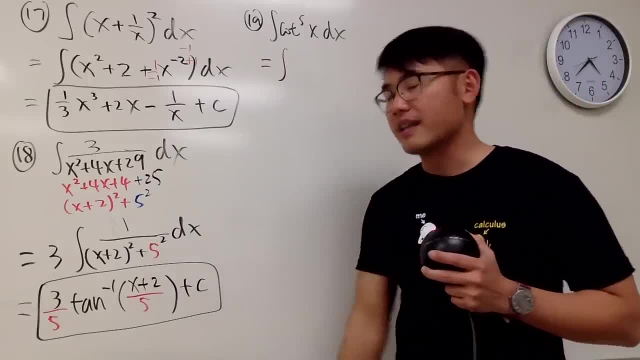 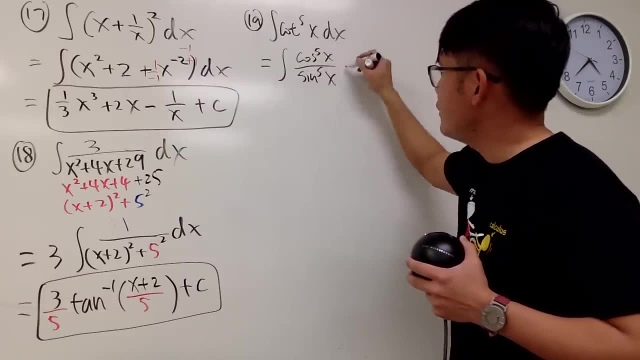 So what we will do is: we know cotangent is the same as cosine over sine, So I will look at this as cosine to the 5th power x over sine to the 5th power x. This is very nice. Well, odd numbers. 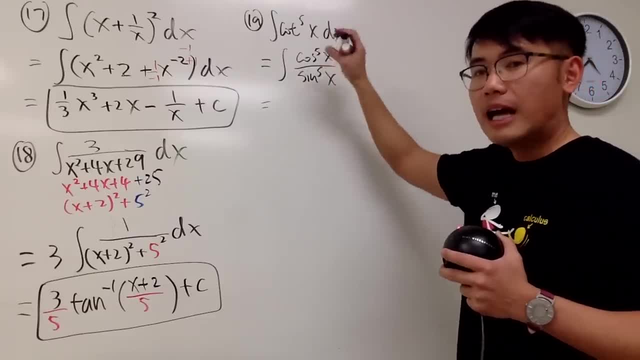 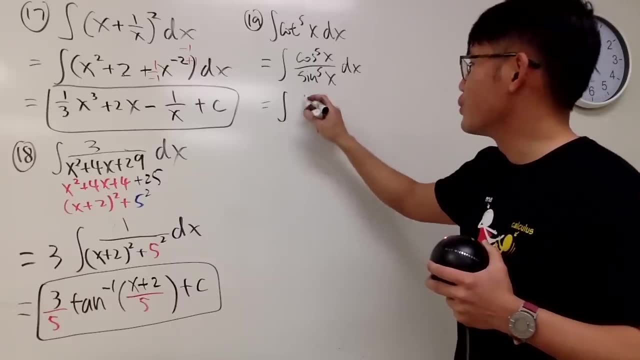 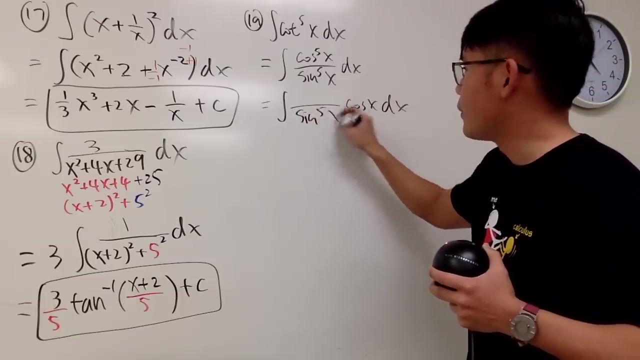 especially the top one. I want you will just take one out to save me for the u sub u c. Let's look at this as the integral of cosine to the 5th power, x. So I want to put down cosine x on the side. 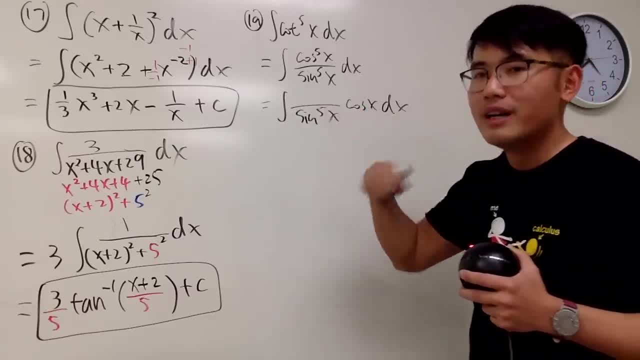 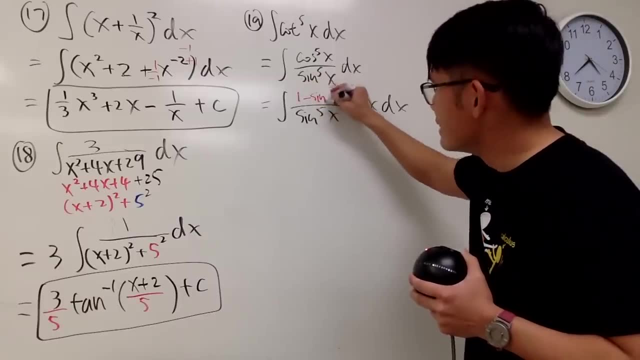 on the bottom. here we still have sine to the 5th power, x. This is going to give us cosine to the 4th power. in another word, cosine squared and squared. and cosine squared is the same as 1 minus sine squared x. and then 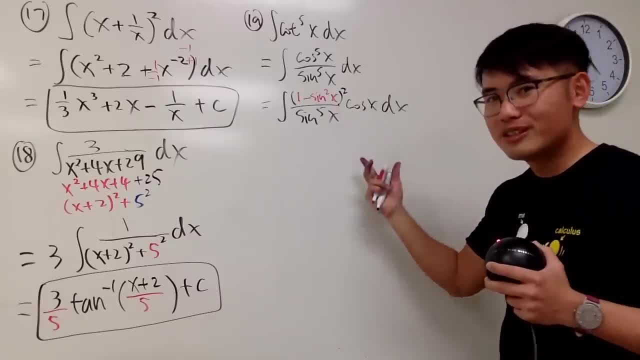 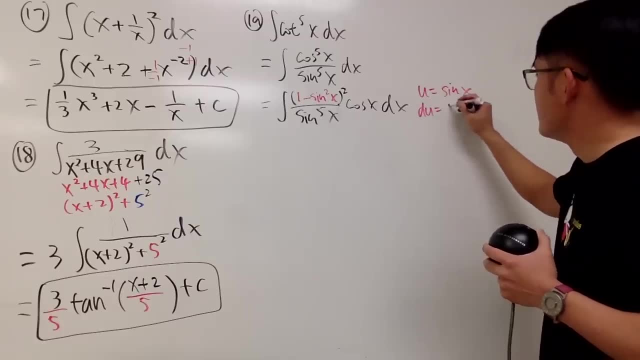 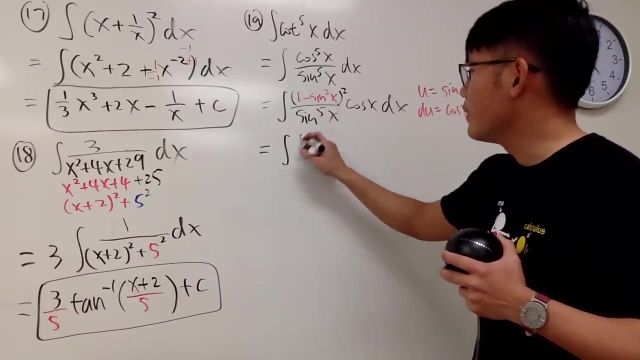 you square that, So they are still equivalent. And the beauty of doing so is we can take u sub sine x and du will be precisely cosine x, dx, So I can take this to the? u world right away. This is the integral of 1. 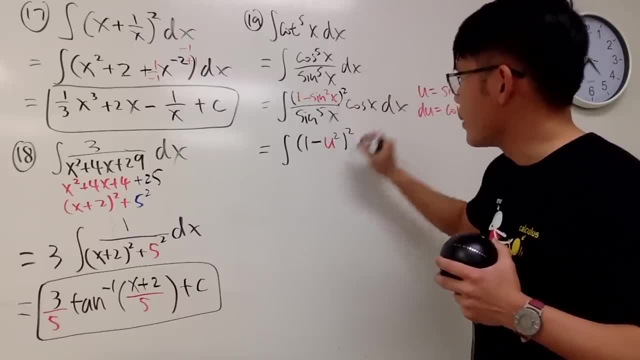 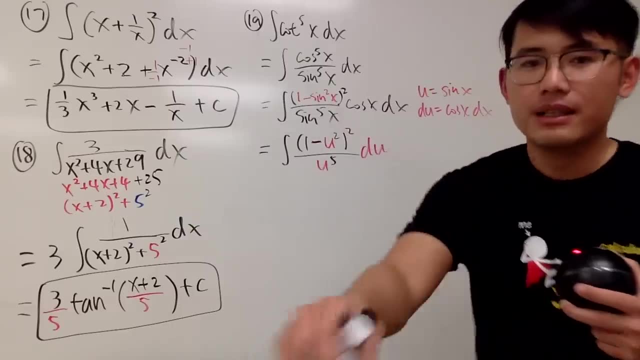 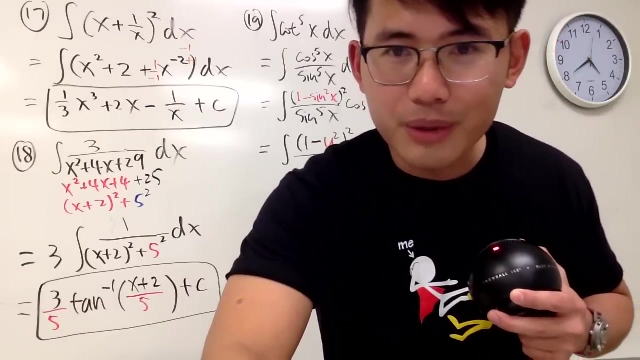 minus u squared and then squared over u to the 5th power, and this part is just du. Alright, So that's the deal. I forgot to send my laptop to sleep, so let me do that right now. Don't go to sleep. 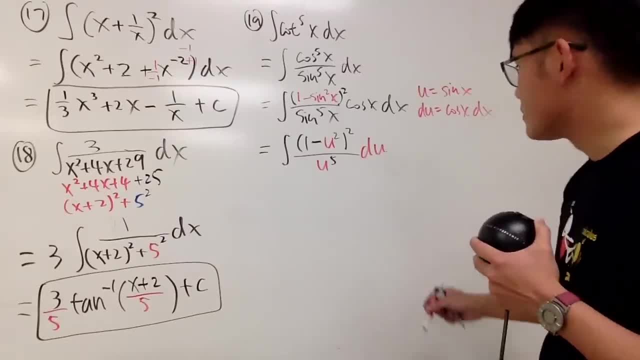 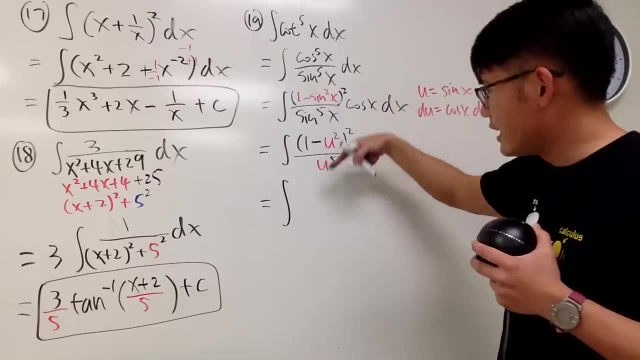 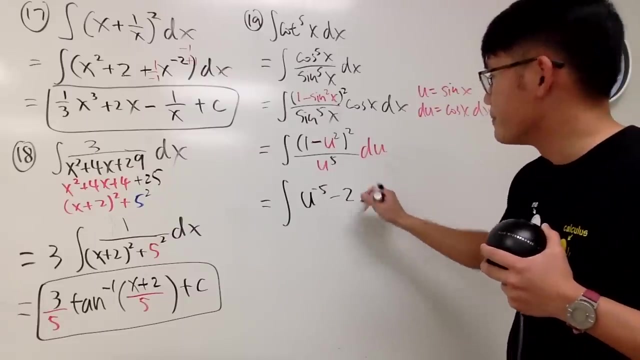 okay, Don't go to sleep. Okay, I'm not going to go to sleep neither. Now let's do this in our head: Integral Alright 1 squared divided by u to the 5, so you have u to the negative 5.. 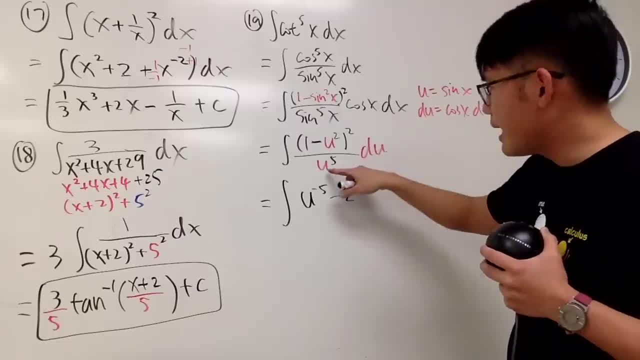 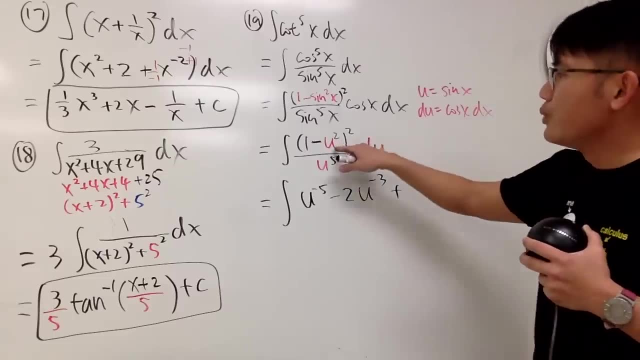 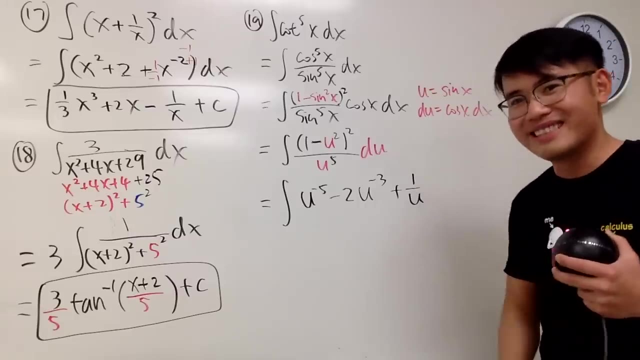 Next you have minus 2, plus u to the 5, so you have u to the negative 3.. Right, So far, so good. Lastly, you have, plus u to the 4th, power over u to the 5, which is just 1 over. 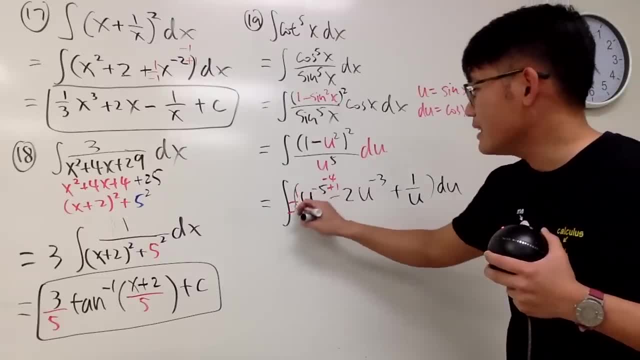 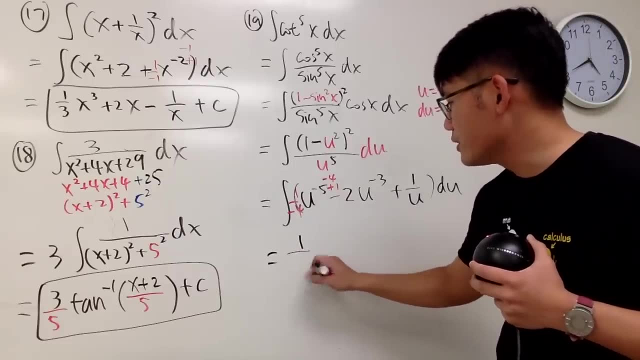 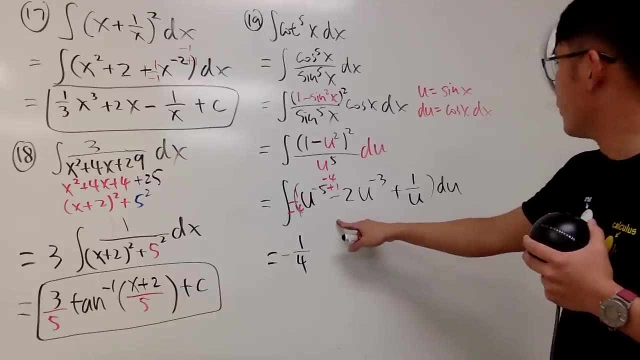 u. I want to write this down because you guys like the ln right. So u to the negative 4. so perhaps I'll put the negative in the front like this: and u to the negative 4. we can put u in the denominator, but notice. 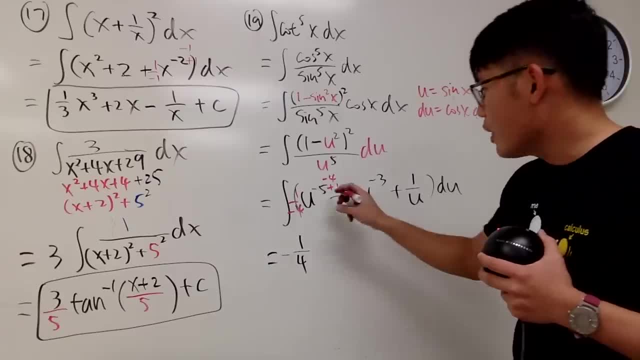 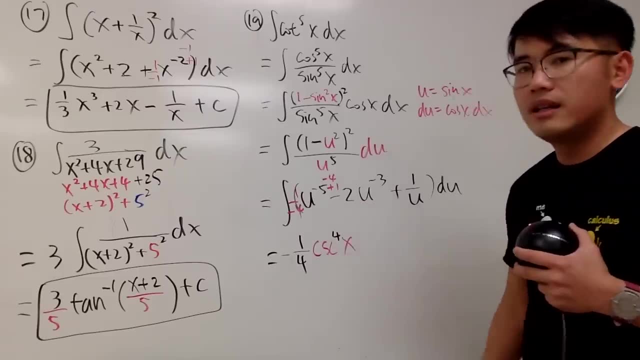 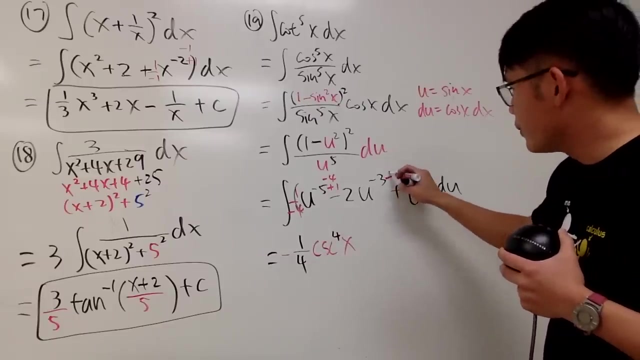 u is sin x. when you have that in the denominator it becomes cosecant. so u to the negative 4 becomes cosecant to the 4th power. yeah, Next, right here we are going to add 1 to the power which is negative 2. 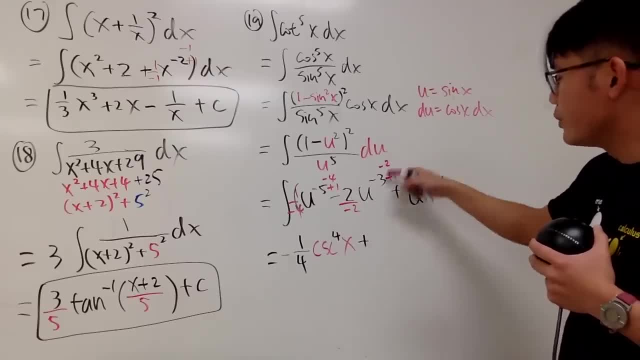 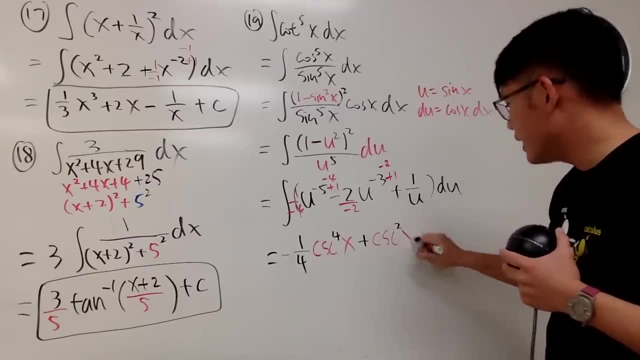 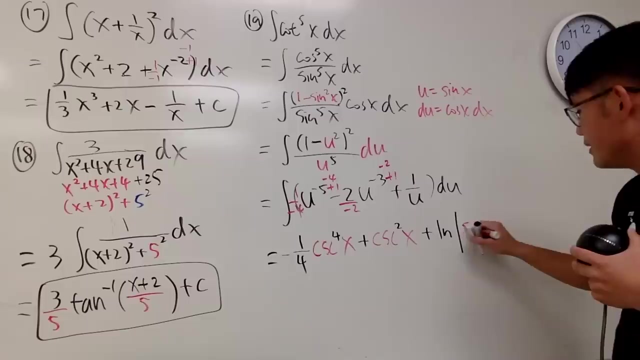 divided by negative 2. negative 2 divided by negative 2 is plus 1, and again u to the negative 2 is the same as saying cosecant in our case. so we have cosecant square x and lastly, we add cosecant to the. 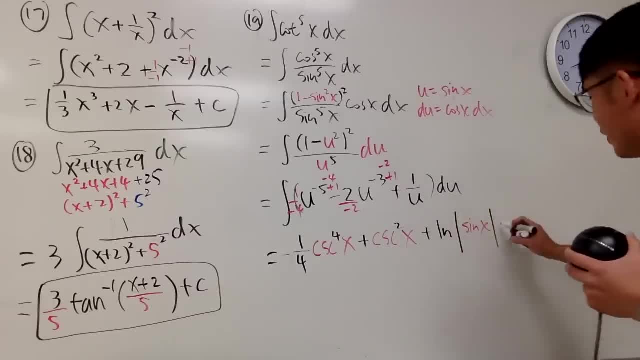 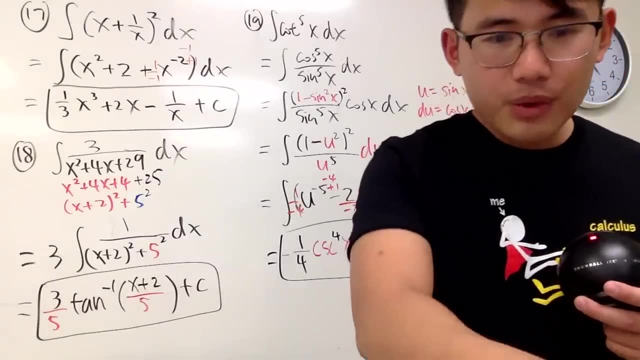 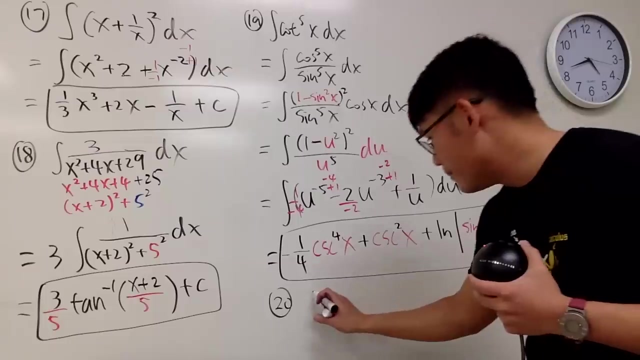 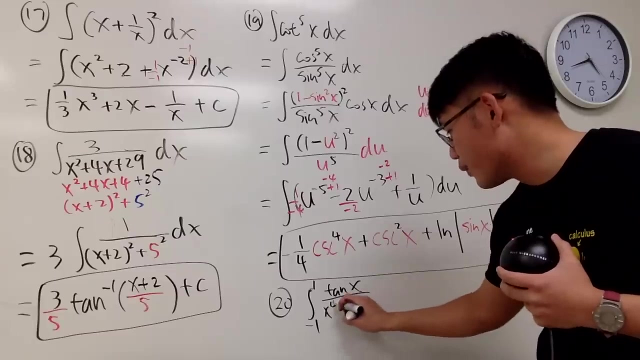 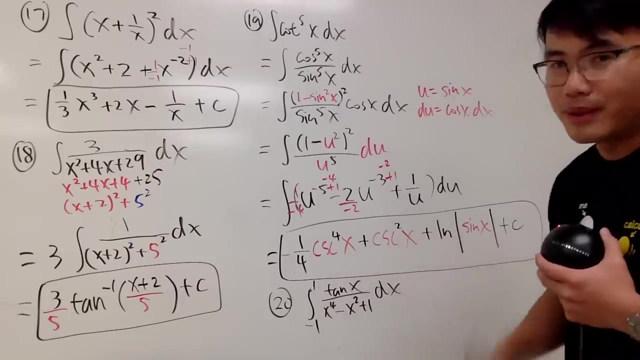 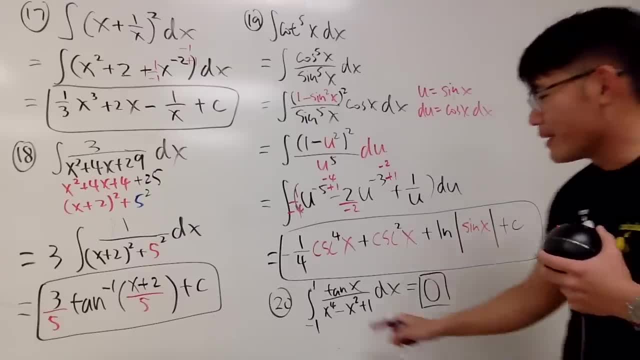 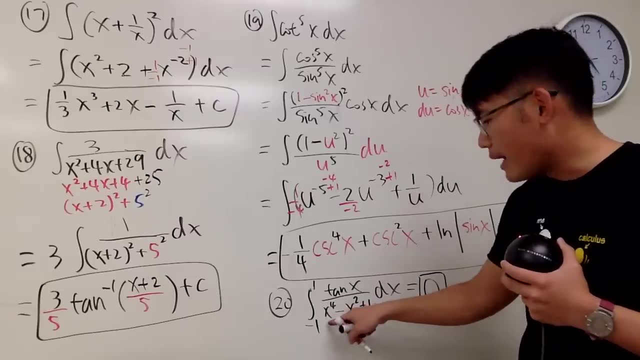 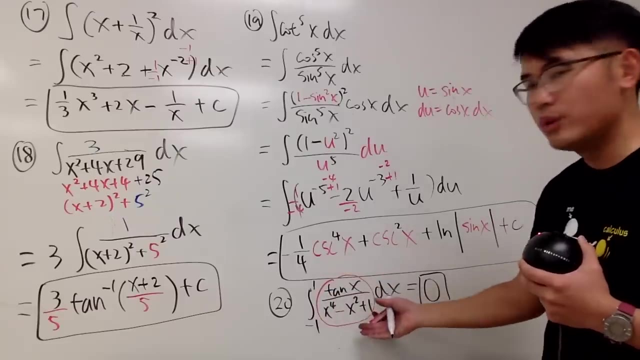 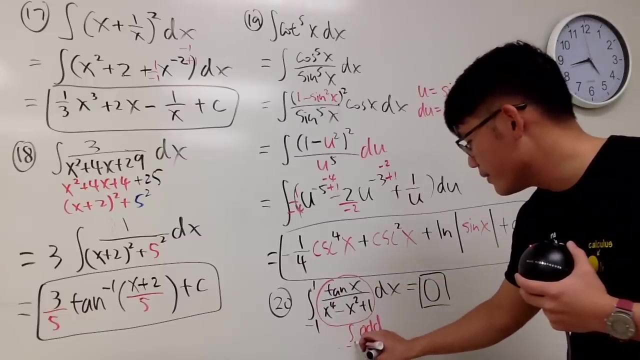 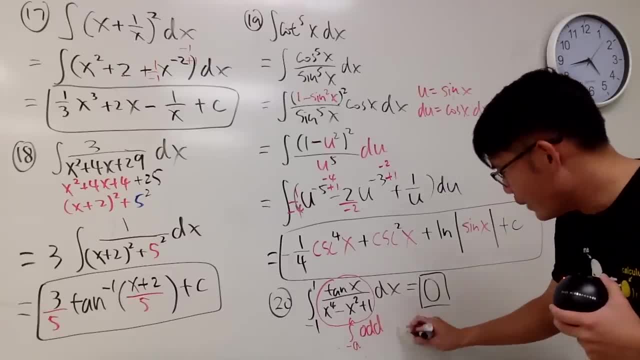 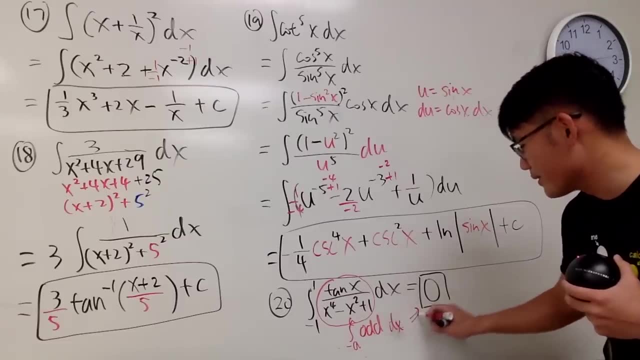 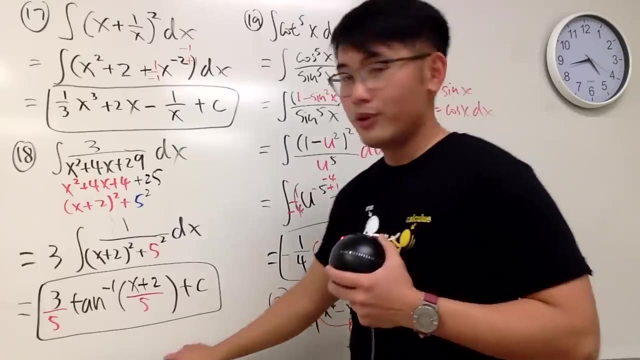 ODD dx, ODD dx. oh no, no man, ODD, let's just put ODD dx. this way, he'll give you 0, okay, So that's it. Yeah, so that was nice. Now, moving on to question number 21.. 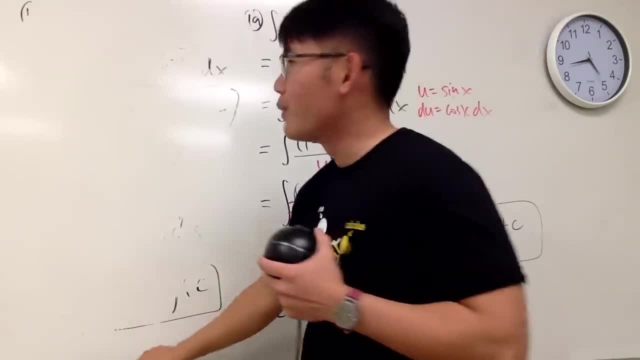 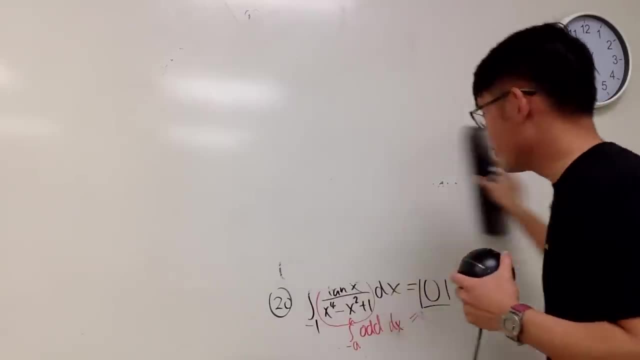 So so far 1 hour and, oh my god, it's going to be like 5, 6 hours. I don't know if I have this much. I don't know if I have much memory to record everything on my laptop. 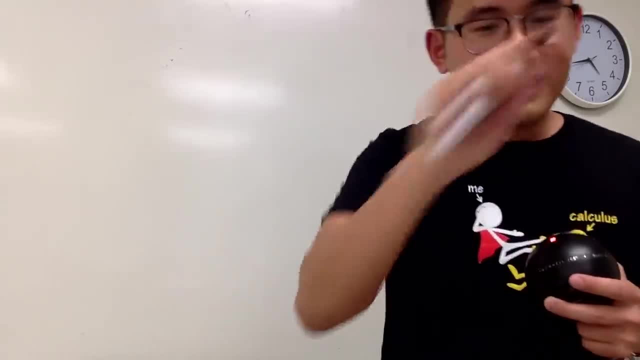 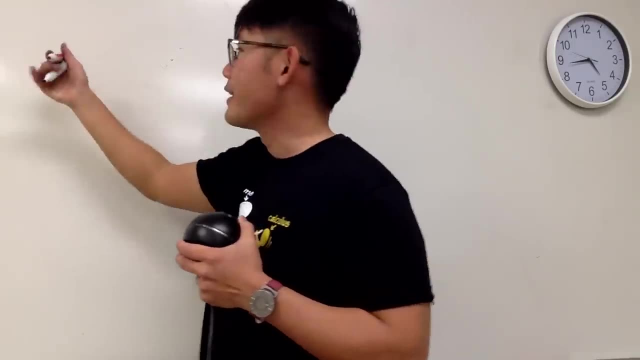 But hopefully at least I have a backup. I don't know, man, seriously, That's it, Number 21,. I don't need to hold this paper, Number 21,. right here I have the integral and we have. 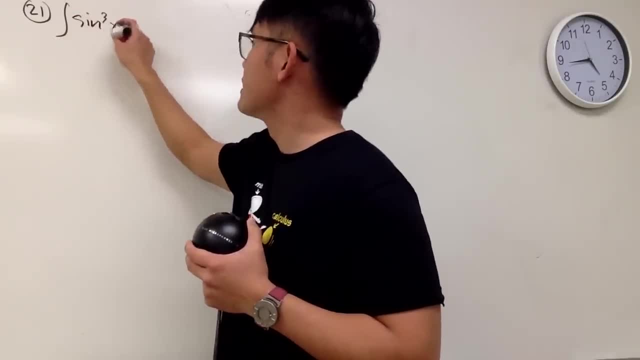 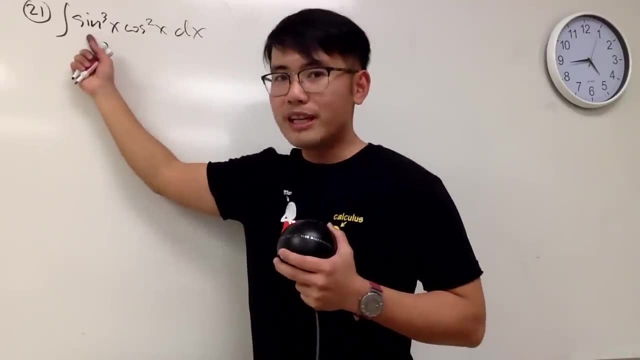 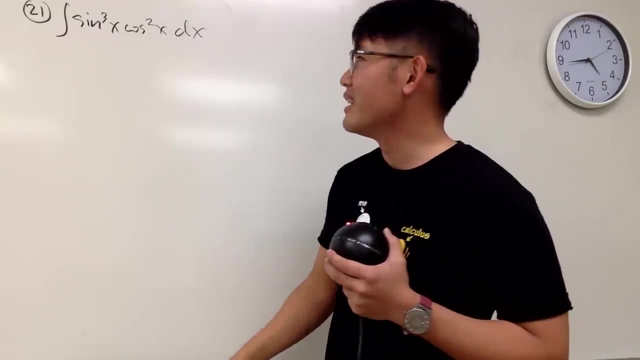 sine to the third power: x times cosine. squared x, dx, right, Well, well, hmm, play it wrong with the exponent This right here. perhaps I can just take one. take one of the sines out so I can look at a substitution in terms of, like that: u equal to cosine. 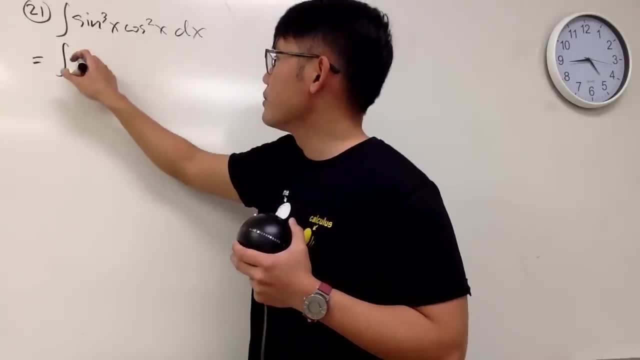 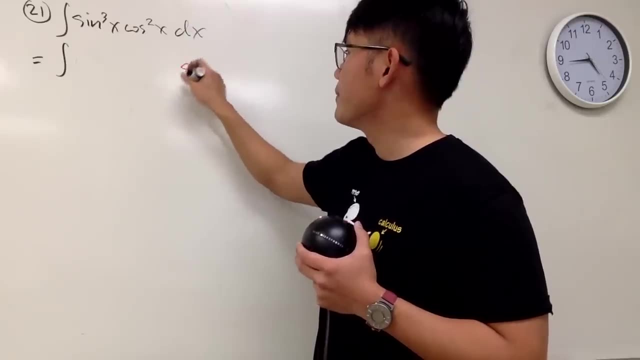 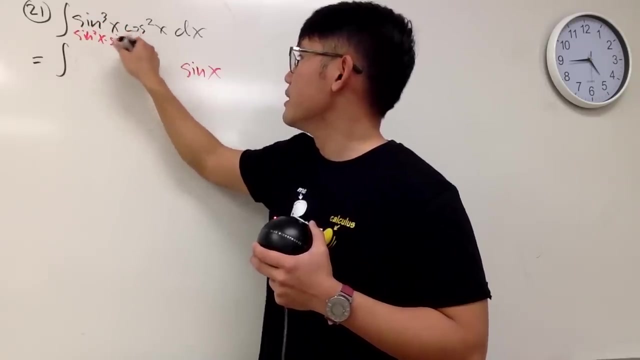 So here we go. This is integral and let me just look at this as sine squared. but I will put that down like this: I will put a sine right here and we'll get sine squared x times sine x. This right here is here already. 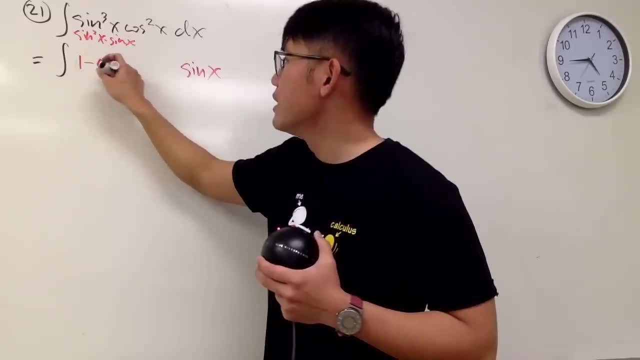 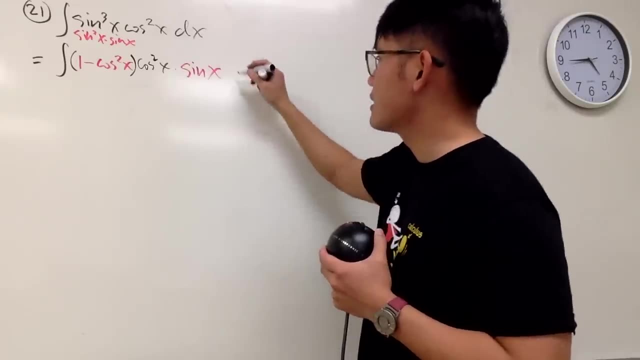 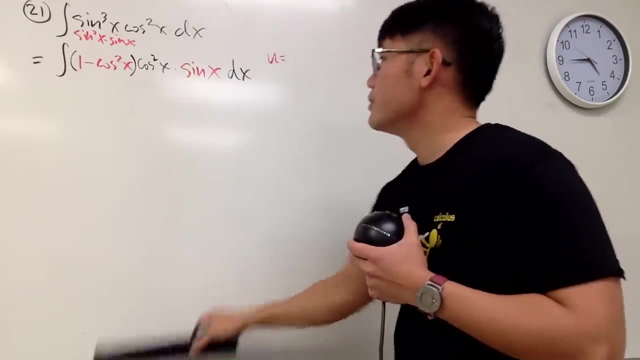 and sine squared is 1 minus cosine squared. so that's nice. And then we multiply by another cosine squared, x, like that, and times sine x and then the dx. Very nice, And with that said, I'm going to just take a use of that- u equal to cosine x. 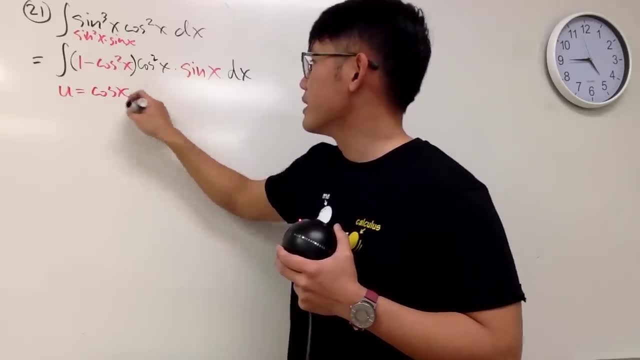 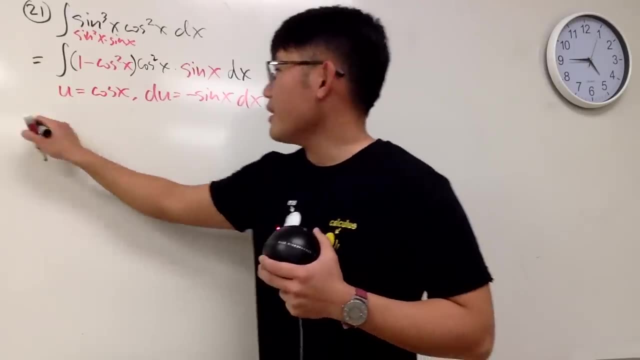 so if I do that, that u equal to cosine x du will be negative sine x dx, And I'm going to do this now. okay, You know you are going to get this and that being canceled, so I will put a negative on the outside like this already. 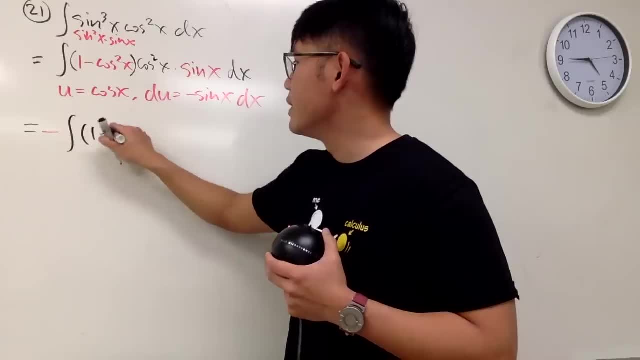 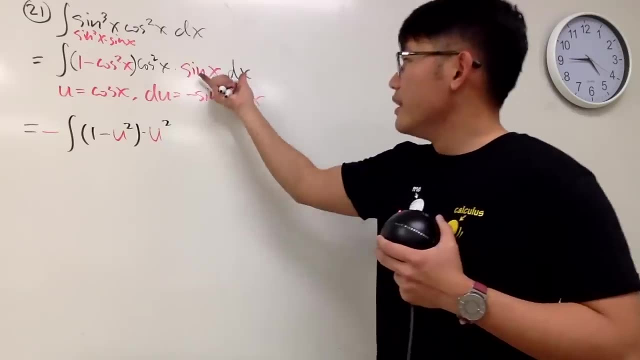 and then you have the integral, and then you have 1 minus u squared, and then times u squared, like this: This with this negative sine together, we have that du. so this is nice. And then, of course, you can continue this real quick. 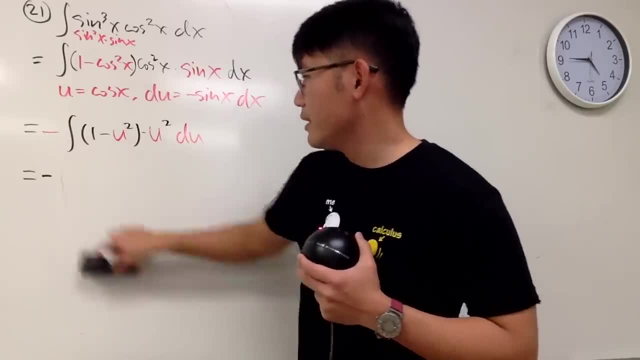 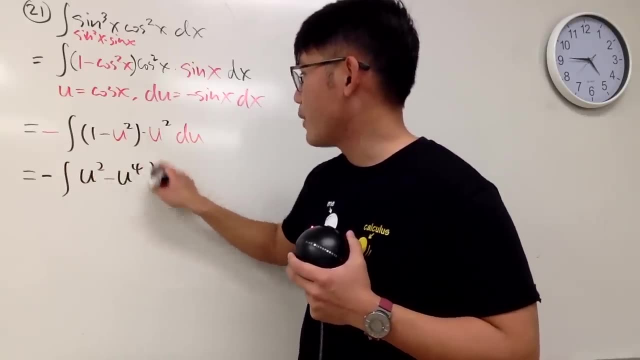 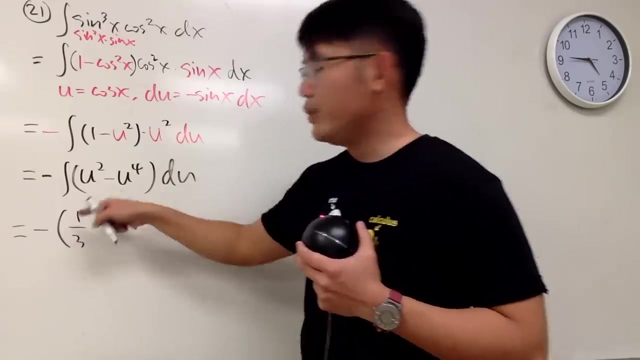 This is going to be negative parentheses. Well, actually, let me- Yes, I have two erasers, by the way- Integral distribute. you get u squared minus u to the fourth power, du. And now negative parentheses: one-third u to the third power: u is cosine. 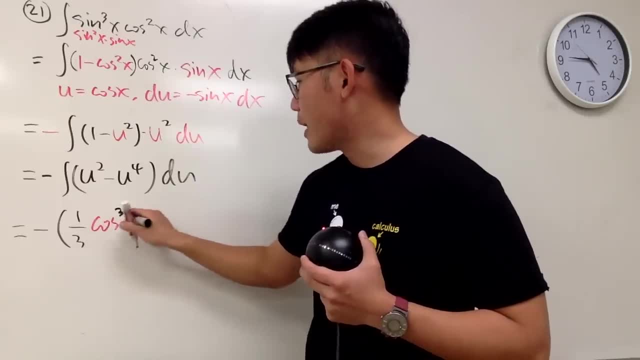 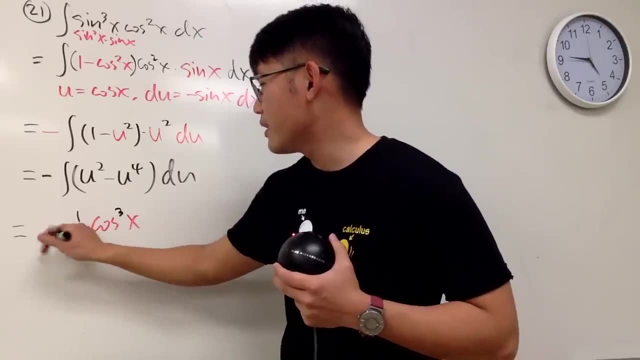 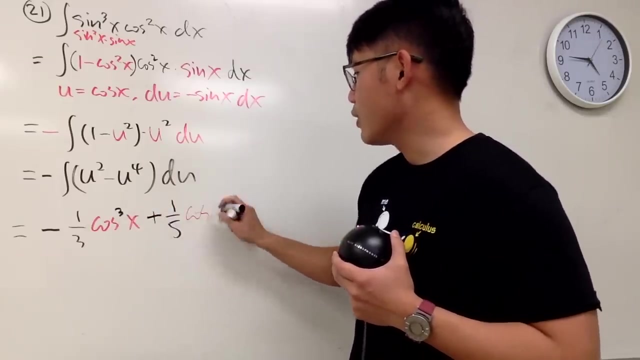 so we have cosine to the third power x. Actually, let me just distribute. distribute the negative so we'll put a negative right here. Negative times, negative will give us plus and then the integral of that is 1 over 5,. cosine of fifth power x. 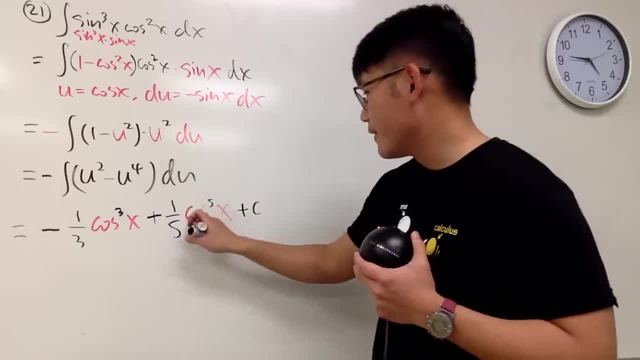 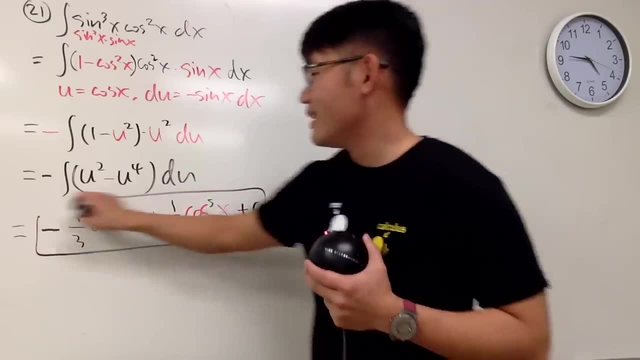 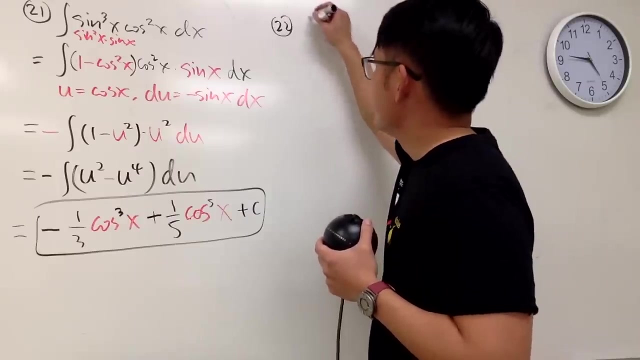 We are done like that. This is a quick and easy one, Yeah, Like this, Okay now, oh my god, number 22.. Let's see what's up with this Number 22,. integral of 1 over x squared, square root of x squared plus 1, dx. 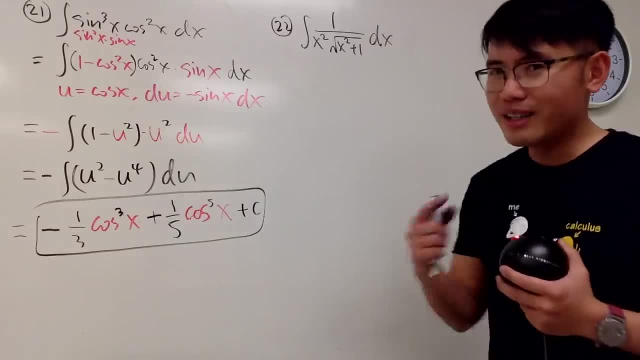 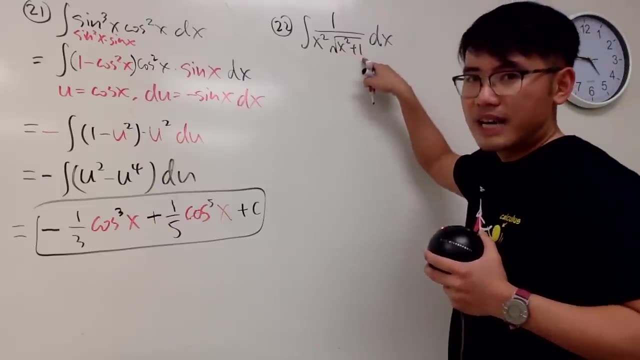 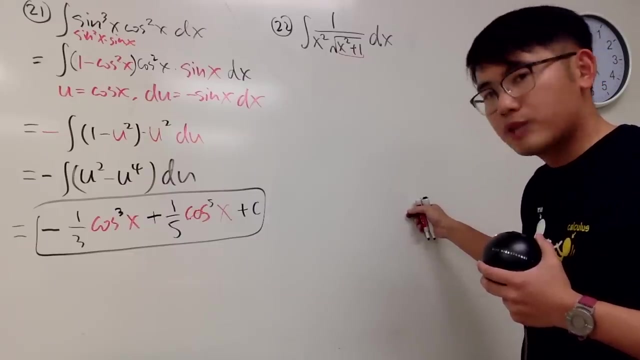 Tricks up, maybe Anyone. No, I can do use-up right here. Let me show you how. Let me show you how to do it. Look at the inside here, right? Notice that the derivative of x squared plus 1 is 2x. 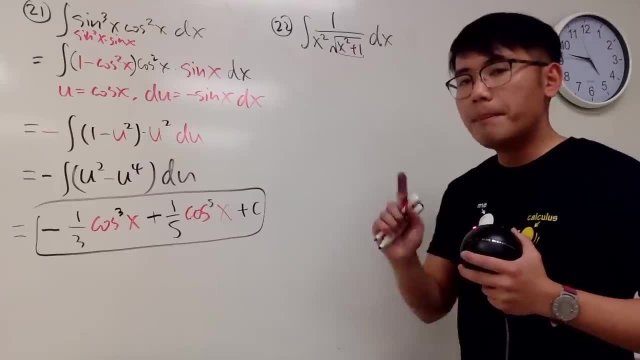 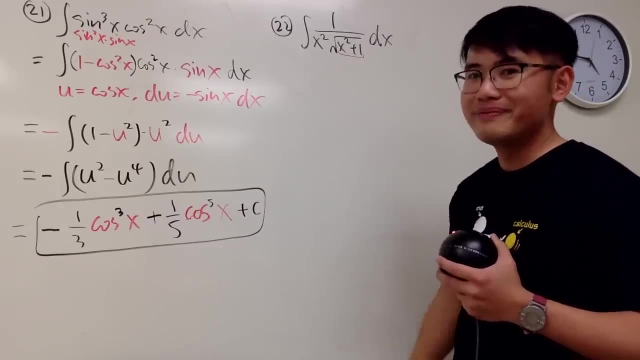 2x to the fourth power, 2x to the first power. right, We don't have 2x to the first power, But if you factor out x squared, you end up with x to the negative 2 somewhere. If you set that to be the? u you end up with, you know, x to the negative 3 power. 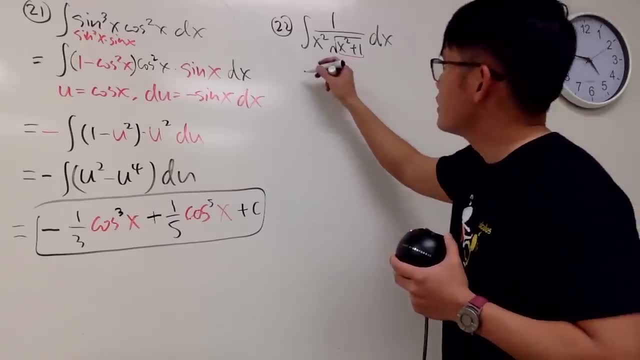 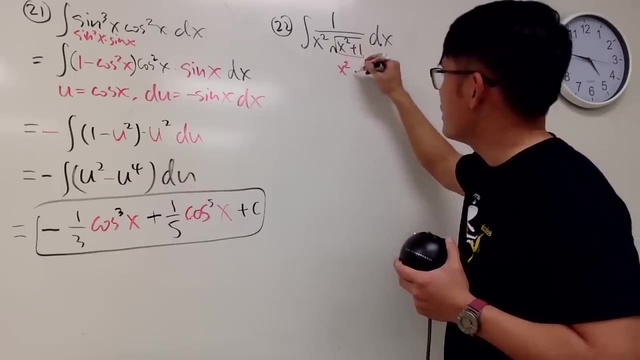 something like that. It's very nice, Let me show you. So here's the deal. I'm actually going to factor something out first, right here. This is the same as saying: I can factor out x squared and I will end up with 1 plus x to the negative 2.. 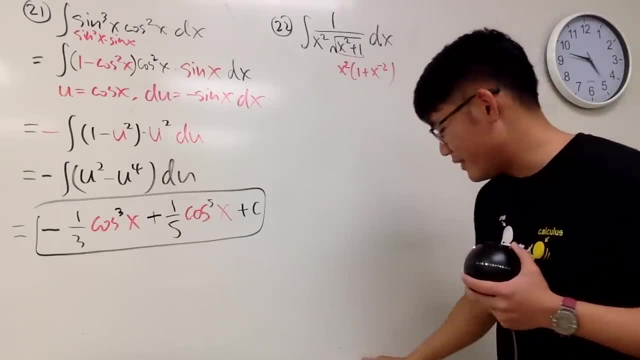 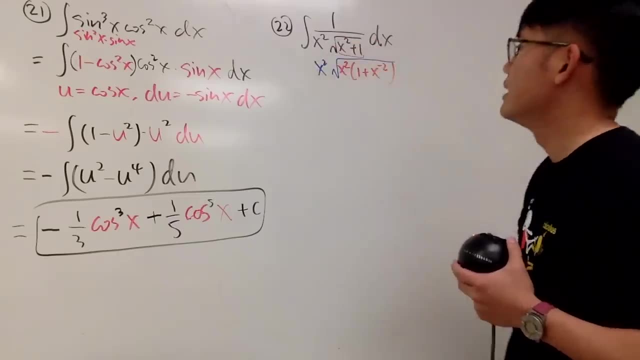 How's that? Don't forget, we still have the square root in the denominator like this, right for that. And of course, you still have the x squared on the outside. Well, well, when you have the square root of this times, that. 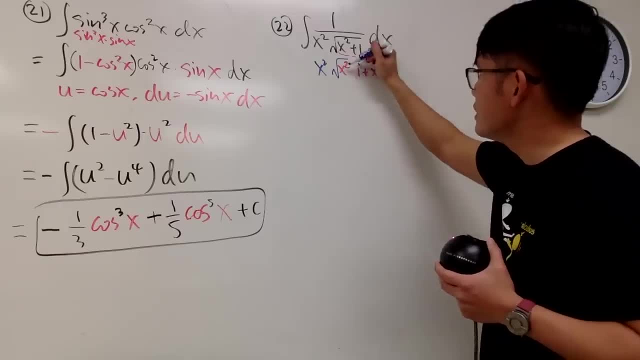 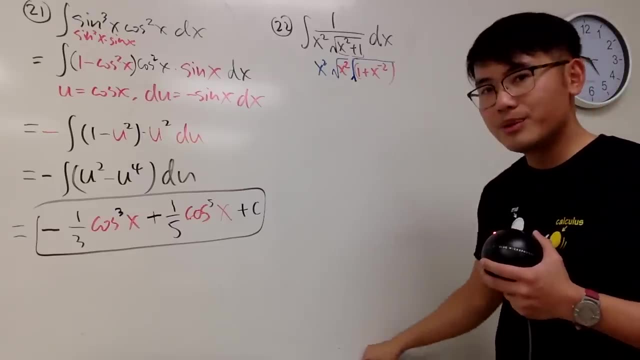 of course, we're just focusing on the integrations in this video, So I'm just going to do this. And now here's the beauty. okay, You are going to get the following: This is going to be the integral, This is x squared and this is x. 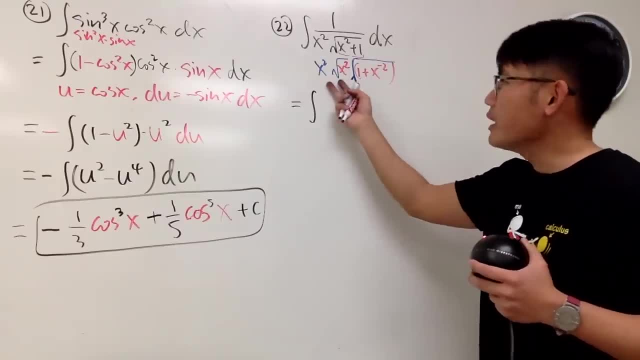 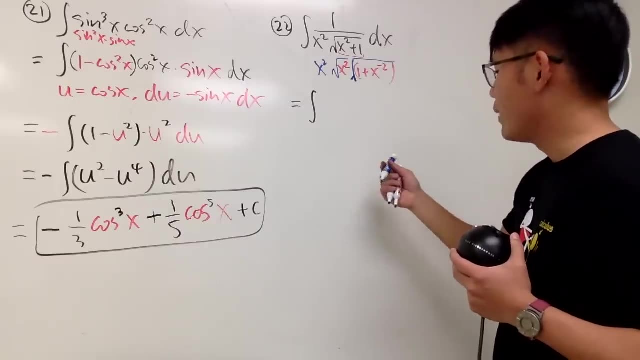 x to the first power. Don't worry about the absolute value All to get this x to the third power. if you bring that to the numerator, you get x to the negative 3.. So that's what I would like to show you. 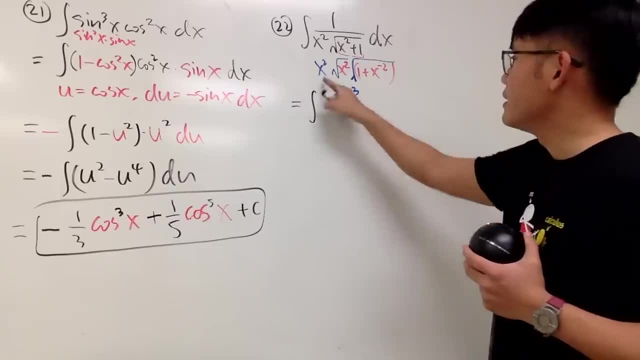 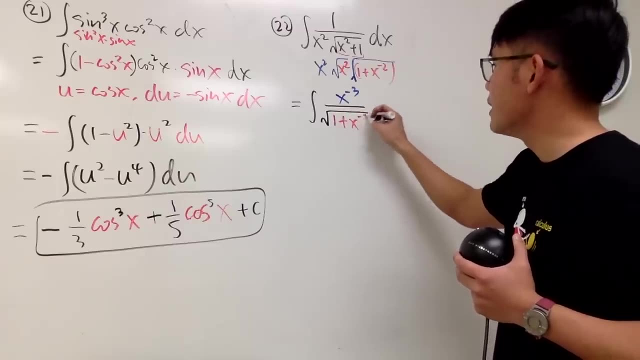 Let me just put this down right here: x to the negative 3, like this and that, And then for the bottom, you still have the square root of 1 plus x to the negative 2, dx. And when we do this, 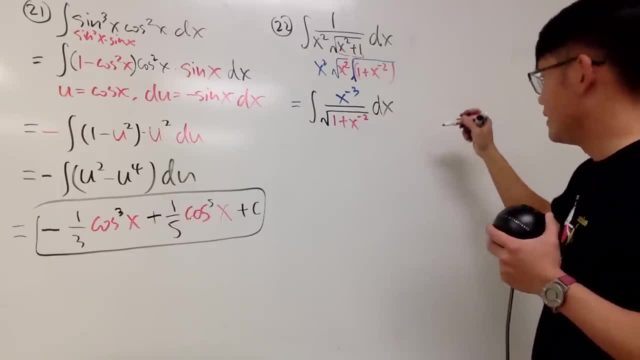 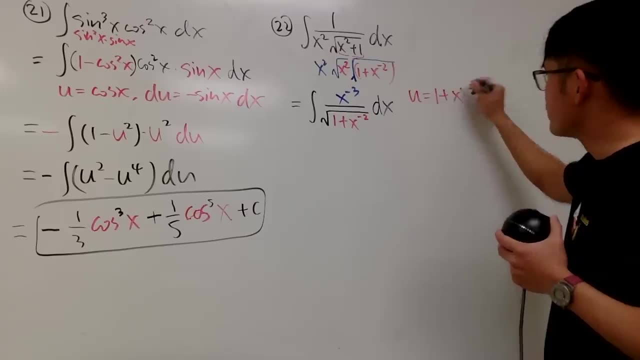 we can just take a u to be 1 plus x to the negative 2.. Let me see if I can do another one. Maybe not just do something So real quick: 1 plus x to the negative 2.. Differentiate both sides. 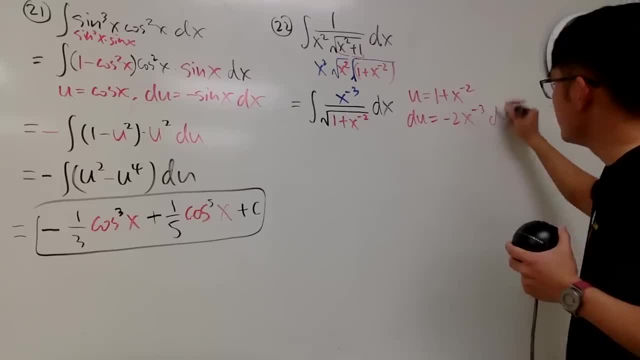 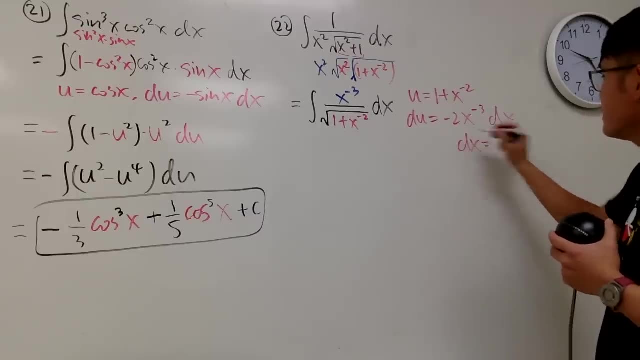 we get du being negative 2 x to the negative 3 dx. Ha ha, that is going to help us out, So perhaps I'll just isolate this real quick. dx is the same as du over negative 2 x to the negative 3.. 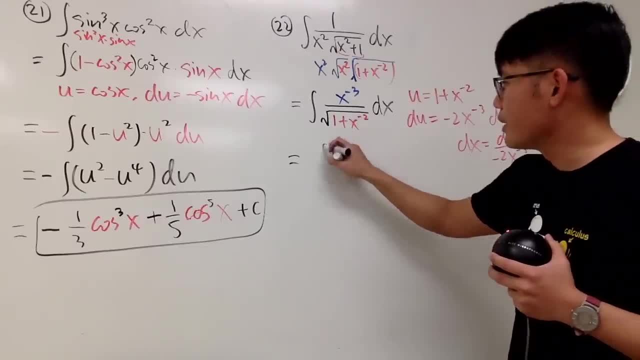 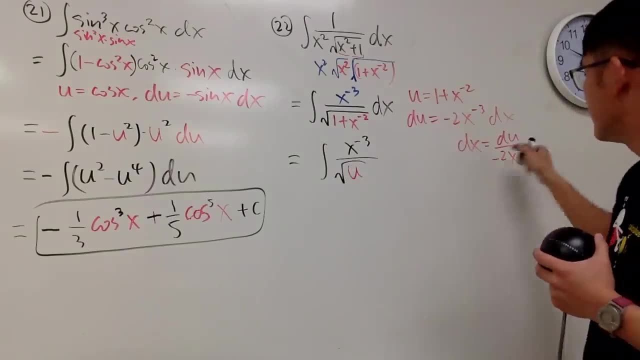 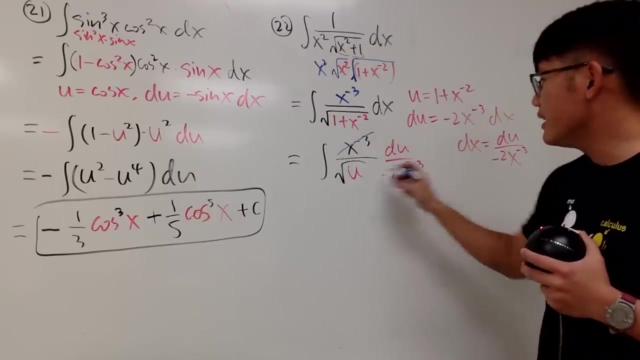 So you are going to see, here you have the integral x to the negative 3, over square root of u, And the dx is that which is du over negative 2, x to the negative 3.. And this and that cancel each other nicely. 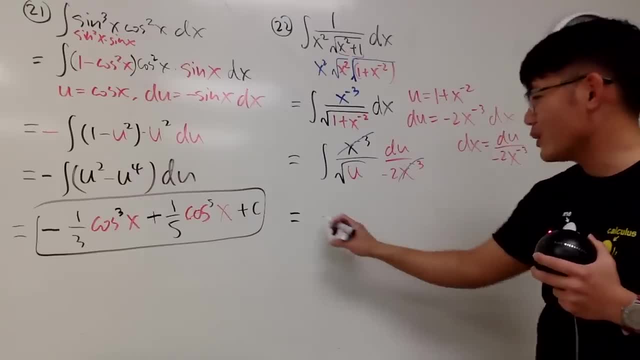 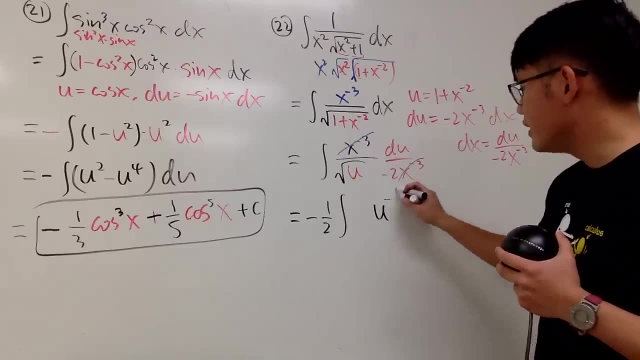 So wonderful, isn't it? Yes, it is, of course. Here we have negative 1 over 2, right In the front, And we are integrating This- right here is the same as u- to the negative 1 half power. 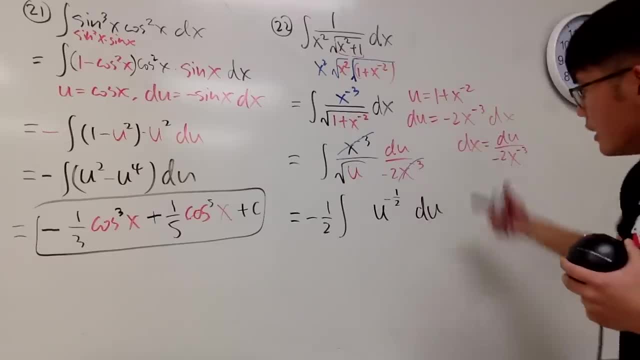 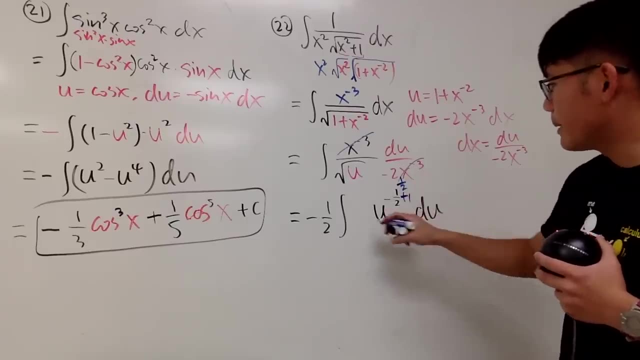 And we are having the du right here. Okay, So I'm going to add 1 to the power And which is going to give us positive 1 half. Divided by positive 1 half is the same as multiplied by 2 over 1.. 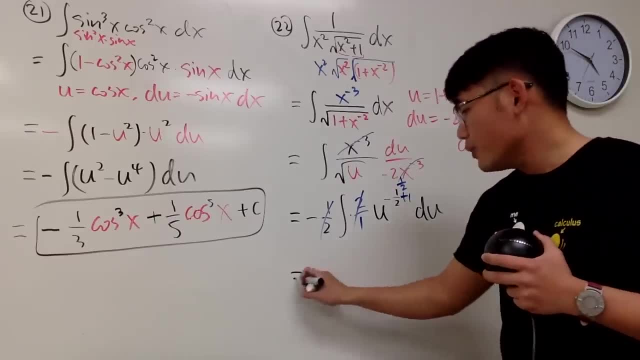 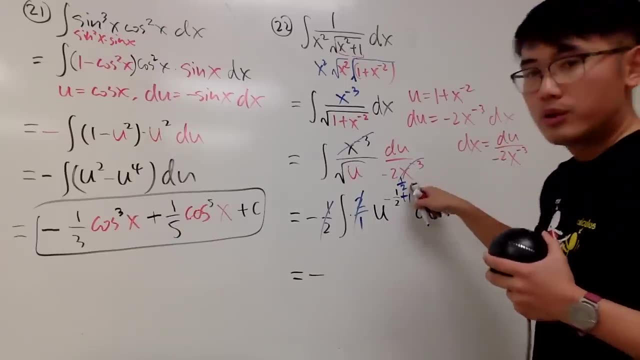 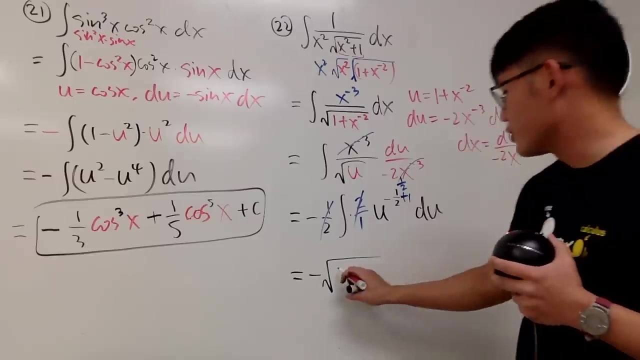 They cancel each other out. Very nice. So we are going to end up negative, Negative, And then u to the 1 half power named the square root of u. Well, I will just put down: square root u is this guy. 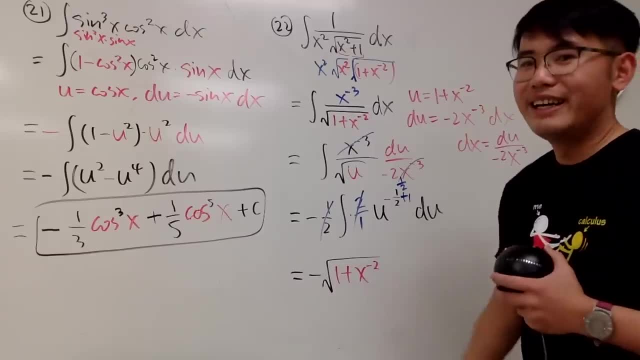 So I just put down 1 plus x to the negative 2. And with that we are done. How wonderful isn't it? Yeah, Let's see, This is good. Yeah, Okay, So that was number 22.. 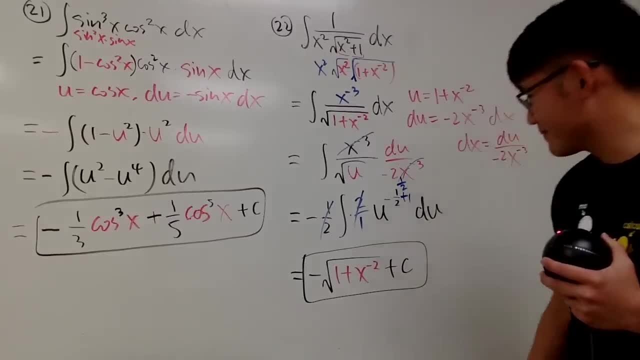 And now moving on to question number 23.. I will just come here and erase Question number 23.. Oh my God, I'm almost a quarter way through. Oh my God, Oh my God, Oh my God. 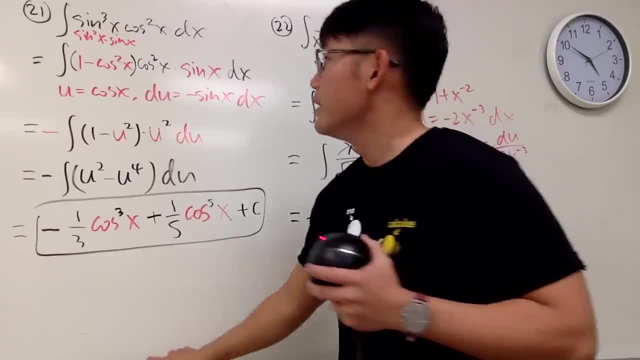 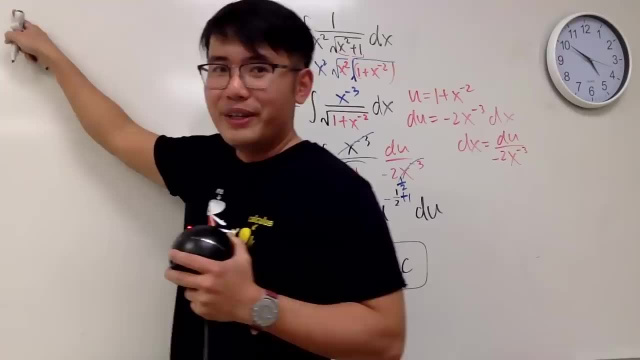 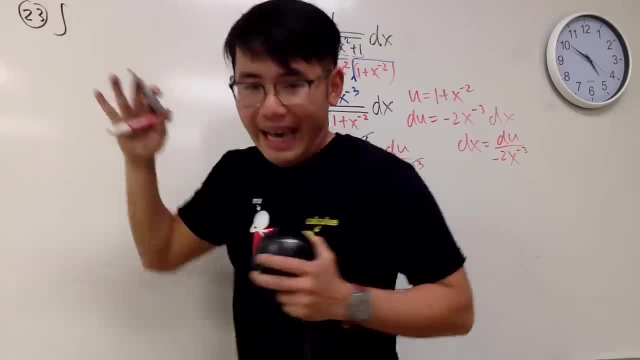 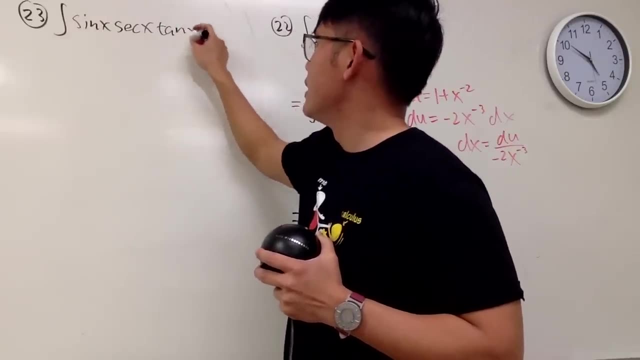 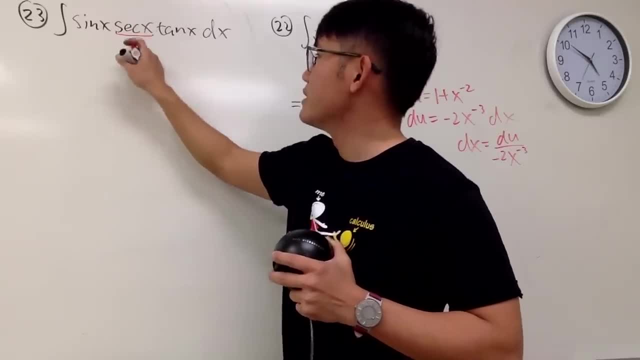 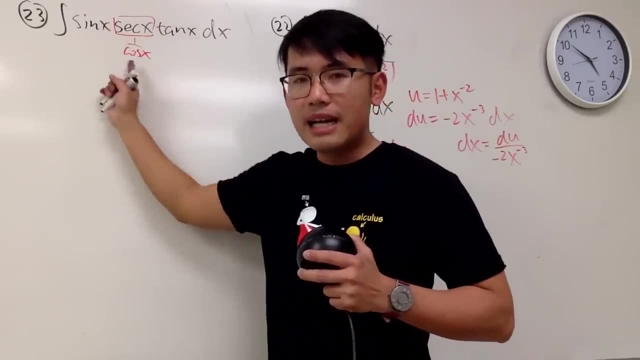 This is not bad at all because- notice this right here- is just the same as 1 over cosine x. This is the same as 1 over cosine x, And then this times that is tangent and times another tangent. yes, you just get the integral. 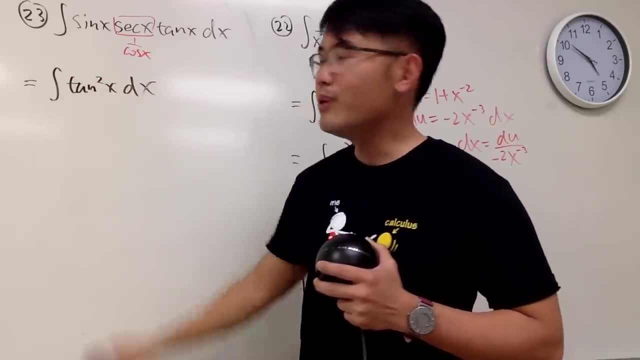 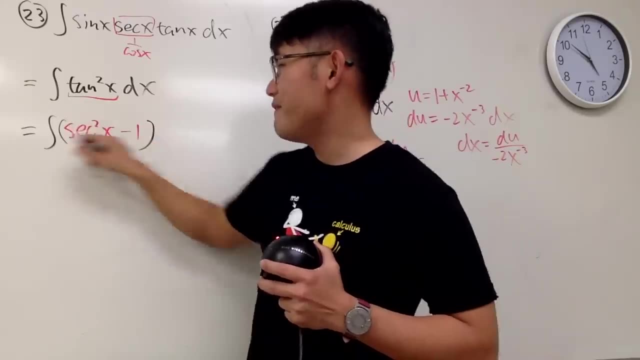 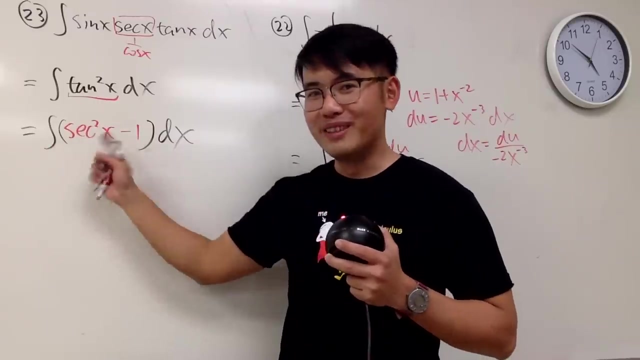 of tangent squared x, dx And for u- Integrate tangent square, it's the same as integrating secant squared x minus 1.. Very nice, I have a really short video, only 20 seconds long, on the integral of secant squared. 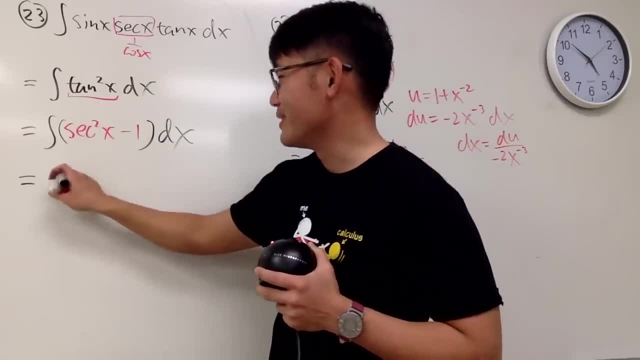 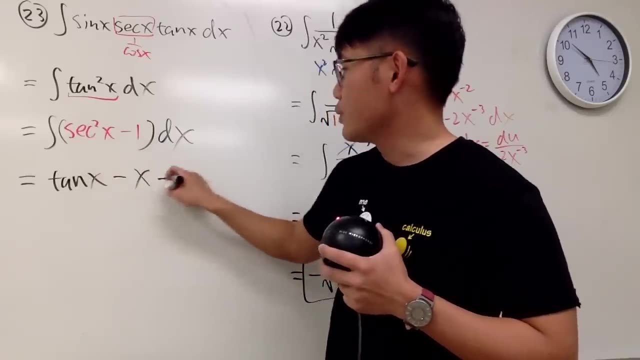 People didn't like it because I just told them the answer to that integral is just tangent x. But that's it. you have to know your derivative table really well. And then minus x and you're done. plus c, Very nice. 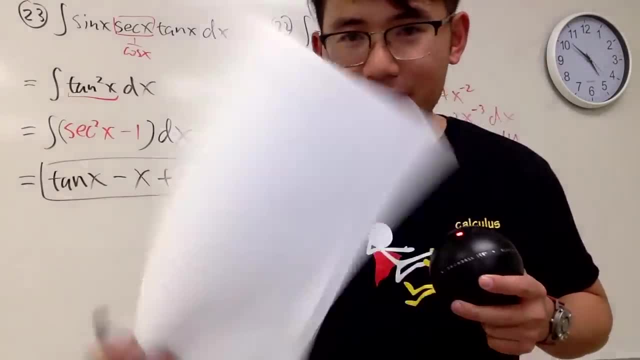 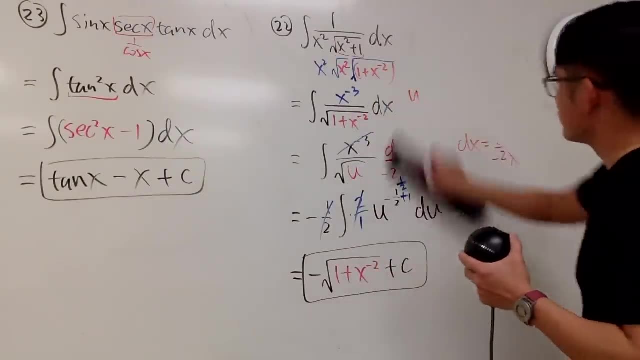 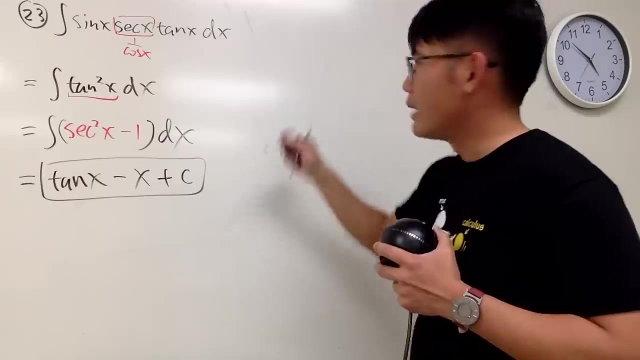 Okay, number 24, we have secant to the third power x. That takes some space and I will do this from scratch, but I will do it pretty quickly though for you guys. So I will just show you guys how to do this right here. 24, integral of secant to the third power x- dx. 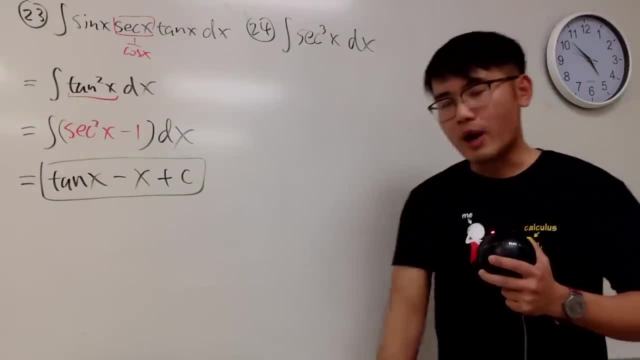 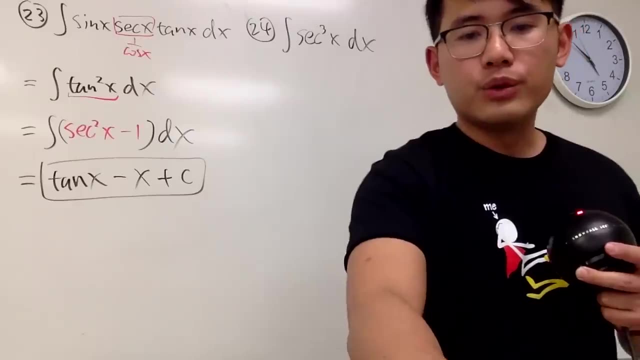 Yeah, All right, this is a famous one, so you have to know How to do this. We will be using integration by parts. We have to break this apart into: secant to the first power times. secant to the second power. 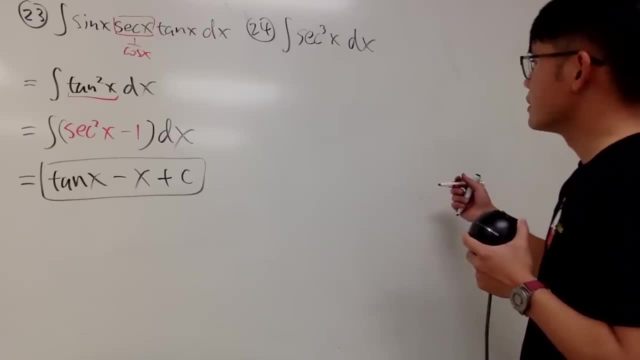 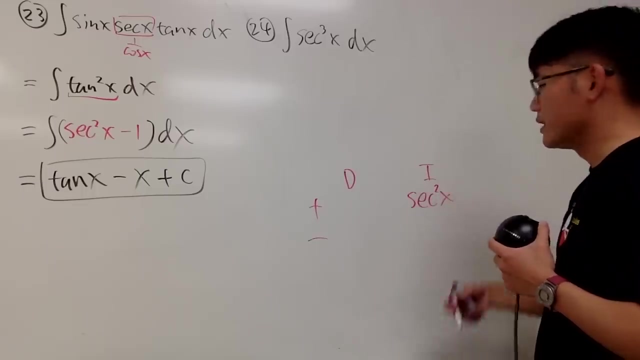 And when you do that, perhaps I will just write this down right here for you guys. All right, I will put this down right: d and then i plus minus. Okay, so I will be integrating secant squared x, because we know how to do that. 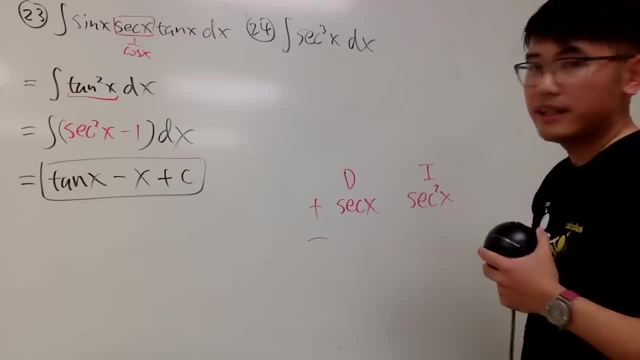 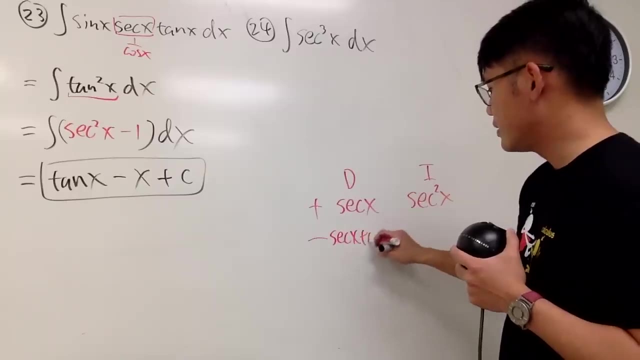 We just did the help there And now we will be differentiating secant x. All right, And when you differentiate this, you get secant x, tangent x. And when you integrate this, you get tangent x. Very nice. 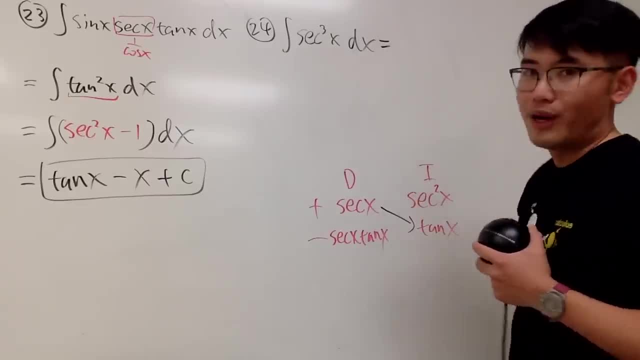 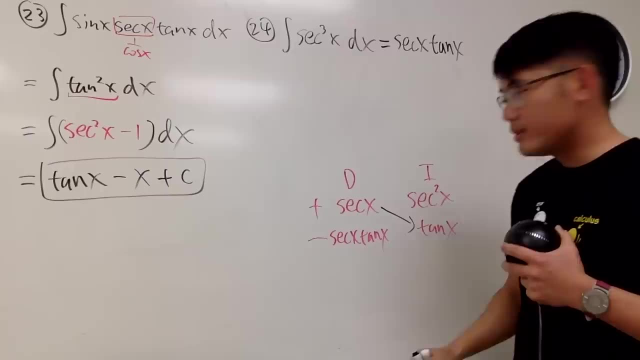 So, in other words, when you multiply this and that you get the first part of your answer, which is secant x times tangent x, But don't forget, you still have to multiply this row, which is still going to be an integral. 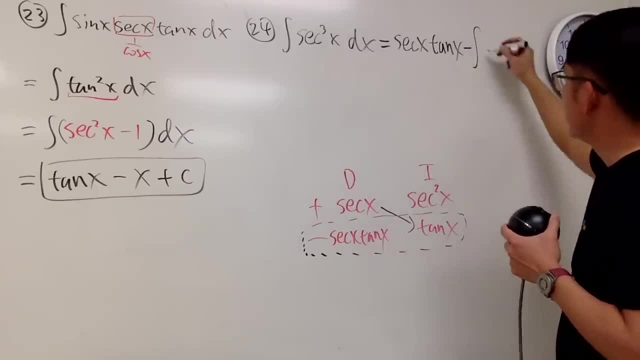 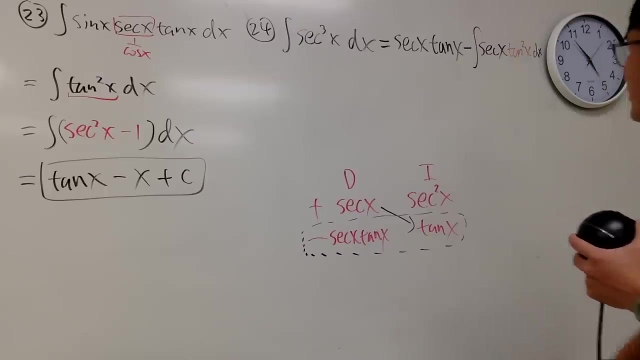 So minus the integral, and you have the secant x and you have tangent, tangent, which is of course tangent squared x. I'm sorry, clock. Yeah. Well, hopefully I don't knock you down, because it took me a while to put you up. 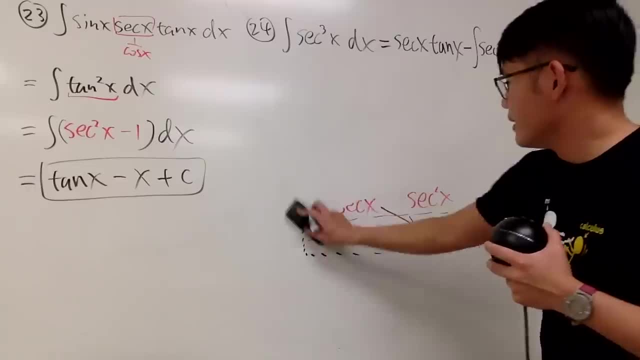 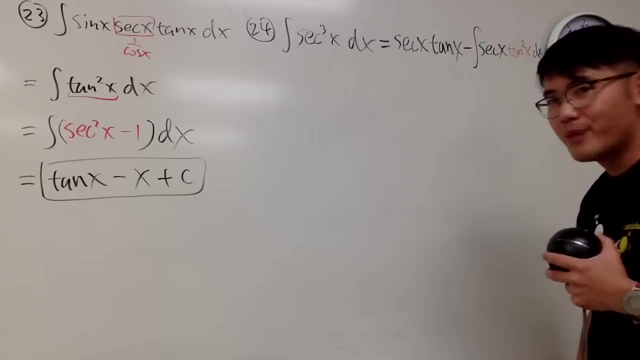 So that's pretty much the idea. Well, you apply the integration by parts, and this is going to be a repeated situation, because if you look at tangent squared, well, we know that secant squared minus 1, we did that over there already, right? 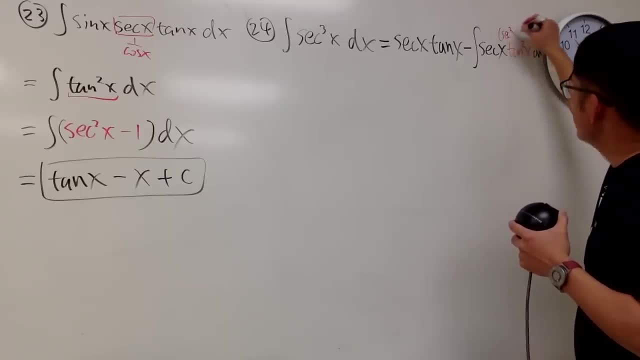 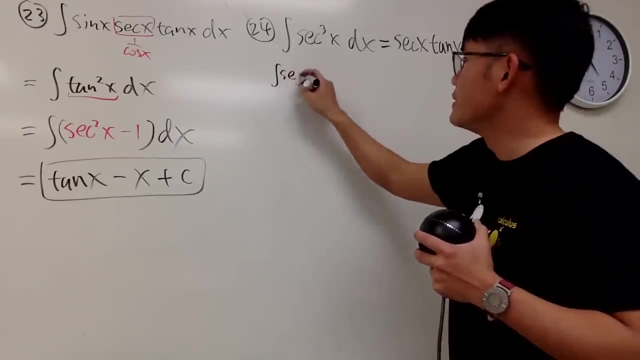 So let me just write this down. This is the same as secant squared x minus 1.. And you can distribute, distribute. I will write this down again for you guys: Integral of secant cubed x, dx is equal to. this is the first part of the answer. 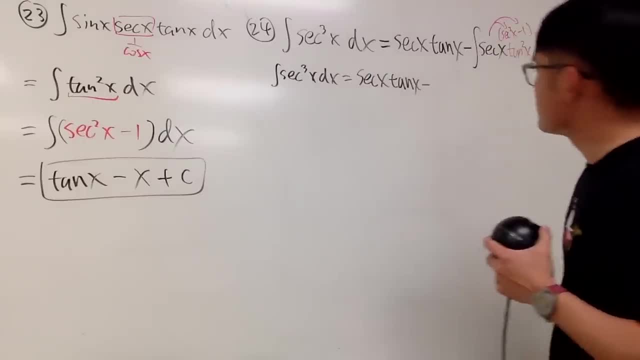 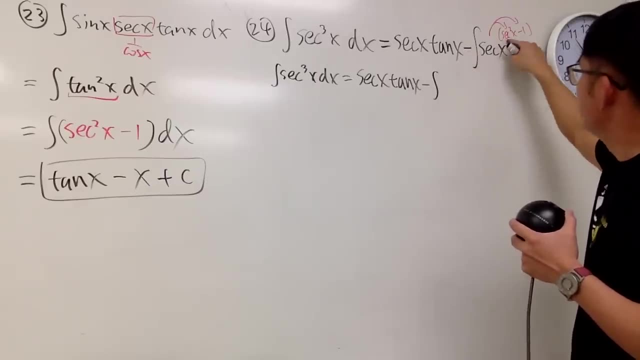 secant x, tangent x, But you have to minus two integrals. I will split this down. The first integral is the integral, So secant squared, So secant times secant squared, which is another secant cubed x. 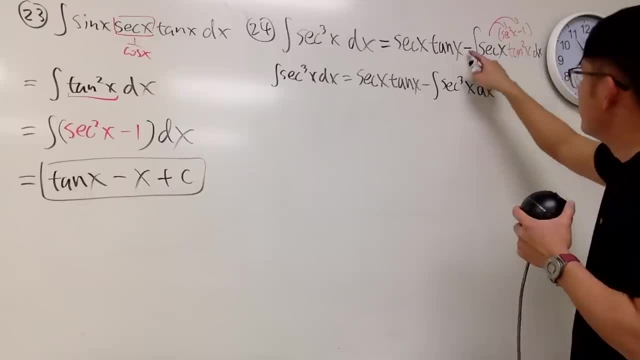 And I will close this integral, And then the next one is minus. minus becomes plus, and then we have the integral: secant x times 1 is secant x- dx, like this. All right, Here we will do two things at the same time. 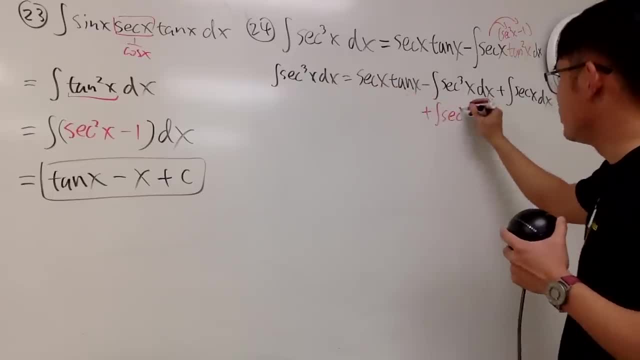 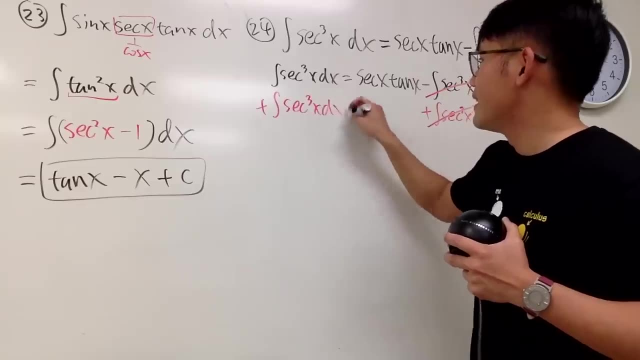 First, I will add this on both sides, because I see the repeat. So add this, So they cancel. So just like the Google Algebra days, isn't it All right? And in the meantime, we can also figure this out. 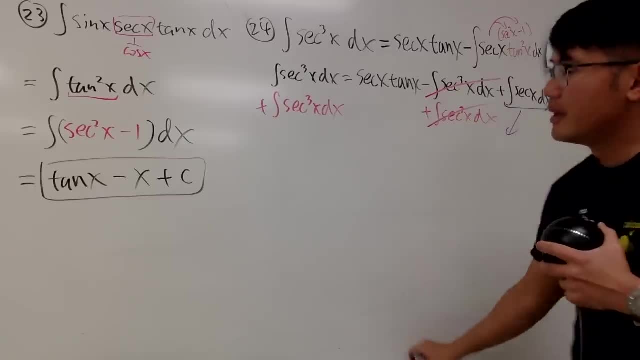 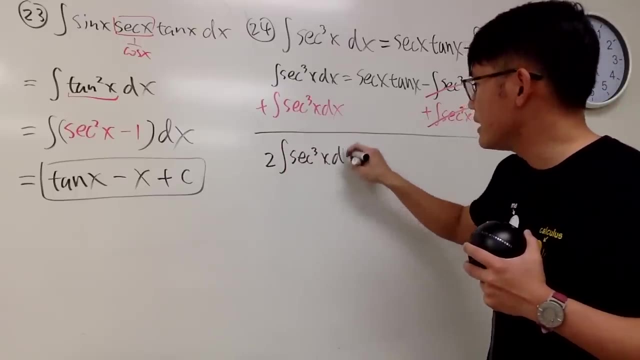 But I will just put on the answer right here for you guys in blue. So when you do that on the left-hand side you get 2 times the integral of secant cubed x, dx, And this is equal to that which is secant x, tangent x. 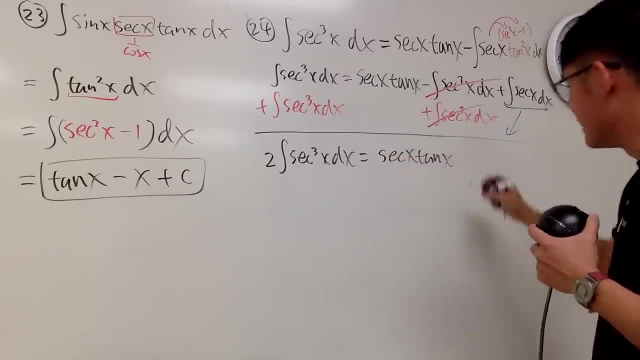 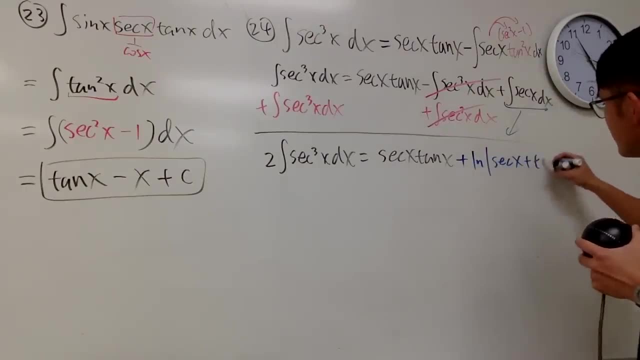 But you are going to add. this is an addition. addition, okay, not addiction. You add the integral of this, which is natural log, absolute value of secant x plus Tangent x. like this: In the end, divide everybody by 2.. 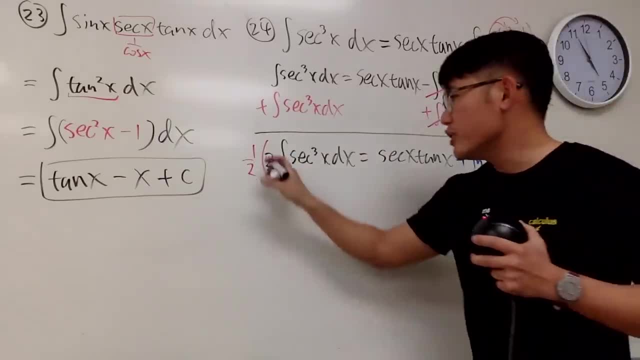 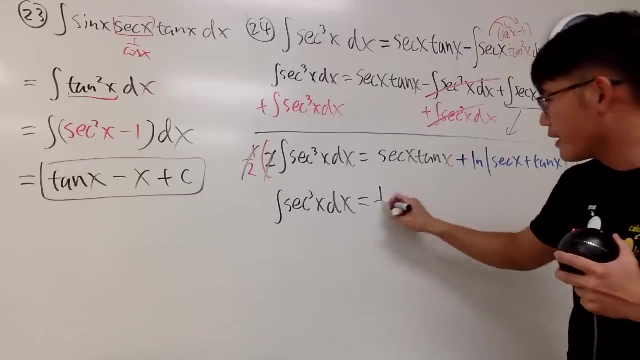 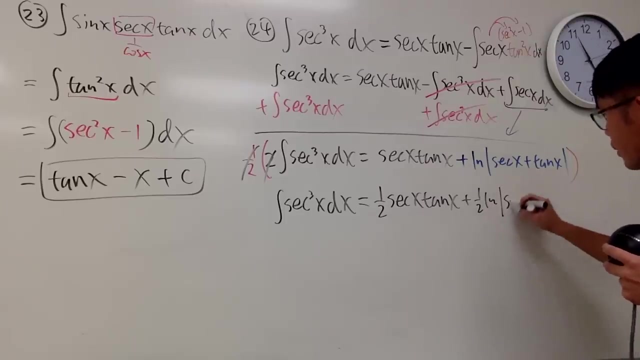 So multiply everybody by 1 half. So, ladies and gentlemen, let me tell you guys that the integral of secant cubed x dx is 1 half times secant x, tangent x plus 1 half natural log. absolute value of secant x plus tangent x. 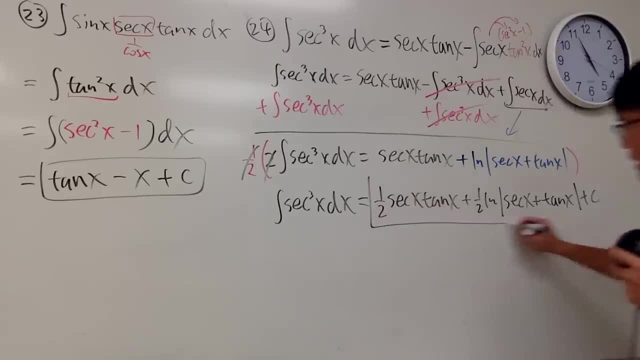 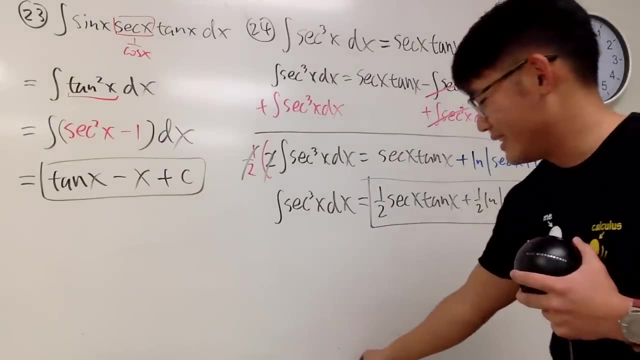 And we are done. So put plus c This right here. is it All right? So it was not bad. If you practice a few times, you can do it too Seriously. I don't know how many times I have done these integrals with my students already. 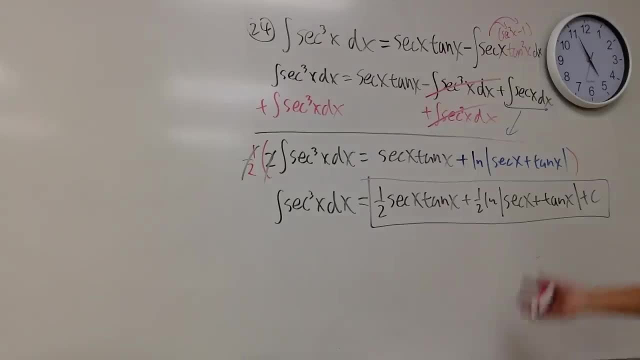 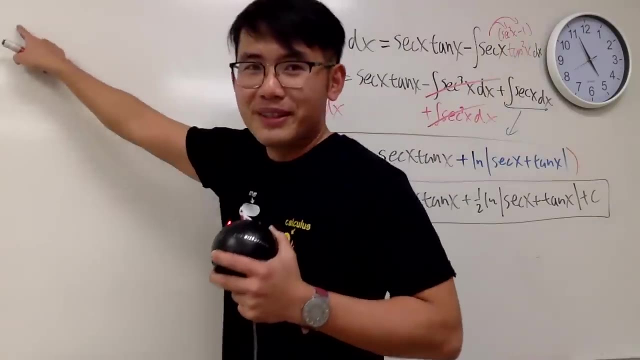 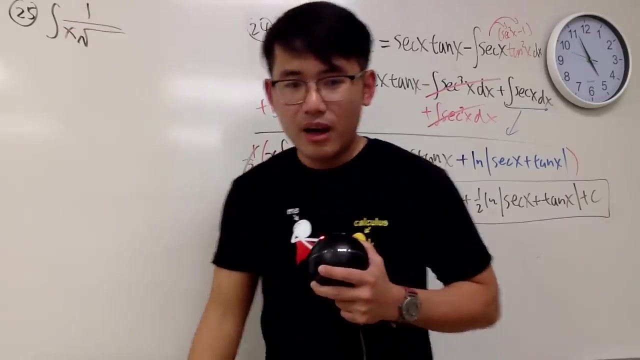 So, yeah, All right. So let me just show you guys the work. Okay, Number 25.. I feel sore over the legs already. Number 25.. The integral of 1 over x times the square root of x, squared minus 1 dx. 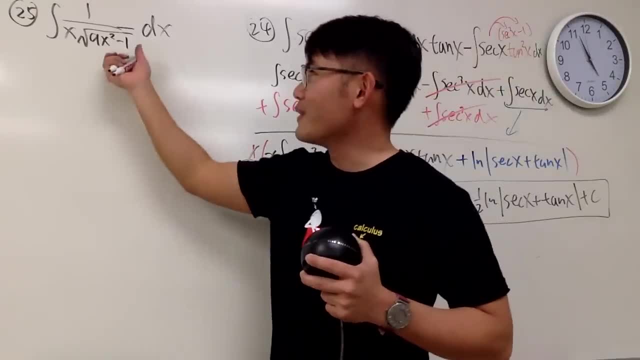 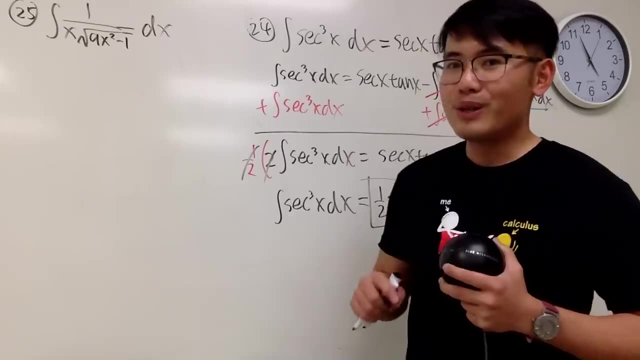 And here's the deal. Unfortunately, we cannot just factor out the x squared whatsoever and then do the use up. I don't think that's the case, unfortunately. However, though, we can do some tricks up now. This is how we are going to do it. 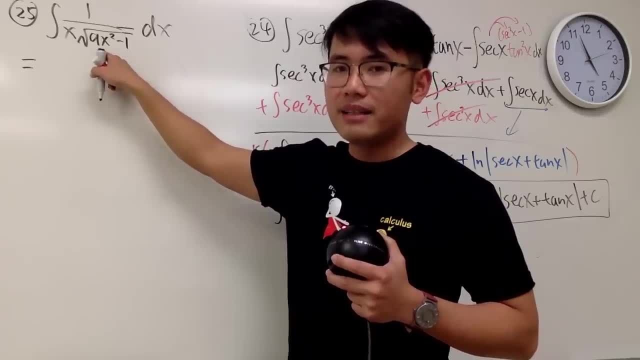 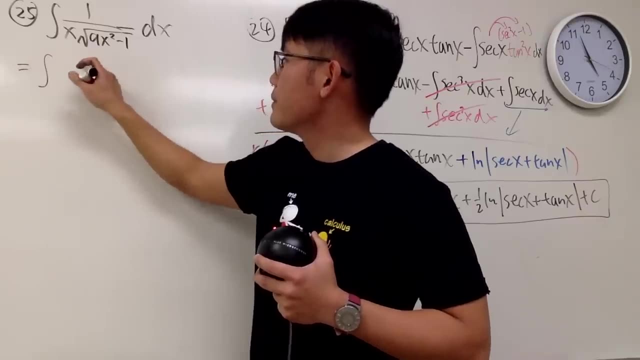 First of all, you may be noticed that 9 is bothering us, So I will be doing this right. I will write this down As the integral of. Actually, I will just save my time When you have 9 in front of the x squared. 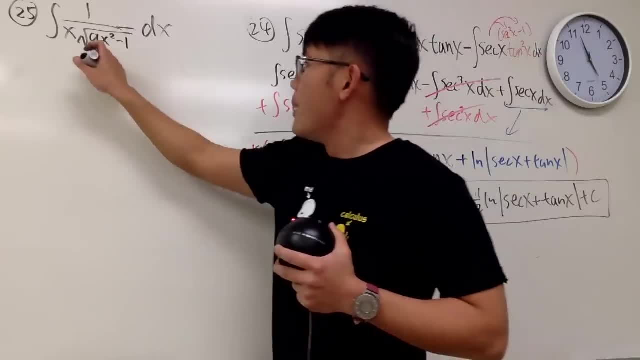 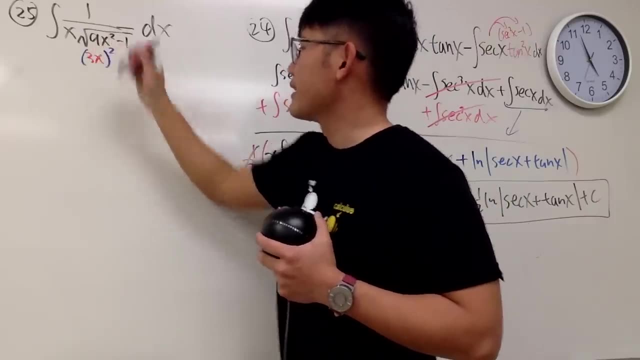 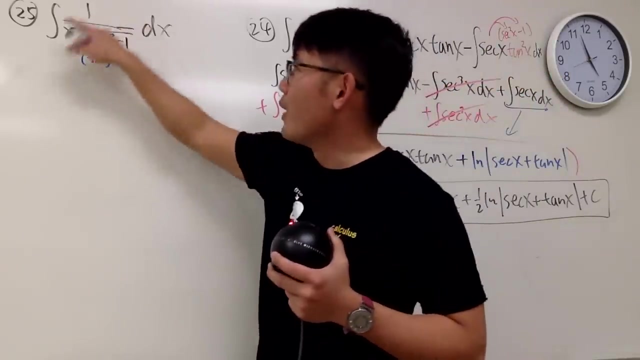 you are going to be looking at this as parentheses with 3x inside and then square like that, And then technically you do use up and all that stuff. But here is the beauty, When you have the integral 1 over x times the square root of some number, times x squared minus 1,. 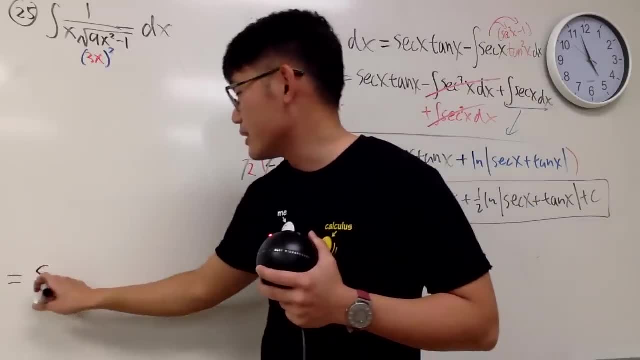 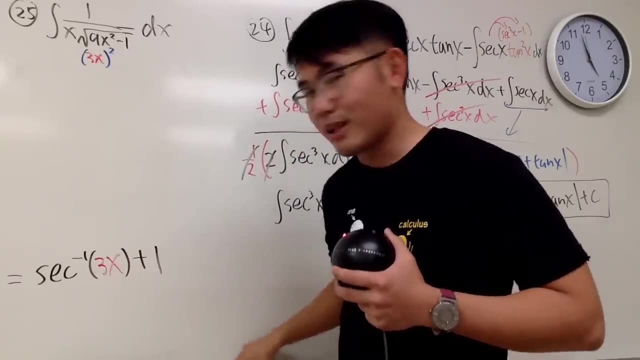 I will tell you guys the answer. The answer to this right here is actually just the inverse secant of that input, which is 3x, And technically you are Oops, not plus 1.. Technically it's not wrong to put plus 1,, but this is it. 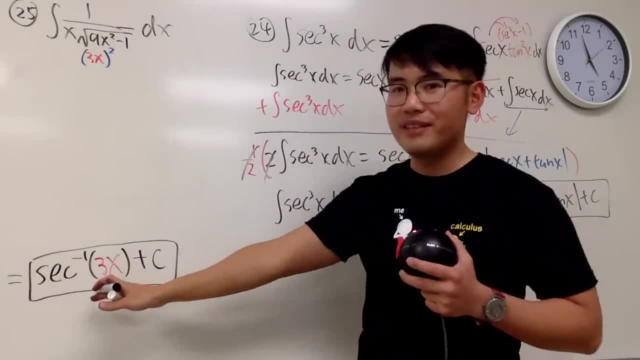 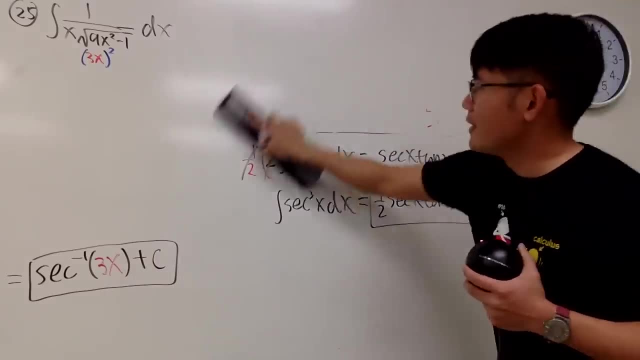 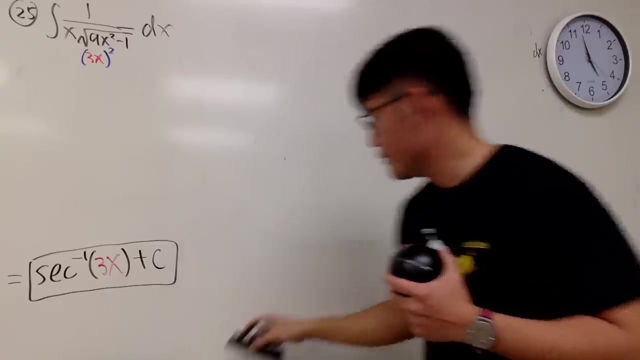 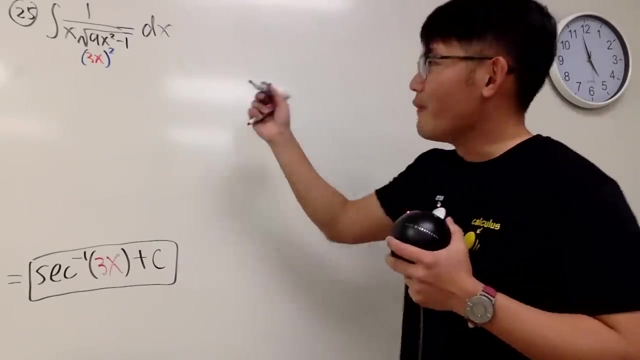 Whenever you have the integral in this form, you have the inverse secant. Seriously, that's it, But I will still show you guys the trick. sub right here for you guys, real quick, All right, Okay. So first of all, notice that you have something squared minus 1,. 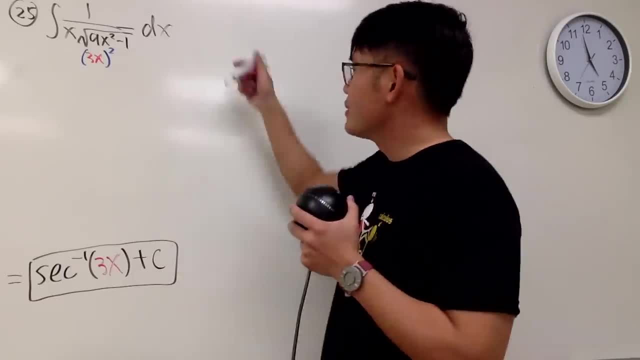 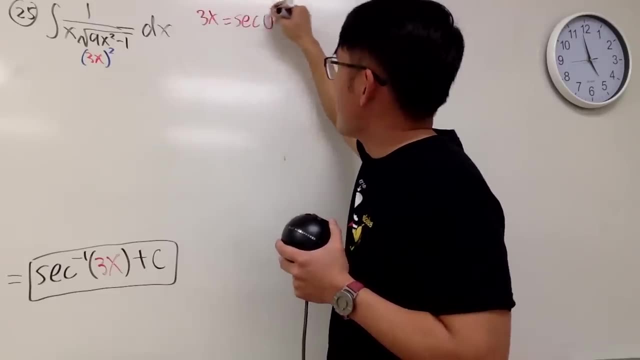 and the goal is you want to use the secant to help you out. So I will put this down right here for you guys. I will say: put this right here: 3x to be secant, theta, All right, And of course I want to get the dx. 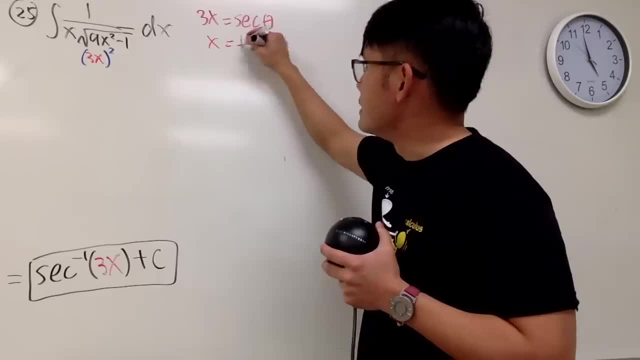 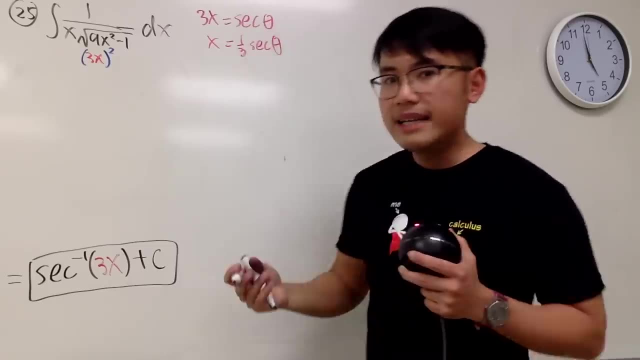 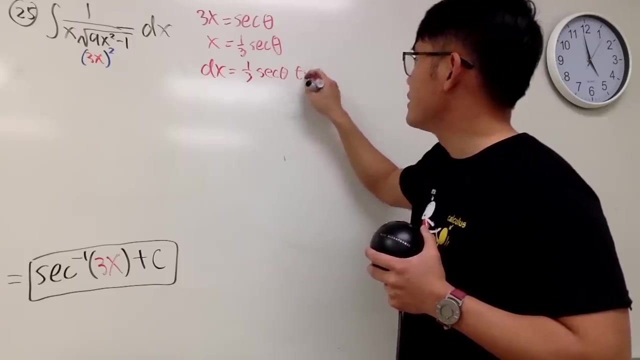 so I will So divide both sides by 3.. So x is 1 third. secant x I mean secant theta, And I will differentiate both sides. So dx is equal to 1 third. This right here will give me secant theta, tangent theta, d theta. 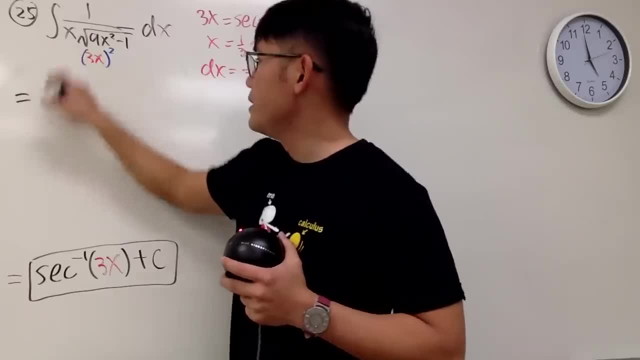 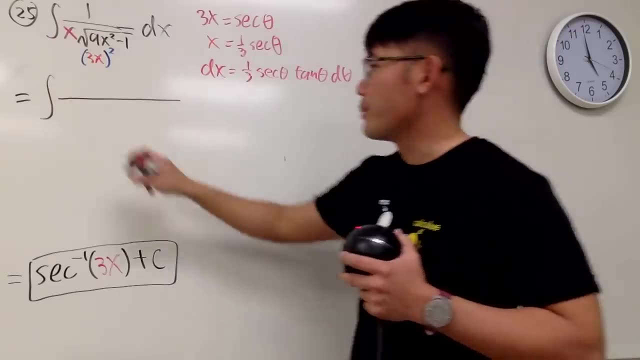 And I will take this to the theta world. You will see, this is going to be the integral For this x. well, it's 1 third secant theta, So I'll put this down right here: 1 third secant theta. 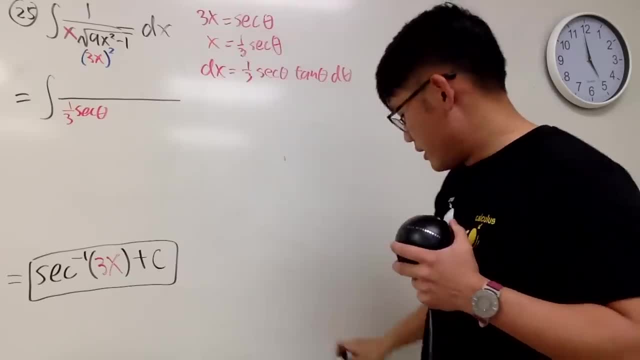 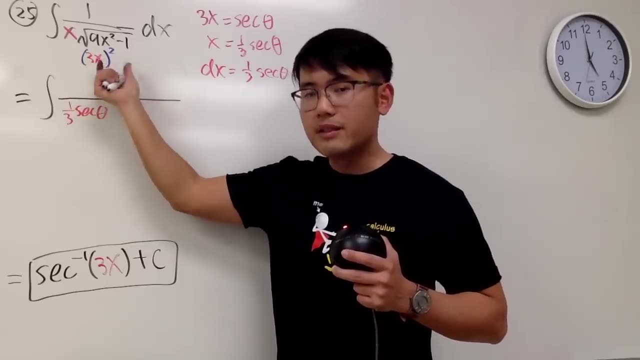 And, as I said, if you put this right here, the secant theta for 3x and then you square that, you get tangent square inside because you have the minus 1 after that Secant square theta minus 1 is tangent square. 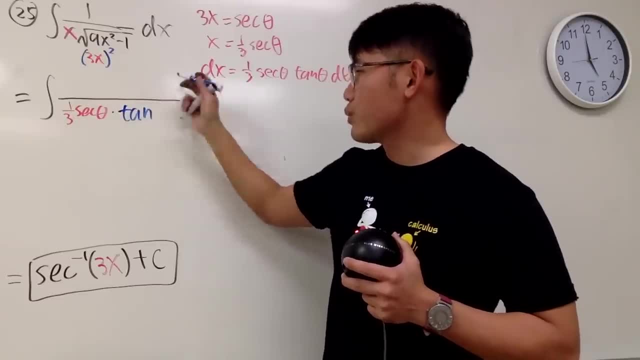 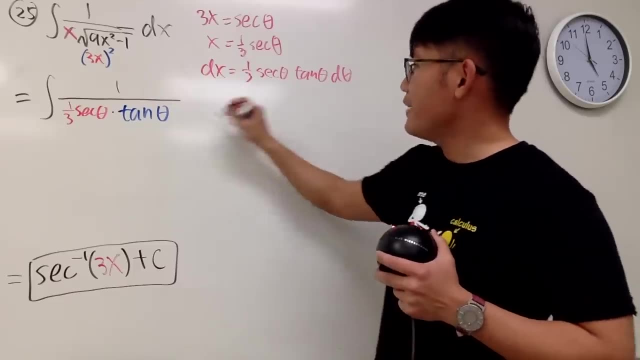 And in the square root, you just get regular tangent, Tangent to the first power like that: Right, All right, On the top of course you still have 1.. And over here you have the dx being this, which is the same thing: 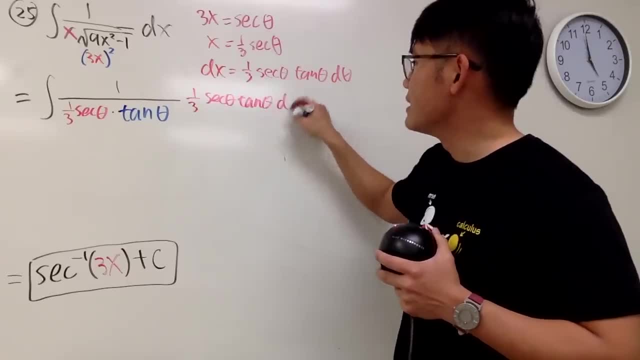 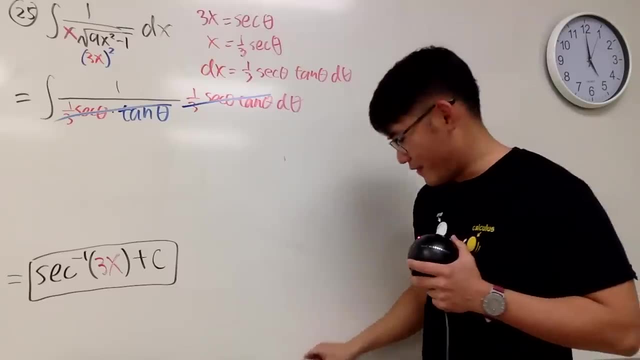 1. third secant theta, tangent theta d theta. And yes, you got it, We can cancel these guys out. Very nice, Very nice, Very nice. So you are just looking at the integral 1 in the theta world. 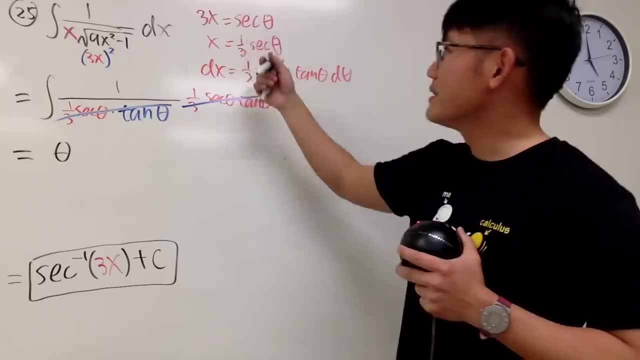 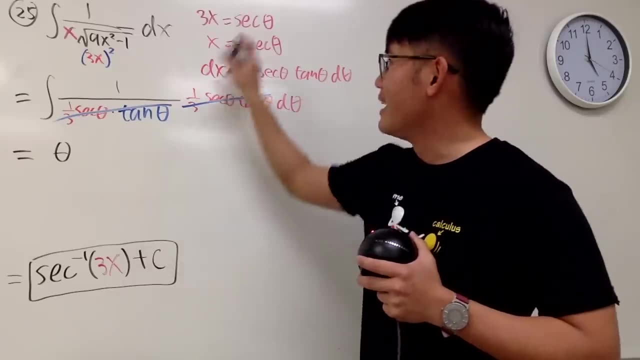 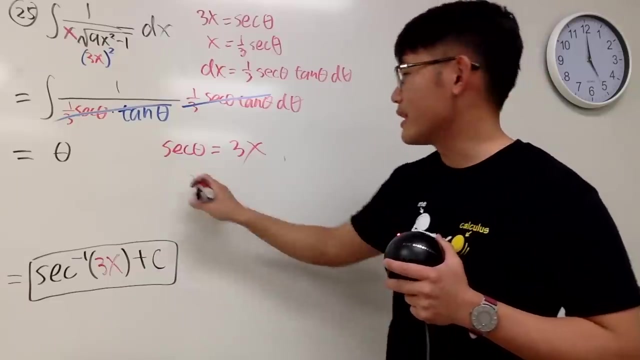 which is just going to be theta, And because, oops, this is good to well. actually, no, I'm right, All right, Theta. So you see we have secant theta being 3x. Take the inverse on both sides. 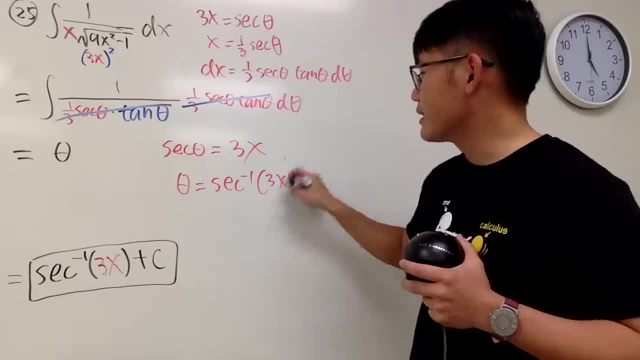 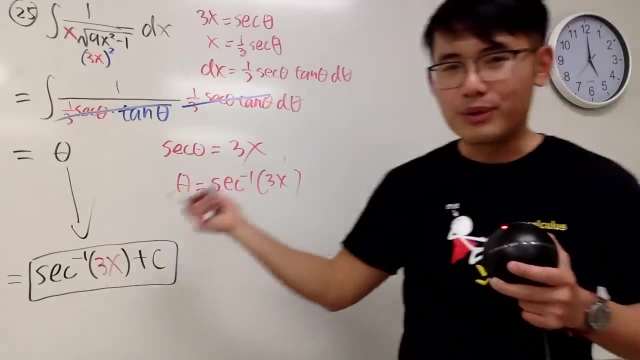 and you're going to do a theta is equal to the inverse secant of 3x. So you are done right there. So up to you And depends on your situation. Maybe you have to show the work, maybe not. 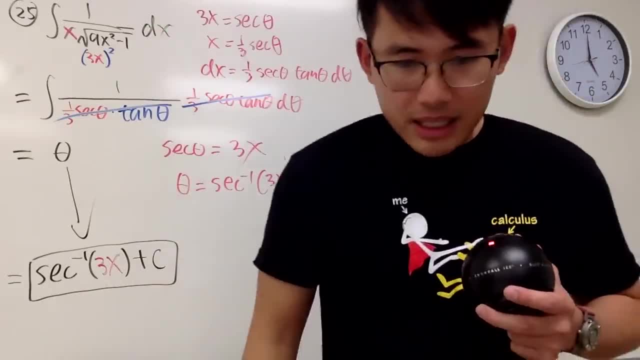 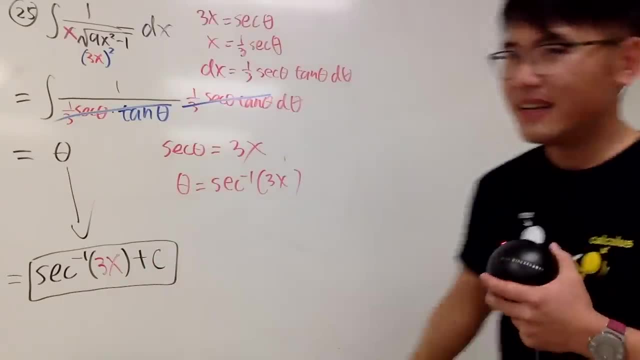 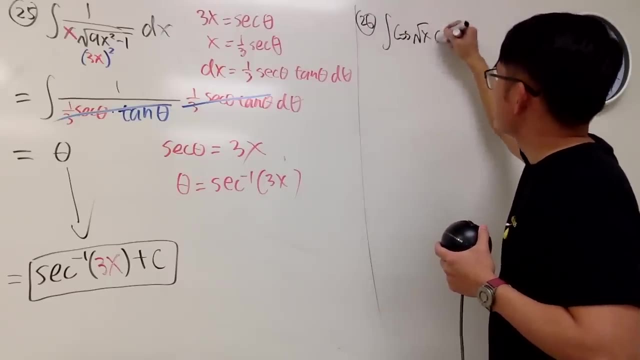 But you know you can actually go from here to there right away, All right. Next one Cosine of square root of x. All right, Let's see how to deal with this. 26 integral of cosine square root of x, dx. 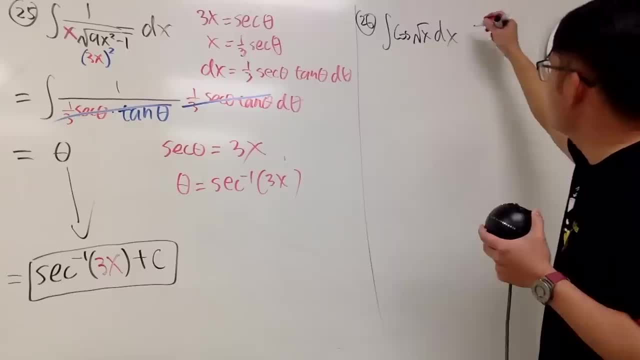 It seems that I don't know what to do in the x world, so I'll take this to the u world real quick. I'll take u to be square root of x and I will square both sides, and I get x is equal to u squared. 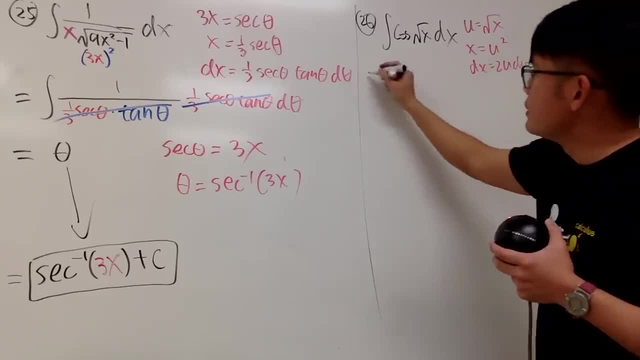 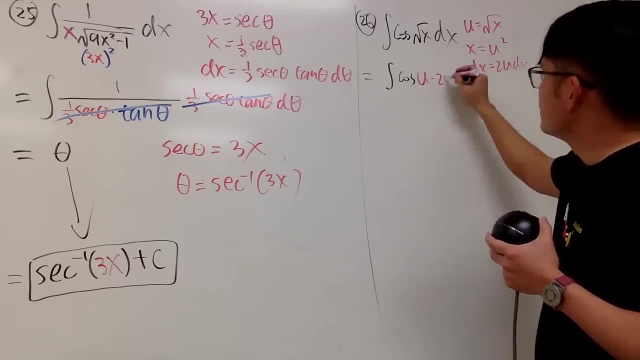 and then dx is equal to 2u du. So, as you can see, this is going to be the integral of cosine, and then the input is u, and then we multiply by 2u, 2u du, And I will do the following. 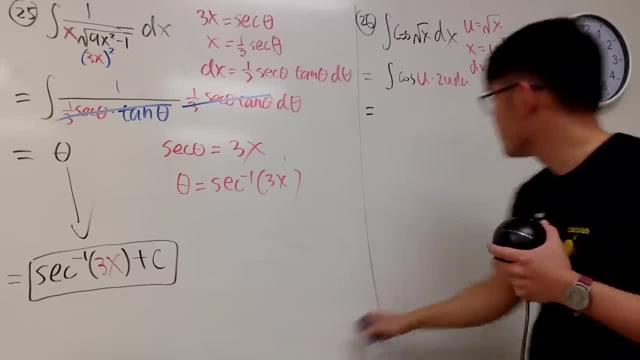 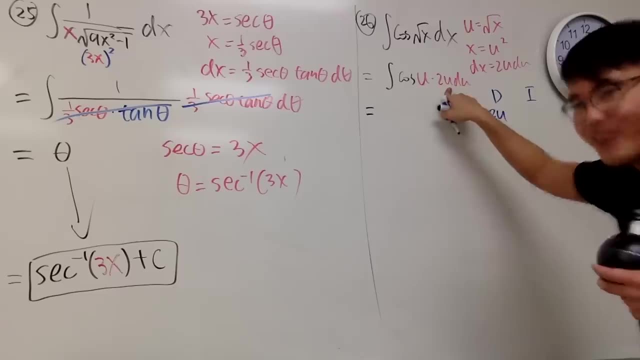 We can do integration by parts right here. That's very nice. So I'll put this down in blue. So d and then i. I will be differentiating 2u. Okay, I'll take the 2 with me as well. 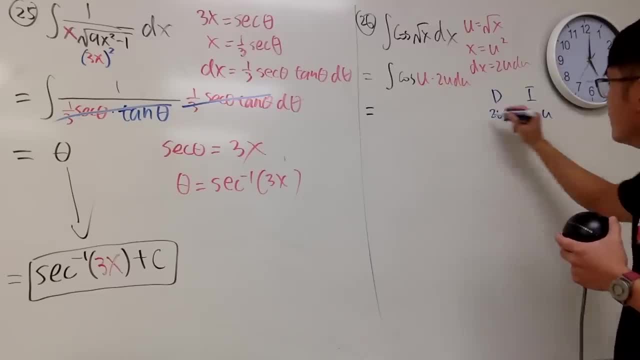 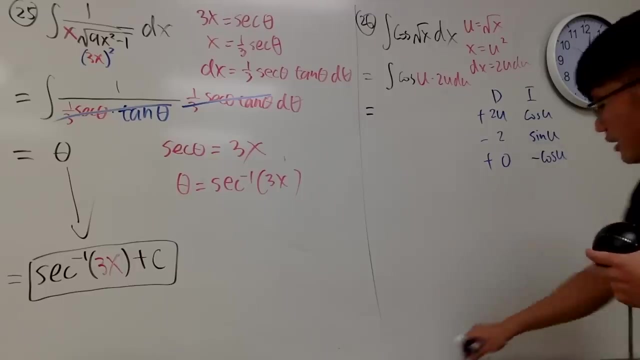 And then I will be integrating cosine u plus minus, plus, Differentiate this, differentiate. that That's it. Integrating cosine u, you get positive sine u, and then integrating sine u, you get negative cosine u. So you have this, and that being our answers. 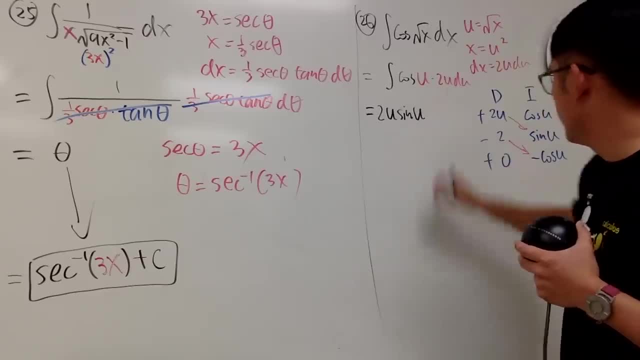 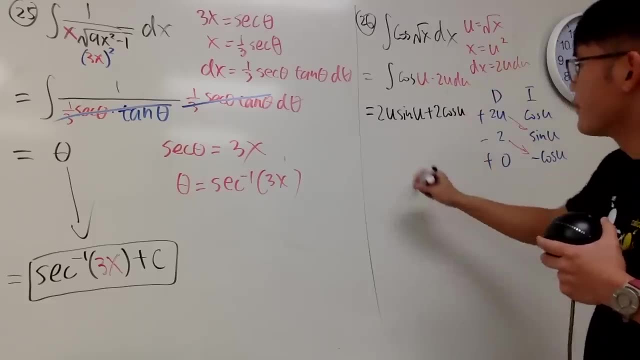 So let's see we have 2u sine u and then negative times. negative is plus 2 cosine u, right, And of course in the end we put the u back, which is 2 times the square root of x. 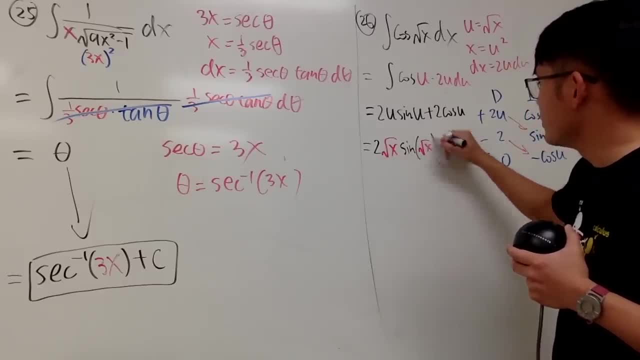 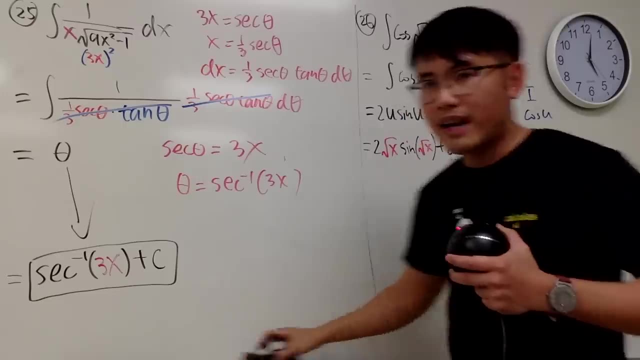 and then we have the sine of the square root of x for the u, and then right here we add 2 cosine of square root of x, like this. So we are done. I will erase my d-i method right here. 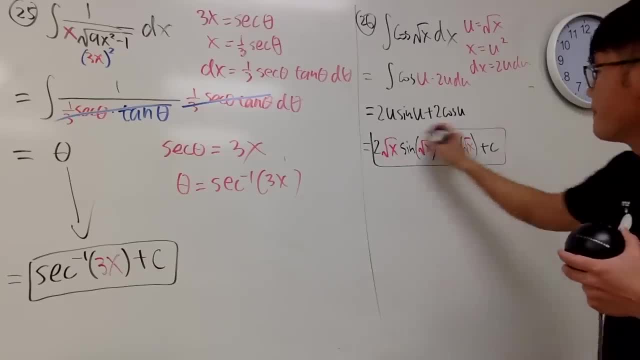 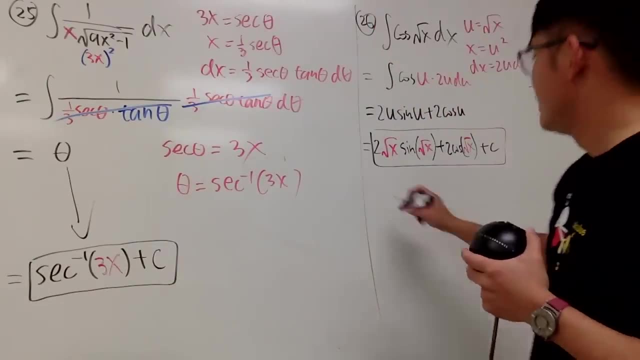 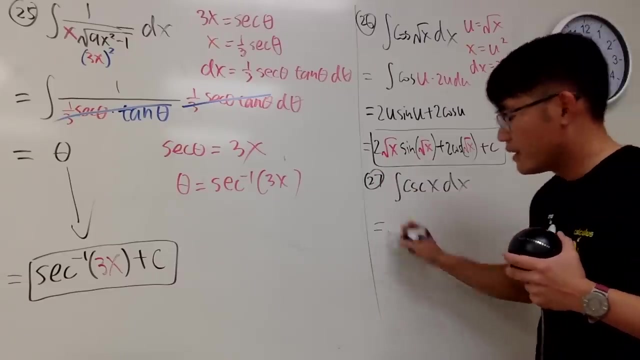 And we just put on plus c, like this. It wasn't too bad, isn't it? Okay, good Cosecant, Okay, cosecant, Cosecant x, Integral of cosecant x, dx. Cosecant should remind you of secant. 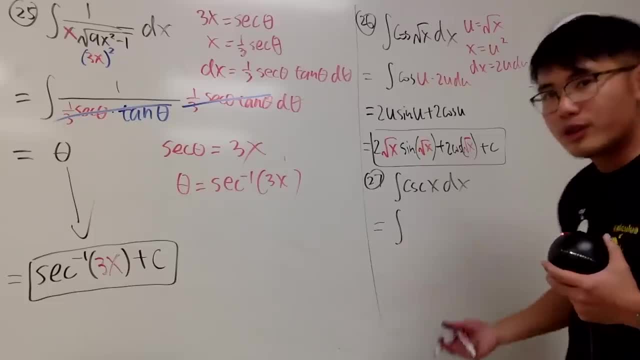 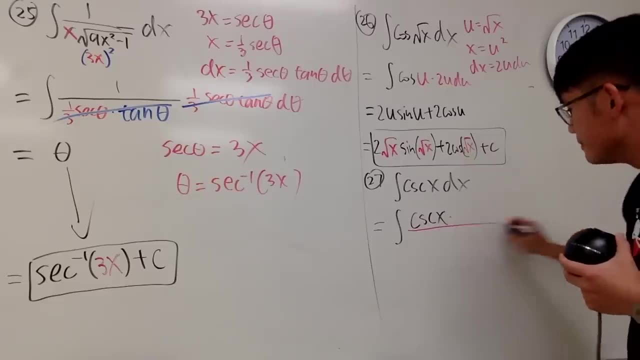 And, yes, the way to integrate them are very similar. but I will show you guys the standard result. I will look at cosecant x and I will multiply the top and bottom by cosecant x minus. Technically, if you want to do plus, it's okay as well. 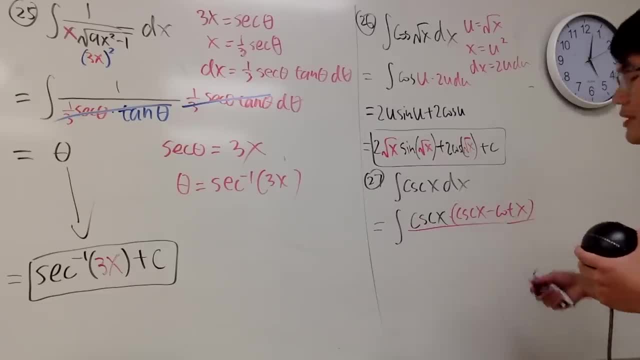 I have a video on that, if you guys want to see Cosecant and tangent. I mean cosecant and cotangent are best friends in integral, so you subtract them in this case And then you have the minus cotangent Cosecant x. 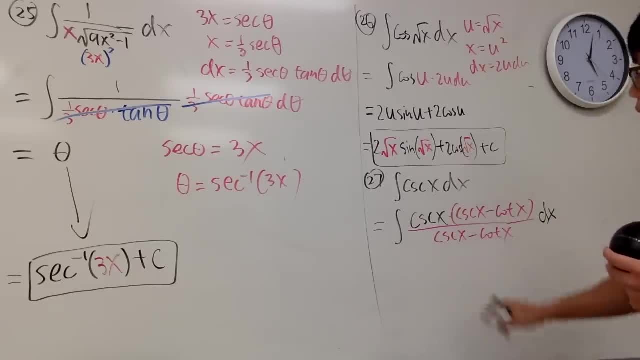 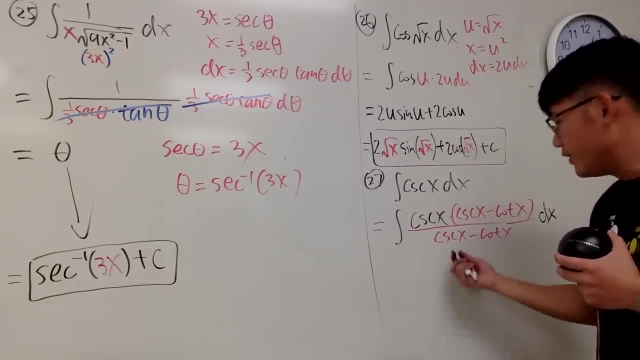 Right, And you have the dx, of course. Check this out: Here you get cosecant squared and then negative cosecant cotangent. If you differentiate this right here, you end up with negative. Let me just write down this for you guys: 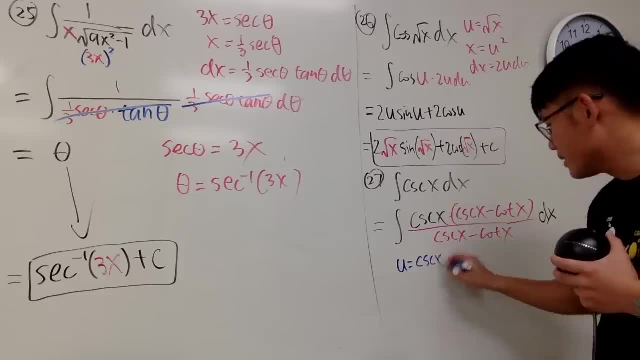 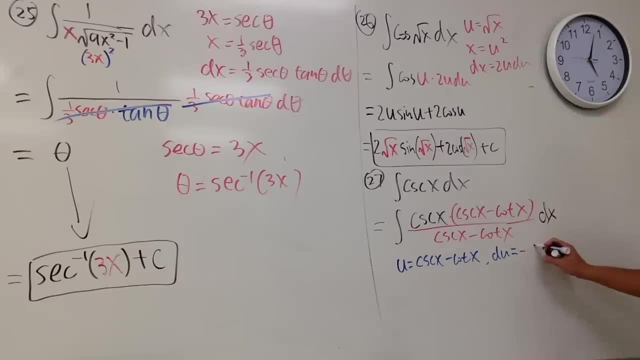 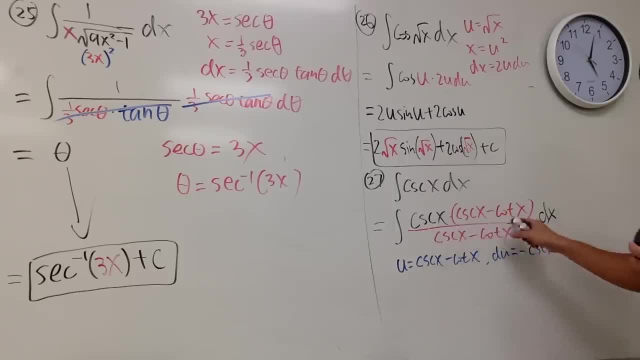 du will be. the derivative of this is negative. cosecant x, cotangent And you are going to get that on the top. You see Negative this times that This is going to be for that And you are going to differentiate this. Negative times the derivative of that, which is going to be positive. 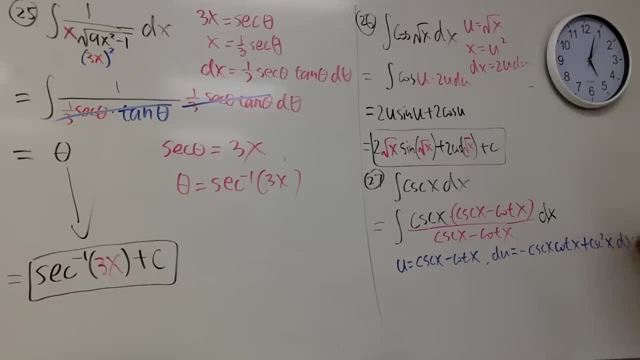 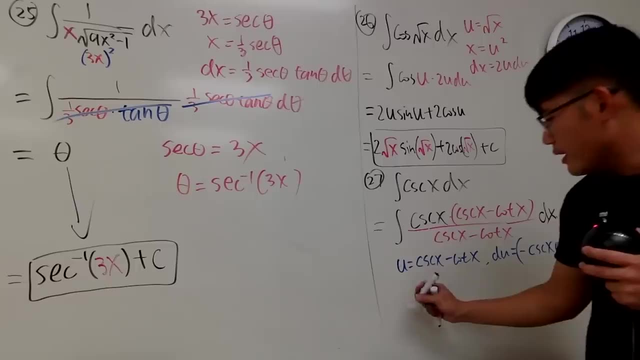 cosecant squared x, dx. So the point is that this is the same as the top After you distribute it and then you take u to be this. so in the end you have to integrate 1 over u, which is going to be natural log of u. 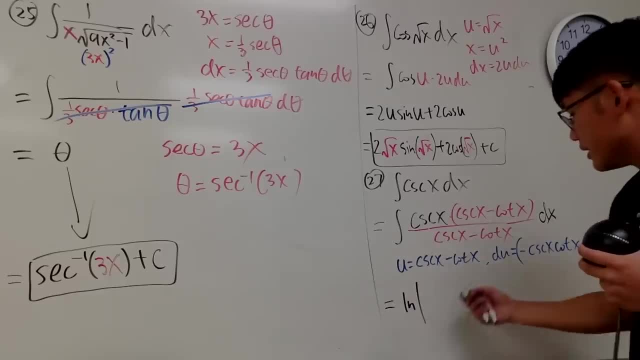 Which is the opposite of u, And then the u is the denominator, which is the cosecant x minus cotangent x, And then you are done. Put a plus c, And it depends If you are in a hurry or not, or maybe if you don't need to show work. 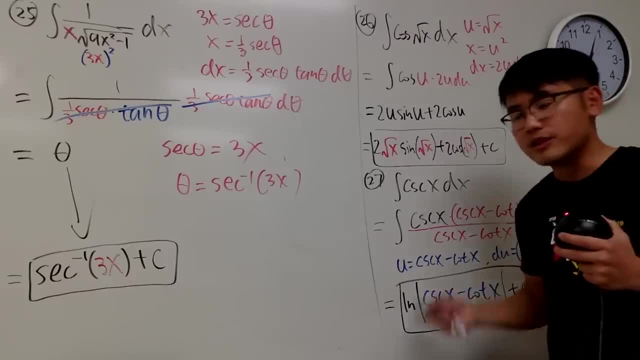 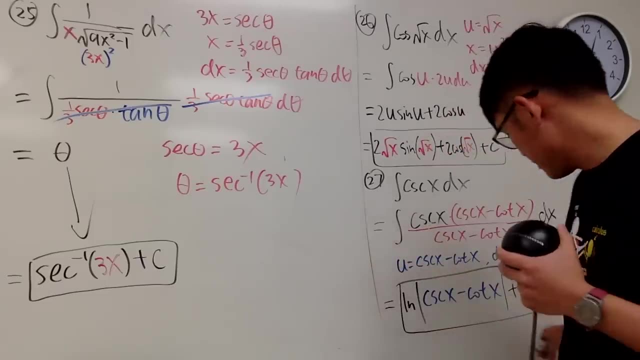 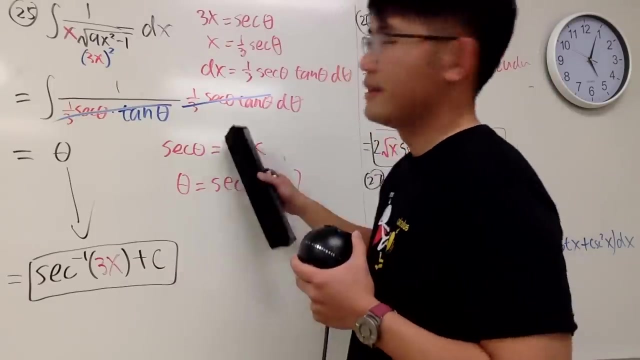 then you can actually just go from here to here. This is the standard result that you guys can just quote and be happy with it. I think that's the deal for many situations. Okay, So 27 already. We have 73 more to go right. 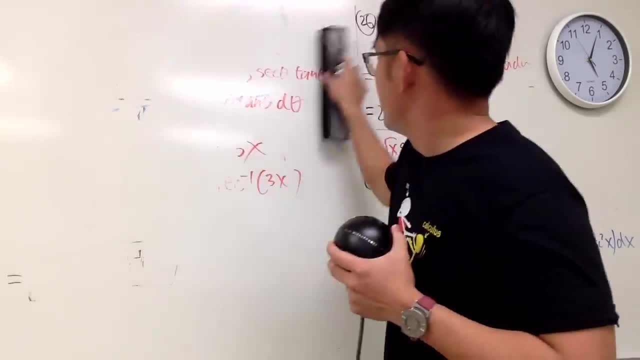 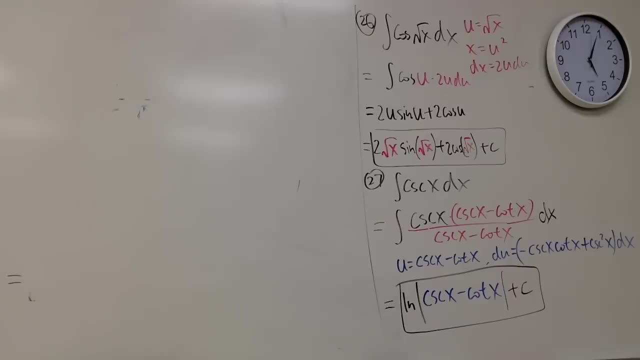 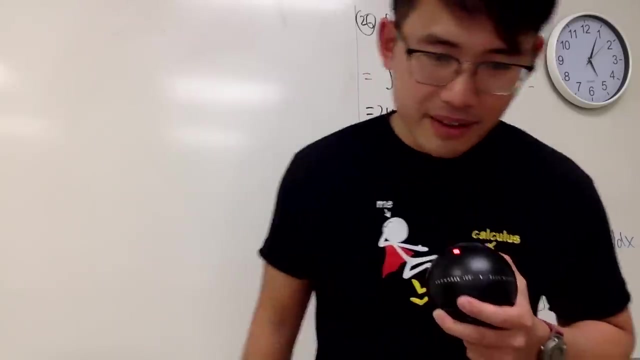 Let's see. Let me see how the- Yeah, My iPhone is still recording. That's good, Good news, Okay. 27.. And now we have 28.. Let me put it down right here for you guys: 28. 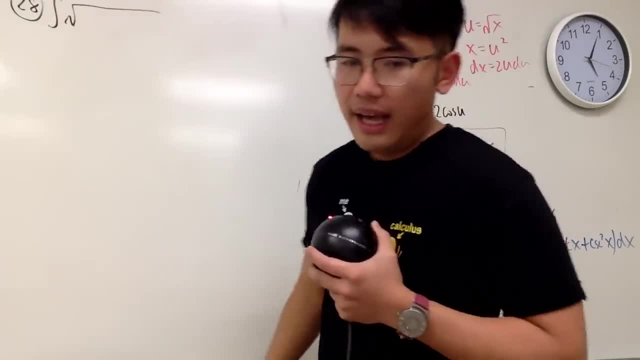 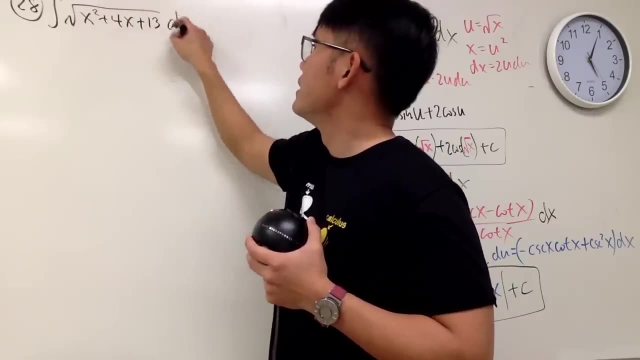 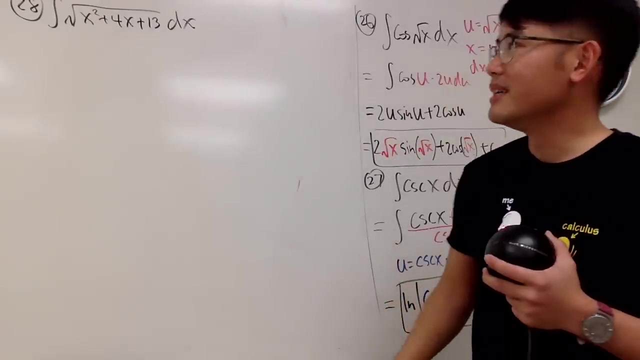 And then we have to integrate square root of x squared plus 4x plus 13 dx. Not yet, Don't do tricks up yet. In fact we have to complete the square because we have three terms inside, So let's go ahead and complete that. 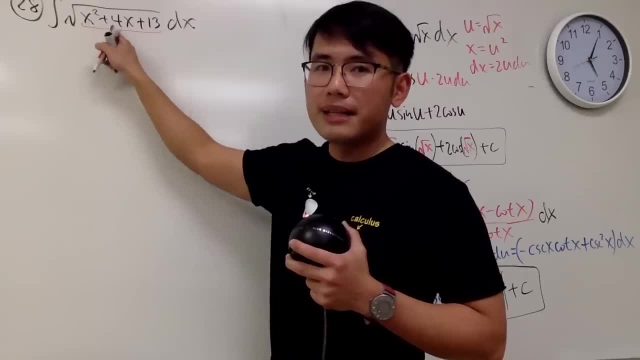 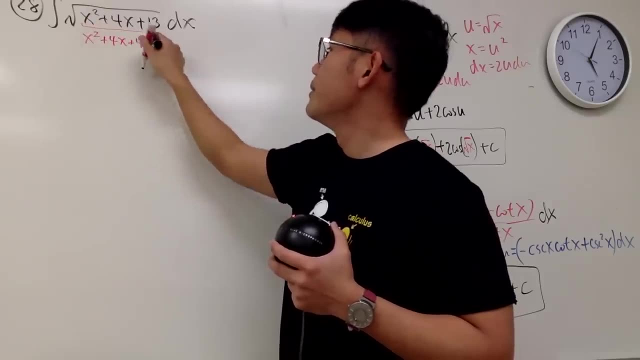 Well, look at this right here. You know you have to have x squared plus 4x plus 4.. Look at this as x squared plus 4x plus 4.. And then to get 13,, of course, you have to put a plus 9.. 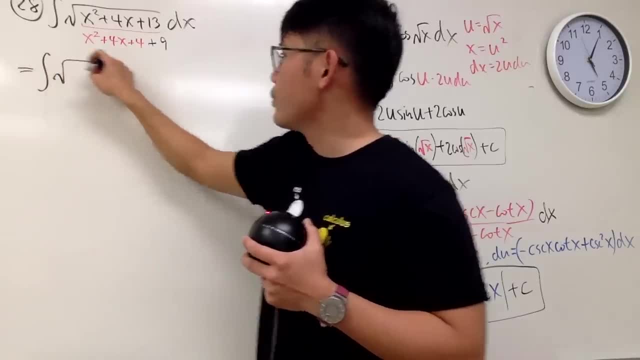 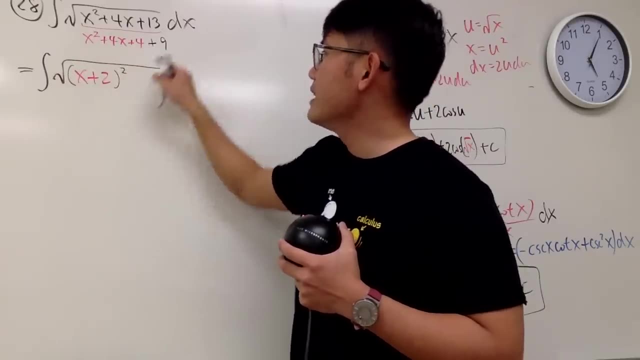 So in another word, we can look at this as the integral or as the square root: This, this and that will give us parentheses with x plus 2 inside, And then square that And then the 9 will be plus 3 squared. 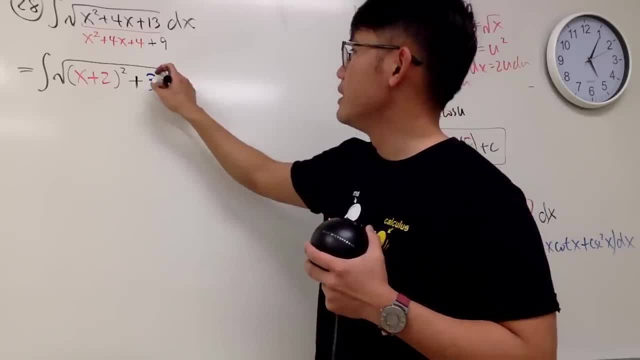 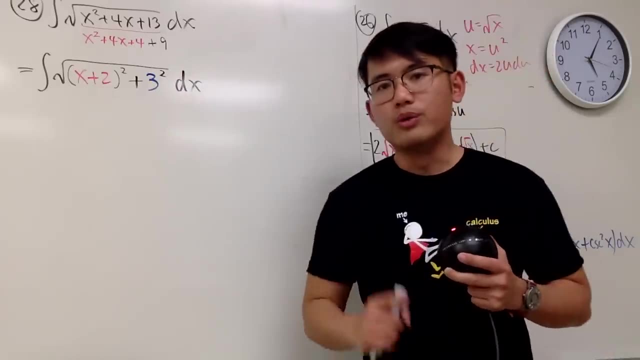 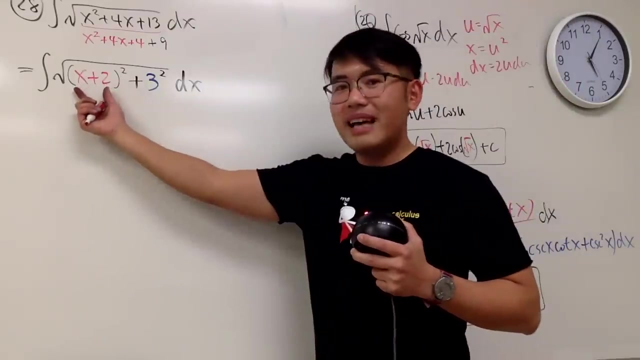 This is pretty nice. So put a plus 3 squared like that, Okay. And then, of course, we have the dx next to it. Now we do tricks up. Well, here is the small trouble. Yes, you take this as the? u. 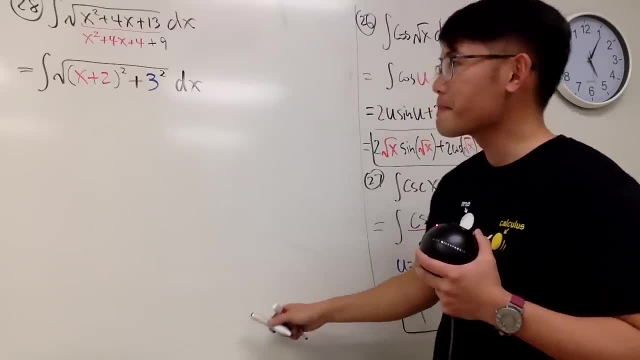 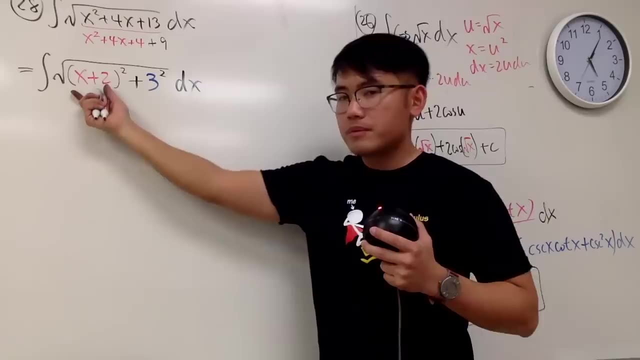 So I will actually just skip that part. Okay, But notice, we don't just add plus 1 squared, We are adding plus 3 squared. So you want to get this to be well tangent, Because tangent squared plus 1. 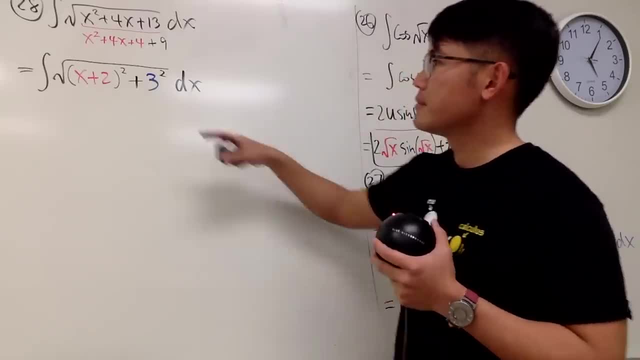 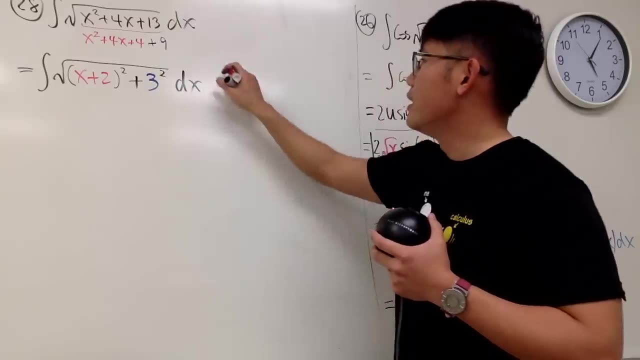 will give us secant squared, But you want to match with the 3.. So the one that you have to do is you have to take this right here, Name the x plus 2.. You have to set this to be with the 3 in front. 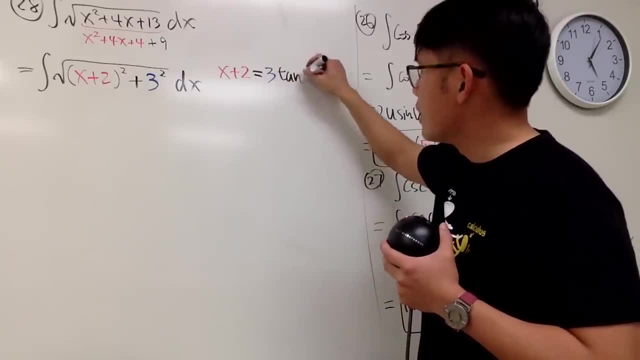 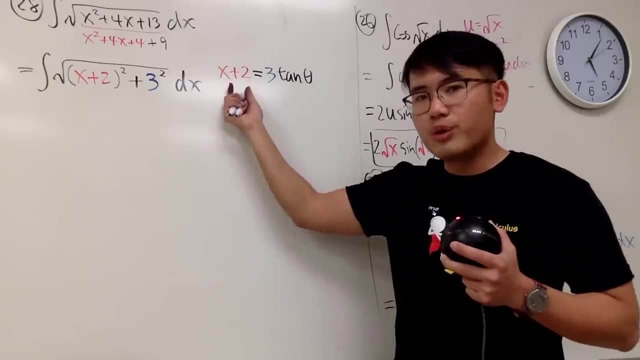 when you multiply this and then the tangent theta: Okay, Again, take this. If you want to do u sub, it's up to you, But you can just put it right here real quick. And then you have 3 tangent Because, again, you have this right here. 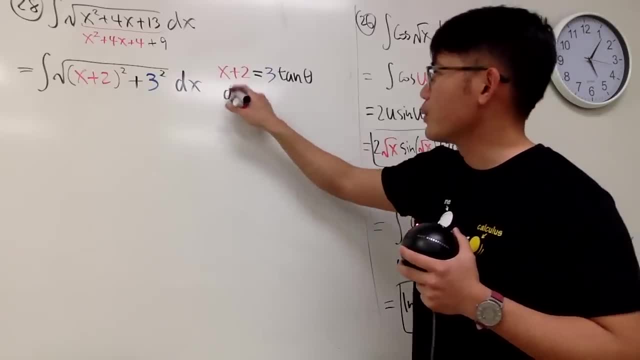 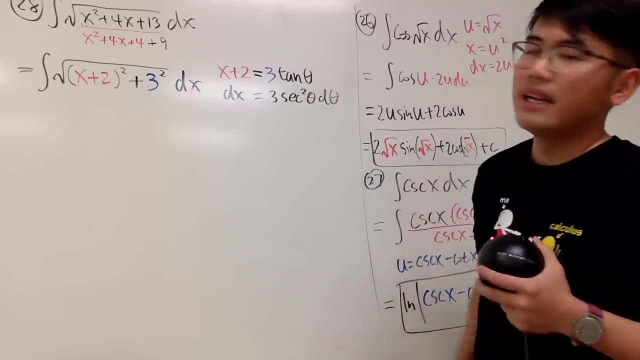 And I will differentiate both sides, because this right here will give me dx right away anyway- And the derivative of this is 3 secant squared theta d theta. Now we go to the theta world, So we will have the following integral of square root: 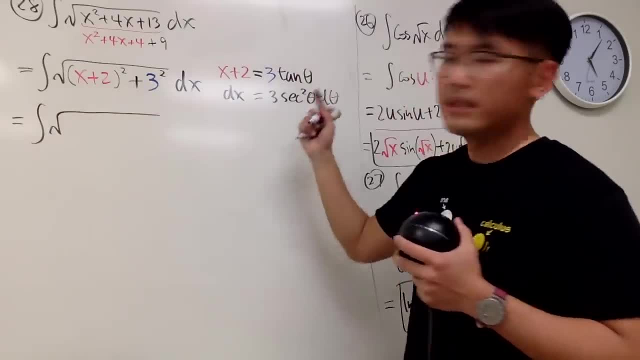 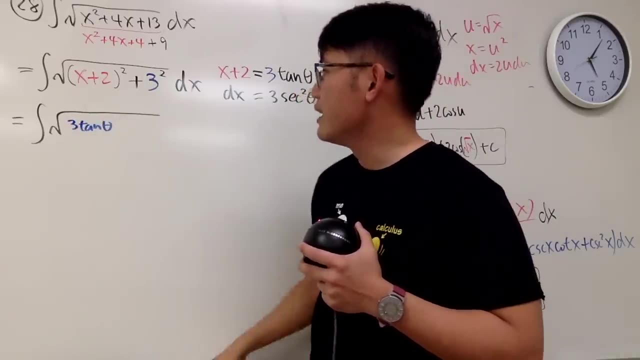 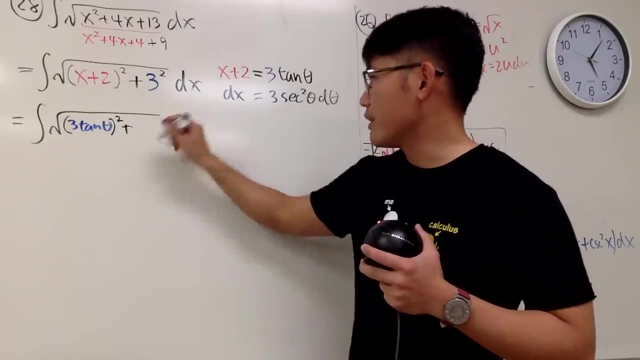 This right. here is the 3 tangent theta, right, So I will put this down. I think we'll just do it all in blue for you guys: 3 tangent theta, And then you are going to square that, And then you are going to put down plus 3 squared from earlier. 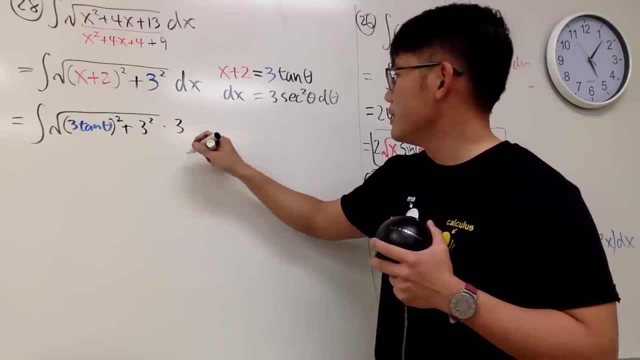 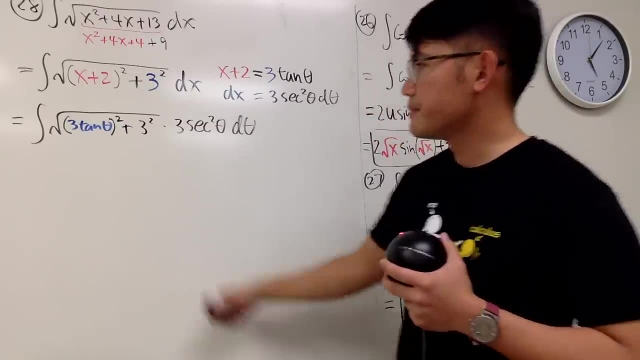 times dx is all that. So multiply by 3 secant squared theta d theta like this. Okay, Here is the real. Let's do this in your head. You'll get 9.. You'll get 9.. 5 times 9.. 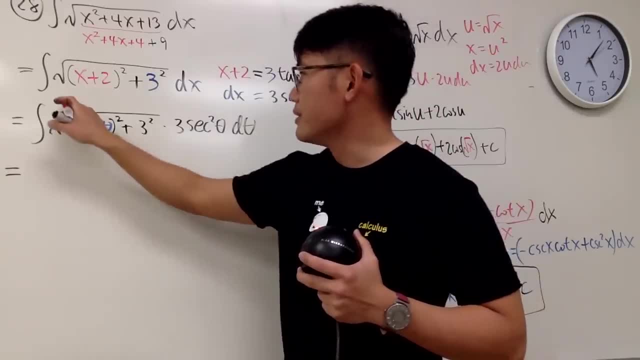 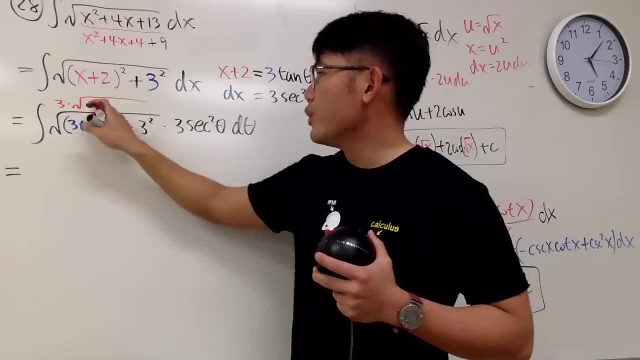 Take the square root of 9. You get 3.. Okay, You have a 3 right here, So you give me 3 times, And then you have the square root, Tangent squared plus 1.. As I said, you will get secant squared theta. 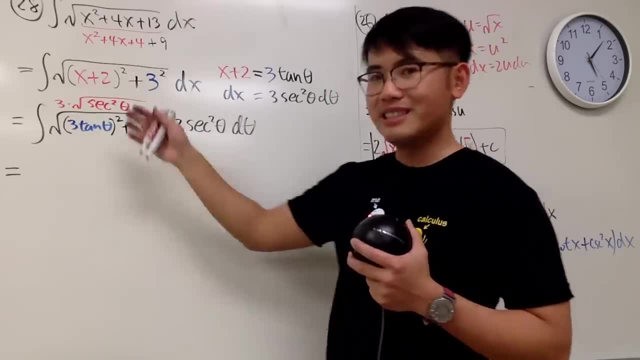 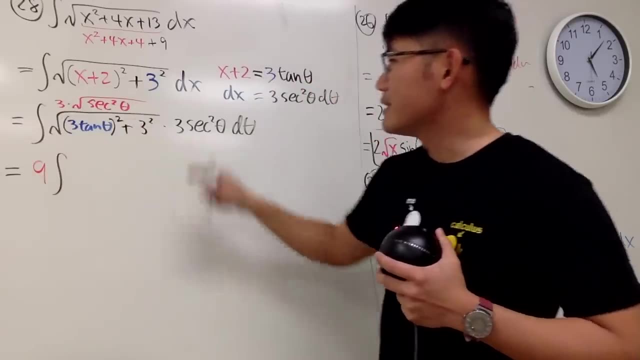 And when you cancel the square with the square root, you get secant to the first power. Anyway, oh no, 3 times 3 is 9.. Put that all the way in the front, And then integral, And then this times that is secant to the third power. 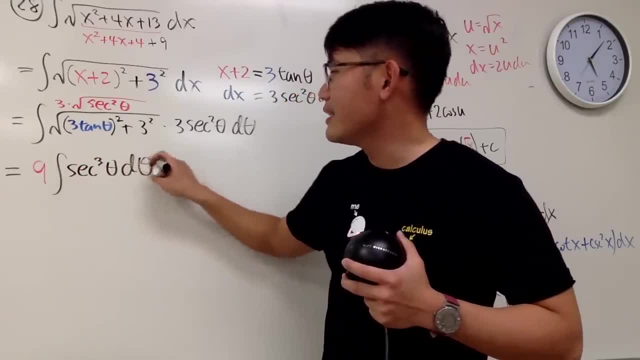 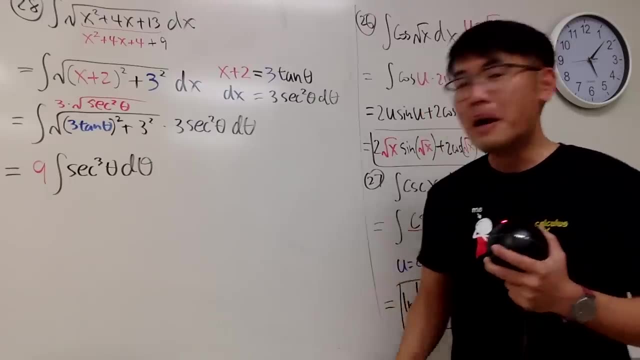 So you put down secant to the third power, theta d theta. Oh my god, I'm dealing with the secant to the third power in this data world. But the good thing is that we can do this. Okay, We can do this. 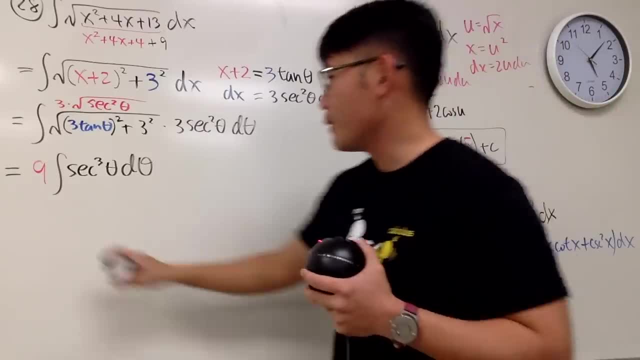 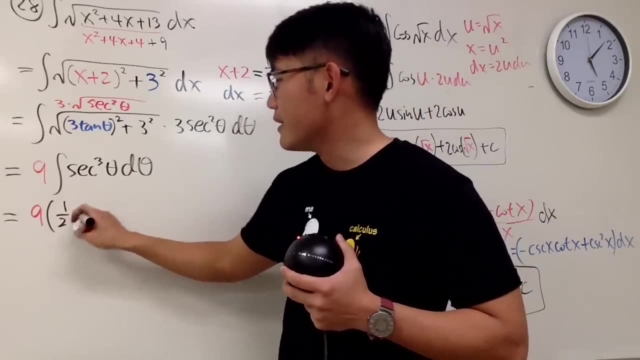 Okay, We can totally do this, because we did that earlier, So I'll put down the answer for you guys. All right? So here's the deal: 9.. And I'll write down the answer right here, which is: 1 half times secant theta, tangent theta. 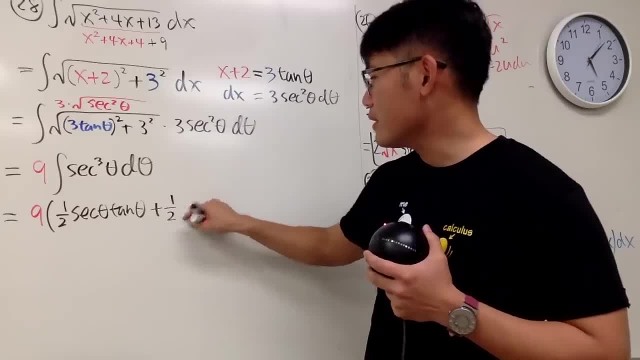 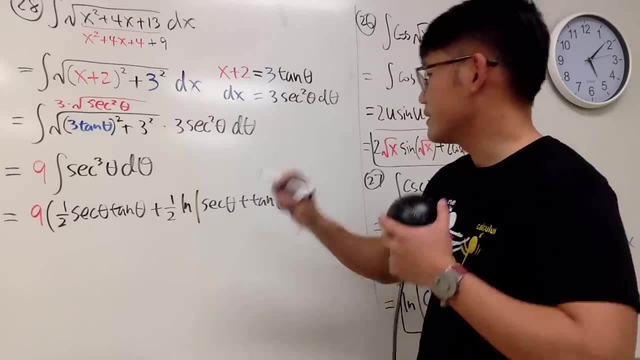 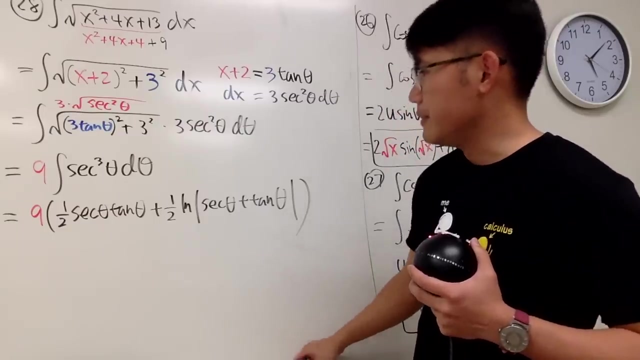 And then you add 1 half Natural log Absolute value, Secant theta plus tangent theta in the absolute value, like this: In the end we have to go back to the x world. This right here is slightly trickier. So let's see. 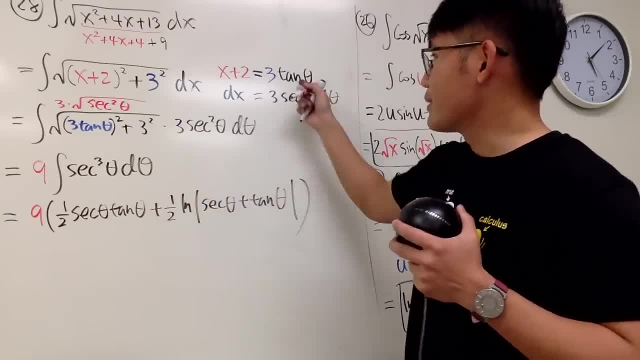 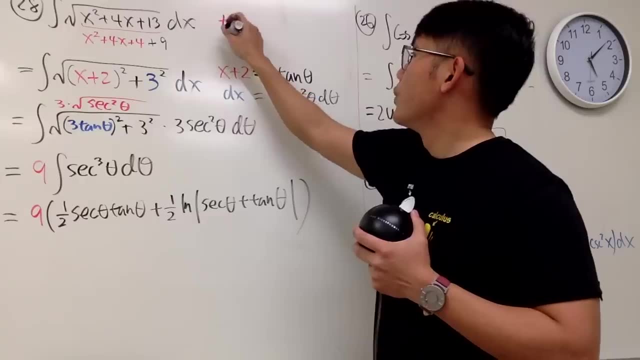 Secant theta? I don't know, I know tangent theta is this, So check this out. So let me put this down right here for you guys. I'll put this down. Great, We know tangent theta. We can divide both sides by 3.. 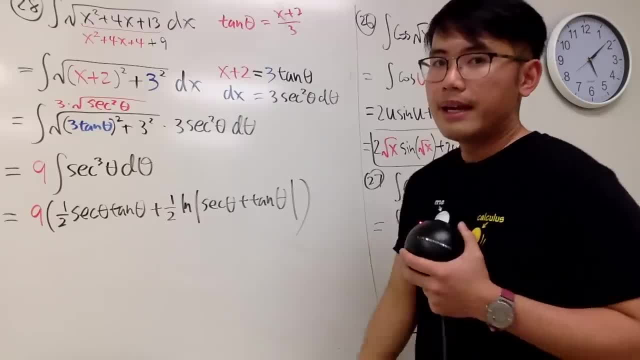 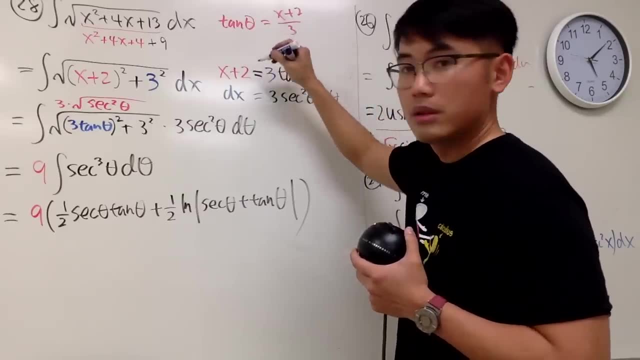 In other words, we get x plus 2 over 3.. Right, And from here we can draw a right triangle, And I'll put this down in blue for you guys. now, Why not Let me put down a triangle here? 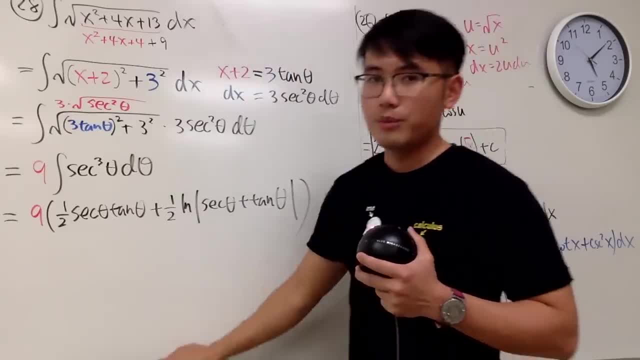 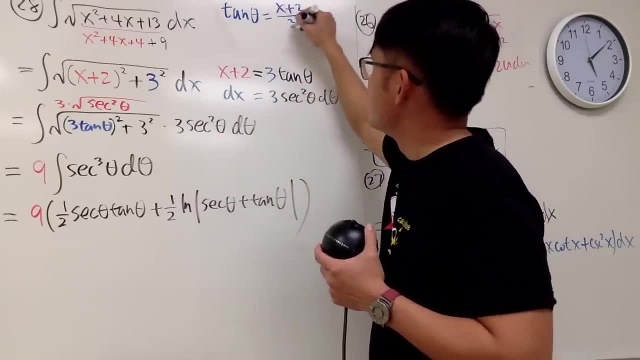 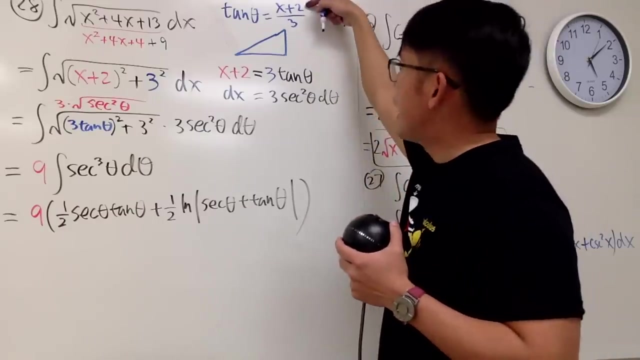 Actually, let me just write this down a little bit above, so I can have more space. Tangent- theta equals x plus 2 over 3.. And now draw a right triangle right here. Tangent is what? Yes, Tangent over adjacent. 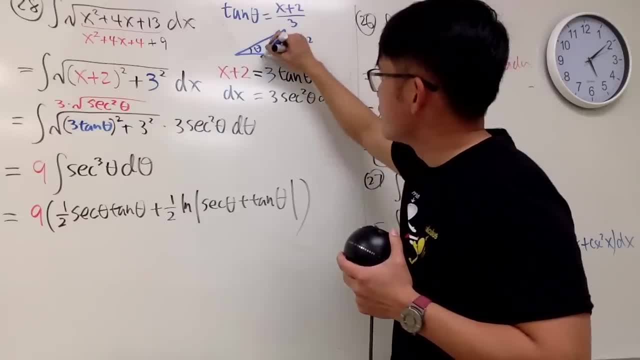 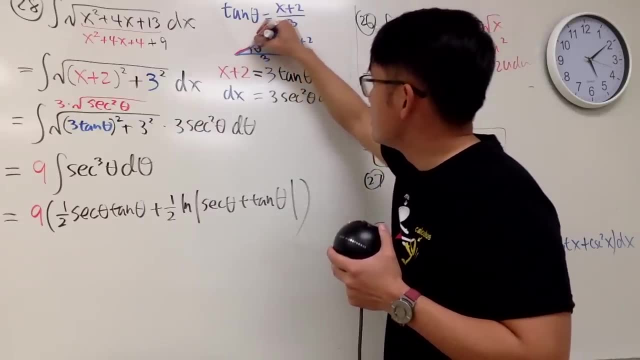 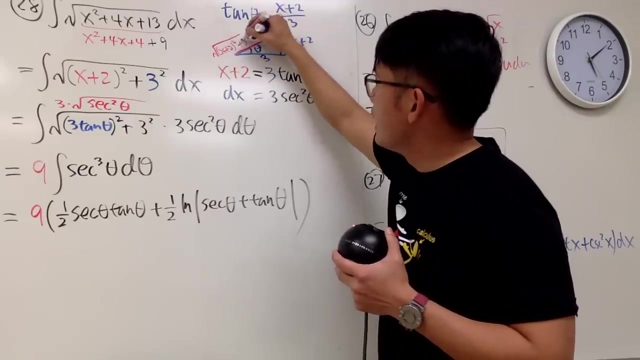 So you have the angle here. This will be x plus 2.. This right here will be 3.. That's very nice, And we also have to figure out the hypotenuse. Of course, this right here will be the square root of parentheses: x plus 2 squared plus 3 squared. 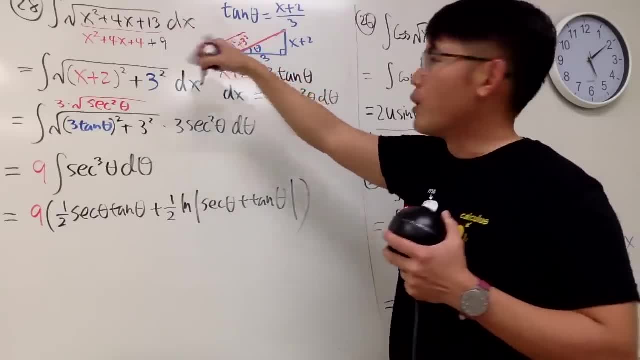 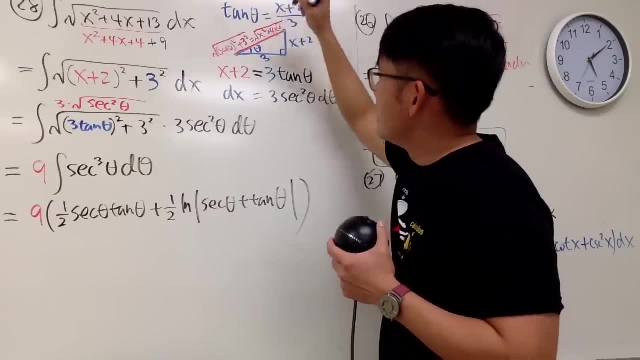 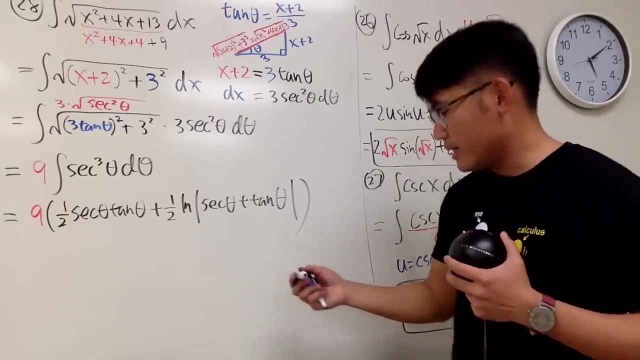 And guess what? This right here is exactly our original. So this right here is just the square root of x squared plus 4 squared plus 13.. Right Now, let's do the usual business. I'll do this in black and blue. 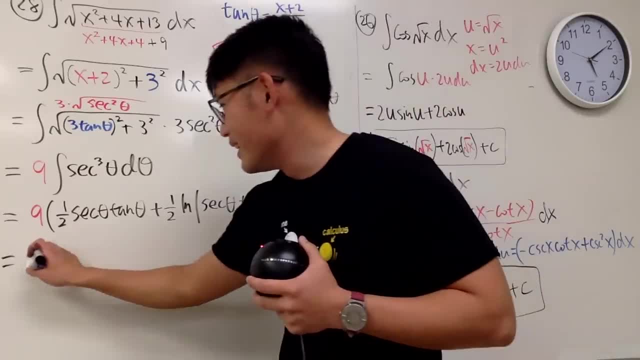 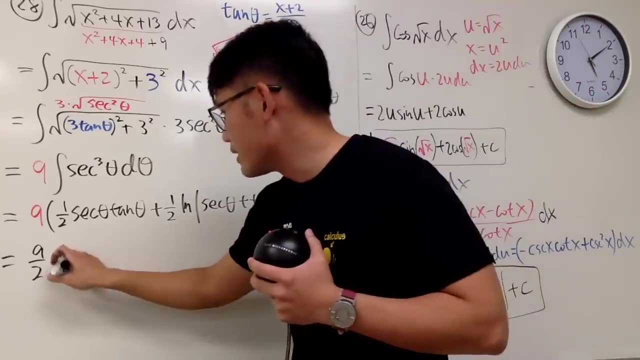 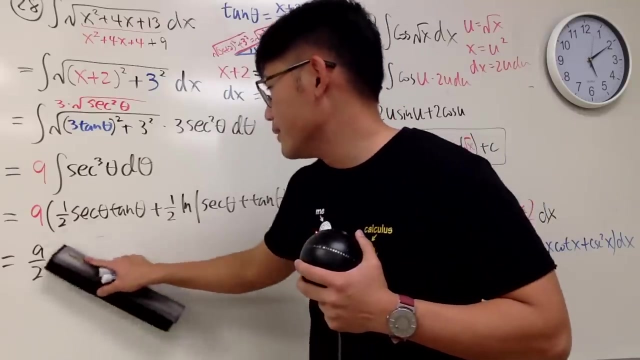 First, 9 times 1 half. Do the easy one, of course: 9 over 2.. Tangent theta is hypotenuse over adjacent, So you have this over that. So, in other words, you get square root of x squared plus 4x plus 13 over 3.. 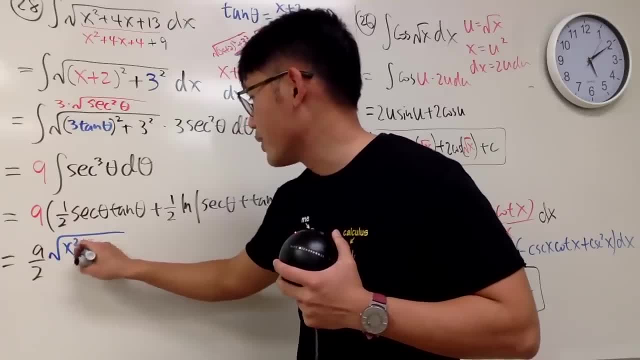 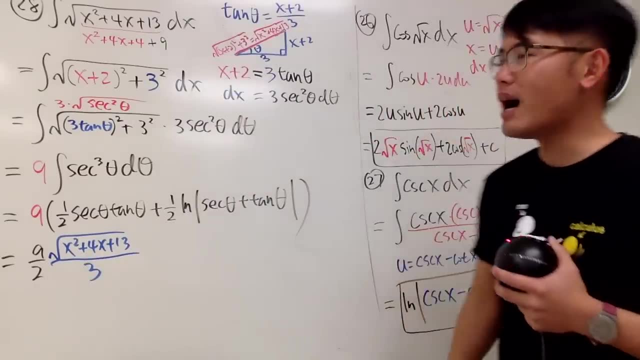 Right, I've already done it in the wrong color. I told you I was doing it in blue, So let's see, Like this Over 3.. Tangent theta is what 9x squared x plus 2 over 3.. 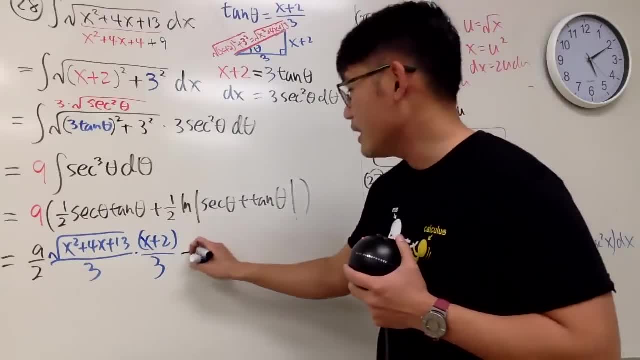 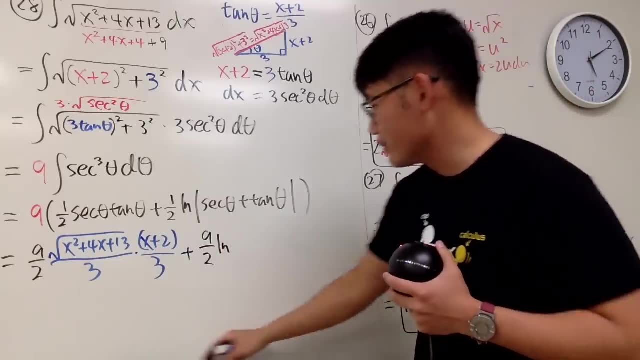 Right, And then it's going to be the same for the rest, Plus, don't forget to distribute, Otherwise it will suck 9 over 2.. And you have the natural log: absolute value. Secant is this again. 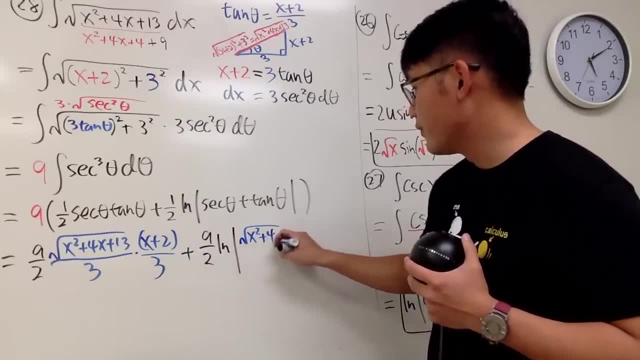 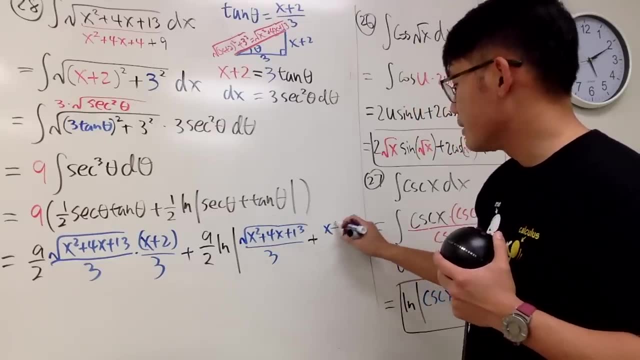 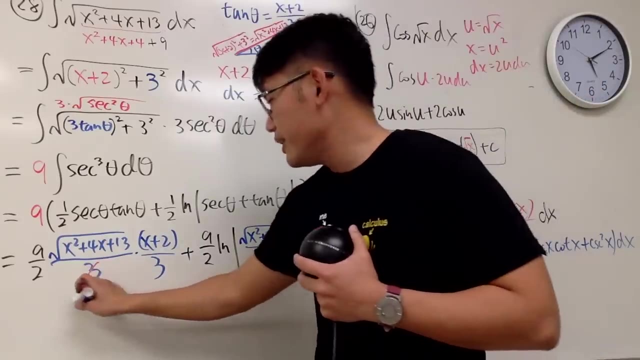 Which is the square root of x squared plus 4x plus 13 over 3.. And then, lastly, we have plus x plus 2 over 3.. Right, Not done yet. 3 times 3 is 9.. 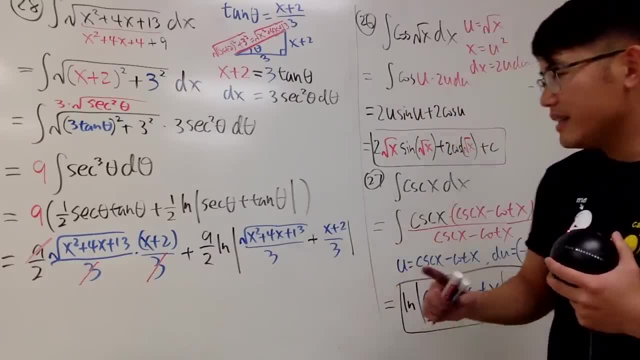 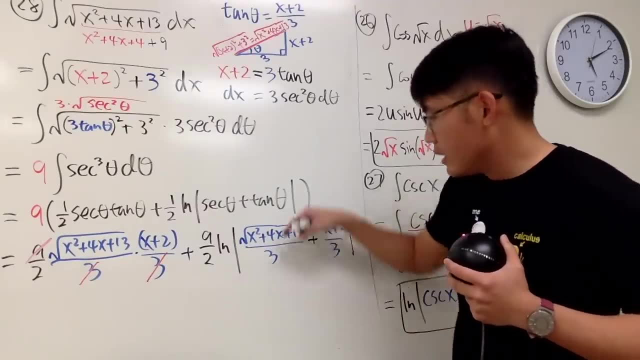 Can be cancelled with that 9.. Right, So that's good. And here is the deal. Right here, As you can see, I can put this down together into this: plus that, or over 3 instead of the natural log, When you have a quotient instead of the natural log. 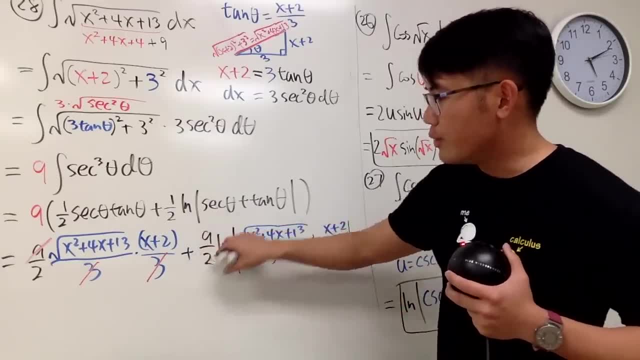 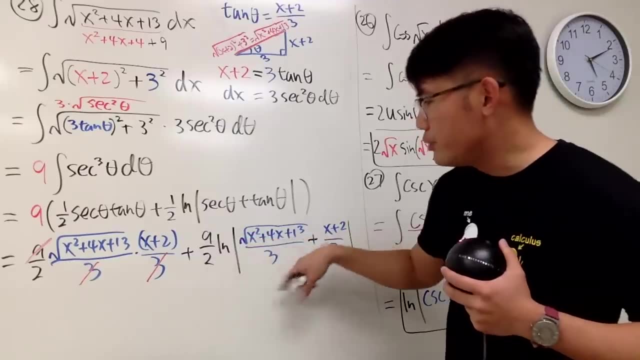 You can write this down as 9 over 2 natural log of the top, minus 9 over 2 natural log of the bottom, But the bottom is 3.. So you have 9 over 2 natural log of 3. Which is just a constant. 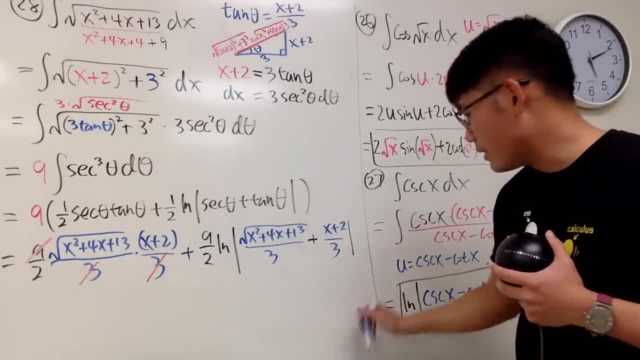 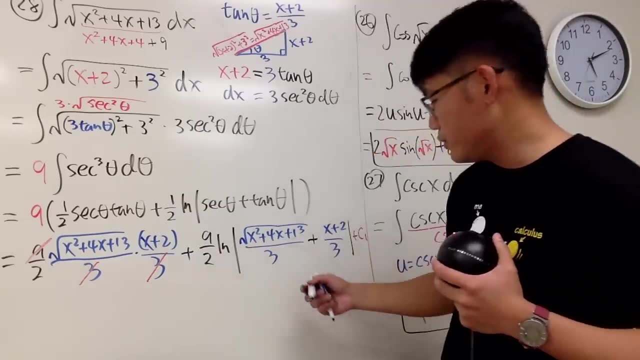 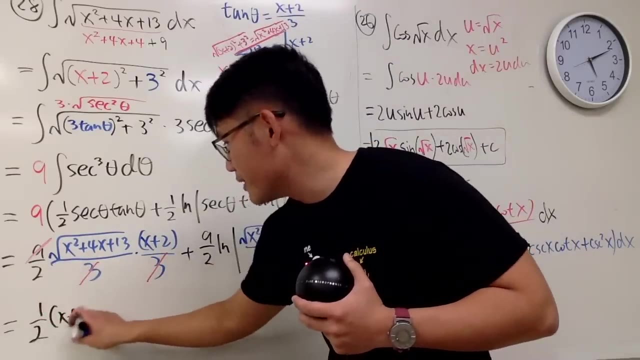 So right here, if you would like, you can say this is plus c1.. Put down this: right here, plus c1.. And this is how I will end up. This is how I will finish the answer for you guys. First, 1 half x plus 2 in parentheses. 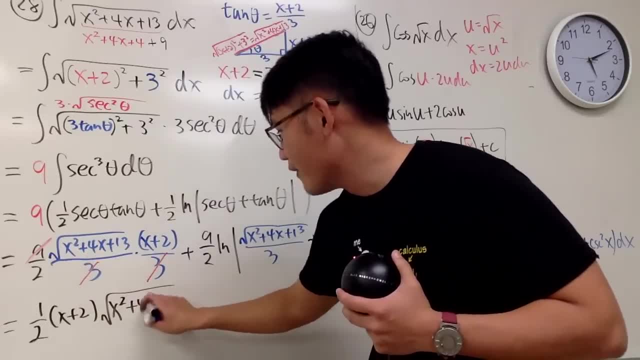 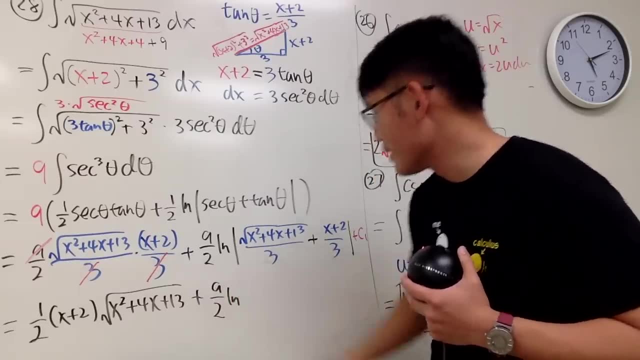 And then square root of x, squared plus 4x, plus 13.. And then plus. I will just write down 9 over 2 natural log And here is the deal. In fact, I did not need a absolute value. 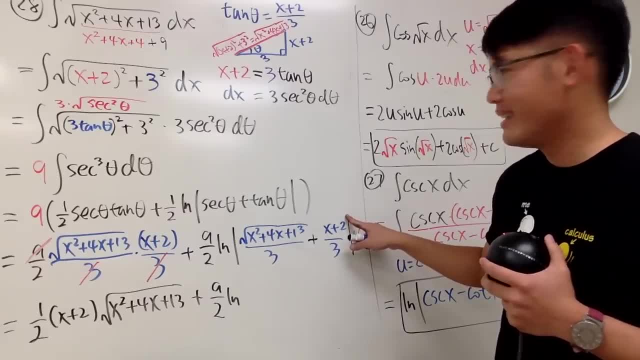 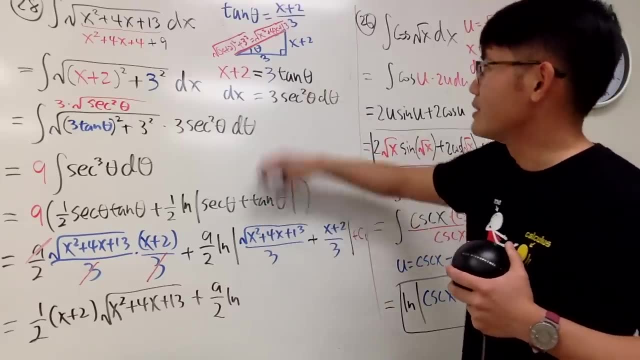 Absolute value. Why is that This? right here it's always bigger than x plus 2,. I believe Why. Because you have the hypotenuse It's longer than x plus 2 for sure, So I did not need the absolute value. 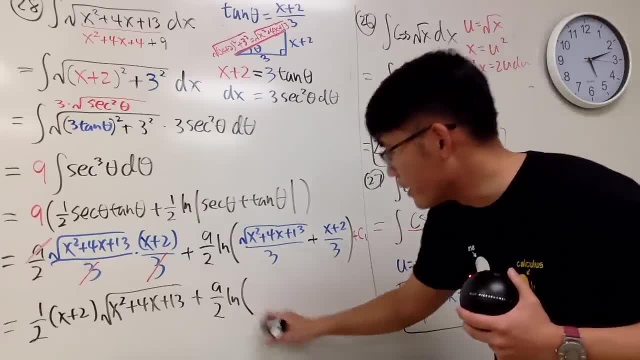 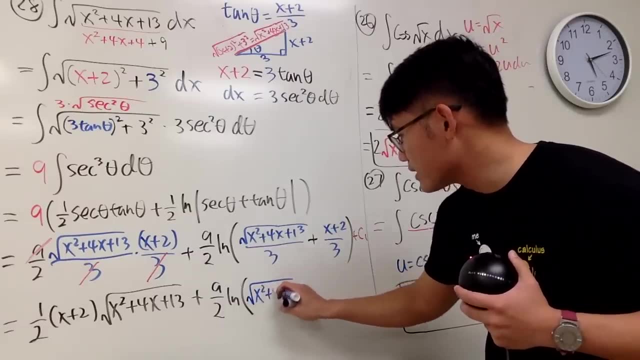 Right, You can put down parentheses. I will put down parentheses. I will just write on the top. I will put this down right here. So you will have the square root of x squared plus 4x, plus 13.. And then plus. 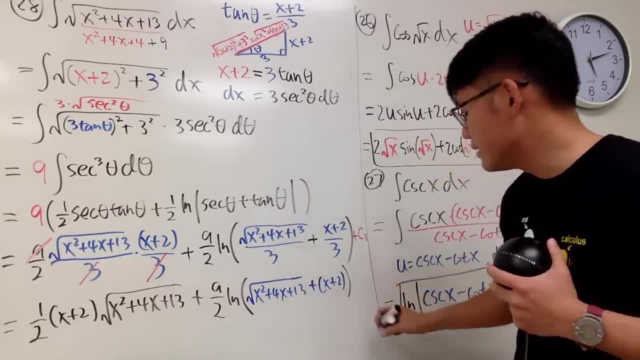 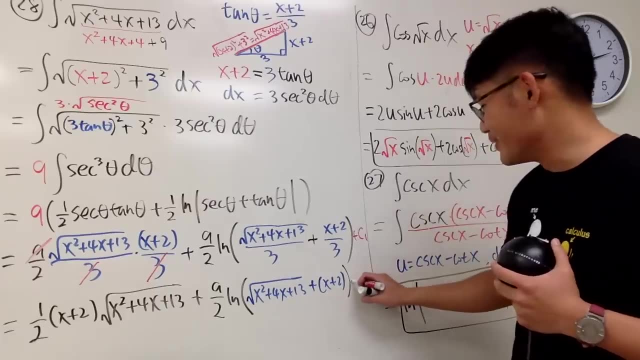 Parentheses. This is x plus 2,, if you like Parentheses, And then minus a constant And then plus c1.. I will just label that to be plus c2.. Okay, So this will be the clean answer. 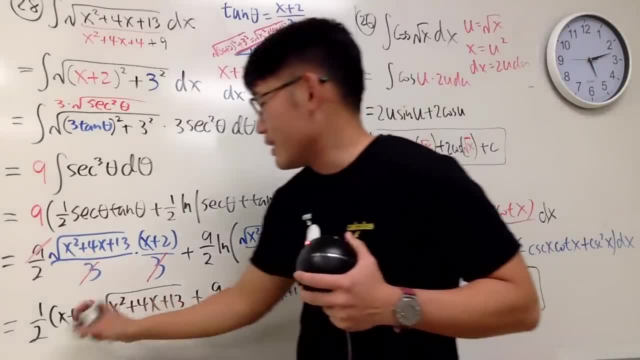 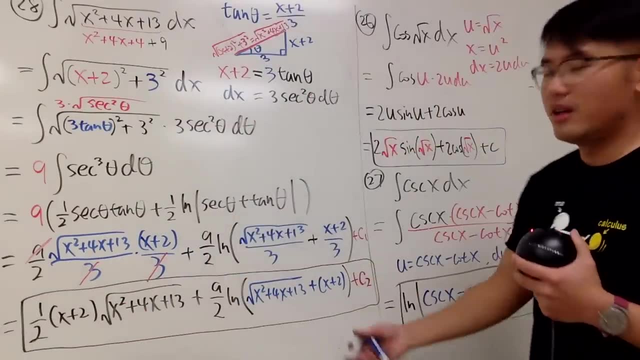 All right, But if you keep it as this, nobody is going to get mad at you. if you just write that down on the test, I think your professor, your teachers, will give you full credit as well. But I think this is good. 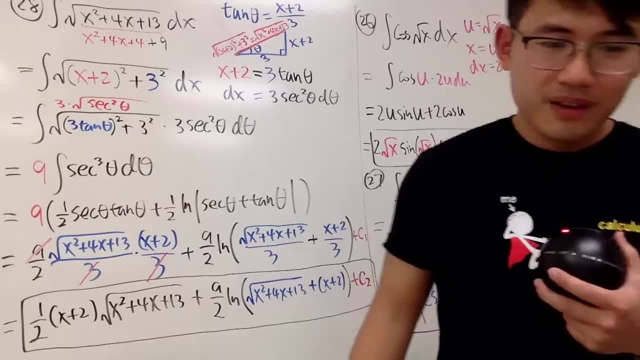 Okay, Oh, my god, One hour and 40.. No, I'm not going to look at time. Okay, Twenty-nine, Okay, Twenty-nine, twenty-nine. I don't know how many of you guys are still watching. If you're watching this, give me a time stamp right now. 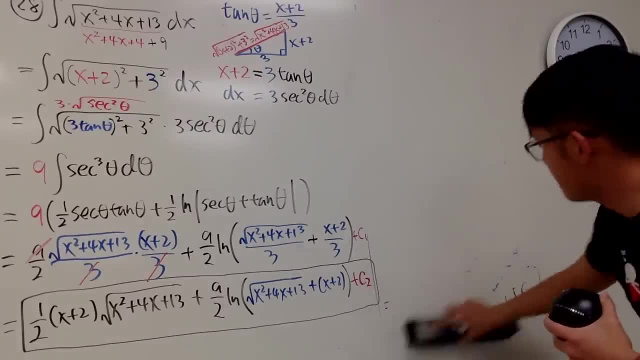 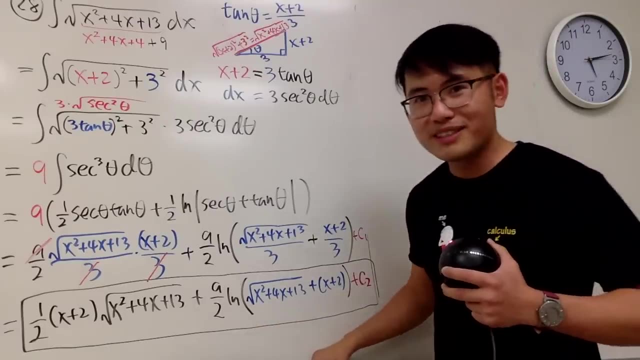 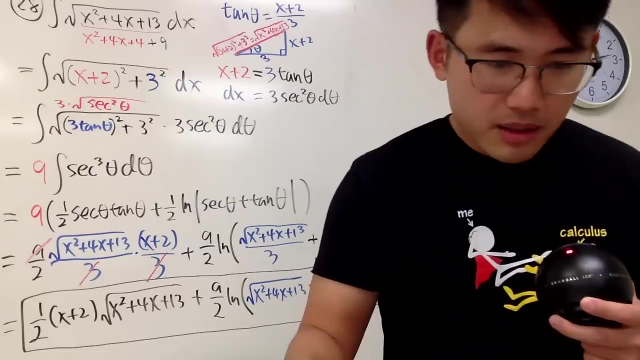 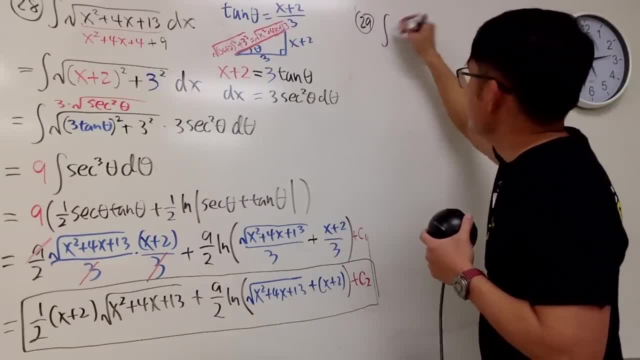 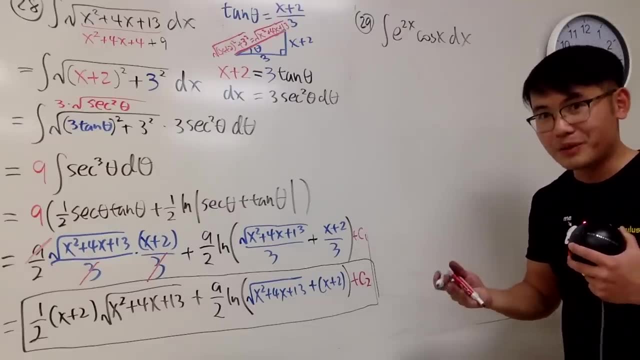 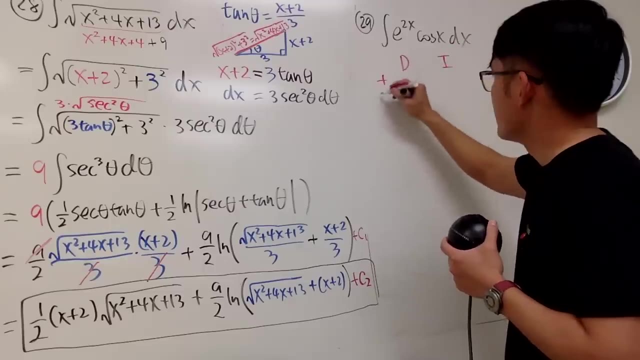 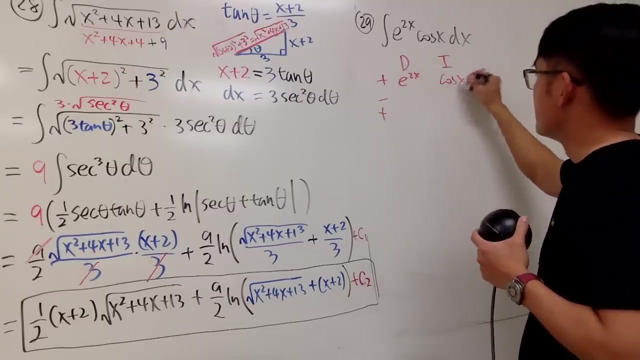 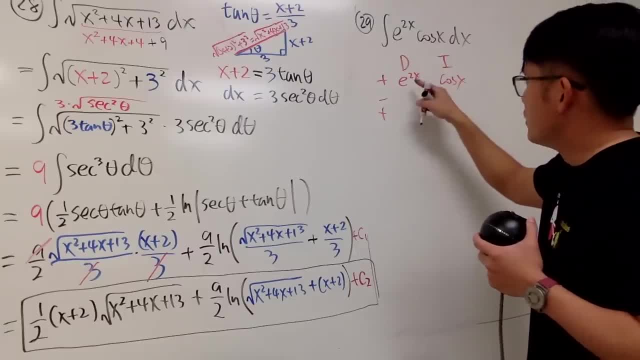 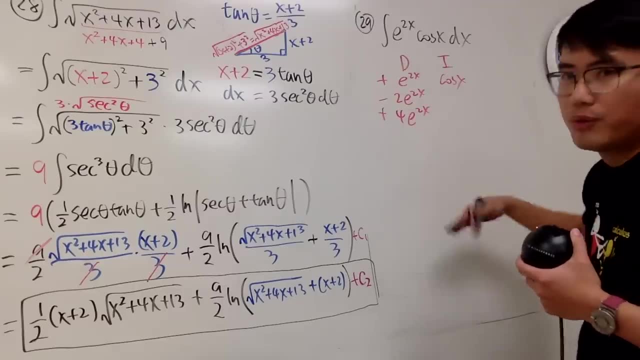 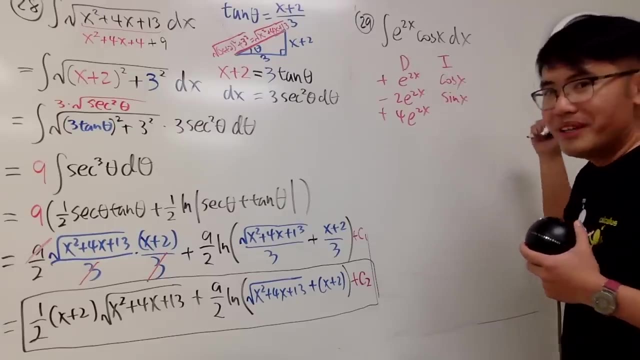 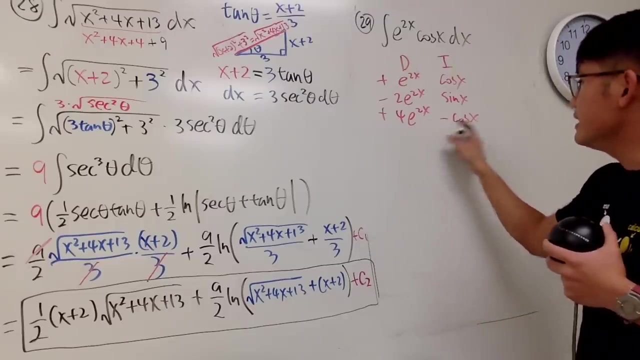 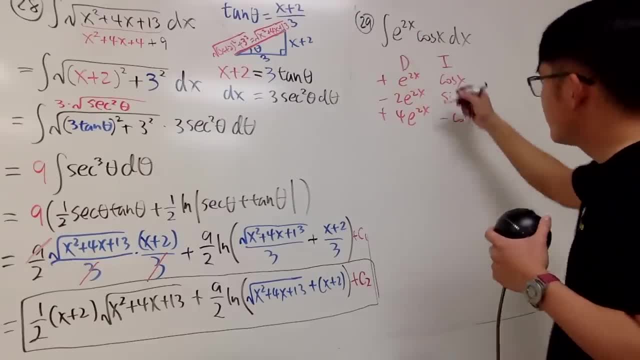 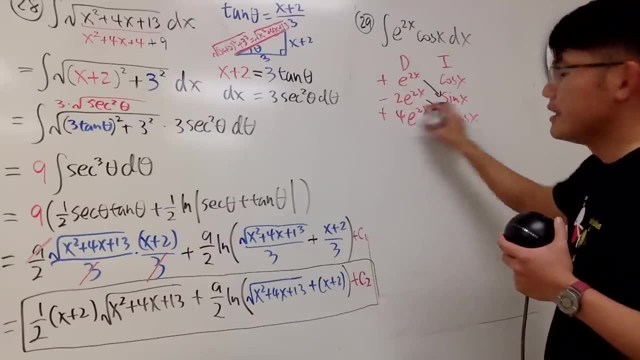 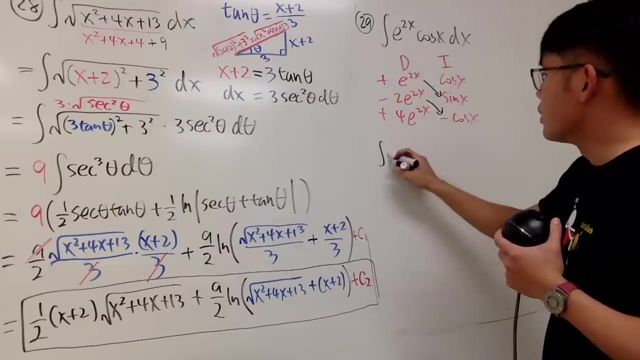 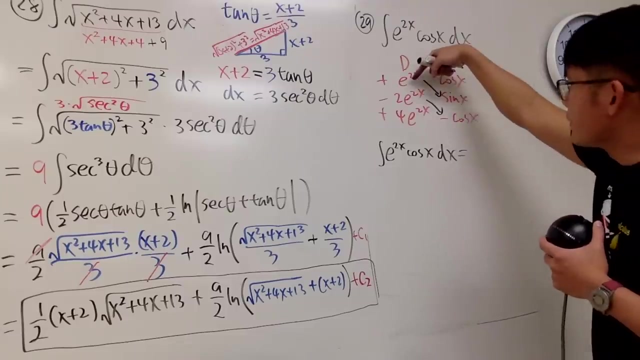 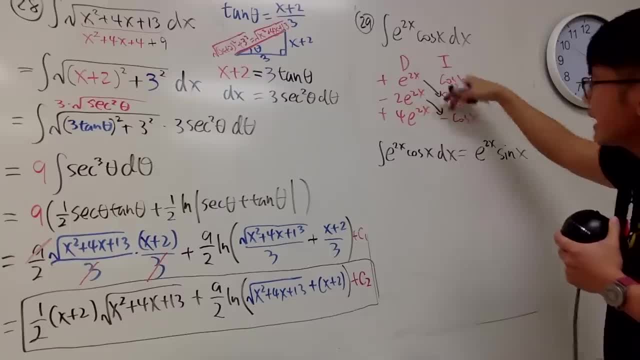 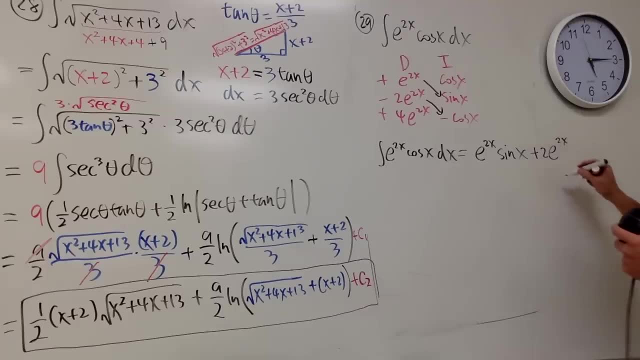 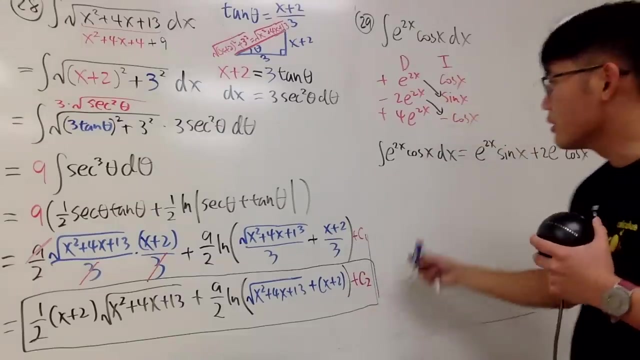 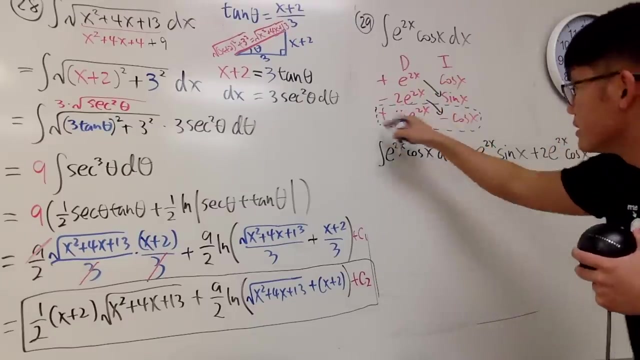 Easy, Easy, Easy, Easy, Easy, Easy. e to the 2x times cosine x. again, negative times, negative. Lastly, though, you are going to multiply this row, and this is still an integral, and don't forget, this is going to. 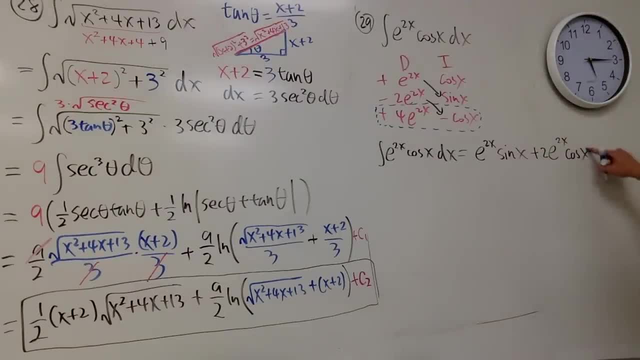 be a minus situation. you have minus and you can put a 4 in the front, and then you have the integral e to the 2x and you have the cosine x, dx, right? Well, it doesn't really matter because I will be adding this on both sides. so I will just say we add 4 integral. 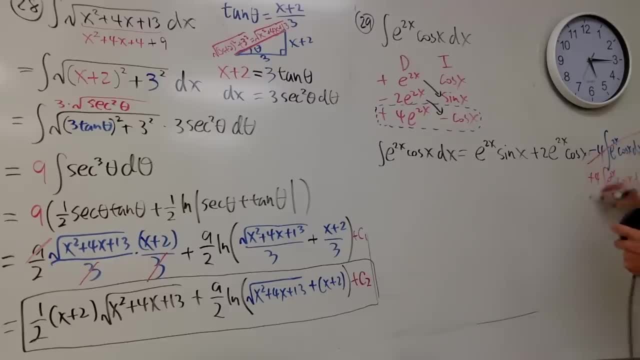 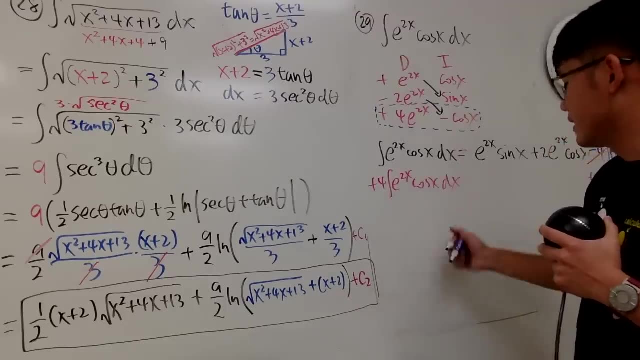 e to the 2x cosine x dx. so this and that will be cancelled. I will bring this right here. we add 4 integral e to the 2x cosine x dx. So let's do a few things in our head. 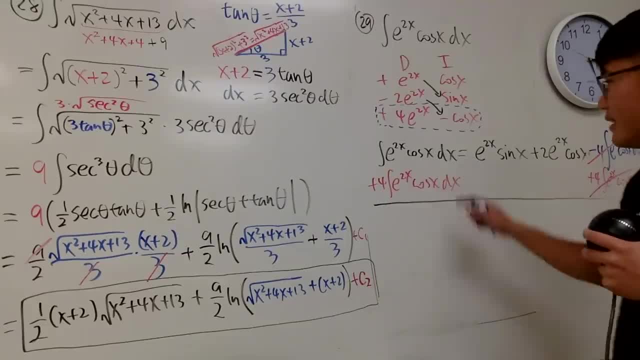 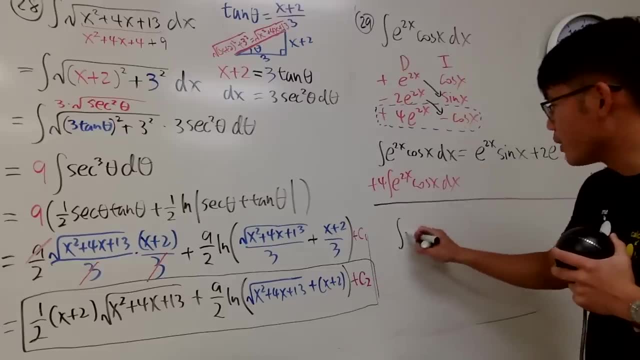 okay, That's gone. So 1 plus 4 is 5, I will divide everybody by 5, so when you end this up, you will end up with integral of e to the 2x cosine x, dx, and then give this a 1 over 5, so 1 over. 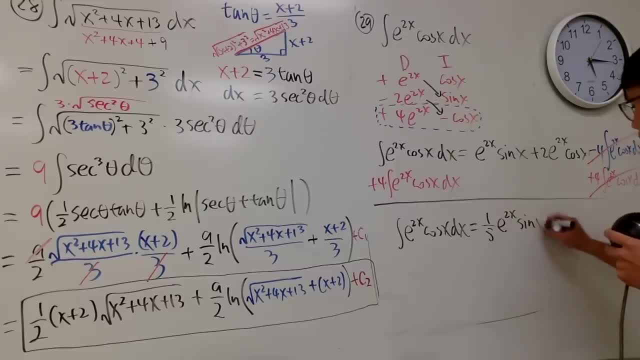 5, e to the 2x sine x and also multiply this guy by 1 over 5, which you will get plus 2 over 5, e to the 2x cosine x, and you are done. put a plus z alright. 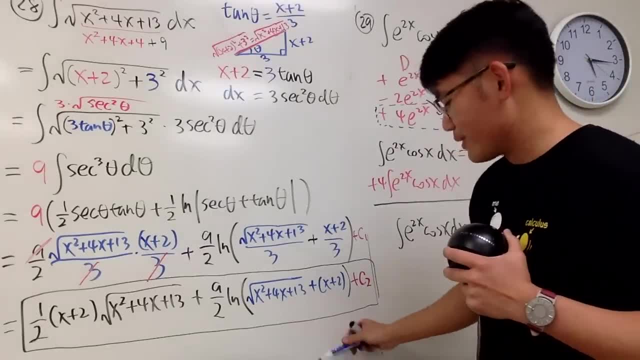 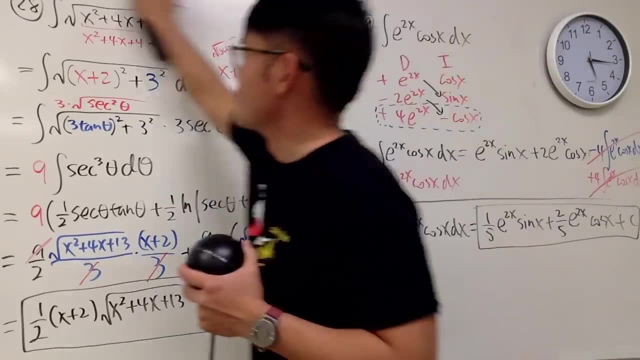 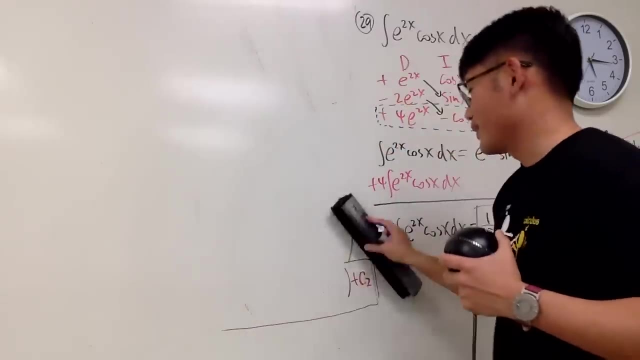 So that's it. Now continue to number 30, it's a definite integral, so hopefully it's good. if not, I don't know. I really don't know. Well, I don't know. let's see. if you wonder who came up with all these questions? yes, 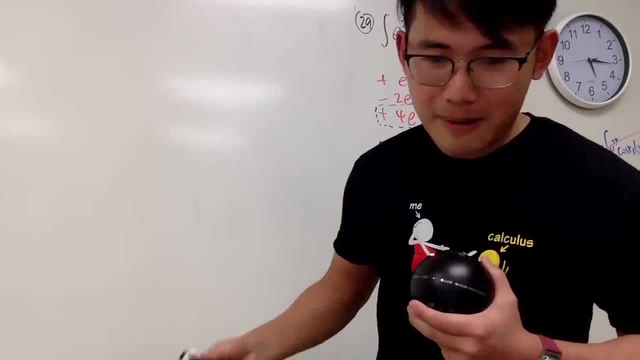 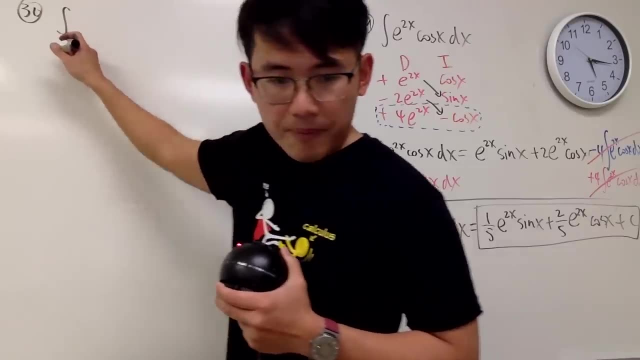 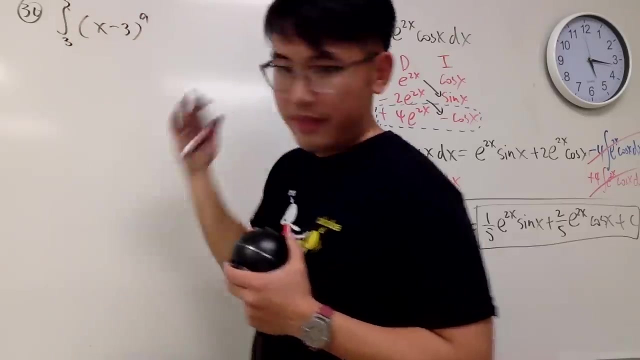 the person was me. Alright, number 30, let me put this down right here. number 30. Definite integral from 3 to 5, parentheses x minus 3, to the 9th power. it's nice as. 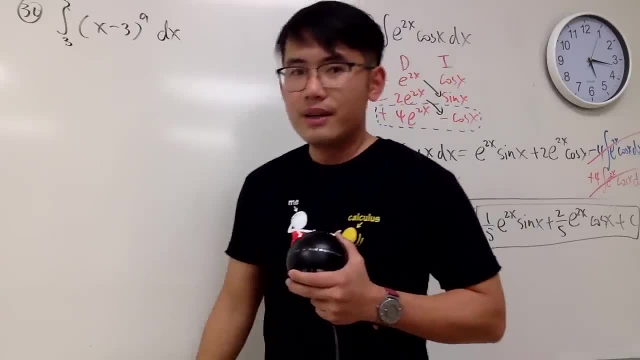 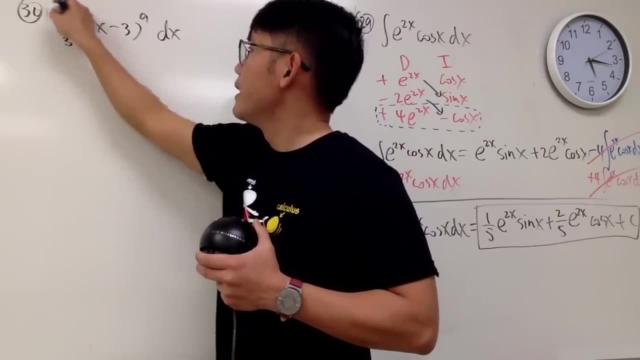 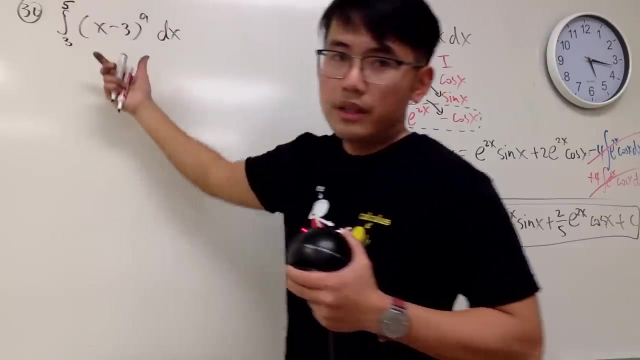 well, dx. Okay, here is a small thing I want to show you guys. Here is the power of the u-sub. okay, Because, because, because, because you just multiply this out and you have to expand that x plus 3 to the 9th power. 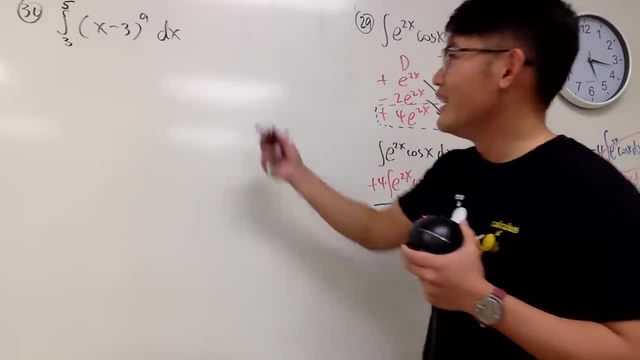 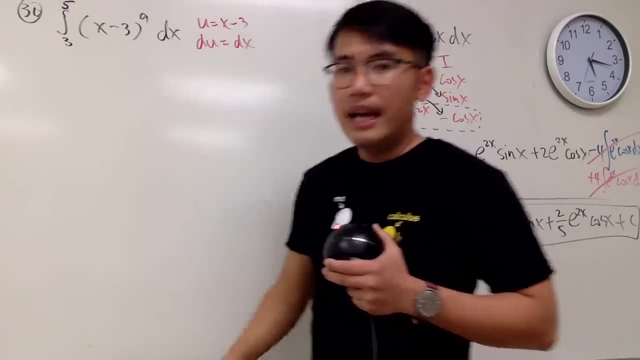 and then you can integrate that plug-in numbers up to u or you can just do u-sub When you let u equal to the inside. this is very nice. du is the same as dx And you can take this to the u-world and finish that. 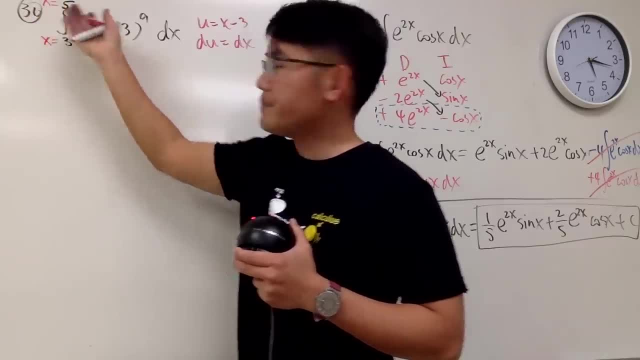 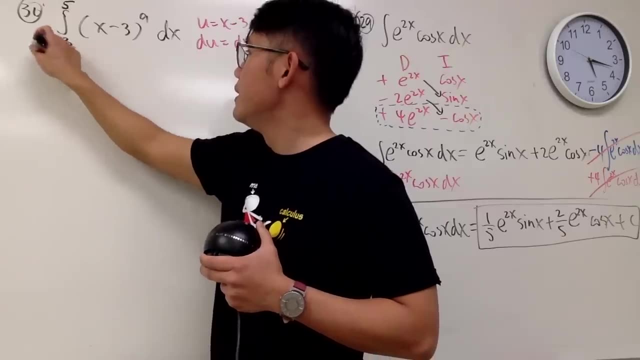 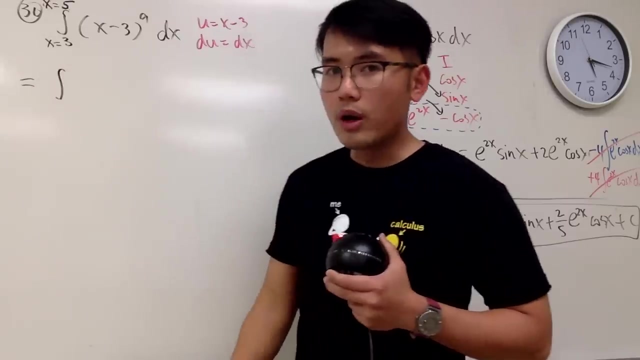 This right here. don't forget: x equals to 3, up to 5, right, These are the x values. These are the x values: x going from 3 up to 5.. Well, you are going to take this integral to the u-world. you put in 3 in here, u minus. 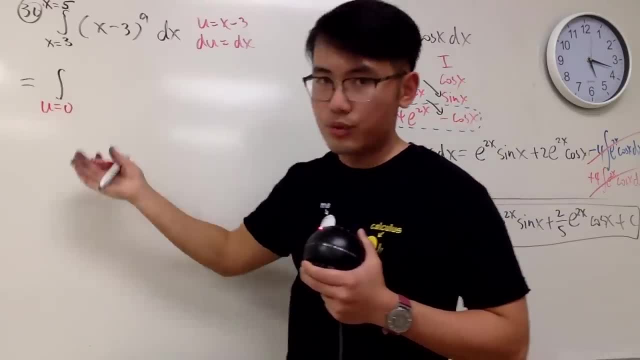 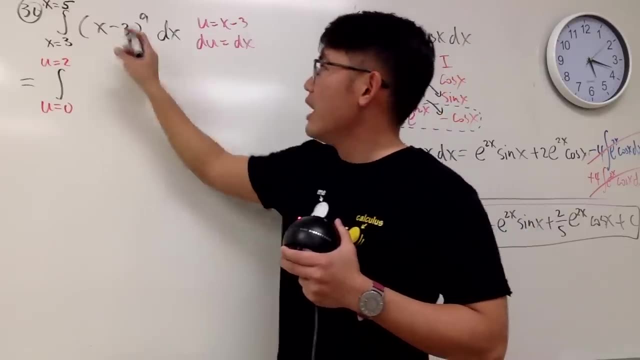 3 is 0, that means you have u begins at 0, and then you put 5 in here you get u will be finished at 2,. very nice. And then you just have u to the 9th power and then du is the same as dx, so you can. 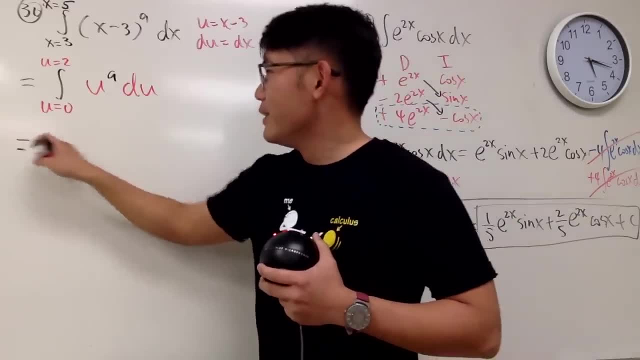 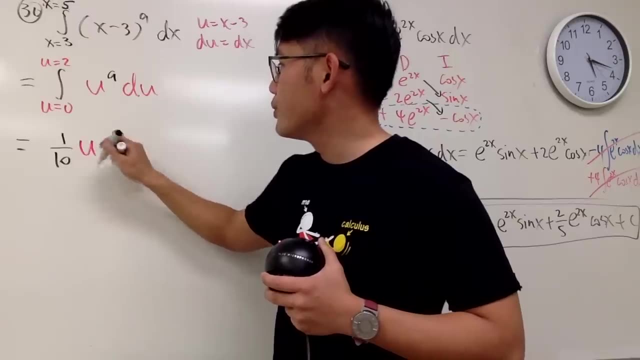 just du that And then integrate this guy Right. Finish everything in the u-world. Add 1 divided by the new power, which is 1 over 10, and then you have u to the 10th power and then you are going to be plug-in numbers right. 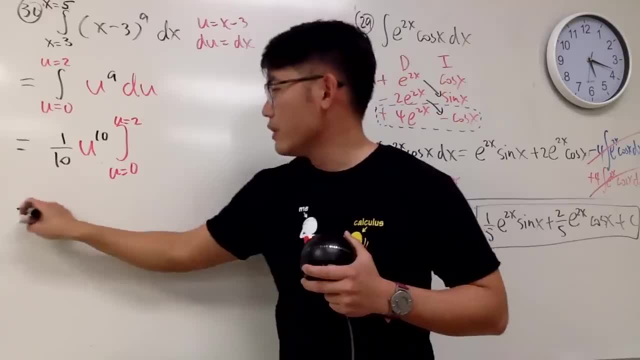 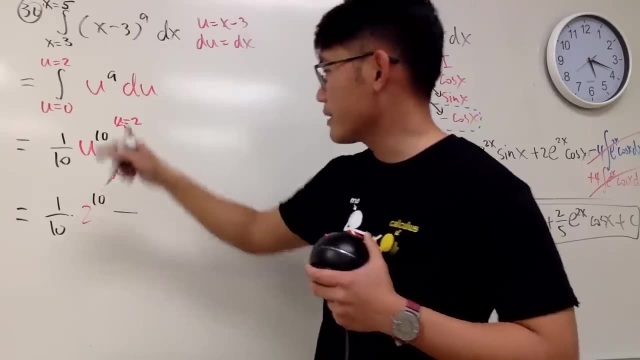 And again, these are the u numbers. So the first thing that you are going to do is plug-in 2, so you have 1 over 10 times 2 to the 10th power, minus plug-in 0, 1 over 10 times 0 to the 10th power. 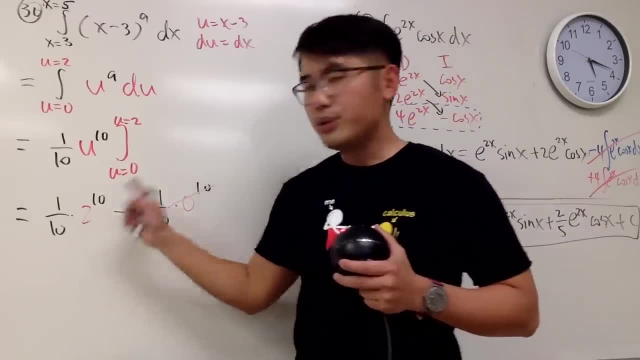 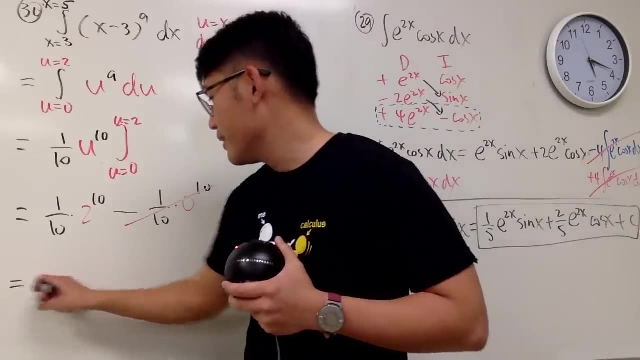 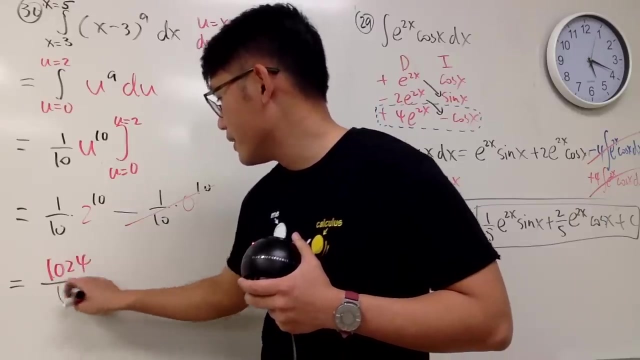 This right here is just 0,, so it doesn't matter. And 2 to the 10th power shall be a famous number, 1024,, especially if you study computer science right. So this right here is 1024 divided by 10.. 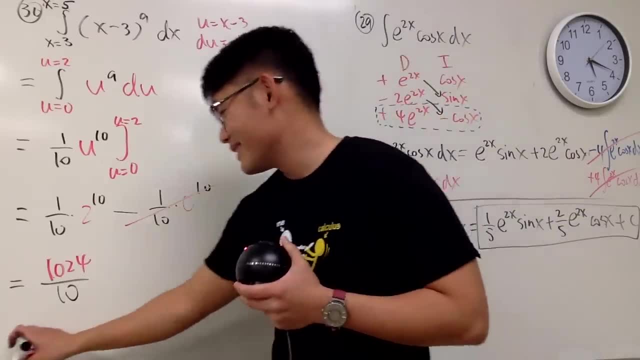 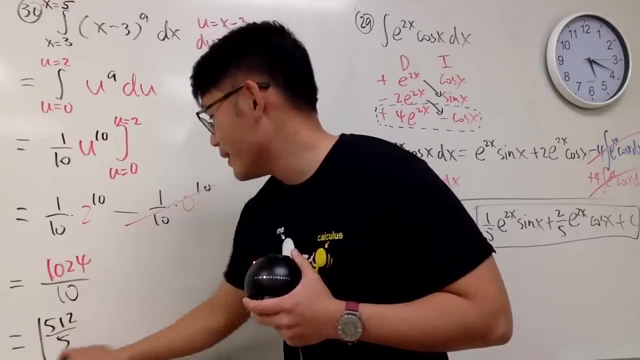 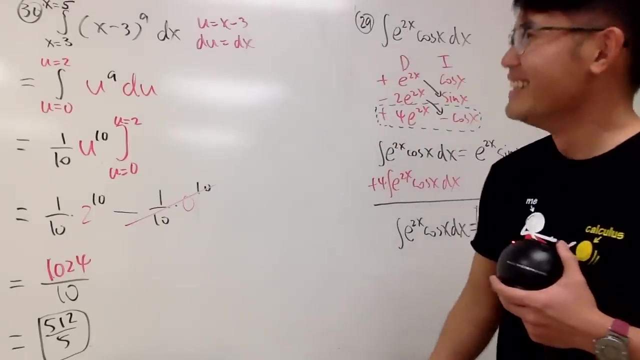 And now, of course, you know, take your pride, reduce the fraction, you know, 512 over 5.. And seriously, if you use decimal, sure, fine, whatever, 102.4, up to you, All right, number 34,, no number 31.. 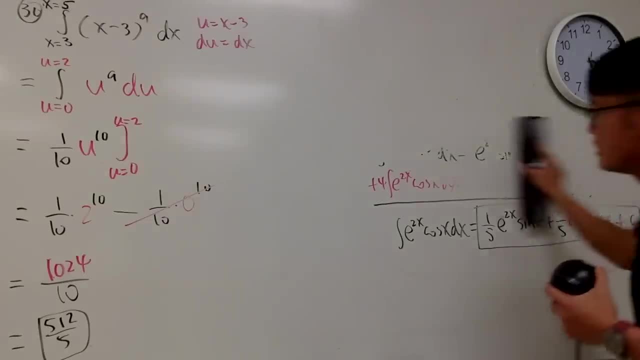 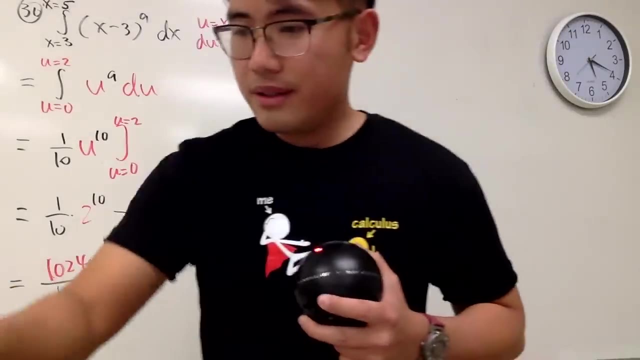 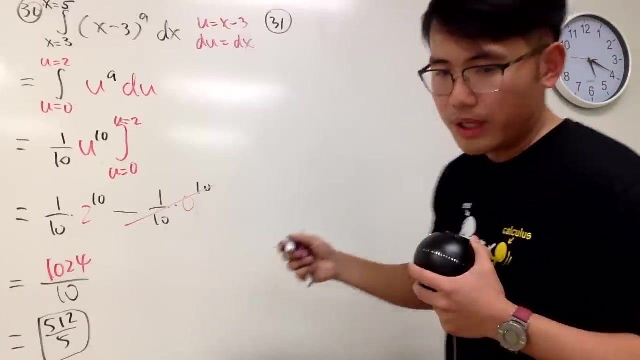 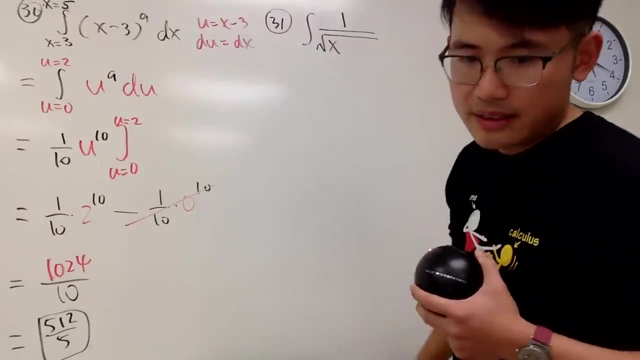 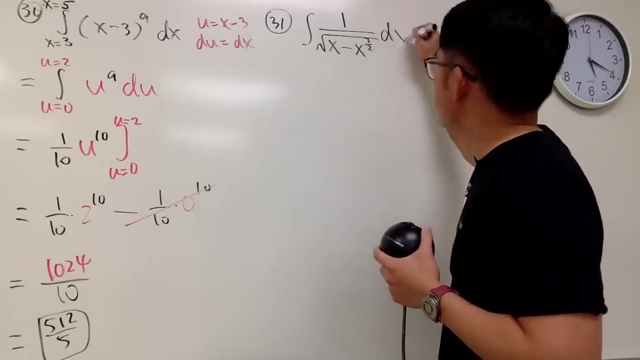 I'm going to erase this right here now. Number 31. Number 31, we have the integral of 1 over square root of x. Ooh, we have the x inside of the square root And then minus x to the 3 over 2 power. 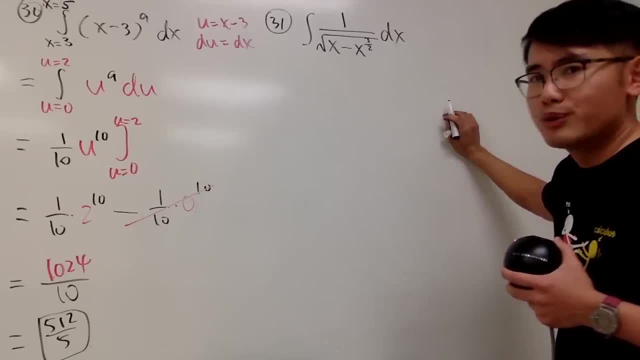 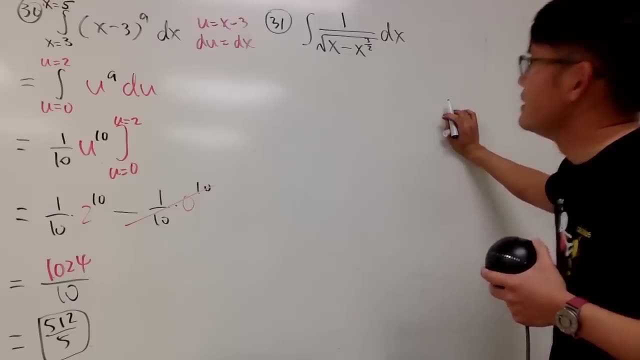 Huh, weird. I don't think I want to do use-up, You know what I mean. I don't think I want to do tricks-up. Let's see, This is, I say, what The first power, namely 2 over 2.. 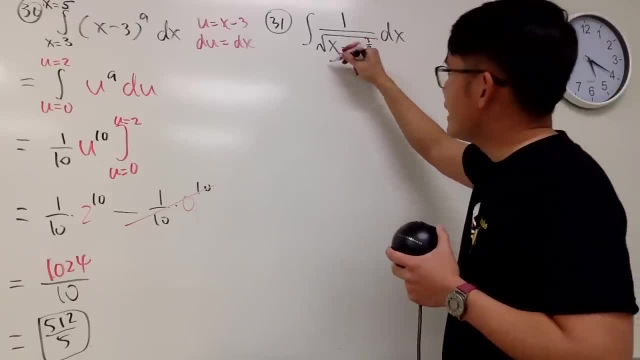 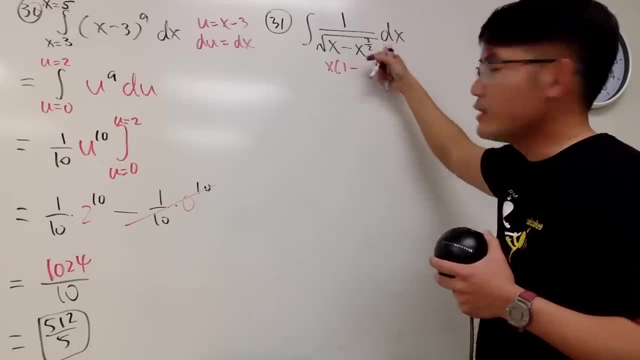 We can factor something else, right? So when you do that insidewise, you can see you can factor the x and you get 1 minus OK, you factor out 2 over 2, pretty much, so you get x to the 1 over 2, like that right. 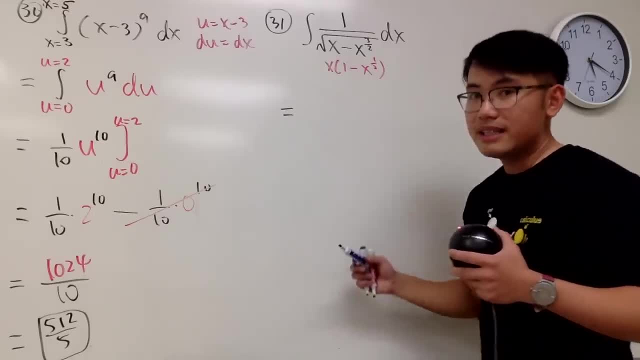 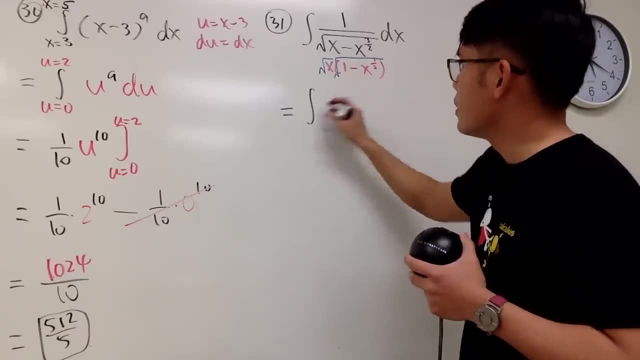 So in another word, you will see, don't forget, this is still inside of that square root. So you can square root of that, square root of that. So you get the integral of 1 over square root. This in the front. 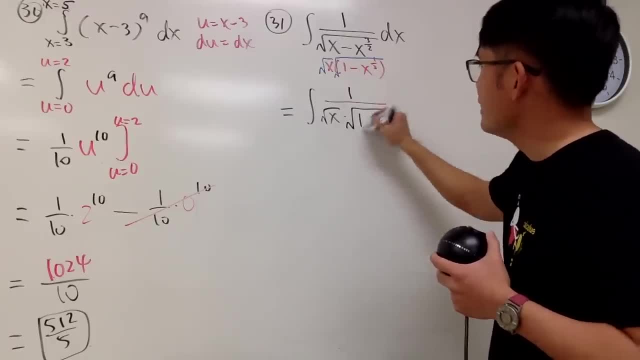 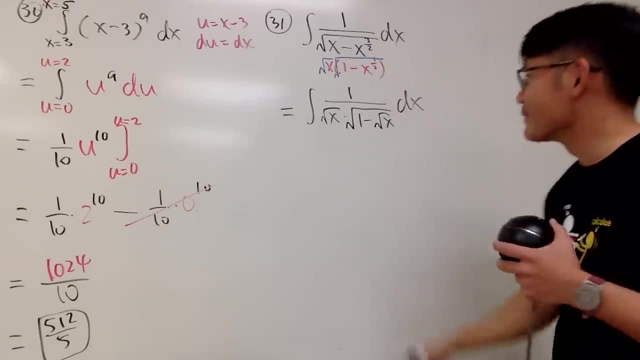 And then you have square root of 1.. And then x to the 1 over 2 power is another square root. Oh my god, this is way too fun, And you guys know. OK, now do a use-up. Let u equal to this right here. 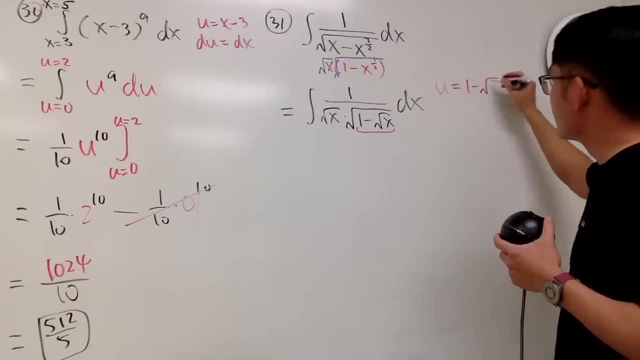 I think you will work out pretty nicely, so let's do it. Let u equal to 1 minus square root of x And let's go ahead and finish this. du will be. the derivative of this is negative 1 over 2 square root of x. 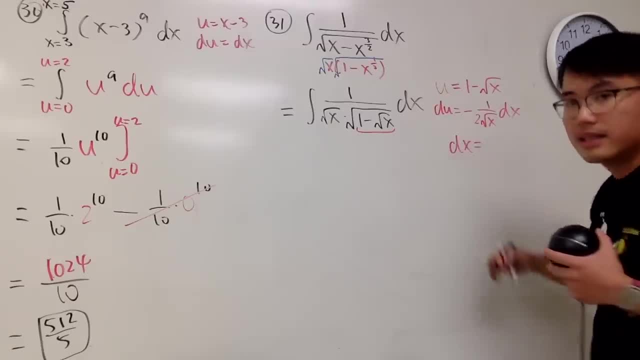 dx. and then, of course, dx is the same as. multiply this on both sides, you get negative 2 square root of x over 1 du And of course, take this integral to the u-world, you get the integral of 1 over. 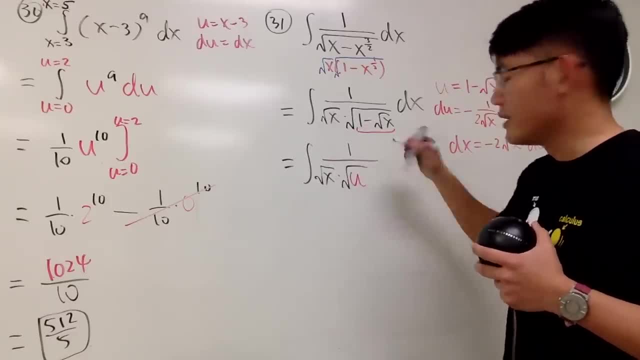 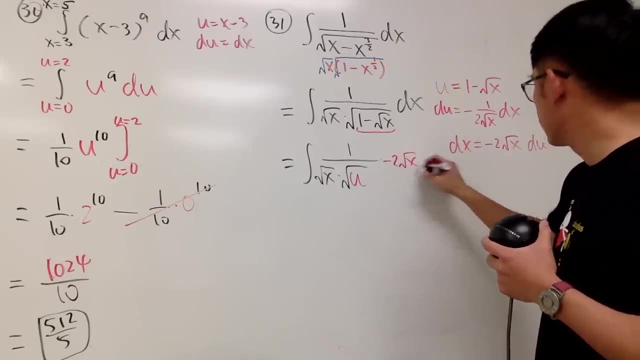 keep this for now. it's going to get killed pretty soon, though- and you get the square root of u, and then dx is this guy. so you multiply by negative 2. square root of x, du. Yeah, look at this. and that cancel very good. 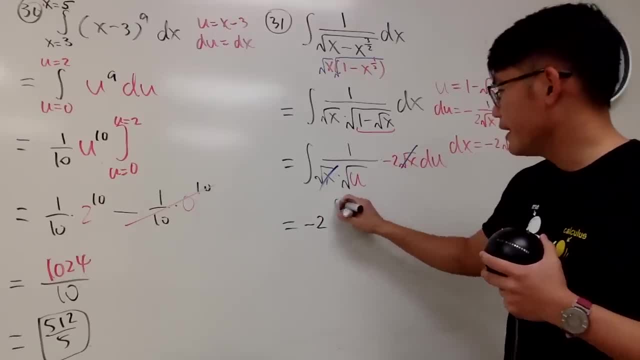 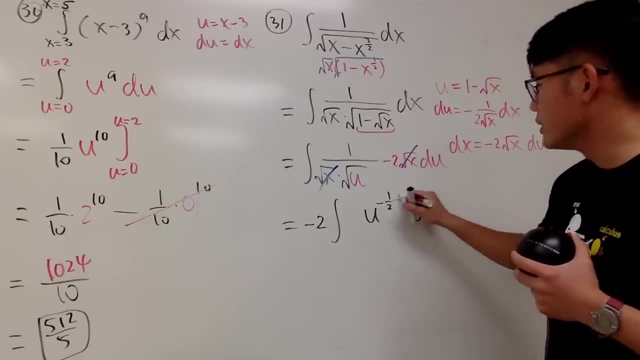 And now you're looking at this as negative 2 integral 1 over square root of u. it's the same as saying u to the negative 1 half power, the u-world. so add 1 to the power which is 2 over 1,. 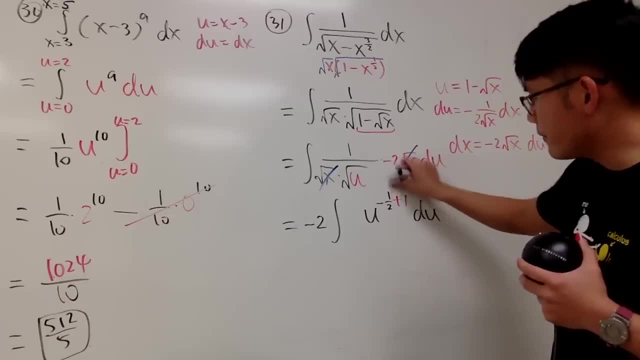 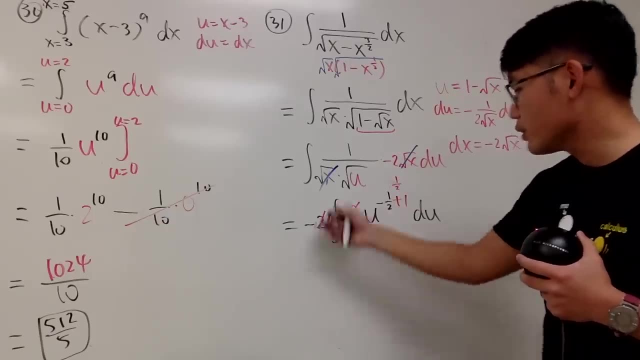 and well, that's. I'm one step ahead of myself. Negative: 1 half plus 1 is 1 over 2, divided by the new power, which is multiplied by 2 over 1, cancel, cancel. you still have the negative, though. 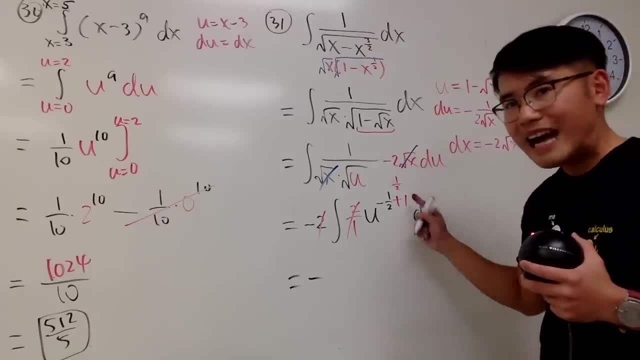 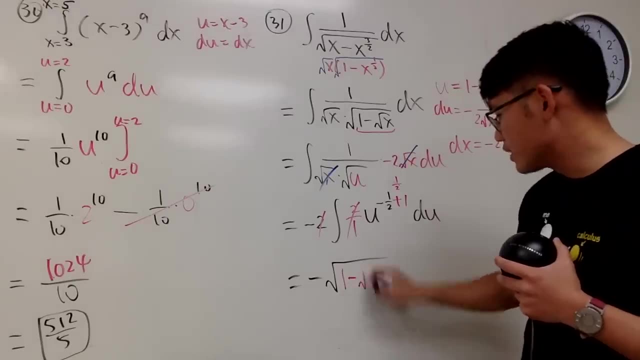 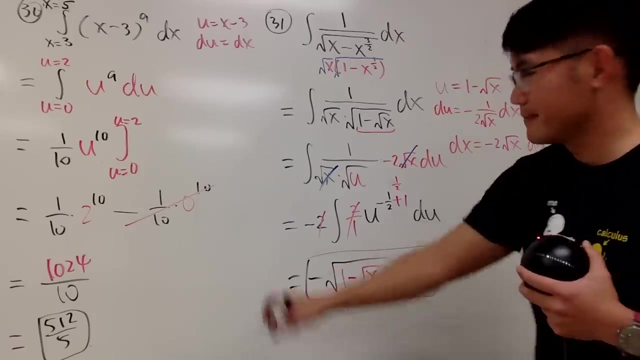 So negative u to the 1 half power which is the square root of u and u, is that? so I will just put that down right here: 1 minus square root of x and we are done for plus c. Very nice, very nice. 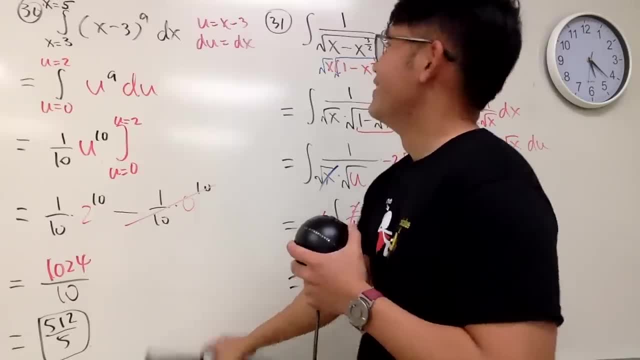 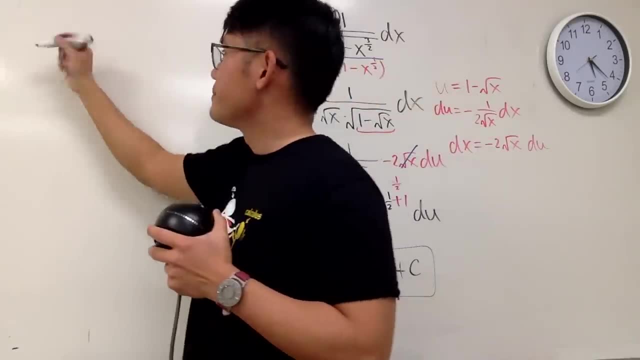 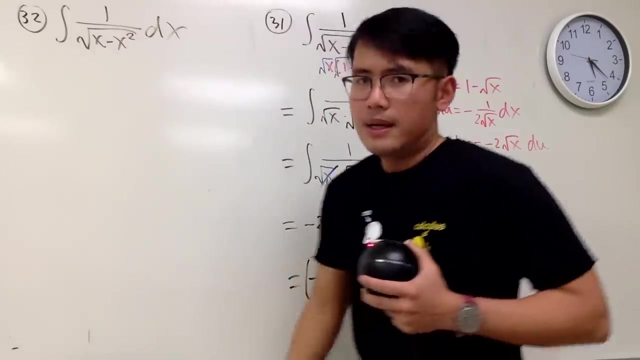 Okay, next one. oh man, very similar, very similar. We'll see if this is going to work or not, so don't be surprised, right? Number 32: here We have the integral of 1 over square root of x minus x squared dx. 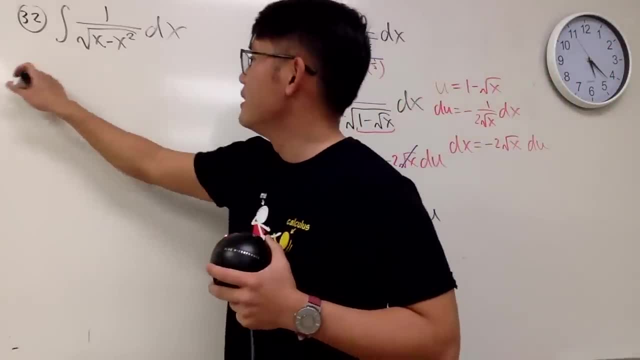 Let's factor it just like that This time. we'll do it in our head. This is the same as the integral of 1 over. factor out an x in the square root. in another word, you can take out the square root of x. 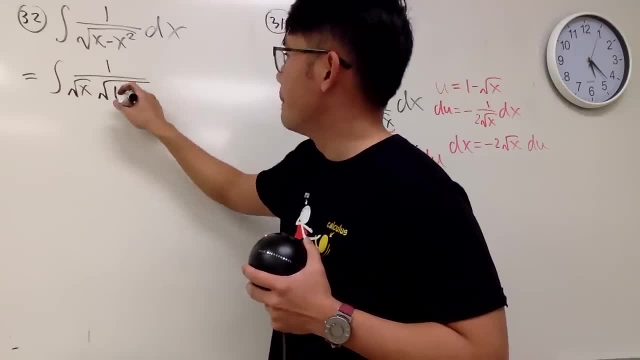 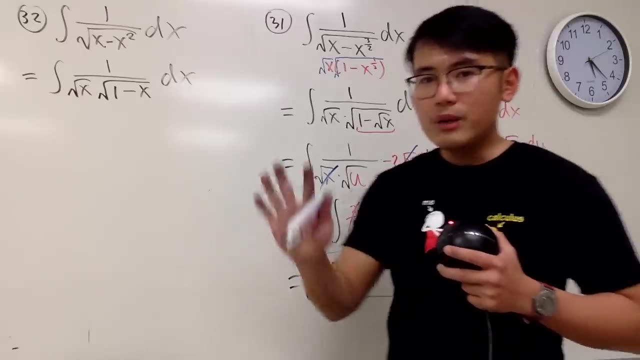 and then you have square root of 1 minus x, Like that, right? You can just look at x times this times that you get this. By the way, if you notice why my hands are getting dirtier and dirtier, 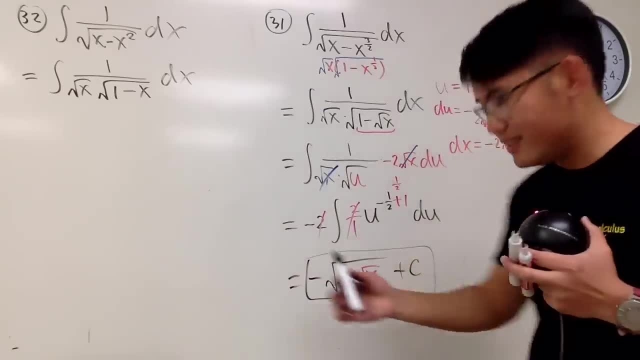 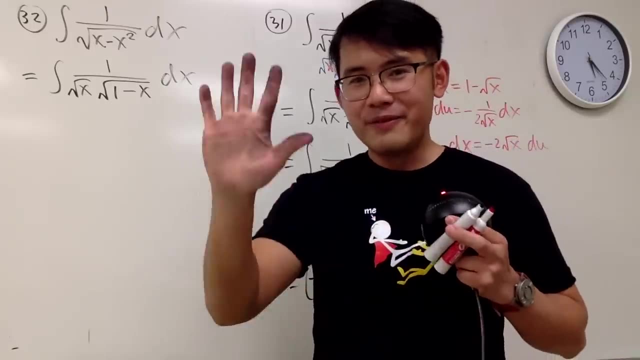 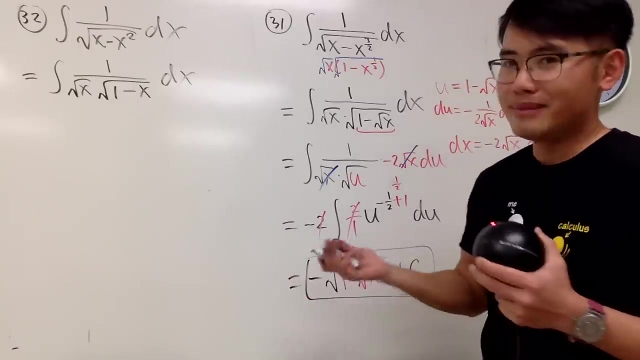 it's because of the marker. I have some new ones. This is how the new ones look like And the locals are going to be on my hand. Yeah, unfortunately. Yes, this marker sucks, But I love my markers, so I need them. I need them okay. 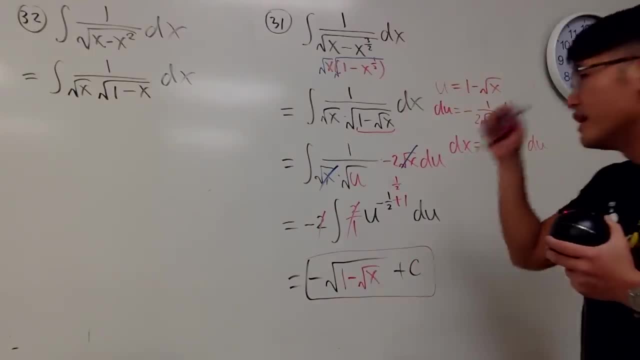 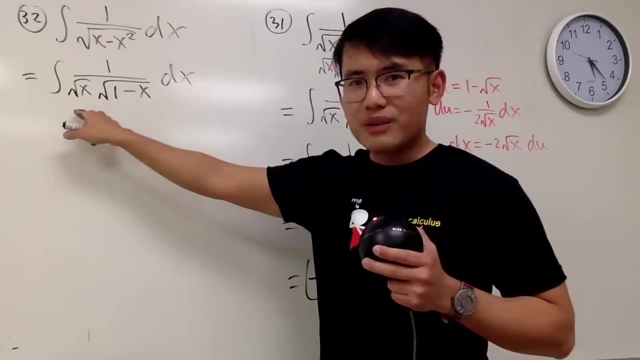 Oh, my god, let's see. Here is the deal, though Earlier, when I have the square root, I can somehow cancel the square root outside. I have this square root on the outside, I don't have the square root inside. so help me out. 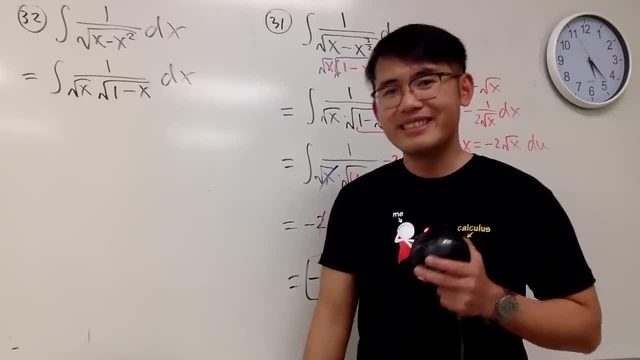 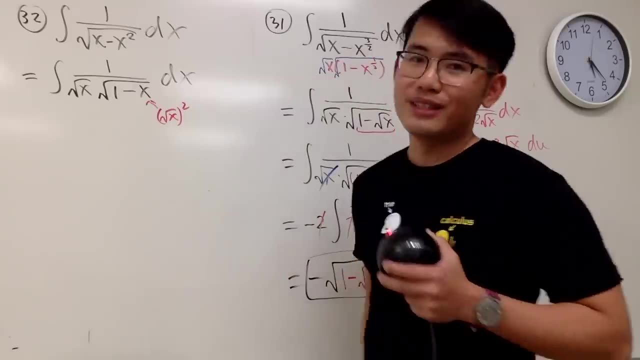 But can I somehow squeeze out the square root? Yes, we can, Because this x is the same as saying square root of x squared. How's that Sure? So we can look at this as the integral of 1 over square root of x. 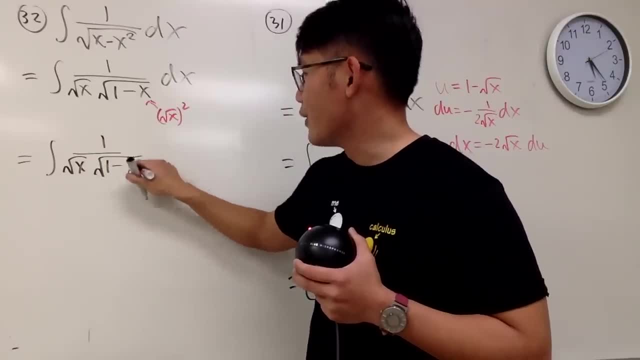 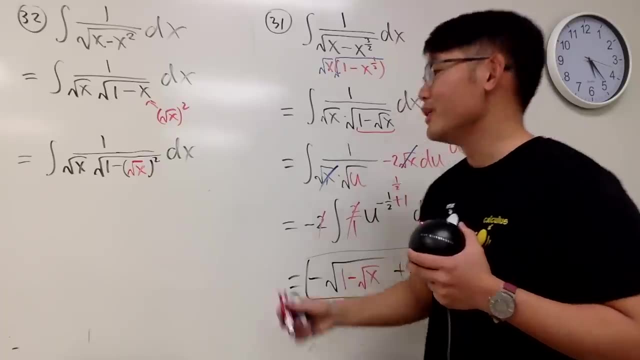 times the square root of 1 minus x, 1 minus square root of x. squared like that, Very nice. And then from here I will do a u-sub. I will let u equal just the square root of x though. 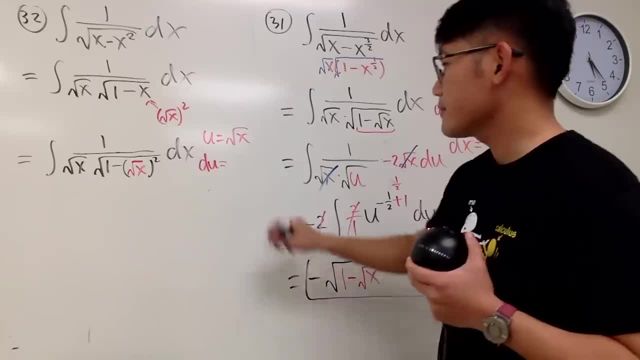 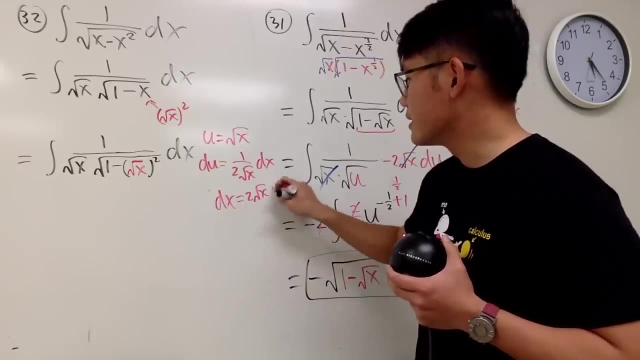 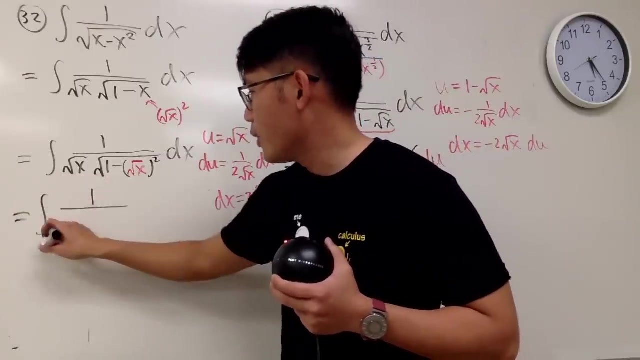 Just the square root of x du will be 1 over 2 square root of x dx And, of course, dx will be 2 square root of x du. Well, here is the deal. We have the integral of 1 over square root of x. 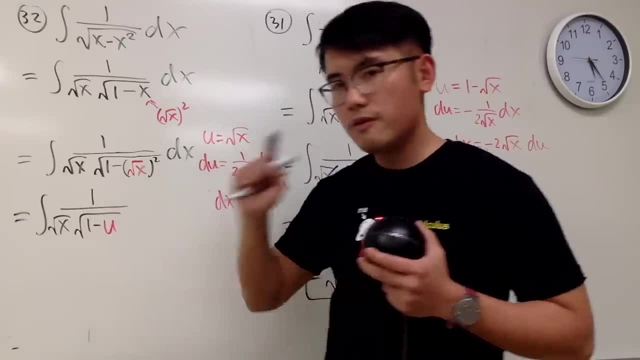 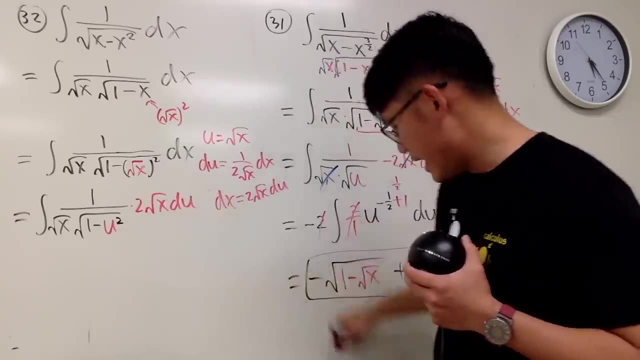 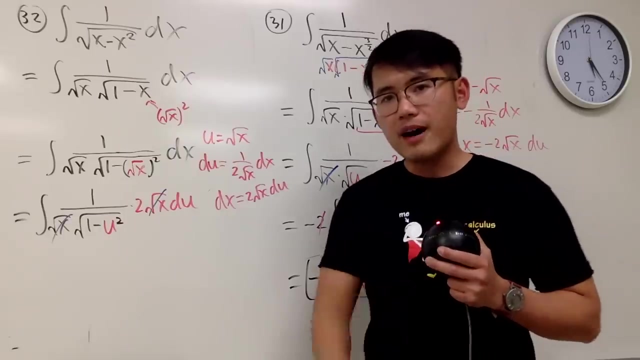 And then this is the square root of 1 minus u squared. And then dx is this guy. So you multiply by 2 square root of x, du, And you can cancel this out. Very nice, And now do we recognize how to integrate 1 over square root of 1 minus u squared. 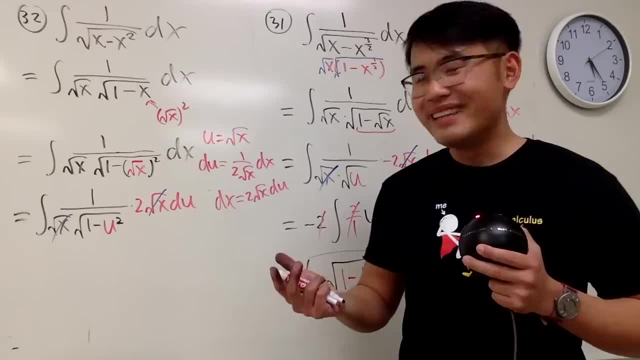 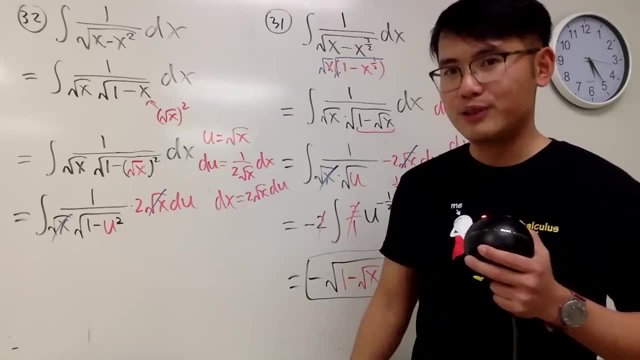 If you would like, you can do a trick-sub. You let u equal to sine theta And you do that, blah, blah, blah And you end up with inverse sine at the end, Right? So here's the deal Right here. I will just put down a 2 right here for you guys. 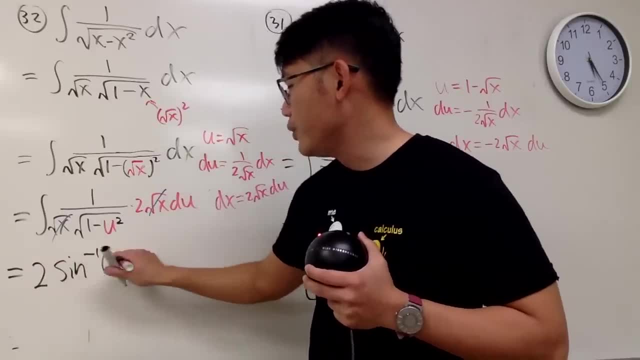 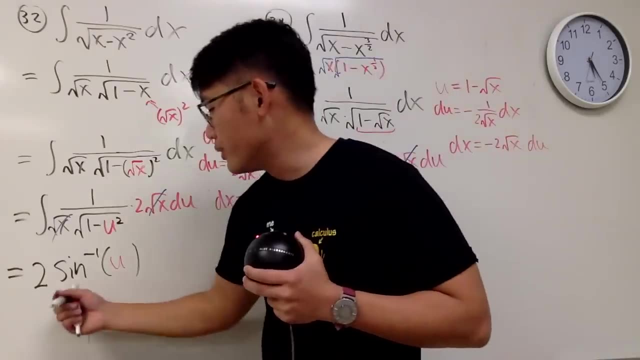 And then we will get an inverse sine of u. when you go from here to here, u is square root of x. Of course, finally, we'll put it back And we get 2 times sine Inverse with the inverse sine of the u. 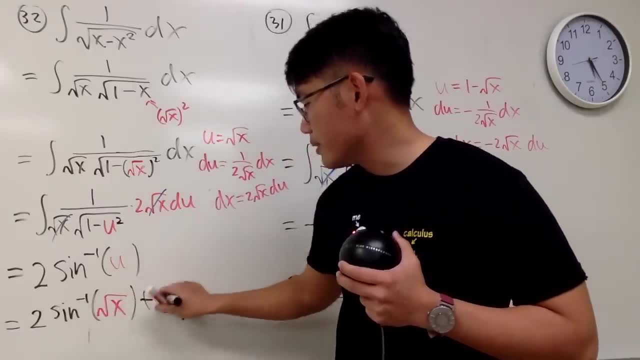 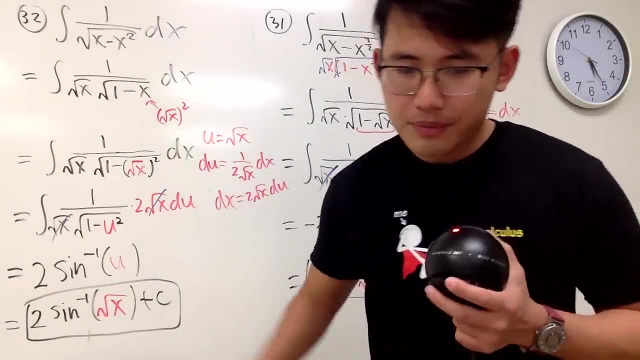 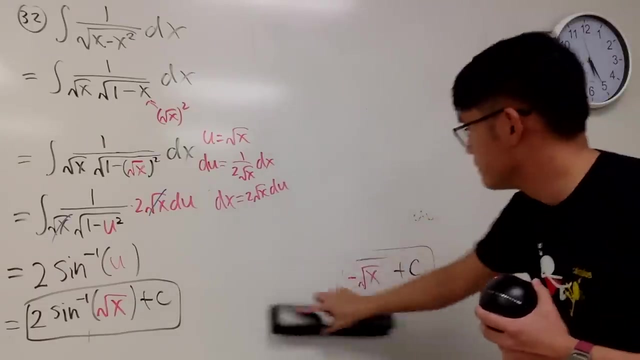 which is the square root of x. Like that Plus z, We are done. Okay, Now moving on to: Oh my god, Finally something easier. The next one, All right, Next one, next one, next one. 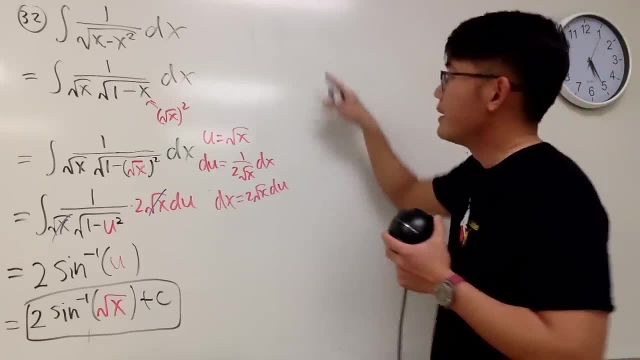 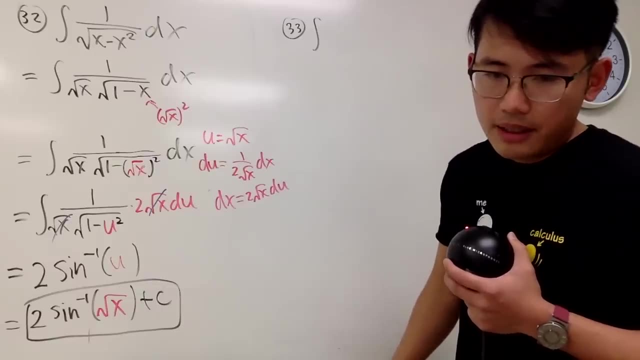 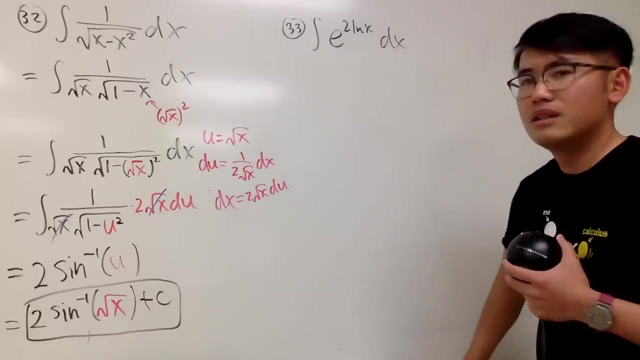 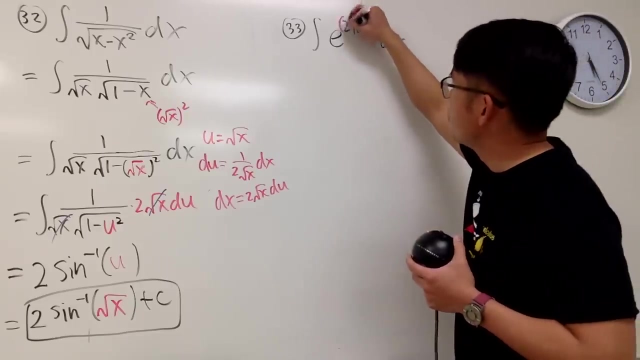 Which is 33.. Question number 33.. Integral of e to the 2 times ln x. Huh, Weird. Can I cancel them out? Not now. First you have to put the 2 to the power And you get this as the integral of e to the ln. 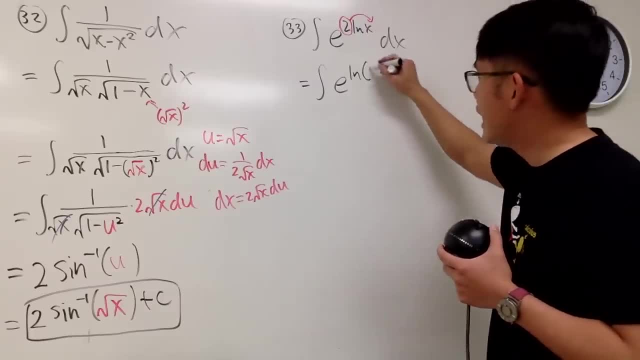 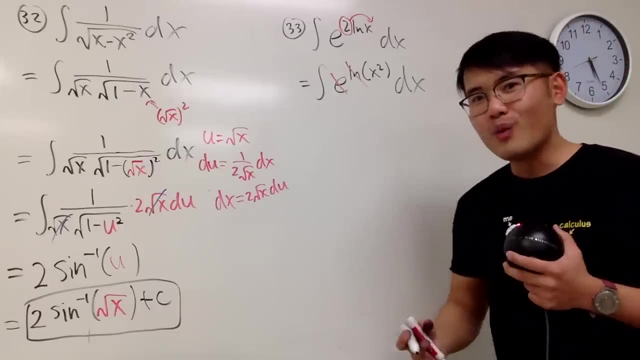 This right here has to be clean, And then you have x squared, like this dx, And then you can cancel them out. That's fine. All in all, we are just integrating x squared, So we have this being 1 third x cubed. 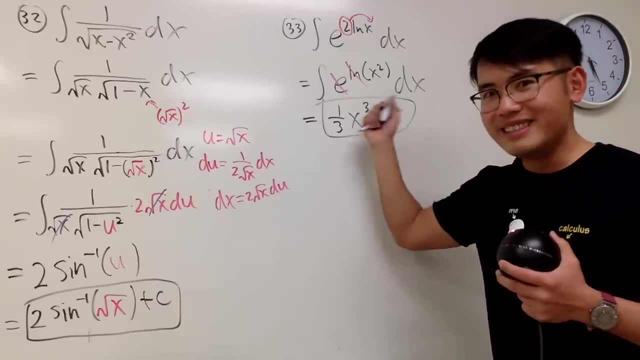 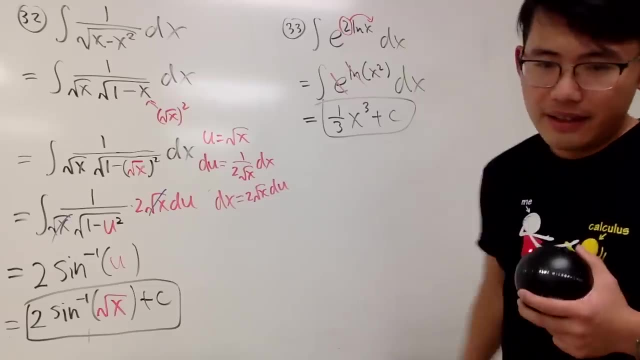 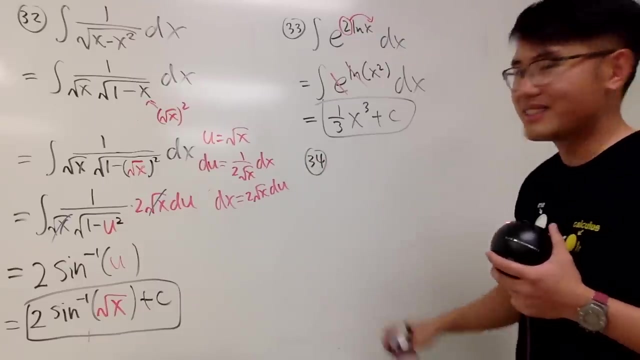 And we are done, And I think this is pretty much everybody's first integration, isn't it Like integral of x, squared And you get this All right. Next one, Number 34.. I actually put this one on my test. 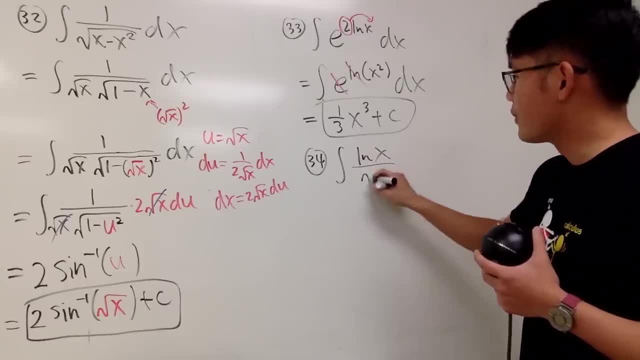 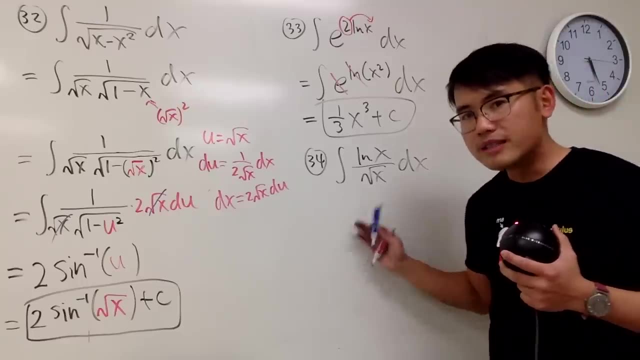 for my Cal 2 student recently: ln x over square root of x dx. Here's the deal: Whenever you have the integral of x to some power times, ln x, you can do this by integration by parts. So we will again do it by integration by parts. 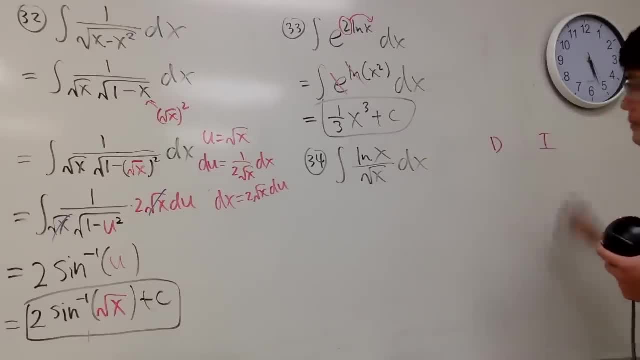 Of course we'll do this by the di setup First, the. I will choose ln x to be differential, Because if you want to integrate ln, you have to use integration by parts. again, right, I will be integrating 1 over square root of x. 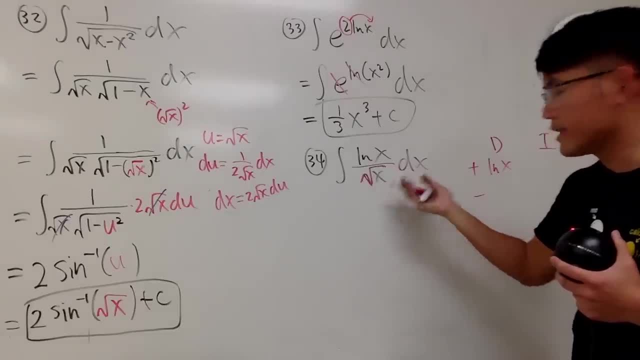 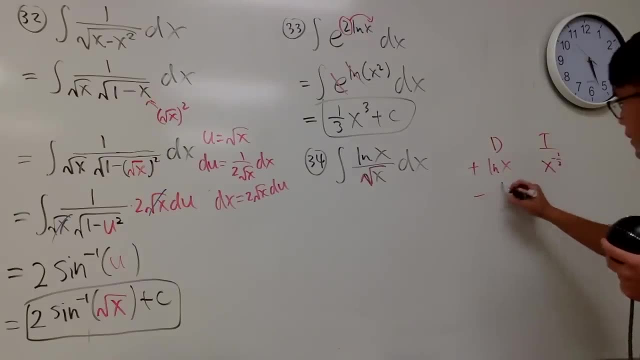 So you see, we have the square root of x in the denominator, In other words, x to the negative, 1 half power. All right, Enough talking This right. here is 1 over x. Integrating this guy, I will add 1,. 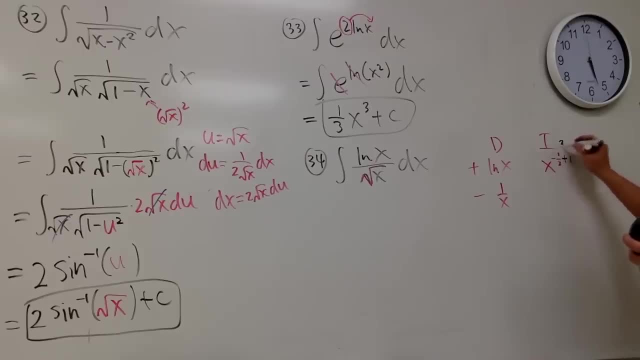 which is going to be 2.. Let me 1 over 2. And then divide it by that which is multiplied by 2 over 1.. So I get 2 x to the 1 over 2 power. 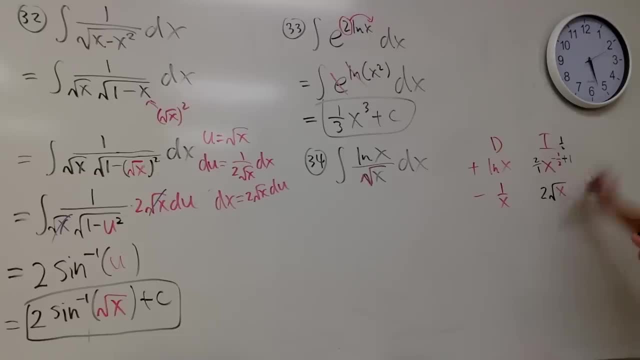 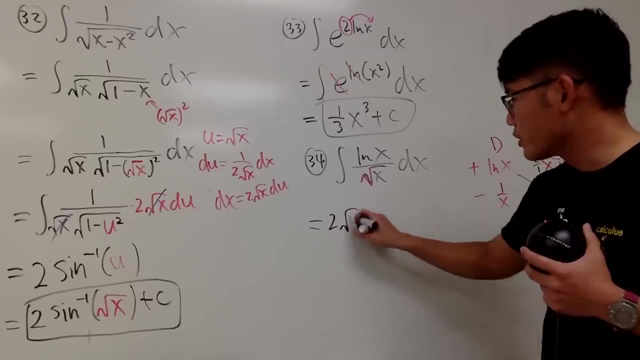 which is square root of x, Like this. So the first part of the answer is this: times that. So I put this: times that, which is 2 square root of x, times ln, x, And right here do not put down absolute value around the. 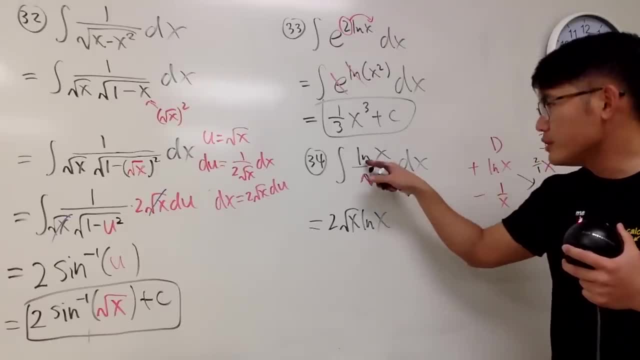 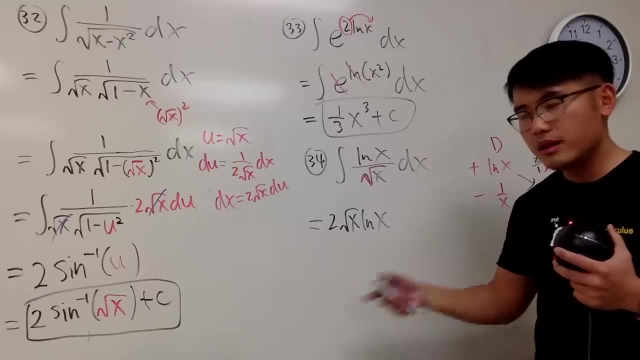 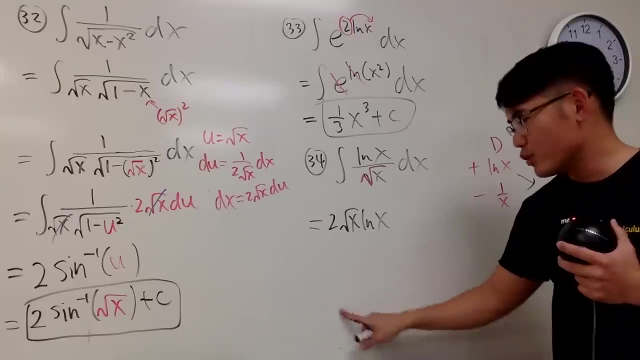 ln. Why? Because originally you have ln x right here. You only put down, You only put down absolute value of x around the. You only put down absolute value around the natural inside of the natural log when you do the integral 1 over x. 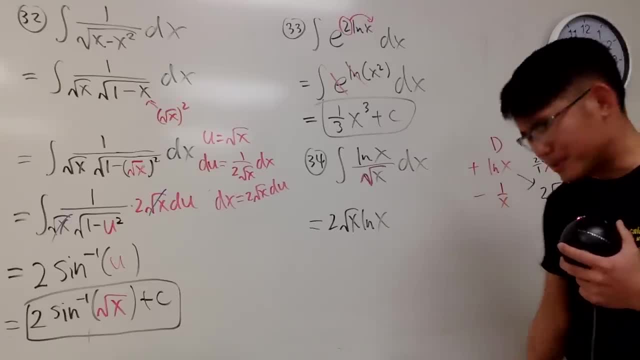 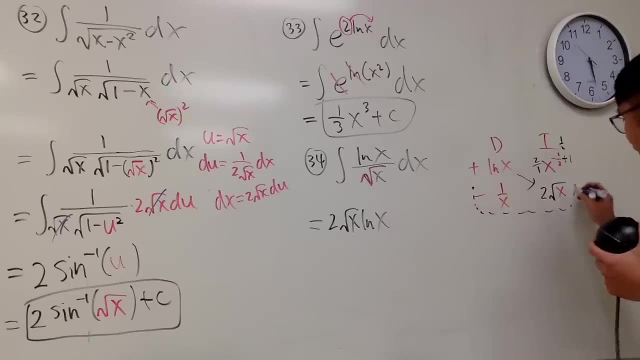 And you get natural log absolute value of absolute value of x. You know what I'm talking about. Anyway, here's the deal. Multiply this right here, and you still have to write that as the integral, So you have the 2,. 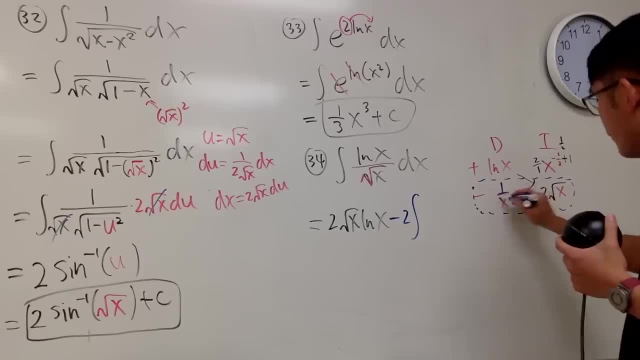 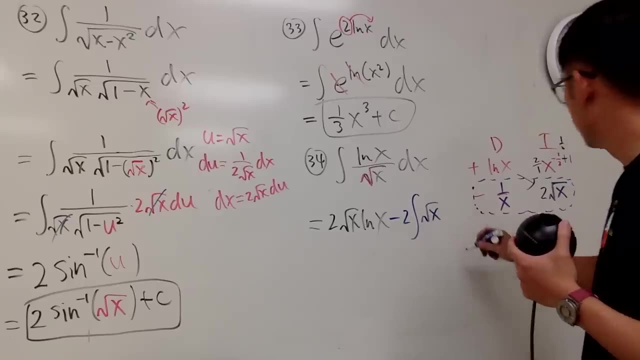 and that's a minus integral. Okay, 1 over x times square root of x, In other words, square root of x over x. you still end up with square root of x. All right, Square root of x, right here. 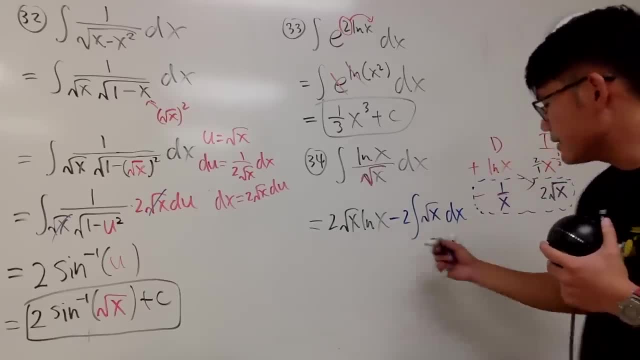 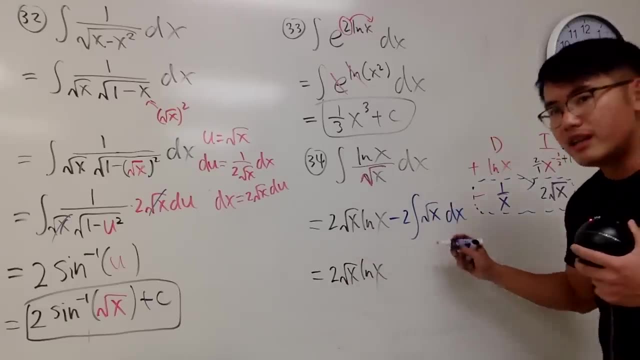 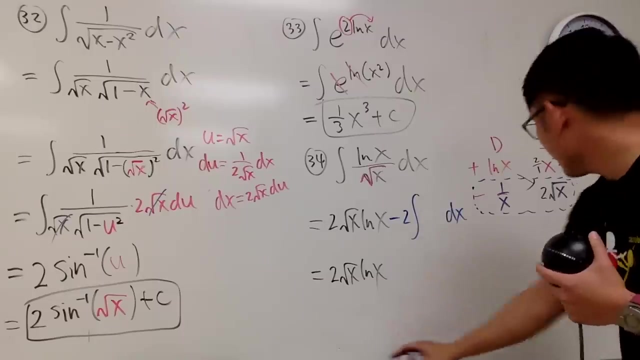 dx. So here is the final answer. I'll just write this down right here for you guys. Answer is 2 square root of x times ln x. This right here. we did it earlier when we went from, Sorry, All right. 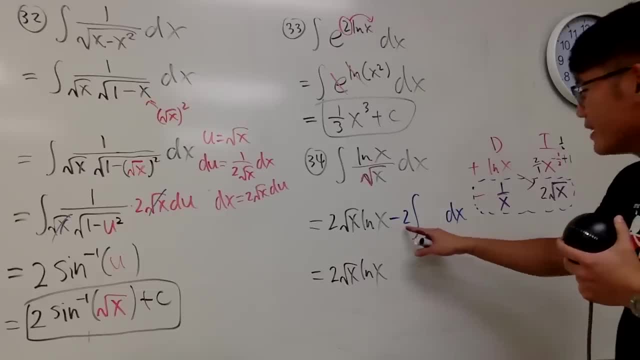 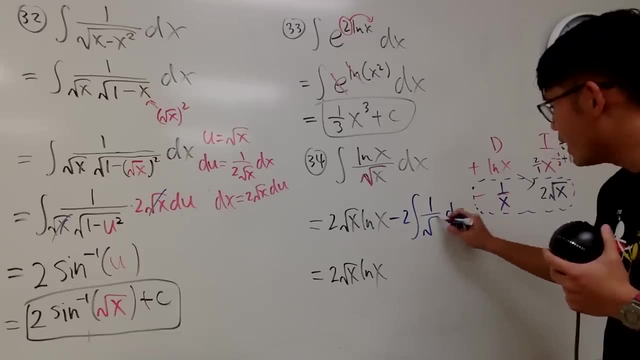 Here is, Let me do it again. I have negative 2 integral, this times that Square root of x over x. we have 1 over square root of x. Okay, We have 1 over square root of x, And here's the deal. 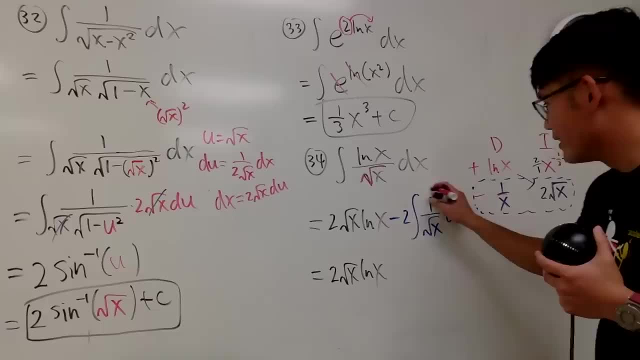 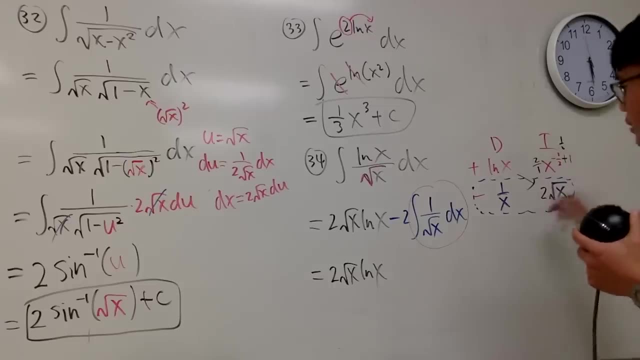 We did this one earlier already. It was the red part, x to the negative, 1 over 2.. And then we end up with 2 square root of x. So this right here is 2 square root of x. Okay, 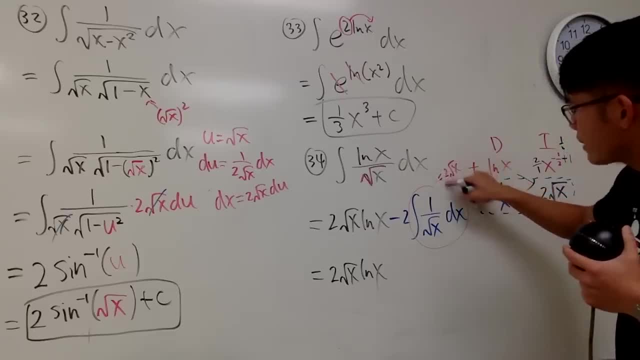 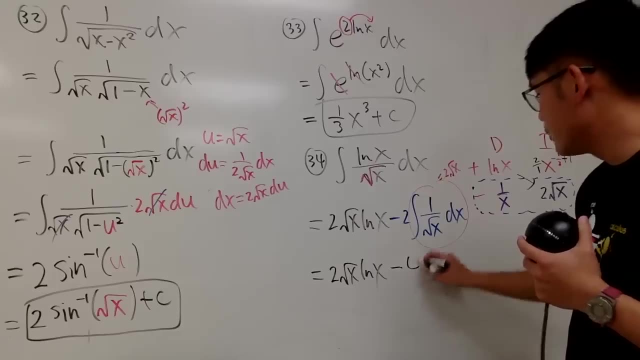 So what we are going to do is 2 times 2,, which is 4.. And we are going to subtract 2 times 2,, which is 4.. And we have the square root of x. With that we are done. 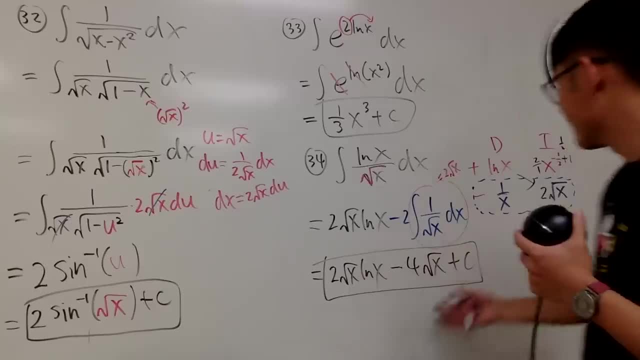 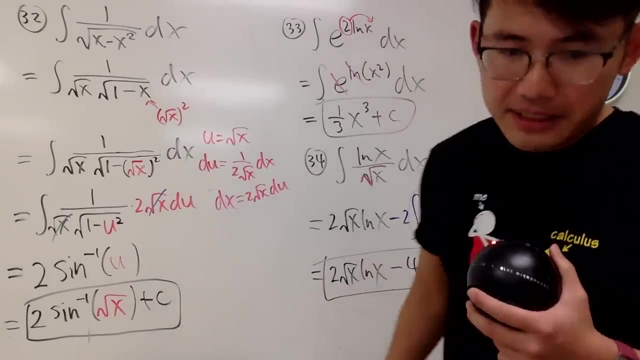 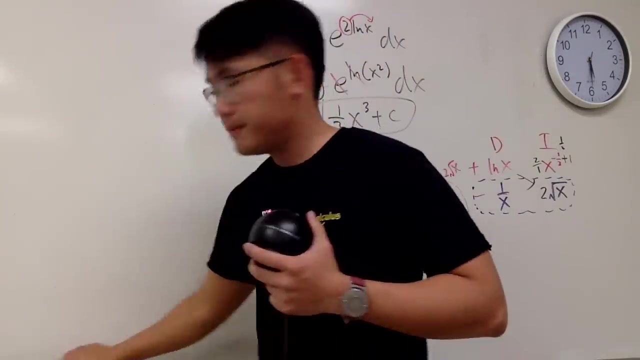 This right here is it All right. So that was positive, So keep it positive. All that stuff Very nice, Okay. 35.. 35.. 35.. 35,, 35,, 35.. Integral of 1 over. 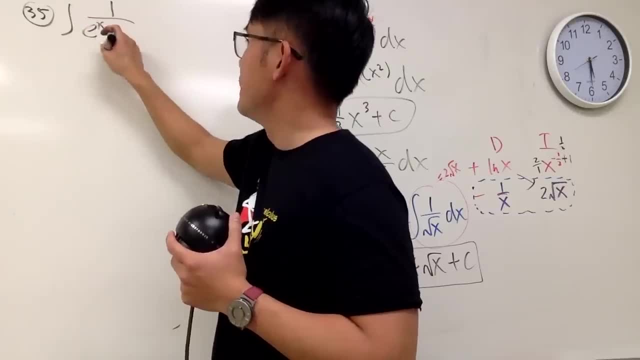 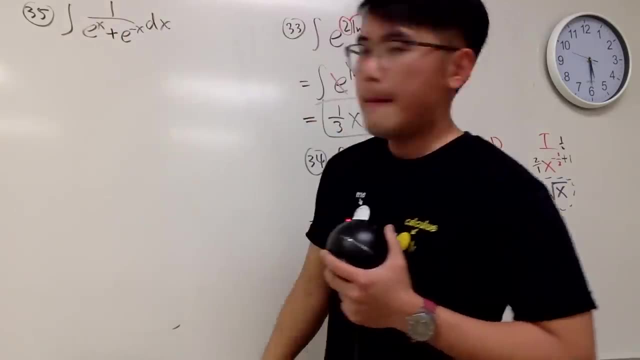 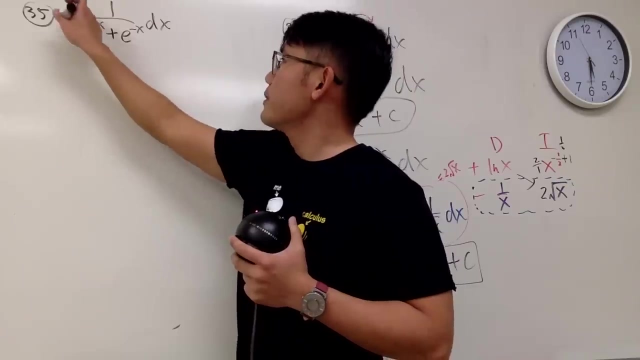 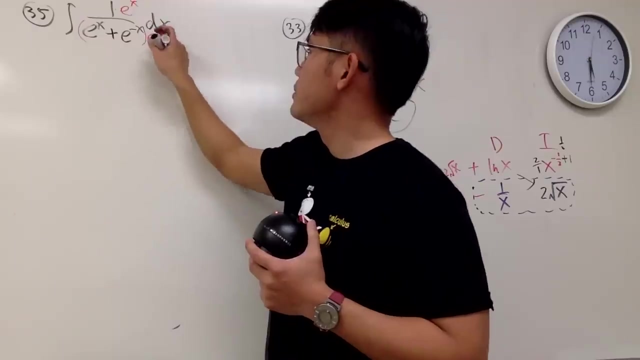 e to the x plus e to the negative, x. Right, Hmm, Oh my god, we have negative exponents. Usually we don't like to have negative exponents. what can we do? Well, we can just multiply the top and bottom by e to the x, e to the x. 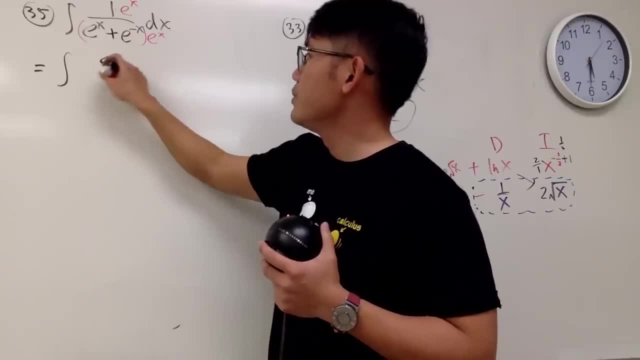 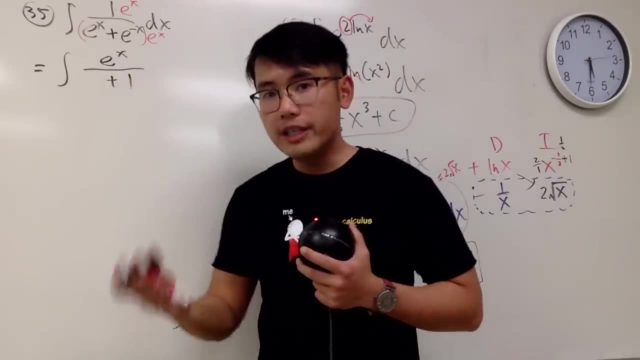 And with that said, you have the integral of e to the x on the top. over this times that will give me just 1.. It's a nice 1.. This times that will give me e to the x, and then square, Let me. 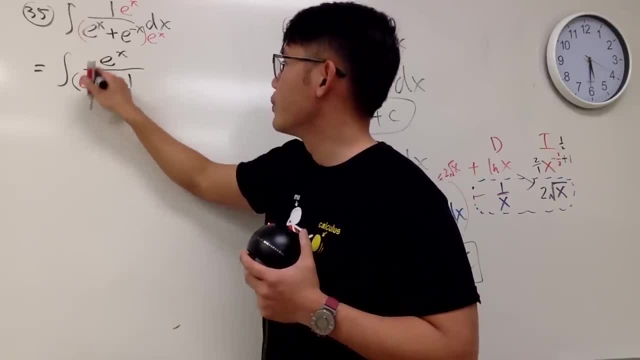 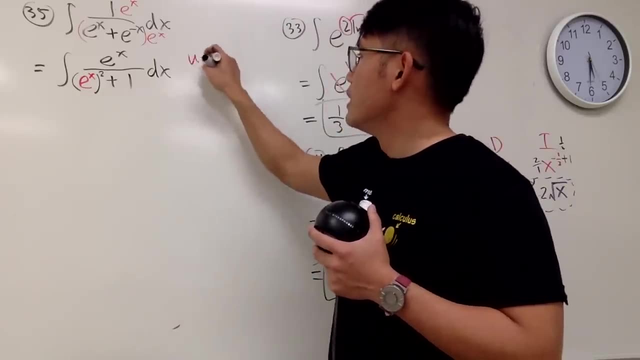 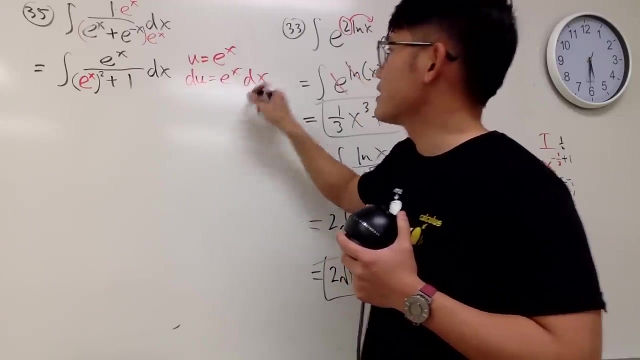 look at it like this: e to the x, and then we square that the x. And why? Because I will take a u sub. let u equal to this, e to the x, And then du will be e to the x, dx. Aha, We have that. 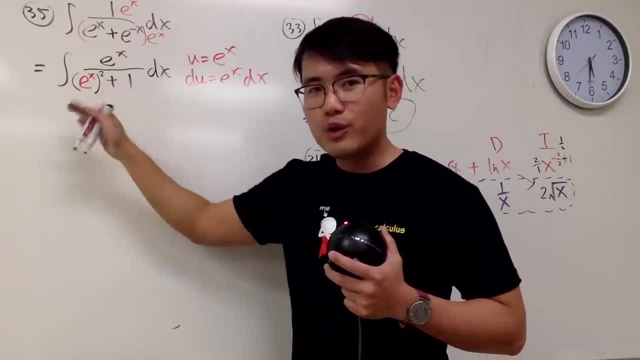 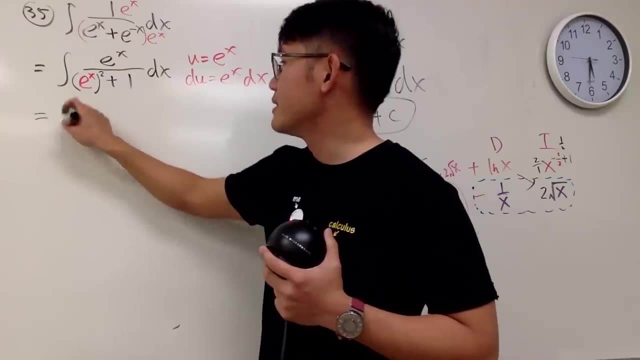 on the top. So you pretty much will have 1 over u squared plus 1 in the u world, And when you integrate that it's an inverse tangent situation And all in all you endow it the inverse tangent of u, which is e to the x, And you can write this down, you can do the u sub in your head. 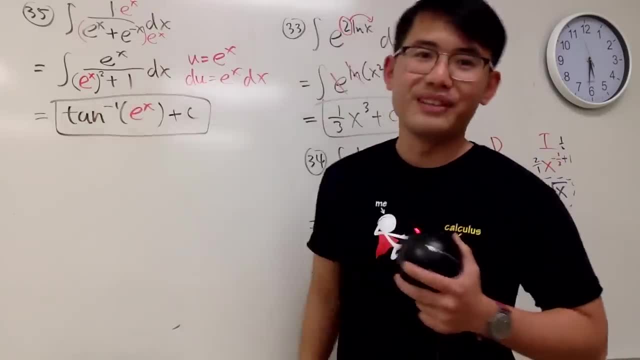 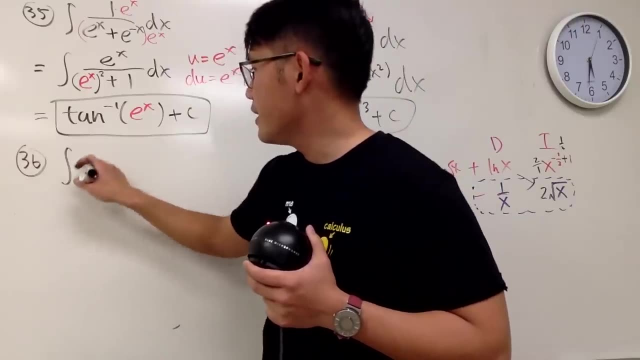 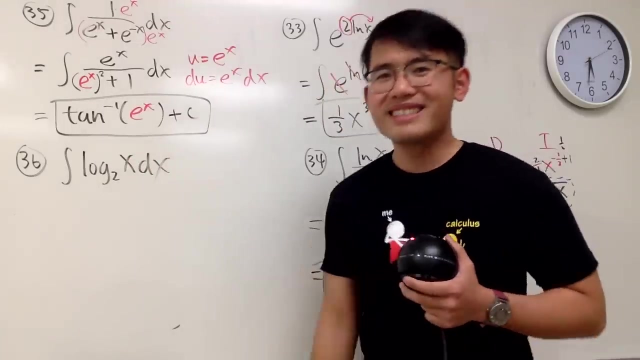 You can also write it down and differentiate it. You will get that for the answer. Very nice, Okay, number 36.. Integrating log base 2 of x- dx. Oh, my god, we don't usually talk about log base 2. 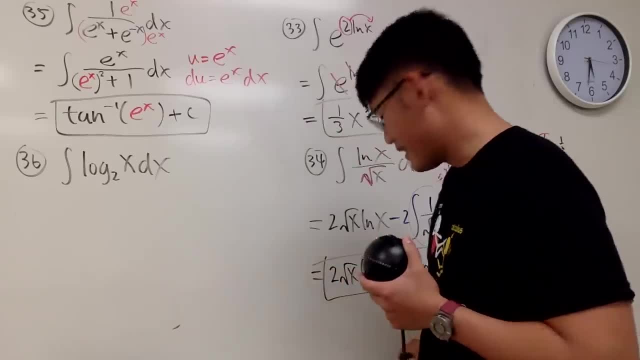 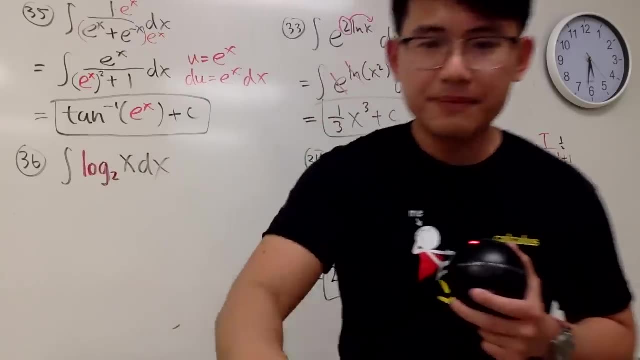 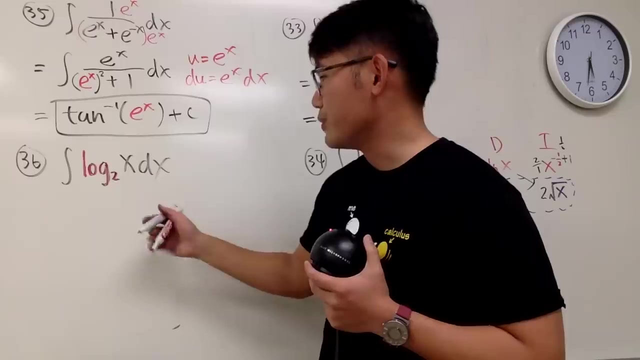 in integrations or differentiation, but we still have to face them sometimes. So here we go. We have log base 2, like that. Okay, we are going to use the change of base formula because we don't like log base 2.. So here is the deal. 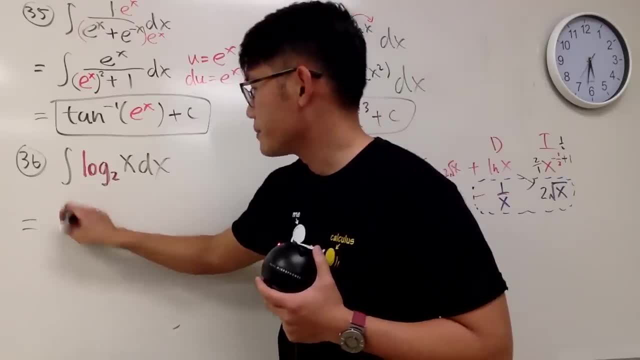 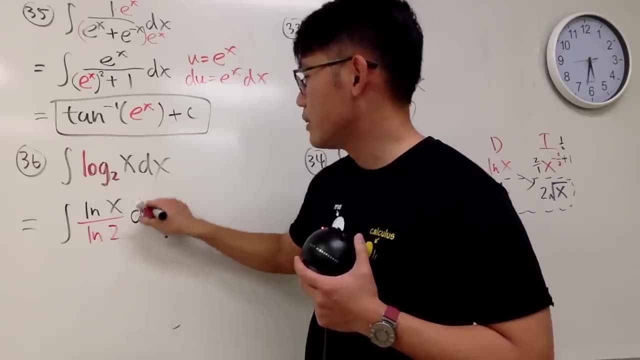 I want to use natural log right. So the change of base formula says this right. here is actually the same as natural log of x over natural log of 2.. And natural log of 2 is a constant. You can just take that to the front. 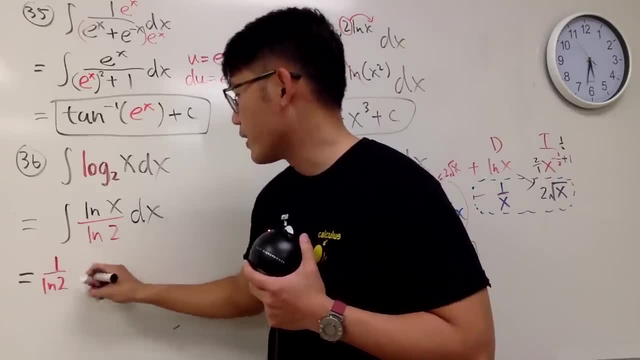 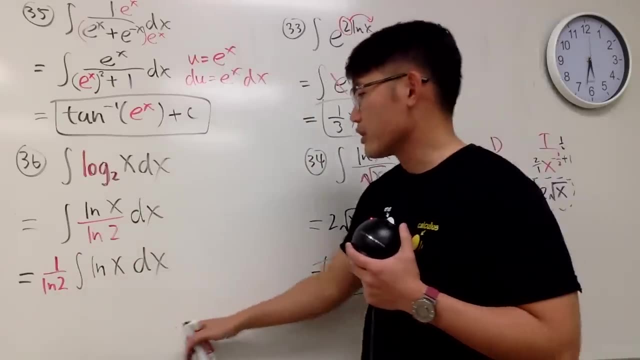 So you have 1 over natural log of 2 all the way in the front And we have to integrate. Not that we areATHING 1000.. We just have to keep integrating until we get an extension нож 4 times natural log of x, like that. 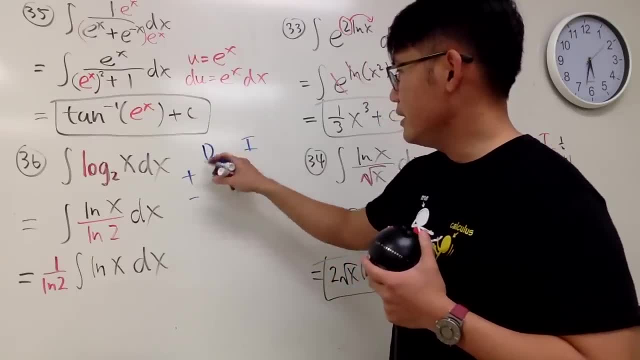 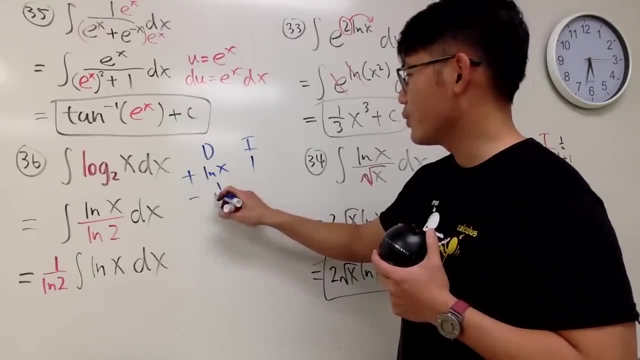 Well, what's the integral of natural log of x? Again, we have to do it by integration by parts. So, if you remember the answer, that is good, but if not, do it Integrating 1, because I cannot integrate the natural log. that is what I am trying to do. 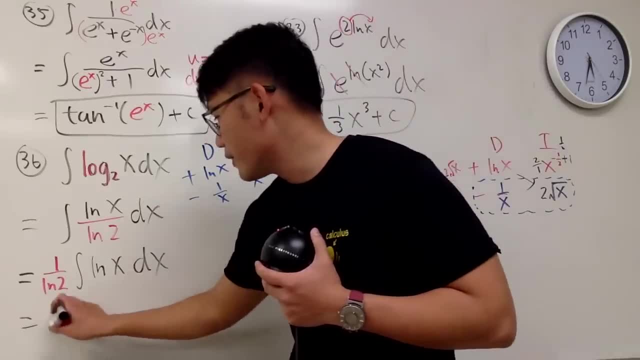 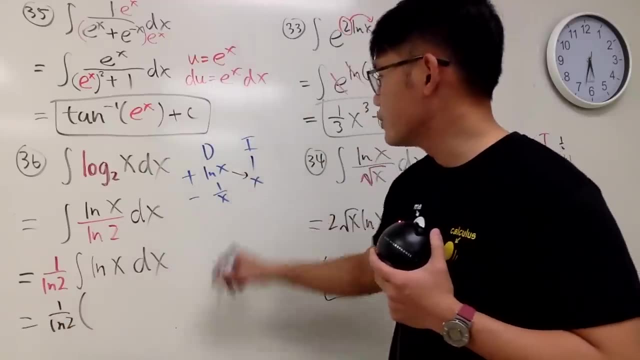 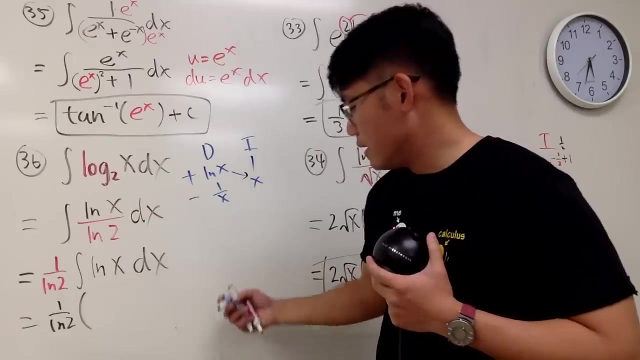 Differential this guy: I get 1 over x. Integrating this: I get x. That is nice. 1 over natural log of 2 in the front parentheses, and we will have the inside being this times that which is x, natural log of x. Let me do this down in blue, why not? I still have. 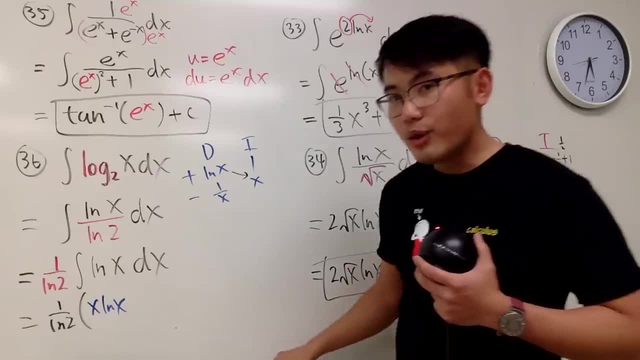 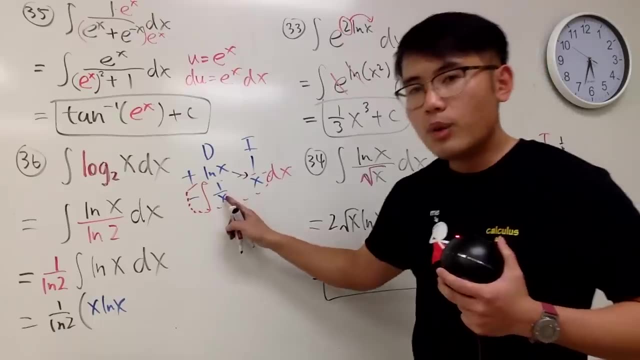 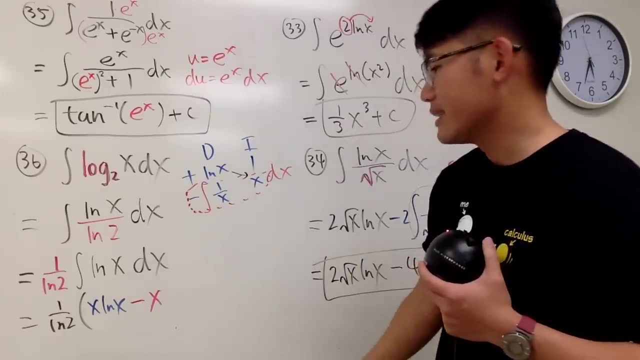 this right here as x times natural log of x. and don't forget, when you multiply this right here, this is still an integral 1 over x times x is just 1, integrating 1, you get x, so you have minus x, like that. okay, So that will be pretty much it, but do you guys? 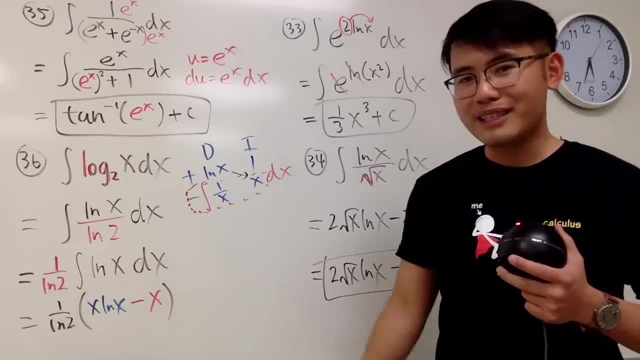 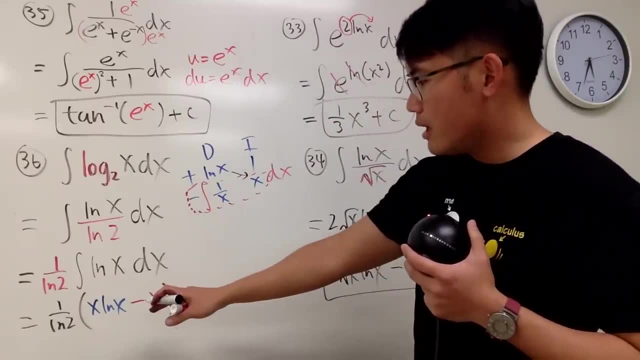 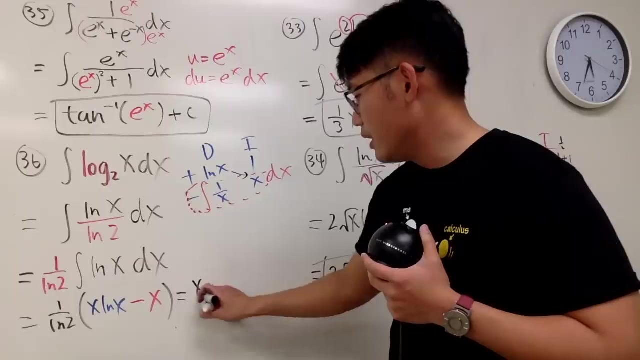 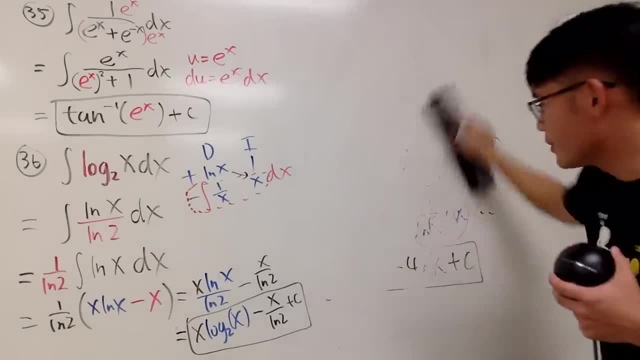 in blue. you get x. I'll put this down in blue. you get x. I'll put this down in blue. you We are doing good. we are doing good, we are doing good. Take a look at my mirrors of metal. 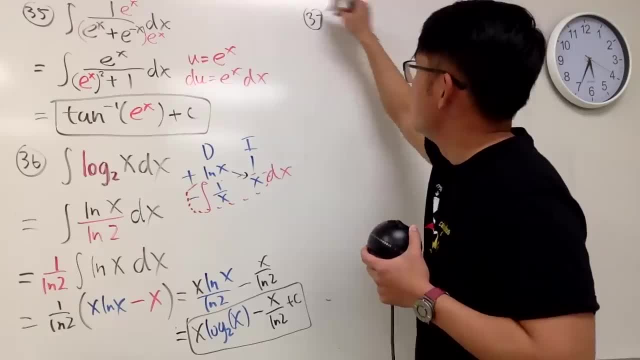 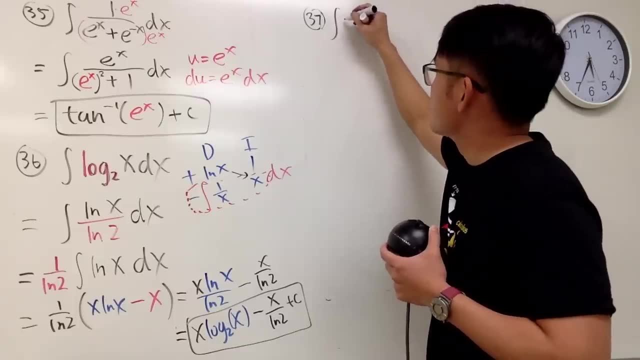 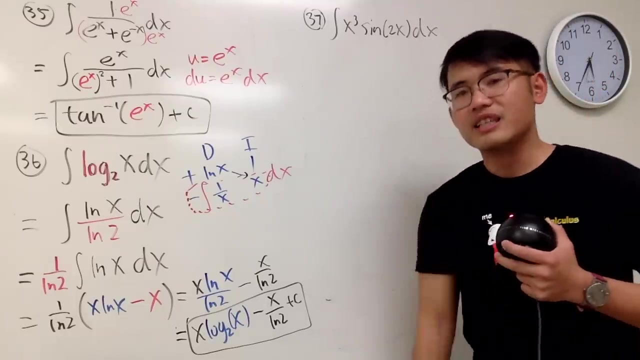 Okay, number 37.. This is a fun one. People like it. People wish that I put this one on the test: Integral of x cubed sine of 2x dx. How do we do this? Yes, integration by parts. 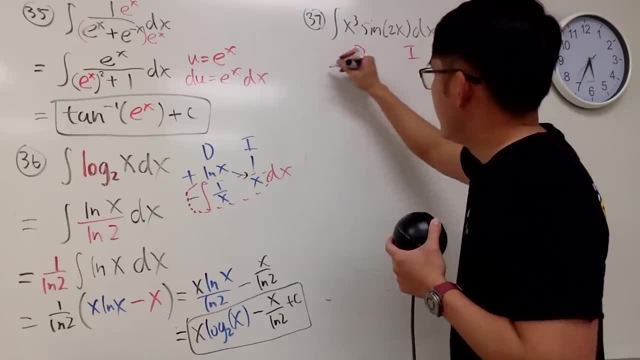 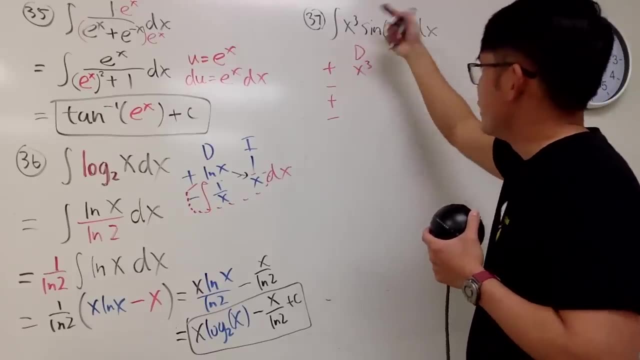 So let's put down d and then the i right here And I will have to have, let's see, plus, minus, plus. I don't know how many I need, But let me just write down: I want to differentiate x, cubed. 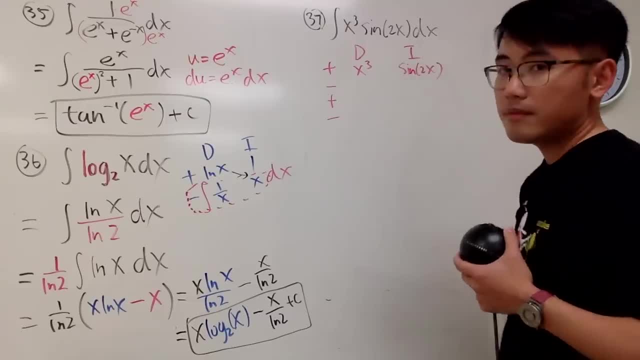 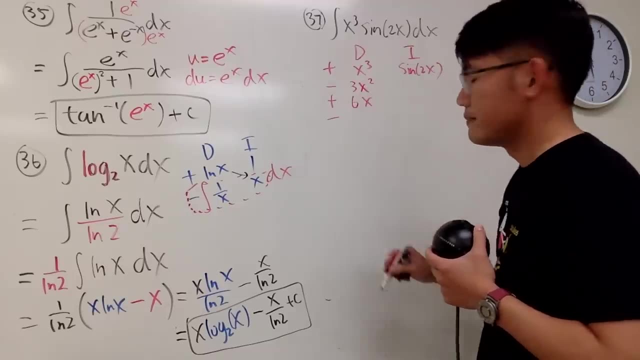 I want to integrate sine of 2x. The truth is, when you differentiate this, it's nice: 3x squared 6x to the first, power 6.. I need one more, So put down plus and then. 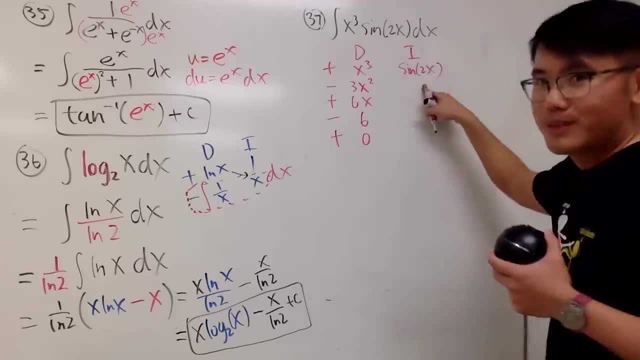 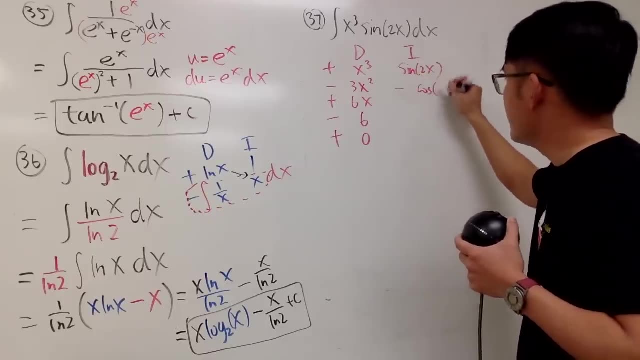 And then the root of 6 is 0, like that. So we also have to face the integration. Let's see, we have to keep our mind straight: Integrating sine, we get negative Cosine, and then the input is 2x. 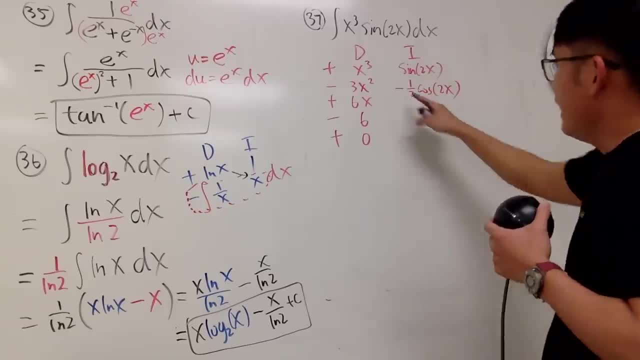 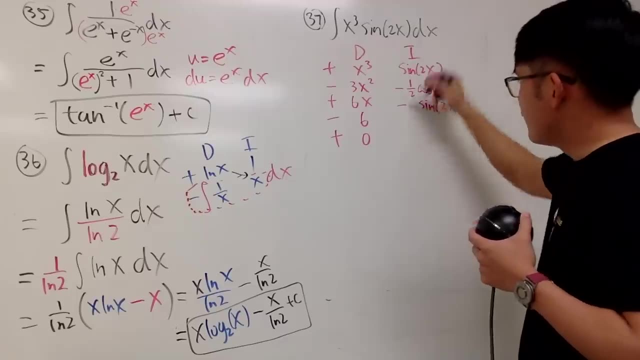 And then you have to divide it by 2. Integrating cosine is positive sine, And then the sine stays the same. The input stays the same. Divide it by 2 again, so you have 1 over 4.. Do it again. 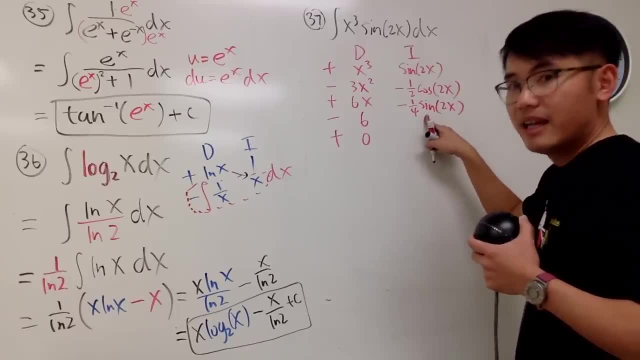 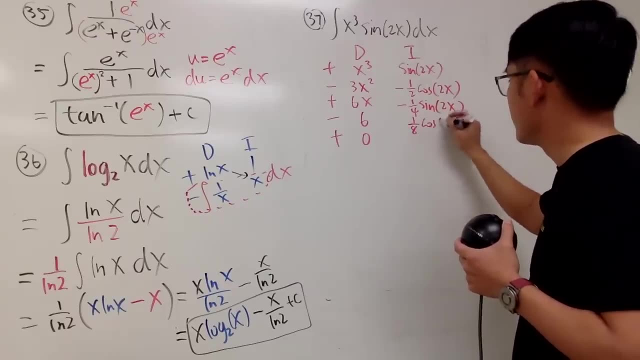 Integrating sine, you get Negative cosine, Negative times. negative is positive, So we have positive And it's going to be 1 over 8, because you have to divide it by 2 again. Do it again, Because this is for that row. 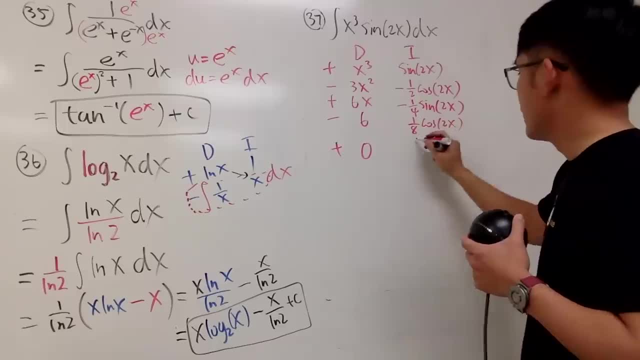 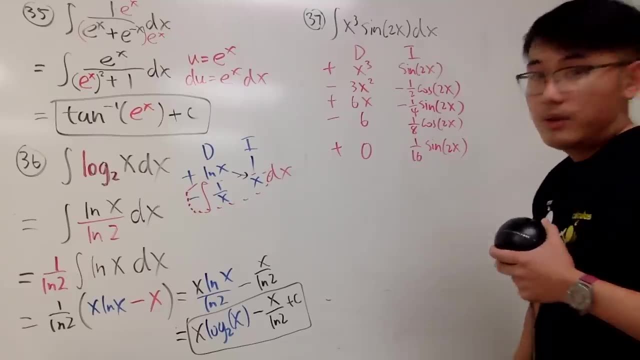 And then let me just write down plus 0. So you have 1 over 16. And then the integral of cosine is positive sine And then the 2x stays. First part, second part, third part, fourth part of the answer. 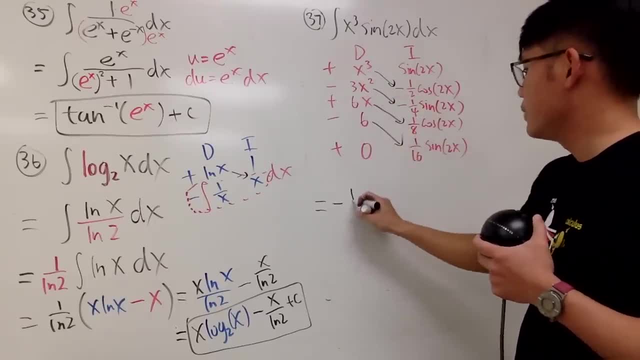 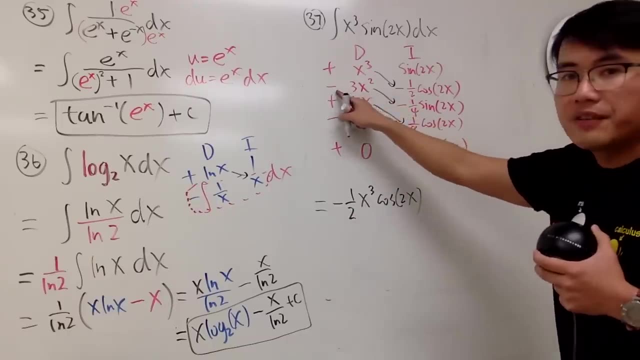 So final answer: let's see, I will do this times that which is negative: 1 half x cubed cosine of 2x, and then negative times negative, I believe that's positive, 3 over 4, x squared. 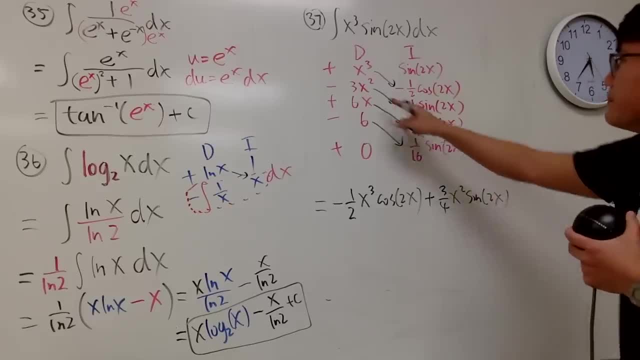 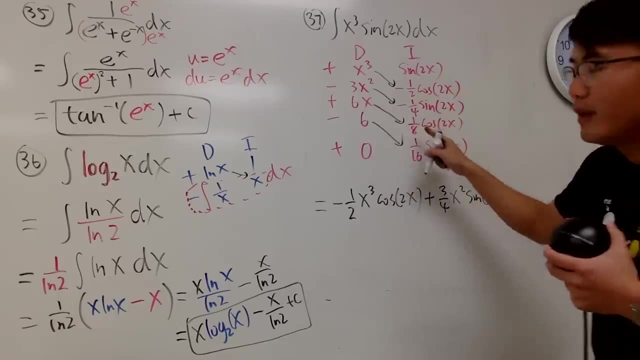 and then we have sine of 2x, right, Yes? And then this times that is positive, 6 over 8 is 3 over 4, so reduce your fraction 3 over 4, and then the x. 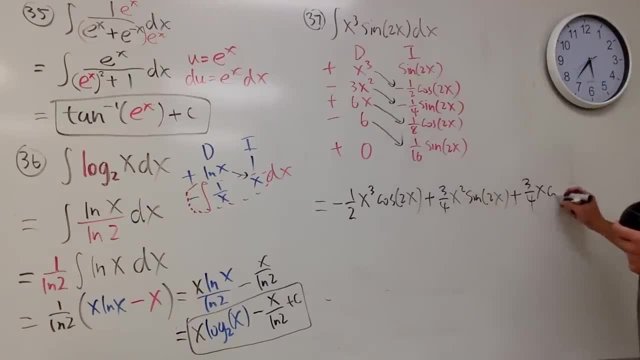 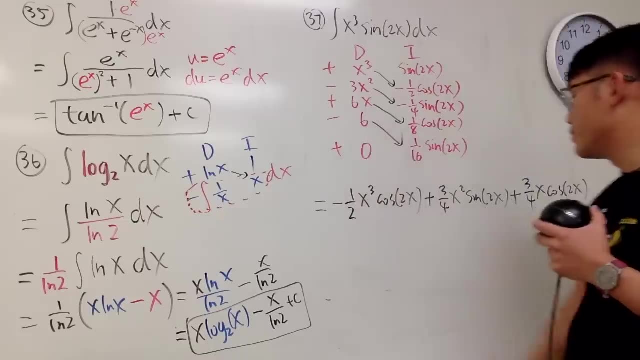 And then again, here we have the cosine of 2x, And lastly, 6 over 16, divided by 2, divided by 2, so we have 3 over 8, and that's a minus minus 3 over 8,. 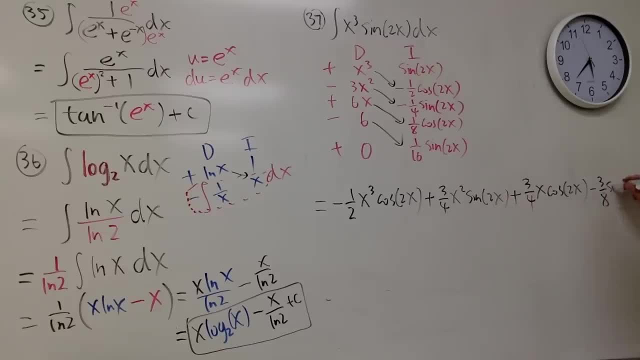 and we have sine of 2x, Right. And in case if you guys cannot put, cannot see a plus C, I'll just put on plus C right here for you guys, Right? So here is the answer, As you guys can see, after 37 integrals. 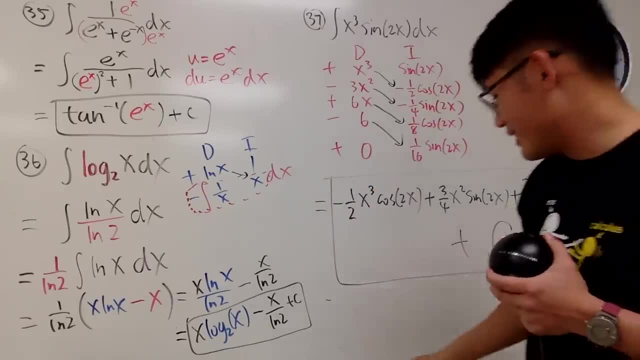 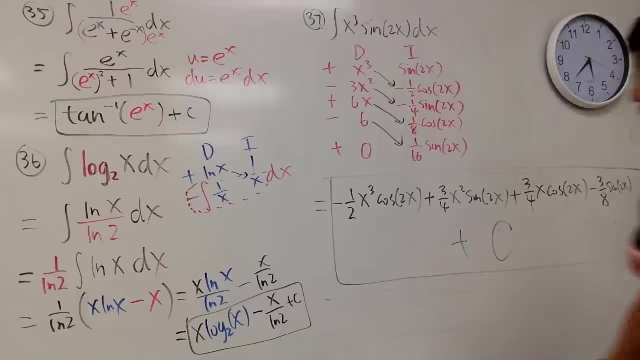 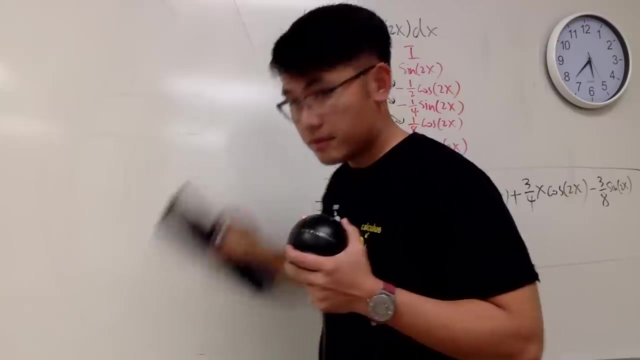 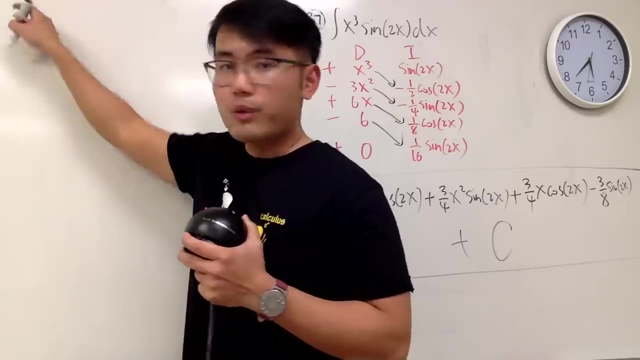 this brand new marker earlier is trying out. But it's okay, We are still strong. okay, We stay strong. So that's number 37.. So now let's see 38.. Let me write it down right here: 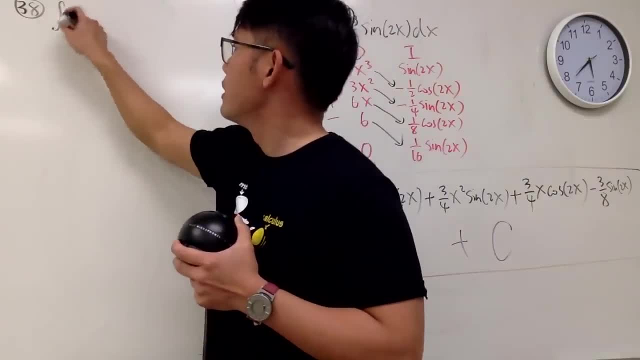 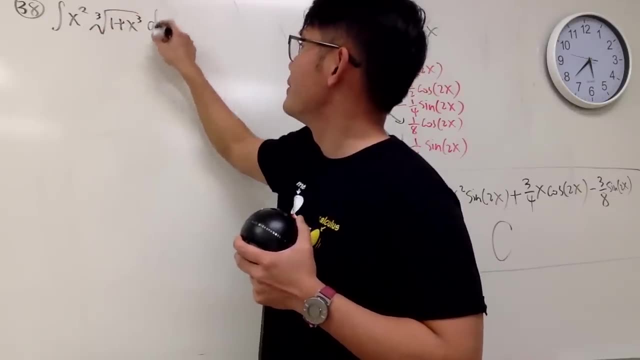 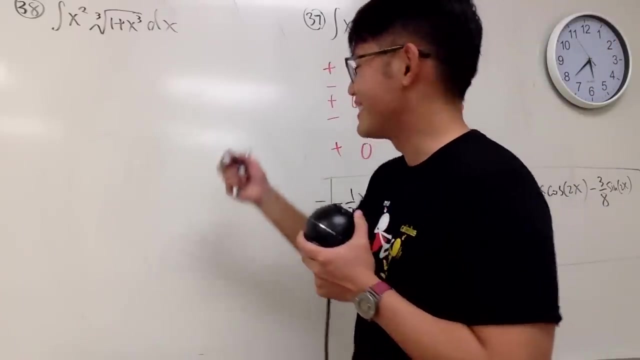 We have the integral of x squared times the cube root of 1 plus x cubed. Looks kind of weird, but it's actually pretty easy because we can actually just do a nice use up for this. Let u equal to the inside. 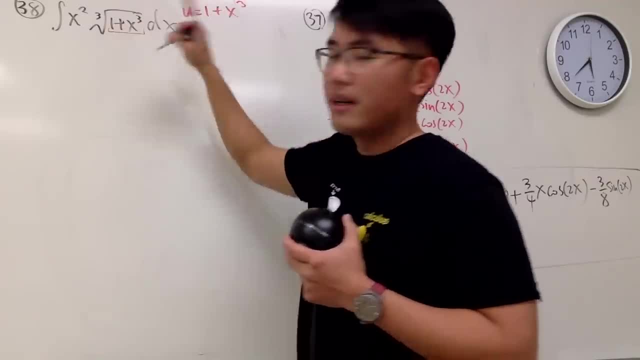 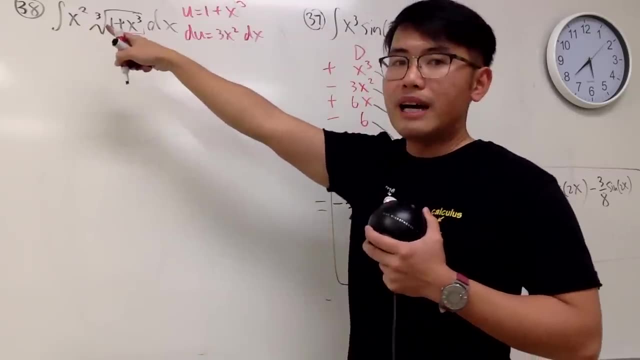 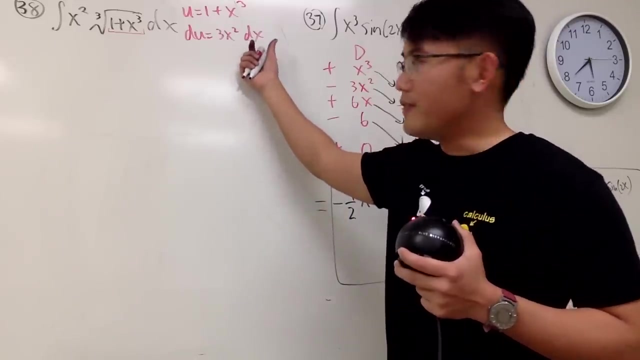 1 plus x cubed. Why? Because the derivative of this du is precisely 3x squared dx, and you see, you have that over there already. Now I will show you guys something that's slightly different. Usually, you can just divide this on both sides. 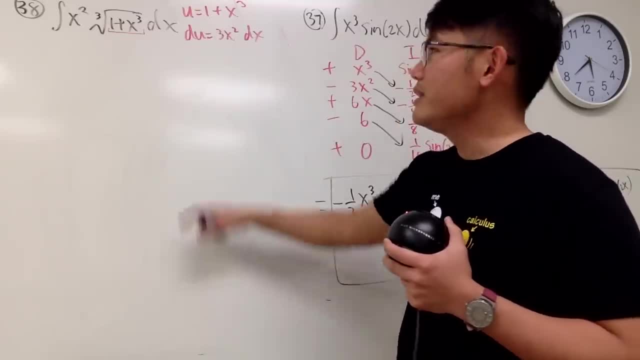 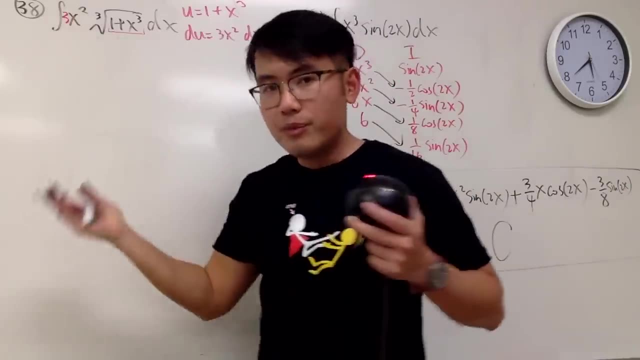 to isolate the dx. But you see, I just need a constant multiple And look at 3x squared. that's what we need. I don't have the 3, so let me multiply by the 3.. But if you multiply by the 3,, 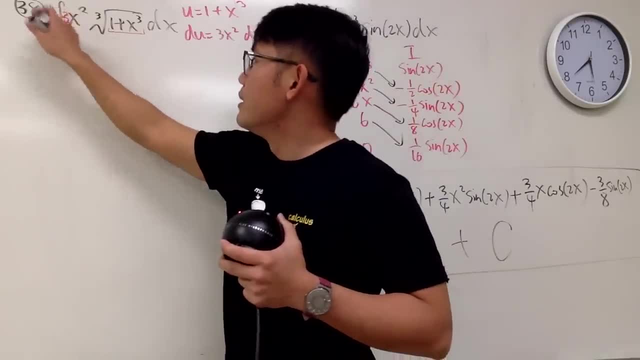 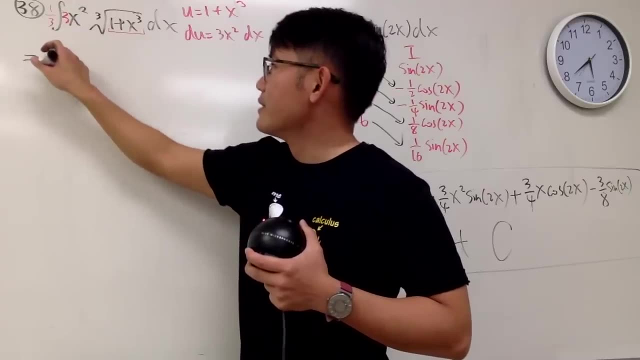 you change the whole thing, so that's bad. So now you can just divide it by 3.. That's okay. So now, what I'm talking about is this: right here is the 1 third. okay, We have 1 third. 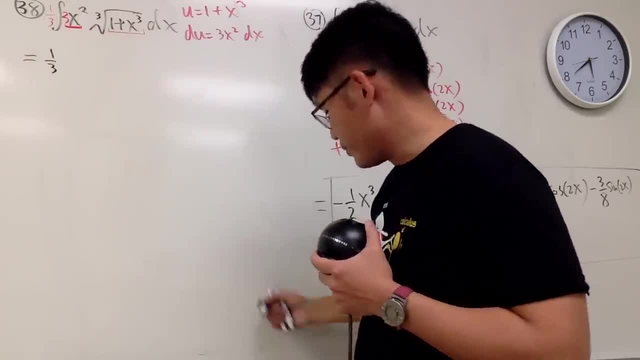 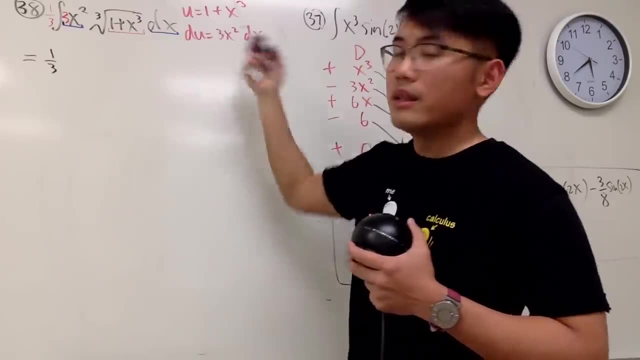 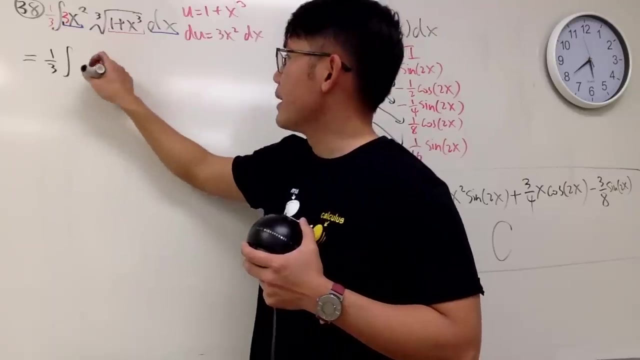 But this and that I'll put this down in blue to make it stand out: The 3x squared along with the dx is our du now Very nice, So I will just write this down as the integral. This inside is still my u. 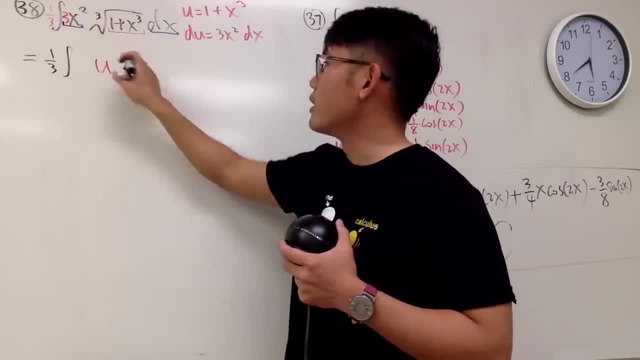 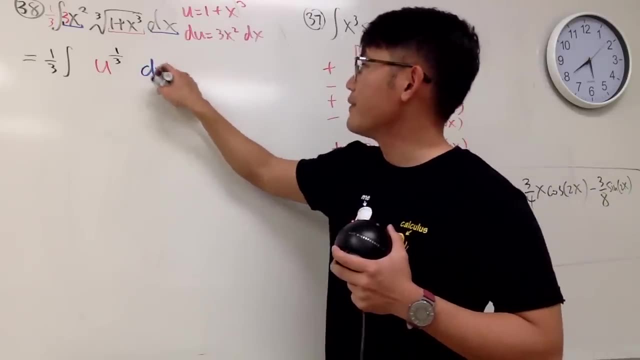 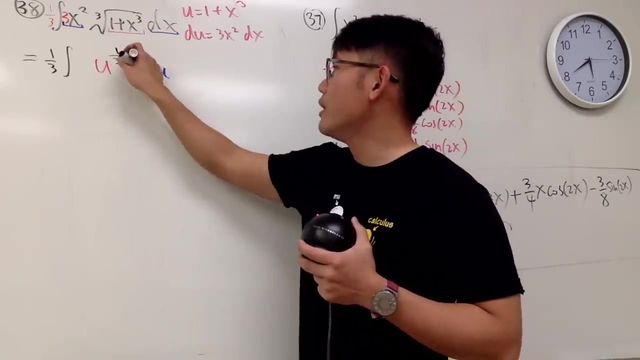 And then the cube root is the same as 1 third power, So I'll put that down as the 1 third power. Again. the rest right there will be the du that we have. Very nice, And to integrate this, of course, we're just going to add a power. 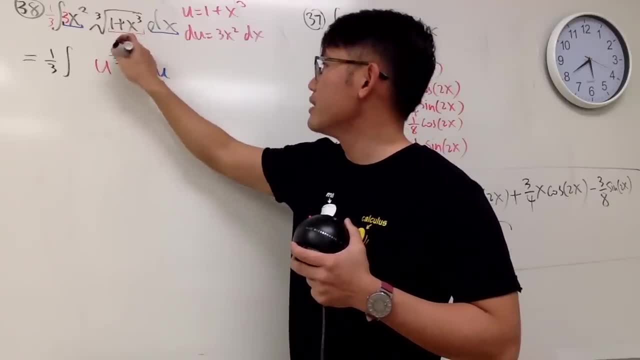 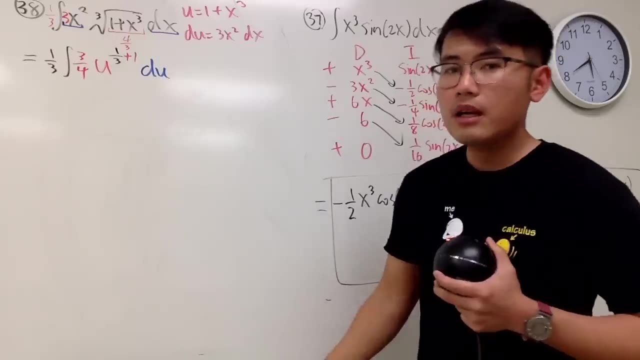 1. third plus 1 is going to be 4 over 3.. So you look at this as 4 over 3, divided by this new power, which is multiplied by 3 over 4, like that. In the end you see that 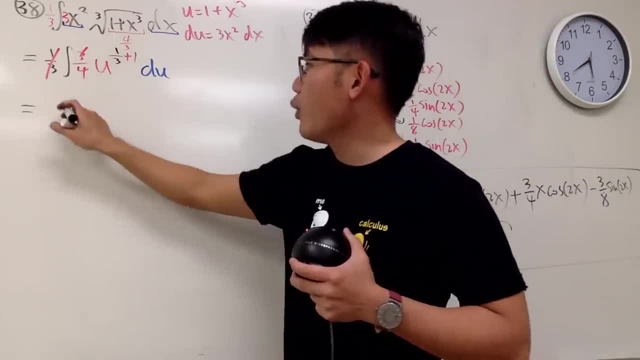 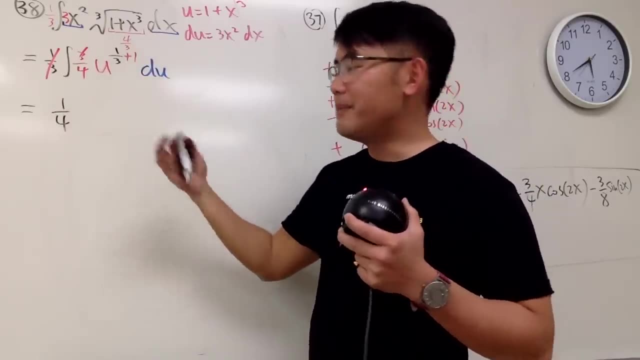 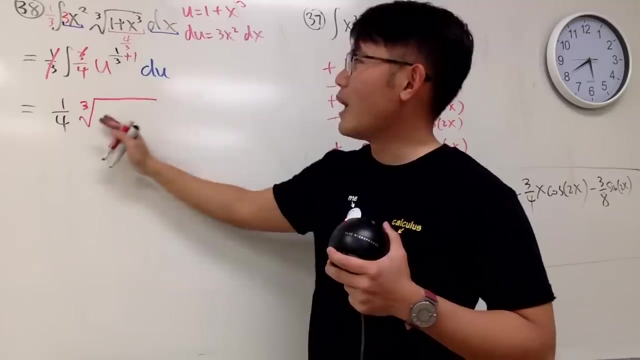 this and that cancel and we have 1 over 4.. You have u to the Well depends how people want to look at it. I think in calculus we are fine. We can just write this as the cube root And then u to the fourth power inside. 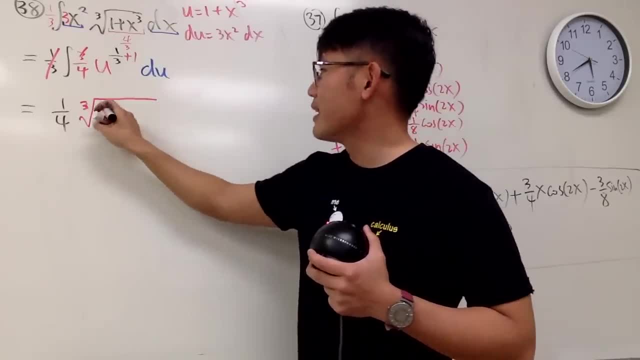 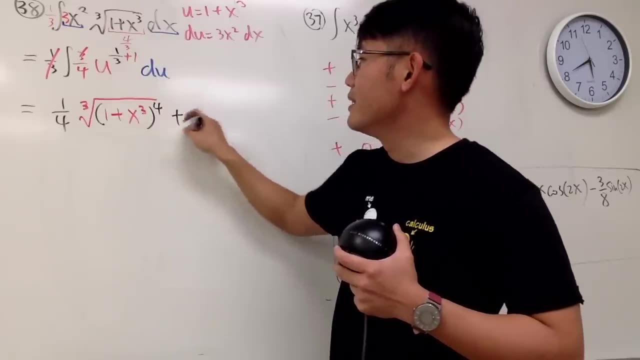 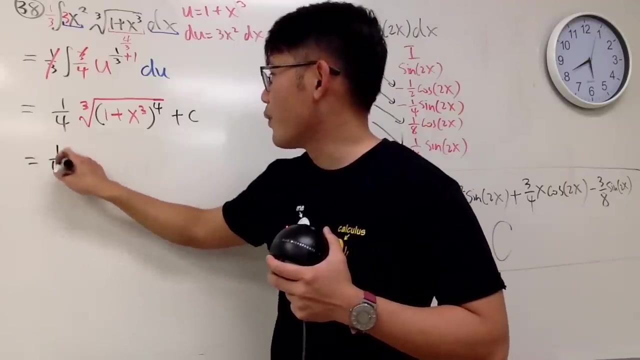 And u is that guy. So I'll just put this down as the parentheses, with 1 plus x cubed, but to the fourth power like this, And if you want to reduce this more you can, You can write this down as 1 over 4,. 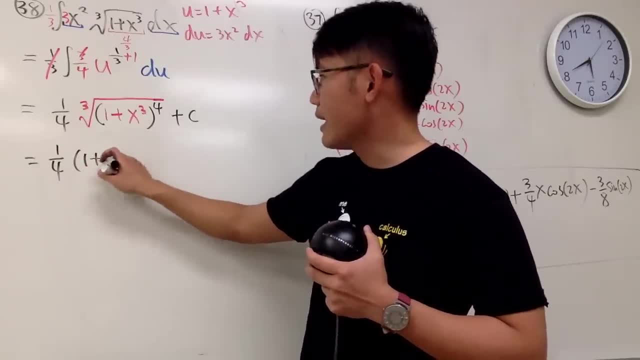 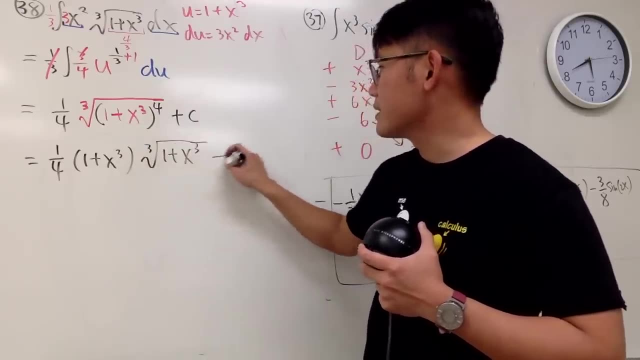 and you can take out one of the 1 plus x cubed to the first power and you will just have the cube root of 1 plus x cubed inside, like this plus c. So I think this might be better for some people. 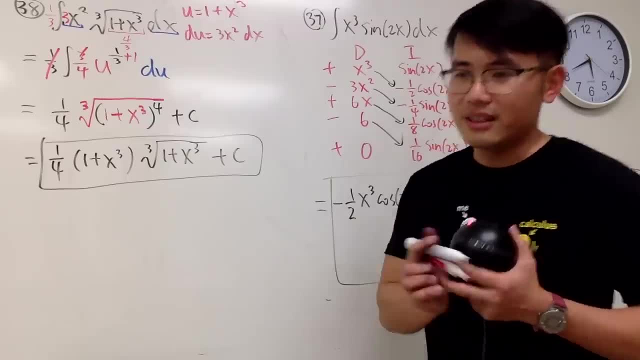 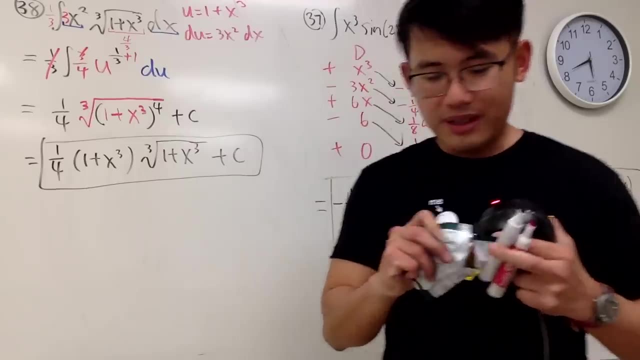 For the textbook question. they may want to just do that for the answer in the back of the book. You know, after you, When you guys run marathons, if you guys like reach the halfway mark, you can eat like. 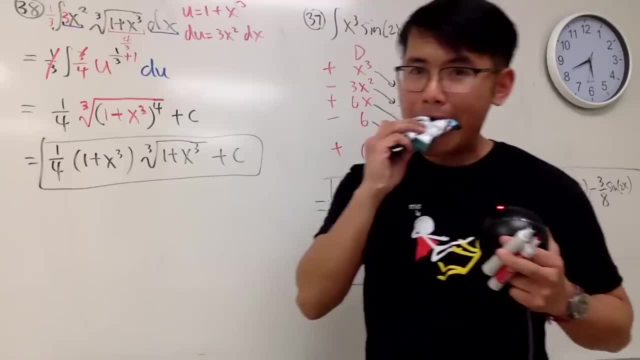 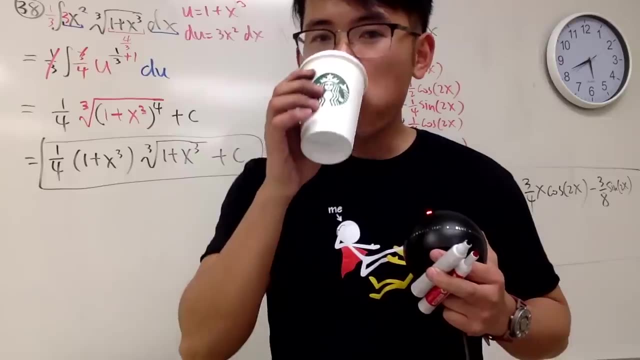 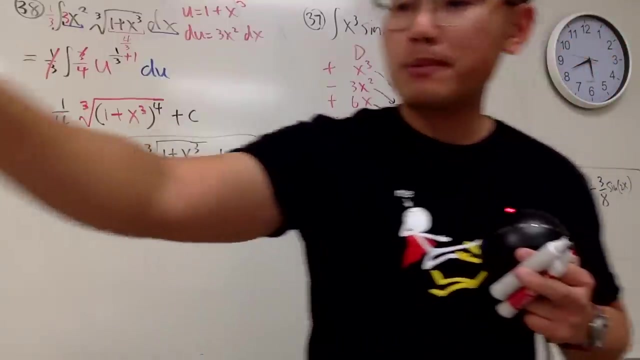 They'll give you like energy gel. So I will eat my clear bar right now And drink some coffee. Maybe later I'll drink some Gatorade. All right, My legs are tired, so that's why I'm like doing this. 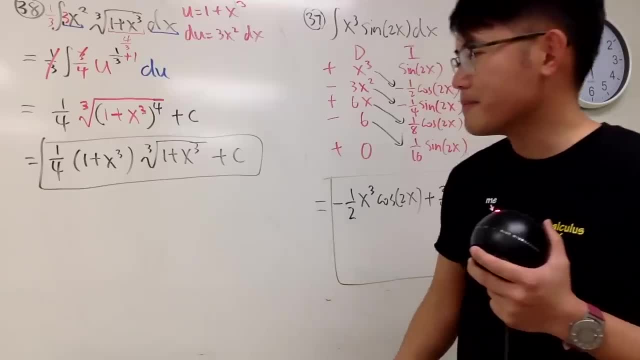 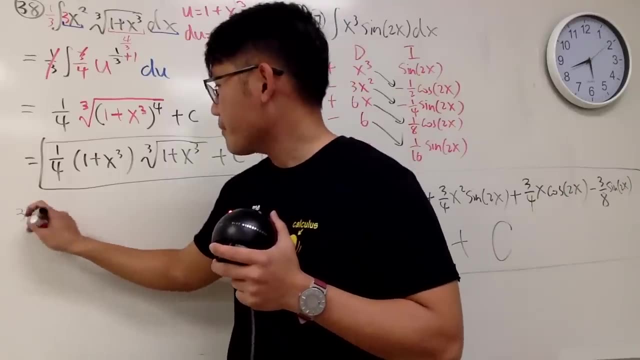 I cannot do 13 notes in this little spot. Well, let's see, I have that behind me, so maybe we can do a lot of this in our heads. So, of course, after 100 integrals, you guys should be like: 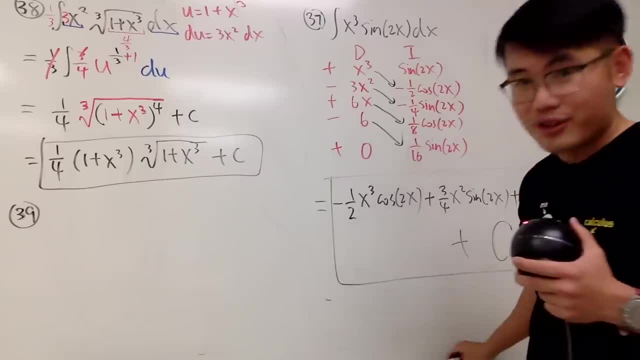 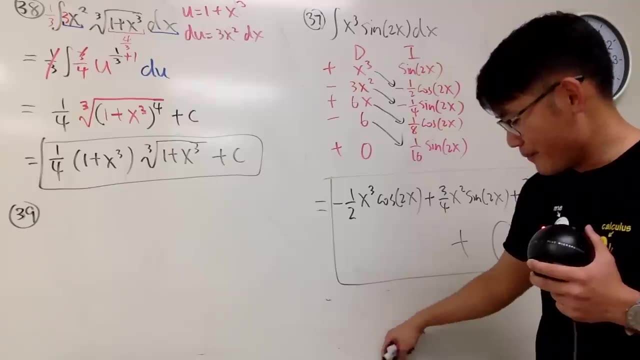 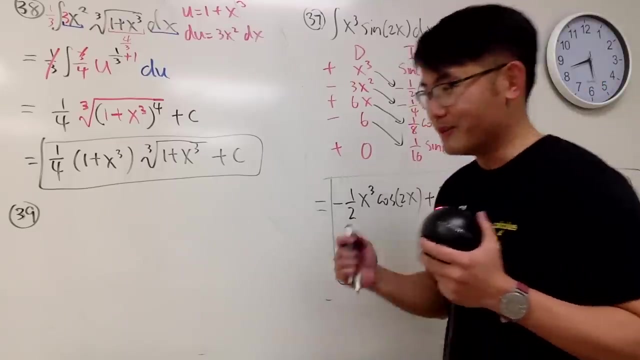 a super expert of integration, right, But the dirty truth is that there are still a lot more out there you have to be careful with. There are still a lot out there in the real life, So be careful, okay, Anyway. number 39.. 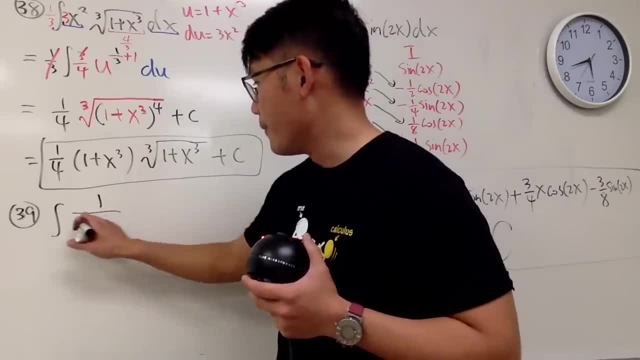 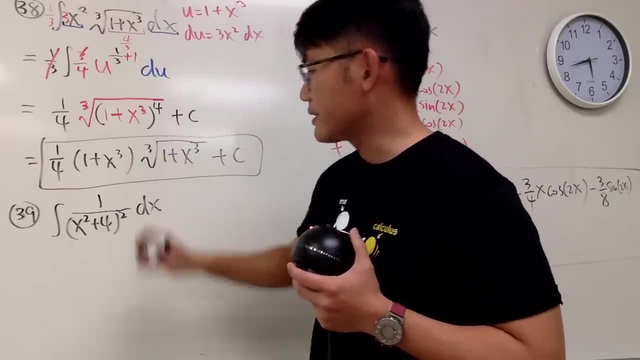 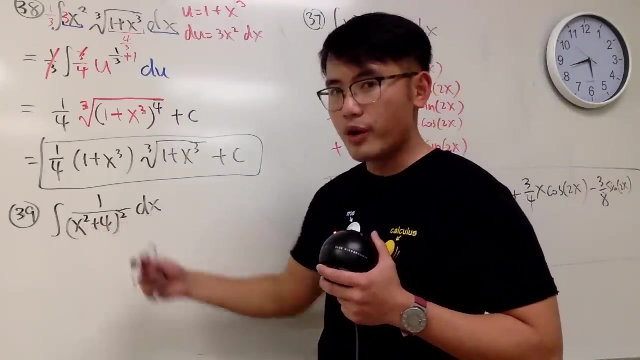 We are going to integrate 1 over x squared plus 4, and then square that like this, And then we have the dx Right: Well, x squared plus 4, which is the same as 2 squared, And in this case, 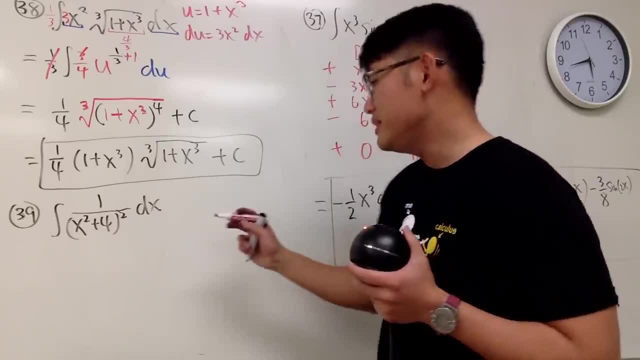 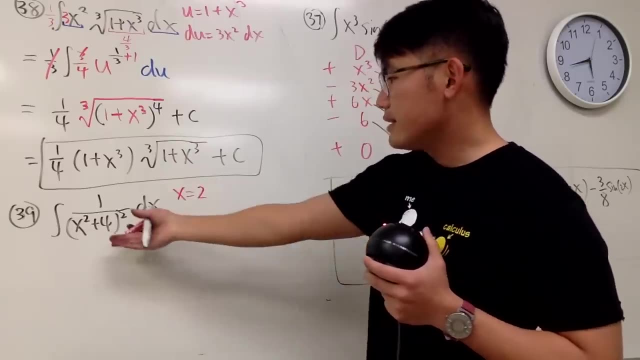 we are going to do tricks up. It's easier this way, in my opinion. What I'm going to do is I will take x to be 2, because the 4 is like 2 squared And this is the sum of 2 squares. 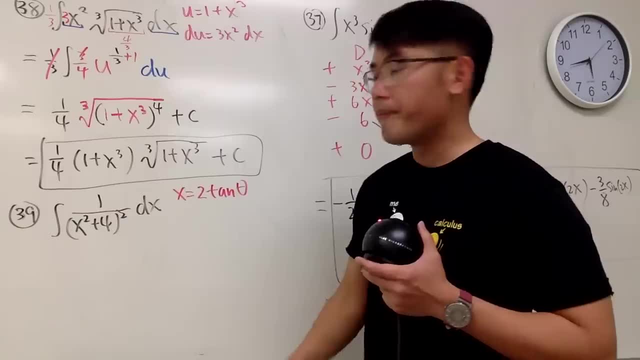 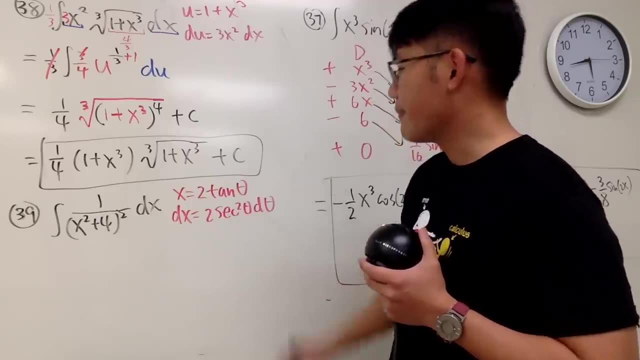 so I will put a tangent for it. So a tangent theta. And then, of course, dx will be 2 times the derivative of this, which is secant squared theta d theta. Now take this integral to the end. This is going to be theta world. 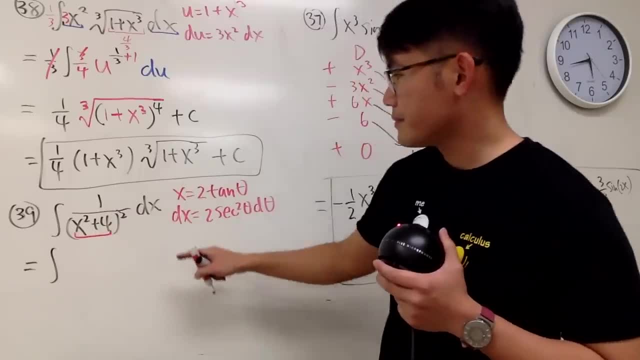 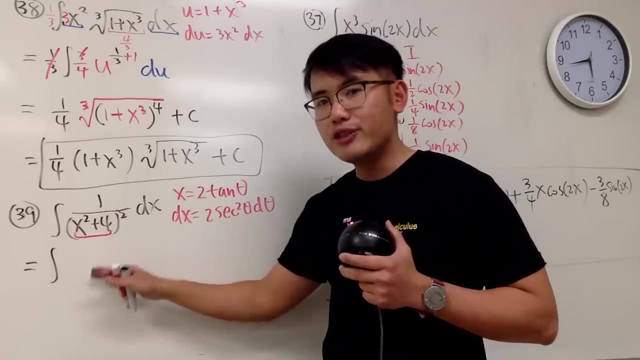 This is going to be the integral. Now check this out. This right here, it's going to give me a 4 in the front if you factor it out, And then tangent squared plus 1, right, Tangent squared plus 1 is going to be secant. 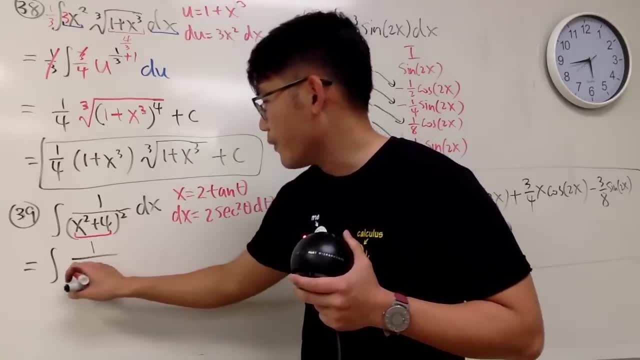 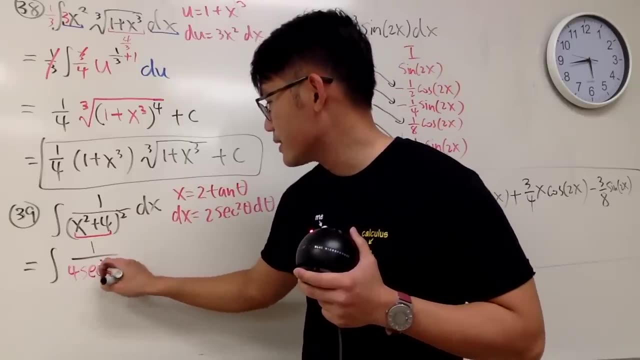 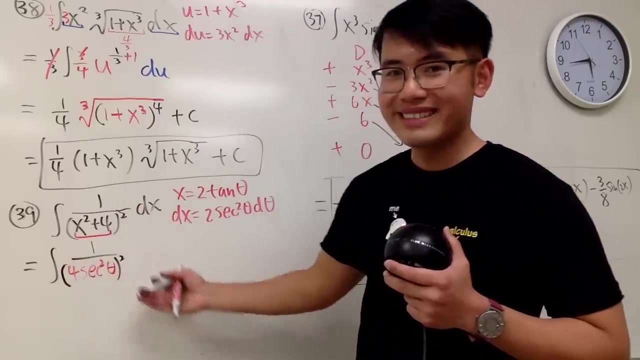 So we will have 1 over 4.. Yeah, 4.. And then secant. Okay, just work this out. Secant squared theta, And then you have to square that right. You still have to square that And you still have to multiply by this. 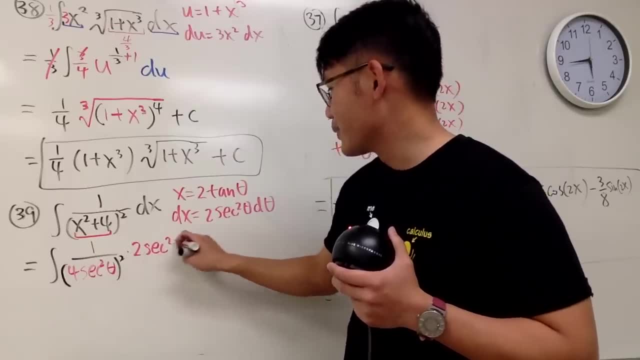 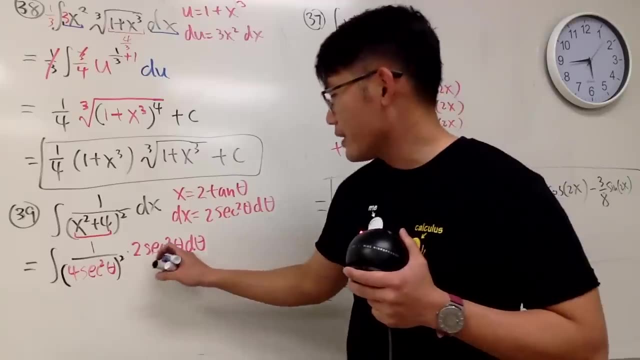 Multiply by 2: secant squared theta, d theta. Now here's the DO. Well, this right here can be cancelled. So you are going to cancel this And this is technically 4, right, Because secant to the 4th power. that's what I mean. 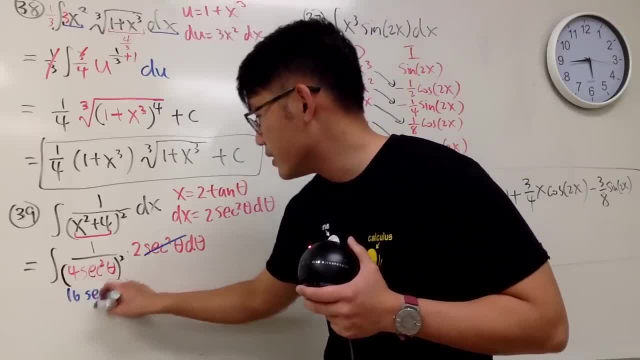 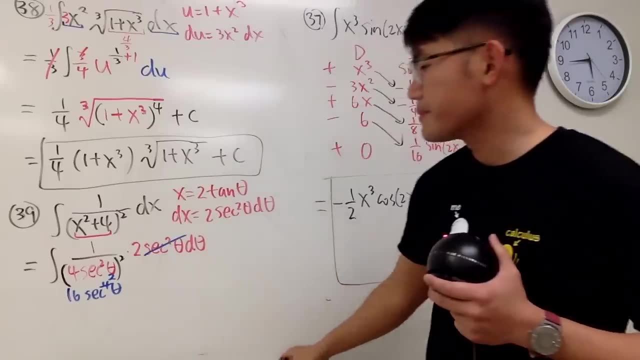 This right here is 16.. Secant to the 4th power: theta. But you can cancel this with 2 of them out, So this is technically a 2. now right, And now, of course, this, and that can be crossed out as well. 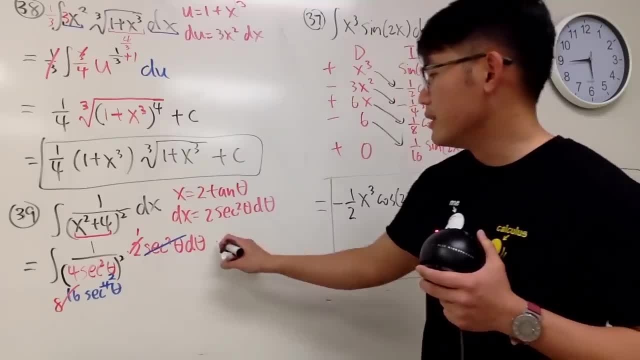 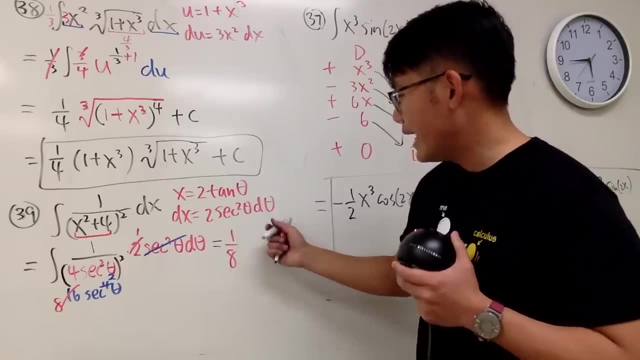 This is going to be 1. And this is going to be 8.. All that little stuff. So technically you have 1 over 8 as your constant multiple, So I'll put that down right here. And then we have the integral. 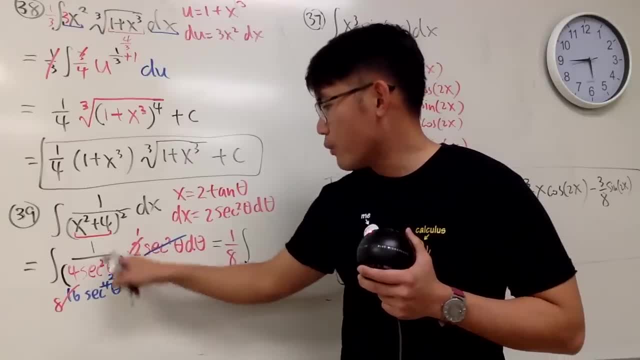 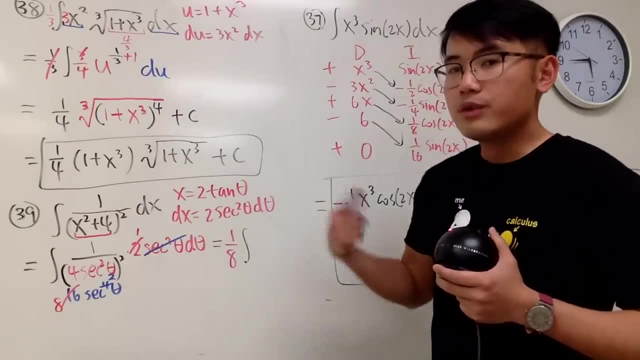 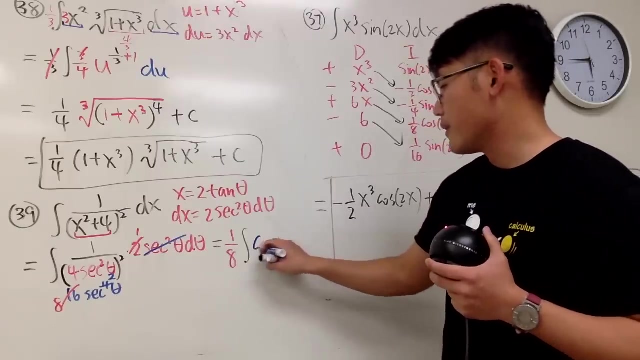 And here's the DO. Now we have 1 over secant to the 2nd power Theta in the denominator, 1 over that, And then to integrate that we have to bring that up to the numerator in another way, which is the cosine squared theta. 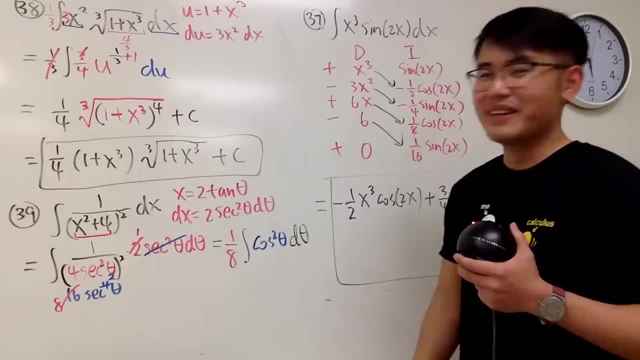 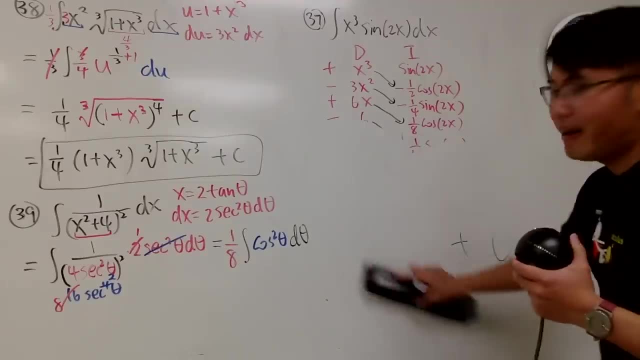 I'm sorry, We cannot do this with this little spot. I don't think so. Let's see, I had to erase this. So to do that, yes, we have to use the reduction, the power reduction formula for for that. 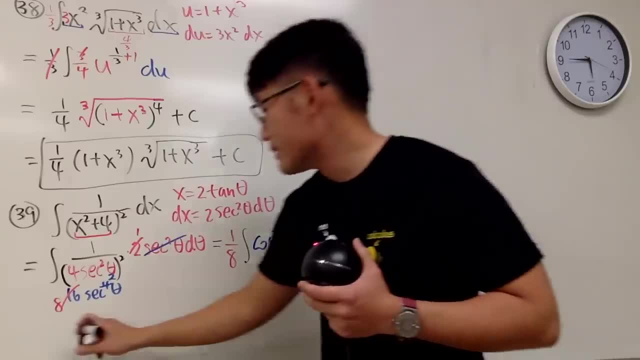 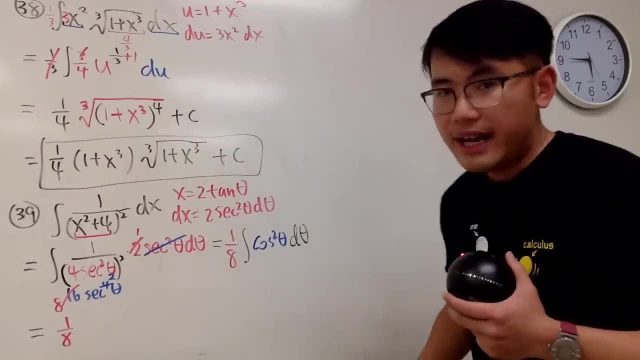 So we will see. Let me try to fit in as much as possible here. Okay, All right, So we have 1 over 8 all the way in the front, And then for the blue part, of course. you know the formula is. 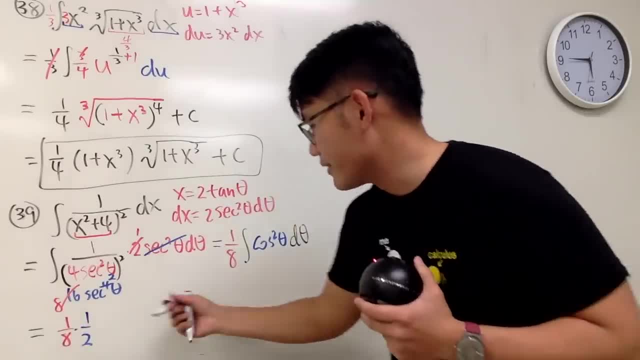 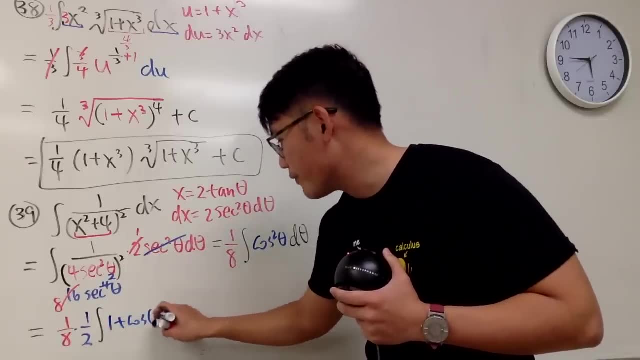 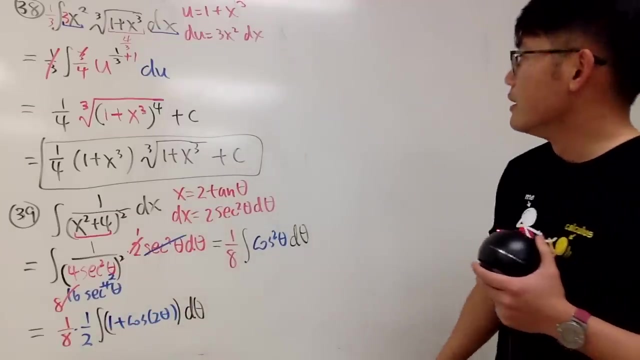 1 over 2.. And then of course, we have the integral, And then the rest is 1 plus cosine of 2. theta like this in the theta world. So it's like that. So perhaps I will just continue right here. 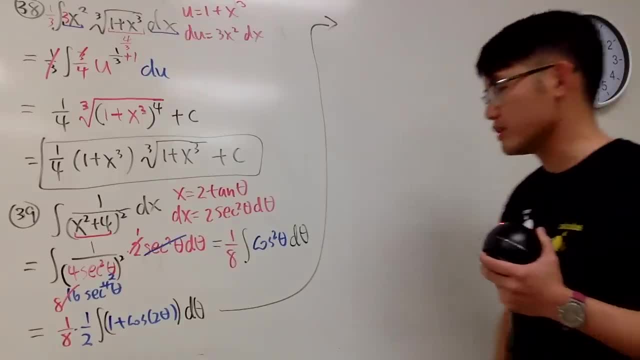 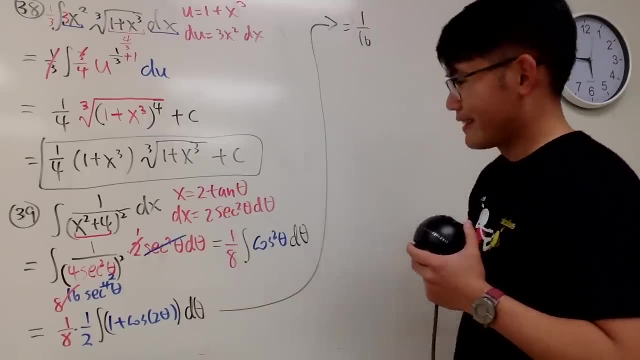 This is also integral. sine you guys So cool. Look at that Now in the front, all the way in the front. this is equal to 1 over 16. And let's put down a parenthesis. and the result: of integration. 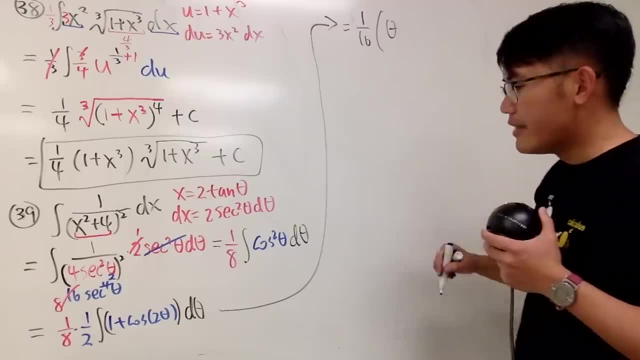 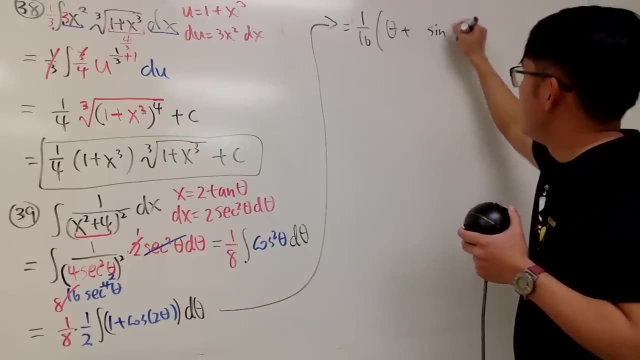 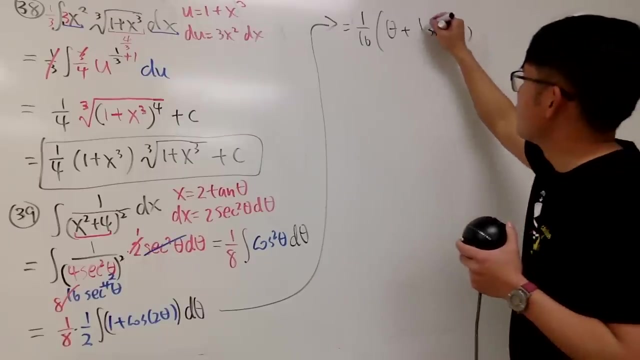 Integrating 1 in the theta world is theta, And then integrating cosine, we get positive sine And the input state is the same. But we have to divide it by that 2, which is the one half right here. All right, 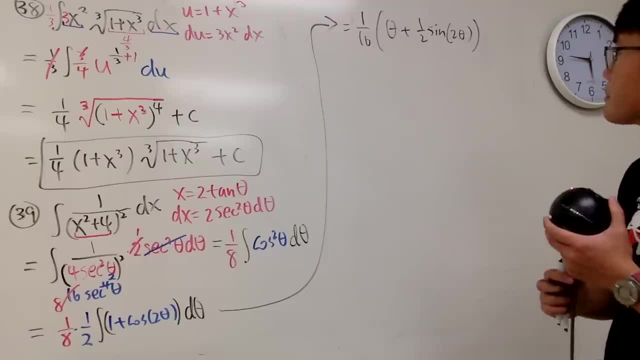 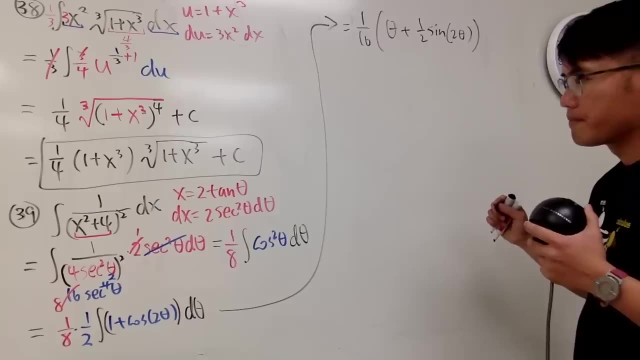 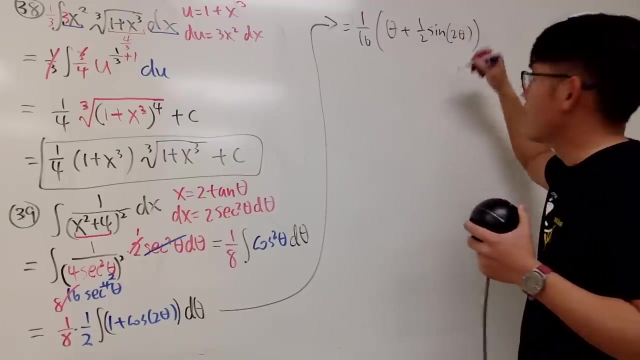 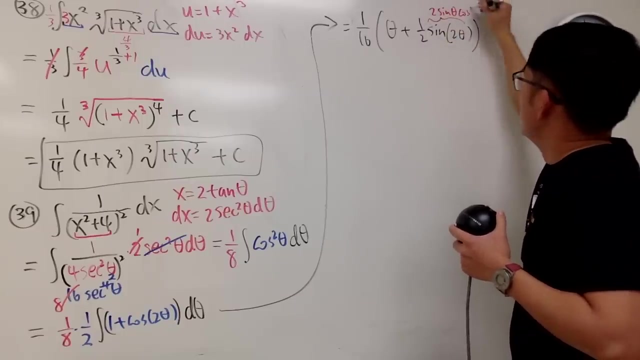 So that's what we have, Yeah, And then we have to go back to the x world Before we do so. this right here is double angle, So I will look at this as let's do this. This is 2 sine theta, cosine theta. 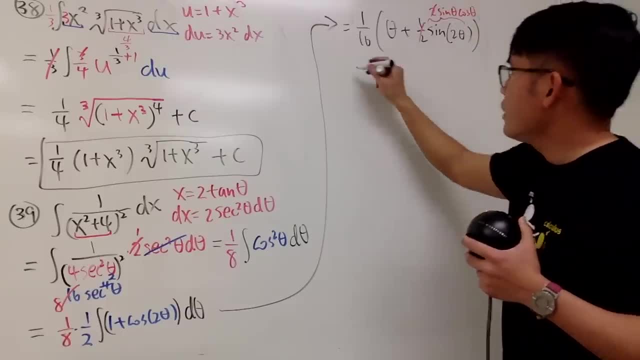 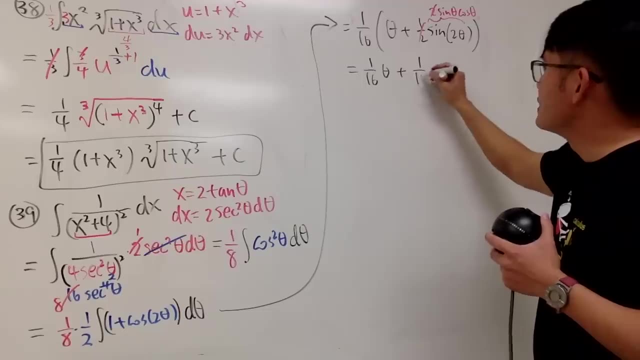 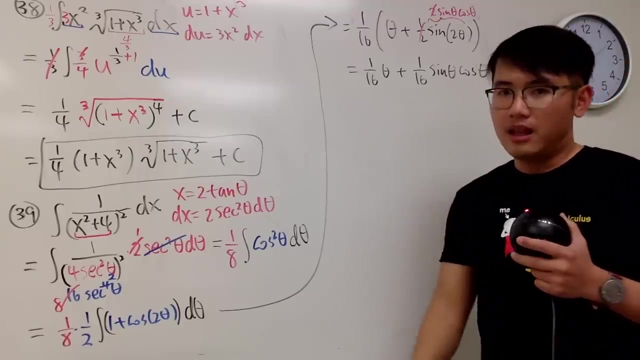 And of course, this 2 and that 2 will be canceled. That's nice. So this is now 1 over 16 times theta, And this times that is plus 1 over 16. sine theta, cosine theta. How can we go back to the x world? 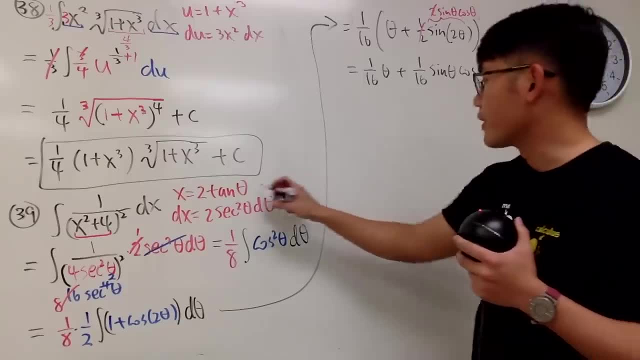 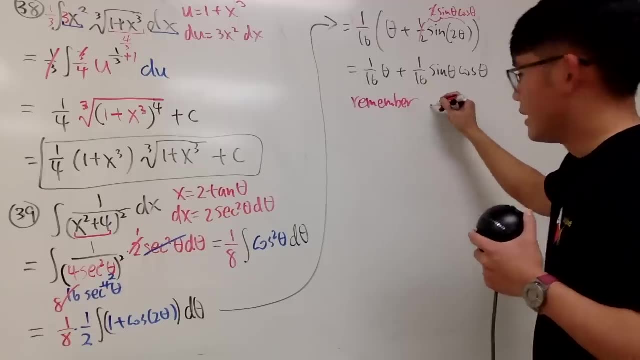 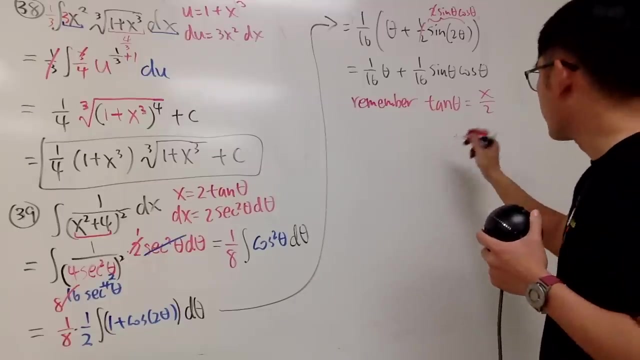 Use that. So you know, from here I'll just say remember, I'll just put down the number. seriously, Remember Tangent theta. This right here is x over 2, because we can divide 2 on both sides. So from here, 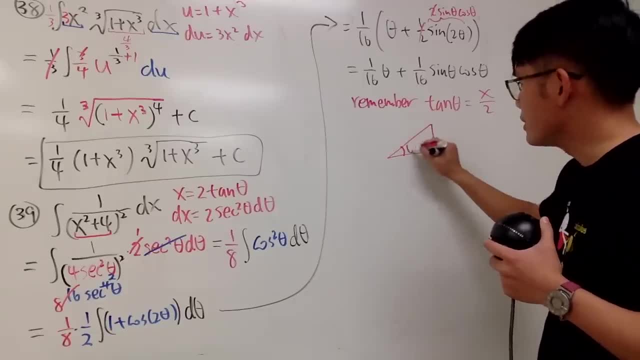 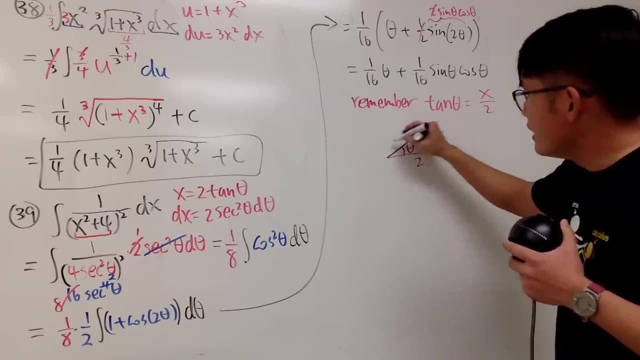 I will just draw my right triangle. This is my right angle, Here is my angle. theta Tangent is opposite, over adjacent, And we also have to figure out the hypotenuse which is right here. And that's just the square root of. 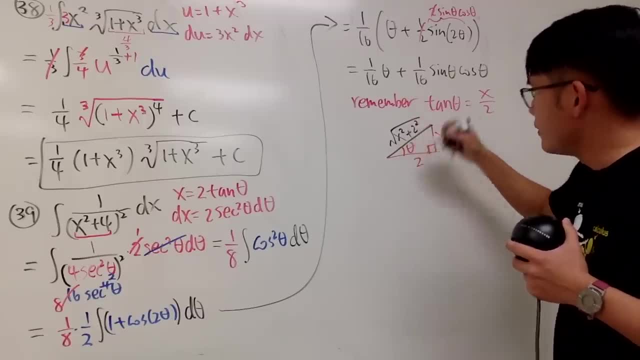 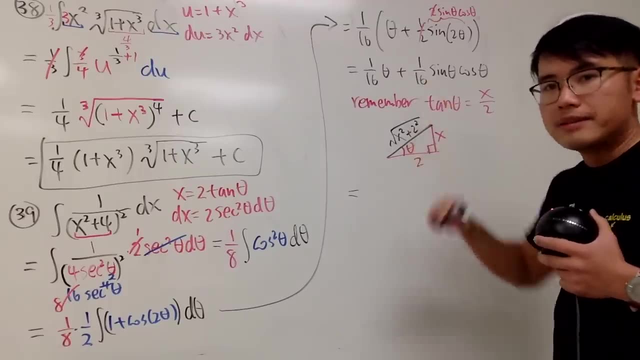 x squared, plus this square, which is going to be 4, but let me put down 2 squared first. Now we are talking. First of all I need the theta by itself, So let me just take the inverse tangent on both sides. 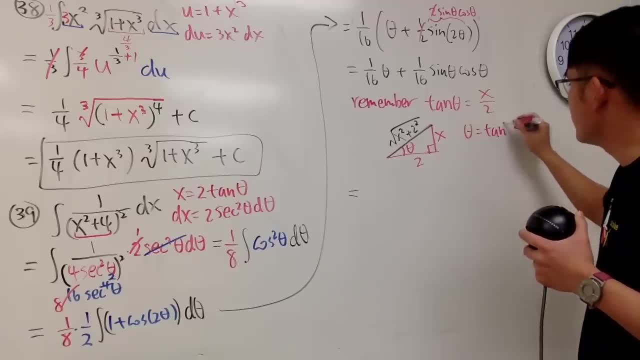 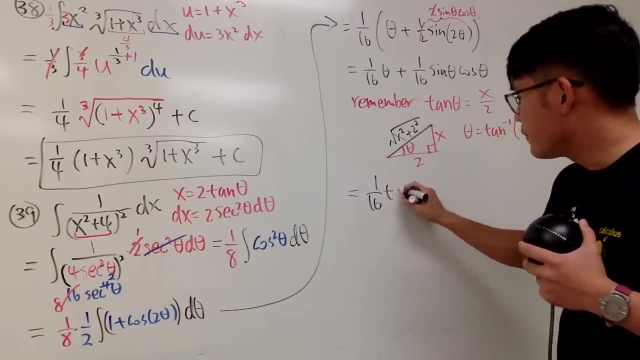 Therefore, you see that theta is just the inverse tangent of x over 2.. I need to put down this for that. So we have 1 over 16.. Inverse tangent. Let me just write it down in real, Why not? 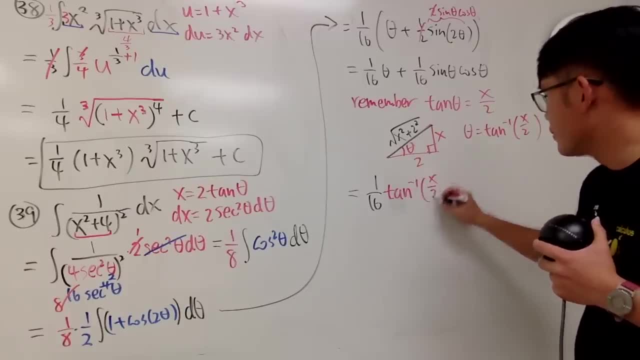 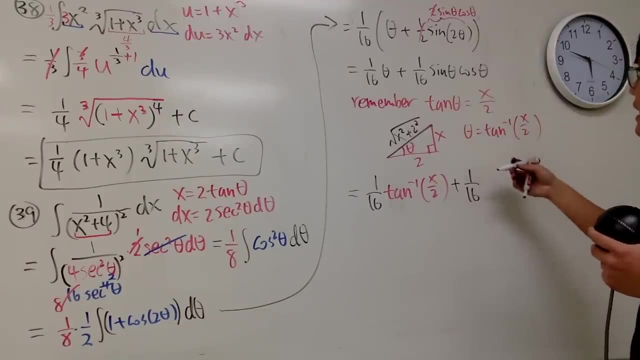 Inverse tangent of x over 2.. And then, right there, we have plus 1 over 16, sine theta. is this over that? And we are all adults? now You don't really have to worry about the square root in the denominator, okay. 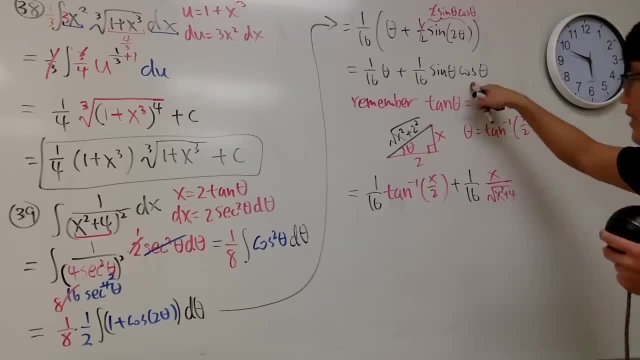 So x squared plus 4 and cosine theta is this over that. So we have 2 over square root of x squared plus 4, like this In the end: cancel things out: This, this is 8.. This, this, the square root, is gone. 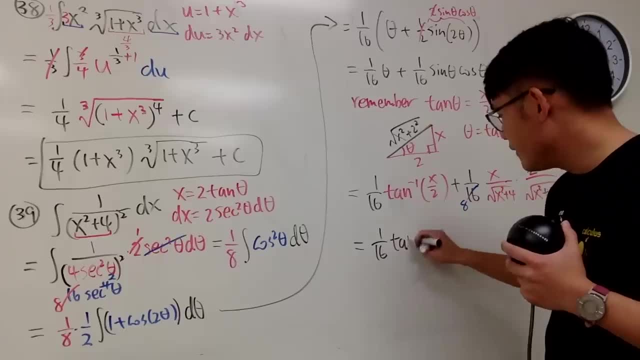 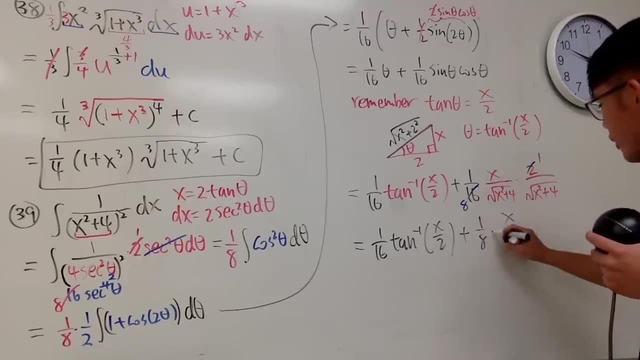 So final answer is: 1 over 16, inverse tangent of x over 2. And then you have plus 1 over 8. And then you have x on top over just this right. And perhaps I'll put down: 1 times x is just x. 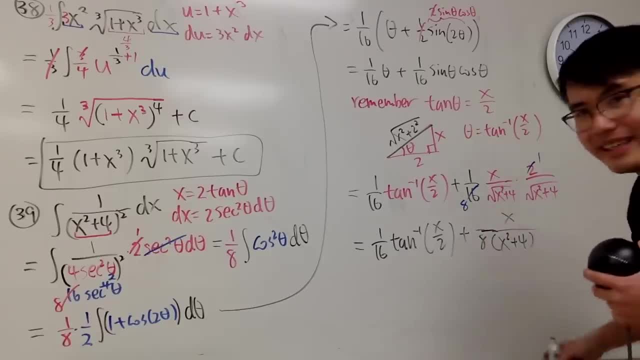 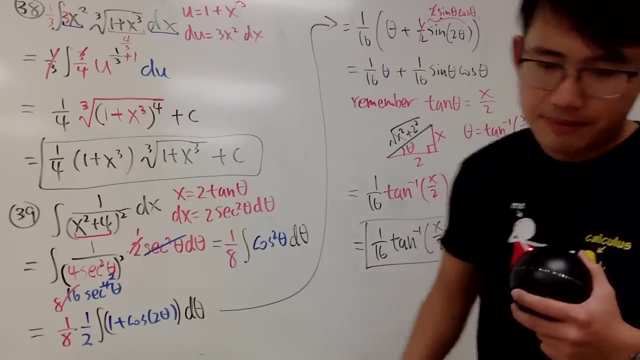 And then parentheses, x squared plus 4.. Like this We're done. Put a plus c. So this, right, here is the answer. Good, All right, Next one. Okay, So let me tell you guys that from question number 40. 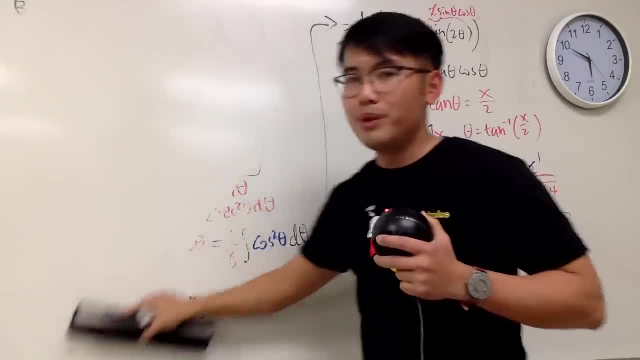 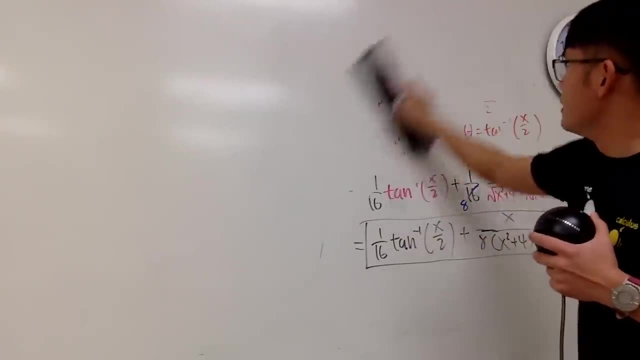 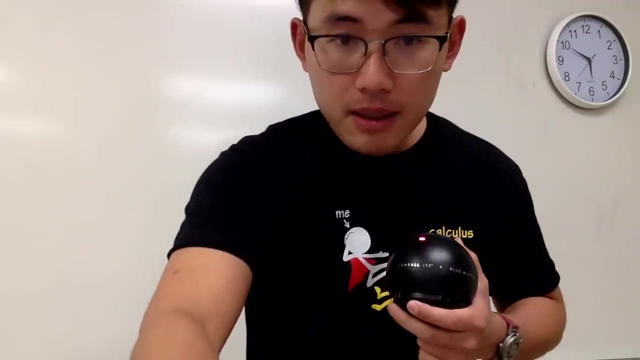 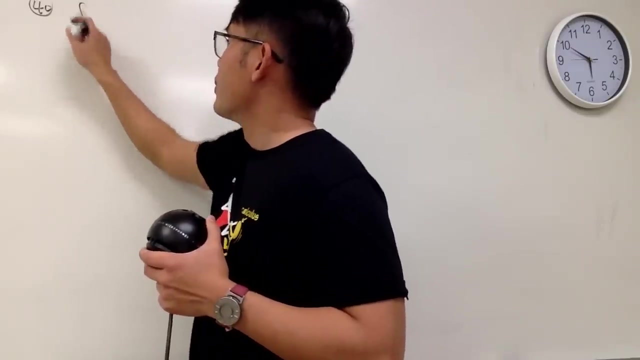 to question number 49,. we will be doing the hyperbolic trig functions, So if you haven't covered that yet, you can skip to question 50.. All that, Okay, All right. Number 40 here: Integral of well, integral from 1 to 2.. 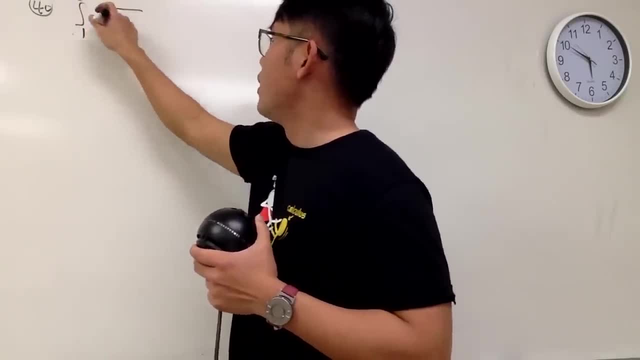 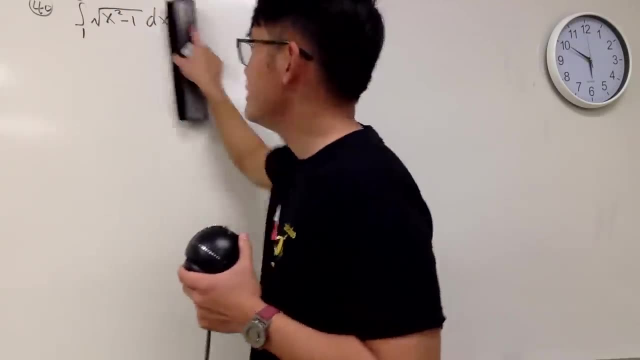 Okay, Integral from 1 to 2.. Square root of x squared minus 1 dx. And the truth is, you guys cannot see the 2, so let me write it down better. Let me write it down here: Number 40.. 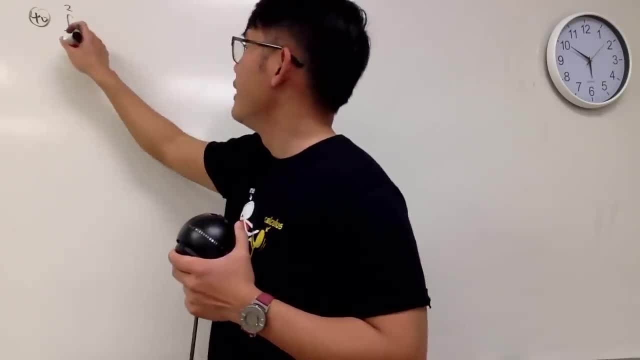 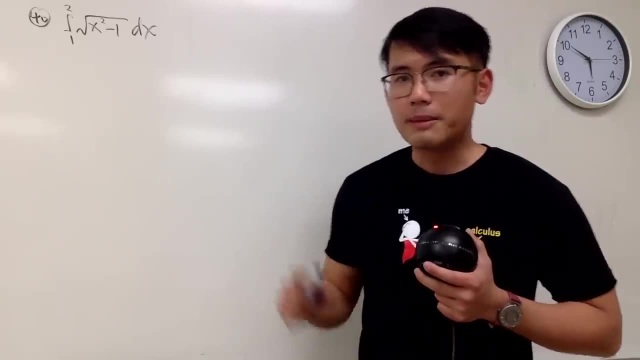 Integral from 1 to 2.. Okay, And then square root of x squared minus 1 dx. The truth is, you guys can also do trig sub for this. but where's the fun if you just do trig sub all the time, right? 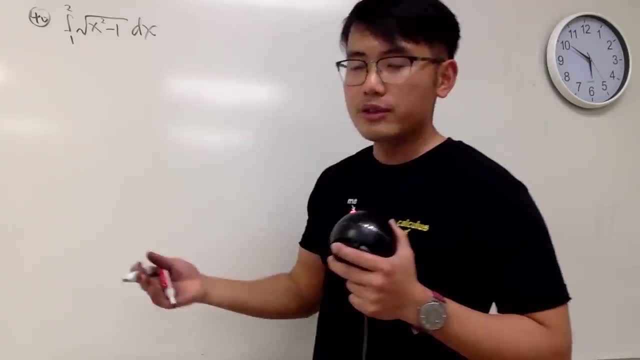 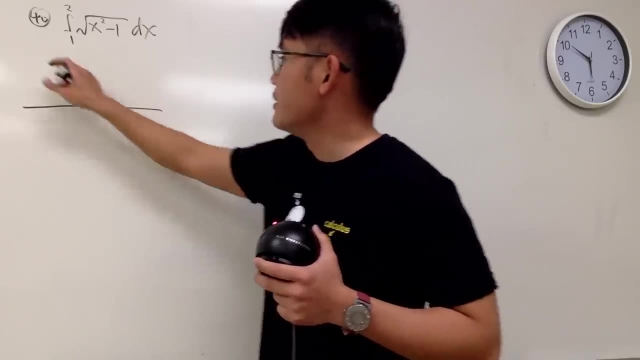 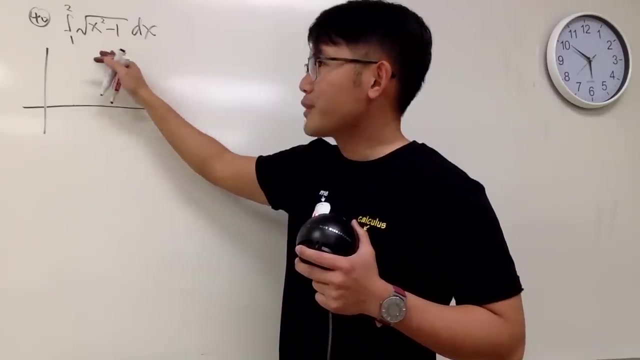 So here's the deal. Consider the graph right here, which is just going to be a hyperbola. Yeah, So we'll look at the right-hand side. Okay, So here's the deal. So you pretty much have x squared. 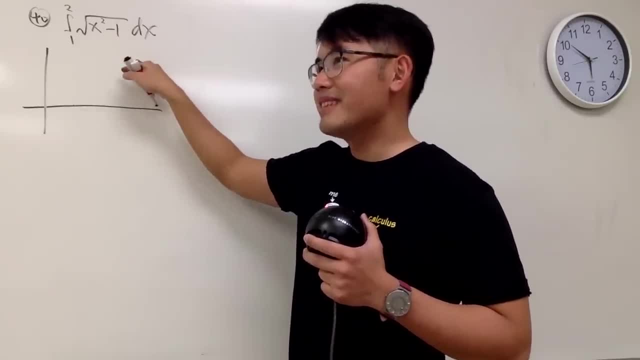 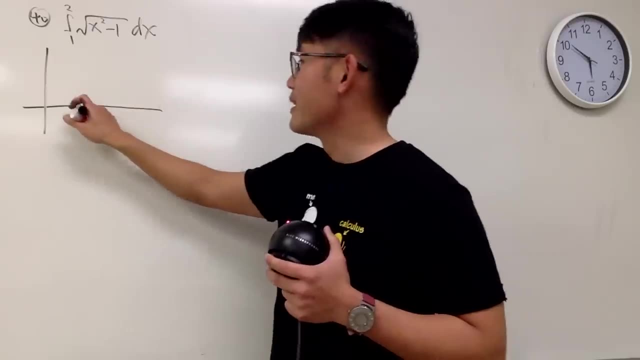 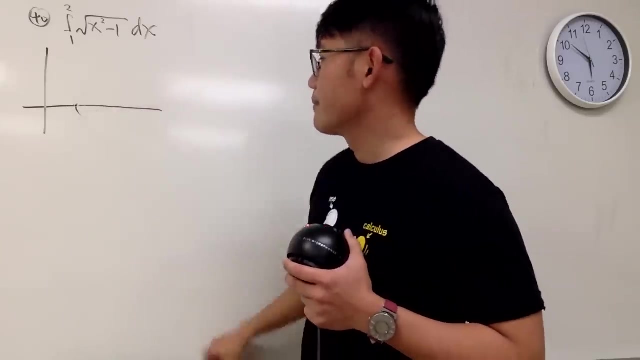 sorry, you pretty much have y squared minus x squared. sorry, sorry, sorry. You pretty much have x squared minus y squared is equal to 1.. And then you get like a sideways hyperbola like this: Okay, So it's more like this: 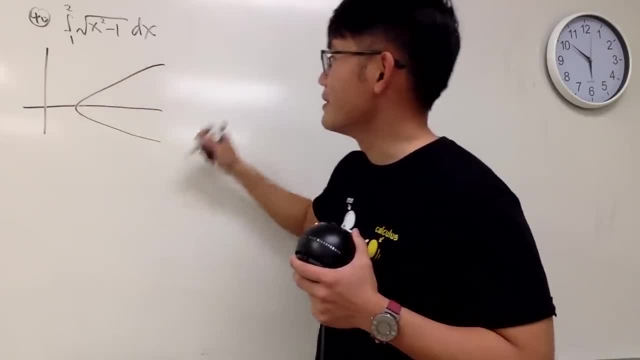 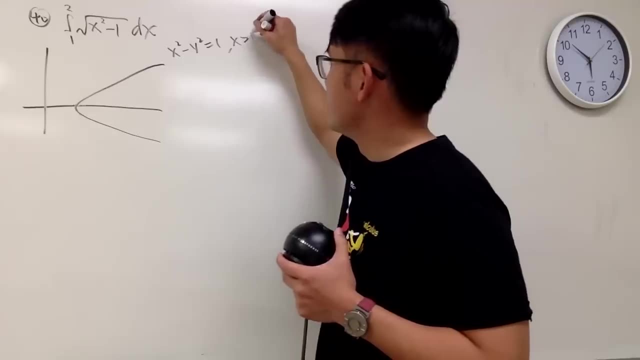 I know I should have just done trig sub also, but like you know, this is the fun part Again, x squared minus y squared equals 1.. And you want x to be greater than 0, in our case, greater than or equal to 1.. 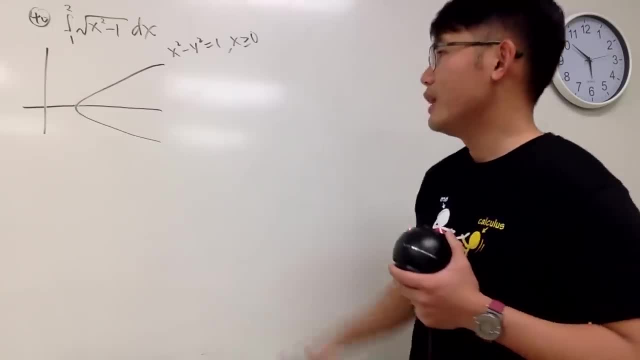 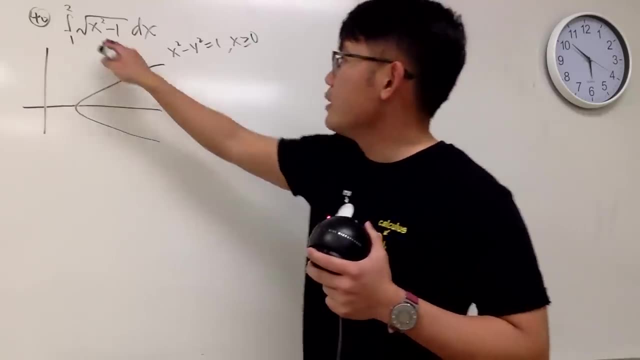 It's just this part, All right. So you have this portion of the hyperbola And remember, when you are doing the definite integral, you're trying to find the area under the curve And technically, when you have the square root, 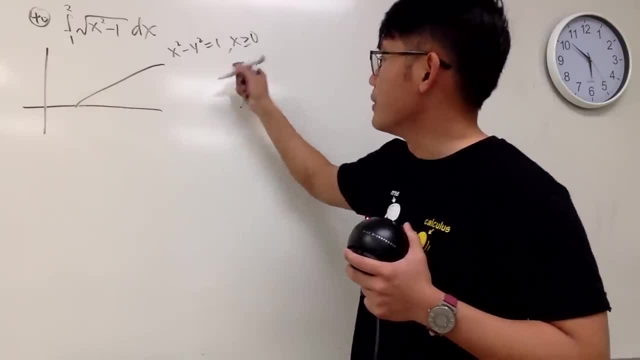 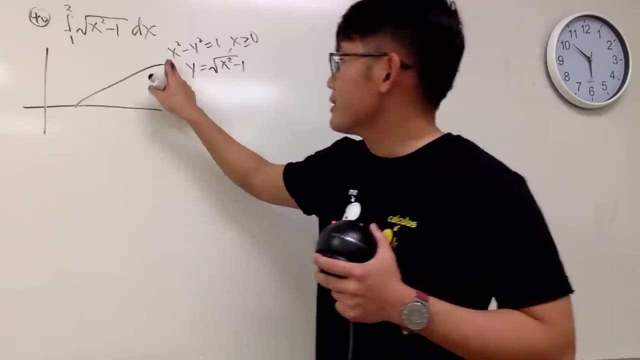 you just focus on the top So you don't really need to worry about the bottom. So this right here is the y equals square root of x squared minus 1.. Right, Looks like. let me do it again. Let me do it again. 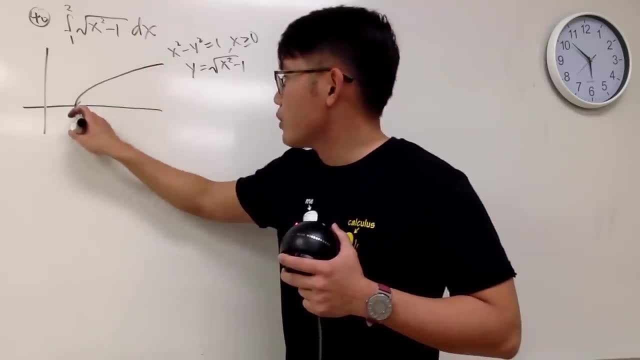 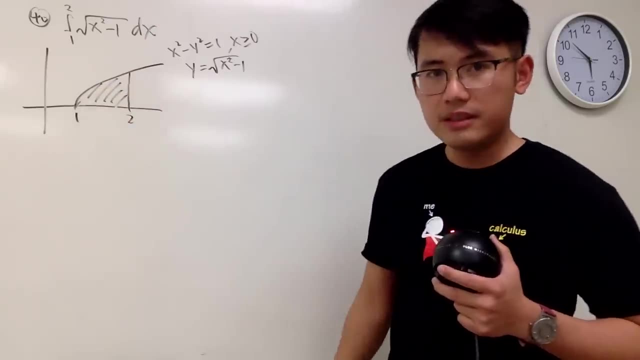 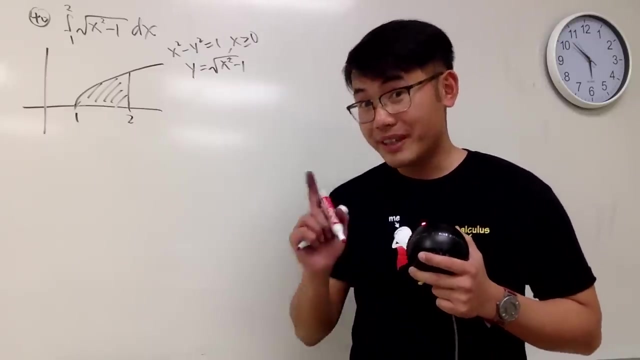 Right, Here we go. Much better Continue Going from 1 to 2.. This is the area that we want. This is the area that we want. Where's the geometry that we can do Here? hyperbolic trig functions. 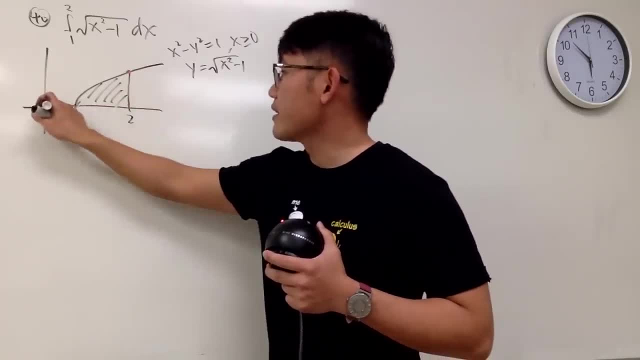 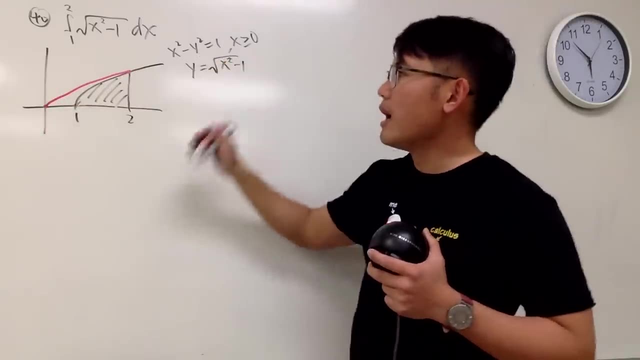 Here is the deal From 1 to 2,. well, I can connect the dots from here to here, And the idea is that when you have a point on this hyperbola, this point right here is denoted by, of course, 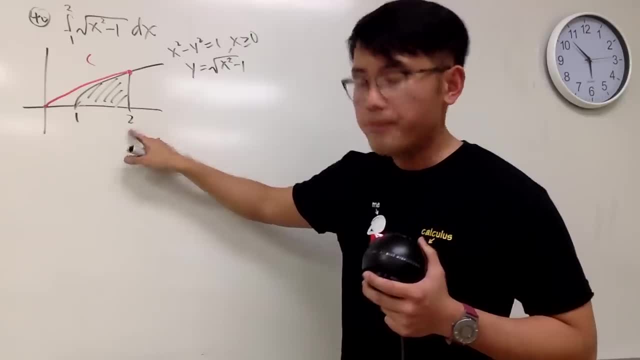 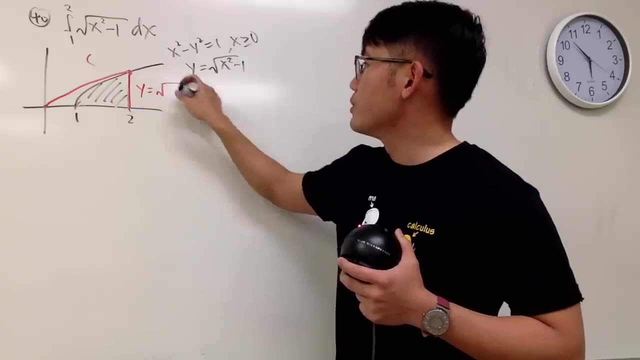 you have two ways to do it. You have the x value, which is 2.. And you also can just plug into here, so you know the y value here is: y is equal to square root of 2 squared minus 1, which is square root of 3.. 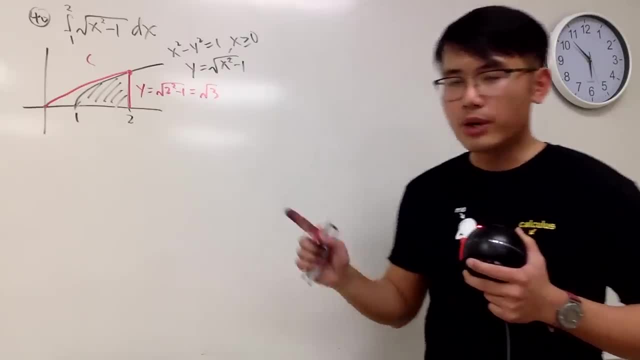 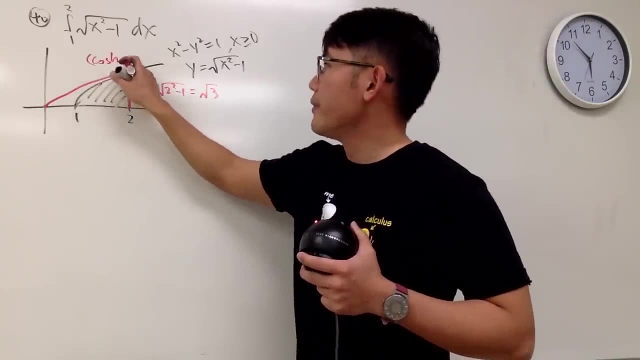 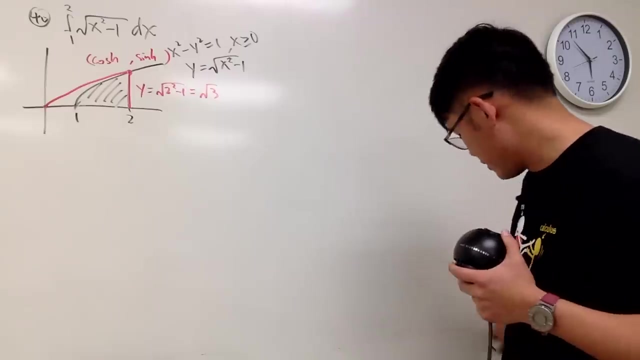 Like that, No big deal. But this right here it's also going to be the following: You can also look at this as the cosh and cinch of something Right Cosh and cinch of something I'm going to put in my blue marker. 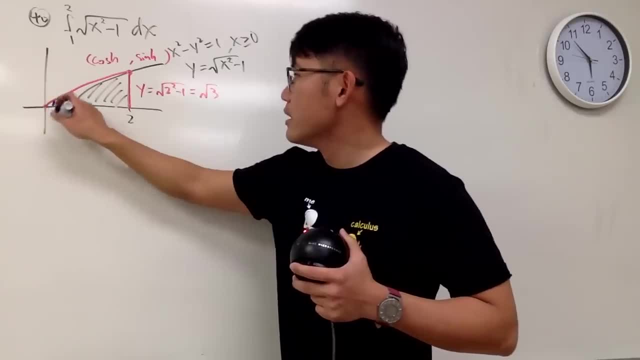 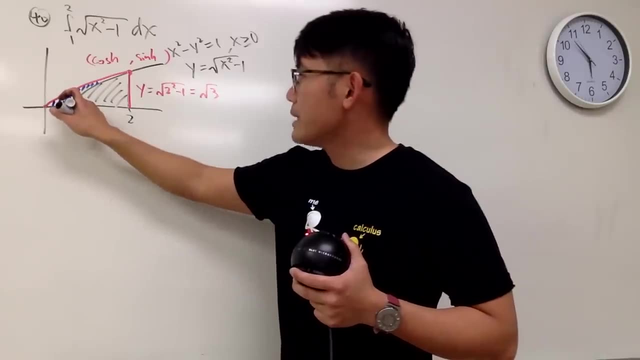 That input is in fact twice as much as that area in blue. So if you don't know what this area is, perhaps I'll just put down T for it. Right, I'll just put down T for it for this. Put down T for it. 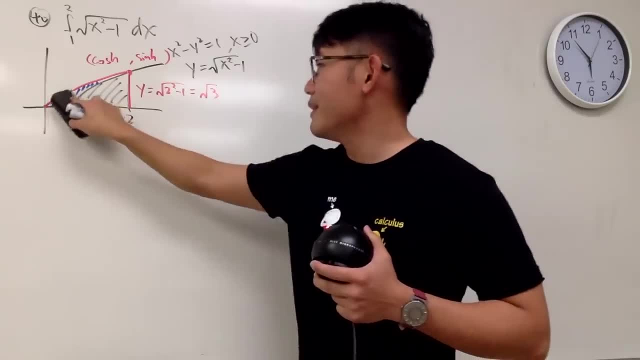 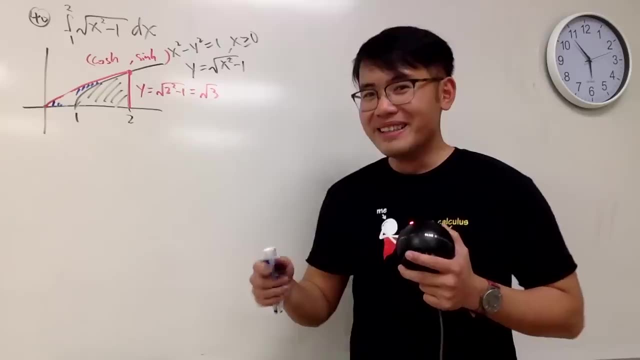 But technically I feel like this reminds me of the Dr, Not Dr. Yeah, this reminds me of the Dr Bing movie, when he was trying to fix the paint and then he made it worse. Anyway, T over 2.. 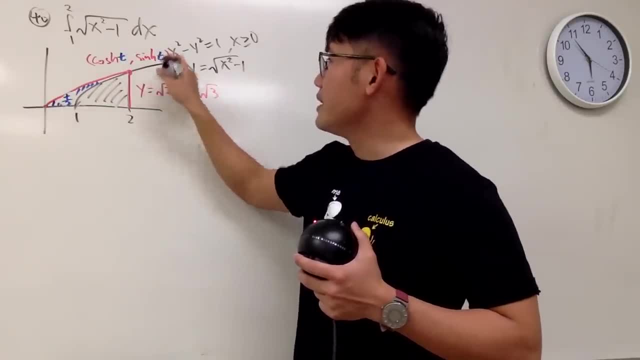 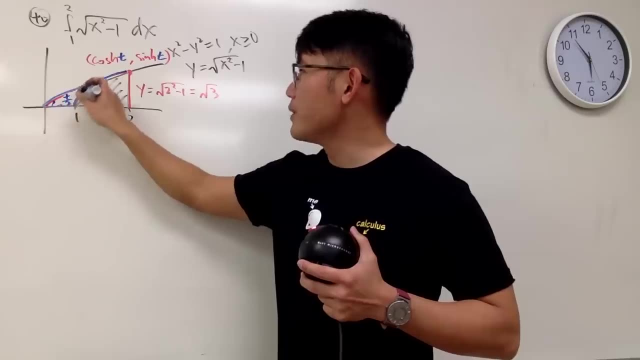 Okay, So that the input will be T and T. If you know this part right here, if you know this area here, and we call that to be T over 2. Okay, Then the input right here is twice as big as that. 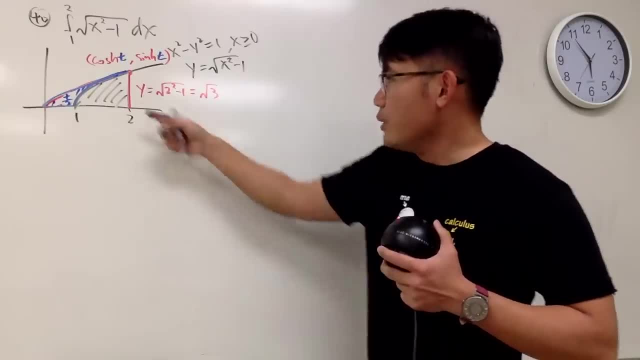 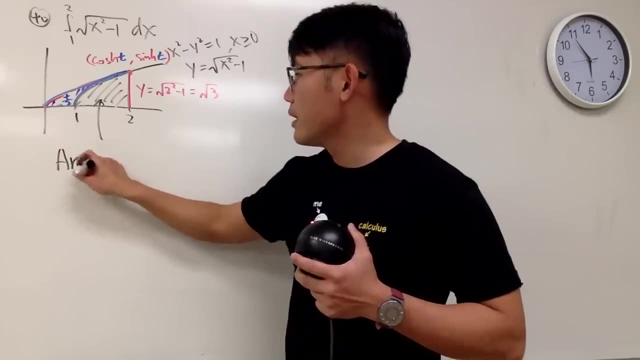 It's twice as much as that, Right? So that's the idea. So how can we find out this area, though? Here's the deal. Let me just show you. This area is going to be the following: Okay, Take a look. 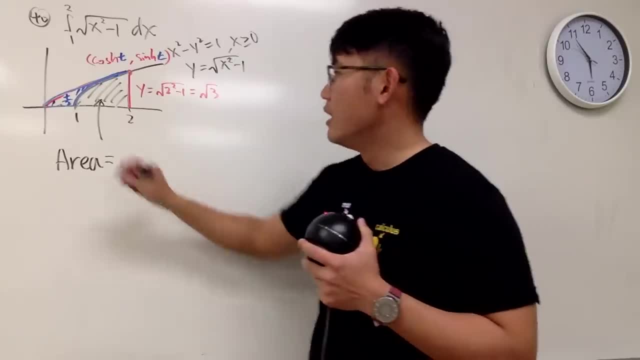 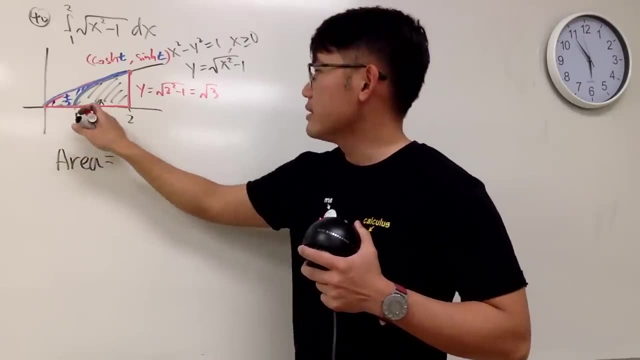 We have a what We have? a triangle first, On the outside, from here to here. of course this is going to be a triangle, So it's just going to be. this length is 2, altogether Right, This length is 2.. 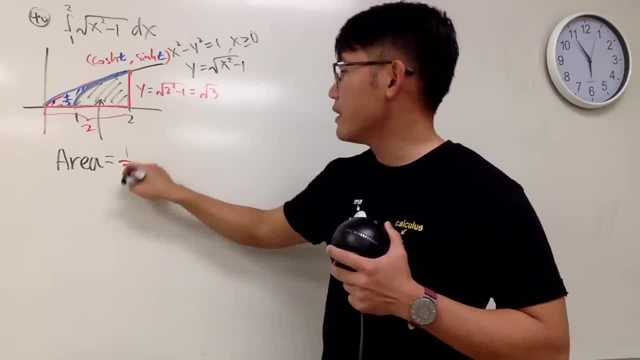 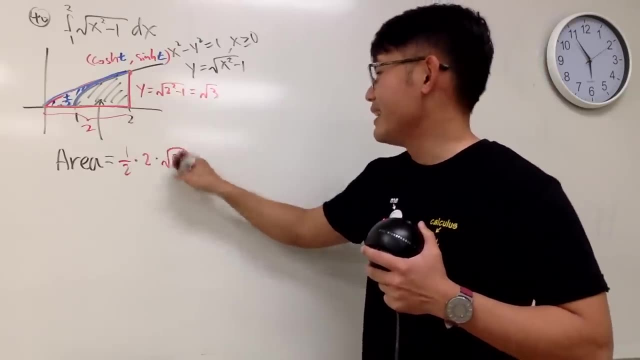 So the area of the triangle is 1 half times, 2 times the height, which is the y-value that we got earlier, which is just square root of 3. And that's very nice. Now we have to just minus. 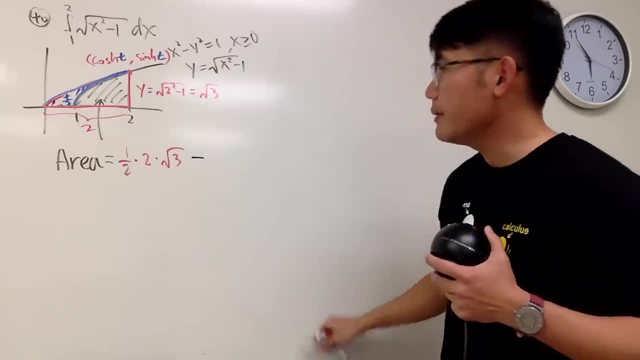 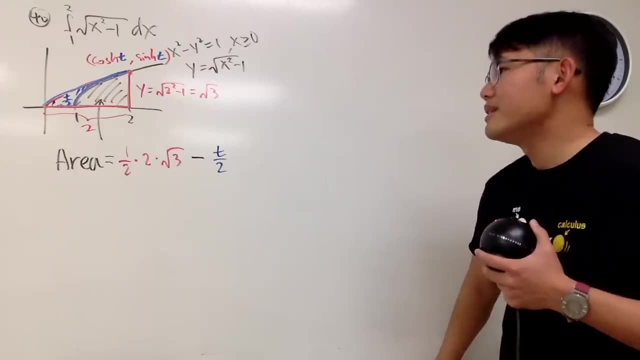 we just have to minus the T over 2.. Right, As I said this, right here is our area, right here, T over 2.. So, uh, what does this mean, though? T over 2?? Well, remember, this is the hyperbolic. 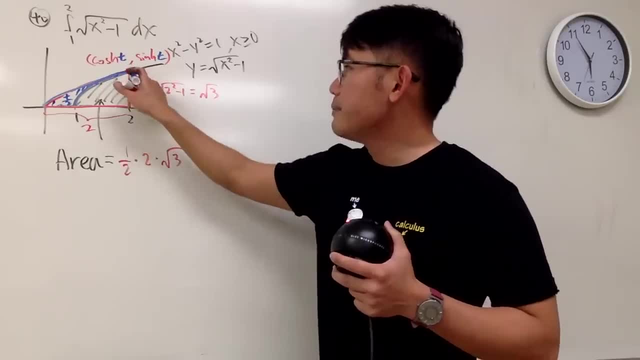 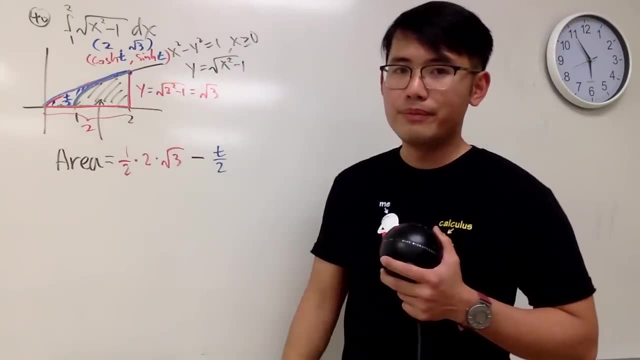 uh, trig functions Technically. this point right here is 2, comma, square root of 3. Isn't it, If you have the x comma y form? So what does this mean? You can say that. 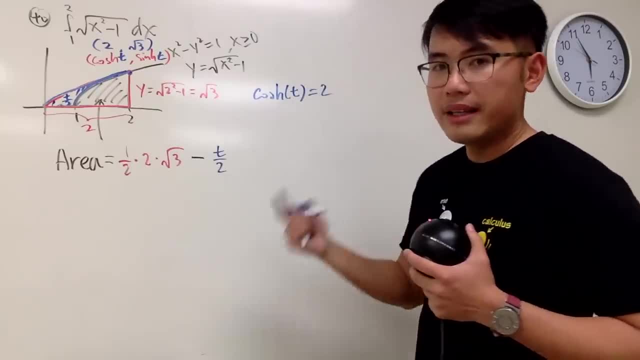 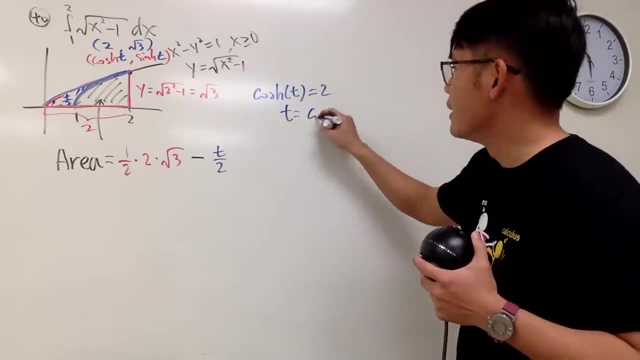 cosh T is equal to 2.. And in another word, you can just take the inverse cosh on both sides, So T is equal to the inverse hyperbolic cosine of 2.. Just like that, Very nice. 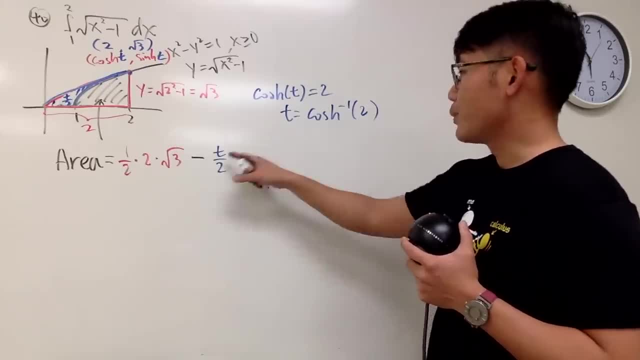 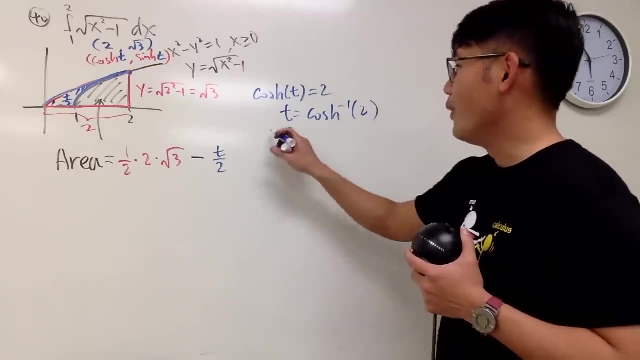 But don't forget, but we have the T over 2 already, so you can just put this right here for the T and you're done. Seriously, that's it. So that's one way to do it. 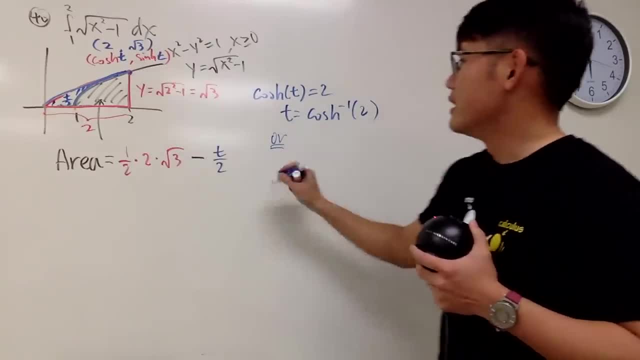 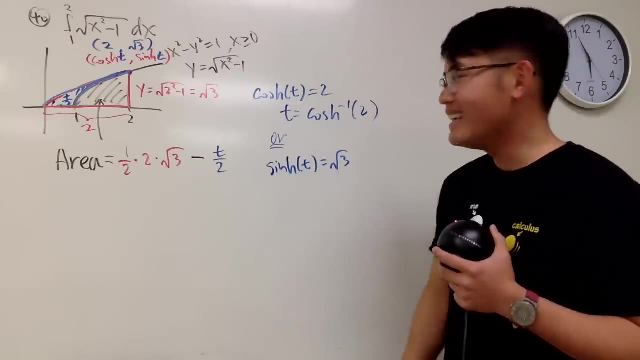 Or I will tell you You can also do this. You can also set sinh right sinh of T to be square root of 3.. And take the inverse sinh on both sides, So T is the inverse. 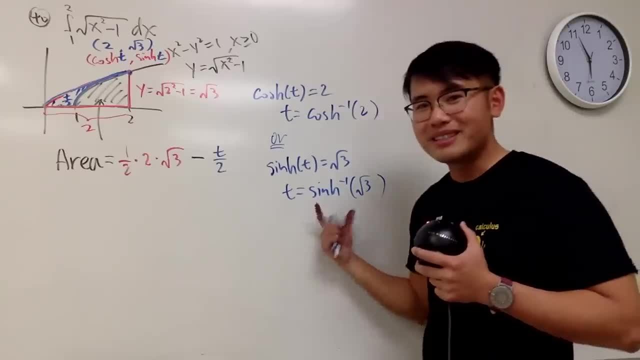 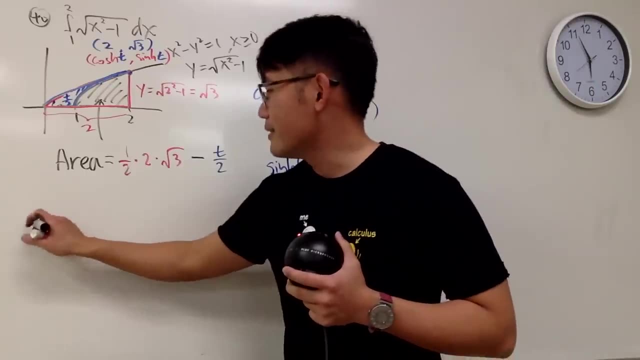 hyperbolic sinh or the inverse sinh. You can also put this right here for the T and you're done. So it depends on how you want to do it. So I'll just tell you guys the answer. 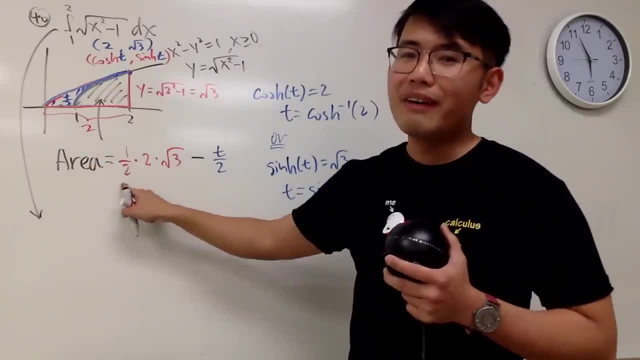 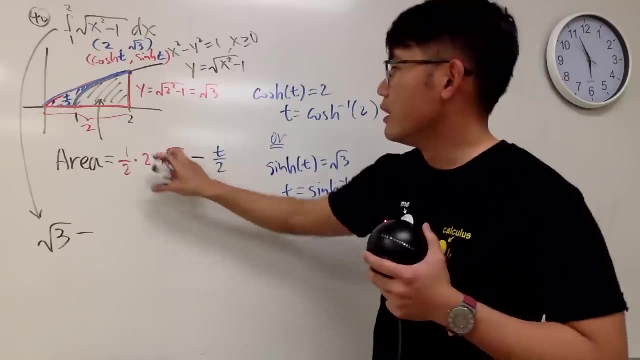 okay, The answer to this integral is through the arrow, Of course. 1 half times 2, is just 1, and then you have the square root of 3.. Minus because you have to have the whole area. 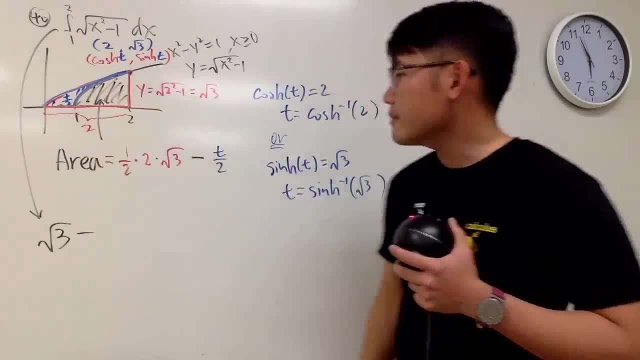 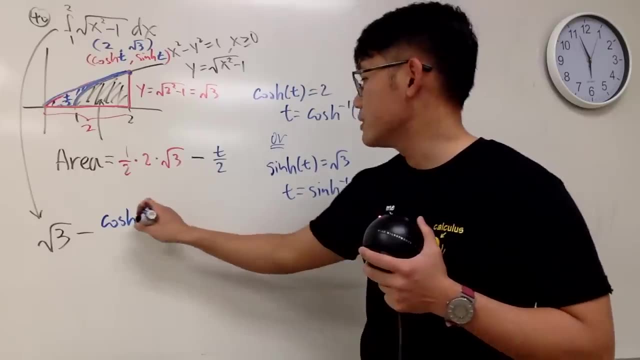 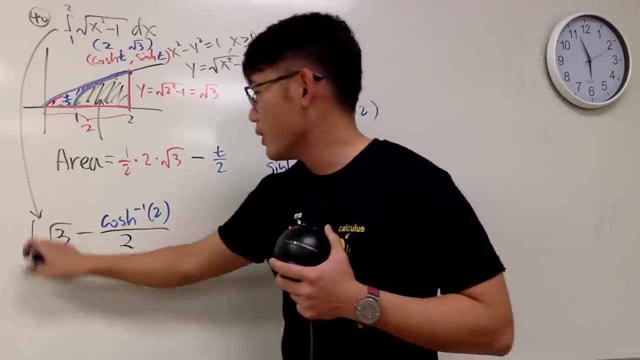 minus the blue area. to get the remaining area here, you can put down this right here: cosh inverse of 2, and then you divide it by 2.. So this is an answer and if you would like, 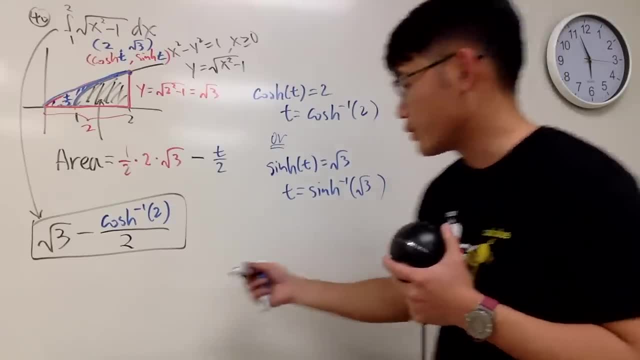 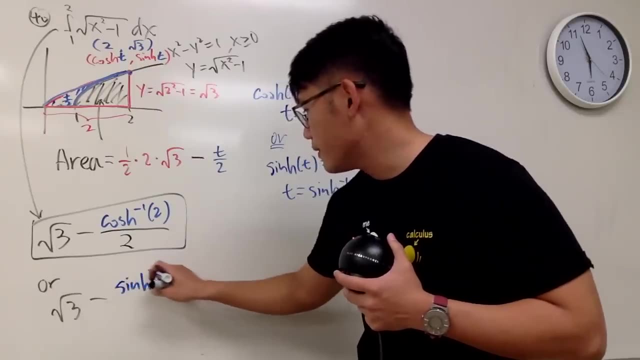 you can also use this, So I'll write this down right here real quick. Or square root of 3, minus sinh of was inverse sinh of square root of 3, minus 2.. 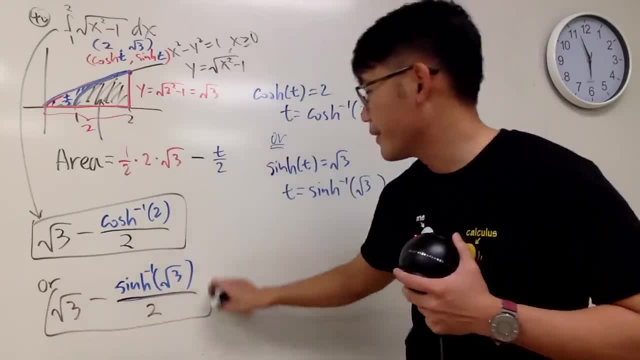 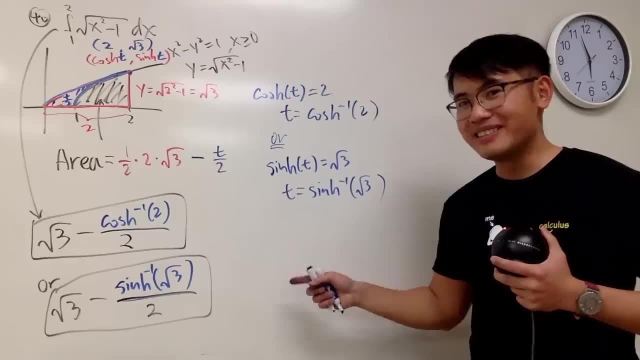 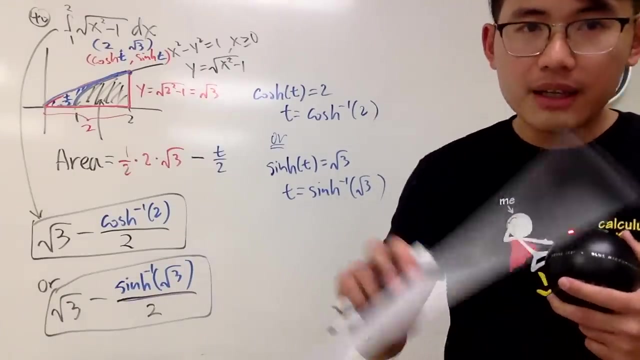 Like that, And do I need to put down plus c? If you are still watching, go ahead like answer that and also leave a timestamp. Yeah, that's it. I think that's really cool, Right? So welcome to the. 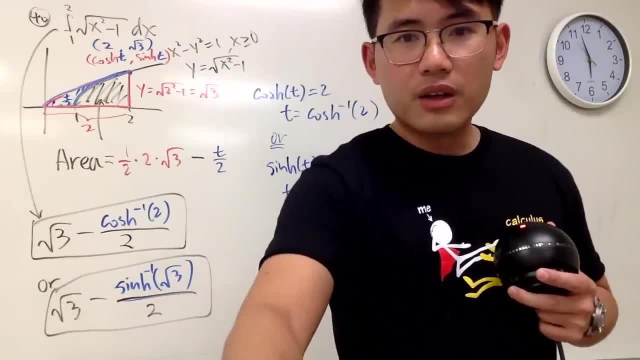 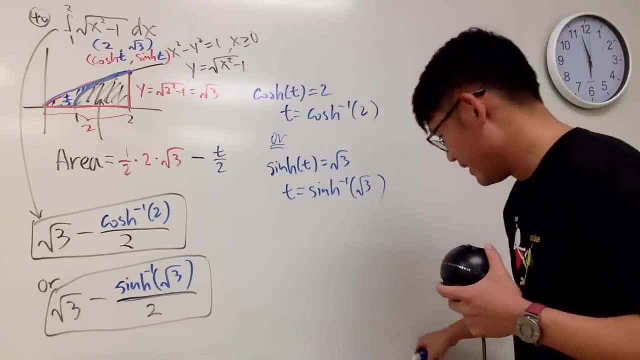 hyperbolic trig function section. Alright, one sheet done, 40 questions. 40 questions Next one. I think I'm going to change marker because this right here is kind of like drying out, okay, So 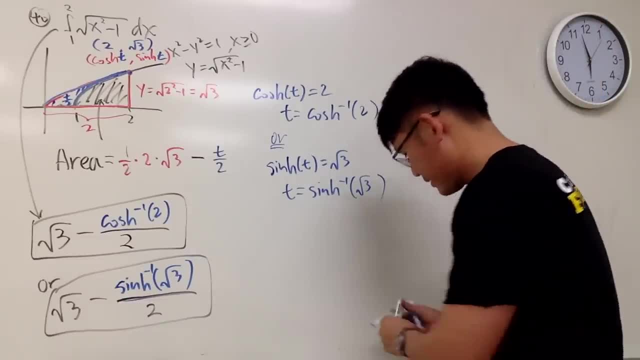 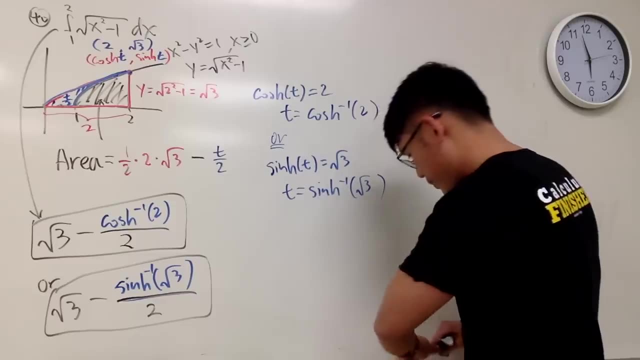 I'm going to change marker. So one marker down, and I'm going to take out my red markers just in case later on. So put this back, hold that, Okay. So I'm going to. 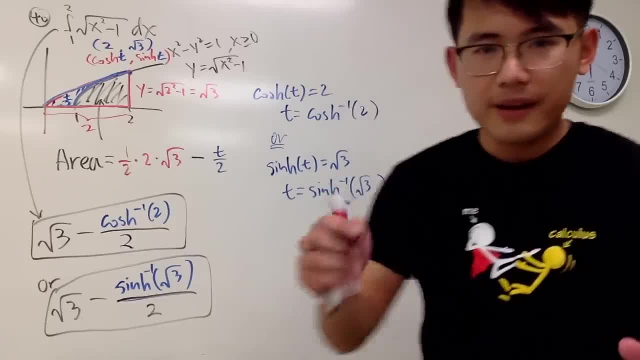 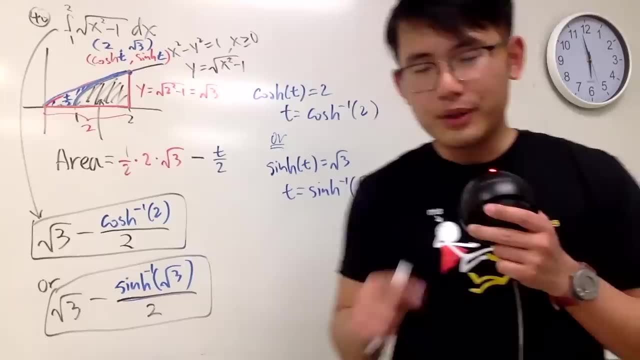 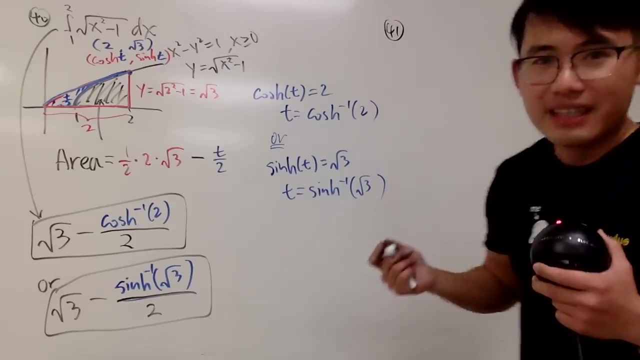 take out my red markers, just in case later on. So put this back. hold that, Okay. Oh, Are you guys still watching? Hopefully, Alright, So now 41. Much better, huh, 41,. 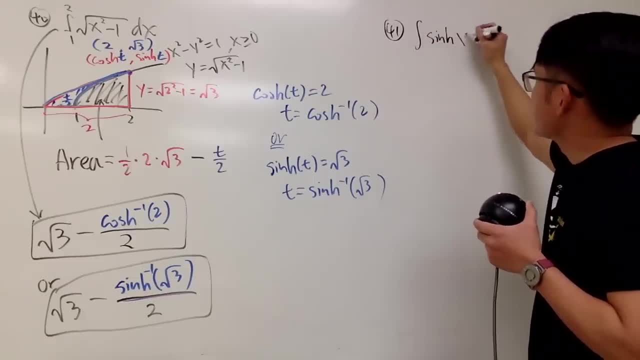 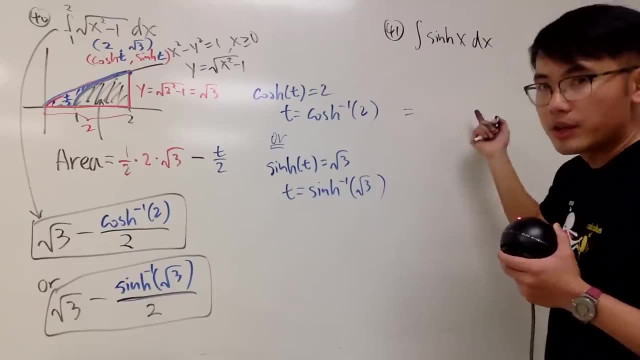 we just want to integrate sinh of x- dx. This right here can be really easy. If you use hyperbolic functions then they will tell you the integral of sinh is just cos of x plus c. 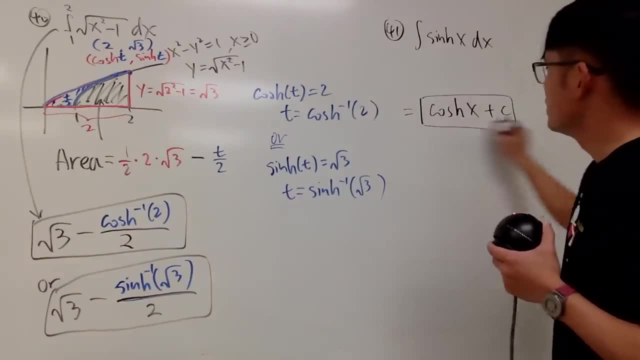 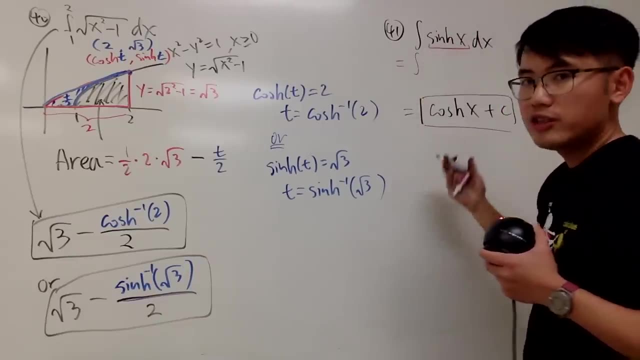 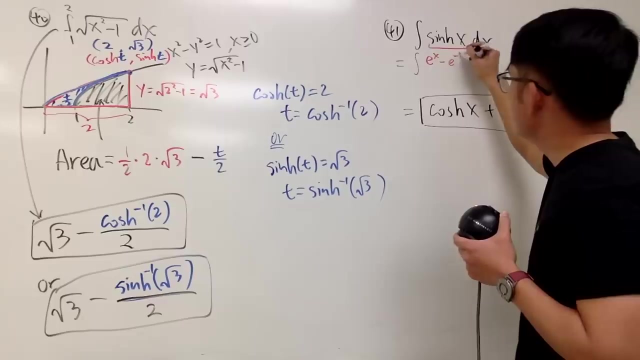 like that And that's it right, that's it. this is totally okay, and the idea is that, if you look at things right here, the idea is that you can also change that to the exponential form, which is e to the X, and this one is minus e to the negative X all over 2 and 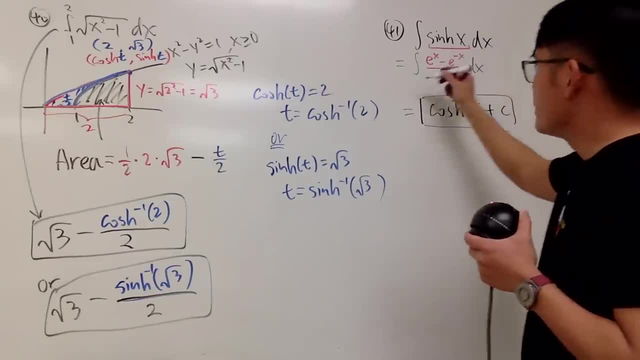 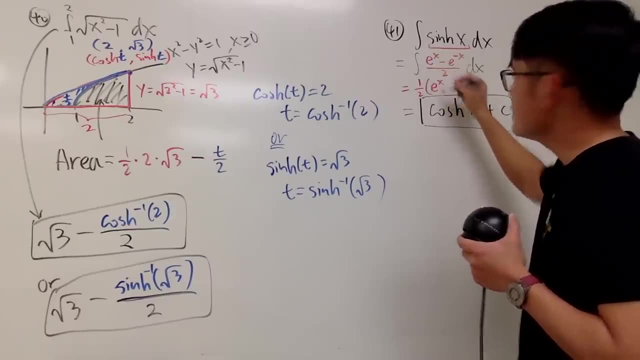 then you have the DX right here and now. if you integrate this, you actually end up okay, the over 2, just always over 2, right? so then you have the integral of e to the X is e to the X, and then the integral negative e to the negative X is. 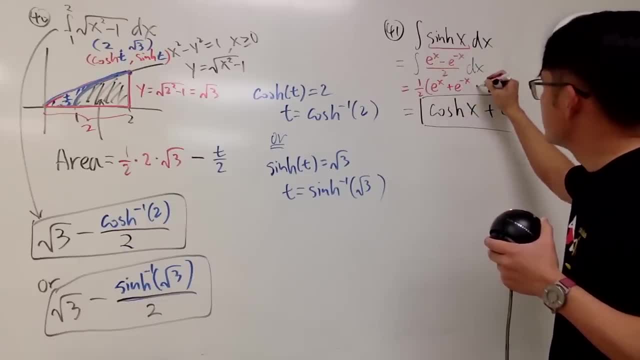 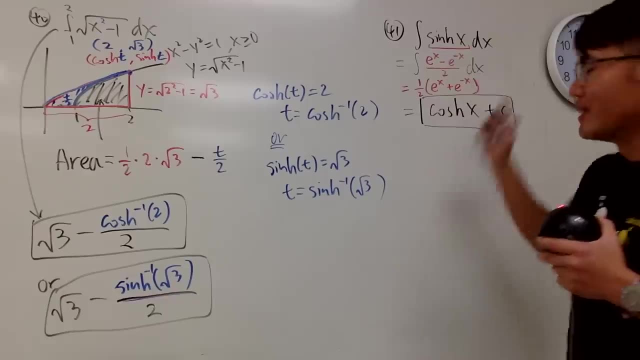 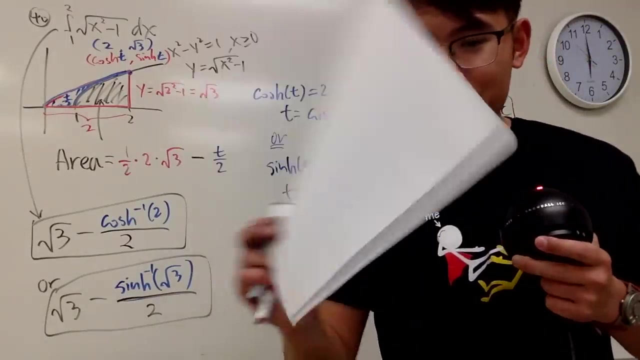 positive e to the negative X, like this, which is the same as cosh. and that's it, yeah, and that's it all right, number 42: yeah, I think she is, with minus in between and cautious in the plus in between. yeah, yeah, I'm just trying to do everything in. 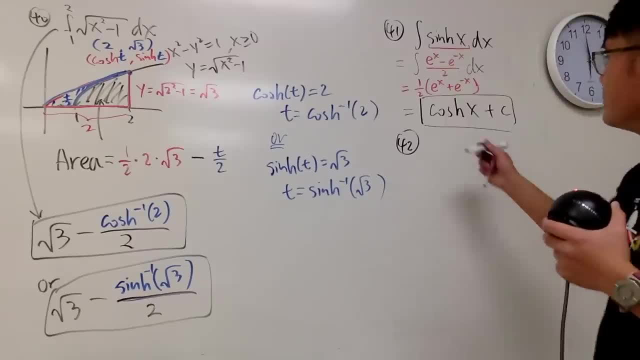 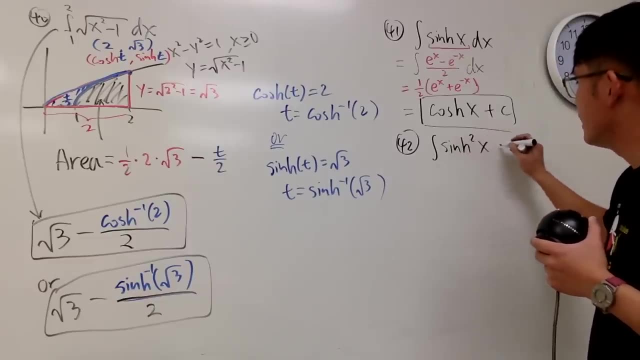 my head. okay, next one: we have the integral of sinh square X, DX, and remember how we do the integral of regular sine square. well, we also have a power reduction formula for this guy. so to do so, let me tell you the end. the identity is 1 half and 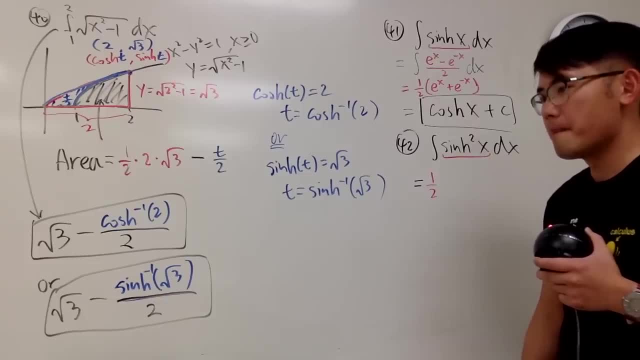 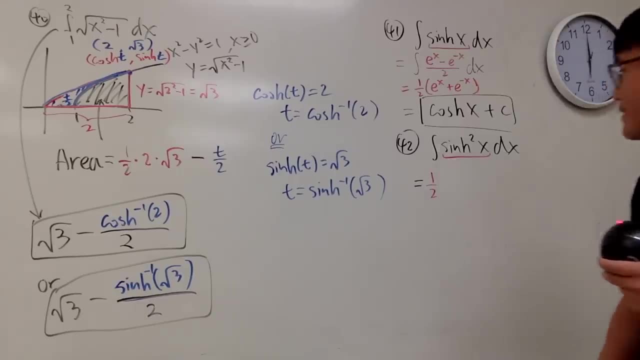 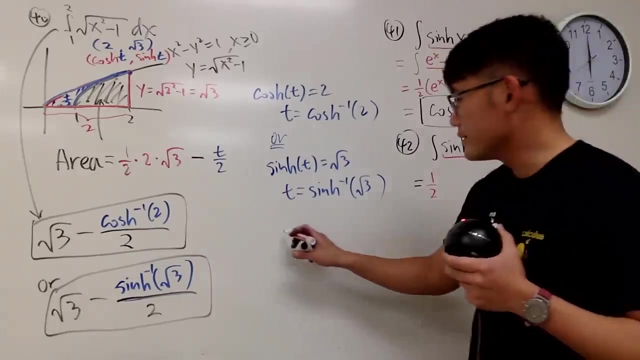 so to do so, let me tell you the end. the identity is 1 half and one, okay. so I will just prove this. ezokic ЯсY mallada erstmal. okay. so I will just prove this: ezokic ЯсY mallada. 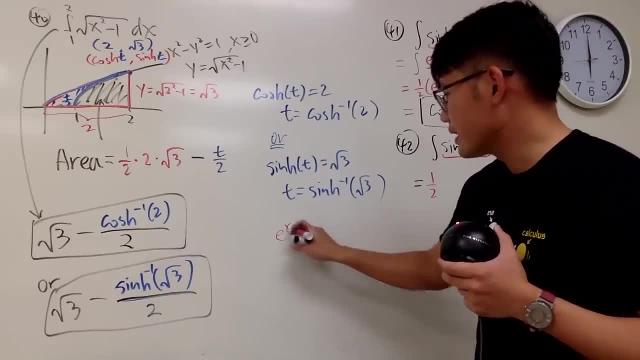 is like how this is. here is the deal. as I gro casually I would kinda forget about, like how does this? here is the deal. as I said, if you take things to be t to the X minus e to the negative, X over 2, right, and this time. I otro squer that, so let me just write: I grounded x over 2 and this time I have to square that, so let me just square that. so you get 1 over 4. so you get 1 over 4, which is 1 of a fall the window. 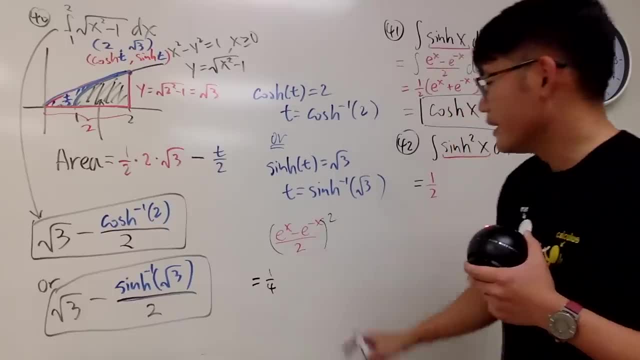 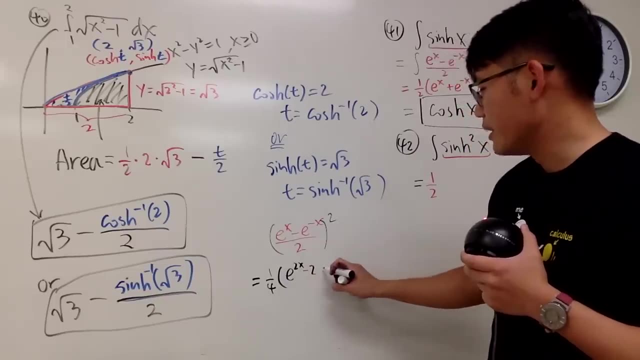 square x. so let me just square that so you get 1 over 4, which is 1 over 4 the window in the front. okay, And then you will have e to the 2x and then minus 2, because this time side is going to be 2 right here- and then minus e to the negative 2x, And I want 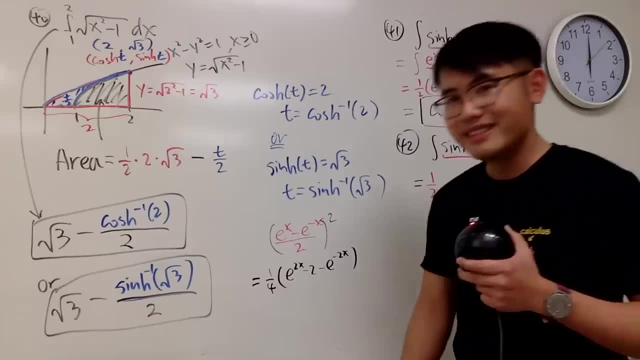 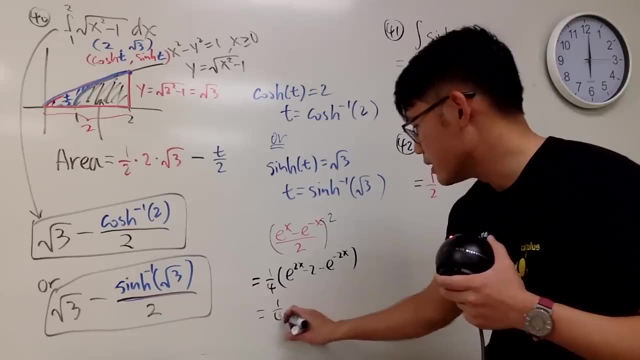 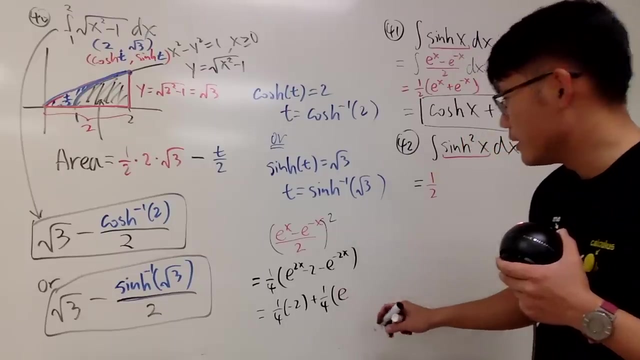 to somehow produce the cosh to help me out. This is how Well, first of all, you can look at this as 1 over 4, times negative 2, and then you combine this with 1 over 4 with this guy, which is e to the oh. by the way, this should be plus 2x, plus e to the negative. 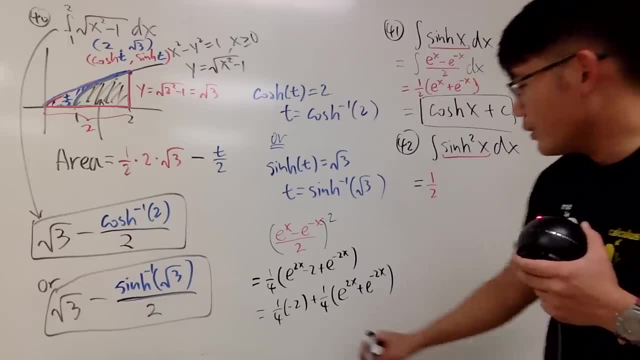 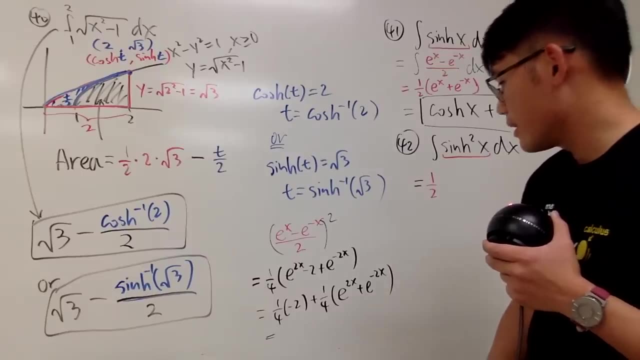 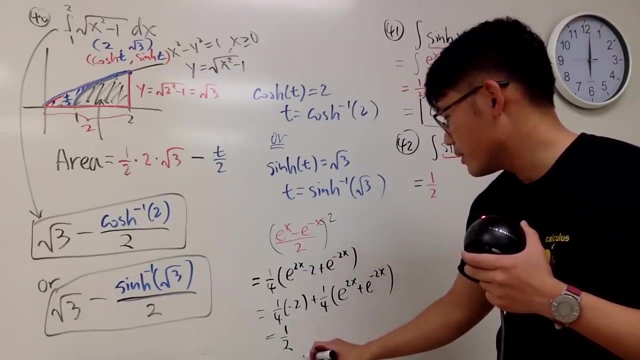 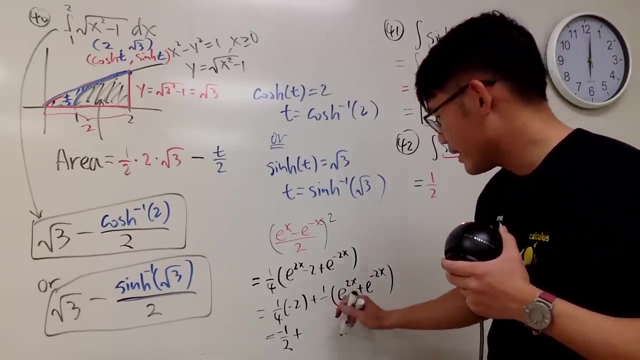 2x like that. So, as you can see, we have. what am I doing? Let's see 1 half all the way negative, 1 half, Yeah, And then plus this right here is a DO- Let's look at 1 over 4s 2 times 2, okay. 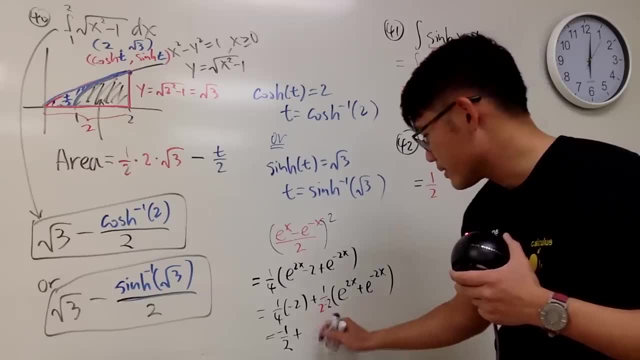 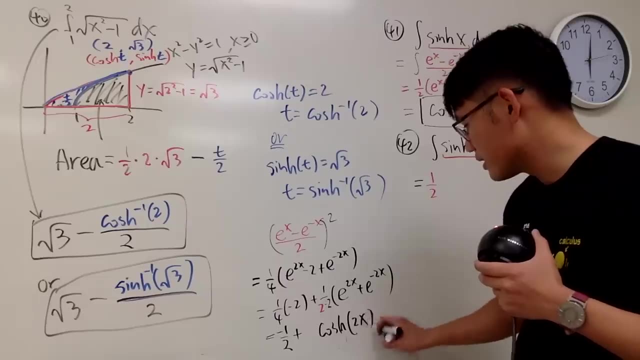 Because if you look at this part in black, you actually get this. okay, You actually get cosh with the input being 2x. That's very nice, isn't it Right? And then you still have the 1 over 2. So it's trickier, right. 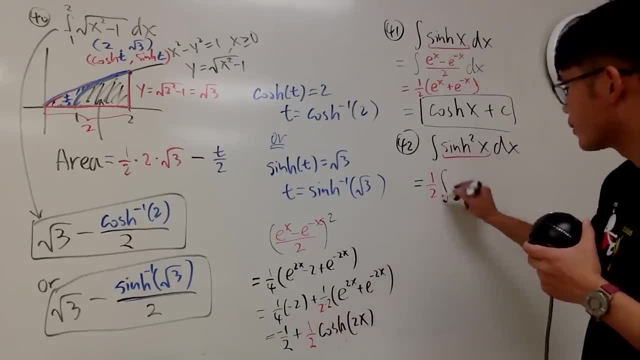 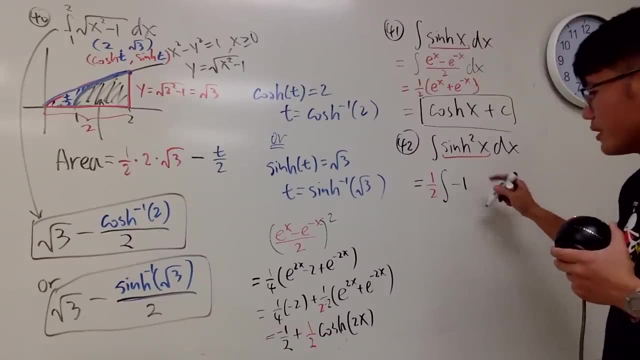 So I can factor the 1 half and then you have the integral and you start with negative 1,. okay, You start with negative 1.. So it's different than the regular sine situation And you add cosh of 2x like this: okay. So the idea is, if you forget about the identities, 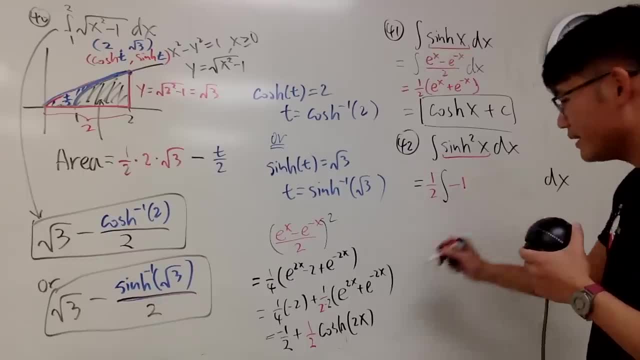 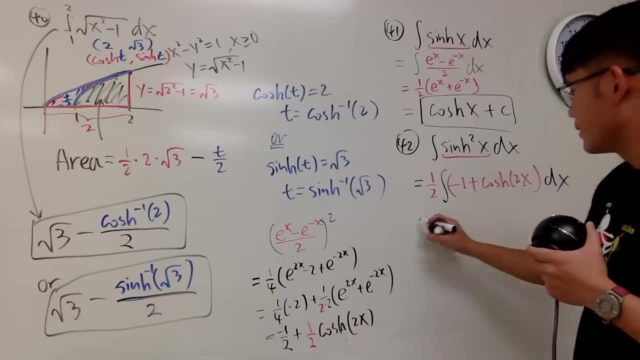 just go ahead and prove it real quick. So anyway, Negative 1. Plus cosh of 2x, like that. All right, enough talking, Here we go. Integrating this, we get 1,. well, 1 half in the front. 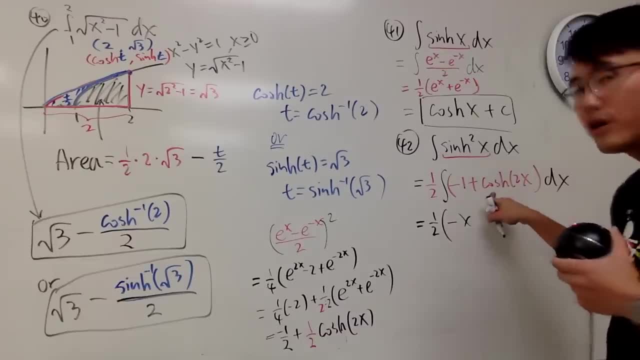 Integrating negative 1. in the x world we have negative x. Integrating cosh is so the same as just sinh Derivative. there's no negative, okay. So when you integrate cosh you get sinh and the input stays the same. but it's divided by 2, so you multiply by. 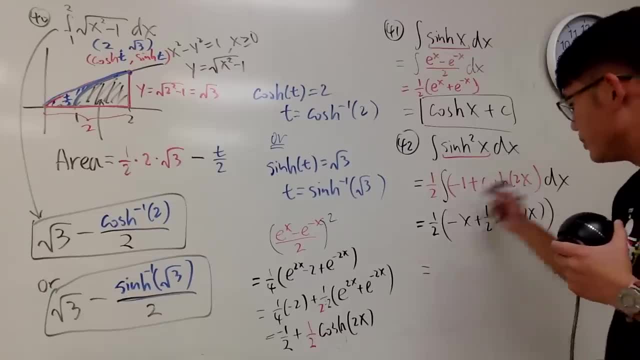 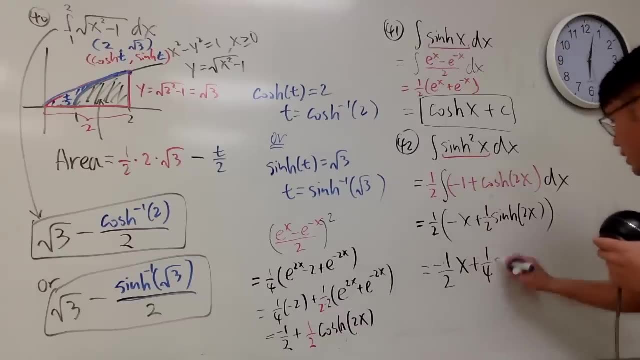 1 half, So you have a negative 1 plus. and then in the end you distribute the 1 half so you have negative 1 half. x this times Z is plus 1 over 4, sinh of 2x. and you've got done. 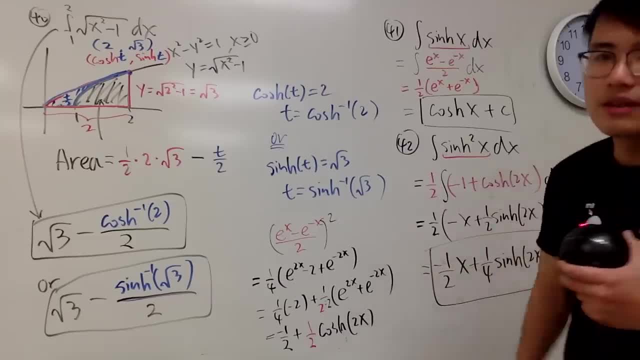 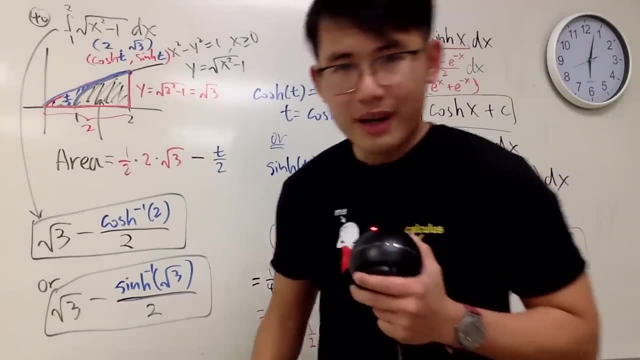 put plus z: Done deal. okay, Done deal, Not that bad, not that bad, huh, Take a look, take a look, okay. Next one: we did the sinh to the first power, sinh to the second power. Of course, let's talk about the sinh to the. 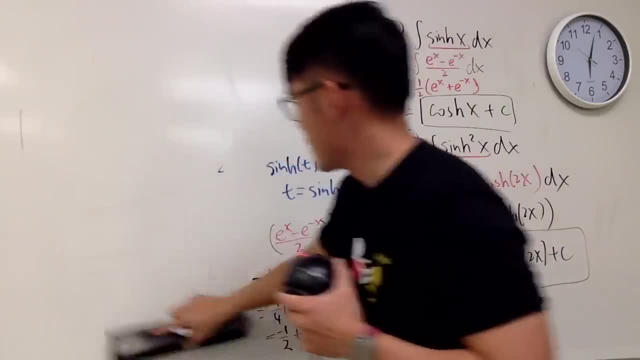 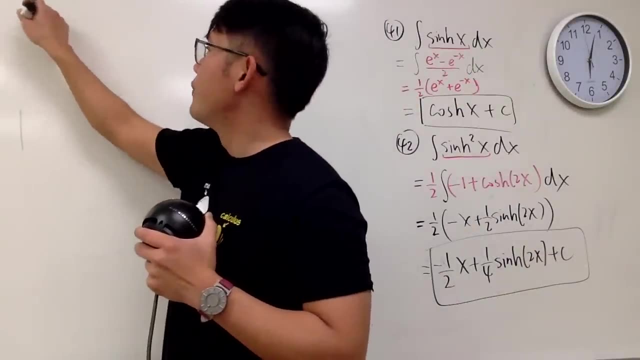 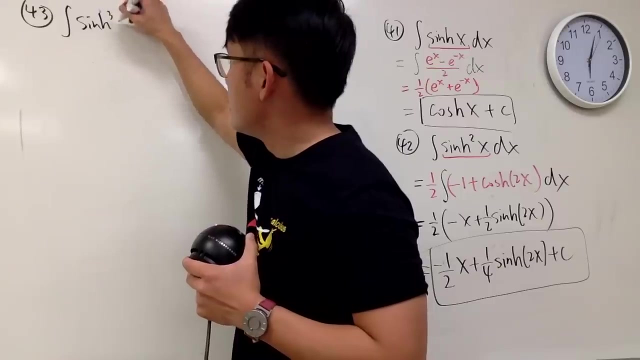 3rd power, Sinh to the 3rd power power. So I'll put this down right here for you guys. Number 43. Let's talk about the integral of sinh to the third power of x, And this time I'm going to do this in a faster. 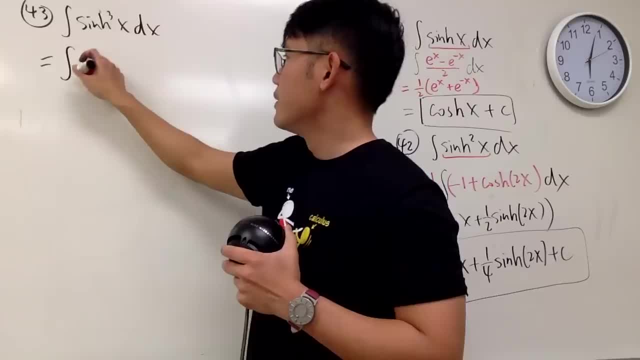 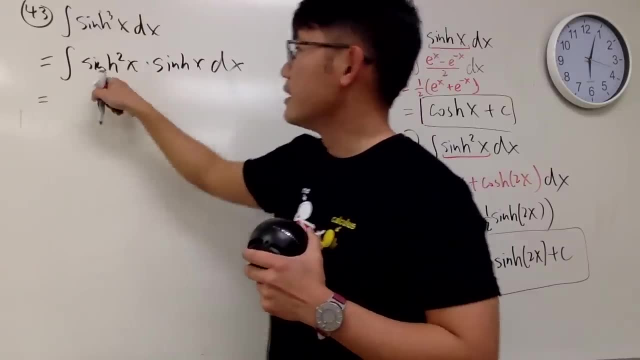 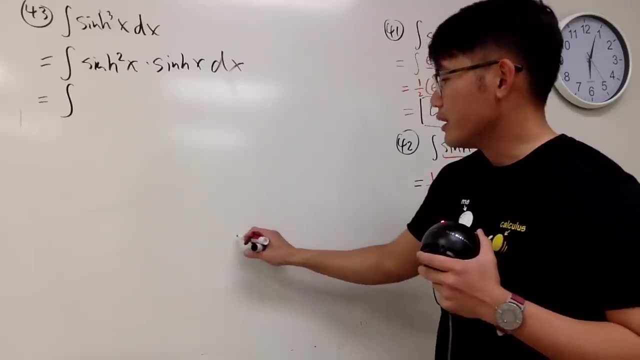 manner To do so. you're going to integrate, well, sinh squared x, You are going to take out one of the sinhs to help you out, And then the idea is: sinh squared is the same as something. Well, again, let me prove it to you guys real quick. The truth is when. 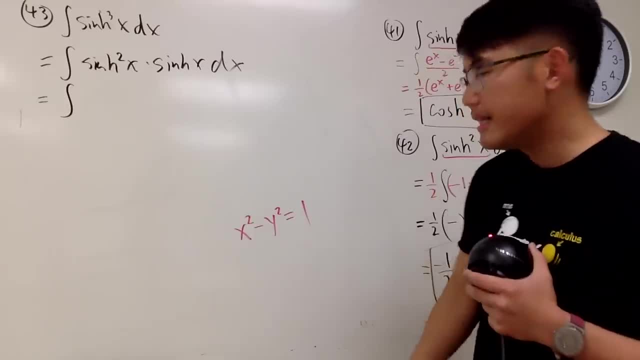 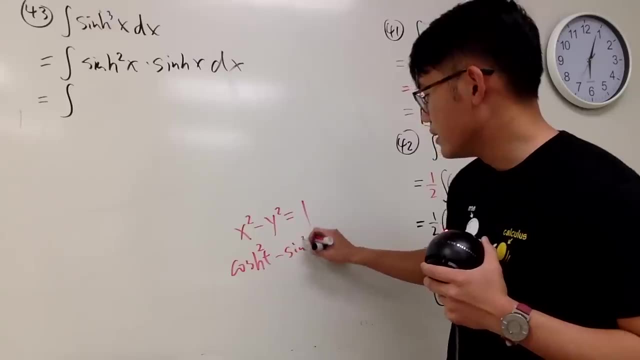 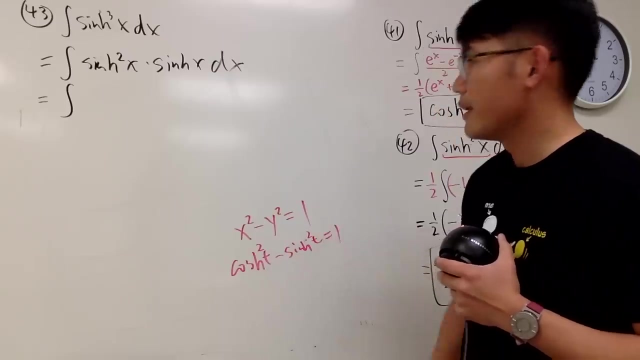 you have x squared minus y squared equals 1.. And the idea is this: right here is cos of t And you square that minus this is the sinh Sinh squared. t like that equals 1.. Over there, I want to have sinh squared. So what I'll do is I bring this to here, I bring the one. 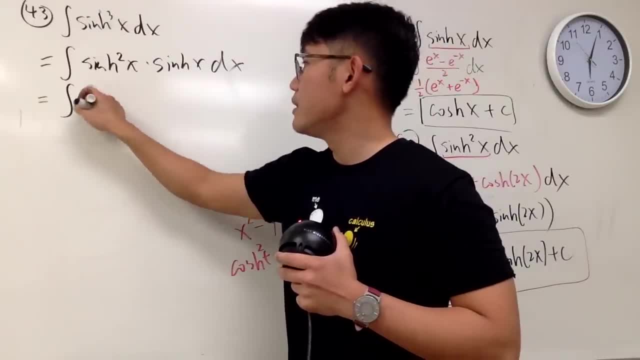 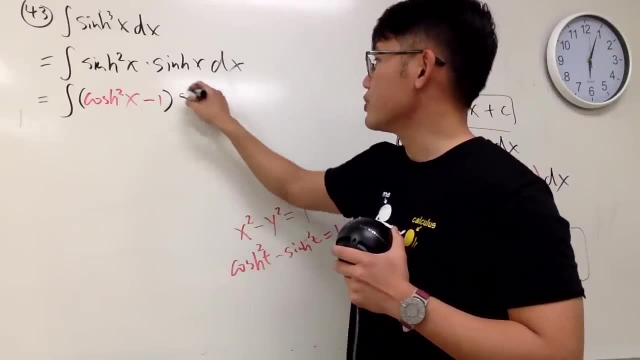 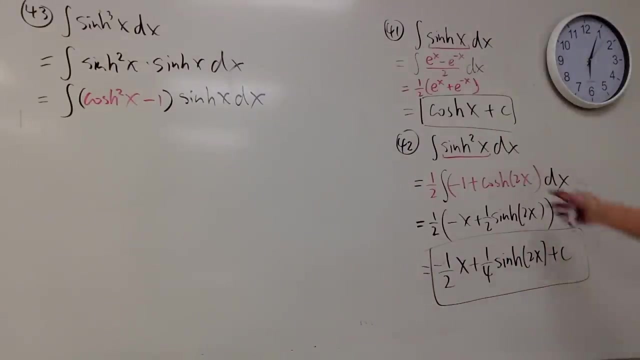 to here. So I will write this down as cos squared x And then minus 1.. Very good, And then we still have the sinh x on the outside. All right, So so far I think I have etched everybody right. Yeah, I did. Anyway, right here I'm just telling you guys that u equal. 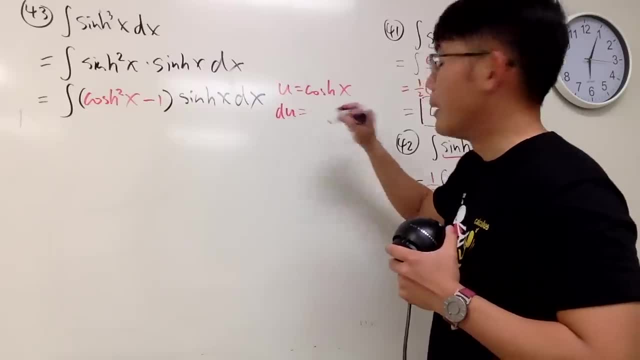 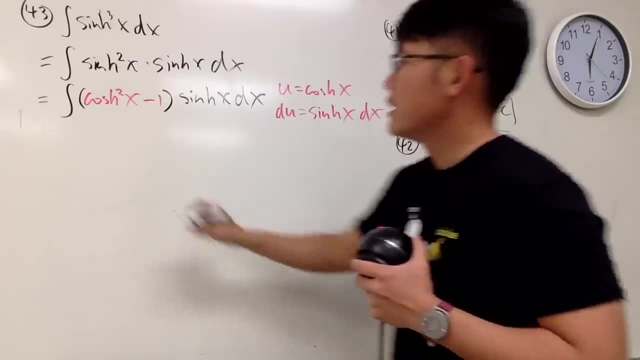 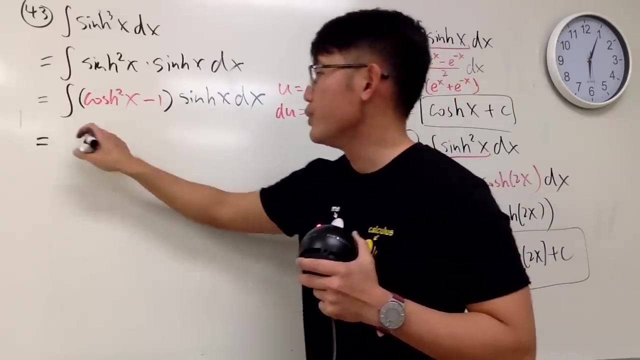 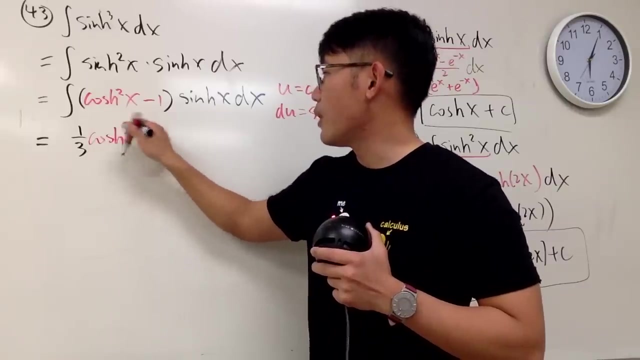 to cos x And then du is equal to positive. The derivative cos is still positive. okay, Positive sinh x, dx. So here's the deal. You get u squared minus 1, du Integrate that, You end up with 1 over u to the third power And u is cos. So I just put down cos to the third power. 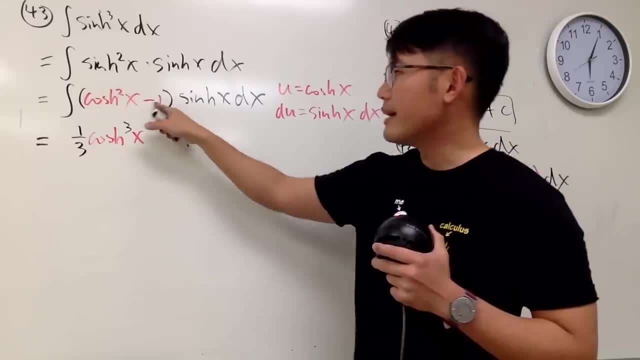 x. And then, don't forget, you have to minus 1, right, And you have to integrate that in the u squared. And then you have to integrate that in the u squared, And then you have to get the product of the u squared And you have to finished. You are done. Now you integrate. 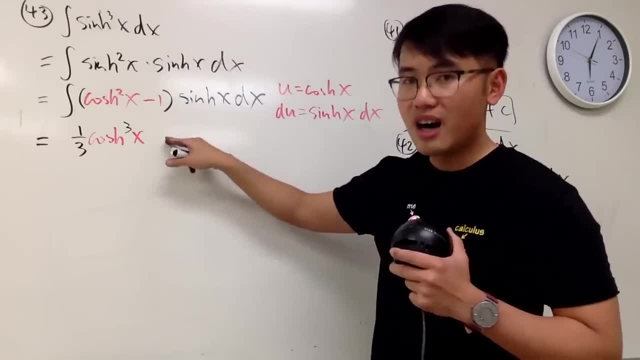 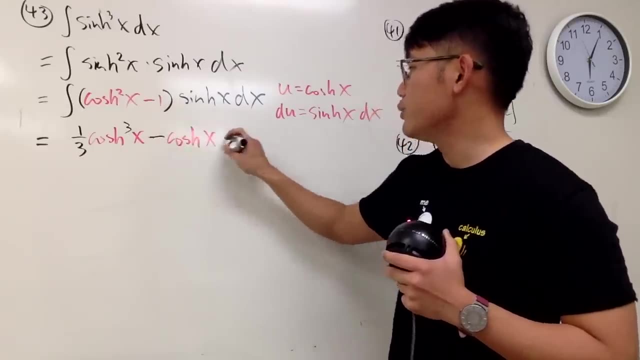 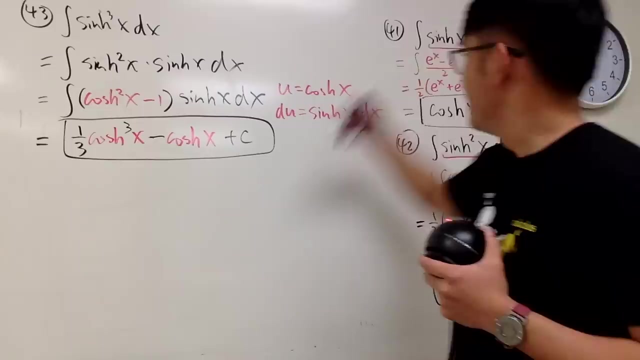 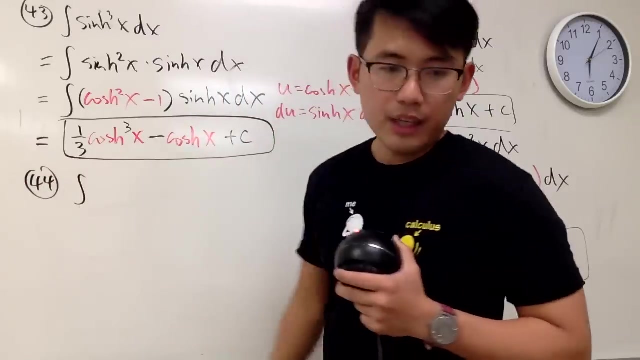 that into the u world. So when you integrate that into the u world you get cos. So you are going to minus cos of x And you are done Plus plus c. That's it. That's it Okay. So sinh first sinh. second sinh to the third power. Now number 44. Integrating 1 over. 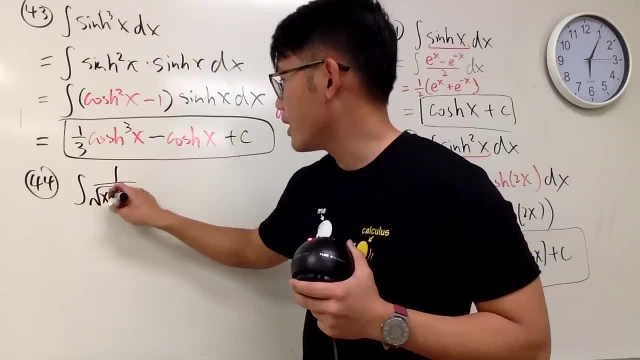 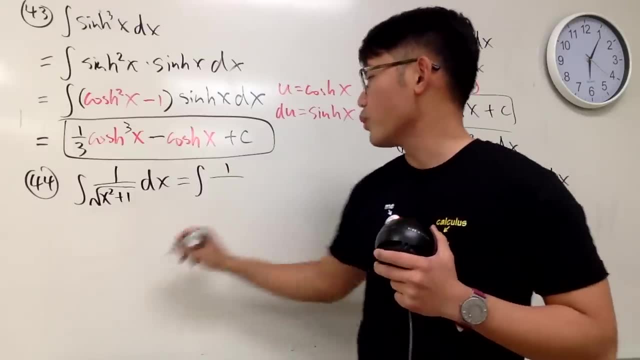 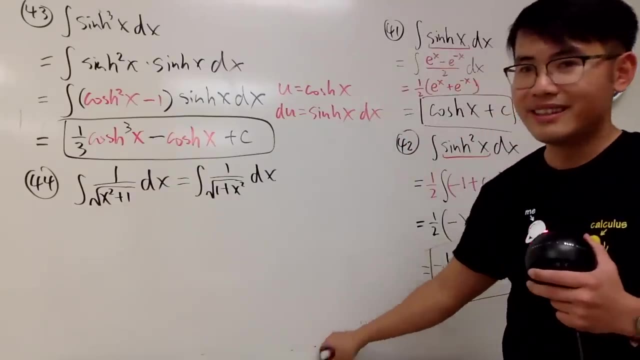 square root of 3.. of x squared plus 1 dx. Of course, this is the same as integrating 1 over. I can change the order, doesn't matter. 1 plus x squared dx. Remind you of something? Yes, you should. 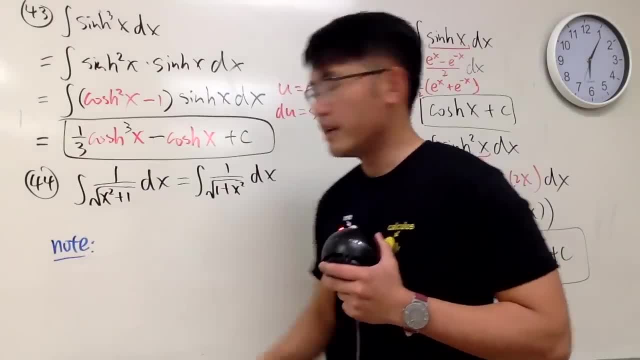 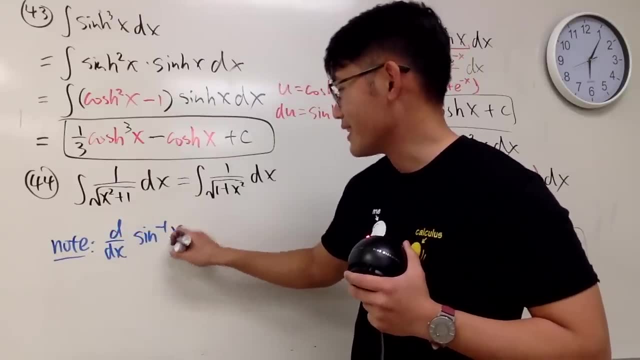 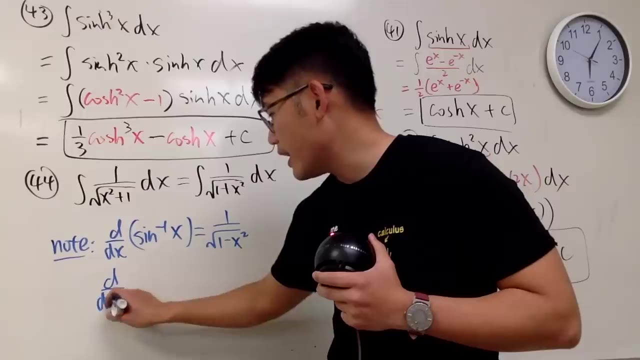 Let me remind you guys, Note, here's the truth: When you differentiate regular inverse sign, okay, regular inverse sign, you get 1 over square root of 1 minus x squared. But when you differentiate the inverse hyperbolic sign of x, 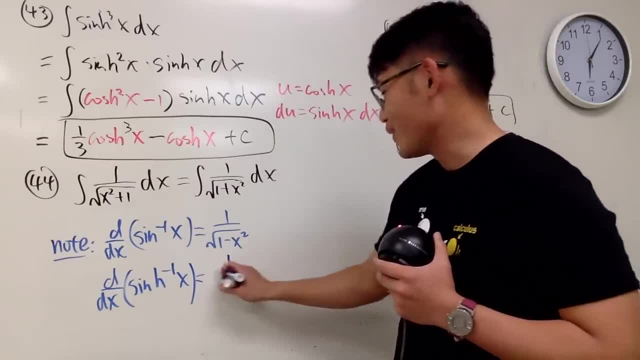 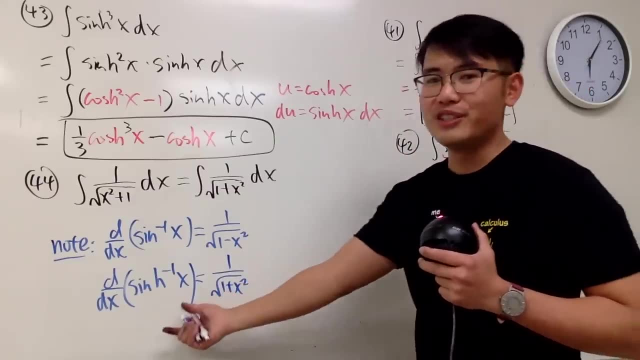 the only thing that's different is, instead of the minus, you have the plus, So you have 1 over square root of 1 plus x squared, And here's the deal. If you know this differentiation, of course you should know this. 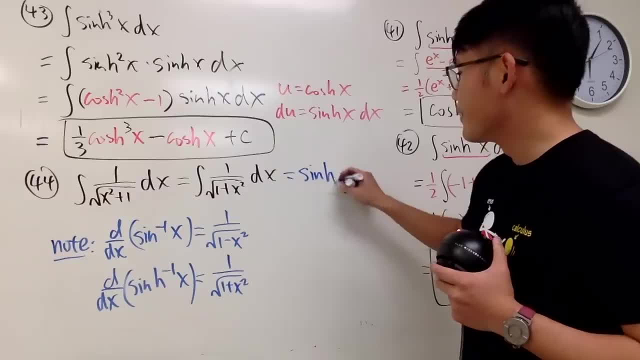 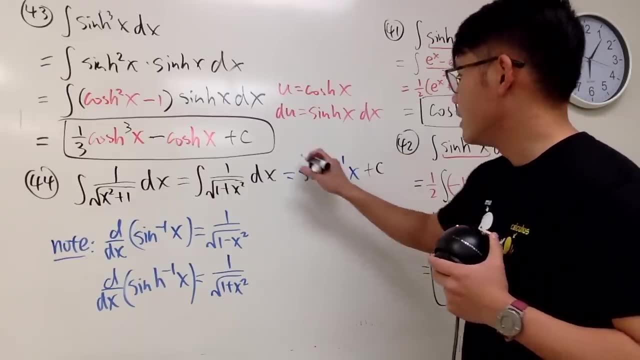 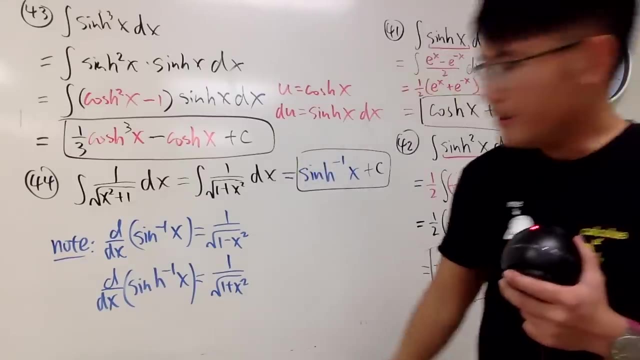 integral. the answer to this right here is just nicely equal to inverse sinh Of x and you are done Like that And if you really want, you can also do a trick for it. but I'll leave that to you guys, Alright, Okay. 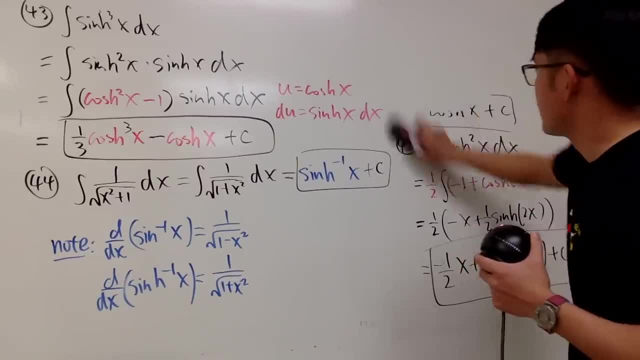 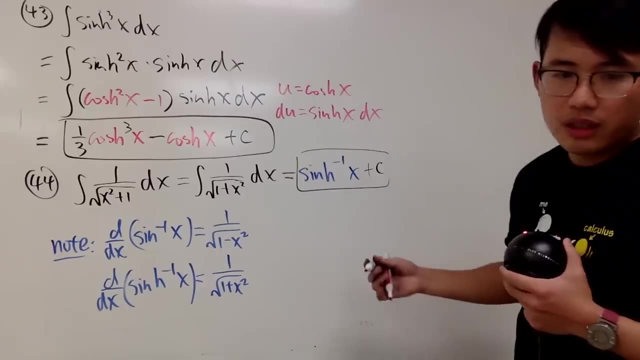 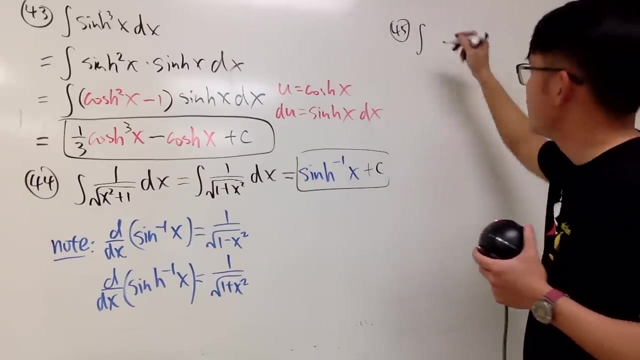 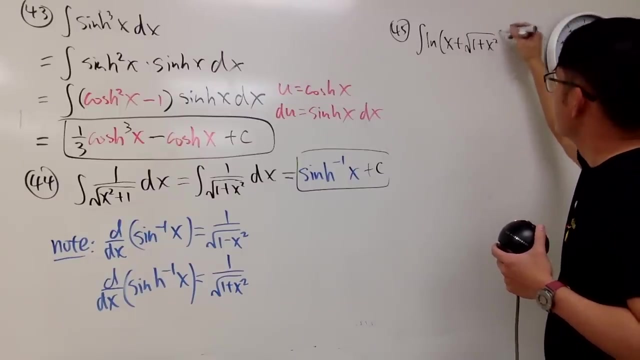 So here is the next one. right here, Number 45.. Integral of natural log of x plus square root of 1 plus x squared dx. Right Here is the deal. The truth is this: right here is asking us to integrate. 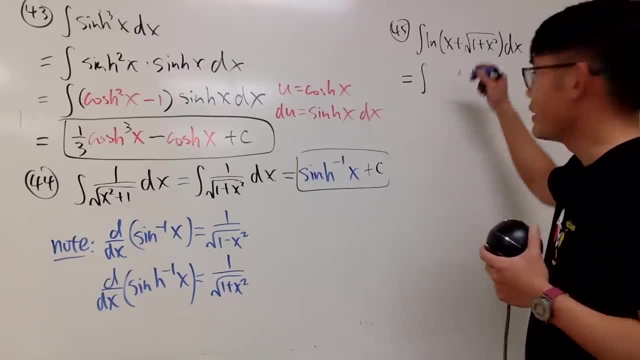 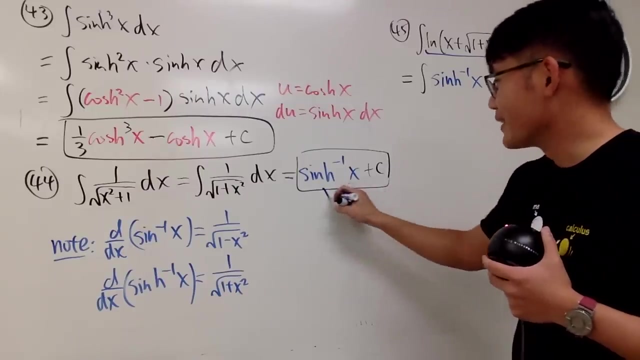 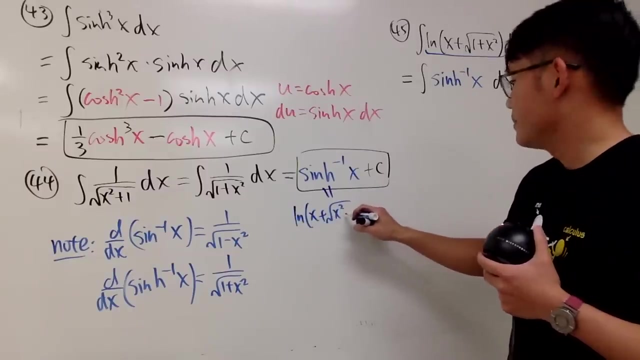 this right here. It's the same as that. It's a negative 1x like this and a dx: Alright. So the truth is, this right here is equal to natural log parenthesis: x plus square root of x, squared plus 1,. 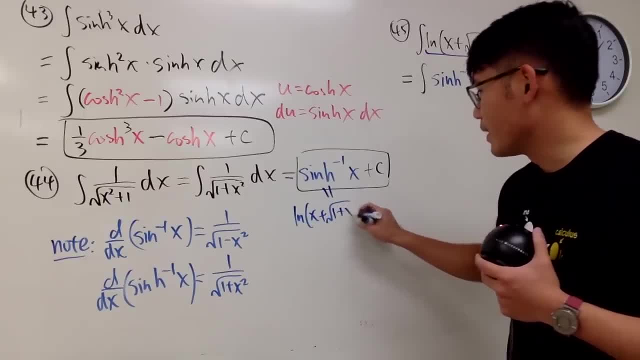 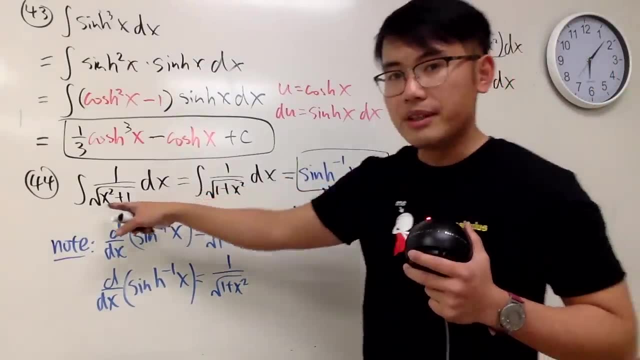 1 plus x squared doesn't really matter. Same thing, seriously. Plus 1. x squared plus 1 plus x squared- like this, They are the same thing. If you guys did tricks up for this, take x to a tangent right, Tangent theta, You end up with this right. 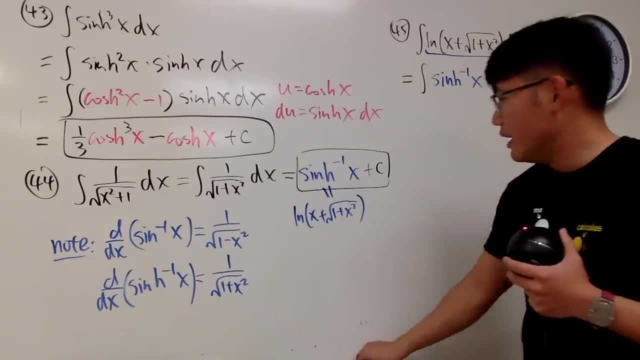 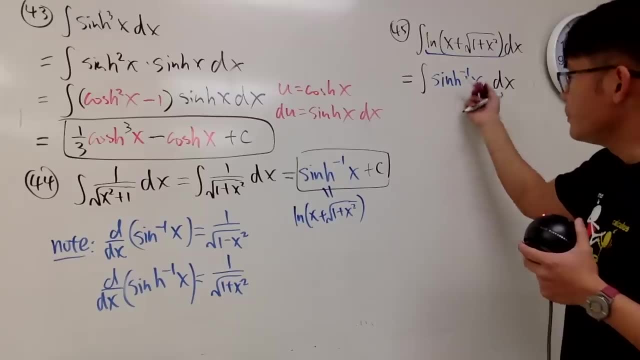 here, But I'll leave that to you guys. And again, you have two forms for the inverse: hyperbolic. This is the natural logarithm form for it, And the beauty of doing so is that this right here, we can do integration by parts, And of course, you can also look at that, Doesn't matter. 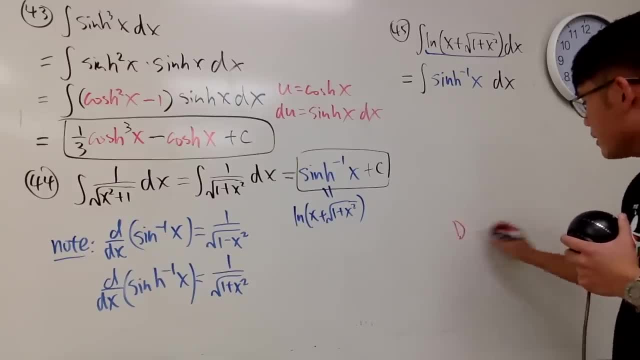 Anyway, here we go. We do integration by parts. I'll put it down right here: De and an. i. I will be differentiating this right here. Okay, The inverse hyperbolic sine of x. I'll be integrating 1.. 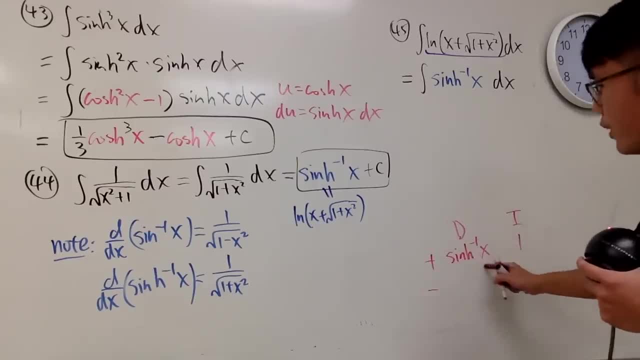 Plus minus, It's enough. The truth is, when you differentiate this, guess what? We did that? Well, I didn't do it, but you should know that, Or you should know how to do it. So I have this: plus x squared. 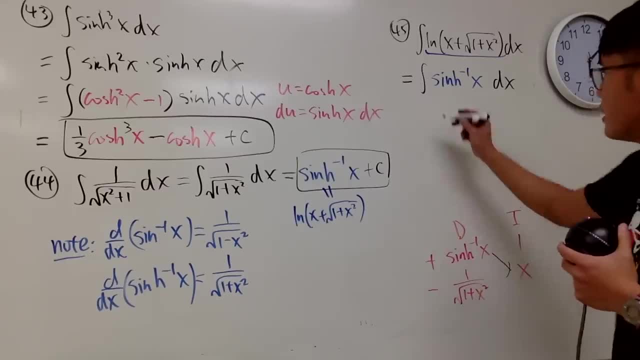 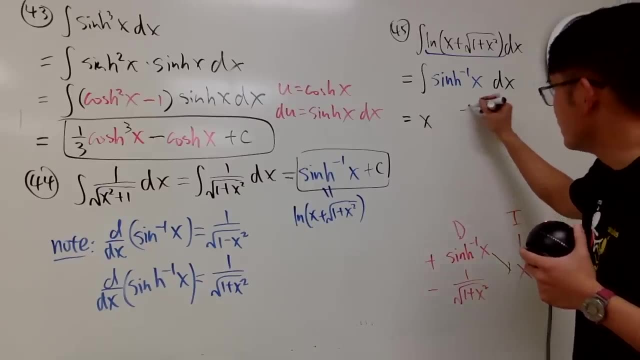 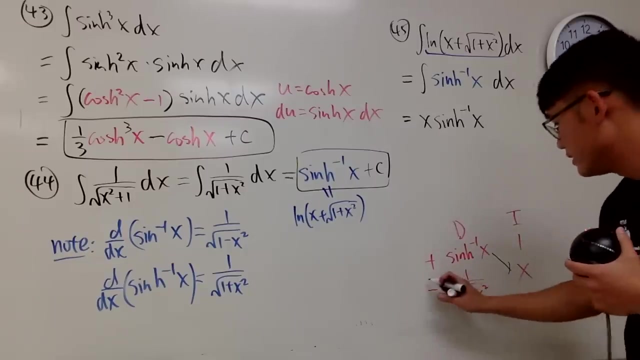 And when you integrate that you have x, First part of the answer. So this is going to be x times inverse. Let me see Inverse hyperbolic sine of x. And then we have to minus this integral. Right, We have to minus this integral. 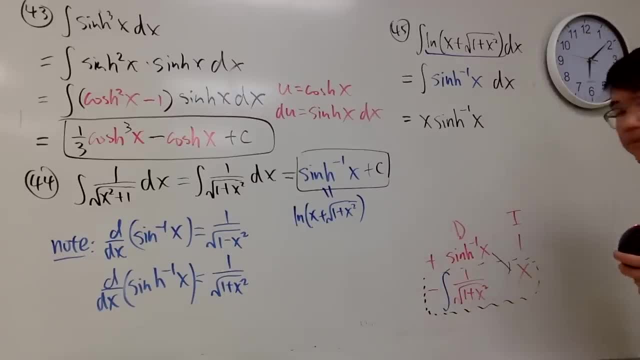 Again, we have to minus this integral. And here is the idea. This is the minus. It stays. When you have x over that, the integral for that is just nicely equal to square root of 1 plus x squared, And then you are done. 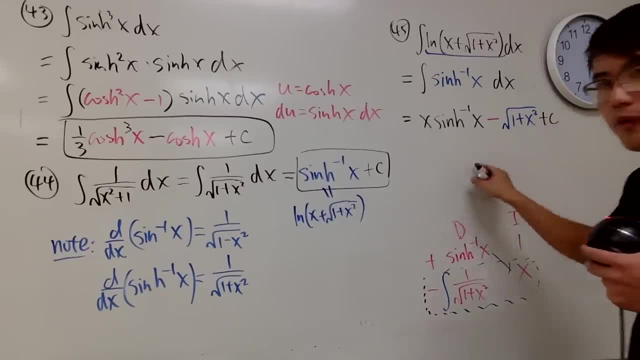 Right, Real quick. if you differentiate this, you see you put 1 over 2 with this inside in the denominator And then multiply by 2x, The 2 cancel. So you have the x on the top over that And the negative is on the top already. 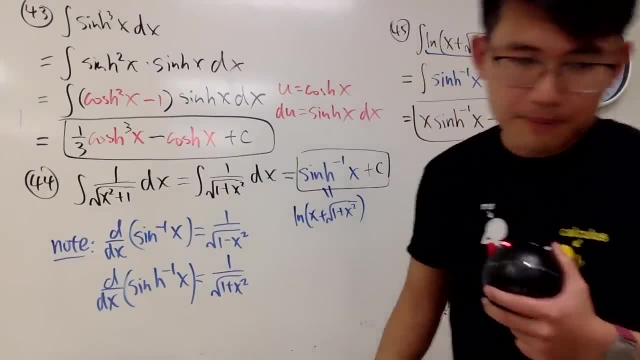 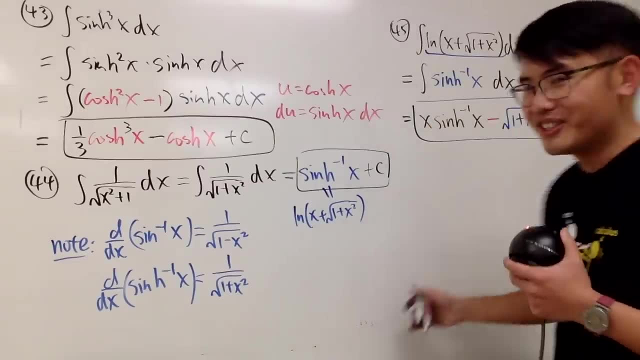 So this is done Like this, Right, So that's cool. Now, okay, we talked about enough of the sinh business, Let's get to somebody else: Tensh, How's that? Number 46. Integral of. 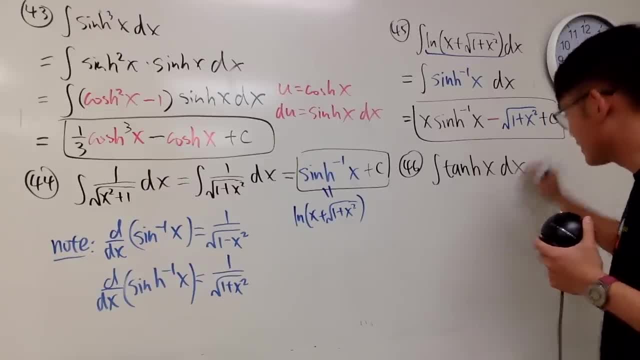 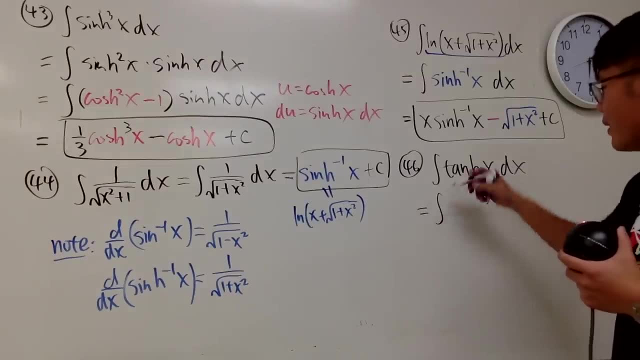 tangent. But what's the h now? x, dx, Woohoo, Let's see. Okay, Of course you can do it this way. This is the integral. This is just like the regular tangent. This is the same as sinh. Yes, I'm still back to sinh. 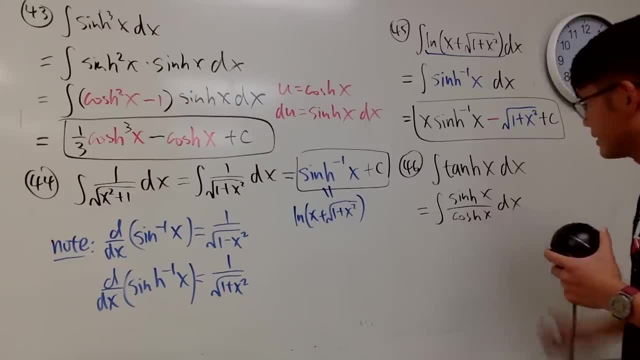 x over cosh x dx. Here's the idea. Let u equal to cosh x, Like that, And then du will be positive sinh x dx. So you have 1 over u in the? u world. Integrate that. 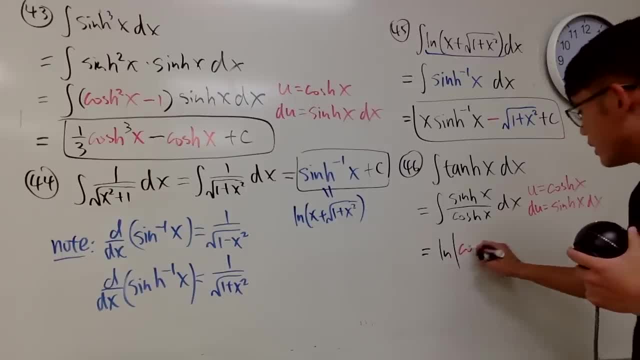 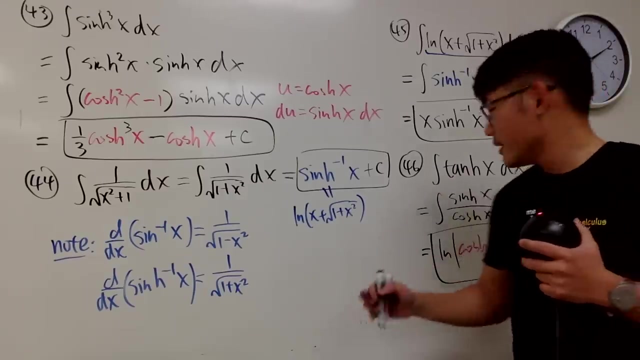 You get natural log absolute value of u which is cosh of x, Like this. Okay, Just like that. And this is very, very nice. And we're done for plus c And we're done. No negative For the regular tangent. here you have. 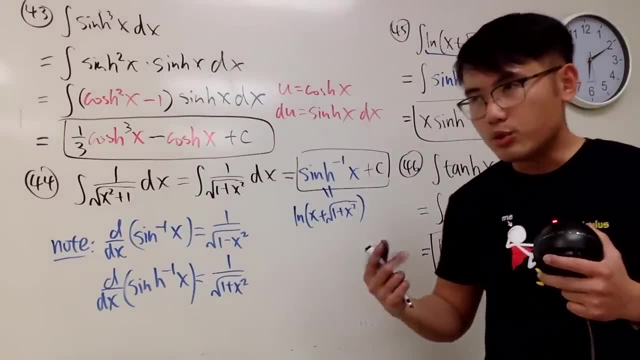 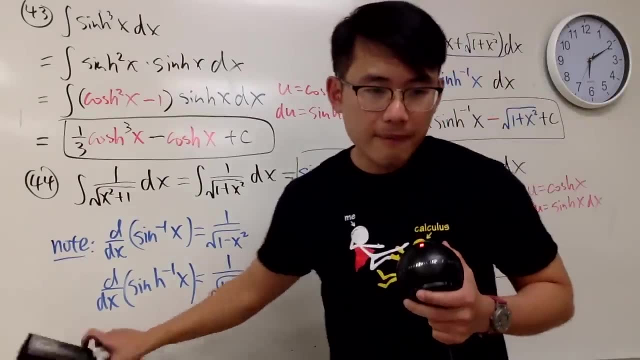 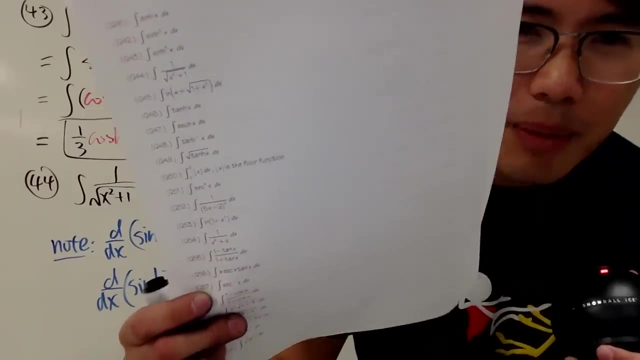 the negative derivative of regular cosines. Regular cosine is negative, sinh x And you have a negative in the front. But this right here is clean, Really, really clean. Okay. Now, seriously, Hyperbolic secant, Hyperbolic secant, Okay. 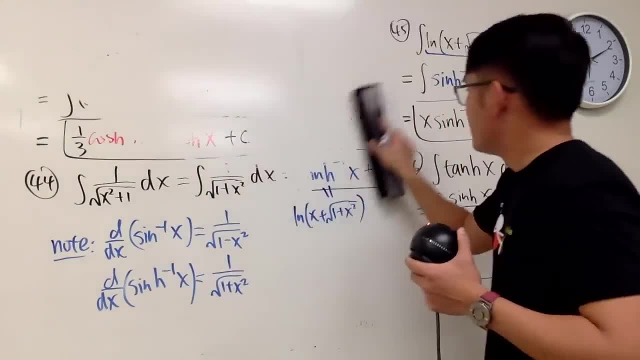 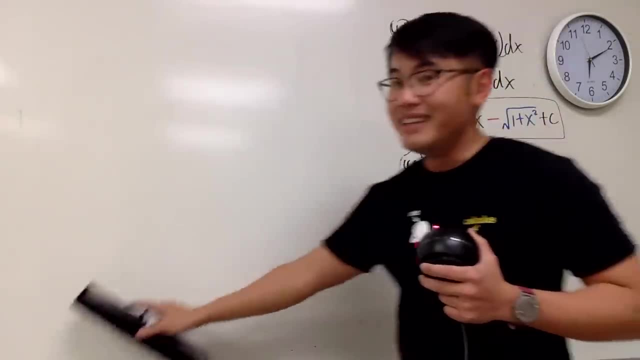 Let's deal with this. We can do it, No problem. 46 integrals, 46 integrals, And hopefully you guys can be convinced that these aren't the easy ones, Right? Not a lot of them are easy ones. Sometimes we do like go. 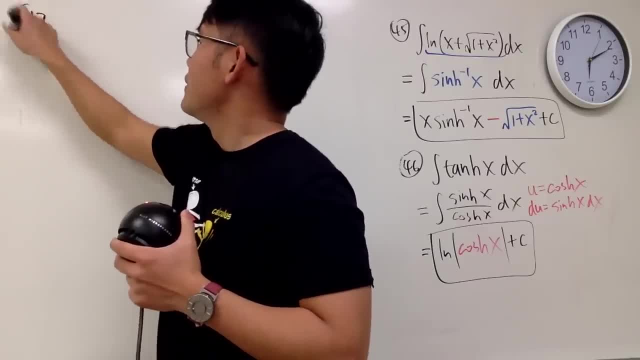 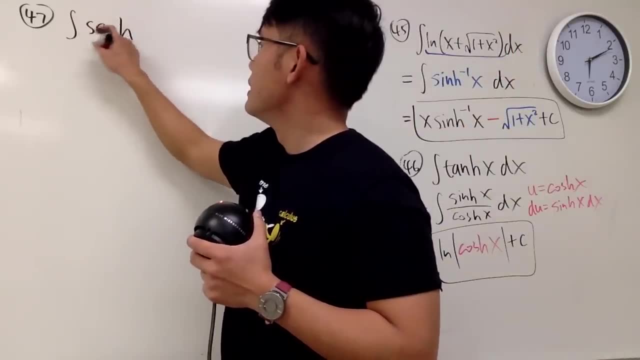 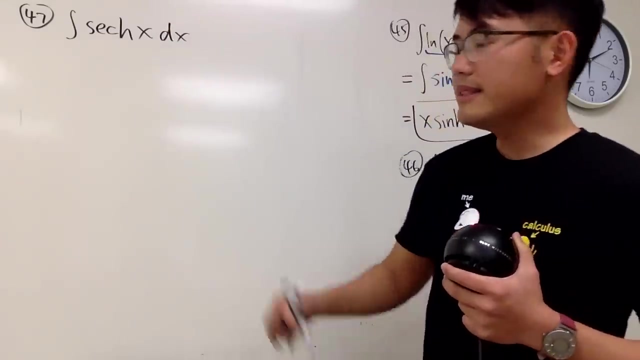 some easy ones once in a while, But you know most of them are pretty difficult, I think. Okay, Number 47. Integral of hyperbolic secant of x, Like this dx This time. yes, you can do the similar trick that I did. 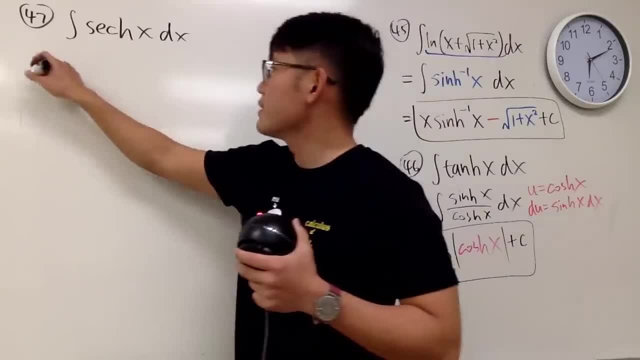 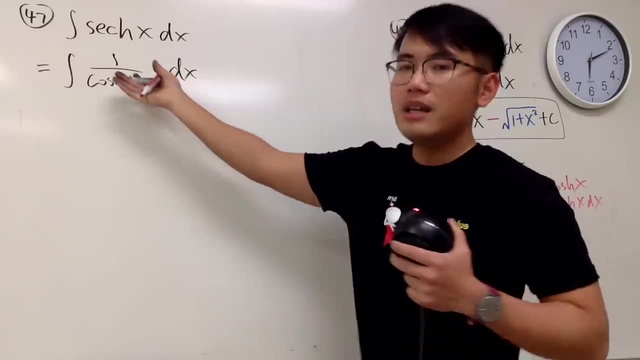 with the regular secant. But I'll show you guys something different. First of all, this right here is the same as 1 over cos, And the problem is that, you see, I don't have the sinh to help me out, unlike this. But it's okay, Don't give up, I'm going. 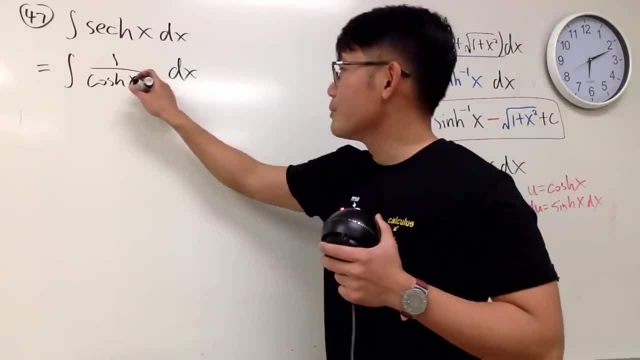 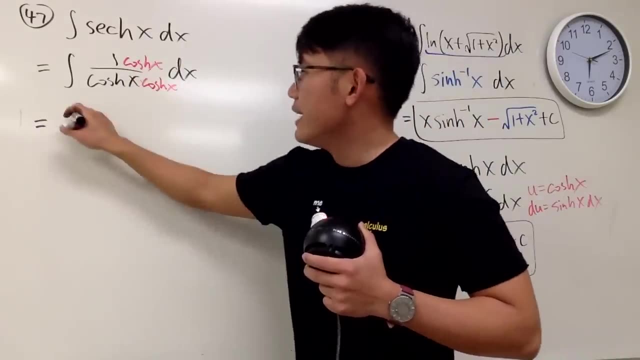 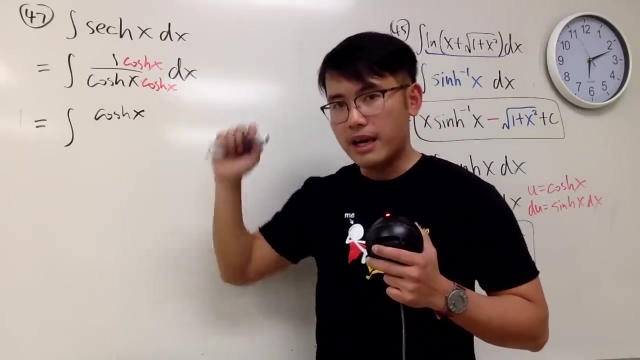 to produce something to help me out as well. Well, I will just multiply the bottom and the top by cos. cos Why? Because the idea is on the top now. yes, I have that cos. And remember: cos is equal to what sinh squared x plus 1.. 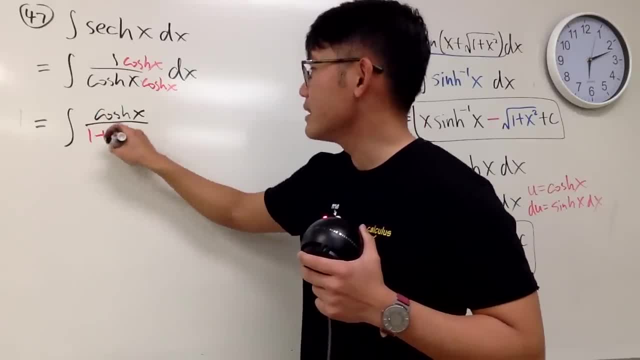 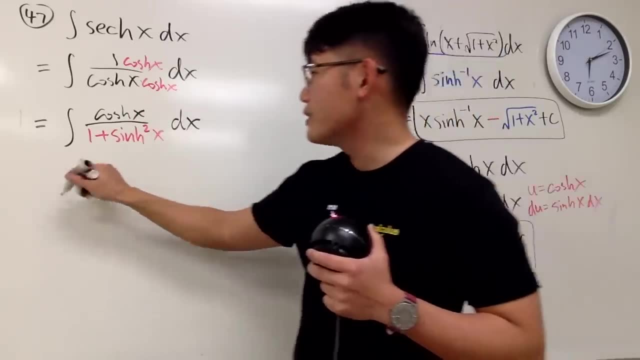 So we can use the identity. I can write down 1 plus sinh squared x, like that for you guys. With that being said, in fact, we can do a little use-up. Let u equal just the sinh to the first power of x, Because 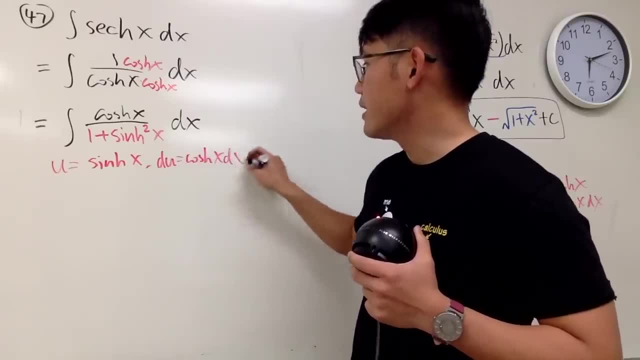 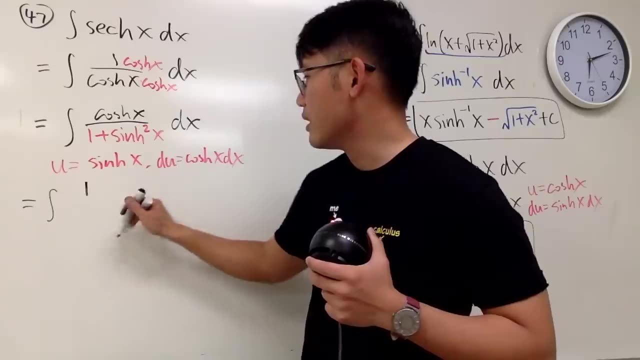 this way: du is cos dx, which is the one that we have on the top, And then we can take this integral to the? u world. Integral of this right here is the du, And then on the bottom is 1 plus u squared. 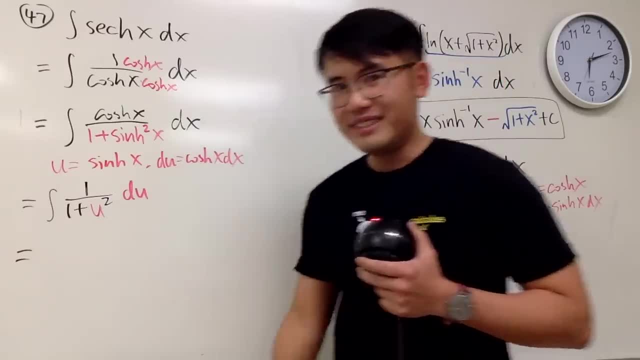 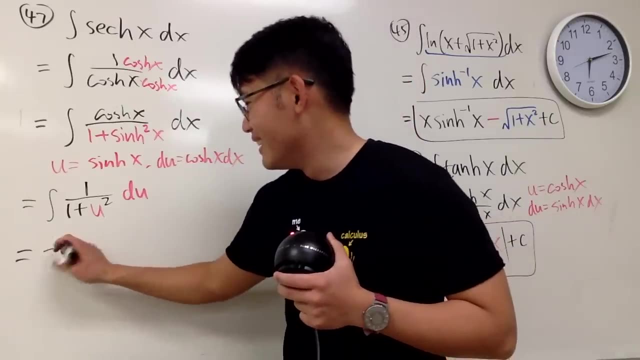 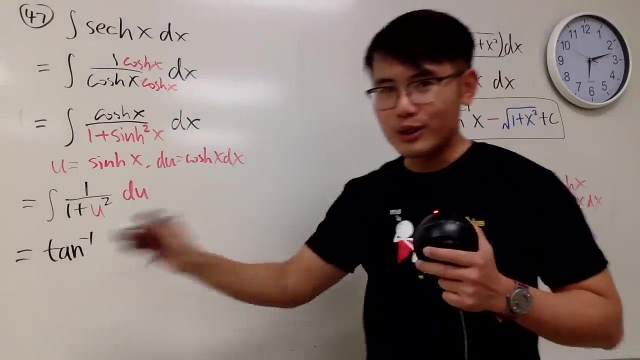 Very nice. So this ends up pretty nicely, And then in the end, of course, you end up with the inverse regular tangent: No h. So far, I think that's the first guy right there- No h, No h. Okay, no h. Inverse tangent. 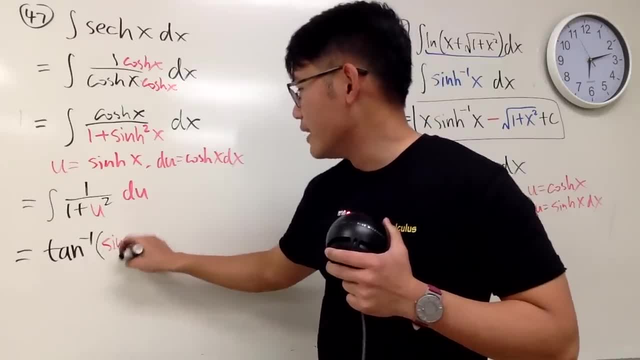 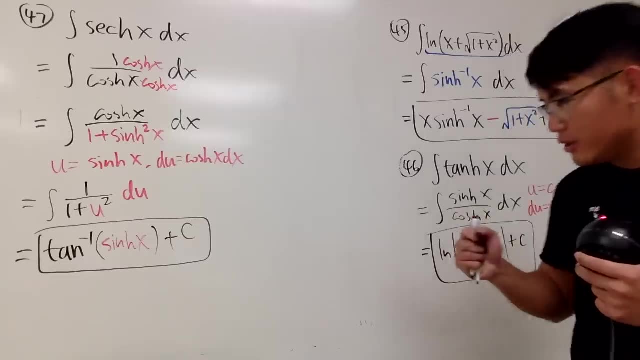 this is the regular version And you put the u inside And then u is of course the sinh of x, like that, And you are done. So put a plus z, Done, Okay. Energy, energy, energy. We still have the energy. 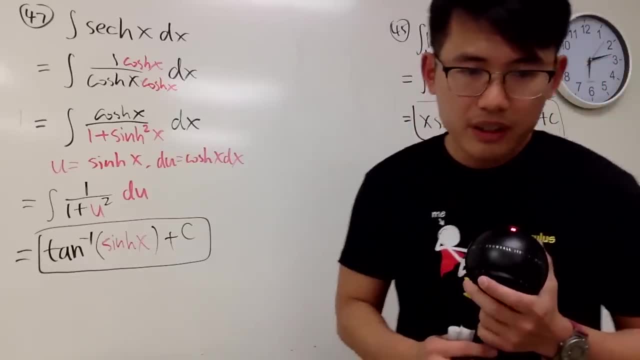 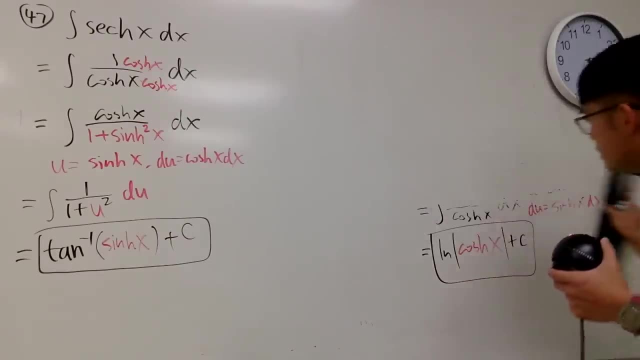 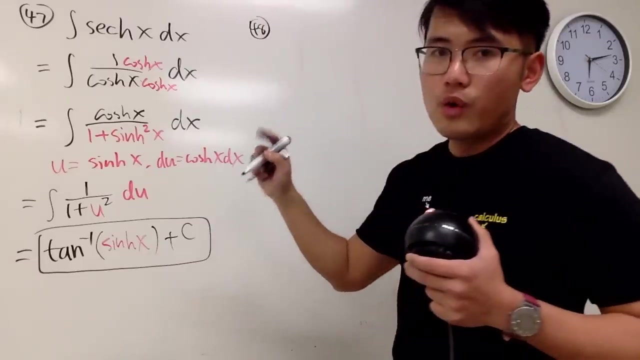 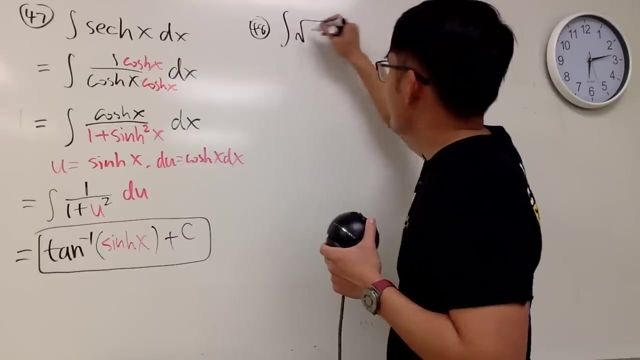 Okay, Now let's see We have 48.. I'm going to erase this now: 48.. I'm not kidding, We are going to be integrating the square root of hyperbolic tangent x, Integral of square root of hyperbolic tangent x, dx. 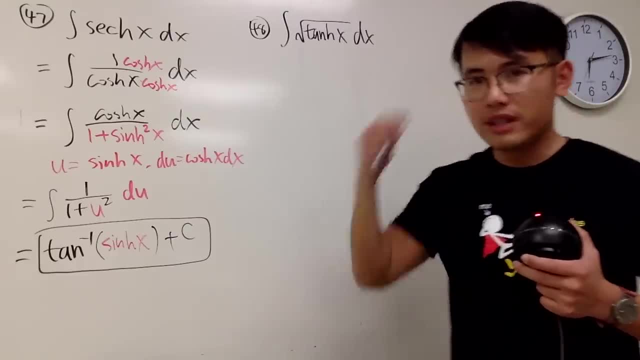 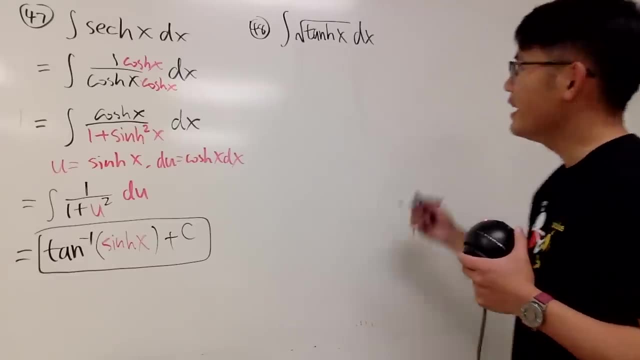 And, in fact, one of my former students, Edward. he was a guest speaker on this, But, you know, maybe some of you guys haven't seen it, So we're going to do it right here. Here is the du. 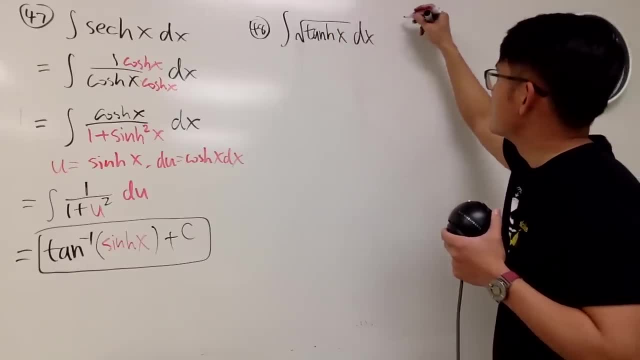 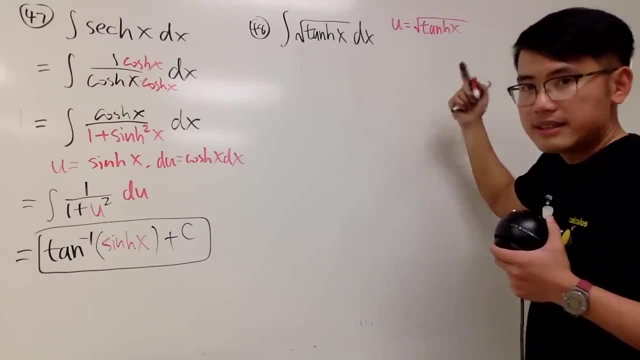 We are going to start with u sub. Let u equal to the whole square root. So let's see u equal the square root of hyperbolic tangent of x. And then let's get the dx. So let's do a few things in your head Square both sides. 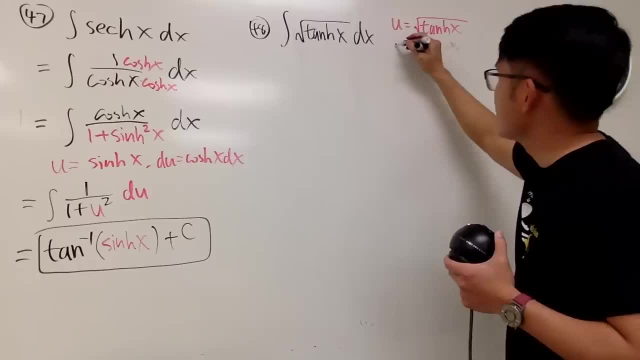 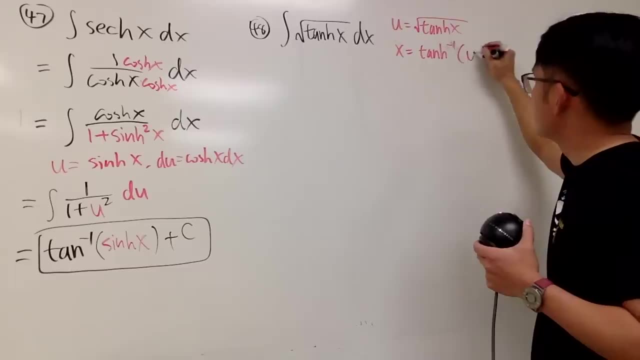 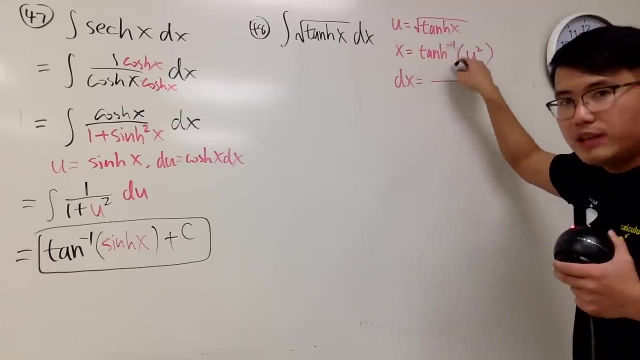 And then take the inverse hyperbolic tangent on both sides. In another word, x is equal to the inverse hyperbolic tangent of u squared. And then I will look at this and differentiate. dx will be okay. when you have the h root, you are going to have the square root of hyperbolic tangent of x. 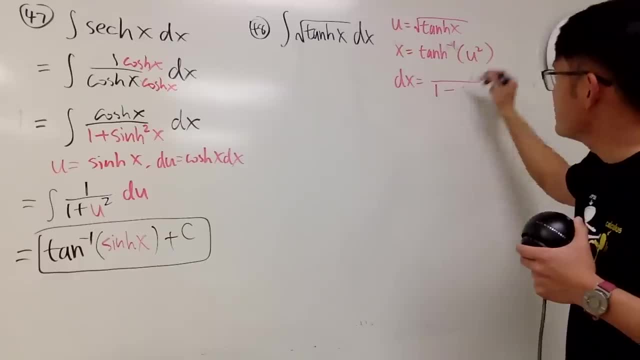 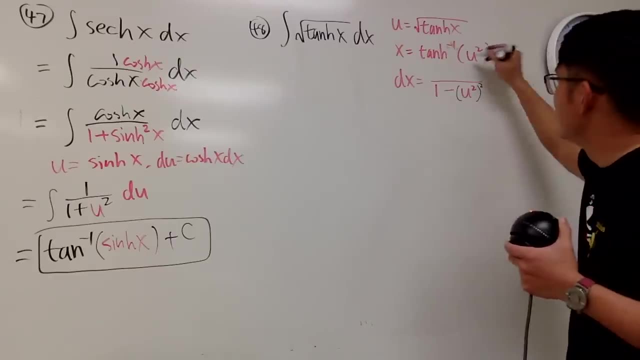 Right here. When you differentiate this, it's 1 over, 1 minus. this thing squared, So u squared. And then you square that. And don't forget the chain loop multiplied by the derivative inside, which is 2u. like this: Okay, It's like that. 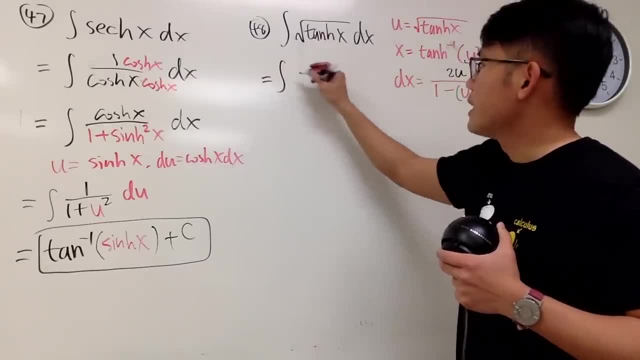 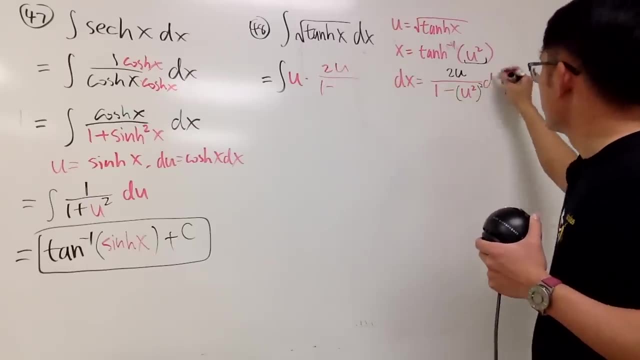 Now we will see. this is the integral. This right here is our u, And then the dx is all this, which is 2u over 1 minus 1 minus u, to the fourth power, du, And then, as you can, 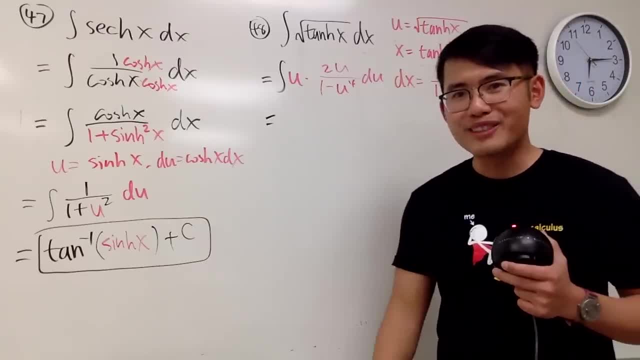 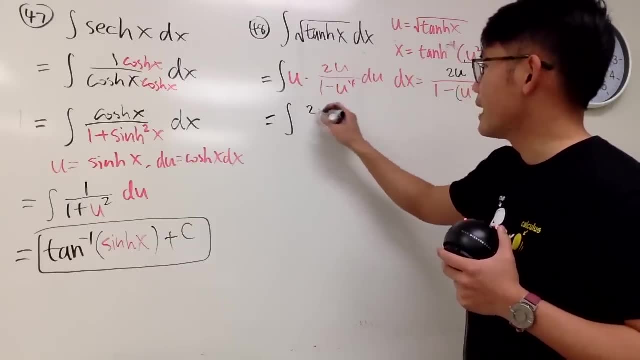 see this right. here you can try to do partial fractions. I'll show you guys this way much better. Right Integral: I will have the 2u squared on the top. Okay, 2u squared over 1 minus u. to the fourth power. 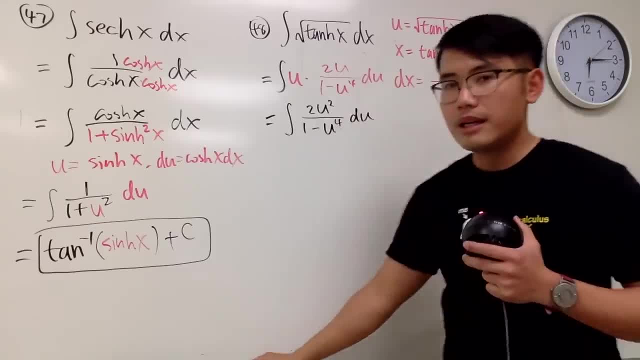 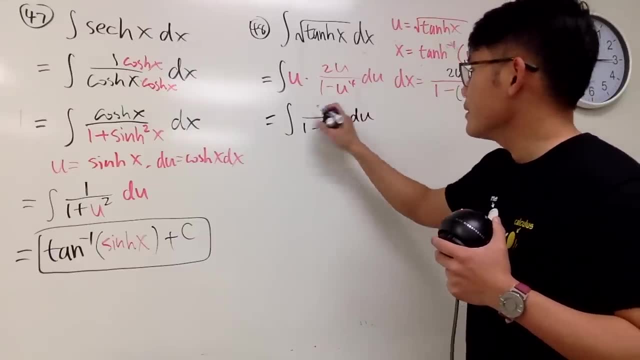 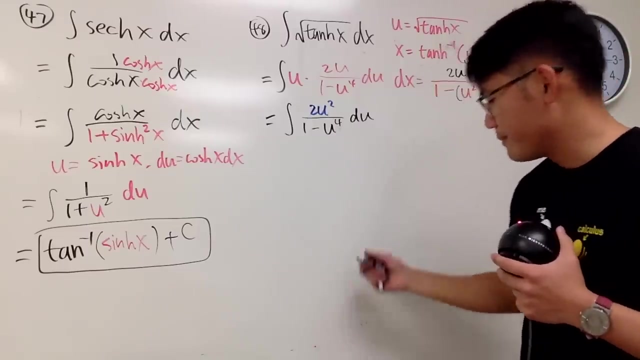 And then the du Right. So let me just focus on the 2u squared. I'm not going to do the usual partial fractions. You'll see, This is better. Well, as you all know, we can factor this out, And if you factor this, you are going to get. 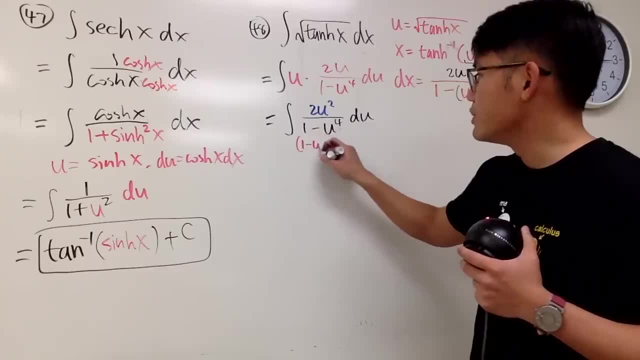 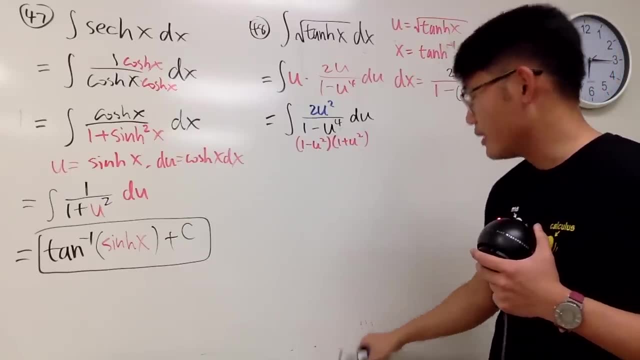 1. This format is going to be 1 minus u squared times 1 plus u squared. Let's talk about how to make things happen. So let's see: on the top We have the integral, On the bottom we have the. 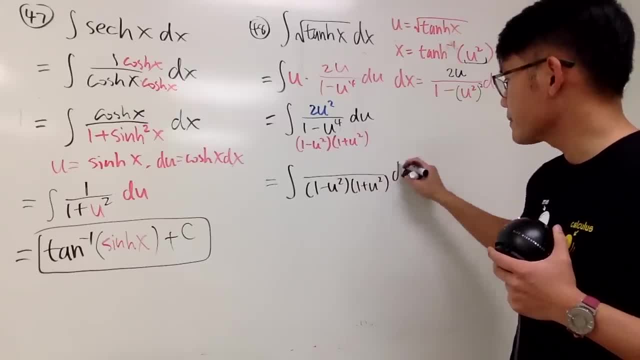 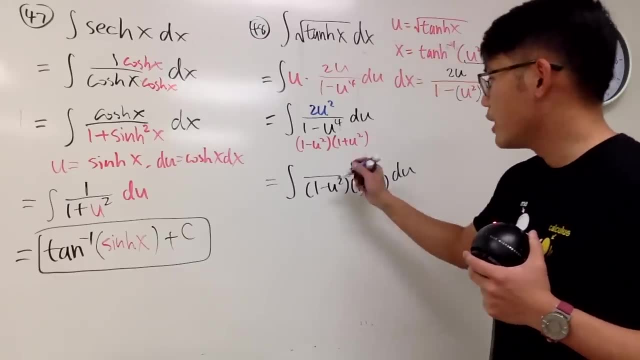 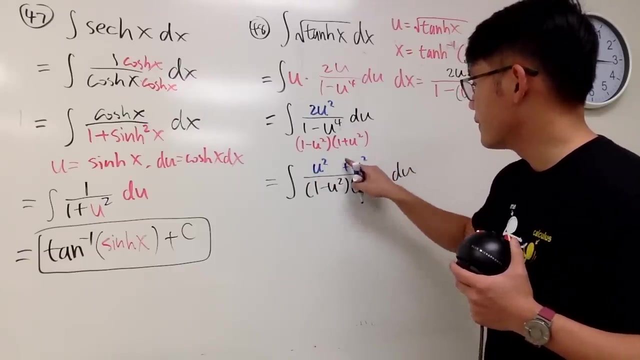 1 minus u squared times 1 plus u squared. On the top we have 2u squared, So we can look at that as u squared plus u squared. How's that Right? u squared plus u squared Like that. So that's fair. 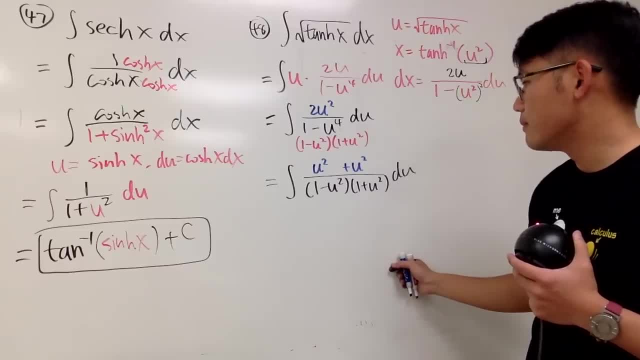 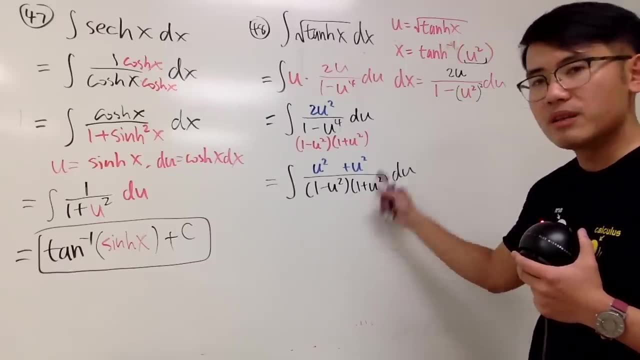 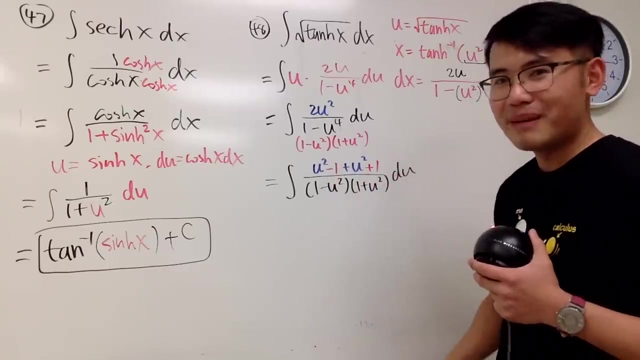 And now, hmm Well, wouldn't it be nice if somebody has a 1, somebody has a negative 1? Well, perfect, That's minus 1 here and plus 1 here. Everybody's happy, And you'll see this right here- is equal to the integral, And let me just write this down clean for you guys. 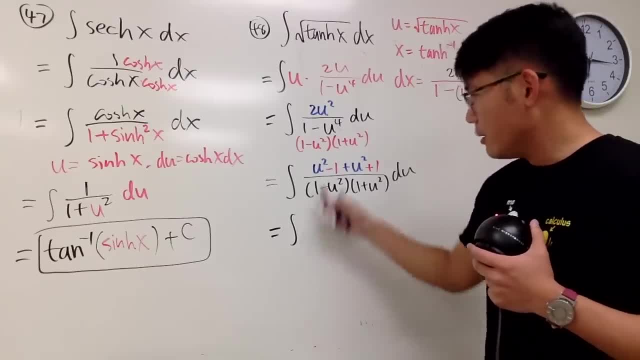 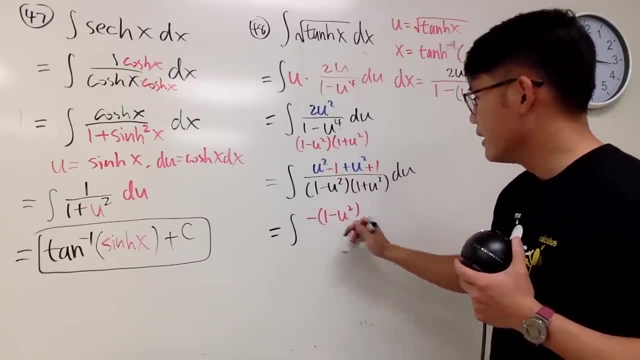 So I'll pair this up, which is going to be, of course, be careful with the negatives. You end out with negative parentheses. if you would like, You can write this as 1 minus u, squared like this, And then over this: 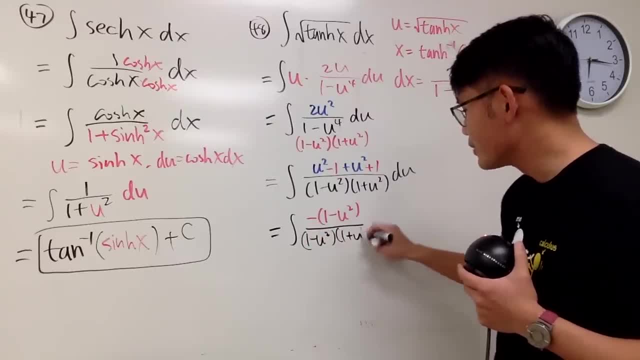 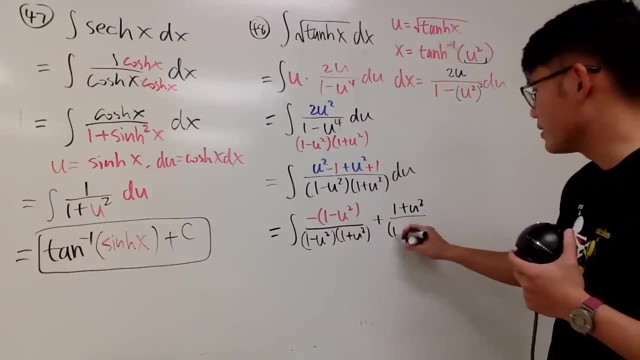 denominator, which is 1 minus u squared times 1 plus u squared, And then right here, plus. This is good, so you don't have to do anything tricky, But I'll change the order just to make that look better. u squared times 1 plus u squared, like this: 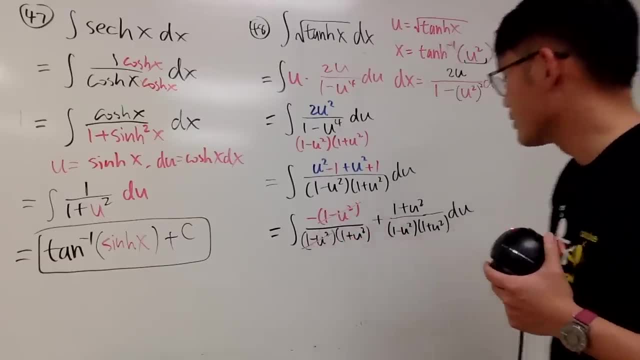 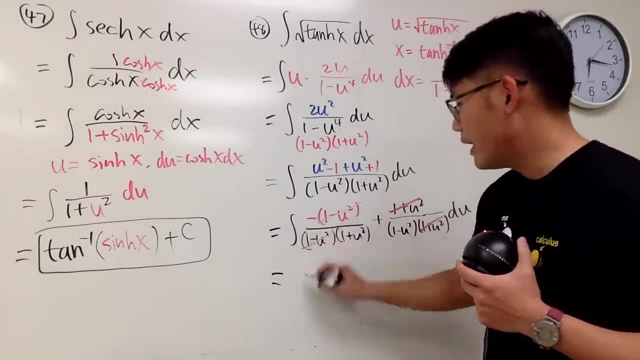 Here's the deal: This and that cancel out nicely, This and that cancel out nicely, Well. well, You have the first one being the integral and you have the negative, 1 over 1 plus u squared, and that will give us: 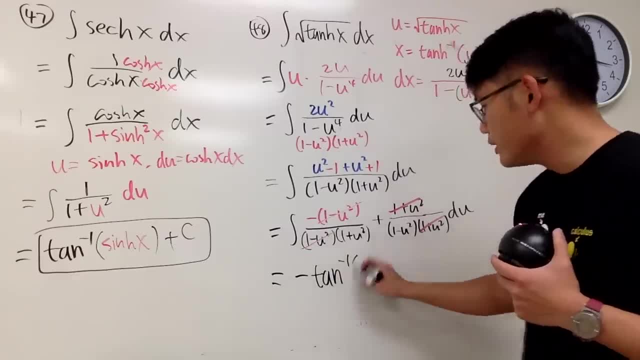 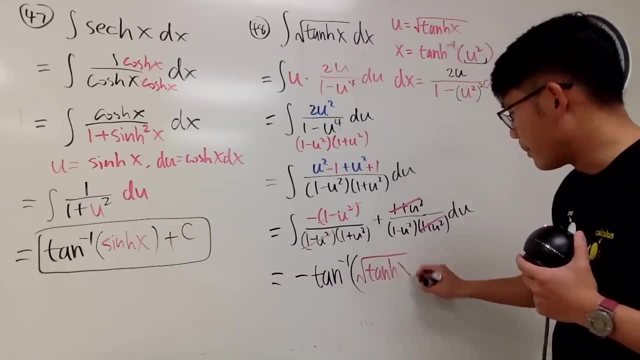 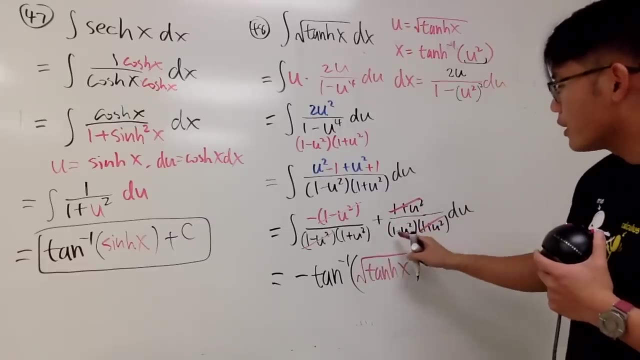 inverse tangent of u and u is this guy. So we put down the square root of the tangent, but you have the h, so the hyperbolic version of the tangent like that, Very nice. And then you add: if you have 1 over, 1 minus u, squared. 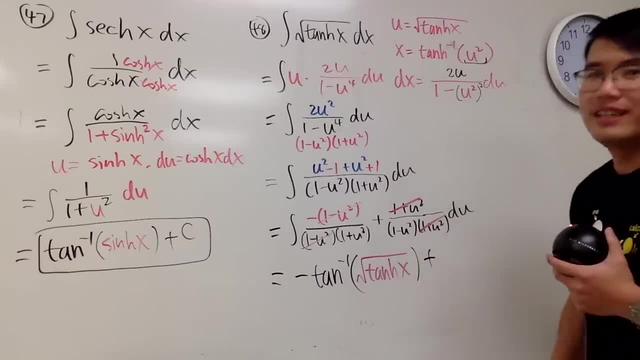 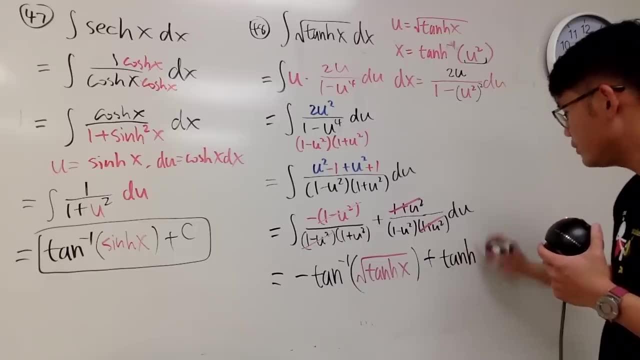 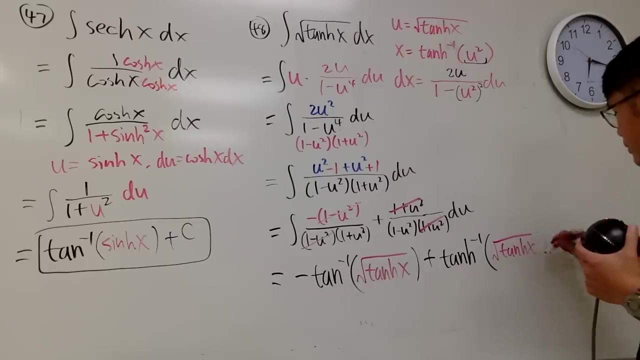 you can use the inverse tangent for it. So we'll just get tan with the h inverse and then it's really symmetrical. Very nice. Square root of tangent x, because that's a, u, And then you are done. 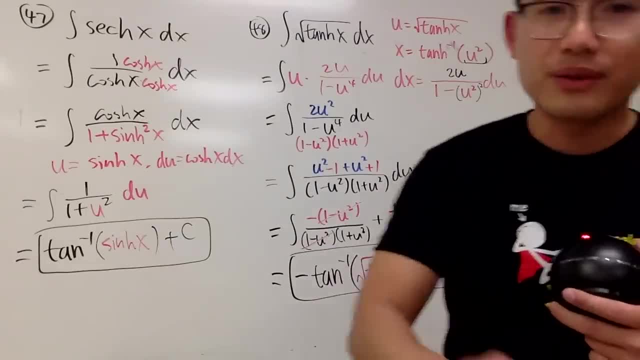 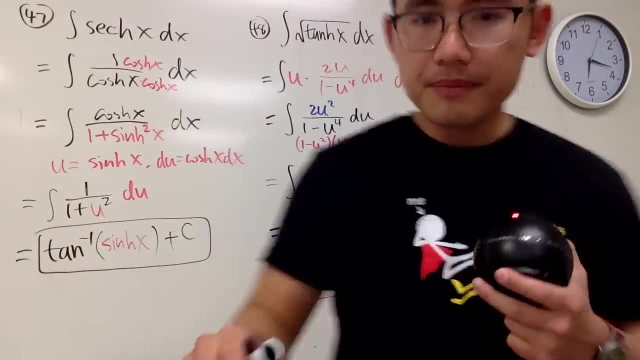 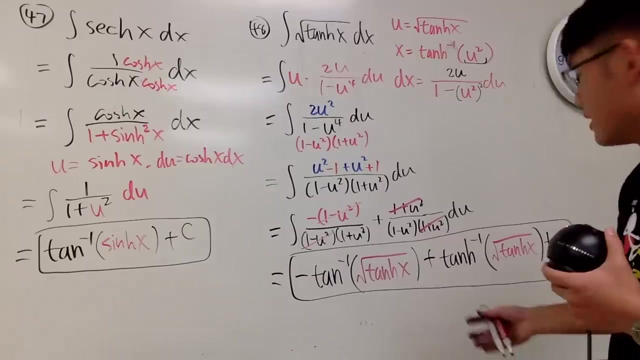 Like this: Right, You are done, you are done, you are done. Okay, I'm expecting to finish this in 6 hours. I don't know if that's the case or not, but we'll try. This is 48.. 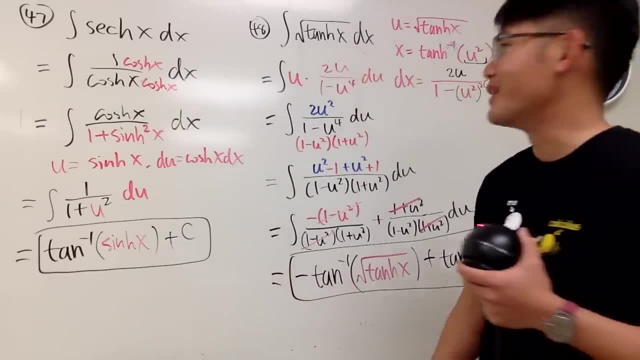 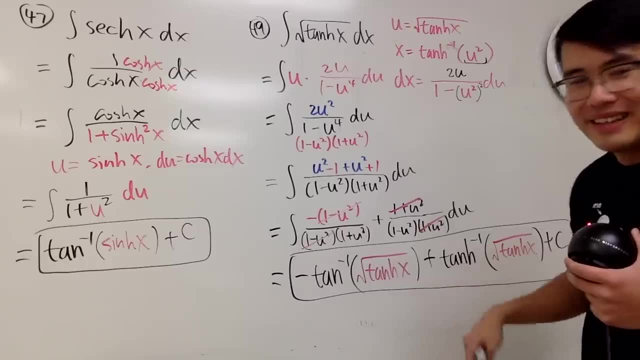 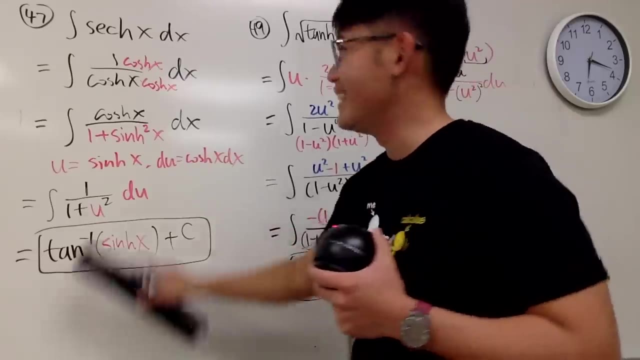 No, My god, I missed it. Sorry, This is technically 49. But the good thing is, you see, this is 49.. 48 is the inverse tangent. My bad, So pretend that you haven't seen this right. 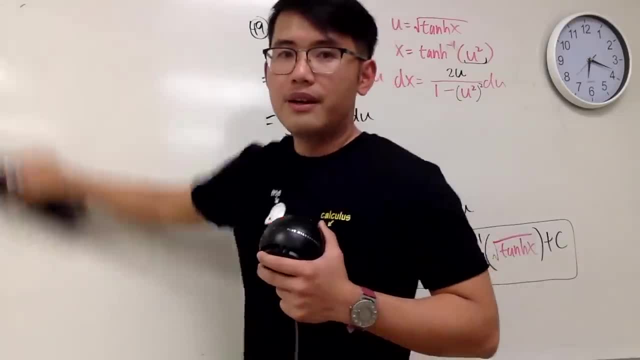 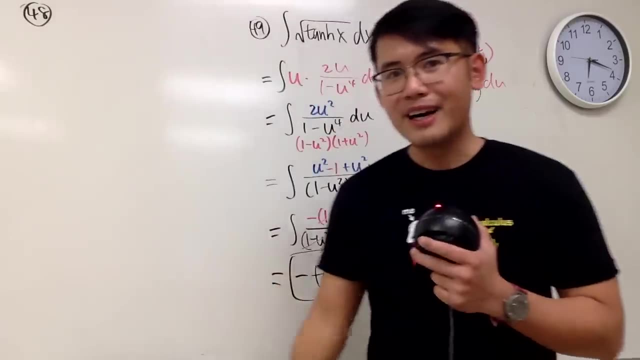 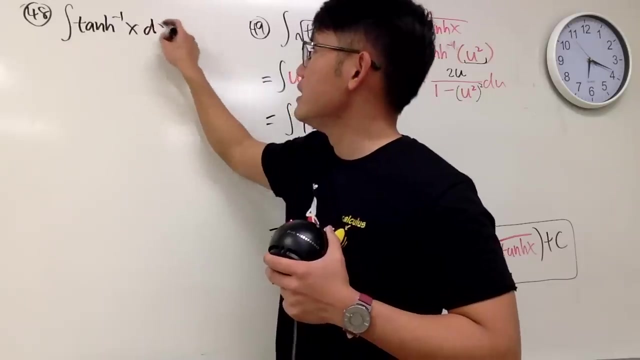 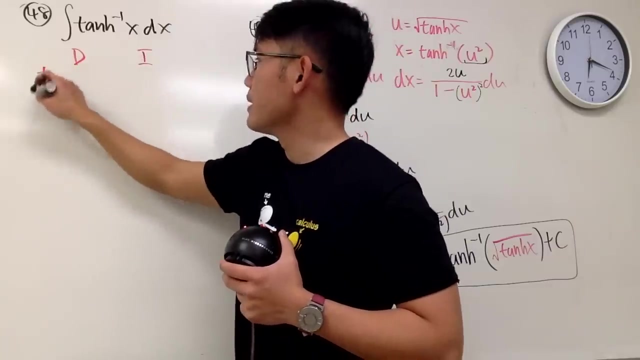 Okay, Here is the deal Number 49. I mean 48. You can travel back in time integrating inverse hyperbolic tangent of x, dx, Integration by parts in action. So d and then i, which is put on plus minus differentiating. 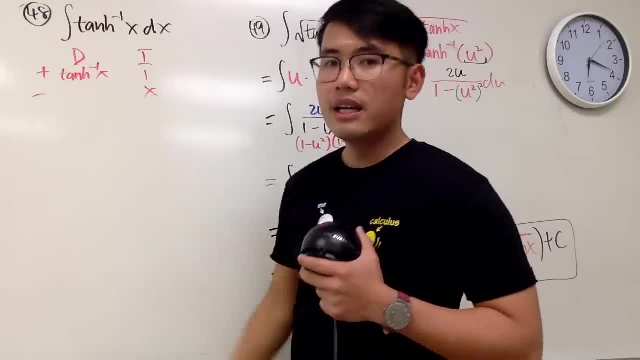 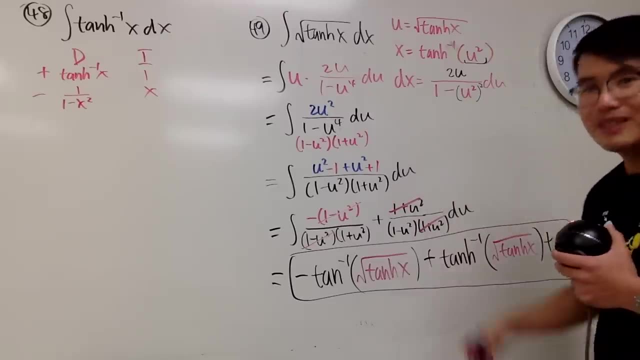 the inverse hyperbolic tangent and then integrating 1, which you get x, And then when you do this, you get 1 over 1 minus x squared. I meant to show you guys this first so I can talk about this much better. but like no, You guys can handle this right. 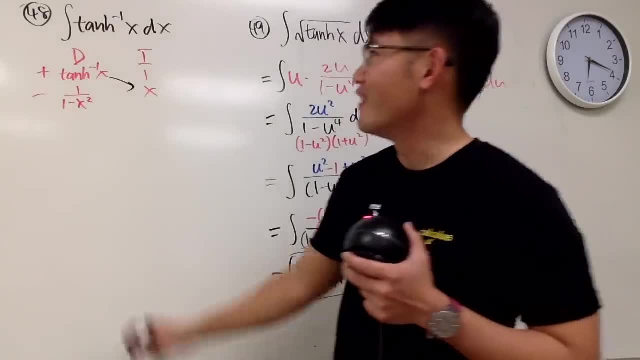 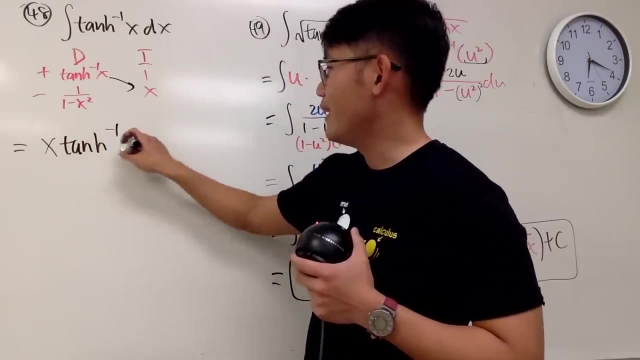 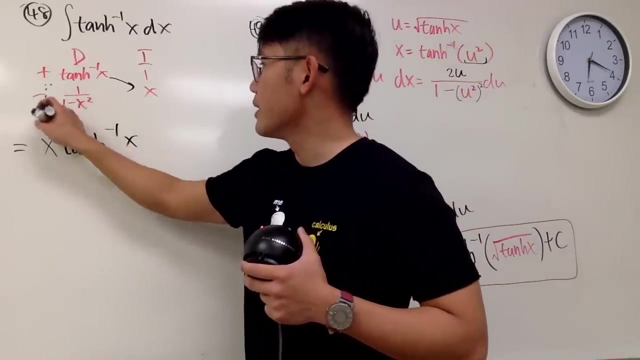 Anyway, this times the first part of our answer. Very nice, So you get x times the inverse hyperbolic tangent of x, like this: Next you are going to be subtracting and you have to do the integral of this right. So multiply this. 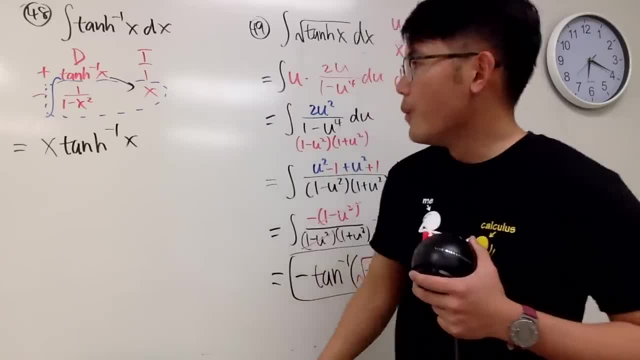 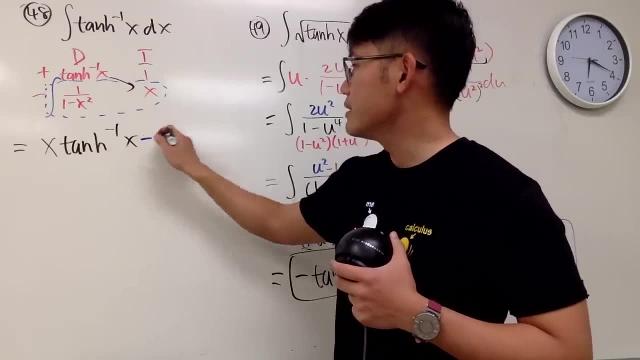 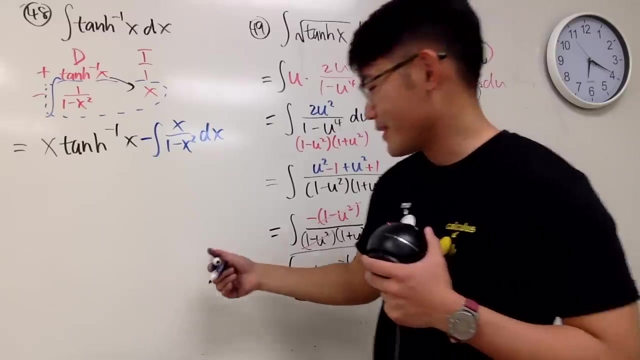 Don't forget the integral x over that. Well, let me just put this down in blue for you guys, Just to make it clear. We have to minus the integral of x over 1, minus x squared dx. But I will do the u sub in our head, right, So I will put down. 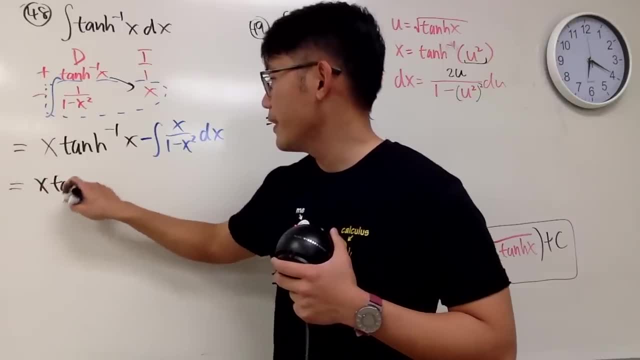 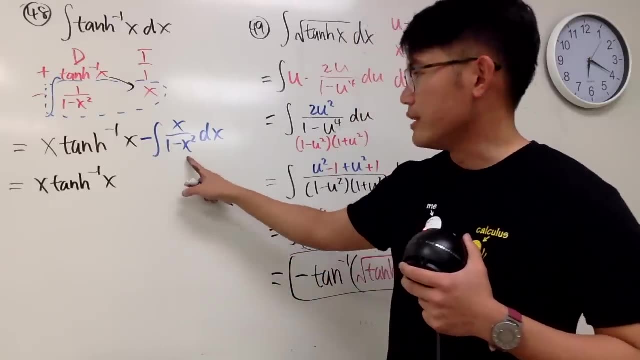 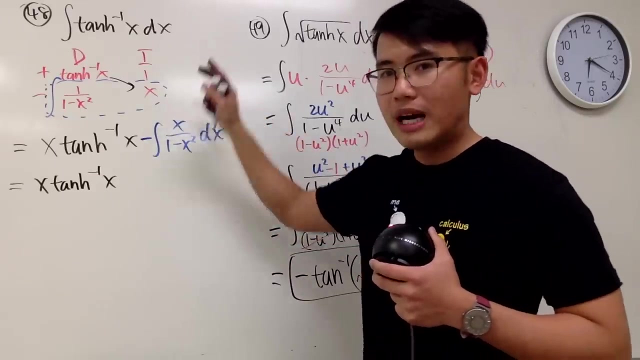 the part in black. first the first part, Again x, inverse hyperbolic tangent of x. This part, you let u equal to the denominator and when you differentiate that you get negative 2x And then of course dx and x will cancel. so you have the negative 1 half Negative times. 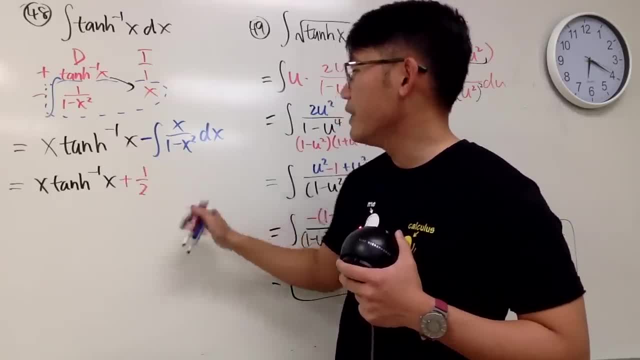 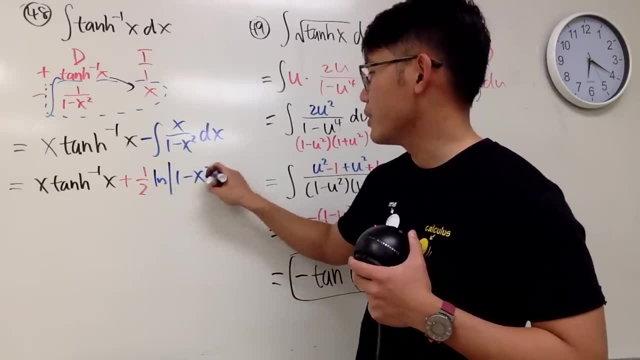 negative becomes positive, so you have plus 1 half and you get a natural log situation. so you have natural log and this might be negative, so you have to put up the value at 1 minus x, squared like this. So that's pretty much the idea, and the deal is that if you differentiate, 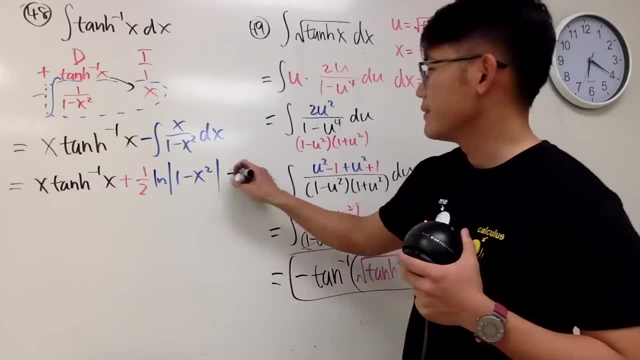 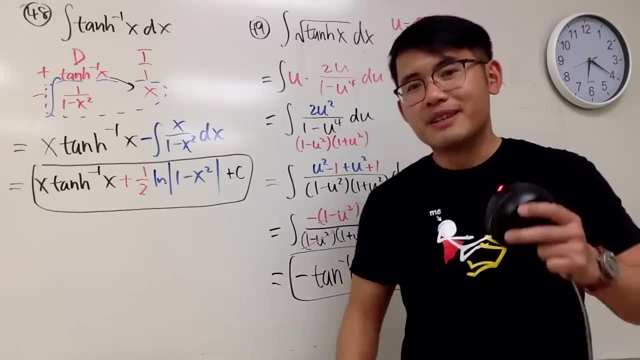 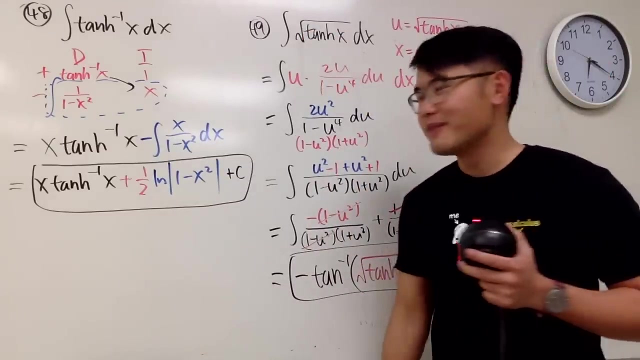 this. yes, you will get that, So I think that's clear. Plus C: Okay. Tiring This thing is heavy when you hold it for 3, like 2 hours and 15 minutes. That's my iPhone over there. 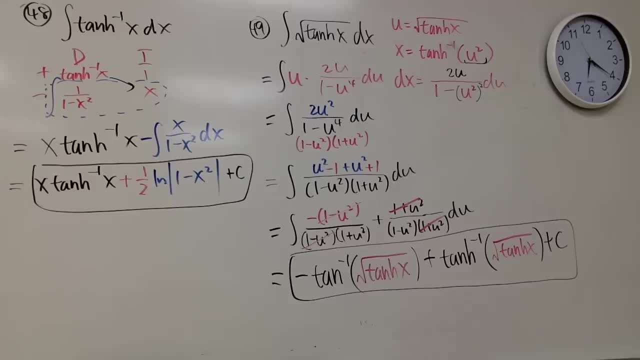 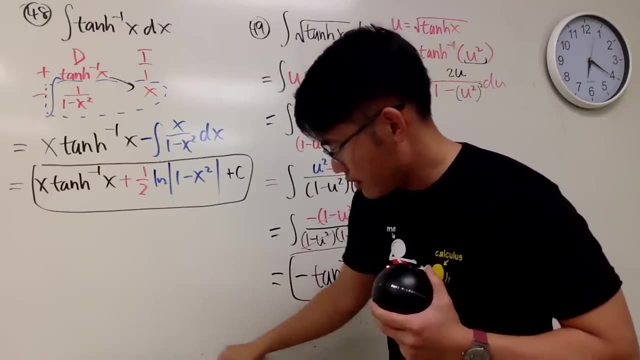 Let me take a look at my iPhone. It's still going strong, Very good, I like it. I'm also going strong as well. Hopefully that's the case. Alright, So 49. Now let me just erase both. 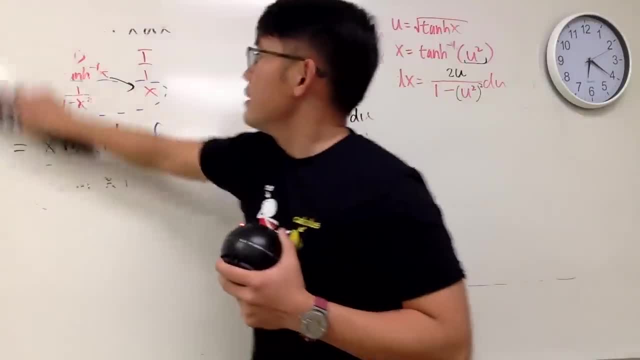 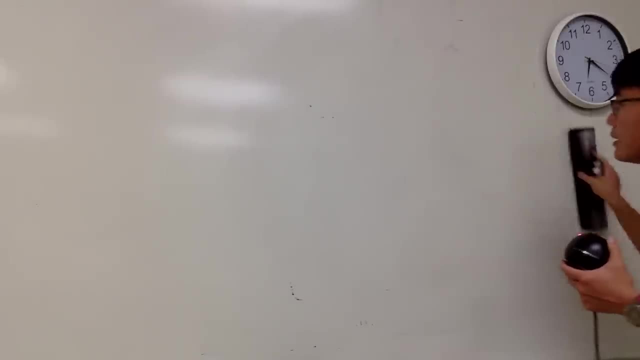 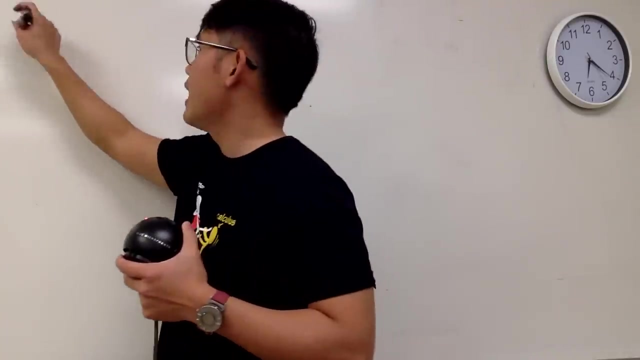 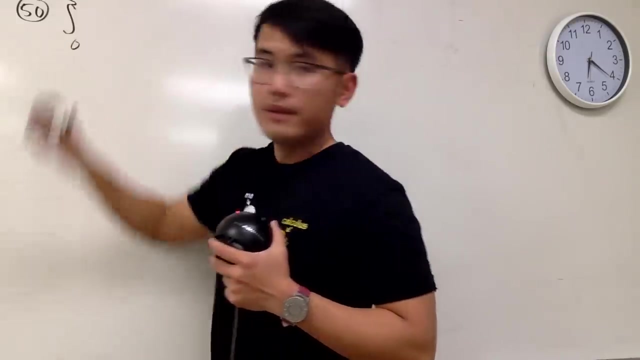 of them and we'll do 50, which is a very different style. question Number 50.. We're halfway done. Oh my god. Integral of I mean integral from 0 to 5.. Oh my god, man, Let me do it again: Integral from 0 to. 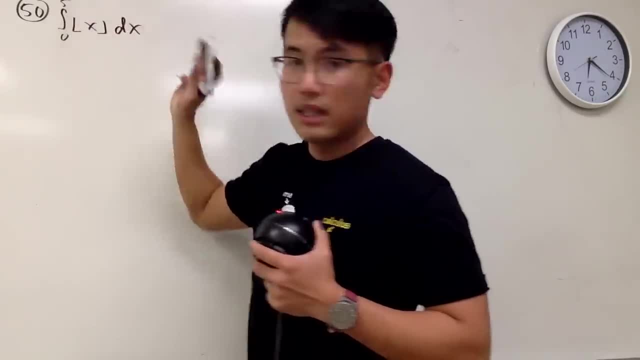 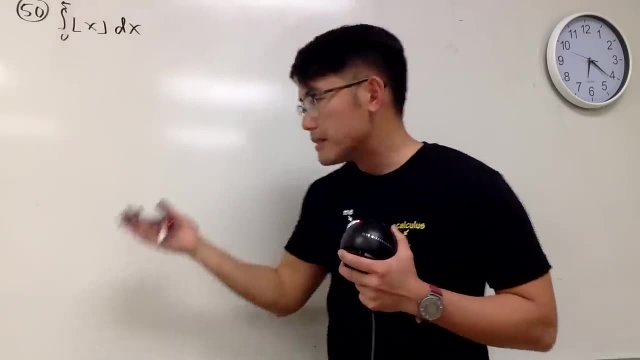 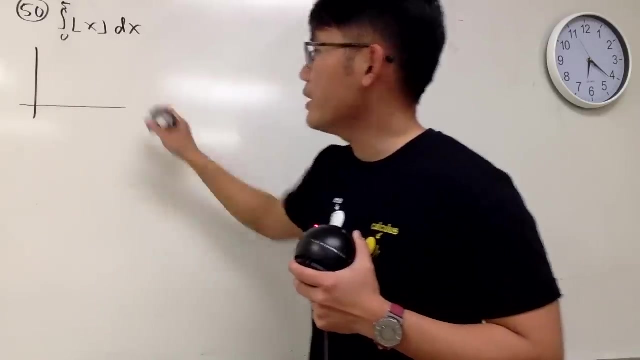 5 of the full function of x, dx, like that. This is the integral from 0 to 5.. Perhaps the best way to do this is to show you guys a graph of the full function. So to do so, I'll just show you guys this right here, real quick. The idea is that you're going to 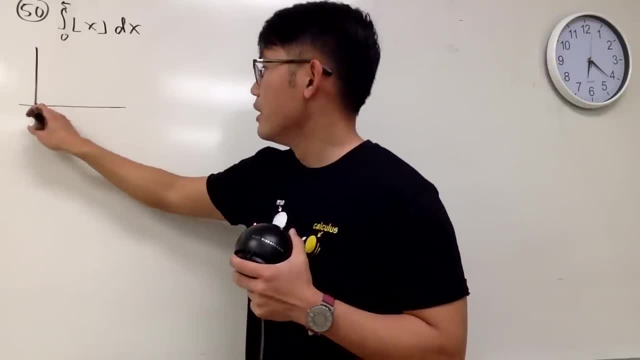 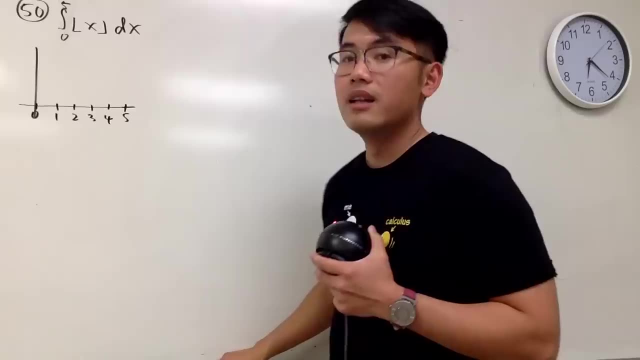 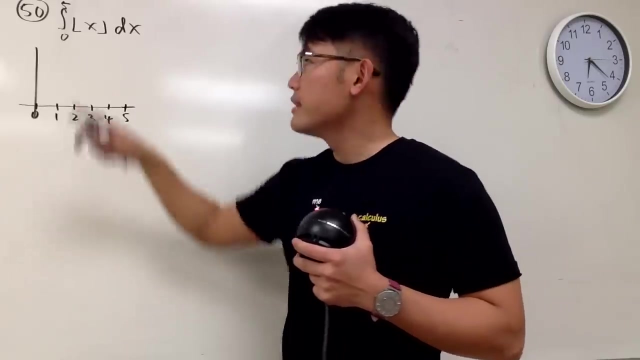 pay attention to the integer values, first starting at 0, and then you have, of course, 1,, 2,, 3,, 4, 5.. And here is the deal: When x is 0, full of 0 is 0.. When x is 0.1, it's still 0. 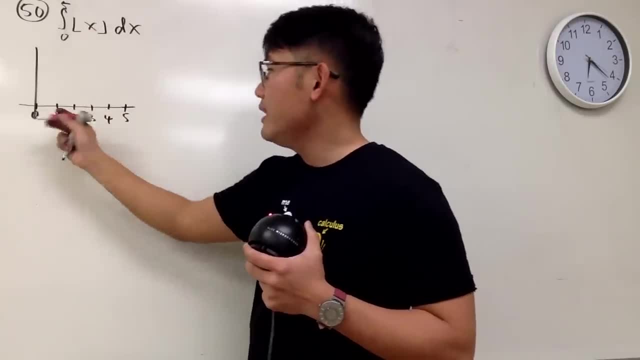 When x is 0.1, it's still 0.. When x is 0.1, it's still 0.1.. When x is 0.9, you still get 0.. Anywhere in between 0 and 1,. 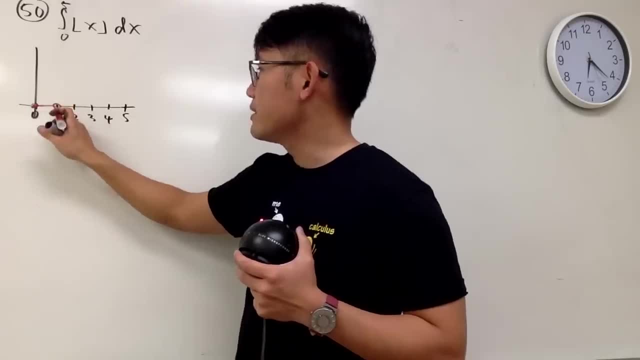 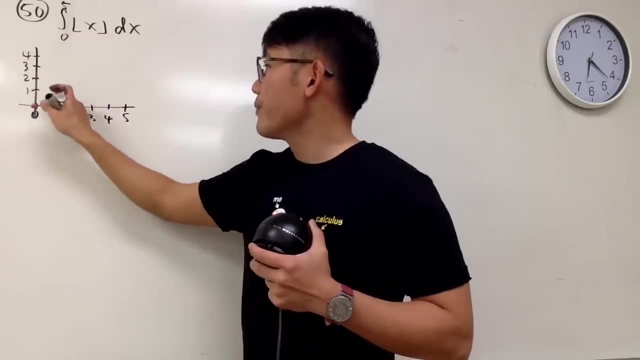 you get 0,, including 0,, but not including 1.. But when x is 1,, you get 1, so you have 1 right here. You're going to have some y values, So you are going to get. 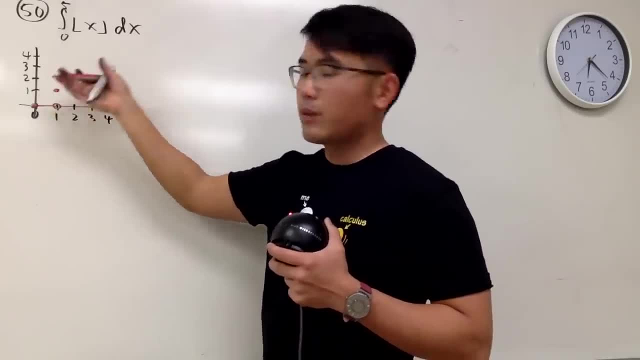 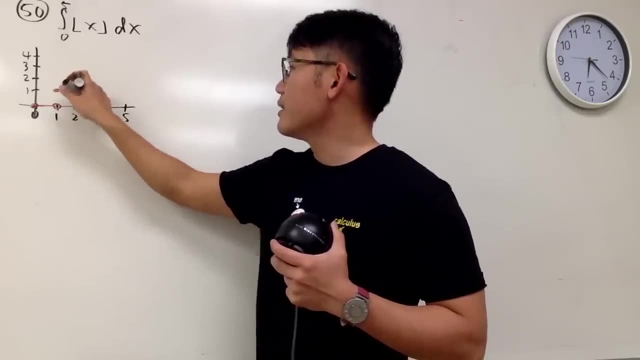 a bunch of this. Likewise, when x is at 1.7, you still get 1.. So it's going to be a straight line up to 2, and then when x is 2, you have a solid circle there, and then you pretty much do all this. 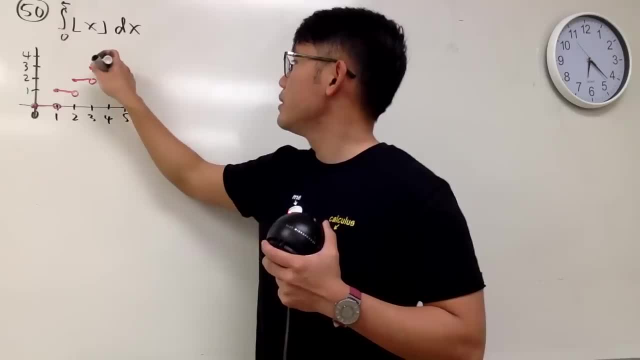 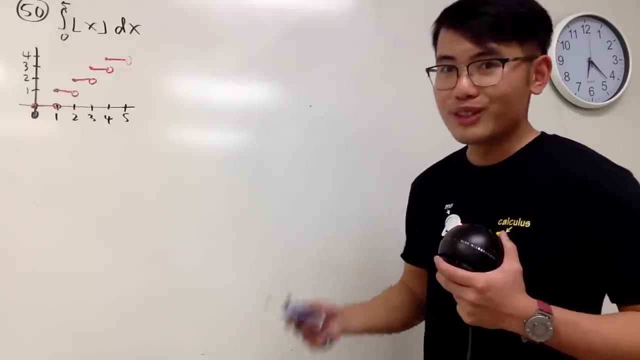 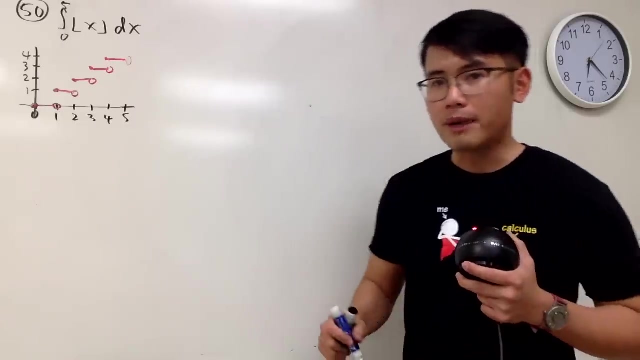 Jump, jump, jump. It's like playing Super Mario and you stop right there. Well, for this, right here, we can just find the area under the curve, Although it's not continuous, but we're not using the fundamental theorem of calculus, part 2.. We're just finding the area under the curve. 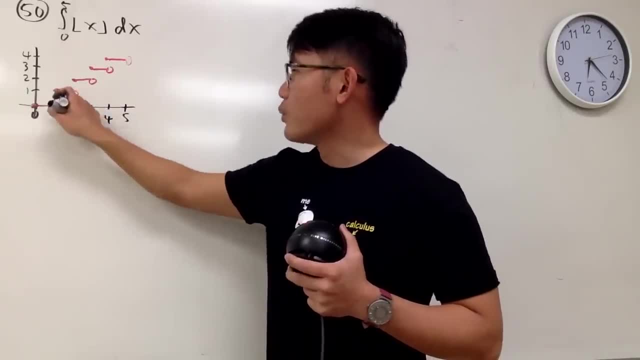 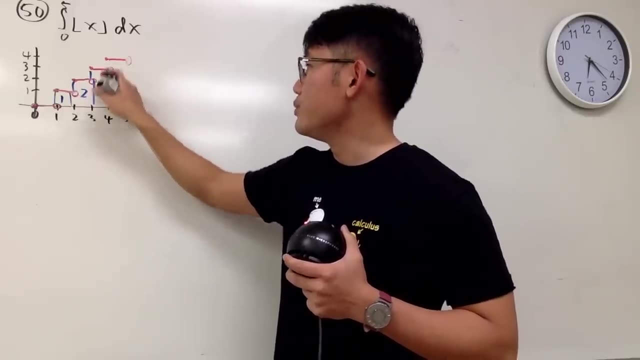 Alright, so the base right here is 1 times the height is 1,, so this is 1, and then this right here is 1 times 2.. The rectangle here is 2,, the area is 2, and then 3,. 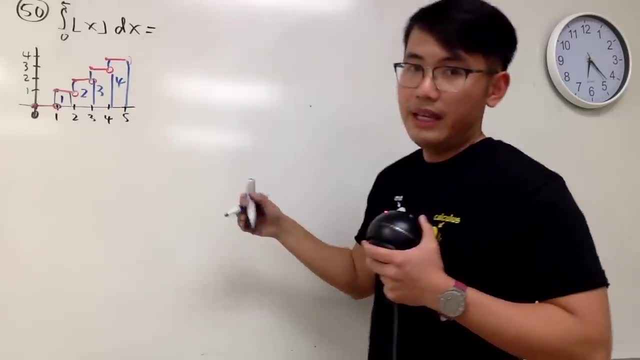 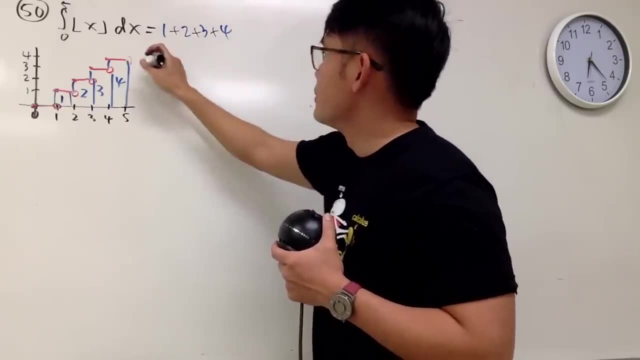 and then 4.. In the end, the answer to this right here is- just let me write it down- 1 plus 2 plus 3 plus 4.. And I'm going to do this one carefully. I believe the answer is 10.. If I add this: 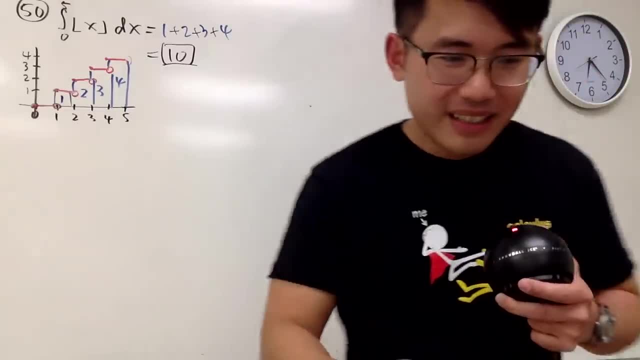 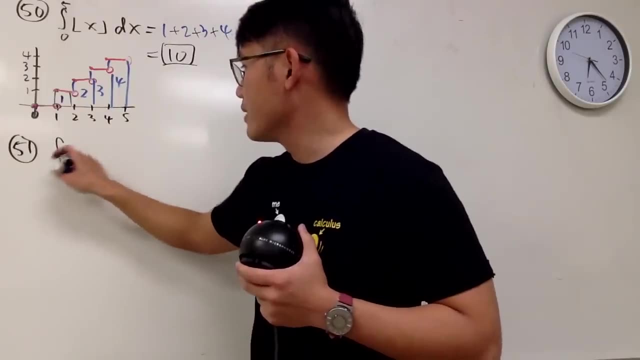 one wrong. it's going to be bad, but I think the answer is 10.. Okay, let's see. Okay, next one: 51.. Getting back to the regular trig functions Secant to the sixth power of x, dx. 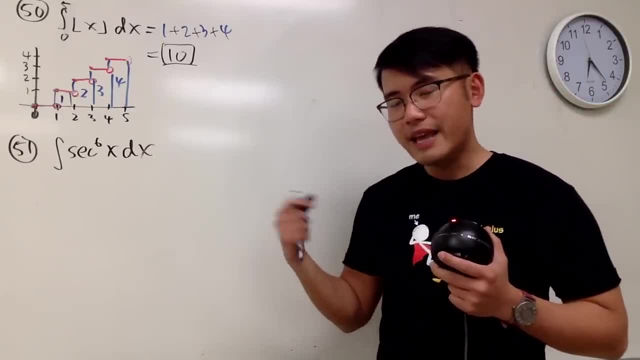 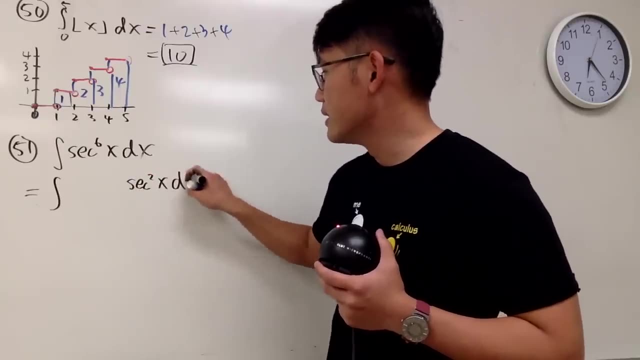 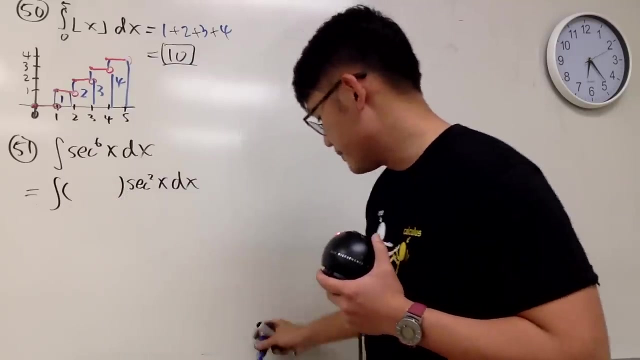 How do we do it? Take out two of the secants and then do some identity business. Very good, Integral secant squared x, dx. Inside here I will have secant to the fourth power. in another word, secant squared and squared. 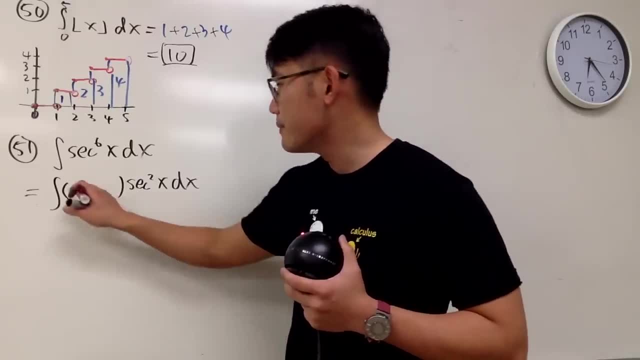 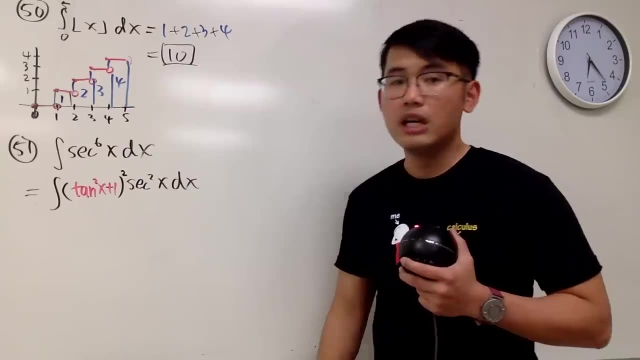 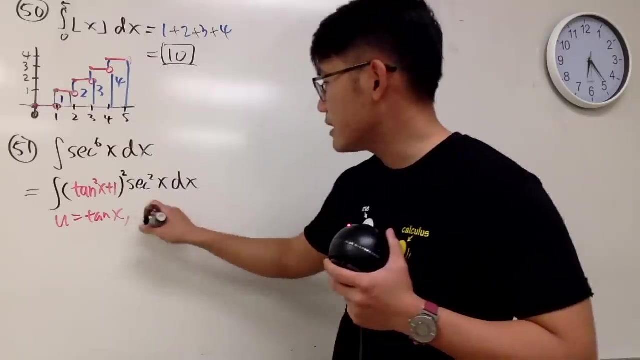 And the secant squared is the same as tangent squared x plus 1, and then you have to square that right. That's pretty much the idea. So you take a u sub that u equals tangent x, and then you get du equals. 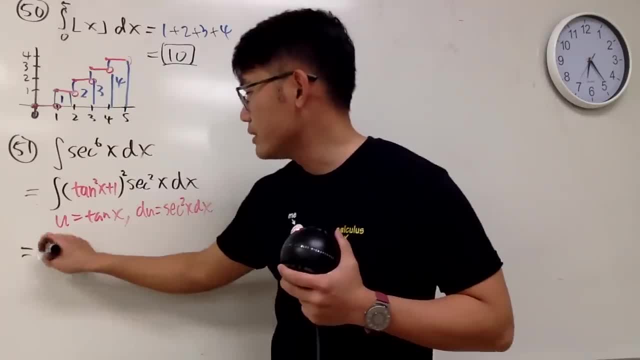 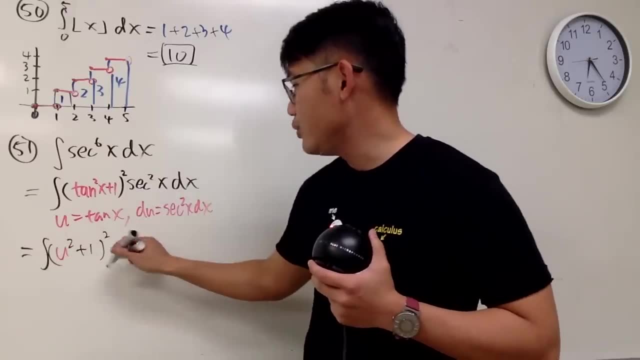 secant squared x, dx, and then you can take this to the u world. this is the integral of u squared plus 1, and then you square that and then you have the du on our side Like this. Very nice, Very nice. 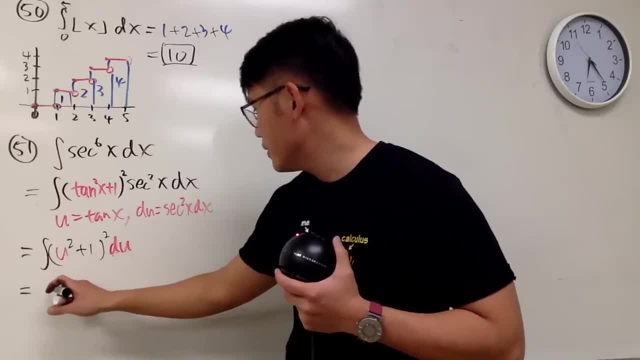 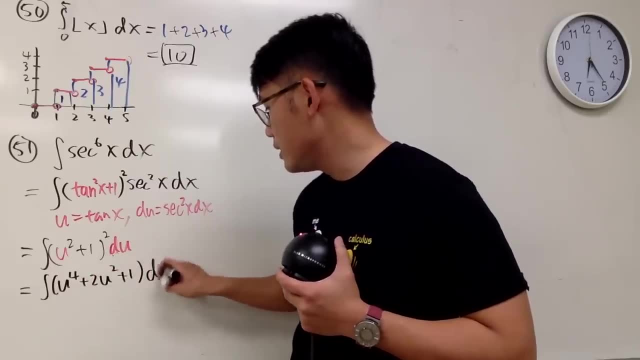 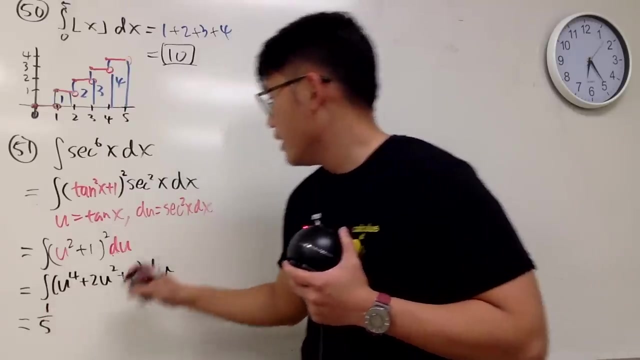 Alright, expand this real quick. You get u to the? u to the fourth power, plus 2u squared plus 1 du, and then, lastly, we are just going to integrate this and put back the answer. You get 1 over 5.. u is tangent, so you have. 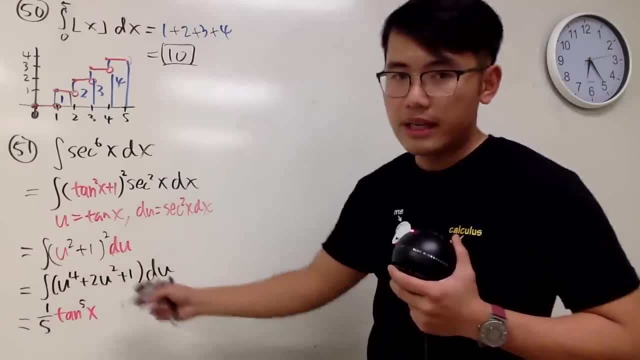 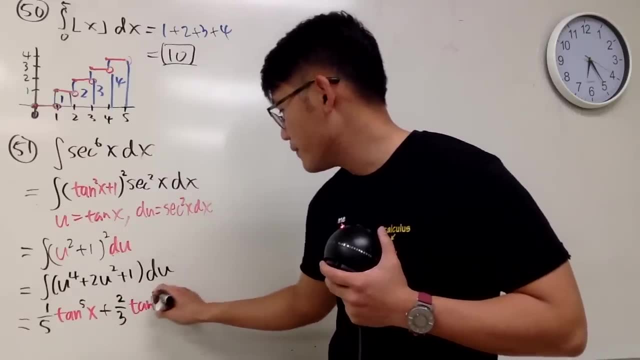 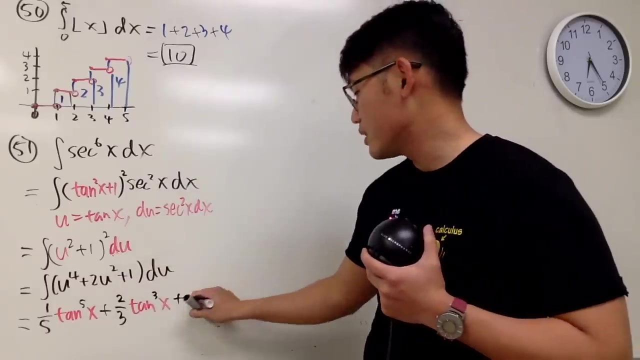 tangent to the 5th power, right here x, And then integrate the next term, we have plus 2, third tangent of, or to the third power of x, and then plus u, u, which is tangent x And plus. 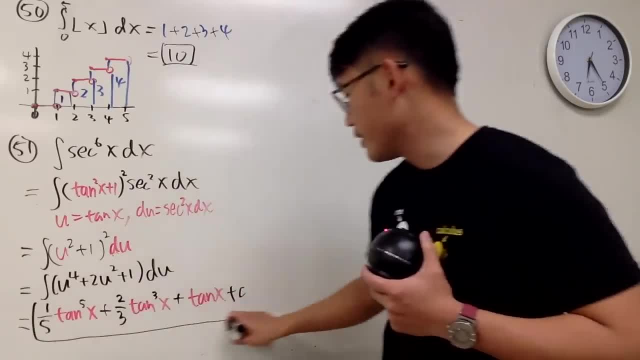 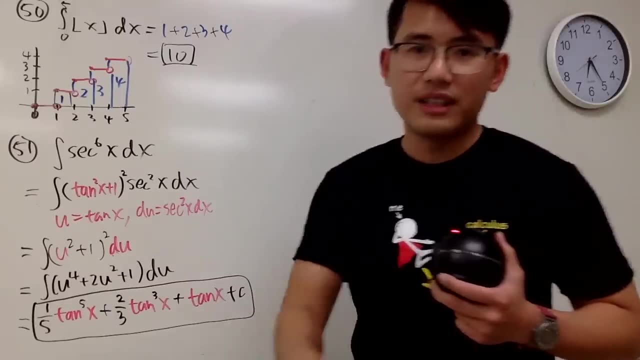 u, and then that's tangent and you're done Plus c. So this right here is it Right. See, after 51 integrals, this right here seems pretty nice and easy, so that's it Okay. now 52.. Let's see. 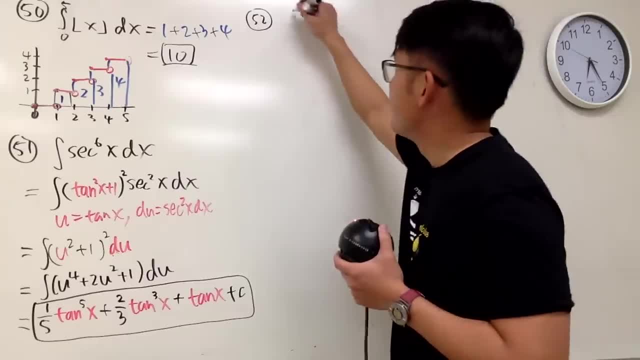 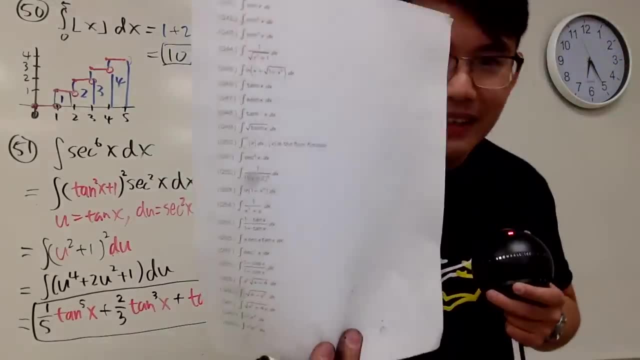 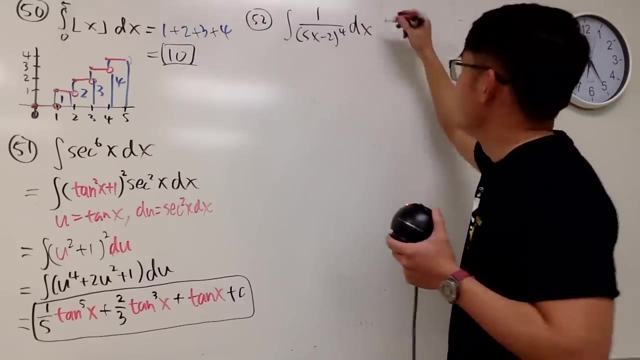 Alright, integrating 1 over parentheses, 5x minus 2 to the fourth power. That's it right. That's it Again. do not have the natural law of addition. This right here. you have this to the fourth power. Technically, you will do u sub, So you do u. 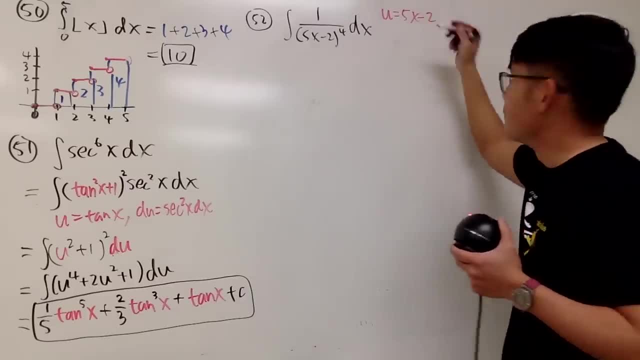 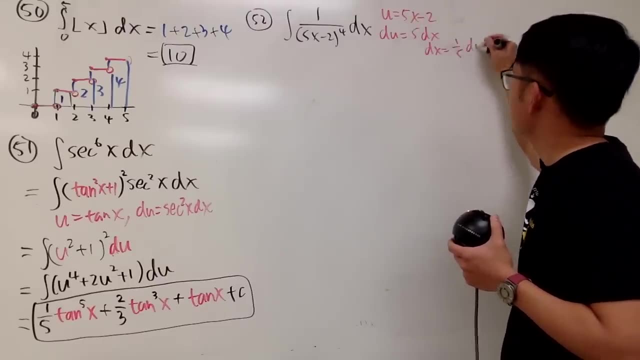 equal 5x minus 2.. And then do the derivative real quick. The? u will be 5 dx. dx is 1 over 5 du, So take this to a u-world. This is going to be the integral of 1 over u. 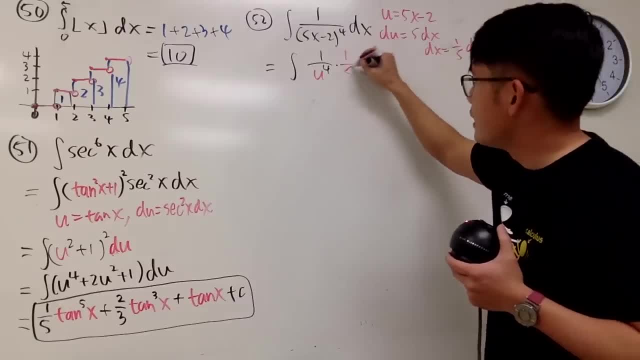 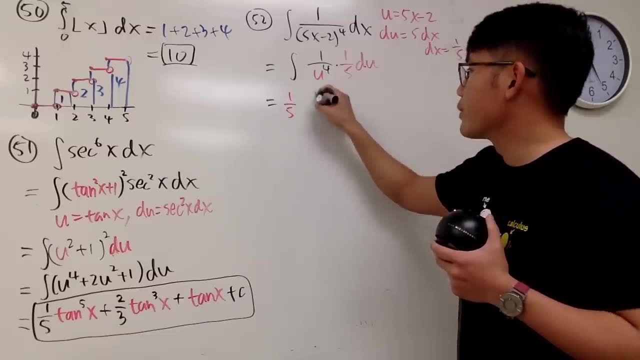 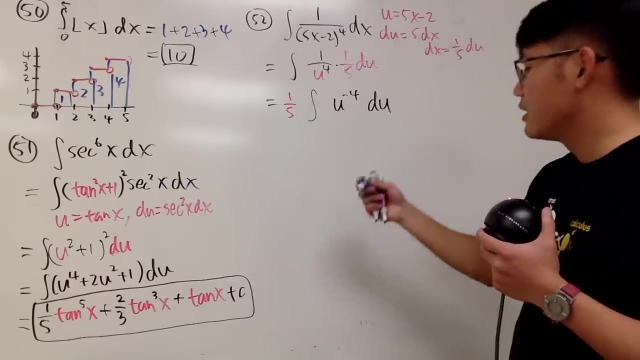 to the fourth times 1 over 5 du. So now we are integrating 1 over 5 in the front, Integrating, and this is u to the negative 4 du And with that said we can say we can just add 1 to the power which. 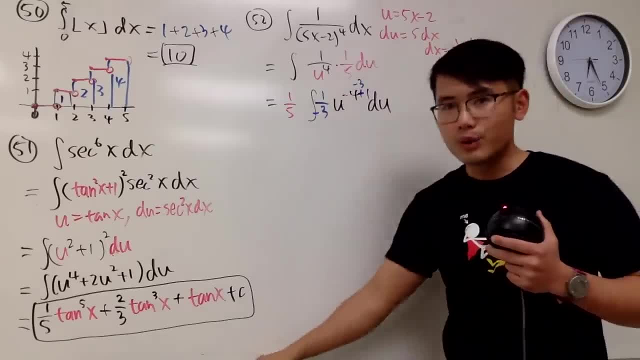 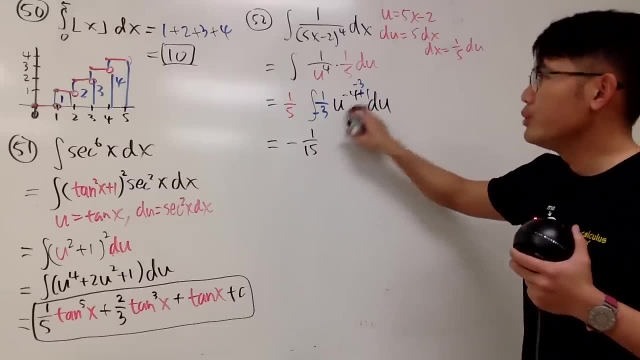 is going to give us negative 3, and then divide it by that new power. So we have that. So all in all we have negative 1 over 15, and then we have u to the negative 3 power. We can bring that down to the denominator This: 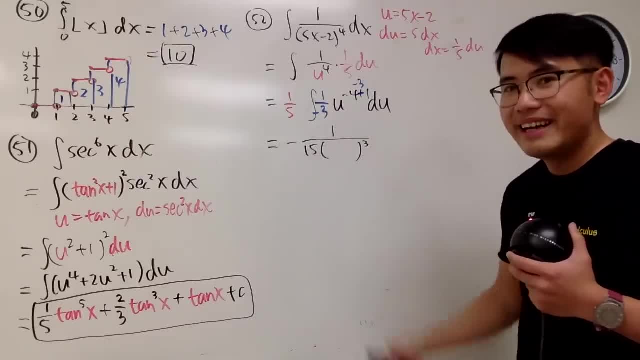 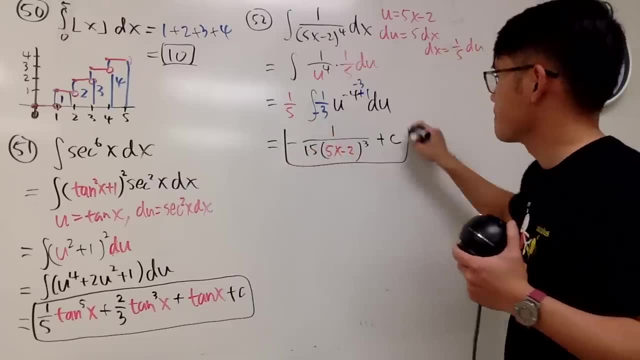 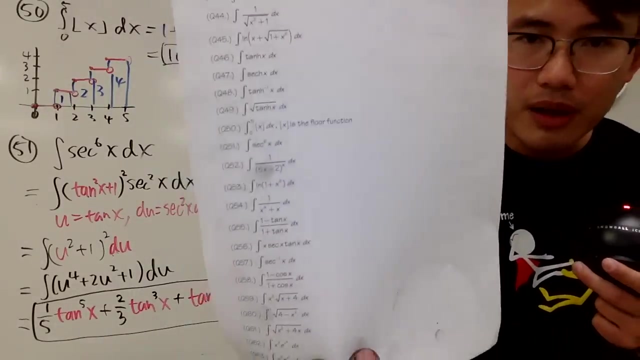 to the third power. Maybe put a 1 better. This should be u, And u is 5x minus 2.. And we are done, Plus c. Now next one. Integral of natural log of 53. Integral of natural log. 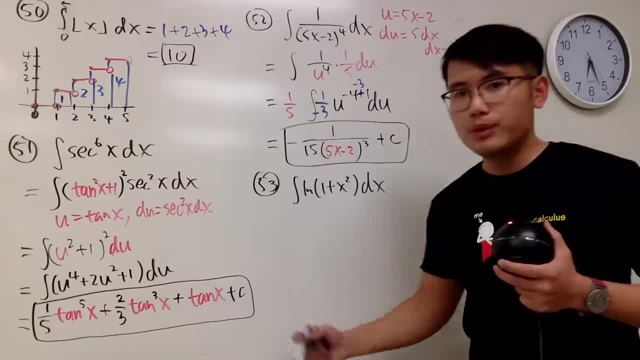 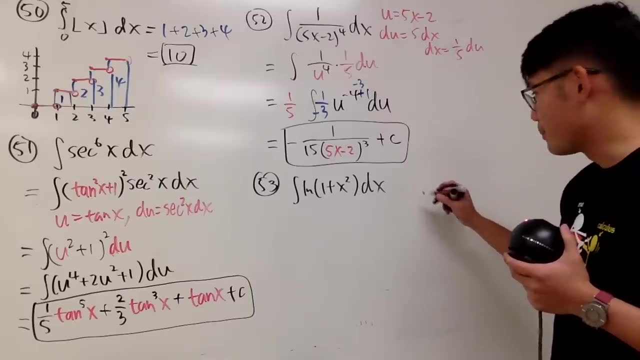 of 1 plus x squared dx. Can we do u sub? No, I don't have x in the front to help me out, But I will do the integration by parts. So d and then i Integrating just 1, and then. 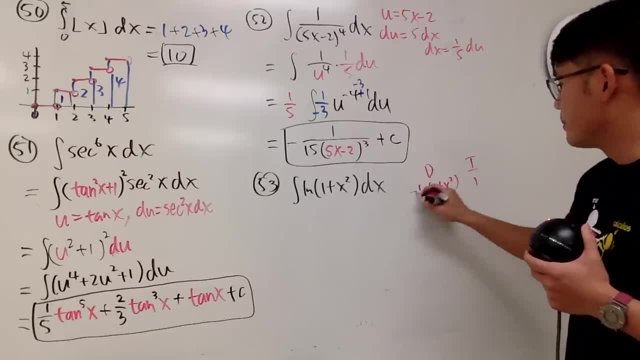 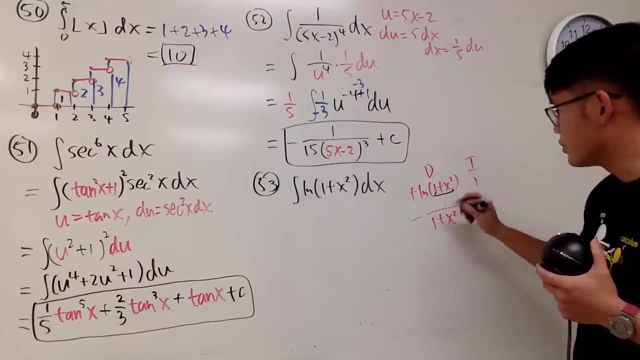 differentiating natural log of 1 plus x squared plus minus. Differentiating this, you get 1 plus x squared, and then you multiply by 2x And then, right here, you have the x. So here we go. 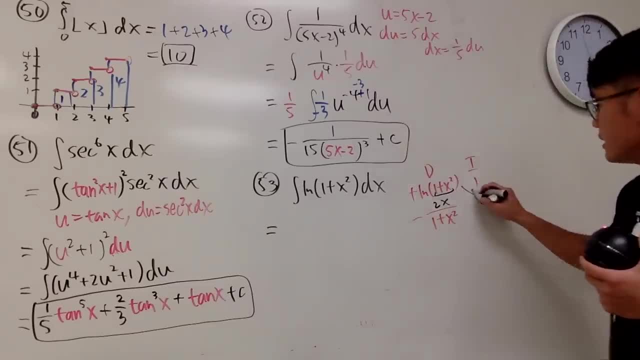 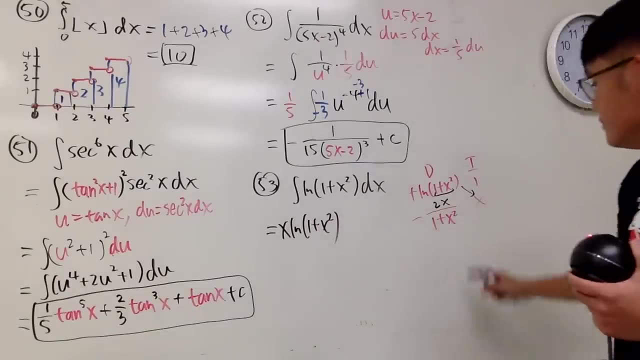 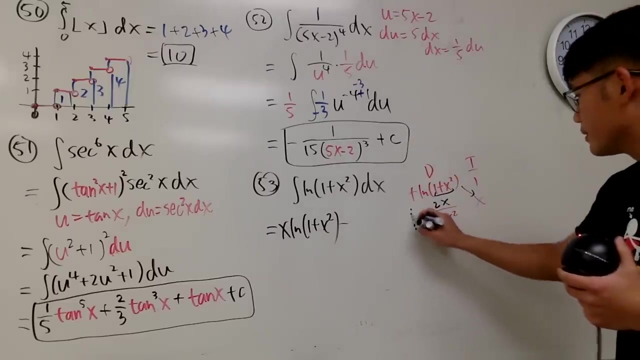 This right here gives us this times that. So we have x times natural log of 1 plus x squared. And then we have to integrate this guy which is minus, And let me put this down in blue: So minus the integral x times x is of course x squared. 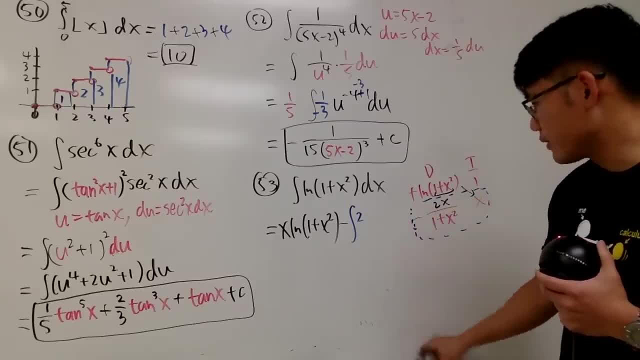 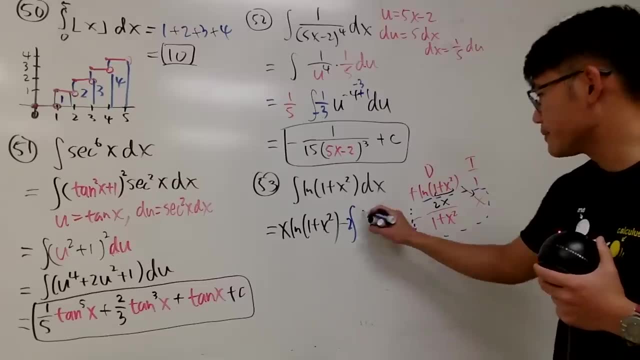 So we have 2x squared, And perhaps I will write this down right here for you guys. I will put a 2 in the front, 2 in the front And then the x squared over 1 plus x squared dx. 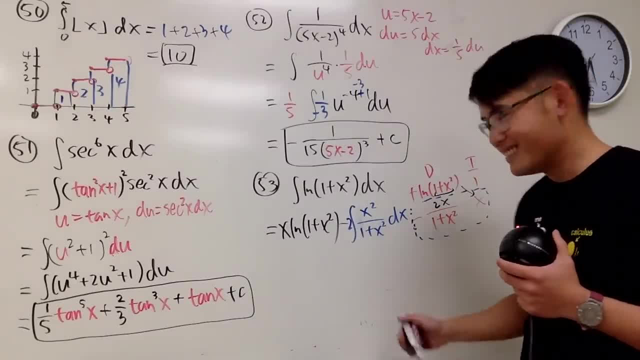 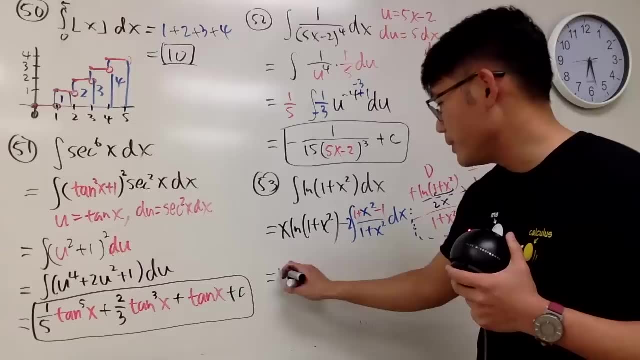 And what's this? Yes, this is one of my favorite integrals, So while I'm going to do this, I will just dump 1 plus here and a minus. Very nice, So in another way you will see this is going to be x. 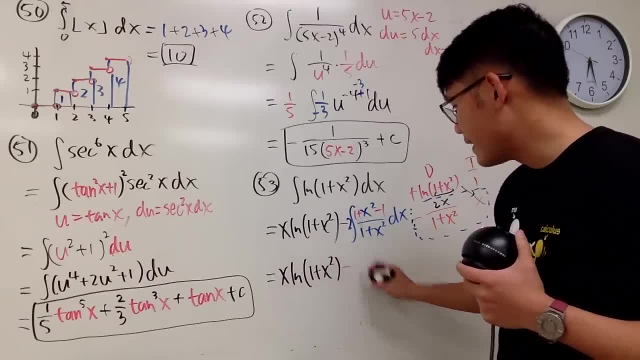 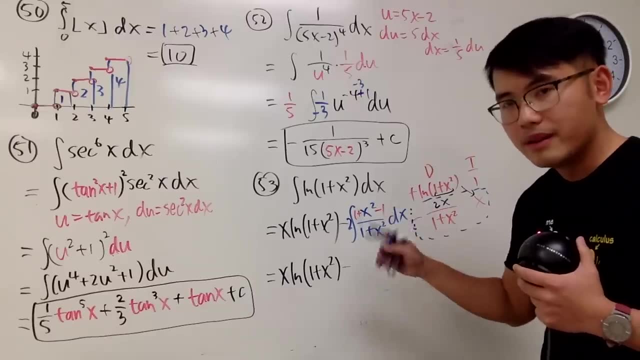 natural log of 1 plus x, squared minus. Alright, let's do the integrals first. yeah, Check this out. You pair this and that up, It's just 1.. Integrating 1 in the x world, you get x, And then. 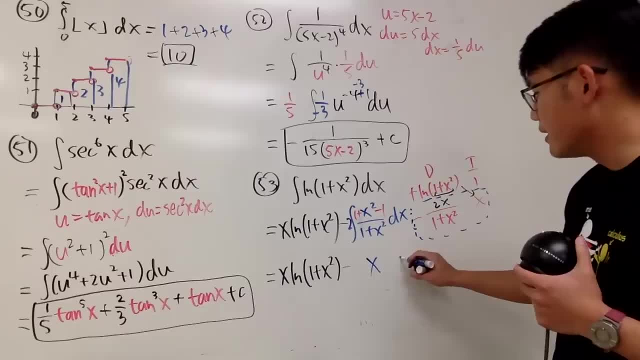 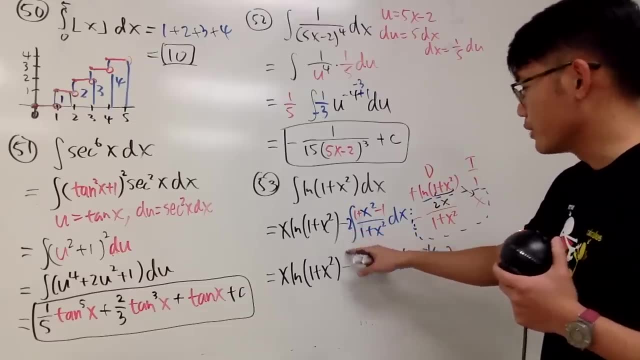 the next thing is 1 over that, which is going to give us inverse tangent, And this is the regular version. Well, don't forget, we still have the 2.. So you have to distribute it right here and then distribute it right here, And technically that was a negative 2.. So negative 2. 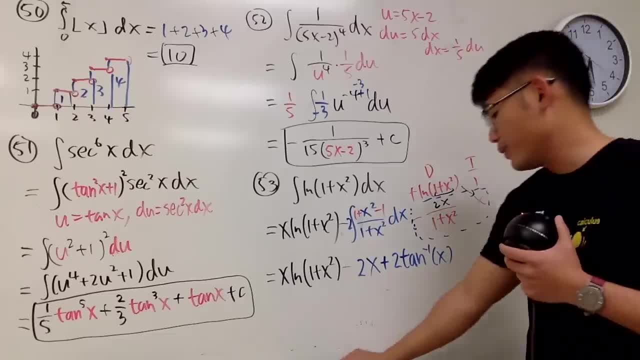 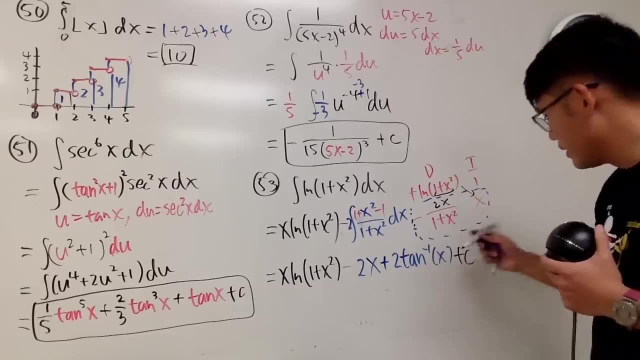 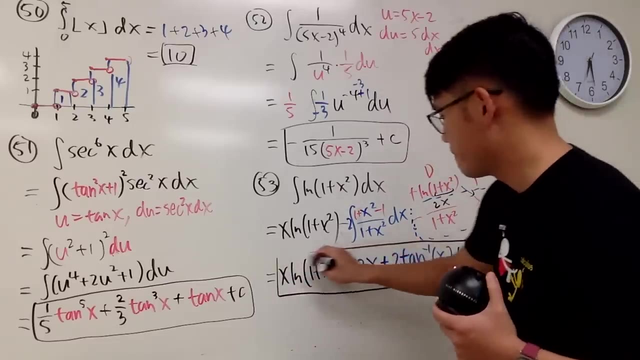 here, Negative, negative becomes plus. So with step set, we are done. We are done right here. Where is my? You see, it's only been a while and now it's like this dirty tooth. Oh my god, Let's see. 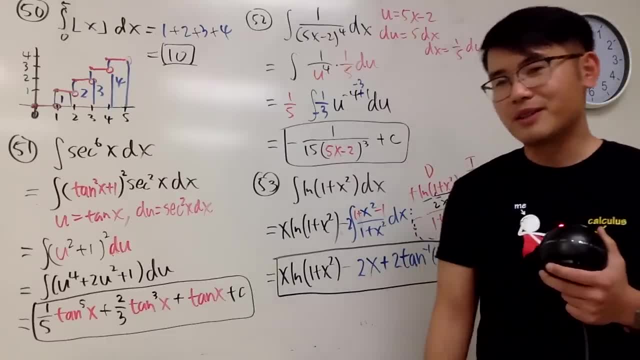 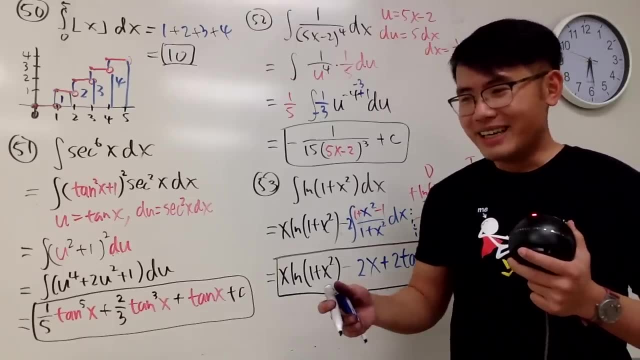 And if I make any mistakes, I don't know, I'm sorry. Maybe this- No, I shouldn't say this- It's going to be a remake, I don't know. And seriously, after I finish this, if you guys want to challenge, 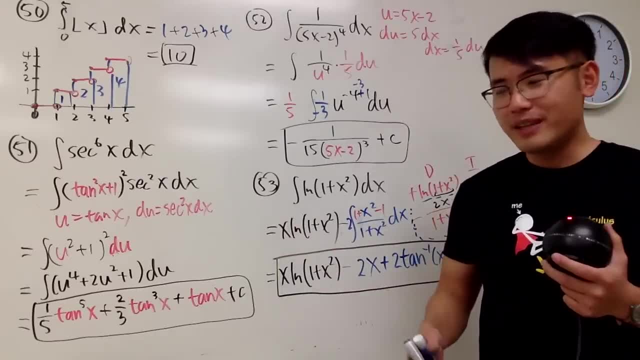 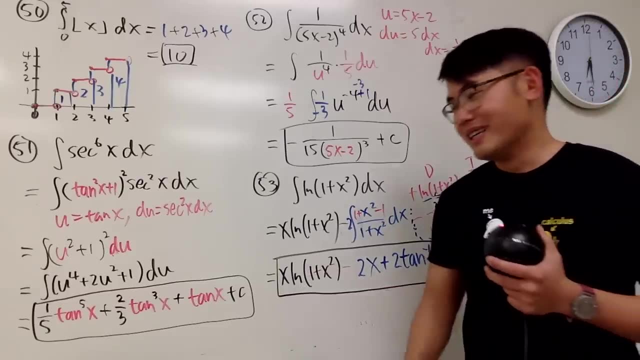 the record. go ahead and do so If you can do. let's say, 110 integrals in one video. guess what? I will do: 150 integrals to beat you. So that's not going to be healthy, So just. 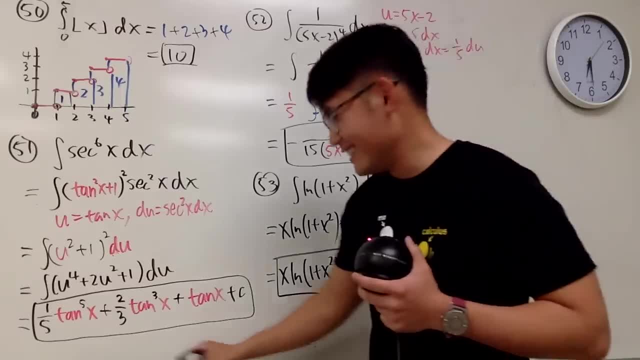 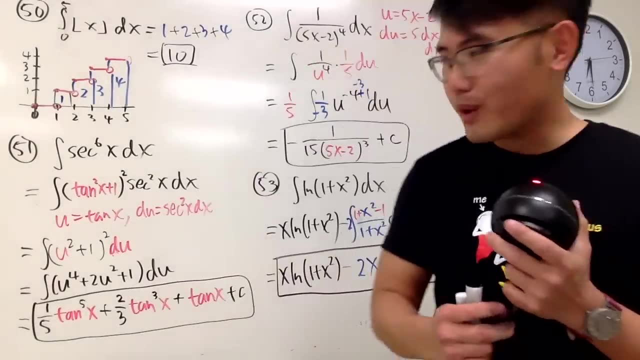 don't, don't, don't, don't, do it. Yeah, Alright, So that was number 53.. We have 47 more to go 3 hours Right. 47 more to go, So it's looking good. 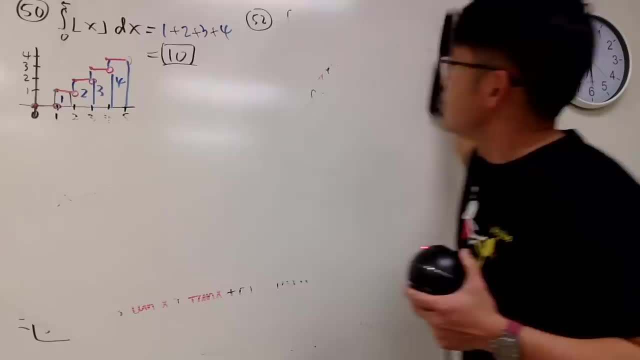 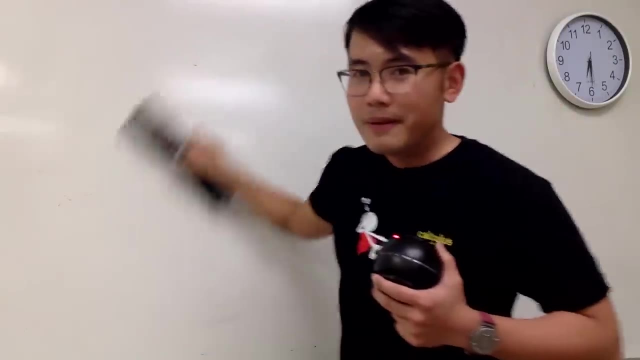 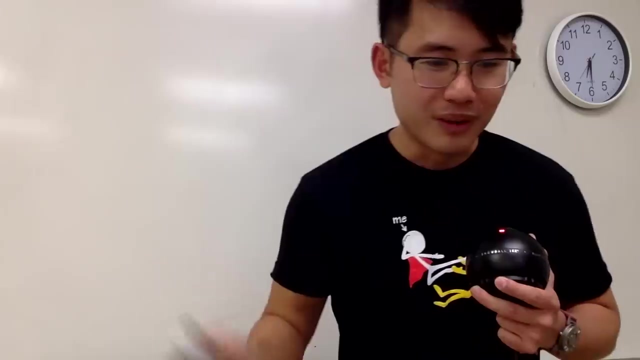 It's looking good. So how are you guys doing so far? Huh, I don't know what you guys are doing at the moment while you guys watch somebody integrating for like 5,, 6,, 7 hours. I don't know, Anyway, number. 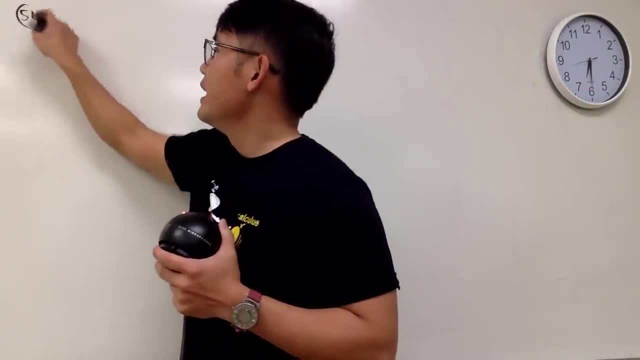 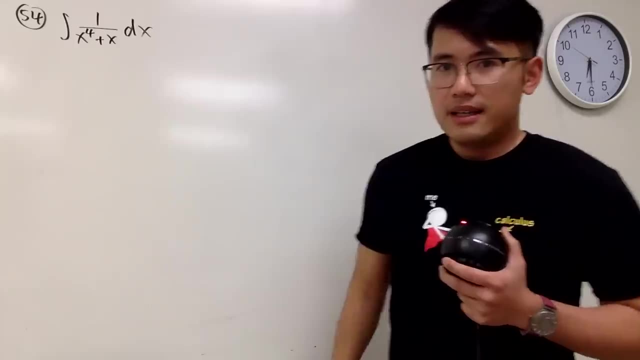 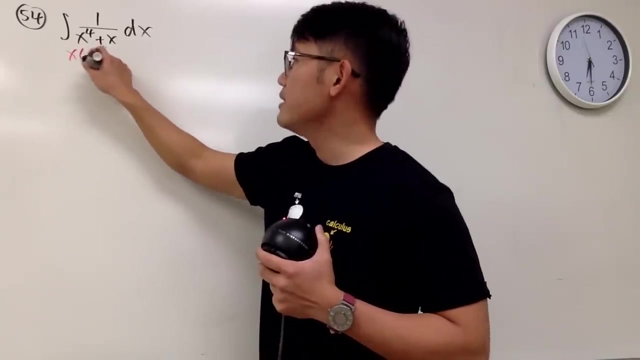 54. I already done right here for you guys. We are integrating 1 over x to the fourth power plus x to the x. Yes, We can factor things out. We can factor out an x Parenthesis, x cubed plus 1.. 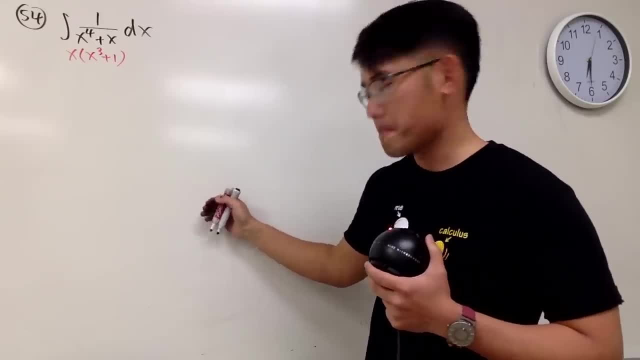 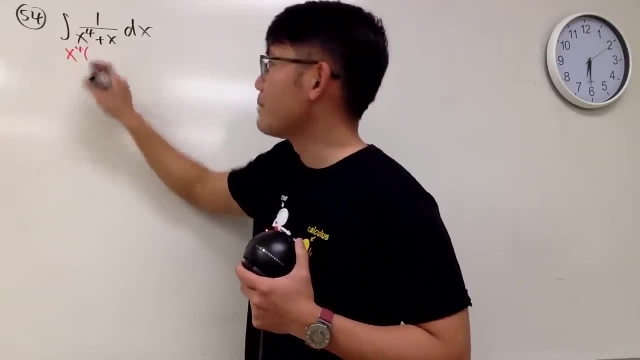 And you can actually factor more and you can do some partial fractions if you would like, But no, I'm not going to factor it this way. This is how I'll factor it: I will factor out an x to the fourth power And you'll see This right here will be 1.. And this right here will give us x. 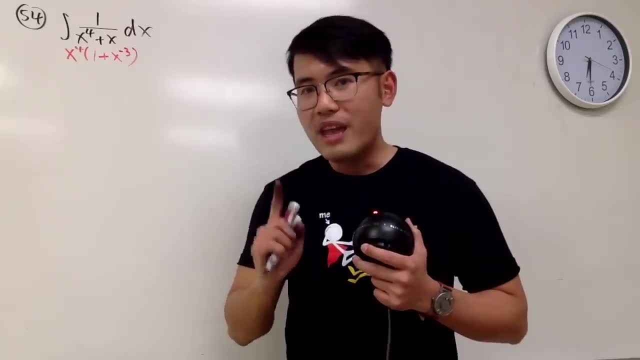 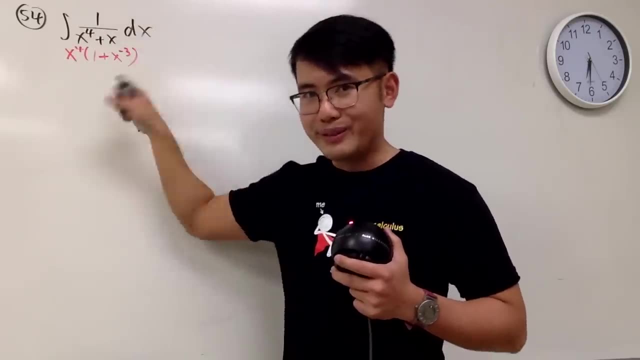 to the negative 3 power. Here's the deal: Whenever you have 1 over x to some power plus x, x to a whole number, power plus x, you can do this. It's going to be working out really nicely, Okay. So you see. 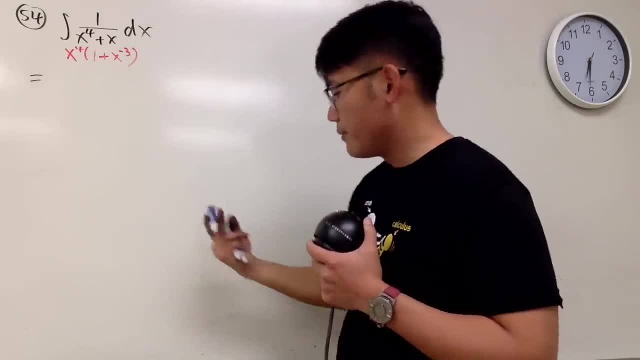 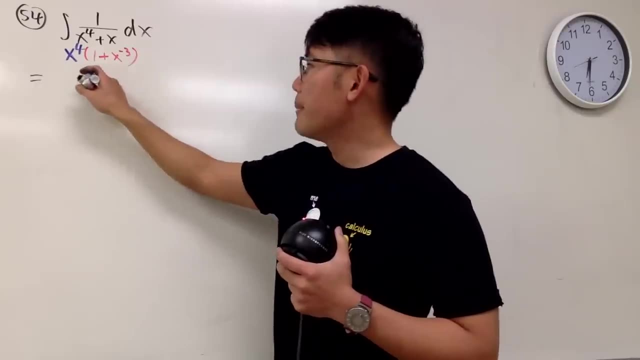 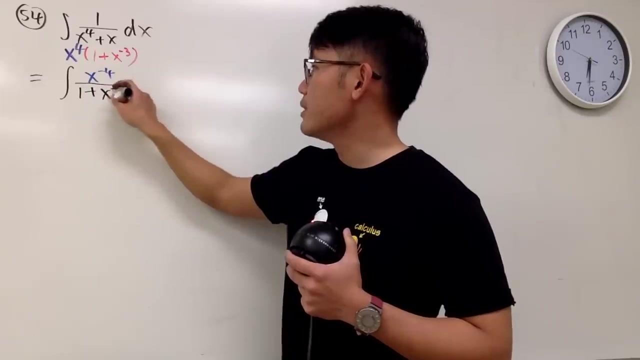 that. the idea is that this is equal to when you have x to the fourth power in the denominator, you can put that up as x to the negative 4. Isn't it? And then you have 1 plus x to the negative 3 power, And from: 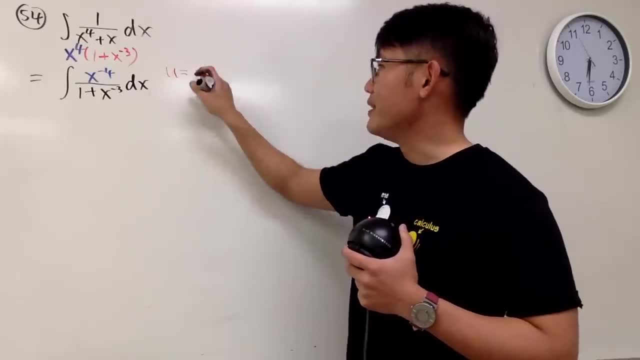 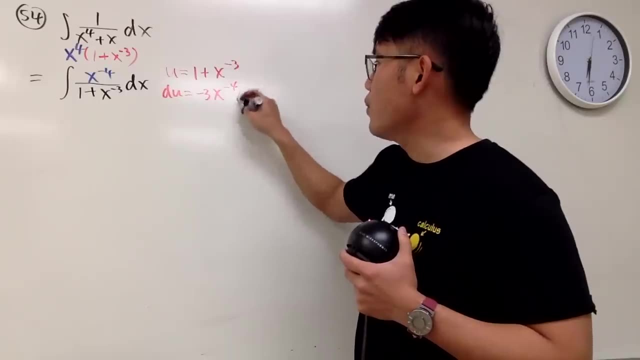 here we take a u-sub. Let u equal to the denominator 1 plus x to the negative 3.. du is equal to negative 3x to the negative 4 dx. Let me show you guys. a cancellation dx is equal to divide this. 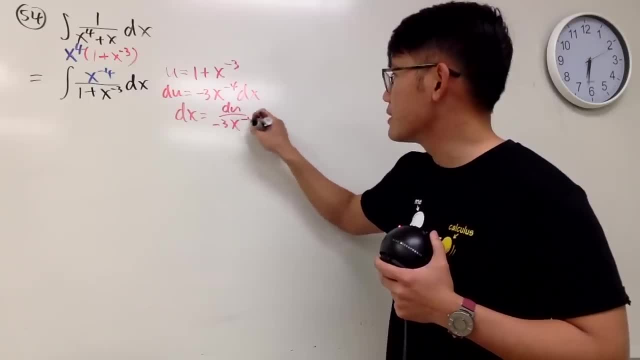 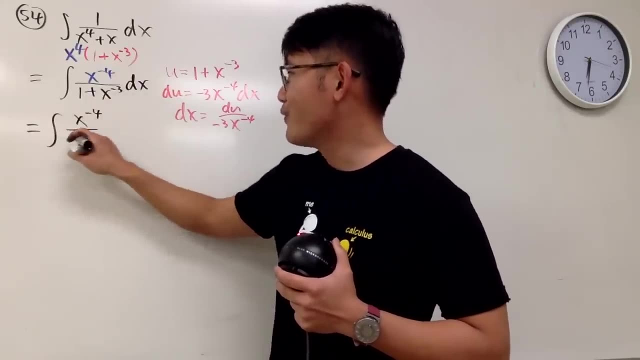 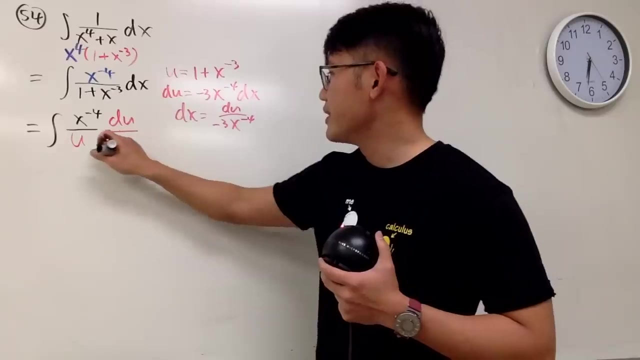 on both sides: du over negative, 3x to the negative, 4.. Now take this integral to the u-world. This right here is the integral of x to the negative, 4 over u. This is very nice, because dx is this: You have du over negative. 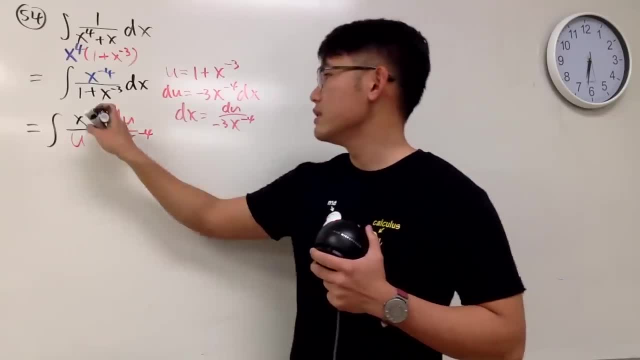 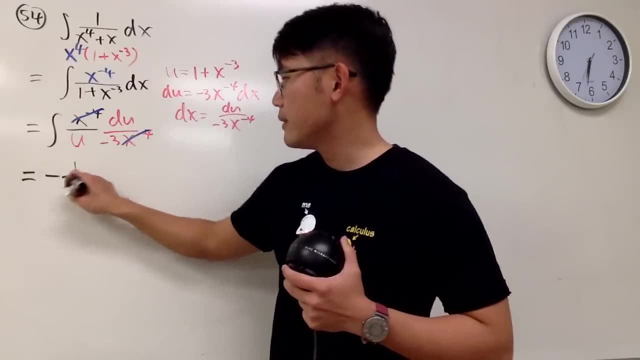 3x to the negative 4.. And guess what? Yes, This and that can be cancelled, And now you have negative 1 over 3. And then integrating 1 over u in the u-world. of course, that's natural log, absolute value. 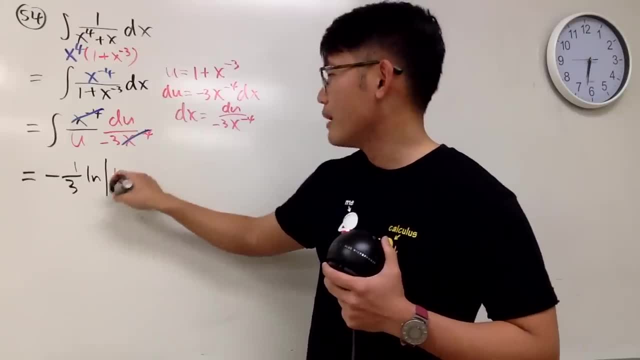 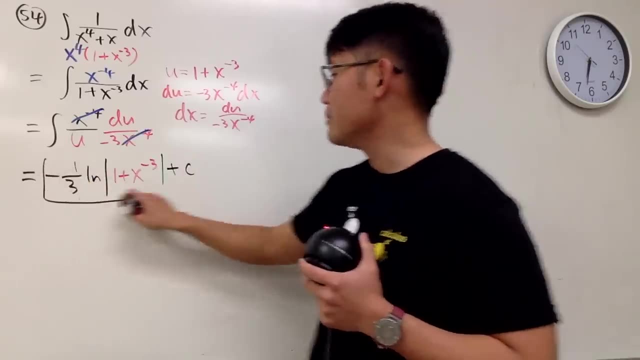 of u And u is this guy. Just write it down: 1 plus x to the negative 3 power And guess what We are done. You don't need to do partial fractions sometimes. When you have this situation, just go ahead and factor the. 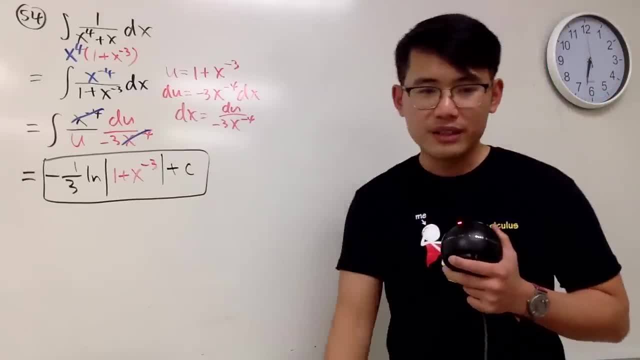 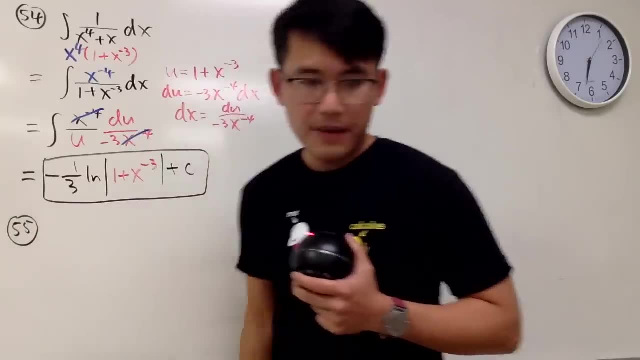 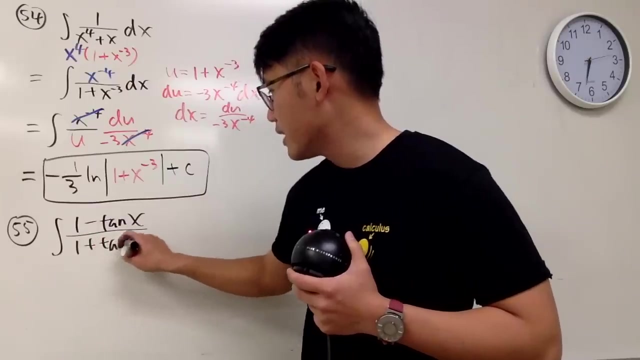 biggest power And this is going to work Very nice, Very nice, Very nice. In fact, we have seen a question like this earlier, So that was good. Number 55.. Integral of 1 minus tangent x over 1 plus tangent x, dx. 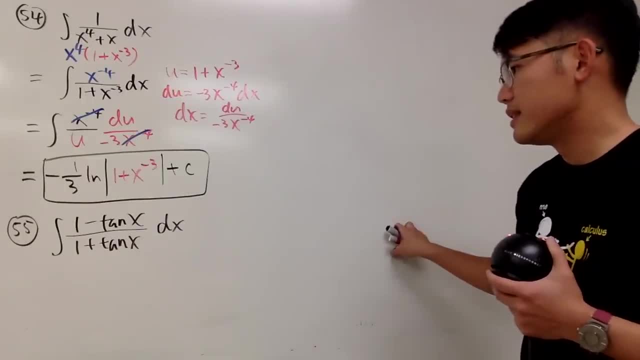 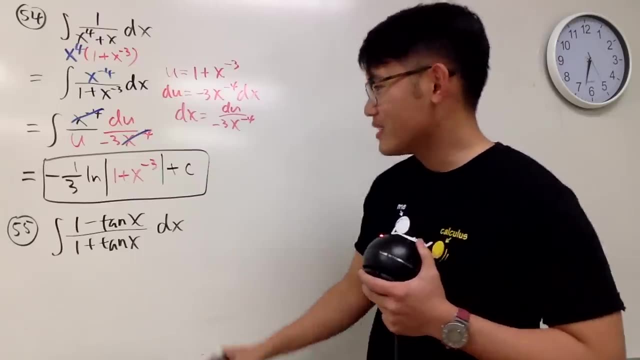 My god, Okay, No big deal. I don't like to work with too many tangents. in the integral We can look at the tangents as sine over cosine. So this is sine over cosine. Likewise, this is also sine over cosine. We can multiply the top and bottom by. 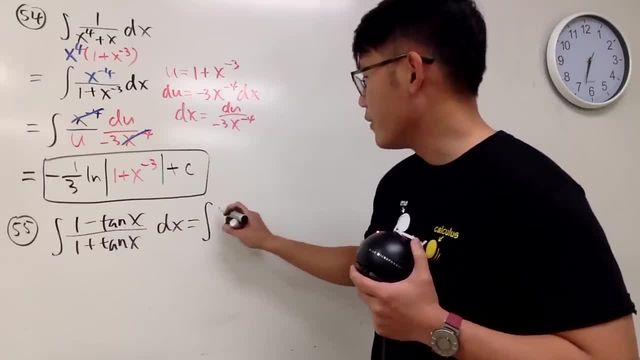 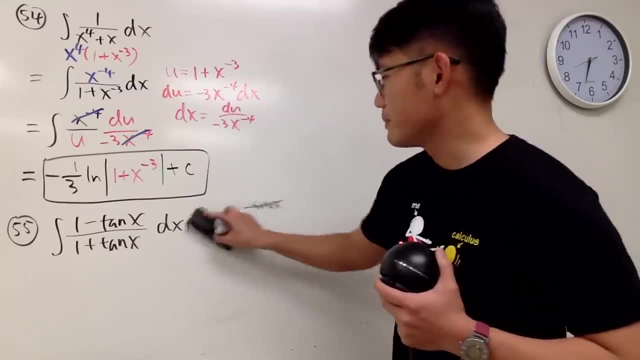 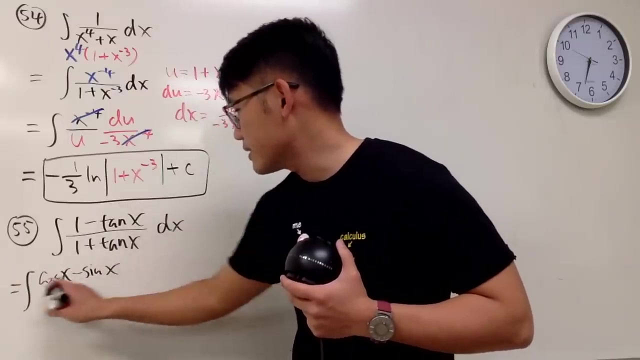 cosine In another word: this right here is the integral of cosine x minus sine x. Let me actually write it down over here We have space. This right here is the integral of cosine x minus sine x. over this right here is again cosine x plus sine. 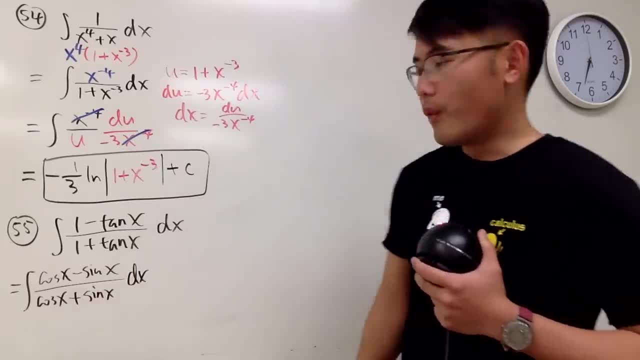 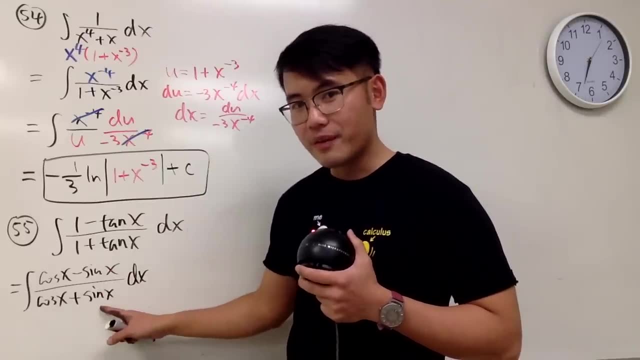 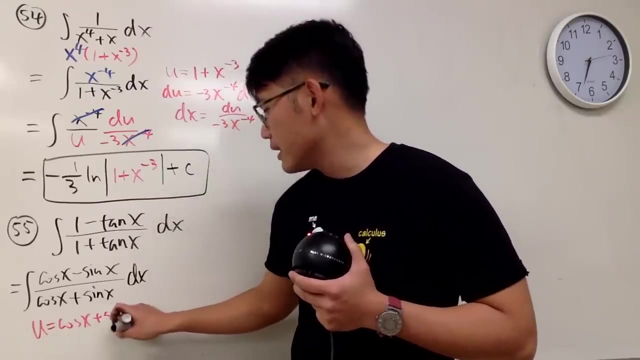 x- dx. Well, what's so good about this? Look what's the derivative of cosine Negative sine. What's the derivative of sine Positive cosine. So you can just take a? u and write it down u real quick You can say u is equal to cosine x plus. 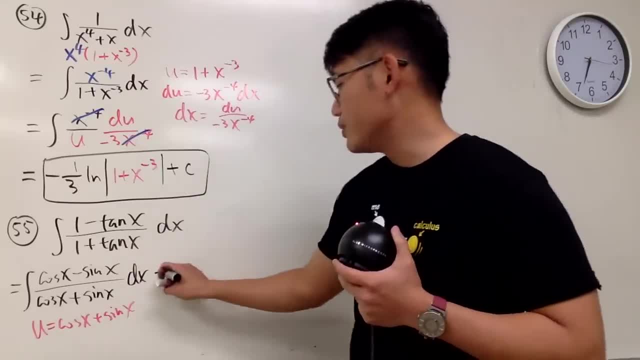 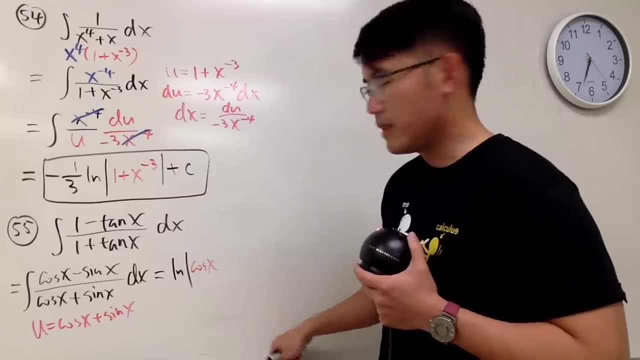 sine x, and then you can get the du. It's the top which is just going to give you natural, log, absolute value of the denominator, which is the cosine x plus sine x. Let me actually just write down the answer over here to save some space. 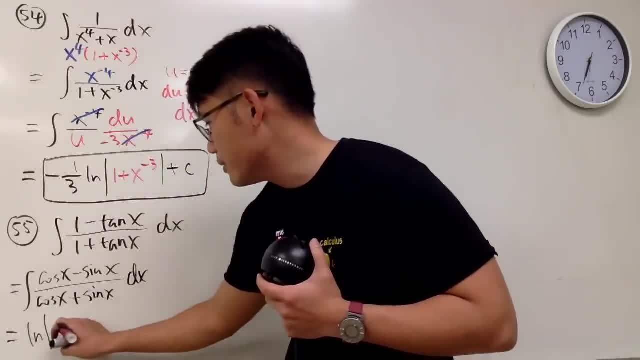 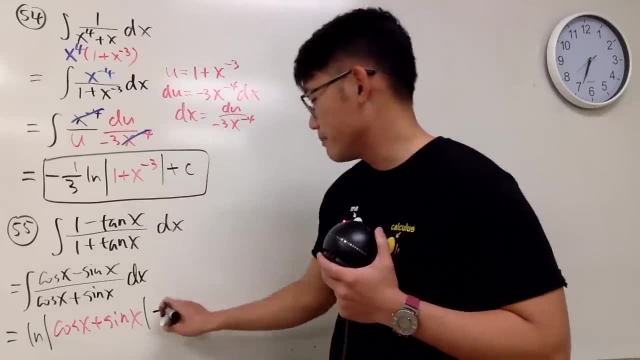 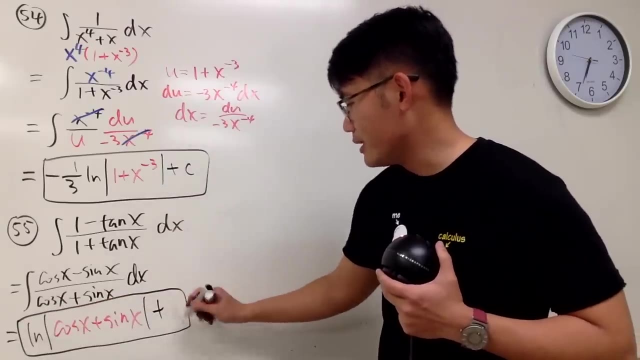 So natural log, absolute value, the denominator, which is cosine x plus sine x, Like that Very nice, Plus c. I think my c is getting smaller and smaller. I'm sorry, I shouldn't be disrespectful to the c. Anyway, that's it. 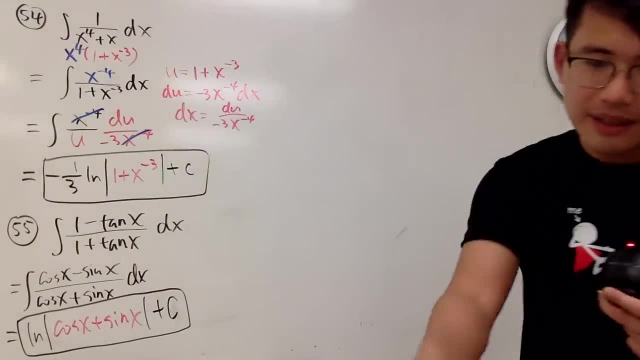 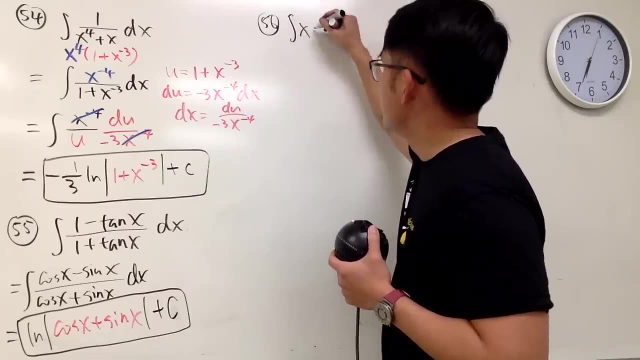 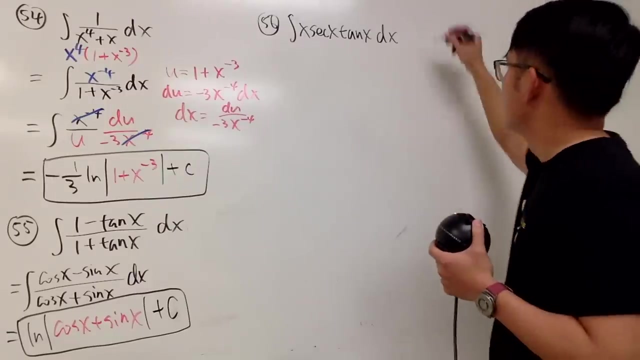 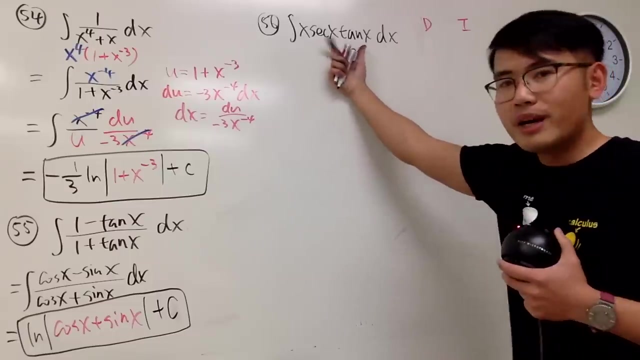 Okay, x times secant tangent. Okay, So number 56.. Integral: x times secant x. tangent x, dx. What do we do? Integration by parts, Di on the side Integrating what, though? Can we integrate tangent: Yes. Can we integrate secant tangent: Yes. 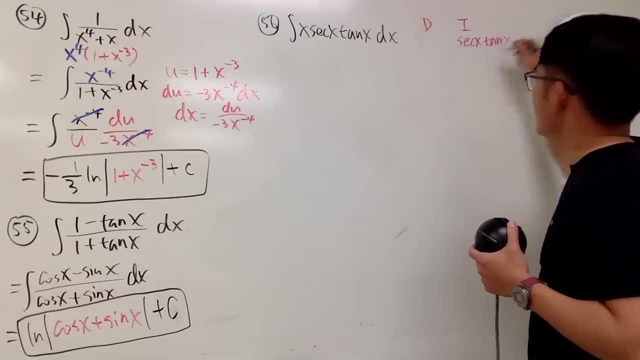 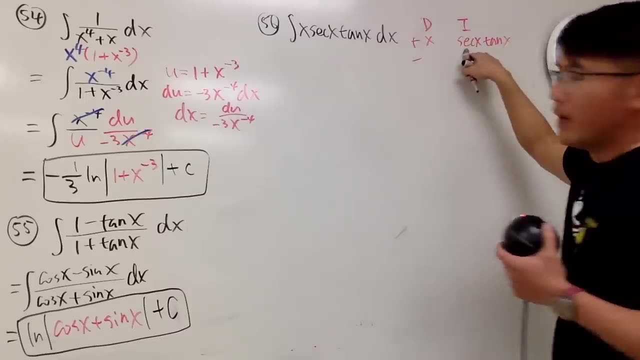 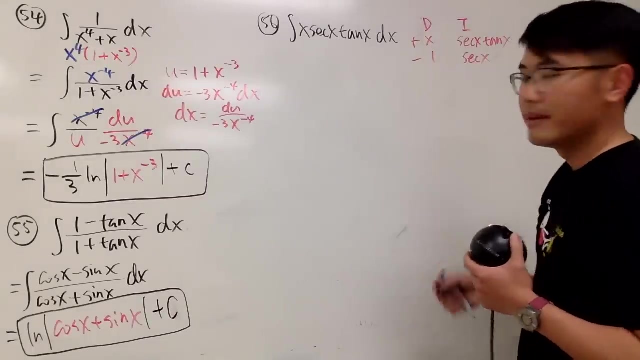 Let's go ahead and integrate secant x, tangent x, Differentiating just x, Even though you have three functions multiplying together. but no worry, When you integrate this guy, you get secant x. That's very nice. When you differentiate x, you get 1.. But can we keep going? 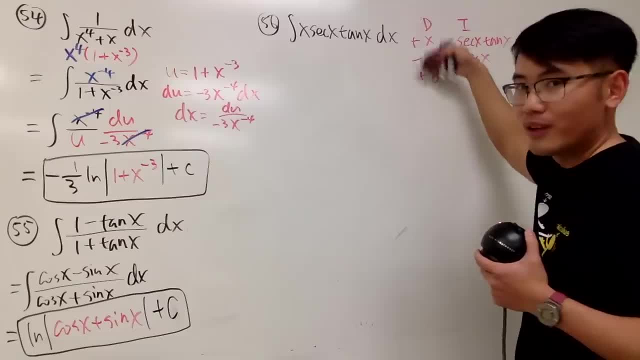 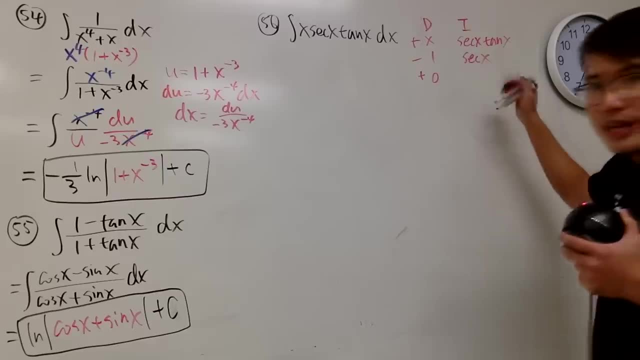 Yes, Because when you differentiate this again you get 0. And don't forget, the signs have to be plus, minus, alternating on the side. And then when you integrate secant, you get natural log absolute value of secant x plus tangent x. 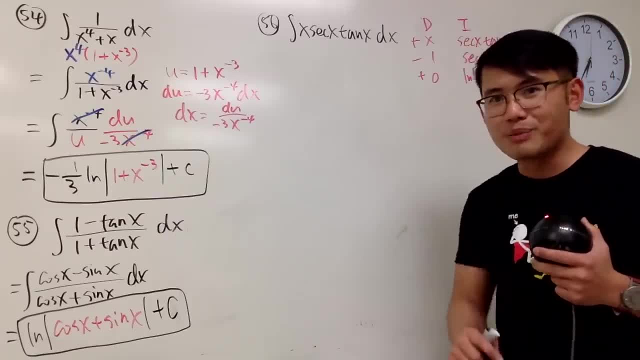 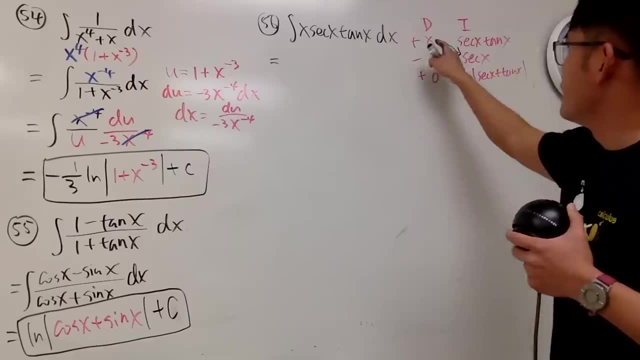 I was just trying to check to make sure that everybody is working properly for my QuickTime player. Hold on, okay, I was looking at the answers. whatsoever. Anyway, this times this, Then the x, times secant x, And then minus this times that. 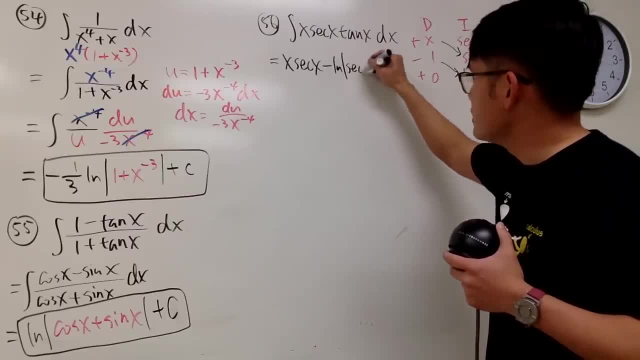 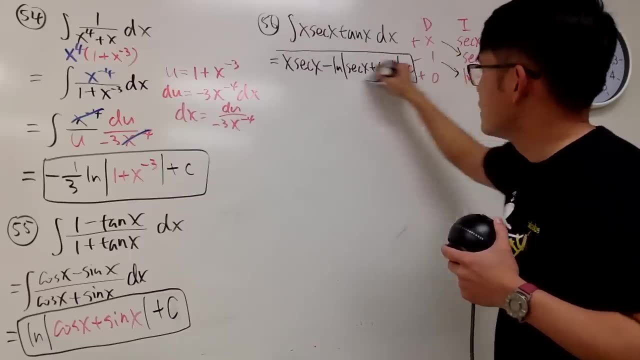 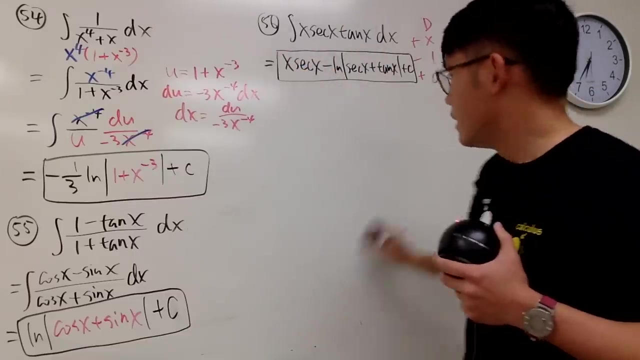 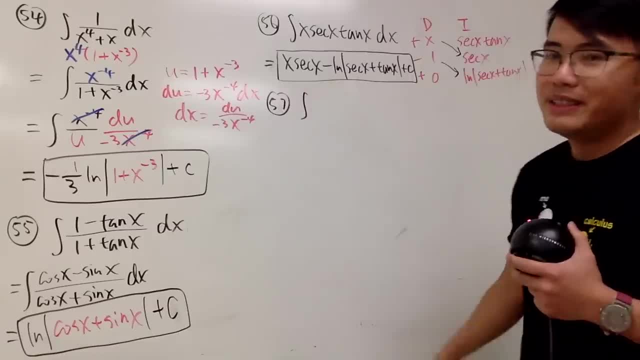 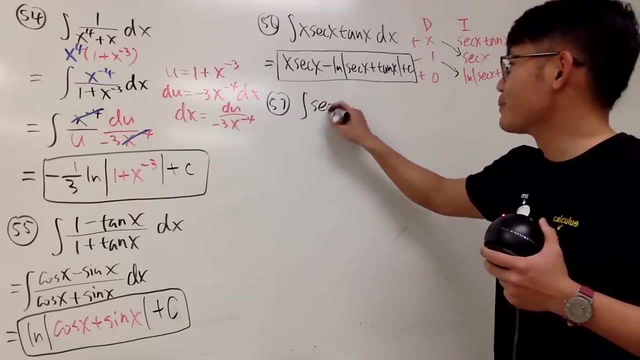 57. You know some professors. they are going to take some questions from here and then they are going to put it on the test. So you know it's a really good practice if you are in Cal 2 or if you just want to know how to integrate. 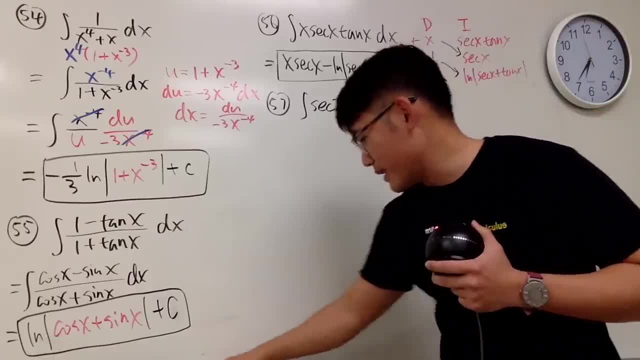 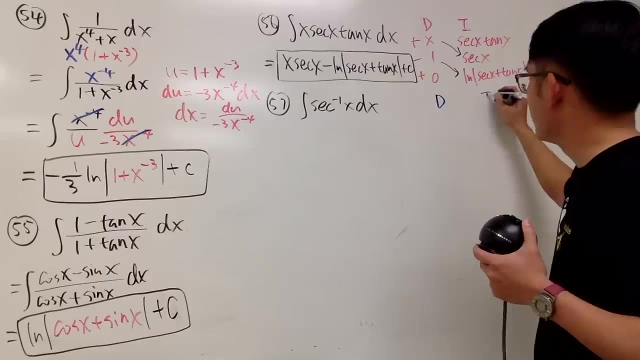 all these things correctly, and all that, I'm going to use a blue pen. What do we do? Yes, Integration by parts, It's right here. d and then the i, So plus, minus, Differentiating. what, though? That, of course. 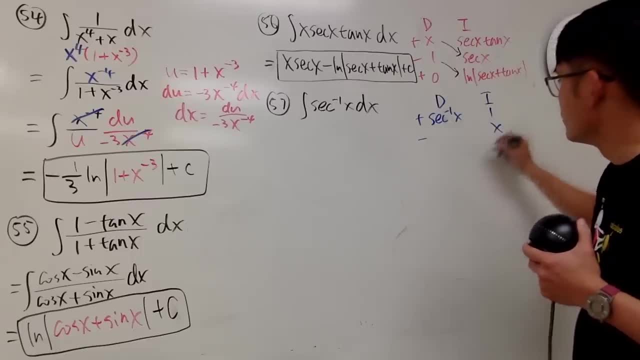 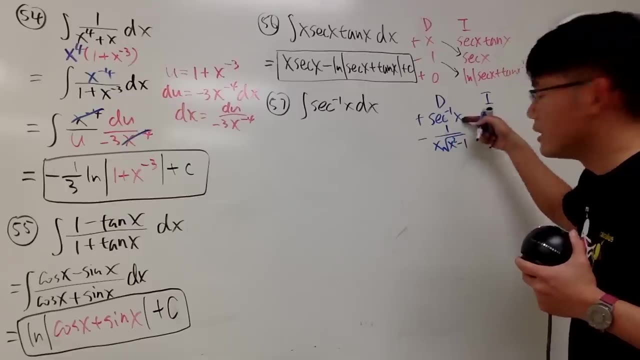 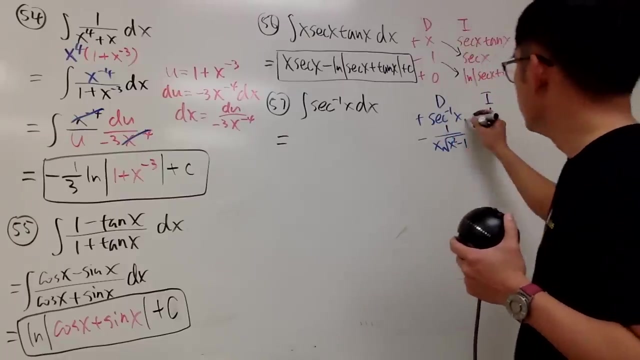 Integrating 1, which is x. Differentiating this, you get 1 over x times the square root of x squared minus 1.. That's a derivative of inverse secant. Okay, So we see that this right here this times. that is the first part of the answer. 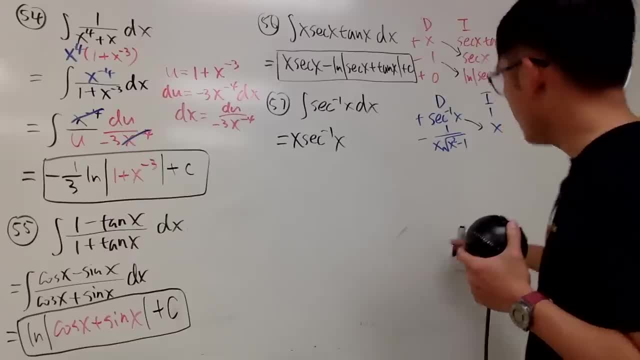 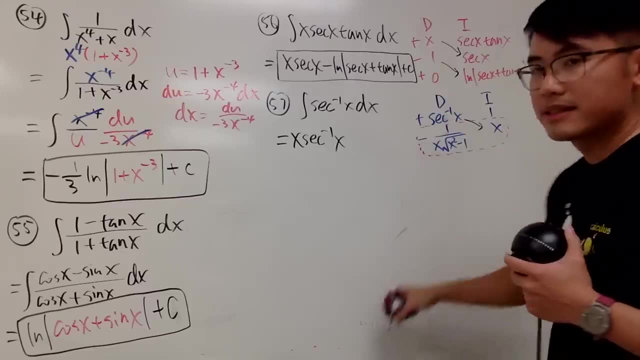 Then the x times inverse secant of x, And then of course you are going to do this right here, which is still going to be an integral. but x times x in the denominator here cancels out x times this, this x cancels out. 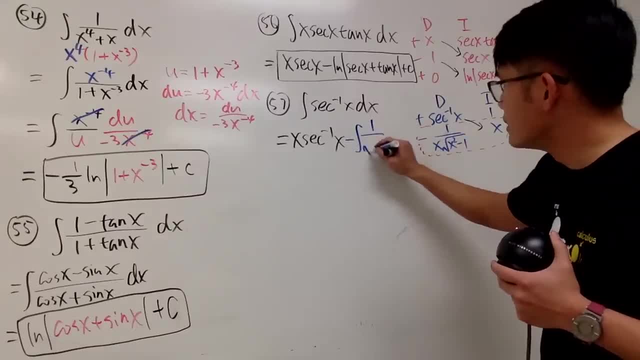 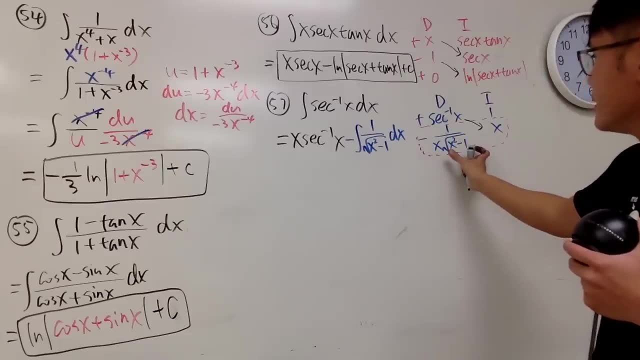 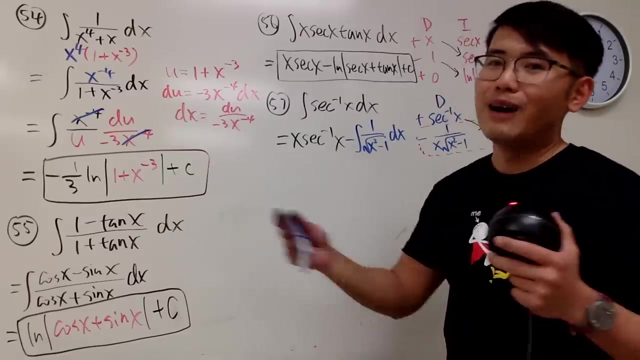 So you have to minus the integral of 1 over square root of x, squared minus 1 dx. Okay, Yeah, And how do we do this? Well, maybe you can do some hyperbolic trig functions business, but I'm out of those things, right? Because that. 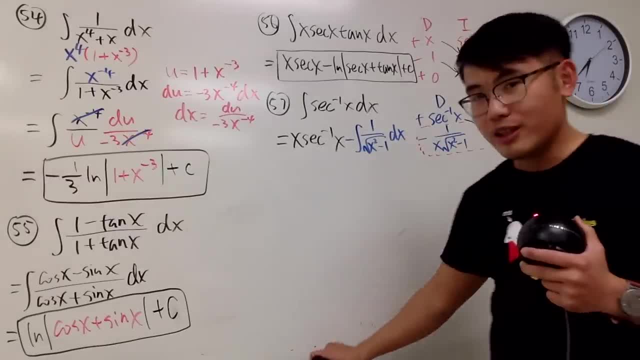 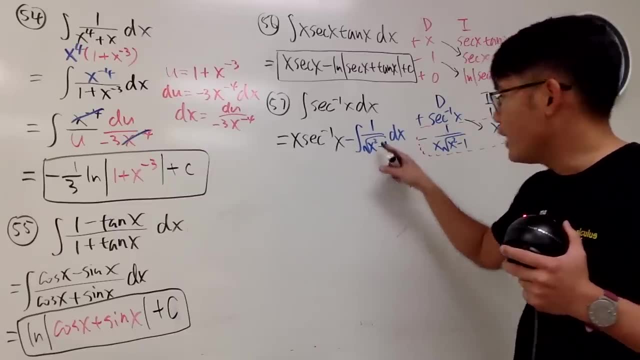 was just from question 40 to question 49. So I will do this one legitimately with you guys. Notice, this is slightly harder because you have the square root of x squared minus 1.. If you have 1 minus x squared inside, that's inverse sine. That would be easy. But anyway, right here. 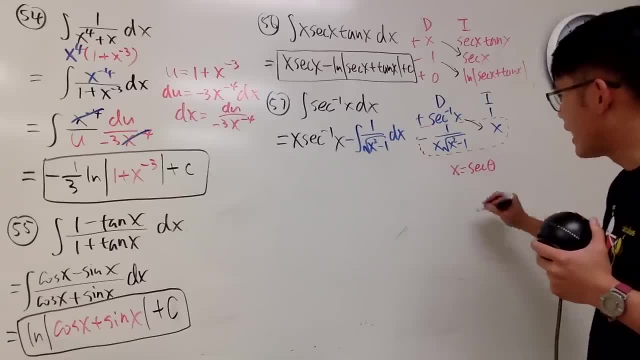 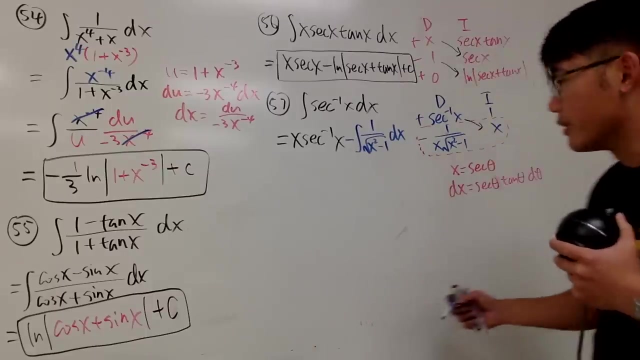 I will take x to be secant theta and then dx will be secant theta d theta. Secant theta, tangent theta d theta. Sorry, Like this Right, So perhaps I'll just do this one in blue for you guys right here and I'll put down all the answers over there real quick. 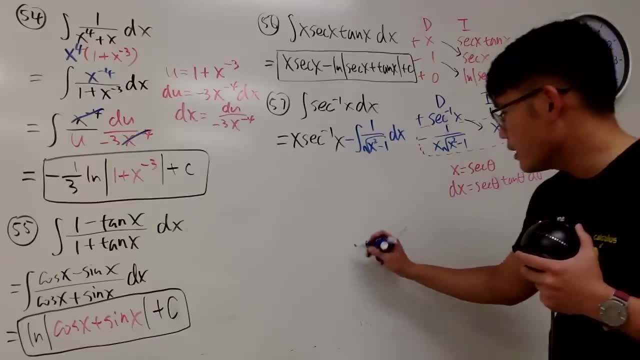 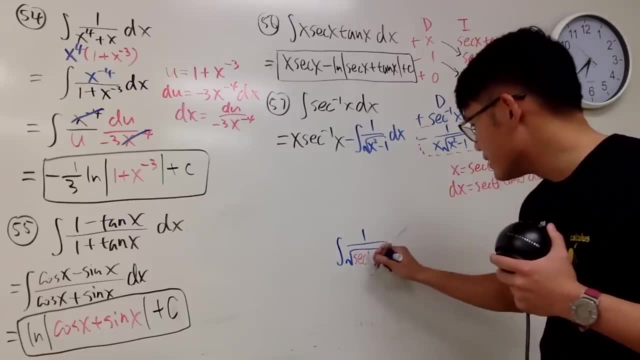 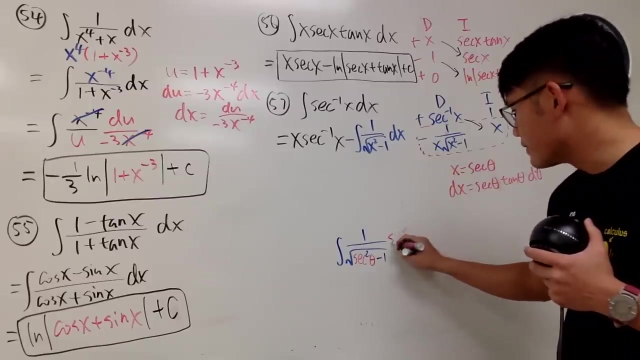 So this integral is going to be the integral of 1 over square root. x is secant theta now, So you have secant squared theta and then minus 1.. And then dx is this as I said, So we have secant theta tangent. 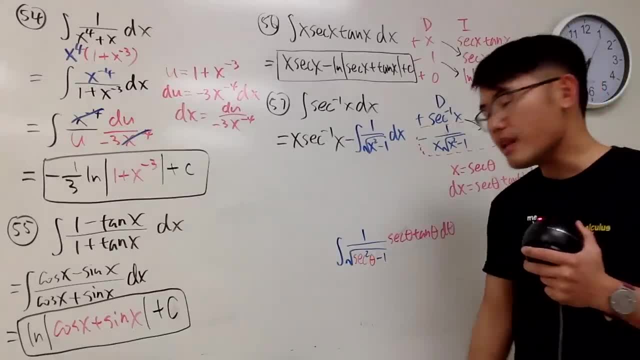 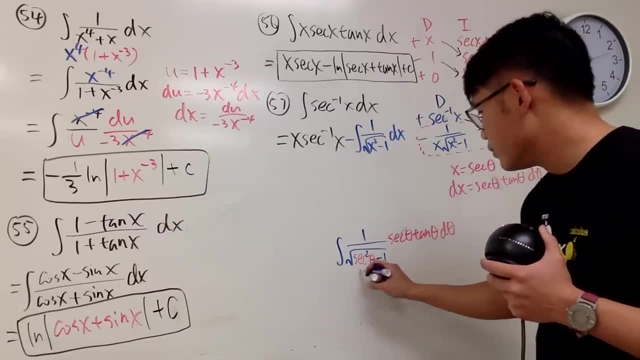 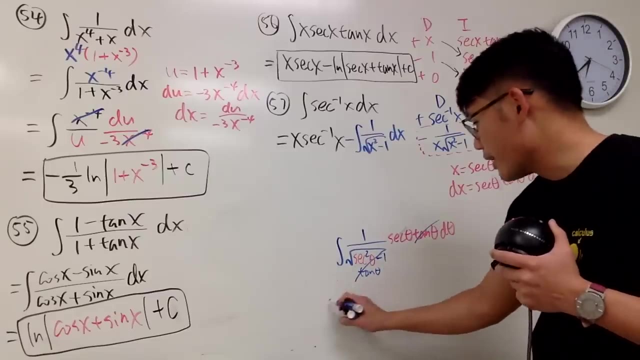 theta d theta, Like that. Alright, Now this right here is tangent, squared in the square root, which is tangent. So you have actually just tangent right here, Tangent theta, But this right here is going to be out of that, So you are just integrating secant theta. 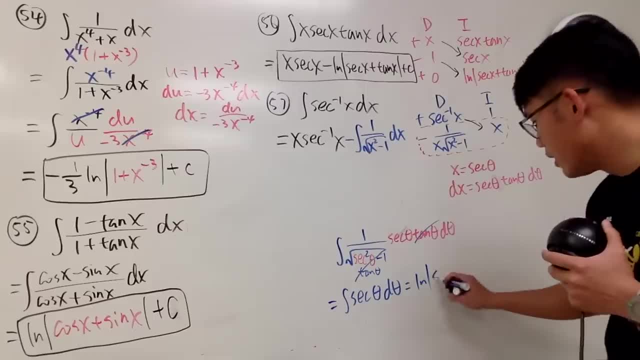 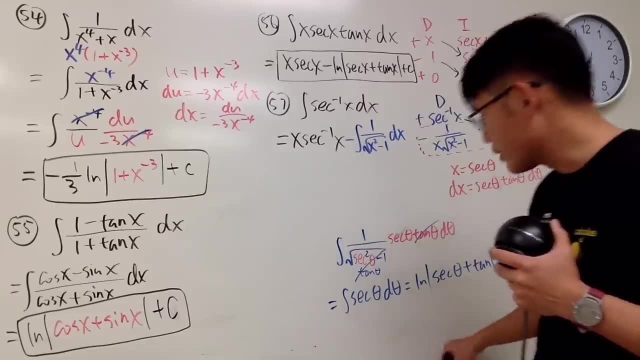 d theta, which is going to be natural log epsilon value of secant theta plus tangent theta. Like this right To save some time, I will actually go back here now because I pretty much know what will be going on. This right here is. 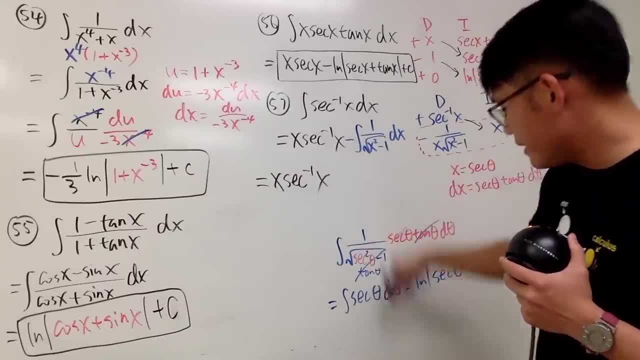 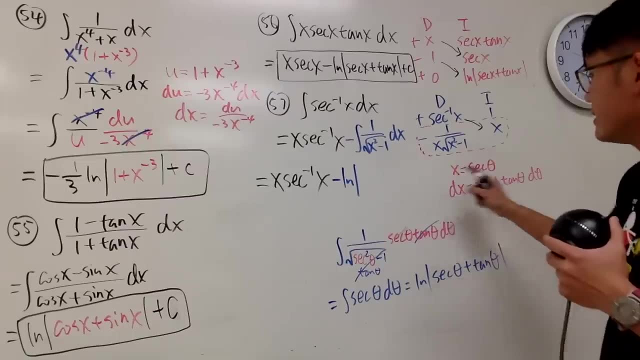 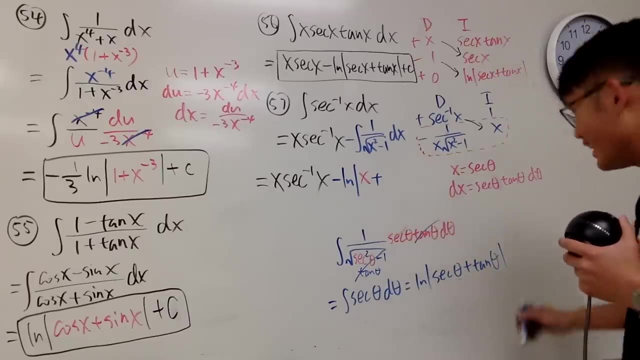 x times inverse secant of x and then minus. well, we have the natural log absolute value Secant theta is x. So that's nice. And then we have to add what's tangent. though. Go ahead, draw the right triangle real quick. This is the same. 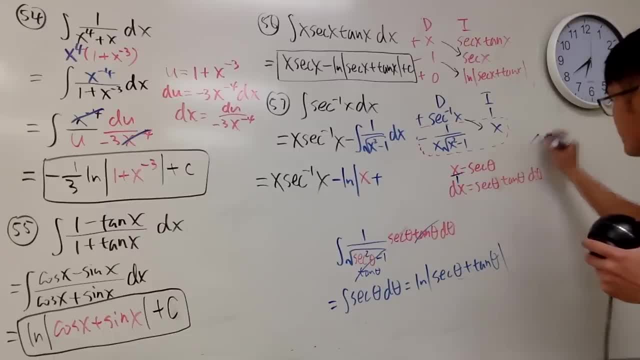 x over 1.. So if you draw right triangle right here, put the theta here: Secant is hypotenuse over adjacent, So x over 1.. On the other side here this is the square root of x squared minus 1.. 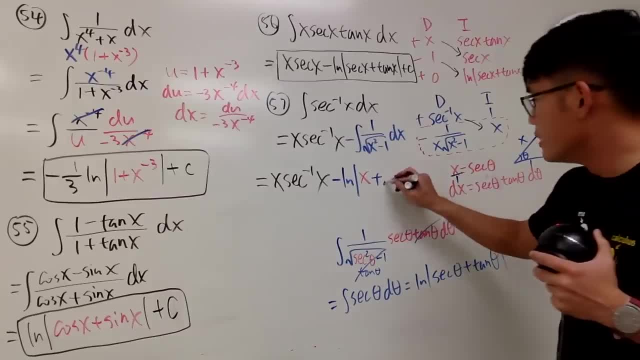 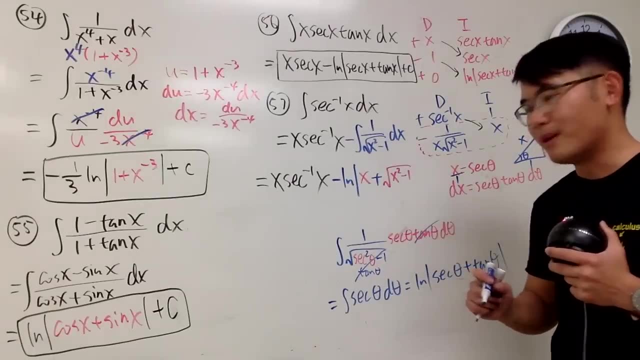 Tangent is opposite, over adjacent, So tangent theta is just going to be square root of x, squared minus 1.. I believe this is the inverse hyperbolic cosine, But I'm going to leave that to you guys. This is too bad. 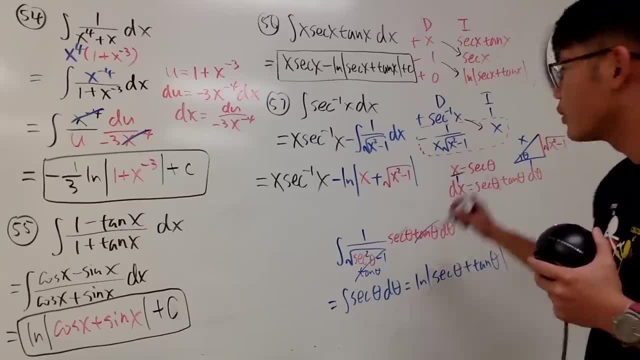 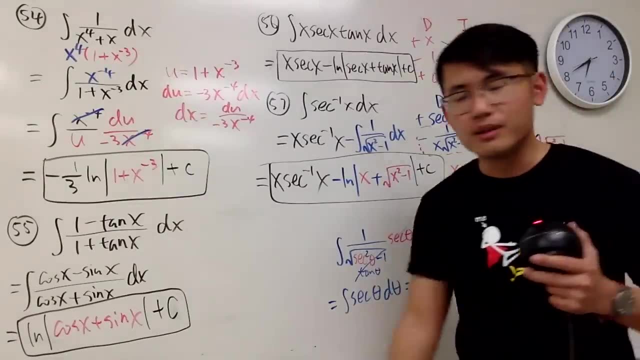 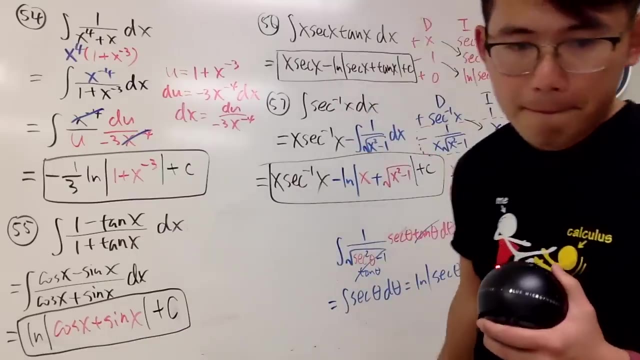 Anyway, with that said, we are done right here. So I put a plus c. This right here is the answer. So take a look, take a look, take a look. Okay now 58.. I'm not going to put on this. 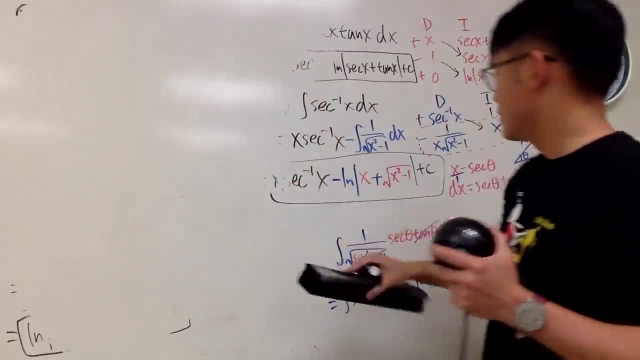 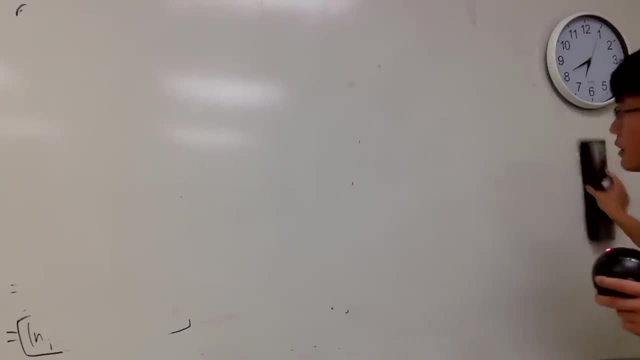 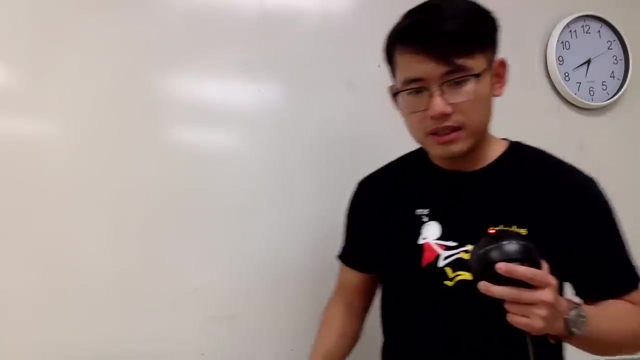 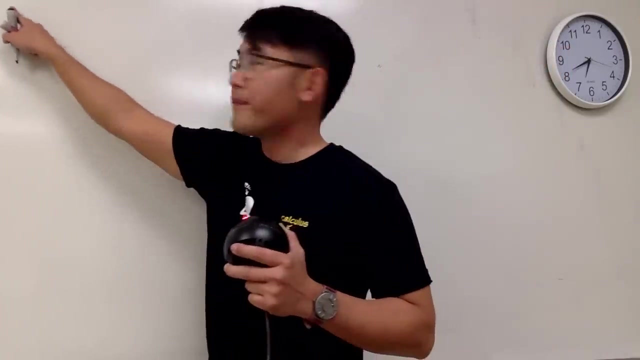 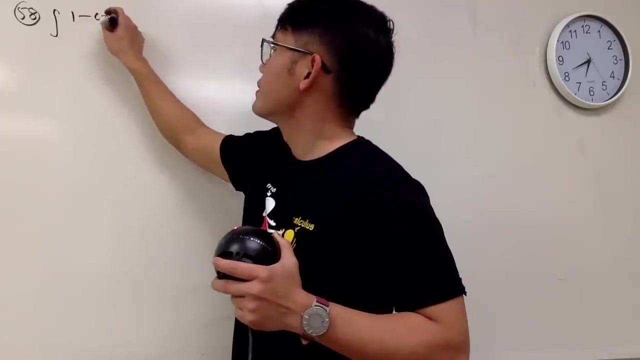 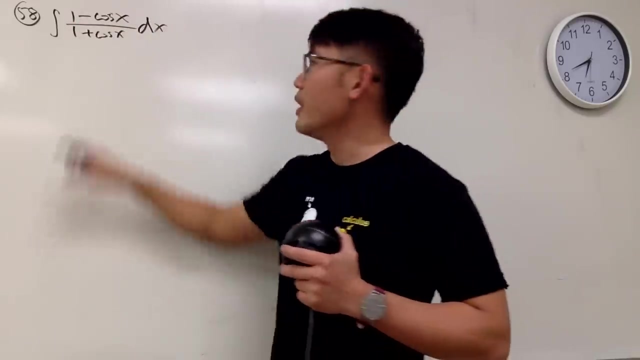 So take a look, okay, I'm going to erase everything. I can do this, Okay. 58.. Right here. 58.. Integral of 1 minus cosine x over 1 plus cosine x dx. Now you have choices. One: you can multiply the bottom and the top. 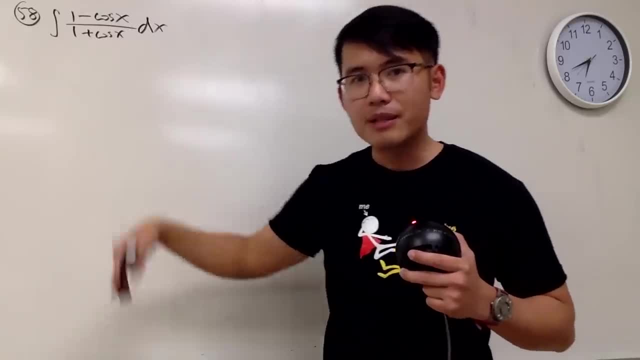 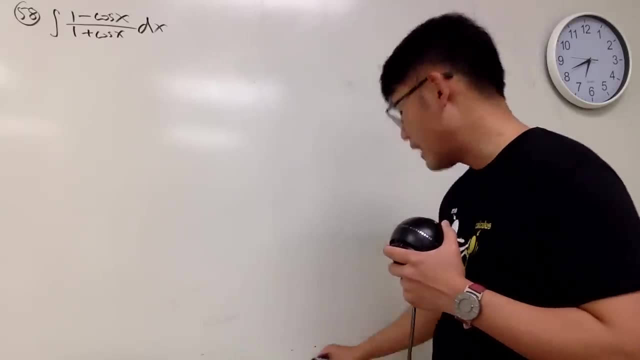 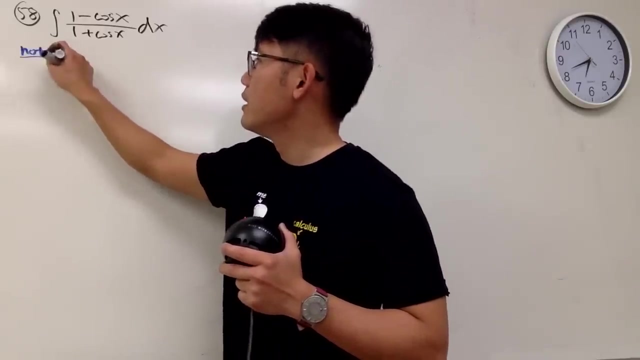 by the so-called conjugate, Namely you multiply the top and bottom by 1 minus cosine x. That will work. Or you can also do the following, Because you have seen that well, notice when we have the reduction formula for the squares. 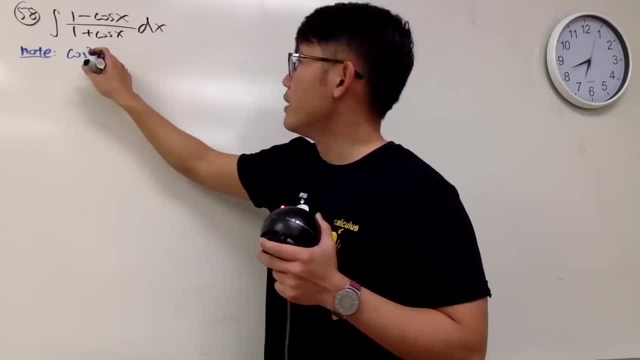 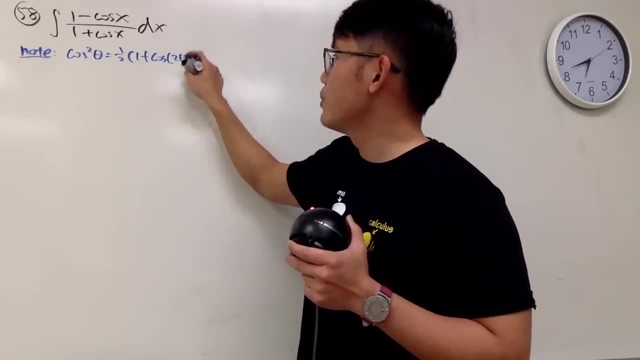 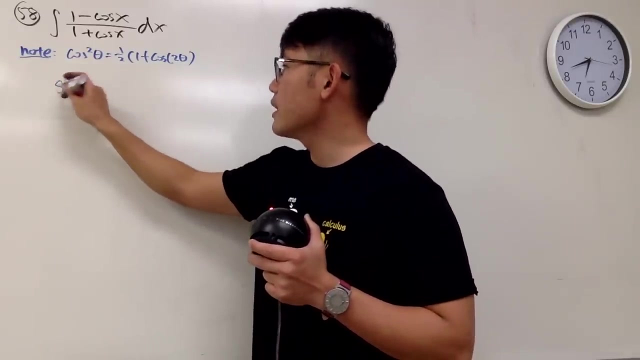 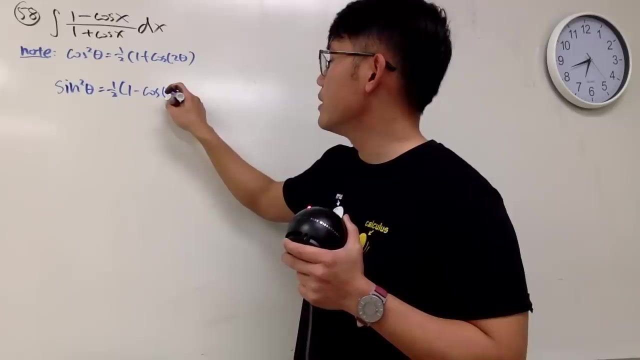 you know cosine squared theta, this is 1 half parentheses, 1 plus cosine 2 theta right. And similarly you also know that when you have sine squared theta, this right here is 1 half times 1 minus cosine of 2 theta, like this: 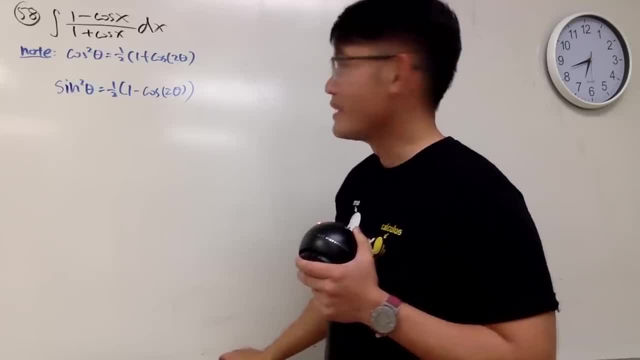 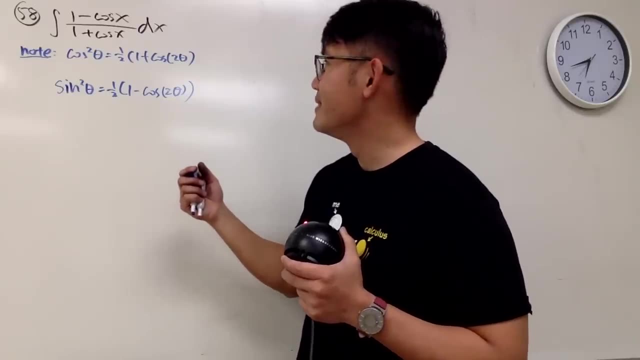 So these are good And we can utilize them. So the deal is that first of all we can multiply both sides by 2. And then just plug in x over 2.. Yeah, for the theta, Then we can get this done. So 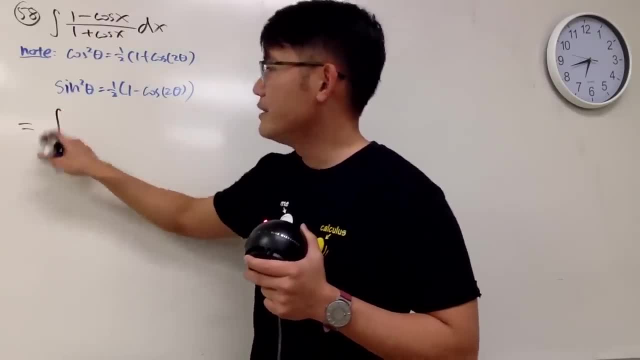 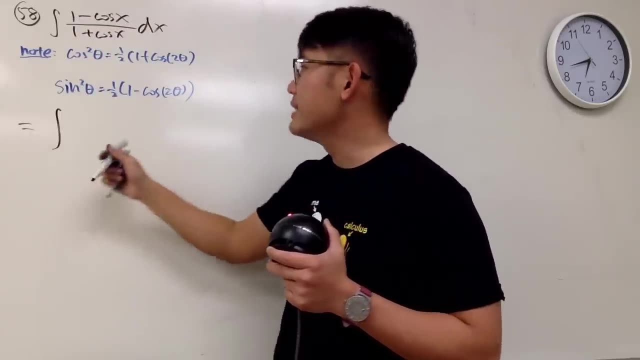 I'm just going to work this out right here for you guys. Here is the deal. This integral is the same as To get 1 minus cosine x. I can look at this. I will multiply by 2 on both sides, I will. 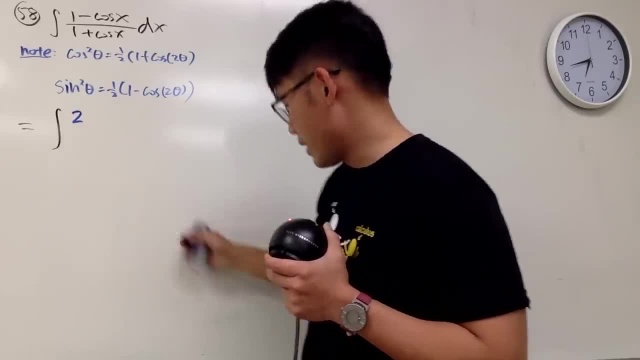 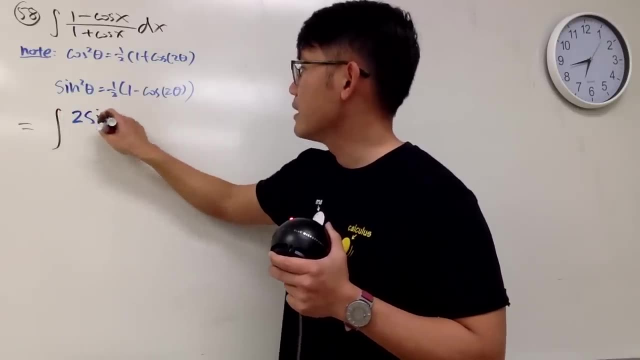 get 2 right here. Okay, I'll get 2 right here And then I will have sine right. The top one is sine squared. But, as I said, this right here is 2 theta You have to put in. 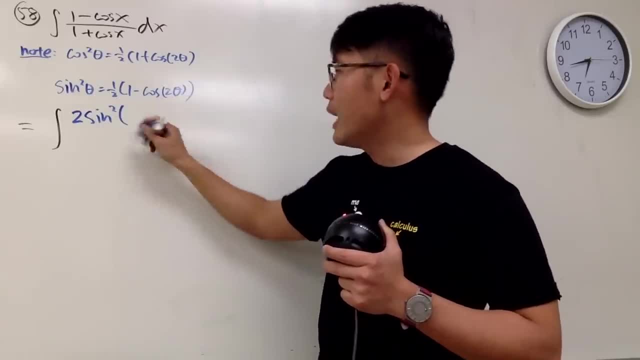 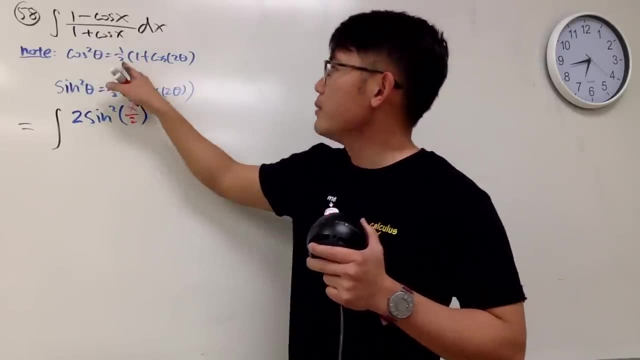 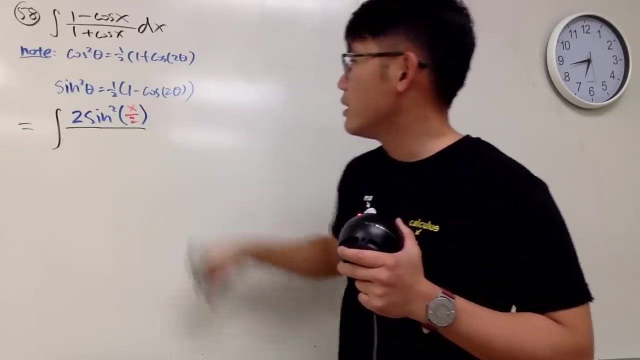 x over 2.. x over 2.. So here you have x over 2.. Right, Like that. Similarly, on the bottom, multiply this equation by 2, this identity by 2.. And then, and then let's see. 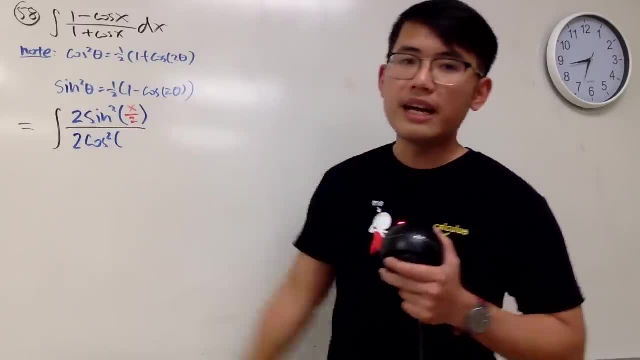 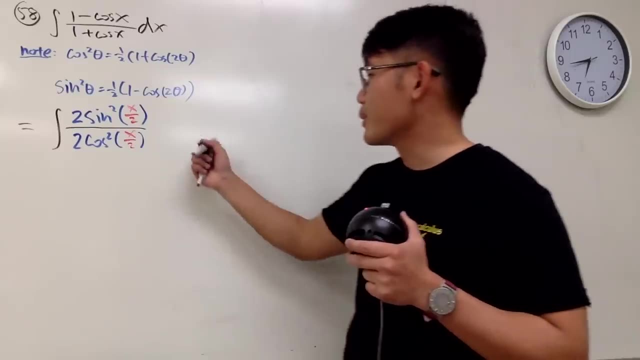 you have the cosine squared Again. you put theta as x over 2.. So you have x over 2 here. like that, This is going to be quicker. Okay, This is going to be quicker. So if you utilize this, that would be good. 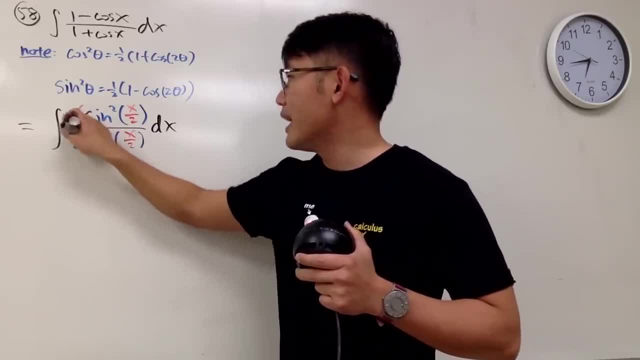 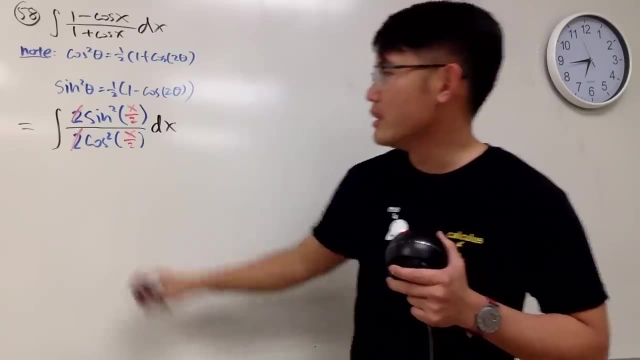 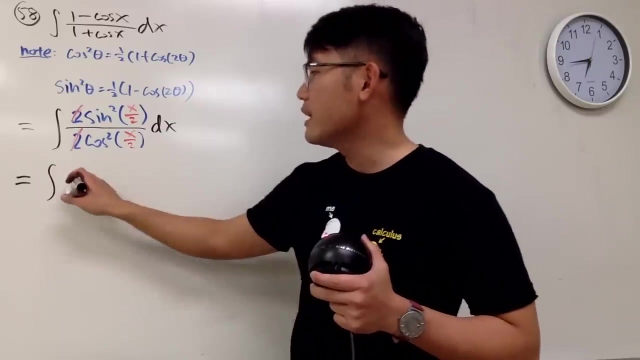 Of course the 2's cancel And the beauty is that this right here is just going to be tangent squared, with x over 2 as the input To integrate tangent squared of something. you will look at the secant version for that. 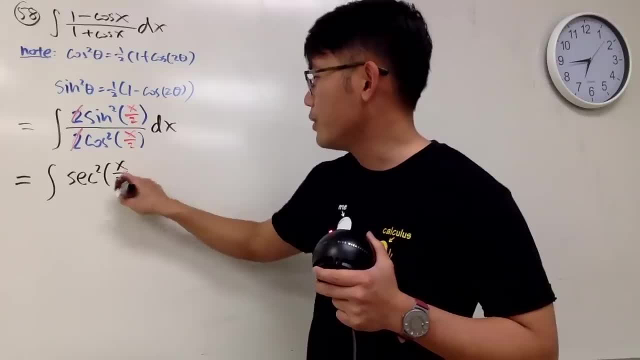 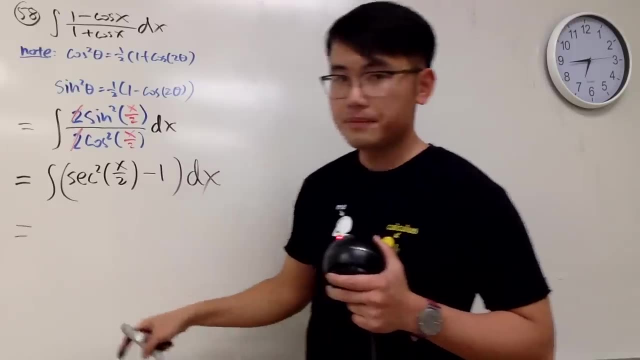 So, in other words, you look at this as the secant squared of x over 2 minus 1 in the x world. So now when you integrate this guy, well, integral of secant squared is tangent and you put the input to be the same. 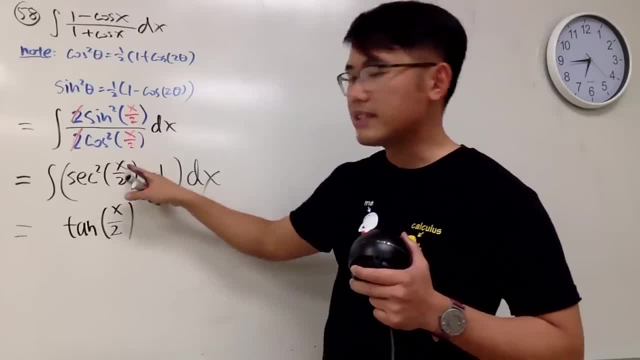 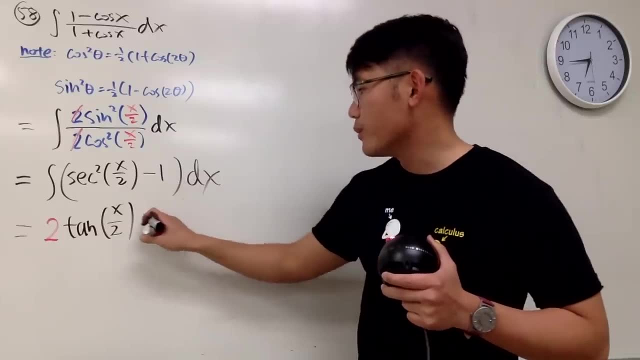 x over 2.. But you have to divide it by the derivative inside. The derivative of this is 1 half, so you have to multiply by 2.. And also integrate minus 1, which is minus x, like that. 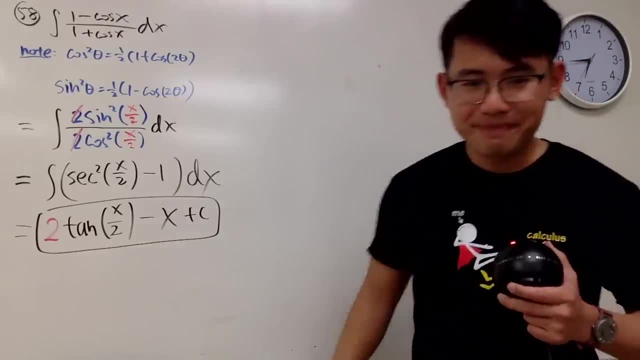 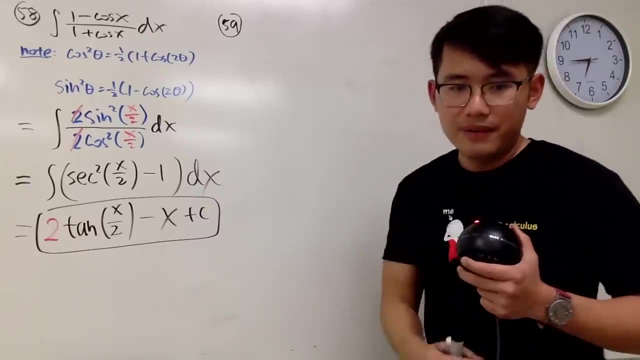 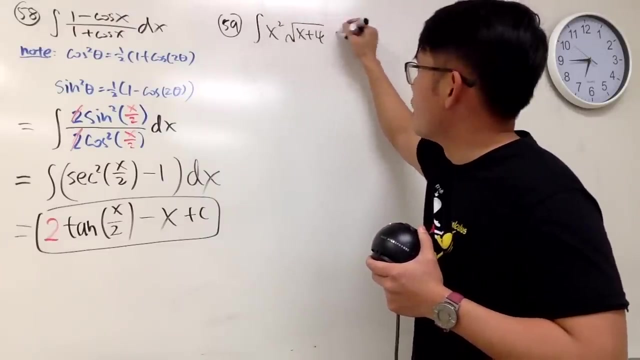 Well done, Plus plus z. This is it? Okay, Not bad. Okay. next one, Number 59.. Number 59.. Number 59. We have the integral of x, squared squared root of x plus 4 dx. Here's the deal. 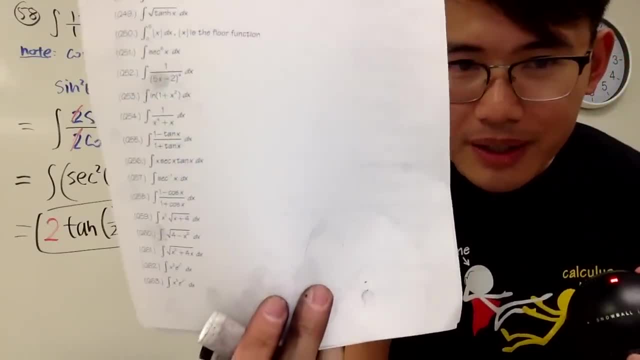 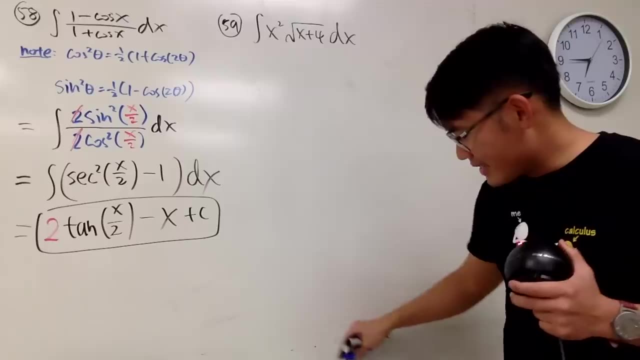 Why- Okay, you can take a look. 59 is that? Why don't people put a square inside and then make this the first power? Why don't people do that? And yes, I'm pretty much blaming myself? Okay, we can still do. 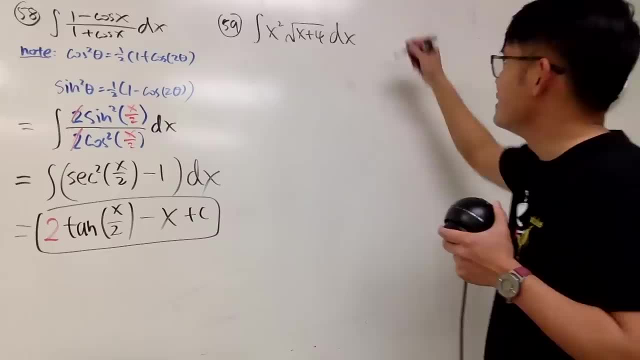 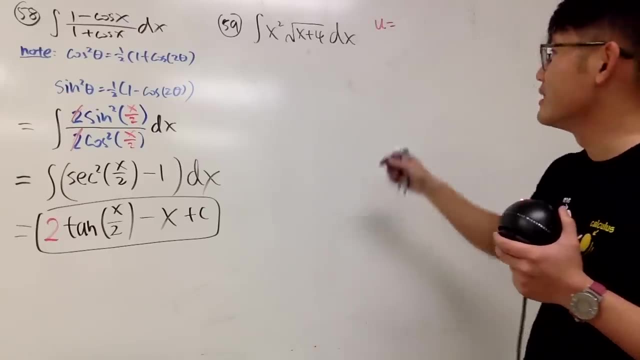 use of for this. Believe in the U world. U world sometimes is much better. Take u to be x plus 4,, if you like. If you take the square root of x plus 4, I think that's okay as well. but 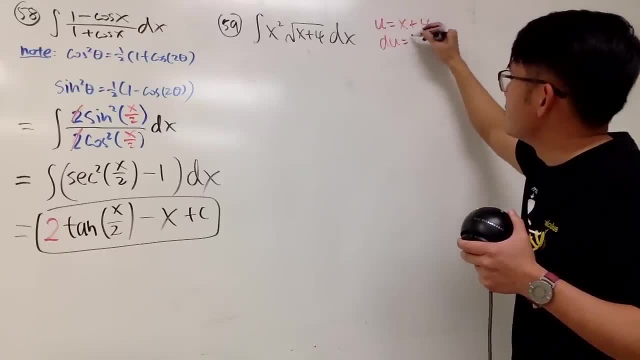 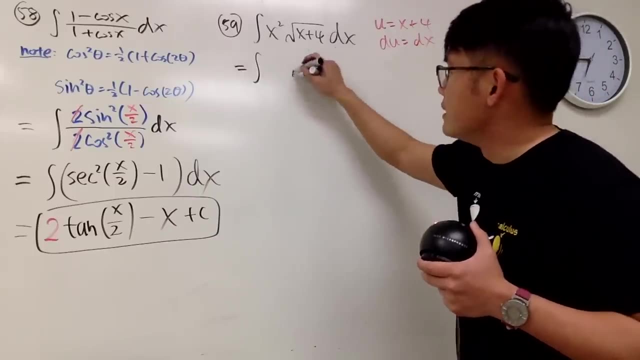 I'll just take u to be x plus 4.. du is the same as dx, So let's go ahead and get going This right here, the integral. By this time, though, you will see, this is the square root of u. 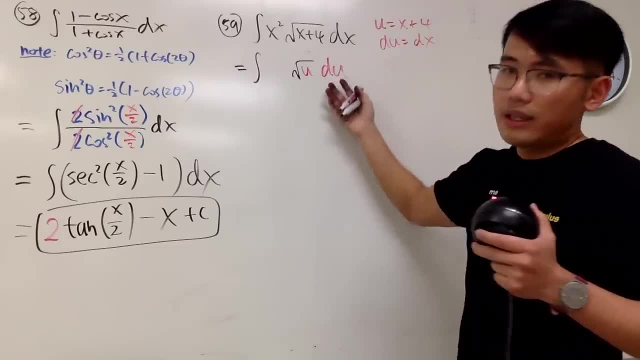 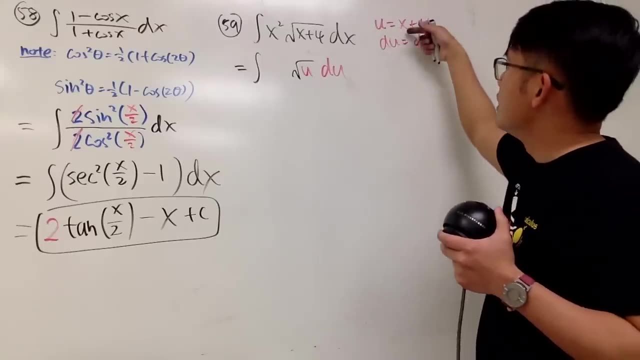 and the dx is du, So there's nothing to be cancelled with x squared. x is not allowed in the? u world, so you have to look back to see what x is. You can subtract 4 on both sides. in another world, x is equal to u. 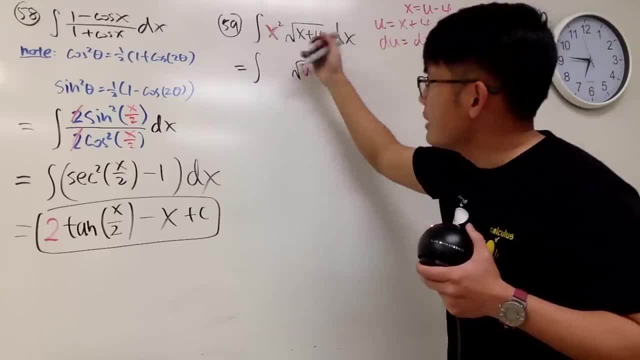 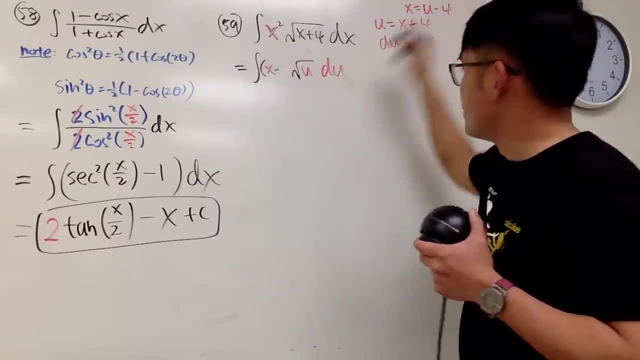 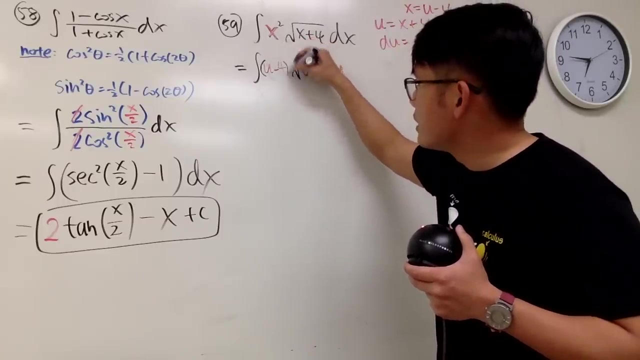 minus 4, so look at this x and plug in x minus 4 for it. So parentheses x minus. I mean u minus 4 for the x, u minus 4 for this guy, and then we have the square. Okay, we still have the. 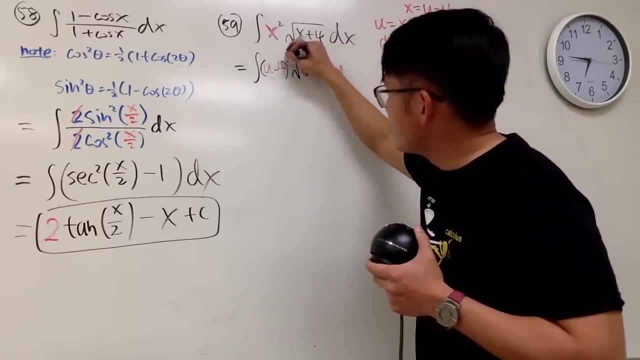 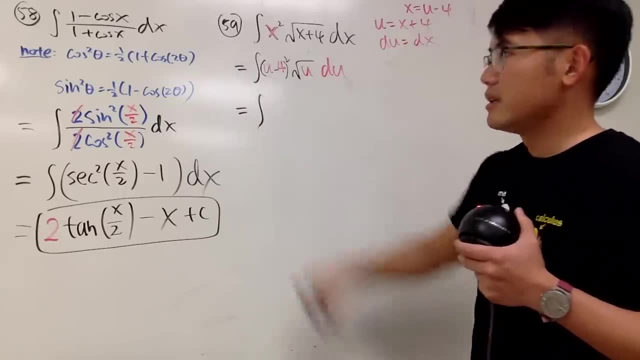 square. This right here is actually not so bad, because you actually just will end up with power functions. So let's do this right here and we have to be careful with the powers now because it's question 59.. This right here. 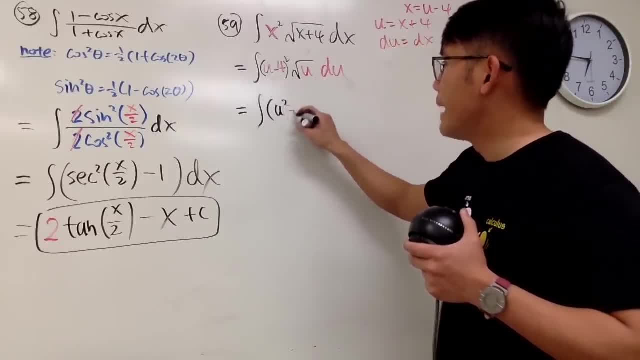 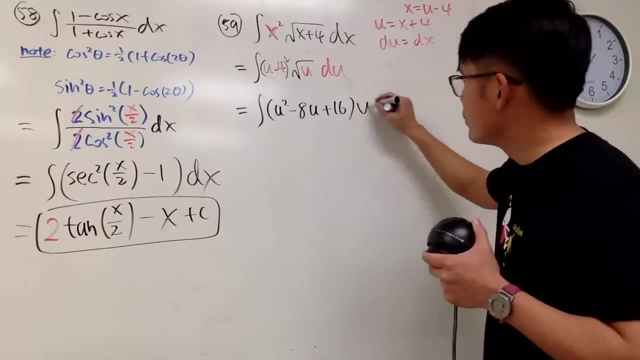 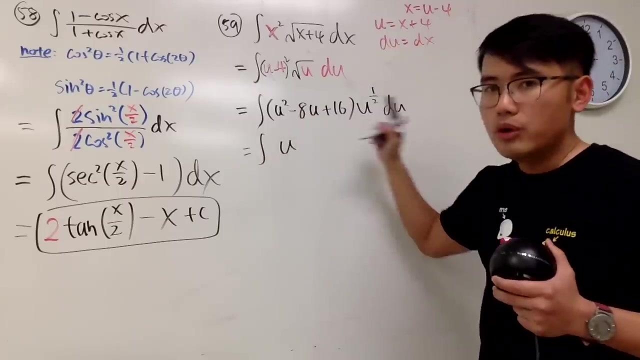 we have u squared minus 2 times this and that which is 8,. u to the first plus 16, and then this right here is the same as saying u to the one-half power, du, and then distribute everybody. So first you have u 2 plus 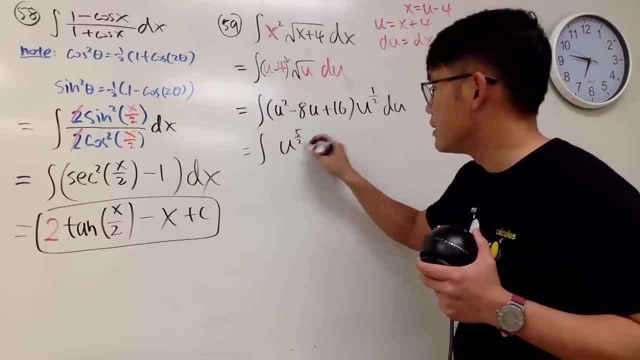 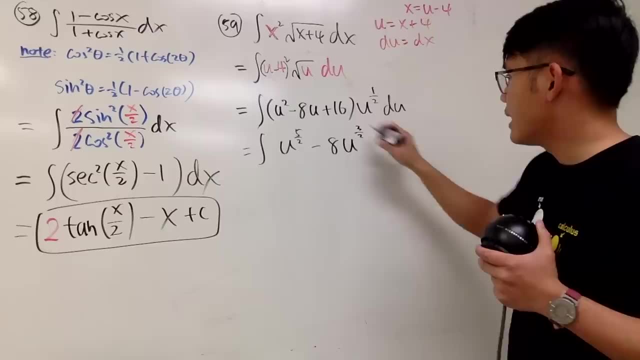 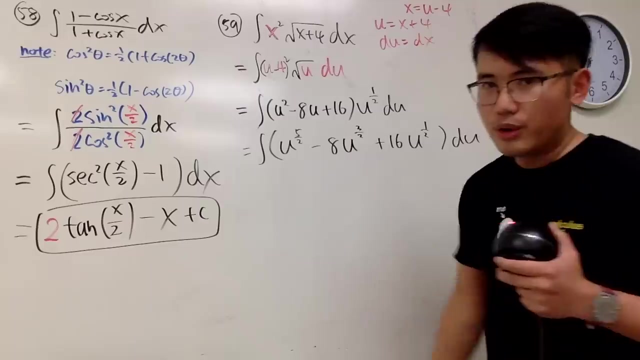 one-half, you get 5 over 2, I believe Yes. and then minus 8 times u. 1 plus one-half is 3-half. Lastly, plus 16, u to the one-half power. okay, du, Still good. 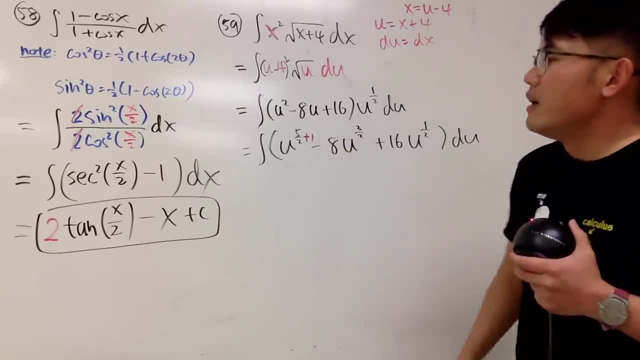 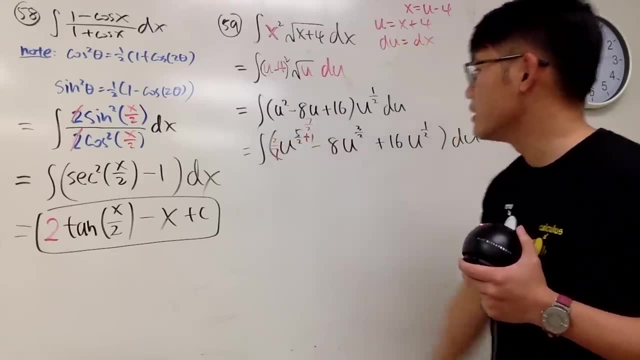 Now go ahead, add 1 to the power. 5 plus 2 is 7 over 2, so I'll put that down right here and then divide it by the new power, which is 2 over 7.. This right here. 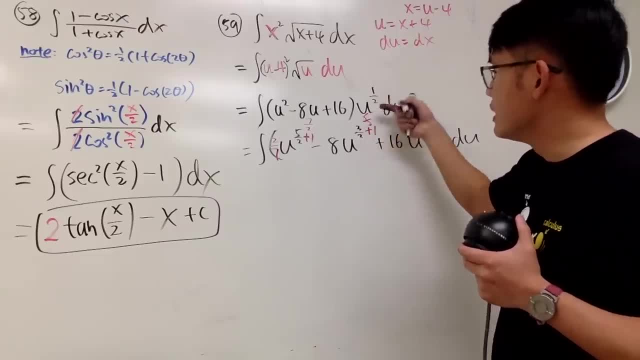 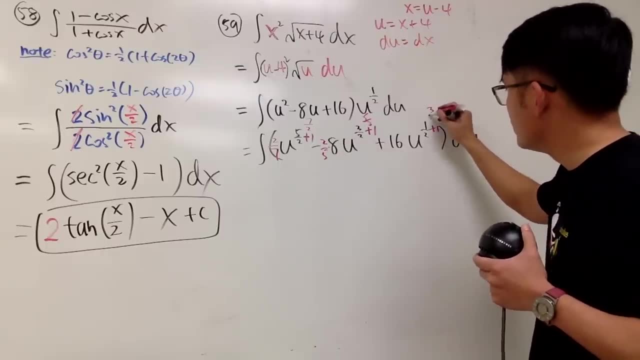 I will add 1,, which is going to be 5 over 2,, divided by that, which is the same as multiplied by 2 over 5.. And then, right here, I add 1,, which is 3 over 2,, and I'll. 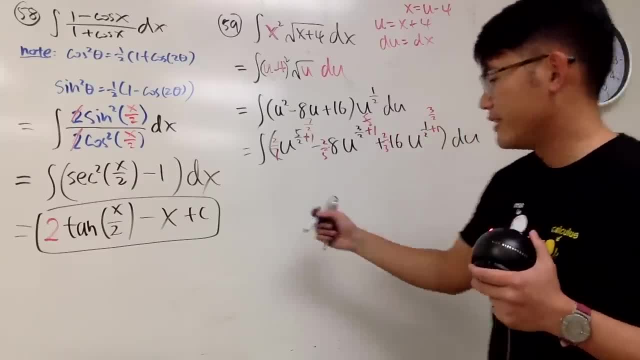 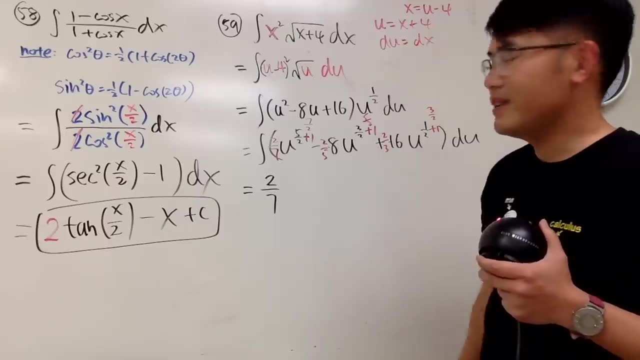 divide it by that which is 2 over 3, like this. Alright, now let's see, We have 2 over 7, and I'm not going to write it in the radical form, I'm just writing it down in the power form, okay. 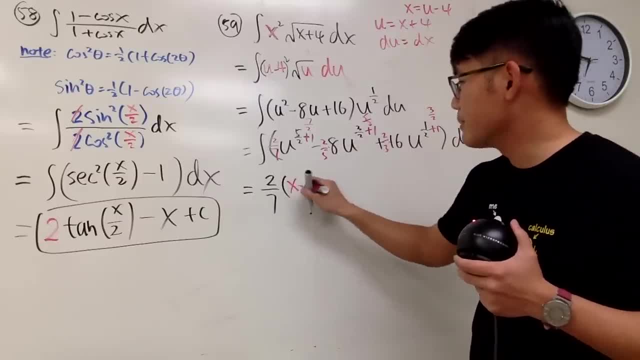 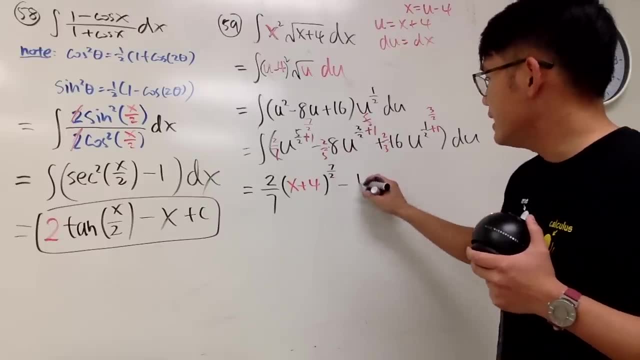 I have u, which is x plus 4, so I have x plus 4 for the? u to the 7 over 2 power, and then, of course, this times that you get minus 16 over 5, u is: 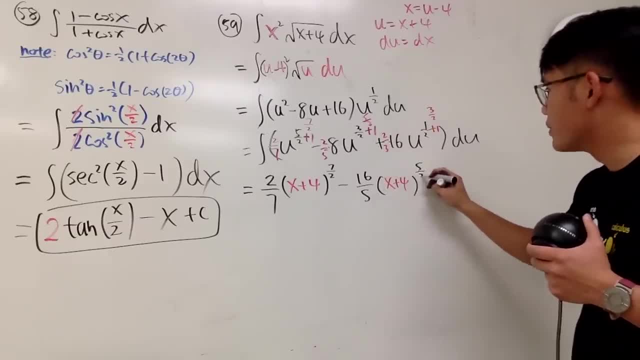 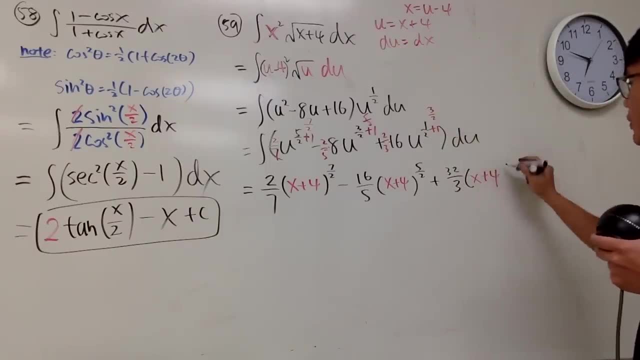 x plus 4, and then you have the 5 over 2, and this times that is plus 32 over 3, and this is x plus 4 to the three-half power. and this is a totally okay answer. Don't tell me to factor. 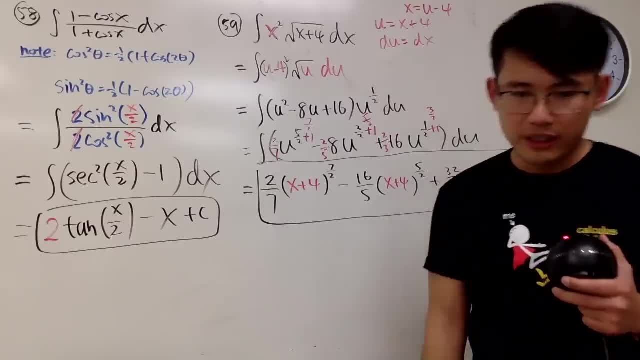 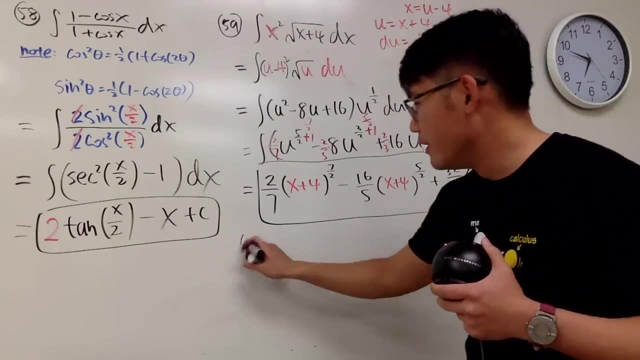 forever. Seriously, I'm not going to care about factoring. This is good. okay, This is good enough. Now number 60. I will challenge myself to fitting number 60 right here. We are going to be integrating, I'm going to. 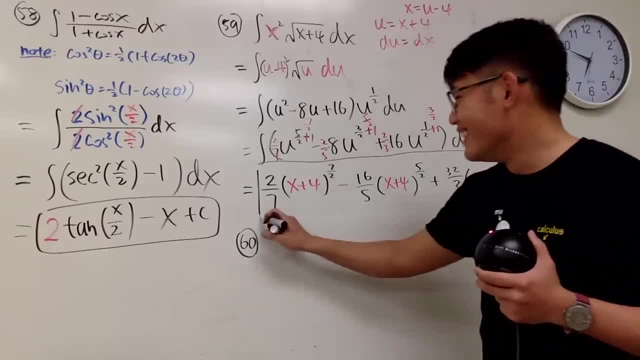 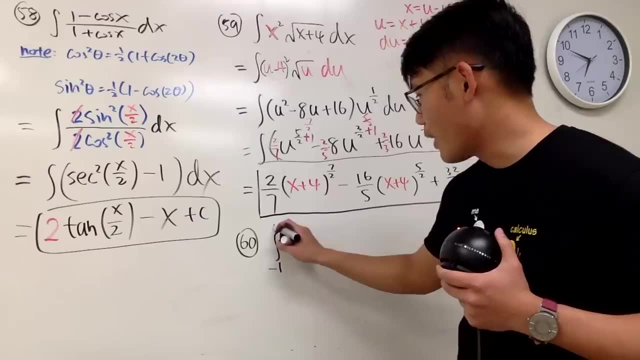 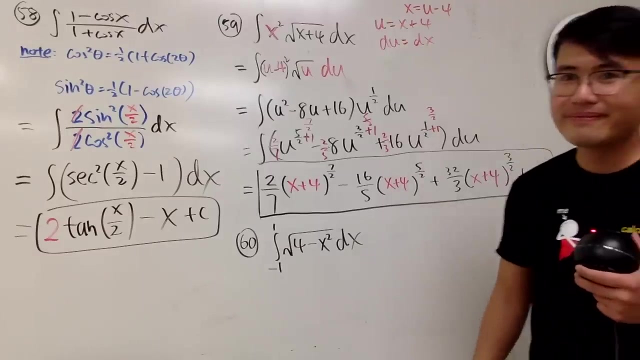 erase this a little bit to have more space. Right, We will be integrating from negative 1 to 1 square root of 4 minus x squared dx. Let me tell you: if this equation was from negative 2 to 2, it might be easier Why. 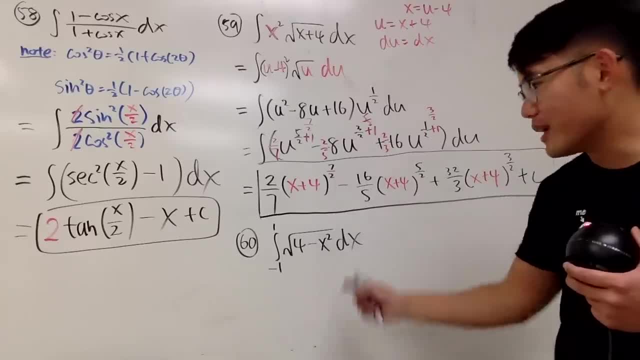 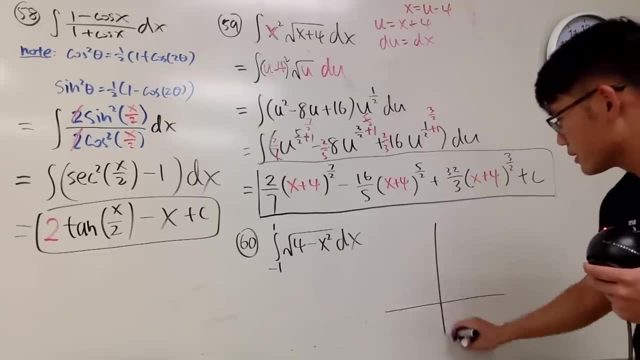 Because this right here is the semicircle with radius 2, right This right here. So I will probably just put this down right here. It's going to be bigger, like this Semicircle with radius 2.. So this right here will be. 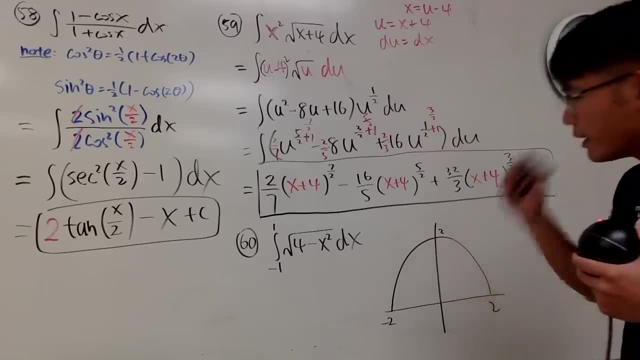 negative 2,. this right here will be positive 2, and this right here will be 2 as well. If you go from negative 2 to 2, that means you find the area of the semicircle very easy: pi r squared divided by 2.. 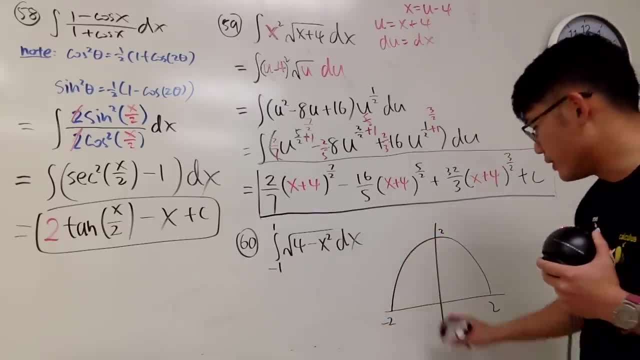 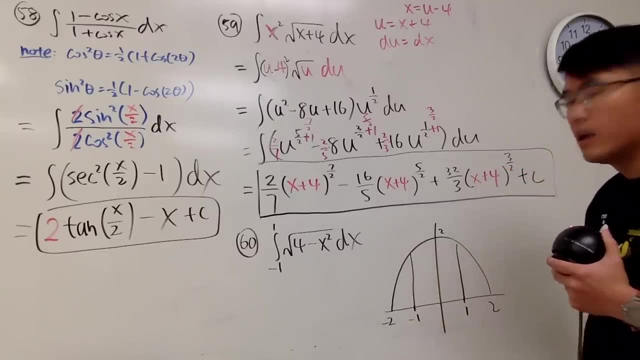 But we are going from negative 1 to 1, so this is how we do it. So this is negative 1, let's say this is 1, so you are going to go from here to here. As you all know, we can. 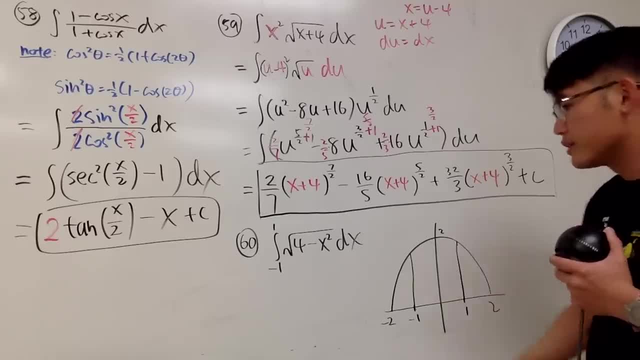 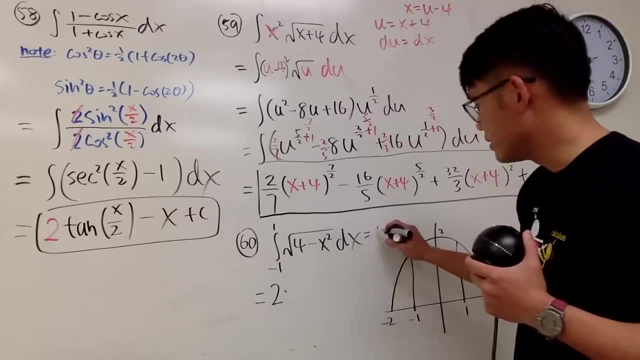 just find out one of the area and then double it. so let's go ahead and say this is the 2 times this area here. okay, The integral from. let me just write it down: this is 2 times the integral from 0 to 1,. 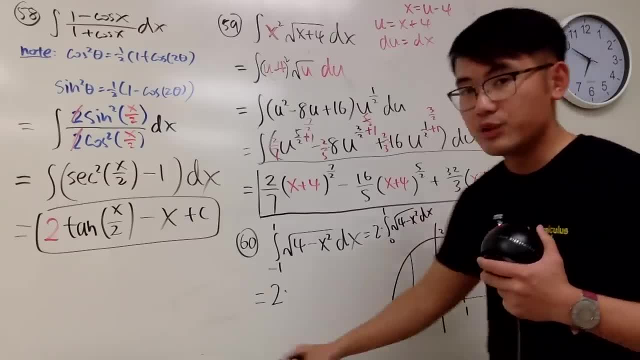 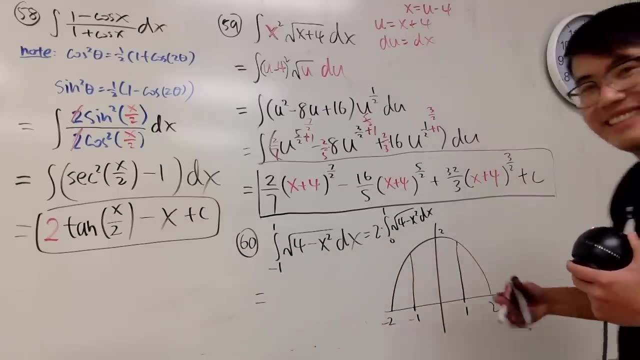 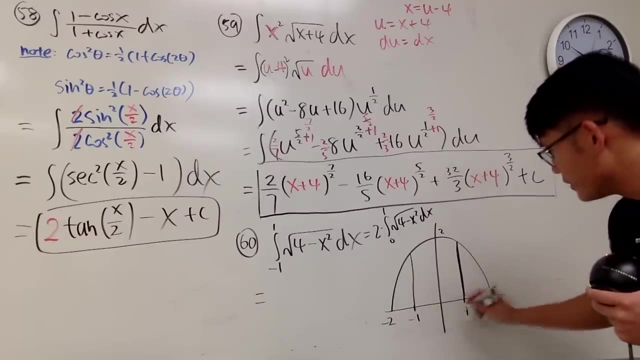 square root of 4 minus x squared dx. Easier this way, Right, So we'll be focusing on just this part. How do we do it? By geometry, First of all. if you want to get this area, of course you can. 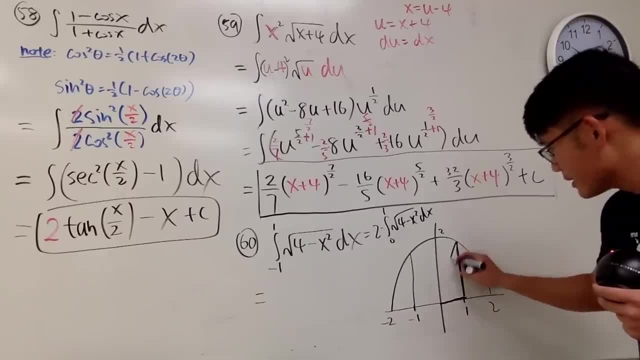 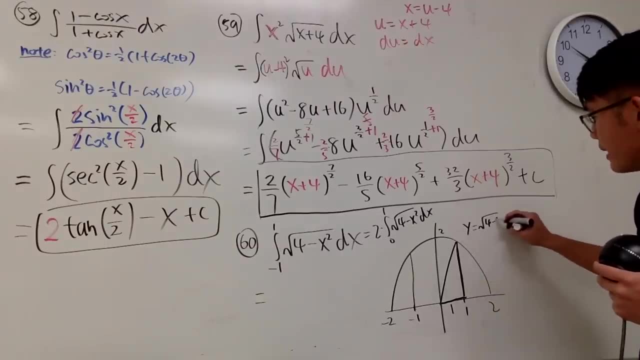 see, we have a triangle like this. This right here is 1.. What's the height, though? Well, y is equal to square root of 4 minus x, squared When x is 1, the square root of 3, then, isn't it? 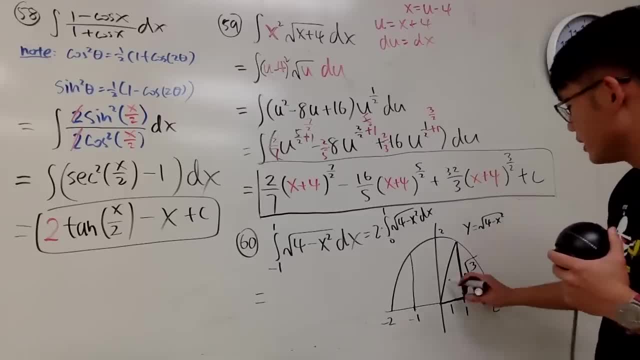 When x is 1,, you get 4 minus 1, which is square root of 3.. So, first of all, don't forget, you have the 2 in the front right. You have the 2 in the front. 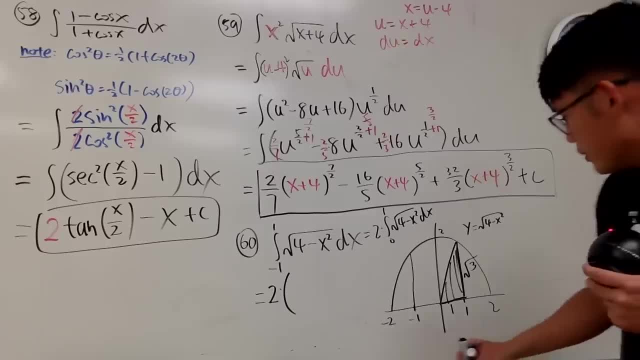 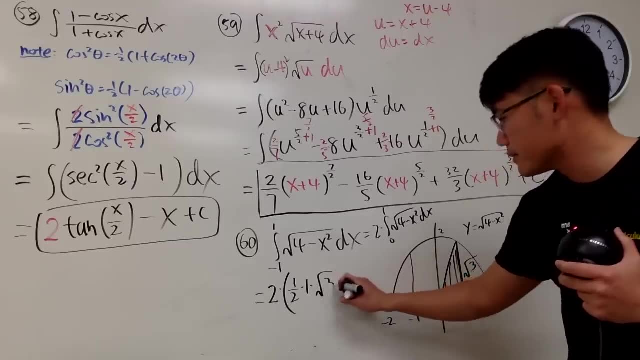 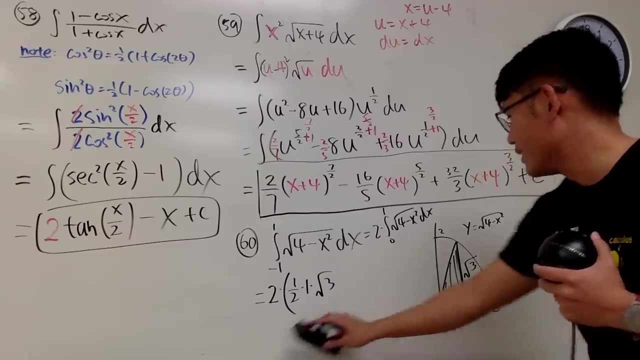 And then you are going to multiply the area of this triangle, which is 1 half times, 1 times square root of 3.. Okay, And I'm going to have more space, so I'm not going to look at the. I want to have more space, so I'm not going to look at the left hand side. 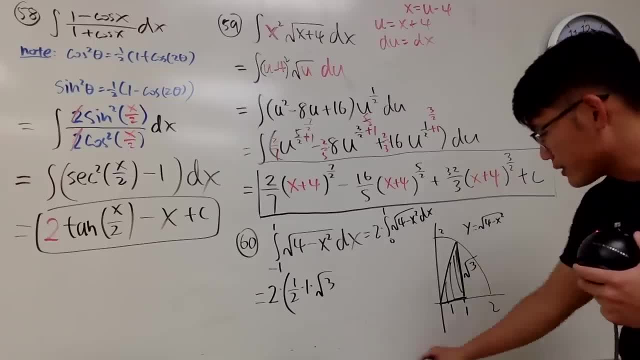 I'll double this anyway. okay, Now I need to figure out this right here, because you want to go from 0 to 1, so you need to go from this right here, which is 0. And you need this. 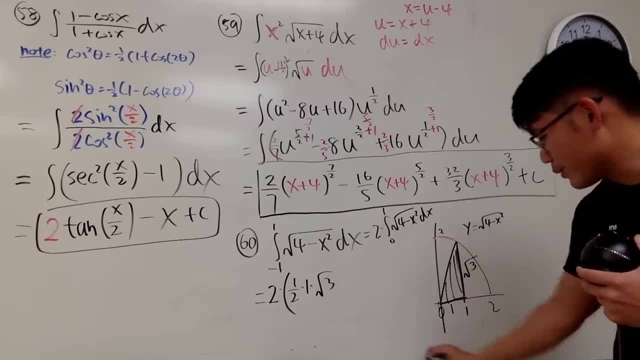 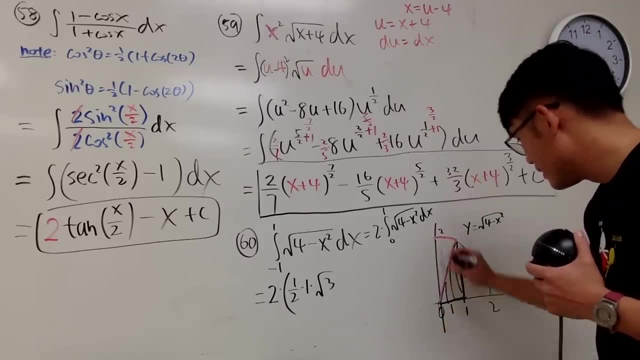 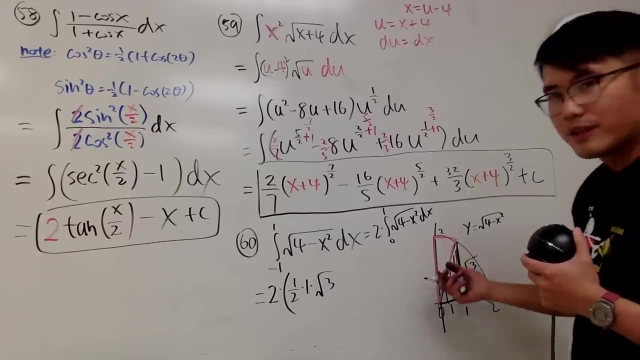 which is the area of a sector, And this marker is not the one I want. This is. I have a lot of markers right here just to get ready, So the area of a pizza. pizza sounds really good now. Well, first of all, 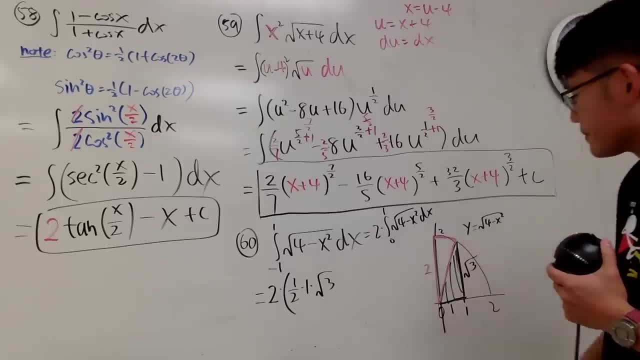 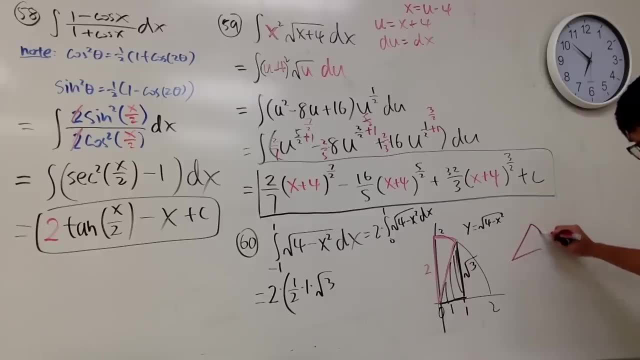 we have to know that the radius is 2, right? And how do you find the area of the sector? Don't worry, I will write it down right here for you guys. So when you have a circular sector like this and when you have the angle theta. 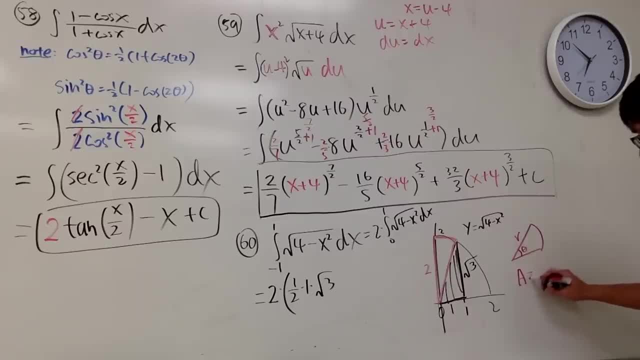 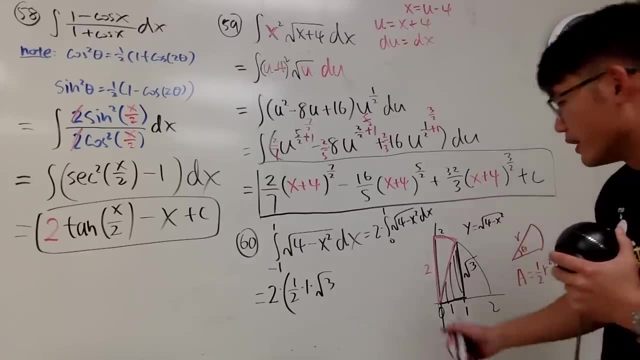 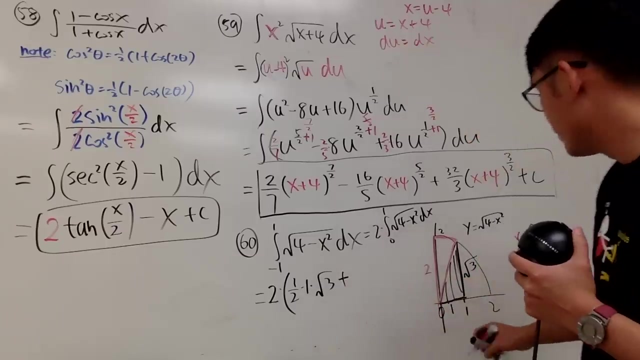 here with the radius r, then let me tell you: the area is equal to 1 half r squared theta. Alright, So r is 2.. That's okay, And of course you have to have this black triangle plus the red sector, so you have to add: 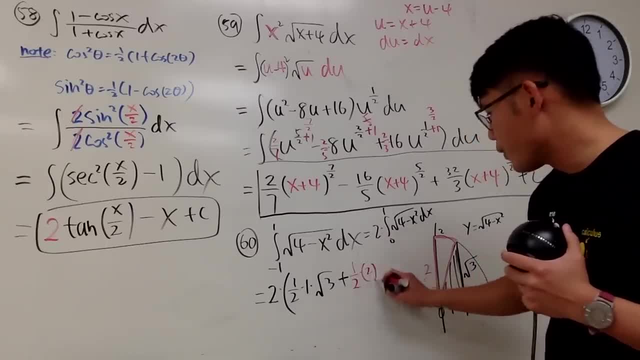 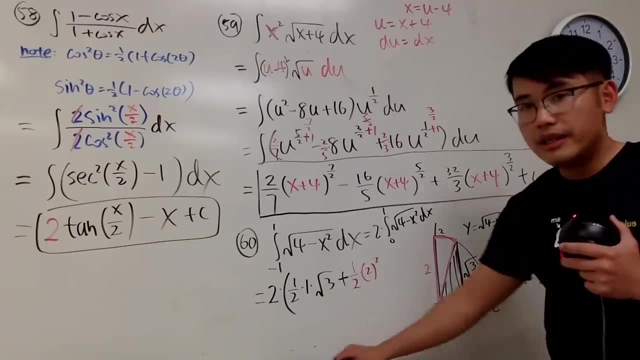 first, let me just put down the 1 half times 2 squared. That's good, And now we have to figure out the angle theta. Well, where's the angle then? The angle is of course, this right here: This is the angle theta. 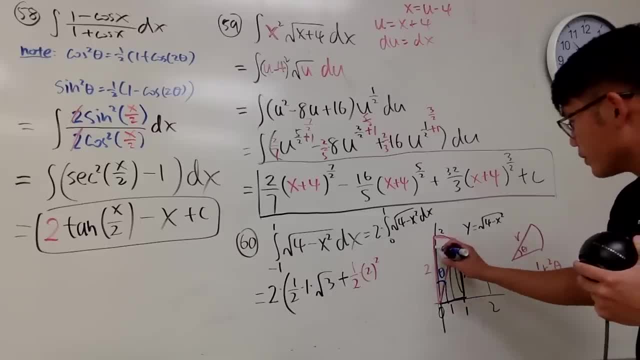 But how can we do it? Notice this: right here is 1.. So of course, you know this. right here will also be 1.. And check this out. You have a right triangle now by looking at this. You have a right triangle now. 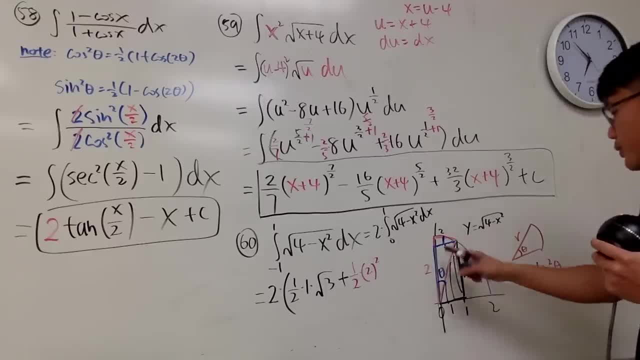 like this And you don't know this, unfortunately. Well, you do know, but we are not going to use it. Let's use 2.. This right here is 2 as well, Because when you use this, you can use the inverse sign. 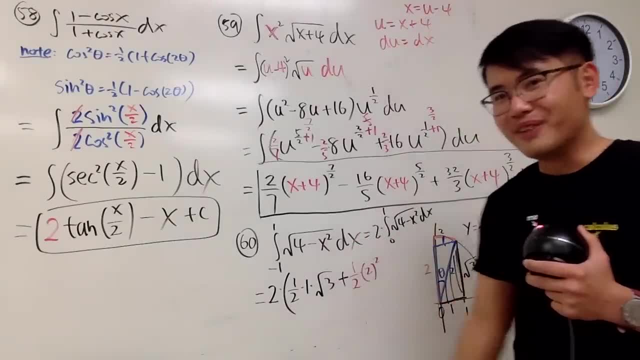 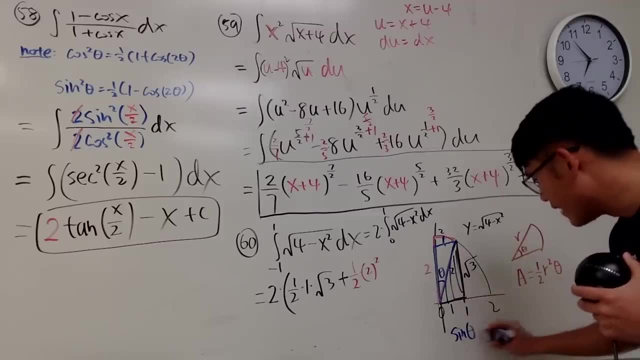 And in fact, if you do this by tricks up, you end up with the inverse sign somewhere as well. Anyway, in this situation, you know that sine theta is equal to opposite. This is the opposite over adjacent, which is 1 half. 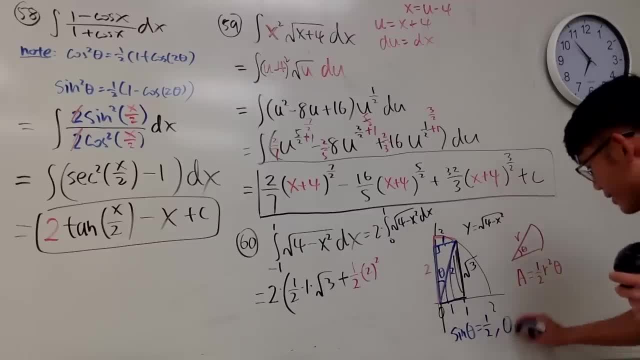 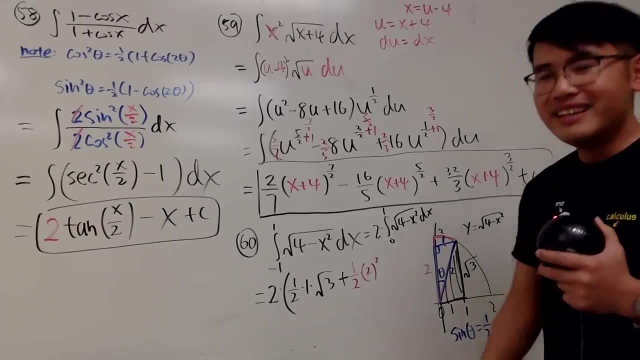 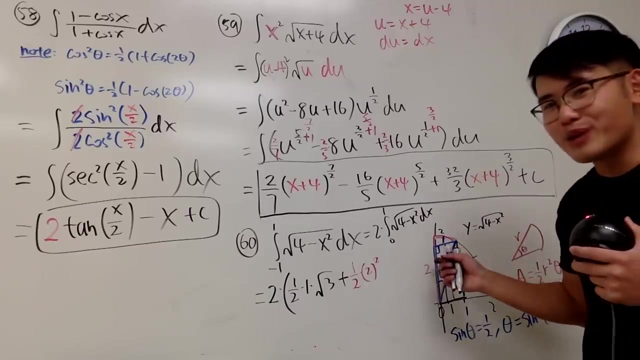 Like that. So can you guys tell me what's theta? then Of course it's the inverse sign of 1 half. But seriously, can you guys tell me sign of what will give me 1 half? Well, this is a special right triangle. 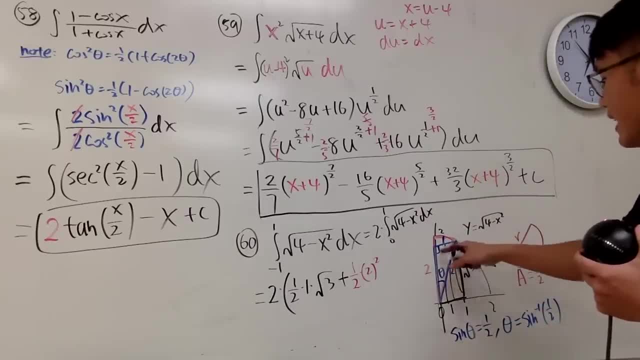 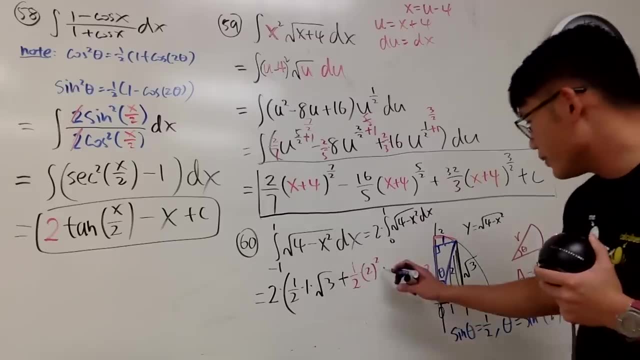 isn't it? Yes, it is. This is 30,, 60,, 90 special right triangle. This is 30 degrees, which is what Pi over 6.. So you just multiply by pi over 6. Like that, And you are pretty much done. 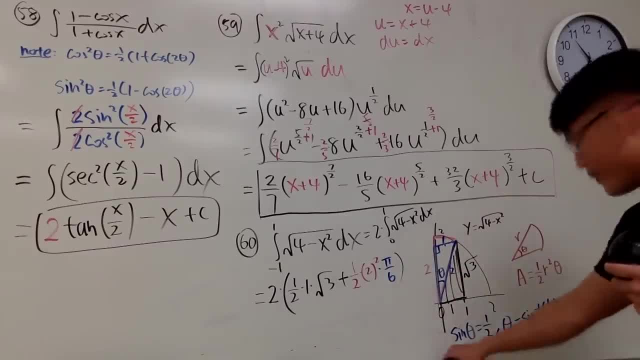 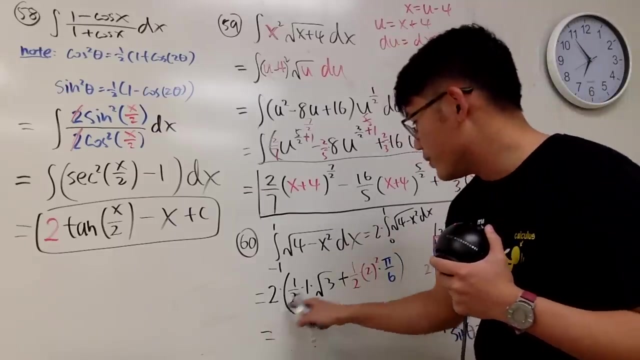 Okay, So this right here is pi over 6.. For the 30 degrees: Okay, Let's see if I can do this map in my head. First of all, 2 times. this is just gone. You have square root of 3.. 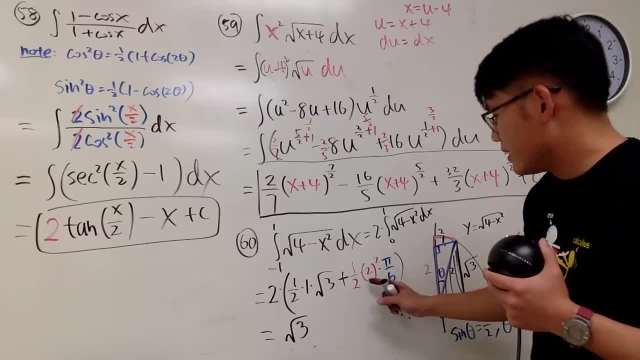 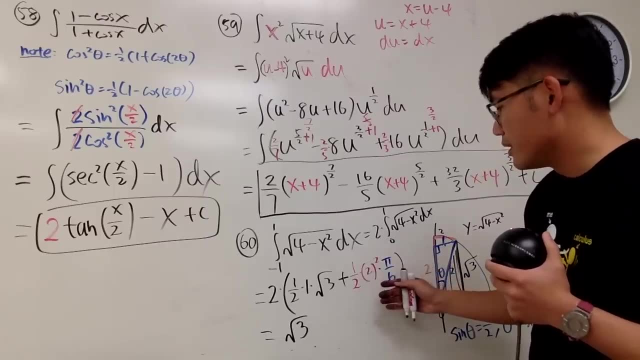 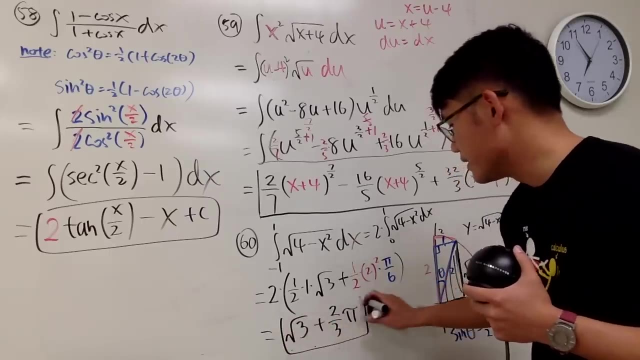 Alright, Check this out 2 times. this is gone. You have 4.. 4 times something over 3 is 2 thirds. So plus 2 thirds And you have the pi next to it. I believe this right here is the answer. 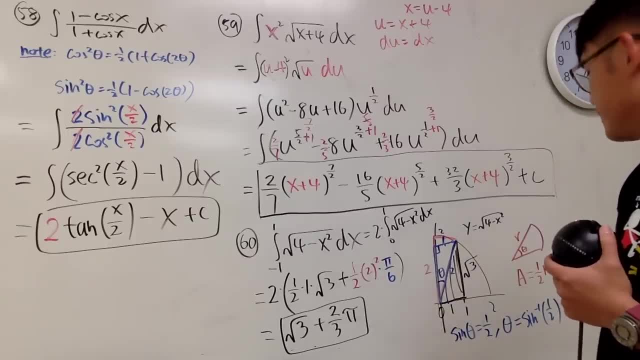 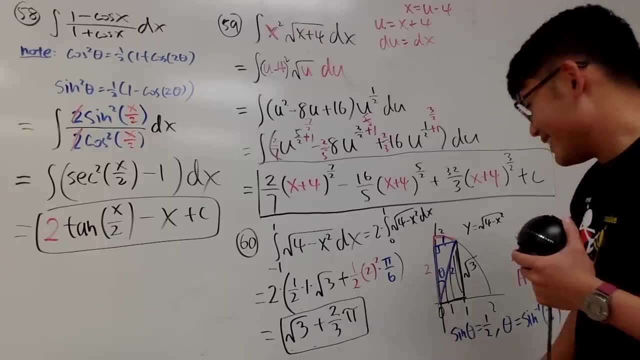 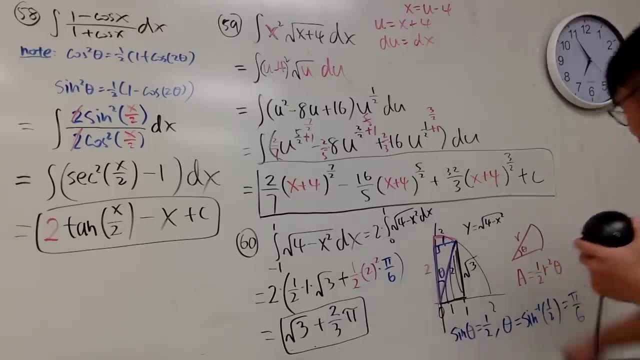 Let's see- Yeah, I think so- Let's see 4 beyond 2.. Yeah, That's it, That's it. And in fact, if you use this- that would be square root of 3- and use the inverse cosine And you just 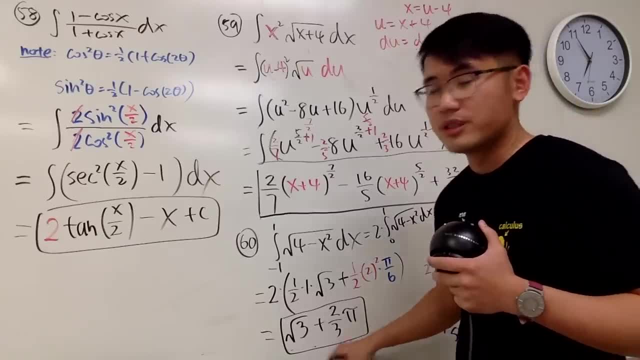 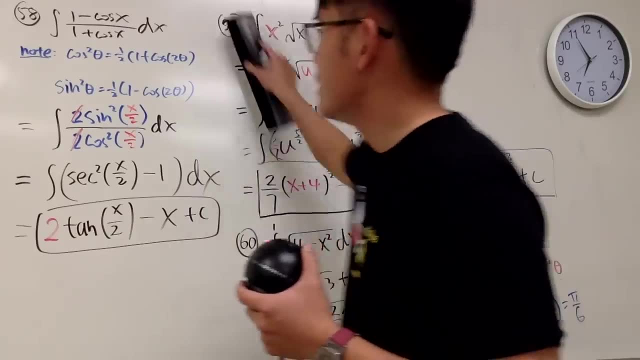 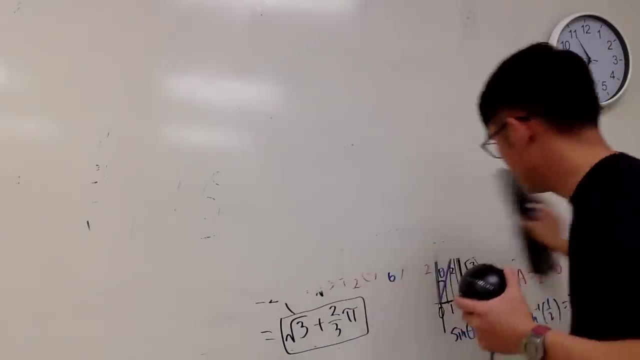 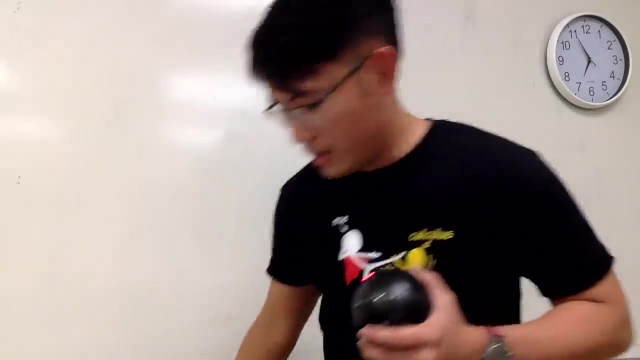 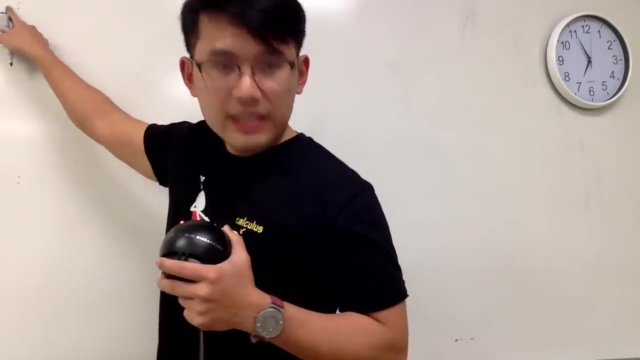 get the angle, You still get the same angle anyway, So it doesn't really matter which one you use. Okay, So 40 more to go. Oh my goodness, Alright, Number 61.. 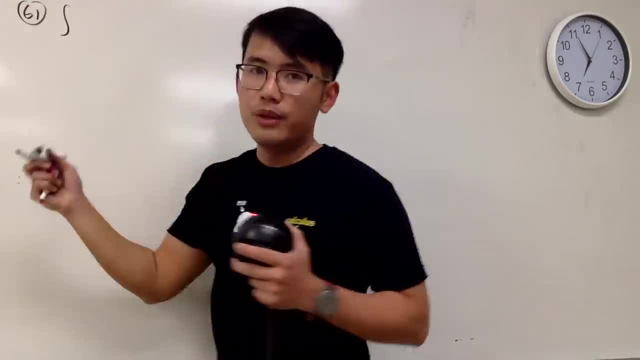 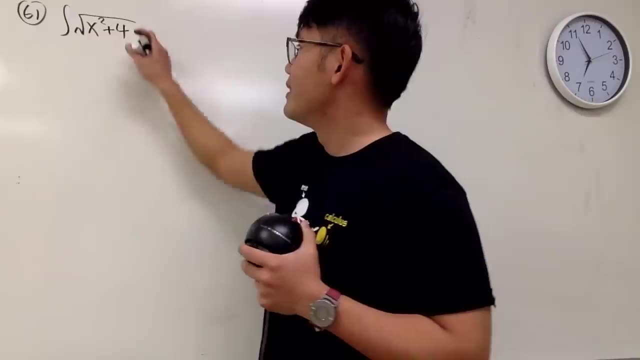 Alright, Number 61.. This is also a pretty long one, so I'll do it fast. Square root of x, squared plus 4.. So what's next? Next to it? dx. So this is the one I have planned. 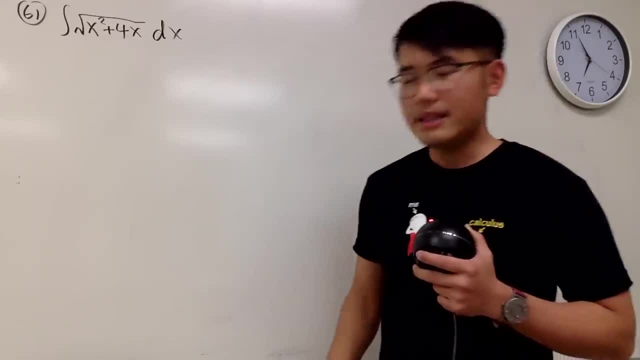 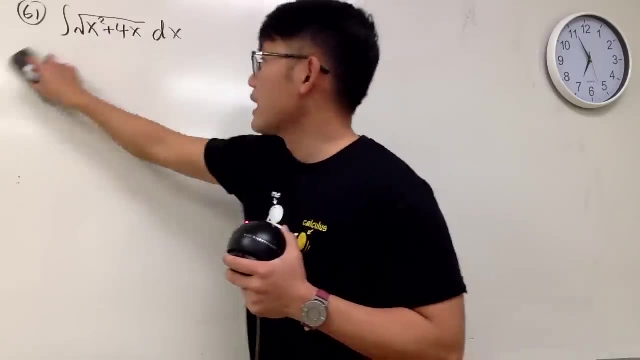 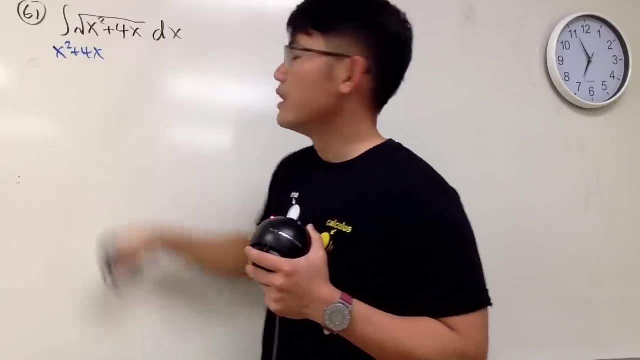 for you guys. okay, Tricks are not now. You have to complete the square first To do so. well, let me just make a note right here for you guys. Here is the idea: When you have x squared plus 4x, 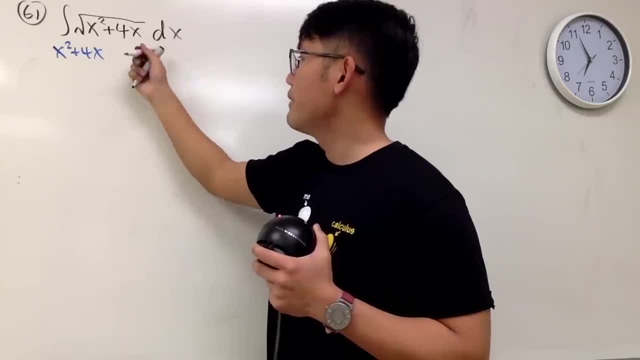 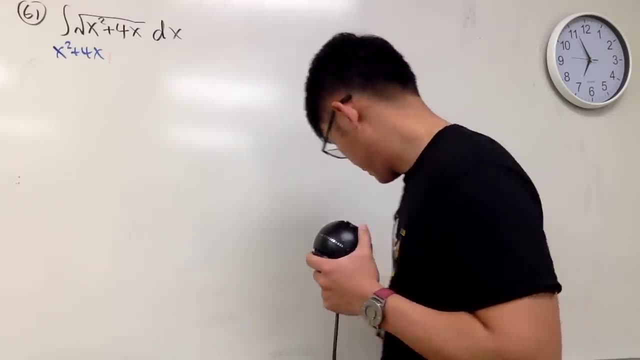 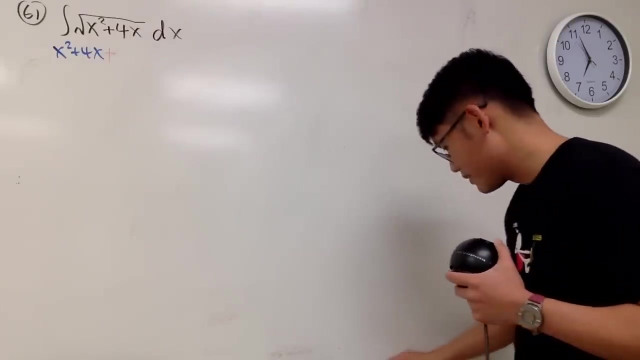 to complete the square, you need a plus 4. after that, right, This marker doesn't work. No, It's not the one I want. This is the one You want. to add the 4. after that, This marker doesn't work anymore either. 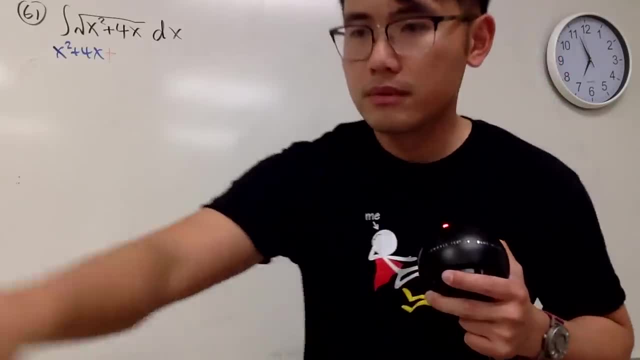 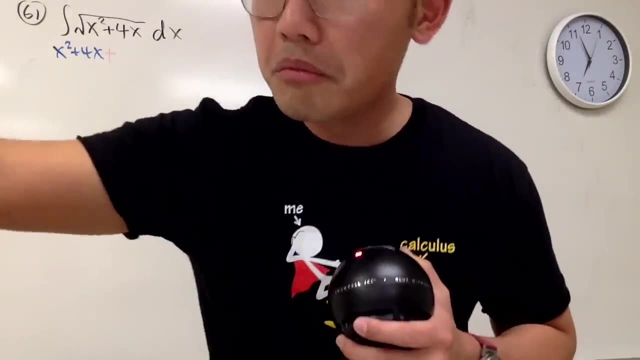 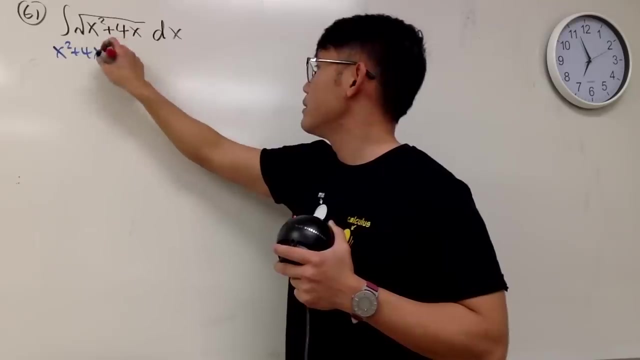 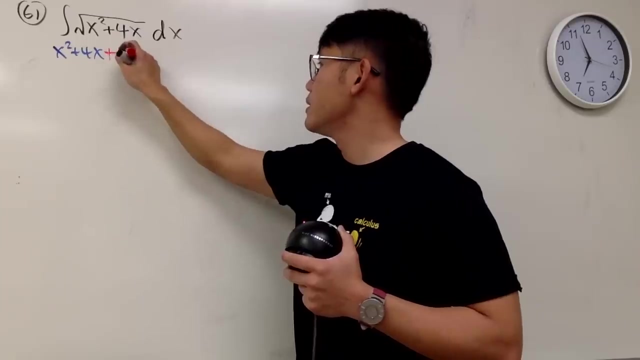 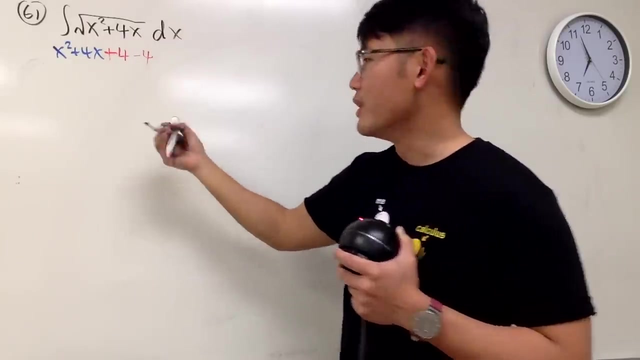 Use this one instead. Okay, Add 4, and then minus 4.. Alright, This right here will be a perfect square: x plus 2 squared. and then this right here is minus 2 squared. 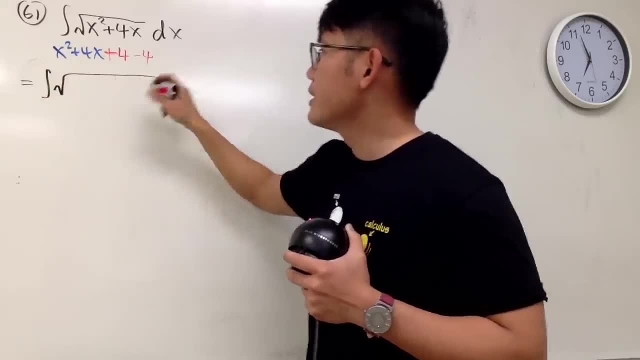 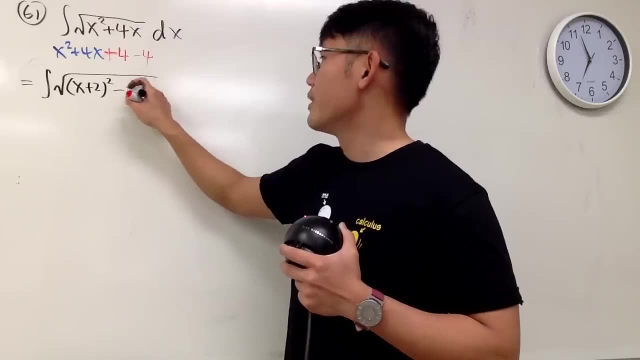 So here we go. This right here is going to be the integral and you have the square root. Let me just put down this right here as x minus x plus 2 squared, and then minus 2 squared. right here for you guys. 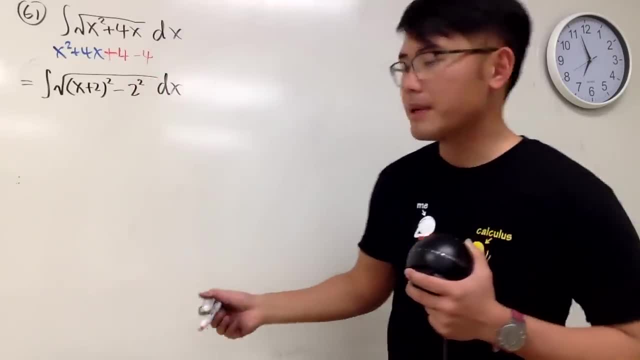 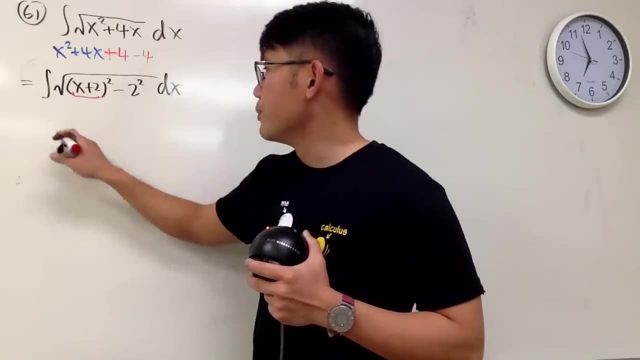 dx. So this one: here we are going to do a trick, sub alright. So this one, we'll actually do it legitimately. So I will take this right here, this input, to be my secant. I want x plus 2 to be my. 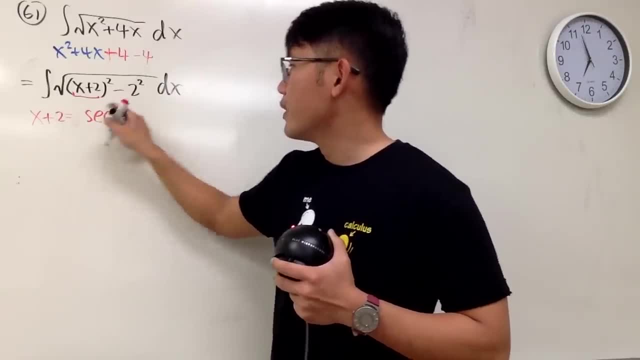 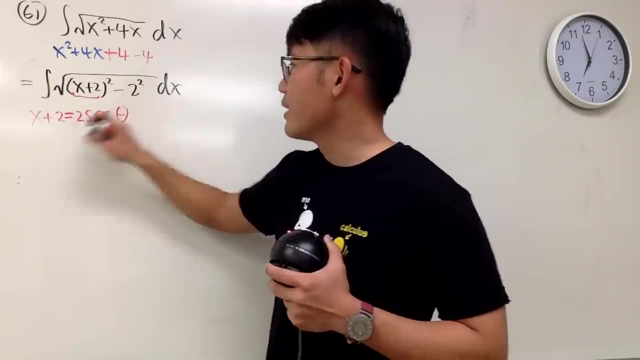 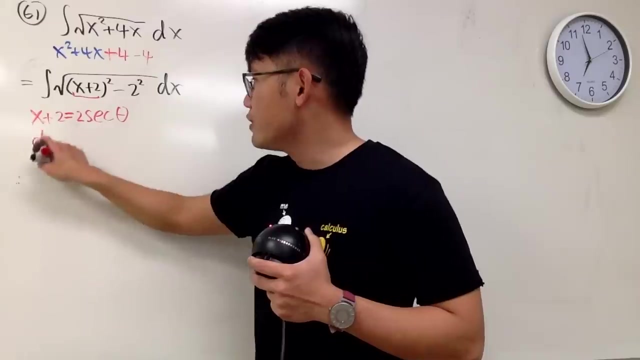 secant. But here is the deal. We have a minus 2 squared, so it's technically my 2 secant theta right here. okay, Technical difficulty, I'm sorry, With the markers. Okay, Now differentiate both sides. 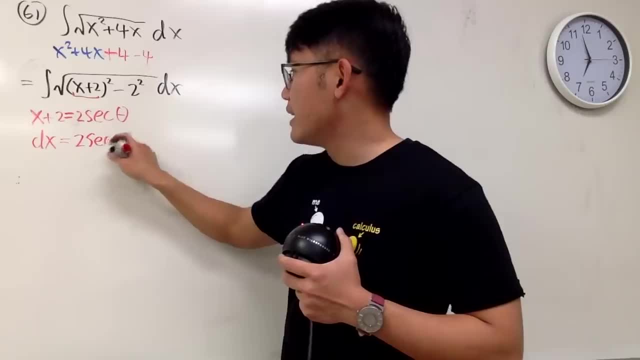 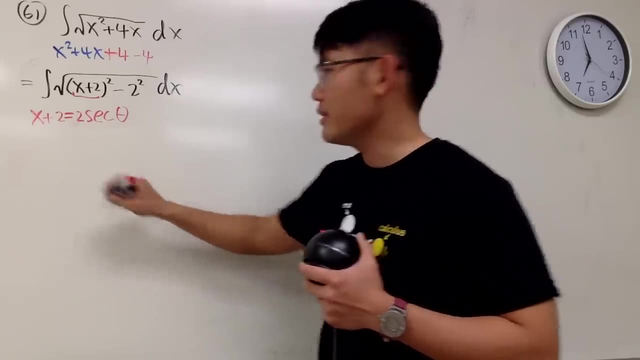 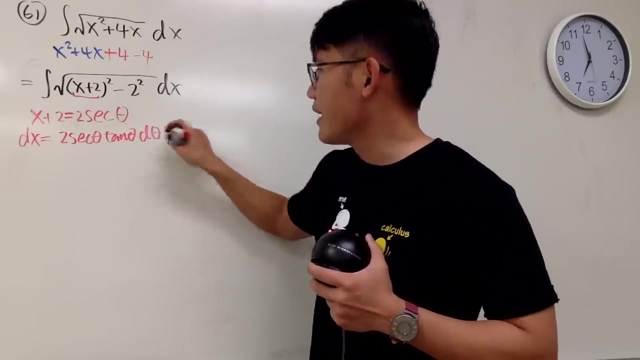 dx will be the derivative, which is 2 secant theta. Let me actually write it down. Yeah, I think this is okay. dx is equal to 2 secant theta, tangent theta, d theta, And now we'll take this integral to the. 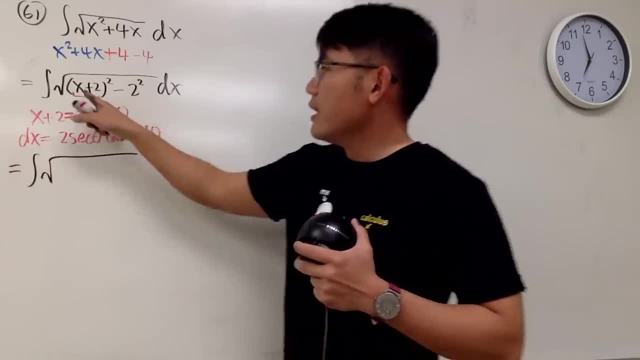 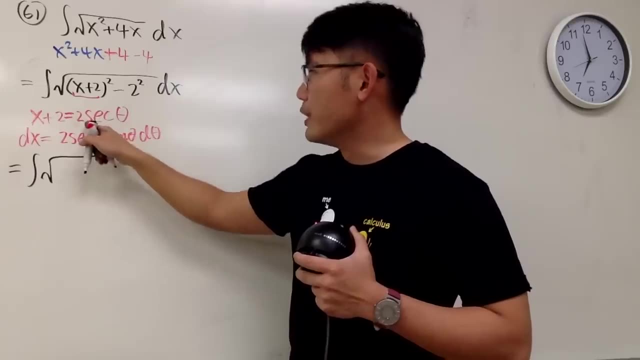 theta world. This is going to be the integral of the square root. Okay, This right here, Let's do. Let's just do this. This right here. I'll put the 2 secant theta inside and then I'll square that. 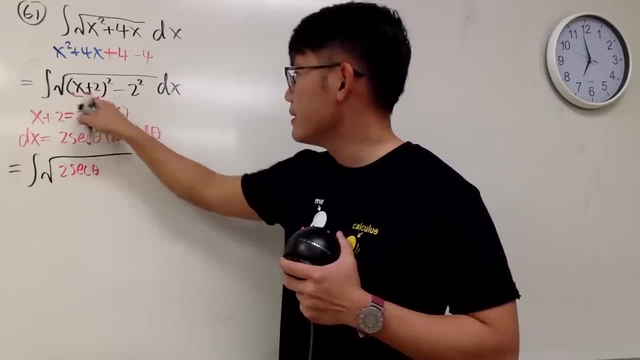 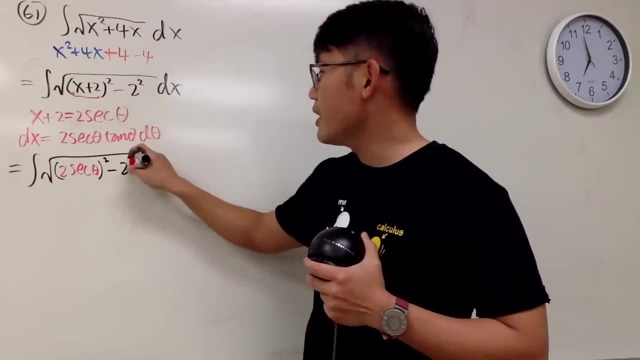 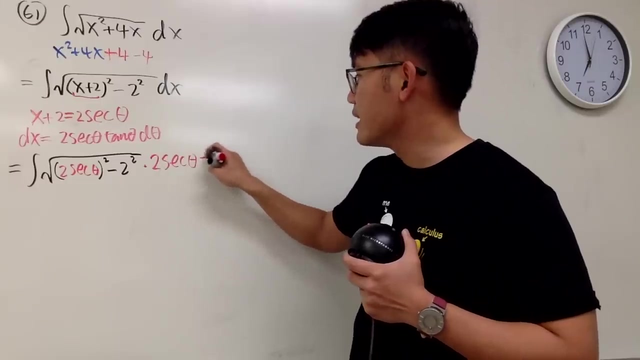 So 2 secant theta- okay, This is my whole this. and then I will square this guy and then minus 2 squared and then dx is all that, which is 2 secant theta, tangent theta, d theta. Now we'll see. 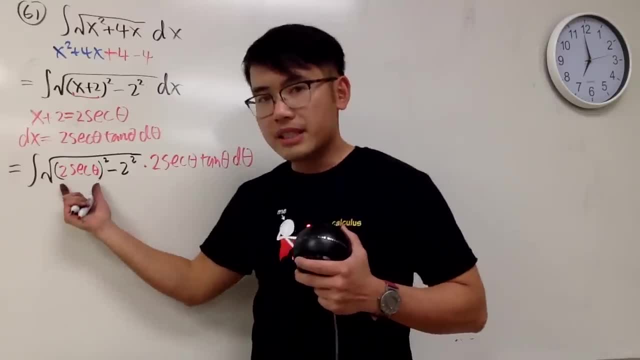 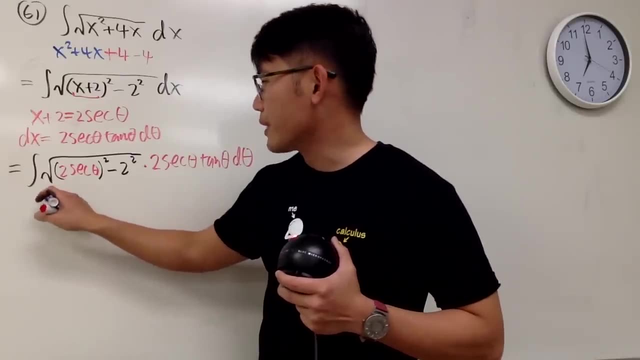 let's just do this right here real quick. This is 4 secant squared minus 4, factor out the 4, and you have the square root of 4, which is going to be 2,. okay, So let me just 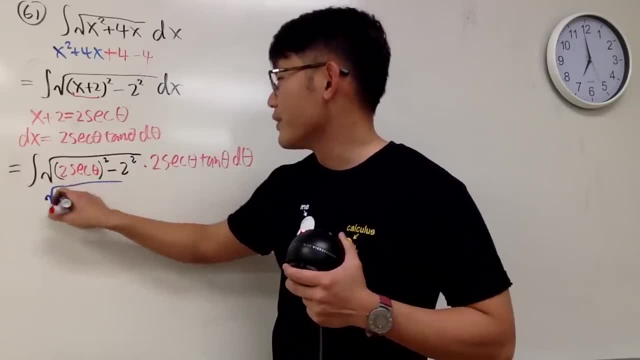 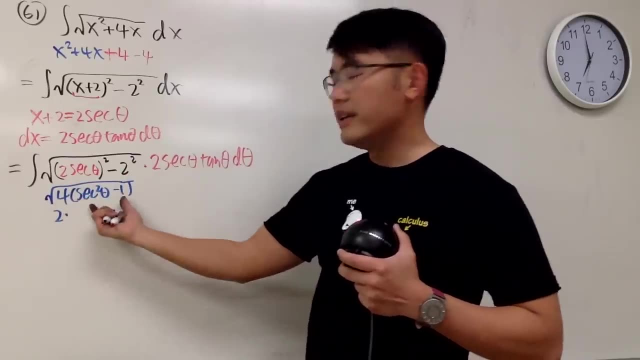 let me show you guys. let me just show you guys the work. There are 4 times and you get a secant squared, theta minus 1.. And square root of 4 is 2.. Square root of this, which is tangent squared, 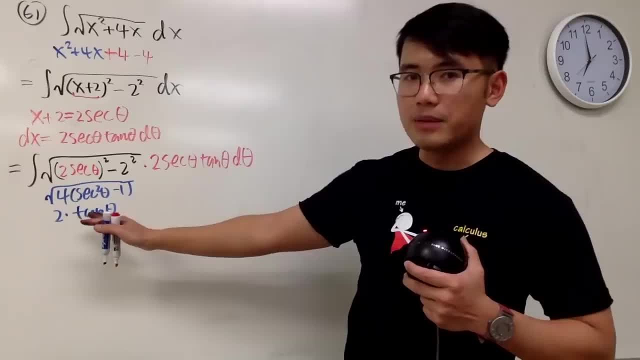 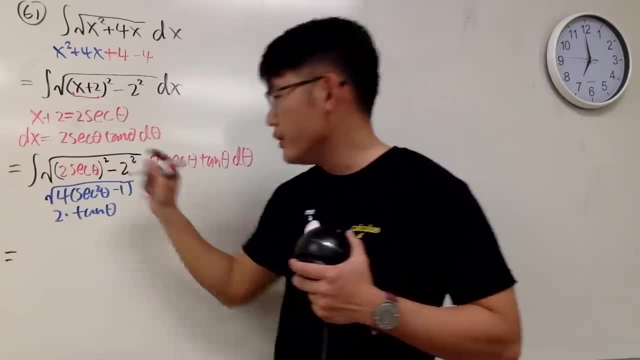 you get tangent. This is not denominator. You have to multiply this with that. Therefore, in fact, you end up with 2 times 2, which is 4.. You can take that outside, and then you have the integral and you have. 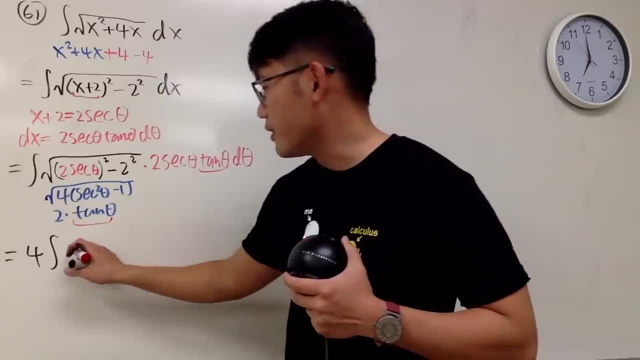 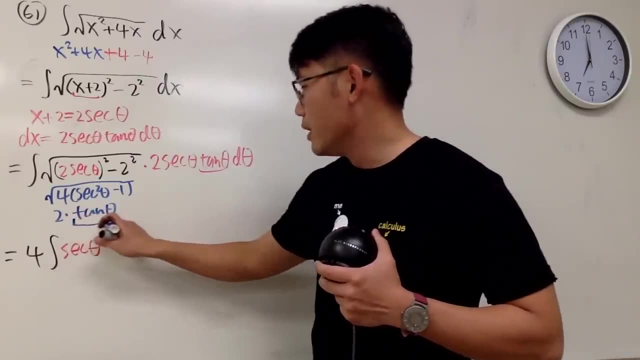 tangent tangent, which is tangent squared, and you have the secant here. So, in fact, let me put down the secant theta here and I will actually do this To integrate secant theta times tangent squared theta. I will 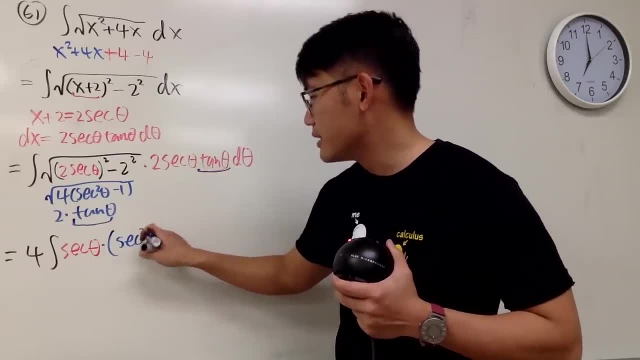 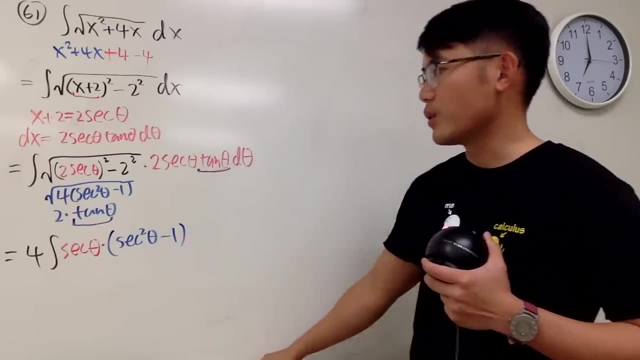 actually first change the tangent squared theta to secant squared theta minus 1, like this right? So again, this times that is secant squared. so that's what we end up with, yeah, And then we have the d. 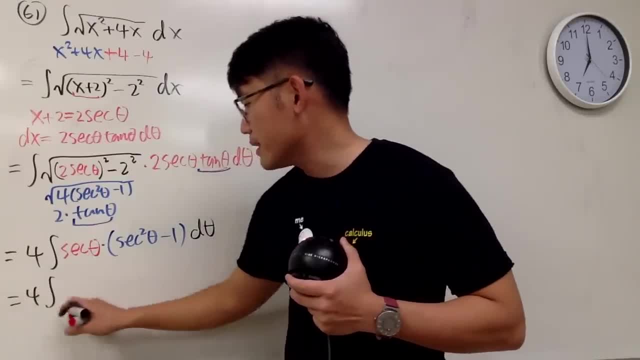 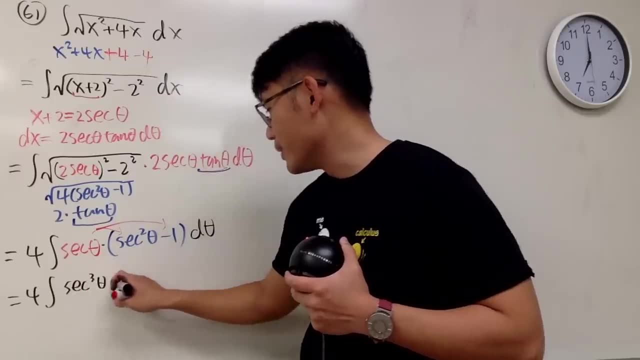 theta, And now you are looking at this as 4 times the integral of yes. this times that is secant cubed and this is the secant to the first. Thank god, we did all that earlier, didn't we? Yes, we did. 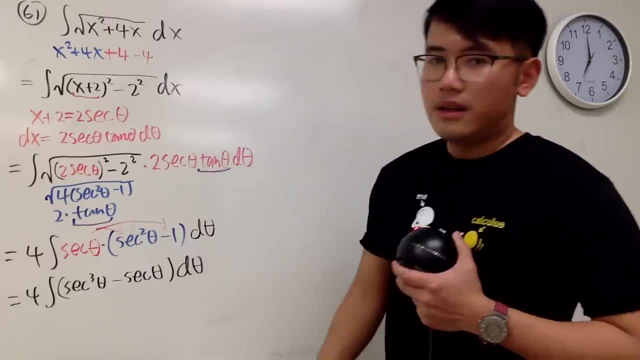 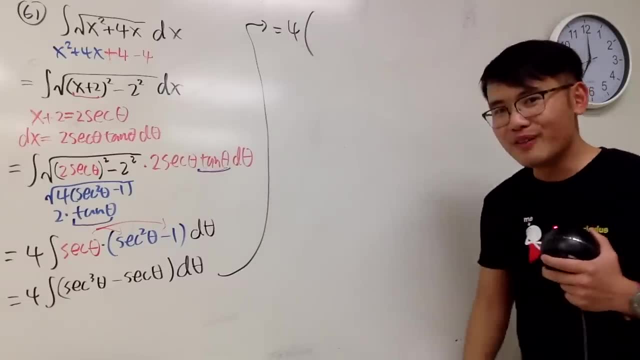 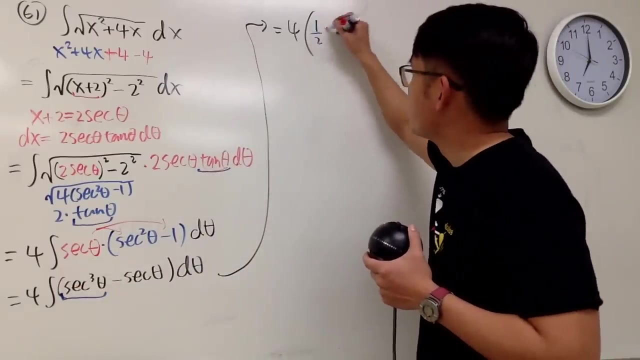 That's nice Sigh Big integral sign 4, and then let's put down the result of the integration. What is the integral of secant cubed? Put this down in blue: 1 half secant theta times tangent theta plus. 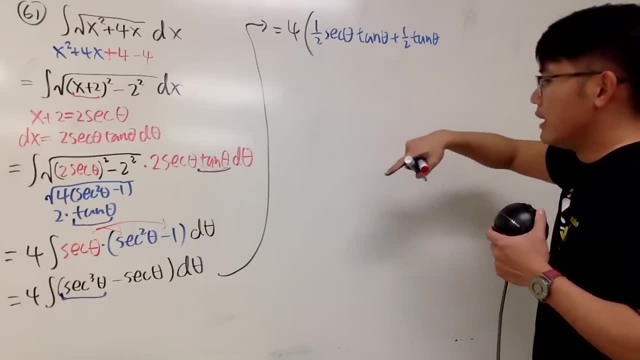 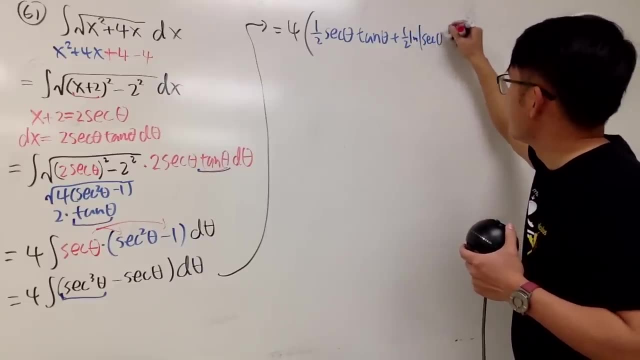 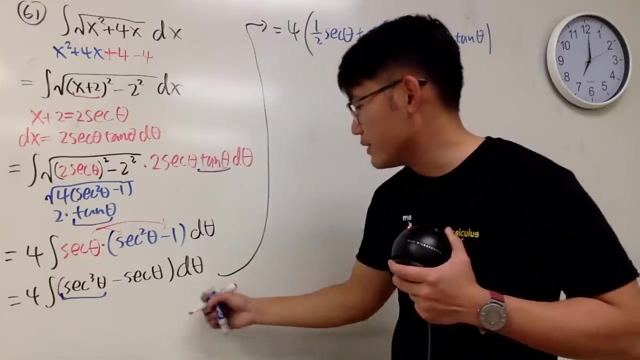 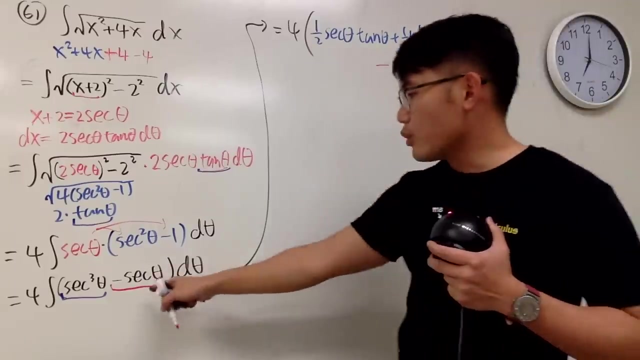 1 half tangent theta, uh, sorry, 1 half ln secant theta plus tangent theta Right. And then we also have to have the minus right here. the minus, uh, secant theta. Well, minus and the integral of secant theta is: 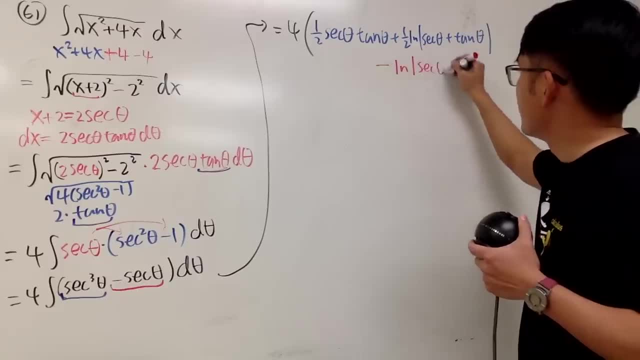 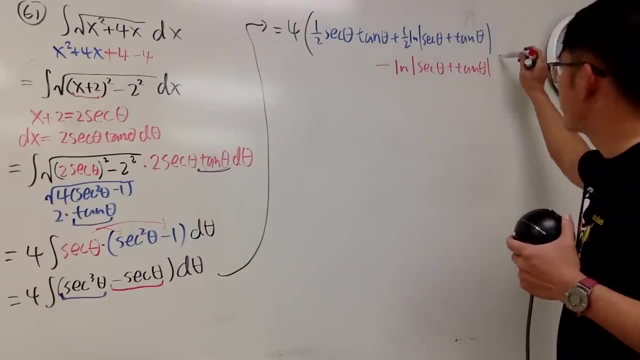 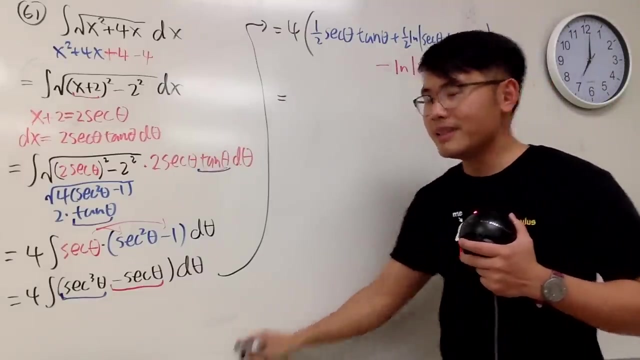 1 ln. absolute value: secant theta plus tangent theta. like this Right, This right here is still in that big parentheses. Now let's do a few things. First of all, let me just combine this and that together real fast. 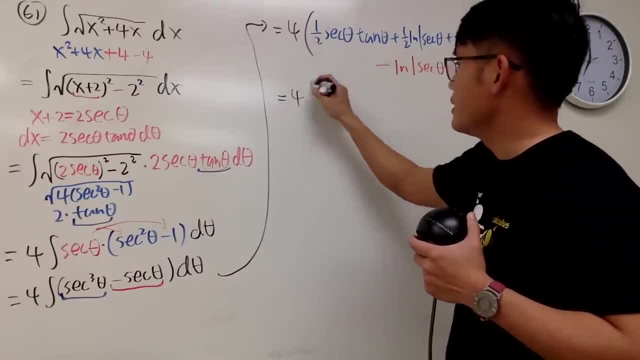 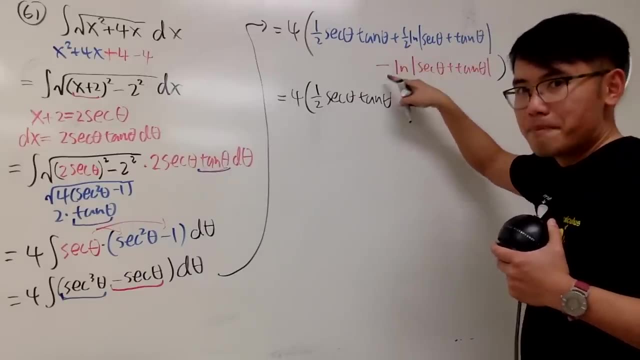 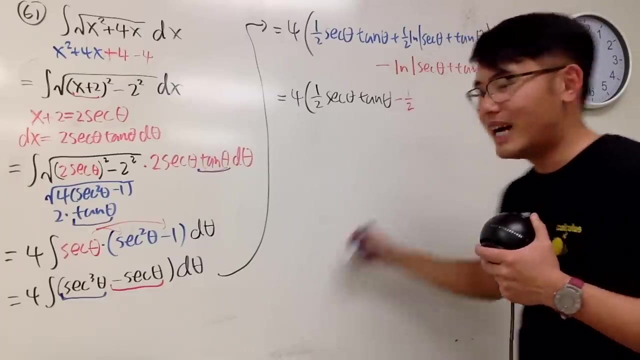 This right here is 4 in the front and the parentheses. this is 1 half secant theta tangent theta. 1 half minus 1 is negative. So let me just write down negative 1 half. And then of course we have: 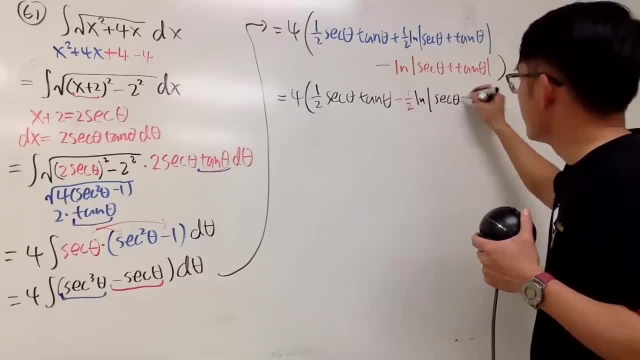 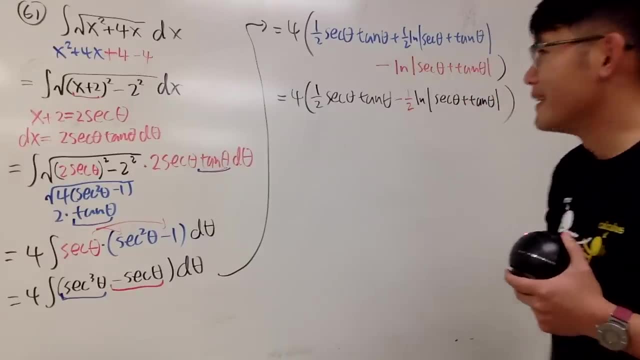 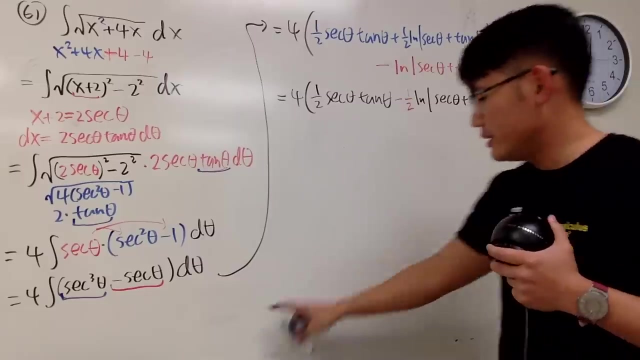 the natural log: absolute value: secant theta plus tangent theta Like that. Okay, Here is the deal, Of course, going back to the uh x-world. So enough talking, Let's take a look at this right here. Let me do this in. 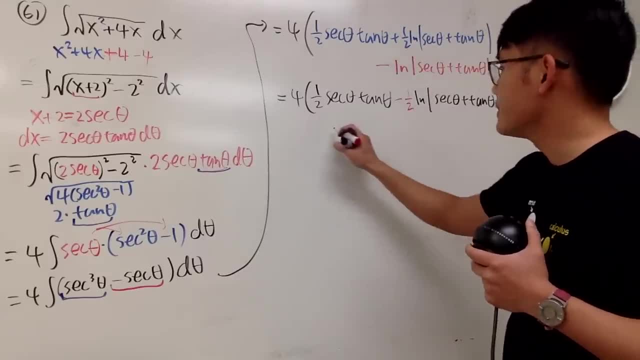 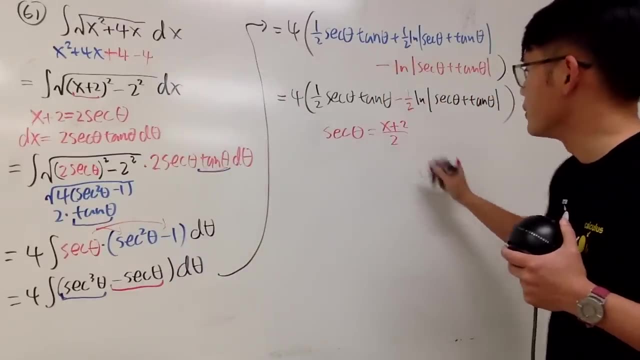 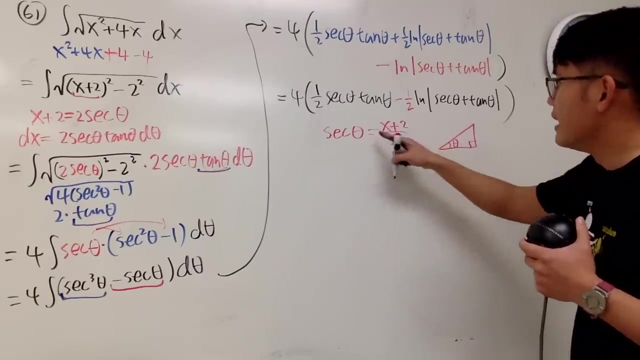 red. We know that secant theta is equal to divide 2 on both sides, So we get x plus 2 over 2.. From here we can draw a right triangle real quick. Here is the triangle and here is the angle theta. 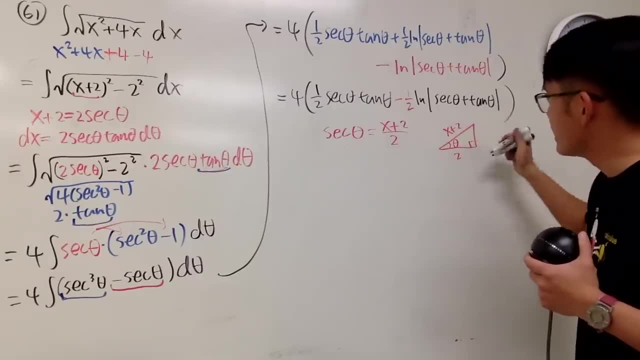 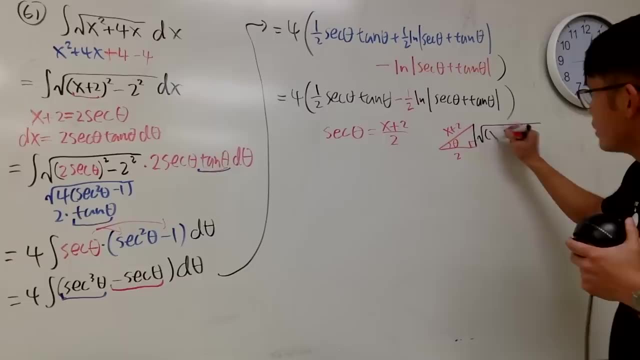 Secant is hypotenuse over adjacent, and the opposite side is going to be the square root of this square, minus that which is square root of x, plus 2 square minus 4, right, Minus 2 square technically, but it's minus 4 anyway. 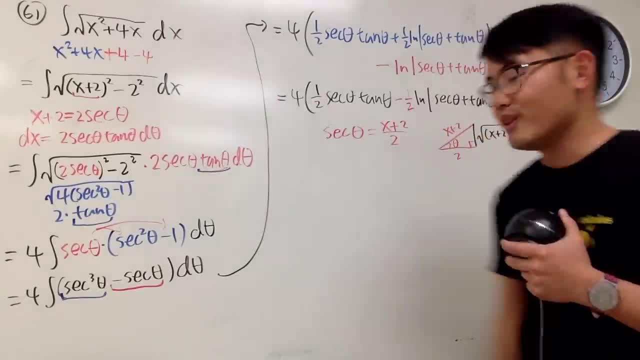 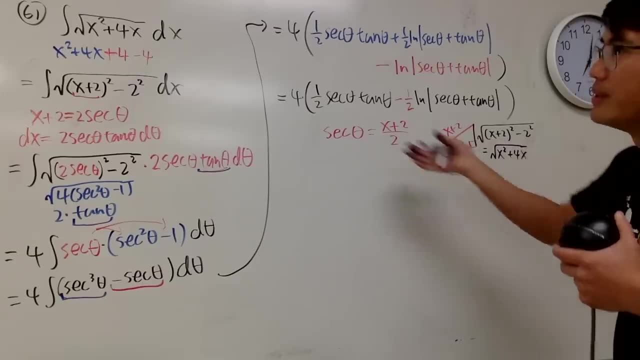 And guess what? This right here is the original. So this right here is the same as square root of x, square plus 4x. You see how much trouble we have if you don't have the right thing. So yeah, Anyway. 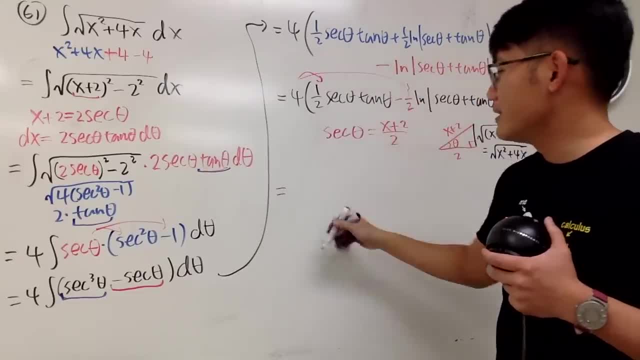 I think we are ready to go though This times, this, this times, that This times, this is 2. Don't forget: the 2. Secant theta is this: so I'll put this down in red. So we have. 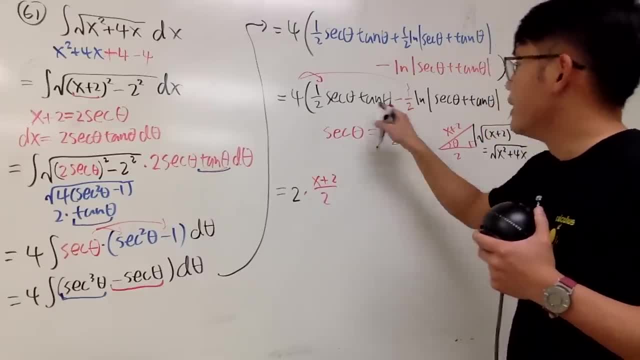 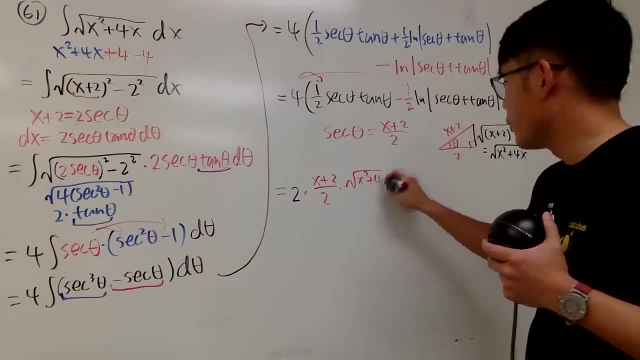 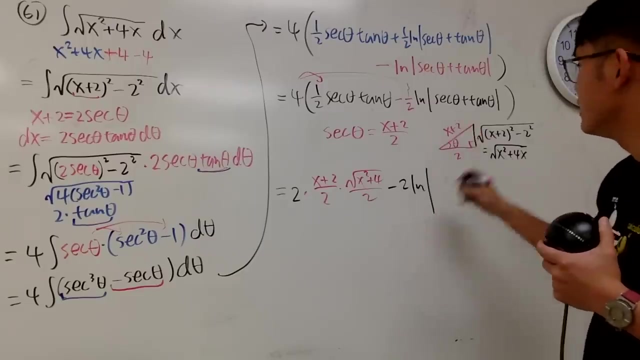 x plus 2 over 2.. Tangent is what Tangent is this over 2, so we multiply by square root of x, square plus 4 over 2.. This times that is minus 2, natural log absolute value. Secant is: 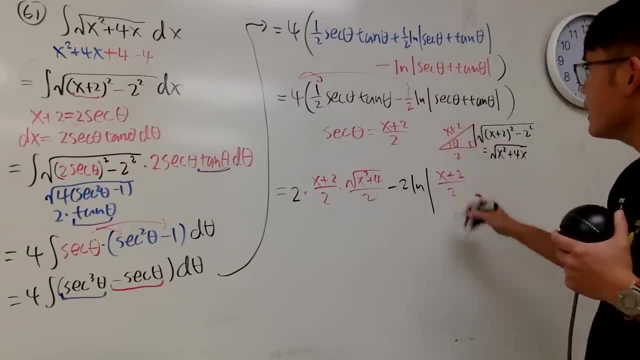 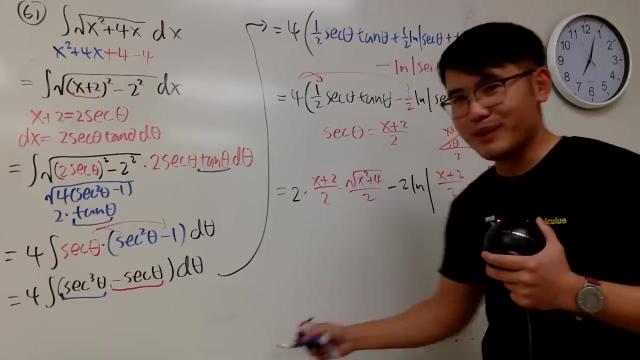 this again: x plus 2 over 2, and then we add this over 2 for tangent, So square root of x, square plus 4x over 2.. Very good, very good, very good. Of course, you can do better. 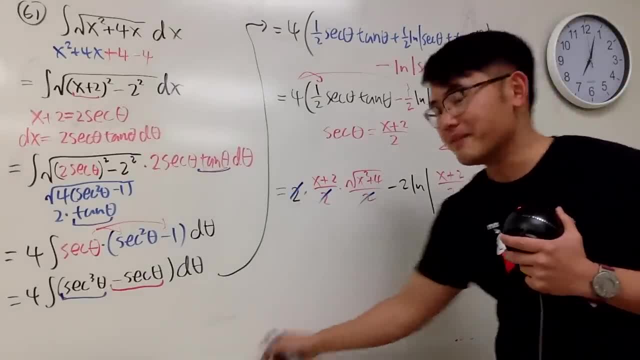 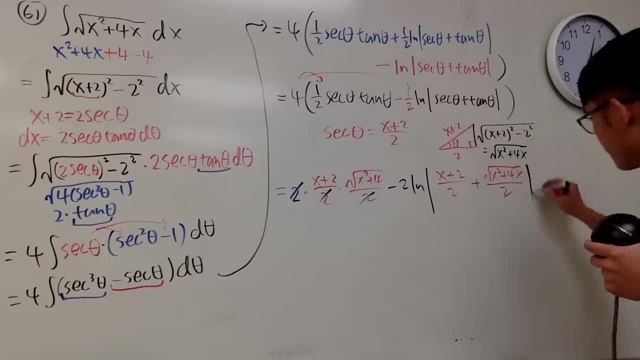 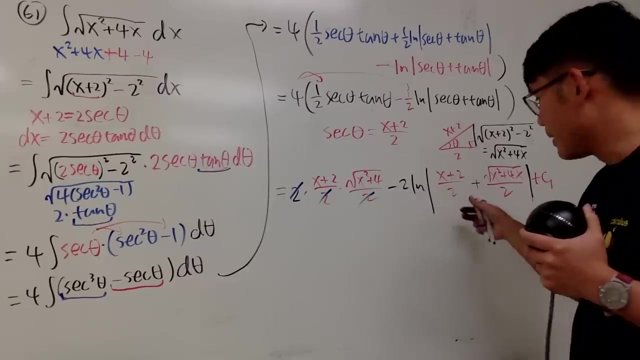 First, this, this, this, they all cancel. Second, this is technically plus c1. I should put this down in red: Technically plus c1. Because right here again you have the natural log of the top divided by the bottom. 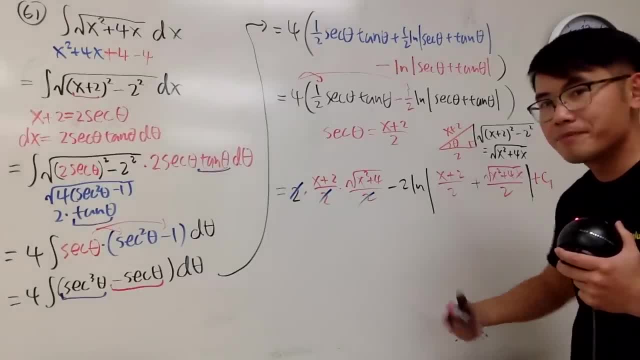 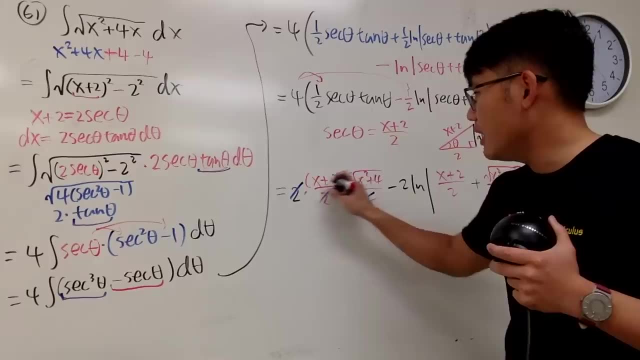 So you have natural log of the top minus the natural log of the bottom, which is a constant. You're going to combine with that constant This right here, of course, put parentheses around the x plus 2.. Finally, I'll write this down right here for you guys. 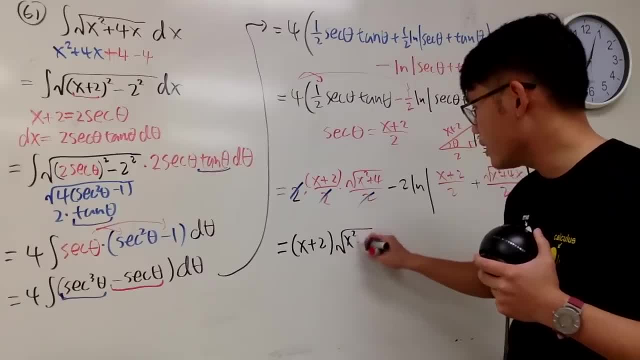 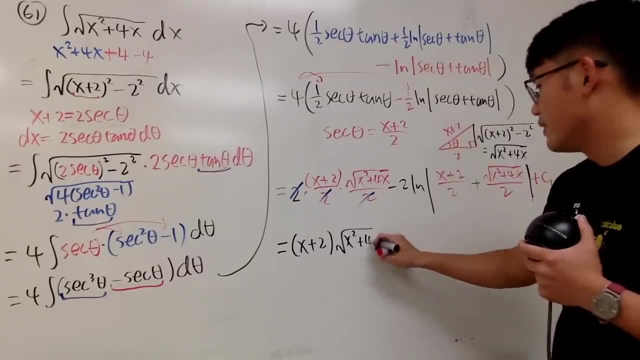 x plus 2 times the square root of x. square plus, it should be a 4x. Okay, It should be a 4x. I caught my mistake. Oh, that's good, But I'm not sure if I made any mistakes earlier. 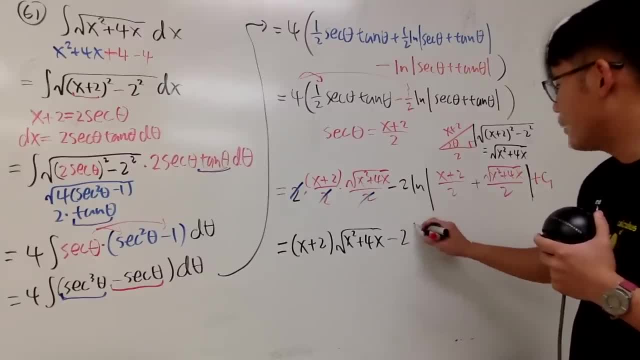 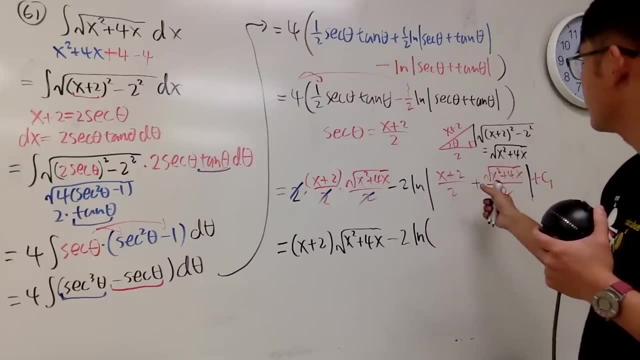 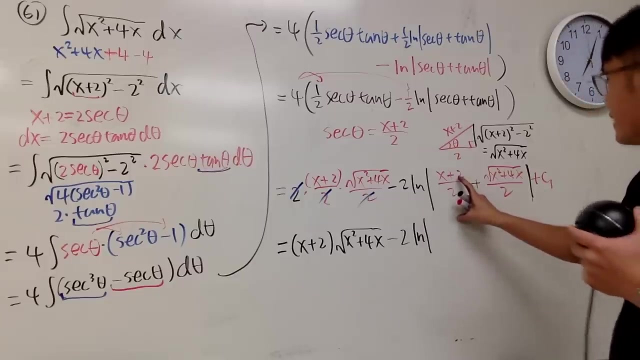 or not, though Minus 2.. I will just put a natural log of the top, which is just this. And the truth is, I think this sometimes could be negative. I believe If negative is uh, x is a big enough negative. 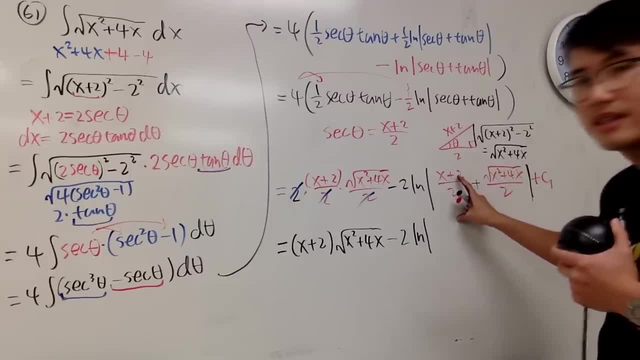 number, I think Let's see. if x is negative, I don't know. Well, this is longer than that. If x is big enough negative, let's see. Okay, Do I need absolute value or do I need parentheses? Let's see. 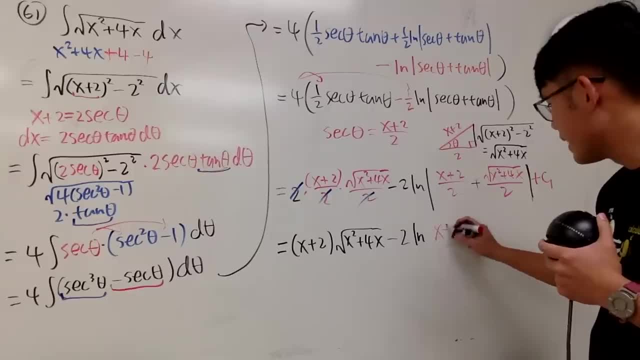 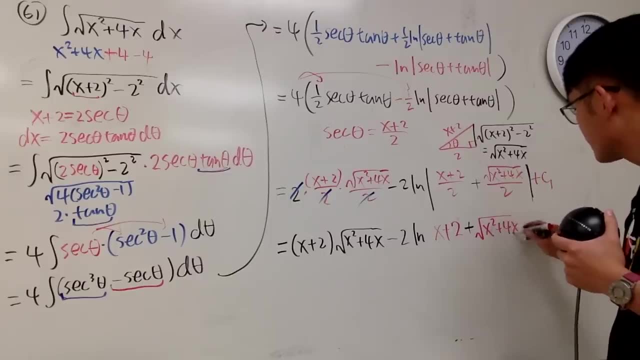 But what I'm saying is I will just put down x plus 2 along with the square root of x, square plus 4x. If x is negative 5, this is going to be negative 3.. This is negative 3.. Negative 5. 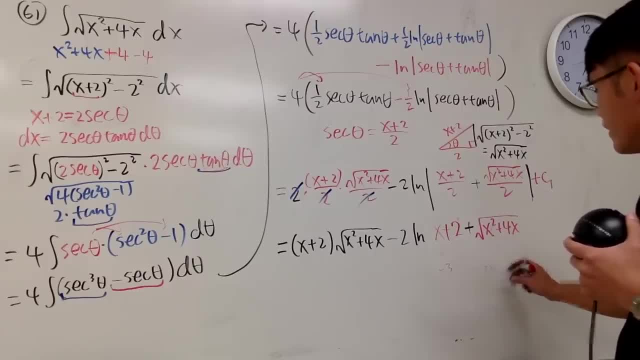 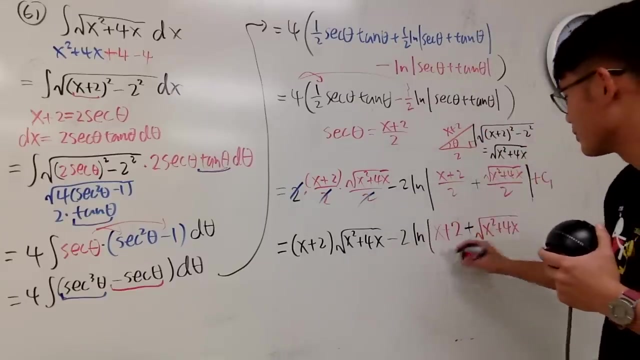 is going to be 25.. Negative 5.. Yeah, Wait, Negative 5 is 25.. And then minus 12.. Okay, Well, you know what? I'm not going to worry about the absolute value or not, I'll just put down absolute value, just to be safe. 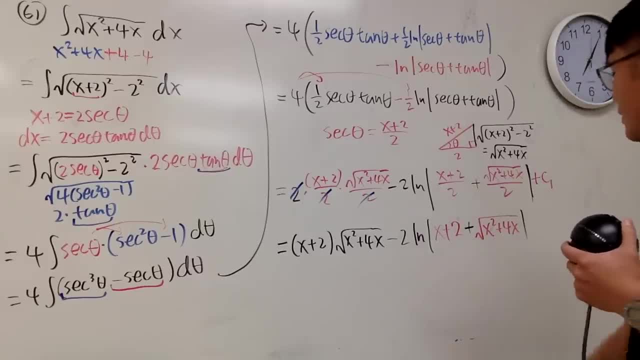 Don't. don't. don't be mad at me if I have the absolute value, But the deal is that divided by 2, that's just a constant. Okay With all that. So I will just put down, finally, plus c2.. 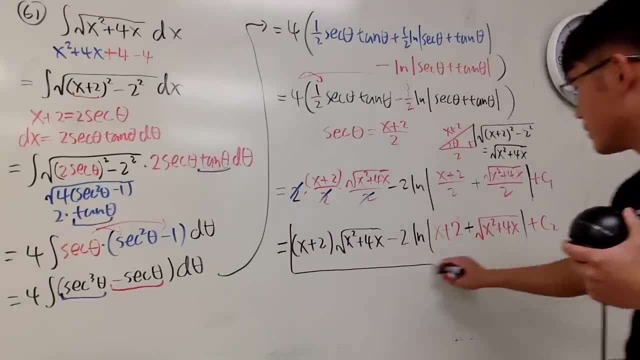 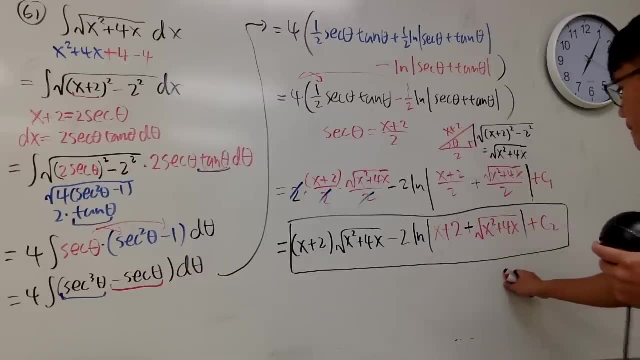 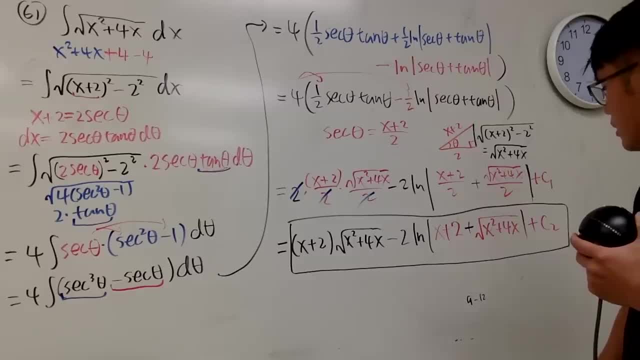 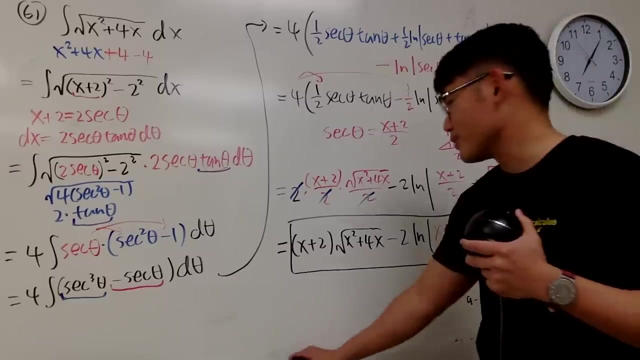 Wait, If x is negative 3, how come x cannot be negative 3? Negative 3 will be 9.. And then negative 3 times, that is minus 12.. Which is no good, You know what? Let's not worry about the domains whatsoever. 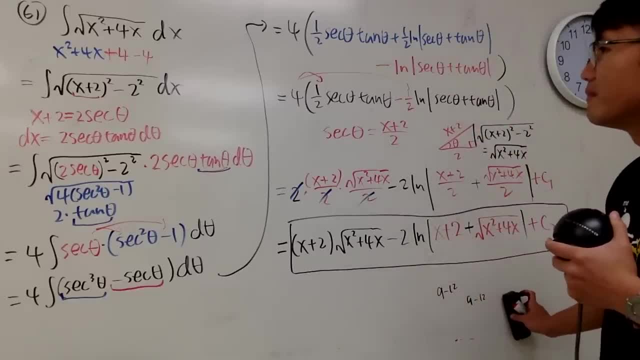 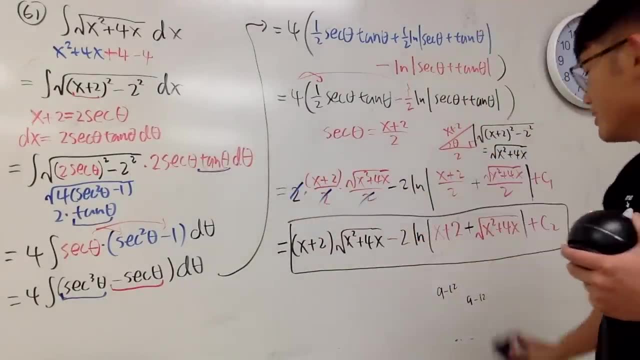 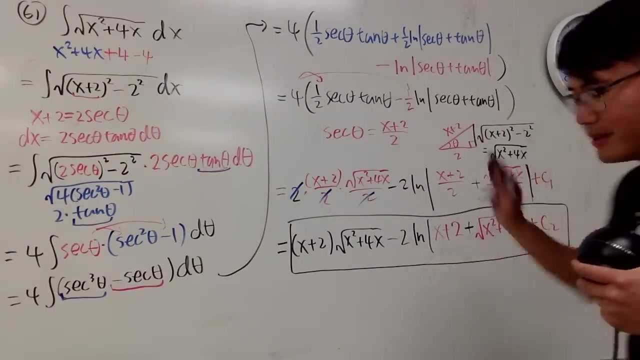 Yeah, So, Oh, I see, Because you have a hyperbola and then you shift it around places, all that stuff. So Just just worry about that on your own. But I showed you guys the integration step. I just 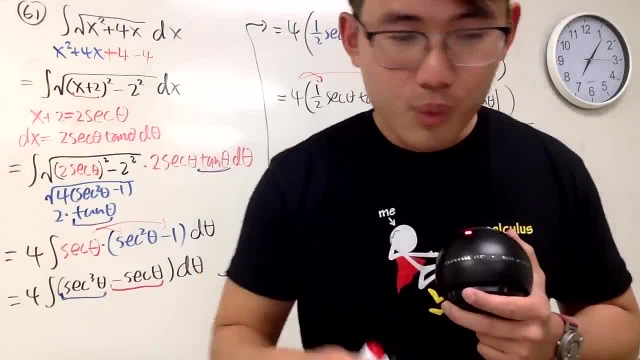 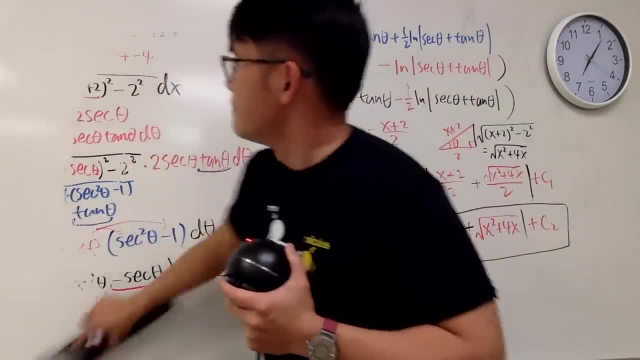 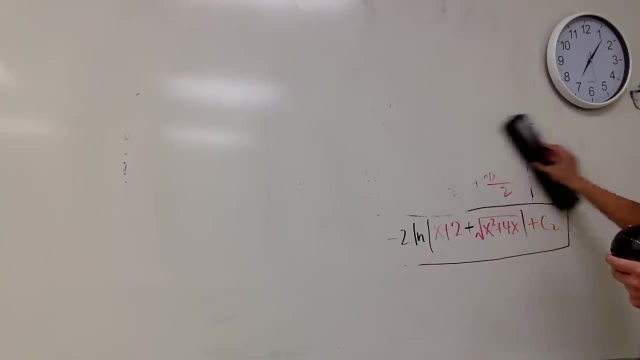 That's all. Okay. So that was 61.. Took us a long while to do that, Okay, So take a look. Alright, Well, that was like the first question that I actually have to use the whole board, huh, Because the other ones? 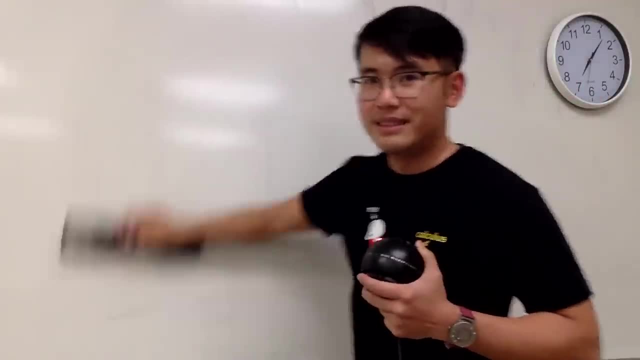 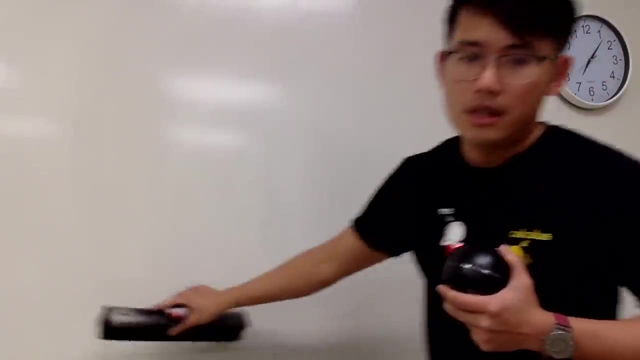 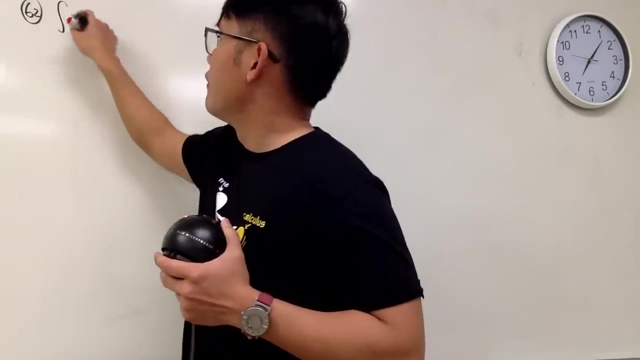 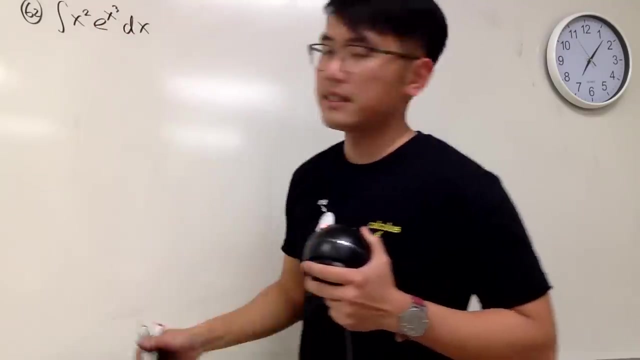 I can kind of fit into the other ones. Alright, 62 integral of x squared. And then we have e to the x cubed dx. This is how I show you Check this out. It's nice, because the derivative of x cubed is what? 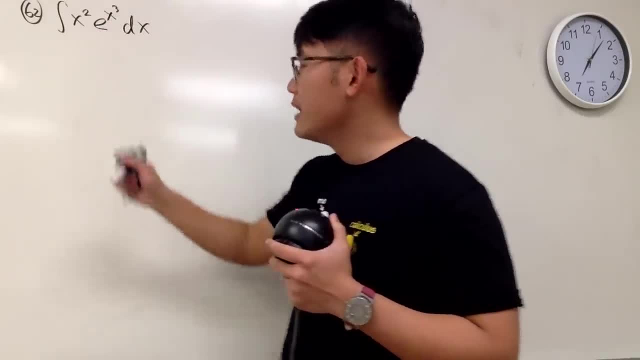 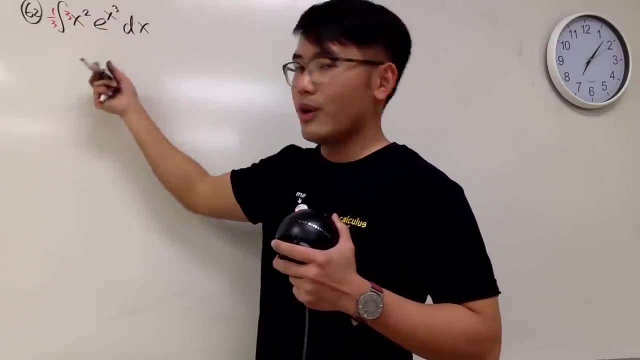 3x squared. I have x squared, but I don't have the 3.. So let me just multiply this by 3, but divide it by 3.. So this is pretty much the derivative of that Right. So the answer is: 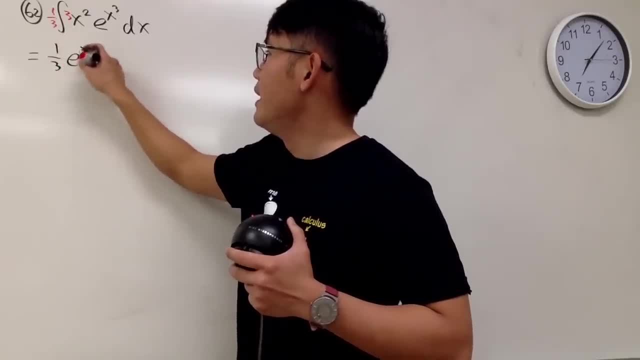 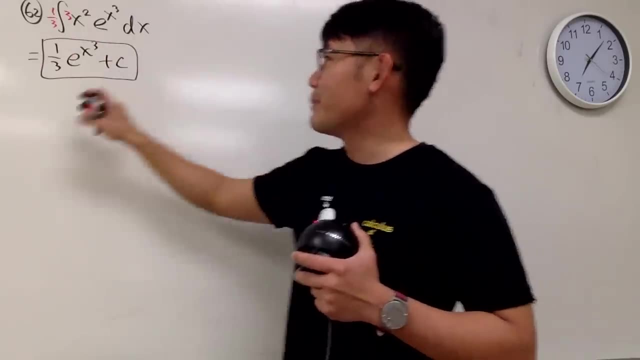 just gonna be 1 third e to the x cubed plus z. This is nice. If you do u sub, you end up with the same answer, but like you know, now it's quicker. Well, the point with this question is, if you 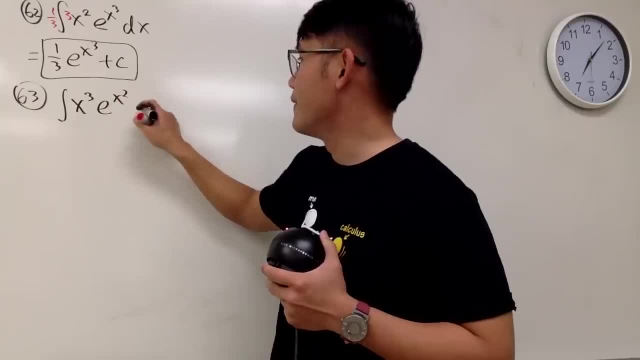 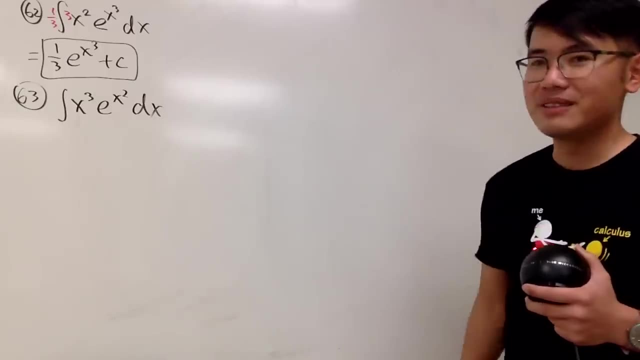 switch this a little bit. if you have x cubed, e to the x squared, I want to insert that. that's a crying meme, but, like you know, I am not gonna edit this video, but like that one, you know. 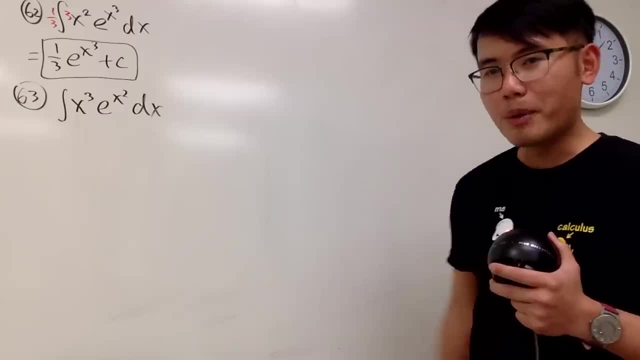 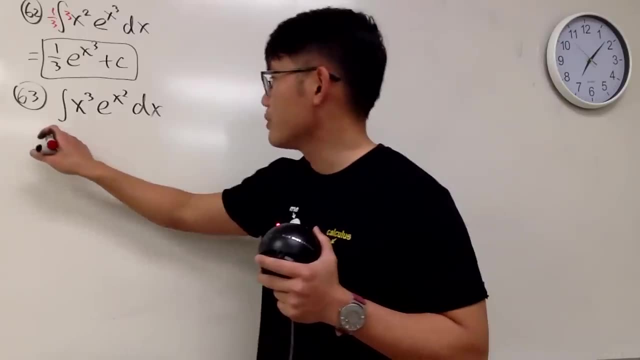 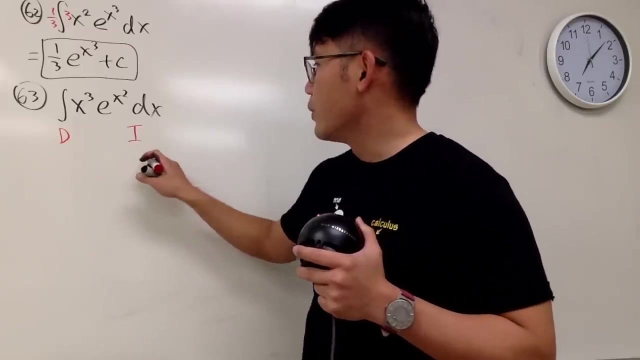 Hmm, Integration by parts. Give it a try, Let's see. This time we have to think carefully, though. Like what kind of integration by parts? How are we going to make things work? i is the most important one first, so let's do it Well. 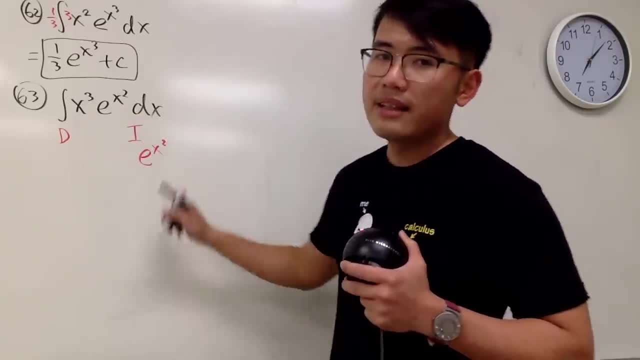 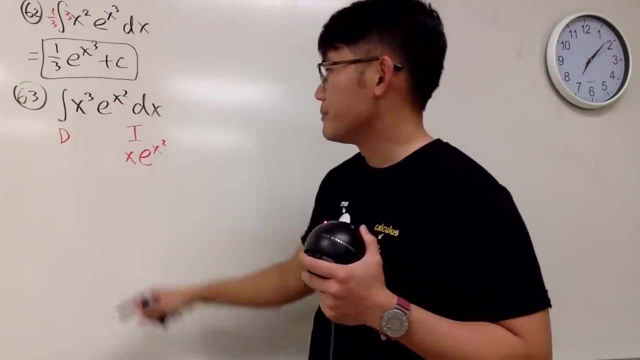 I most likely have to deal with the e to the x squared, but I cannot integrate this. I will have to have an x in front to help me, just like this earlier, huh. So I will do that right here And in the. 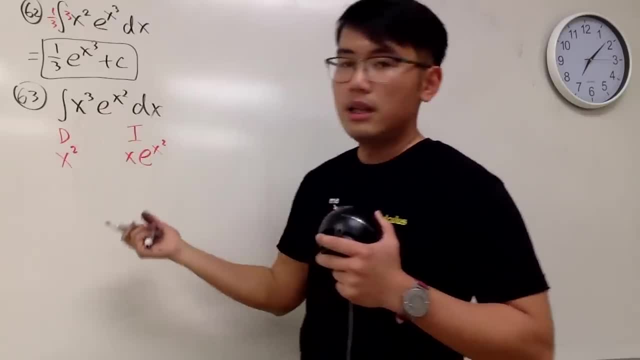 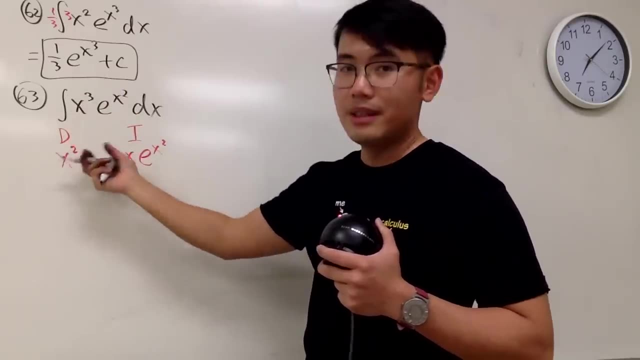 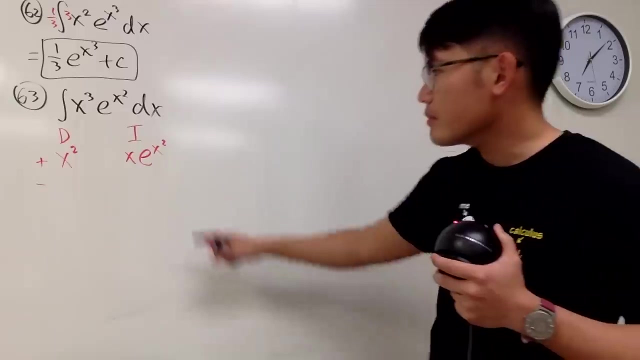 meantime, let's see, I have x squared left, so I will have to, I will have to, I will have to differentiate, I will have to differentiate x squared. And here is the deal: When you integrate this again, you can do that. 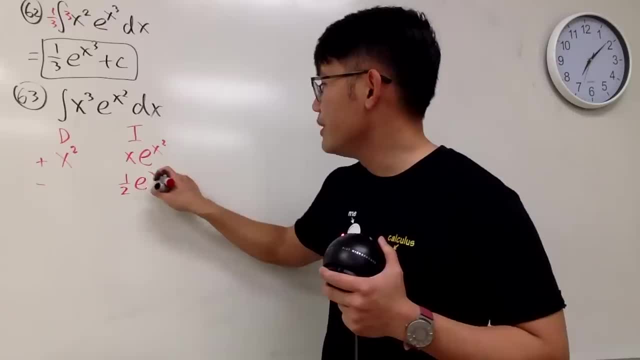 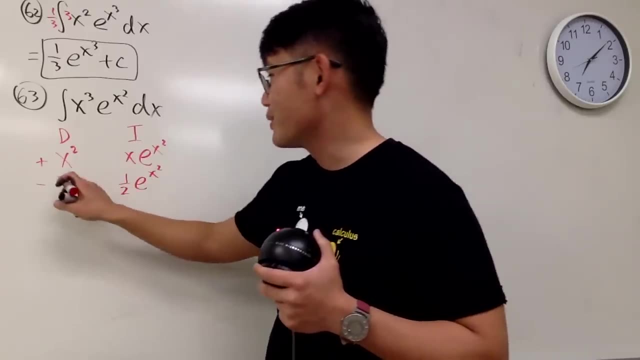 and you end up with one half e to the x squared. This is doable And we can integrate this again. Check this out. Well, no, I mean you can differentiate this, which is 2x. Here's the deal, Yes. 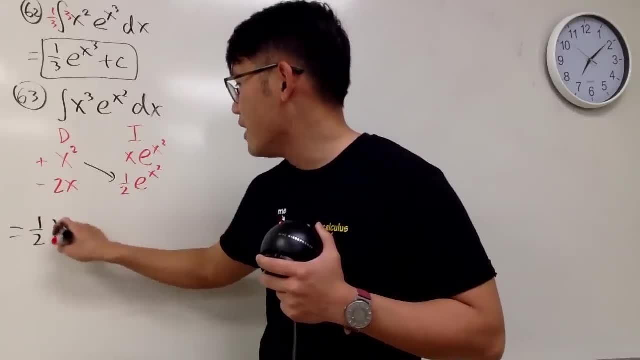 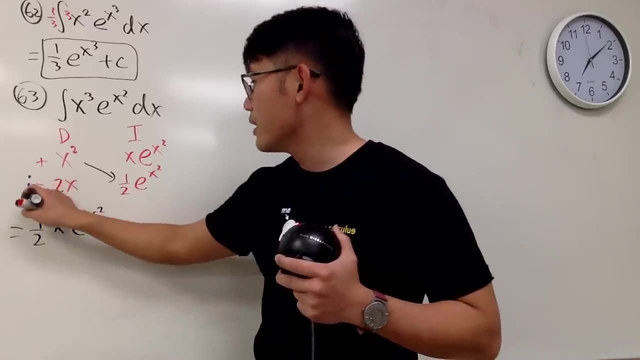 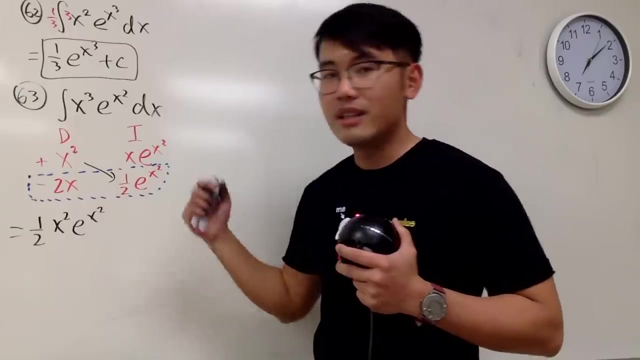 the first part is going to be this times that, which is going to be one half x squared e to the x squared. That's nice. And then you are going to be integrating this times that. So integration by parts works Because you have this x, that's. 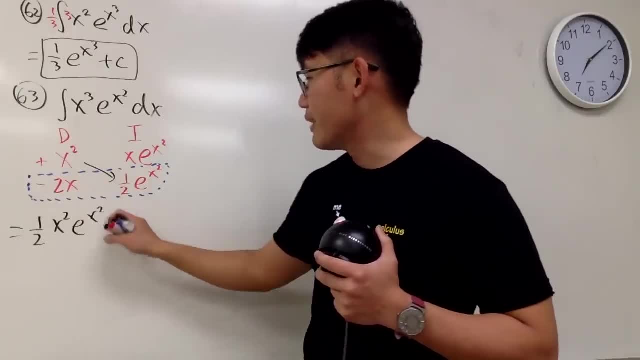 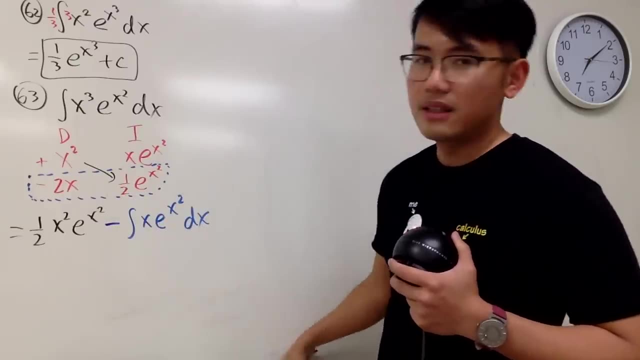 helping you out. Well, let's see, let me put this down in blue. So we have to minus the integral 2 and one half, cancel. you have x, e to the x squared dx. Ah, similar, huh. So we can do it. This is. 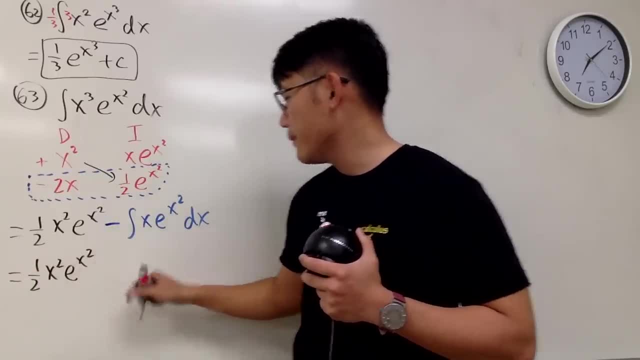 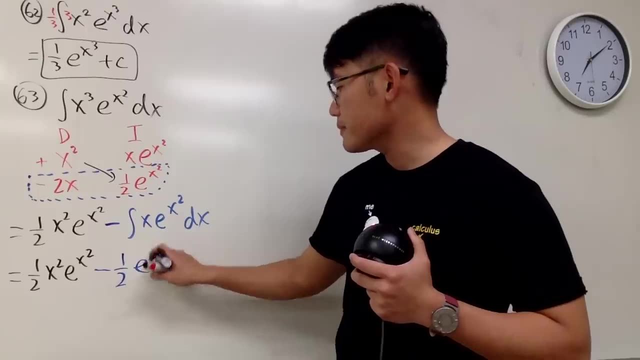 going to be one half x squared, e to the x squared, and then I will just write down the rest in blue Minus: I need a 2, I need to divide by the 2, so just doing your head Well done. 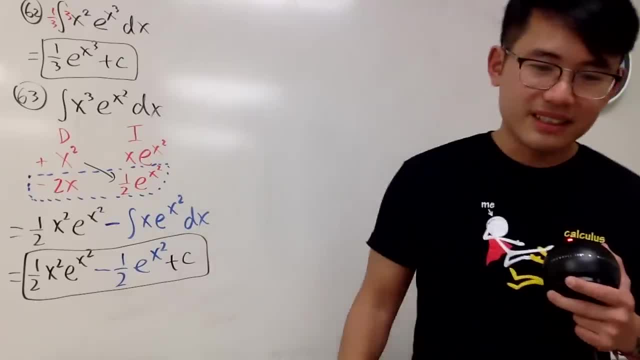 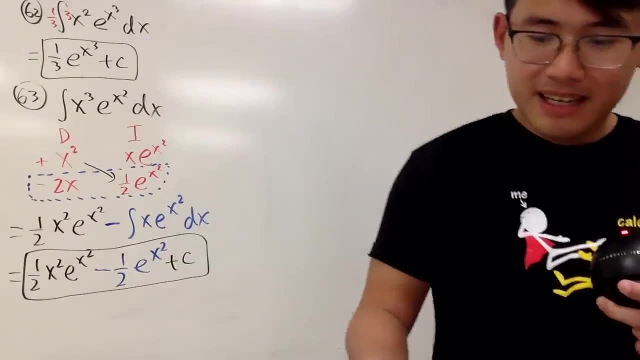 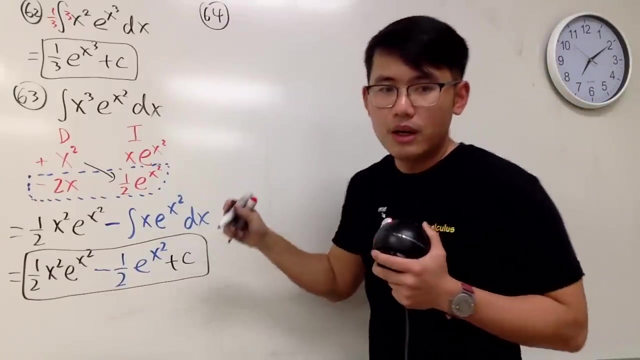 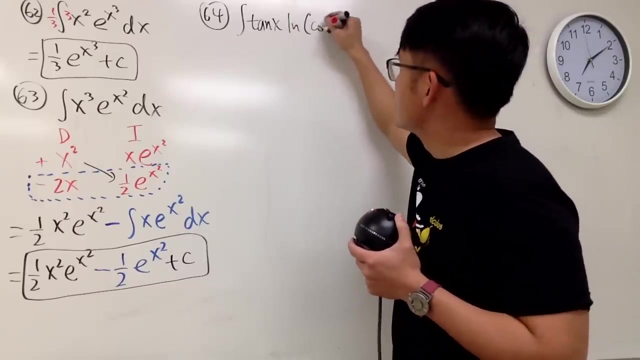 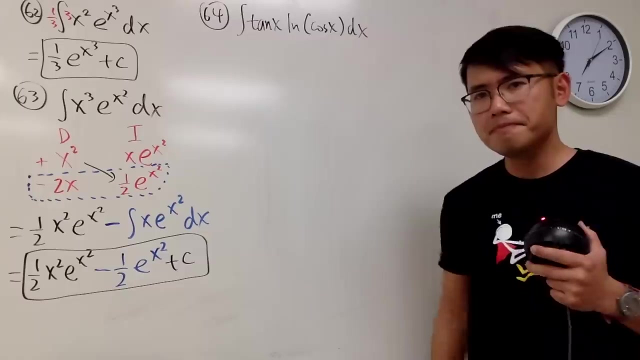 Well done, Done. yes, Alright, I have two more pages, Alright, number 64.. Number 64. I have the integral of tangent x times the natural log of parentheses, with cosine x inside Integration by parts. again, Anyone No? 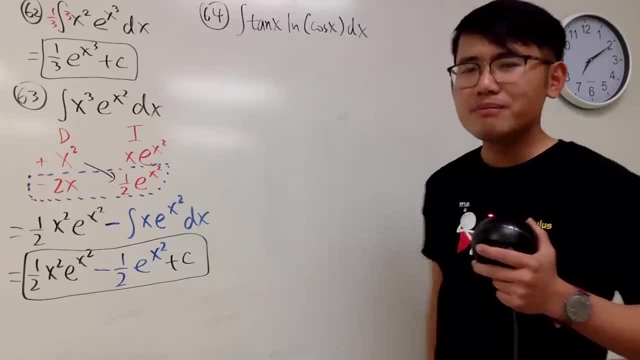 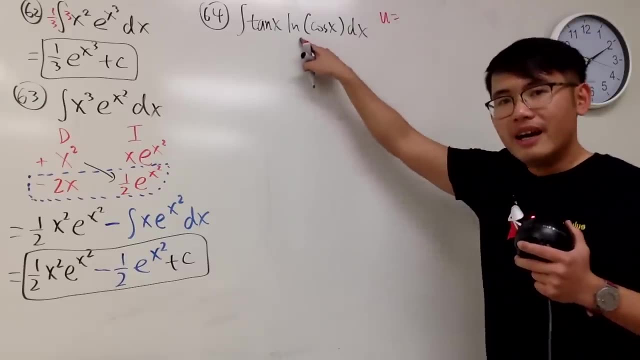 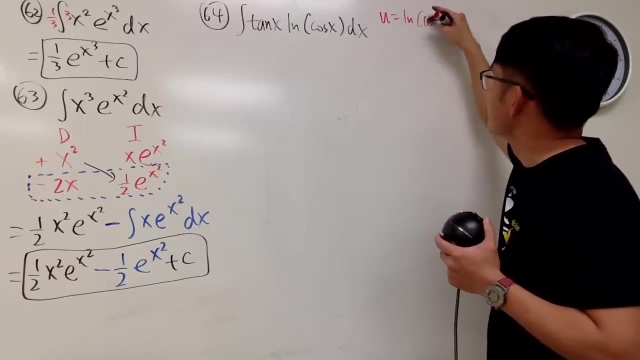 You sup, If you take this to be sine over cosine, Maybe, But better choices I can let u equal to natural log of cosine x. Check this out: Natural log of cosine x like this Why? Because when you differentiate this, the derivative natural of. 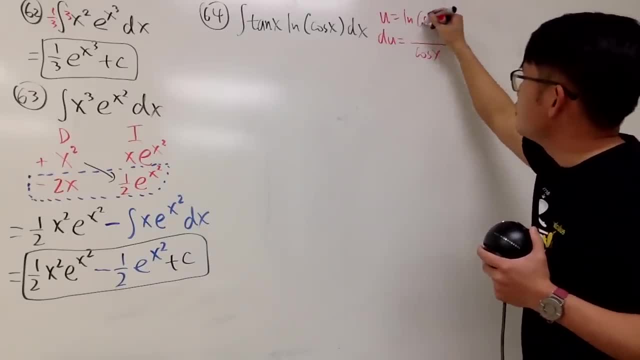 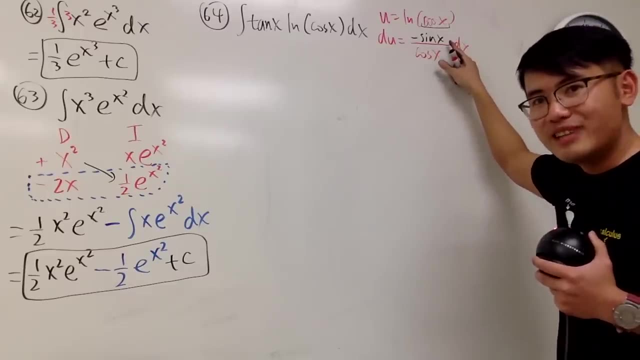 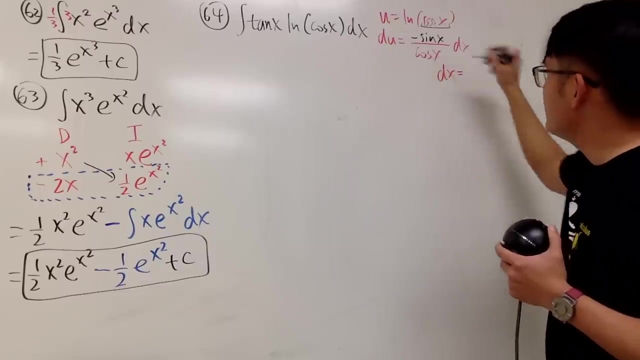 something is of course one over nothing. and then the channel says: multiplied by the derivative inside, which is negative, sine x, dx. This is precisely tangent. but you have a negative, Doesn't matter. So we know dx is just negative. 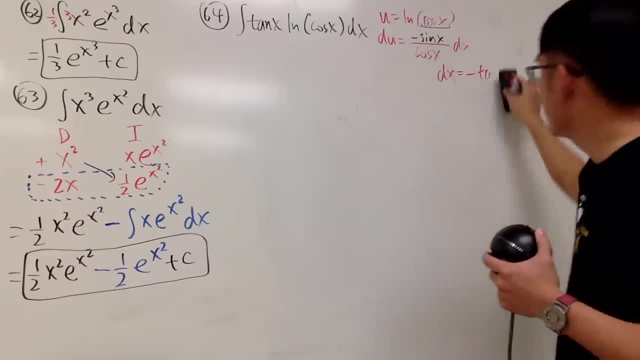 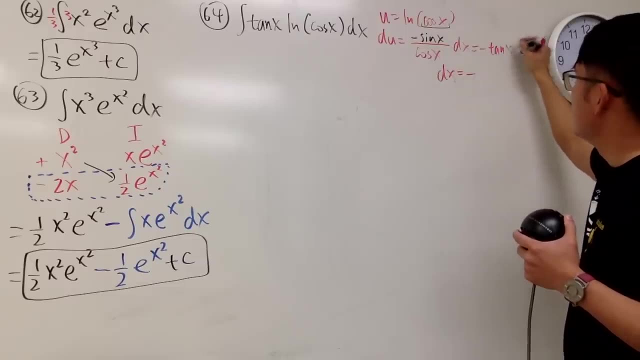 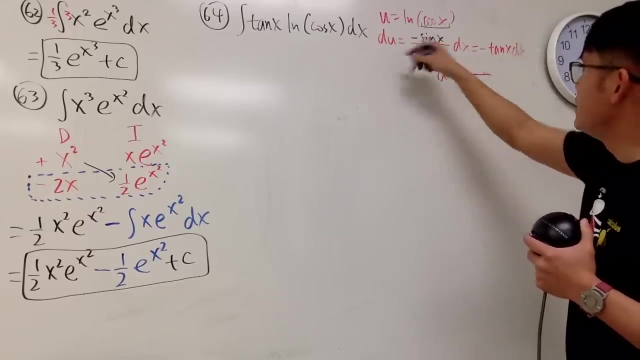 and then you have the tangent. Well, technically alright, let me just make this clear: This is negative and this is tangent x, dx. I will have to divide the negative tangent on both sides. so dx is du over negative tangent x. 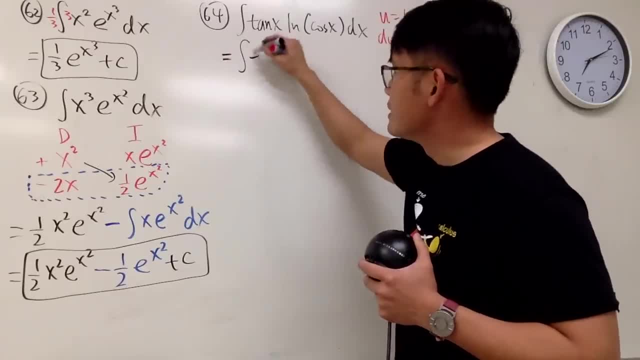 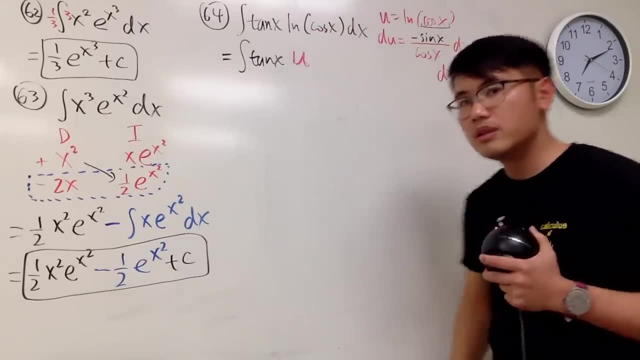 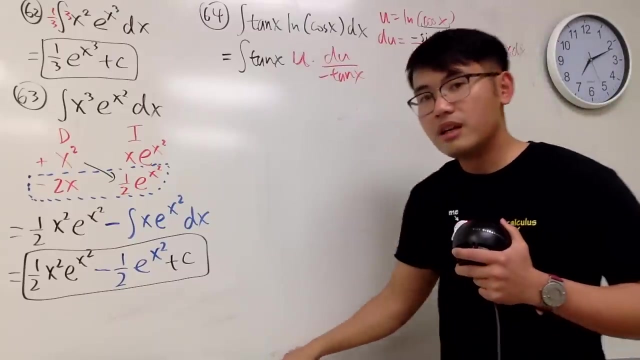 Very nice, huh. So you have the integral and this is tangent x. This right here is our u, This is our big brother, u dx is this guy. so you multiply by du over negative tangent x. Tangent tangent Cancel, cancel. 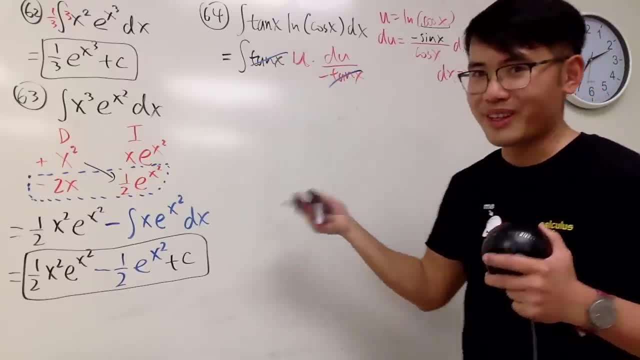 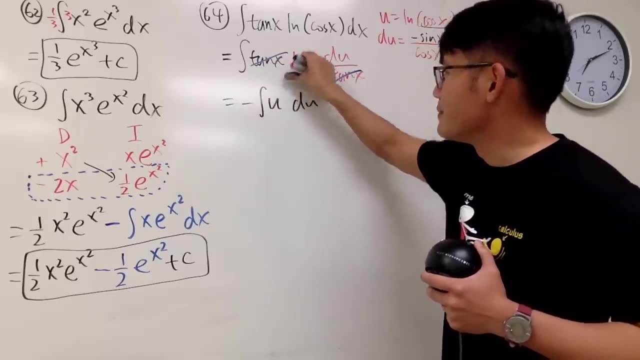 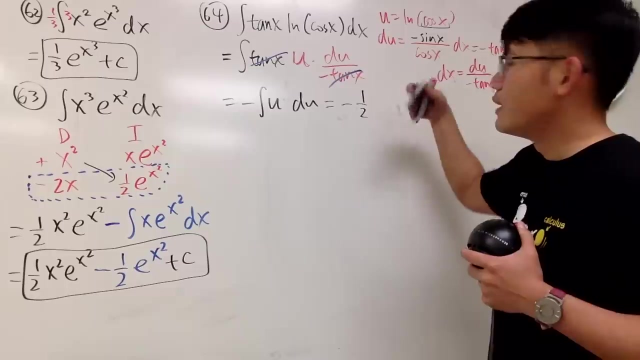 Negative. negative, Just one. okay, Just say it twice. Negative still here. negative integral: u squared. well, that's almost the answer Now. integral of negative: Negative integral of u du this right here gives you negative one half. 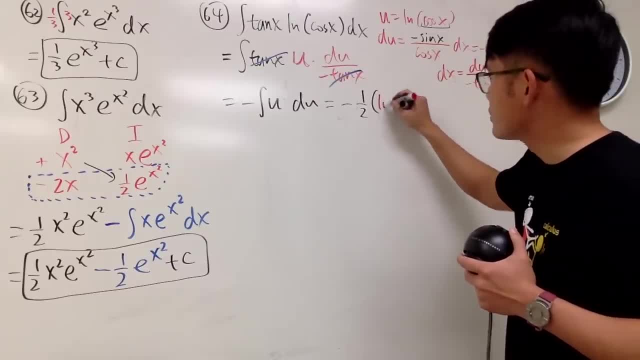 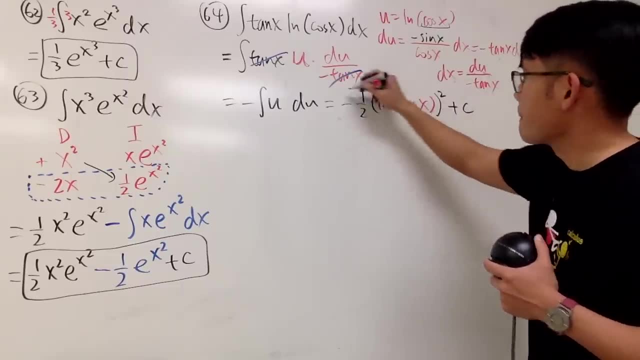 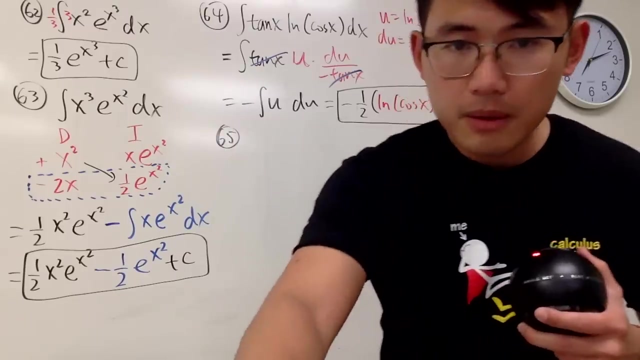 u squared u, is that? so put this in parentheses with natural log of cosine x inside and you square that and you're done. Plus plus c b, half p, 65.. Right, Ah, Let's see Integral of 1 over. 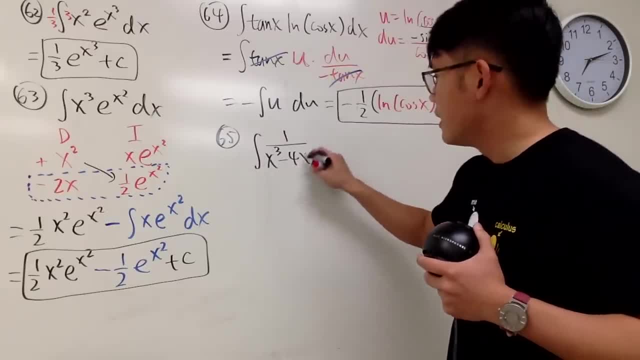 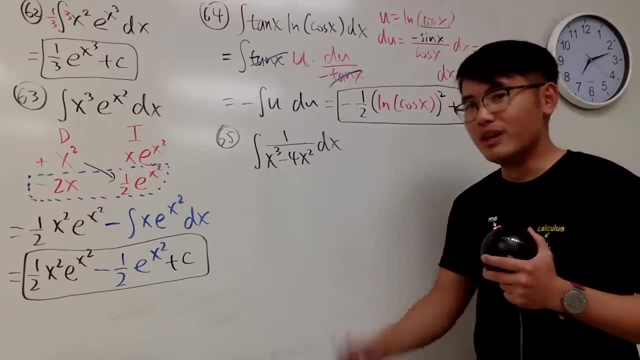 x cubed minus 4x squared. Unfortunately, this one, it's not the one that we can just factor out the highest power and then make things work. We have to do the dirty work, to do the partial fractions. So here's the deal. 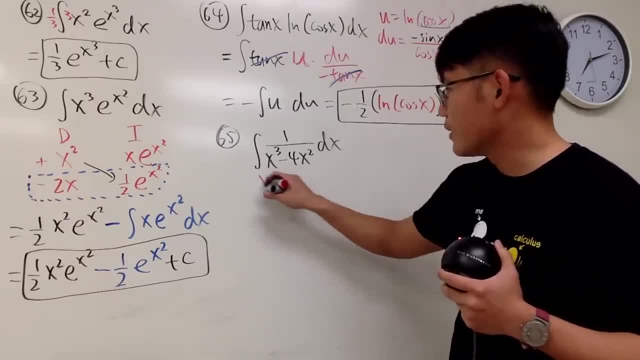 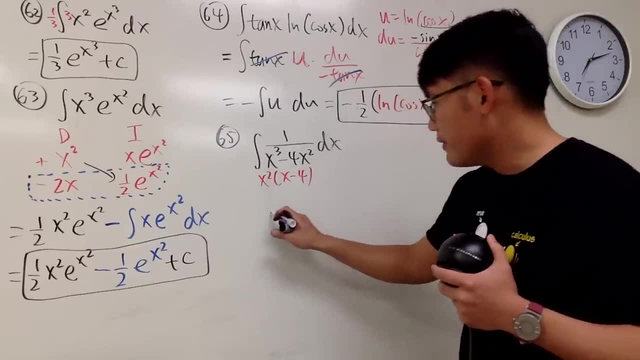 I will do the partial fractions here. maybe I will have to factor out the x squared, and this is going to be x minus 4.. Huh, So here is the setup for the partial fraction. On the left-hand side, I have 1 over. 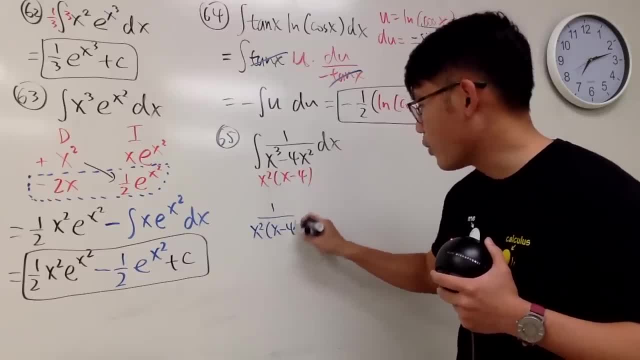 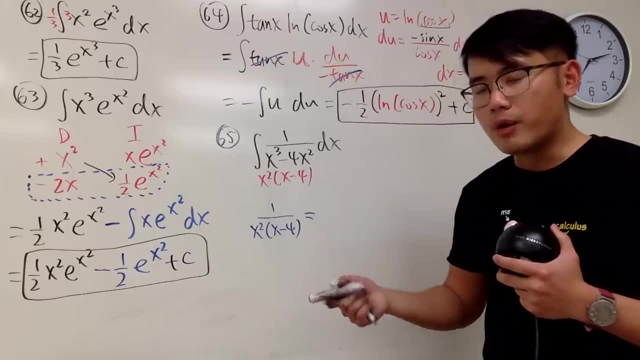 the original denominator, which is x squared times x minus 4.. And the setup is this: This is x squared. You have to build out the power. Well, maybe you haven't seen this before, but I will show you how You can look at this as. 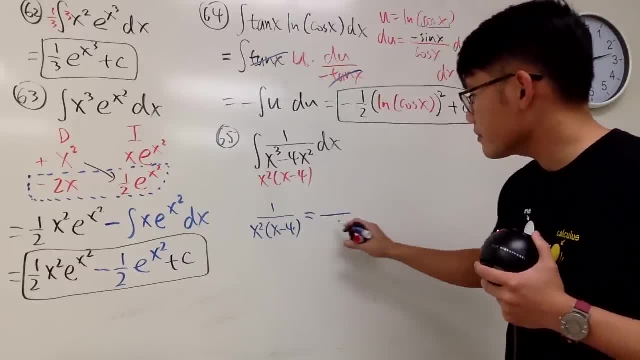 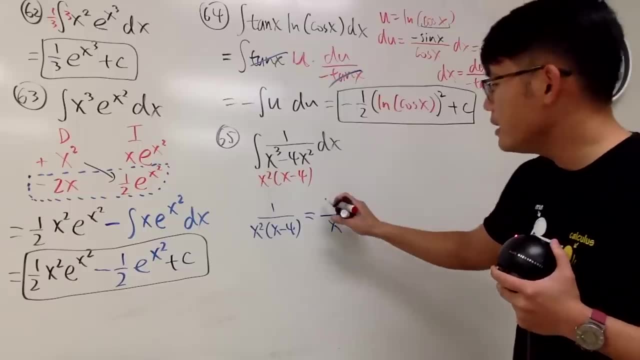 quadratic, no problem. If you look at this as x squared like this, then you will have to make sure you have a linear term on the top, Namely, you will have to have ax plus b on the top, And then you have. 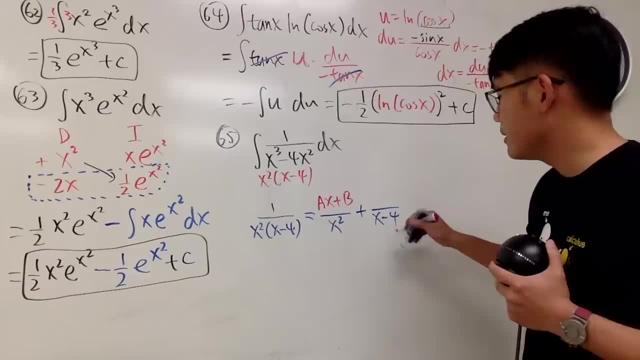 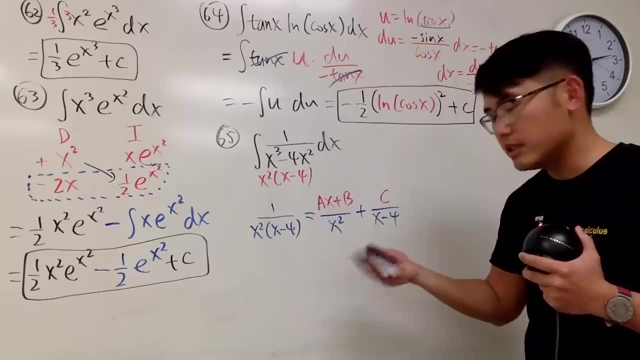 a linear term. so you are going to add x over 4 in the denominator, x minus 4 in the denominator and then a- c. But in fact this is what I mean by build out the powers in my previous video. 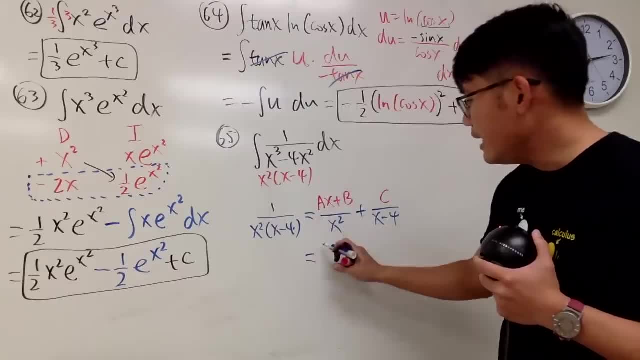 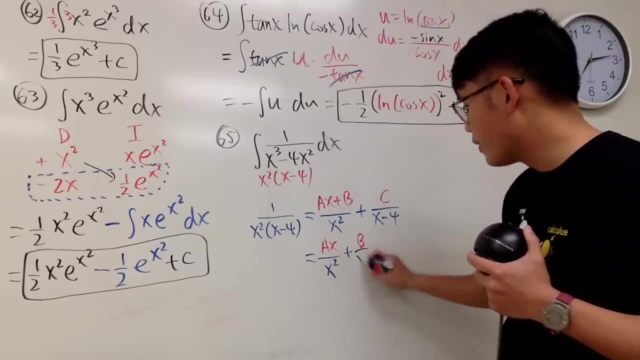 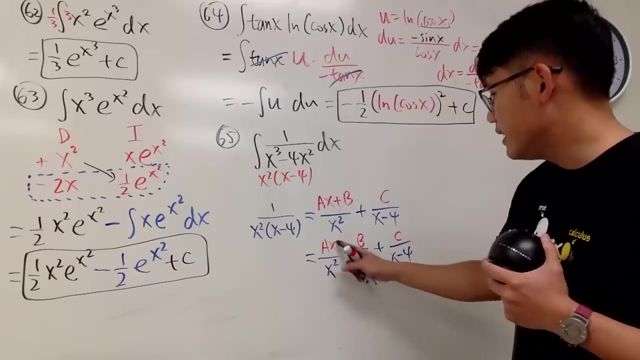 Right here. you can split the fraction and you get ax over x squared and then plus b over x squared, and then plus c over x minus 4.. Look at this: x over x squared they cancel out. So you actually just have: 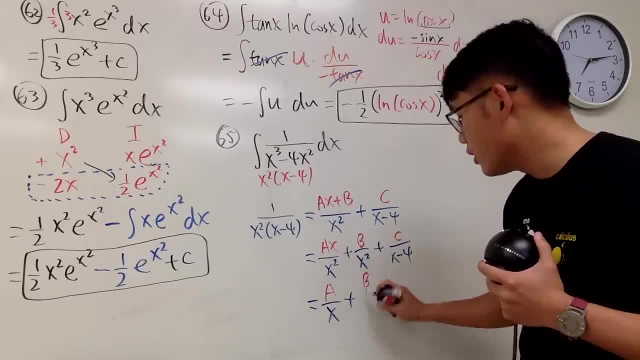 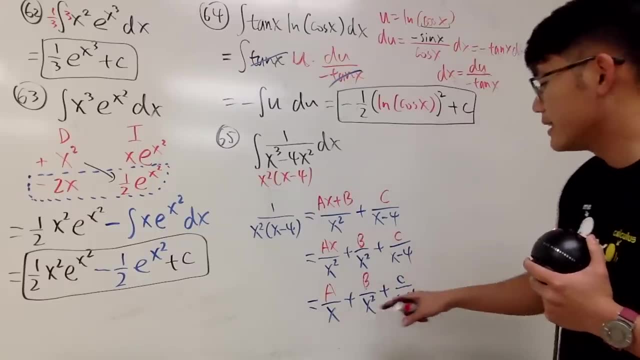 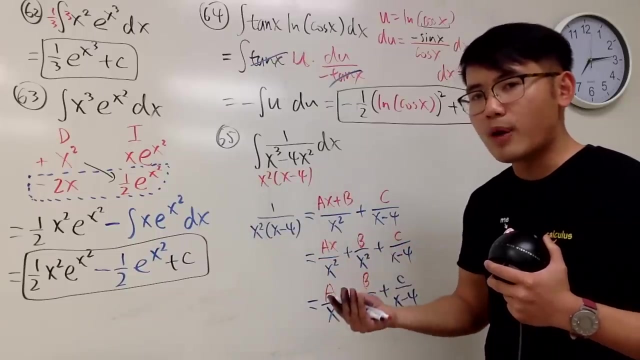 a over x plus b over x, squared plus c over x minus 4.. Again, the idea is that if you have a repeated linear factor, this is technically saying x to the first power times x to the first power. In that case you have to build out the power. 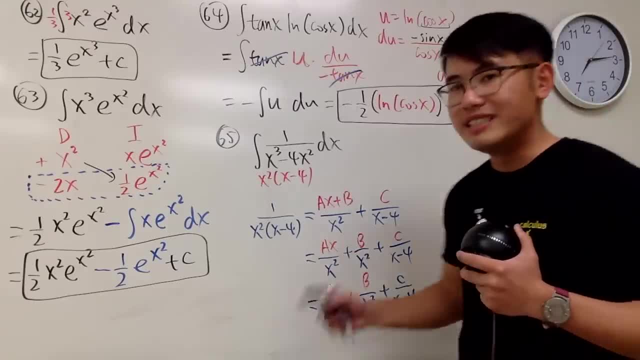 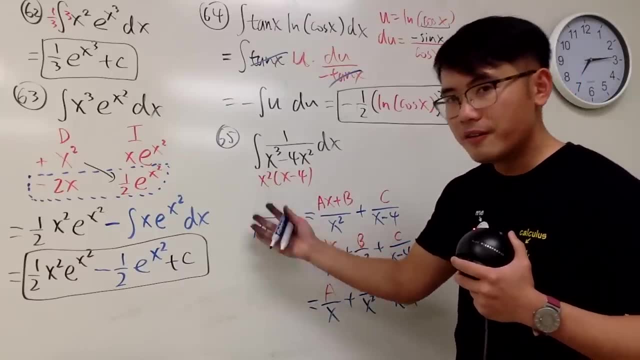 So you can actually just go from here to here every single time, because this is going to work. You can imagine: if you have 1 over x to the 5th power, the 5th power, then you will have to have a over x to the first. 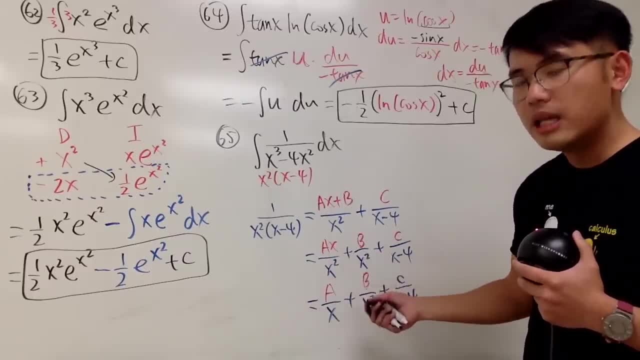 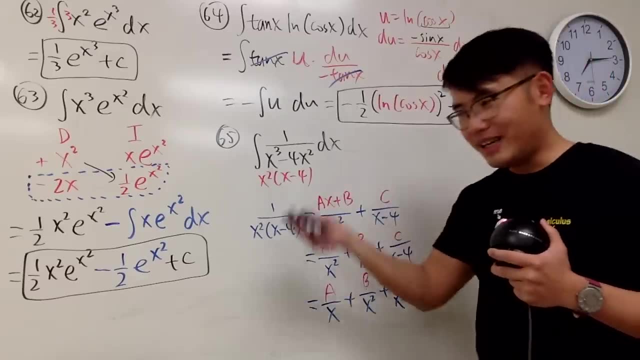 plus b over x to the second, plus c over x to the third, plus d over x to the fourth and plus e over x to the 5th, and then plus the next alphabet over x minus 4.. Alright so. 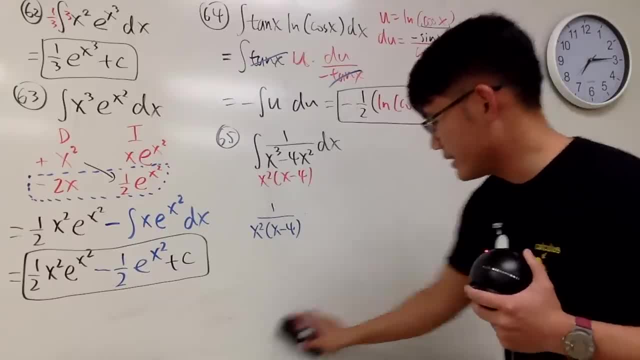 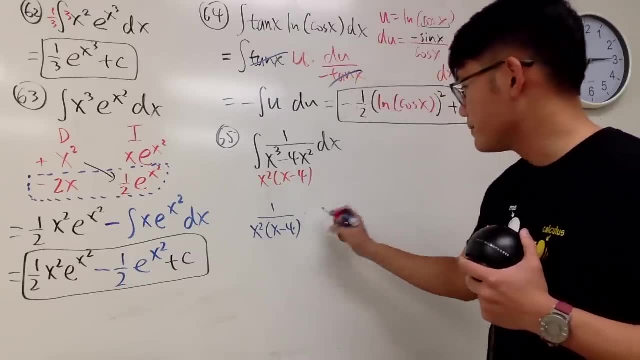 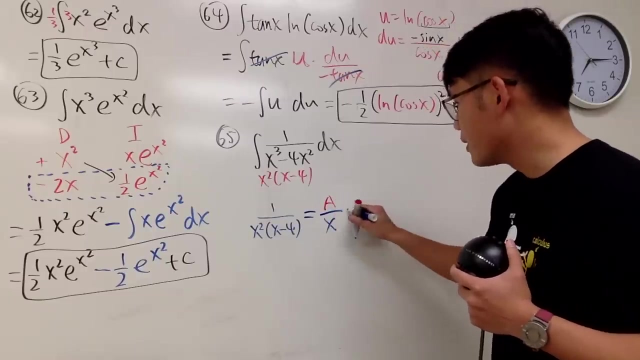 I will just pick this up right here for you guys. We are going to be integrating this right here. Well, not yet Partial fractions. So we have a over x to the first power, and then we build out the power b over x, squared. 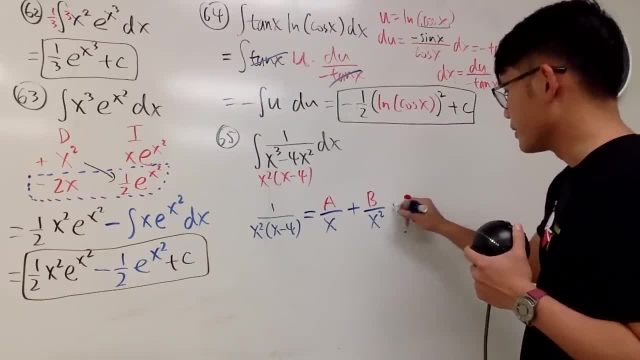 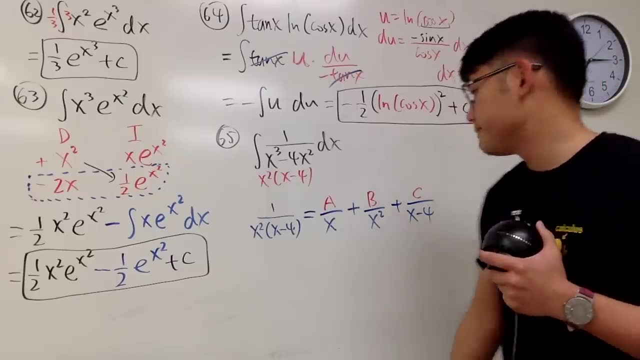 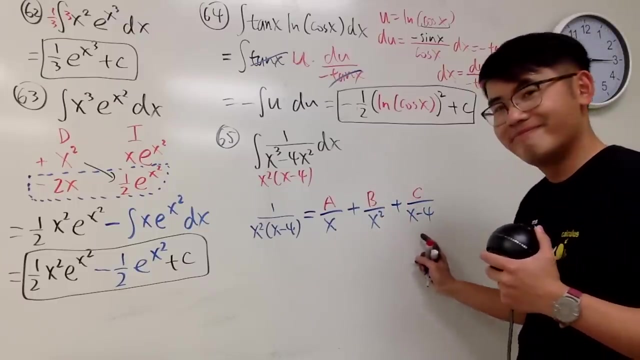 Again, thanks. we don't have x to the 2. The second power, that's good, Plus c over x minus 4.. Here is how we are going to do it. I will do cover up for b and c. Unfortunately, A will have to do some more work for it. 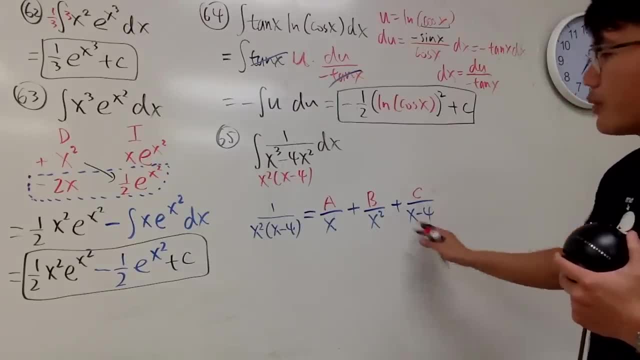 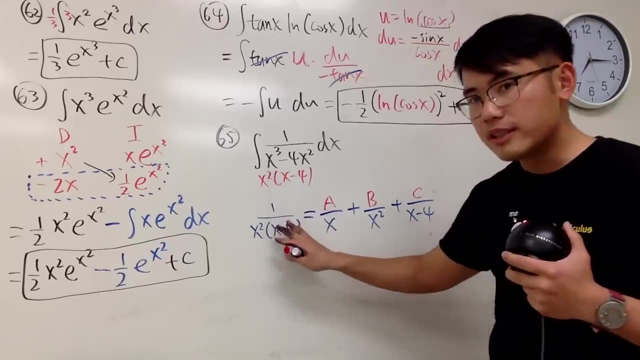 Check this out. To integrate, to get c, you come here and you cover this up and you have to let x equal 4.. Okay, Because this is, x has to be 4.. 1 over 4 squared, you get. 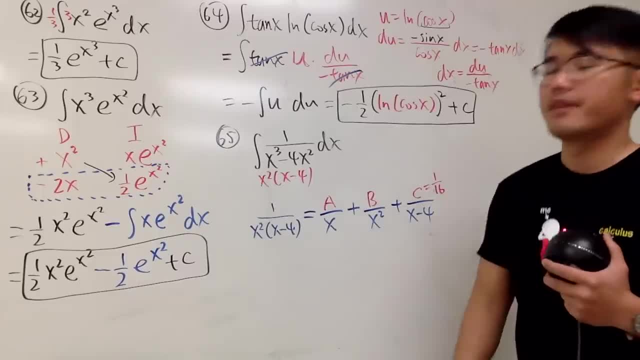 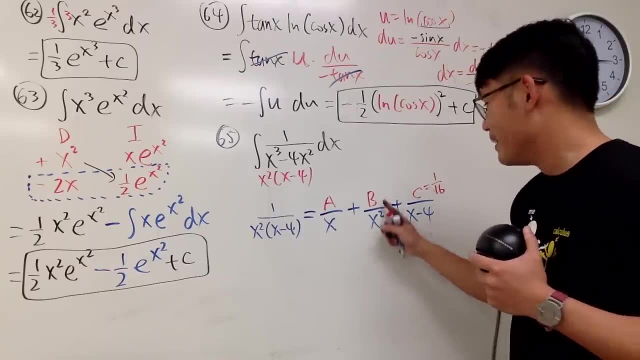 1 over 16.. Good, And then when you have A over x, you come here. well, no, sorry, Because you have to have the same exact denominator, b over x squared. you are going to come here and cover up the entire x squared. 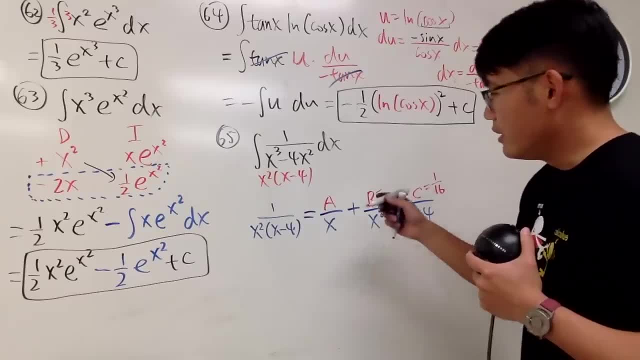 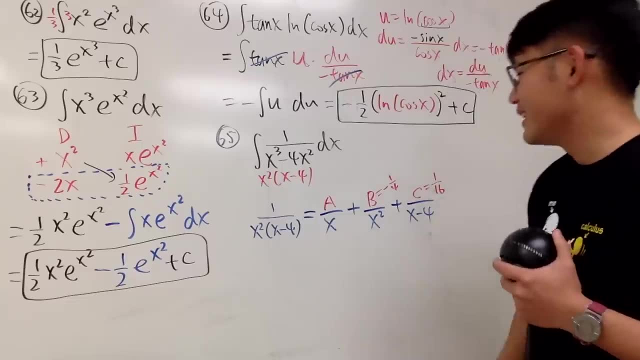 and you plug in 0 into here, so you have 1 over negative 4, in other words, negative 1 over 4.. This is good For A. unfortunately, you have to do more work for it. But remember, you used 0,, you used 4,. 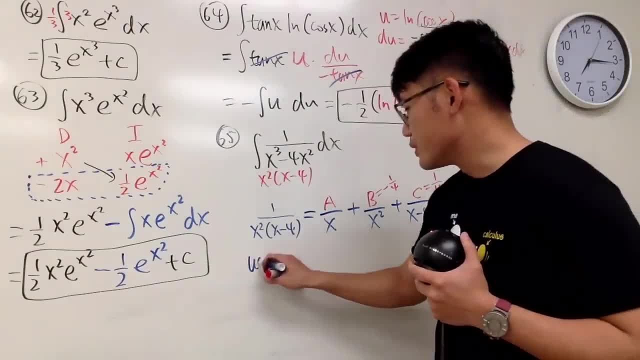 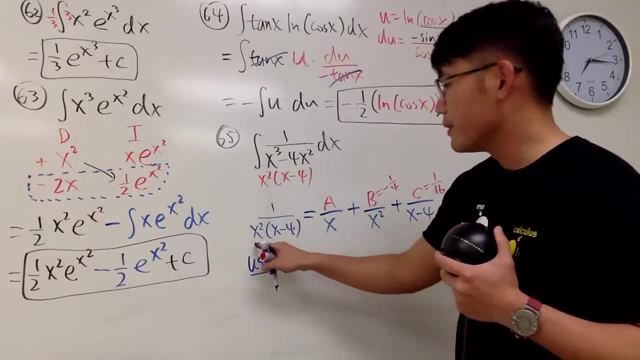 you haven't used 1, and it's a nice number. So just say: use x equal 1 for A. put 1 into all the x, you see that this is going to be 1 over 1 times negative 3,, which is. 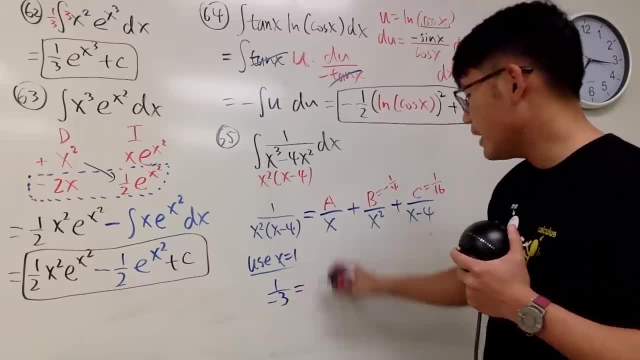 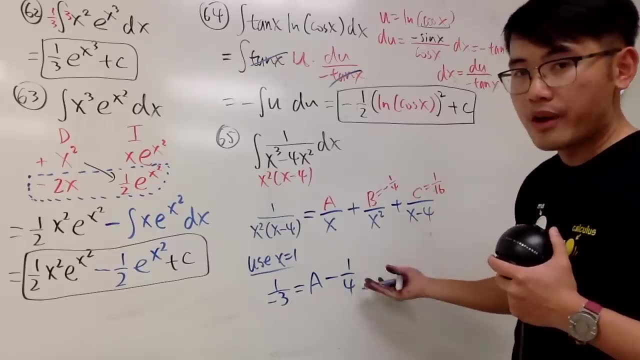 1 over negative 3, and this is going to be A, I don't know. over 1 is still A. and then this right here is: minus 1 over 4. over 1 squared is still this Okay, Putting 1 into. 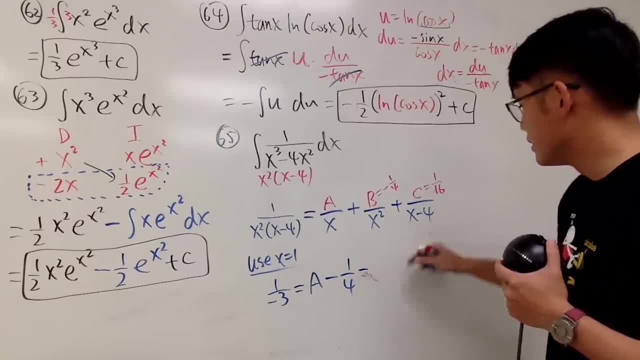 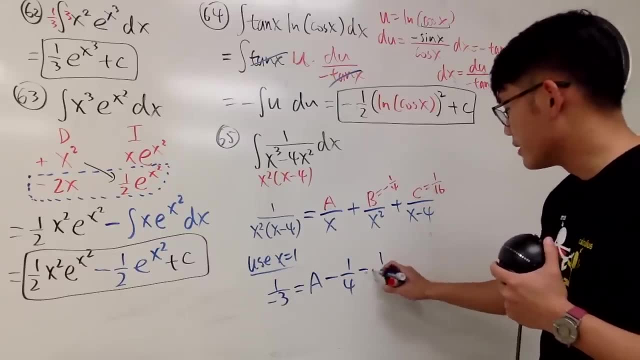 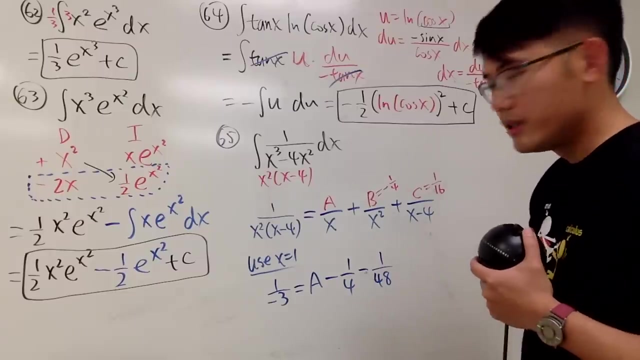 here you have. this is going to be minus because you have 1 over 16, over negative 3, so you multiply the denominator, so you have 3 times, that is 48. Like this, And then you get your little. 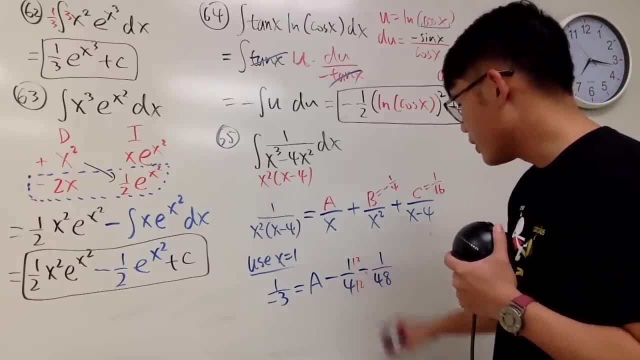 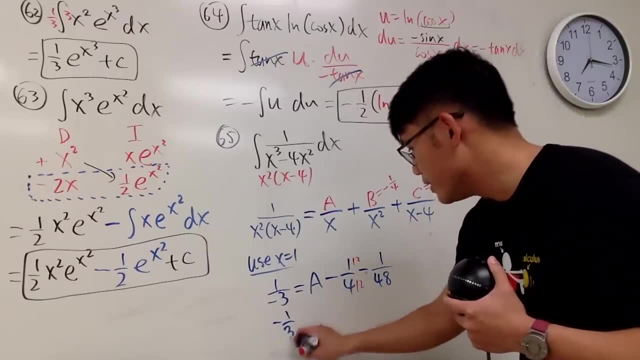 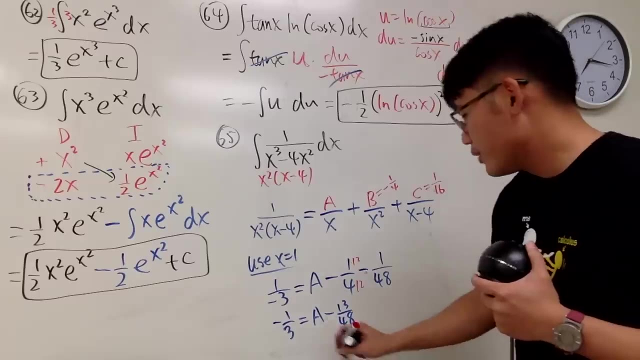 common denominator. so you multiply this by 12,, multiply this by 12, so you get. let me just do this real quick: this is negative. 1 over 3 equals A minus 13, over 48, and then you are. 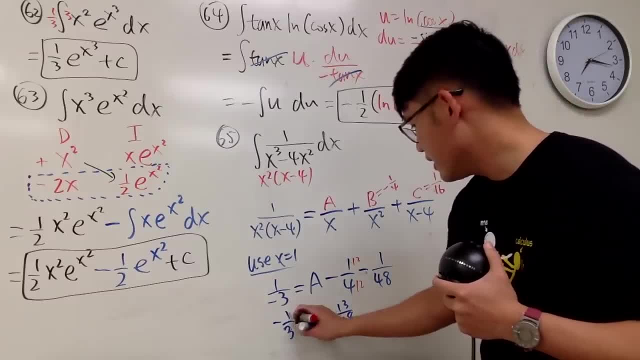 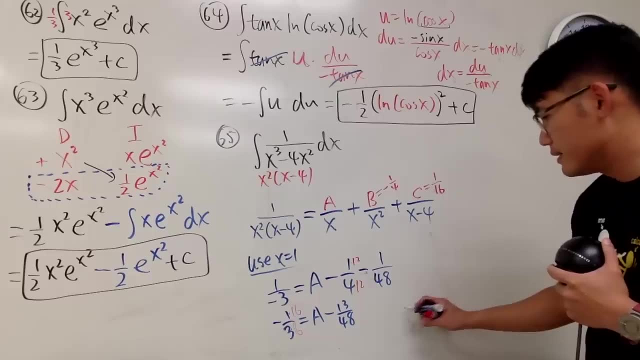 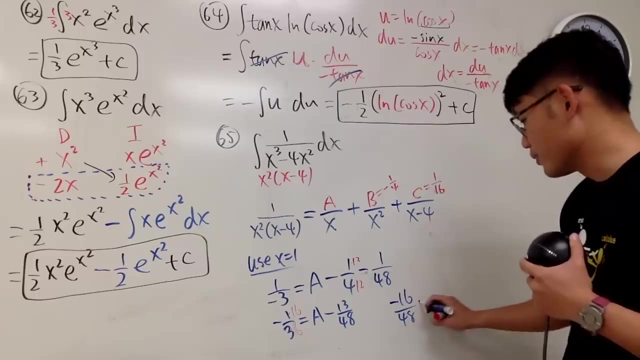 going to multiply this by 16 and 16.. And then you get this is 16,, this is okay, negative 16, I kind of know the answer, but let me just show you guys all the work And then, okay, I'm going to make sure. 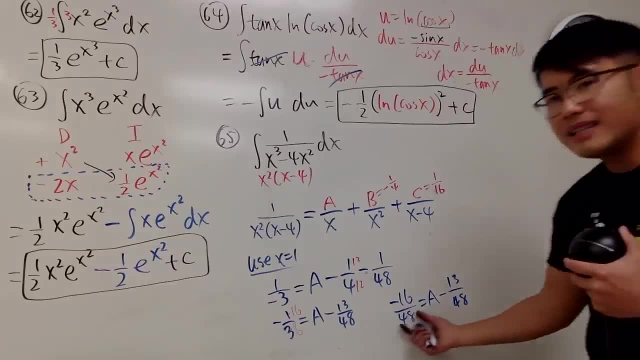 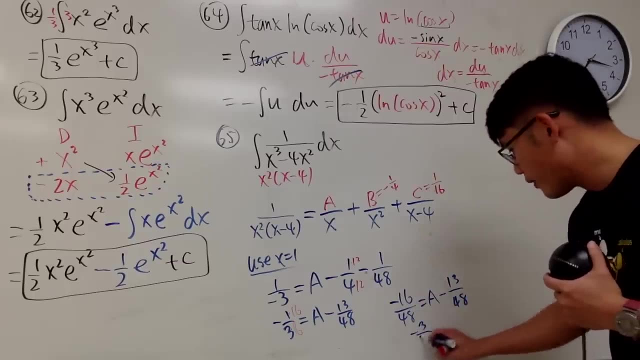 that I don't make a mistake, because if I do make a mistake, that's not good. I add the 13 over 48 on both sides, so I will end out with negative 3 over 48, right here, right, And that's equal to A. 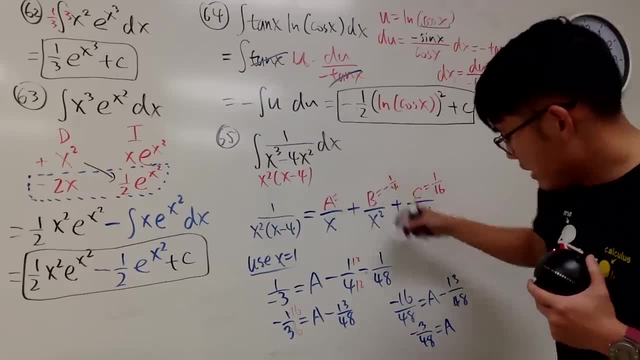 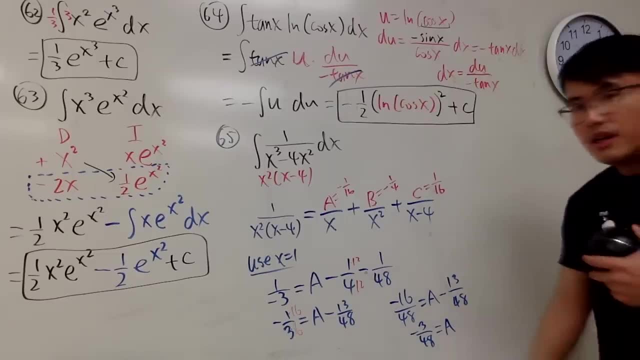 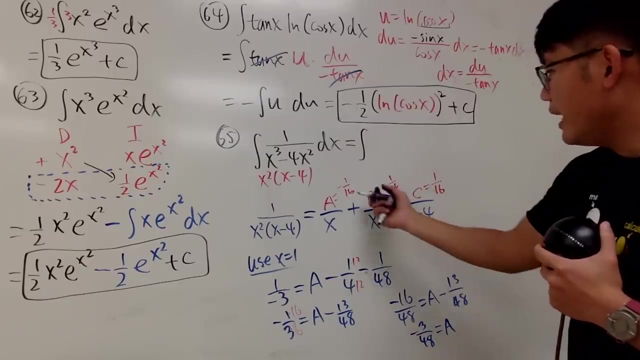 which A is equal. to reduce that, you get negative 1 over 16.. I think that's good Alright. now what we are doing is coming back here and then write this down: as the integral A is negative 1 over 16 over. 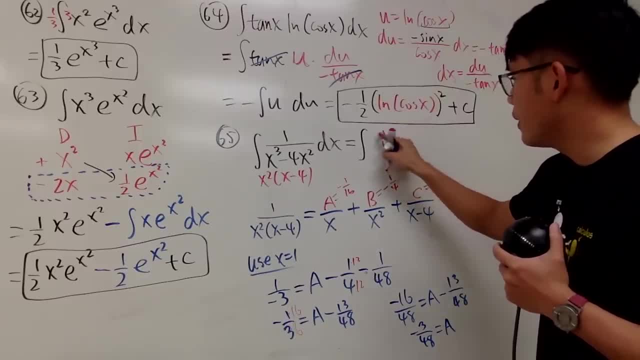 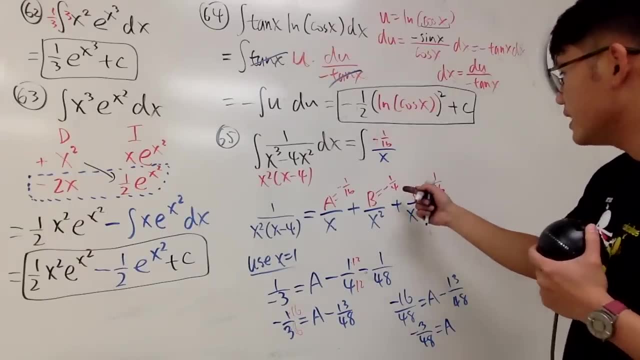 X. so let me just put that down: negative 1 over 16, right, and then we have the over X. That's the first one, Alright, and then the next one, B, is negative 1 over 4,. so 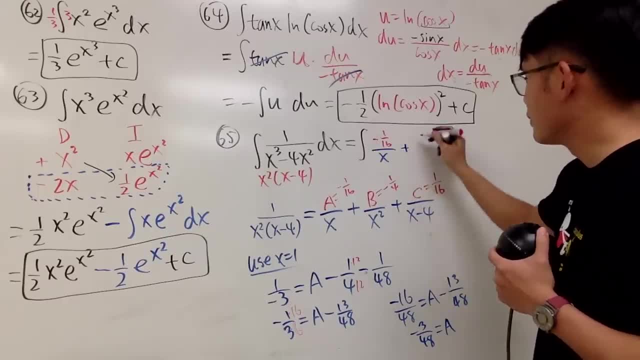 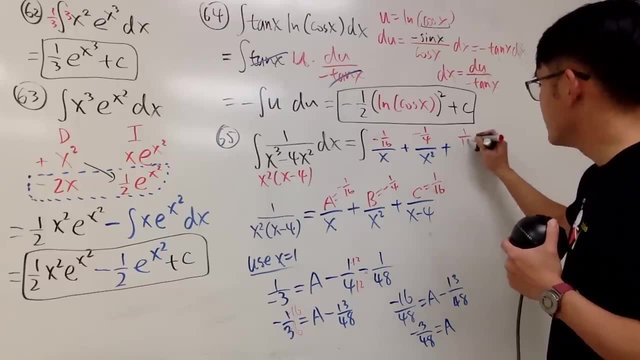 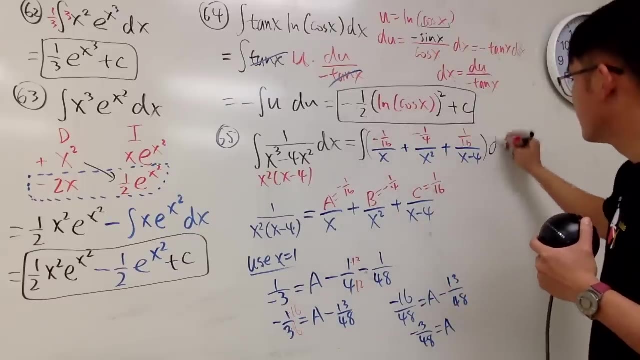 let me just put down plus negative, 1 over 4, like this over X squared. and lastly, we have to add 1 over 16 over X, minus 4, like that, Pretty good. And then I will take this: 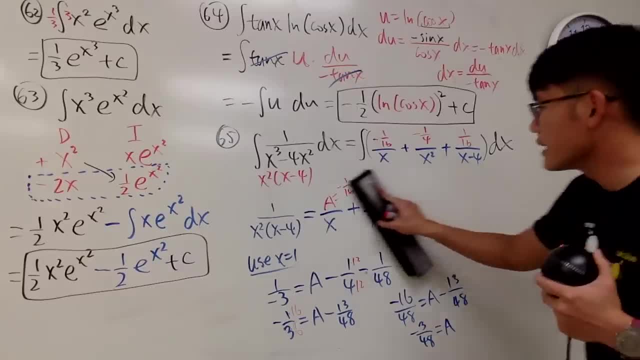 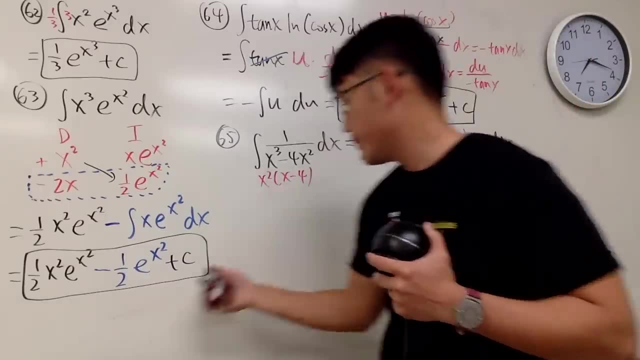 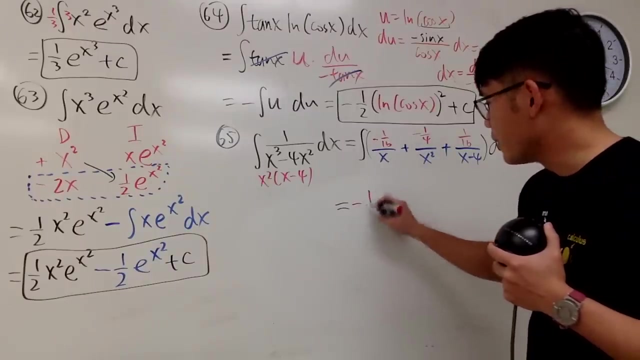 and put the dx right next to it. Alright, so that's pretty much the idea. Here we go. let's integrate this in our head. First of all, this is just a constant multiple Write it down: negative 1 over 16,. 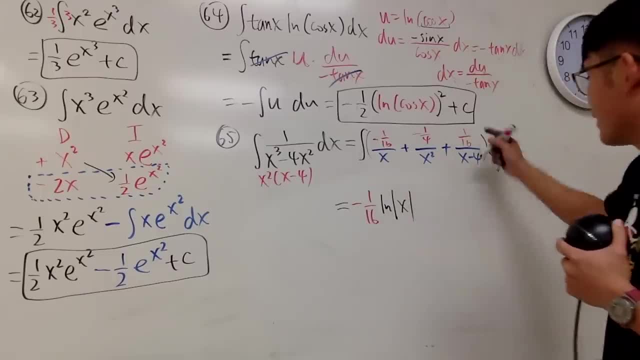 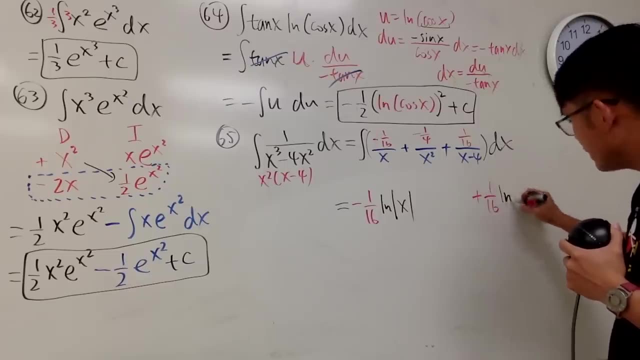 natural log: absolute value of X. Good, This right here is just as easy. so I will put down plus 1 over 16, absolute. well, negative, absolute natural log: absolute value of X minus 4.. I know I put down plus C. 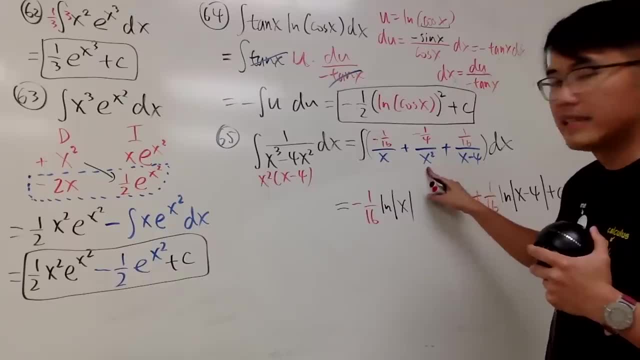 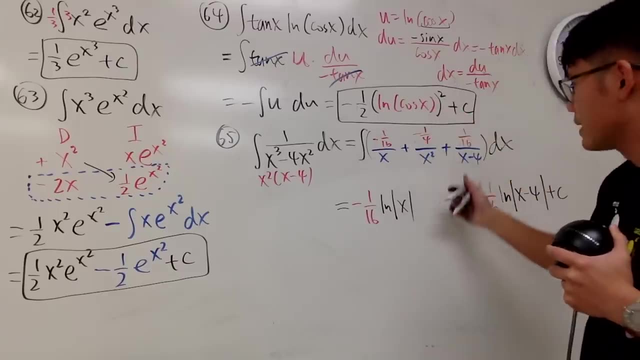 I could not, technically not. Here is the idea. This is, I think: X to the negative, 2, add 1 to the power, which is negative, 1, divided by that negative times, negative is positive, so you have a positive. so I put down plus. 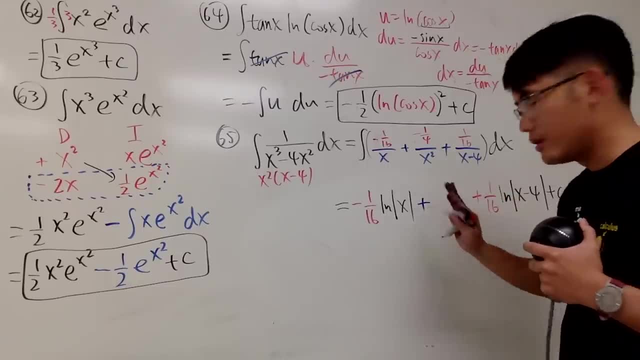 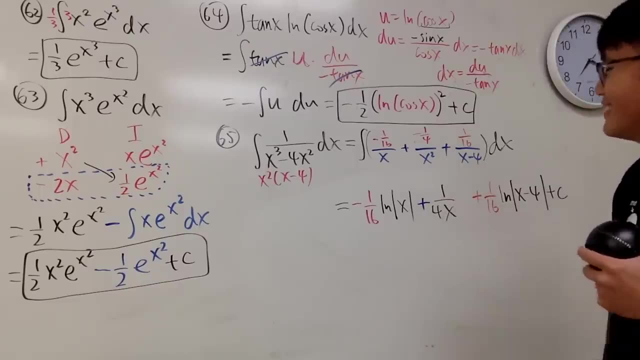 This is the plus. Do not put down natural log here. you end up with 1 over 4, and X like this. So if you differentiate this, you get a. yeah, you have the answer. So build up. 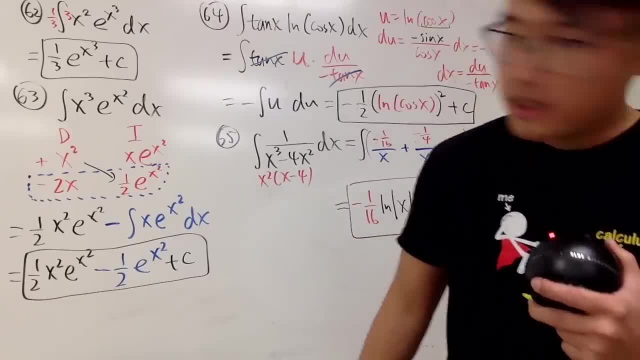 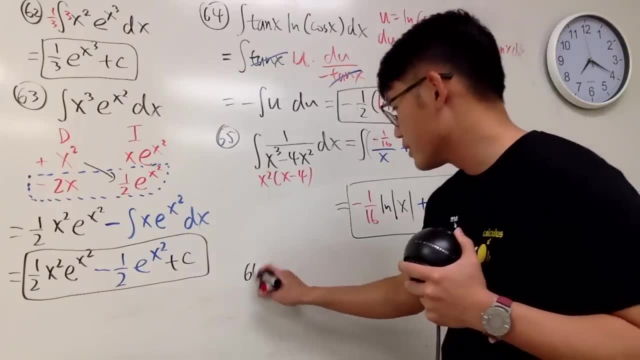 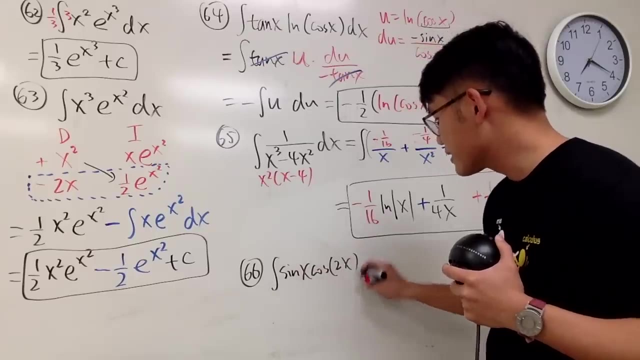 the power. when you see the power is being repeated. Okay, like that Number, that was 65,, 66, I will fit in here. And then let's see: this is the integral of sine X times cosine of 2X. 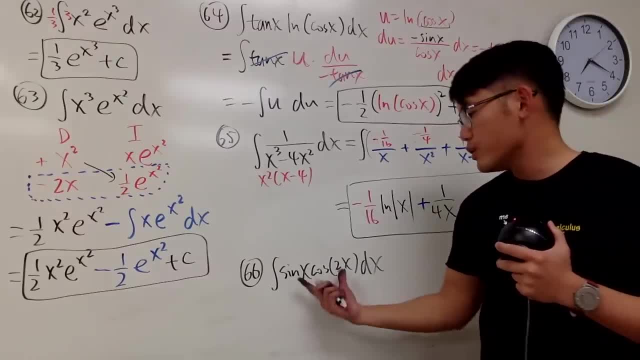 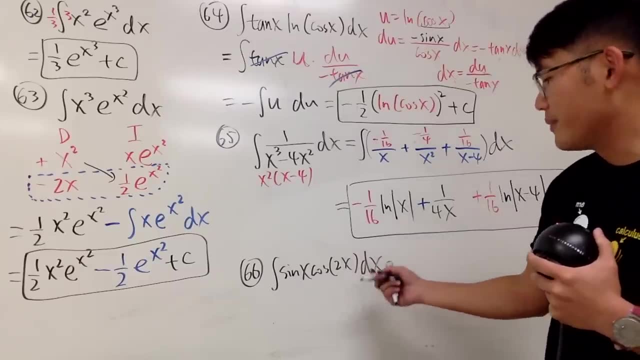 You have two choices to do this. You can use the product to sum formula or you can just use the double-angle identity for cosine. I will use the double-angle identity for cosine because this right here. in fact, you have three versions to do it. 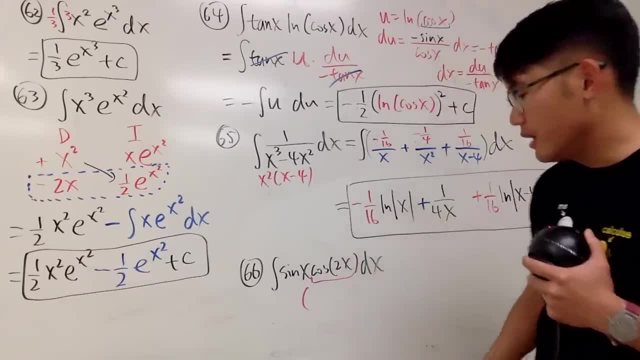 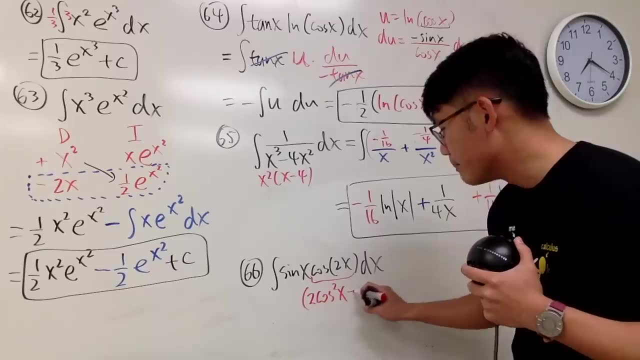 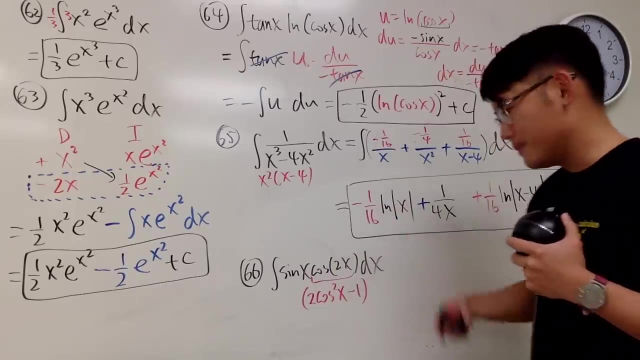 but you have the sine X in the front. In fact, you want to stay with cosine. here. I will put down: 2 cosine squared X minus 1.. And does this look familiar to you guys? It should right, Because if you add one of that, you can prove the. 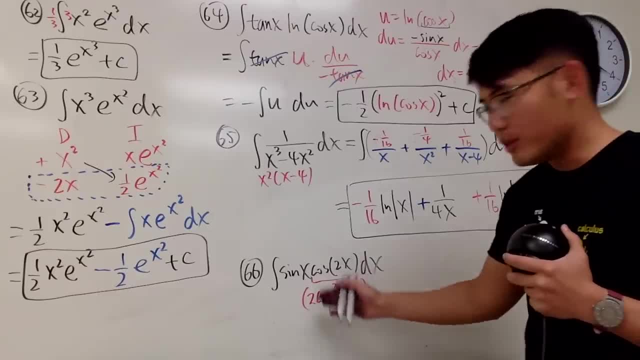 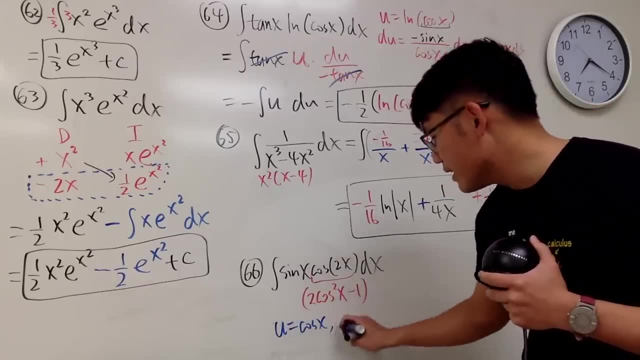 power reduction formula. So anyway, this is pretty much the idea for that, and then from here you actually have to take a U-sub. I will just say that U, equal cosine X and DU will be negative sine X, DX, of course. 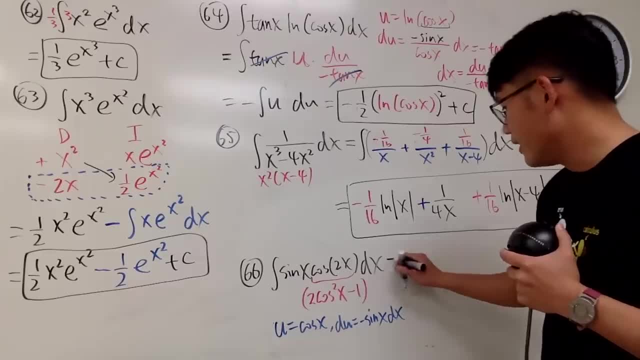 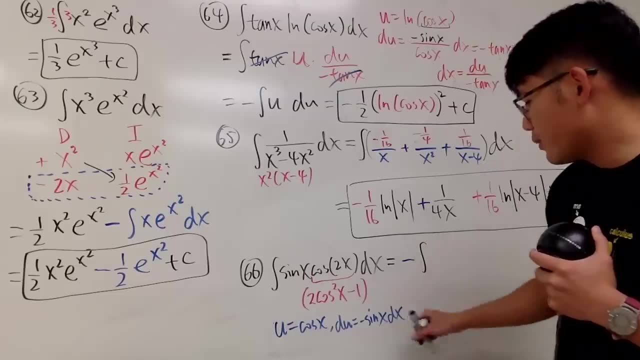 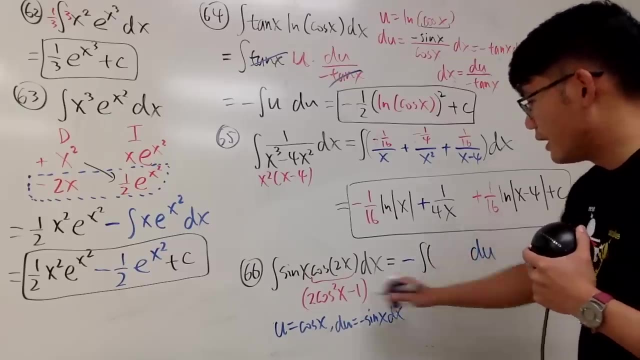 And this is only a sine. so you know you have to have a negative in the front, okay, And then you have the integral this and that will be DU. so you have the DU right here, okay, And then you have 2, and then you have. 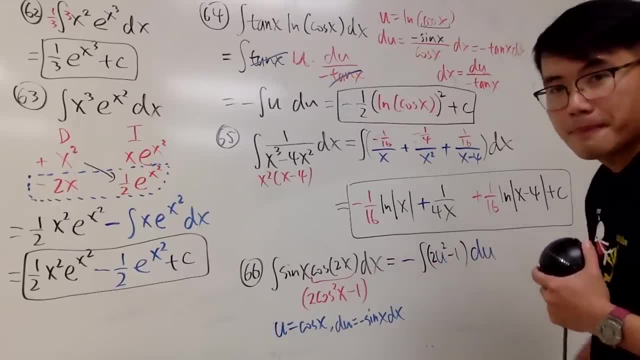 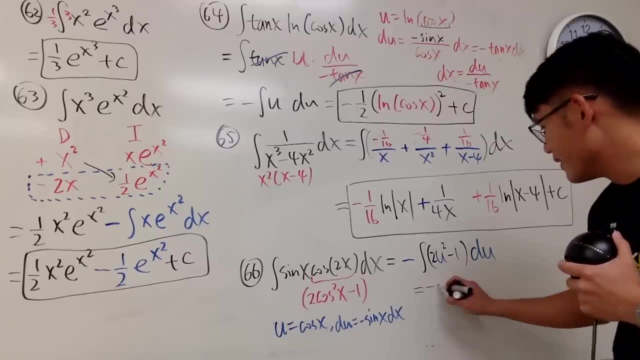 U squared minus 1, right, Yes. And then you are going to just integrate this Negative parentheses. this is going to give us 2 third. U to the third power. let me just actually make it clear for you guys: U to the. 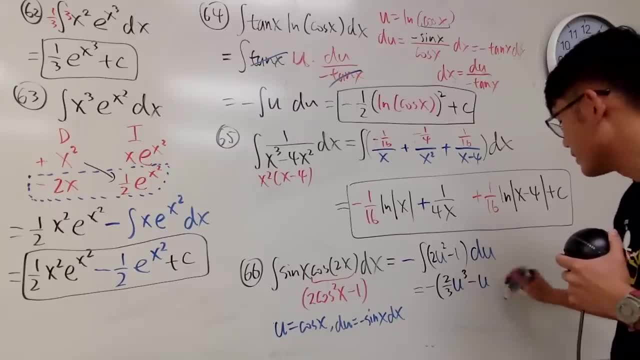 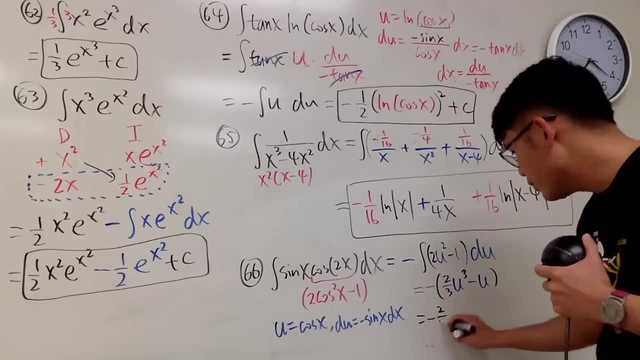 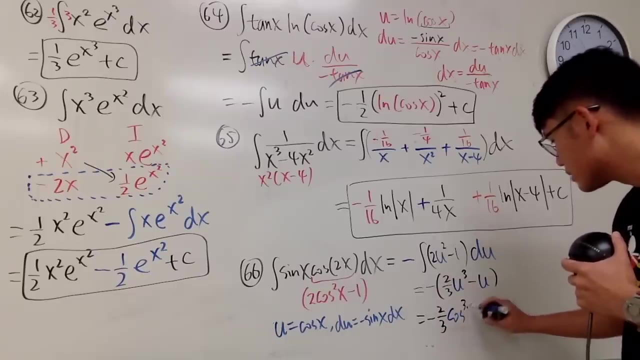 third power. why not Then minus U like this: Alright, finally distribute and then take this back to the X world, so you get negative 2. third, and the U is cosine, so we have cosine. to the third power, X. 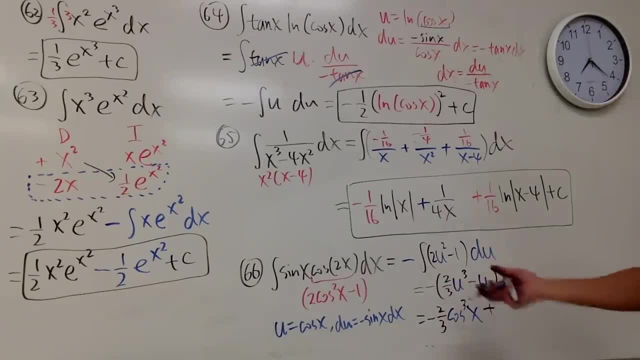 Negative times. negative is positive, and then you have cosine. Do not just put down X, you have to integrate one in the U world. so that's why it becomes cosine here, Cosine X, like that, and we're done. Put plus C. 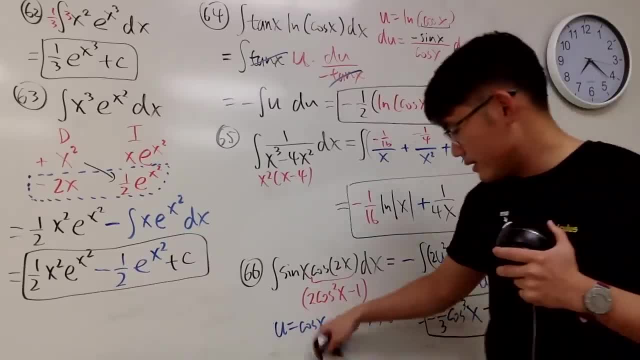 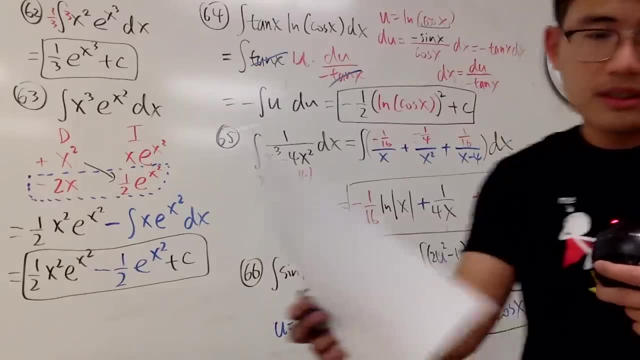 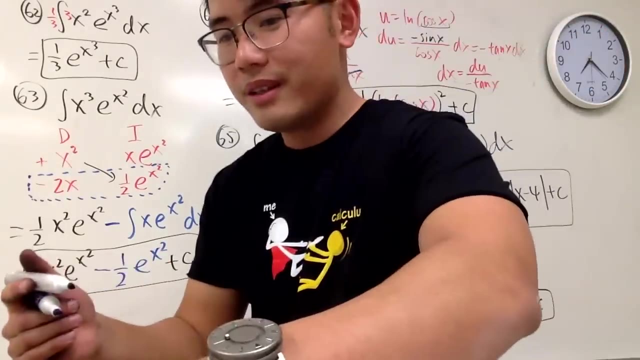 like this right. So that's it for that and I am going to see this is 66.. I'll put this down. I will go take a quick restroom break, but like the restroom is kind of far away, so 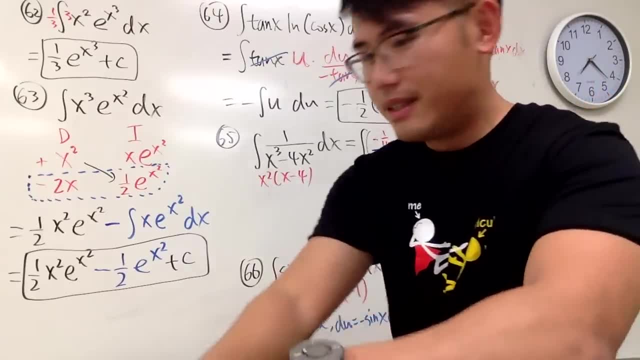 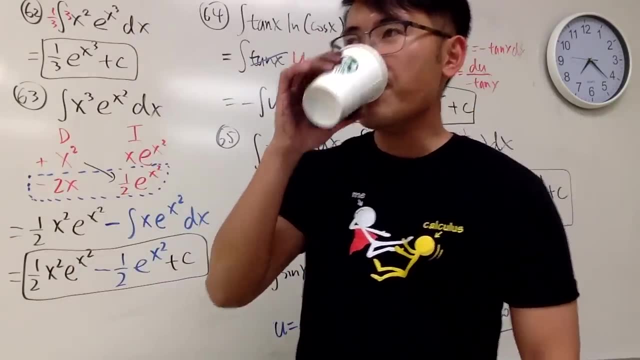 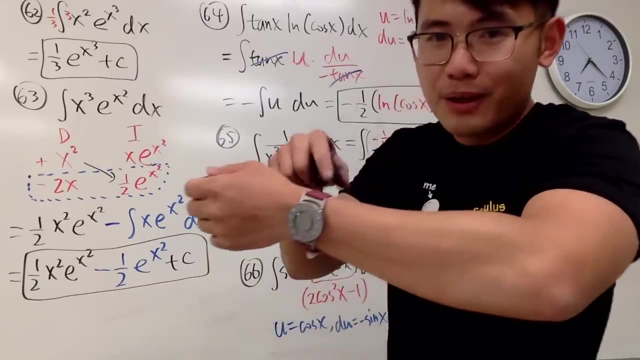 I'll close the markers over there. Still recording, still recording, okay, And I'll drink some coffee. I did a lot of integrals, non-stop Tiring. By the way, my girlfriend got this for me, Cool huh. 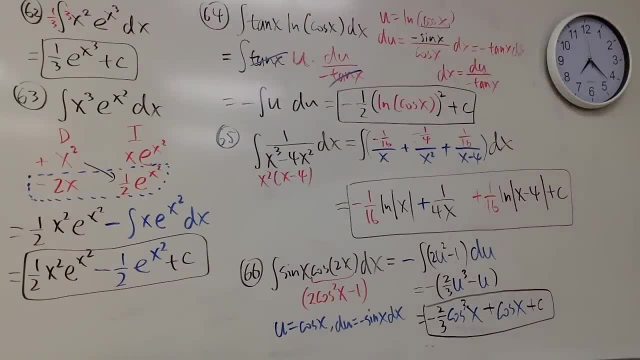 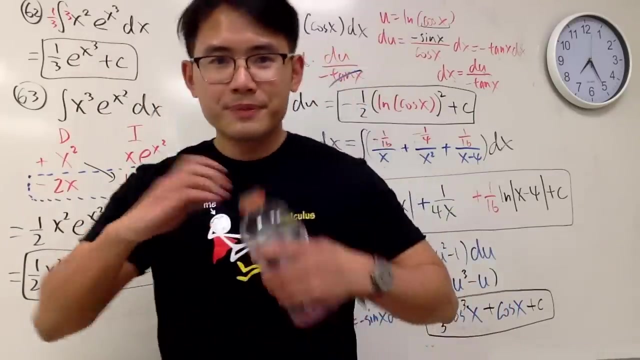 Alright, be back soon, Bye. Subtitles by the Amaraorg community community- wwwamaraorg. wwwamaraorg. Subtitles by the Amaraorg community. Okay, almost four hours. Subtitles by the Amaraorg community- wwwamaraorg. 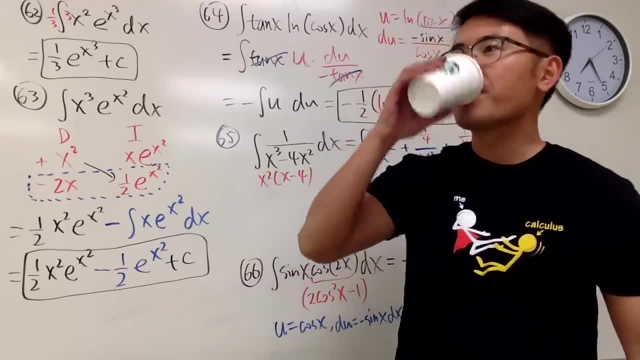 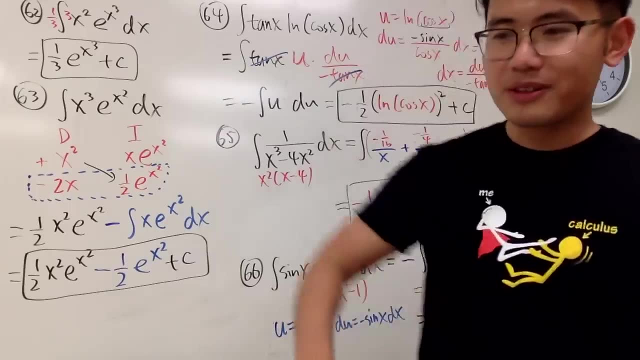 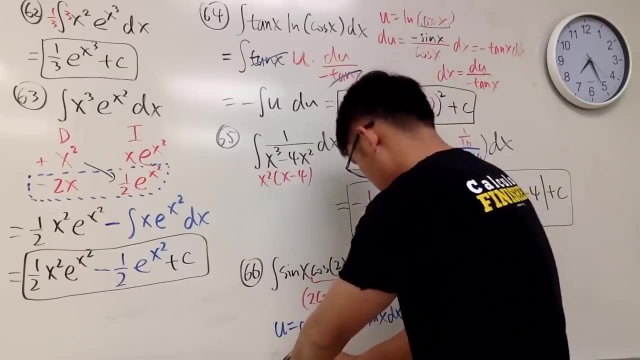 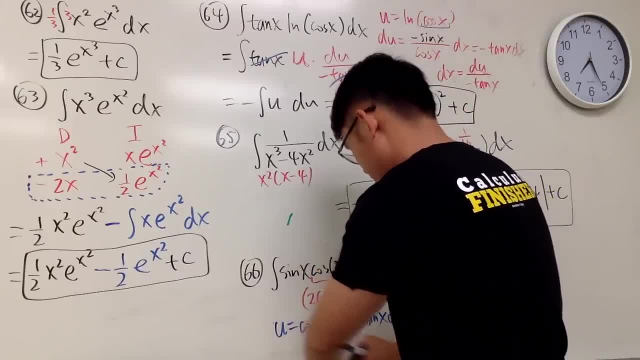 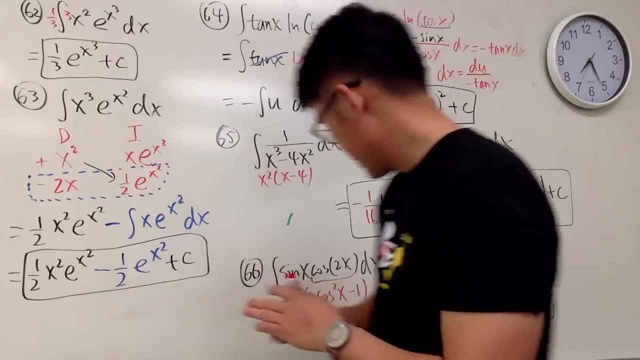 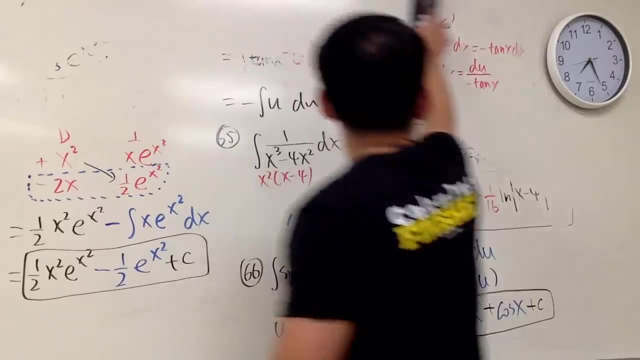 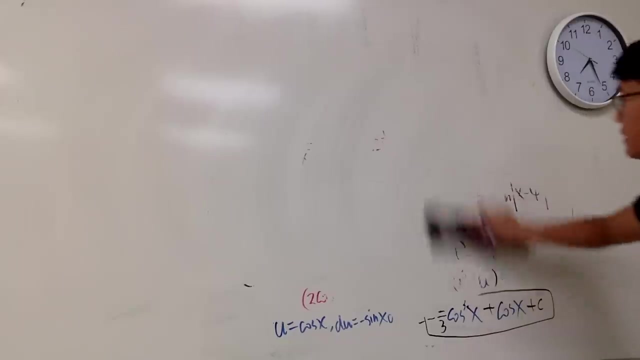 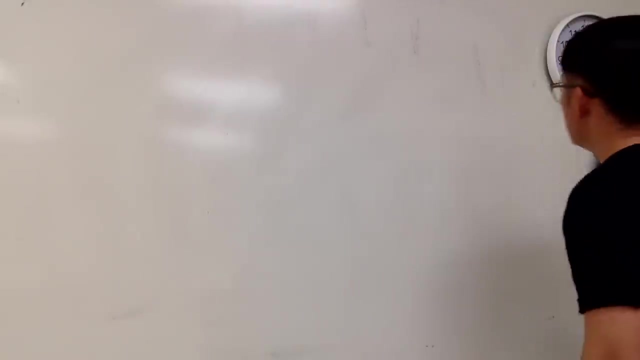 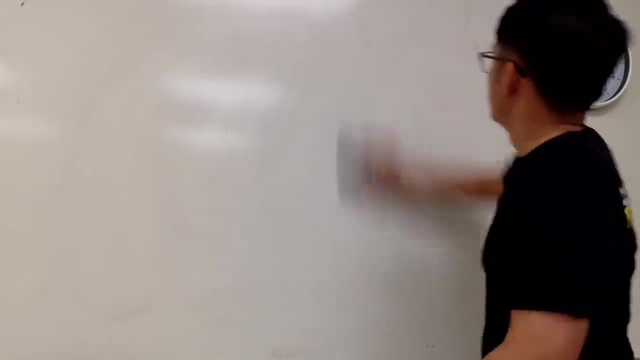 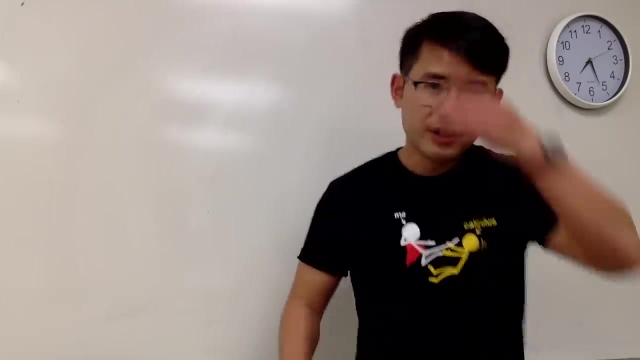 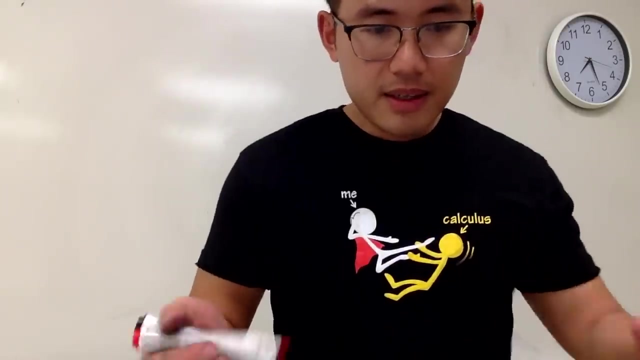 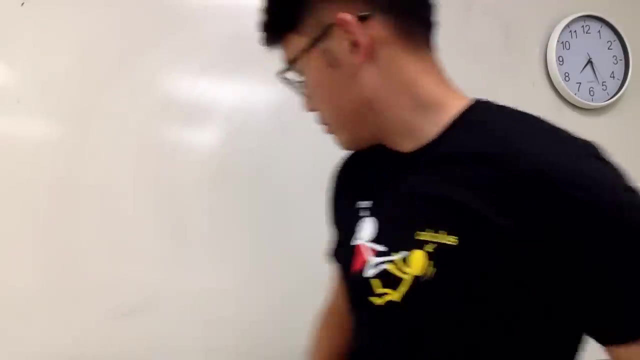 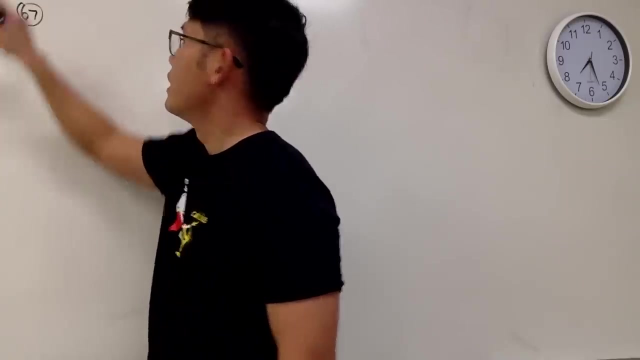 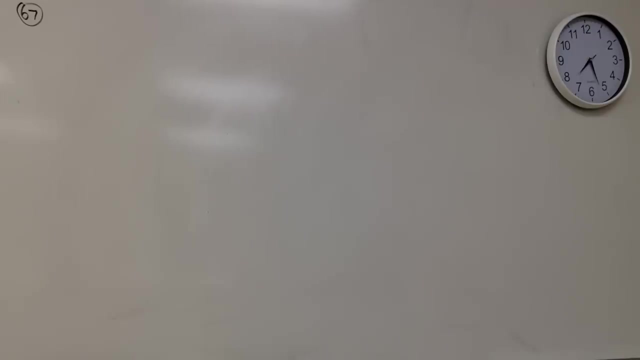 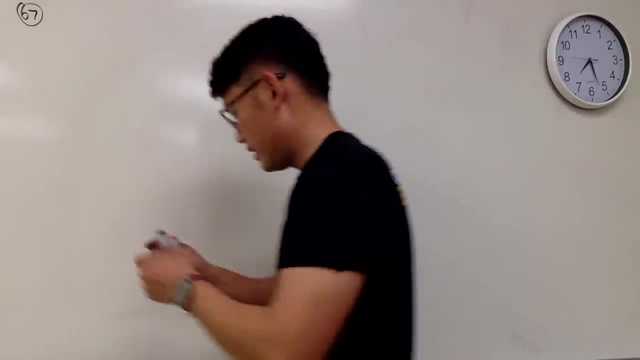 Show you some. Maybe now, okay, Maybe All right, so continue, All right. 67,, I believe. Okay, so 67,. and then, in case I need more markers, I'll have more, I'll have more black ones. 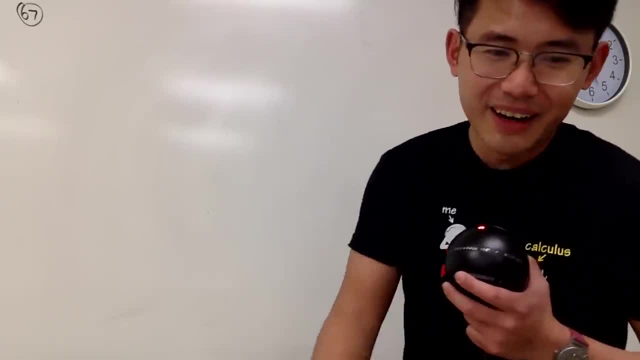 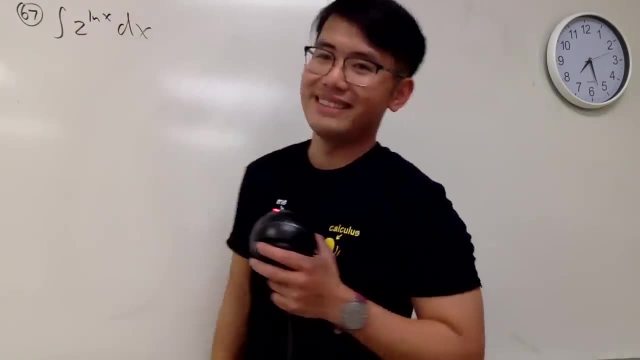 Okay, Okay in this video- no, just kidding, I know I'm recording, okay. So number 67, integrating 2 to the natural log of x power. As you can see, the power is a function. that's no good. 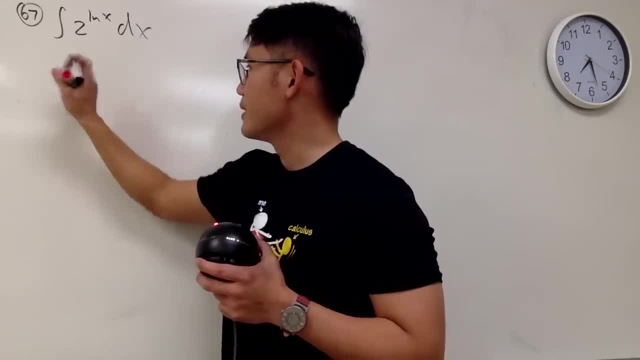 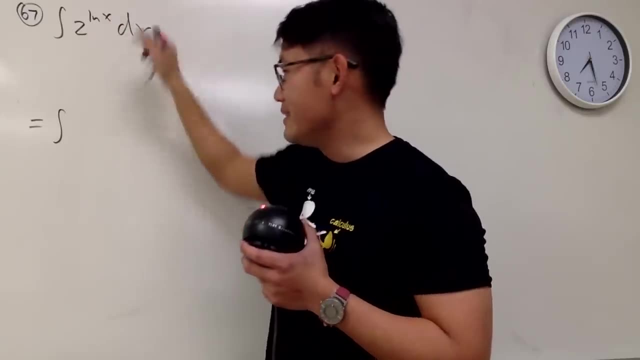 And here is the deal. I'm going to prove this to you guys in two lines or so, but this is actually the same. This is really cool. You can actually switch this and that This is actually the same as integrating x to the natural. 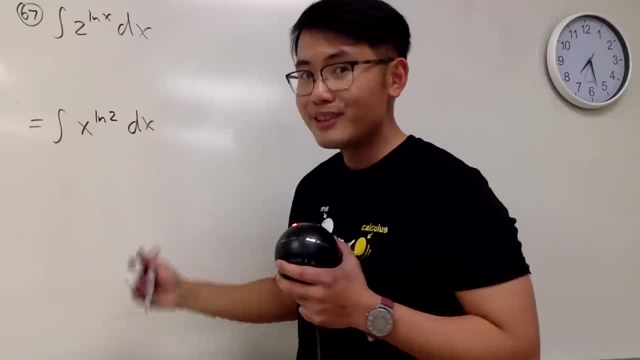 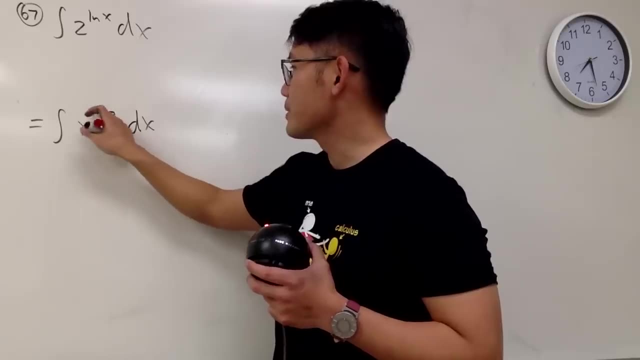 to the natural log of 2 power And the deal is that this is a constant now And you can do the usual thing: You can add 1, but perhaps I will just put- let me put parentheses first- add 1,. 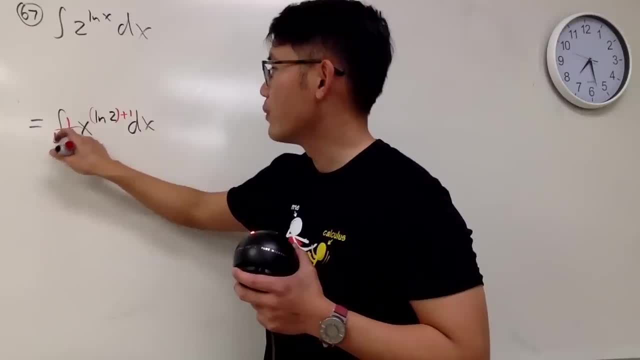 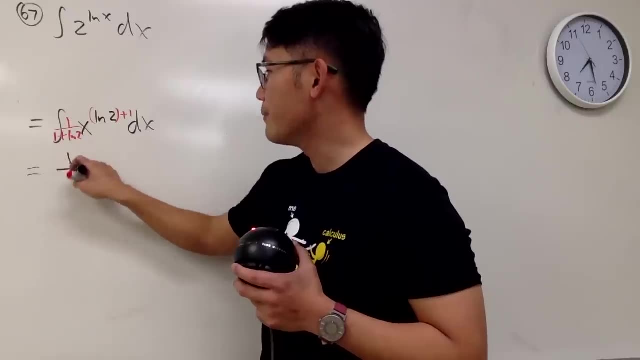 and that's the new power, and you divide it by the new power, which is 1 over 1, plus natural log of 2.. So in the end you can actually end up to get 1 over 1 plus ln 2,. 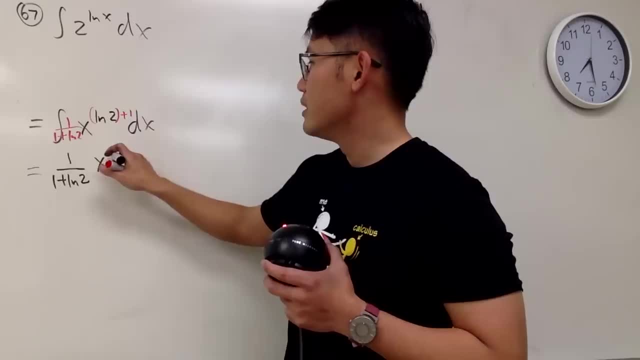 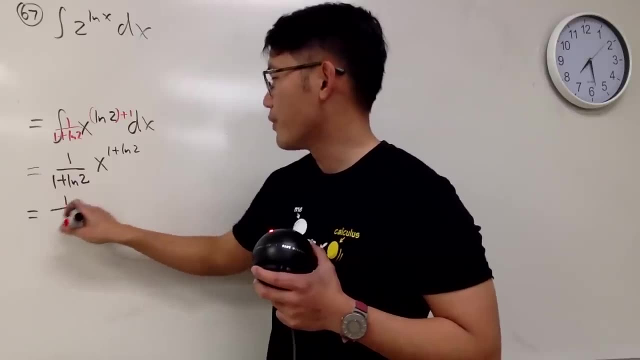 and then you end up with x to the 1 plus ln 2 power, right, And if you would like, you can write this as 1 over 1 plus ln 2.. And you know, this is the x to the first power. 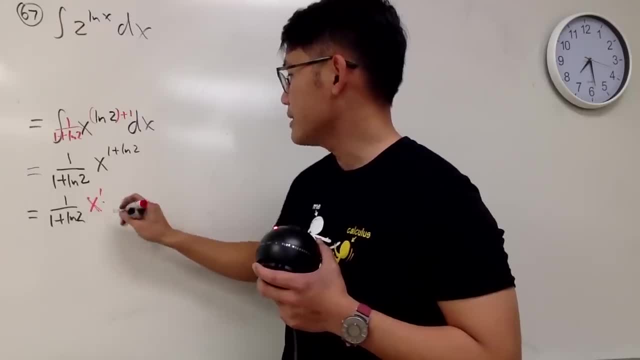 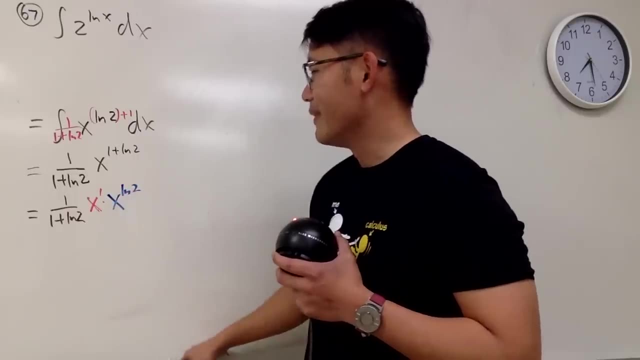 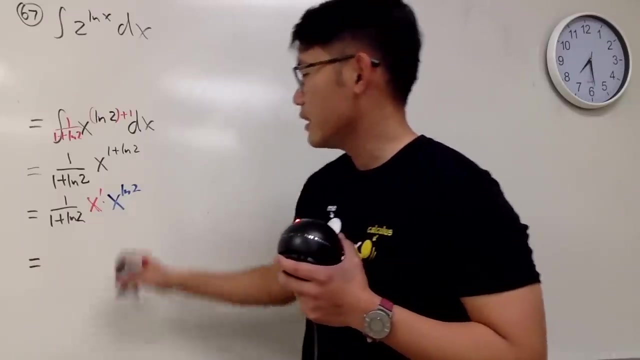 x to the first power times, x to the ln 2 power, x to the ln 2 power, And the deal is that this is the same as the original. So if you really want, you can do the following: This is the same as put down x right here. that's how it is. 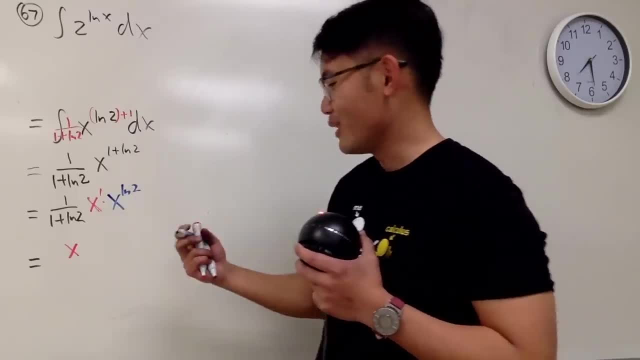 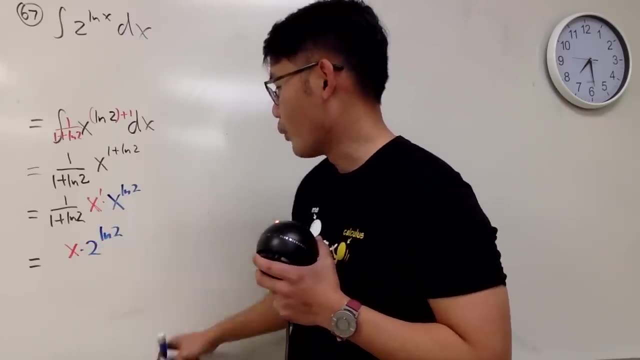 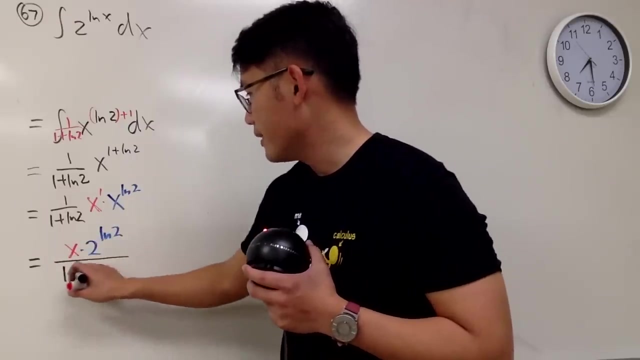 but this. I will write it back as 2 to the natural log of 2.. So we have: multiply 2 to the ln 2 power and then divide this guys by 1 plus ln 2, like this, and we're done. 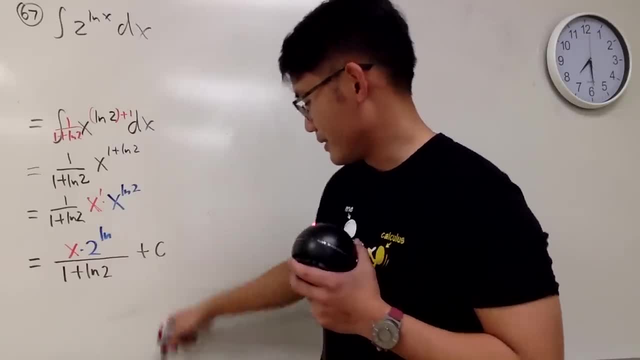 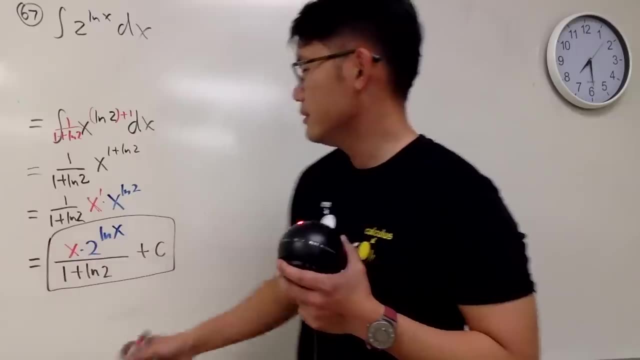 Plus 2, no, no, no, no, no 2 to the ln x power. sorry, sorry, Like that. okay, So we're good. Okay, Now I'll take some time to show you guys, why this is true. 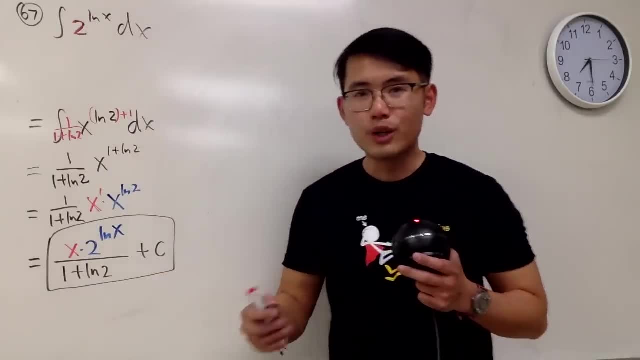 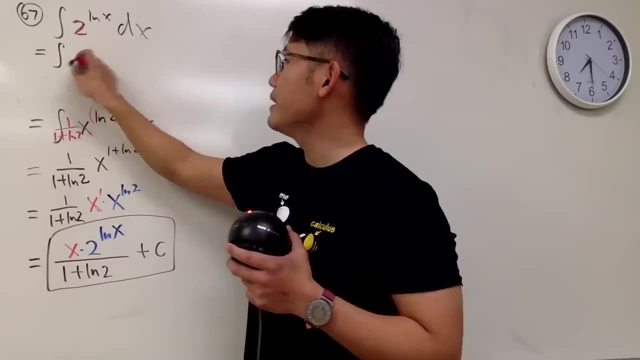 Because, as usual, we don't like to work with space 2.. We like to work with space e. okay, So this is what we can do. We can look at this as integral 2 is the same as saying e to the ln 2 power. 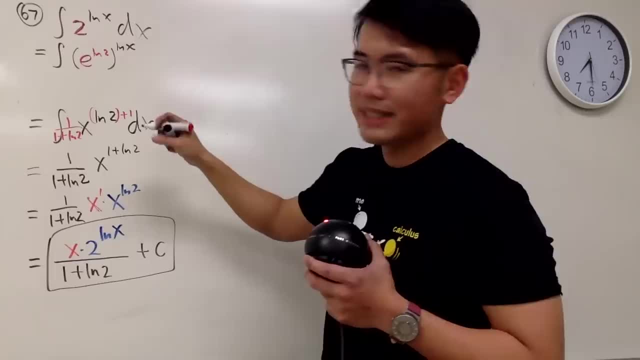 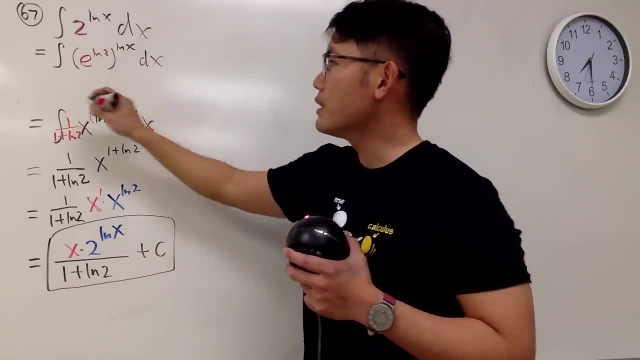 And then you take this raise to the ln x power, like that right, And then of course you still have the dx. But once you have this right here, you know you can multiply the powers. you can look at this as the integral of e right here. 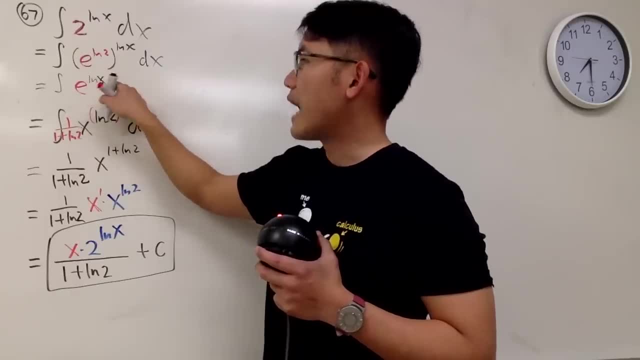 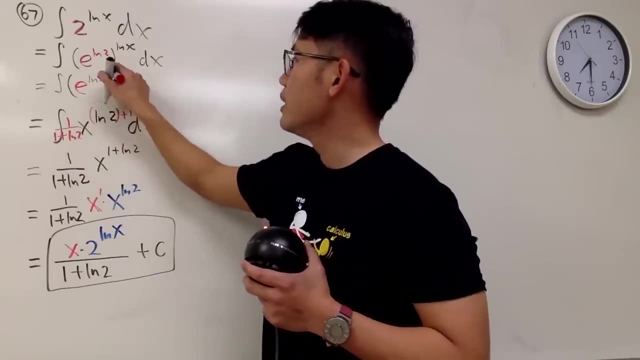 and then ln x times ln 2. And you can actually take the ln 2 to become a power. So you can look at this and then raise that to the ln 2 power, like that, And then the dx. Very nice. 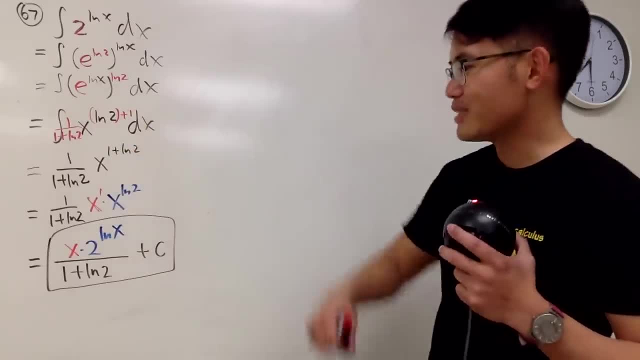 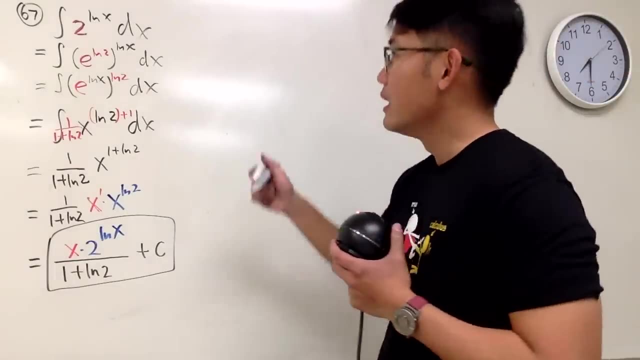 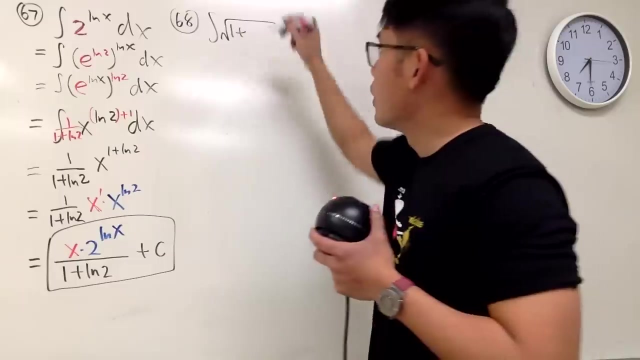 And this right here is just a nice x Nice, And that's why this works right. So that's pretty much it Now. next we have number 68,, which is the integral of square root of 1 plus cosine of 2x. 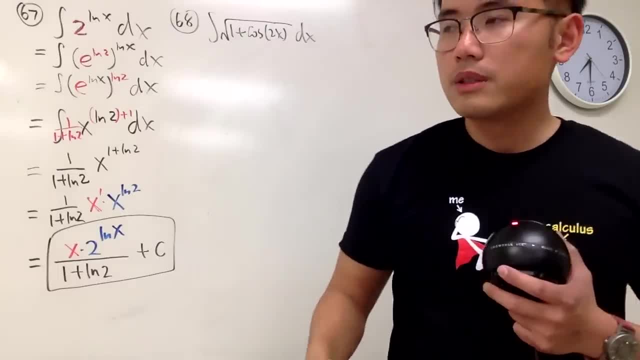 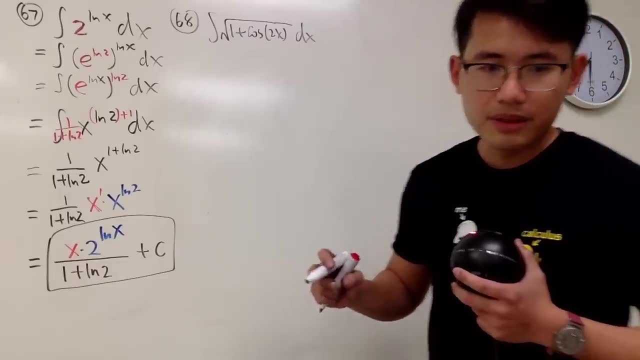 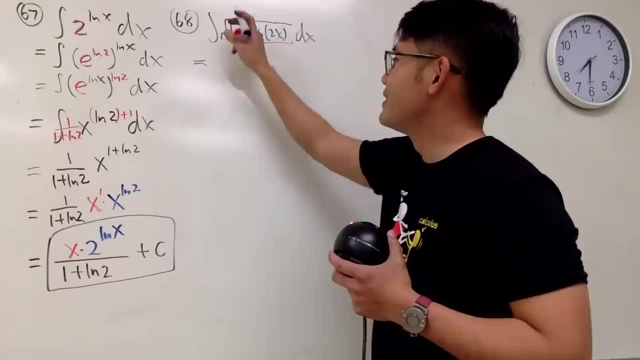 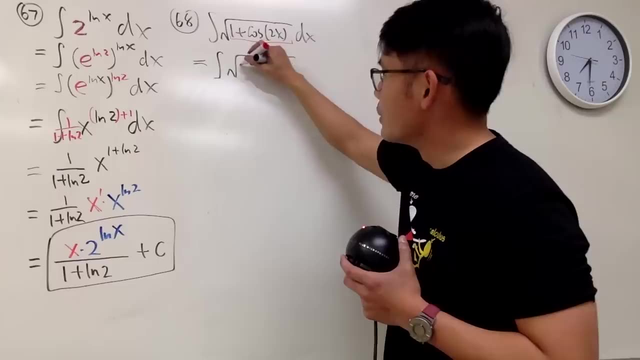 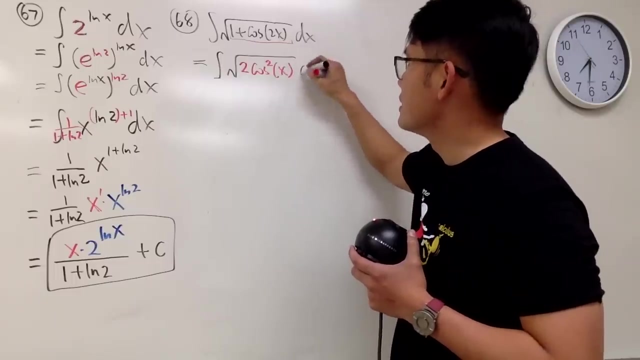 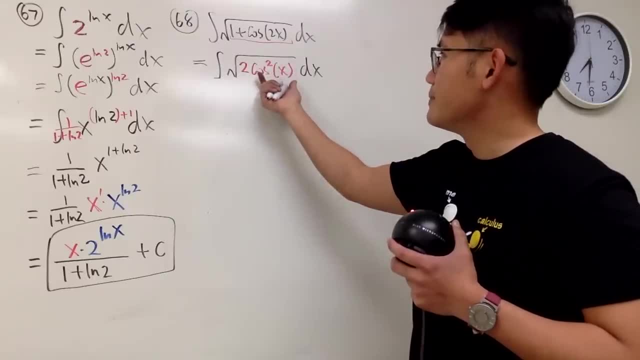 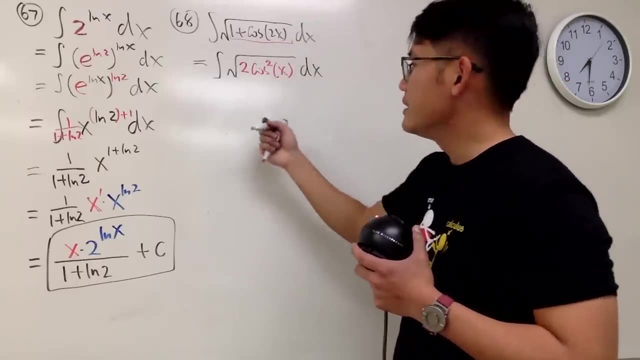 Right Again. if you use the, We can also just plug in Again, this being 2 cosine square x minus 1, which is just very nice. And here's the deal. This right here is square root of 2.. 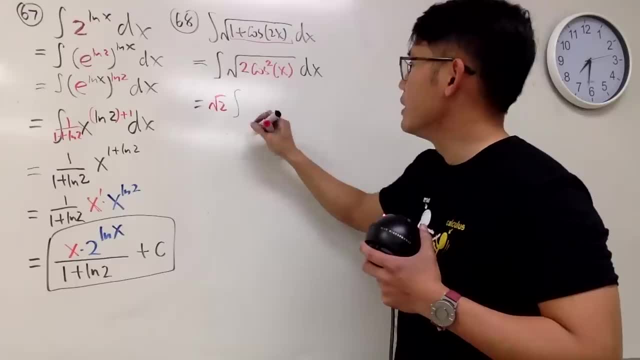 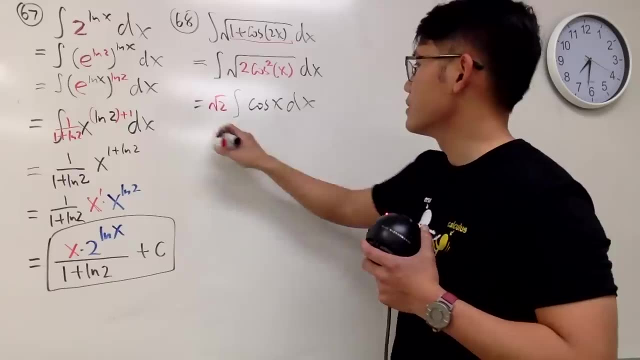 You can just take that out and then you have the integral and then you have square root cancel. So you just have to integrate cosine x- dx. So in the end this is just square root of x. Integral of cosine x is positive sine x. 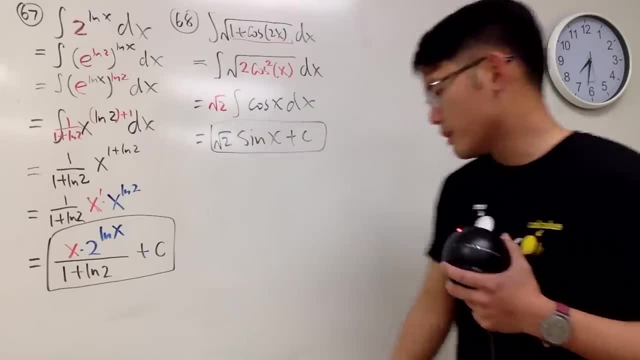 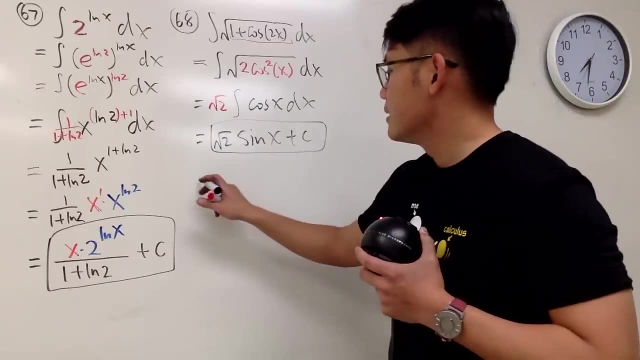 and you are done Very nice. It looks weird, but it's actually decided to be Pretty nice. Now number 9.. Oh God, Let's see Number, Not number 9.. Number 69. Right here. 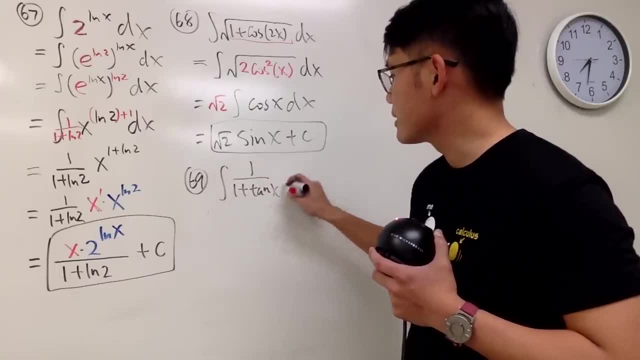 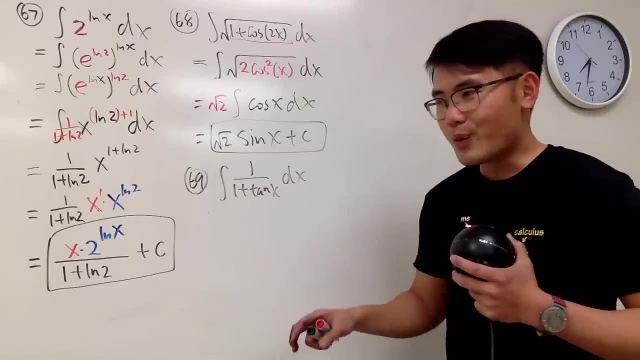 Integral of 1 over 1 plus tangent x, dx. This is bizarre, because if you write this as sine over cosine, let me tell you it's not going to work out nicely. You have to really. Yeah, you can do it like that. 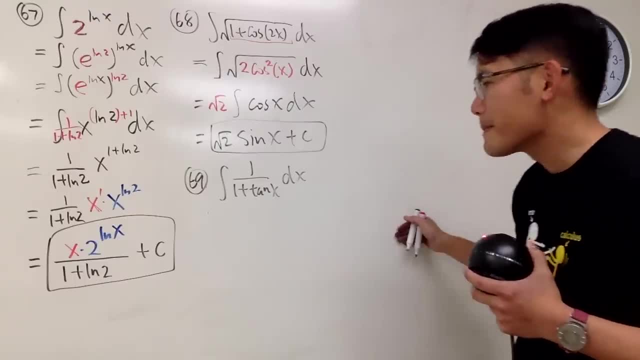 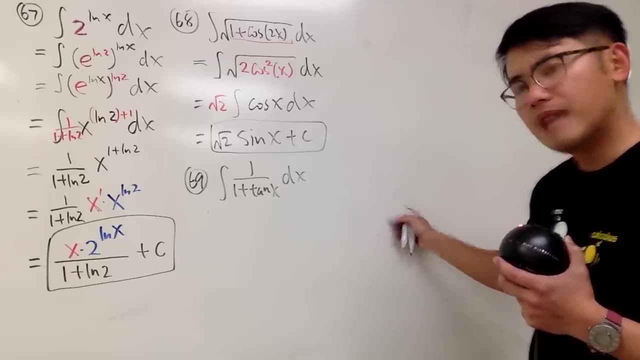 but you have to think harder, You stop, It's not going to work out nicely. okay, We are going to do that, But don't do the conjugate. So now let's see. Have we done this earlier already? 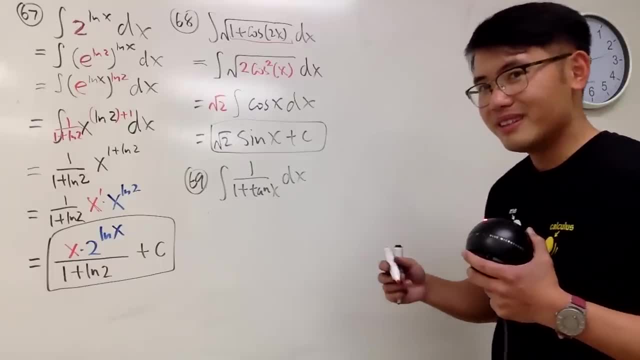 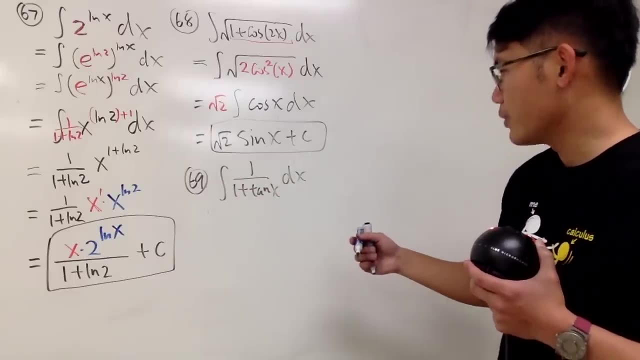 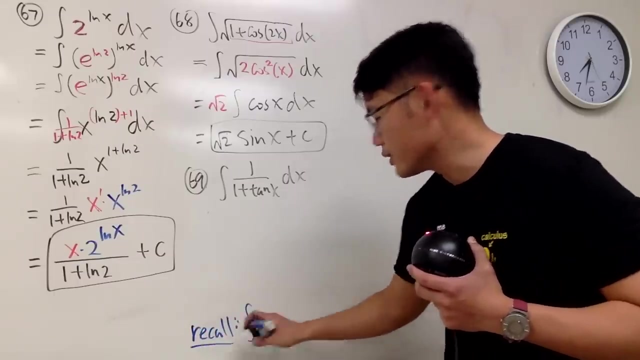 Yes, we have One of the questions we have done earlier. is the 1 minus tangent x, right? So I will just tell you. we recall, Let's put this down right here. Recall one of the questions when we have the integral. 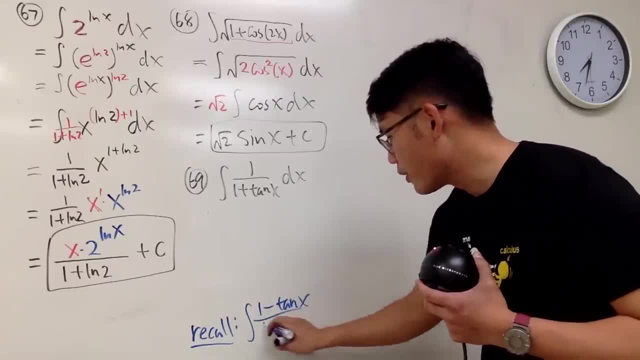 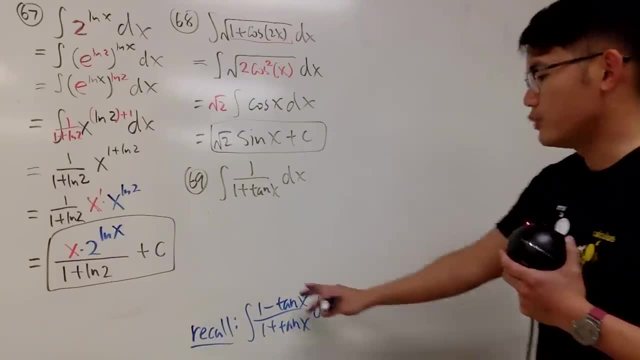 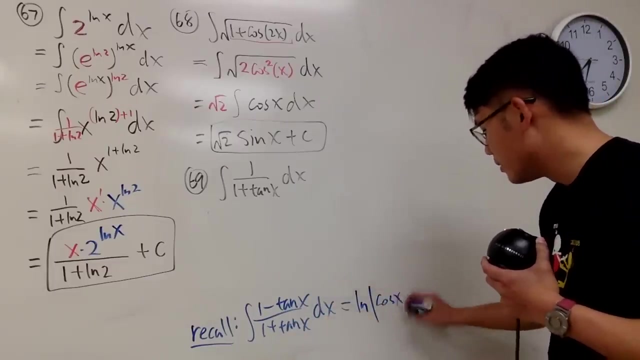 If you have 1 minus tangent x over 1 plus tangent x, dx This right here. it was actually pretty easy. You can rewrite everything in terms of sine cosine and you end up with natural log of absolute value of cosine x plus sine x. 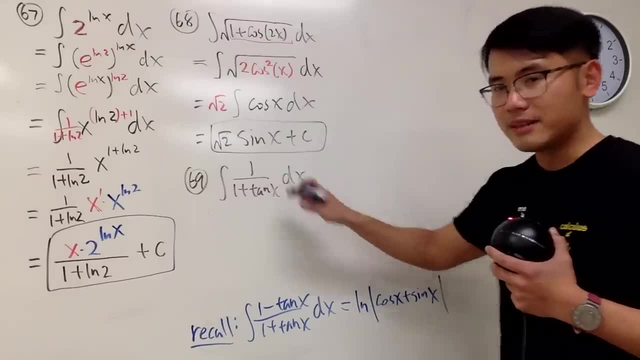 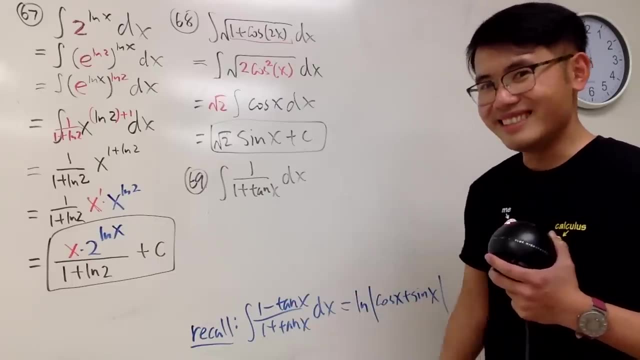 And, of course, I'm not going to put on plus t, because this is just. This is the main issue. This is not. This is easy. We did it, And imagine if you have the plus right here. That would be also just as easy, isn't it? 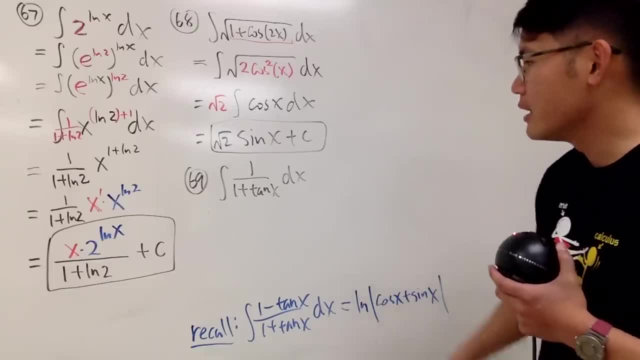 Because that would be just 1.. Now we are going to see how to make things happen. alright, So I am going to: Okay, let's look at the one right here. I have two integrals. I know better, Not this, though. 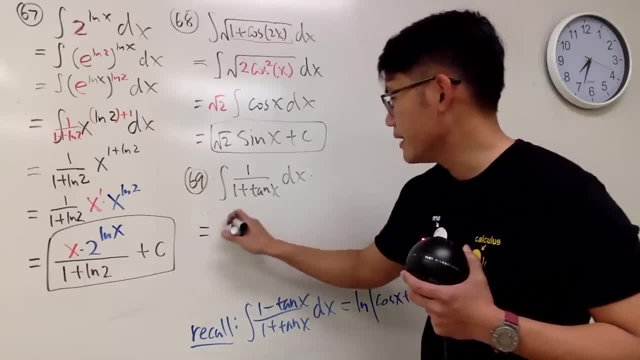 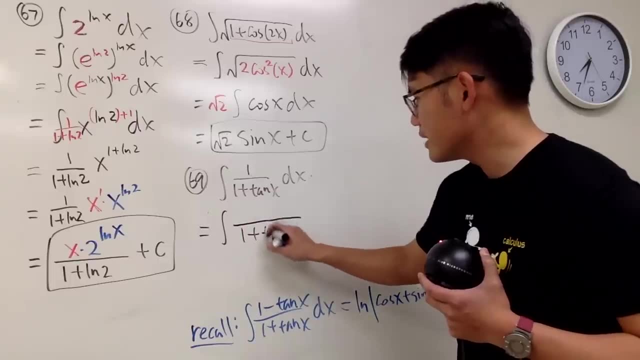 So I'm going to write this down right here. This is the integral. Okay, so here is the deal. I want to have 1 plus tangent x in the denominator Sure, And I also want to have this guy on the top. 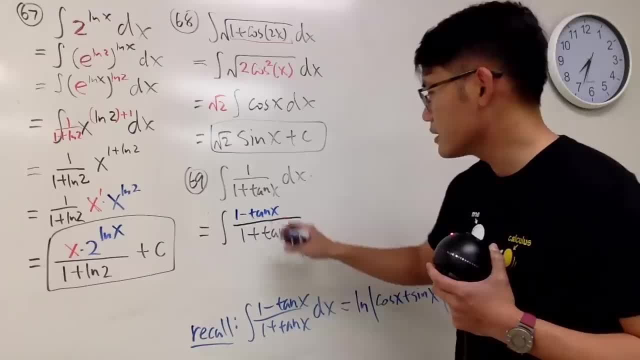 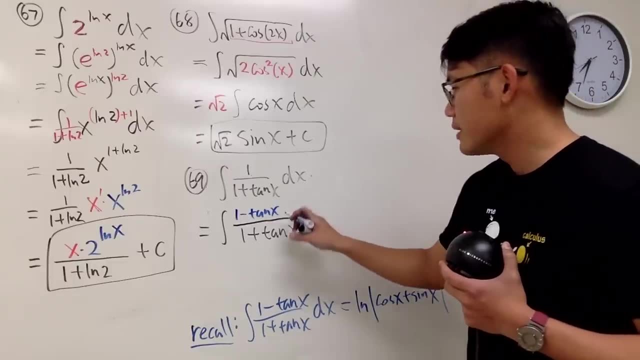 which is 1 minus tangent x. Well, in that case. well, I will just add a tangent x to it. That's okay And sure, Let's do this way. I'll do Peer out the colors for you guys better. 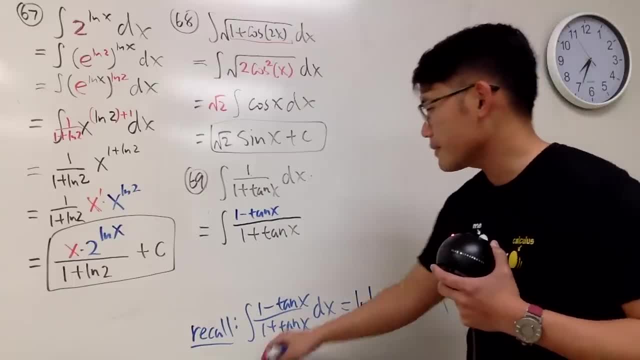 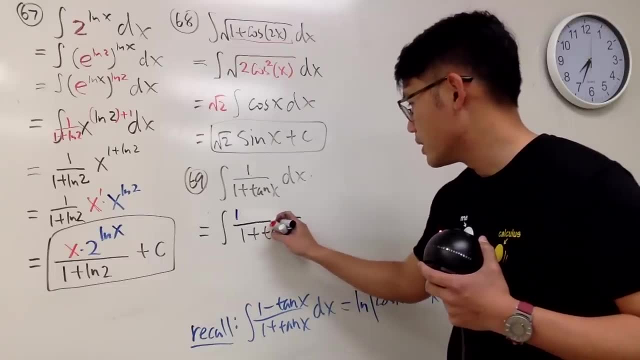 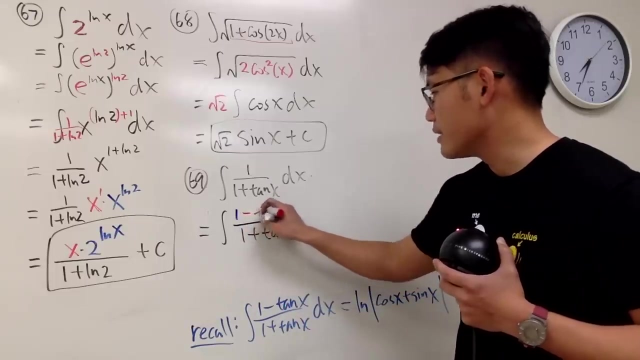 Let's do this in blue and red like Spider-Man, Alright, So let me write this down better for you guys. So I have 1, and then I want to. As I said, this was the easiest of minus tangent x, okay. 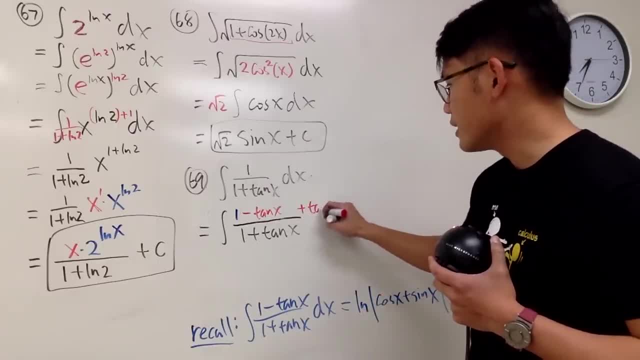 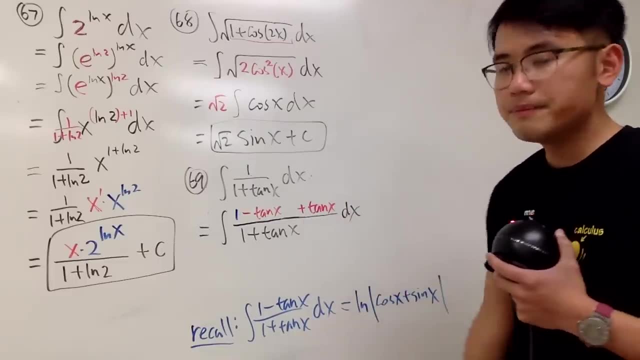 But this is not the same as the original, so let me just add the tangent x back. alright, So that's what we have, However, however. however, if you just have tangent x over that, it's kind of hard. 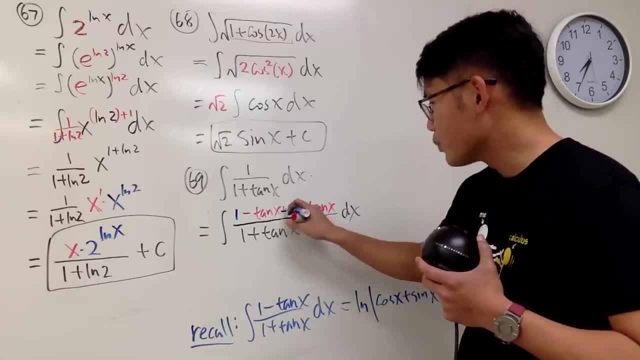 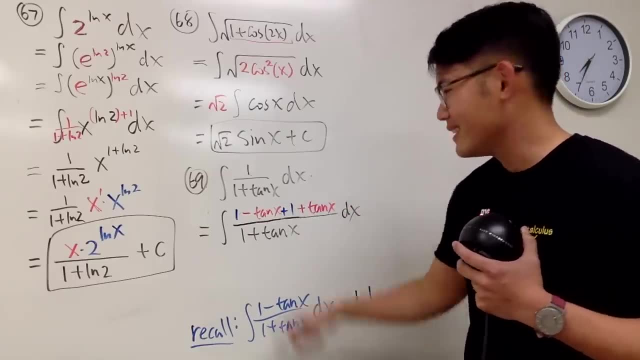 I want to have a 1 right here as well. Now let me just say plus 1 right here. But if I add 1 right here and then minus 1, that kind of defeats the purpose. But guess what? 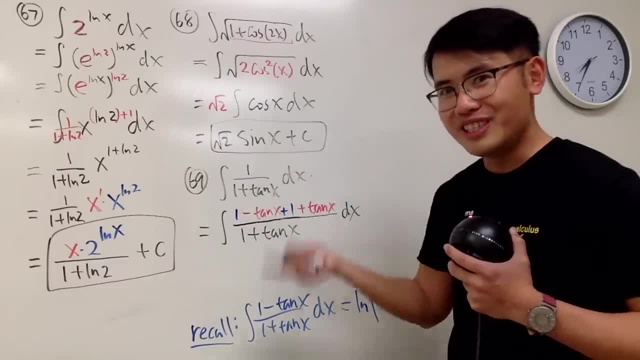 1 plus 1 in blue is 2.. To get 1, we can just divide it by 2.. So I will just put down the 1 over 2 right here. In fact, this is still equivalent to the original. 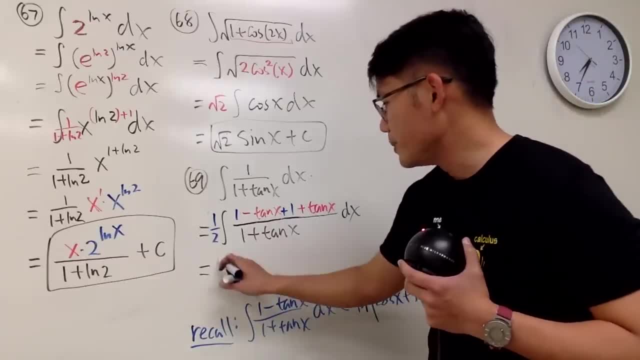 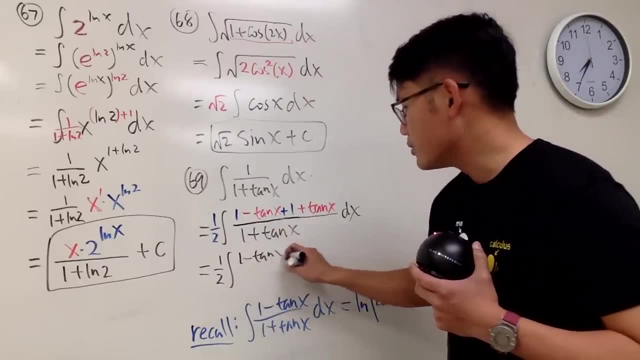 That is very nice. So in fact this is going to be 1 half. And now let's pair things up. We have the first 1 right here, which is 1 minus tangent x over 1.. So 1 plus tangent x and let's close that integral. 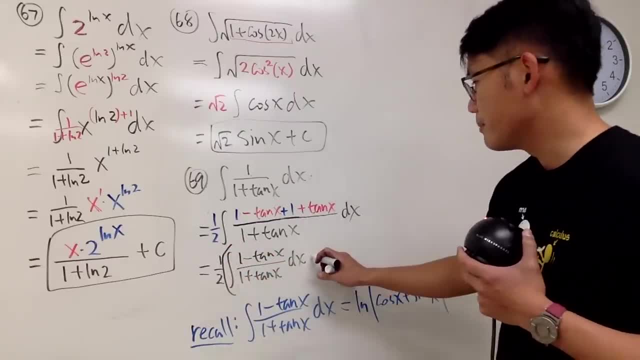 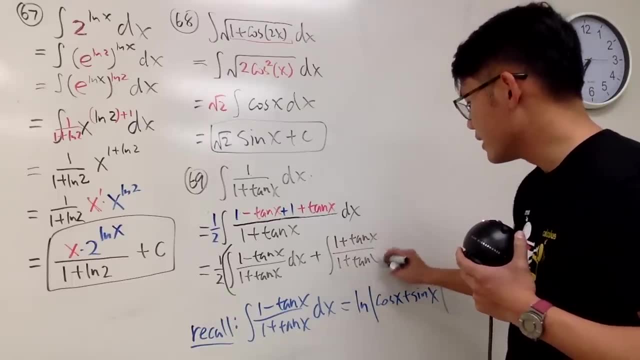 And I'm going to split that into another integral. So I'll just say plus the other one, which is the integral of 1 plus tangent x over 1 plus tangent x dx. Very nice, very nice, And we know this already, which is that 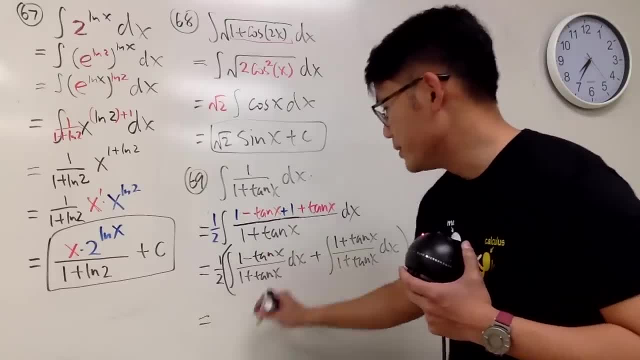 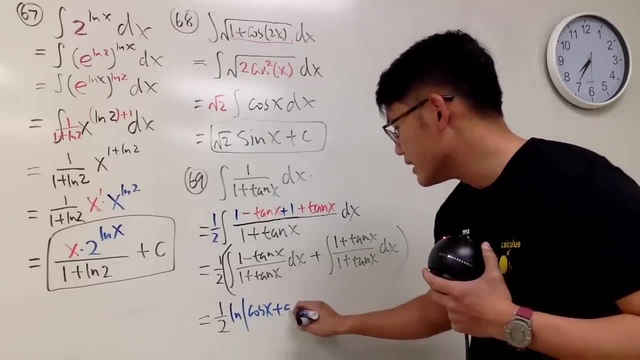 So I'm going to just write this down. I will distribute the 2,, which is 1 half, And the answer to this integral was natural log absolute value of cosine x Plus sine x. all right, And the answer to this integral is just x. 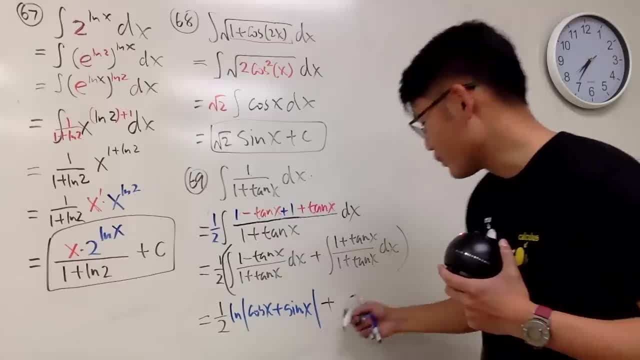 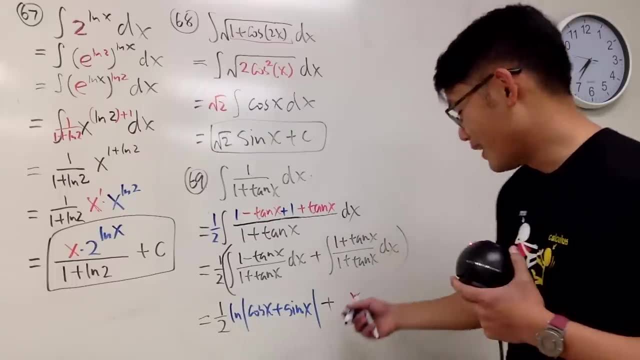 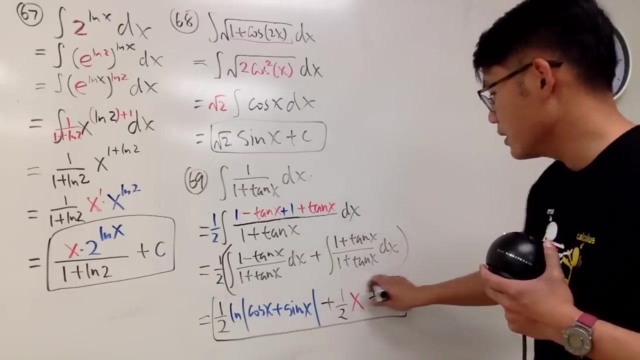 So we add- perhaps I'll put this down in red- why not x? Yes, I still have to multiply by the 1 half. I remember that. okay, And then we are done, plus c: This right here. 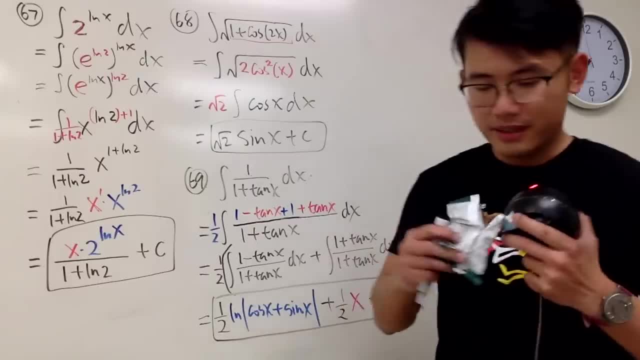 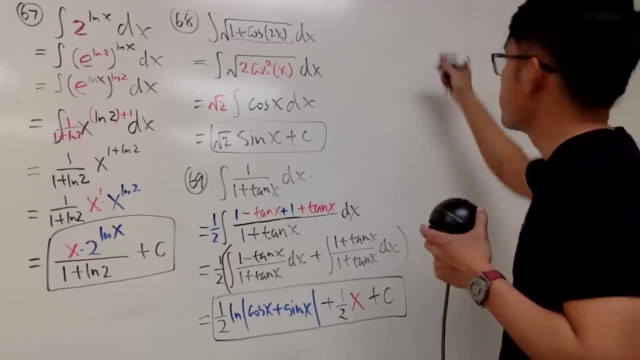 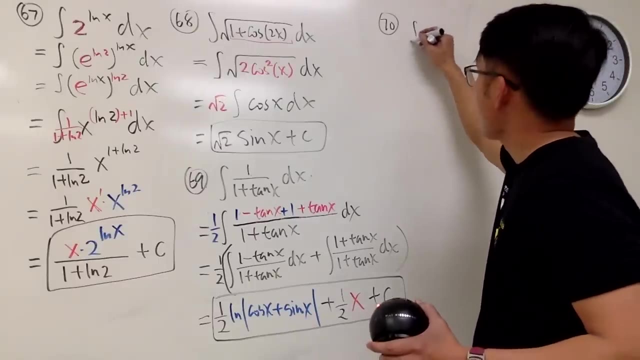 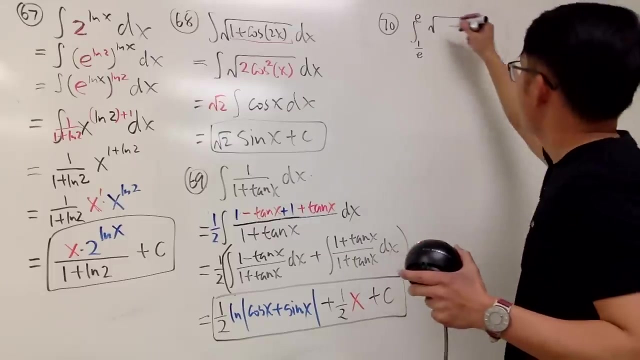 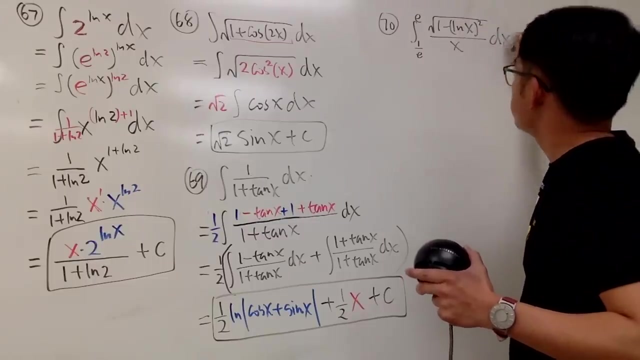 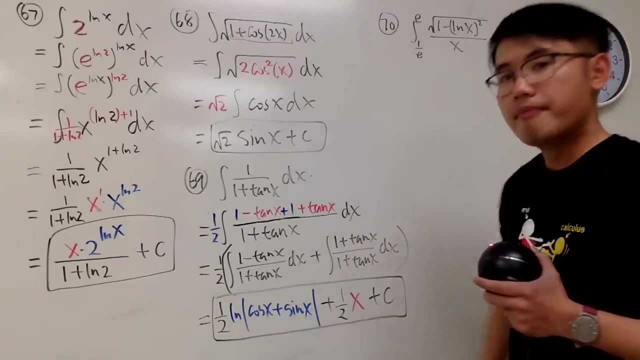 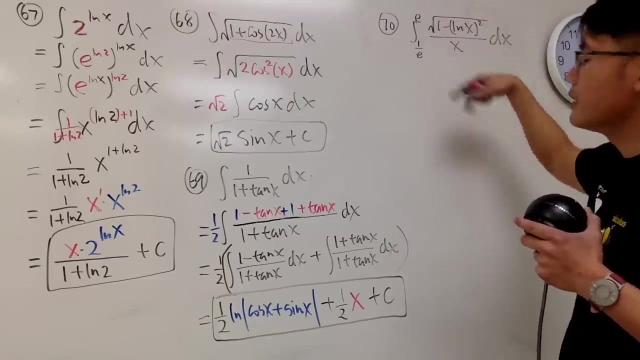 This is it, All right. click four times, seriously, All right, so that's the deal. Now number 70.. The integral from 1 over e to e, square root of 1 minus natural log of x and then square and then divided by x. 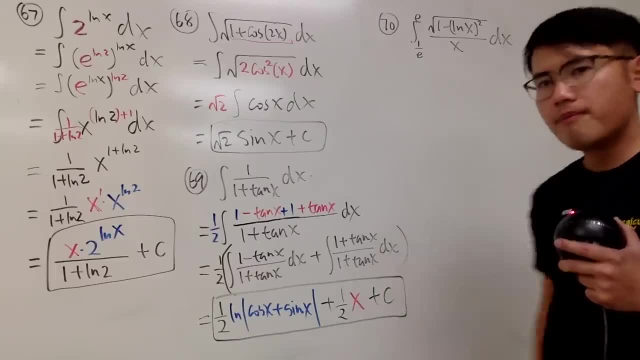 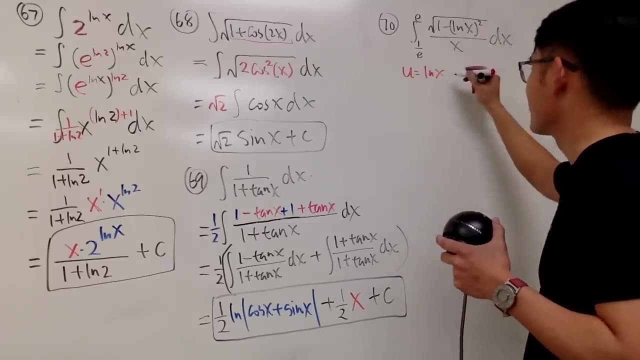 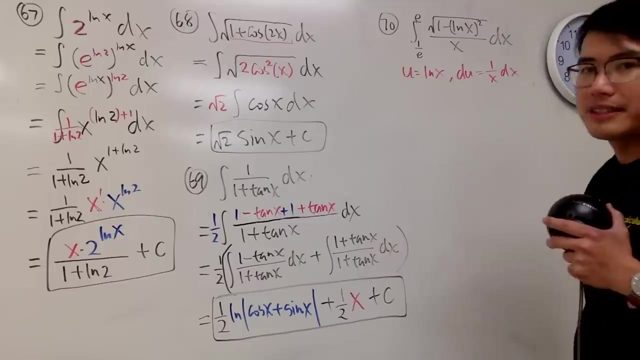 Okay, Well, u sub. of course, let u equal natural log of x, because that's our only candidate, That's the one that makes the most sense. And then du is of course 1 over x dx. Ha, that's very nice. 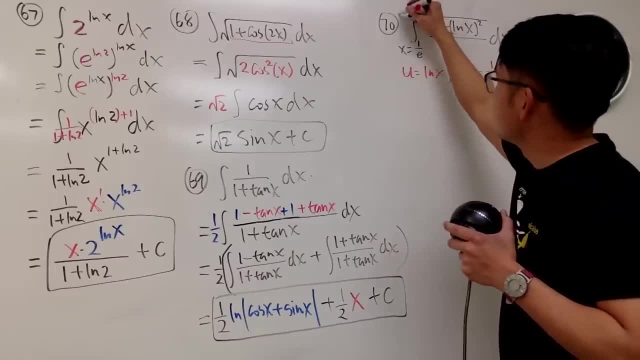 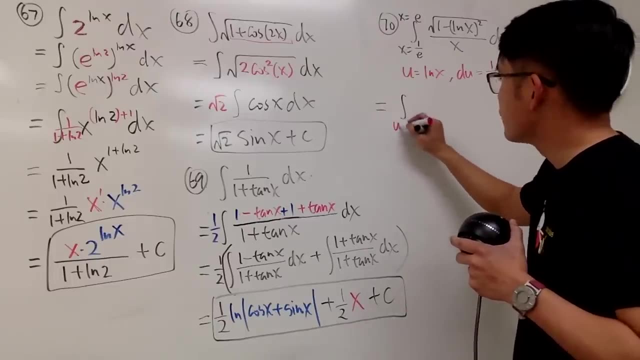 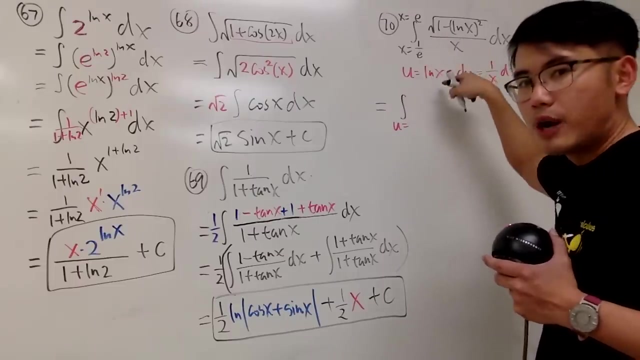 Well done. Now, don't forget, this is x going from 1 over e to e. So here is the deal. Take this integral to the? u world. u goes from what? When you put 1 over e in here? 1 over e is the same as saying e to the negative 1.. 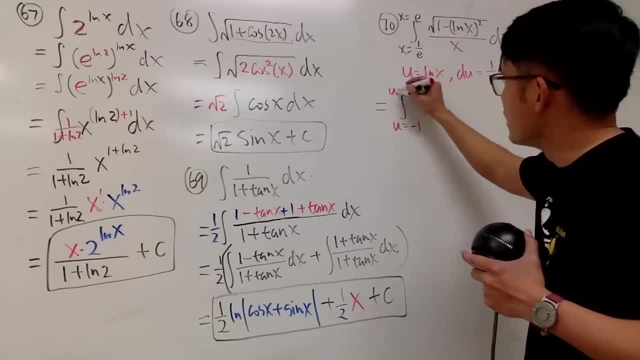 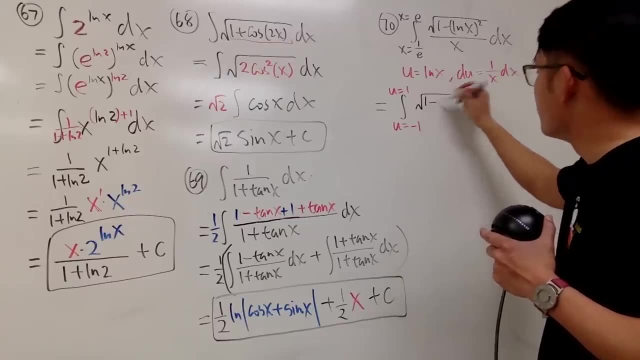 Put into ln, you get negative 1.. e in here, you get positive 1.. So u goes from negative 1 to 1.. And then you get the integral of the square root of 1 minus u squared. And then you get the integral of the square root of 1 minus u squared. 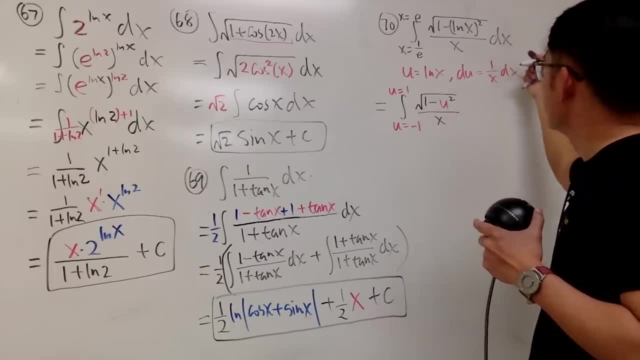 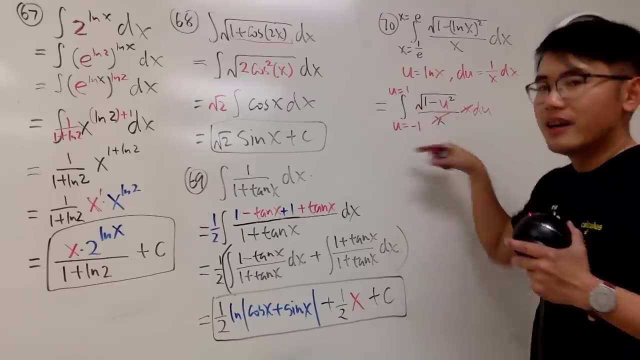 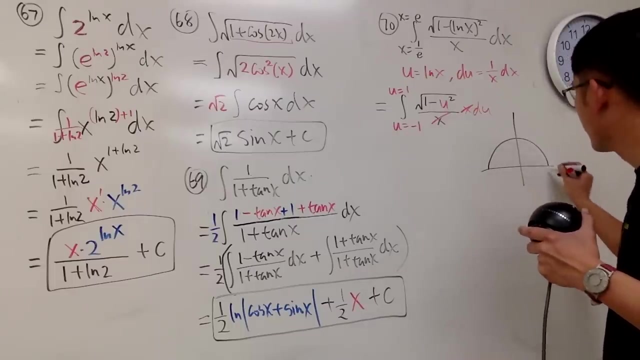 Here over x And then dx. Well, dx is technically x du, if you multiply x on both sides. so they cancel out nicely Here. Nice, Very nice, Because this right here is precisely a semicircle with a radius 1.. 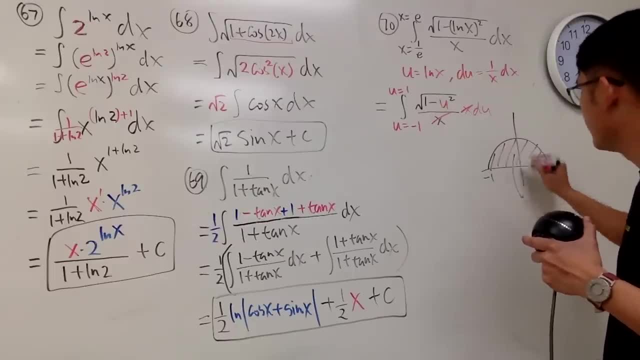 And we are going from negative 1 to 1.. And we just need to find the area. Of course It's just going to be pi times r squared, pi r squared, but since this is just a semi-circuit, so you divide by 2,. 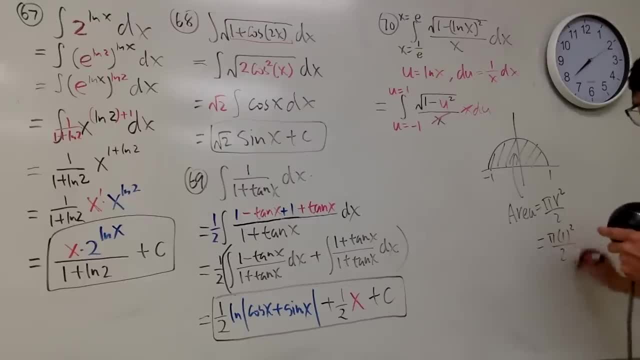 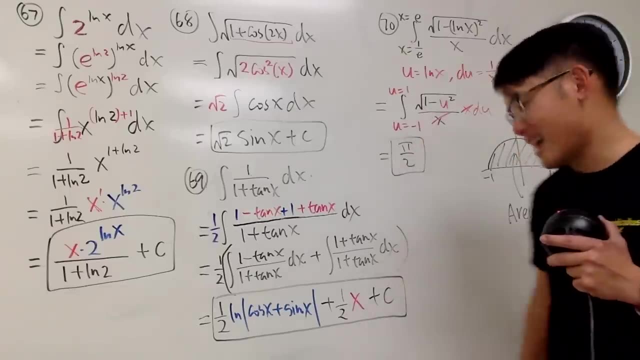 so, therefore, pi times 1 squared over 2,, in other words, pi over 2,, pi over 2, and then we are done. Very nice, isn't it? And now I'm going to see if I can switch another marker. 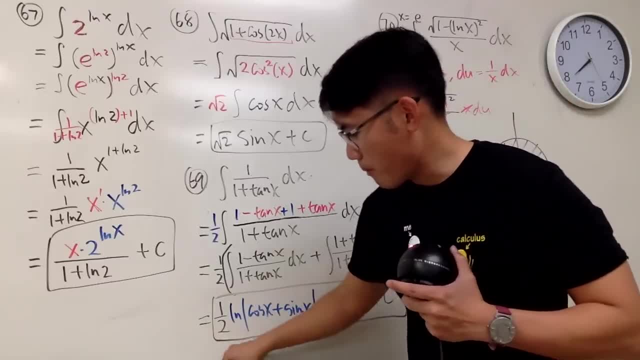 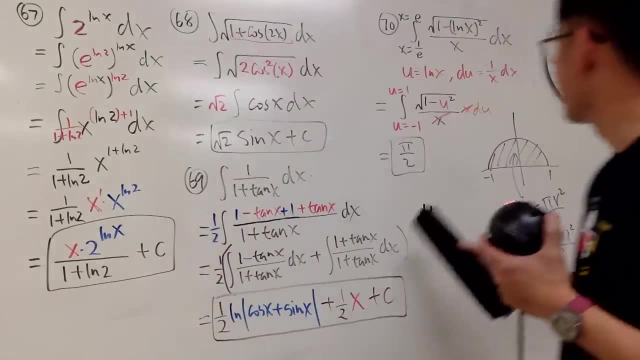 I don't know if this is going to be a better one. I don't know. I have an X-pole. usually the X-pole works better. we'll see if this one is a good one or not. So that's it, and 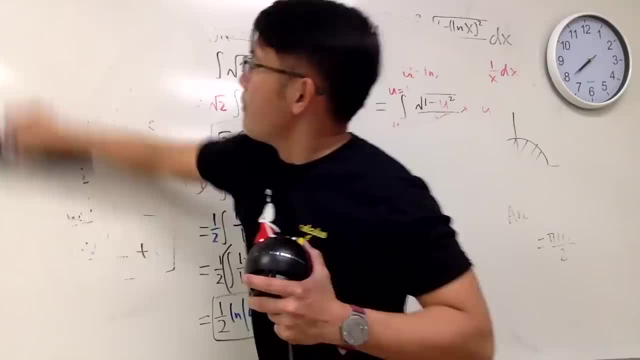 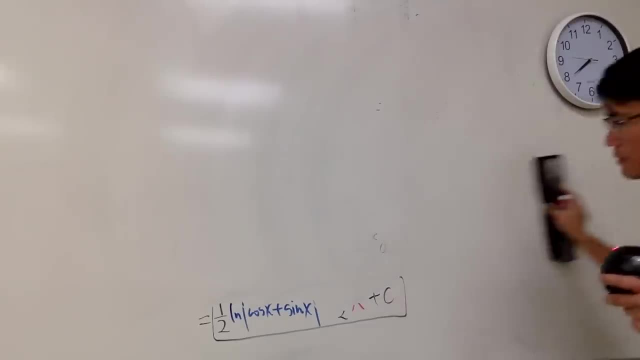 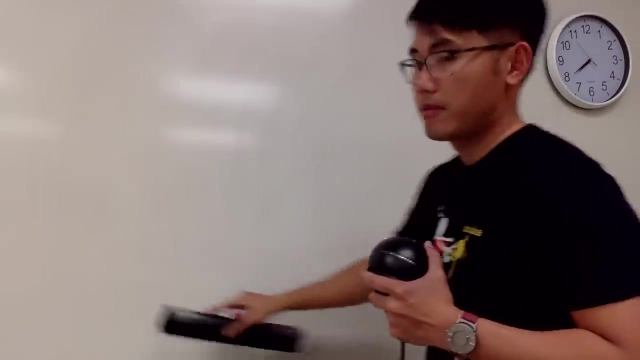 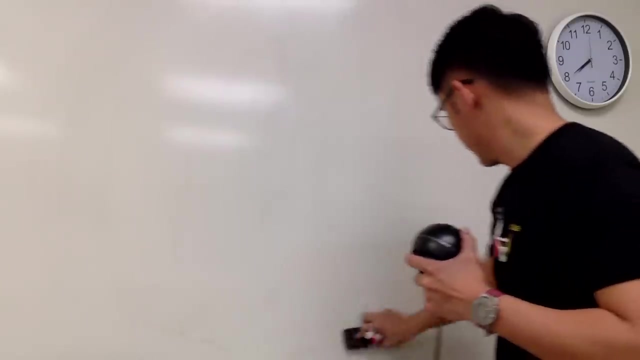 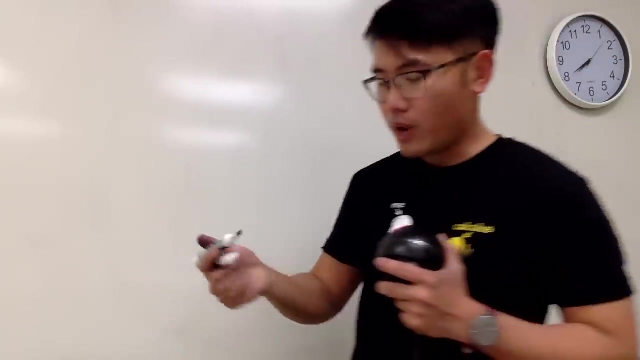 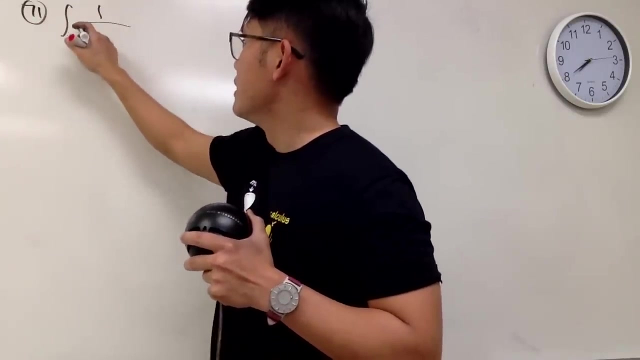 that was number 17.. Okay, number 71, here we go, And in fact, let me just do this, because this is what I do a lot- Let me write down two integrals on the spot for you guys. The first one is: 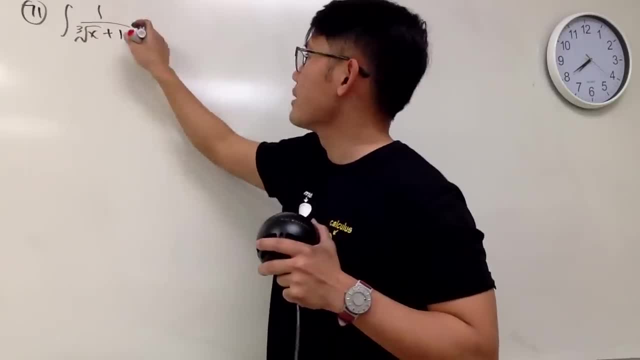 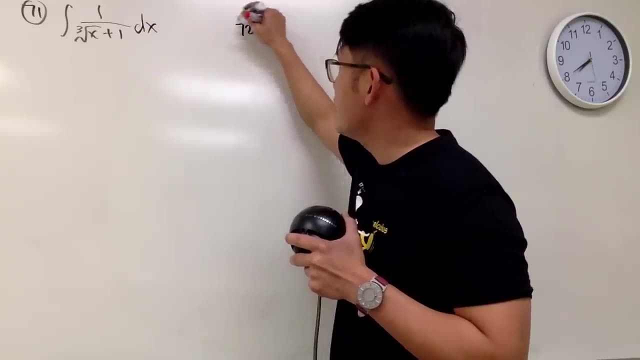 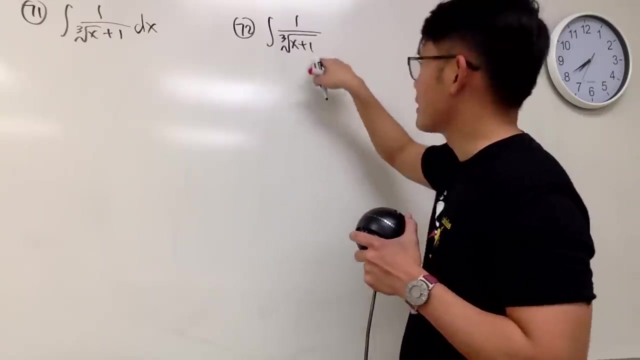 the integral of 1 over cube root of X and then plus 1 on the other side, And then I write down like this: and then number 72, let me just write it down on the side right here: it's the integral of 1 over the cube root of X plus 1, both of them inside. okay. 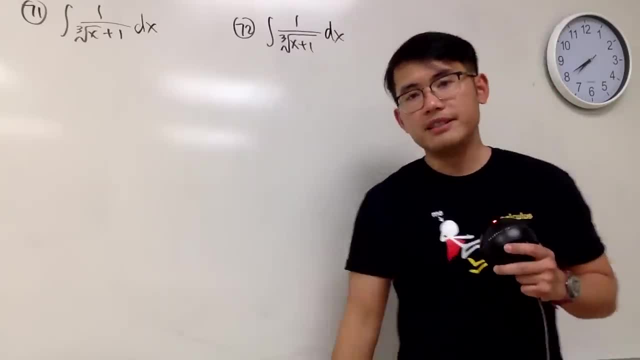 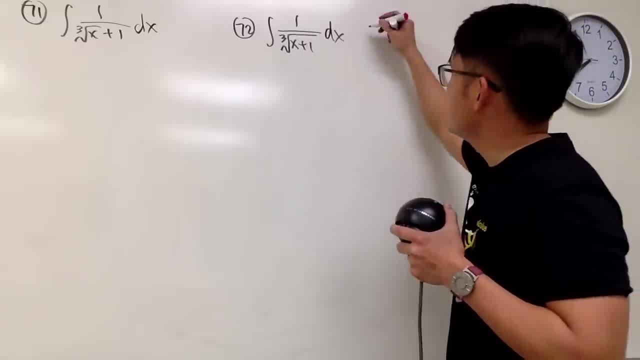 like this and then dx: Which one do you guys think is easier? The answer should be this one, because we can just do a simple u-sub. right, We can take u to be this, so u is equal to X plus 1, and in fact you don't really need to do the u-sub, because we can just 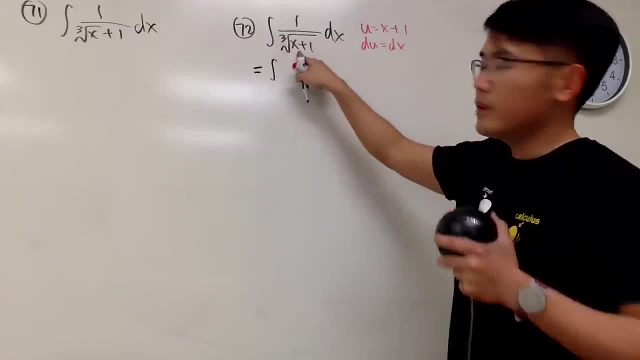 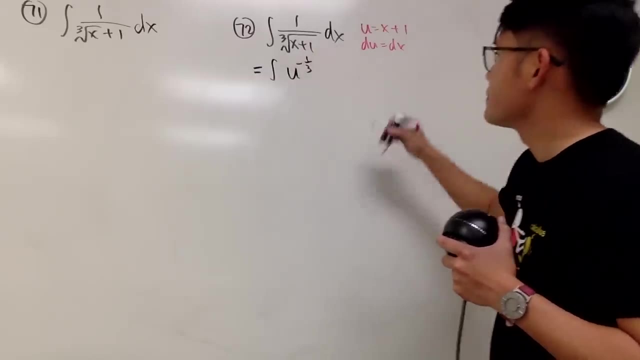 do this. This right here is just seriously pretty easy. Integral, you know, this is u in the denominator, which is the cube root, in other words, u to the negative, 1 over 3 power, and then this is the du right here, right? So let's go ahead and add 1 to the. 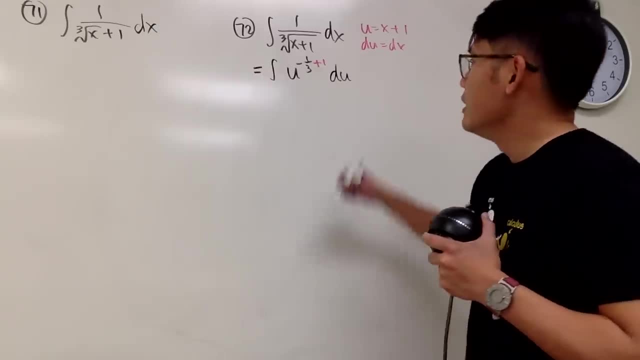 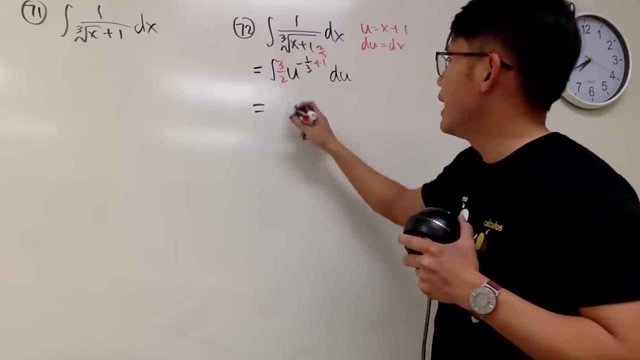 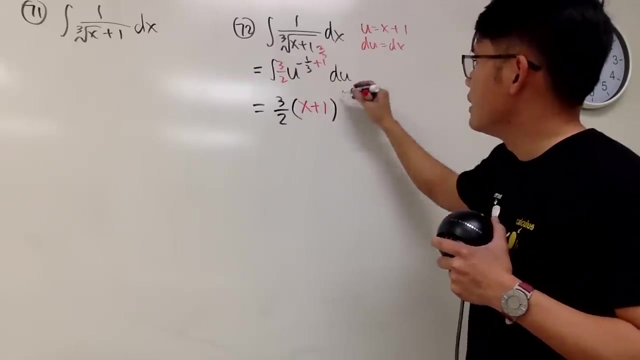 power negative. 1 third plus 1 is positive, 2 third. divided by this, power becomes 3 over 2.. So in the end we have 3 over 2, and then u is this guy, which is X plus 1 to the 2 third power and, if you would like, 3 half. 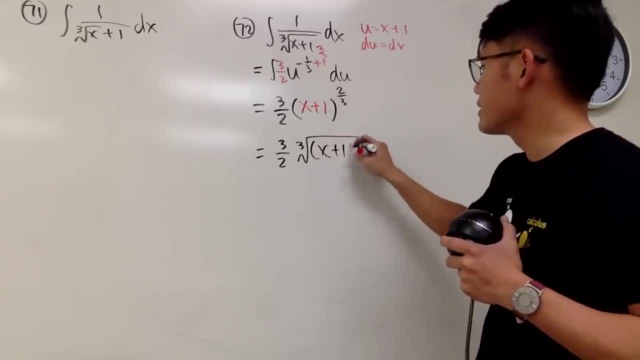 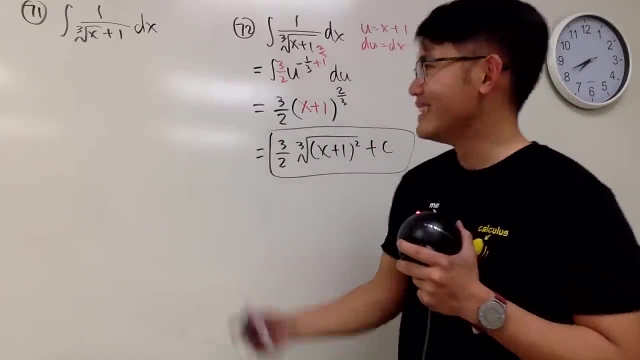 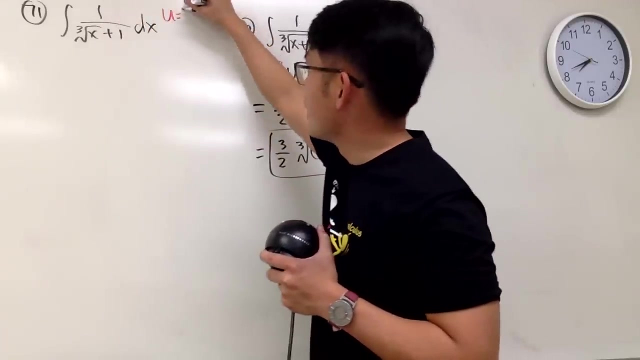 and then this is the cube root of, and put the X plus 1 inside with a square, and then you're done. Very nice, very nice. Now number 71.. Slightly harder, in fact, it's pretty hard. Let's see, take u to be square, no, the cube root of X, and then, along with the, 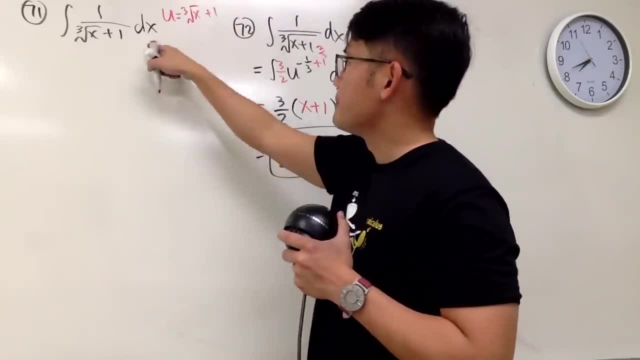 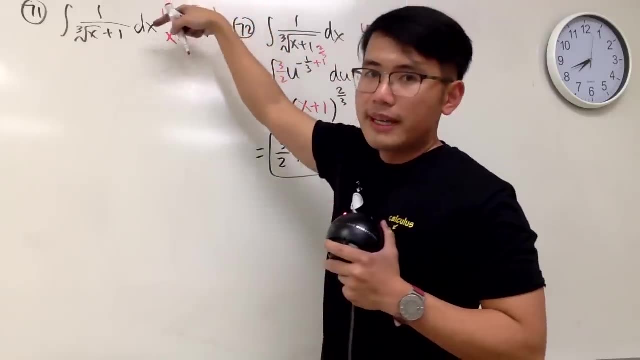 plus 1 constant. I want to get the dx by itself, so in fact let me just get the X by itself first. Let's do this in your head: X is what Minus 1 on both sides, and cube both sides so we get. 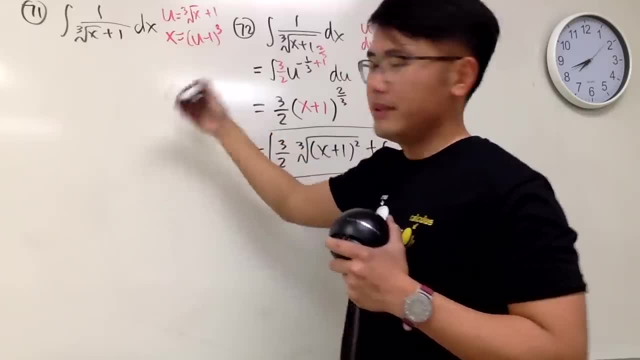 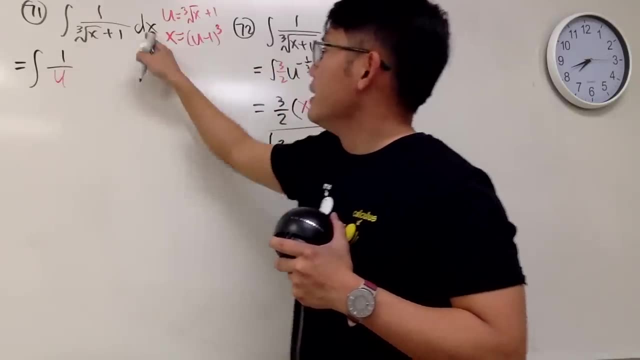 u minus 1 cube and then differentiate this- and I will just put on differentiation right here for you guys, save some time. okay, Integral 1 over this is u dx go. don't forget to differentiate this. you get 3u minus 1 square. 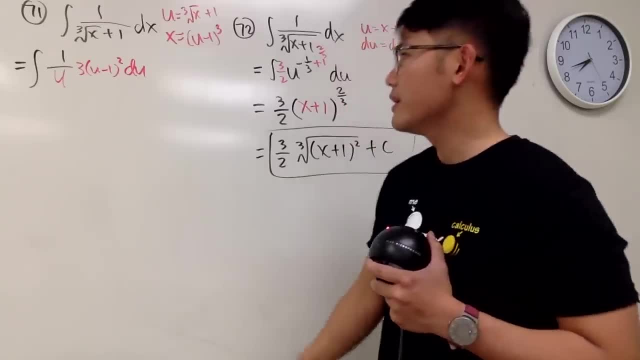 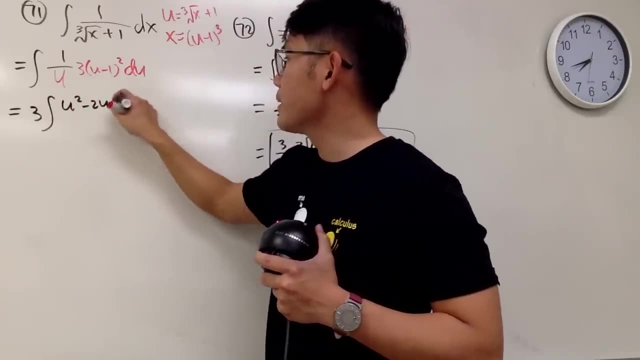 du. that's from here, right. So again, you are going to put the 3 on the outside integral and expand this, which is: u square minus 2u plus 1 over u du. It's longer but it's not. 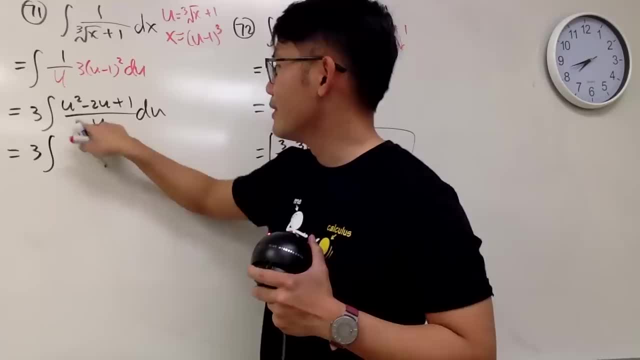 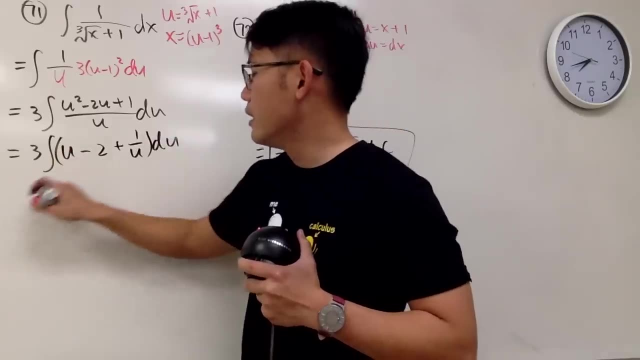 that bad. This is going to be 3 integral divide, divide, divide. so you get u minus 2 plus 1 over u du. All right, this is going to be 3 parentheses and integrate, integrate, integrate. 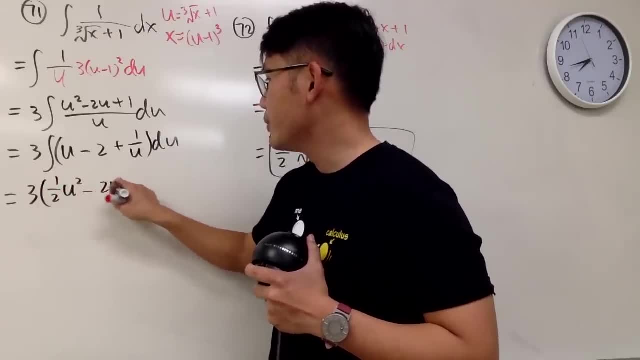 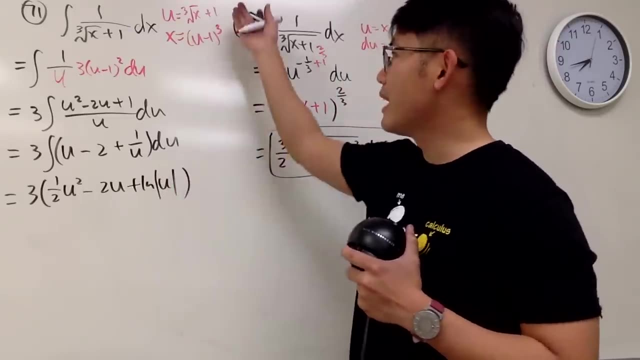 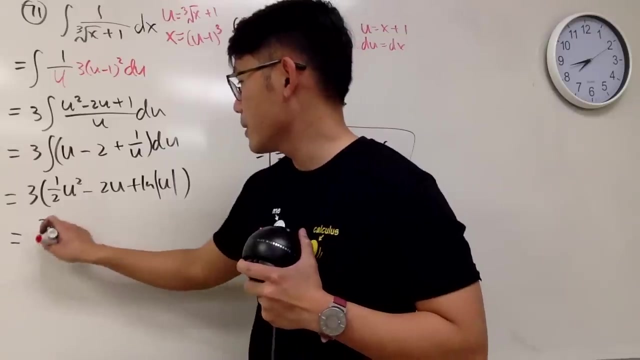 You get 1 half u square minus 2u and then in the end, plus ln u, absolute value. yeah, In the end, put that back. so you have 3 over 2, right, 3 over 2,, of course. and then u. 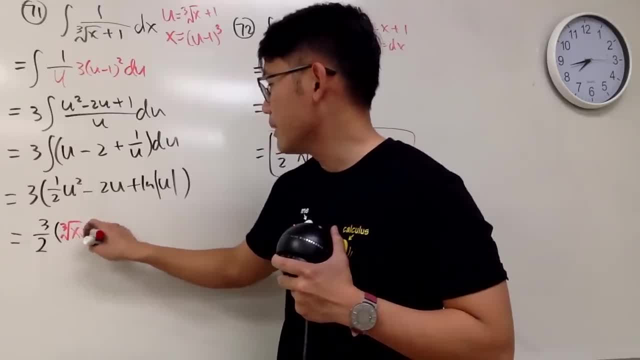 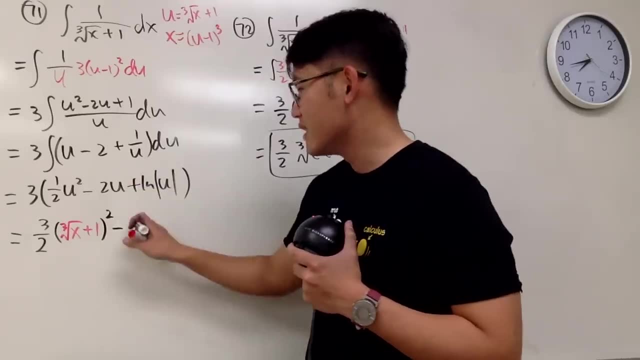 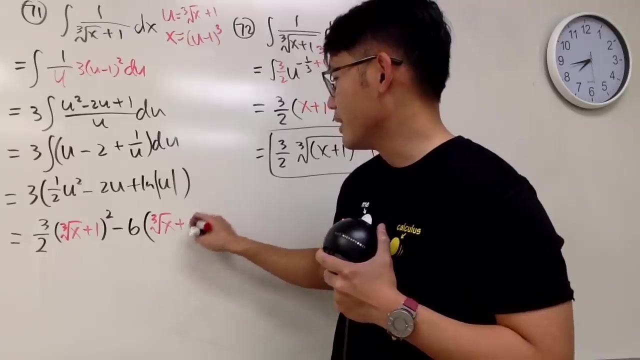 square u is that which is the cube root of X plus 1, and then square that and then minus 2 times 3, 6.. u is that I'm not going to distribute. okay, I'm not going to distribute like this. 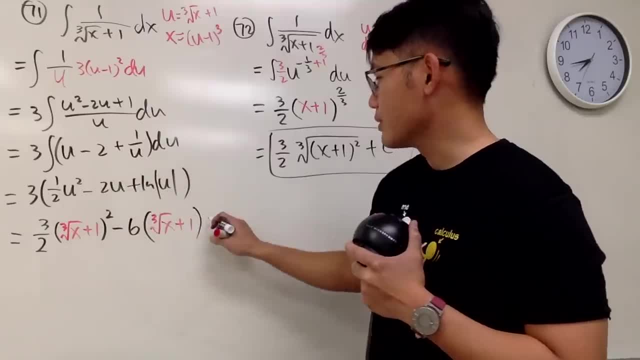 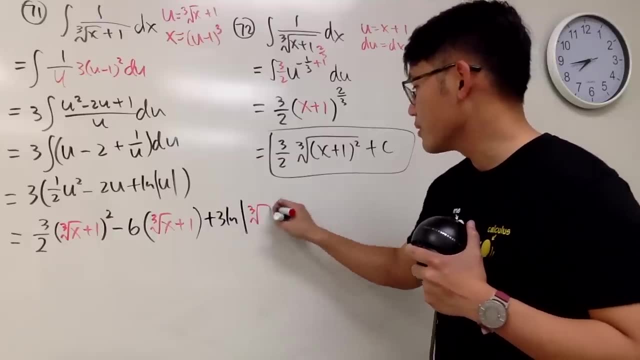 And then you have this guy and then what else? Last is 3 times that, so it's plus 3 natural log absolute value. You need the absolute value because cube root sometimes can be negative, but like you know, we will be study, we won't care that much. That's it Technically. 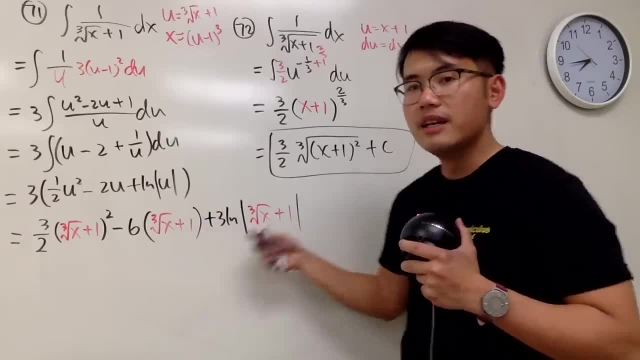 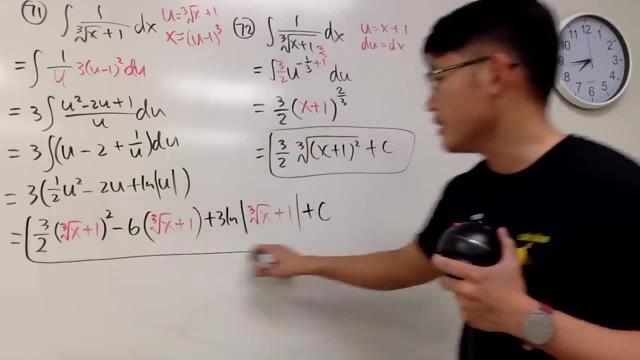 if you would like, you can say negative 6 times 1 is negative 6. But you know that's it And you can just put the constants together and all that. but I would just say: well, I'm not going to distribute anything. This right here is good enough. 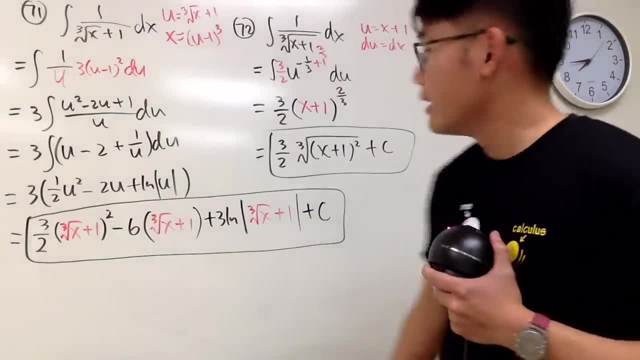 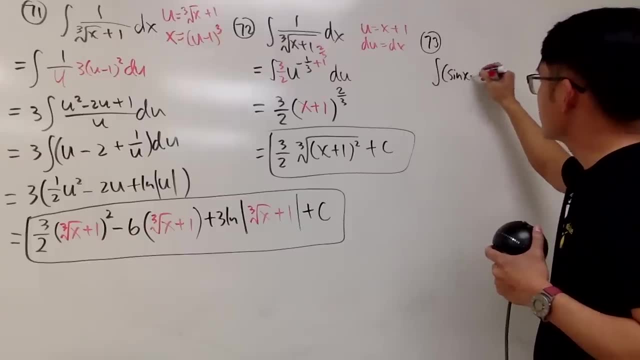 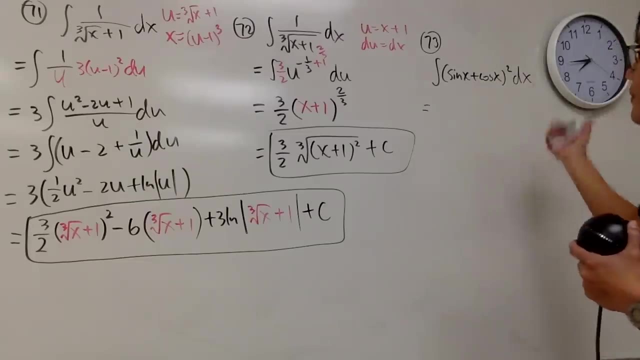 All right, 72.. All right, let's do 73 right here. 73, really classic one: the integral of parentheses of sine X plus cosine X square dx. How do we do this? Well, don't take the u-sub yet. 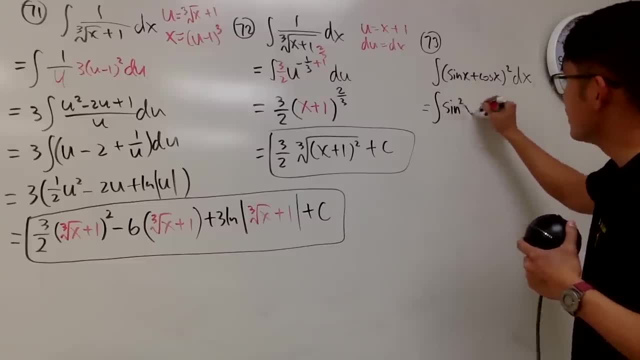 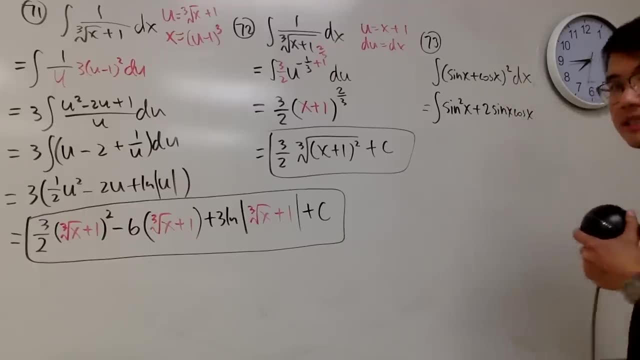 Expand it Not that bad. Integral of the first time, sine square X plus the second time is two. This times W is sine x times cosine x. The last term is cosine square. so we add cosine square X dx Like this, And do you recognize your friends? Yes, Sine square X. 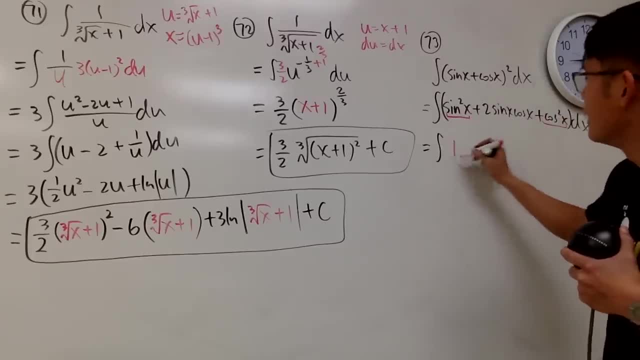 plus cosine square X, this is nicely equal to 1.. And then, do you also recognize this friend? Yes, What's your friend? Do you recognise him? Yeah, So you ask him. Okay, So what's your friend? Yes, Or do you? 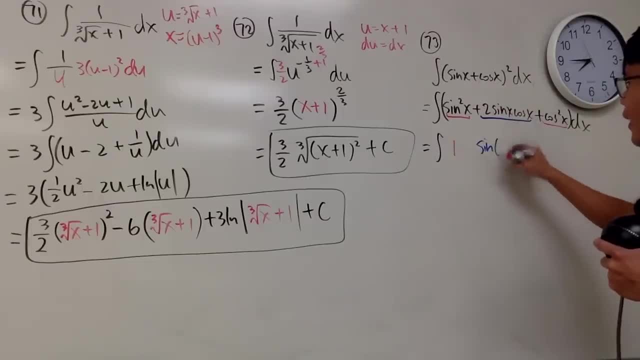 ask for his friend And if that's the case, ask the here. Let's Brian again. What's his friend? This front right here is just sine of 2x the double angle identity backwards. So I will just integrate this guy instead. Very nice. 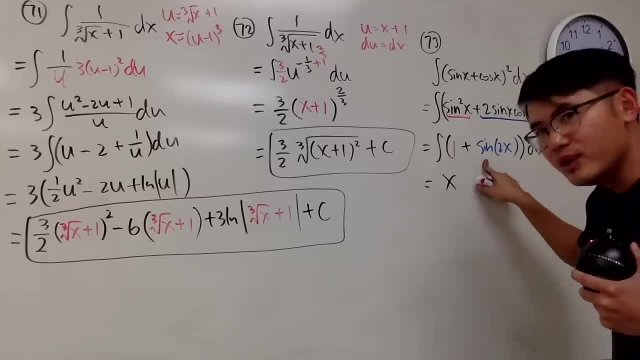 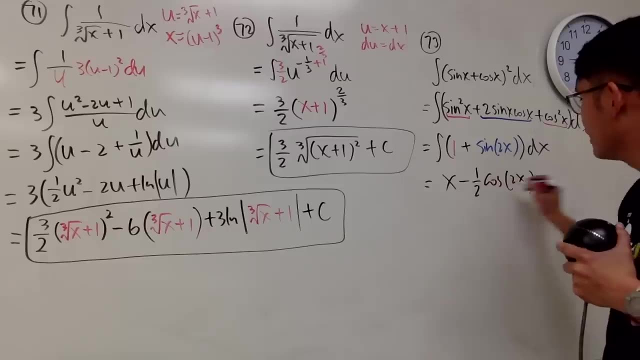 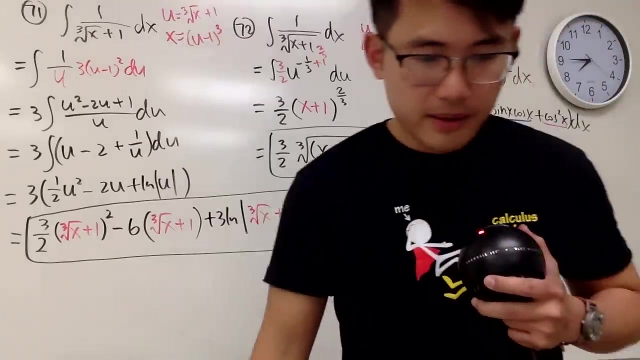 Integrating 1 into x, where it's just x integrating sine, we get negative cosine And the input state is the same and, of course, divided by 2, in the end we're done. Put a plus C. This right here is it. 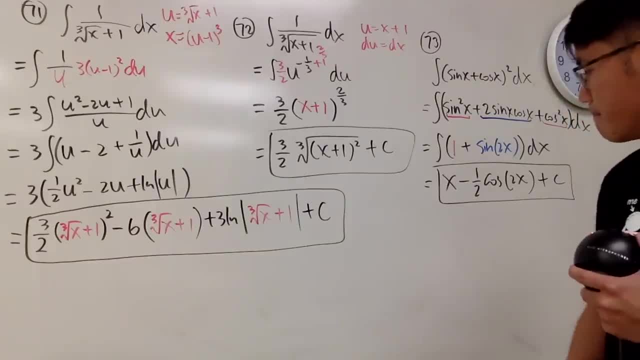 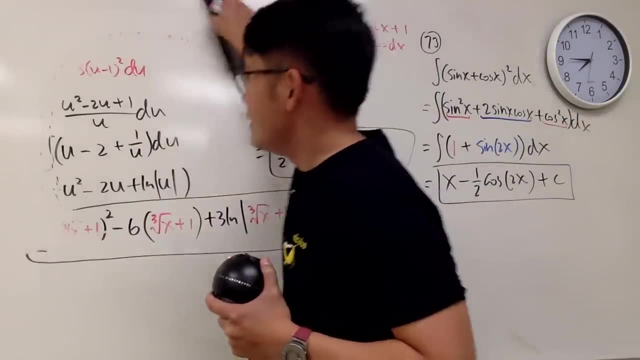 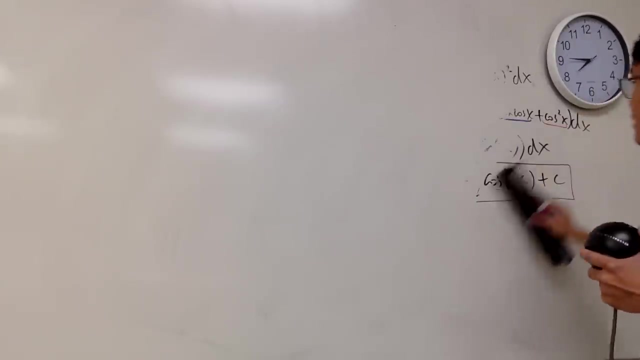 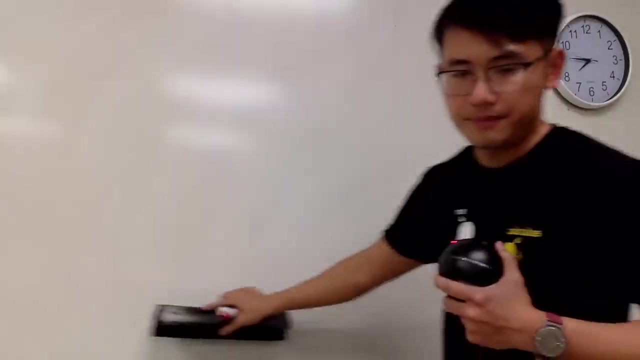 Alright, so that's pretty much I'm debating if I can do the next one right here. I don't think so. Let me just do it like this: Try to see if I can clean the board well enough or not. Alright, 74.. This right here. 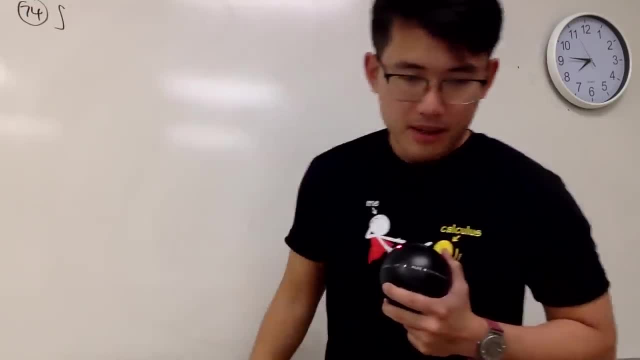 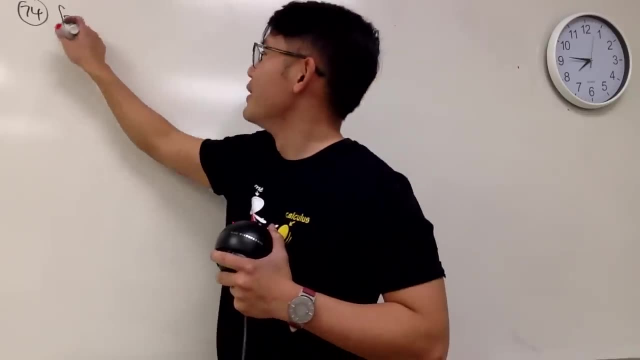 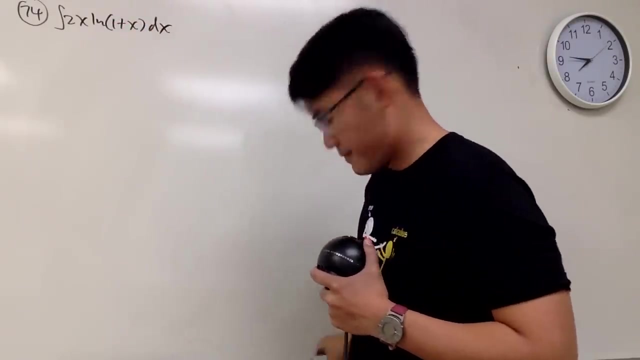 74 will be integrating. I haven't done- I have never done this many integrals in one thing in my life, seriously, 2x times natural log of 1 plus x dx like this. Alright, integration by parts. So let me put this down right here for you guys. 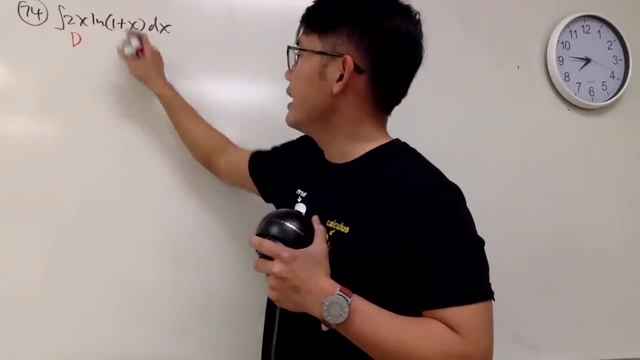 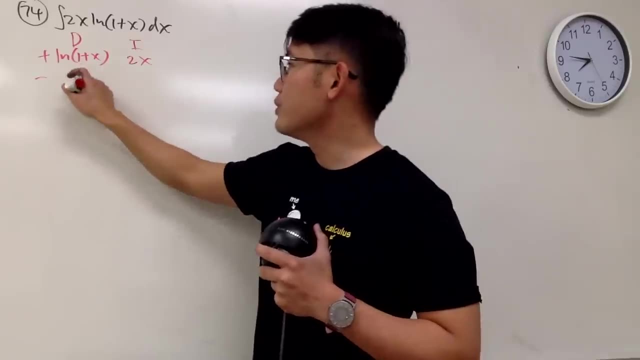 d, and then i Let me integrate 2x and I will differentiate ln of 1 plus x, And don't forget the plus minus on the side. to get ready, Go ahead and do this. You get 1 over 1 plus x. 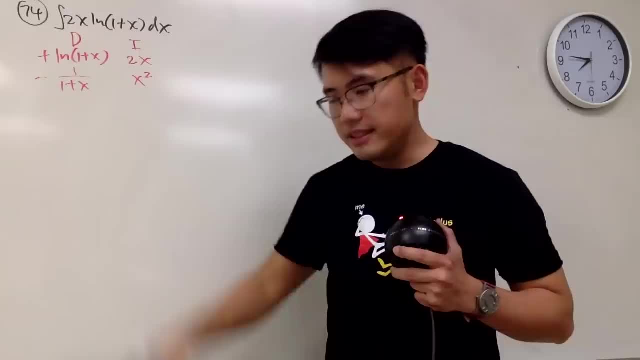 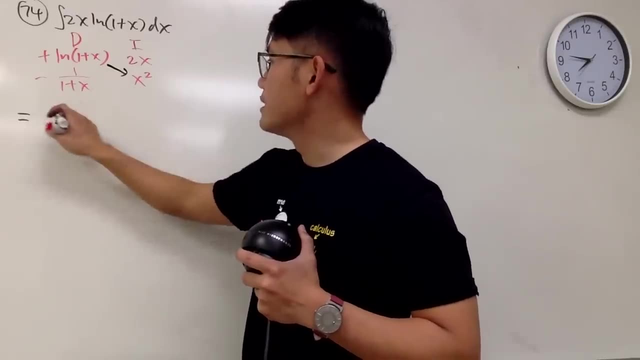 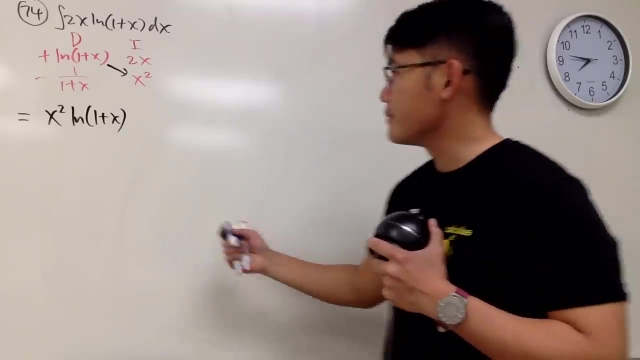 Integrate this, You get nice, It's nice to equal to x squared And then go ahead, do this times this, So you will have the first part of the answer being x squared times natural log of 1 plus x. And then, well, we have to do this integral. 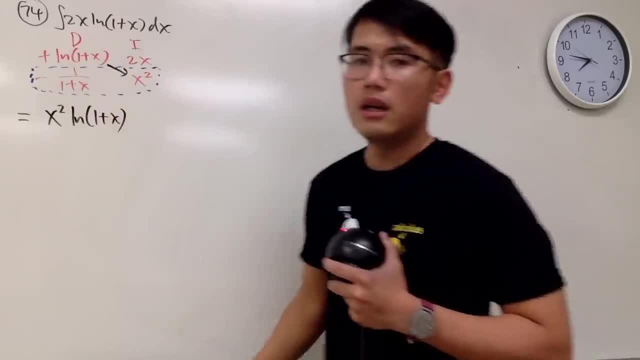 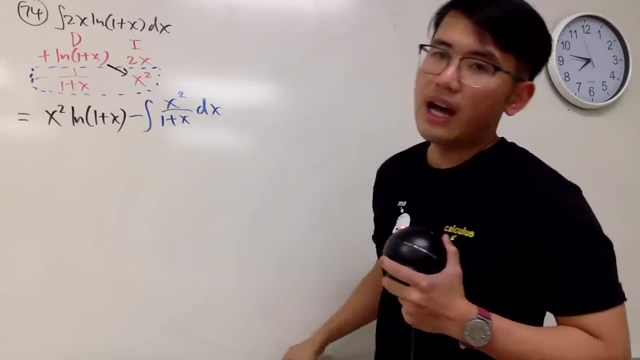 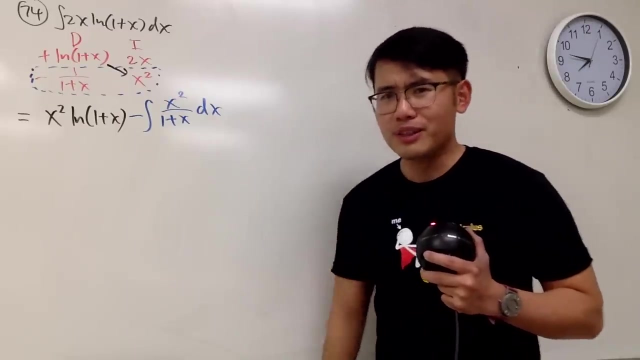 Alright, this is the integral that we have to do, Minus the integral x squared over 1, plus x dx. Now you have two choices: One: you can do USAP or you can do long division. Perhaps long division would be better, so let's do long division, but they are pretty much the same anyway. 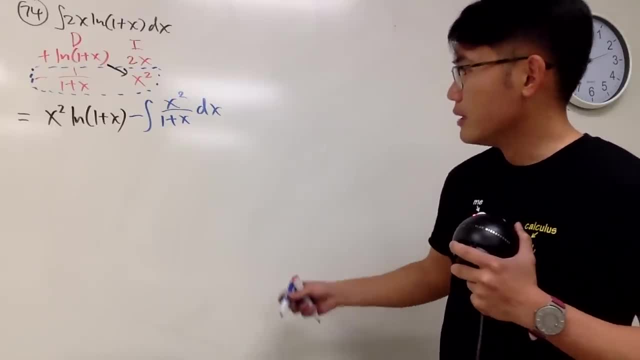 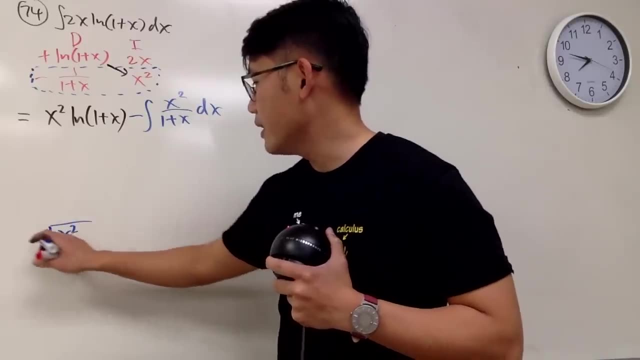 When you do long division, this is what you do, Alright, so I will put this down right here. Let me just do it: Put the top right here and then put the bottom in this order: x plus 1, like this: 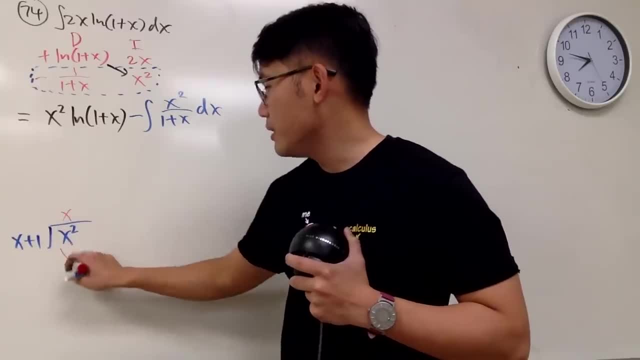 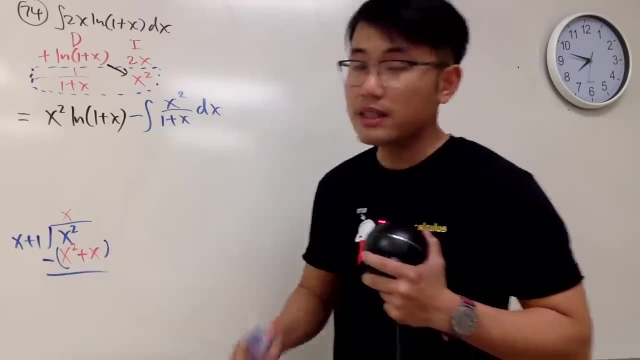 What do we need? We need x. x times x will give me x. squared x times 1 will give me plus x. And you don't forget to subtract. When you subtract this, this minus that is 0.. 0 minus this is negative x. 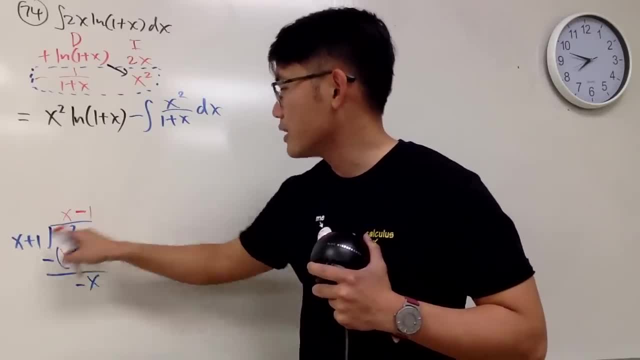 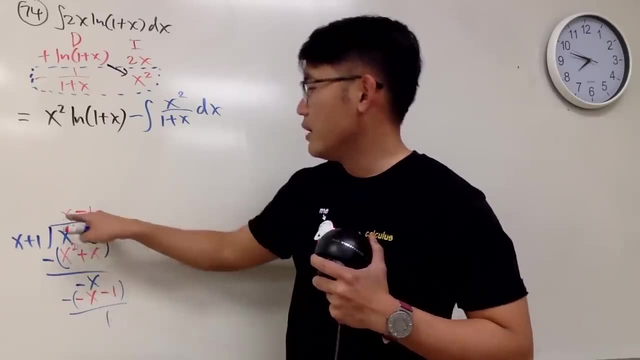 And in fact we can do it again, because we can put down minus 1.. Minus 1, times that is negative x, And then times that is minus 1.. Subtract: we get 1.. On the top the water doesn't really matter. 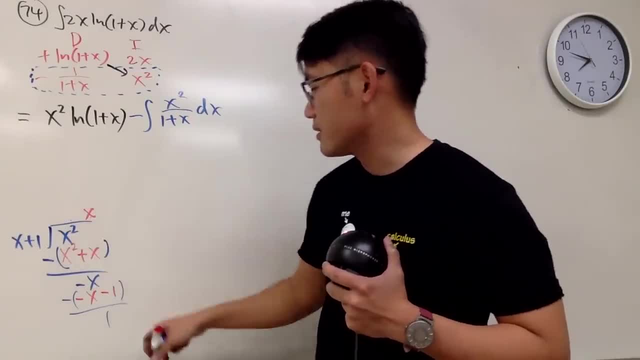 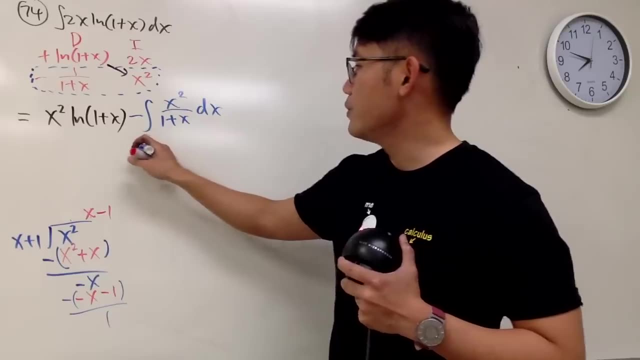 Technically, you should have lined up all the x together like this, though, but it doesn't really matter, And then earlier I needed a negative 1, like that. So if you focus on this part, this is going to give you negative integral. 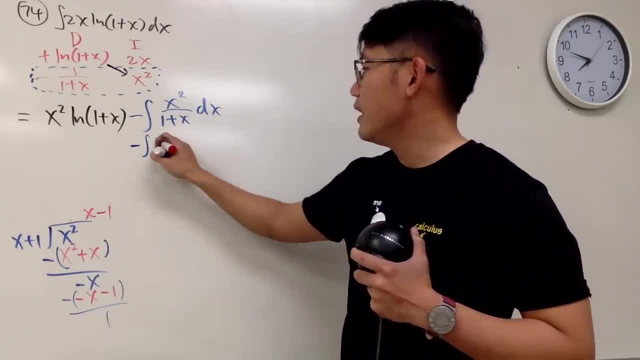 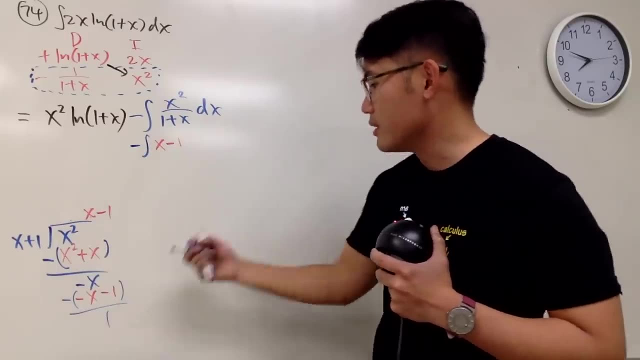 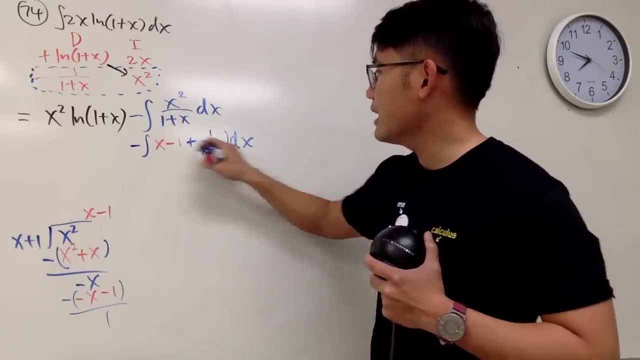 All this together says you have to have x minus 1.. Okay, that's the whole part, And then the remainder is the plus 1 over x plus 1 dx, like that. So up to you, whichever way you want to do it. 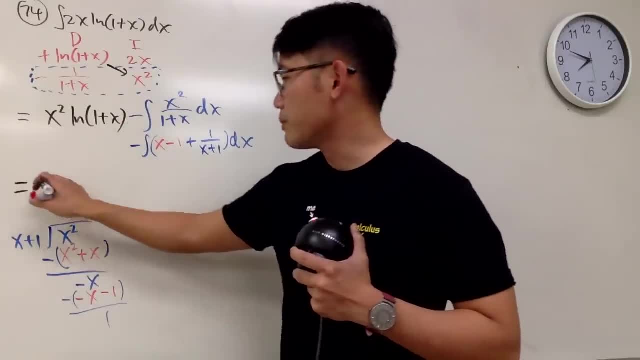 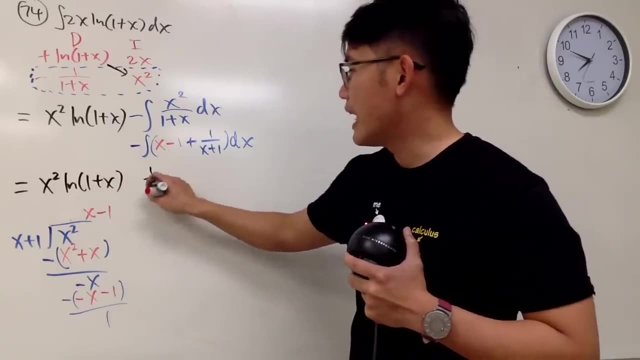 Now we'll see This right. here is the answer, the first part of the answer already, so keep it. Do two things in your head. Integrating this, you get 1 half x squared, but don't forget to distribute. 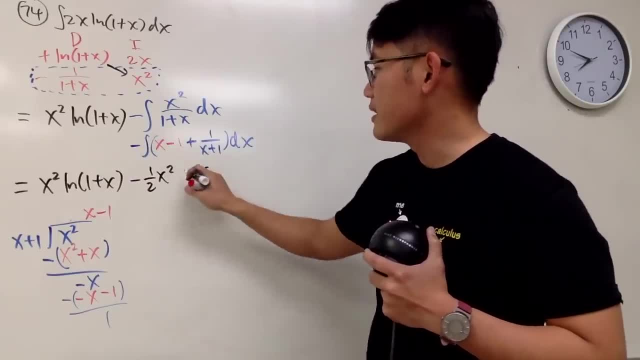 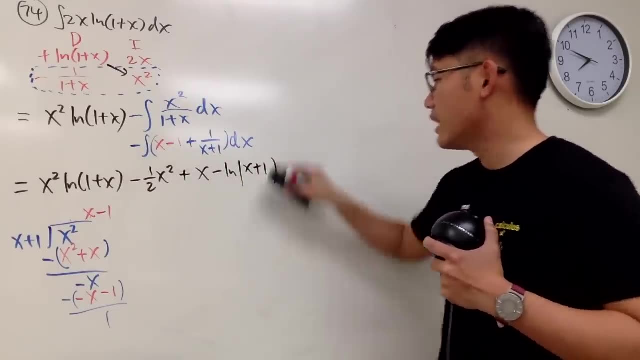 You get minus. Next, integrating this, you get x. But negative times negative is negative, But negative times negative is positive. Lastly, this times that is minus Natural log, absolute value of x plus 1, like that. Okay, And technically let me tell you you don't need absolute value. 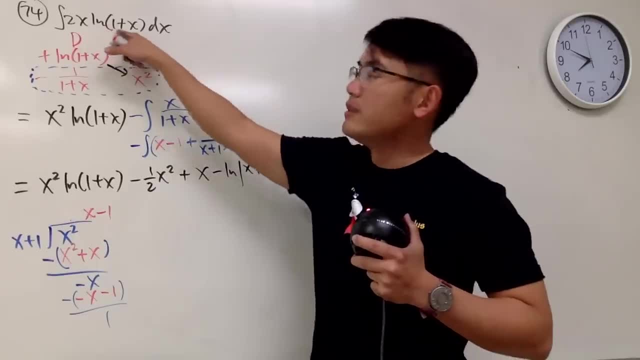 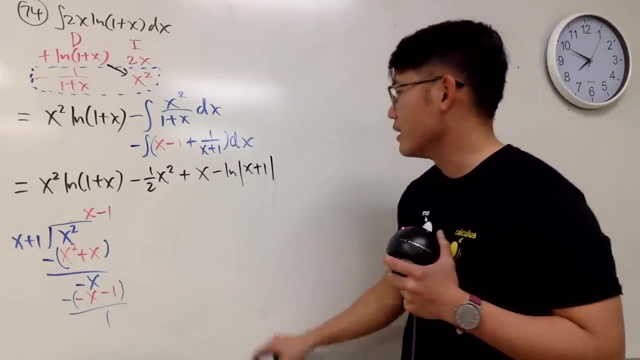 Can you get my point? Because originally, if you put this down already, you are preventing x being less than or equal to negative 1.. So you don't have to worry about that. So technically you could just put parentheses. 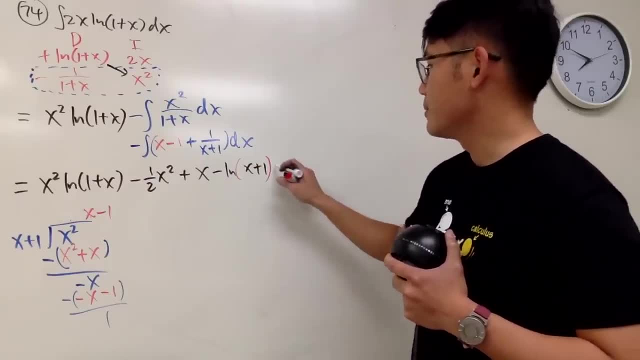 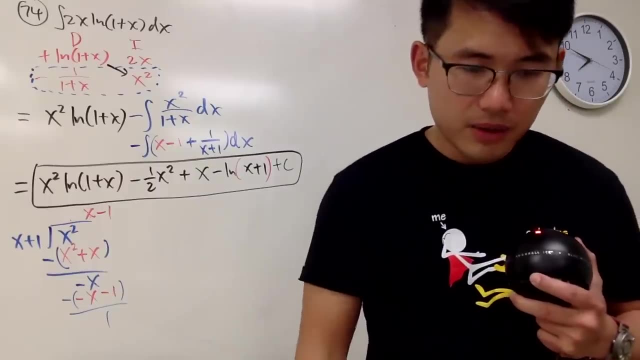 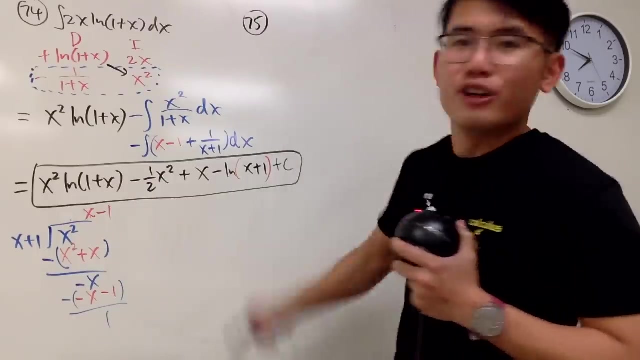 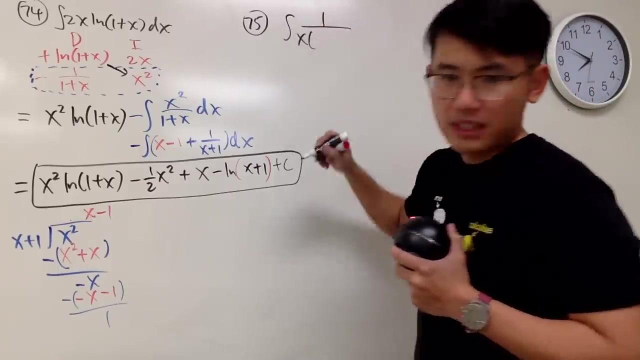 But seriously, I'm not going to care too much. right here, All right, And I'll put a plus here, like that, All right. Now let's see Number 75.. 75%, done, you guys. Integral of 1 over x times 1 plus sine squared of ln x. 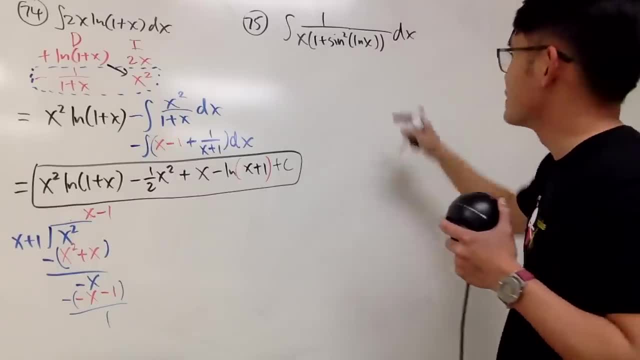 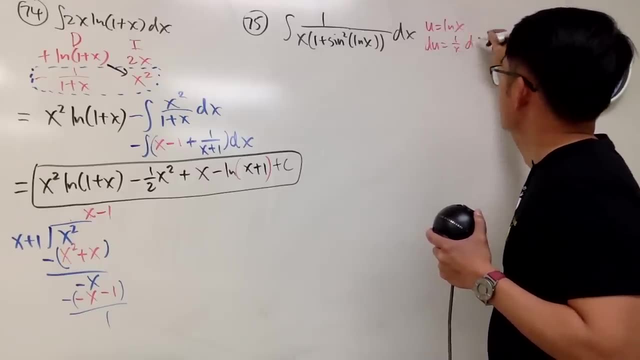 Like this. You stop Get rid of something right. Get rid of the ln, So u equal ln x, And then you will see du will be 1 over x dx. So if you pair this and that up, you get your du. 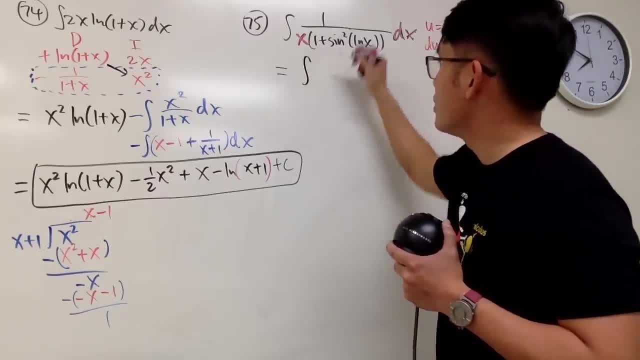 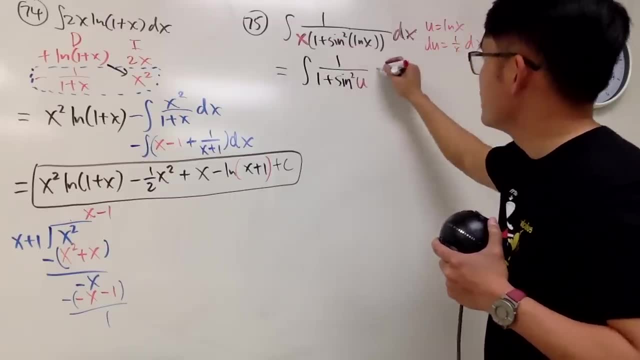 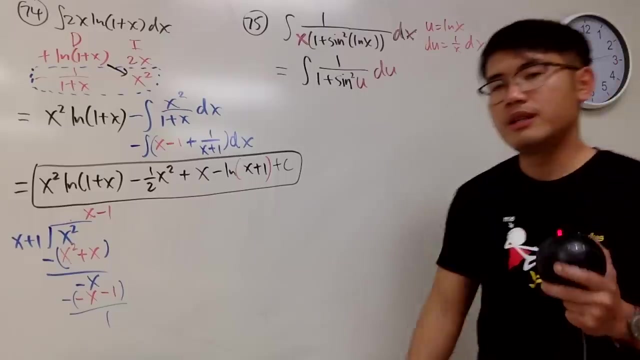 Okay, So, with that said, you are looking at the integral of 1 over 1 plus sine squared u, And then again this and that together will give you the du. So that's good, But now I have some trouble because I don't know a good alternative for 1 plus sine squared u. 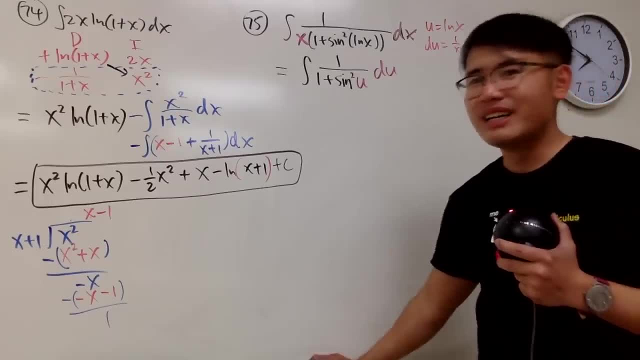 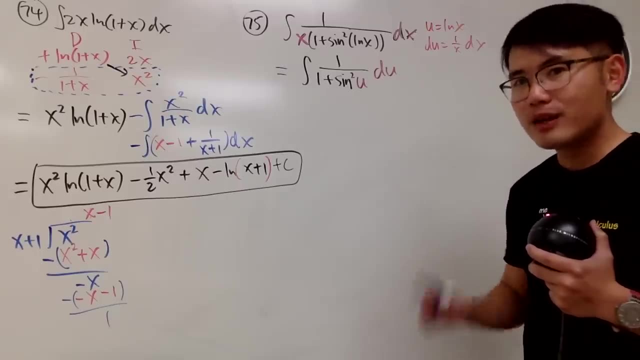 I need to have the cosine to help me out. So how can I do it? You can try to multiply cosine if you like, But I will choose to divide everybody by cosine squared, Because I know sine divided by cosine will give me tangent. 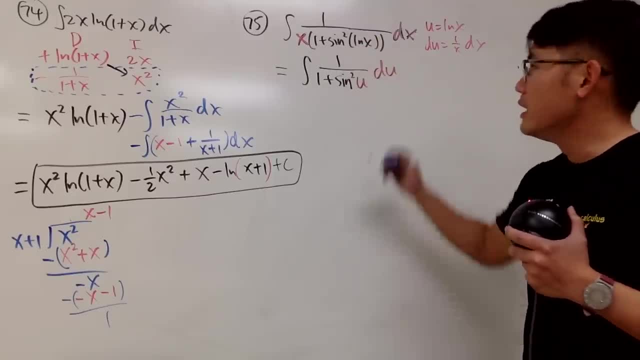 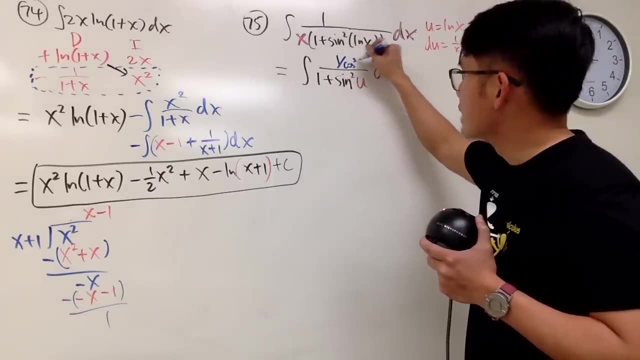 And when I divide it by cosine I will get secant. And since this is with sine squared, let me just divide everybody by cosine squared Right. Divide everybody by cosine squared Technically u Okay, Cosine squared u. 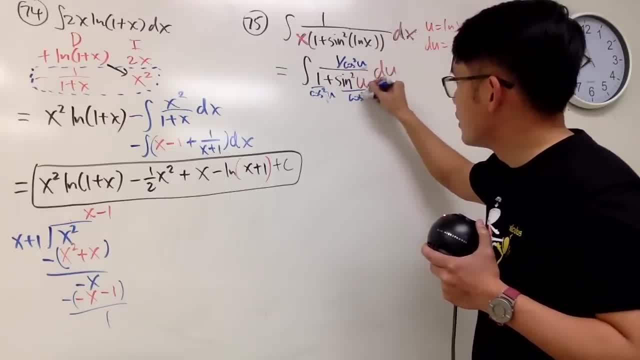 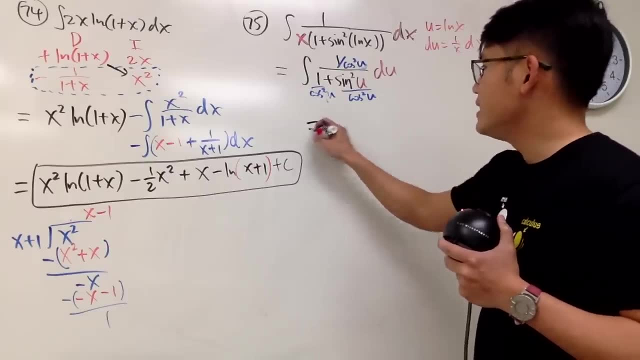 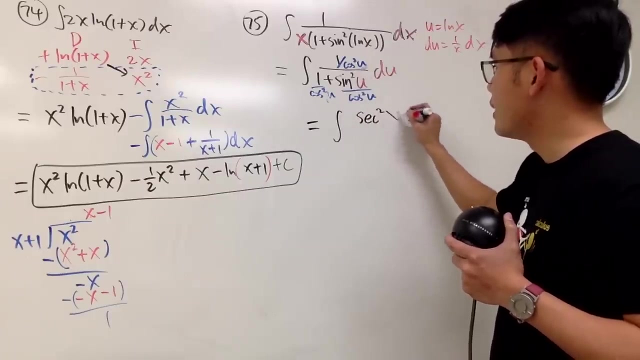 Divide everybody by cosine, squared u Right, Like that, And hope for the best. It will be the best. Let's see what we get On the top now. we will get 1 over cosine, 1 over cosine which is secant, squared x over. 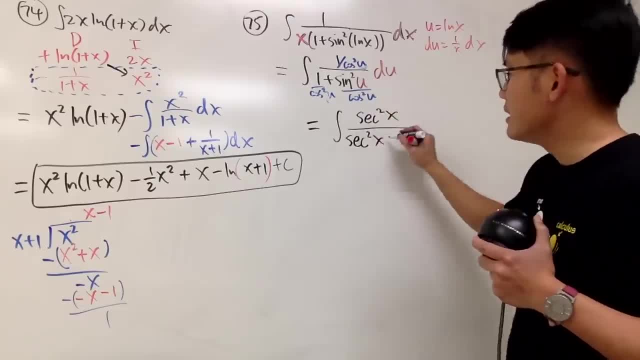 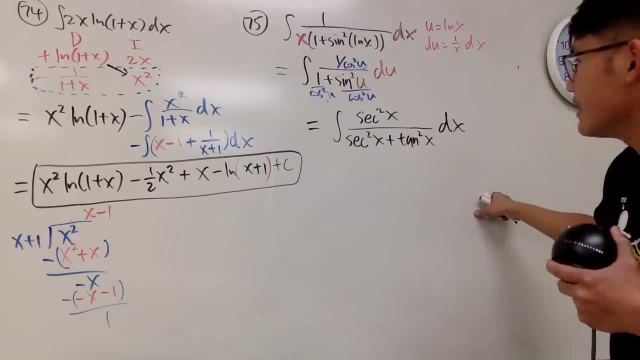 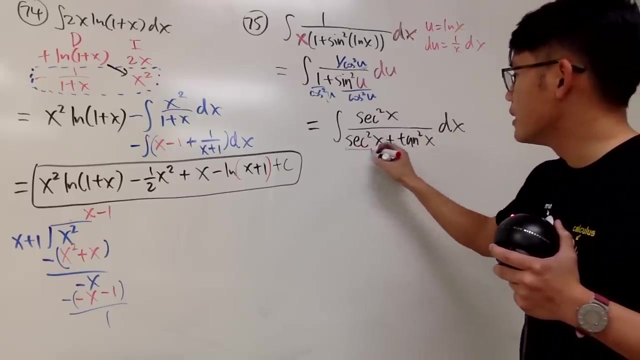 This right here is also secant squared x, And this is tangent squared x, Isn't it? That's very nice, And again, the goal is to somehow- you know, maybe- put this on the side to help me out, And to do so, let's look at this secant squared. 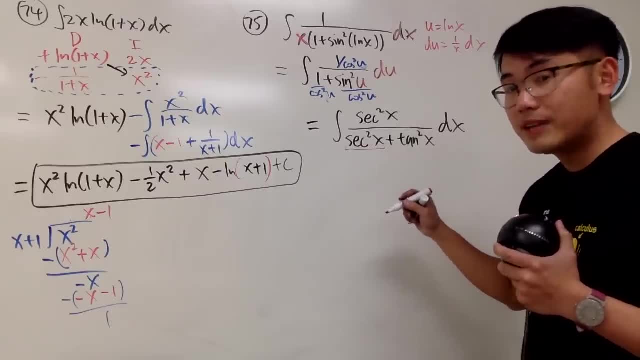 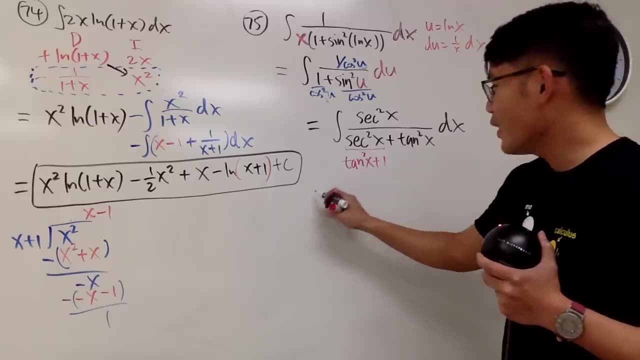 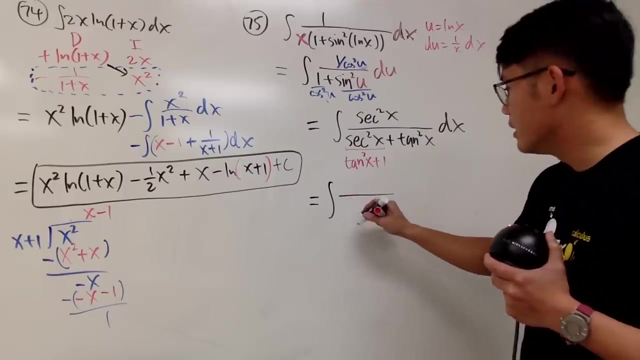 We know secant squared is the same as tangent Square x plus 1.. Isn't it So? as you can see, we have the integral On the bottom, we have this plus that. So I'll write it down as this for you guys. 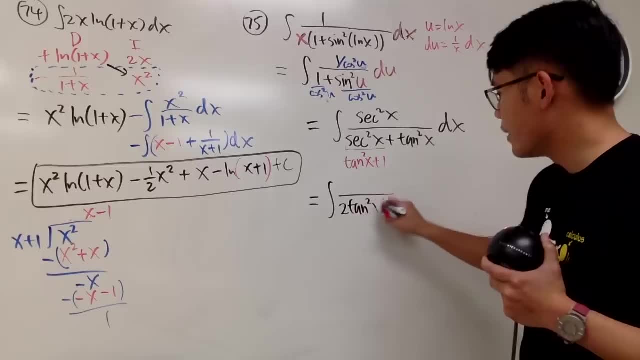 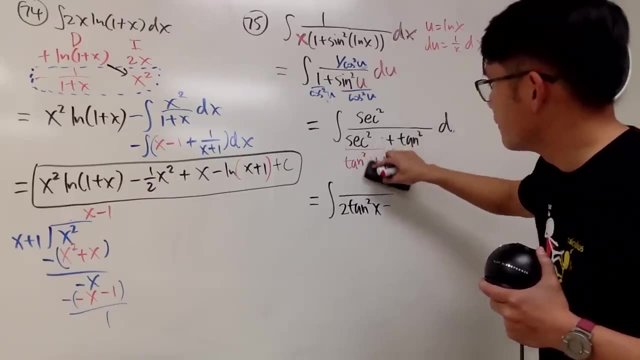 2 tangent squared x. Sorry U, I'm in the? U world. I'm sorry, Everybody should be in U. Okay, In fact I wanted to just show you guys this question, But I wanted to make it slightly more complicated. 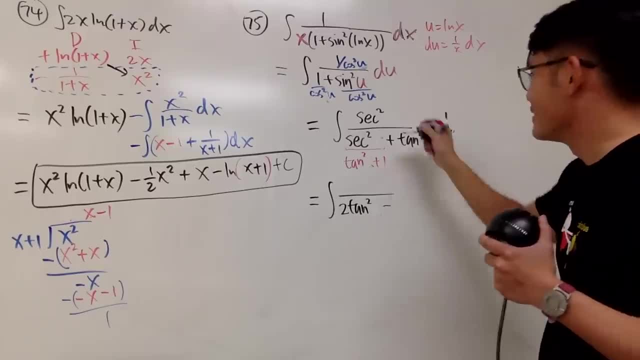 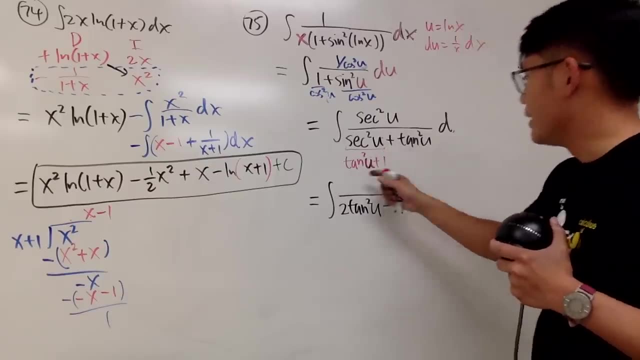 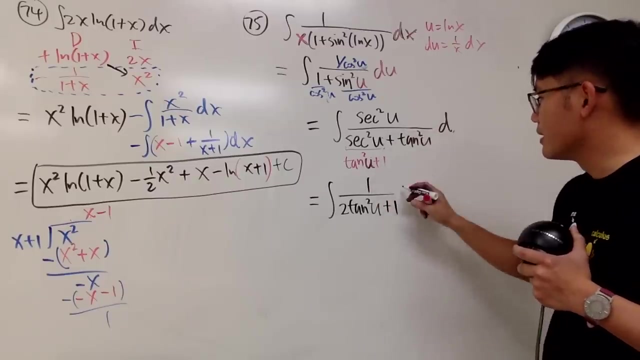 So I did this substitution. So, yeah, Anyway, U U, U, U U, Okay, U Anyway. So this plus that is 2 tangent squared U And you have the plus 1.. And let me just put a secant squared U on the top. 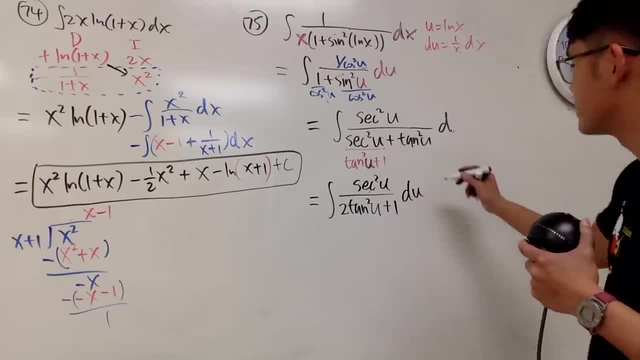 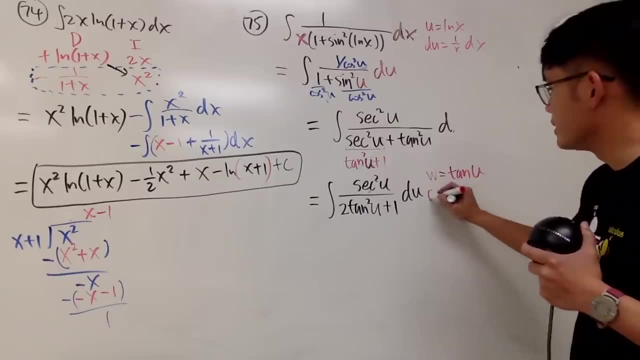 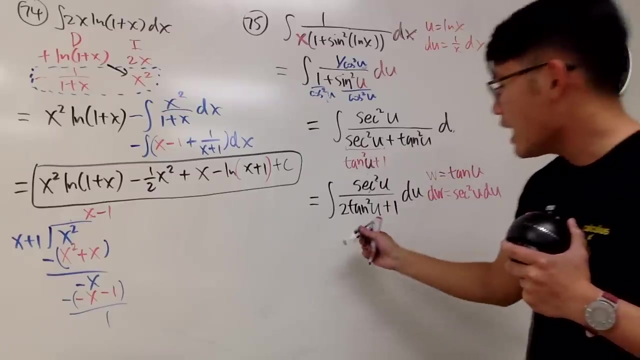 The U. And here I will take another substitution. I will take W to be tangent of U And you will see the W will be secant, squared U the U, Which is exactly what we have on the top. Now we take this to the W world. 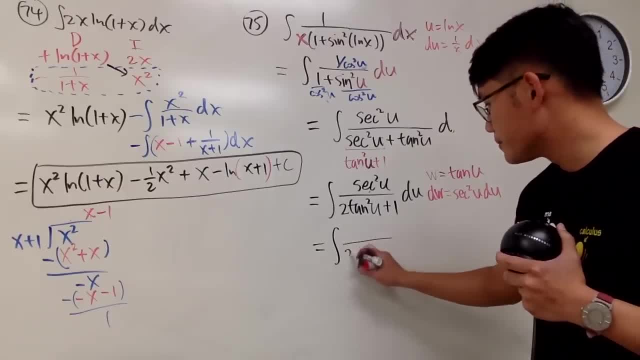 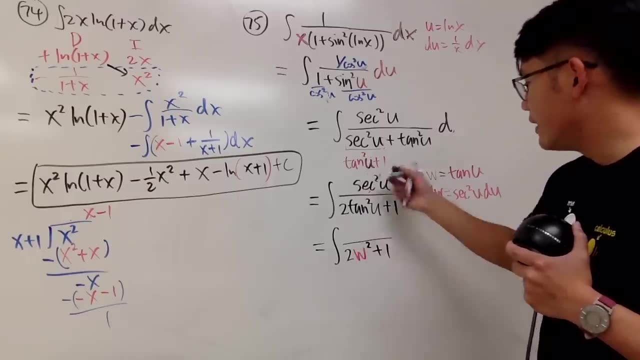 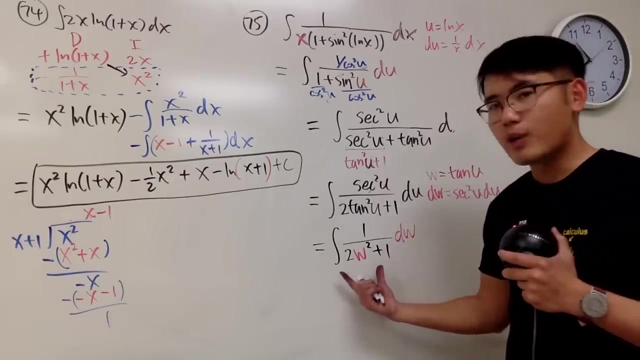 We will get integral of 2. And this is going to give me W squared, And then plus 1. And then all in all on the top will give me the W. Hey, this is almost like inverse tangent, but not quite. 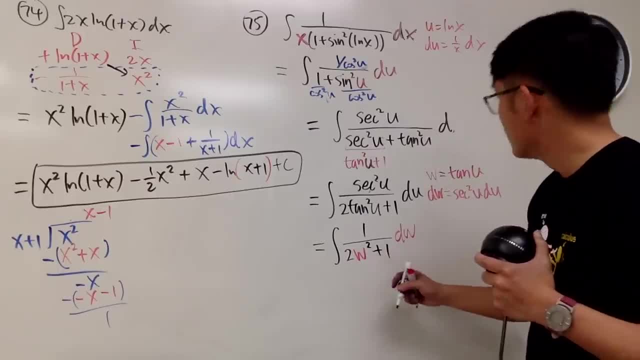 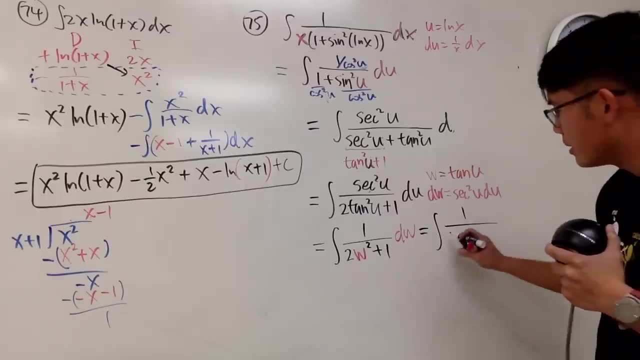 You have to put this down in a nice way. Let's see I should write it down here. Say some space Integral 1 over this, right here, Put parentheses. Fill in the parentheses with square root of 2.. And then W. 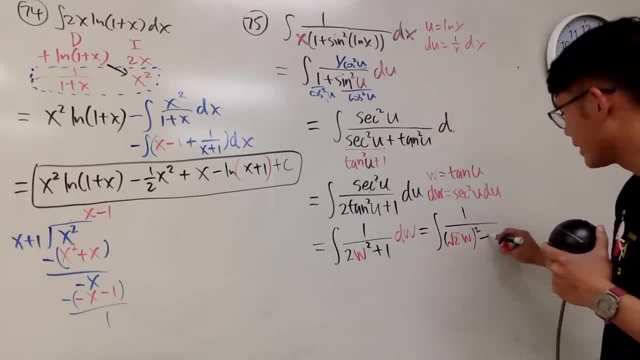 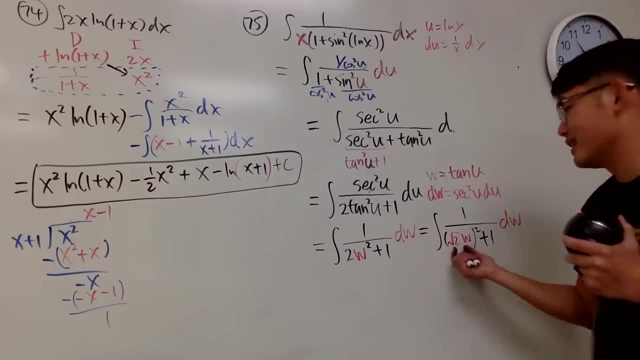 Like this, And then square, And then plus 1. And then the W. Technically you have to do another substitution, That's whatever U, V, W, And then you can use like Y or X or T or whatever you want. 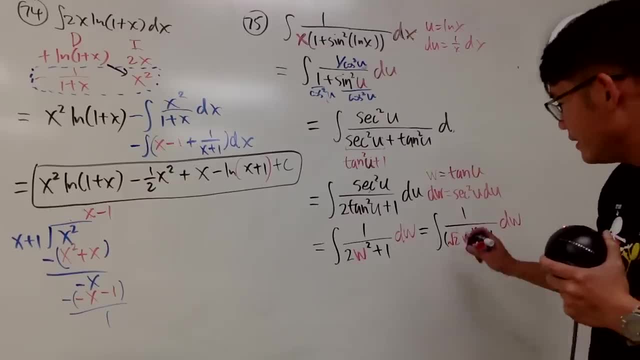 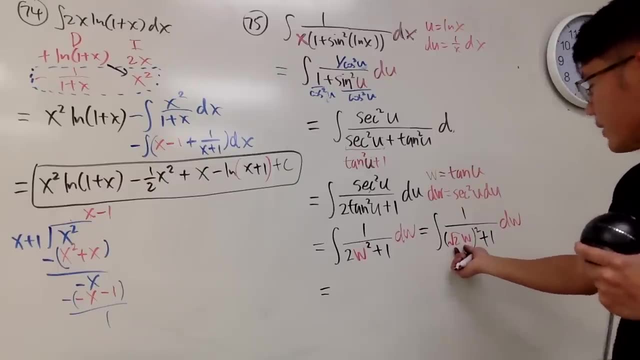 Do this, But let's just do this in our head. yeah, In the W world, this is what we are going to get. If you let T, okay, let's use T- You get. you have to divide, Just divide. 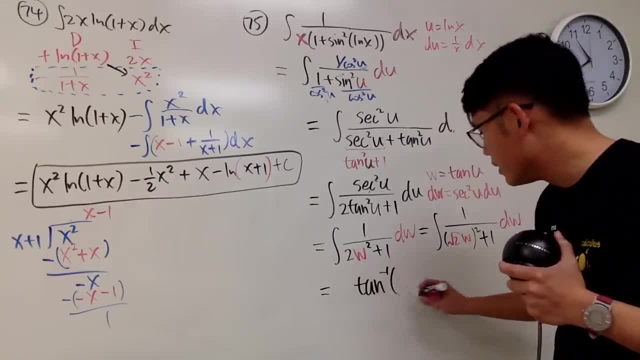 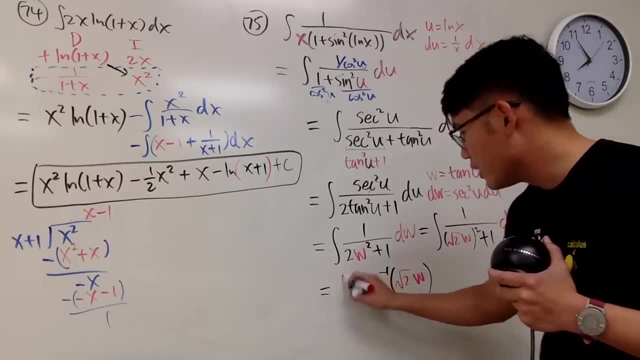 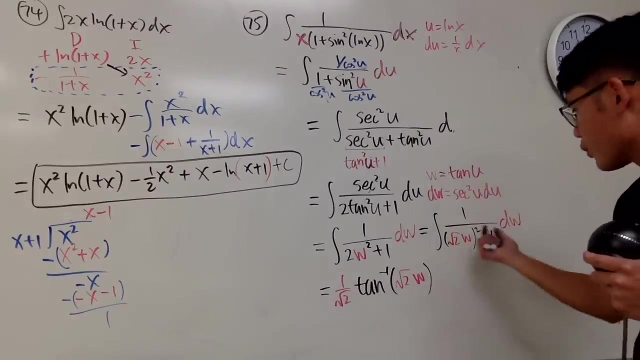 The big picture is you end up with the inverse tangent of square root of 2, W, But divided by the derivative of the input, which is, you divide it by square root of 2.. Like this, Check this out: When you differentiate this, you put this as 1 over this thing squared plus 1.. 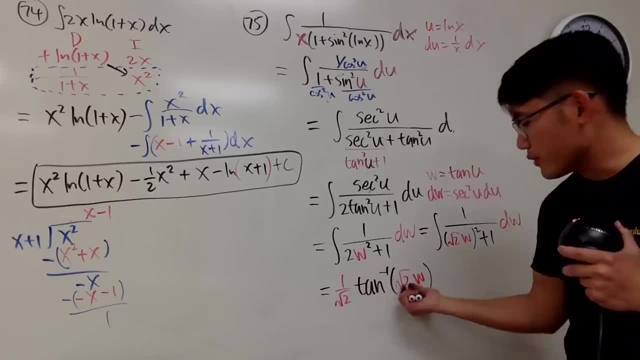 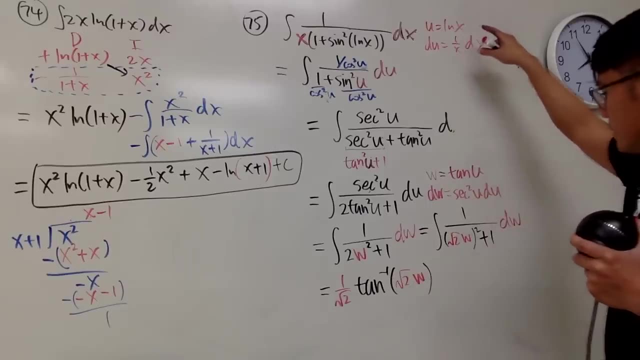 And then you have to multiply by this by square root of 2.. And 1 over square root of 2 cancels. That's good. So that's the idea. Well, U is W is tangent U, And then U is natural log of X. 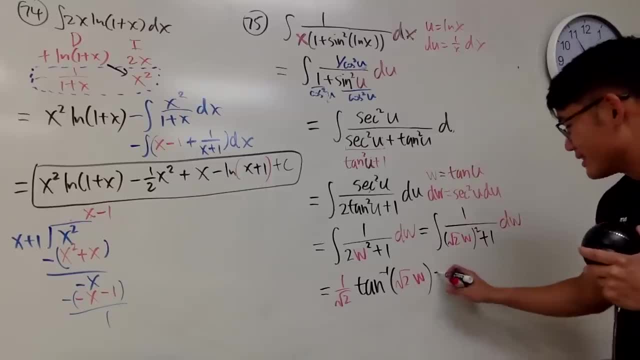 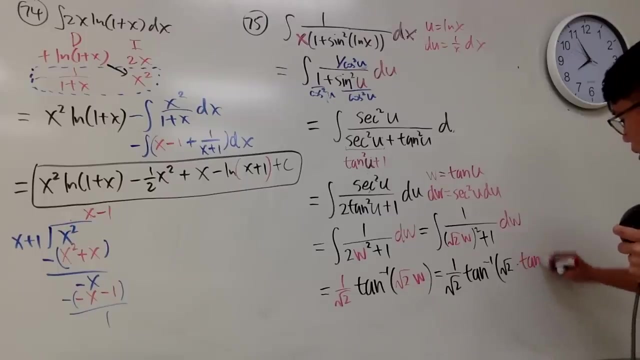 Okay. So now things are getting serious. Finally, we go back to the W, we go back to the X world right away, okay, So inverse tangent square root of 2 times W is tangent of U, But U is natural log of X, right there. 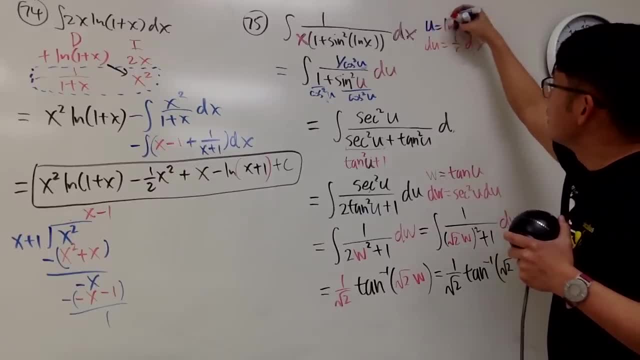 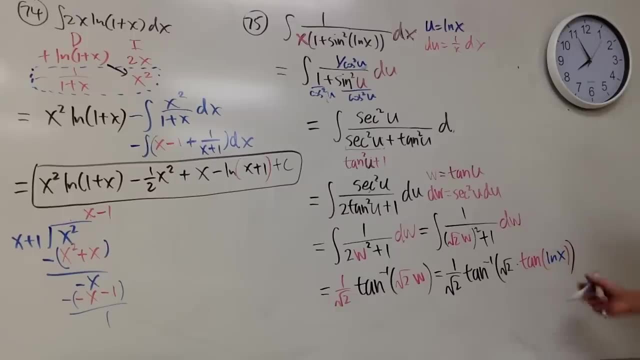 Where is it? U is natural log of X, So I put down natural log of X. Okay, So I put down natural log of X, like this. So this right here could have been a crazy chain loop question, you know, But yeah. 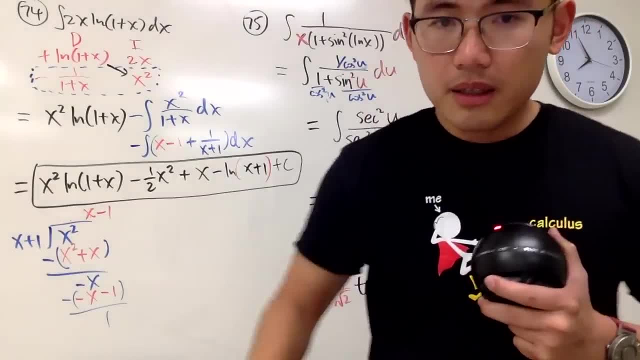 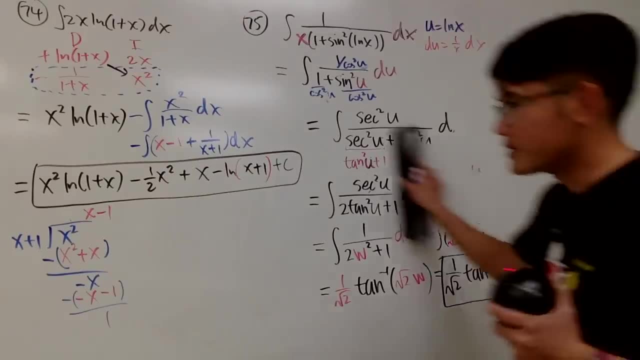 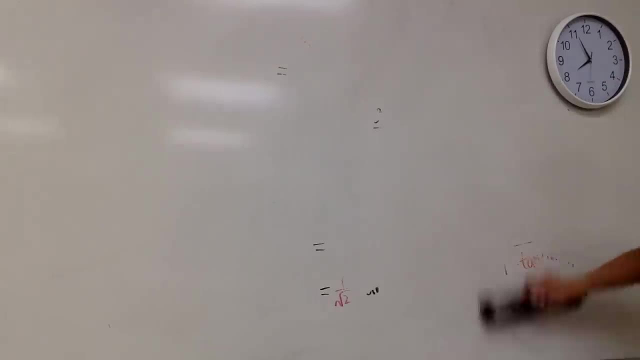 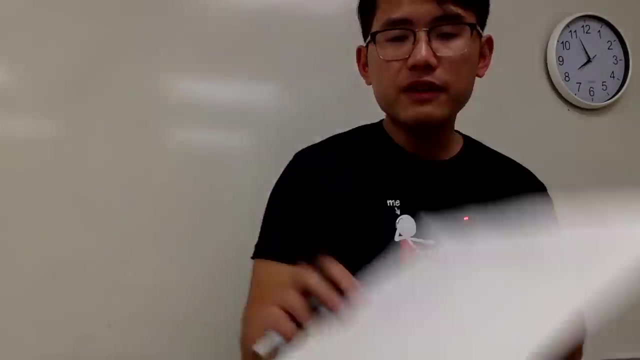 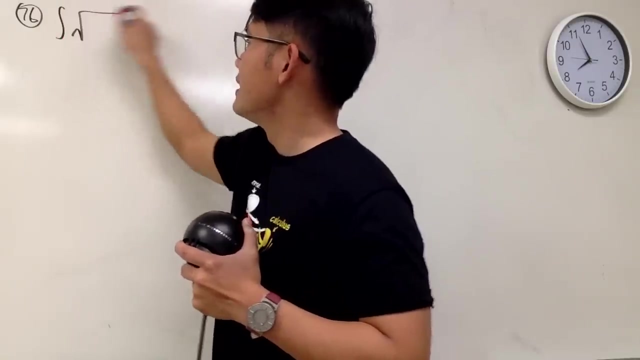 Good, right, Good Now, number 76,. okay, So I will erase all this Number 76, I have a big square root for you guys, Not that big, but you know whatever. 76. Like I said, don't be a 76ers. 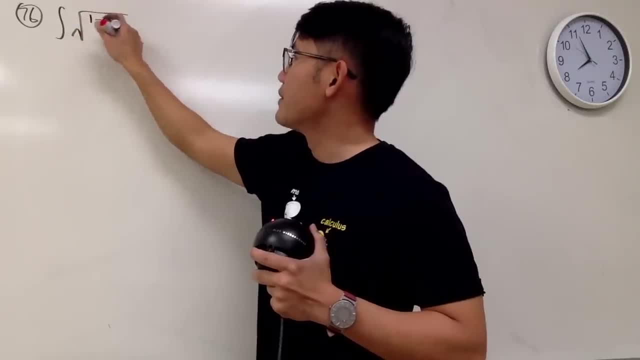 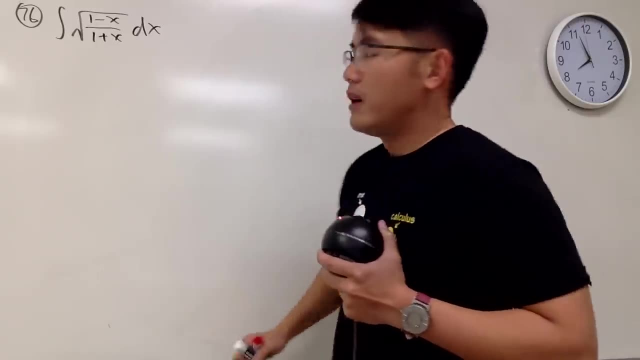 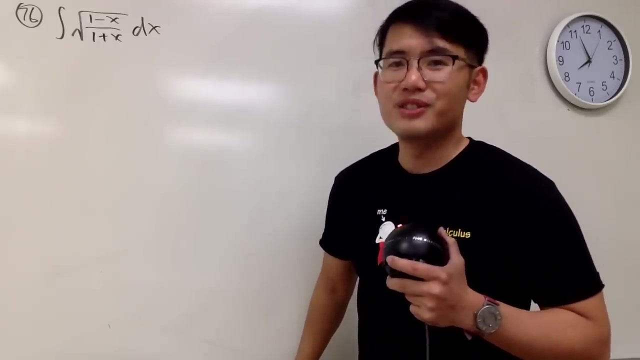 76ers back in the days. I like to watch Allen Iverson playing basketball. all that stuff Nowadays JLMB. right, All right. It's tough. What can we do? Conjugate: Give it a try, But not quite. 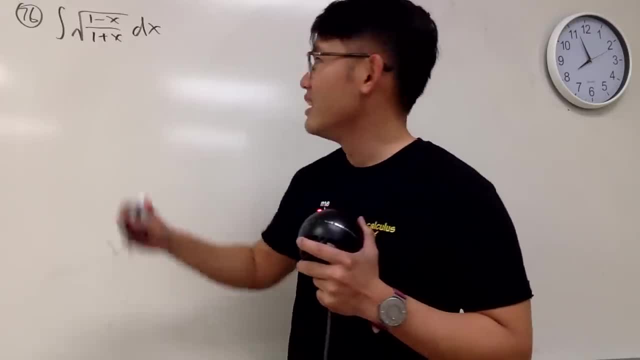 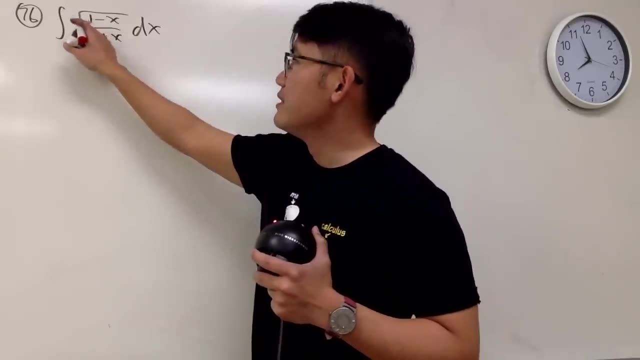 Just have one turn technically right, But inside because I want to get rid of the square root. I want to get rid of the square root on the top. Let me show you how Technically this is the square root of 1 minus X over square root of 1 plus X. 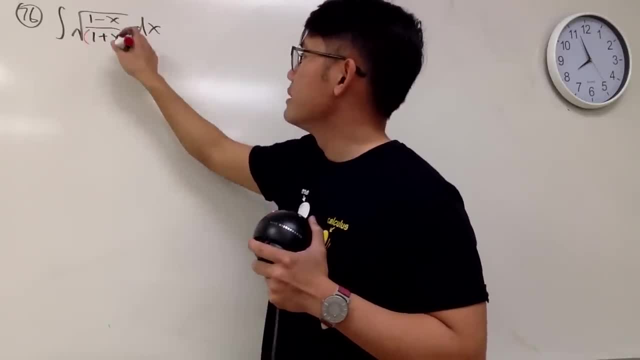 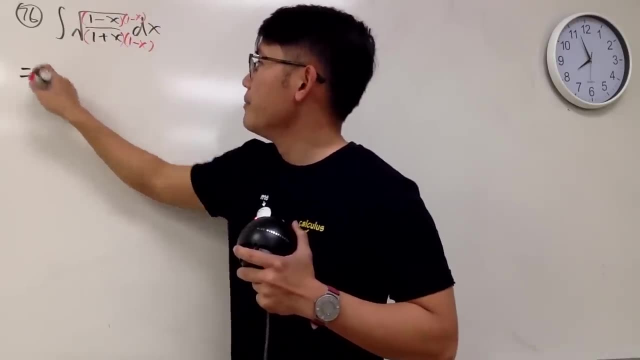 But let me multiply the top and bottom by, inside-wise, just the 1 minus X. Okay, 1 minus X, Like that. Why? Because you will see on the top, 1 minus X times 1 minus X, 1 minus X squared. 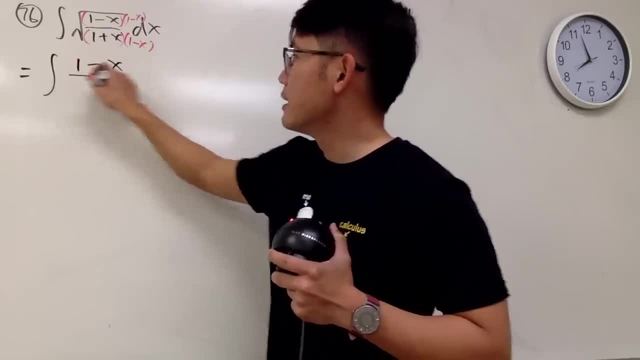 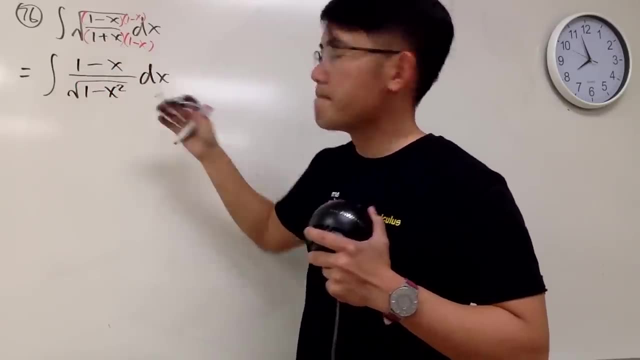 In the square root. you just get a nice 1 minus X On the bottom. you have square root of this times, that which is square root of 1 minus X, squared Like this. Very nice, This time when you look at this, you can split the fraction. 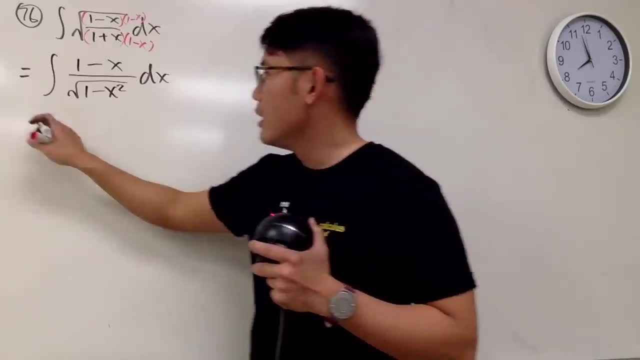 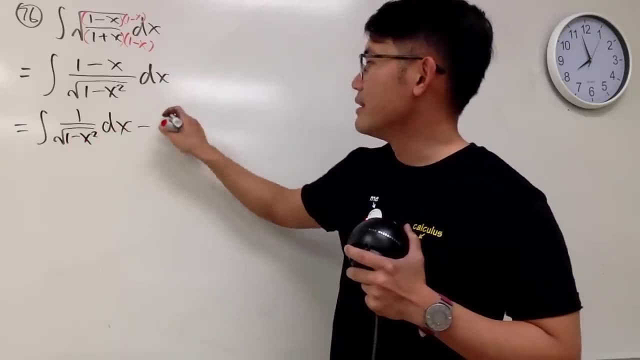 This is the beauty of one turn in the denominator. So you have the inverse. So you have the integral of 1 over square root of 1 minus X squared. Close that. And then you minus the integral of X over square root of 1 minus X squared. 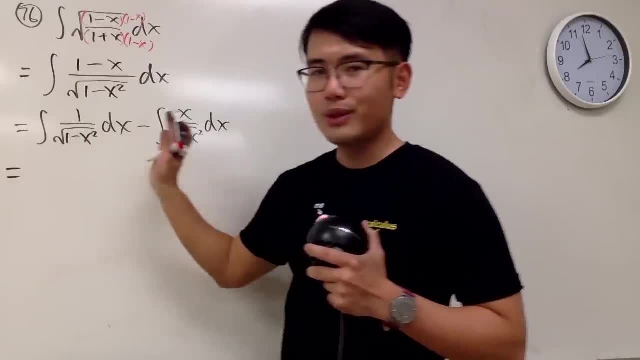 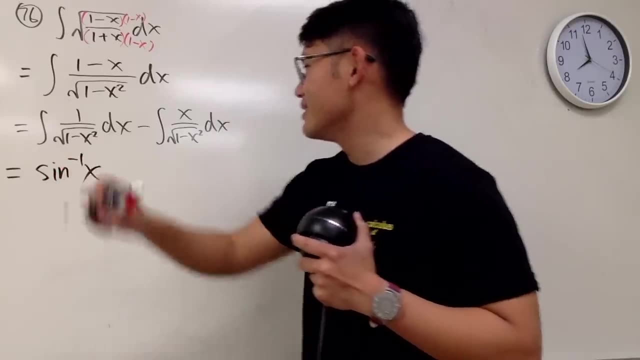 Like that. Very easy. This right here: you can do inverse sine, Or you can do tricks up. You will still end up with inverse sine. So inverse sine X, This right here. We did it earlier, So I'm not going to do it again. 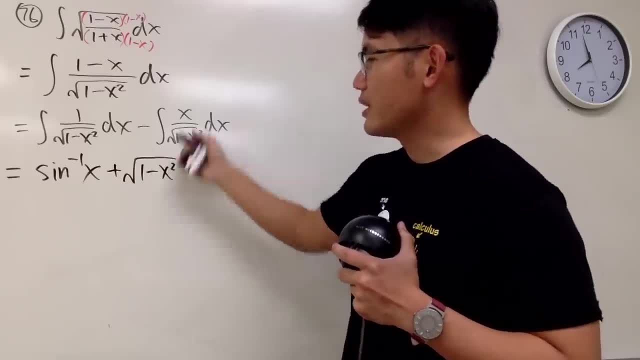 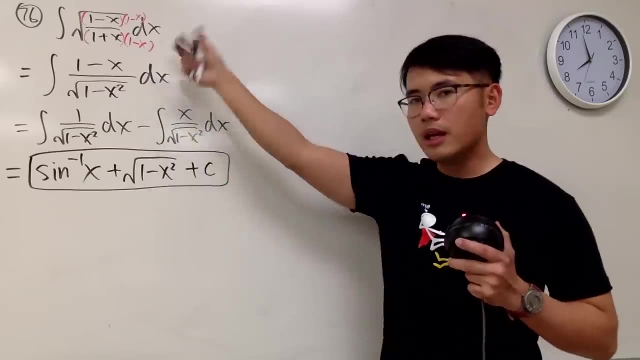 Plus square root of 1 minus X squared. If you differentiate this, you get that. So we are done Very, very nice, Although it looks intimidating. But sometimes just kind of fix the integrand Do some algebra So you can make good things happen. 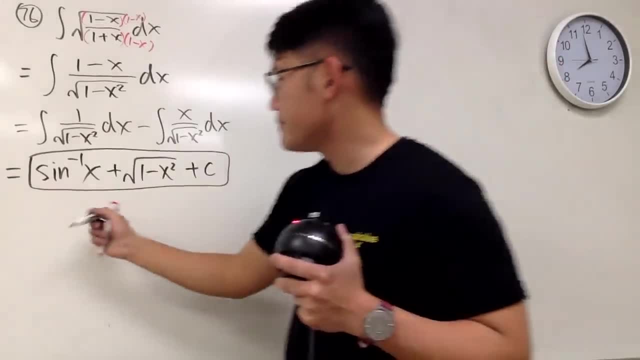 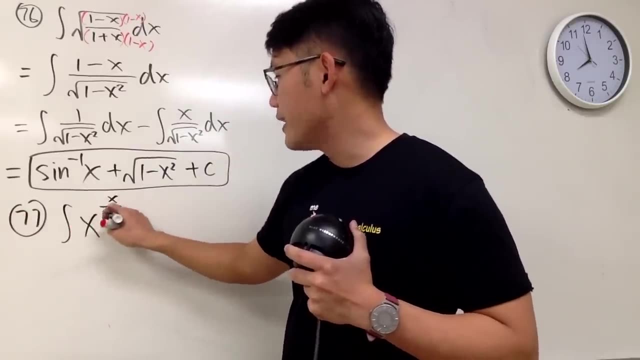 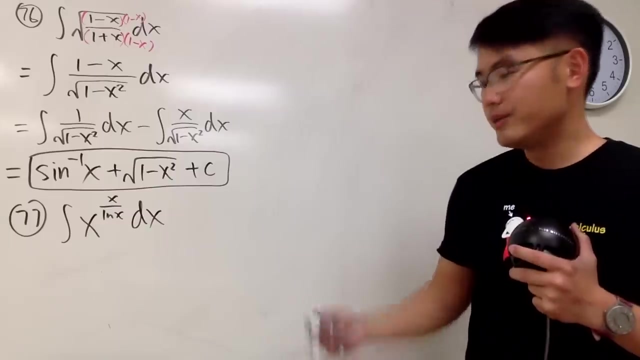 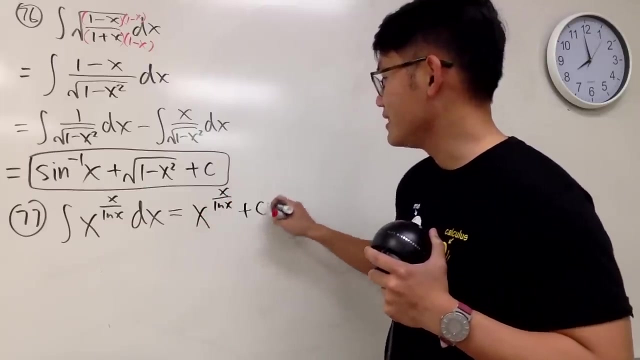 All right, Number 77.. I'll put down a question for you guys first. If you haven't seen the question, I have a crazy one: X to the X over natural log of X. The X For you guys. The answer to this is equal to X to the X over ln, X power plus C. 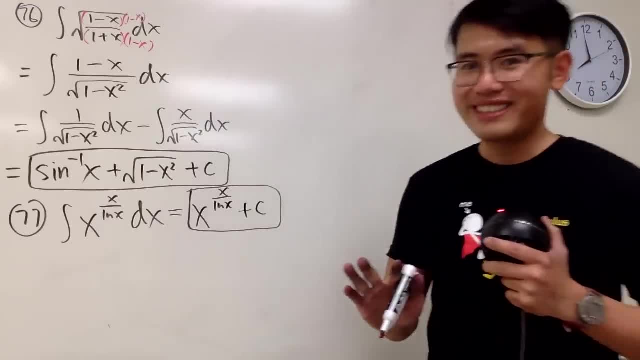 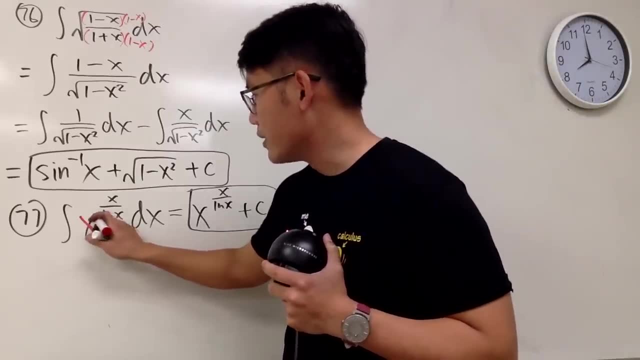 Right, Number 78.. No, I know, Just kidding, Just kidding, Just kidding. So right here I'll show you guys why. Again, same speech like earlier. We don't like to work with space X, Especially if the power is also like forever. 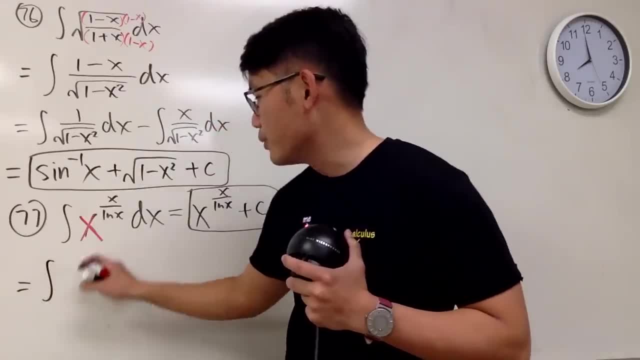 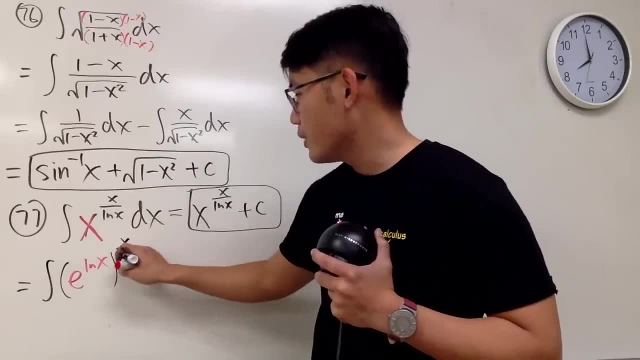 Right, We like to work with space E, So this is integral. We can look at this X as E to the ln X power And then you'll see this is X, ln X power like this. Check this out Power times, this right here: ln X. 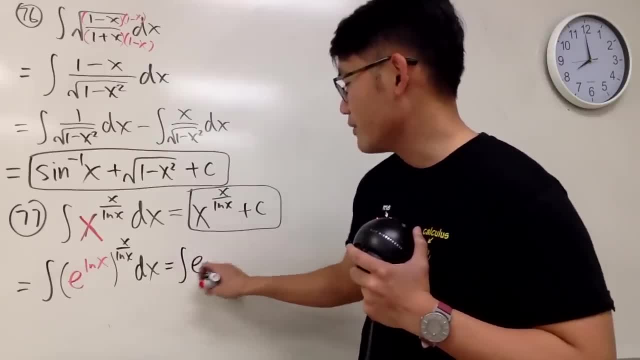 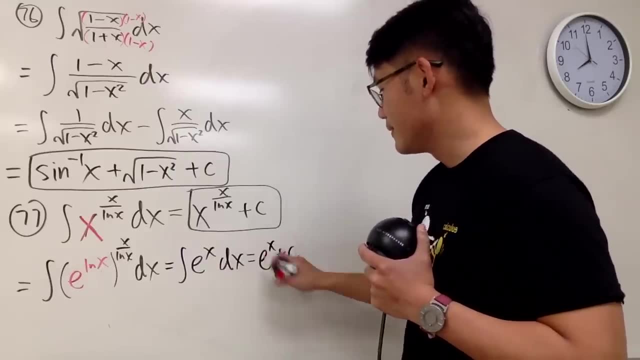 Cancel each other out. So what do we get? It's just the integral of E to the X. Got you Right? The X. Of course, this is just E to the X plus C, But E to the X, Yeah. 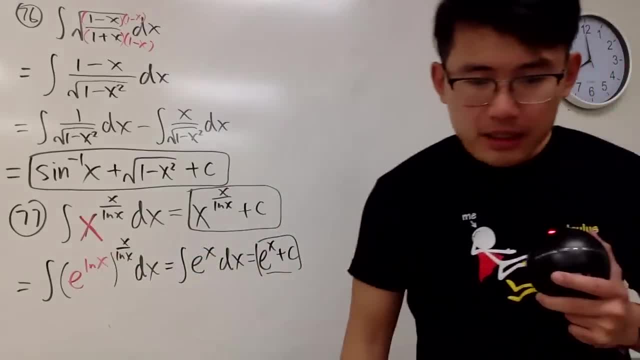 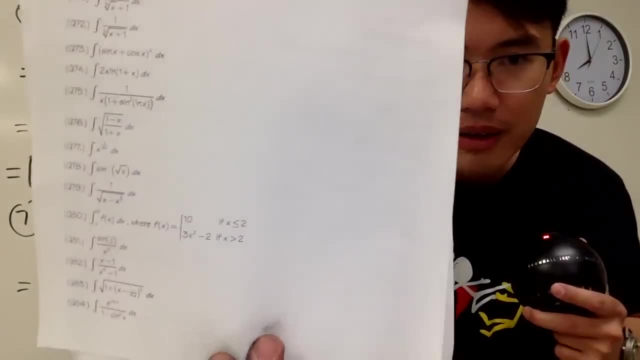 It's actually just E to the X, So that's it. Okay, So number 78.. Right, Number 78.. Okay, Inverse 10.. Why did I put this equation for myself, I don't know? Inverse sine of square root of X, like this: 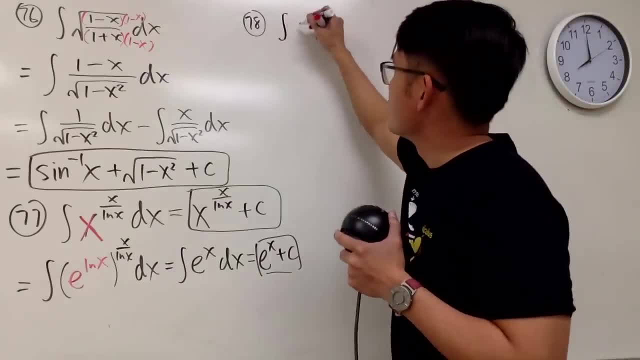 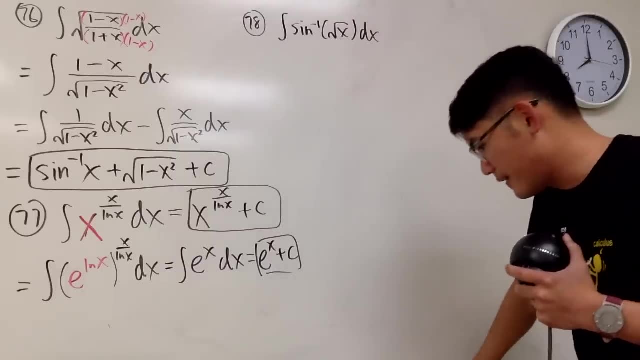 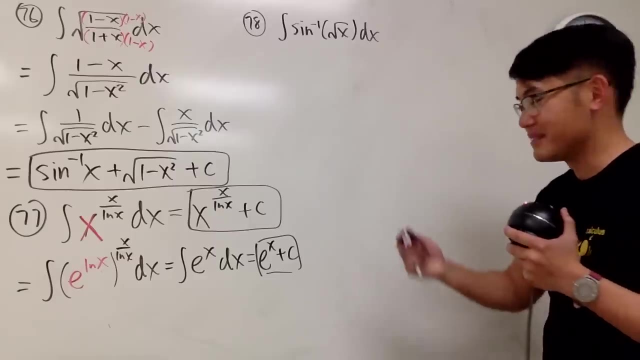 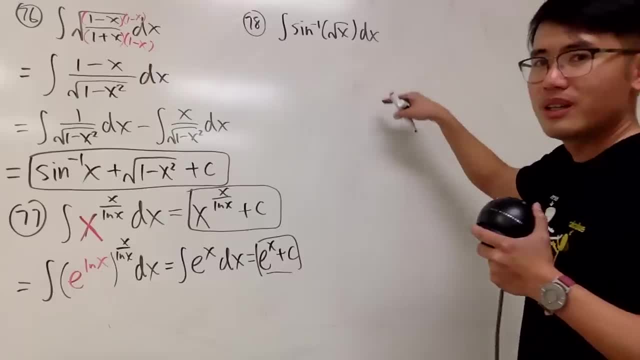 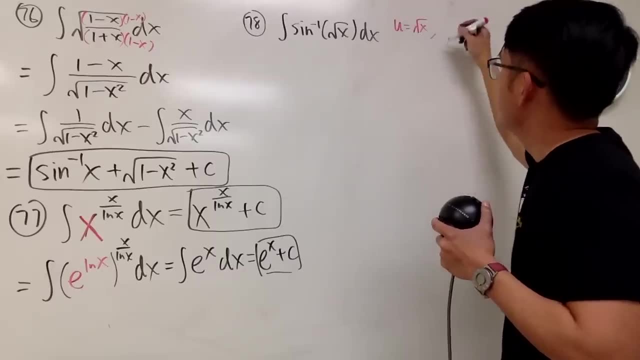 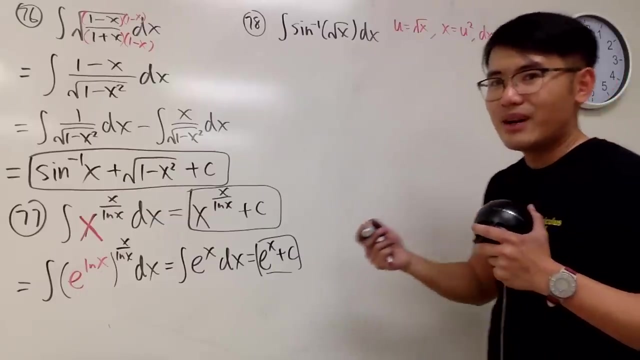 Okay, First of all we have the integral, So perhaps I will do u sub first The square root. Let's do the u sub. Yeah, Let's do the u sum U equal the square root of X and X will. 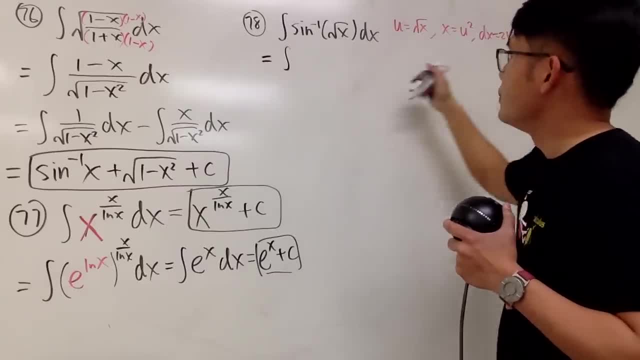 be u squared And dx will be 2u, of course. Now take a look Here. we will have the integral. I have 2u for the dx, So let me just put that down right in front. And then we have the inverse sine of u. 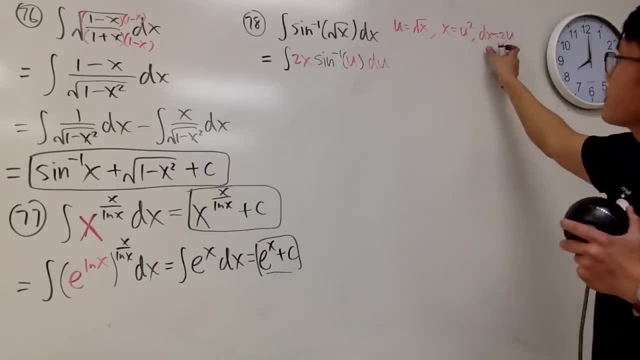 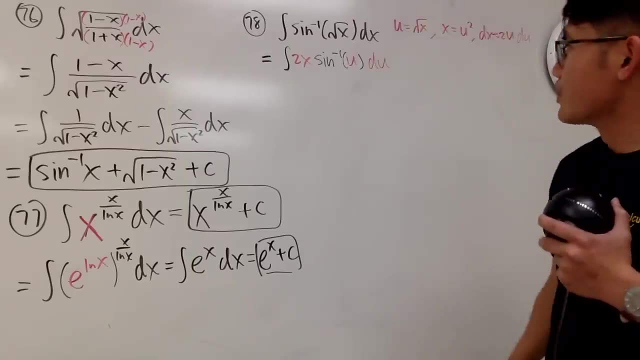 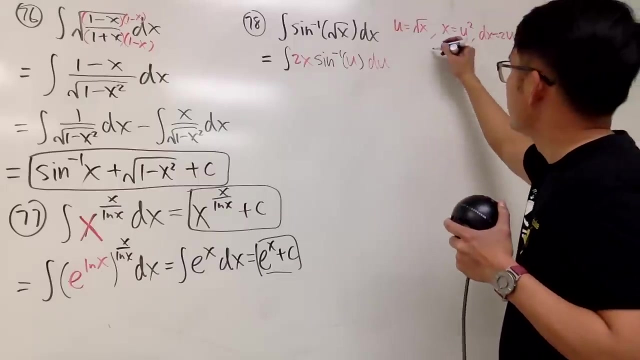 And again, here is my 2u du. Here is my dx. Did I make the question harder? I don't know. Again, try integration by parts. So we'll see. I will be differentiating something and integrating something. Differentiate this. 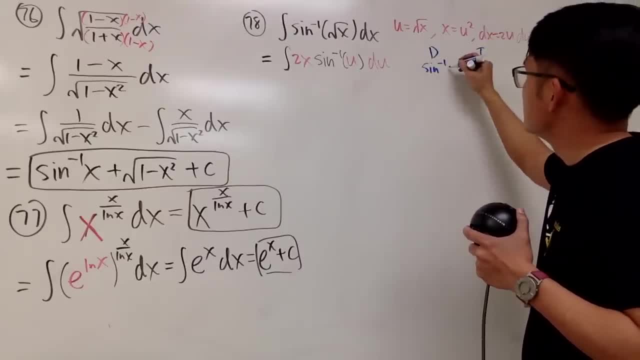 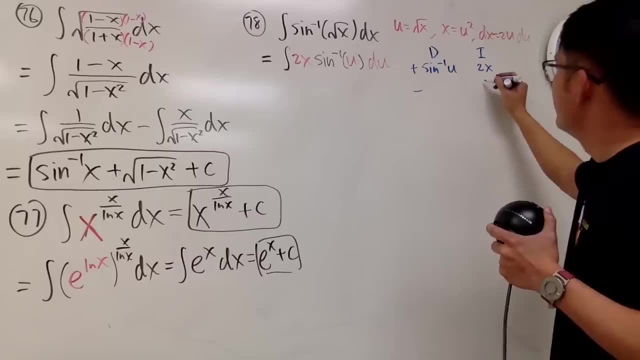 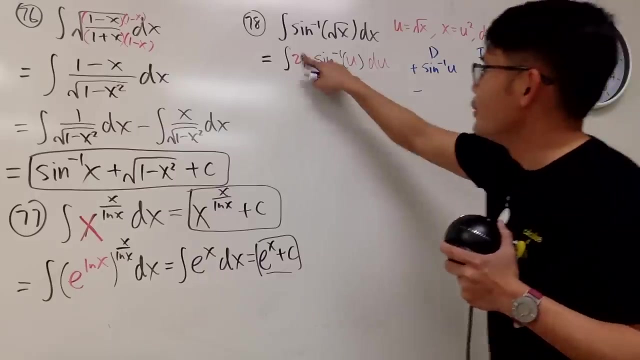 Let's see We're differentiating inverse sine of u. put on plus, minus and then integrating 2x. Integrating 2x is x squared. It's kind of weird. No, sorry, u u, u, u u u u. 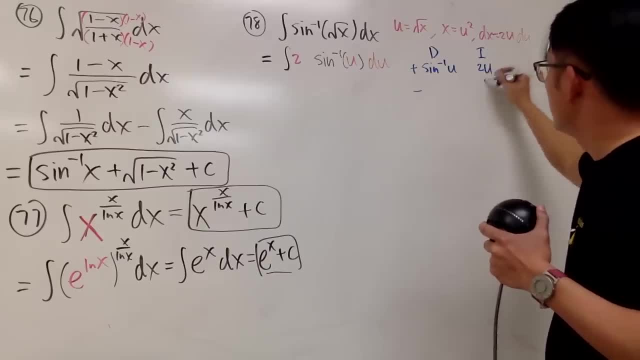 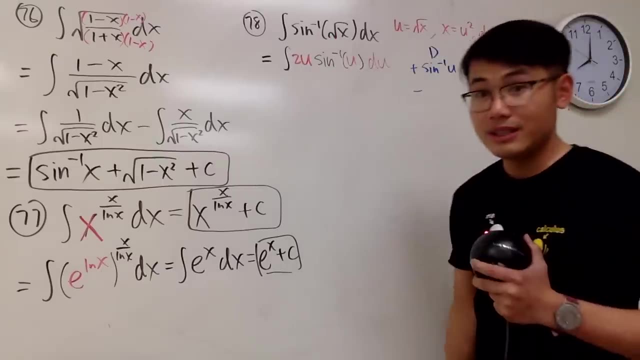 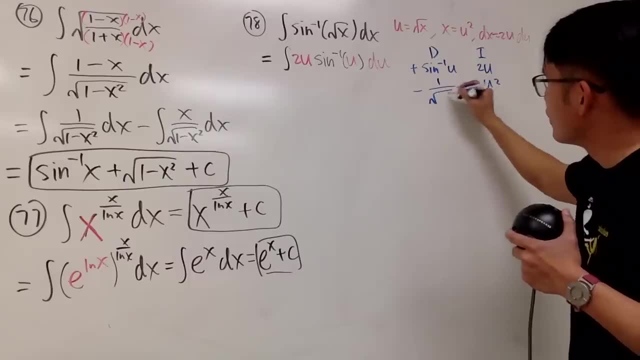 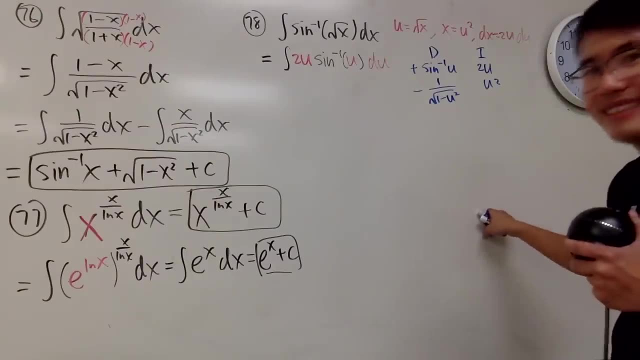 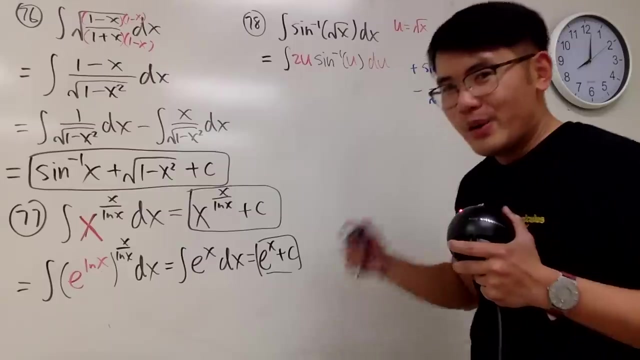 And then this right here is 1 over square root of 1 minus u squared like that right. So that's the idea. That's pretty good. This is going to be pretty hard, Whatever We can do it, So here we go. 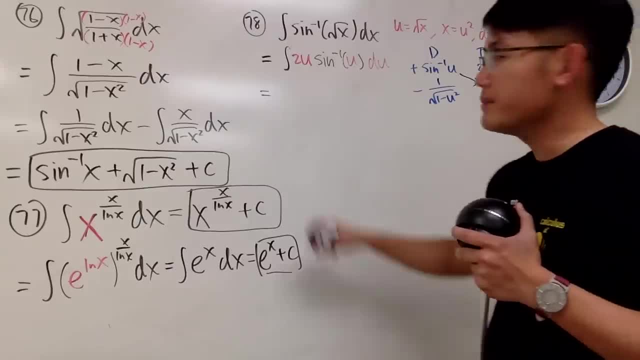 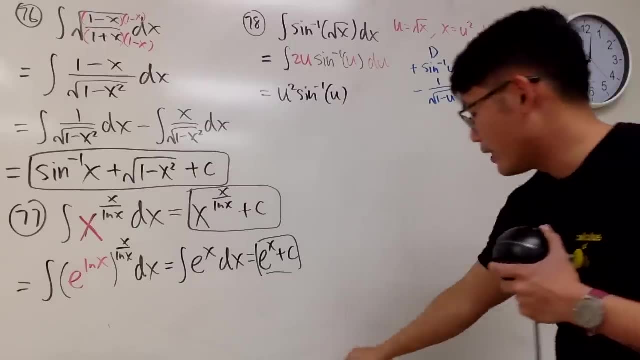 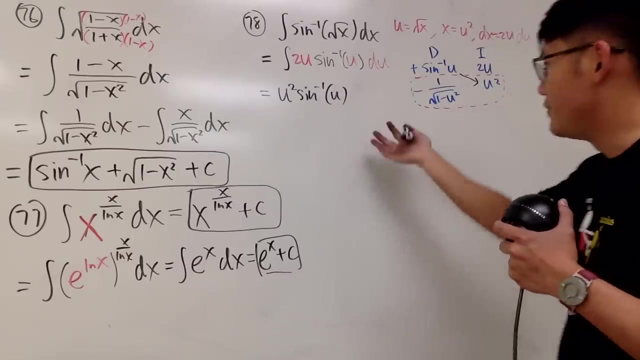 First part of the answer, ladies and gentlemen, we have that which is u squared times inverse sine of u Like that. Next we are going to have an integral which is this times that. But you know what? Let me just fit in. 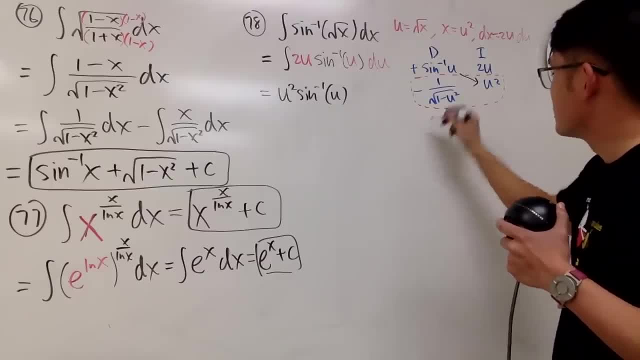 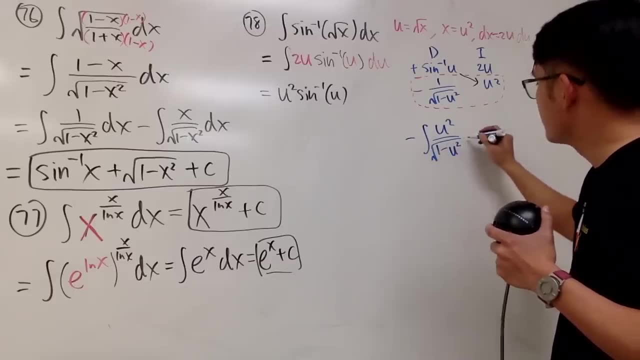 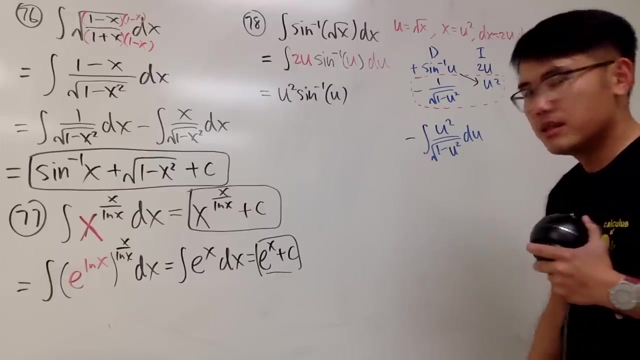 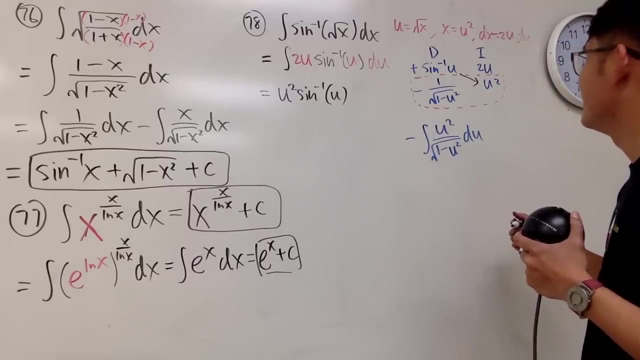 Let me just try to fit everything right here. So let's look at the integral right. So observe the integral negative integral: u squared over 1 minus u squared in the square root. du Tricks up, Maybe seriously. integration by parts. 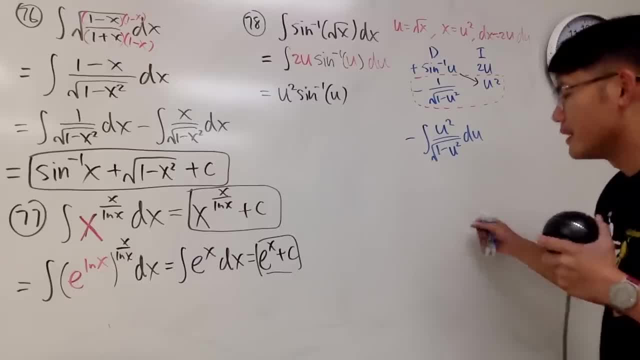 But we did the integration by parts already. Hmm, I think integration by parts might work again. Let's see u over this integration by parts And then, ah, let's try, Let's try, Let's try right. 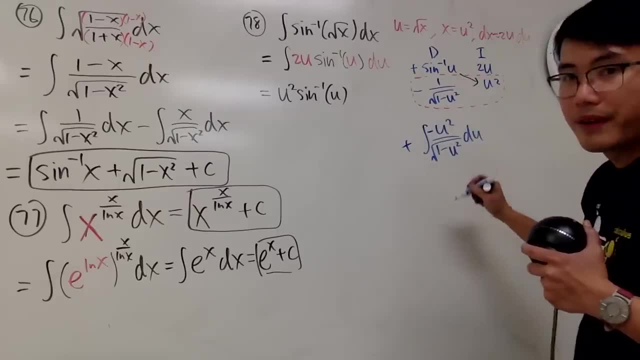 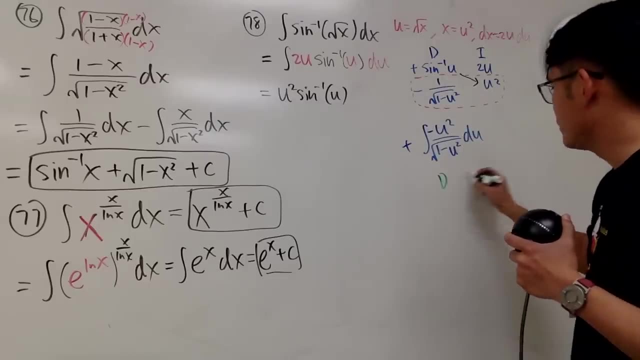 So let me just say a plus Plus negative. that, OK, And now I'll do integration by parts again. Perhaps this is the first time I can legitimately use a green pen. OK, I will differentiate something, integrate something. I am going to be putting down plus and minus first. 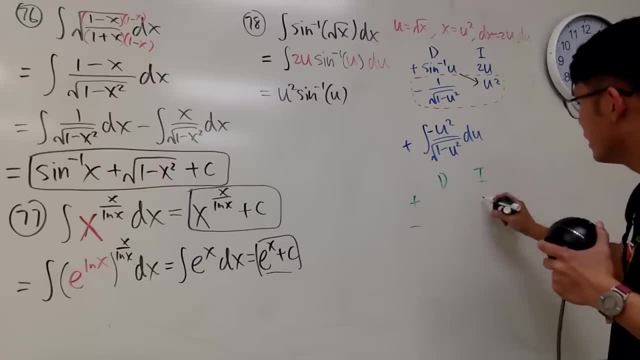 I want to integrate. OK, I have the square root of 1 minus u squared. I will put down negative u on the top for me. OK, And now I'll be differentiating u like this: Differentiating u, I get 1.. 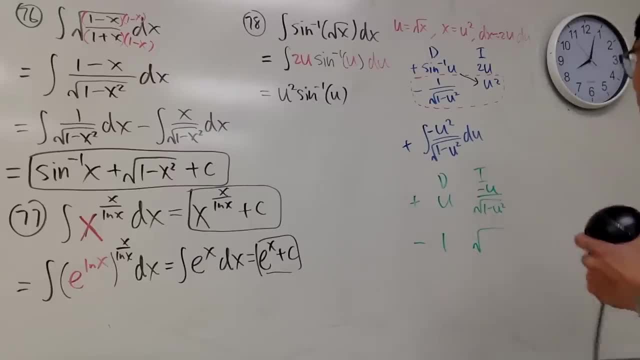 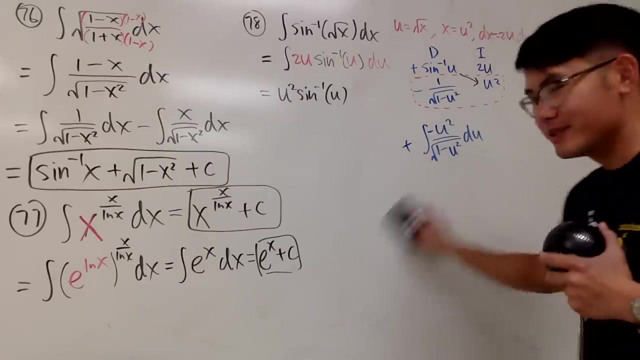 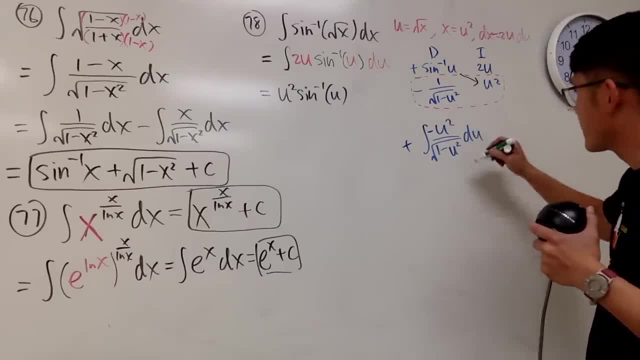 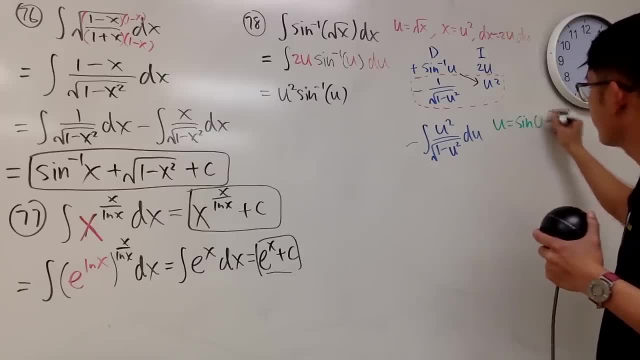 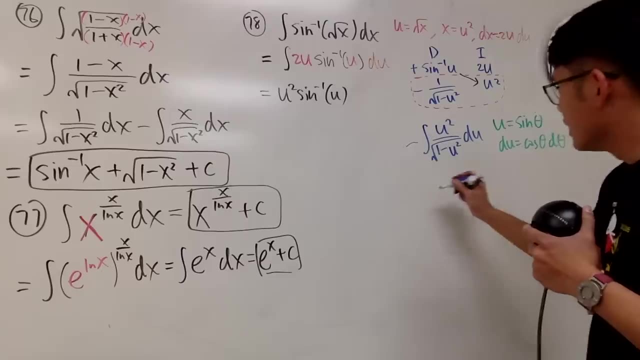 Sine theta. OK, So du will be cosine theta d theta. And now check this out. This is going to be negative integral. I have the negative right. we're going to be subtracting this. see, John, I have the negative right. we're going to be subtracting this. 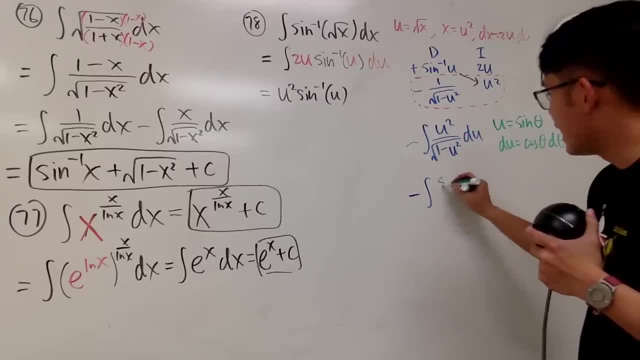 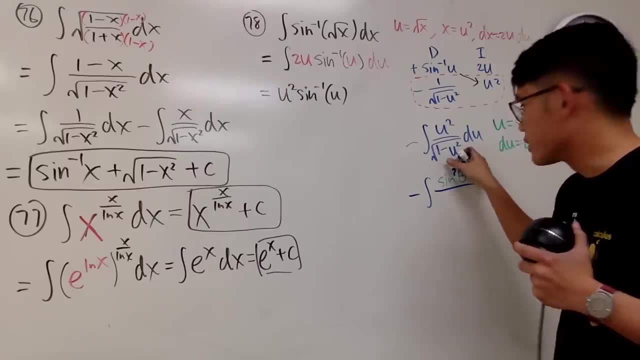 say John, And on the top we are going to get sine squared theta over i. You put sine squared here. 1 minus sine squared is cosine squared. Take div, which is going to be cosine squared, cosine squared over dx Take. i take s1, all right. 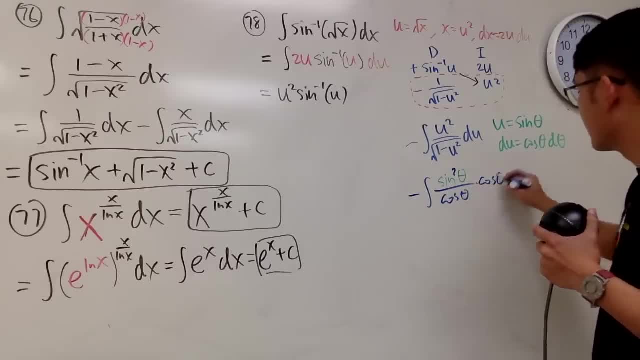 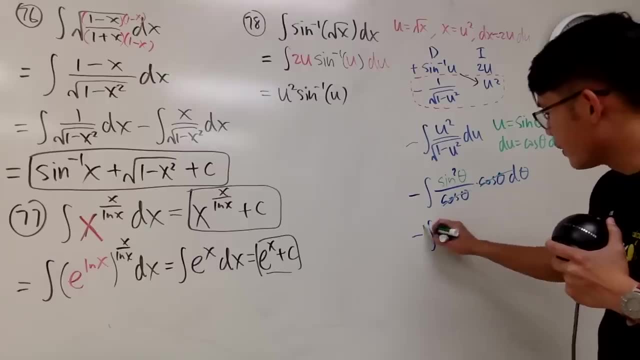 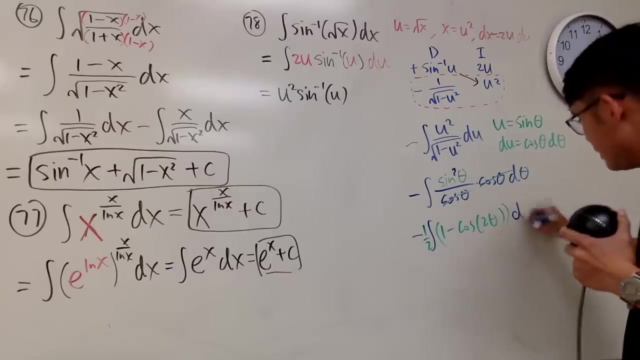 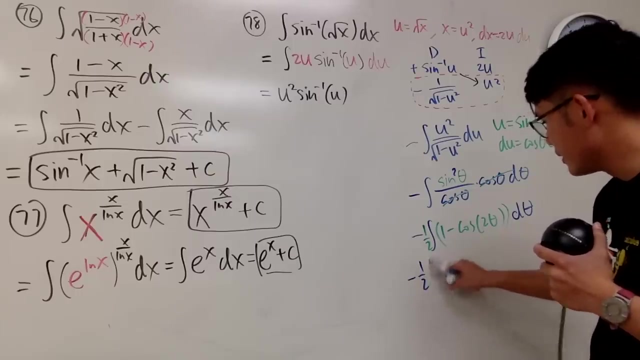 cosine, theta times. cosine, theta, d theta. cancel out this right here, minus integral. do this. you need a one half, one minus cosine, two theta like this: okay, and then d theta. this right here: negative one half. let's do the integral already, which is going to be parentheses. 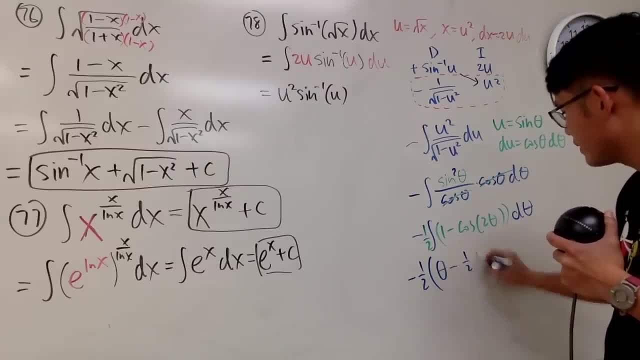 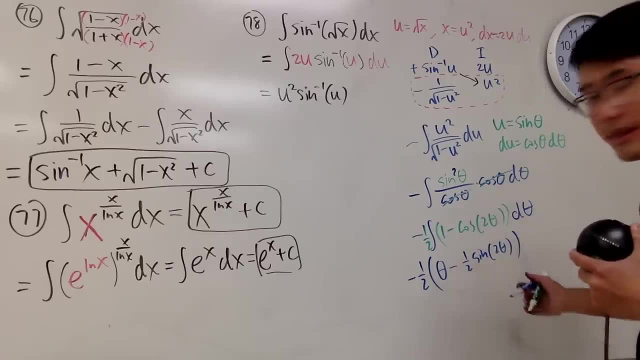 theta still minus one half. and then sine of two theta, like this normal d theta, of course. yeah, like this, okay. and then this right here is the same as two sine theta, cosine theta. cancel the two and one half, distribute the negative one half, you get negative one half. 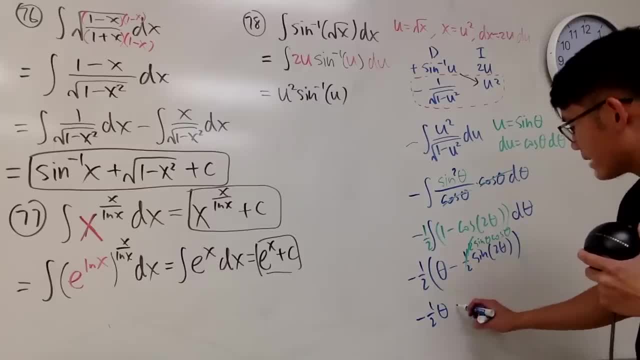 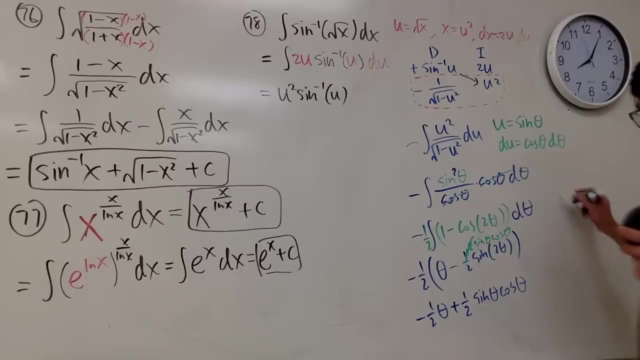 theta negative one half times, that is positive one half. sine you cosine theta. Okay, we finished integration. Let's see Sine is the u and then cosine Real quick to draw the triangle. You know, sine theta is u over 1.. 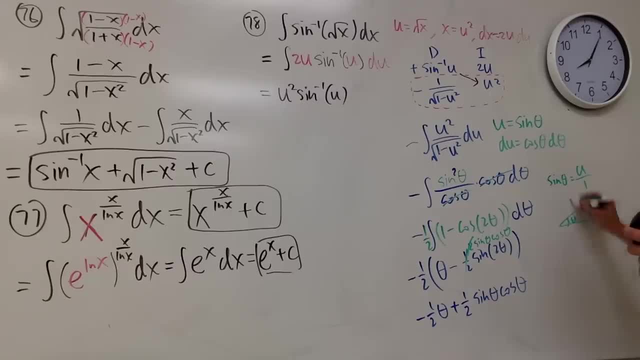 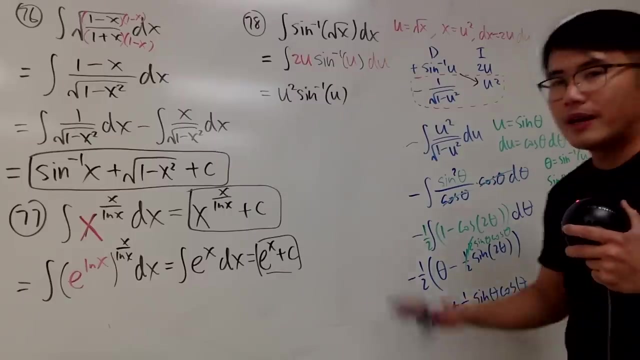 So triangle here, theta, here u over 1, adjacent is square root of 1 minus u squared. So this is nice. And then, of course, theta is the inverse sine of u. All right, So I cannot know what the answer is. I know the answer, right. 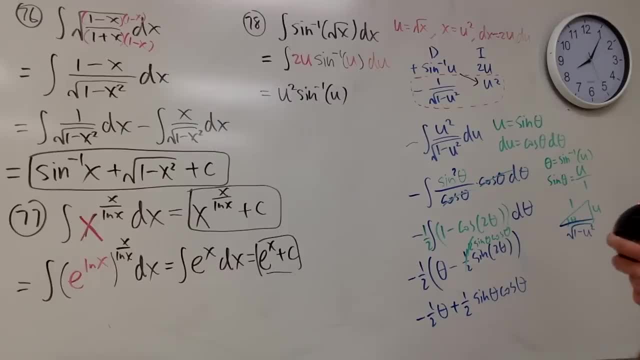 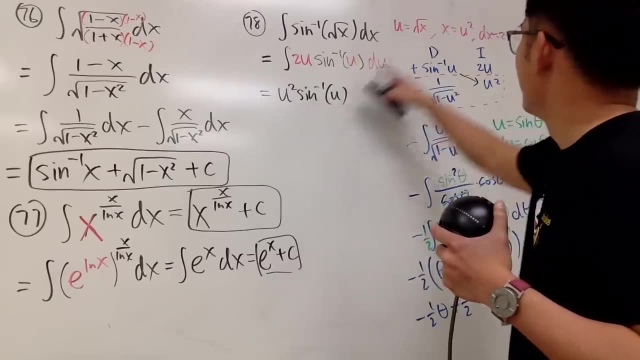 So I will just take this to the u-world and all that, But perhaps let's just write everything down right here. okay, u squared is x, So I'm just going to kind of cross this out. okay, I'm going to cross this out. 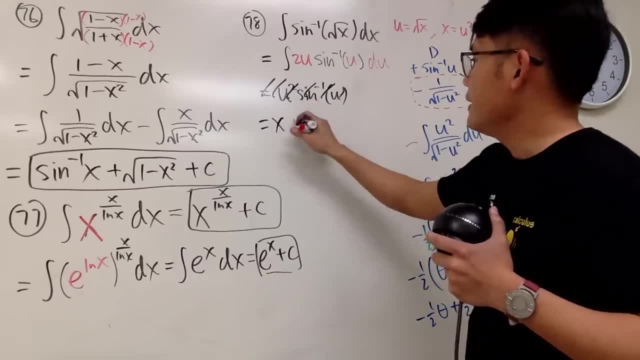 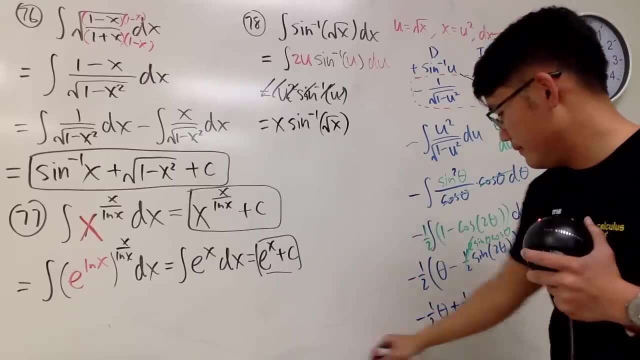 So you guys can see this right. here is x Inverse sine of u, which is square root of x. Done Next, we have this guy right, And then, as I said, I took care of the minus order already. 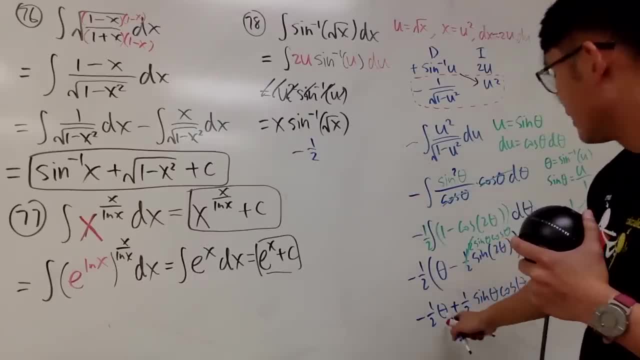 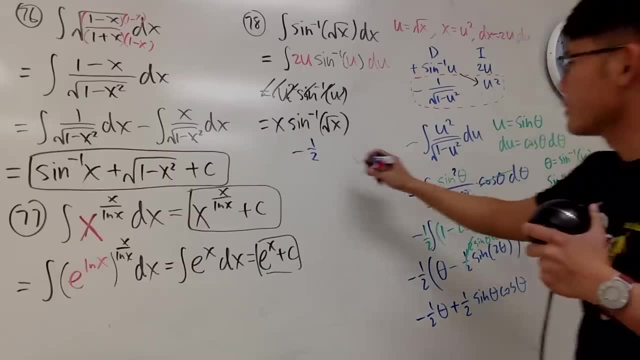 So we have minus 1 half. Theta is sine inverse u and that's the square root of x. So we can just put down the inverse sine of square root of x. So they're almost the same, but not. 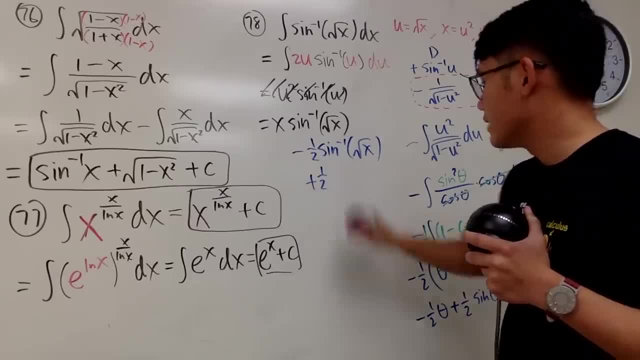 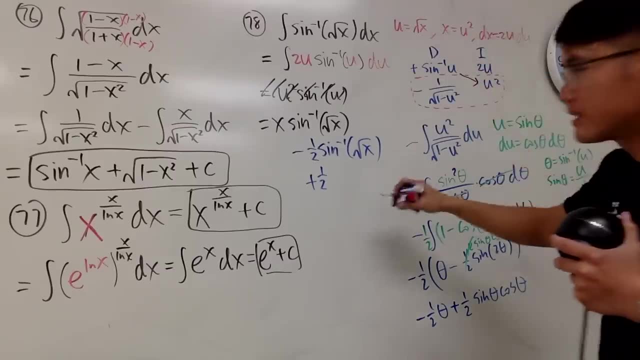 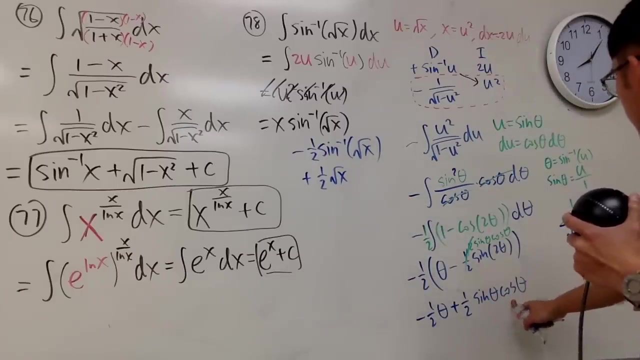 And lastly, we have plus 1 half. Sine theta is u, which is square root of x. So we put down square root of x, right here. Cosine theta is this, right, This over that. So just this. 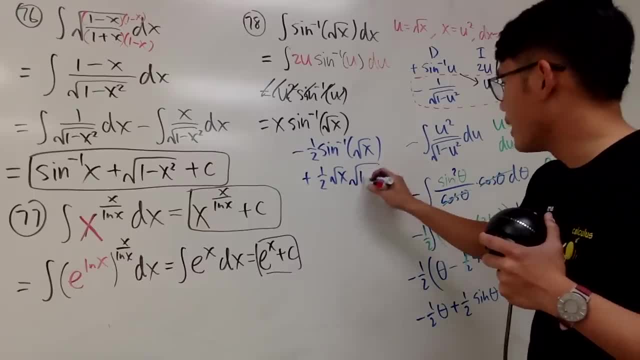 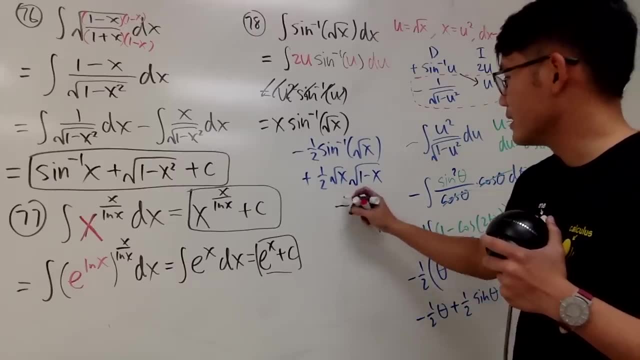 And u squared is x. So it's just that which is square root of 1 minus x, Like that We're done. Put a plus c. Let's make this plus a big c, bigger c, Like that. So this, right here, is our answer. 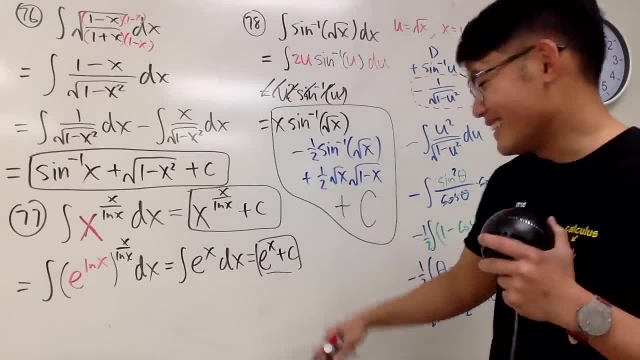 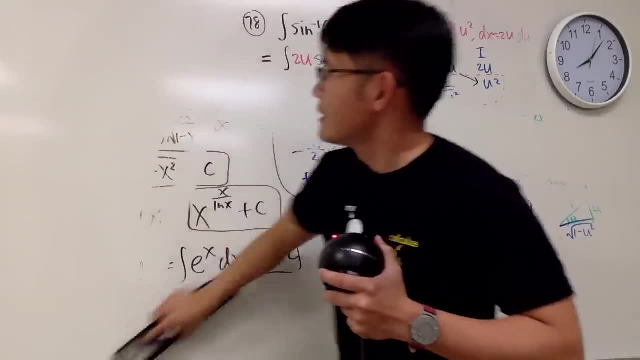 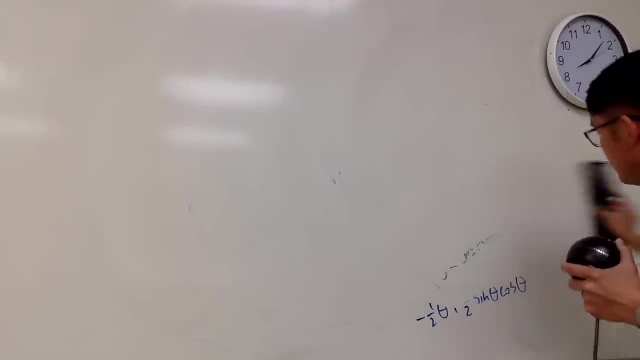 Yes, I came up with all these questions and I am doing them all right. Wow, a lot of things going on. I want to go home before 9 o'clock. I don't know. Let's see, Wow, Wow. 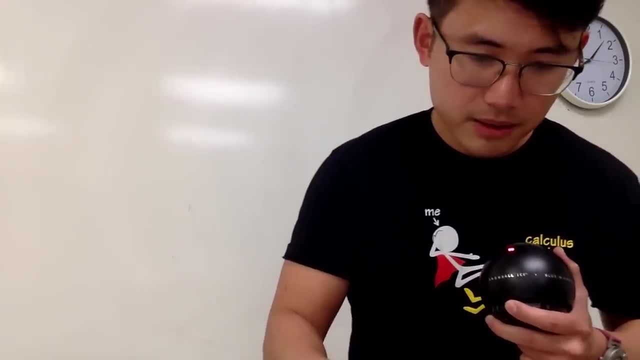 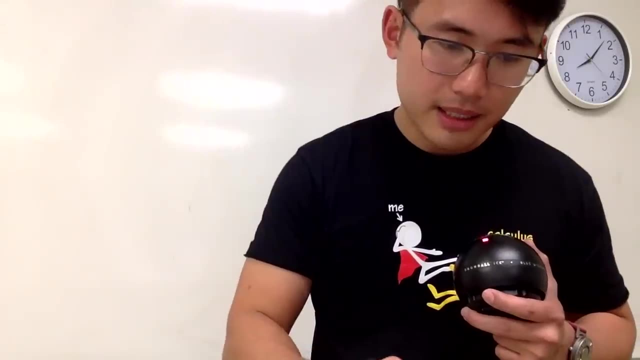 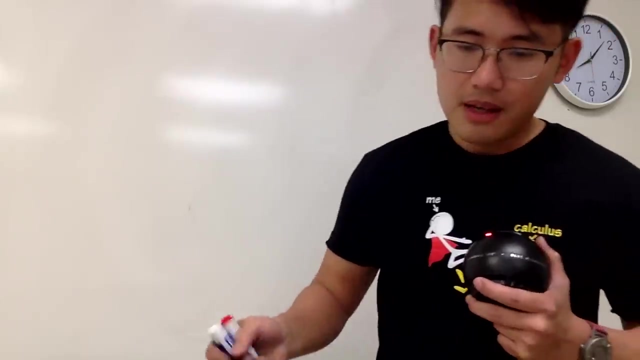 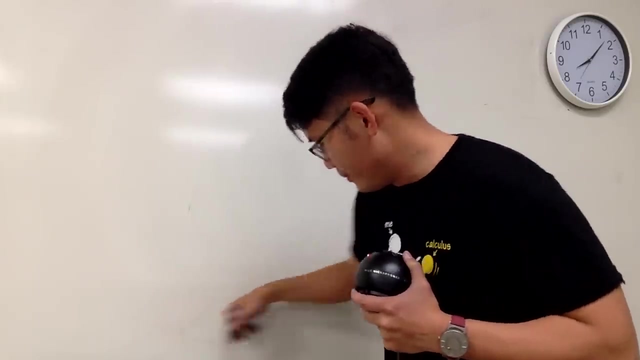 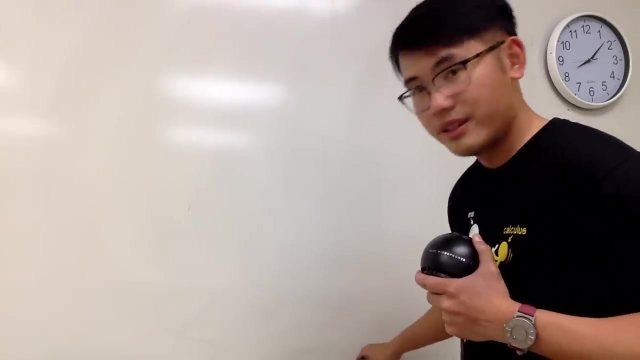 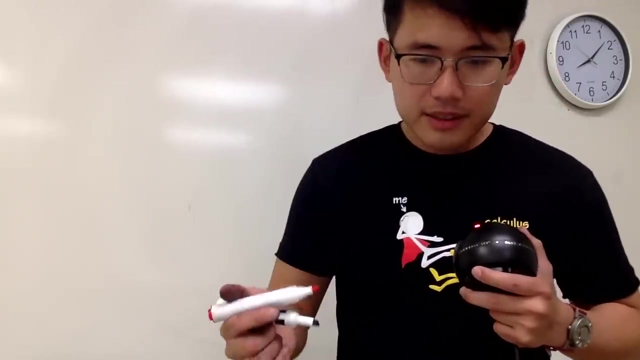 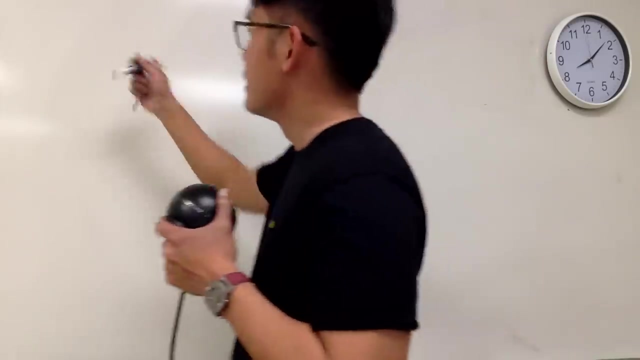 Okay, let me put this back. Take a little right. Let me just put this back in order to get this ready. Let me get the markers ready and all that. Okay, So let's see. That was number 79.. 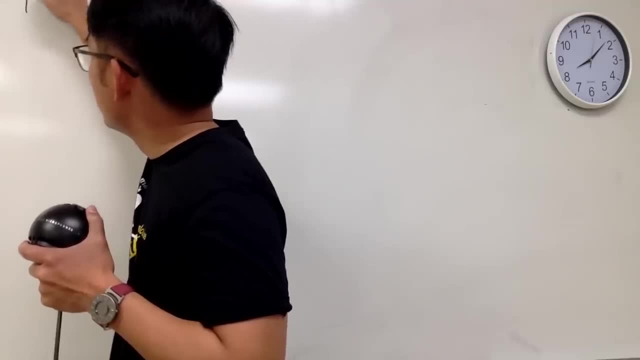 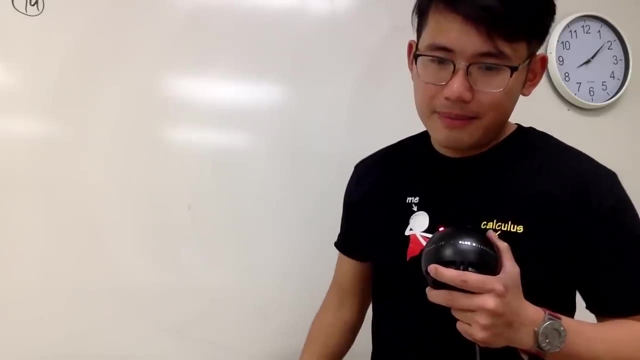 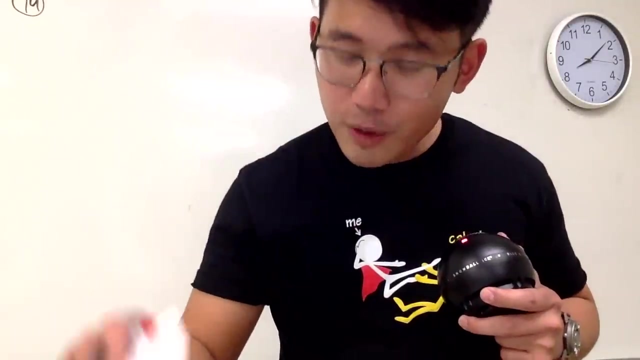 So let me just write this down right here for you guys: Number 79,, right? So, hmm, All right, To be honest, I think I did this question already. I have a duplicated 179.. I think that was the one that we did earlier from 31.. 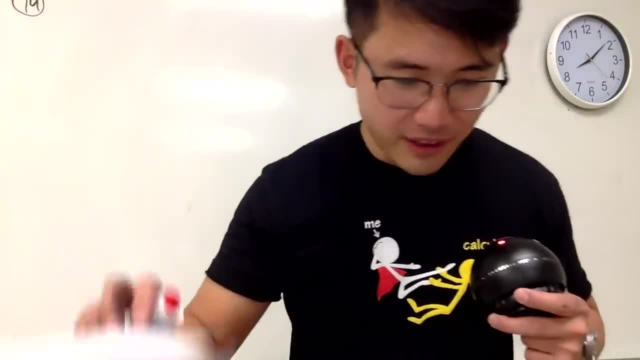 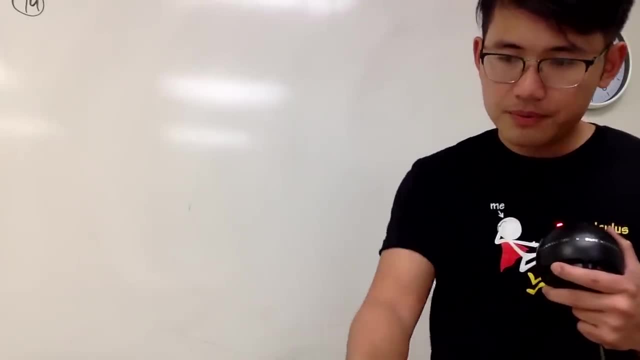 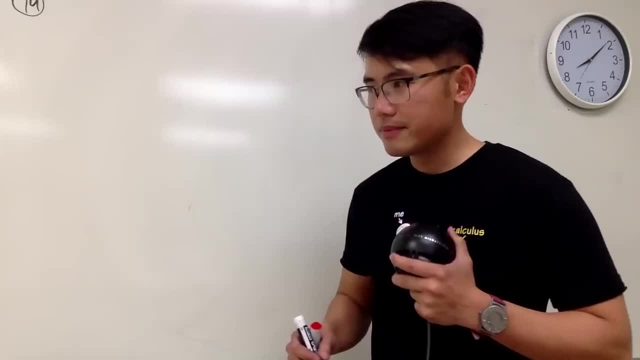 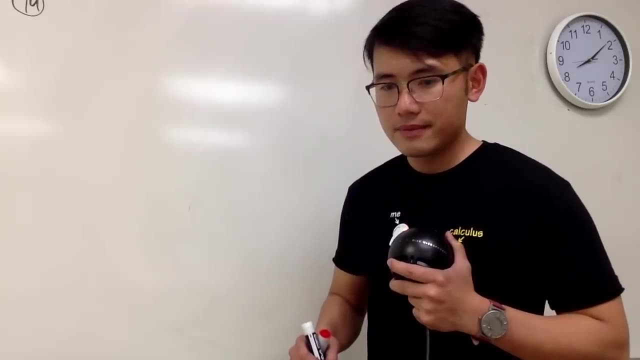 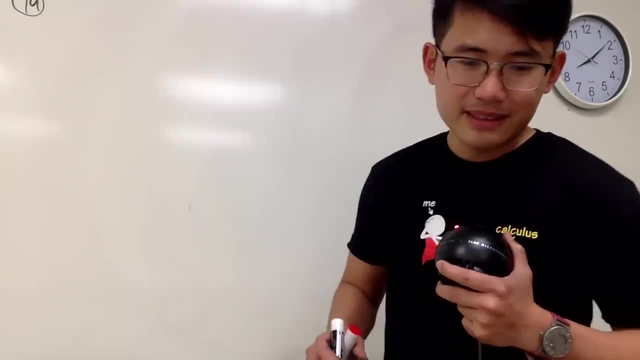 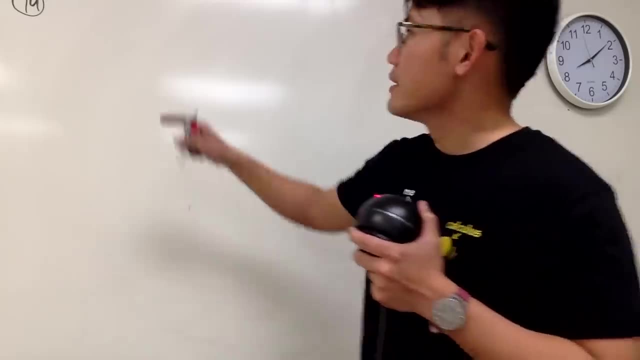 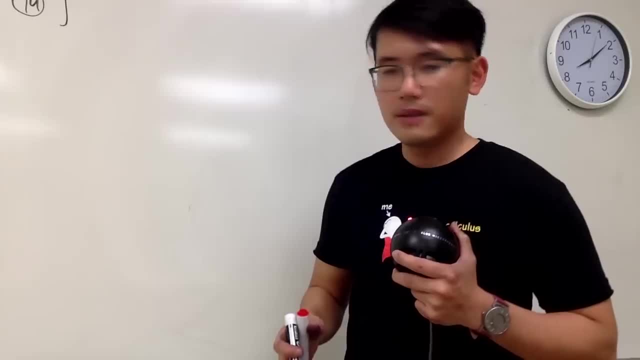 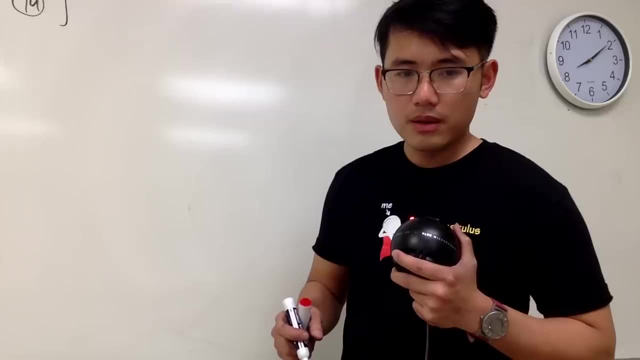 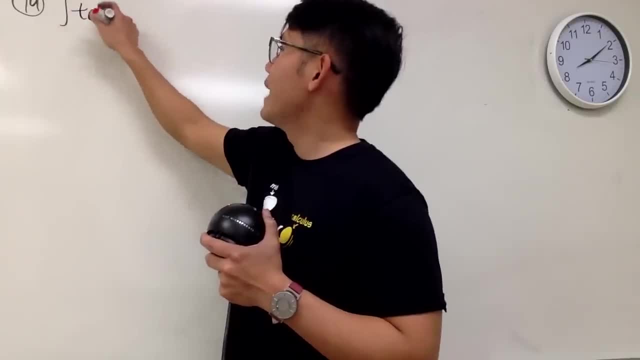 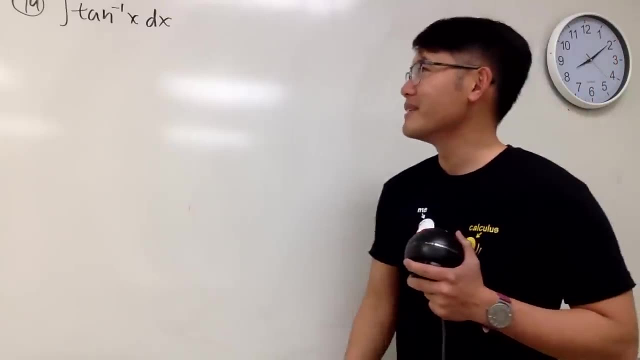 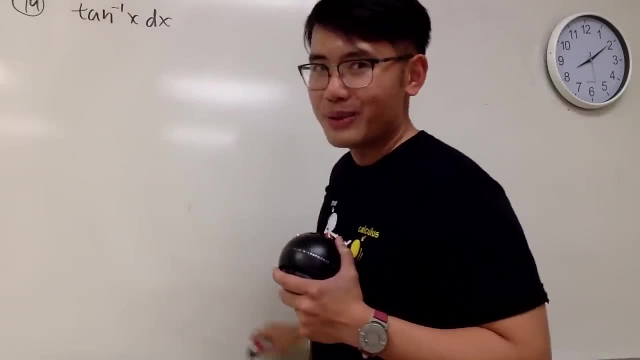 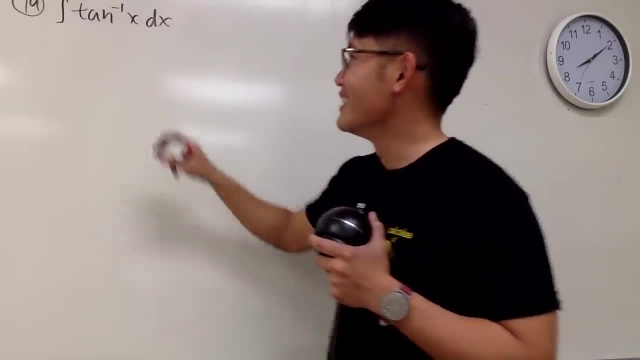 I have a follow-up video for this. I will show you guys how not to integrate this guy, because I gave all the test already, like recently, and I saw so many different ways to answer this- Wrong, of course. So the way to integrate this is you have to use integration by parts. 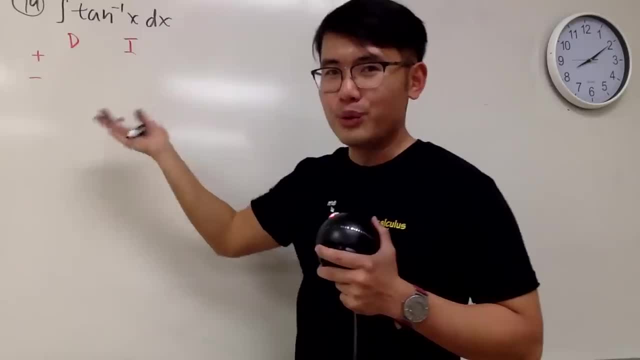 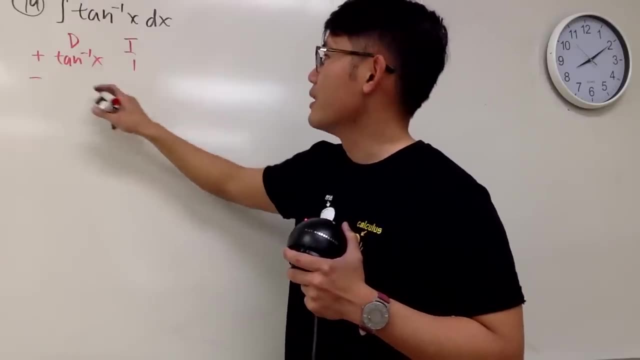 So I put in a d and an i. So this right here can be pretty easy if you set it up the right way. You have to differentiate this And notice this is the inverse tangent x And then integrate 1.. Integrate this. you get 1 over 1 plus x squared. 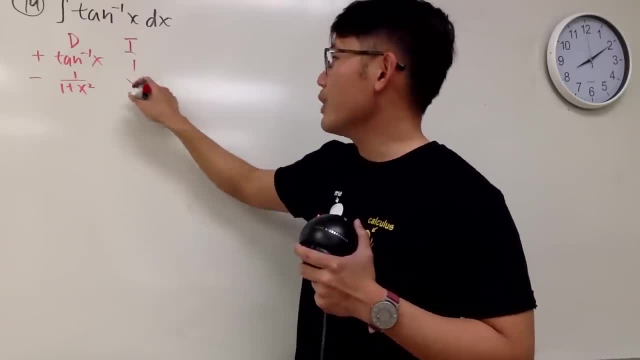 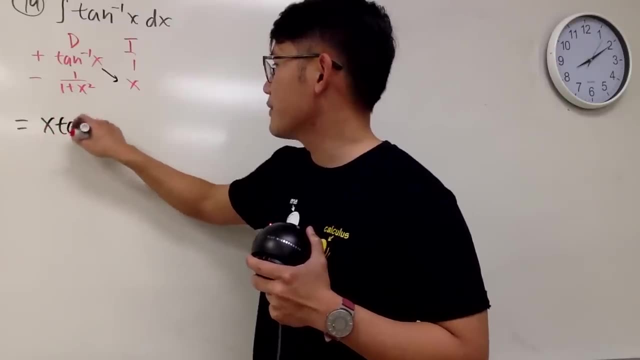 And then I mean differentiate this: you get 1 over 1 plus x squared, Integrating 1,, you get x. So here is the deal: This times, that is the first part of the answer. So you have x times inverse tangent of x. 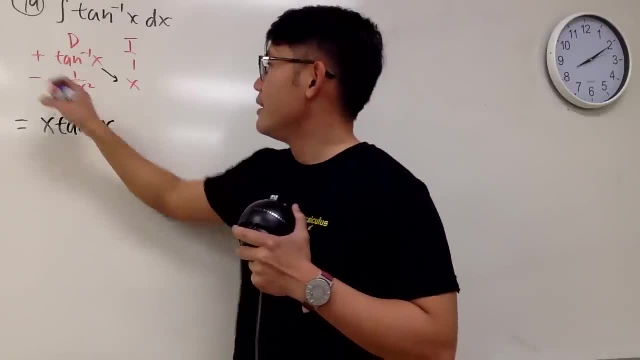 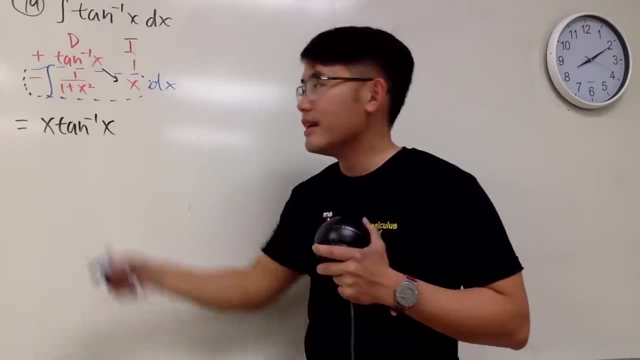 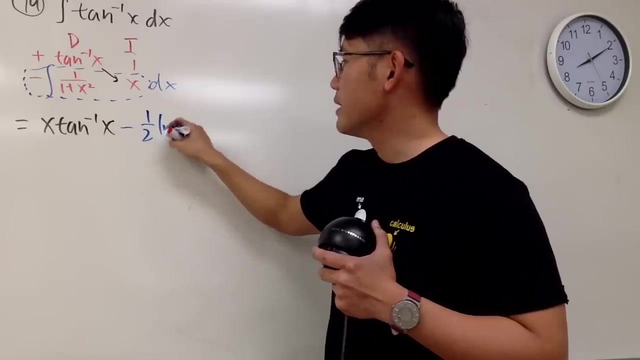 And then this right here: Again, this is still an integral. okay, This is still an integral. And you let u equal to 1 plus x squared. So what you end up with is minus 1, half natural log, And with 1 plus x squared inside, you don't need the absolute value. 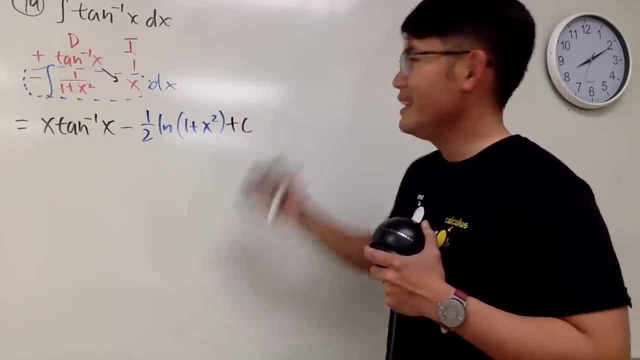 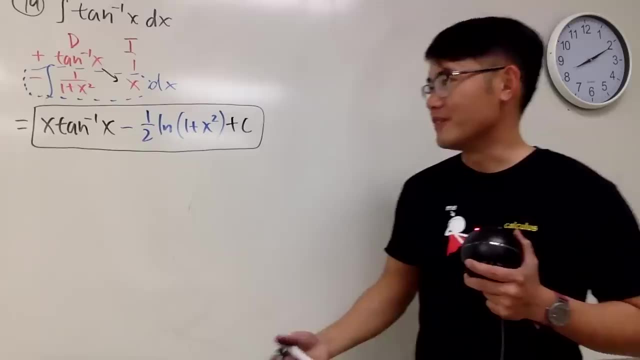 This right. here is it. This is the right way to Integrate it. It can be really easy, But I will show you guys in a follow-up video, In a follow-up video, how people do this incorrectly. All right, So yeah. 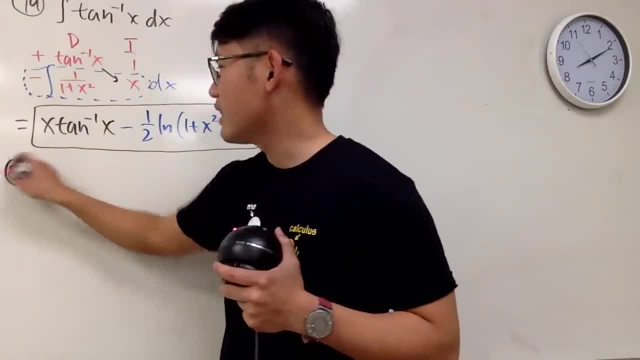 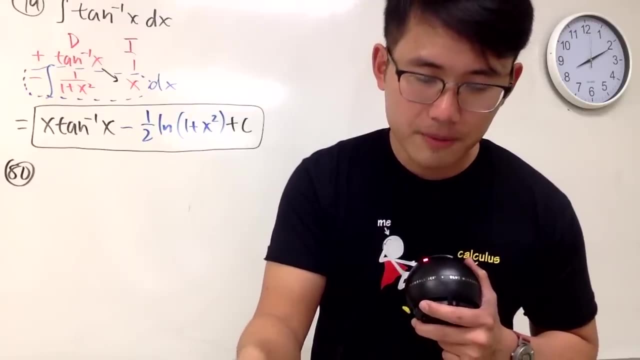 All right, Now number 80.. 80% done, 80% done. I'm worried about I have four hours. I should have another hour or so to do this In terms of the memory, solve the memory, the computer. 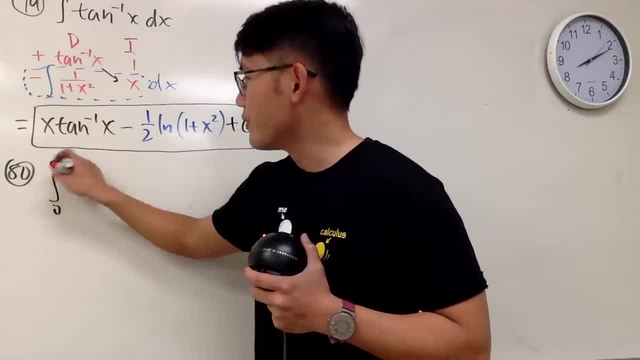 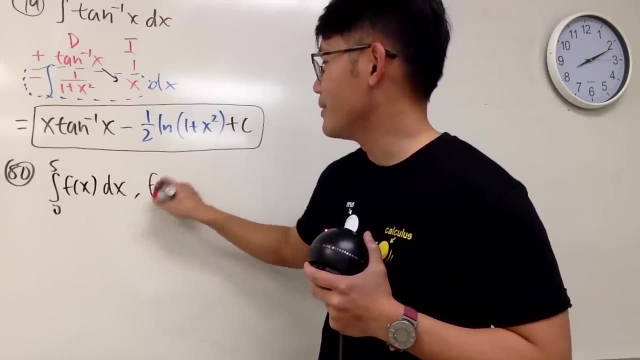 So we'll see Number 80. Integrating from 0 to 5.. f of x. Oh my God, What's f of x? Don't worry, I'm telling you guys that f of x is a piecewise function. 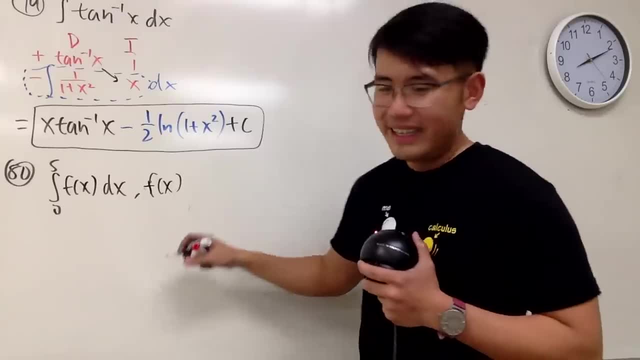 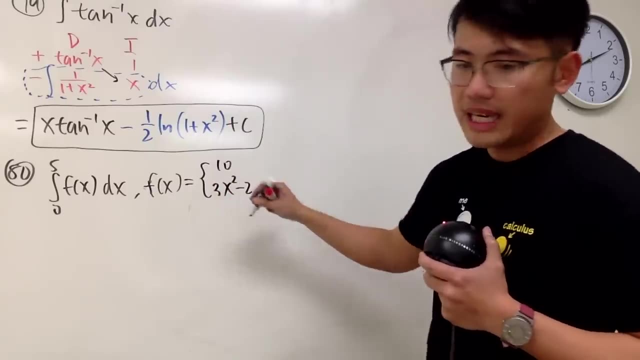 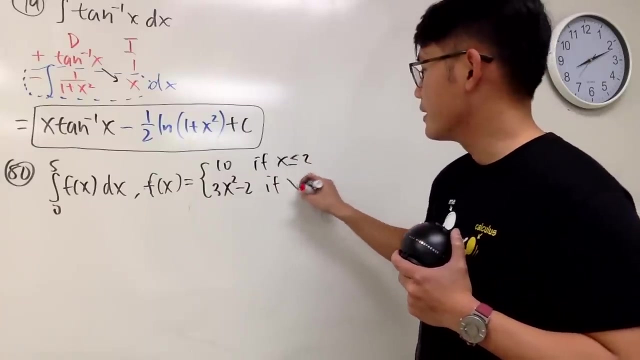 So maybe you have to worry. Yeah, This right here, I make it to be 10.. And 3x squared minus 2 is 10 if x is less than or equal to 2.. And this is if x is greater than 2.. 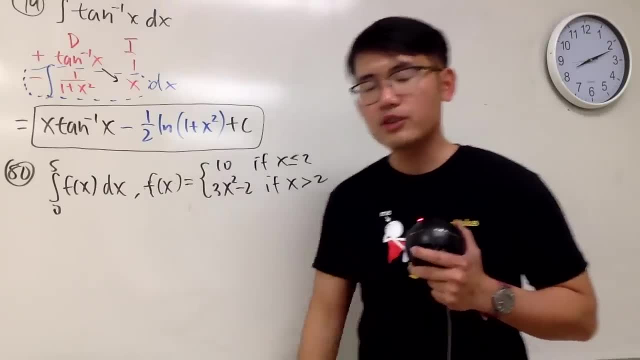 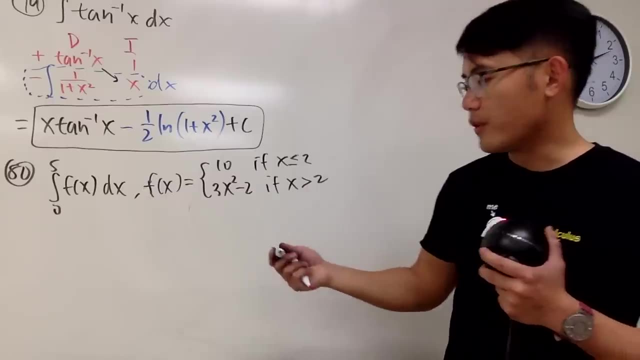 So this is how you are going to deal with the integral of a piecewise function. You are going to just separate them because, especially when you have the equations right here and right here, Pay attention to the interval. That's all, So it's not that bad. 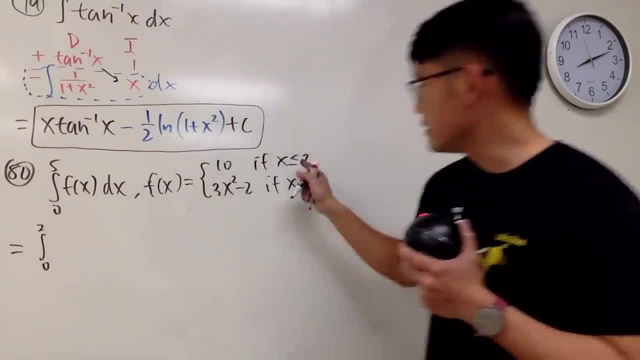 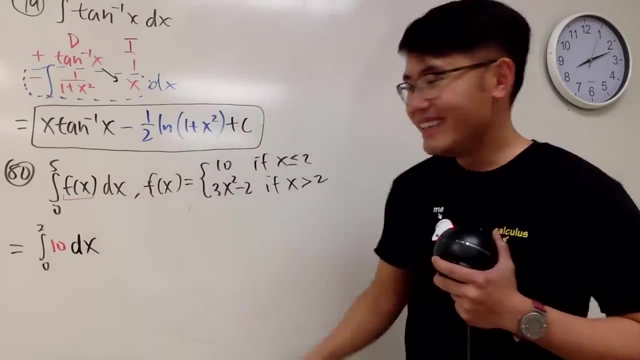 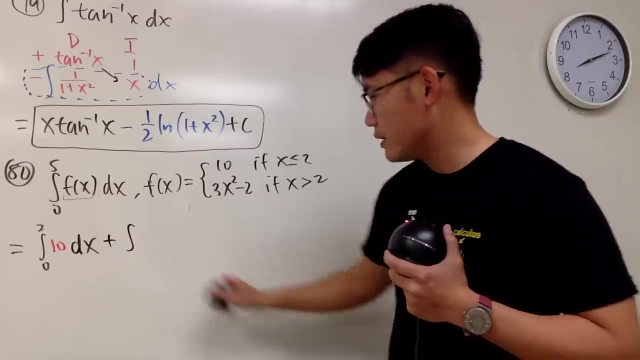 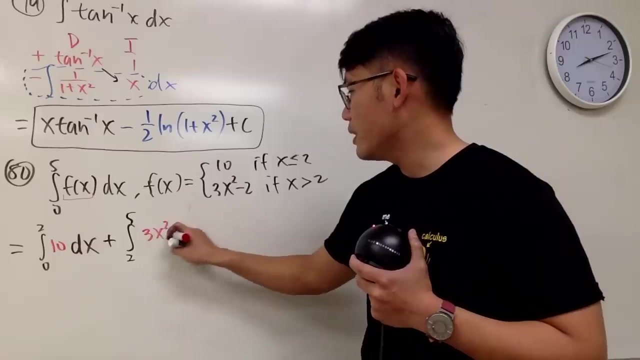 First, you are going to look at this and integrate it from 0 to 2, because it says so, And for that f right here will be 10.. And then dx, Okay, And then you are going to, You are going to add the other part, which is from 2 to 5, and then you have to do this, which is 3x squared minus 2,, like that. 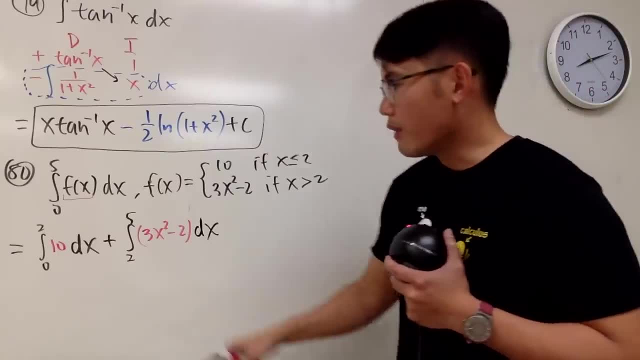 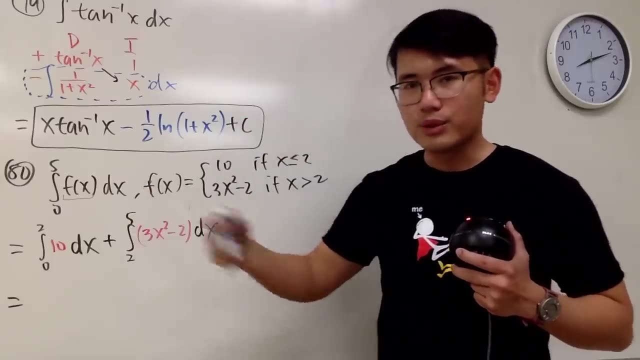 And then the dx. That's pretty much the idea. So this right here, it's actually pretty easy, because it's just 10,, always 10, and you find the area under that curve from 0 to 2. So you end up with 20.. 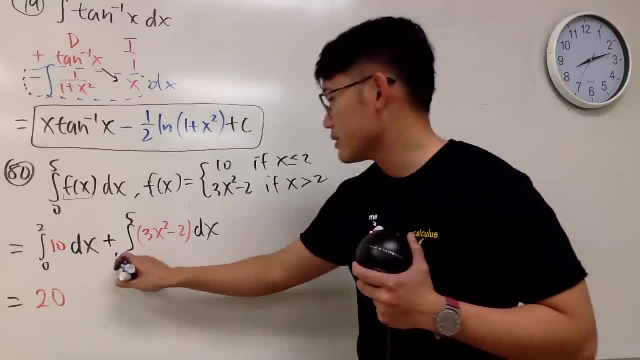 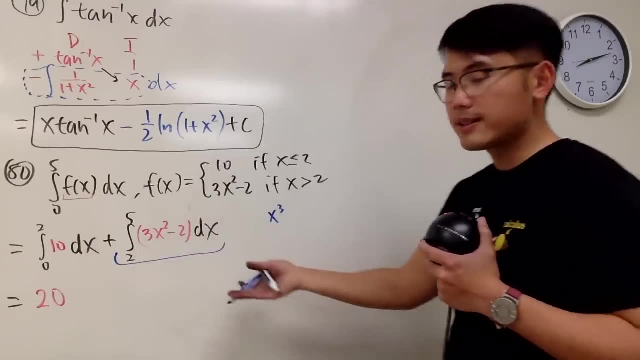 Okay, You end up with 20.. This right here. let's take a look right here real quick. You have to integrate it, which is x cubed, right? Integrate it, you get x cubed And then minus 2x, just like that. 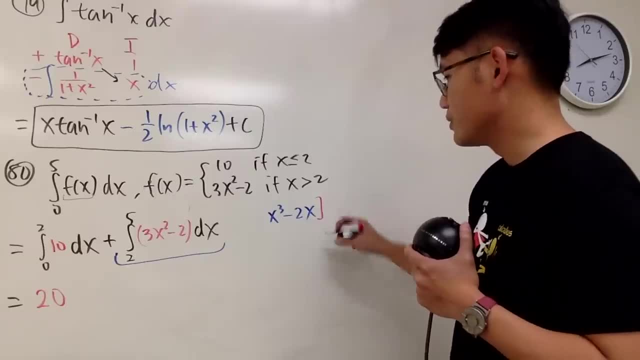 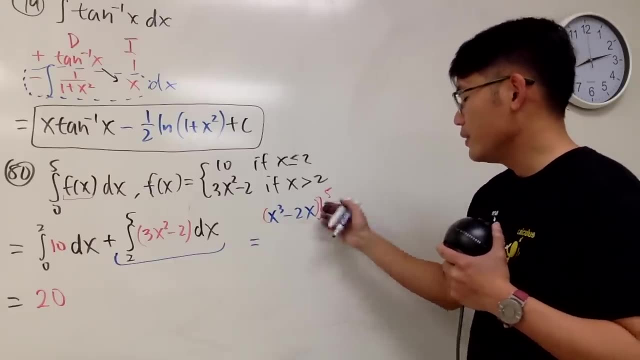 And you are going to plug in, plug in numbers, So just do the dirty work. That's all All right. So let's do this in our head: 5 into there. you get 5 to the third power, which is 125.. 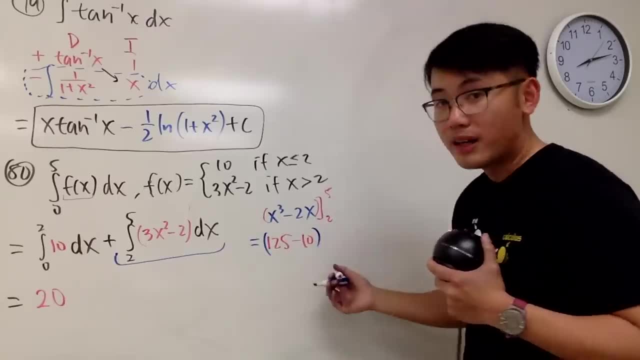 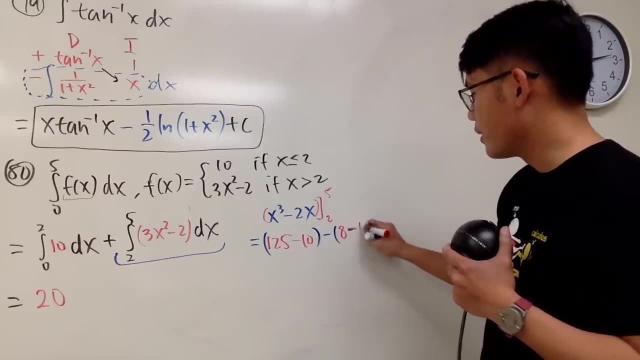 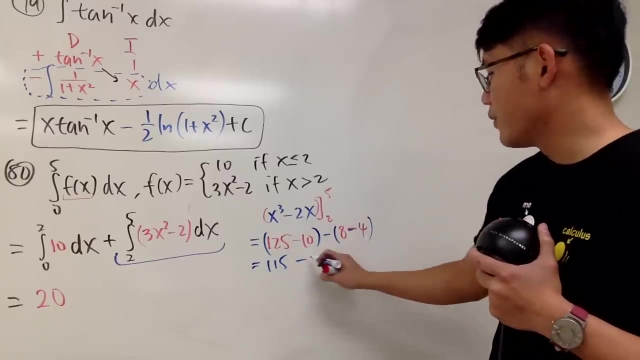 And then minus 10.. This is the first part, and then you are going to subtract. The second part is 8 minus 4, like this, Not bad. So in other words, this is 115 minus this is 4.. 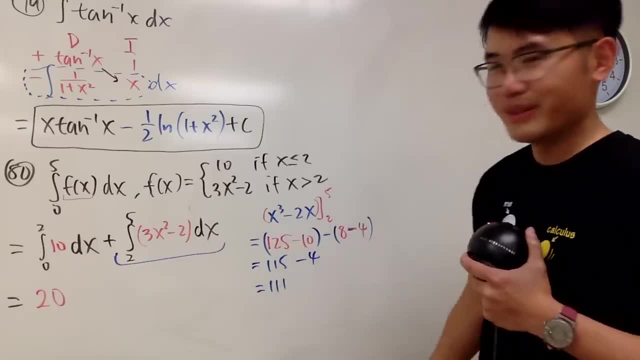 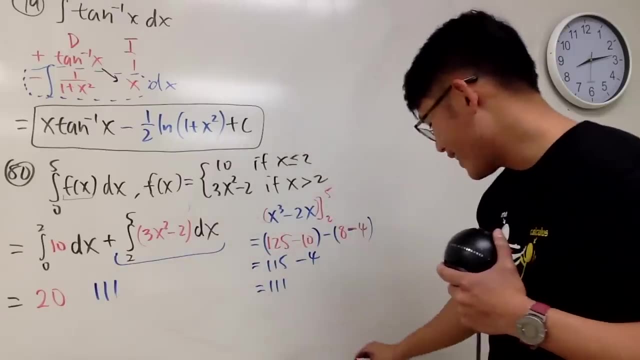 So altogether you have 111.. Cool huh. Double check: Yes, it's correct. So you are going to be adding 111 for it. So So it's not that bad. It's much better than some crazy function. 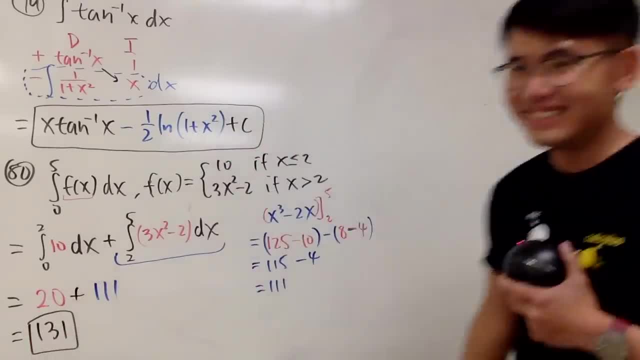 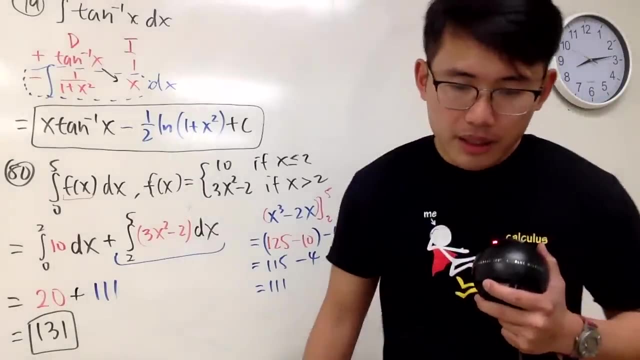 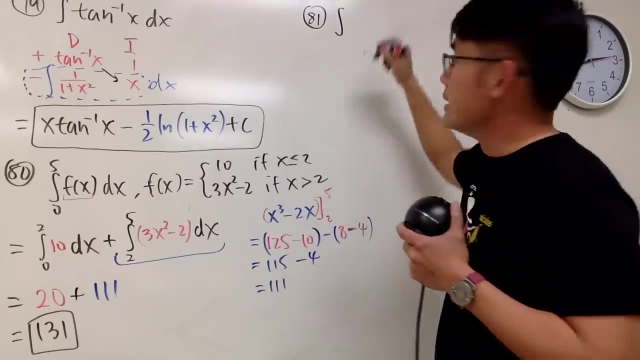 This is not absolute for your street, This is 131.. All right, So that's how you handle piecewise function in an integral right. Continue, continue, continue. An interesting one right here, Number 81,: we are integrating sine of 1 over x over x. 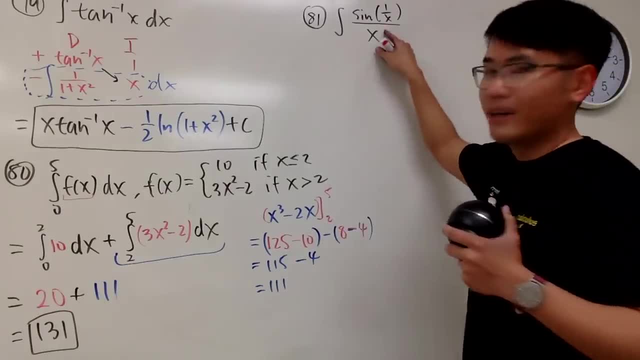 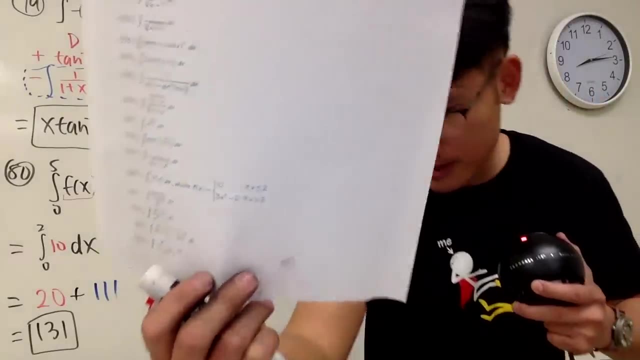 Here's the deal: If it's just x cannot do. If it's x squared, it's easy. But I want to integrate with x cubed on the bottom right. You guys can see that x cubed on the bottom right. 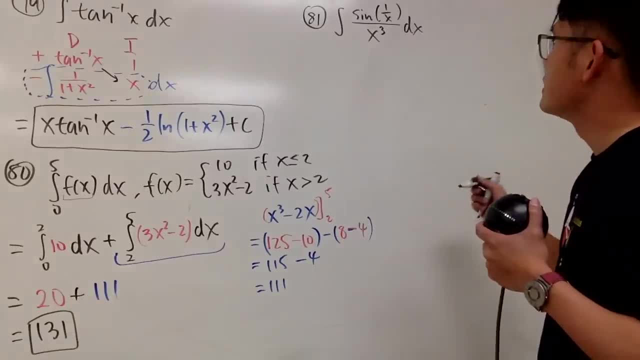 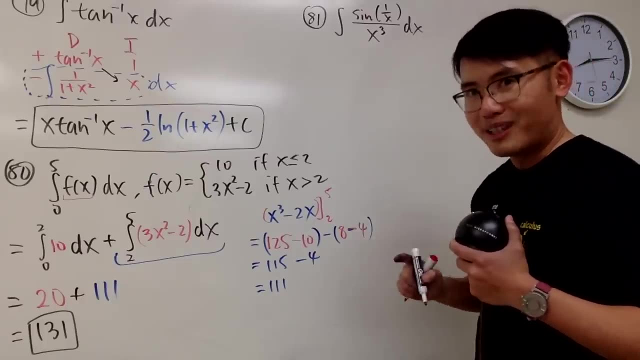 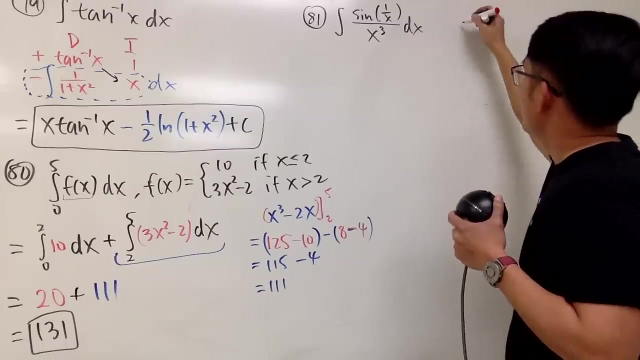 So here is the deal. Let's see All right Integration by parts, Because, as I said, if you have a tool right here, you can do it by yourself, which is actually pretty easy. So I will just try to break them apart. break them apart, okay. 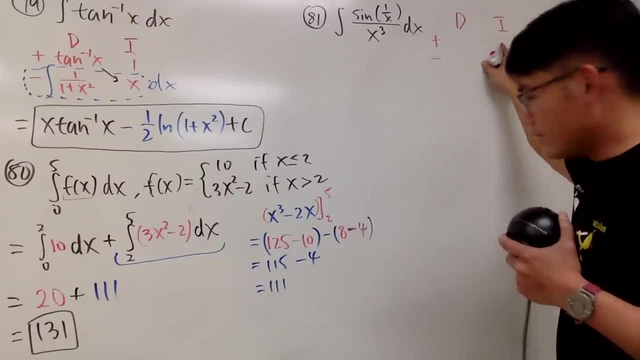 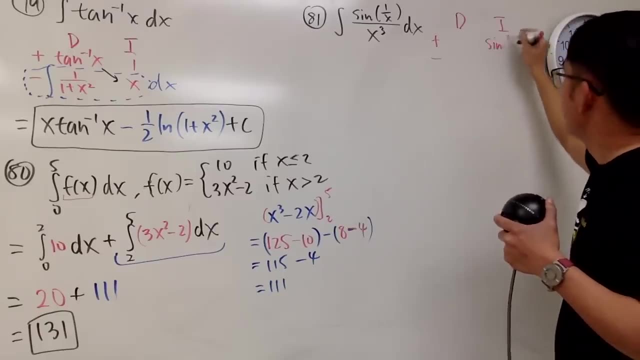 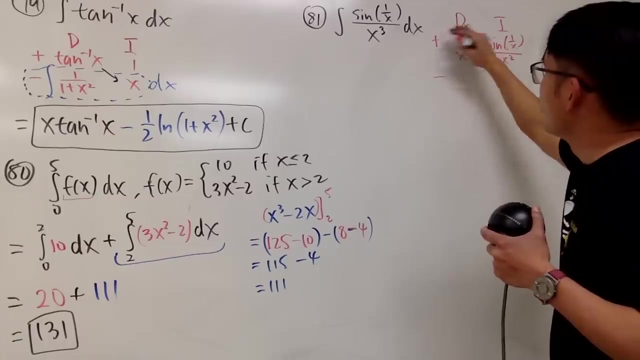 Try to break them apart First, actually. yeah, I think I should just do it right here. I will integrate this Sine with 1 over x inside over x squared in the denominator okay, And then I will differentiate 1 over x like that. 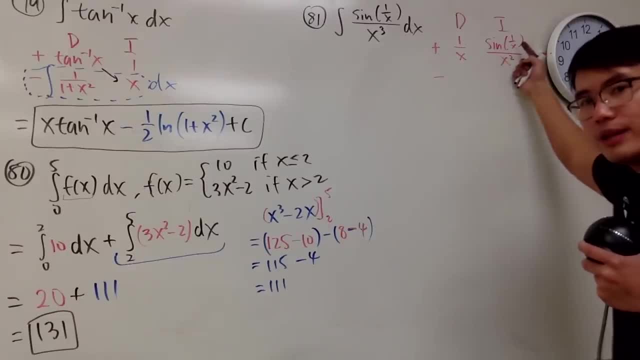 All right, Here is the deal: You let u equal to this And you have to get negative. Be careful with it. And then you can change that to the u-word. You are just integrating negative sine u, which will give you positive cosine u. 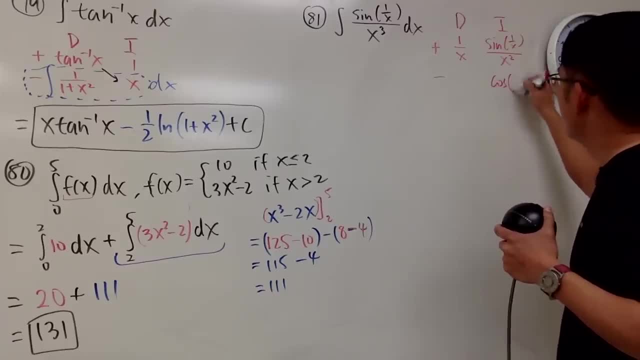 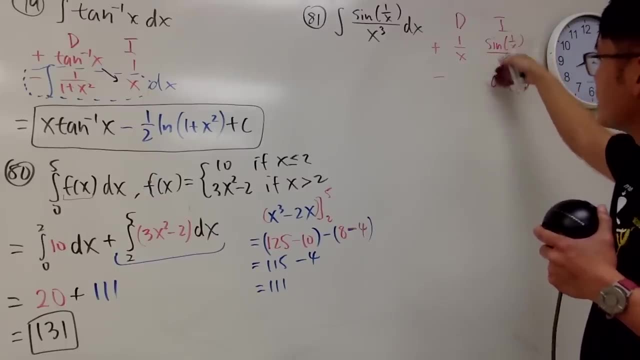 So you end up with cosine of 1 over x Again, if you differentiate this, this is going to give you sine. The inside stays the same, But the derivative of cosine is negative. And then the negative. another negative would be coming from the derivative of 1 over x. 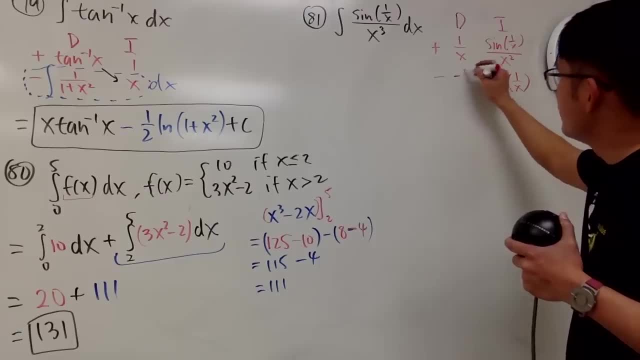 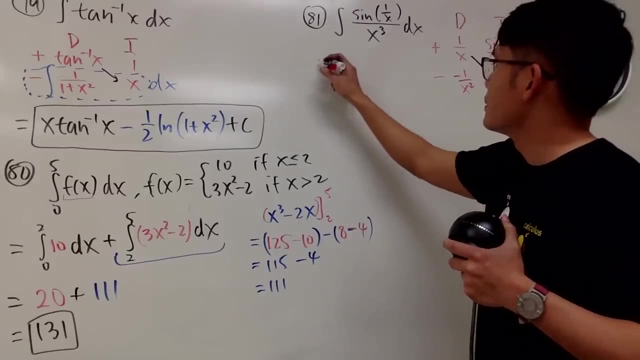 This is good. Now differentiate this. You get negative 1 over x squared. Very nice, I set up this right here, okay, So I will see. The first part of the answer is this times, that which I will just put down. 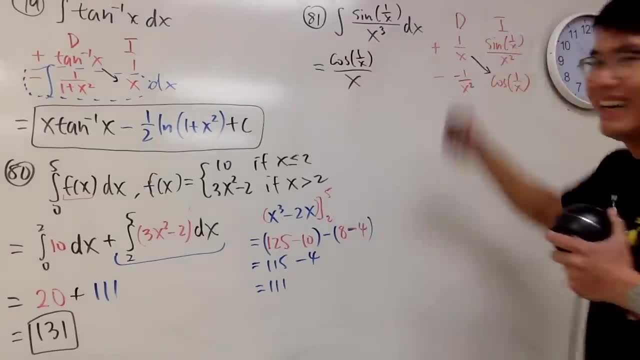 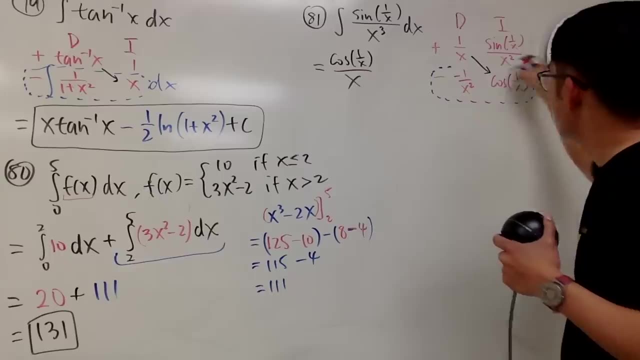 Cosine of 1 over x over x, like that. Real cool, huh. Then we will have to take care of this integral, right, We have to take care of this integral And I will just put down the result for you guys, right? 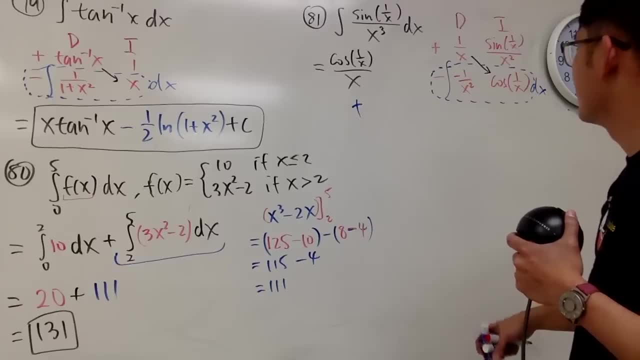 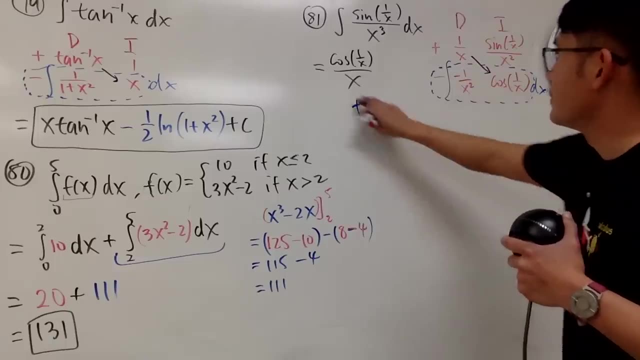 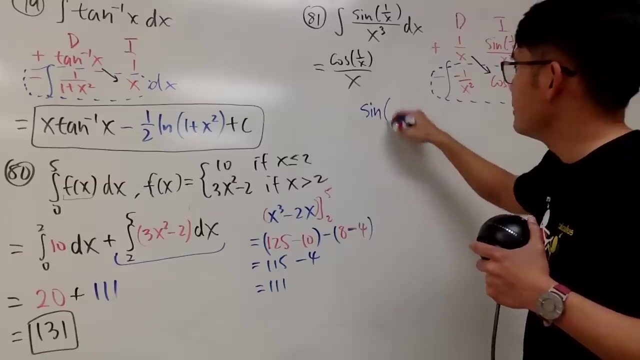 I cannot mess it up in terms of: yeah, whatever, Do another u-sub, Let u equal to this, And you get that back, which is very good. Let's see, The integral of cosine is positive sine And then the input stays the same. 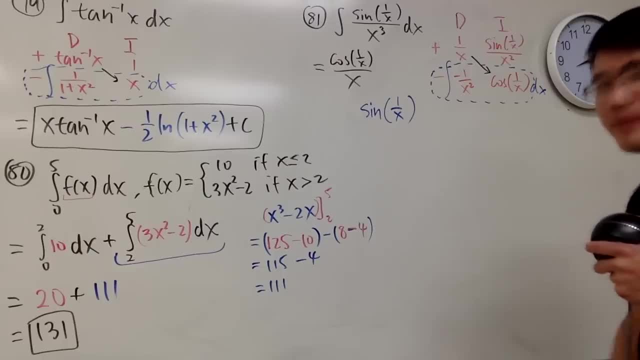 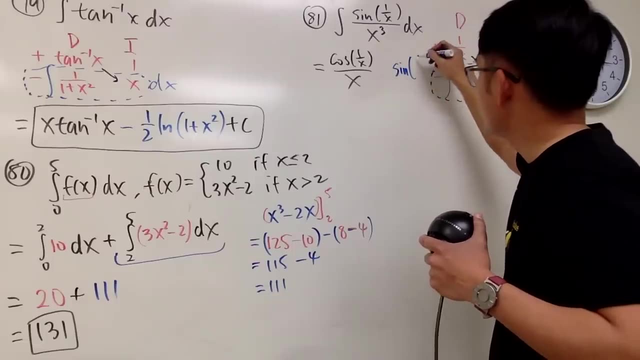 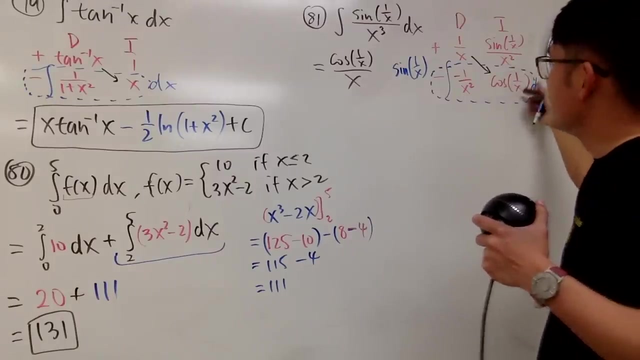 Well, let's see if it's positive or negative. Actually, I don't need to write it down below, I can actually fit in here: Positive sine of 1 over x. When I differentiate this I get: cosine Input stays the same. 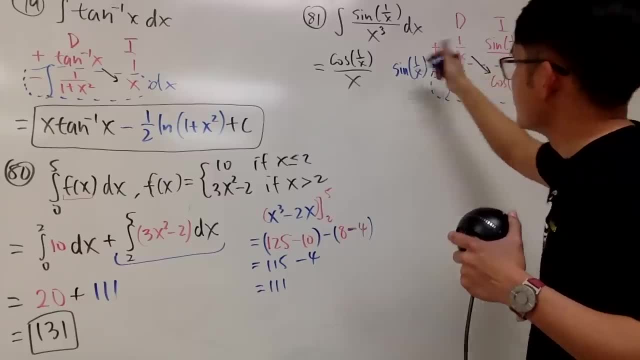 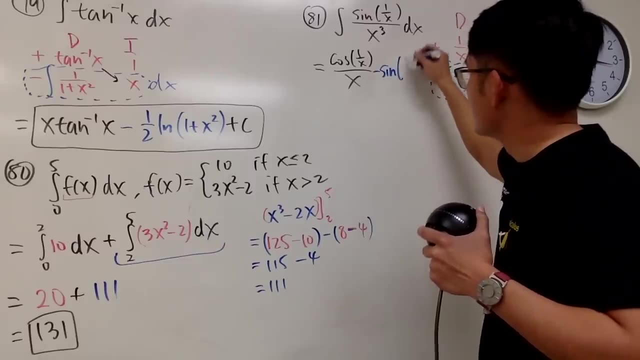 Differentiating that I get Differentiating inside because of Chandu, I get this, So it should have been a minus. So let me just write this down: Minus sine, with 1 over x inside, And we are done. 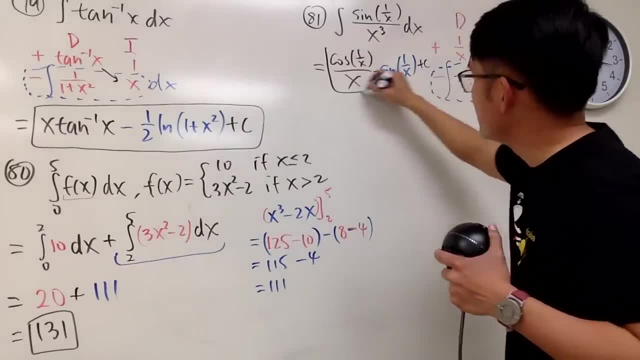 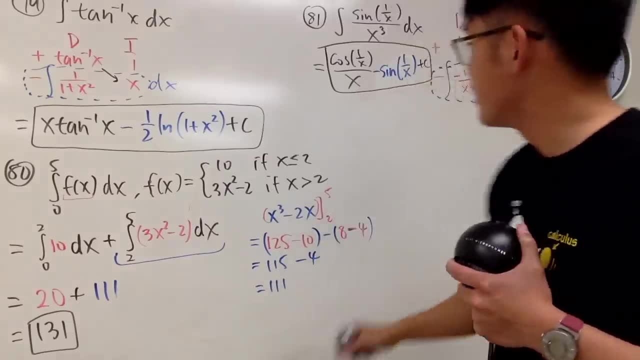 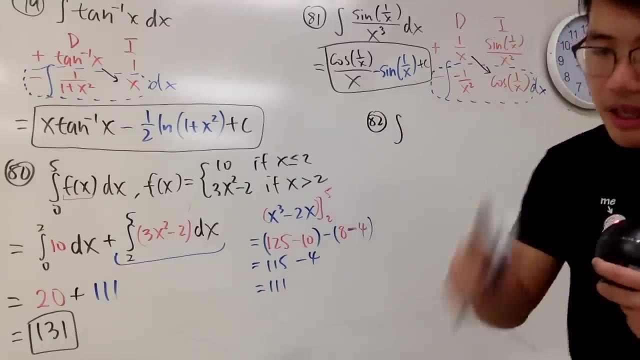 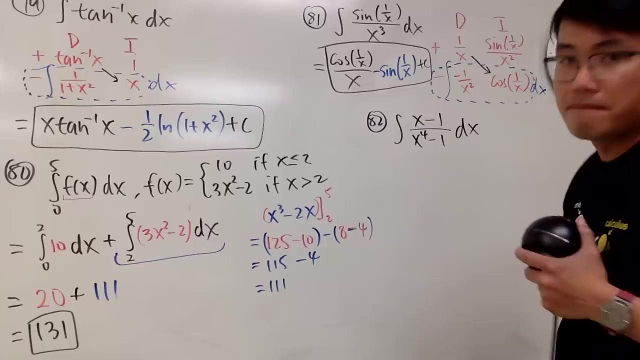 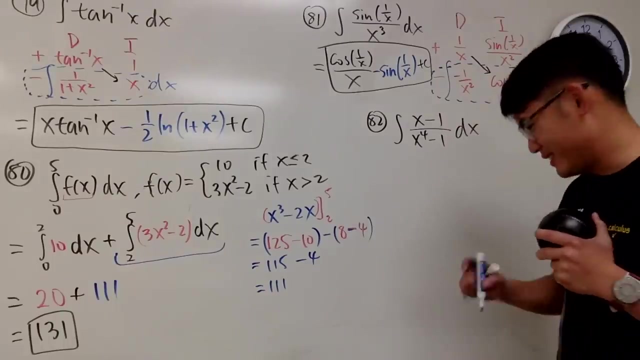 Not bad, huh. So put a plus A plus c, Be happy. Good Number 82. This is, Let's see, 82.. Integral of x minus 1 over x to the fourth power minus 1.. We can cancel something else. 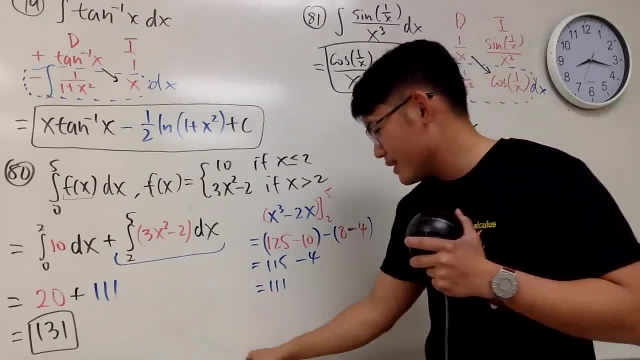 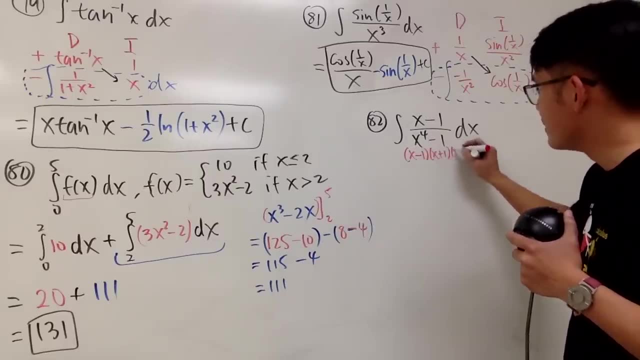 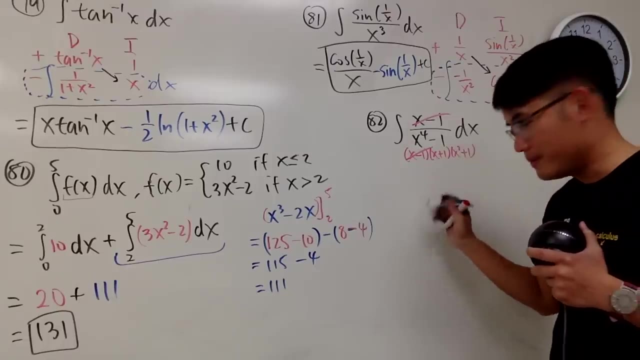 So it's not that bad, Don't worry. Right here, Whew, Right here. this is the same x minus 1 times x plus 1 times x squared plus 1.. And then cancel this out. So you can see that this right here, we can actually just do the partial fractions again. 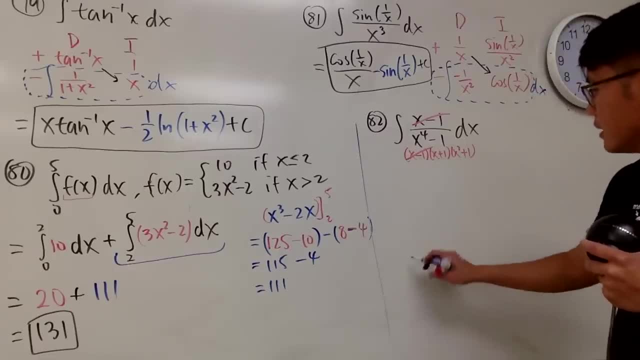 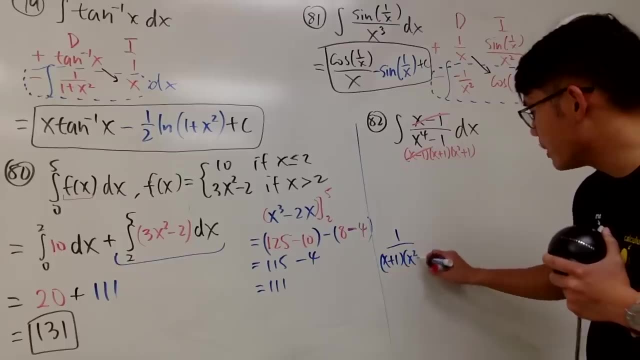 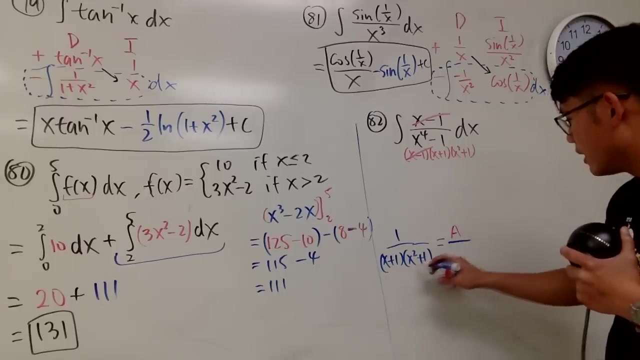 So let me just make this note right here for you guys. So for the partial fraction I need 1 over x plus 1 times x squared plus 1.. And I will have to set this up to be a over x plus 1 and then plus. 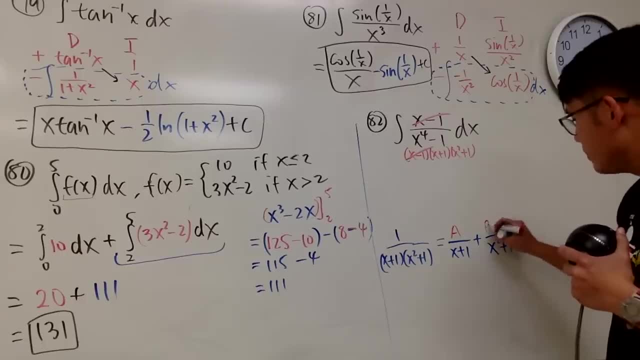 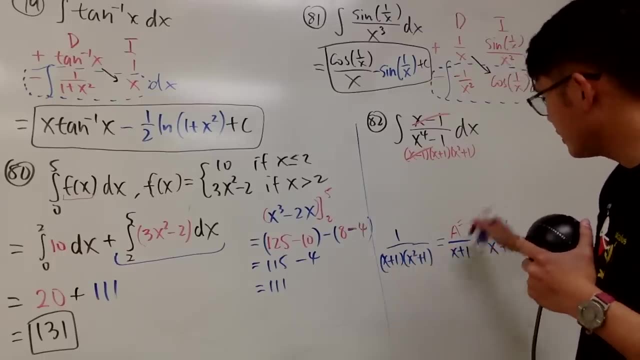 This is going to be an irreducible quadratic, So I will need bx plus c, like that. Okay, What is a? I need to plug in negative 1 here, So you get 1 half. This is nice, Thank God. 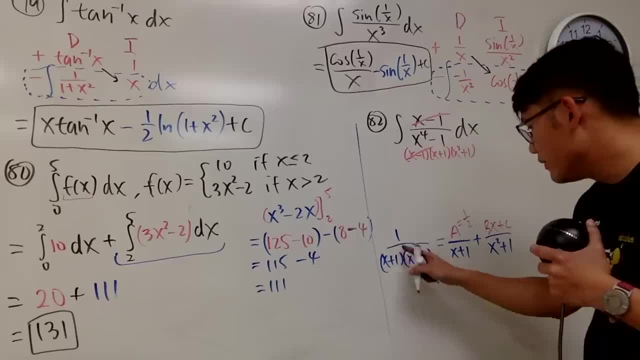 Now use 0. If I get 0, if I plug in 0 into all the x, I get 1.. Okay, Let's say use x equals 0. Then I get 1. And this is going to be 1 half. 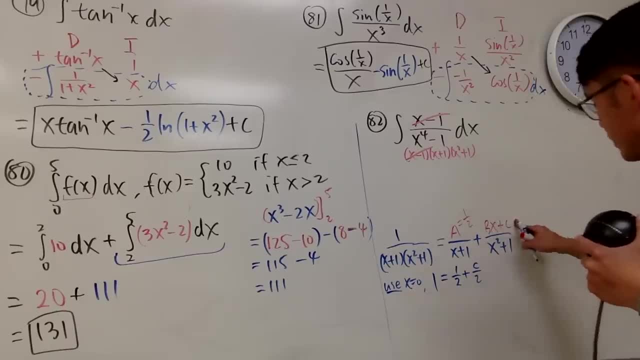 This is 0. So I have c over 2.. Am I right? C over No, c over 1. Which is just, of course, c. Then c will be 1 half. Yeah, That's very good. 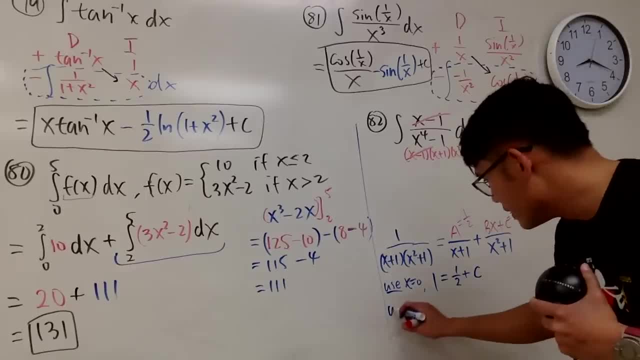 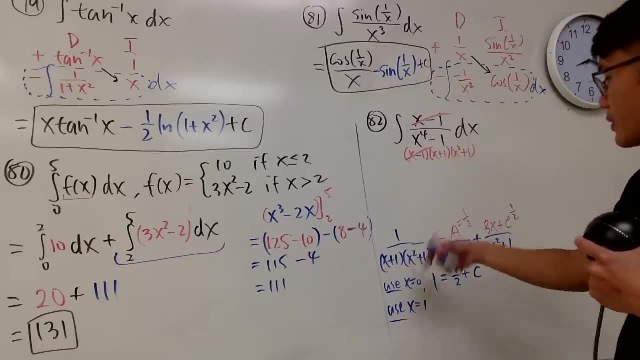 Very good, Very good. Now use: x equals positive 1. Here you get 2., 2. So it's 4.. Okay, So you get 1 over 4 on the bottom, And then, if you're plugging 1 in here, you get 1 over 2.. 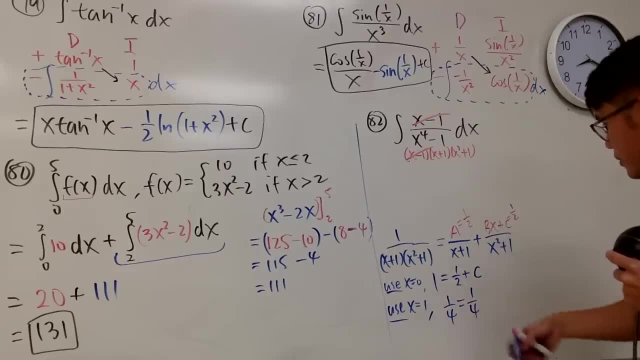 Over 2.. So it's 1 over 4. again, Thank God it will be 0.. And then plus b times 1 is b over 2.. And then plus 1 over 2 over 2.. So it's 1 over 4.. 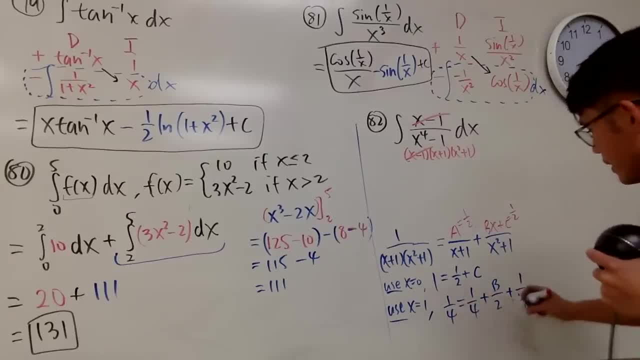 Like that. Check this out: This is 0. And I need b to be negative 1 half, Am I right? If I have negative 1 half, this will be 0 as well, And everybody will be 0. Yeah. 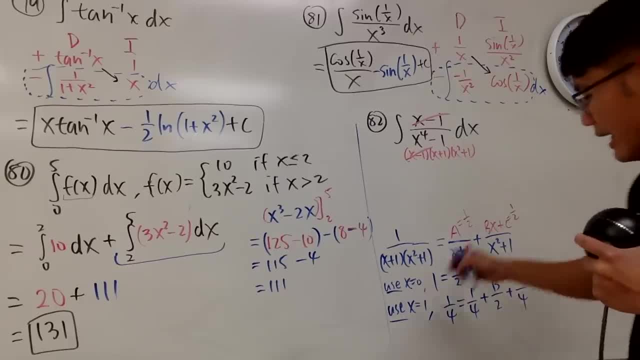 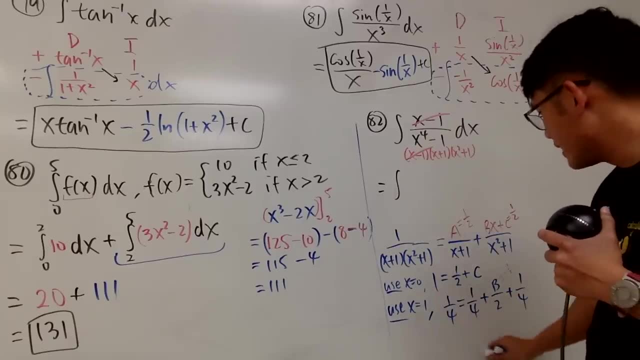 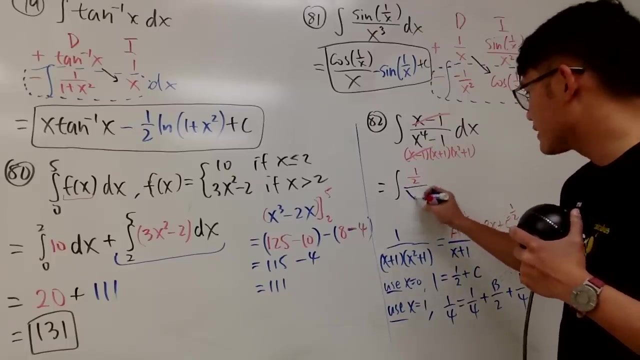 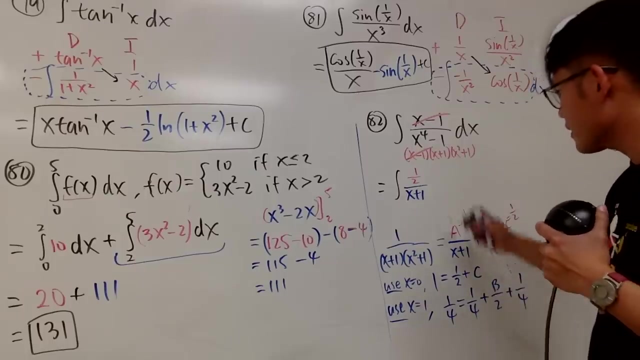 Good. So here is the deal. I will have to integrate this guy as first part, which is 1 half over x plus 1.. Next it's the b, And then I will put this down right here. I'll close the integral. 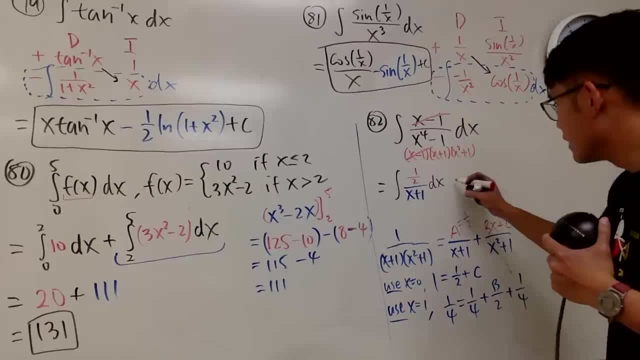 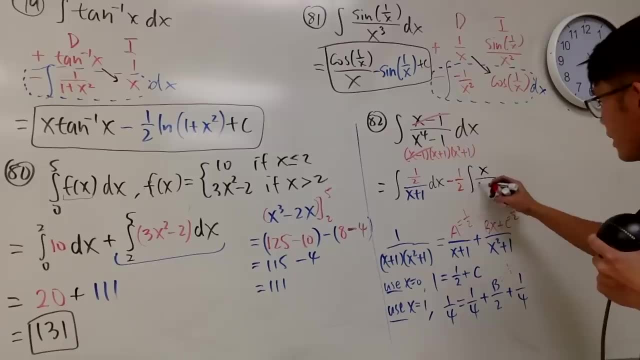 Okay, b is negative 1 half, So let me write it down in the front: Negative 1 half. And then I have the integral sign with the x on the top over x squared plus 1.. Close that Okay. 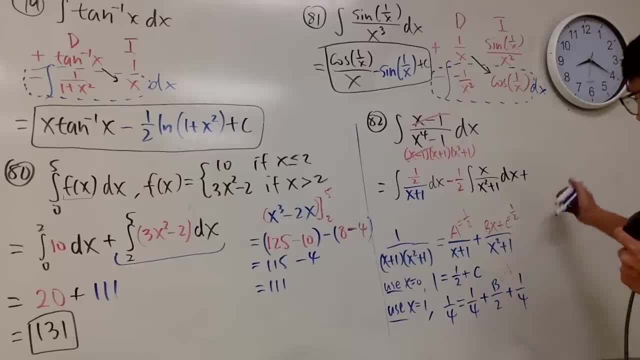 And then c is 1 half. So I put down plus And we have the 1 half And then we have the x squared plus 1.. 1 over x squared plus 1 dx. Like this Look: 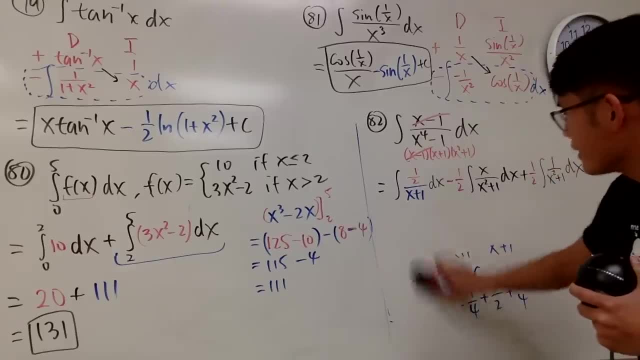 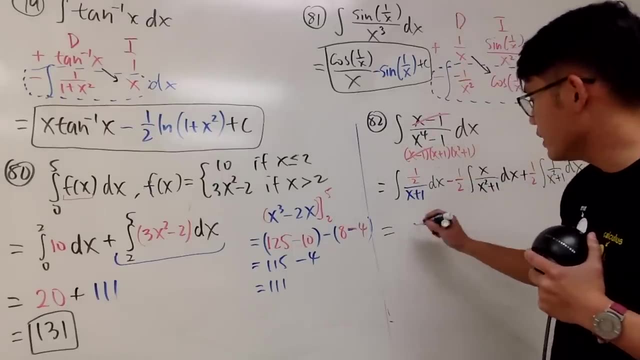 Yes, So of course we can just now integrate term by term. It's not that bad. Check this out. Here is the deal, Right here. the first one is going to give us 1 half. 1 half is still 1 half here. 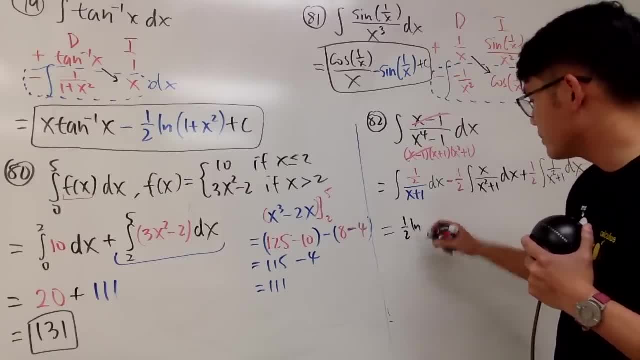 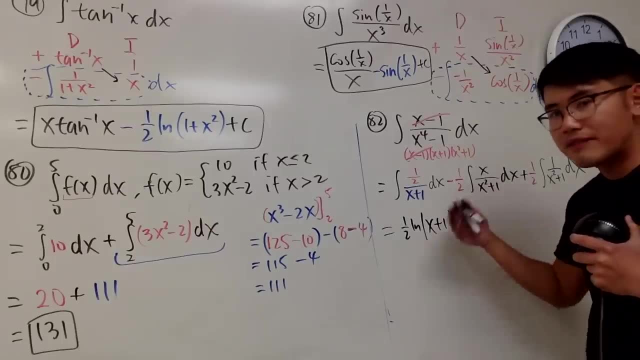 So I just put this down in black right now: 1 half natural log of f to the power of x plus 1.. Next, do it carefully, yo. When you do this, you have the extra factor of 1 over 2.. 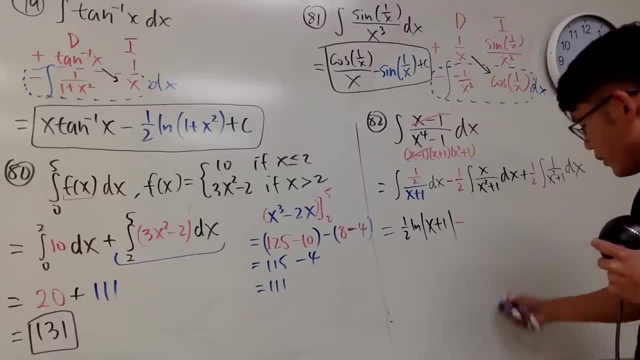 So you multiply by that, You end up with negative 1 over 4.. So I will actually make this in blue right, Because you have to put 2 and then 2 pretty much, And then the derivative is 2x. 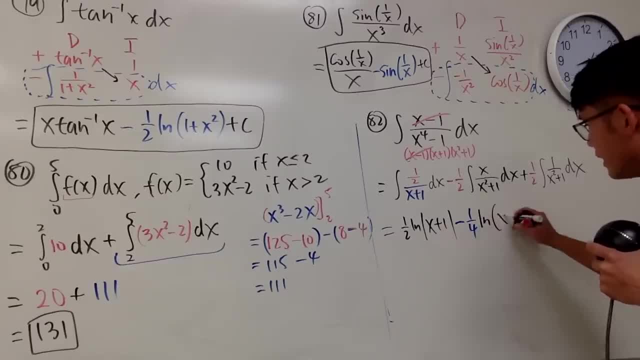 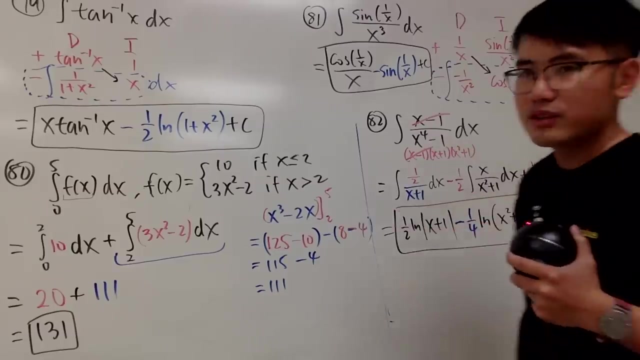 And then you have ln parentheses, x squared plus 1. Here you get inverse tangent of x. All done. Put a plus c, Like that, Done. Partial fractions sometimes aren't that bad, So that is the deal, Right. 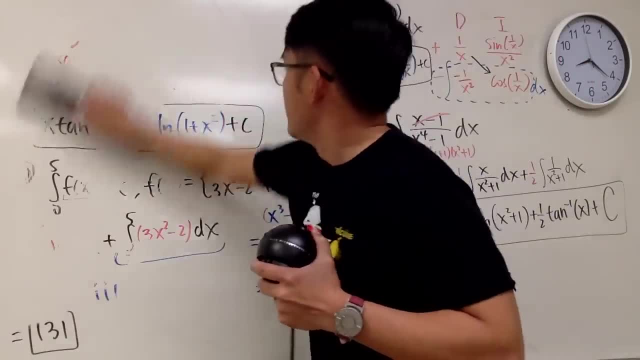 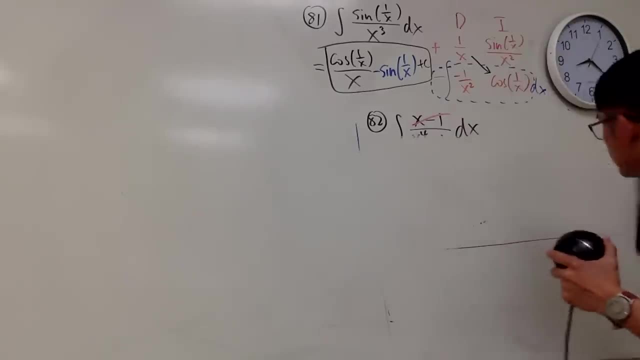 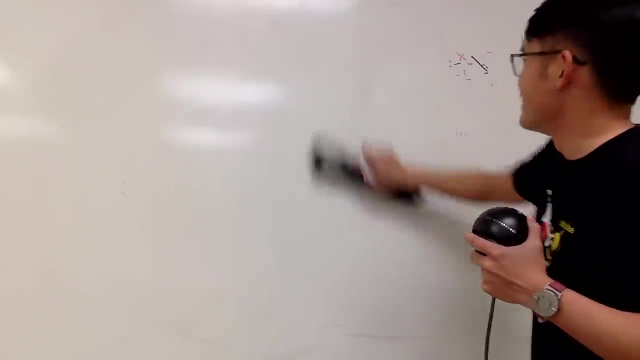 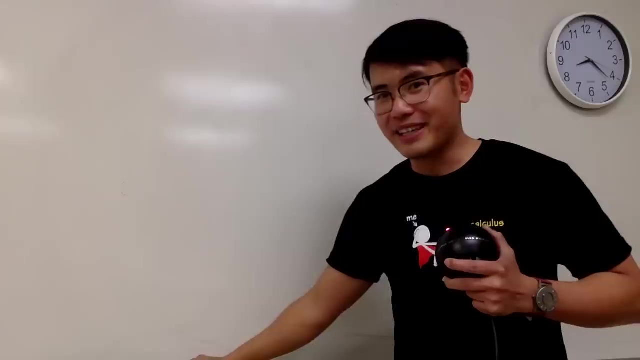 That is the deal, All right. I would really like to see if there's anybody else who would like to do like 100 integrals in one take, Right In one take, Not like just like over several days. 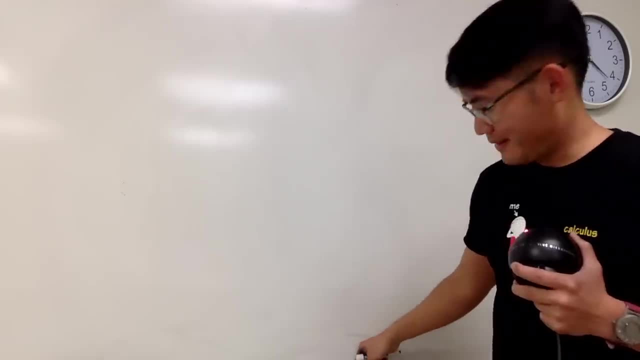 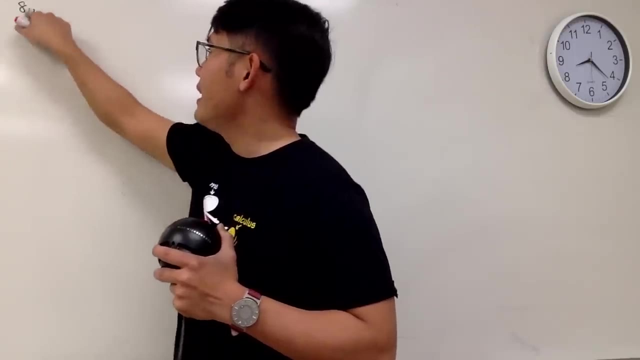 I want to see how many people would like to do that. I don't know, man. Now 83. Almost done, Almost done. This is like when I run marathons and I reach like the 21st mile right. 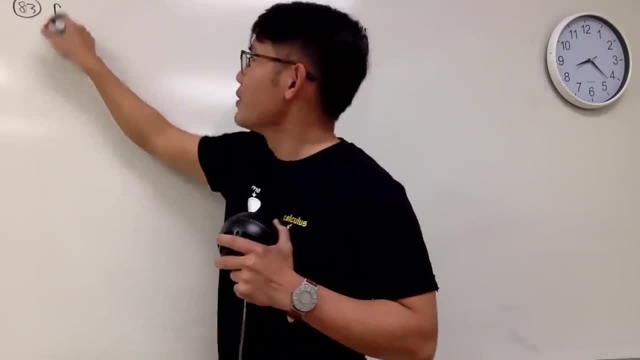 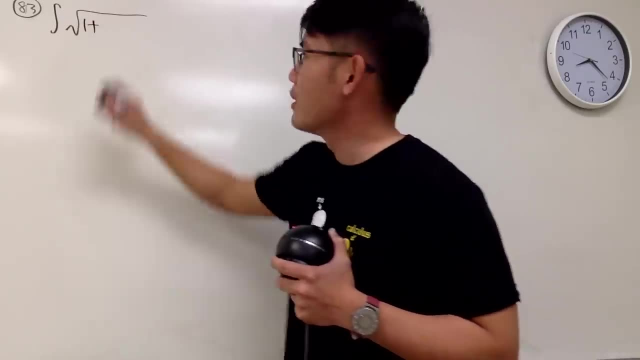 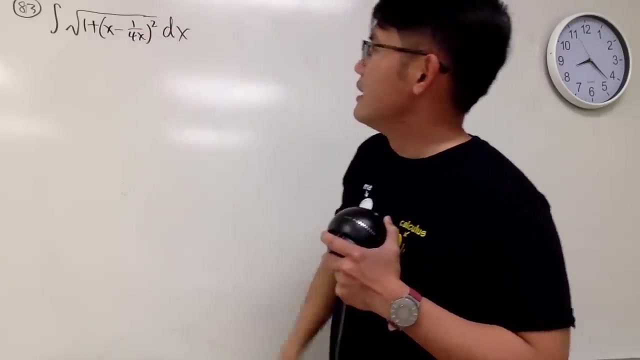 Mile 21.. Almost done, Almost done. And then I start to get emotional. But it's still tough because my body is tired And I still have like five more miles to go, All those things. Anyway, we have this right here. 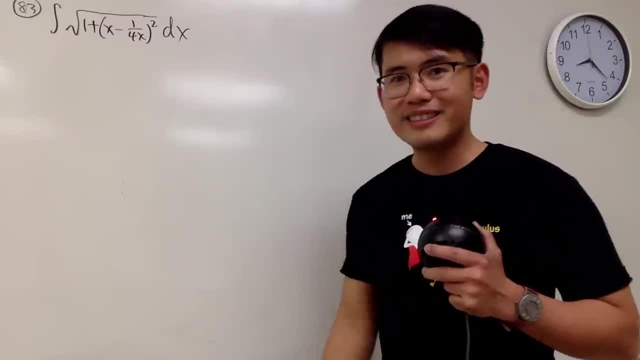 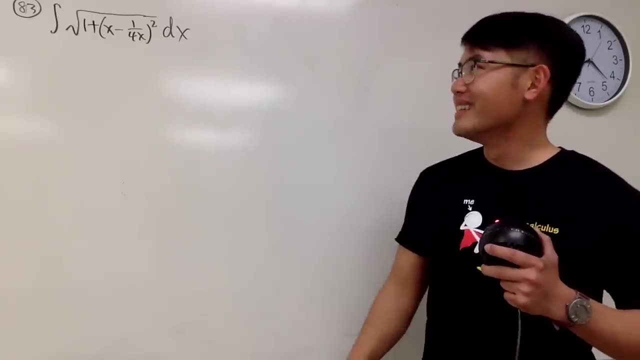 Huh, Do you guys recognize where you can possibly end up with this kind of integral? If so, please comment down below and let me know what situation you have to deal with this integral. But here Now I'll wait for your comments though. 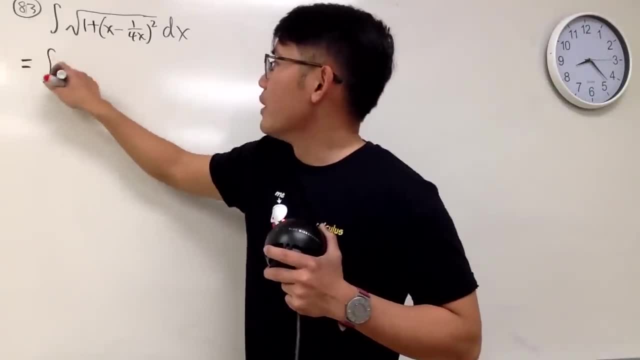 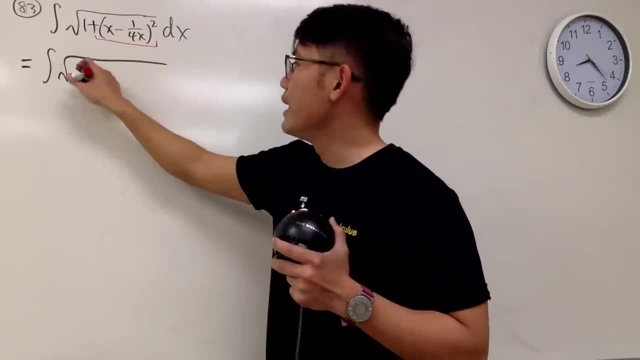 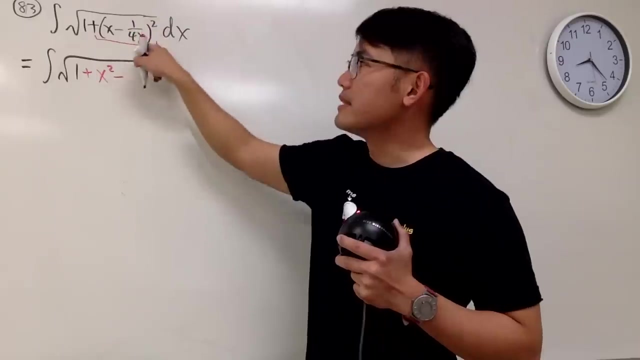 I will just show you guys how to integrate this. This is the integral Square root. 1 is still 1.. But this part you are going to multiply it out And if you do that you get plus x squared and minus 2 times x times this. 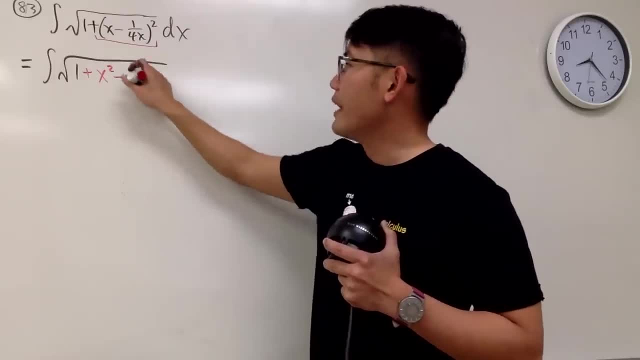 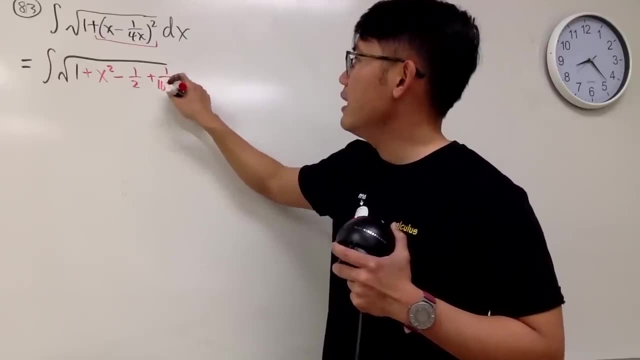 x and x cancel 2 and 4, you have the 1 half right here. It's a negative. And then you have to square that which is plus 1 over 16x. squared Like that, Right. And then you have the dx, like this: 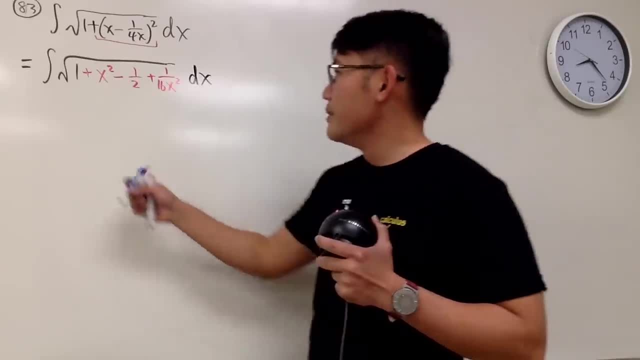 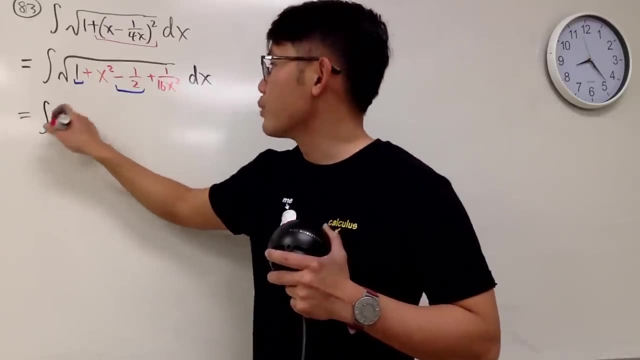 And this is actually not that bad. It's actually kind of cool Because you see that we have the 1 and negative 1 half. Of course that will be positive 1 half And you end up with the integral of the square root. 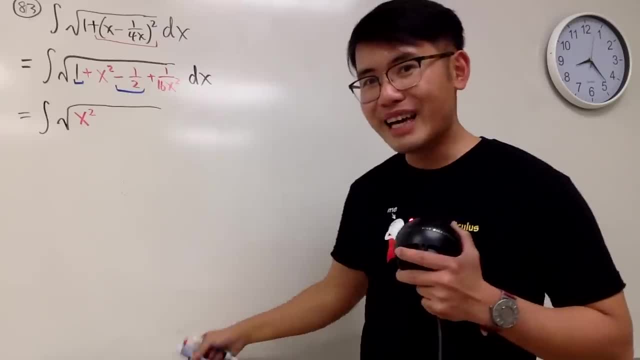 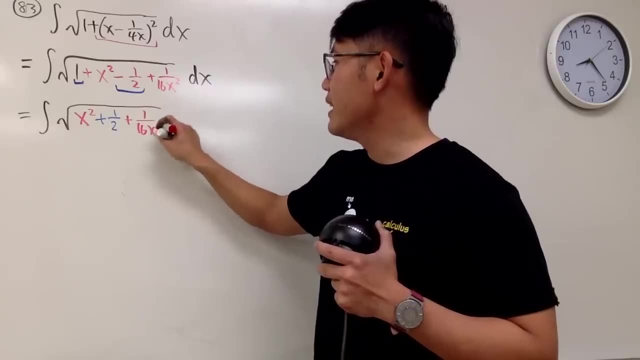 Inside you have x squared plus 1 half instead, Plus 1 half instead, And then you have plus 1 over 16x squared, And then you have the dx. You have three crazy things inside of the square root. 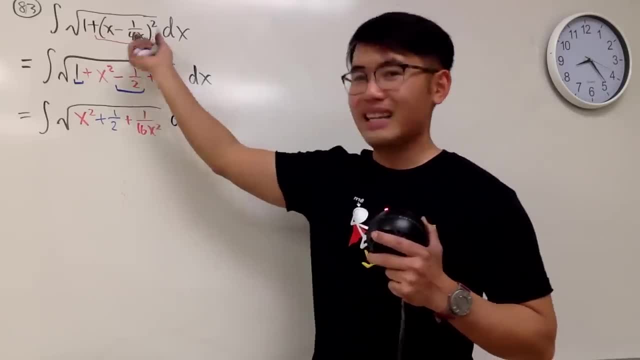 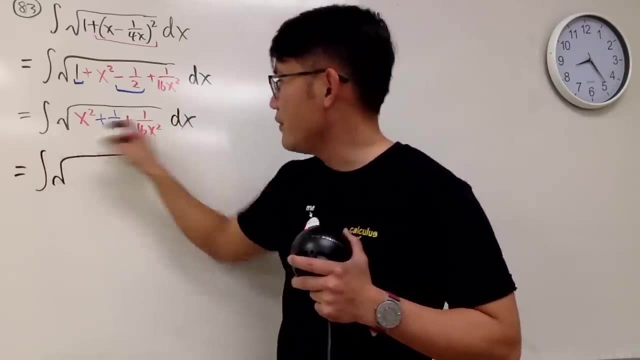 But let me tell you, This is the perfect square, Just like that. But instead of the minus you have plus. So here's the deal. This is the integral square root Inside here. if you factor it or whatever, you end up with x plus 1 over 4x. 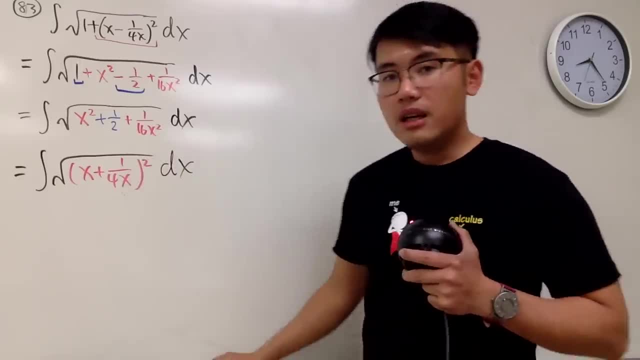 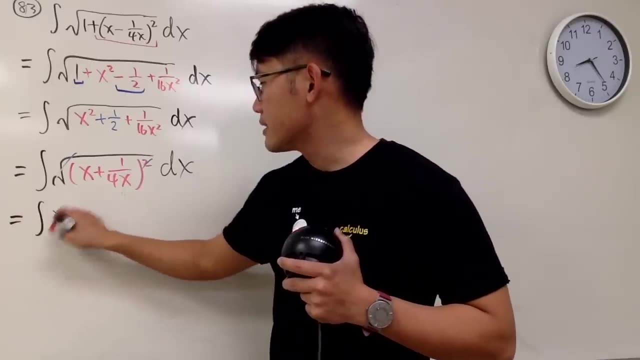 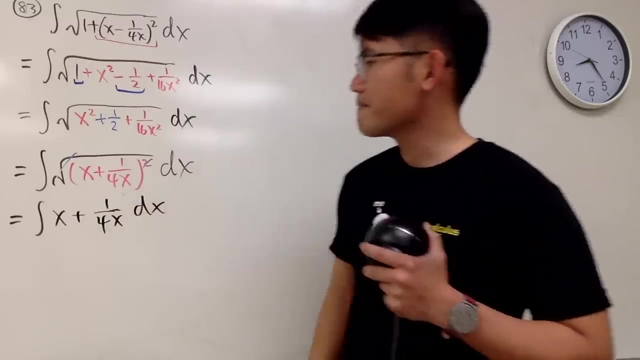 And then square dx. Again, we're just focusing on integration, So you can cancel this out. So you are just integrating x plus 1 over 4x, Like that, Very nice. Huh, We're not done yet. 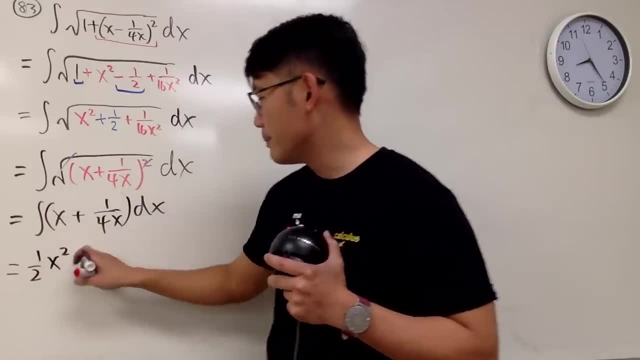 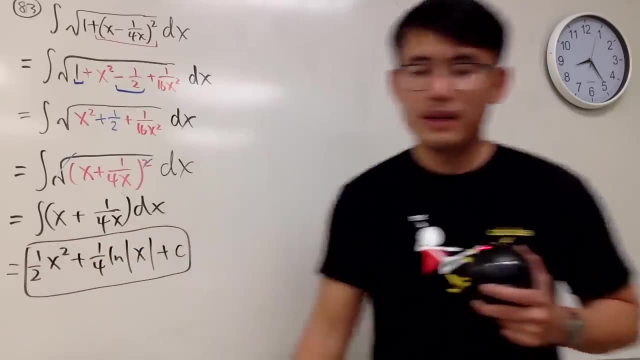 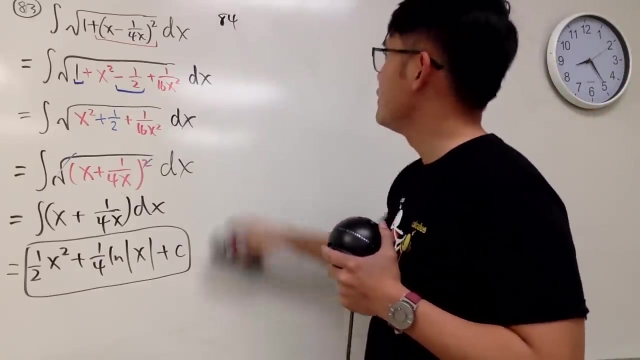 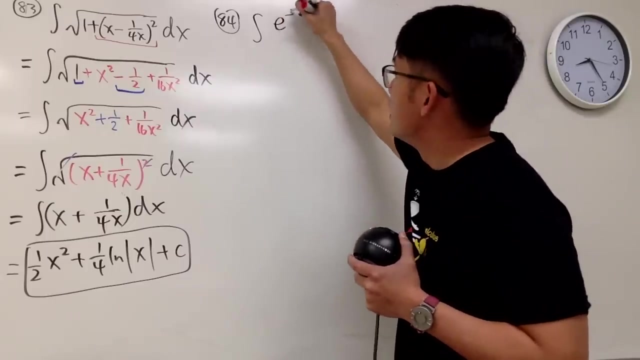 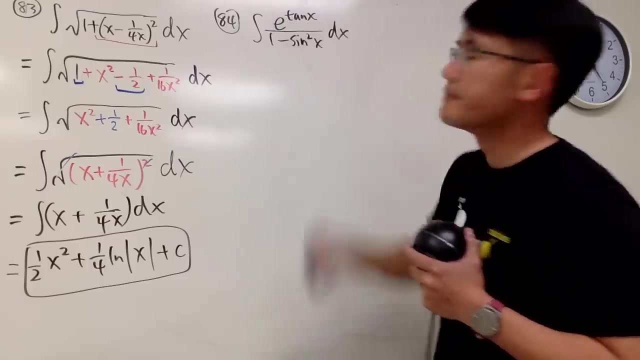 I know, But this is easy: 1 half x squared plus 1 over 4, natural log absolute value of x, Like that, Okay, All right. Number 84.. Number 84.. We have the integral of e to the tangent x over 1, minus sine squared x dx. 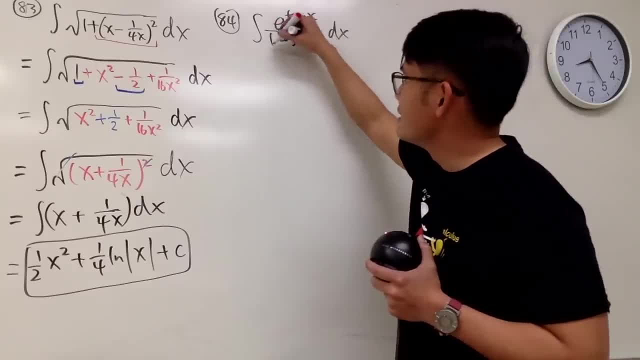 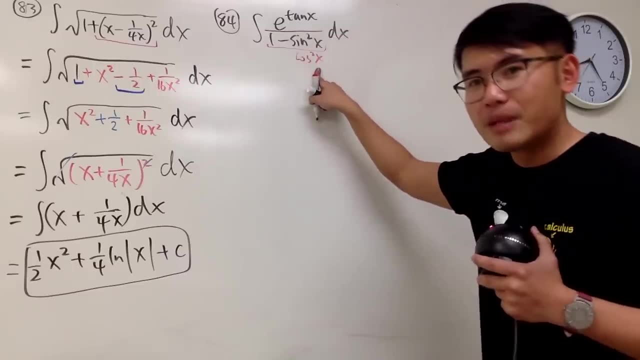 This right here is not bad at all, Because we have seen this a lot. What's this? Yes, It's just cosine squared. And when you have cosine squared in the denominator, what's that? Yes, That's just secant squared. 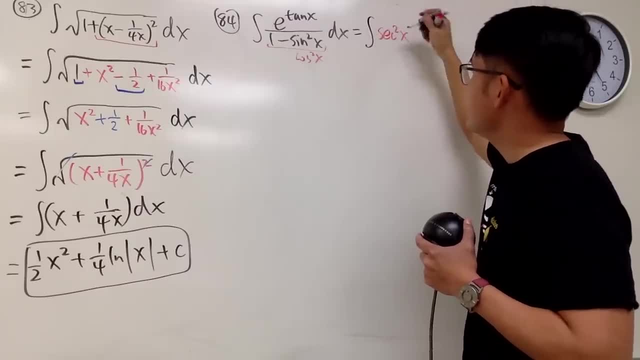 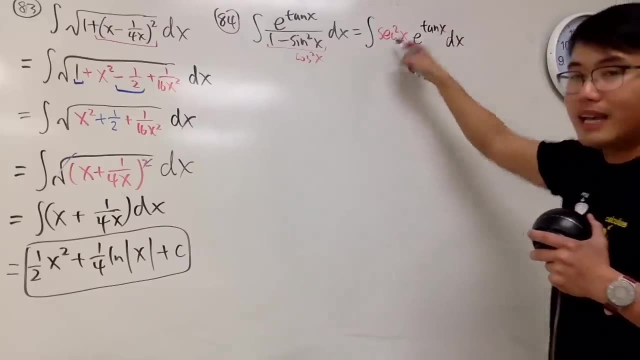 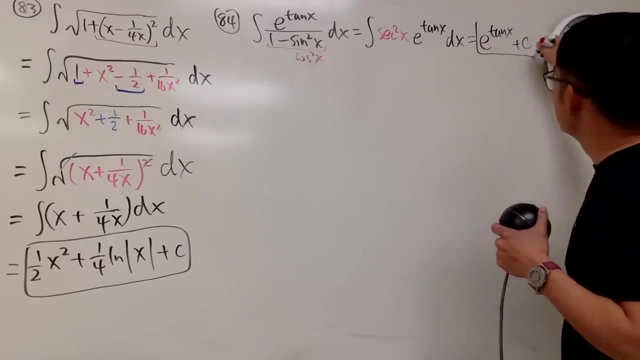 You can just say: this is the integral of secant squared x, And then you have e to the tangent x, dx, And look, The derivative of tangent x is that? So you know? the answer is just e to the tangent x, And you get that for plus c. 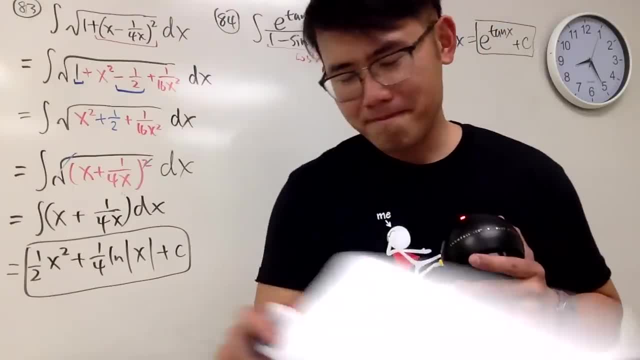 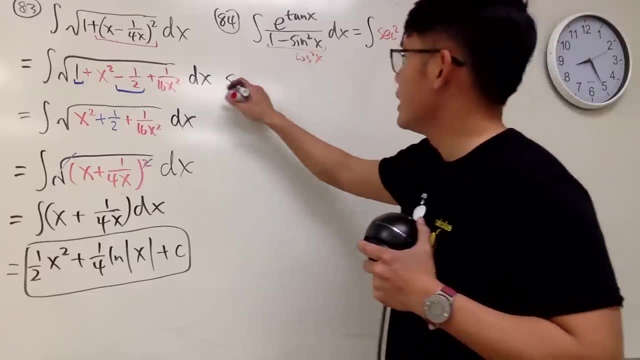 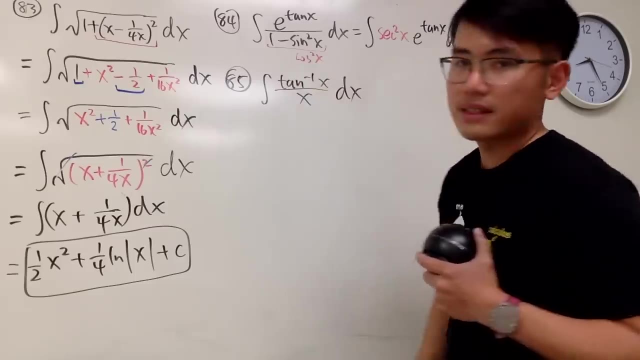 Very nice, Ha ha. Okay, Last page, Last page, Number 85.. Okay, So number 85.. Integral of the inverse tangent, again, But this time divided by x, dx. All right, So let me show you guys how to do it. 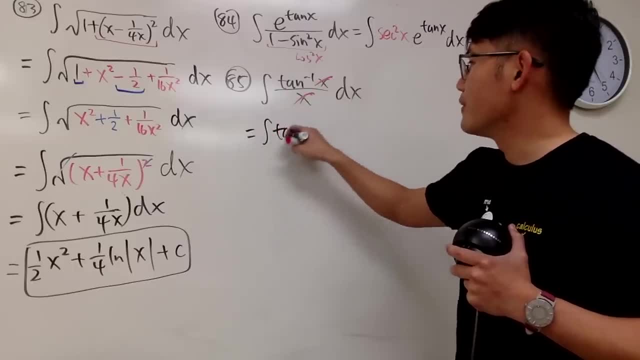 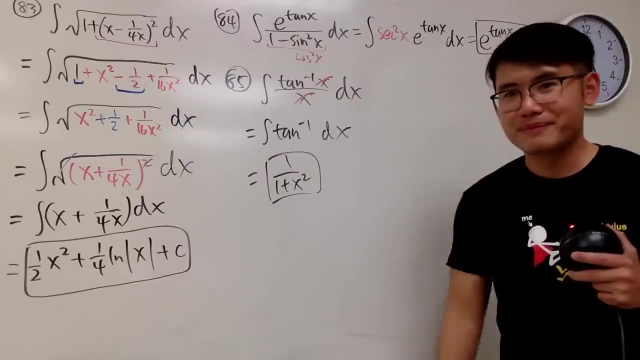 I see x and x, So let's cancel this out. So this is just integral of tangent like this: And then we know the answer is just 1 over 1 plus x squared. Okay, Done, Just kidding, Don't be mad at me. 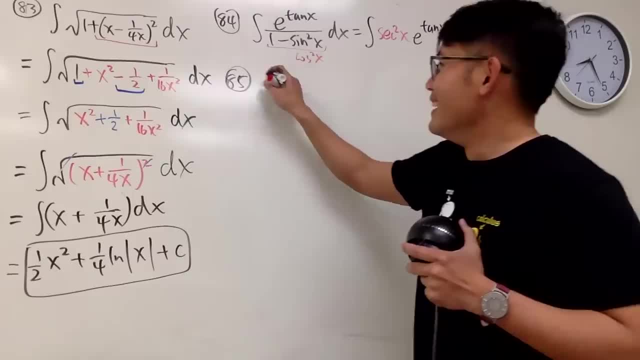 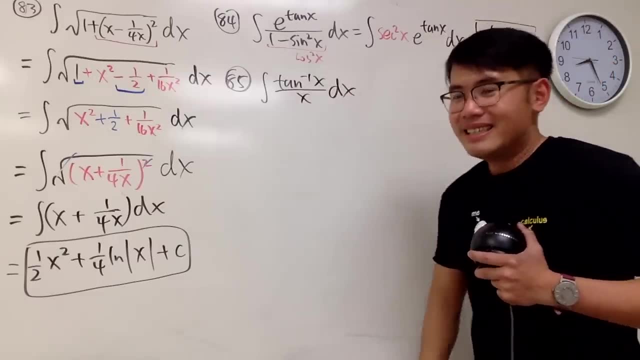 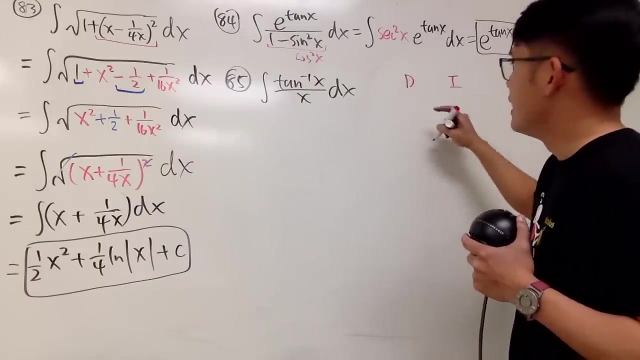 It was just a joke. Integral of tangent negative 1 right here, x over x. Of course we cannot do that. Integration by parts. All right, Let me put this down on the side D and then the i. I am going to integrate this. 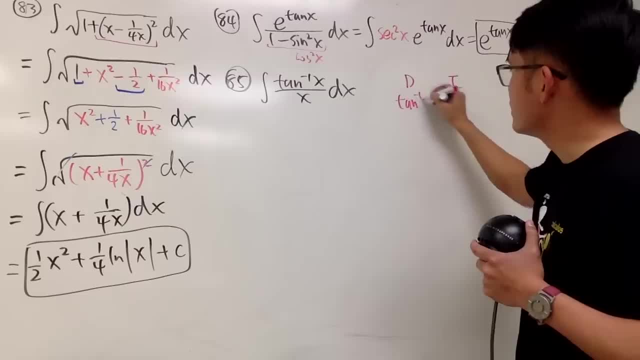 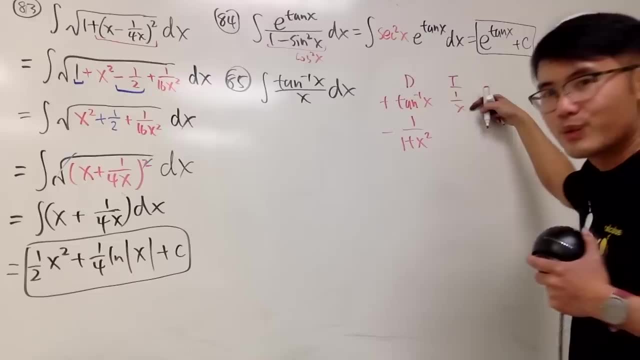 1 over x And I'll differentiate inverse tangent of x. When I do that, I get 1 over 1 plus x squared. When I integrate this, What do I get? Okay, Hold on, Wait, I copied it wrong. 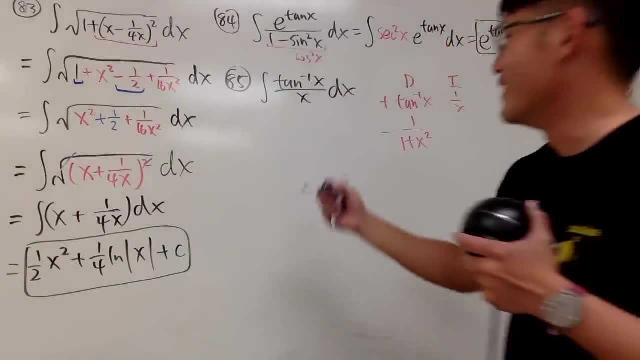 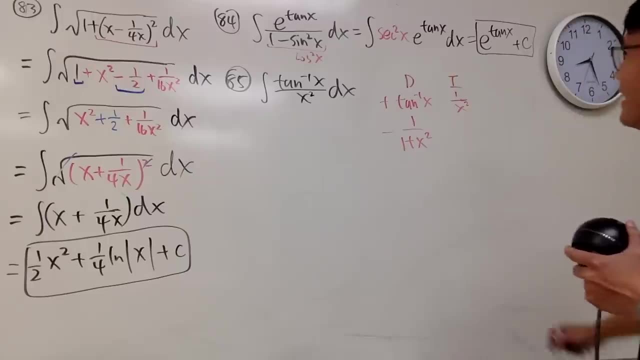 I copied it wrong. No, no, no, no, no, no. I copied this equation wrong. It should be 1 over x squared. I'm sorry, I shouldn't be making that joke with you guys. I thought I was going to get like all mixed up. 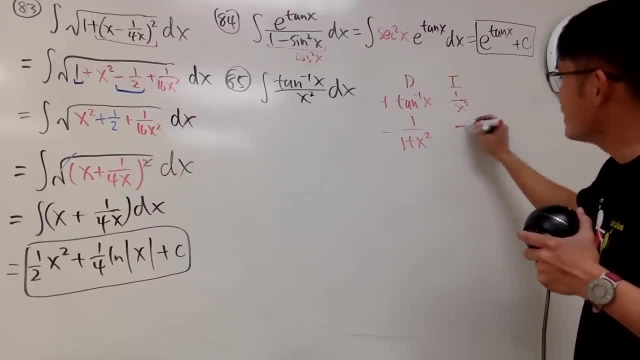 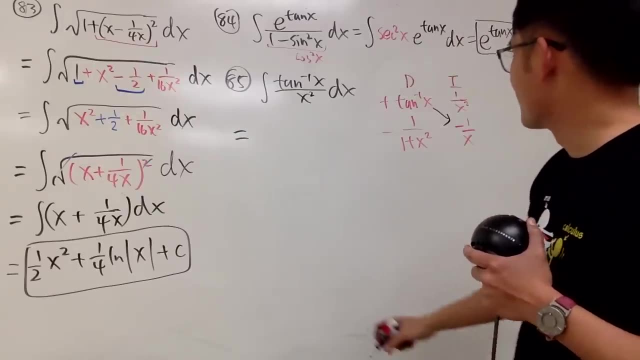 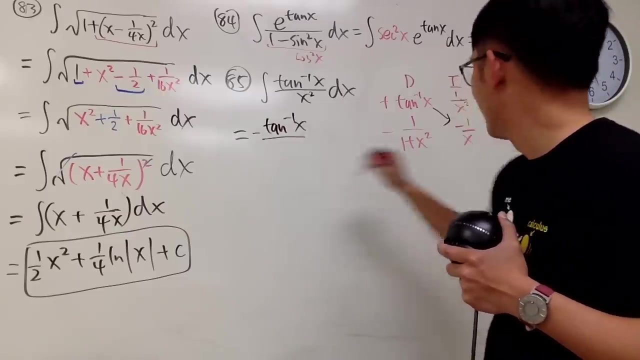 Anyway, here we go. Integrate this. You get negative 1 over x. Okay, All right. So here we go This times this The first part of the answer, And we get- Let me just put down- negative inverse tangent of x over x. 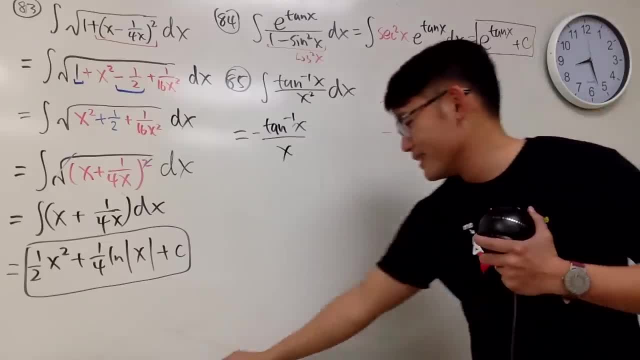 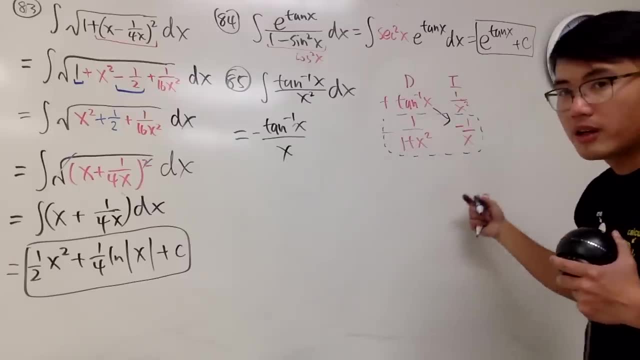 Again, do not cancel the x, Seriously don't do that. And then, of course, here we are going to do this part again, This part We have positive from here. It's a positive integral, because we have negative times, negative. 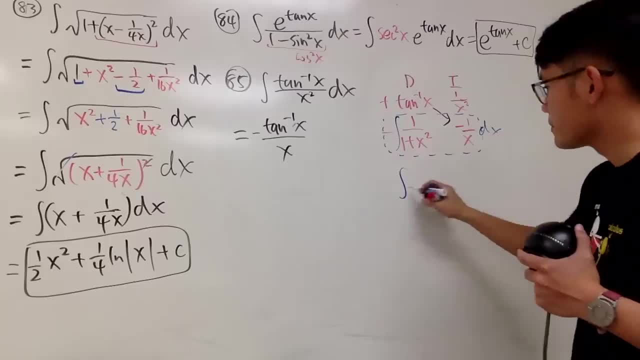 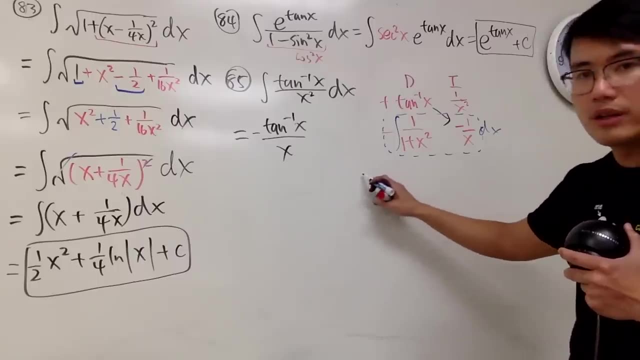 Okay, So let's just focus on the integral of. Let's see if I can. I don't know, Let me see. Let me just do it right here. I should be able to Integral And it's positive Okay. 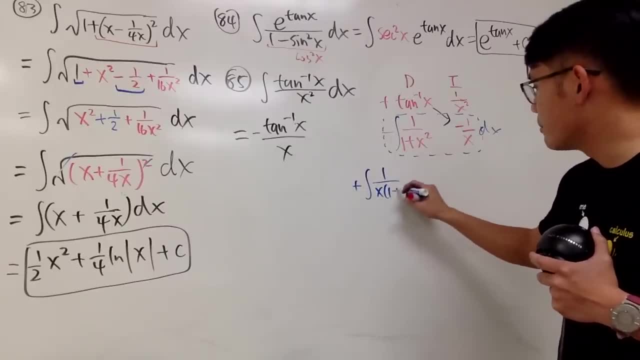 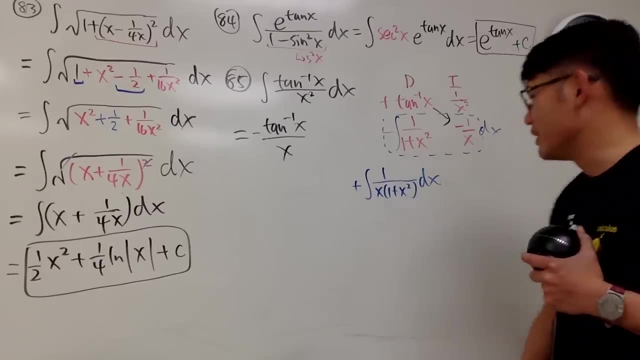 It's positive. So we have to do the 1 over x times 1 plus x squared dx like this. It's not that bad actually. You don't need to do partial fractions for this. You don't have to do partial fractions for this. 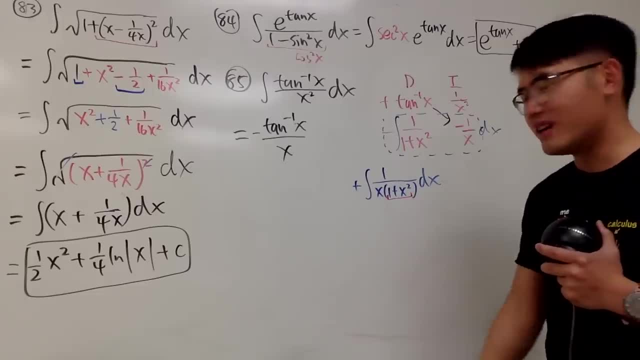 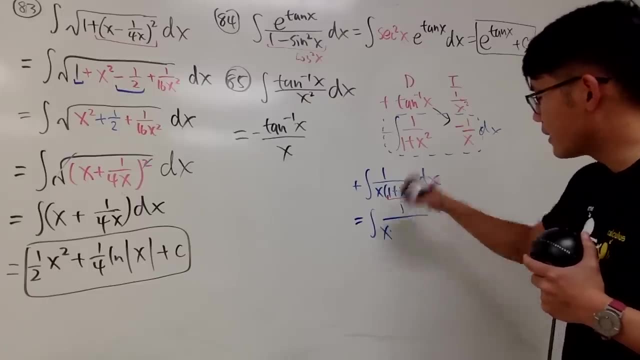 Because right here you can factor out x squared again. So you will see this: right here It's the integral of 1 over x times. Let's factor out the x squared And, with that said, you end up with x to the negative, 2 plus 1.. 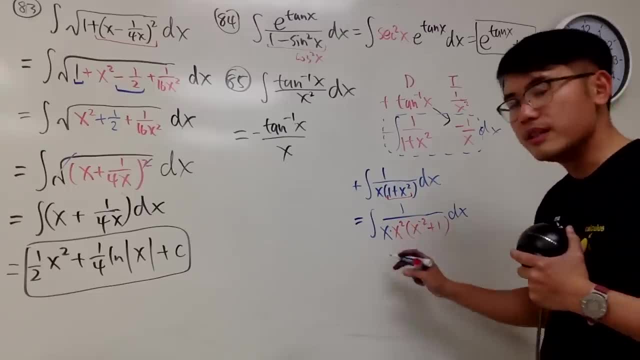 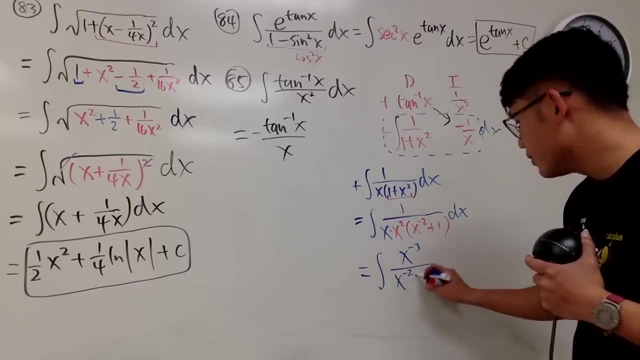 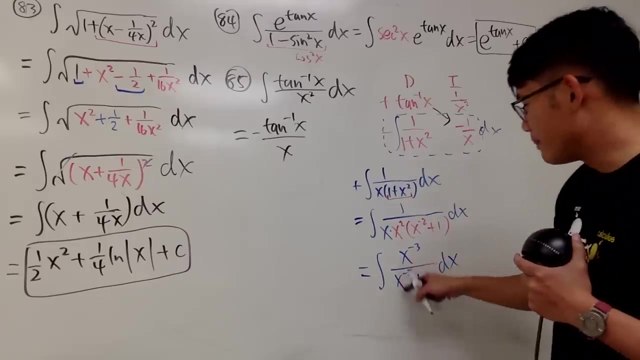 Well, well, This right here is x to the third power in the denominator, You get the integral of x to the negative 3 on the top, over x to the negative 2 plus 1 dx. Very good, isn't it? Well, the bottom, the derivative of the bottom, is almost the same as top. 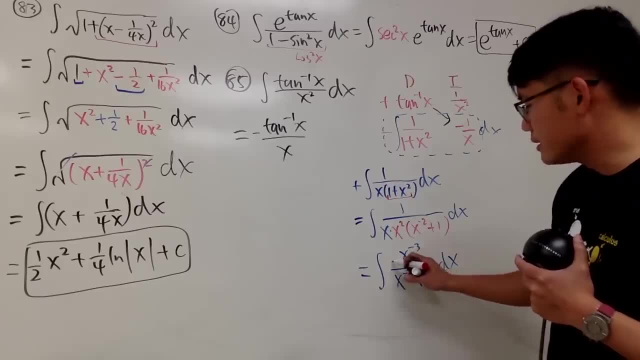 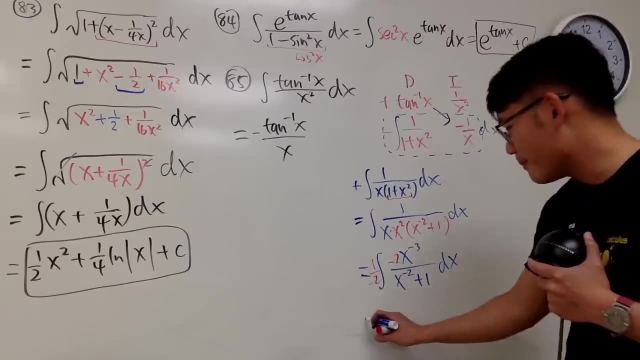 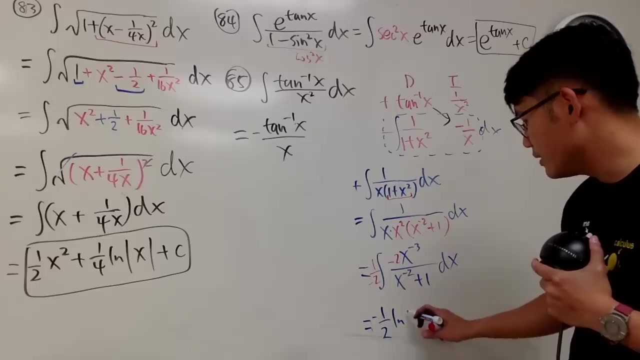 The derivative of x squared. the derivative of x to the negative 2 is negative 2x to the negative third power. So I will have to divide it by that. So you end up nicely. equal to 1 over x squared. Negative 1 over 2: ln. 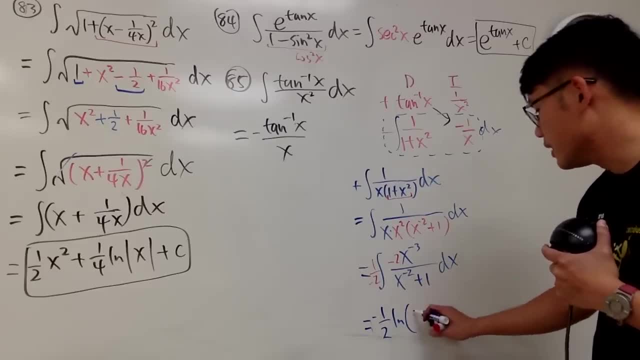 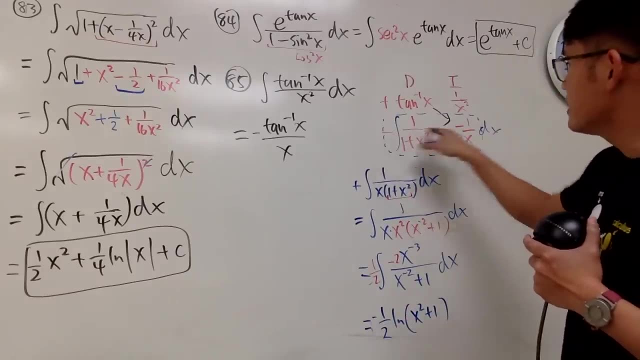 And this is actually always positive. So I put parentheses x squared plus 1.. That's it. This was supposed to be positive. Well, this times this was positive, But the result is negative. So in the end you are going to minus 1.. 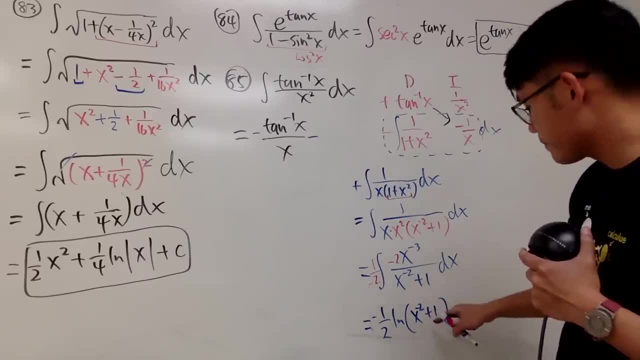 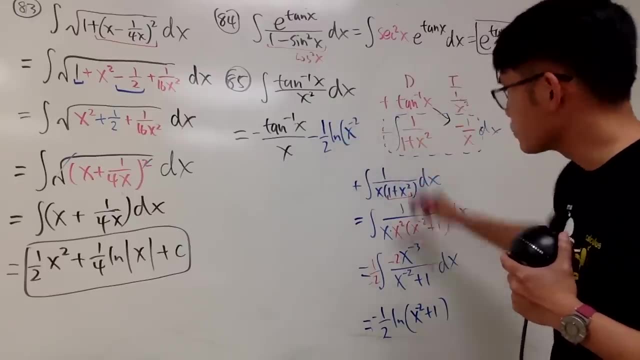 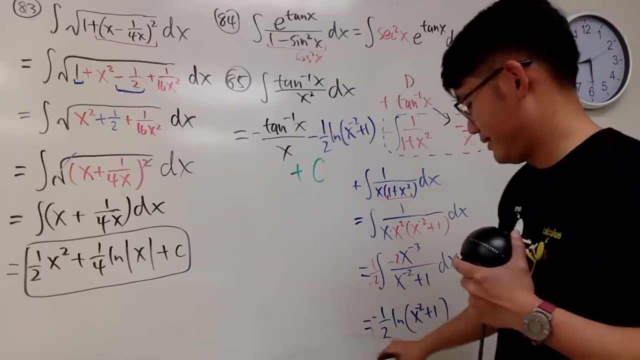 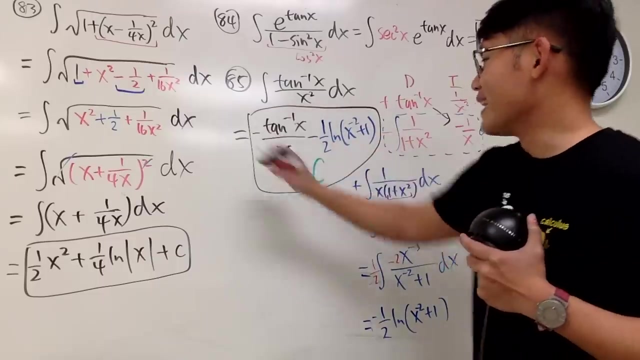 By the way, it's negative Negative exponent: okay, Minus 1 over 2. ln x to the negative: 2 plus 1.. Like that, right Plus d, Okay, And the box is the answer Sorry. 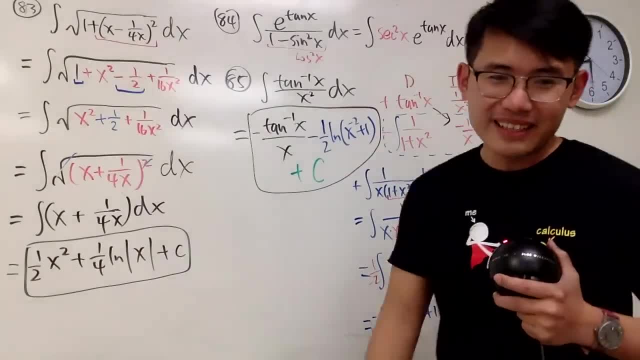 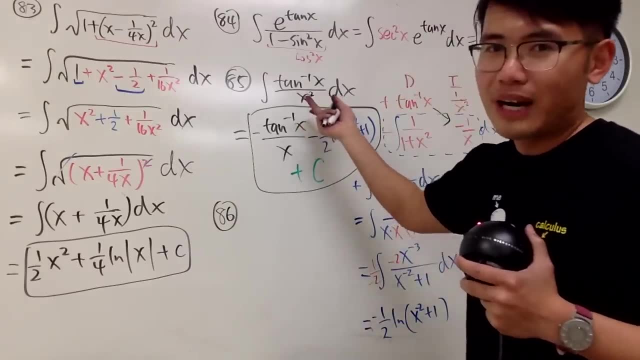 This is not a box. I'm sorry, I'm sorry. Anyway, that's it. Okay, that's it All right, I will fit in another one, Number 86.. All right, So this right here is when you have just x squared in the denominator. 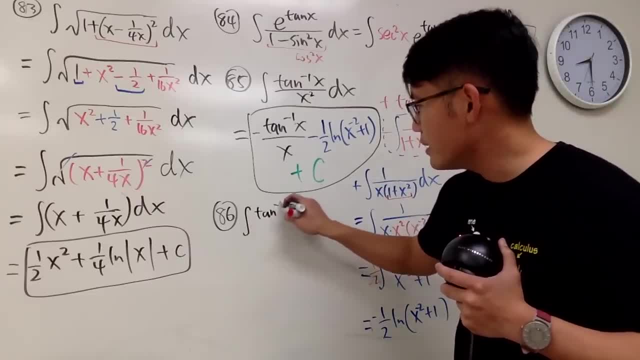 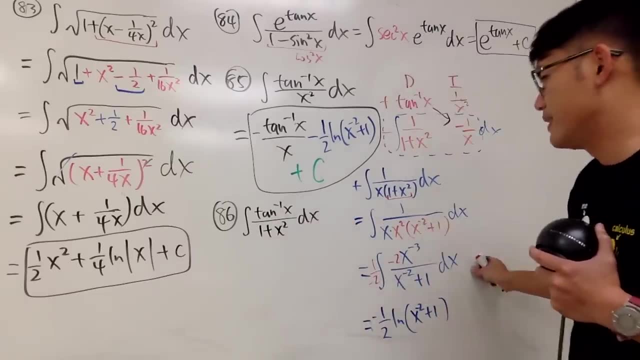 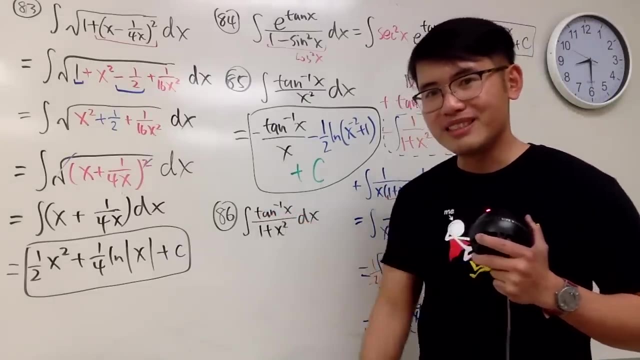 But let's take a look. What if you have the integral of tangent inverse over 1 plus x squared instead? Hmm, How can we do it? Integration by parts again. No, you don't have to, Because what's the derivative of inverse tangent? 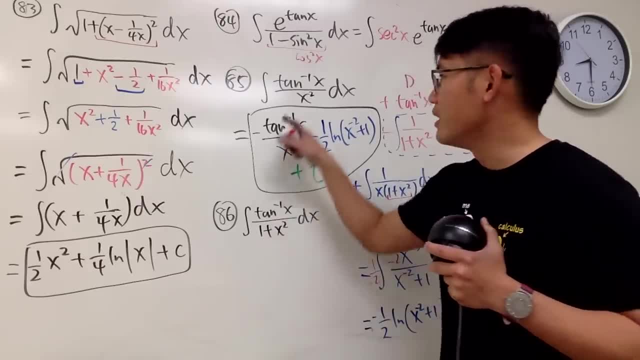 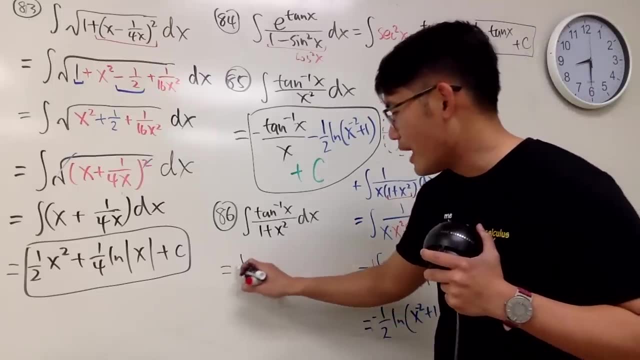 Yes, it's just 1 over 1 plus x squared, And you have that right here. Earlier we didn't have the 1 plus, So that's why it was slightly more work, But this right here it's nicely equal to. 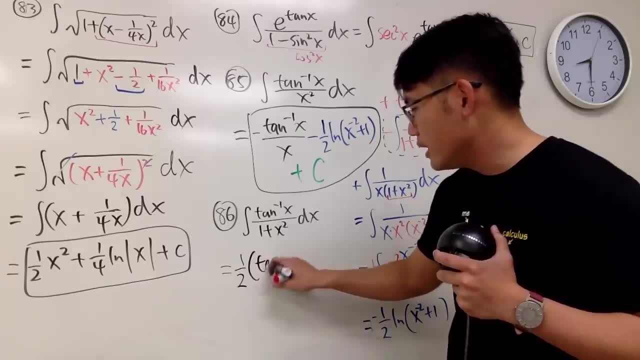 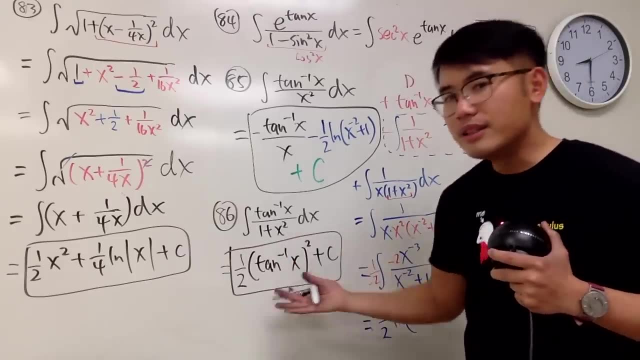 1 half. You take u to be this- Parentheses- inverse tangent of x to the second power And you are done Right here. Okay, So this right here should be a notation for it And if you want to make it clear, 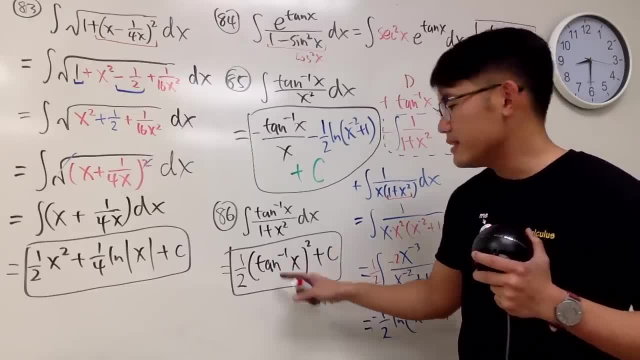 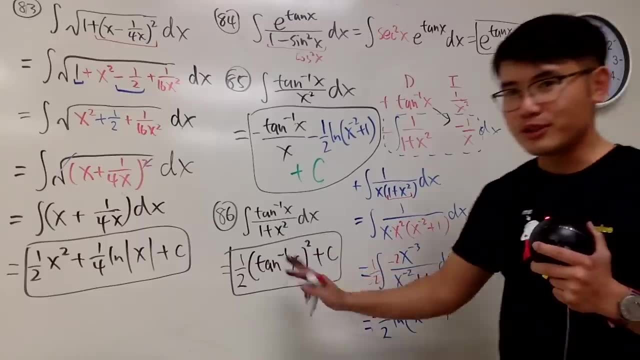 you can also write it as R tangent, But please never write tangent with a negative 2.. Don't, Seriously don't, If you put negative 2 right here, don't? I have a video on that, Just don't. 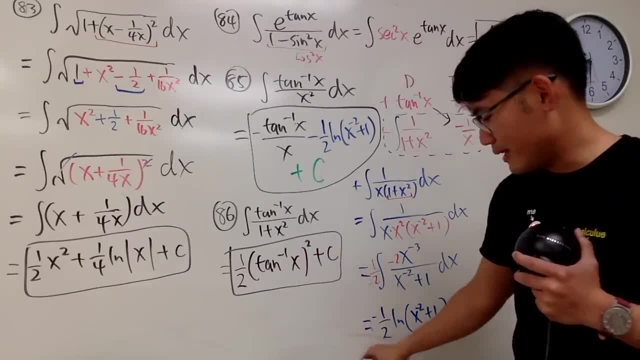 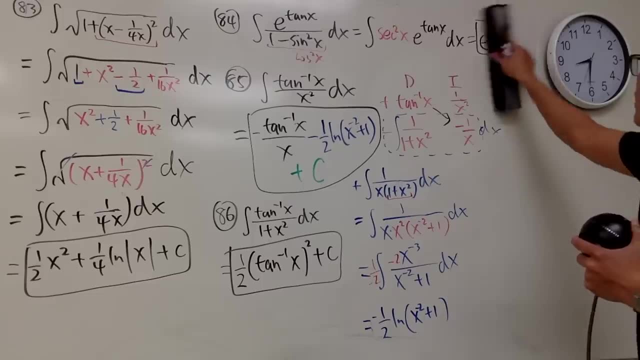 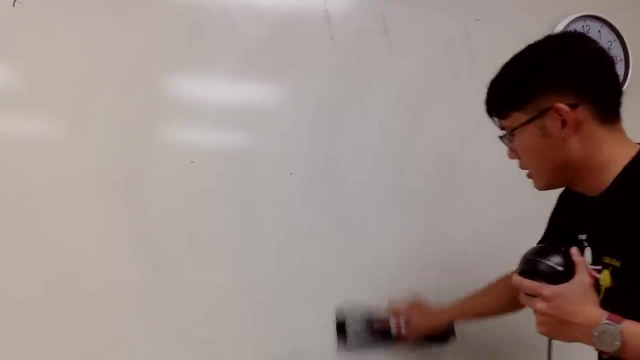 Just don't, Don't, Seriously. I'm making this video, you know, just to show you. No, just don't. Anyway, this is all right here, right? So continue, All right. So again, I'm doing this for loss. 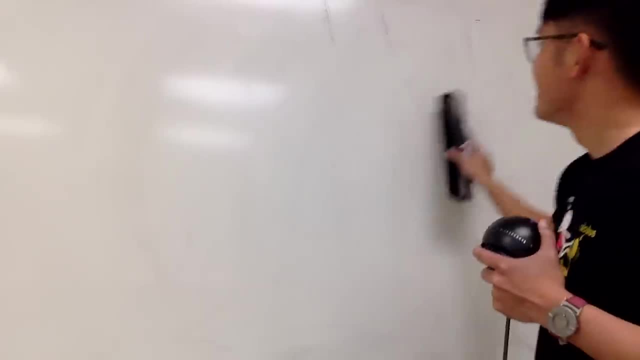 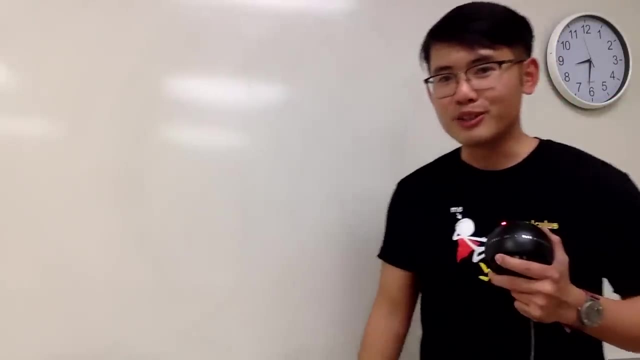 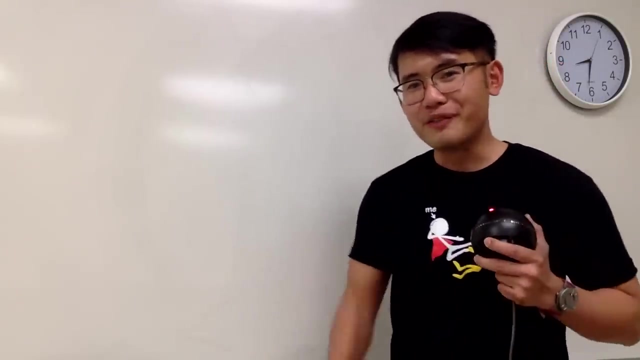 And I wish him the best battling cancer. And I want to say I love my girlfriend so much And subscribe To the people who I recommend you guys Like. for example, my biggest little fan, Wu Han, and Formatica math genius. 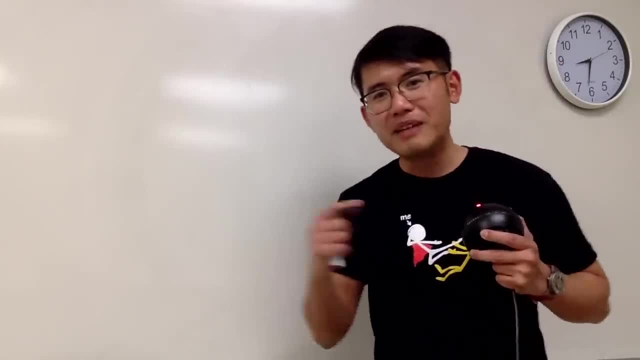 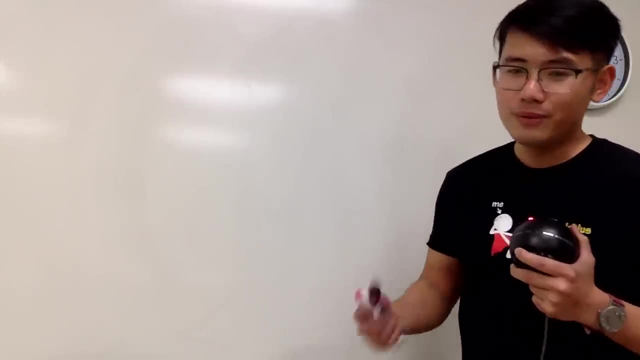 young mathematician in the making And, of course, the happiest mathematician, Dr Payan, And of course, Max and a lot of more people If I don't, if I didn't mention your name, sorry. Okay, It's tiring. 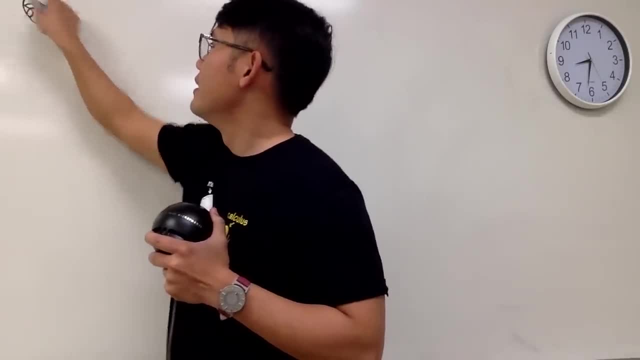 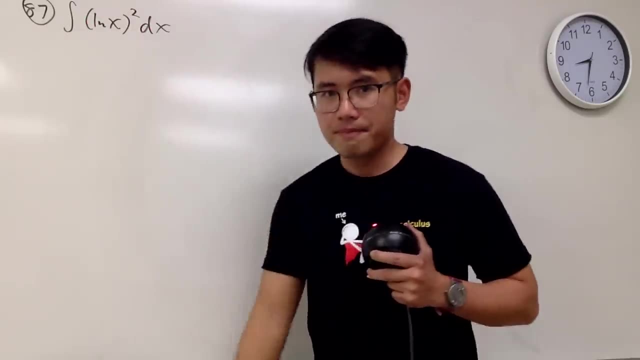 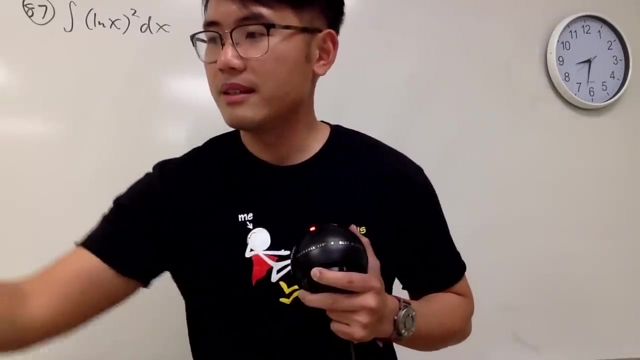 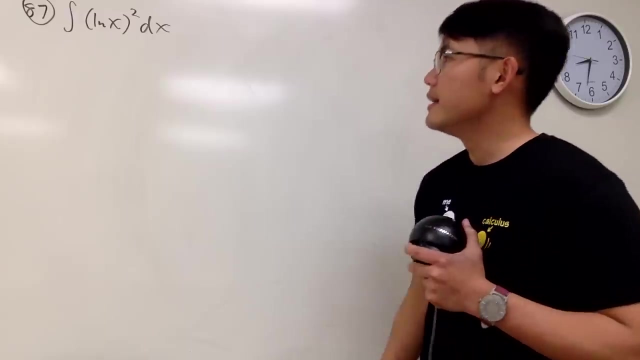 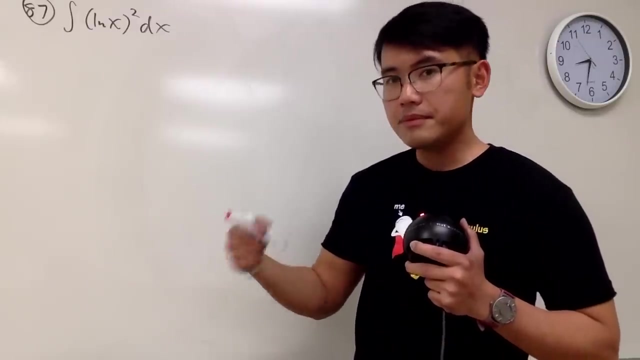 Anyway, number 87.. Subscribe to PewDiePie. Why not Integral Lnx Square dx. What do we do? Drink some tea or something? All right, You can do a use-up, I think. But let's just begin by doing integration by parts. 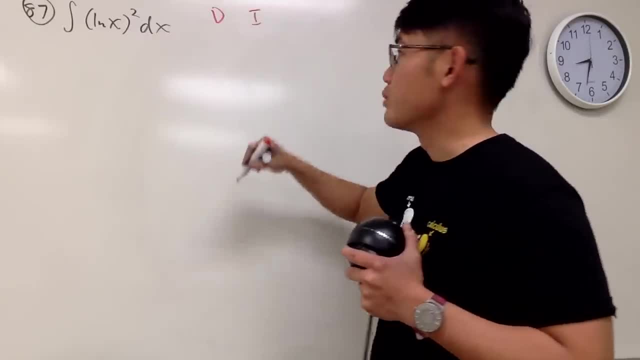 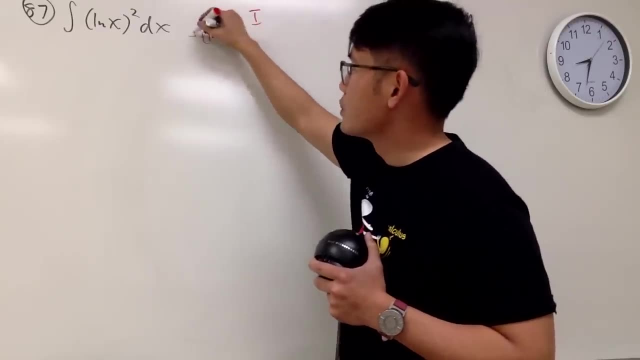 This time, though, I will actually do the dm method Two separate times. You guys will see what I mean by that. I will first differentiate the whole thing: Lnx squared like this, And I know from experience I know this is not going to be enough space. 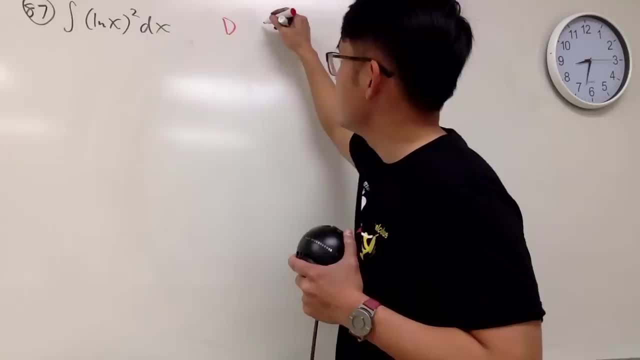 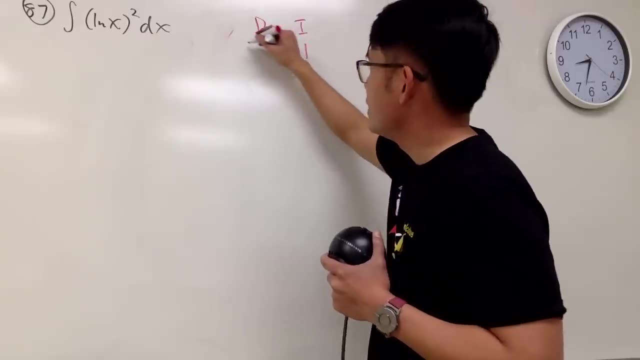 So I will put this down right here. Actually, no, I will put d and an i. All right, Sorry, Let me just make sure I have enough space. d and an i. I will integrate one Differentiate: lnx squared plus minus. 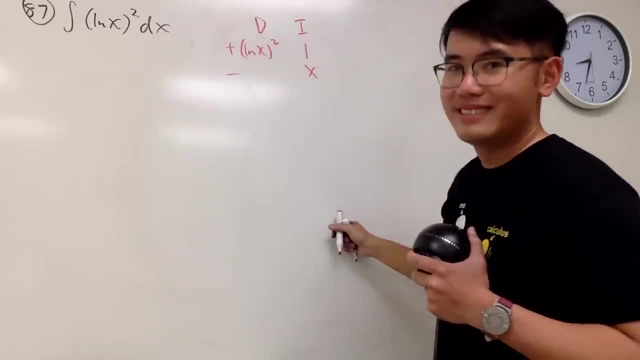 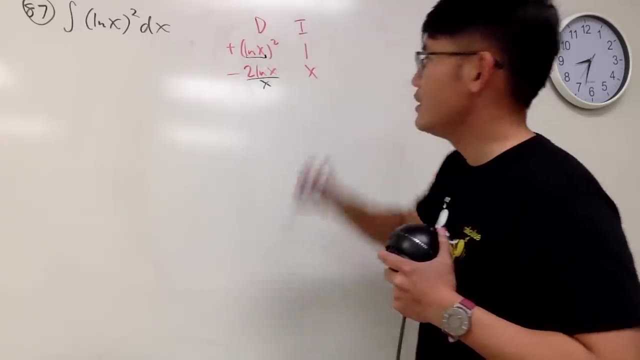 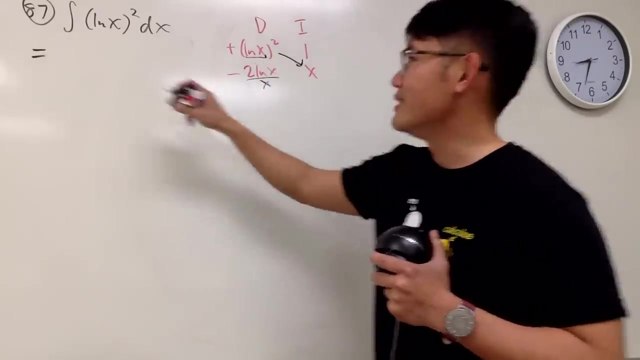 Here we go, Integrating one Nice, Differentiating this to lnx. And then don't forget the chain loop multiplied by 1 of x, Still nice. So first thing, first you have to do this times that. So you end up with x times this, which is x times parentheses- lnx squared. 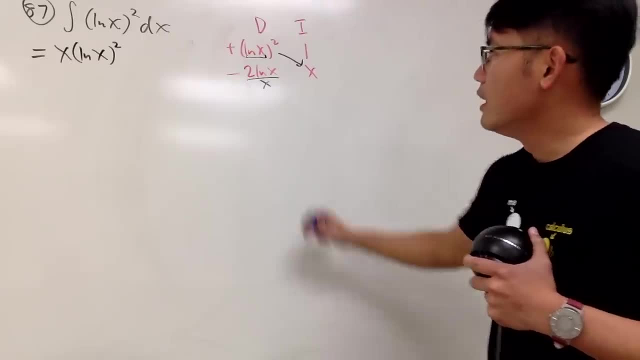 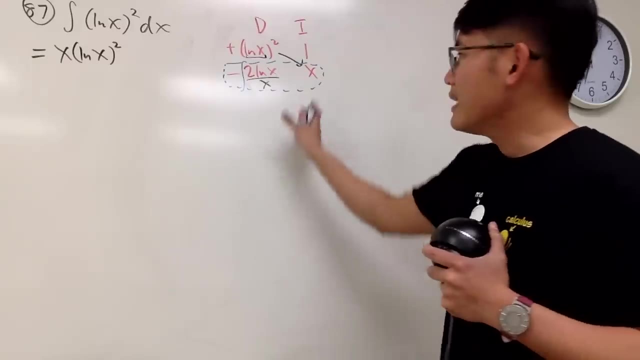 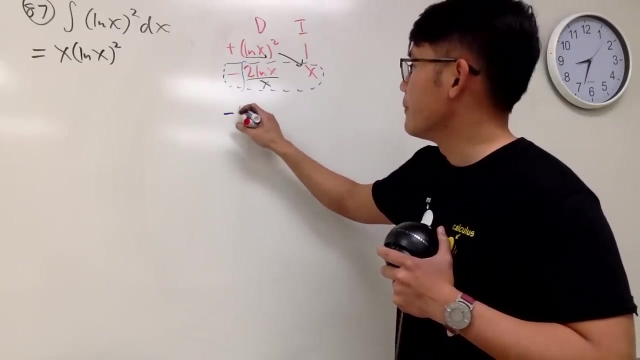 Good, Very, very good. And technically you will have to look at this And again, this is integral, again right, But when you multiply this and that, the x cancel And you have to look at the integral. So let me just write down: minus integral 2, lnx, dx. 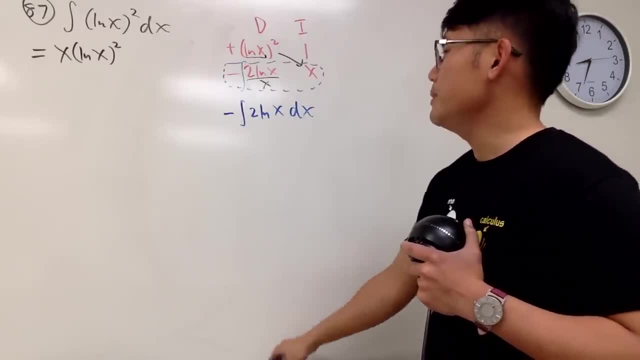 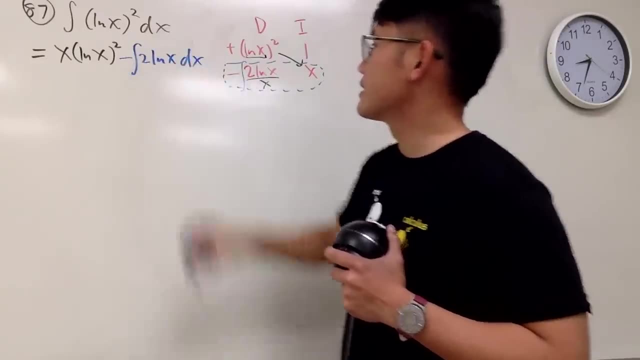 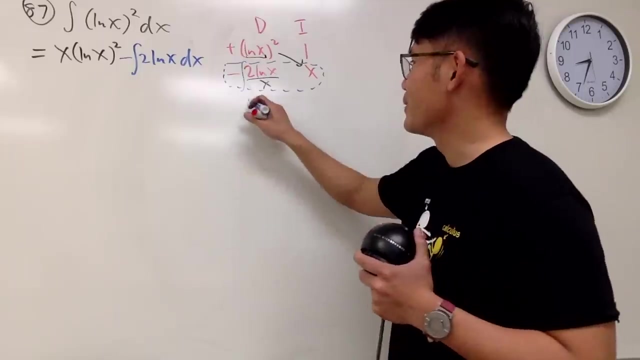 That's what we have to do, right? Let me put it down over there. Why not Go to minus integral 2, lnx, dx, And we have to integrate lnx, So you have to use the dm method again, the technical d right. 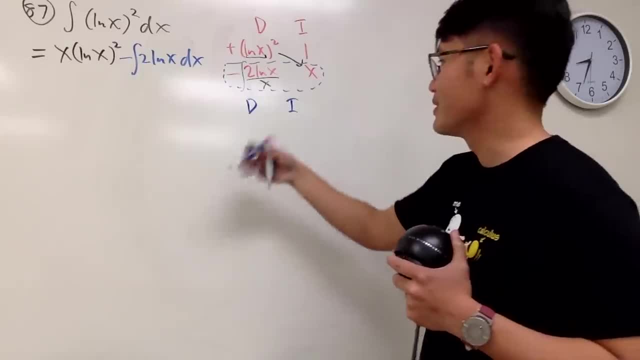 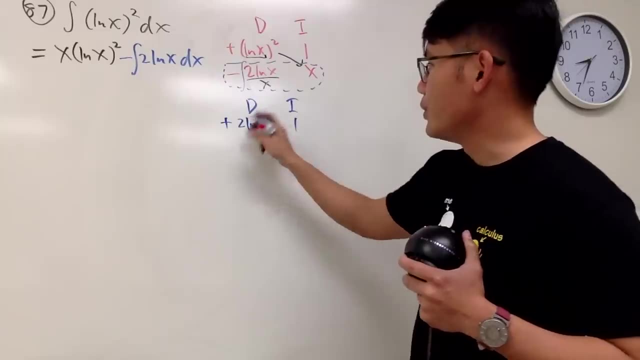 Do it twice. all that. You cannot continue. You just try to just do it again. like that, I will be differentiating. Why not Let's do 2 lnx and then integrate 1. And when you differentiate lnx, you get well. first of all, the plus minus decides the alternating. 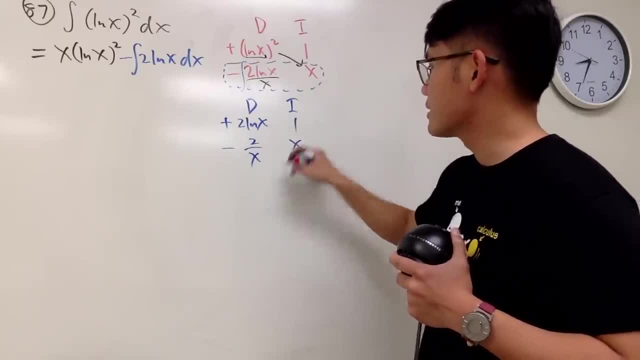 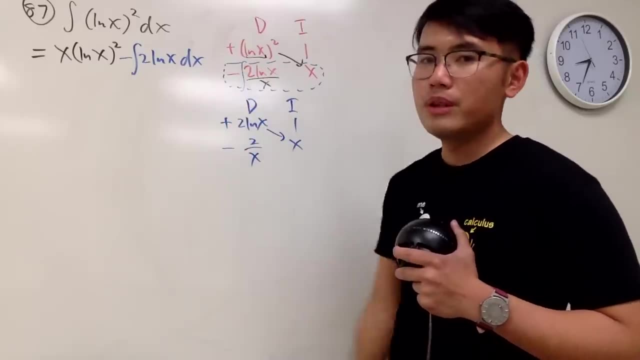 Right here: 2 of x, And then, if you integrate this, you get x right. So again, this times this will be the first part of the integral. This is the answer to the blue integral, And then, of course, you are going to use a blue marker. 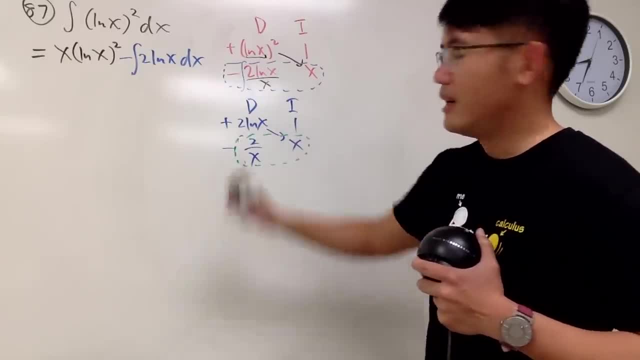 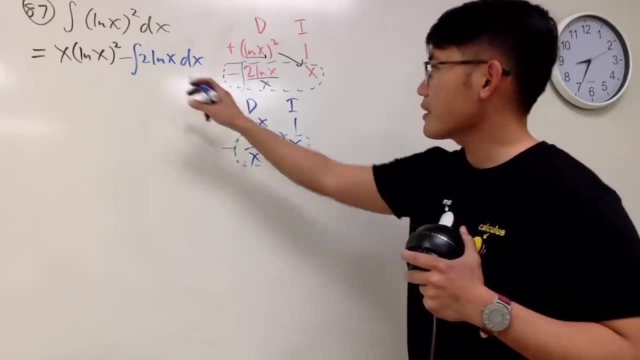 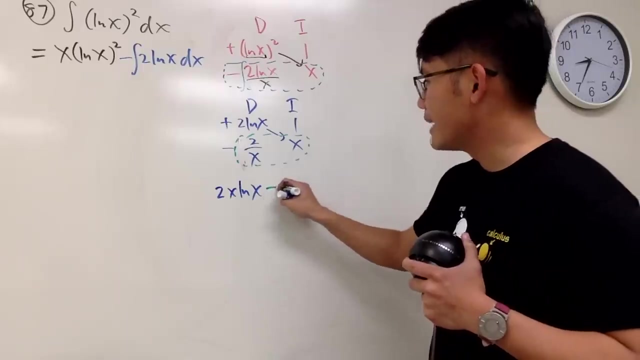 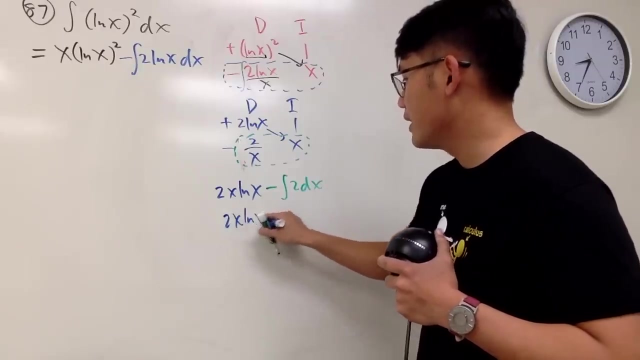 I mean a green marker, And you have to integrate 2, pretty much. Let's see You have 2x lnx And then you have to minus the integral of 2 dx, In other words 2x lnx. 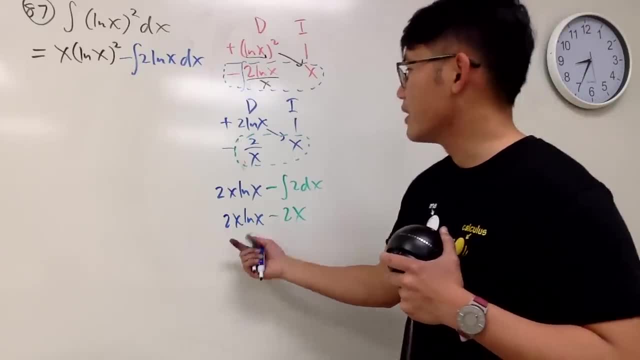 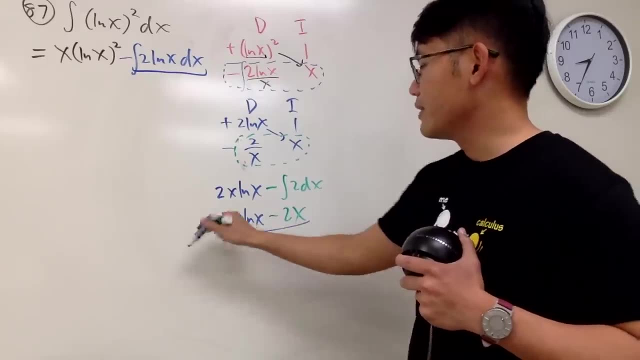 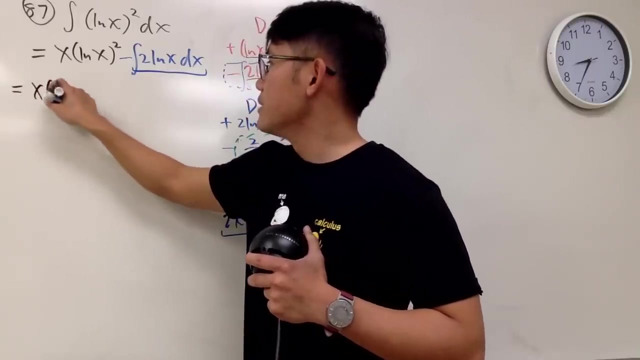 Minus 2x. And then, don't forget this, right here is technically inside of this integral, right here, right, So you have to have the negative in front. So the final answer should be- let me write it down right here for you guys: x times lnx squared negative times that. 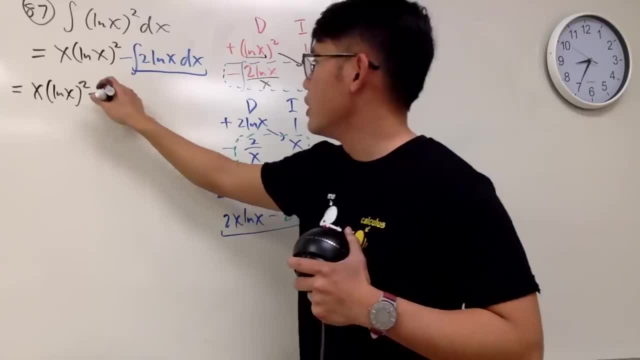 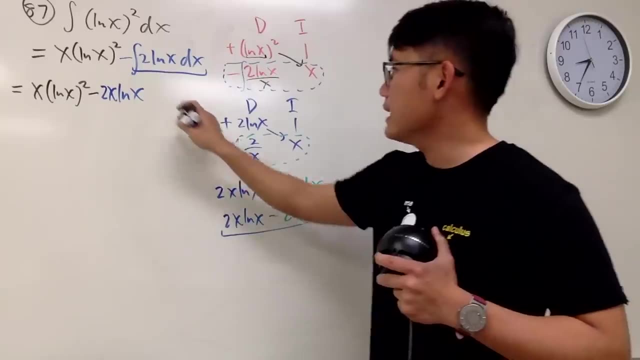 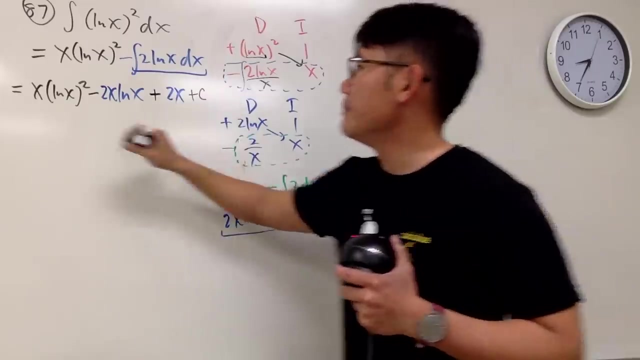 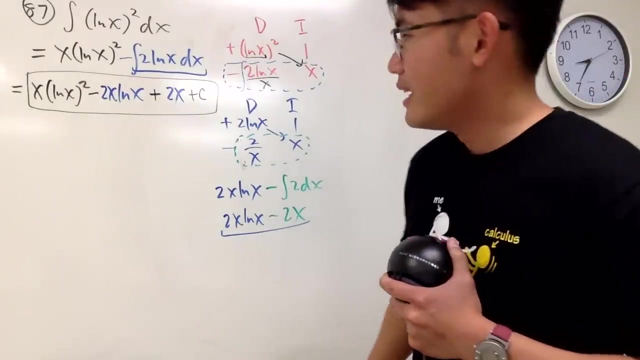 So you have negative and then you have the 2x lnx, And then negative times negative. we get plus 2x And we are done. Put a plus here and be happy. Okay, continue. Number 88.. 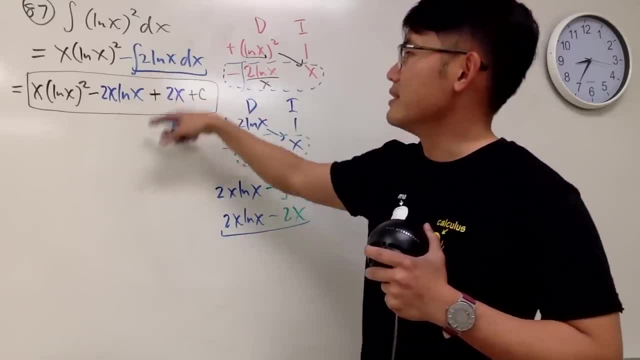 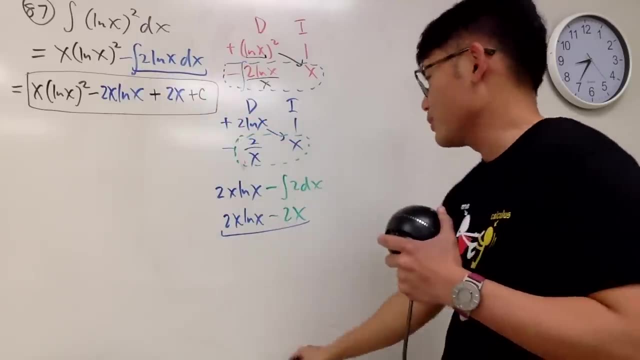 In fact, if you know, the integral of lnx is just lnx x, lnx minus x, And then you distribute negative 2, that's fine too, but technically you should do the Y method again. But like here we stop. 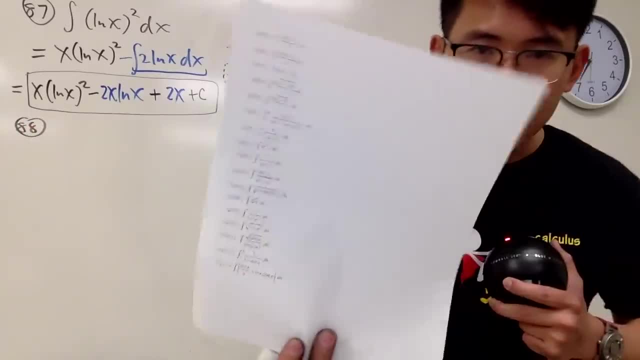 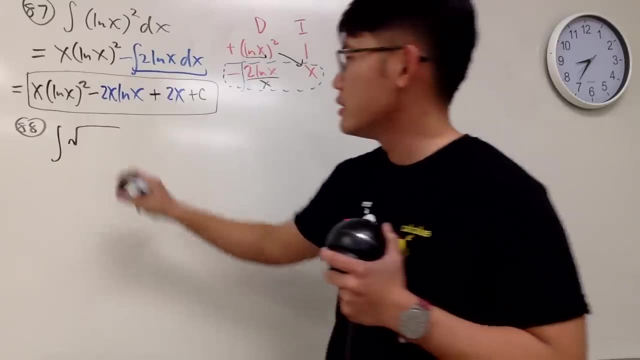 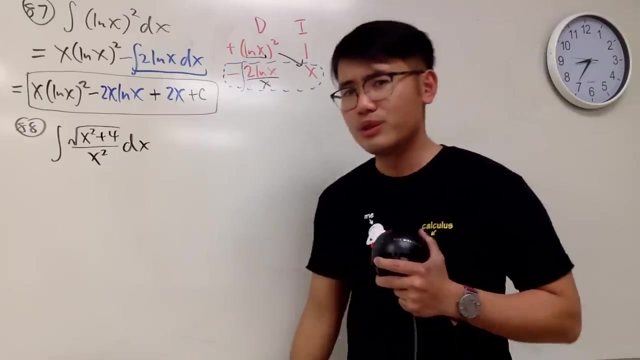 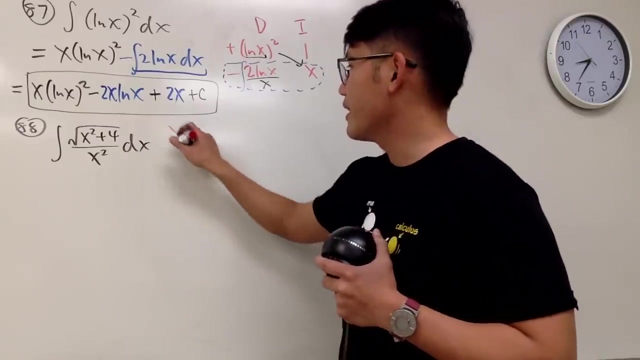 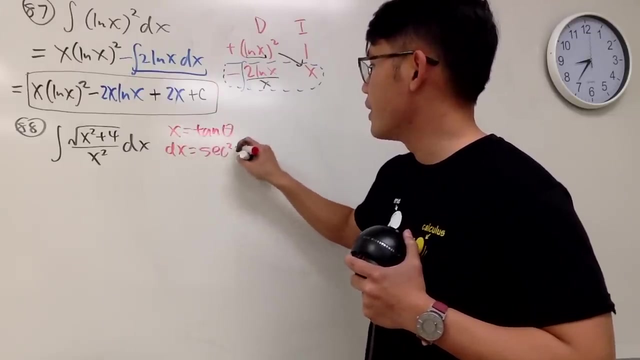 Alright, number 88.. We still have some hard questions, okay, So keep watching. Integral square root of x squared plus 4 over x squared dx. How do we do this Trick? stop, alright, Trick stop. However, right here, take x to be tangent theta and dx will be secant squared theta, d theta. 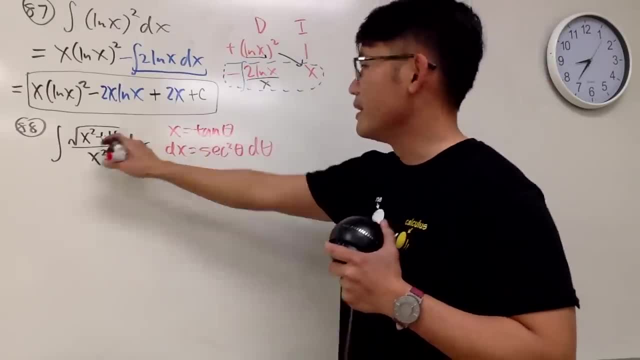 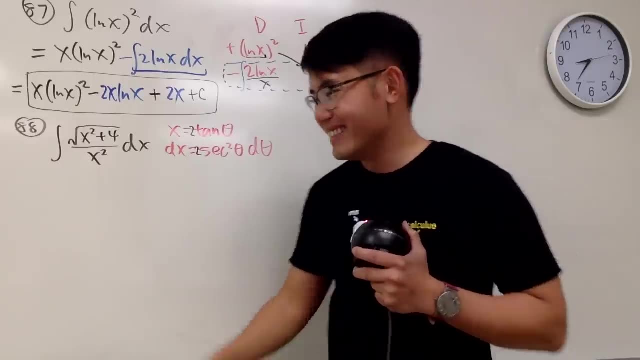 And hope for the best. Actually, sorry my bad, It's a plus 4.. Oh my god, Who put a plus 4?? Yes, it was me. Alright, let's do this in our head. Check this out. 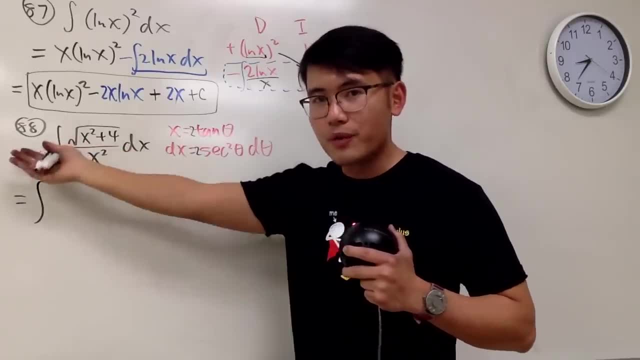 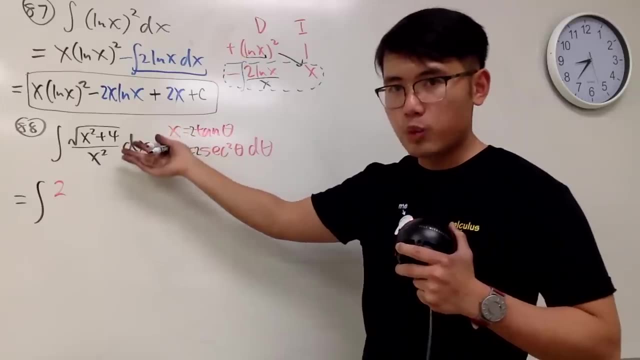 You put a 2 tangent theta in here, You square that, You can factor the 4. And then instead of the square root you get 2.. Okay, You get a 2.. And then you get tangent squared theta plus 1.. 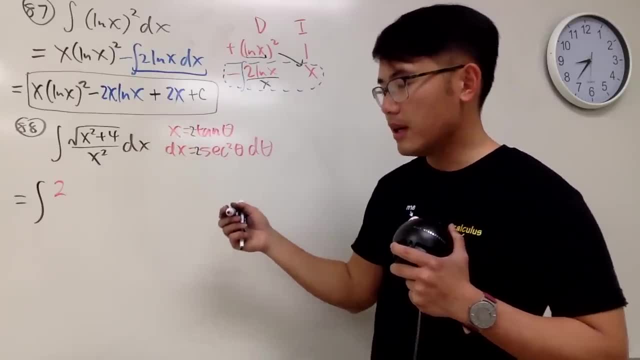 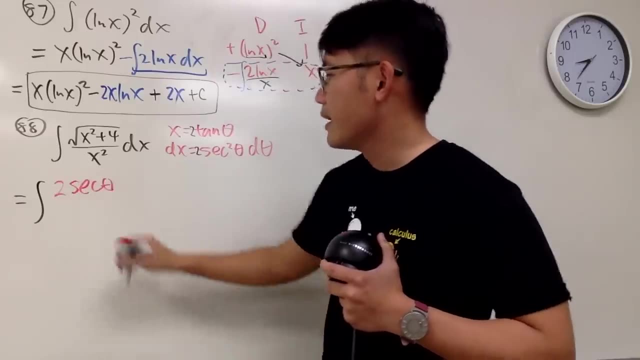 That will be secant squared. Well, secant, It will be secant squared, but in the square root. so you get secant to the first power. So secant theta Over. you have to be careful right here. 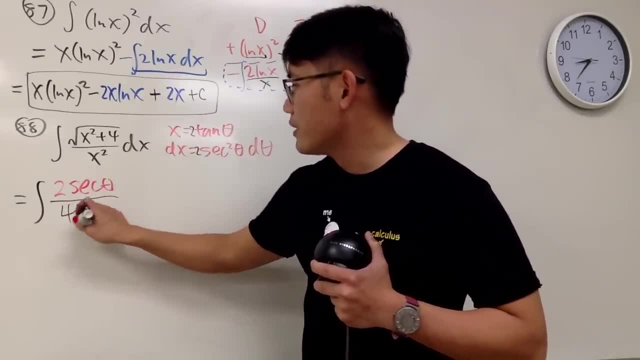 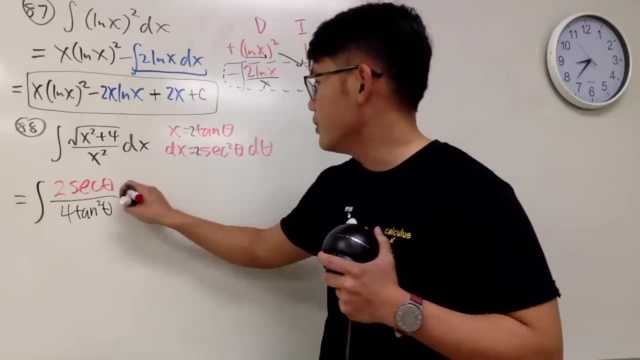 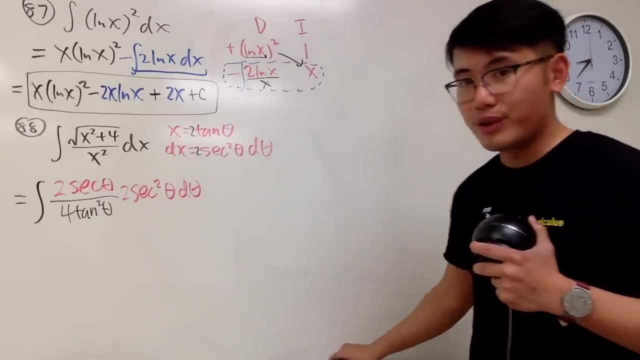 You have the little 2. You have to square that, So you end up with 4 tangent squared theta. And then you also have to have this For dx, which is 2 secant squared theta, d theta. And now something is pretty good happening. 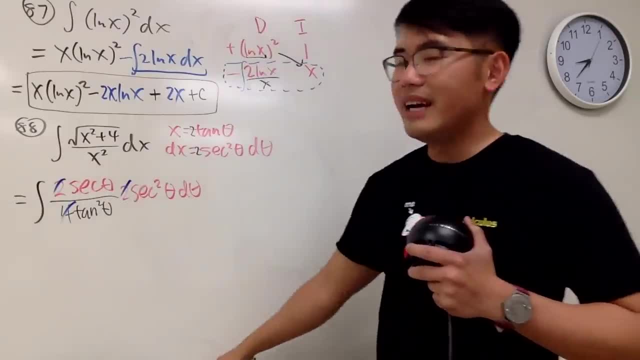 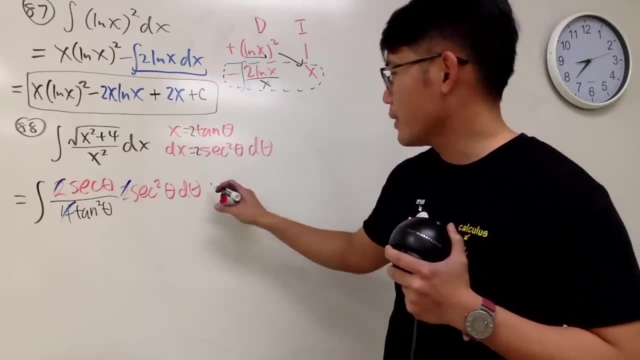 2,, 2,, 2.. They all cancel out. That's good. And then, unfortunately, you have secant cubed. Oh god, Let's see. Alright, so I will do this Integral. So I have secant cubed, which is the same as saying 1 over. 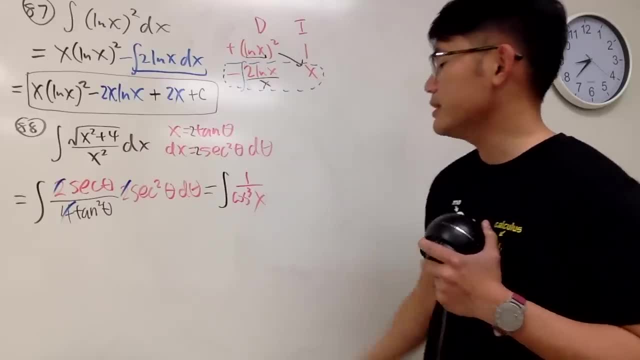 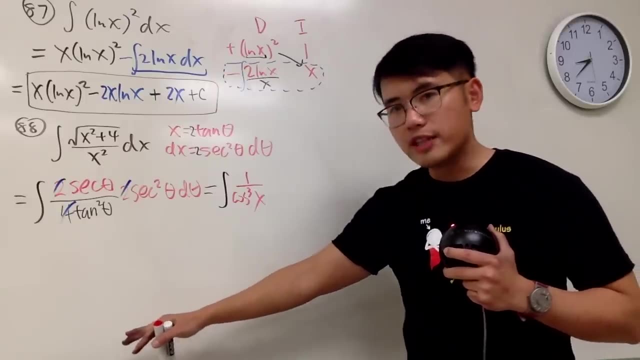 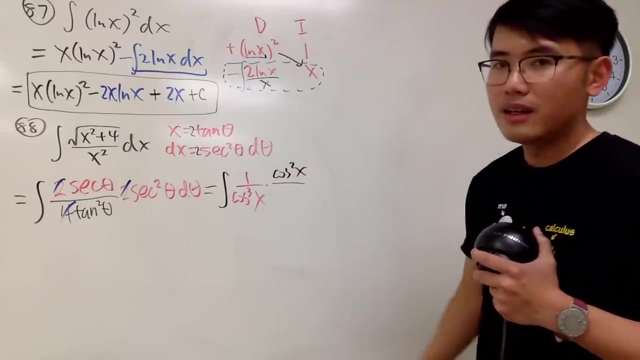 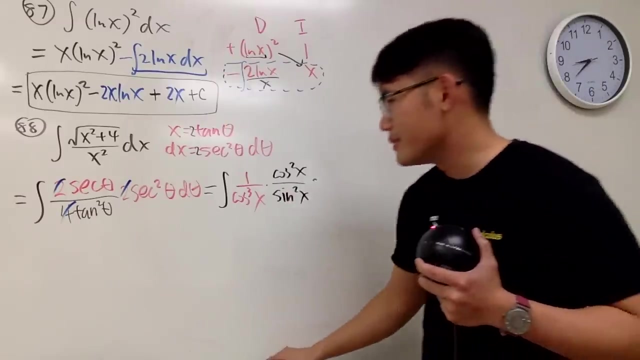 Cosine cubed. Am I right? 1 over cosine cubed. Tangent squared in the denominator is the same as cotangent squared And we can look at that as cosine squared x over sine squared x Like that And we have the no. 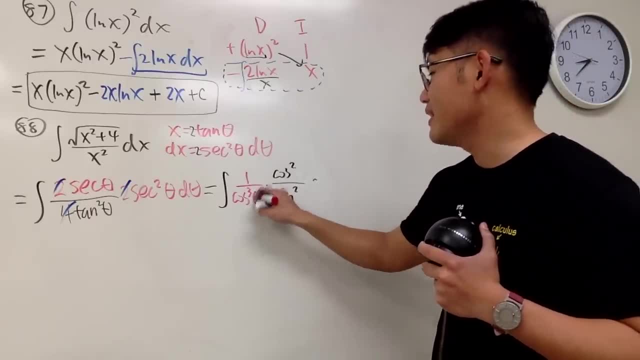 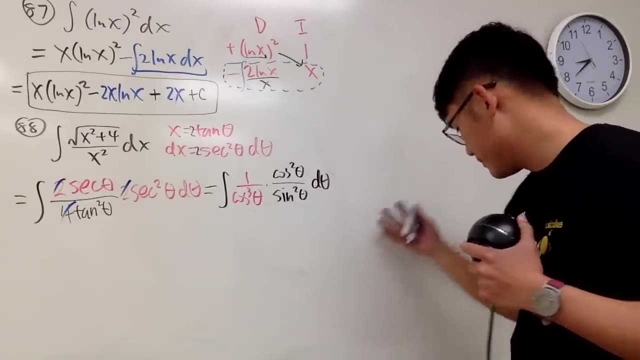 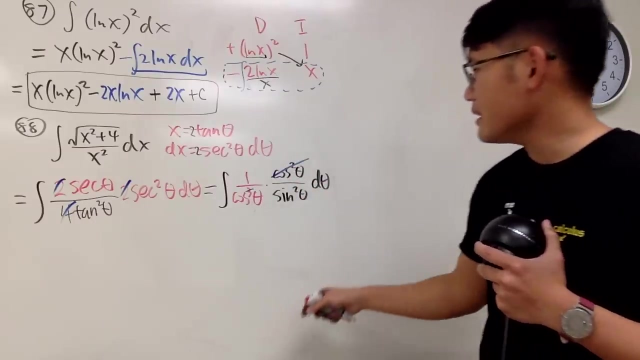 I am still in the theta world. Oh my god, This is with the theta, Theta, theta d theta. Like this And I am like, Let's see This right here, Cancel out. And now I have that. 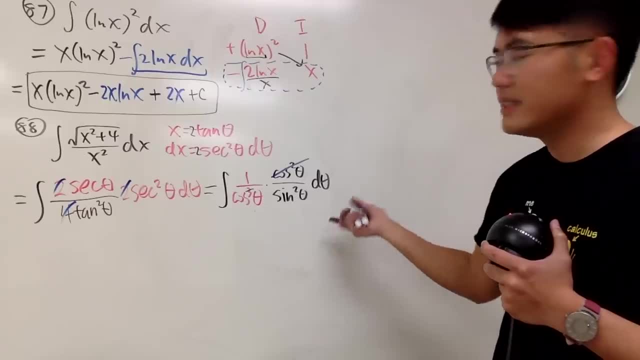 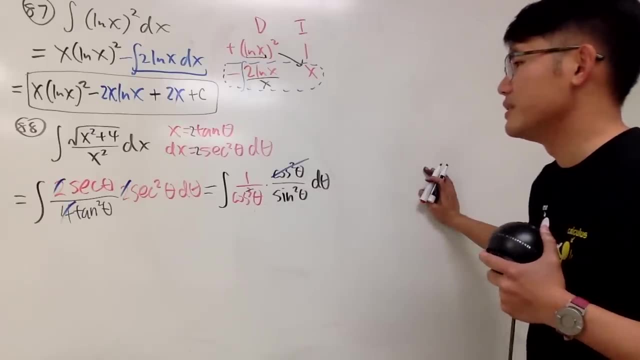 1 over cosine theta times sine squared theta is equal to this. Cosine is in the wrong place. Oh my god, Let's see how we can deal with this. Did I do anything wrong? so far, I don't think so. 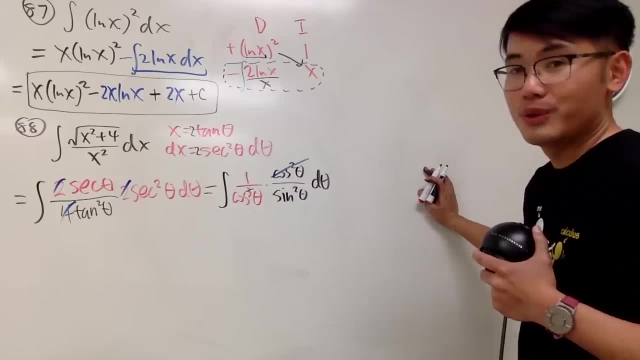 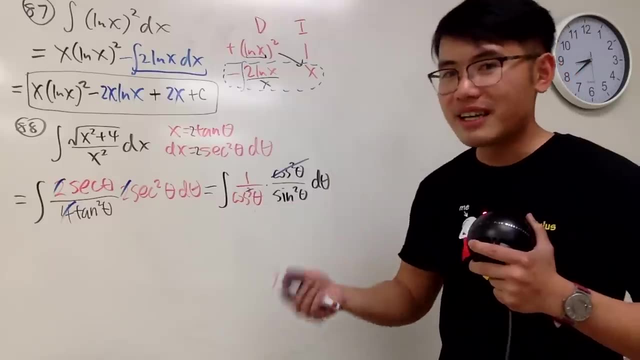 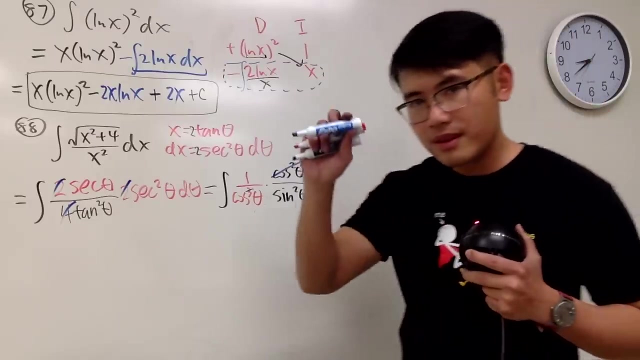 But we just have to deal with this, right. So I just want to make sure that we are doing this legitimately, If you notice, you notice. Yes, we can write the 1 as sine squared plus cosine squared. This time let's introduce blue marker. 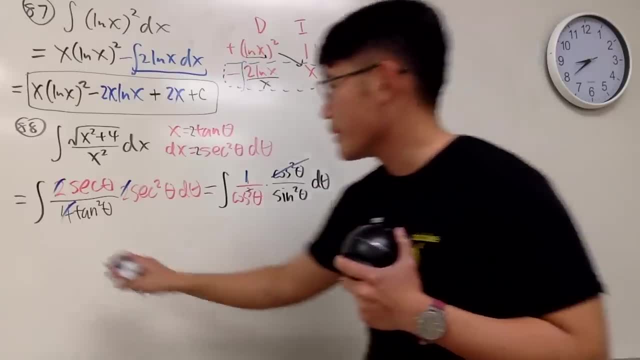 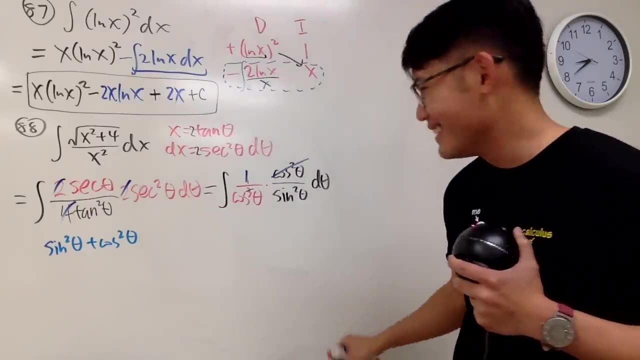 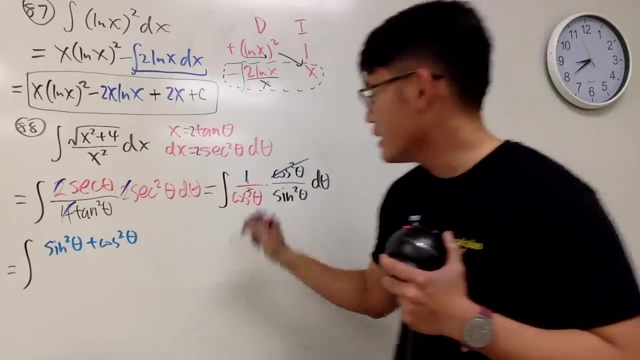 This is prettier, This one. Look at that Sine squared plus cosine squared And we are still in the theta world. So let's put that down, Okay? And then this is integral to this, right here: Well, split the fractions. 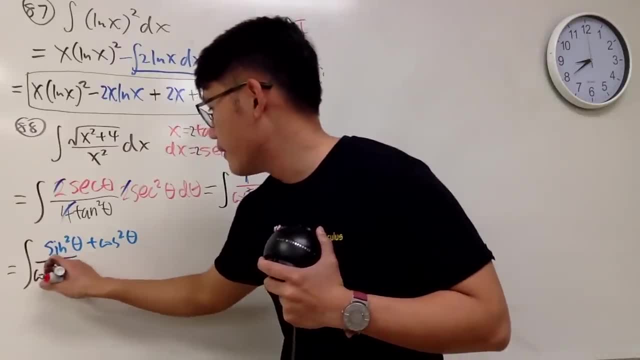 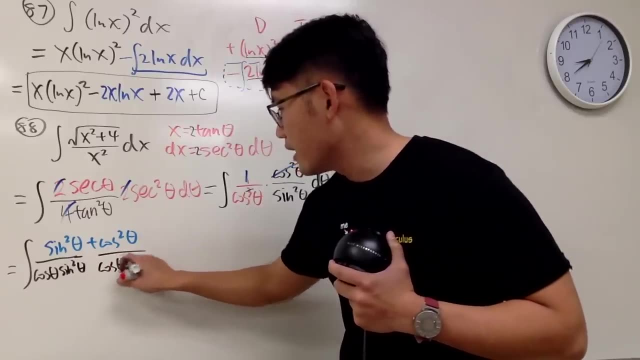 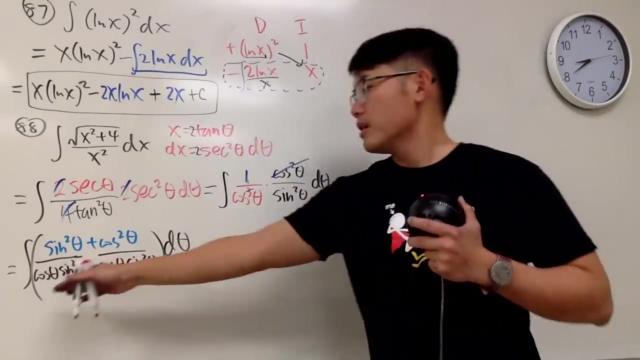 Cosine to the first power: theta Sine to the second power: theta. Okay, This one Cosine: theta Sine squared theta d theta, Like this. People keep on me, People keep wanting me to put the parentheses. 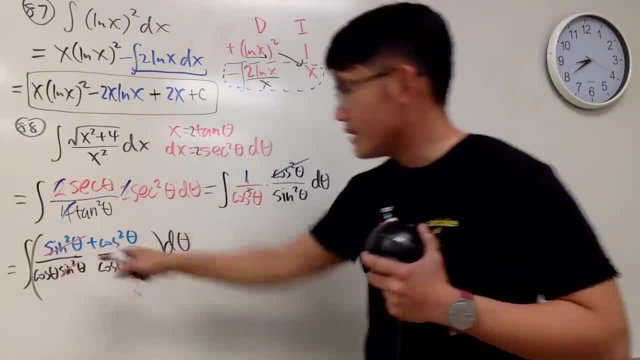 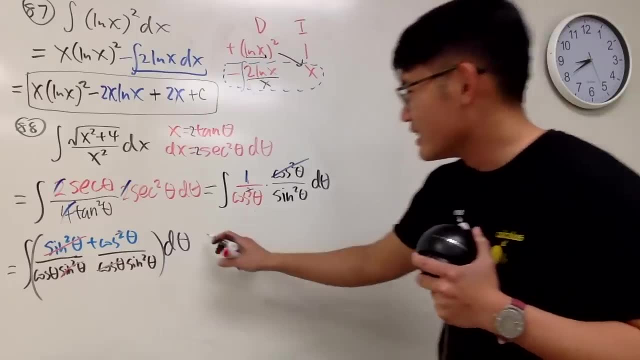 But it's up to you, man. That's easy, That's doable. Now for this one. That's also just as easy. Very good, So we will see. The first one is just integral of secant theta. 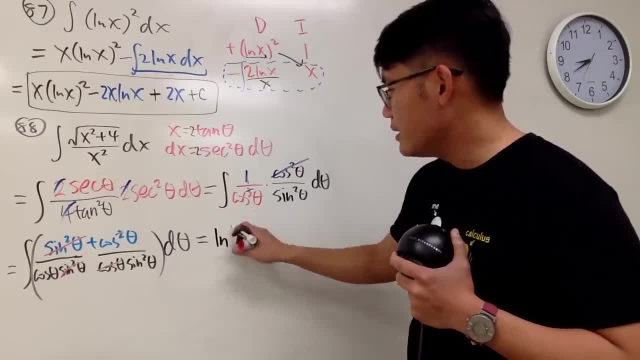 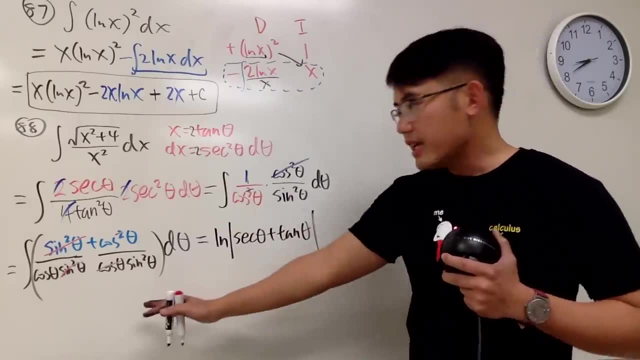 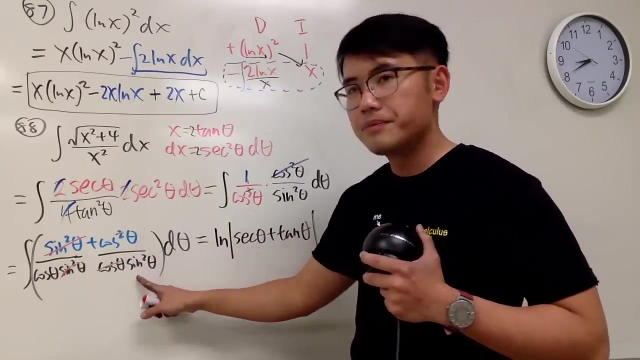 Which we will get ln up to the value secant theta plus tangent theta. Okay, For the second one, Okay, You have cosine to the first power, So you are going to do some use up, Let u equal to this, And then you pretty much have to integrate 1 over u squared. 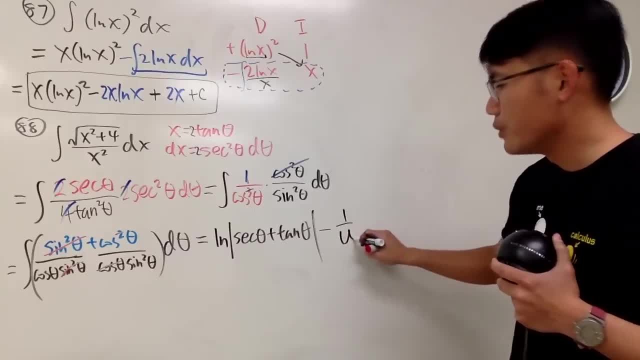 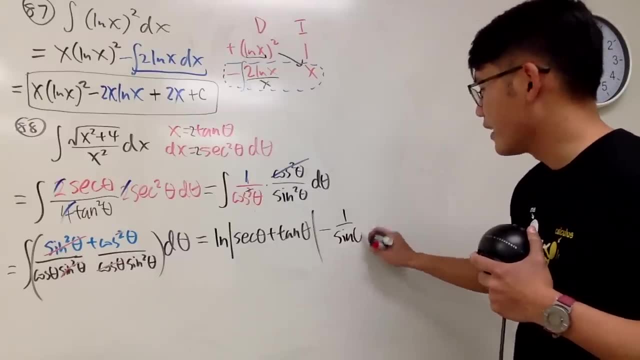 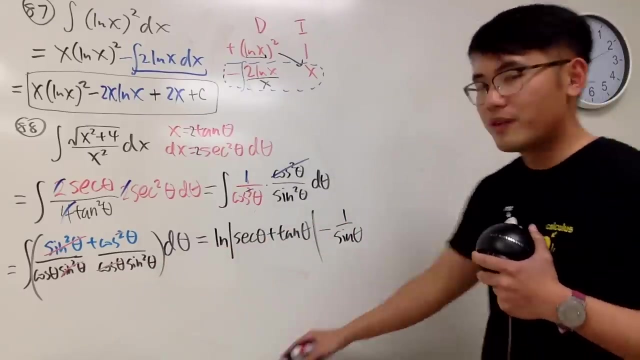 Which you will get negative. 1 over u- Okay, But u is sine theta, So you have 1 over sine theta, Like this: So if you differentiate this guy, you end up with that guy. This is good And, of course, 1 over sine theta. 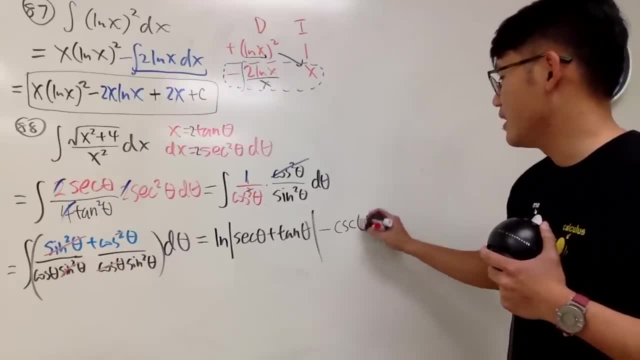 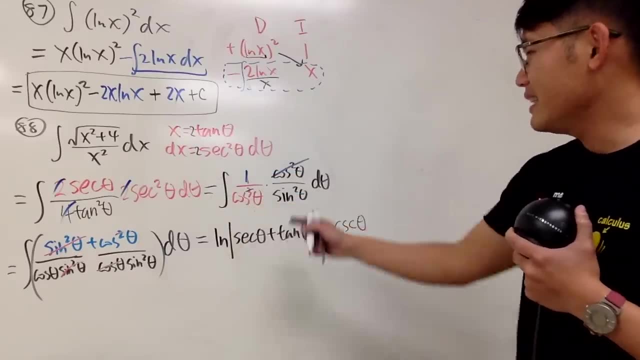 It's just cosecant C-S-C theta. Wow, Everybody is here, huh, Almost. Yeah, Let's see, I have sine, Yes, I have cosine, I have, Oh, I don't have cotangent. I could. 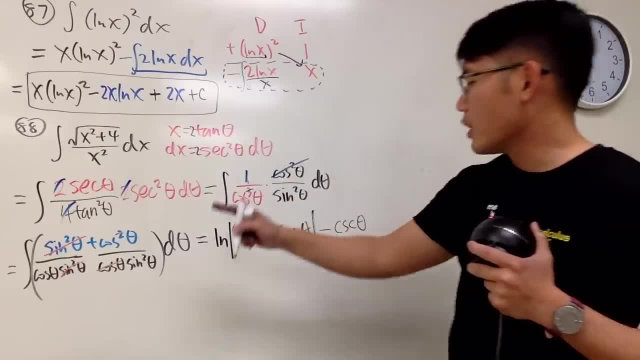 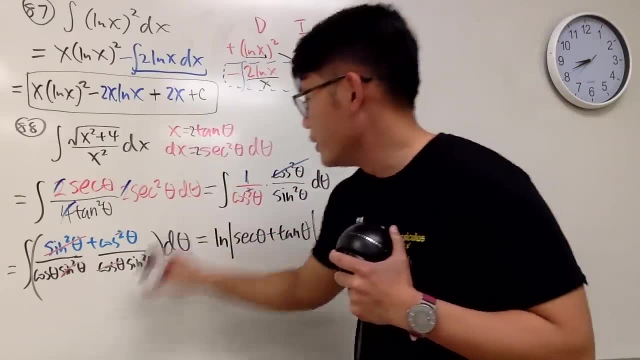 But like I didn't have it, But anyway, Anyway. So here is the deal Right here. we know- Let me put this down here for you guys- We know- tangent theta is equal to equal to x over 2.. 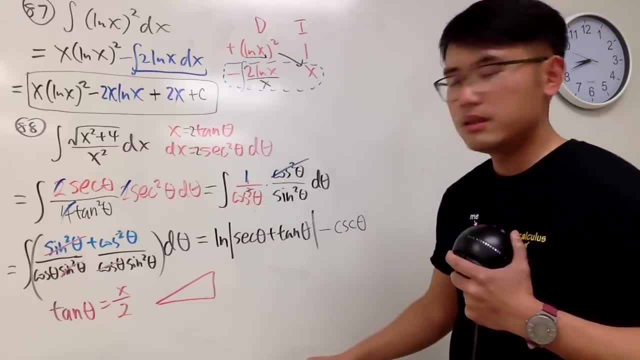 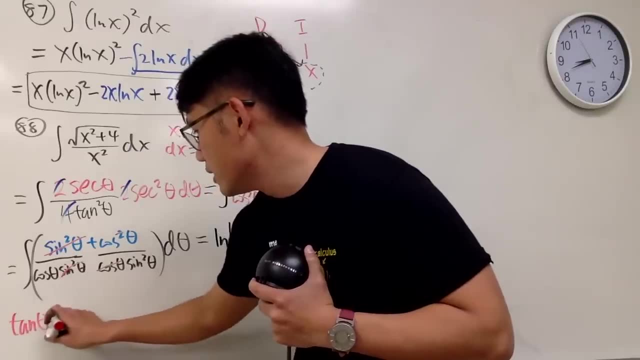 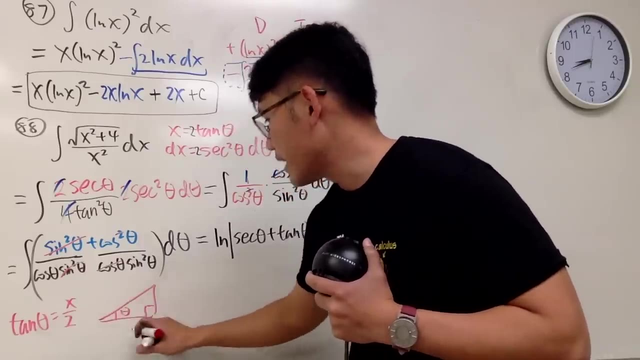 So that means we can draw a right triangle here. And let's see, I want to write it down below. So I will say: We know, tangent theta is x over 2.. And we can draw a right triangle. This right here is theta. 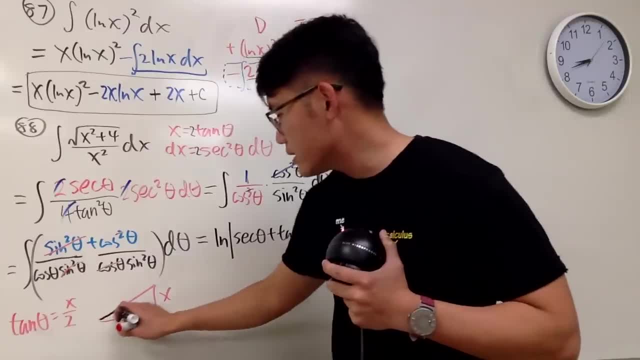 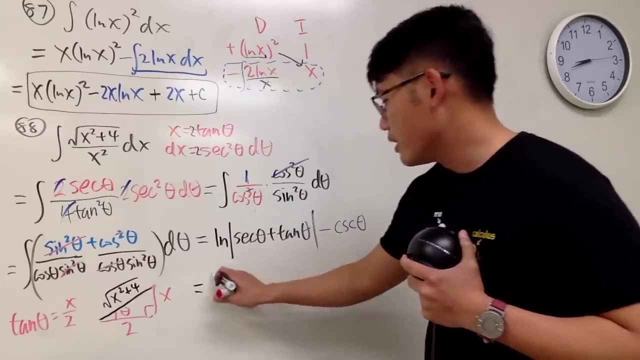 And then tangent is x over 2. And the hypotenuse is this: Of course it's going to be square root of this square plus that square x squared plus 4.. Now we are in business This right here: natural log, absolute value. secant this over that. 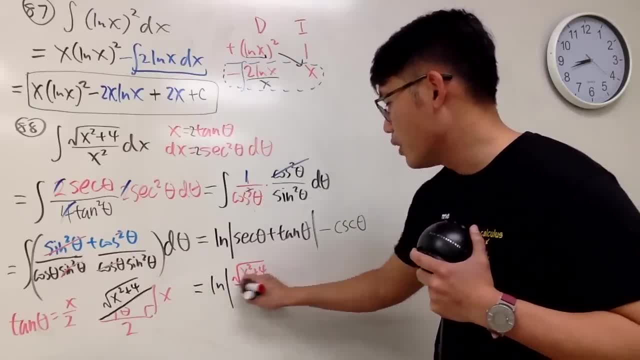 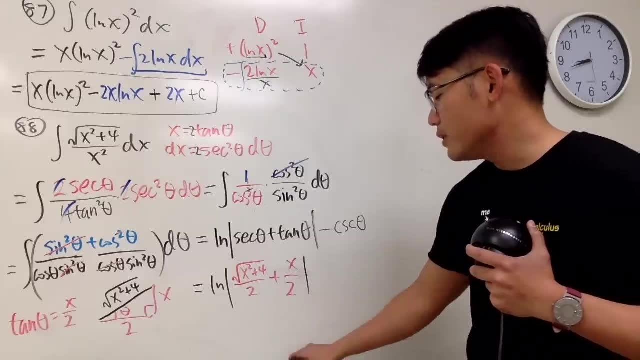 which is the square root of x squared plus 4 over 2.. Tangent this over that, So we can put down plus x over 2.. In fact, everybody there inside will be positive, because this is bigger than that. 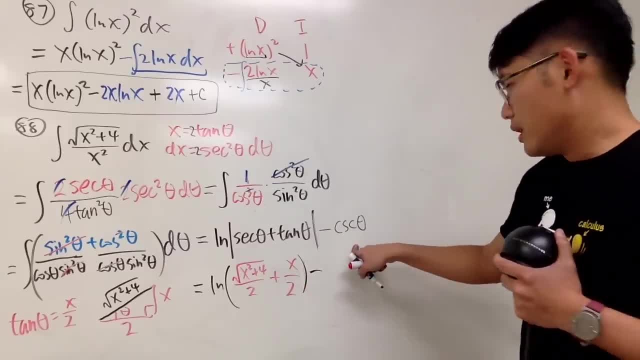 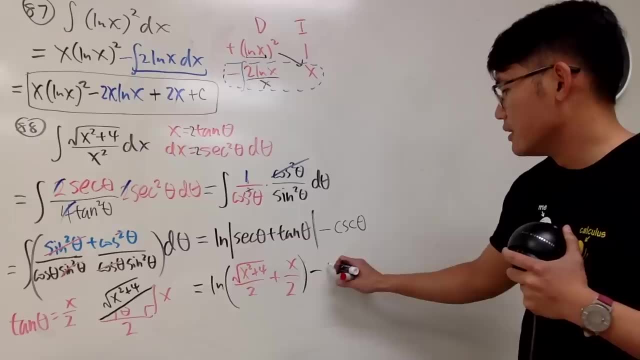 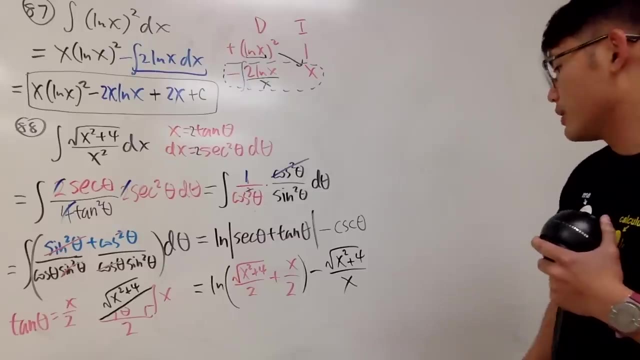 So you don't need the absolute value. And then minus cosecant theta, is this over that. Yeah, So it's square root of x squared plus 4 over x like this: Wow, That was a tough one, And here's the deal. 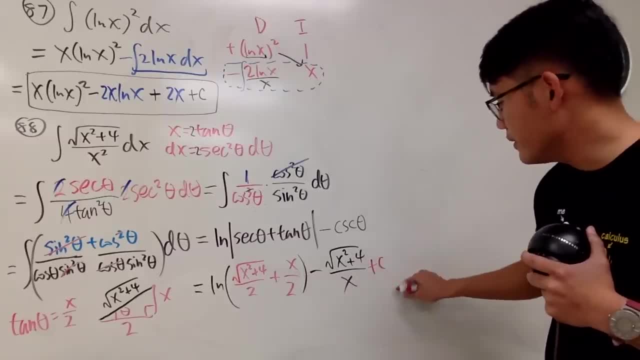 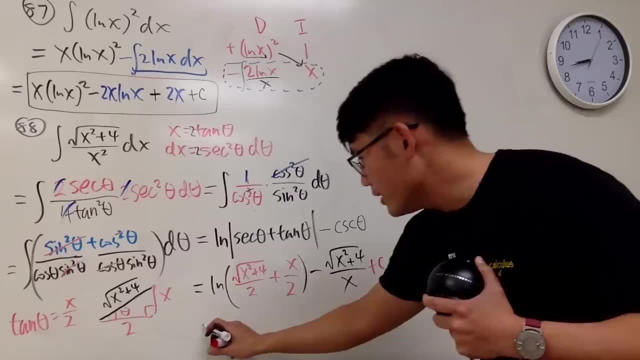 Yes, you can put down plus c1.. Okay, This is good. If you want to just call it for the day, that's fine. Again, ln of the top minus ln 2 for the bottom. So if you want, you can write it down as natural log parentheses. square root of x. squared plus 4 plus x. 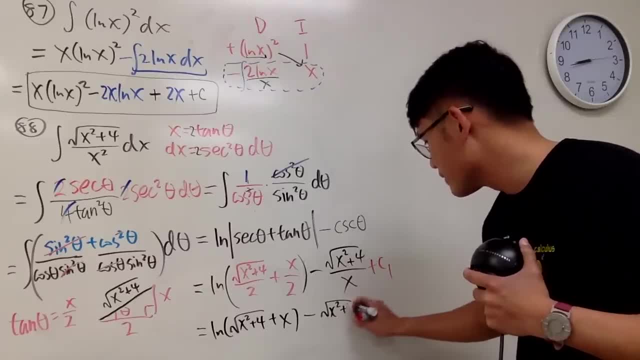 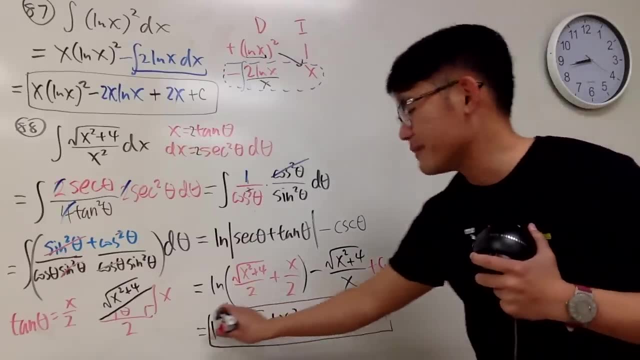 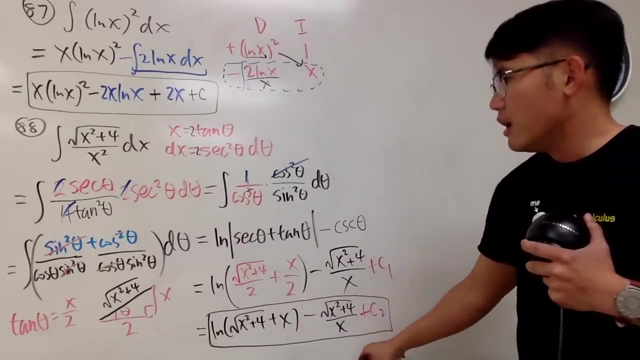 And then minus this guy, x, squared plus 4 over x And then put down plus c2.. I'll box this. If you use Wolfram Alpha, I think they will give you this kind of answer, or the answer in the back of your textbooks. 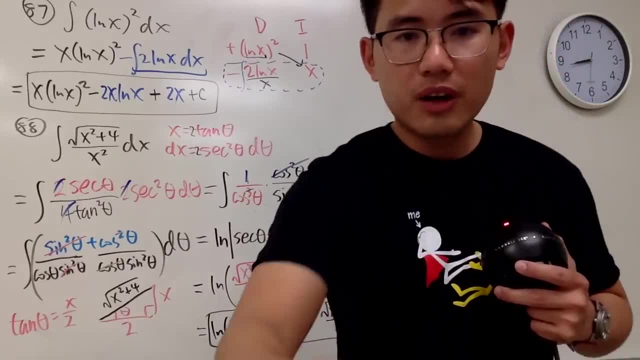 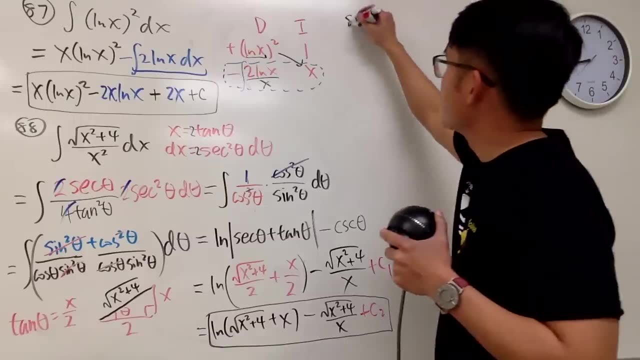 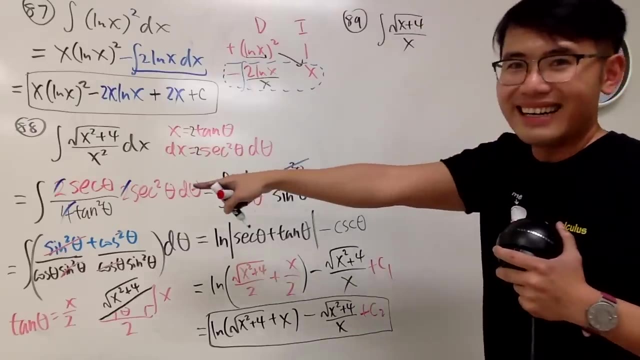 Yeah, So that will be it. Okay, 12 more. Okay, Number 89.. I'm going to go fast. Integral square root of x plus 4 over x. Already I have square square. This time I don't have the first power. 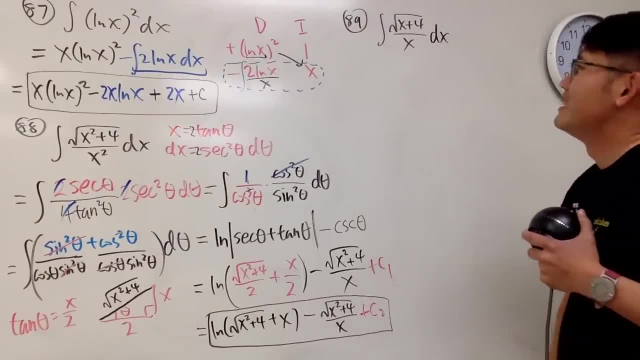 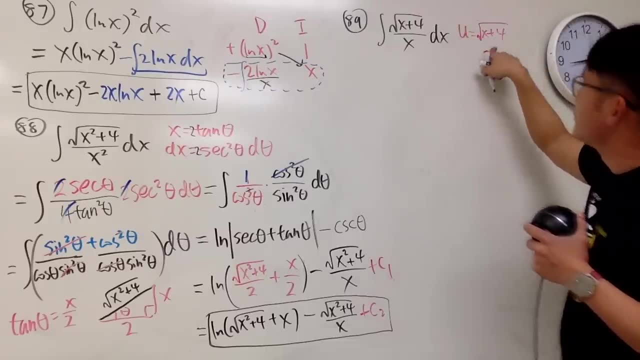 I think this is going to be good. Okay, It's going to be better. How do we do it? Let's do it yourself. Okay, Let u equal the square root, Square root of x plus 4.. And I want to solve for x. 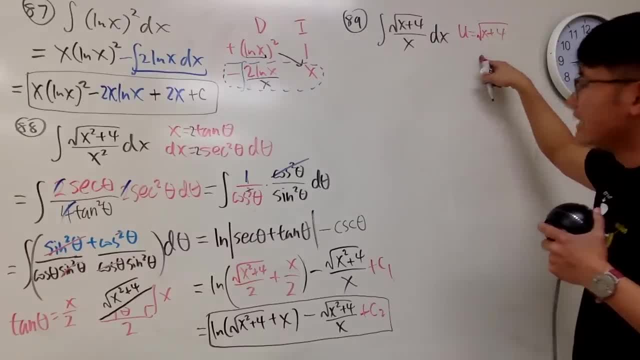 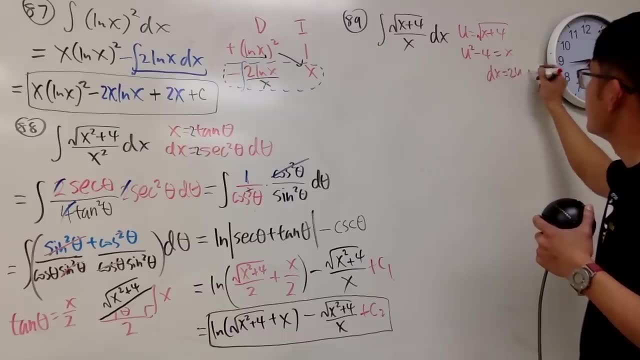 So let me just square both sides and minus 4 on both sides. In another word, I get u squared. minus 4 equals x. dx will be just 2u du. Very nice, Now take this to the new world. 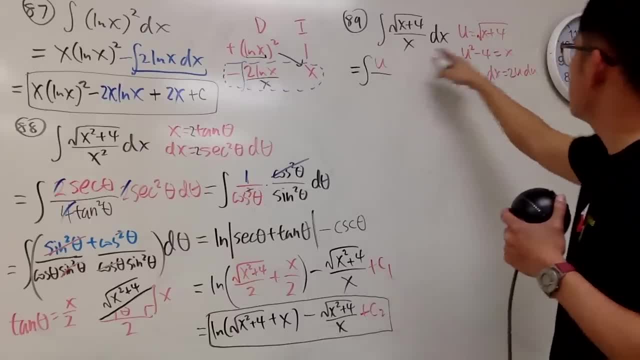 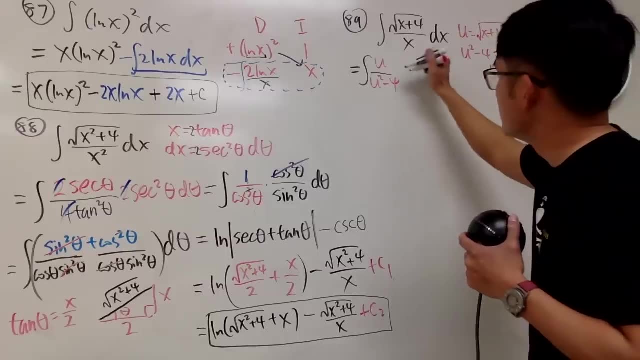 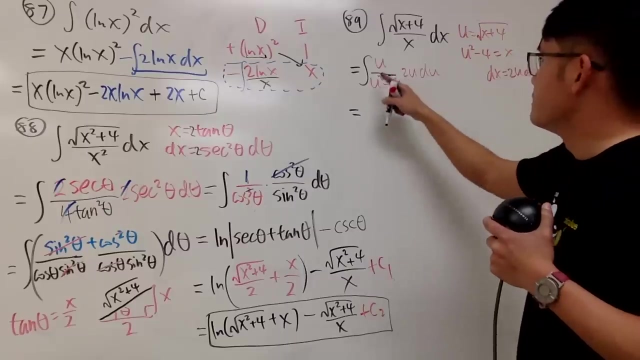 This is the integral On the top is u. On the bottom, x is u squared minus 4.. And then dx is 2u du. Okay, And then let's see, You get integral of 2u squared. 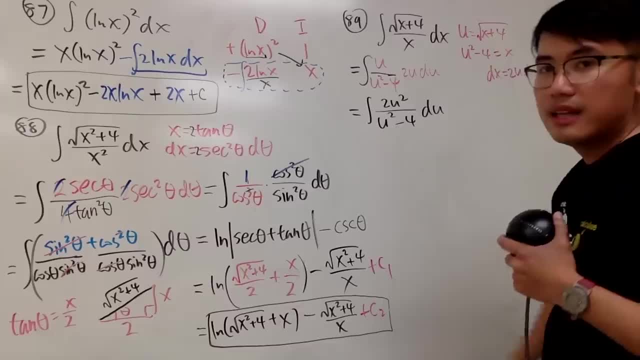 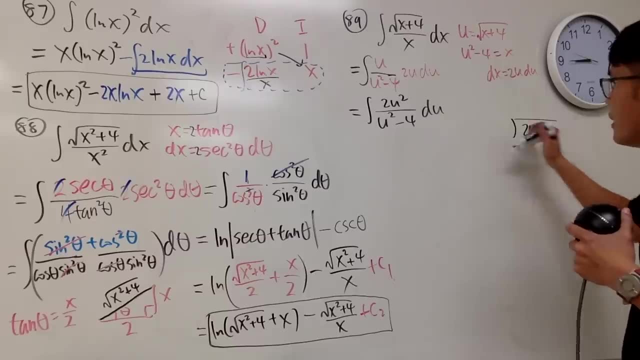 This times that u squared minus 4 du. Yes, We have to do long diffusion this time, So if you would like, you can just put it down on the side real quick. Let's put down 2u squared here. 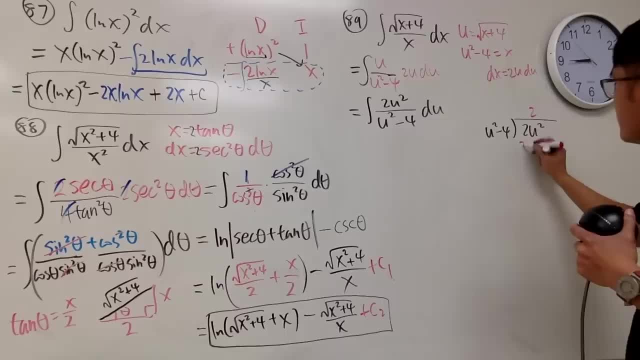 And then we do the u squared minus 4. outside You need a 2.. 2 times this is 2u squared minus 8.. Am I right? Yes, Yeah, And then this is going to be positive 8.. 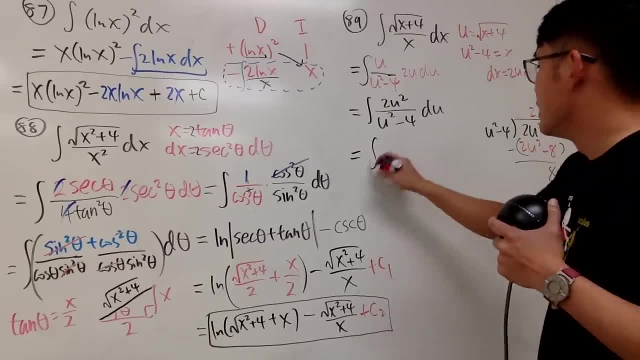 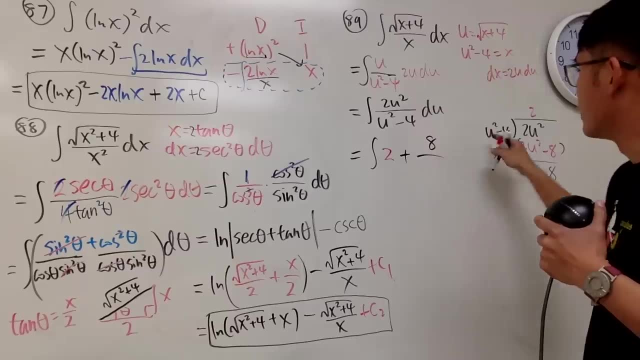 Right. So here's the deal: You have to integrate 2.. Okay, 2 is the number by itself, And then plus 8 over u squared minus 4.. And to do that, let's do partial fraction for this one. 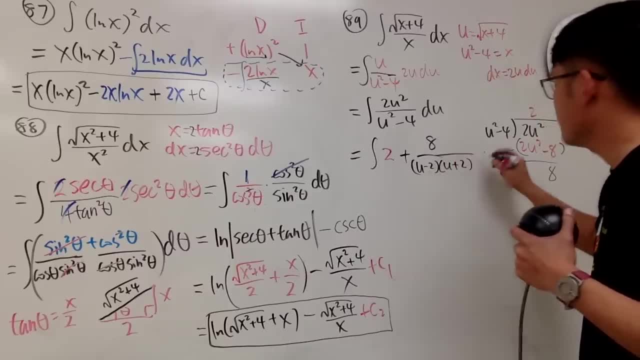 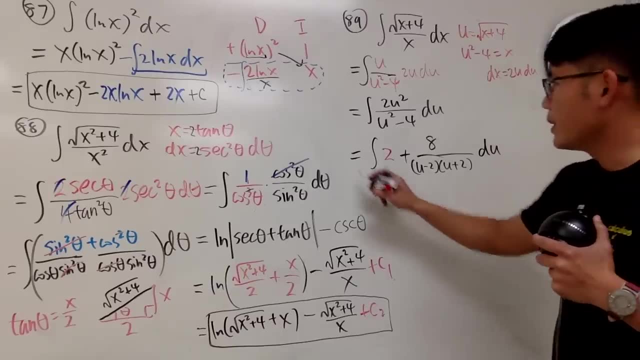 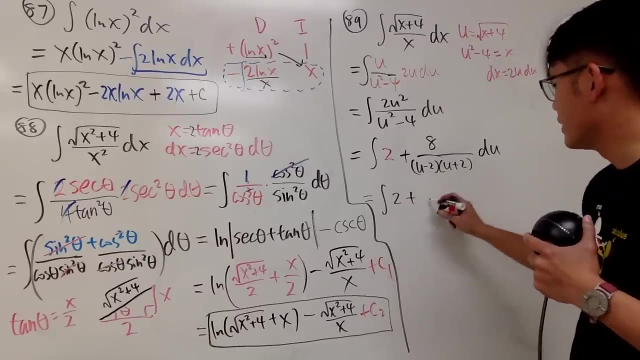 So u minus 2.. u plus 2.. Okay, And then, of course, we will have the du right there. Well, well, well, This right here is the integral of 2 plus Okay. Let's see. 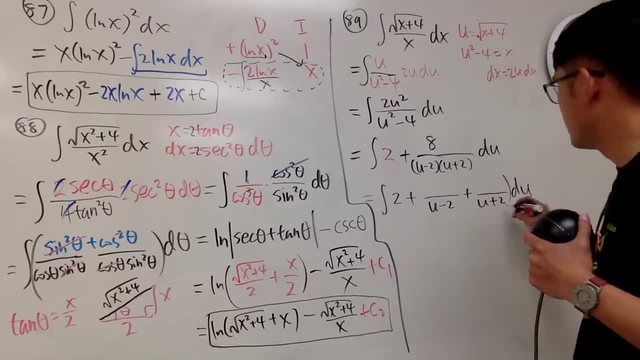 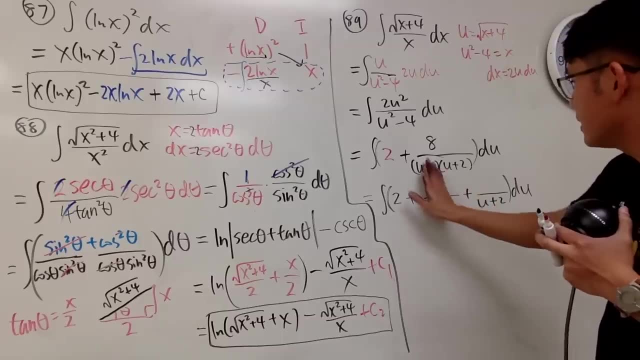 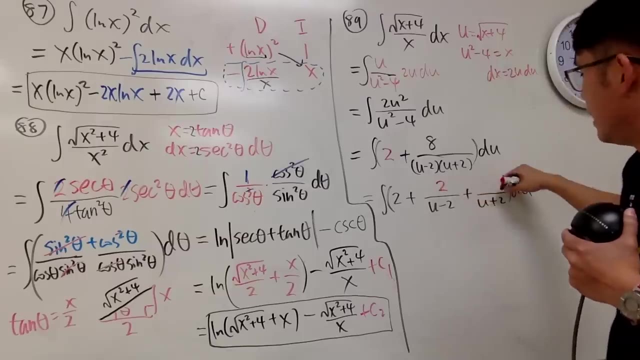 2 plus something with u plus 2.. du, Here is the deal. I will use my left hand or my right hand Cover this up. I need to plug in 2.. 2 in here, That's 4.. 8 divided by 4 is 2.. 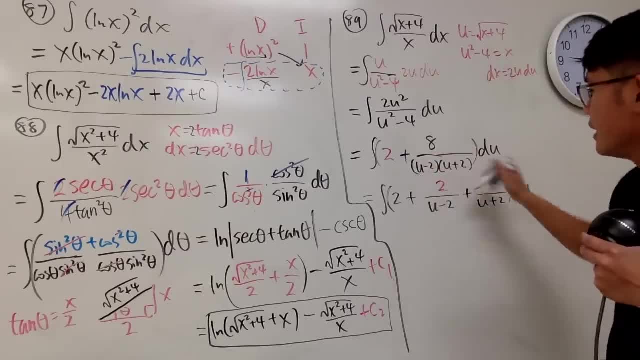 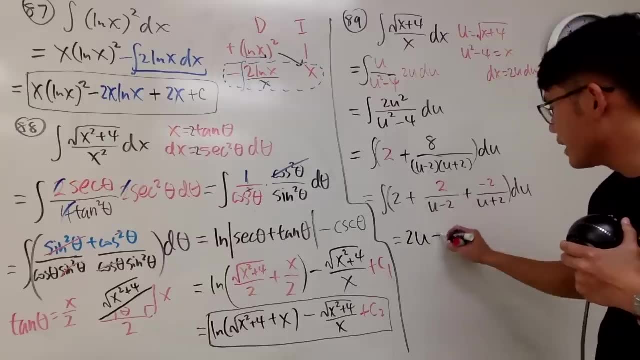 And cover this up. Plug in negative 2 here And you get negative 2.. It's not that bad, So here is going to be. We're just doing the? u world, though. So 2u Plus 2, natural log of absolute value of u minus 2.. 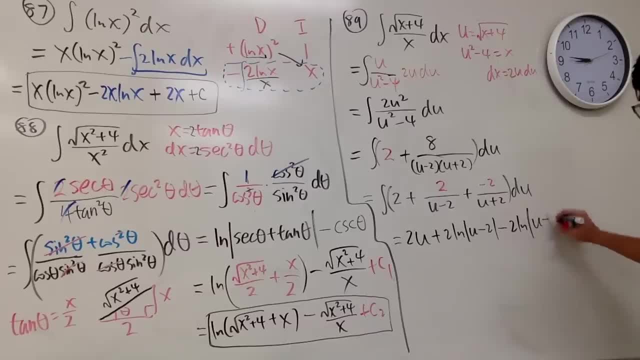 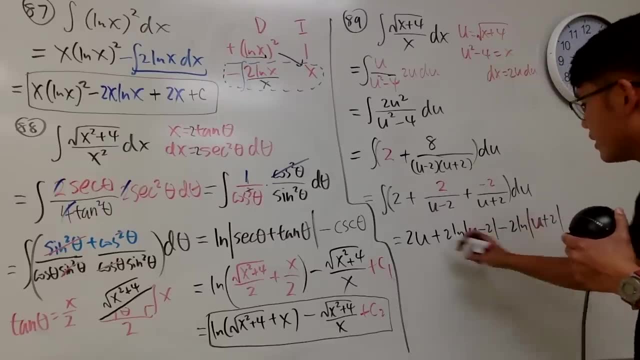 And then minus 2 ln, absolute value of u plus 2.. Finally, going back to the x world, So this right here, This right here And this right here, They all have to be changed. So I will say 2 square root of x plus 4.. 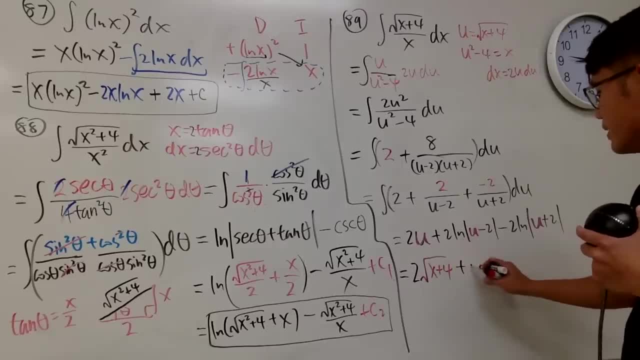 And perhaps let's just put this together: Save some space Plus 2 together And a natural log, And then the top is going to be this: Right u minus 2.. Which is this, Which is square root of x plus 4 minus 2.. 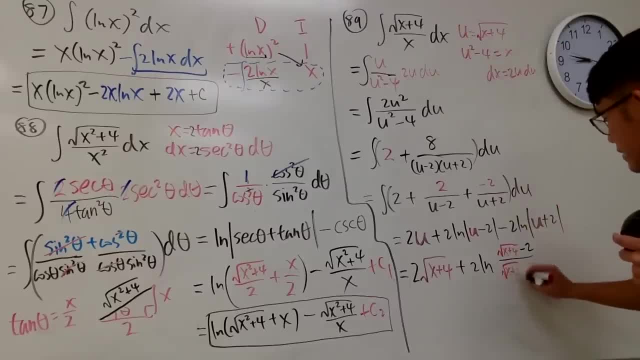 Over this, Which is square root of x plus 4 plus 2.. Like that, Very nice. And the truth is, When you have square root, This is going to be greater than or equal to 2. And you're not going to have 0.. 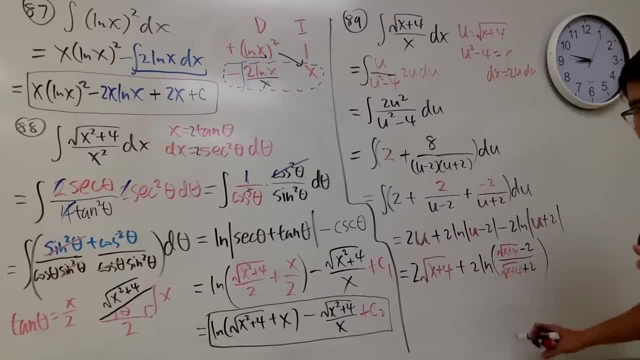 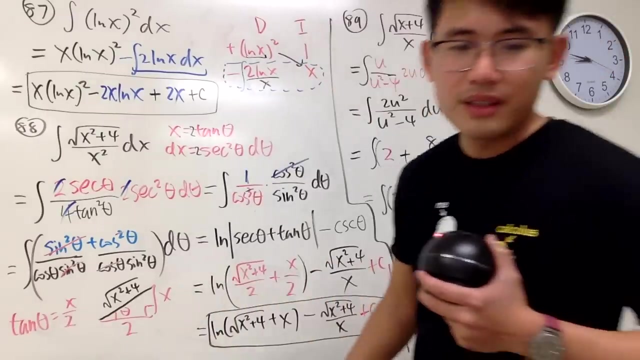 Don't worry. So just no negative Prentices is enough. And plus fish: Okay, Yeah, Done, Very good. Very good, Steve. you are doing good. Steve, this is good. Okay, You can do this. 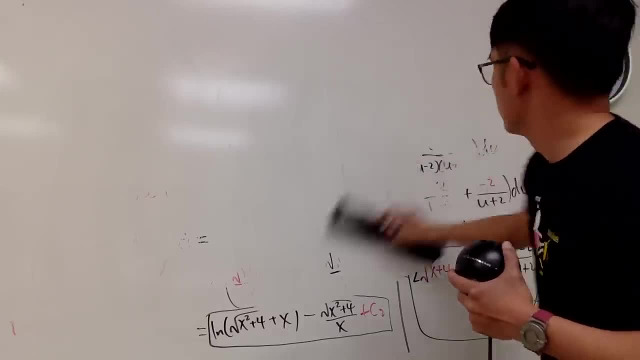 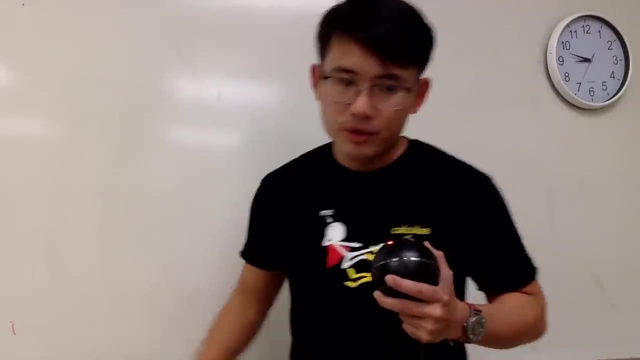 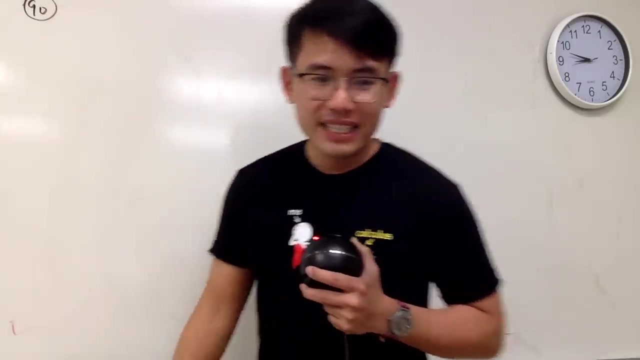 Okay, Okay, Okay, Okay, Okay, Okay, Okay. 10 more questions. No, actually Depends how you count. 11 more questions. Number 90.. Oh my god, This right here. Integral 0 to pi over 2.. 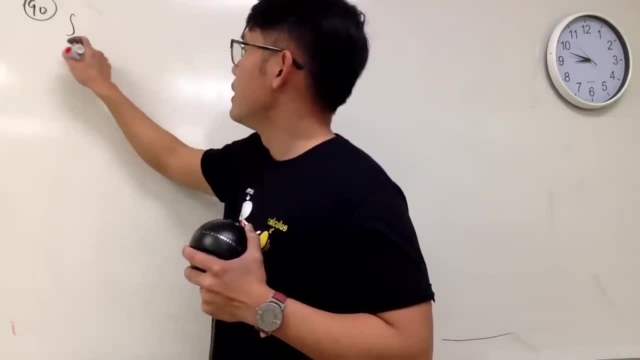 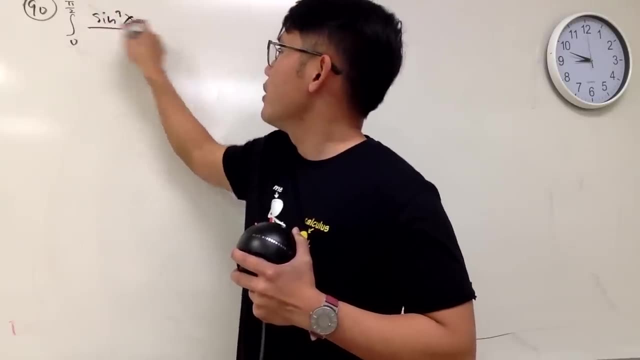 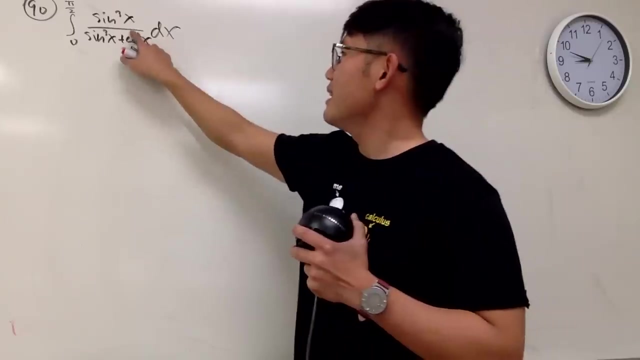 Right Integral from 0 to pi over 2.. Yes, you can see now the third power x over sine to the third power x plus cosine to the third power x dx You serious? Somebody put this question right here. This is actually very easy The answer. 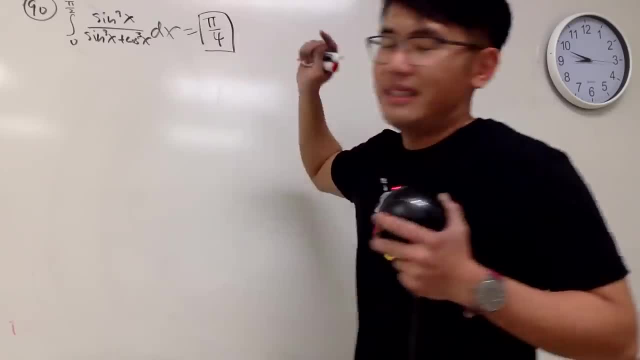 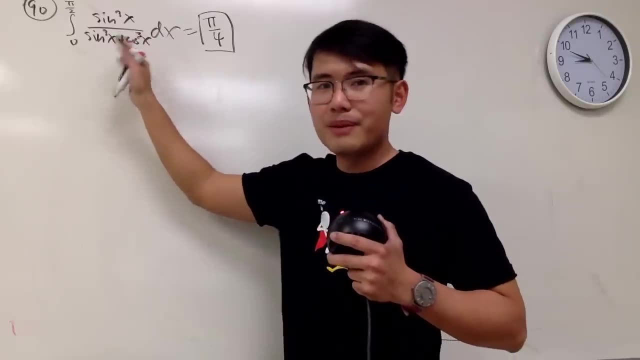 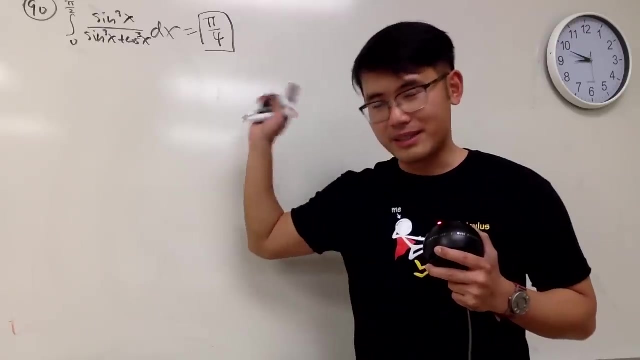 to this is pi over 4.. See this question all the time. You can do this by experience. This is the answer. if they are the same, If it goes from 0 to pi over 2.. This is a famous question. You can just put down the answer being pi over 4.. I don't know if you remember. 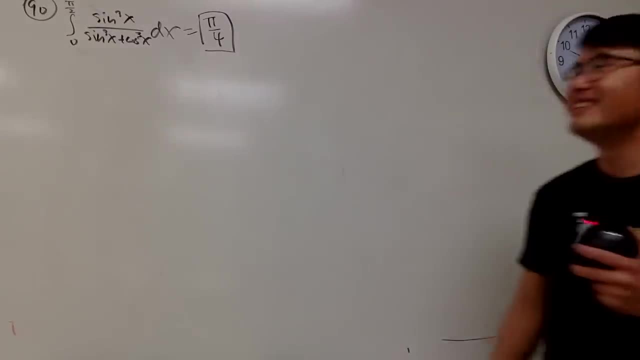 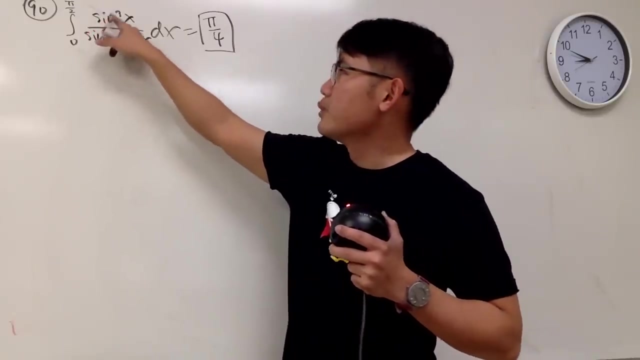 what I said: Put down pi over 4 and then walk away. Detailed explanation will be in the description, but the idea is that in fact, if you have cosine to the third power, x on the top over the same denominator, they have the same value: This integral and that integral. 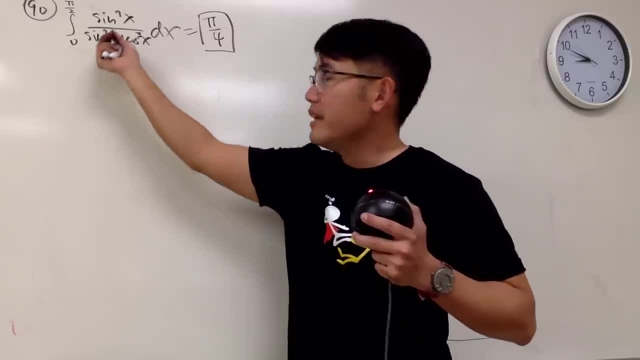 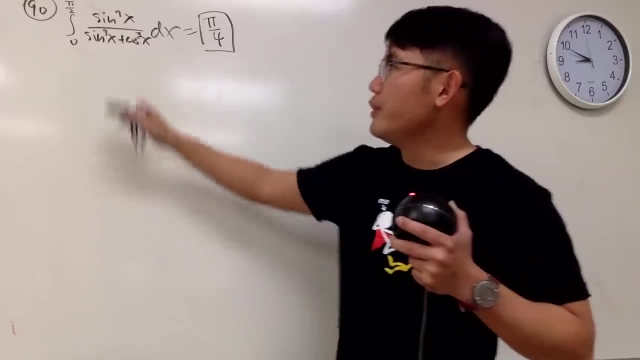 are equivalent. You can add them up and you can reduce the integral inside the integral to be just 1.. And when you add them up you have two of them and if you integrate this with the one inside from 0 to pi over 2, you end up with pi over 2 for the area, But it's two of them. 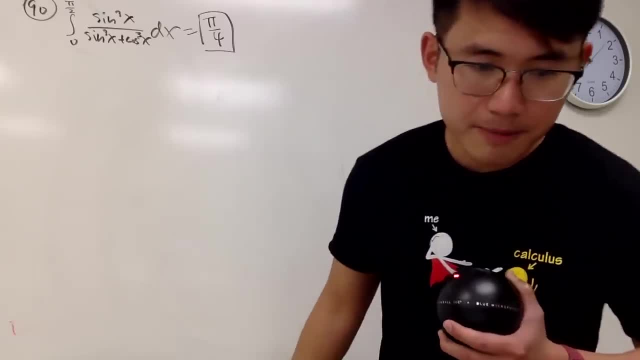 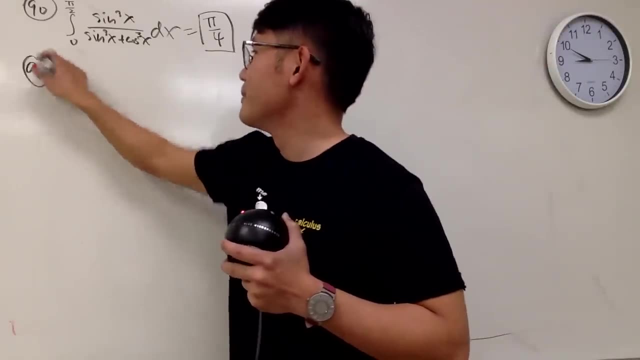 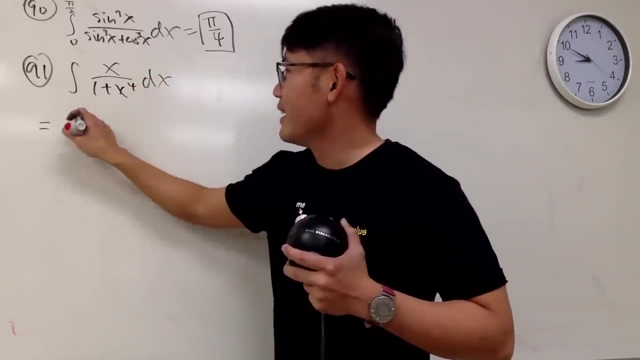 so each area has pi over 4. area Done Ah, number 91.. I love this one. Okay, I love this one, Number 91.. x over 1 plus x to the fourth power. So nice, Why, Okay? 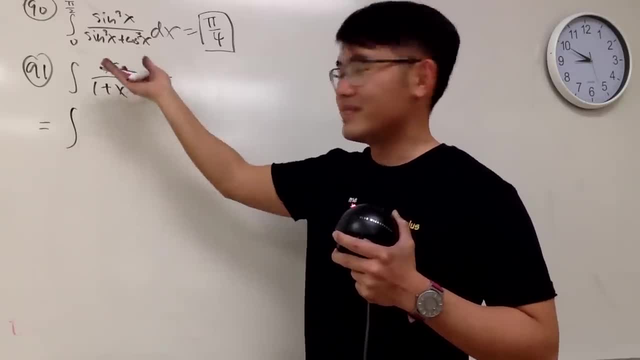 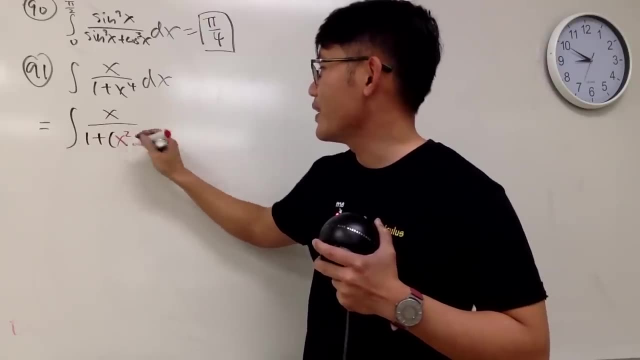 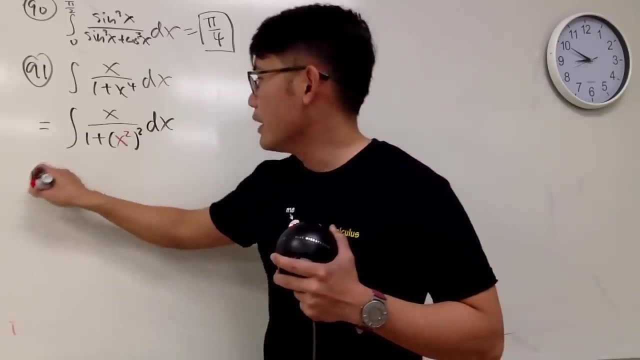 I wish, I wish you have x squared somewhere. So the derivative of x squared is 2x. You can get rid of the x right here, right Well, I produced the x squared myself by looking at the x to the 4x squared. How's that Cool, huh? Right here you let u equal to this And, of course, 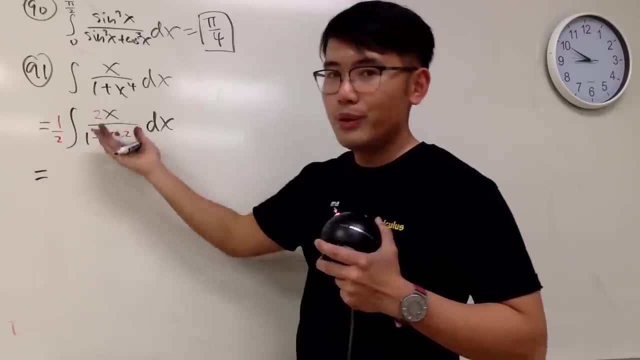 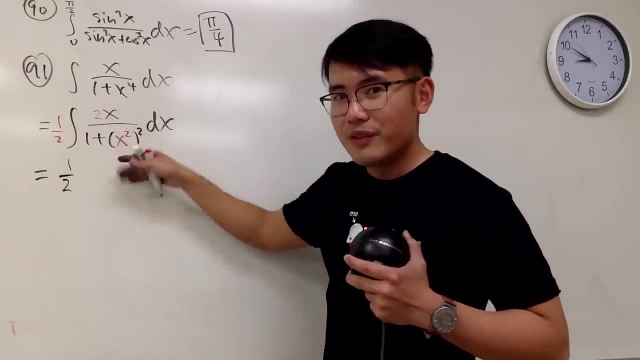 you need 2x so you can put down 2 right here. divide it by 2.. So you have the answer as 1 half. Again, this is going to be the inverse tangent form, if you let u equal to this. okay. 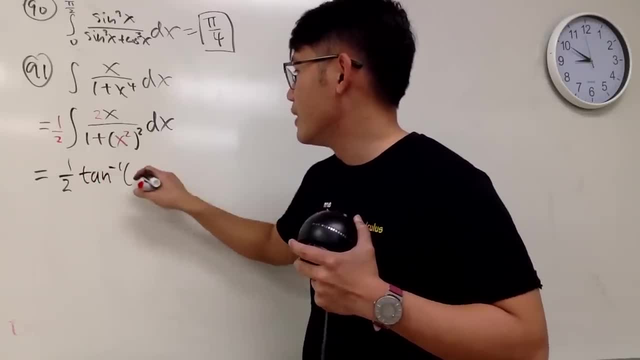 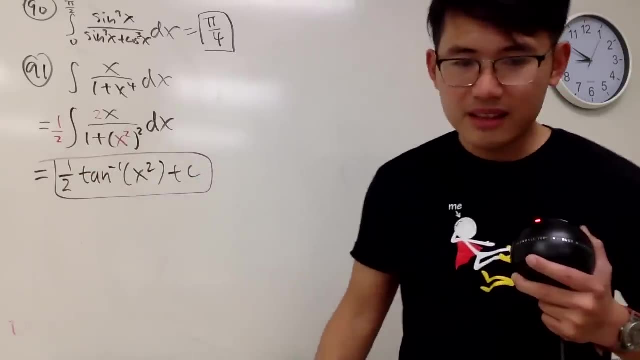 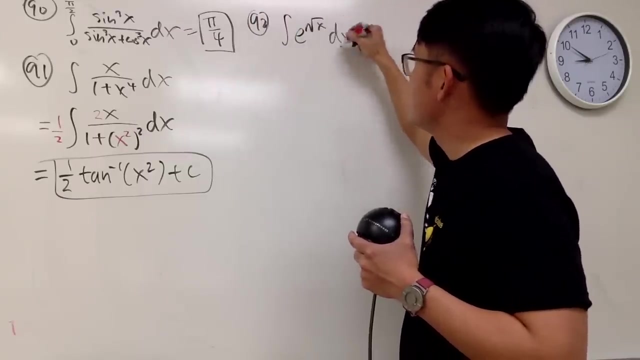 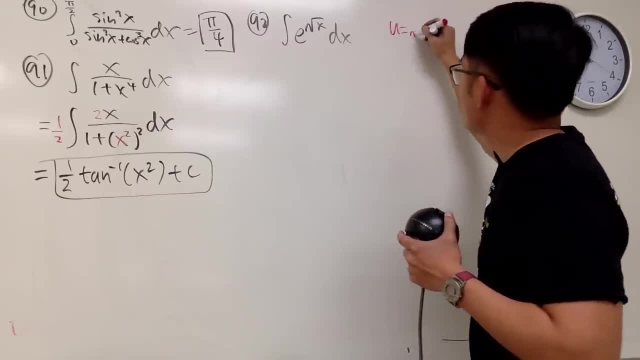 sub first and then do integration by parts. So we will u equal square root of x. x is equal to u squared, dx is equal to 2x, And we get the inverse tangent of x squared. Okay, You want this right Then you then integrate by parts. but you know you do because u is. a square And u gives a square root of x where x is greater than u. squared instead of x, But they're the two, right? So it's going to be the total force. We're going to integrate the y lambda, okay, And we do one divided by y into u. So we'll do one divided by x plus indeed. 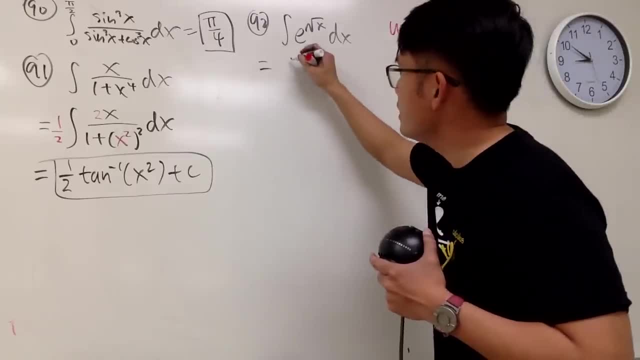 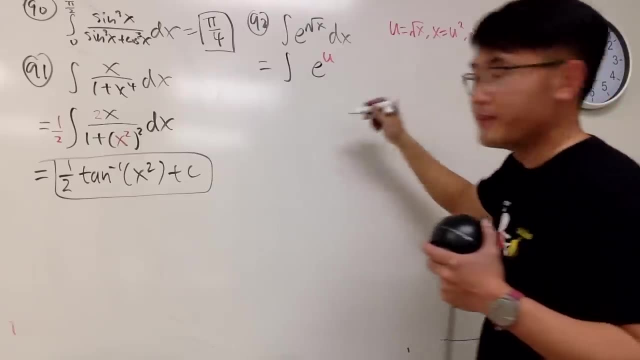 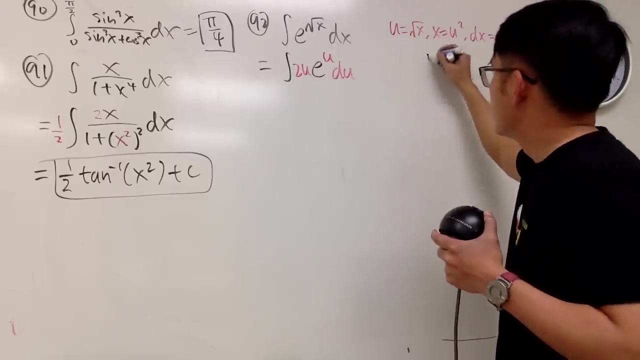 is equal to 2u du and you see this is going to be integral e to the u and then dx is 2u du. so you can put down 2u here, du here, and then you proceed with integration by parts d and then i, and then you are going to integrate, you are going to differentiate 2u and you are. 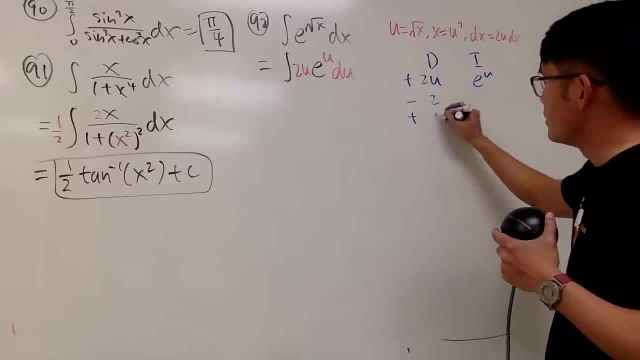 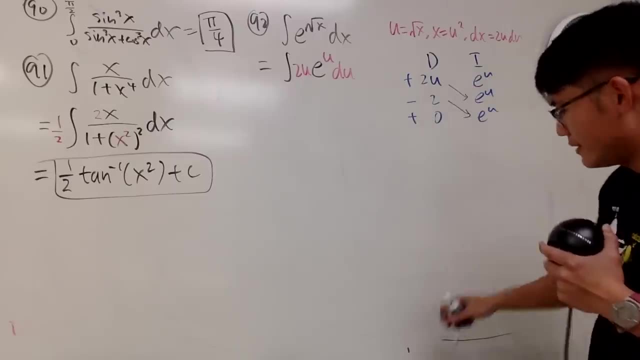 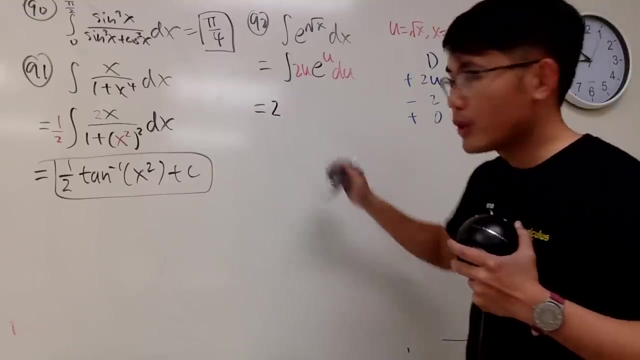 going to integrate e to the u plus minus plus, because this will be 2, this will be 0, and then e to the u is always e to the u. very nice answer, hello, right. so the answer is: ladies and gentlemen, 2u times that. and do we know what u is? yes, we do. u is square root of x, so put on that the square. 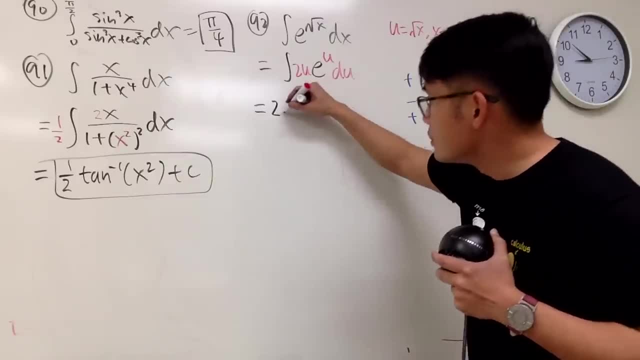 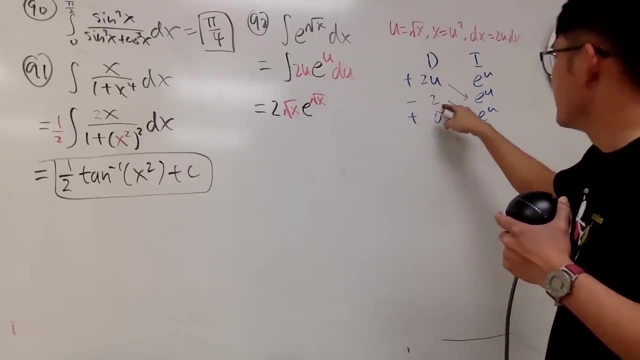 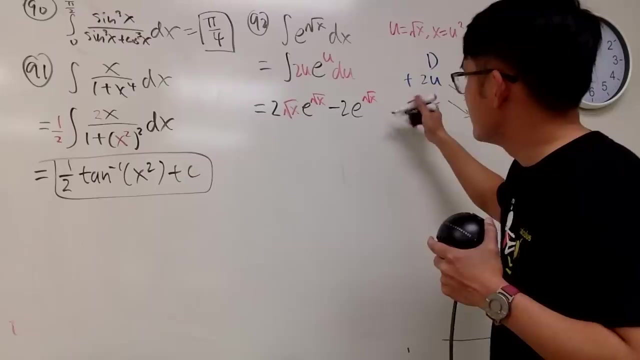 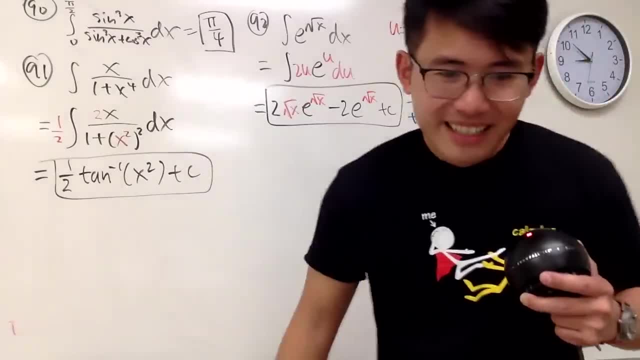 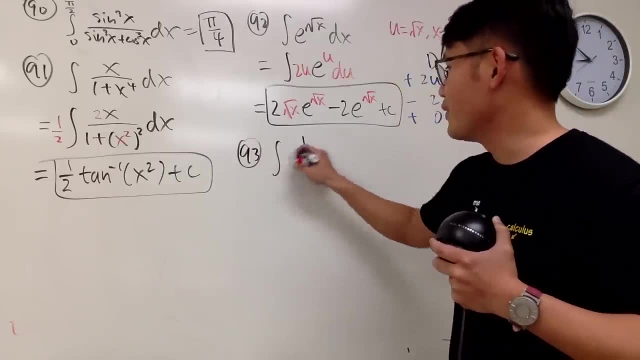 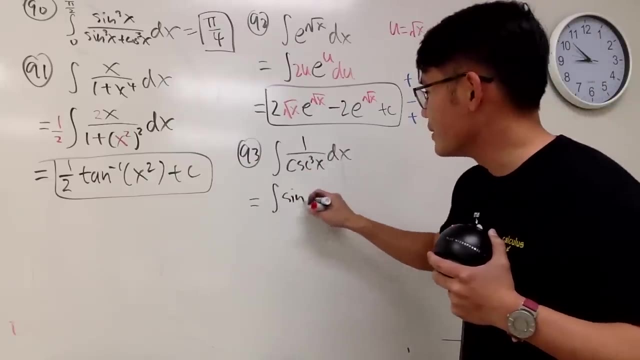 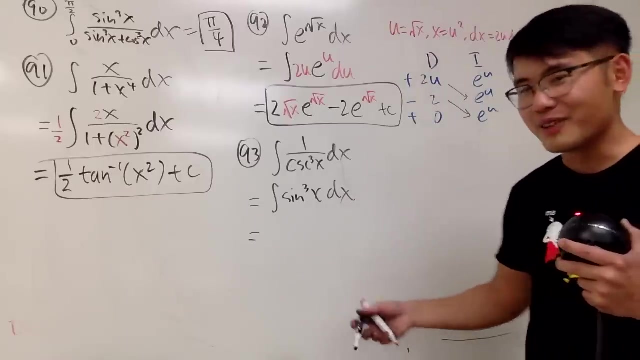 okay, number 93. oh, this is my favorite as well, one over called secant cube x dx. yes, this is just nicely equal to the integral of sine, to the third power x dx. and yes, one of this is one of my old videos. yes, over a lot of views. i don't remember how many, but the way to do is you look at this. 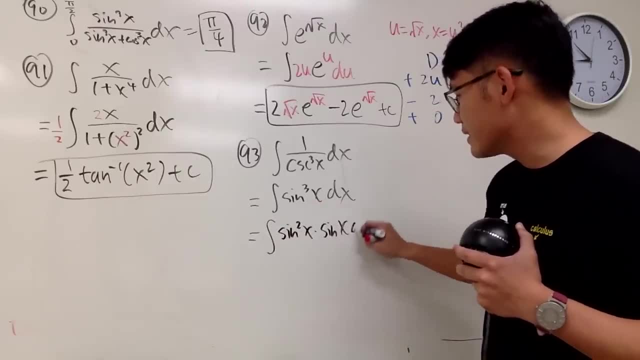 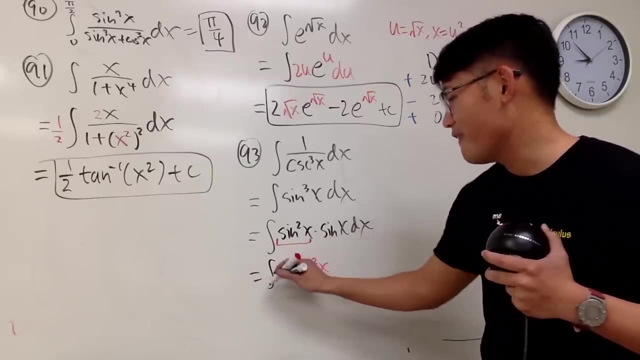 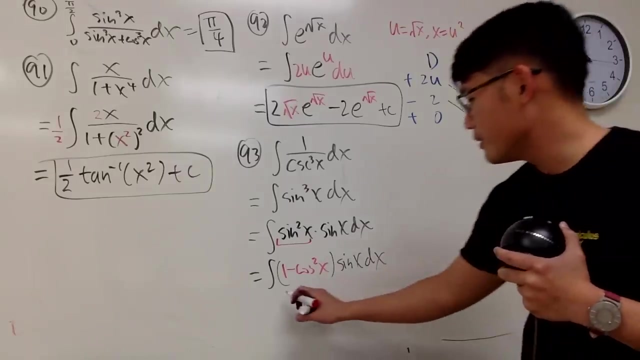 look at this as sine square x times sine x- dx. look at this as what? this right here as 1 minus cosine square x, very, very good. and then you have the sine x dx. and then you take a little u sub right here. okay, you just let u equal to cosine. but uh well, since i i have a lot of. 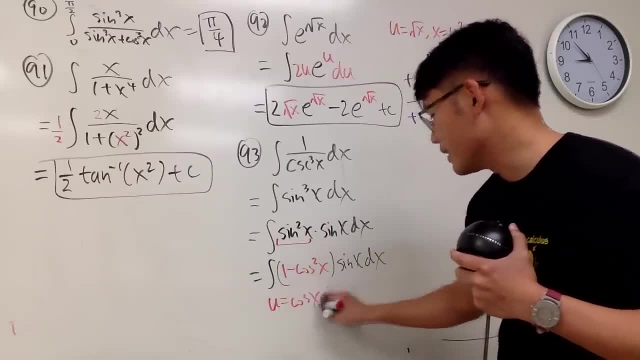 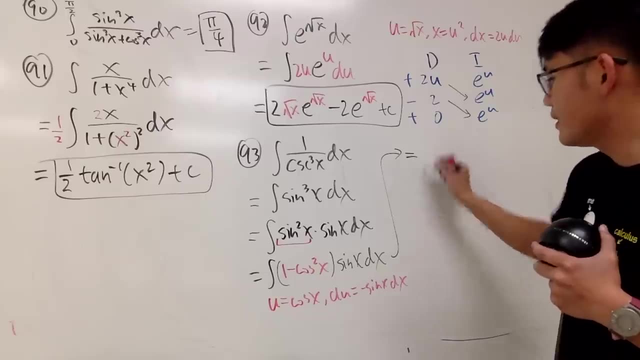 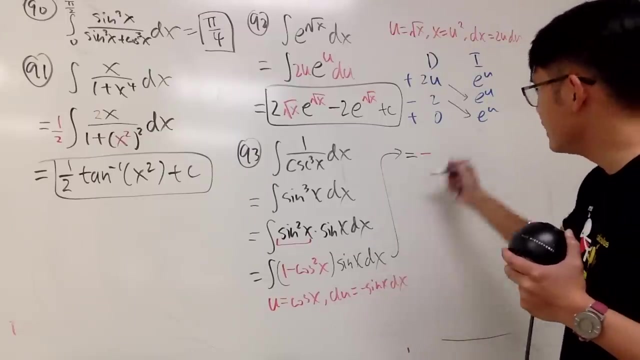 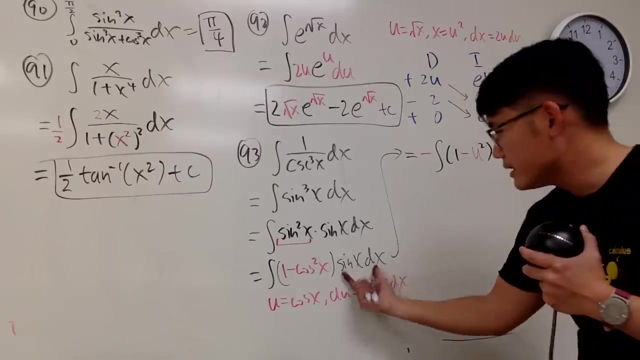 this one, let's. let's do this one, i'm more. cosine x du is equal to negative sine x- dx. so another integral sign this right here. you should have the negative right here. okay, i have a negative right here already, and then that's the integral of 1 minus u square, and then this with the negative. 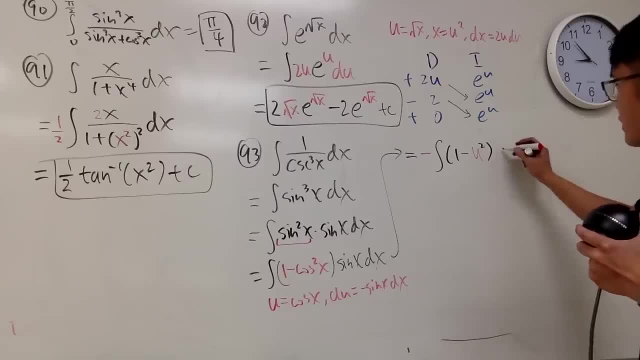 in the front. we have the du. okay, So we have the du. You can just divide the negative on both sides. That's another thing. So negative du is this. Anyway, negative parentheses integrated out: is u minus 1 over 3, u to the third power. 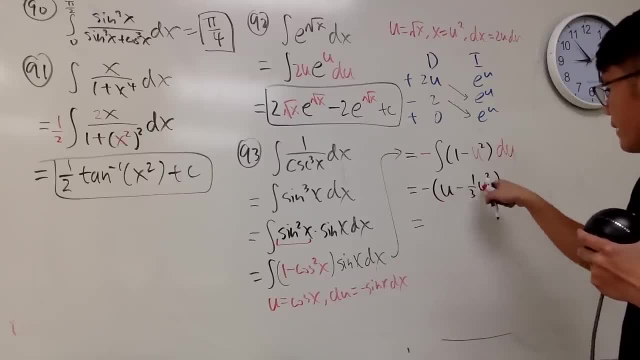 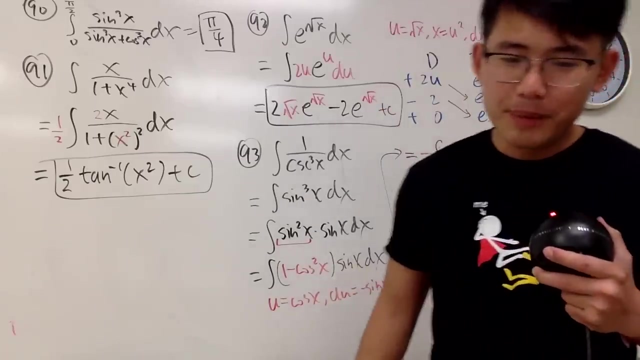 And u is cosine, So distribute. In fact this should go first. So I say 1 third cosine to the third power, x, And then minus cosine x, like that plus c done. Yeah, to be honest, I actually don't know how many people will actually be watching this video and all that. 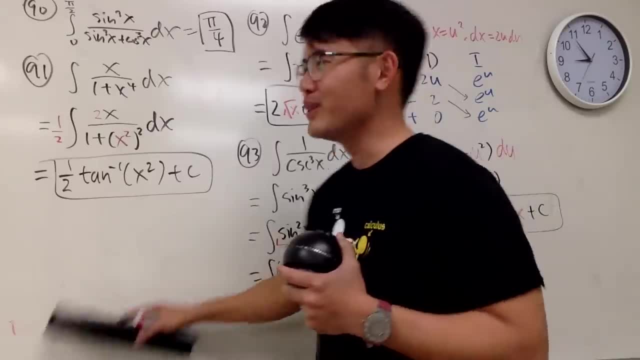 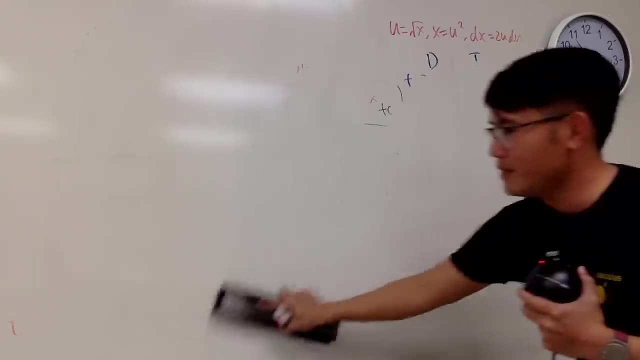 But I think it's fun. I can run marathons, I can do integrate-gen marathon, So of course you can try to beat me. Try to beat me, But don't beat me just by 1.. Seriously no. 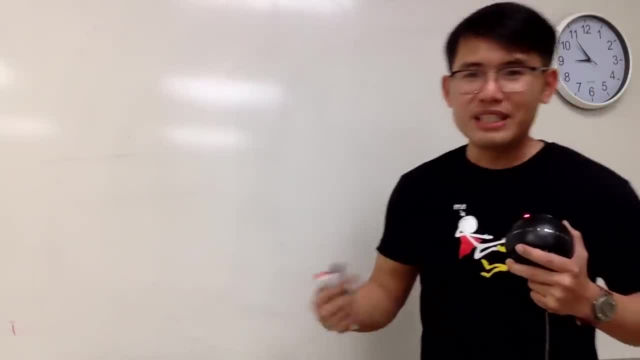 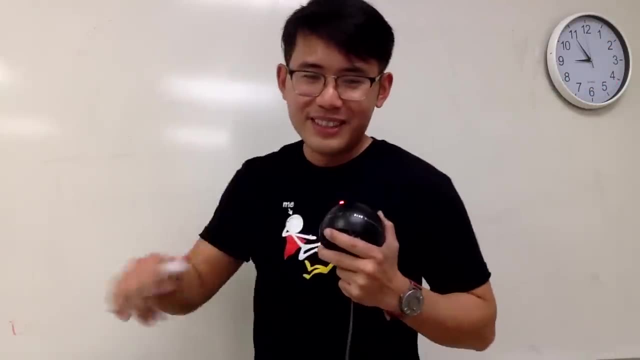 Beat me at least by 10 or 5, at least. And the deal is, if you beat me, I will try to beat you back. Seriously, that's not good to be healthy. So let's just well, let's just don't do that. 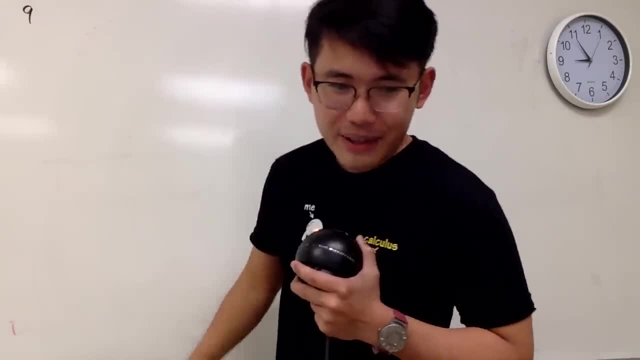 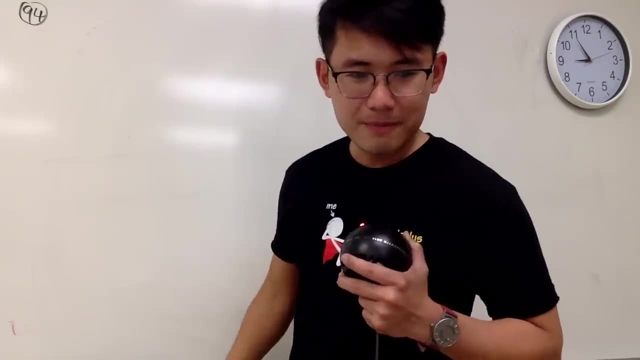 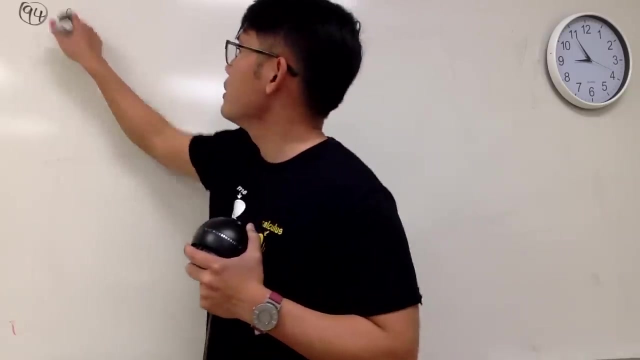 Anyway, 90 something, Question 90.. 4.. Oh my God, This is like mile 24 in my mirror zone. Hello guys, from my cell phone, My iPhone, Let's see Inverse sine, okay. integral of inverse sine x over square root of 1 minus x squared dx. 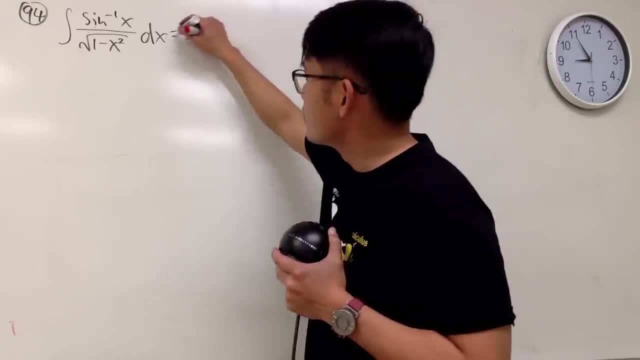 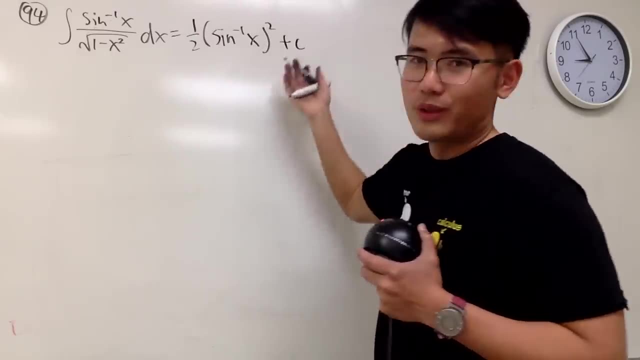 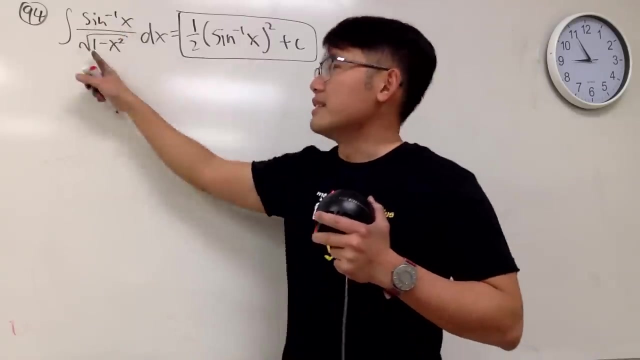 Is it easy or hard? Very easy. This is just going to be 1 half parentheses, with inverse sine x inside squared, And then we're done. I almost wanted to put down dx, Because the derivative of inverse sine x is precisely 1.. 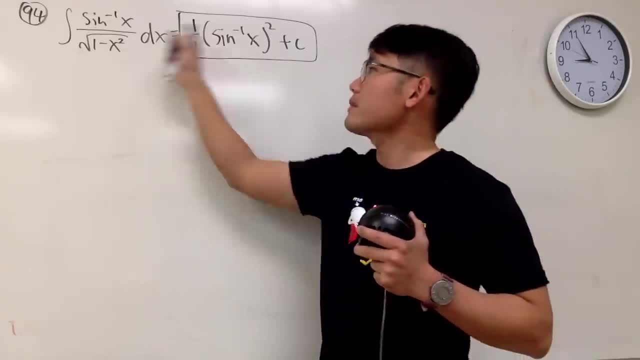 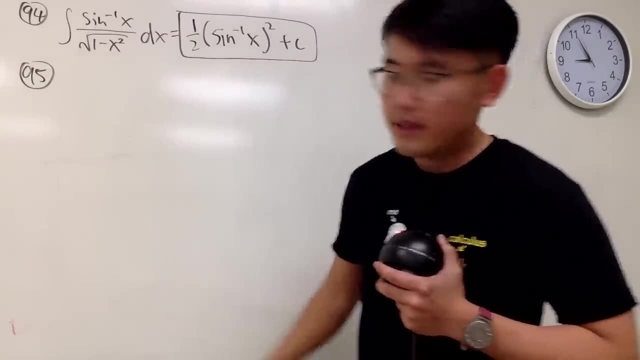 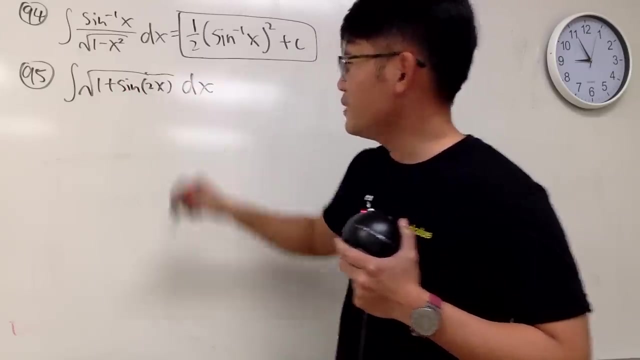 1 over square root of 1 minus x squared. So if you differentiate that, you'll get that Very good: 95.. Okay, 95.. Okay. integral of square root of 1 plus sine 2x. Seriously, 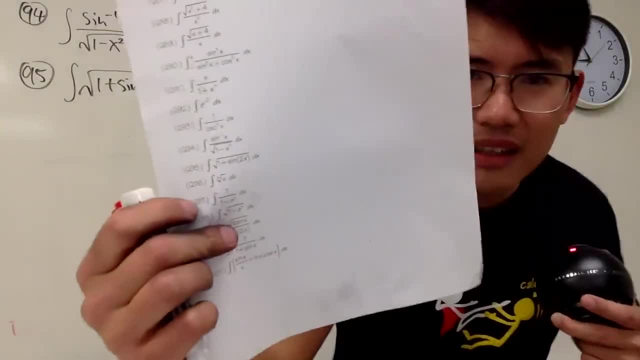 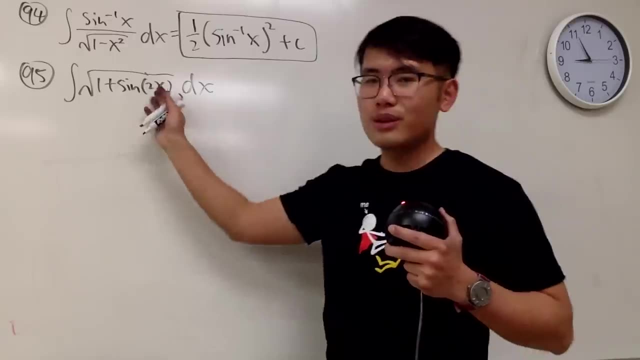 Wait, I put on 2.. I put on sine. I don't know if I should do sine. Yes, we can, We can. Yes, if this is the cosine 2x Here, it's pretty easy. We did that earlier. 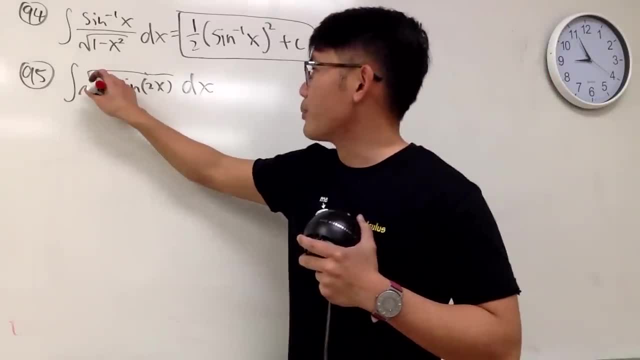 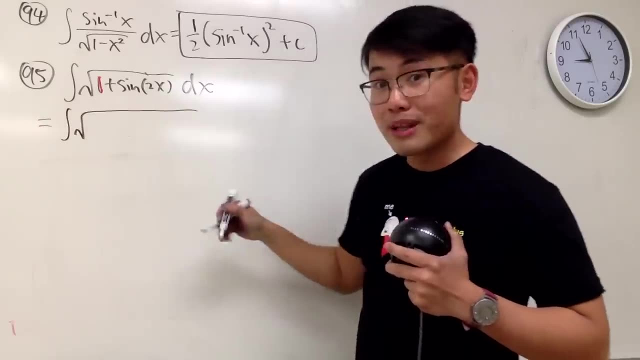 But if you have sine, it's just as easy. Let me show you how. First of all, I'll prove to you guys the following: okay, Look at 1.. And today 1 is pretty special. We'll look at 1 as sine squared plus cosine squared. 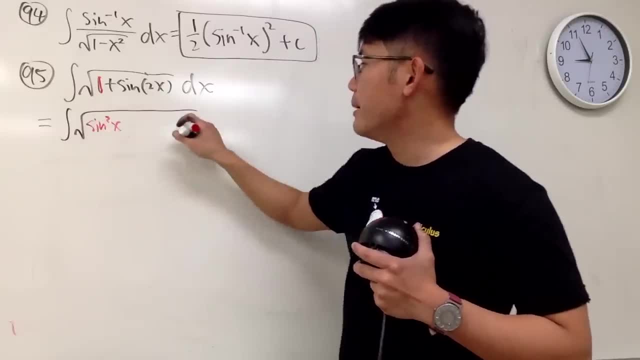 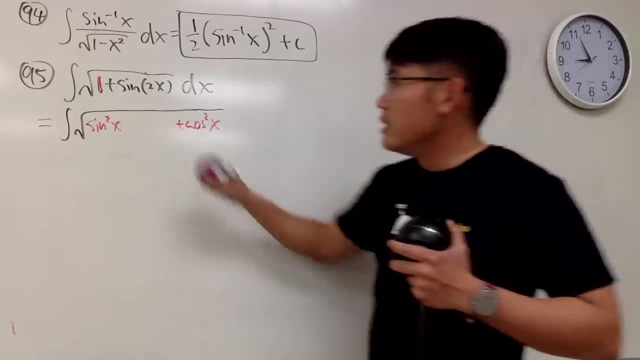 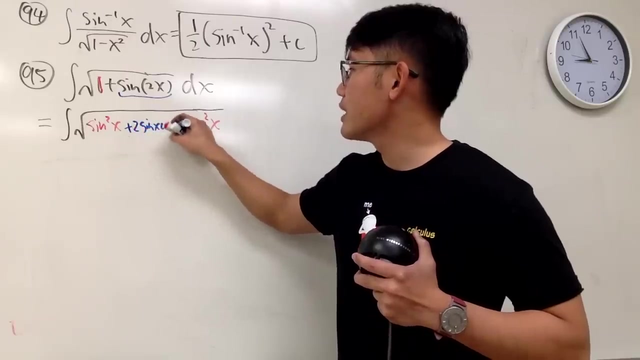 So this, right here, it's going to be sine squared x, and then plus cosine squared x. So we're okay, And this guy Plus 2.. Sine x, cosine x. What's this? Yes, it's a perfect square. 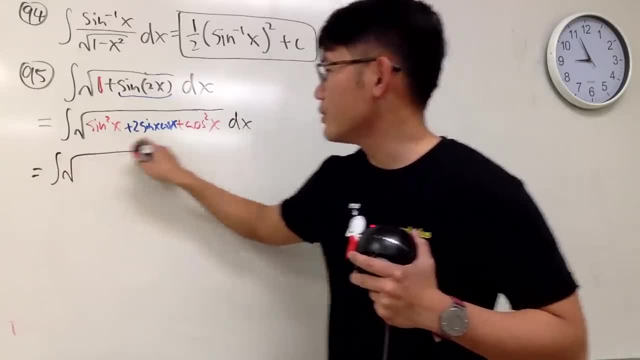 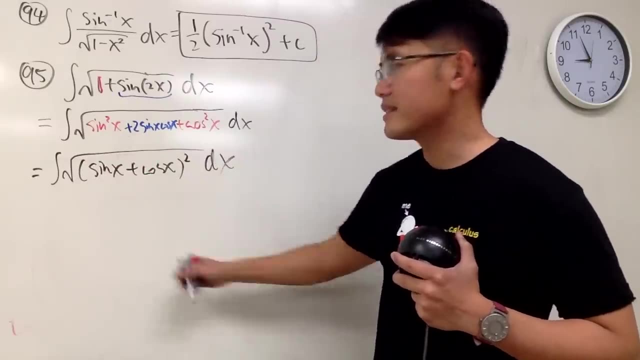 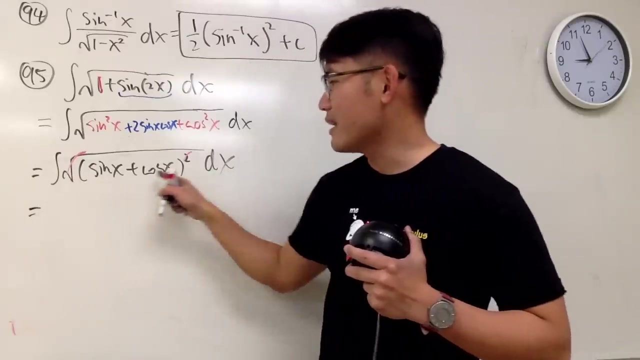 Very, very nice. This right here we have the integral of square root Inside. here we end up with sine x plus cosine x squared dx. Have we seen this earlier? Yes, we have. Okay, So cancel them out. So integrating sine and cosine. 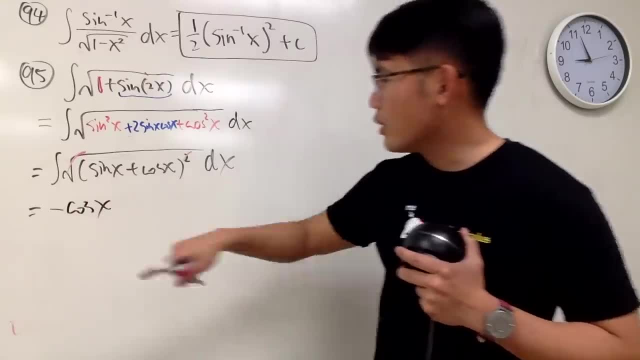 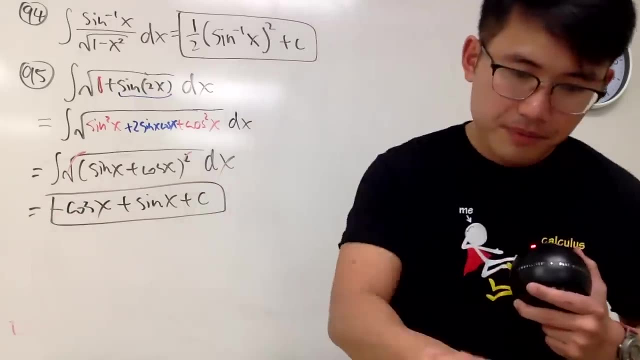 the integral of sine is negative cosine x, And integral of cosine is positive sine x. And then we are done: Plus plus z. This is it Number 96.. Yes, I want to finish happy, So I'll put the number 96 like this: 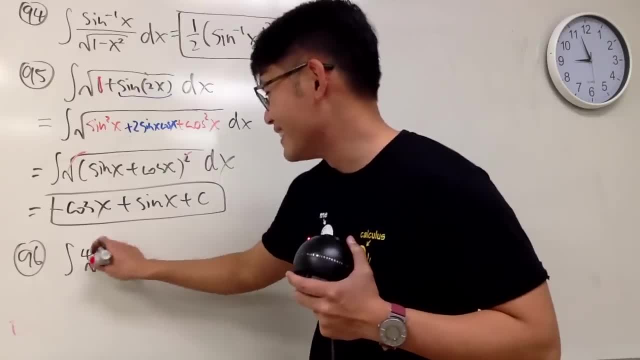 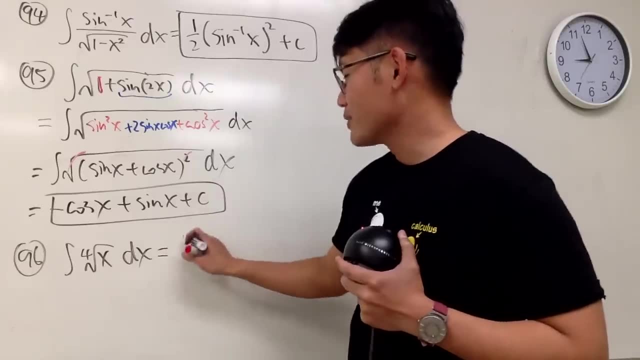 Integral of the fourth root of x. Okay, Don't be surprised that some people still got it wrong. okay, But anyway, let's see. Almost always we treat radicals as fraction exponents. So this is x to the 1 over fourth power, dx. 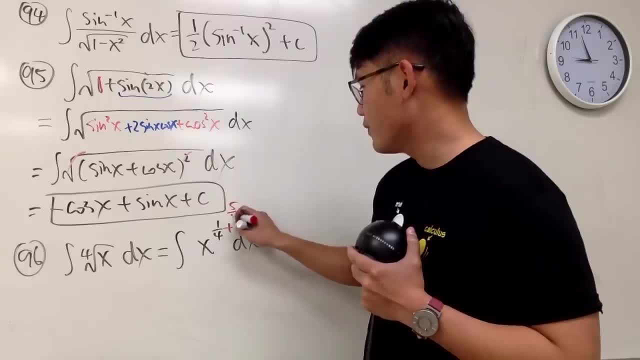 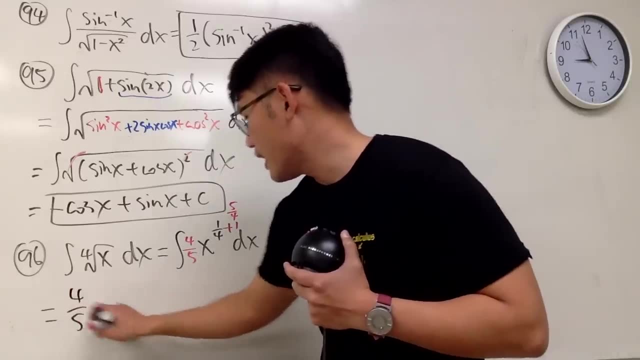 And what do we do? Yes, we add 1 to the power, which is 5 over 4.. You divide it by that power, which is 4 over 5.. And you end up with 4 over 5.. And now just keep this as the fourth root of x to the 5, like this: 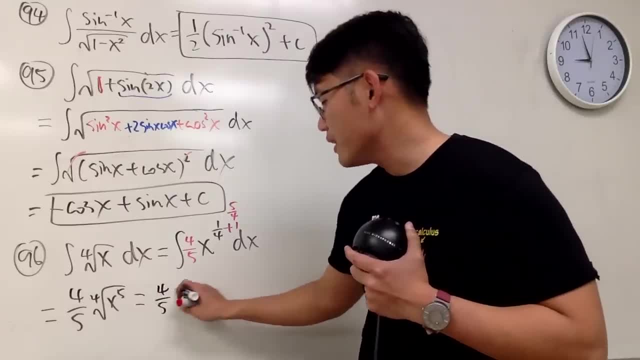 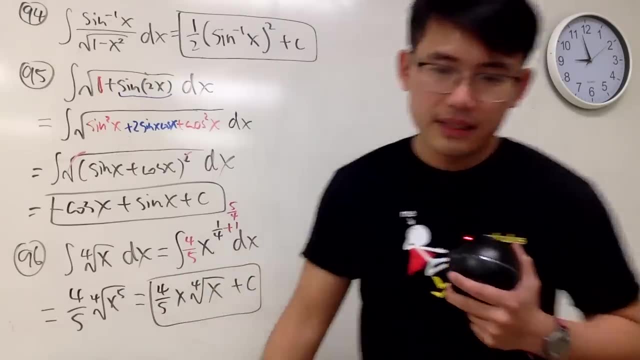 And if you would like, you can take out x, out 4 over 5x And then the fourth root of x, like that, Plus z. Okay, Okay, okay, okay. One of the ones that really got me famous. 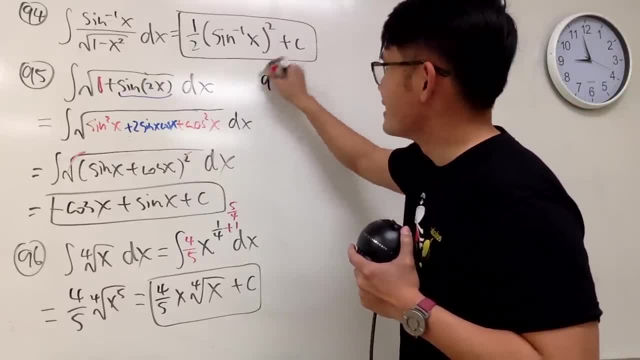 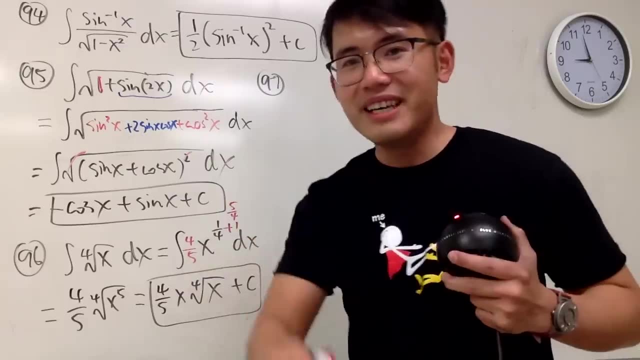 Got me a lot of subscribers on YouTube. okay, So number 97.. Oh my god, Almost done, almost done. How many 26 gig? Yes, I actually. right now it's 26 gig. okay, I actually saved. 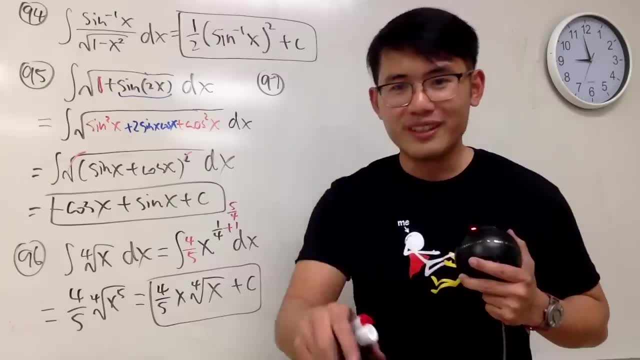 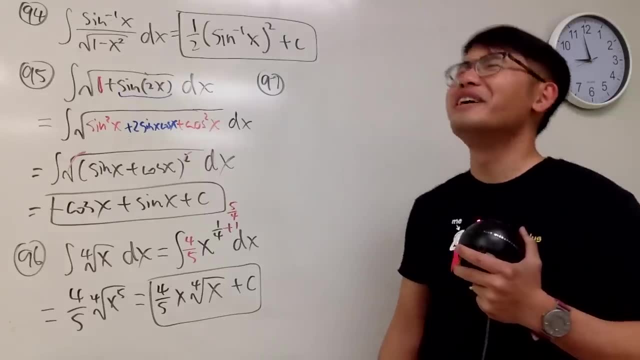 I cleaned up about like 47 gig to record this, So I have plenty of space, But it's 5 hours and 30 minutes. Oh my god, I can finish a marathon already, Seriously. oh my god, Number 97.. 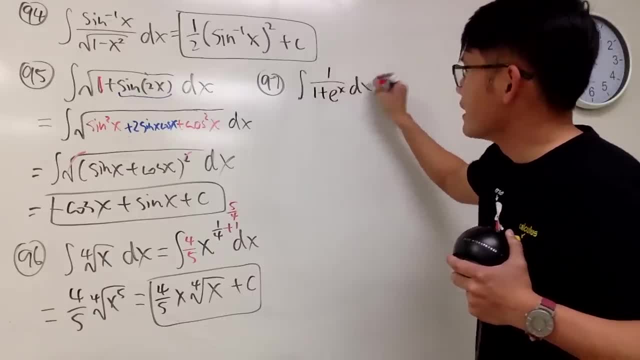 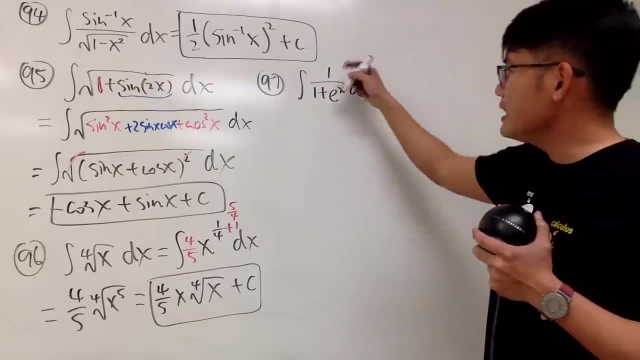 Integral 1 over 1 plus e to the x, dx. The way you do this is that you ask yourself: wouldn't it be nice? Okay, You start by asking yourself: wouldn't it be nice if the top is also 1 plus e to the x? 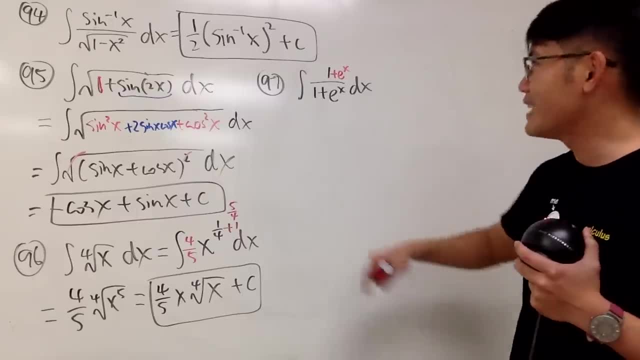 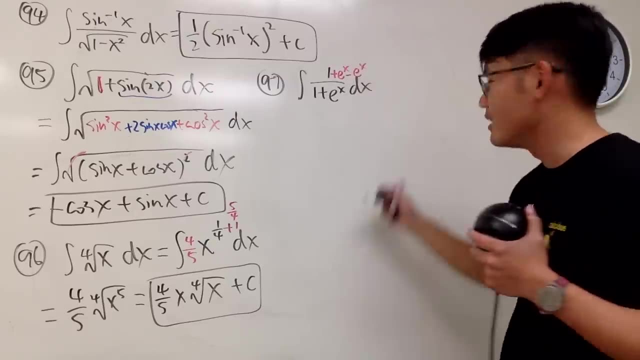 That would be so nice, isn't it? Because that would be 0.. But of course, if you just do that, you are going to change the whole thing. That's cheating, no, But it's okay. You can just minus e to the x and then, haha, everybody happy. 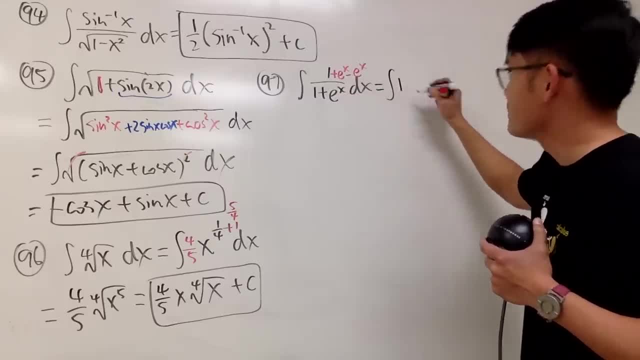 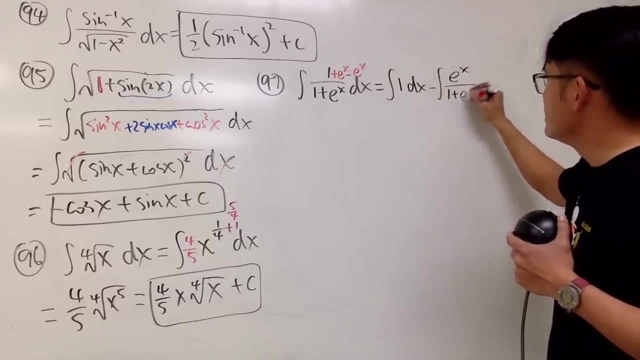 And then you will see this is just going to be the integral. This right here is just 1.. Preferably let's close that and then minus the integral E to the x over 1, plus e to the x dx. Very good. 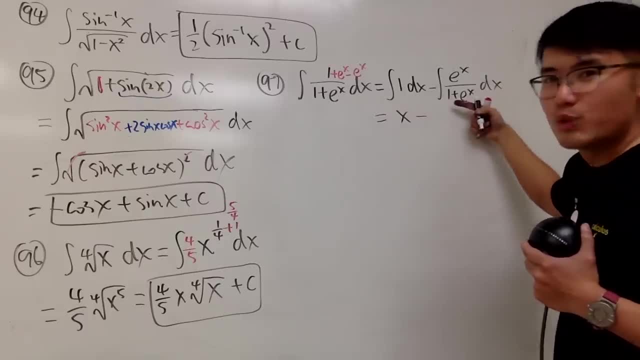 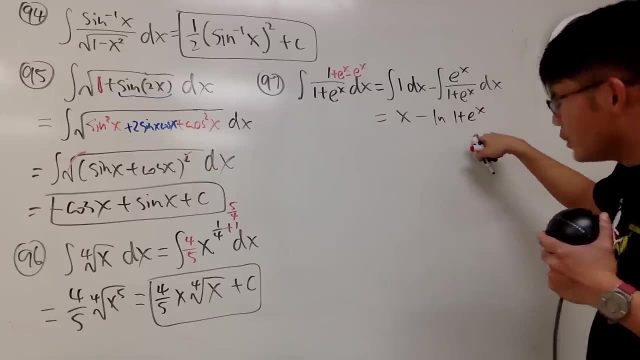 This, right here, is just x minus, this right here. Okay, The derivative to the bottom, precisely the top. So we get natural log, which is the denominator, which is 1 over, which is 1 plus e to the x. And by the way, I told you guys in Chinese, 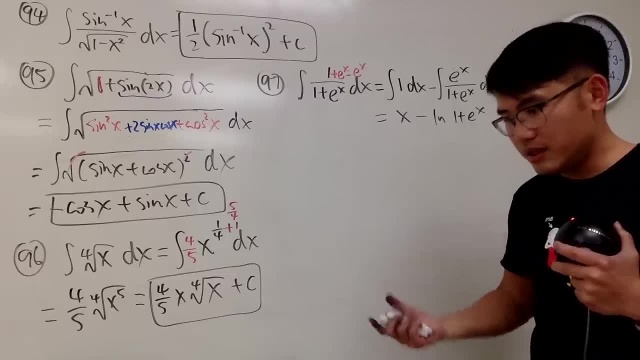 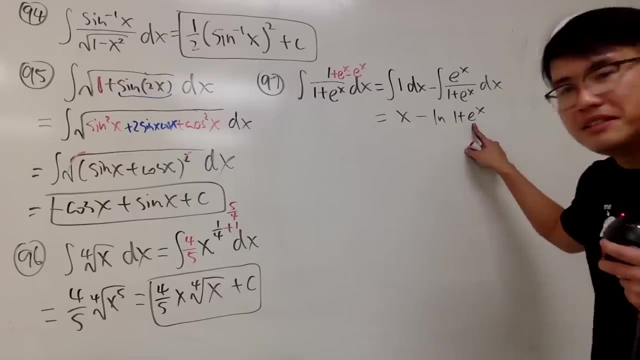 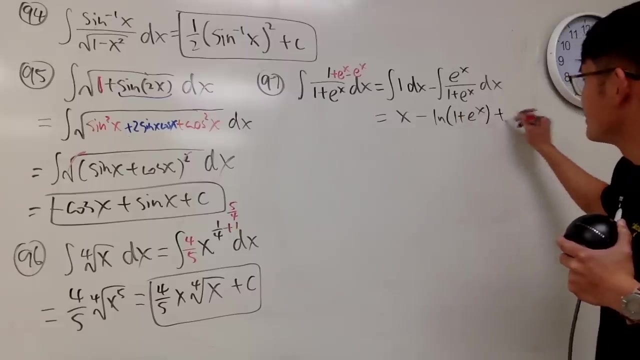 1 is e and e is also e. By the way, don't ask me to say e in Chinese. This is the English alphabet. You cannot say the English word in Chinese And some people will say: no black pen, red pen. you say that every single time. 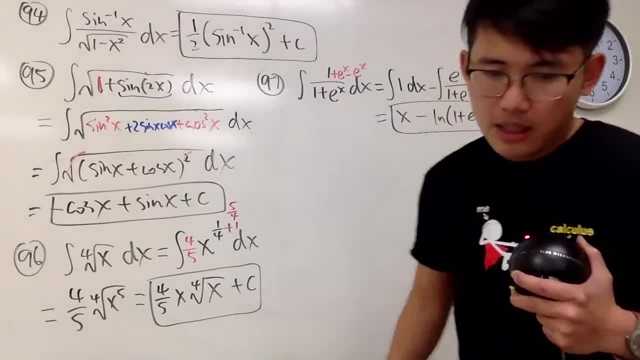 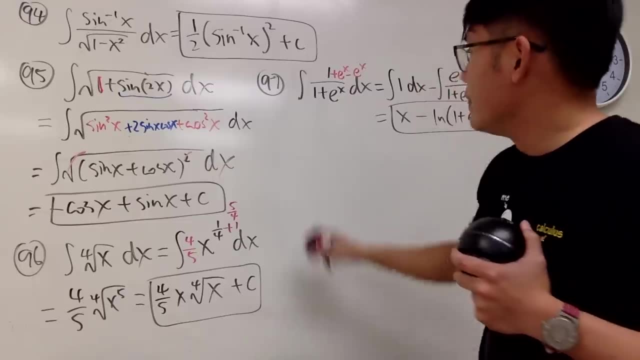 But you know, whatever man, That's it In fact. you have other ways to do it. You can also multiply the top and bottom by e to the negative dx, but I'll leave that to you guys. Number 98.. 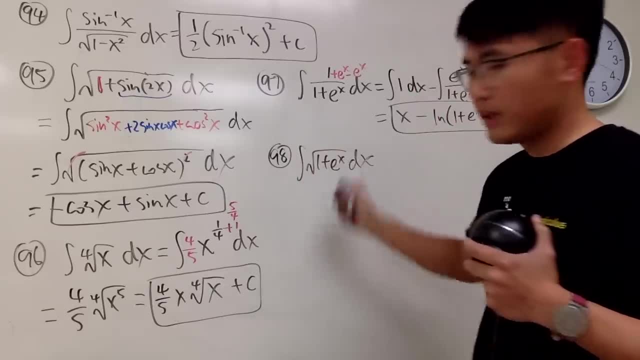 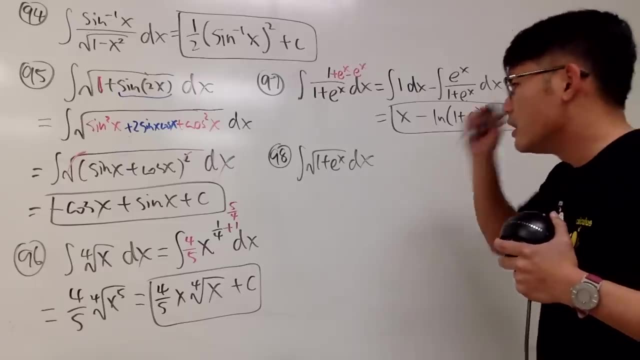 So I still have a hard one right here, Semi-hard one, okay, Let's see it like this: Square root of 1 plus e to the x. god, Ah, let's see I will say: do u equal the square root 1 plus e to the x? 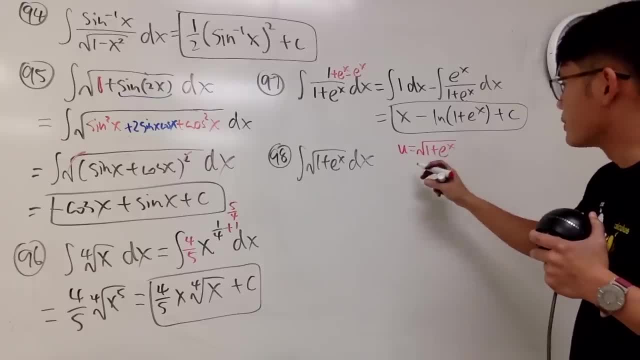 And then let's see, let's see Square, both sides, and then Actually let me show you guys this: That's differential, That du is equal to 1 over, Actually 1 over 2, square root of 1 plus e to the x. 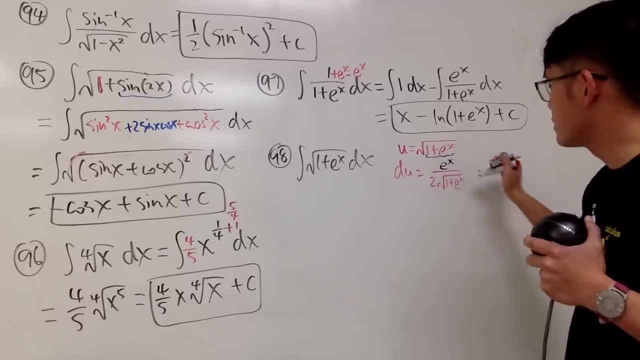 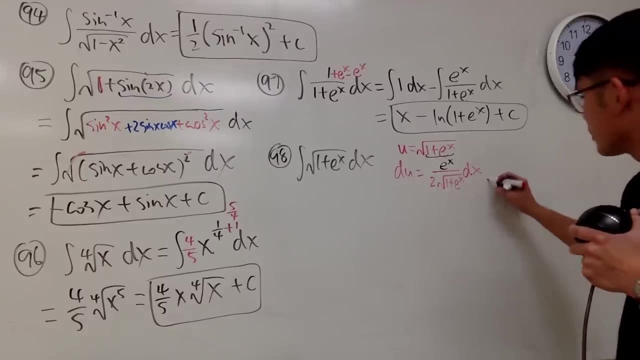 And then don't forget the chain rule. Use the chain rule e to the x. Shout out to Dr Pi Yan. So I have this, and then you know that, Let me just write it down right here: dx is equal to: 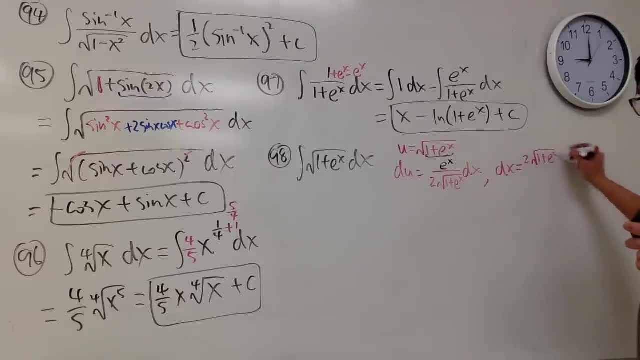 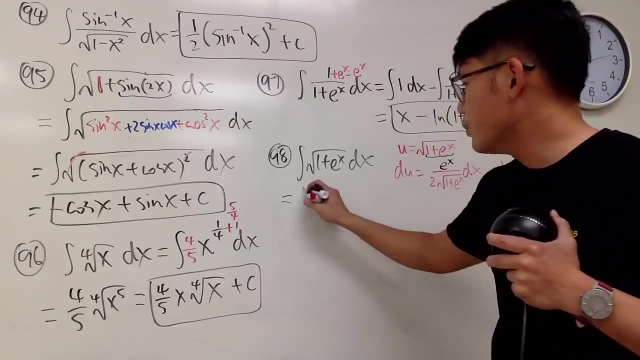 Put this on the top 2 square root of 1 plus e to the x over e to the x du. All right, now take this to the? u world. This is going to be integral of u times. dx is all that which is. 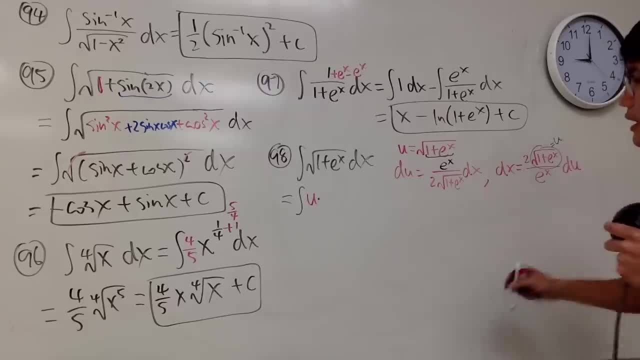 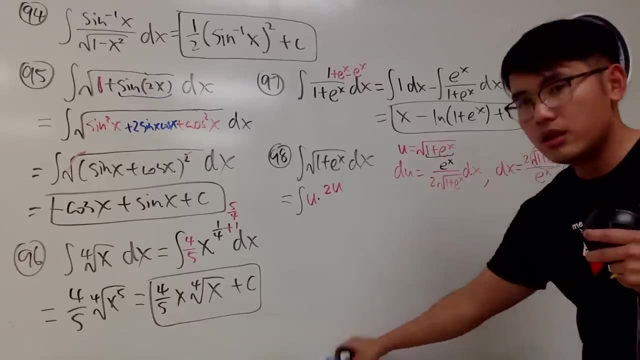 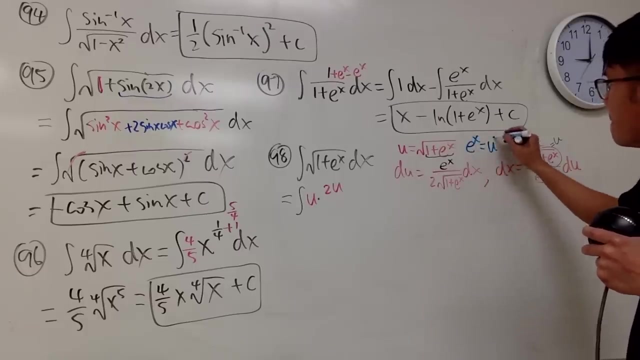 Okay, take a look, This guy is the same as u. okay, So we have 2u on the top, And then e to the x. is what though? Well, don't worry, Take a look right here: Square both sides minus 1, both sides. e to the x is equal to u squared minus 1.. 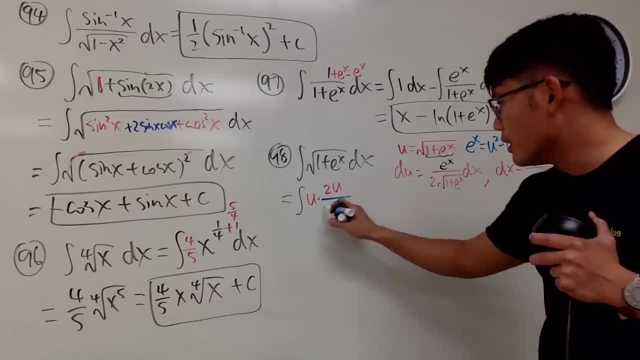 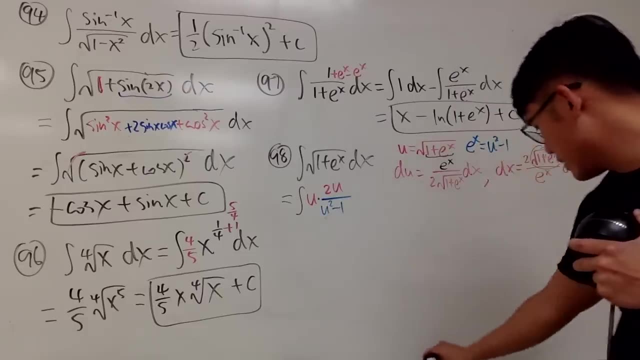 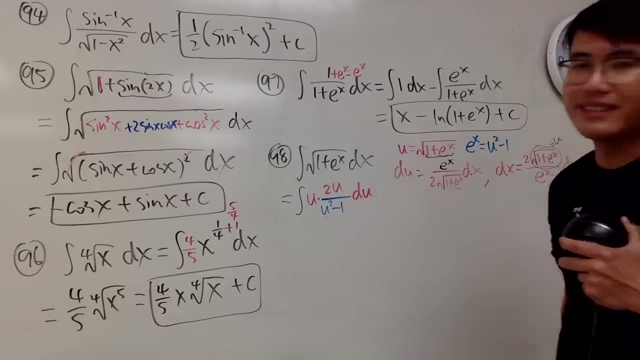 So that will be for this. So I'll put that down over: u squared minus 1.. u squared minus 1, all right, And then, of course, we'll have the du. So this is good, This is very good. 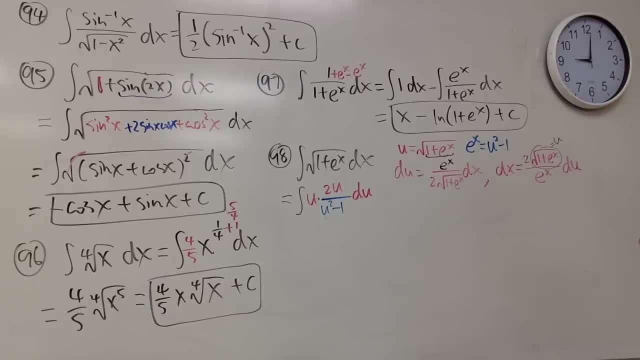 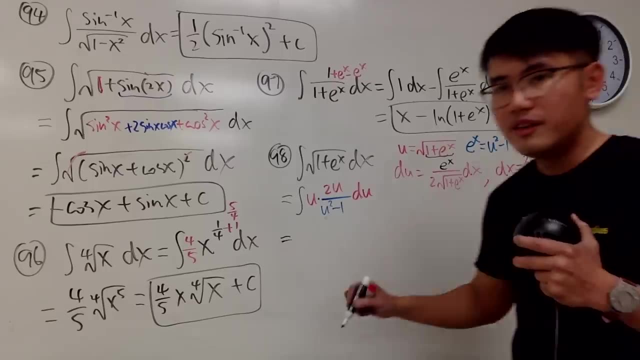 Okay, So this right here is what we have, And now, of course, you're looking at this integral and it's like trouble. Let's see if this is okay. Yeah, everything's okay. It's similar to one of the questions we did earlier. 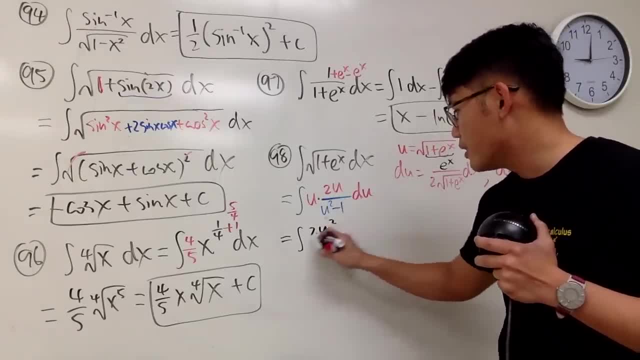 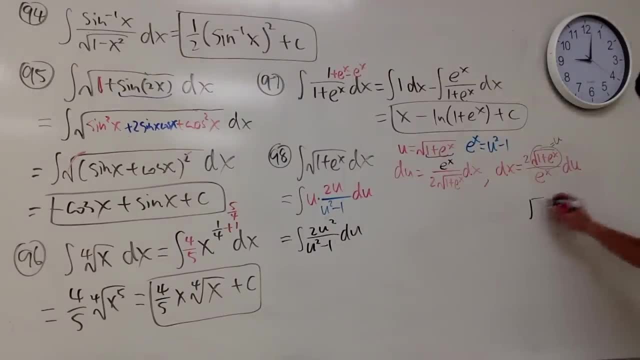 It's a minus, though. Anyway, 2u squared over, u squared minus 1 du Long division. And let's put it down right here: Long division: 2u squared, u squared minus 1.. You need a 2.. 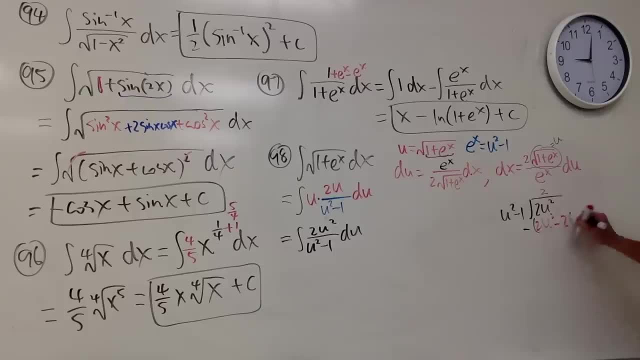 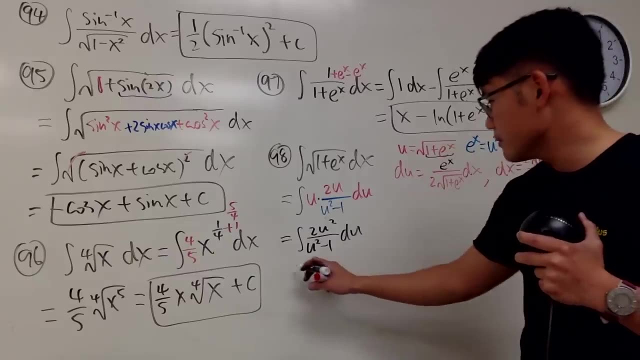 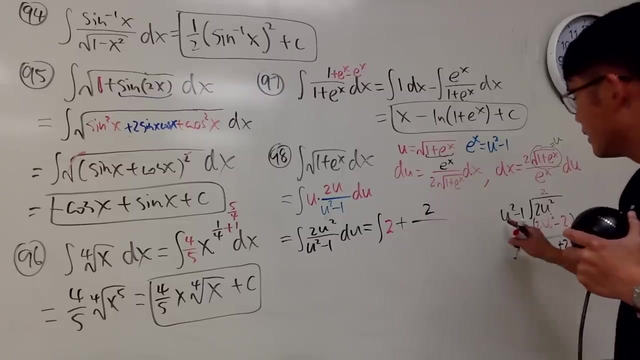 2 times this is 2u squared minus 2 minus, minus minus. So you get positive 2 right here. So what does this mean? That means we have to integrate. Let me put it down here. Let's integrate 2 and plus 2 over u squared minus 1,. 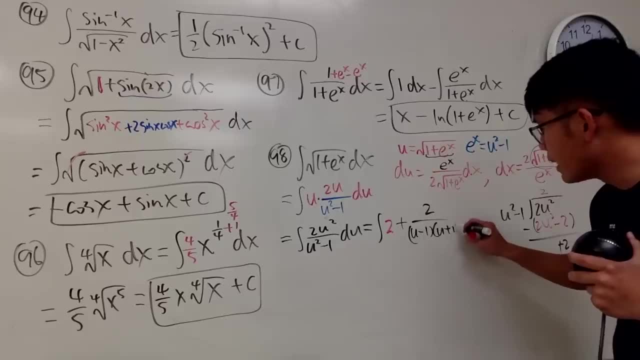 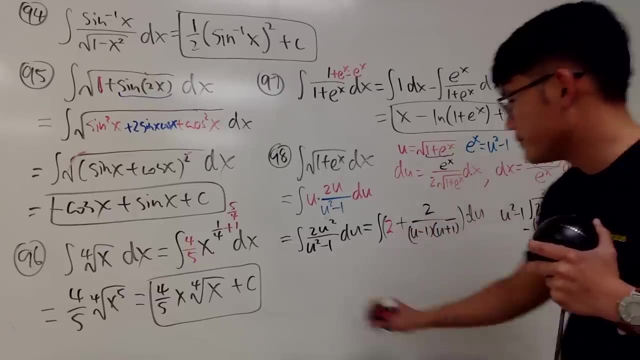 which is u minus 1 times u plus 1.. Yes, Partial fraction. Okay, I'm going to put this right here. I'm going to put this right here. So this is the integral of 2 plus something over u minus 1. 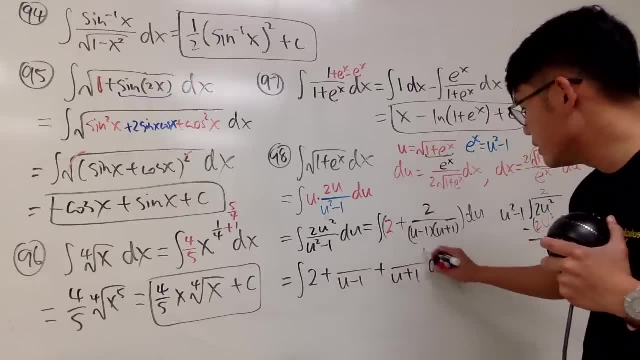 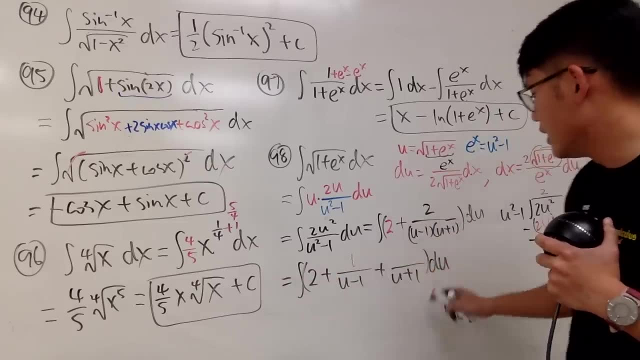 plus something over u plus 1. du like this: I need to plug in 1.. 2 over 2 is 1.. Nice, I need to plug in negative 1.. So it's 2 over negative, 2 is negative 1.. 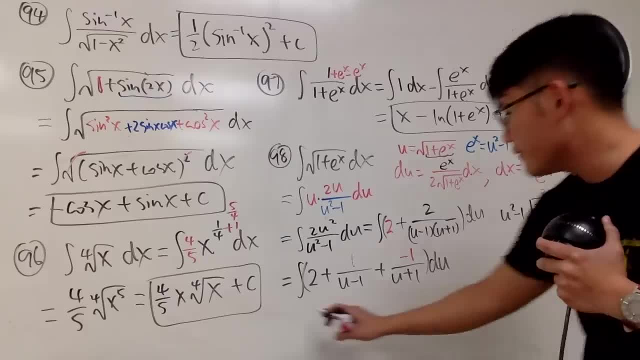 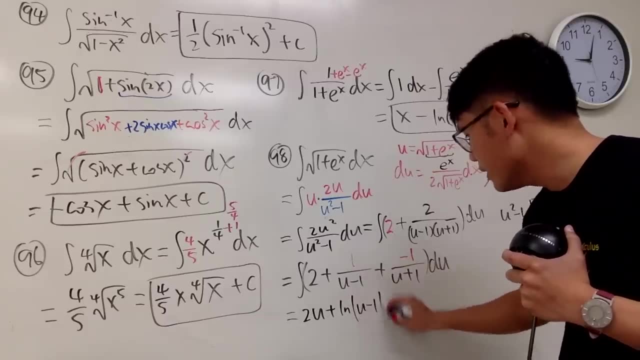 Nice. So we will have integral of this In the? u world. we get 2u And then this is going to be plus ln absolute value of u minus 1.. And then minus ln absolute value of u plus 1.. All right, 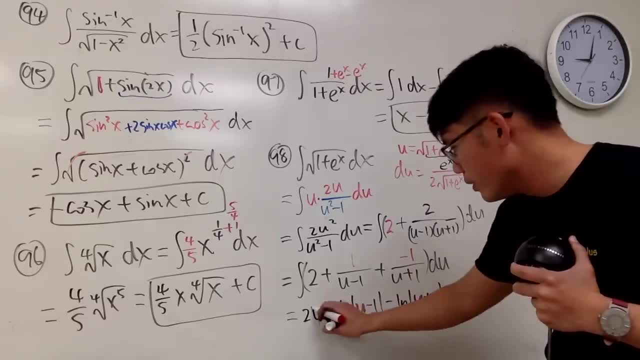 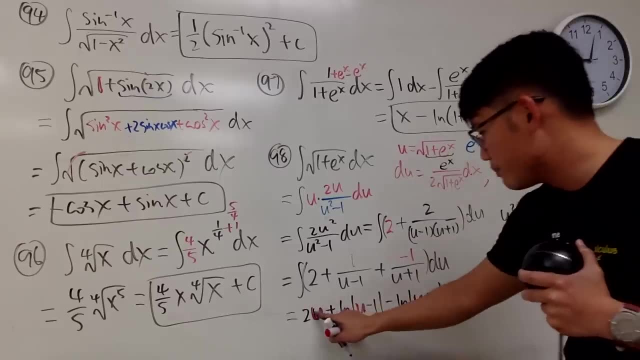 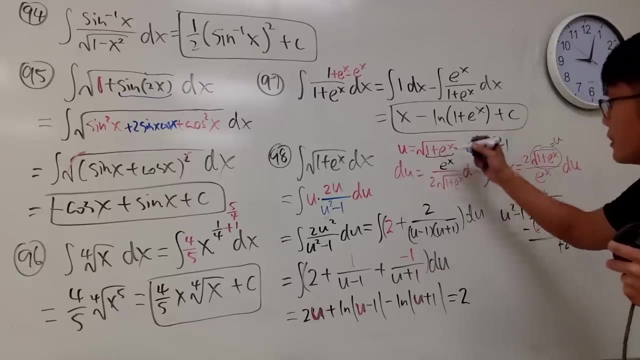 And then u, u, u God, So many u's. It is this guy, So I will just pull everybody back already down here. This is going to be 2u, which is that square root of 1 plus e to the x. 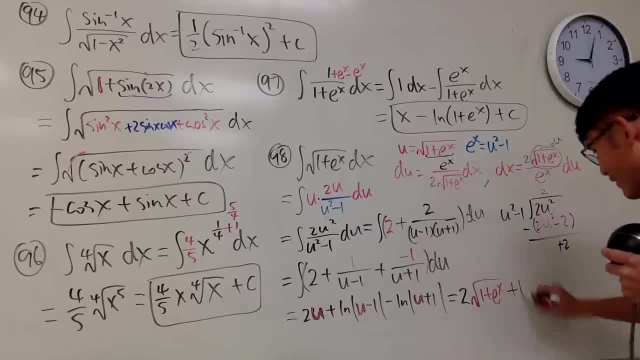 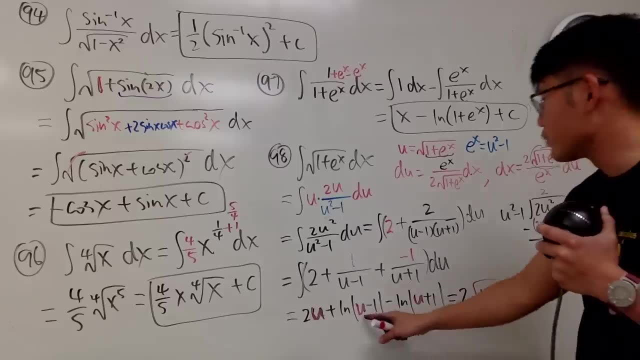 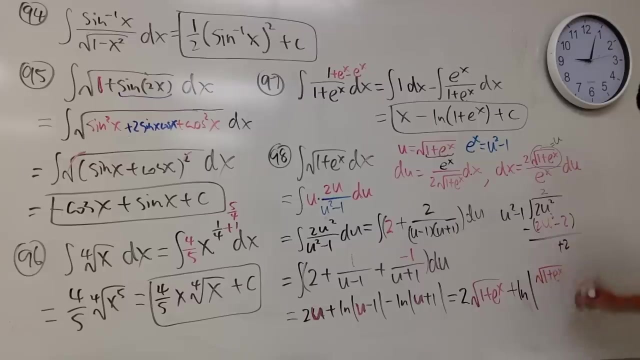 This and that can be combined into just one single logarithm. And then we have ln absolute value, And then u minus 1u. is this Well, I don't think we need absolute value to it. 1 plus e to the x minus 1.. 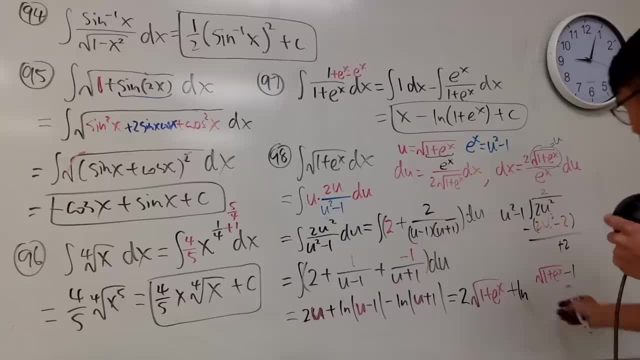 Now, this right here is at least 1 for sure. Yeah Well, this right here is at least 1, so it's good, So it's always positive. Likewise the bottom. you have this guy plus 1. Right. 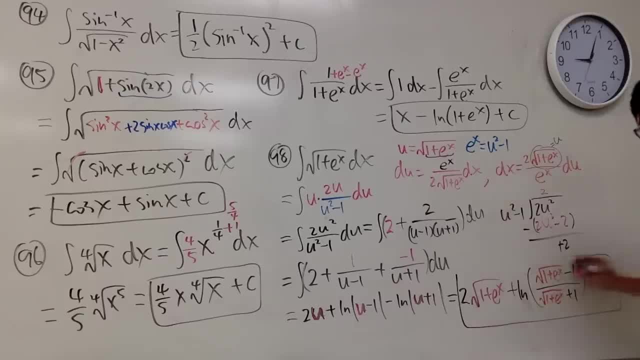 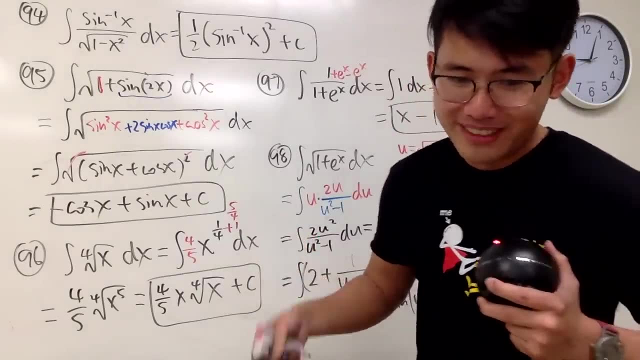 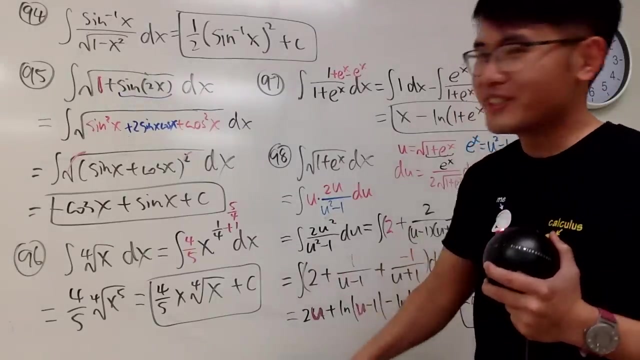 Done. Let's see Cool, This is it. How many more? Two more, Two more. No, I lied, Three more: 99.. Oh, two more, Two more, Two more. All right, So hopefully you're watching this, OK. 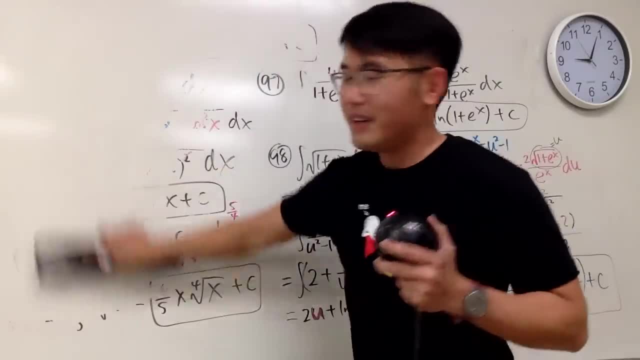 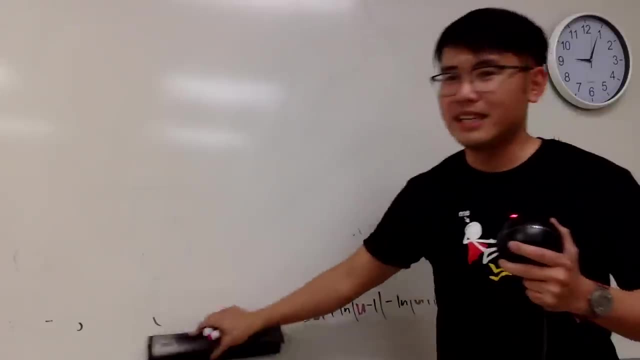 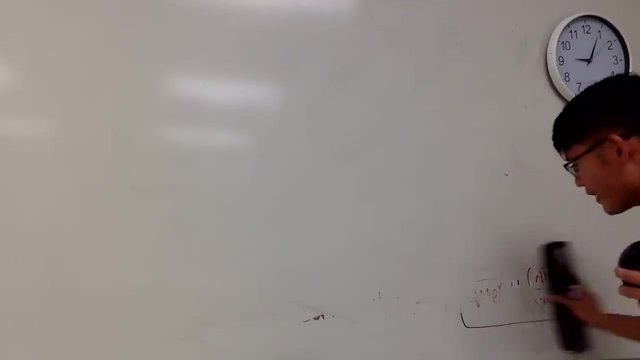 And if there's anybody who is going to break my record, I hope it's you. OK, I hope it's you. And then, in fact, is the only person, of course, besides my girlfriend, that I told about the 100 integrals in one take. 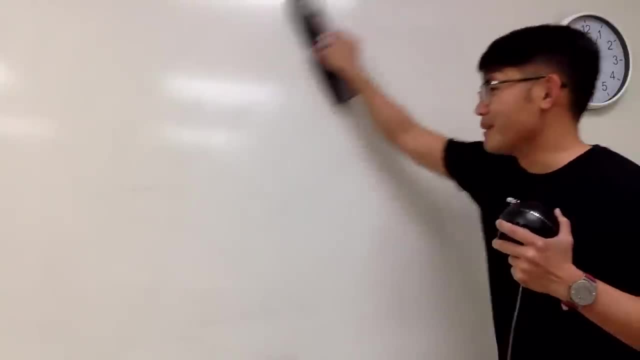 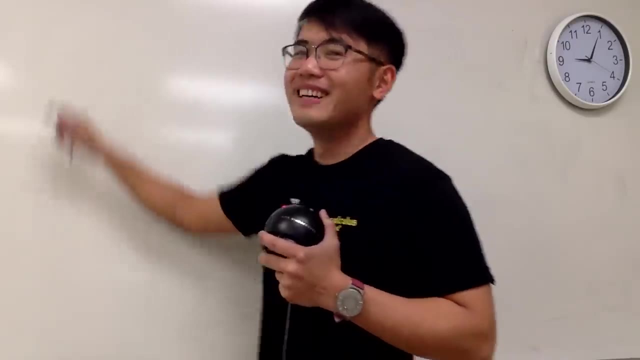 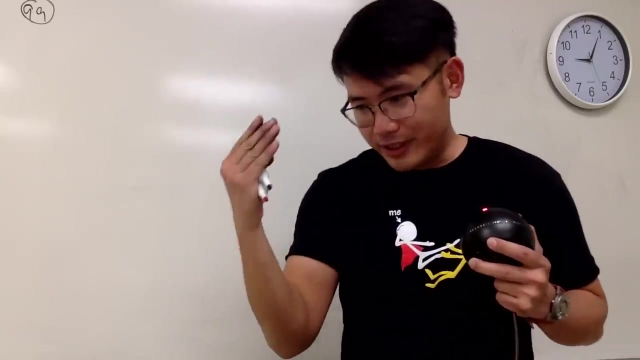 Right, I told Dr Payet I was going to do something really crazy, but he didn't know what it was And nobody else knew neither. Oh my god, Number 99.. This is like you reach the mile 26 in your marathon, but you have 0.2 more miles. 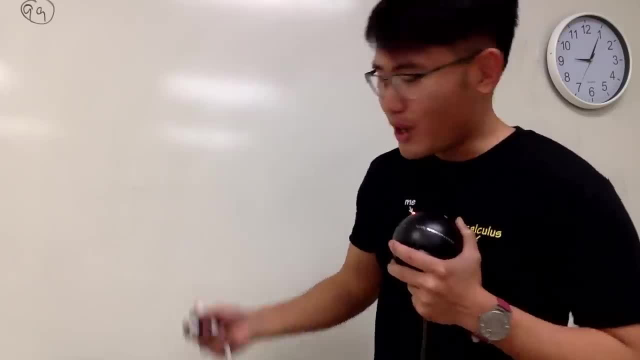 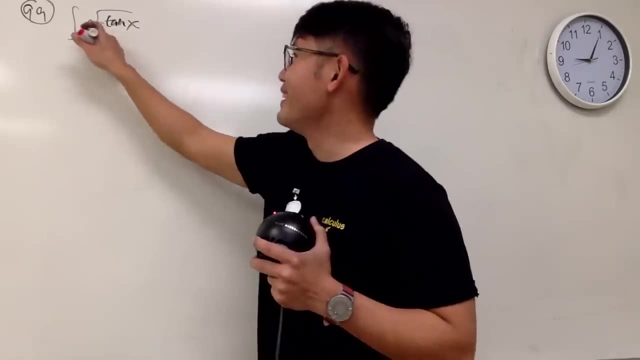 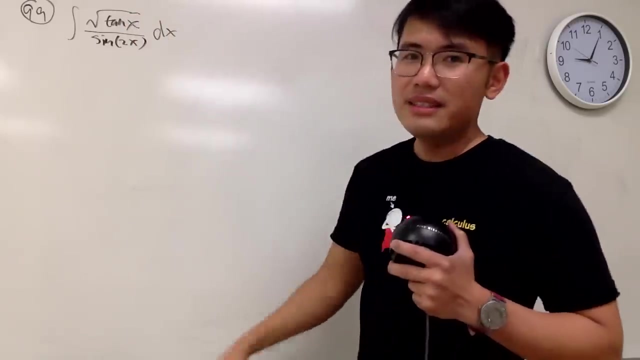 OK, 0.2.. Here we go. Integral square root of tangent x. No, I'm not going to do this. OK, I will do this version with the sine of 2x in the denominator. This is also pretty fun, OK. 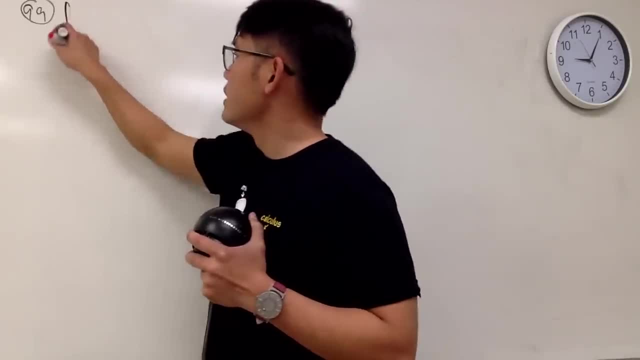 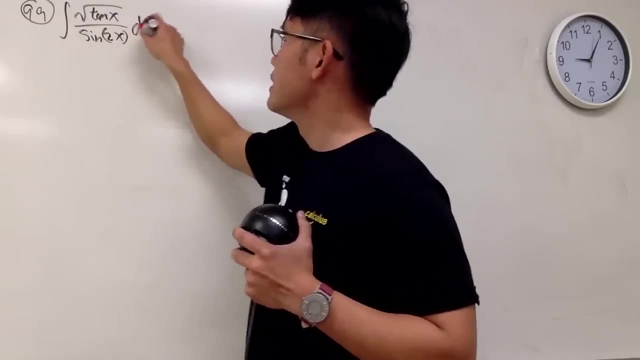 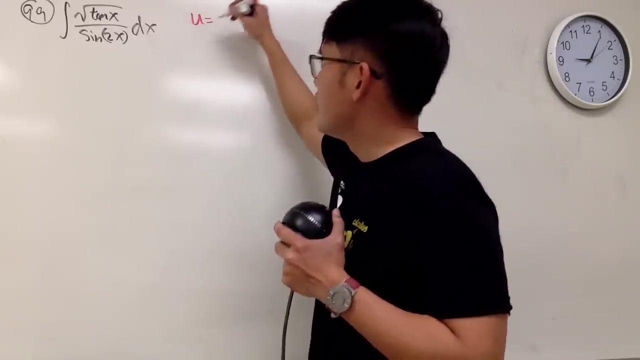 This is also pretty fun, but let me write it down better for you guys. Integral square root of tangent x over sine of 2x, like this: dx. What do we do? Do u stop right? Let u equal square root of tangent x. 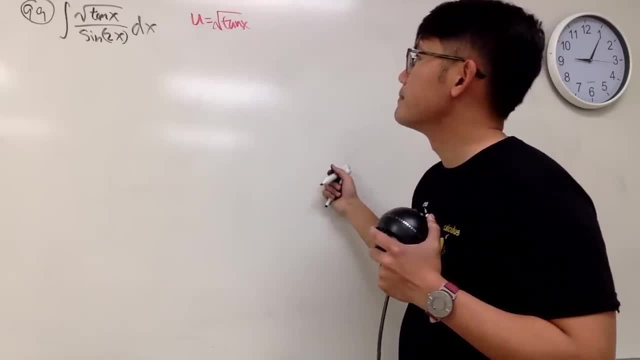 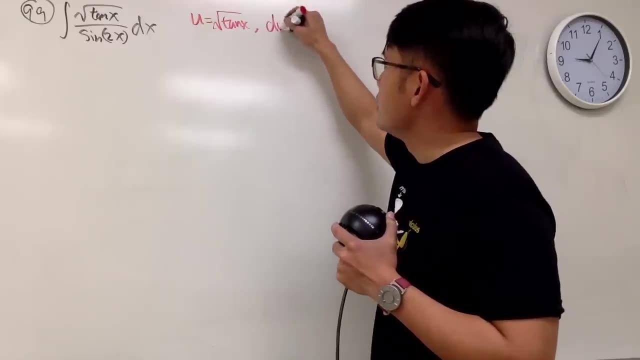 Square root of tangent x. And then let's see: Hmm, OK, Let's take a look. I am going to differentiate both sides, so du will be. let me put it down. Yeah, I don't want to get the inverse. 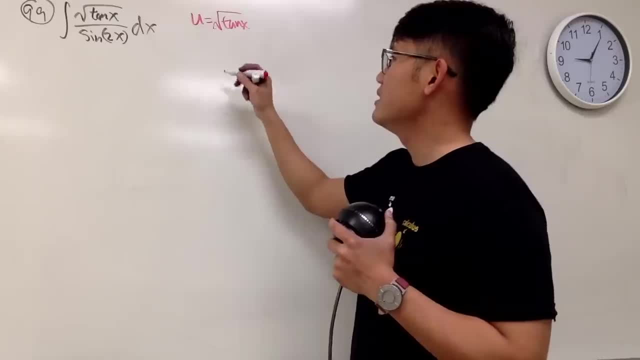 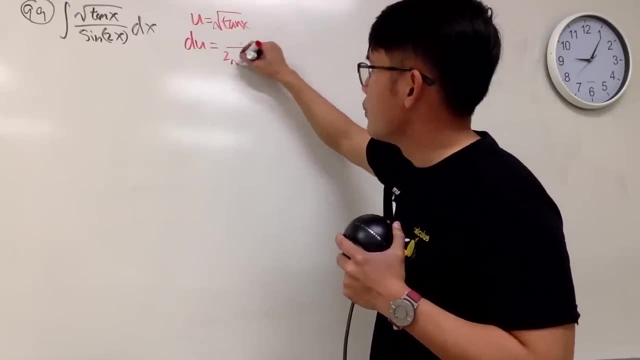 I don't think I want to do that. Yeah, let's see, I'll just deal with this. du equals 1 over. well, let's not do the 1, because you know there will be something on the top, 2 over 2, and 1 over square root of 2 over square root of tangent x, like this: 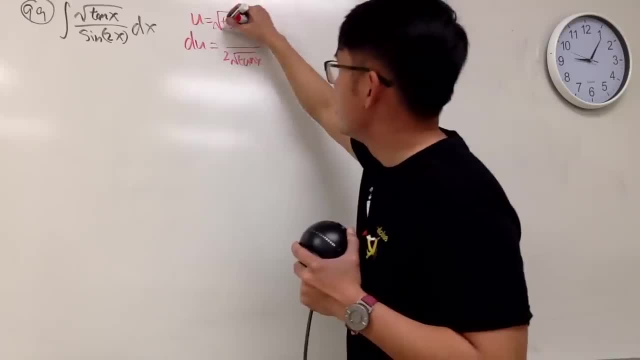 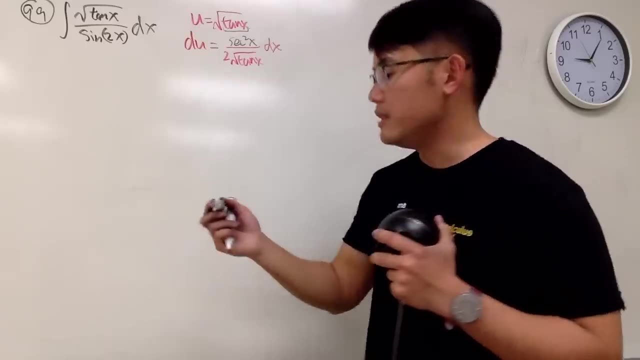 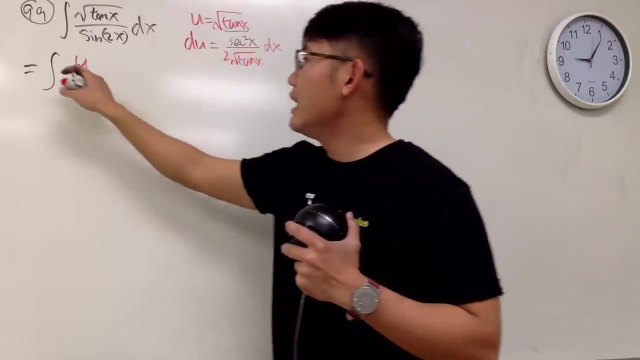 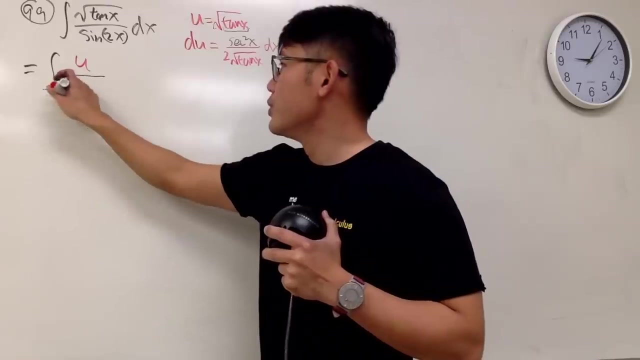 Don't forget the Chengdu. Use the Chengdu. The root of this is secant square x, dx. OK, And now we'll see On the top, this is the? u, That's good. On the bottom, let's use the double angle identity for sine of 2x, which is 2, sine x, cosine x. 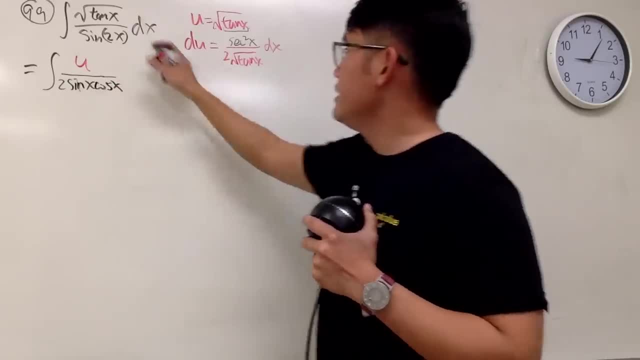 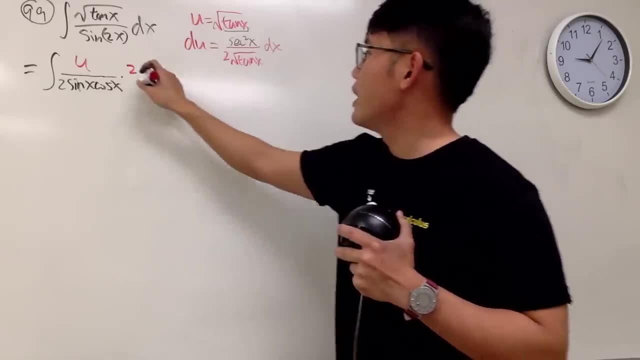 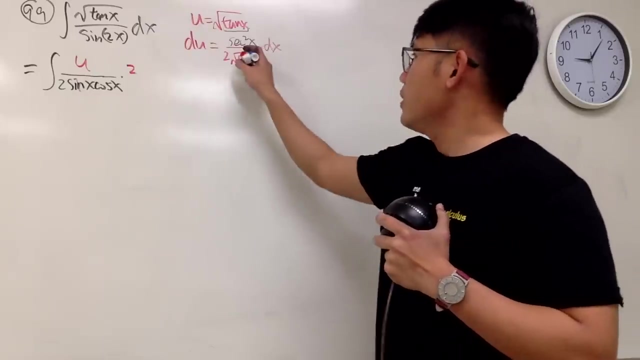 dx. well, do the reciprocal on both sides. So you will multiply this by 2. And then you have the square root of tangent x, And of course that's the same as u. So you are going to look at this as your u. 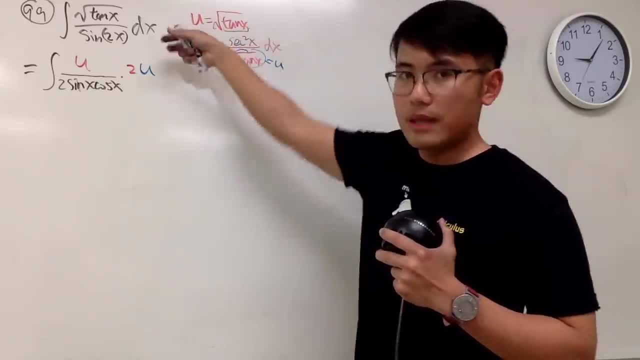 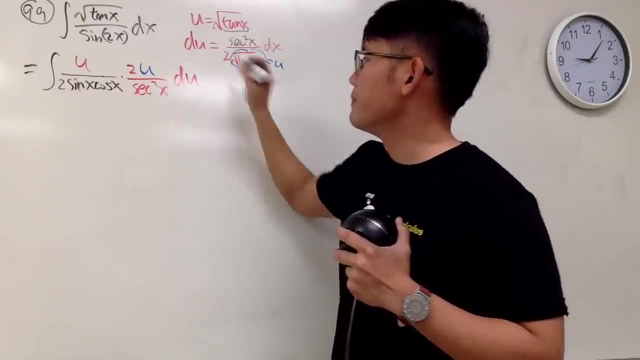 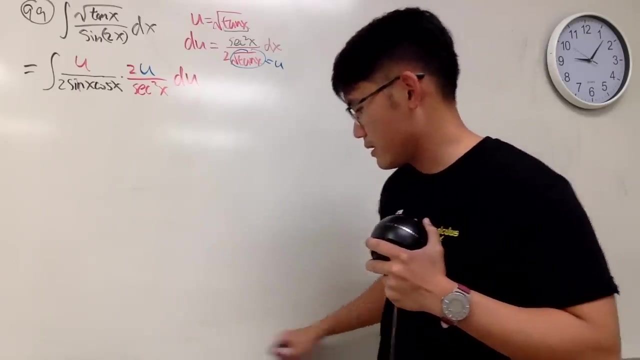 So put on u And I'm going to get a- yeah, you know what I mean- over secant square x, du. OK, So far, so good, OK, Hmm. OK, let's see, I'll use this blue. 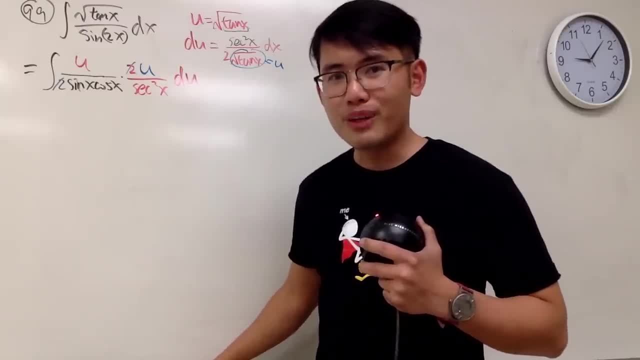 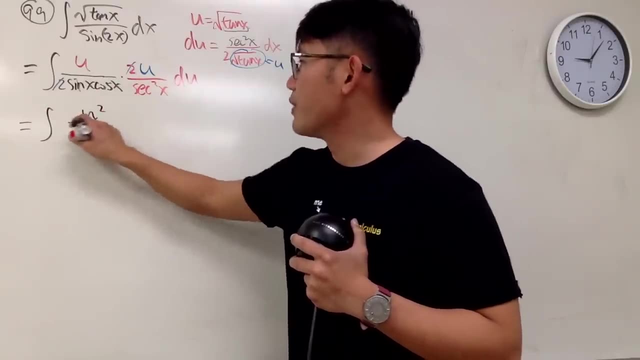 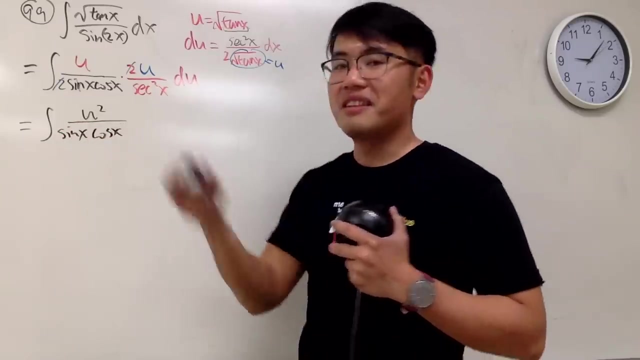 2 and 2 cancel. At least we're making progress. u squared on the top, sure, Integral On the top. we have u squared on the top over. this is sine x, This is cosine x. You're like duh, I know. 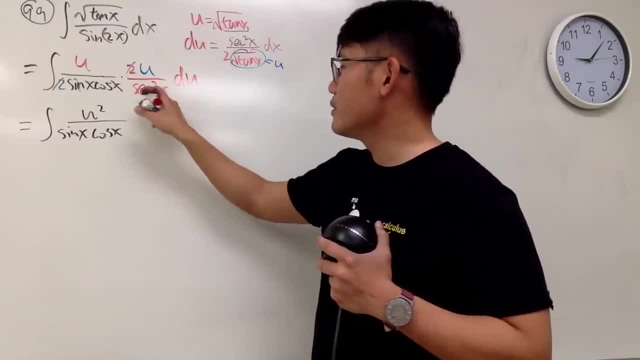 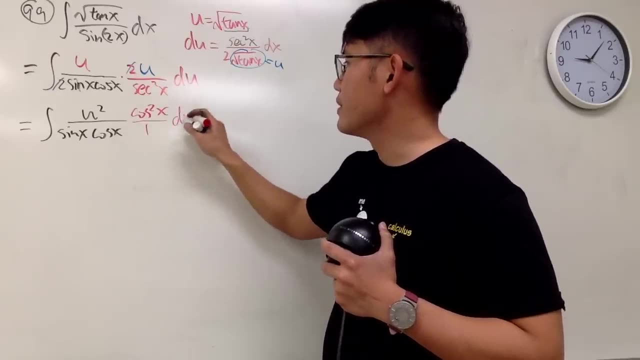 And then you have this over secant, So I can put that down as cosine square x right here on the top And then over 1. And then still have the du right. So that's the du. 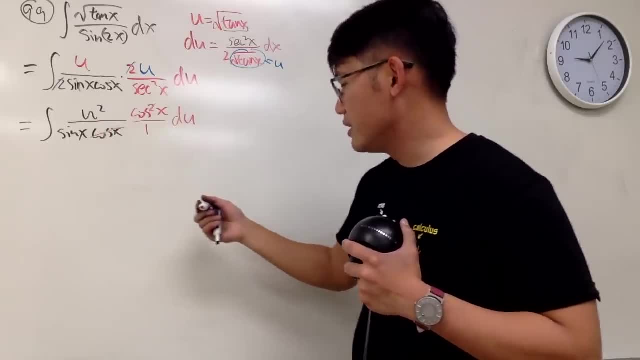 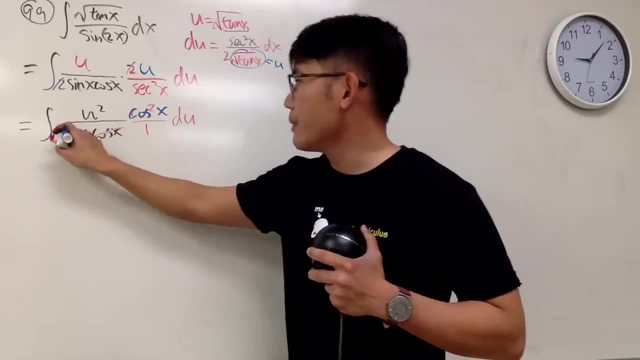 And then the du is that: Cancel this out And check this out. If you look at, we only have the cosine x left And we can pair up with the sine x. They are still in terms of x in the? u world. they're not good. 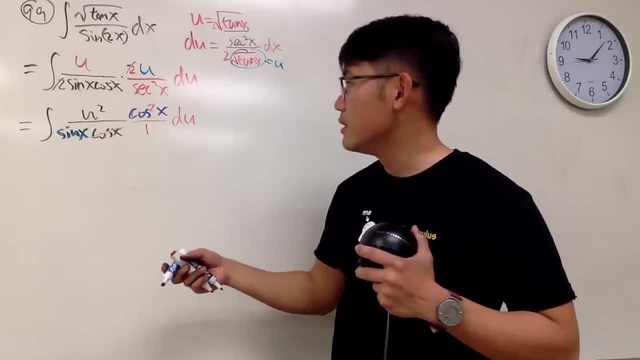 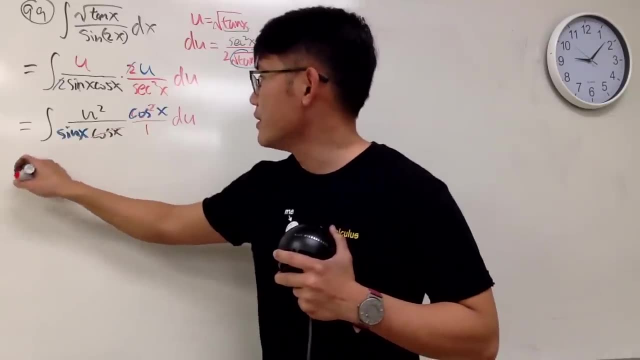 But they can be paired up as the cotangent Or, if you would like, you can bring this down as well. So it depends on how you want to look at it. So here's the du. This is going to be the integral. 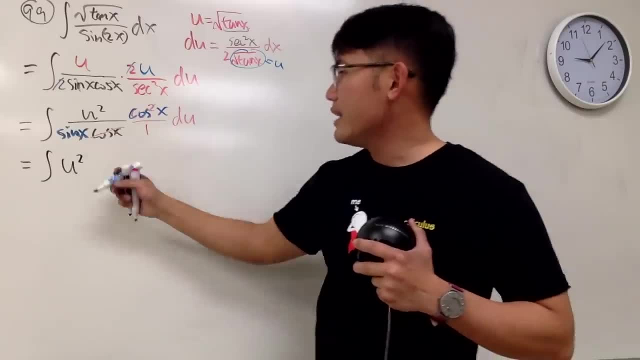 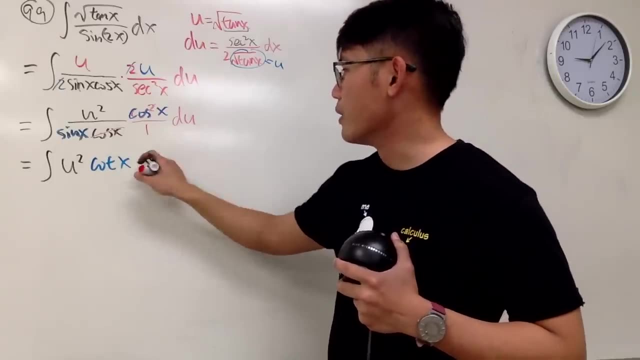 u squared is still u squared. OK, And then this over. that is cotangent. Let me just put on cotangent for this. I haven't seen cotangent for a while, so let's put on cotangent, And then we are in the? u world. 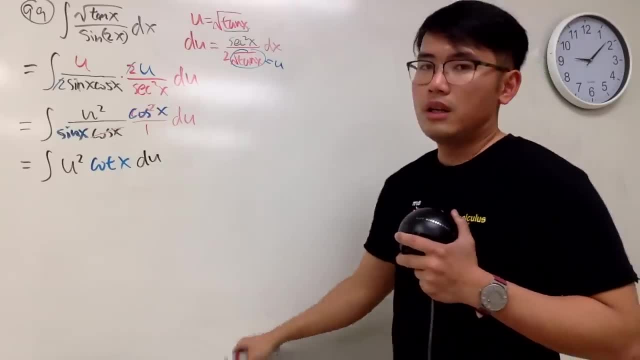 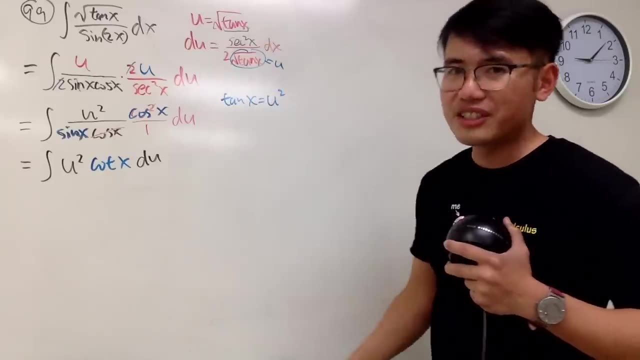 So we still have some trouble because of the x. It's not allowed in the? u world. Let's see Right here. you know, tangent x is just u squared Square both sides, that's good. And if you do the reciprocal on both sides. 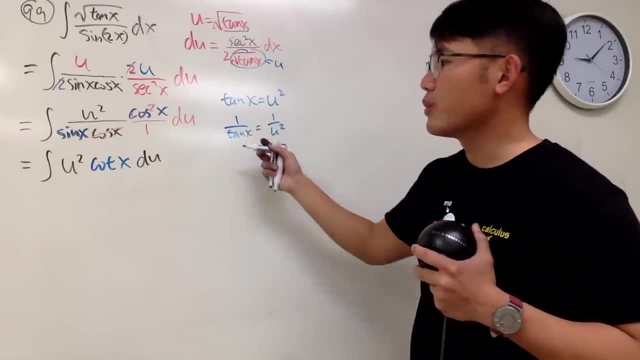 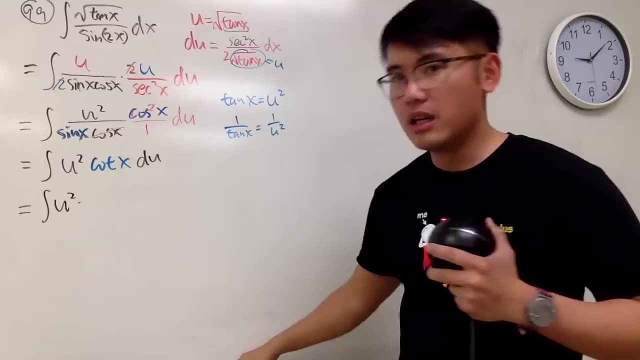 1 over tangent x is just 1 over u squared, namely cotangent for that Good. So you will see this right here. It's actually just the integral of u squared times. cotangent x is just nicely equal to 1 over u squared du. 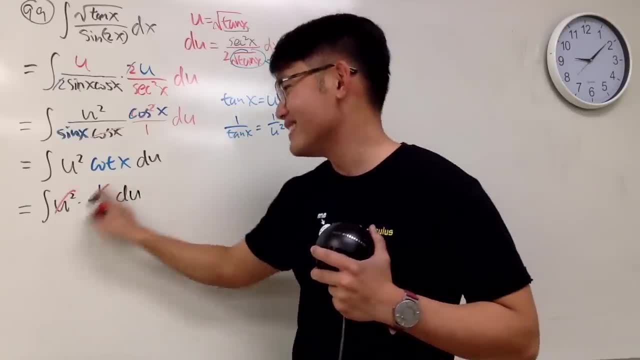 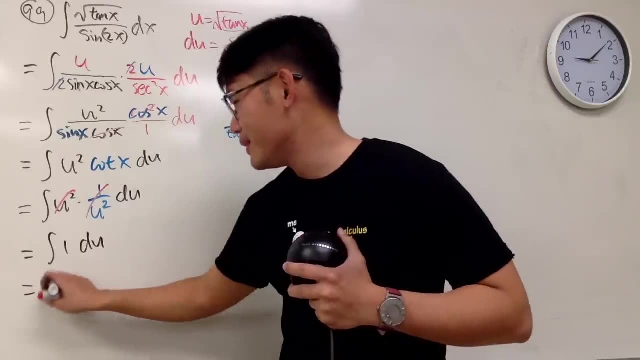 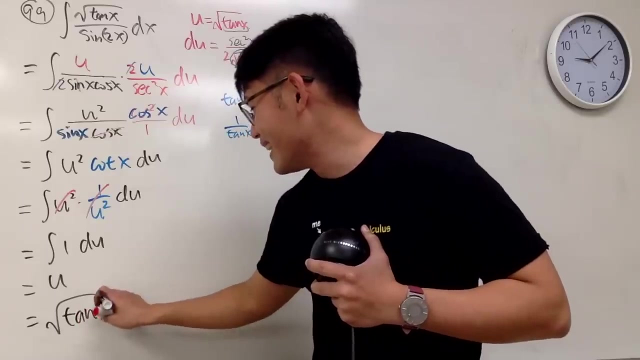 So what exactly are we integrating? Yes, it's just 1 in the? u world Integrating 1 in the? u world. we get u, And what is u? u is square root of tangent x. Wow, look at that. 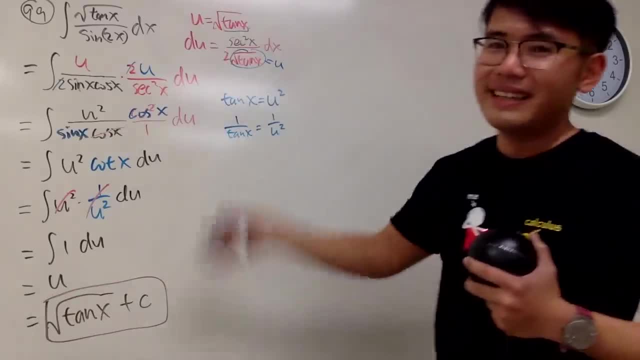 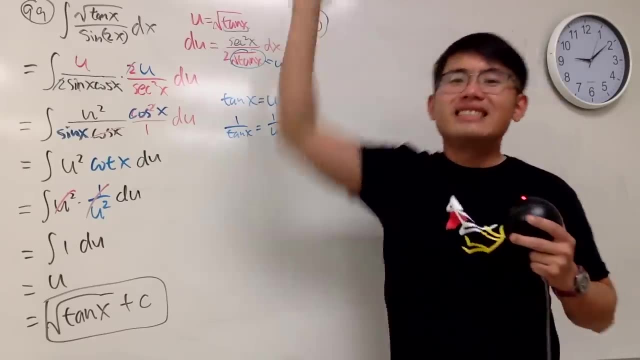 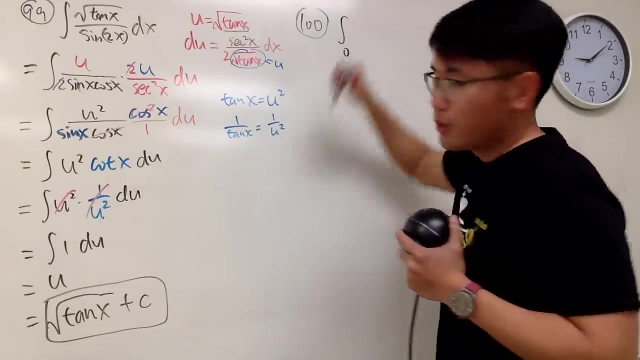 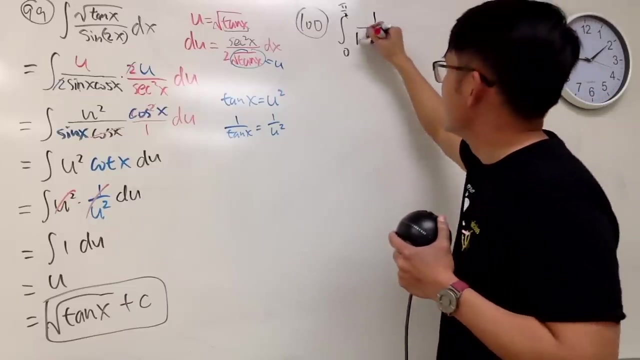 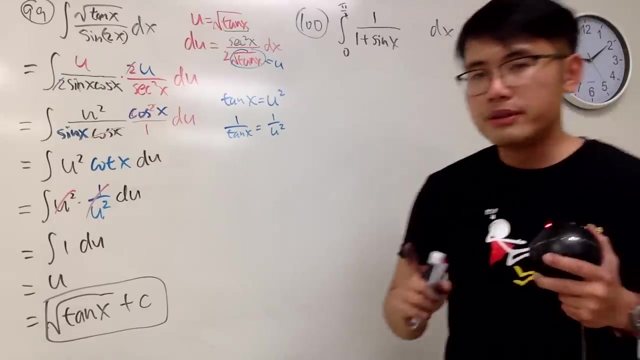 Plus c. Cool huh, Yeah, the answer is so, so, so, so, so clean. Finally, the integral of the integral from 0 to pi over 2, 1 over 1 plus sine x, dx. The reason why I put this down for the last one. 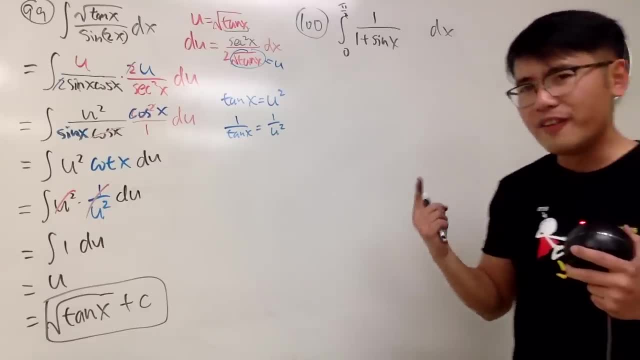 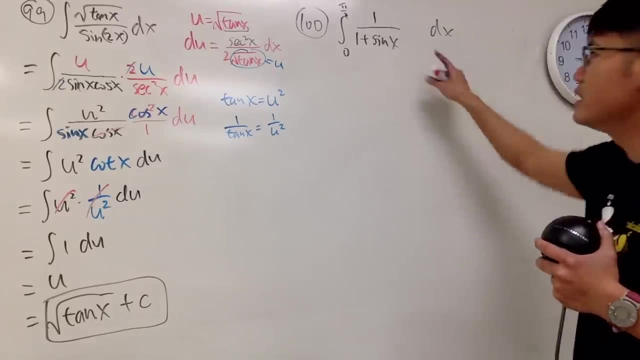 is because I think this was one of the first integral, one of the first three integrals, maybe the first one. okay, Now I did, and I'm pretty sure this was the first one that got me the 10,000 view, the first 10,000 view on YouTube. 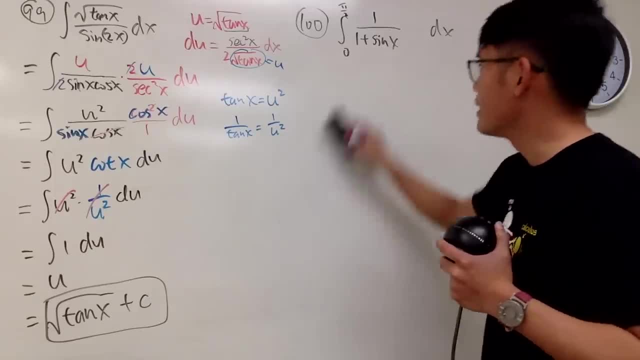 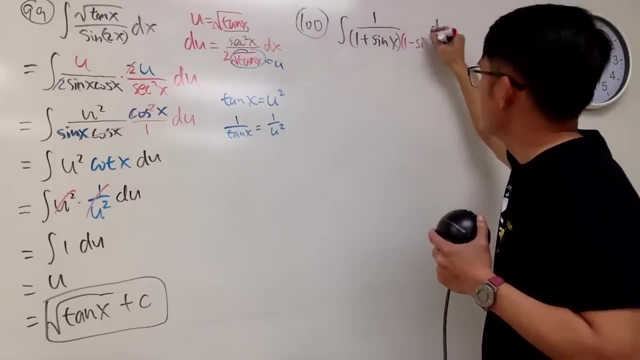 So of course I'm going to finish this legitimately. Technically, the one I did was without the limits of integration, but don't worry, I'll put it back The way I did it was. I multiplied the top and bottom by the conjugate. okay. 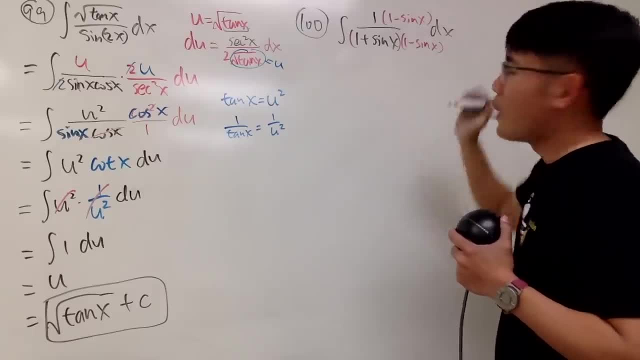 It's cosine. you can do something else nicely, but let me just show you guys what I did right here. So here's the deal. Now I have this times that, which is just cosine squared x- dx, and now on top it's just 1 minus sine x. 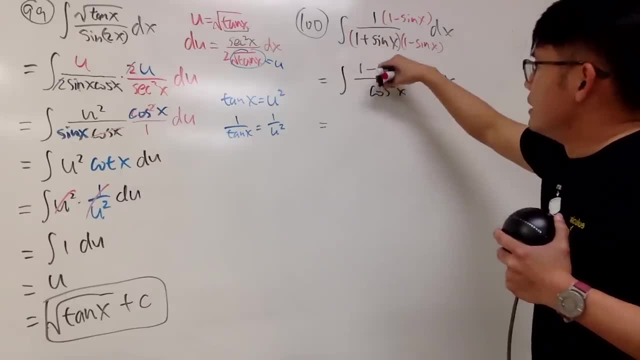 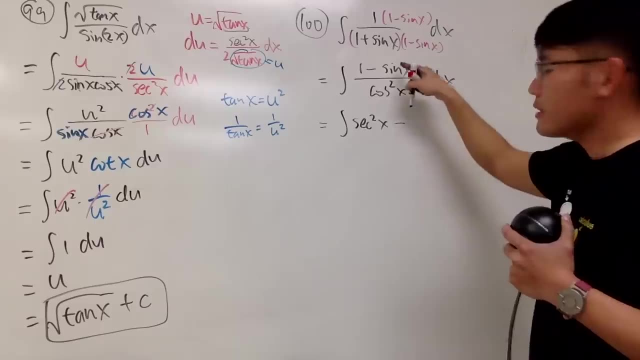 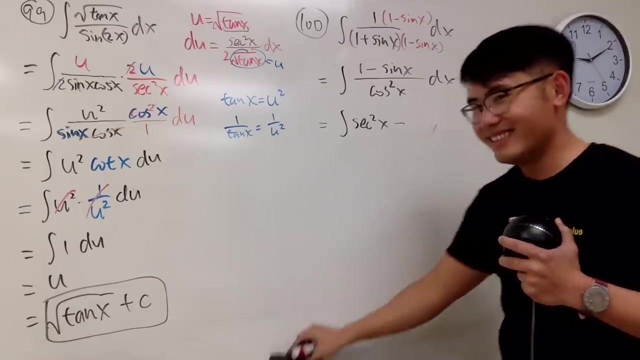 And check this out: This right here is secant squared, so we are integrating secant squared x, This and that we have to. minus sine over cosine is secant. No, sorry, sorry, Too excited. Sine over cosine to the first power is tangent. 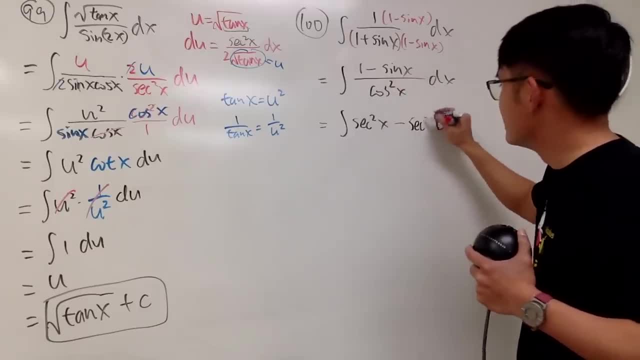 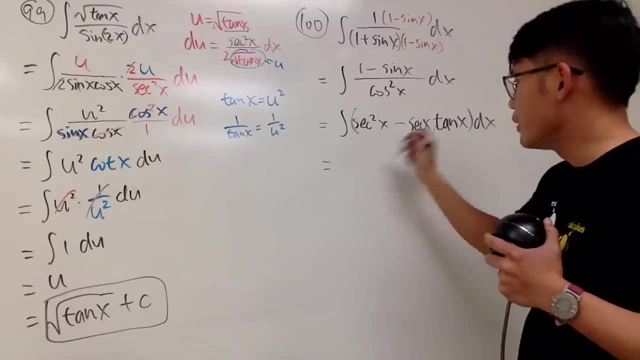 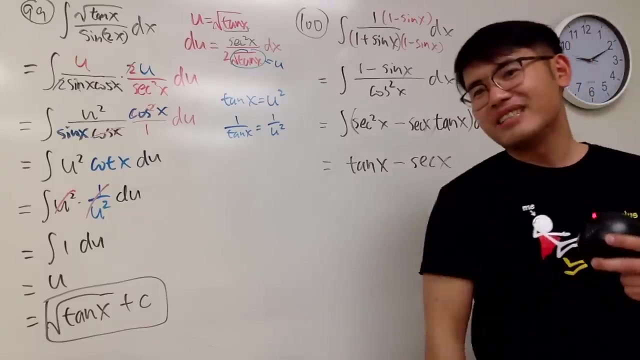 but we have another cosine in the denominator, so it's secant x, like that. And of course let's close the integral and people want me to put parentheses, And then integrating, we get tangent minus secant x. That's it right. 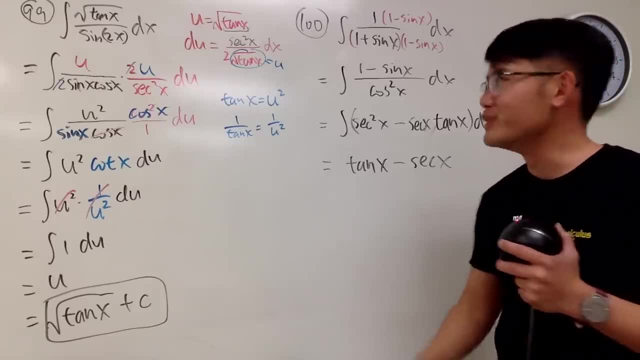 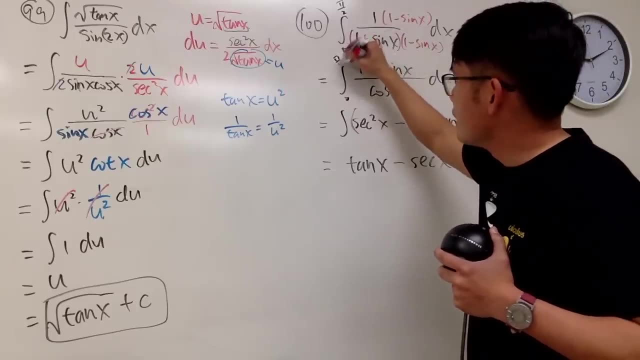 Cool, But as I told you, I'm going to put down a limit. As I said, I will give you guys some definite integrals, so don't forget you have 0 to pi over 2.. 0 to pi over 2, okay. 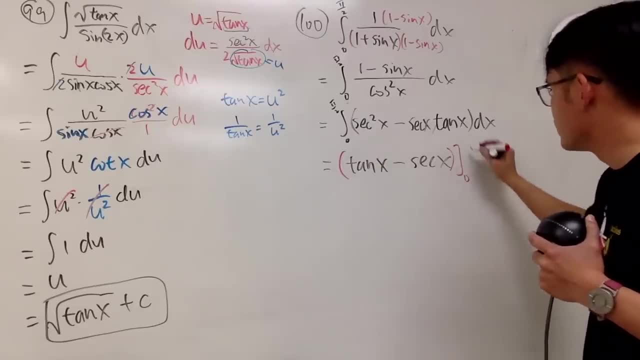 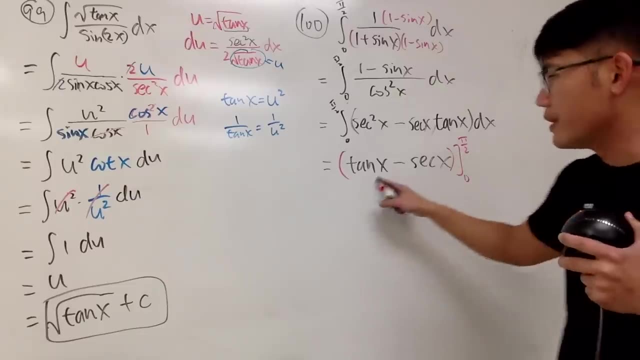 So technically I will have to look at this and I plug in 0 to pi over 2.. But the problem here is that when you plug in pi over 2 into here, tangent of pi over 2 is not defined. No, no. 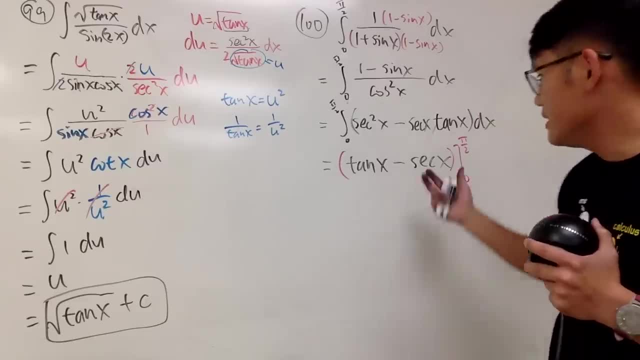 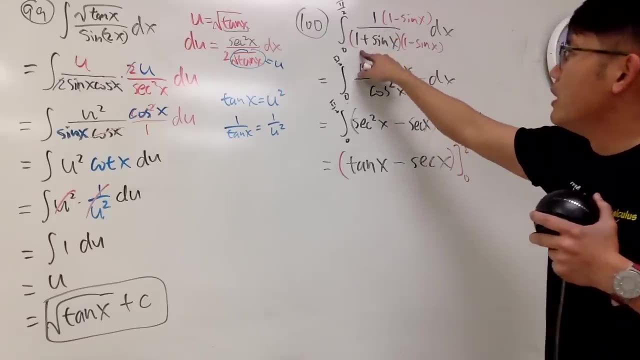 But does that mean this integral originally is not good in the first place? Well, the truth is 1 over 1 plus sine x is good. It's continuous. You can put pi over 2.. Sine of pi over 2 is 1,. 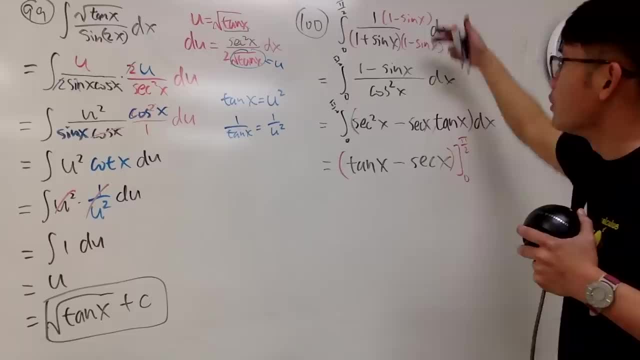 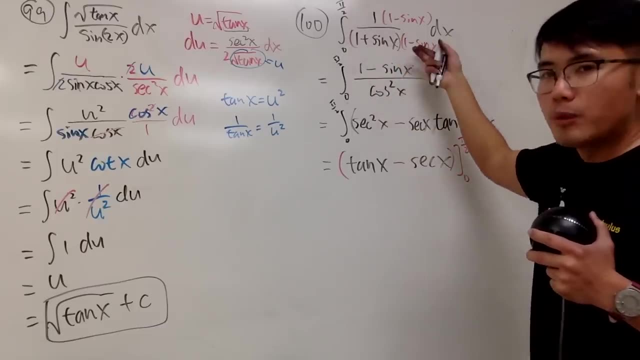 so you just have 1 half. That's good. The trouble is we multiply top and bottom by this: When x is pi over 2, you have 1 minus sine of pi over 2, in another word minus 1, which is 0.. 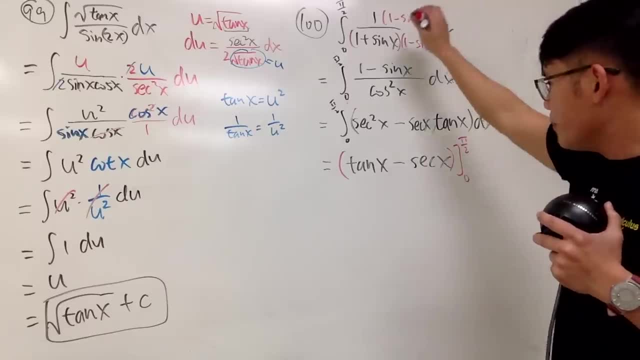 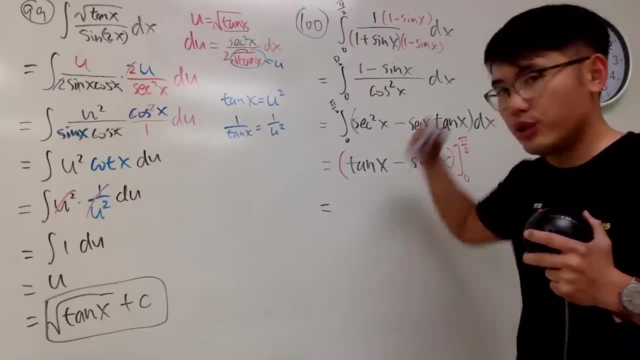 You multiply 0 over 0. It helped us to integrate it, but if you want to evaluate this, it's not that good yet. So the way to fix this is that we have to undo that. So let me show you. Tangent is cosine x over sine. 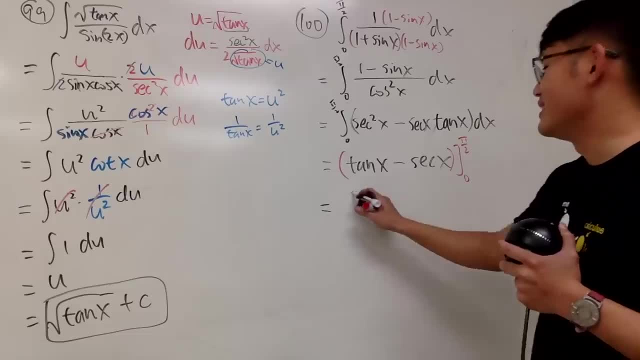 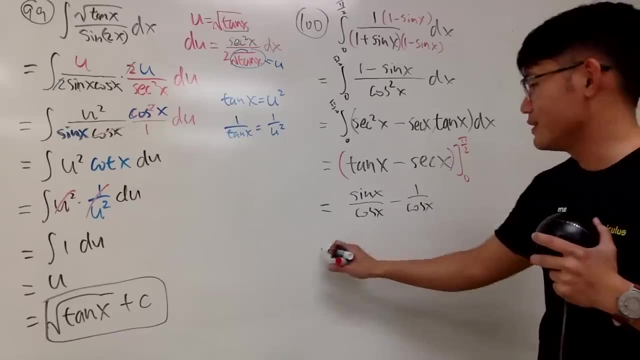 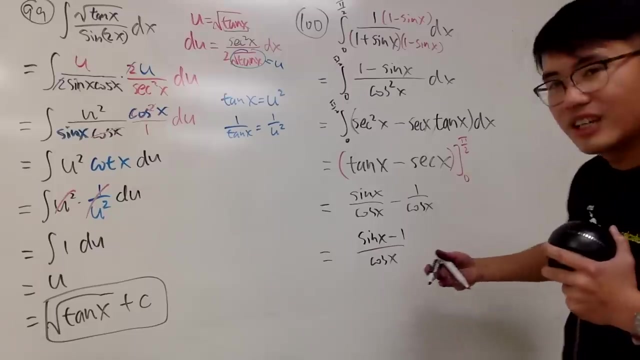 Oh, I'm sorry It's late. It's tiring Sine x over cosine x and then minus sec 1 over cosine x. Does this look familiar? This is sine x minus 1 over cosine x. Yes, I will pretty much do that again. 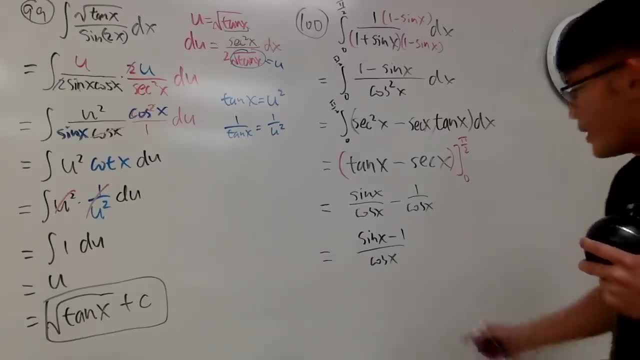 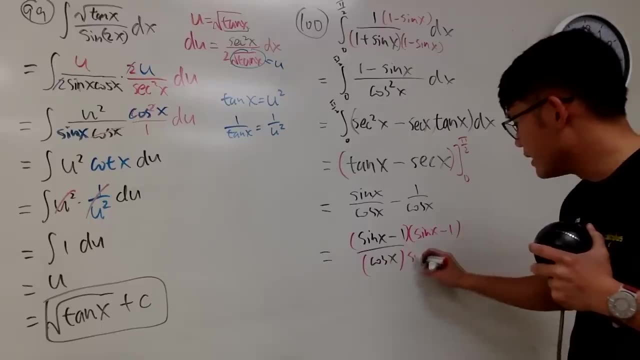 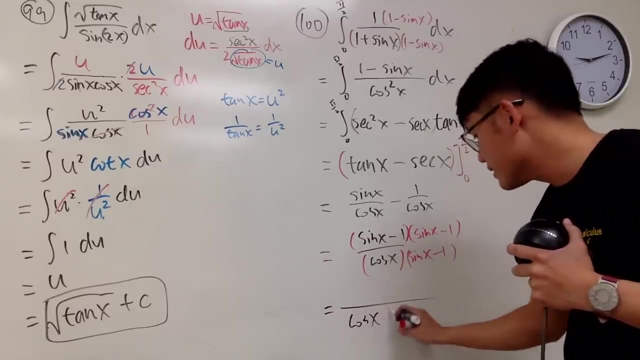 That's pretty much the idea. So what we are going to do is: let's go ahead and multiply the top and bottom by sine x minus 1, and then sine x minus 1.. And, as you can see here, you end up with cosine x times. 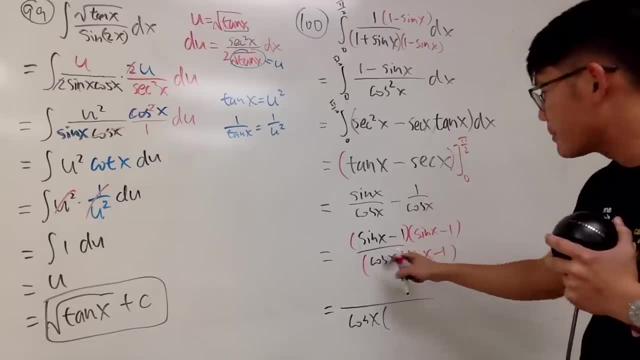 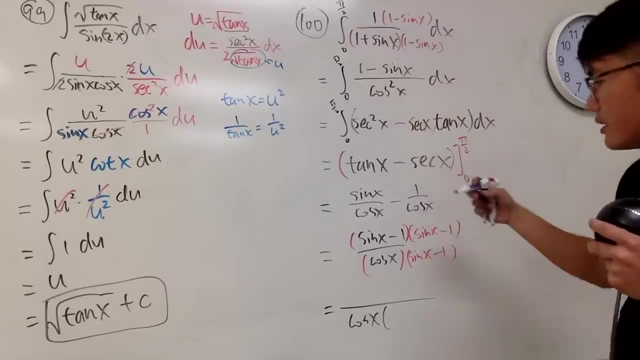 All right, Here's the deal On the top here. on the top here, you end up with negative, because this is the different order Earlier. if it's 1 minus sine squared, it's positive cosine squared. But this is going to give you negative cosine squared x. 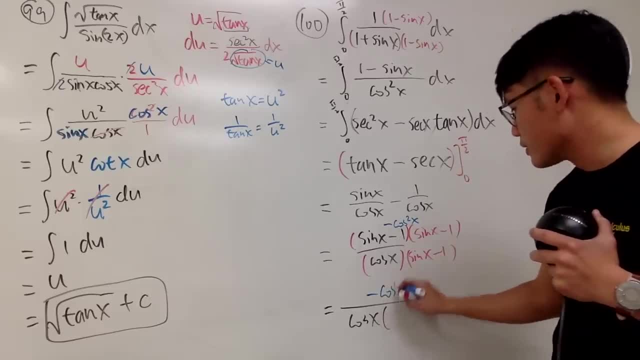 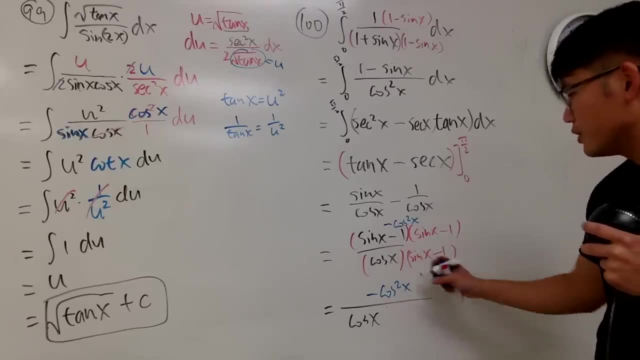 like that. So you put that down. negative cosine squared like that. So that's it for that. But in the meantime, why don't we just change the order right here as well? Sorry, Sorry, I'm sorry, This should have been a plus 1.. I'm sorry. 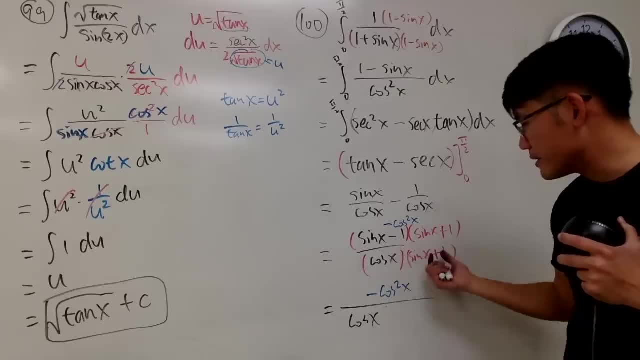 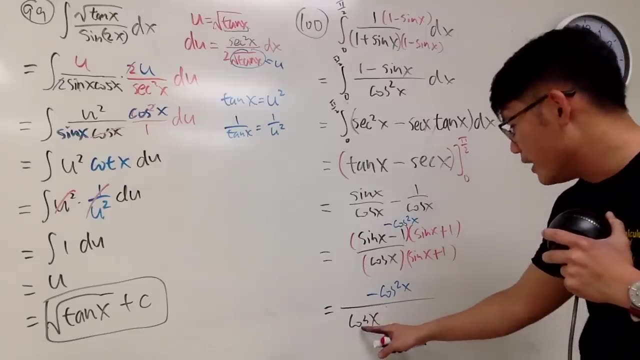 Let me do it again. Take this times the conjugate, Take that times the conjugate, So you have negative cosine squared x on top. This is still good. Okay, Over cosine x times this. So I will just put that down right here. 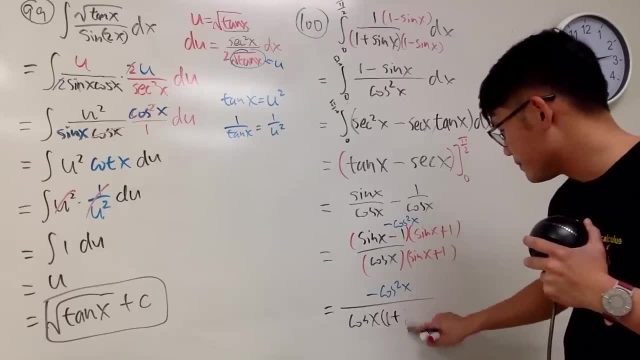 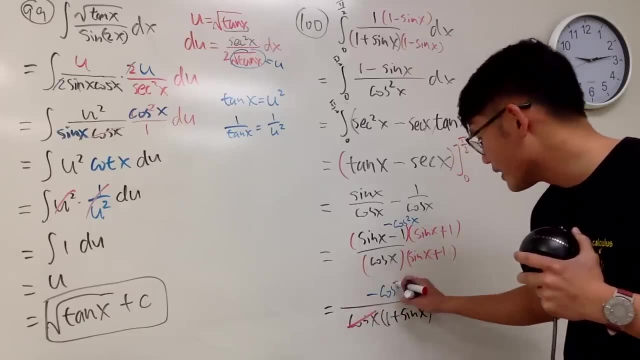 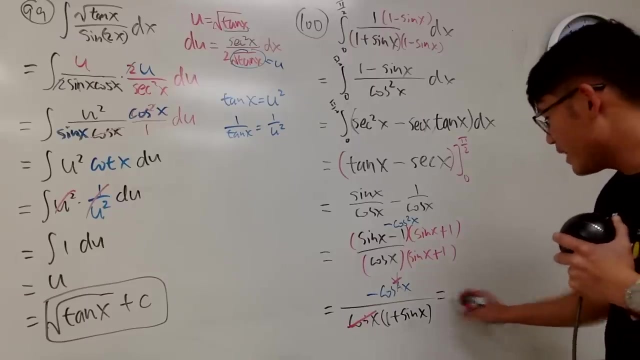 which I can write this as: 1 plus sine x, Doesn't matter, All right. And then, of course, here we can cancel things out: Cancel, Cancel, Sorry, Cancel. So we end up with the integral. No, not integral. 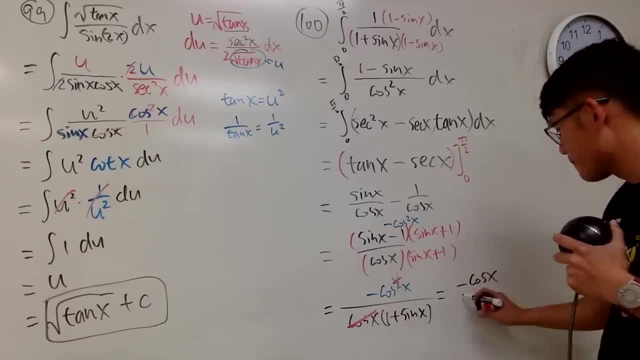 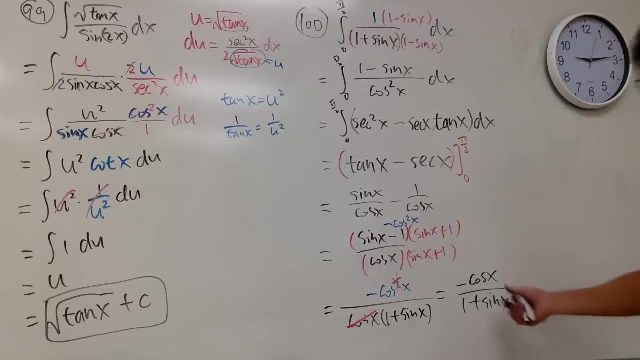 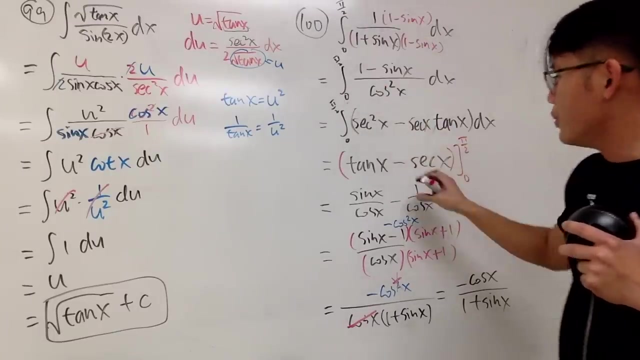 We finish integral with negative cosine x over 1 plus sine x. What are we trying to do? The idea is that: look at, if you want to talk about the indefinite integral, you could end up right here, but it may not help sometimes if you have limits of integration. 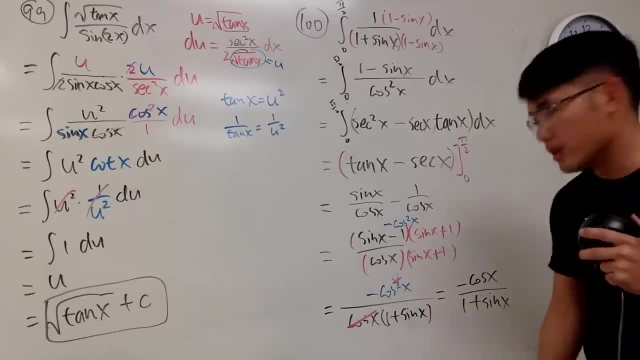 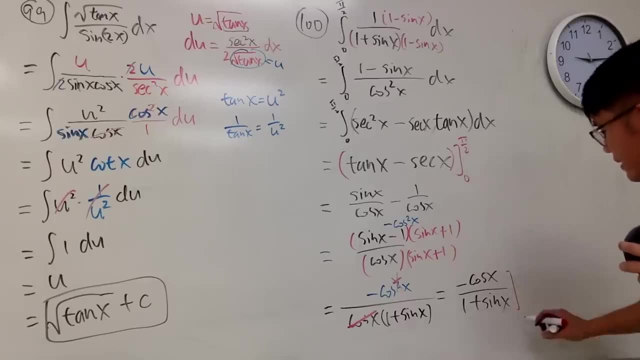 such as from 0 to pi over 2.. Sometimes you have to do more work. This right here will be a better answer. All right, And what we will do right here is we will plug in the number here: 0 to pi over 2.. 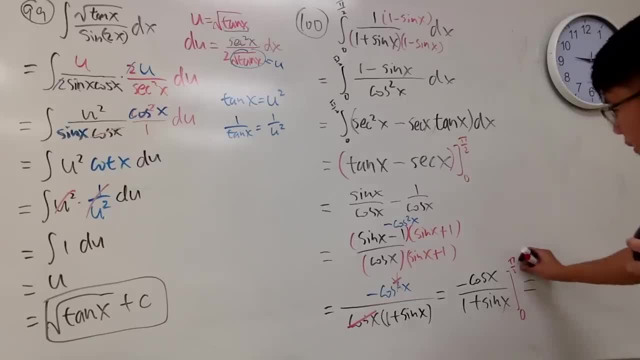 And we are going to do this in our head. When you plug in pi over 2 into this cosine of pi over 2 is 0, so thank God, That will be 0. And then minus, plug in 0 into here. 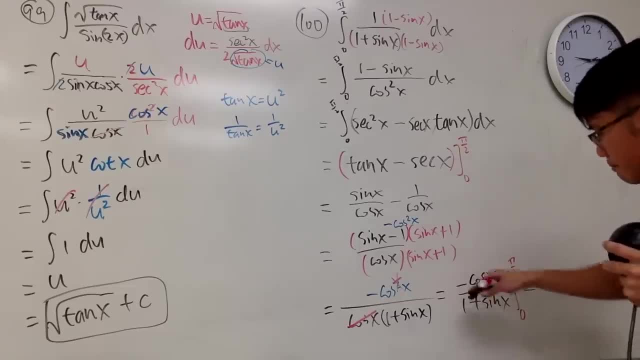 Cosine of 0 is 1 by negative 1.. But remember it's minus, You plug in, so it's minus minus 1.. So it's positive 1 over 1 plus sine of 0 is 0.. So finally, we end up with this very, very nice 1.. 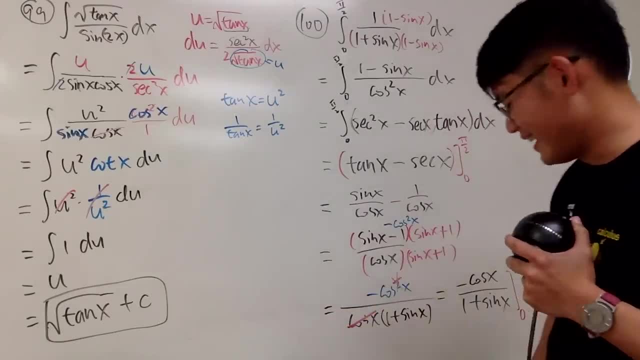 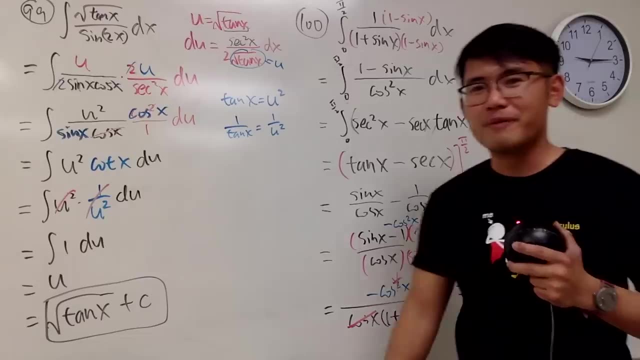 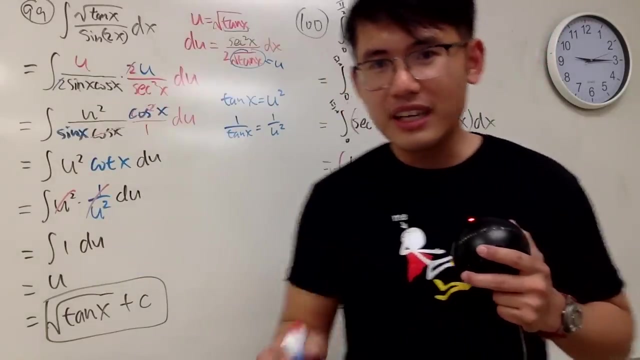 We end up with this very, very nice 1. 100 integrals In one take. I hope this is a world record. But one more thing: Some of you guys might have seen it. Yes, just in case, if somebody wanted to. 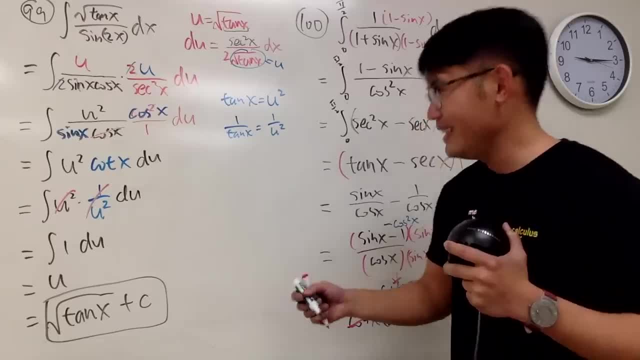 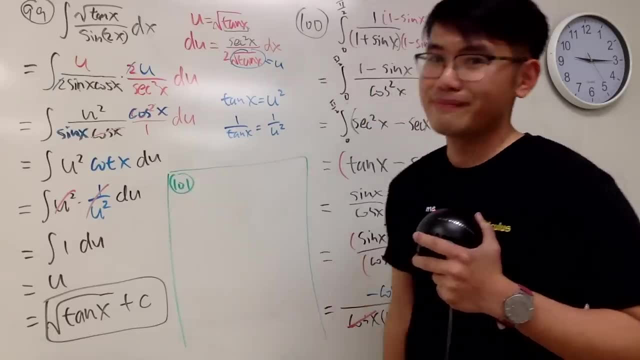 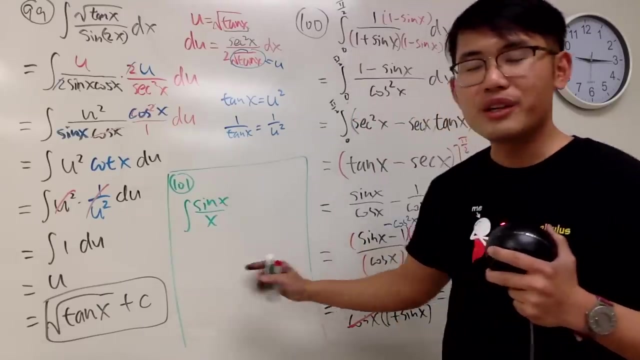 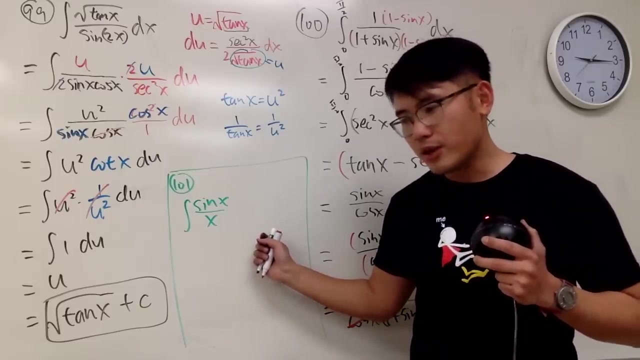 break the 100 integral. they thought they know, but they don't. Here is equation 101.. Okay, Integral of sine x over x. This right here. it's also just a special My differential equation: linear differential First water. linear differential equation. 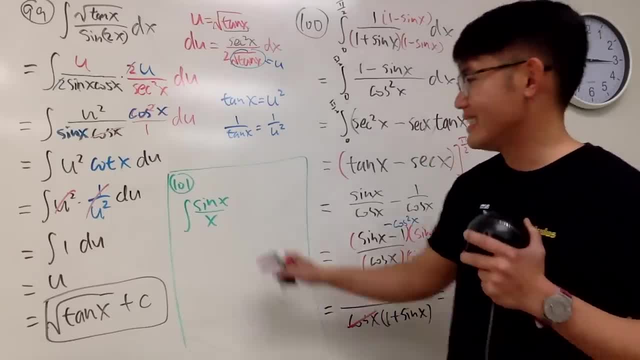 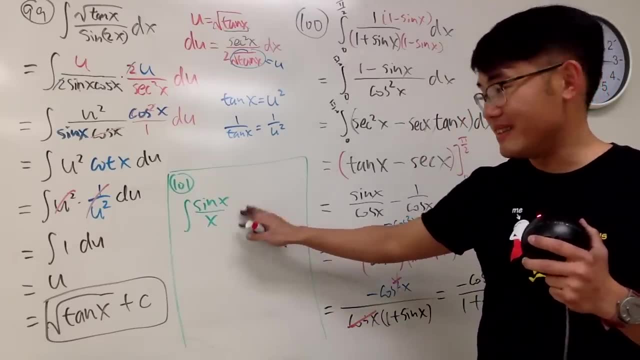 Okay, I use this as example In that video. First of all, integral of sine x over x. Yes, you know I haven't put down the dx And also, even though, if I do, you cannot finish this Okay. 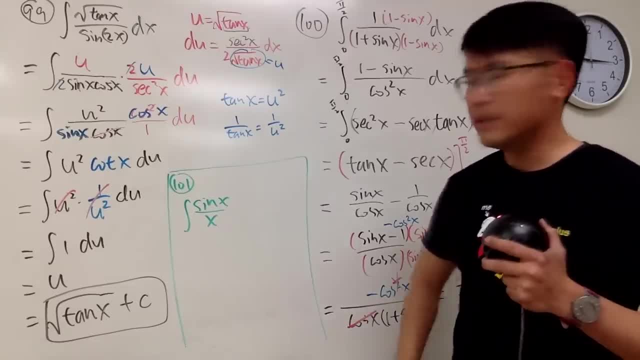 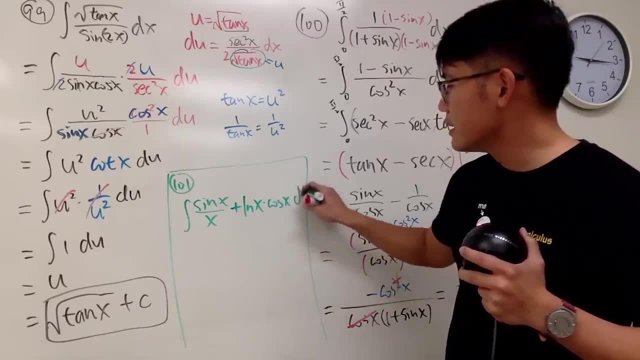 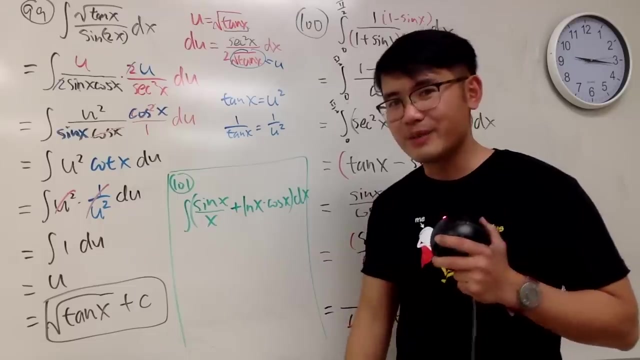 It has no elementary answer for that. No good, But I'll tell you, If I give you guys the other part, ln x times cosine x, dx, like this, well, we will end up with a very, very nice 1.. Very, very nice answer. 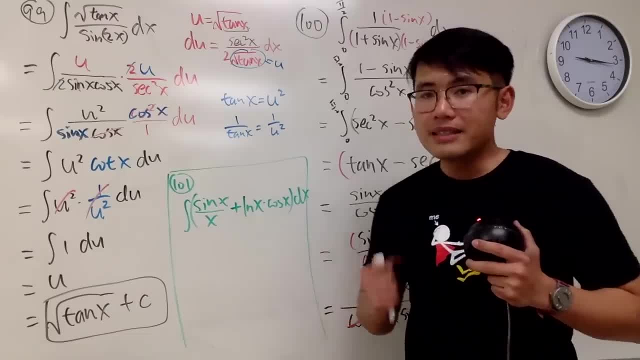 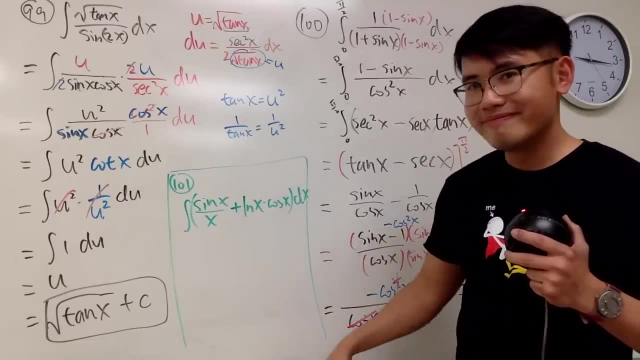 What do you think? See what this is Sometimes when you look at an integral, if you look at the big picture, especially when you have the sum, you know, maybe this came from the product rule, Because remember the derivative of the product. 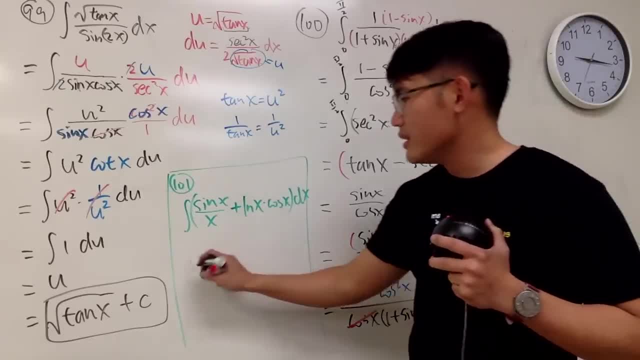 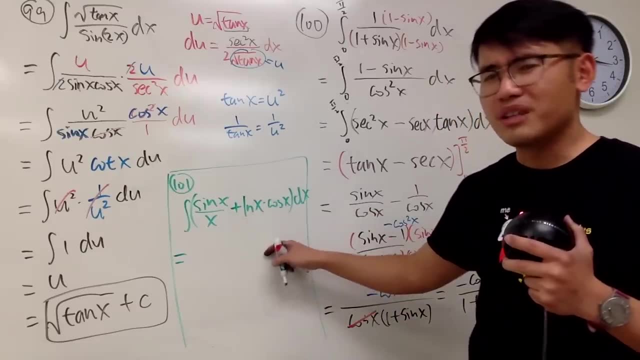 is you know something plus something else. Check this out. Let me tell you This right here is equal to hey, ln, x and 1 over x. isn't that just like derivative of ln x, 1 over x? yeah. 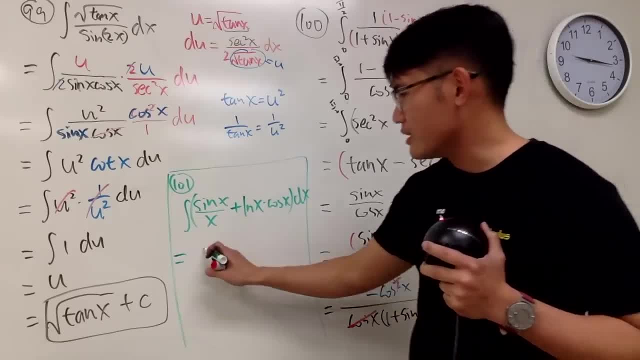 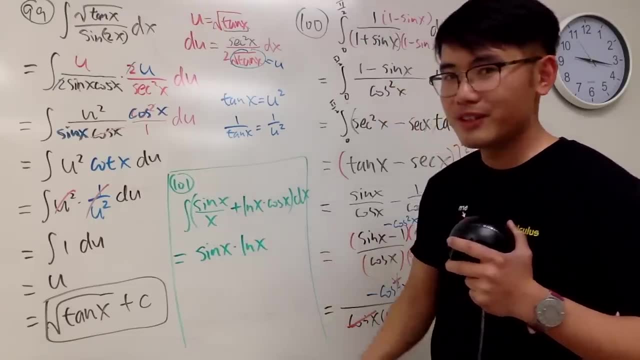 And sin x and cosine x. it's not really. yeah, Maybe the first function is sin x. I keep the first function and then multiply by the derivative of the second, which is ln x. Check this out. I keep the first function. 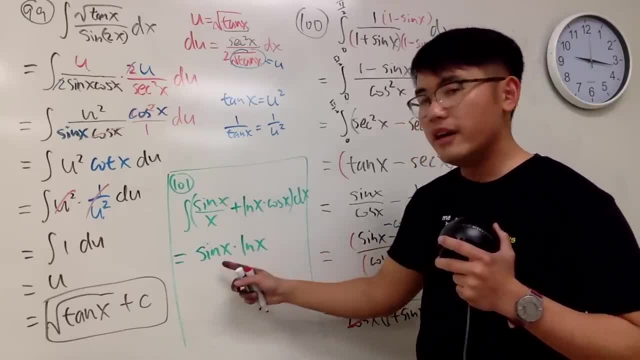 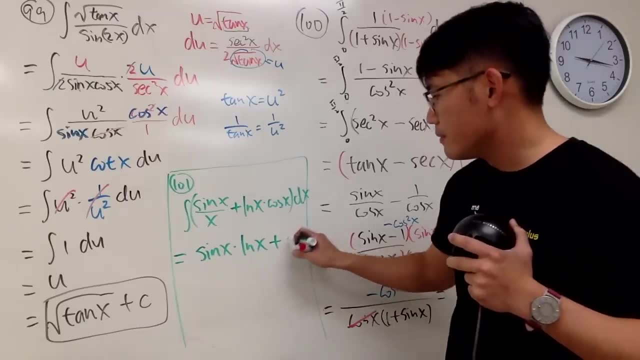 and multiply by the derivative of the second, which is 1 over x, and then I keep the second function and then I multiply by the derivative of the first function, which is cosine, and you add them up. Yes, In fact, this is actually a technique. 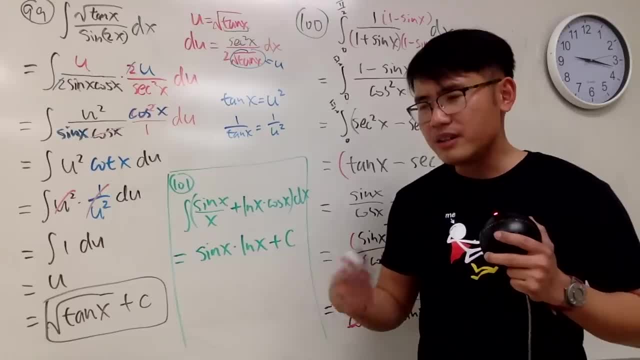 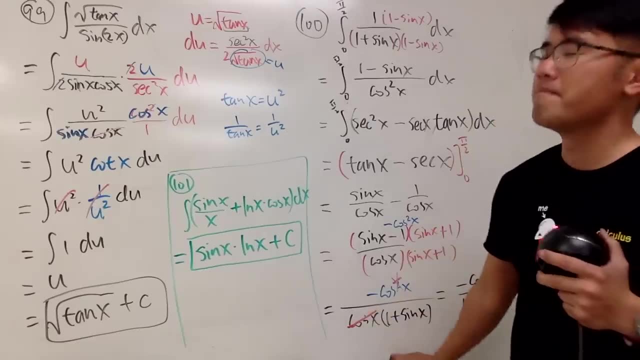 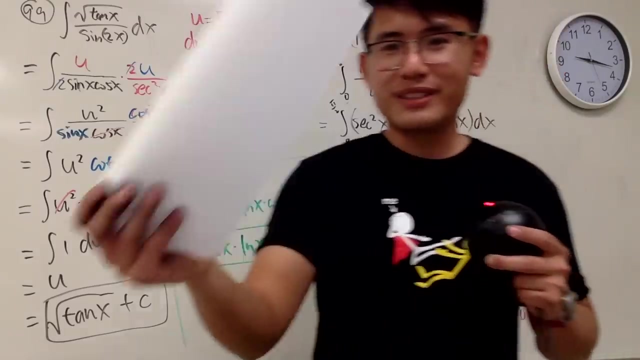 that we have to use when we are doing the first order nonlinear differential, the nonlinear first order differential equation. You have to use the integrating factor to make things happen. Oh my God, 101 integrals. okay, 101 integrals. 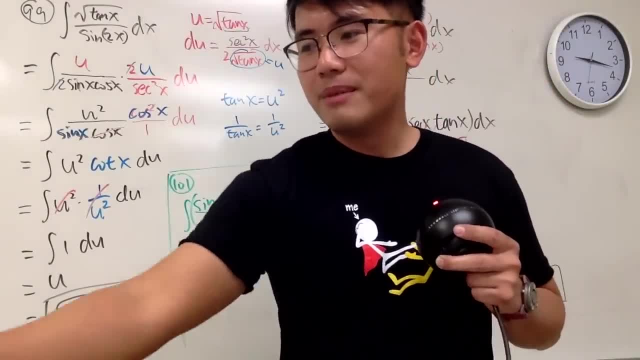 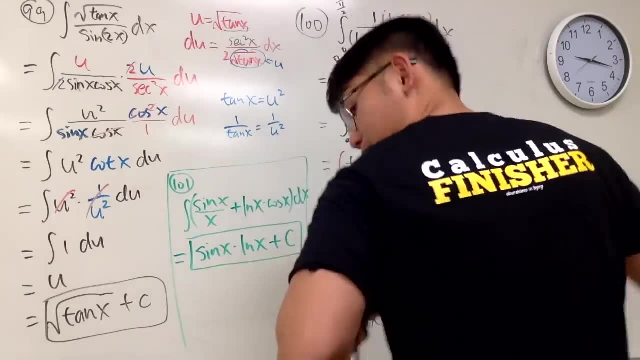 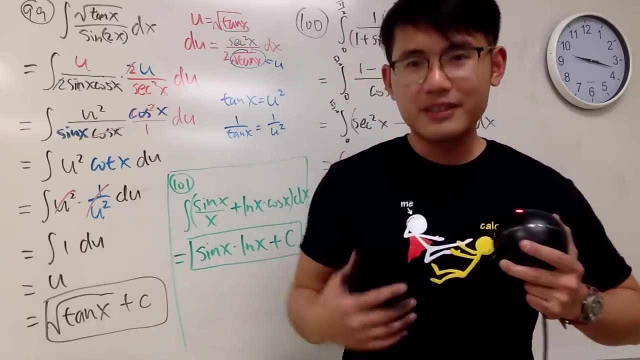 I don't know if I make any mistake or not. I probably did, but calculus finisher, Okay. Thank you so much for designing this teacher for me. I really appreciate it And for the people who don't know, he is just one of my viewers. 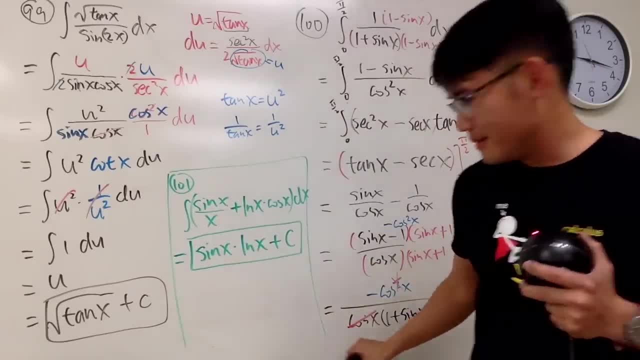 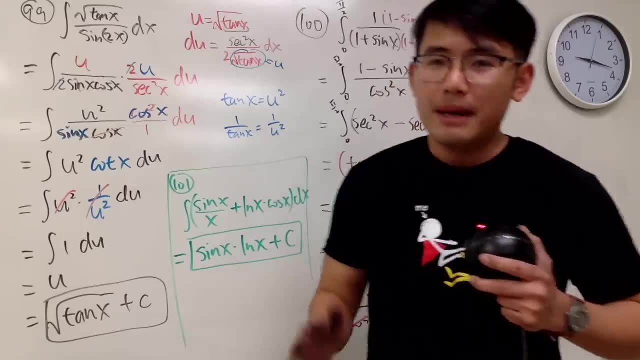 and yeah, I know my hands are dark. It's like all these markers. you see It's gone. And then x-pulse ones are better. I have to wash my hands now, But anyway, he was just one of my viewers. 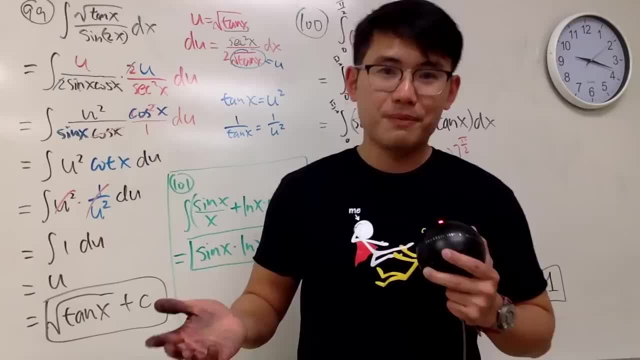 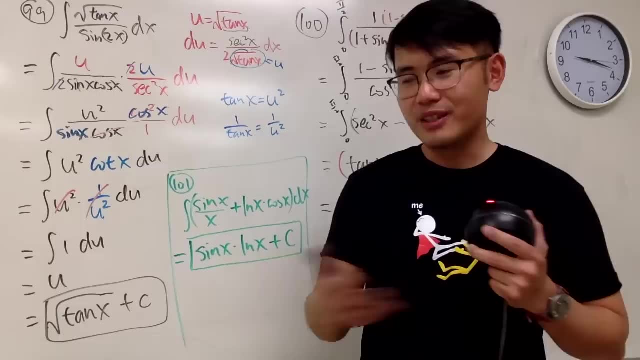 and he didn't. you know, I actually offered him to pay him, but he didn't accept the money and he just want me to do more videos for you guys to give back to the community, And then great person, and I really appreciate your help. 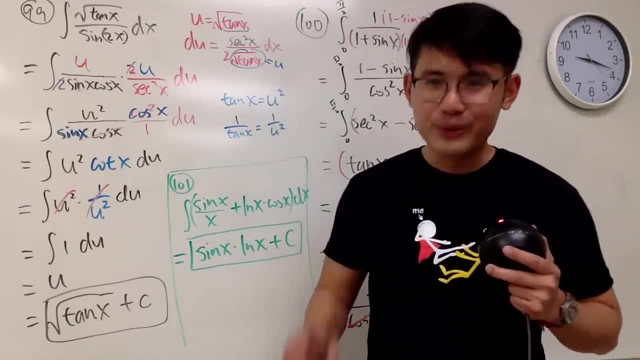 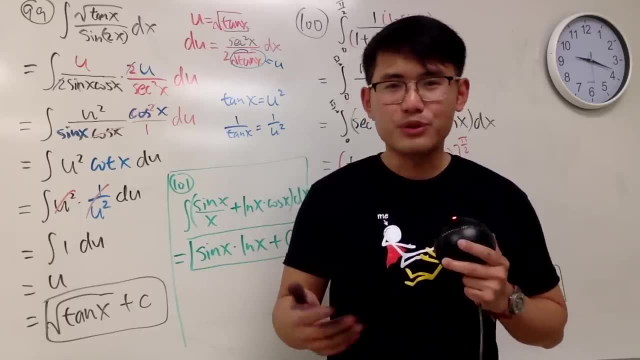 I really like this design. So cool, So cool. And again, Lars I, Lars I. I'm sorry if I pronounce your name incorrectly, but I really really hope the best for you And please let me know, okay. 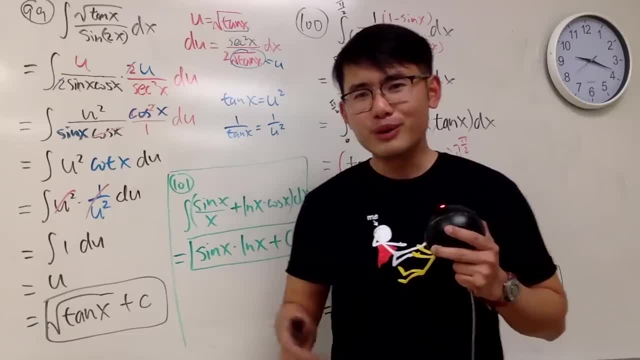 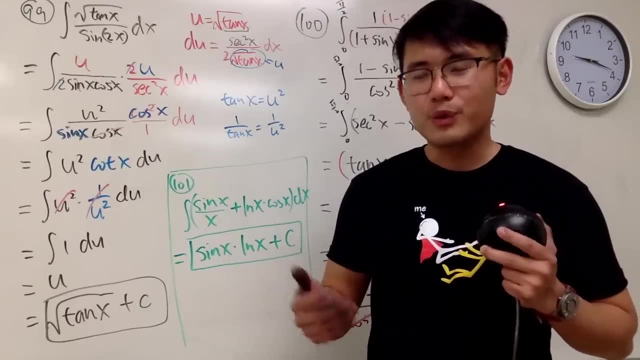 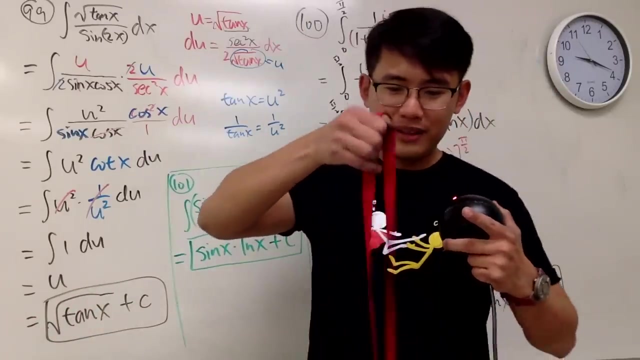 And then for the people, For the viewers, please also leave some nice comment, you know, to wishing him well, To wishing him well. He's battling with cancers, All right. So I finished the mirror, so I will be putting this down. 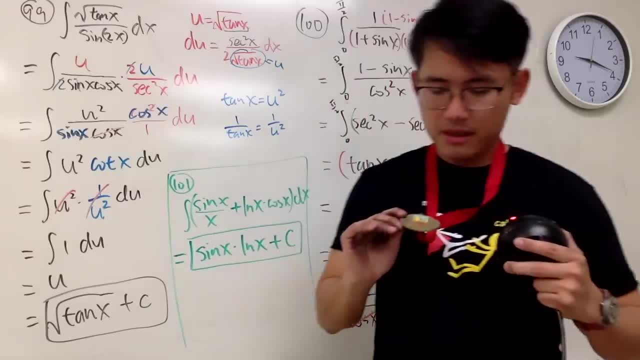 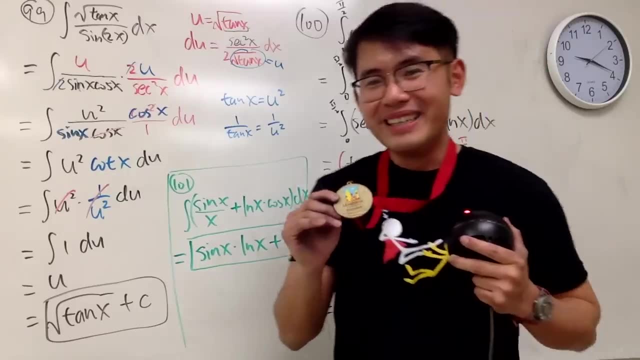 Just like that, This right here, special meaning, because I never knew I would be able to run 26.2 miles per hour, 6.2 miles- when I was like 17 years old and I didn't really train for it. 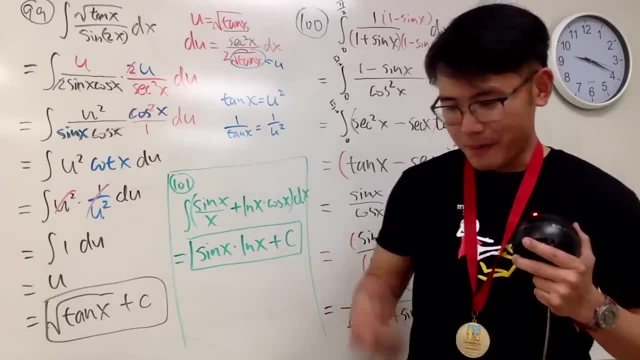 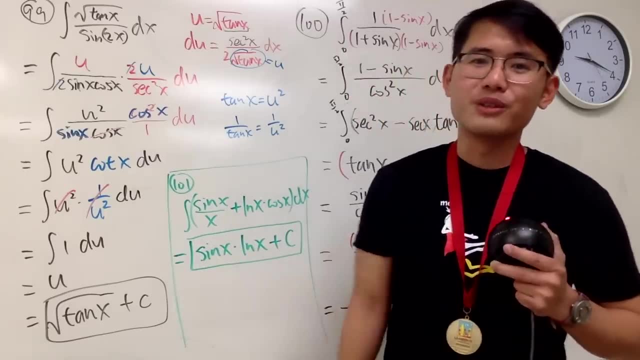 And I ever think that running is just a way that you know is training my willpower. It's like if I want to do something, it's like running a marathon. Life is like running a marathon. So, yeah, Honestly, I don't know how many views that this video is going to get. 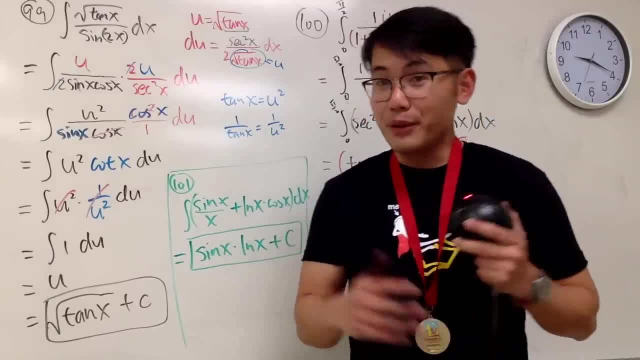 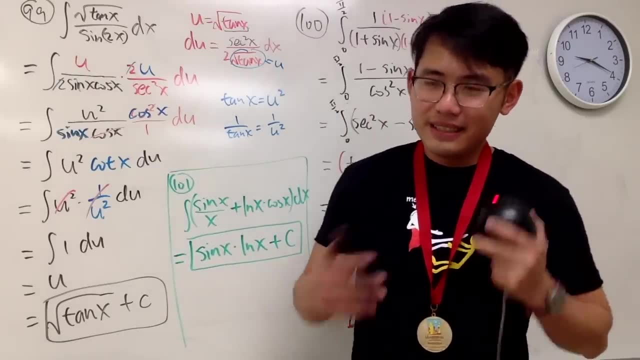 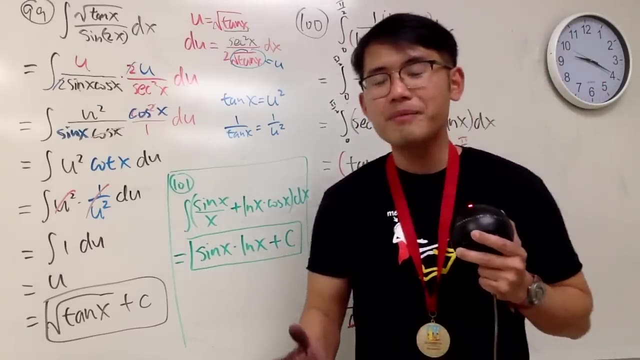 Hopefully decent enough And again, thank you guys so much for watching. Okay, I'm turning 20.. And yeah, Thank you guys so much for watching And hopefully you guys can continue to support my channel. I really, really appreciate everybody. 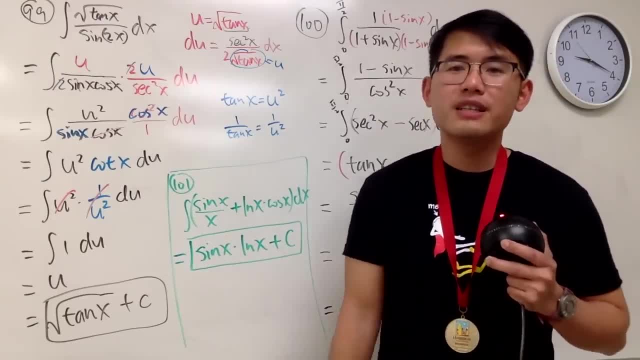 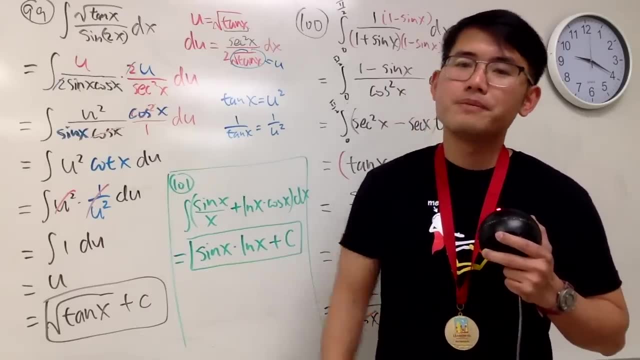 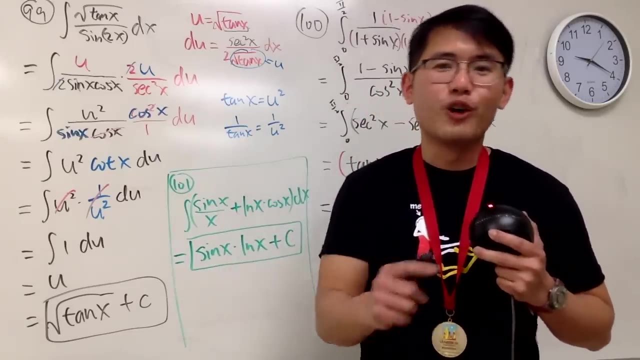 who have been leaving nice comments throughout all these years, And I want to thank all my friends- Dr Payan Wu, Han, Thematica and a lot more people And, of course, my special thanks, special thanks to my wonderful, lovely girlfriend. 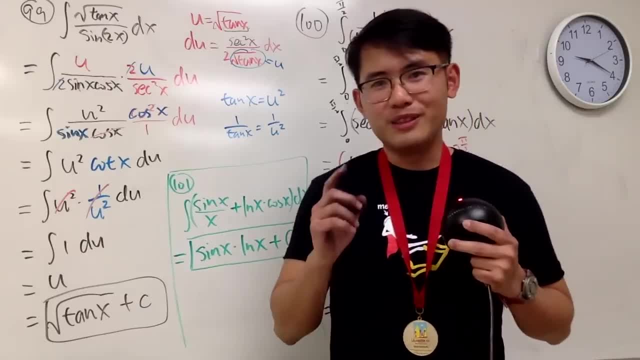 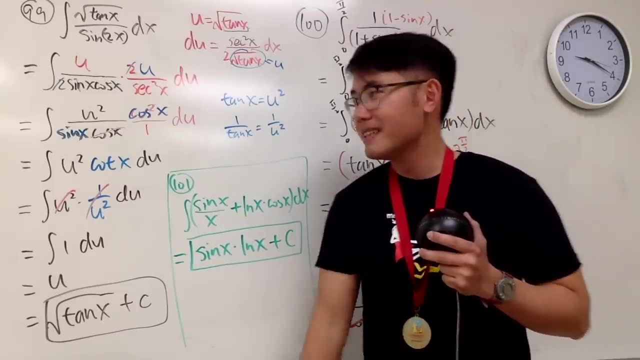 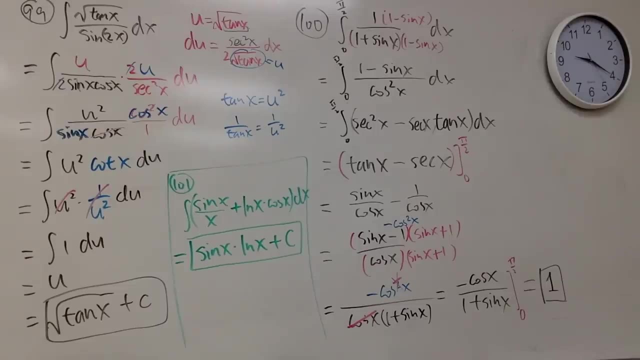 Jia, And I will see you guys soon, And I will see you soon, Okay, Yeah, Oh, my God, Bye, As always, that's it.